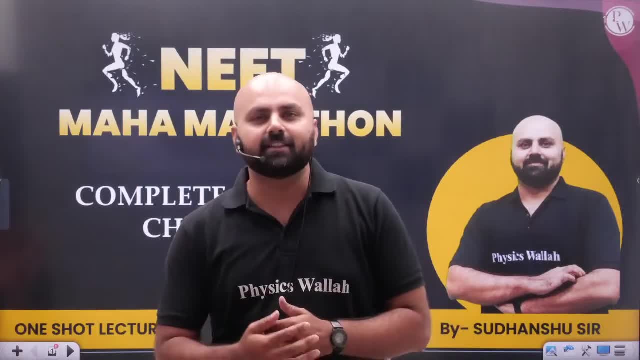 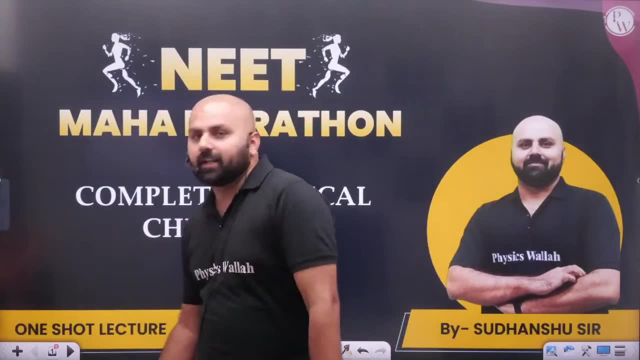 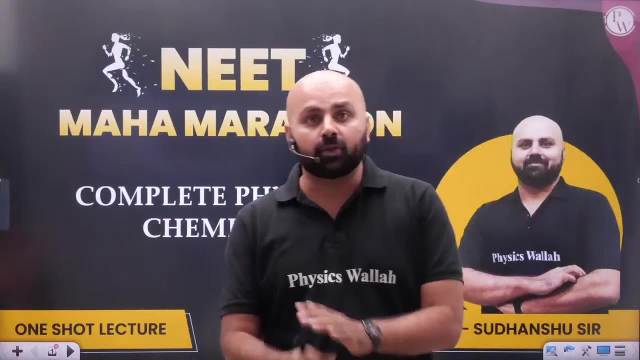 So finish all the marathons and quickly revise and come to do the questions. Yes, brother, Okay, Come on. Let me tell you one thing: Today in my class, I have to study a lot, And especially you know why I have kept the time of 2 o'clock. 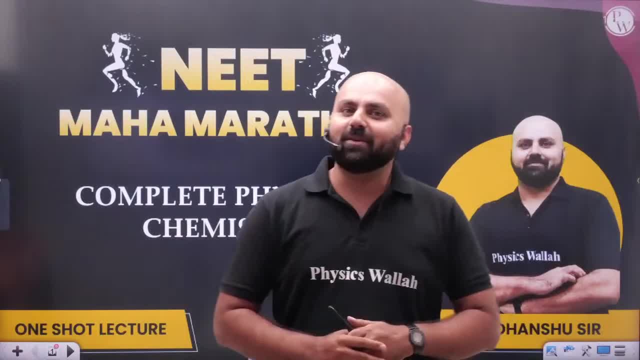 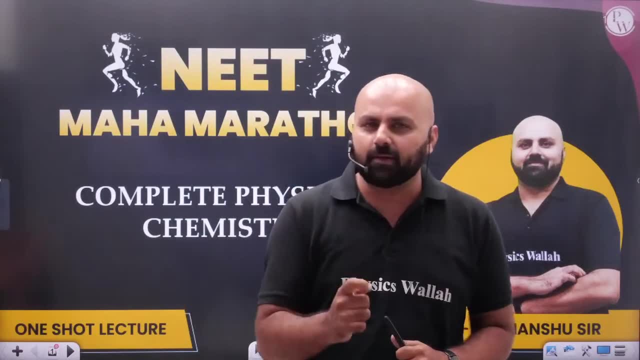 I have kept the time of 2 o'clock because this is the time. This is the time when the race will start, Exactly, Exactly, sir. After 14 days, 13 days, At the exact same time, the race of your story will start at 2 o'clock, from 2 o'clock. 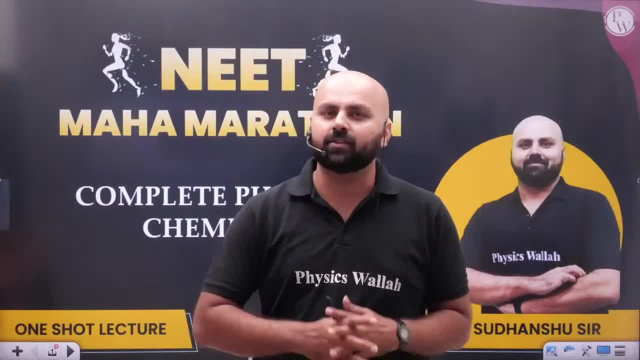 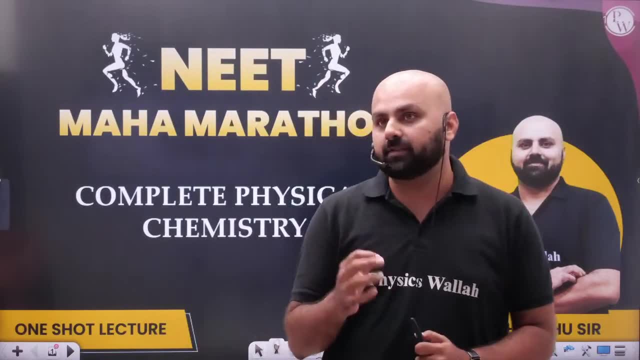 And from 2 o'clock to 5.20, 5.30,, a history of your whole life will be written. So let's try. Sir, we don't have 2 to 3.. The time duration of 5.30 is the best to utilize. 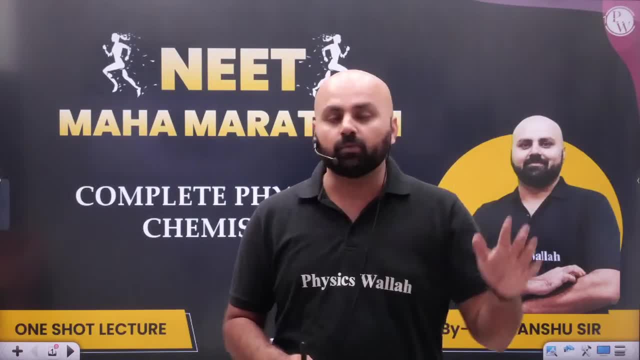 No one will wander here and there. No one will have a break from 2 to 5.30.. Nothing is going to happen. The reason is that you will not be able to take a break in the exam hall. If you will not be able to take a break in the exam hall. 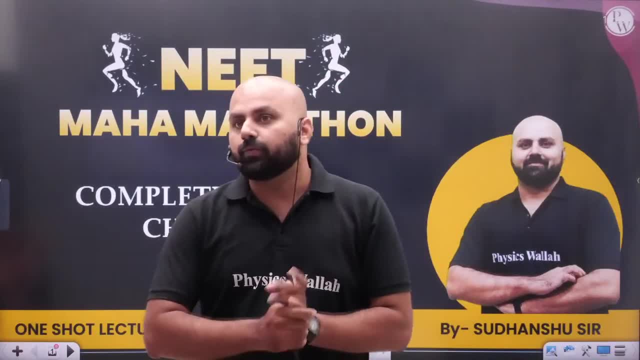 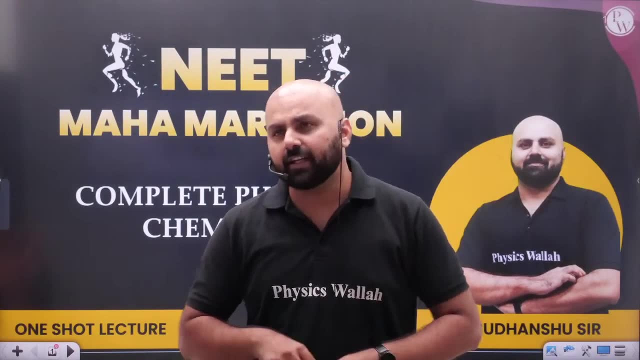 if you will keep your mind on alert mode in the exam hall, then there is no break from 2 to 5.30.. Our first break is going to be at 5.30.. We will see at that time, But yes, in today's class we are going to do a lot of things. 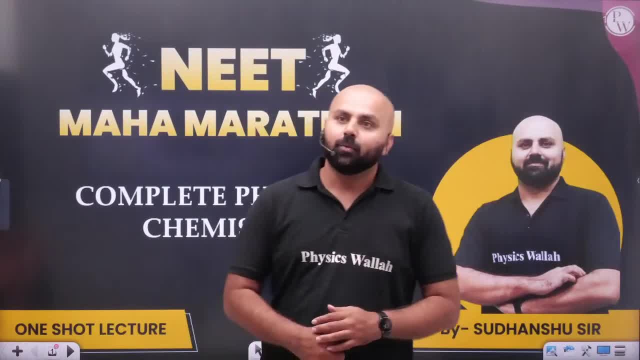 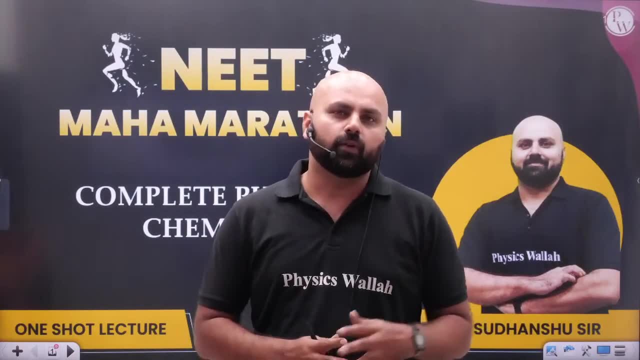 A lot of things. We are going to do the whole physical chemistry. Think about it. We are going to do the whole physical chemistry. There will be theory, formulas, questions, everything. It will be balanced. Obviously, We will see how much will happen today. 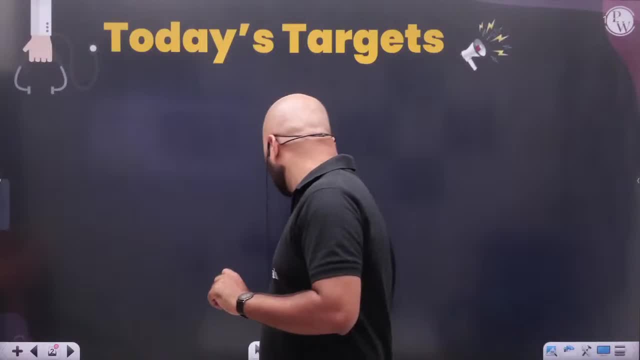 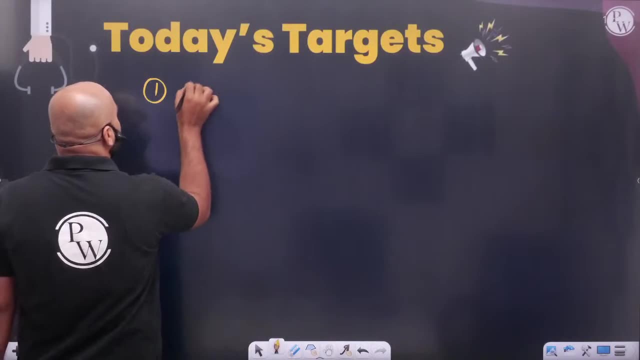 Look, if someone is asking me about today's target, I will write it down straight. My target is to do one chapter. I have to finish the physical chemistry. There are two or three things. My first target for today is that your confidence should boost. 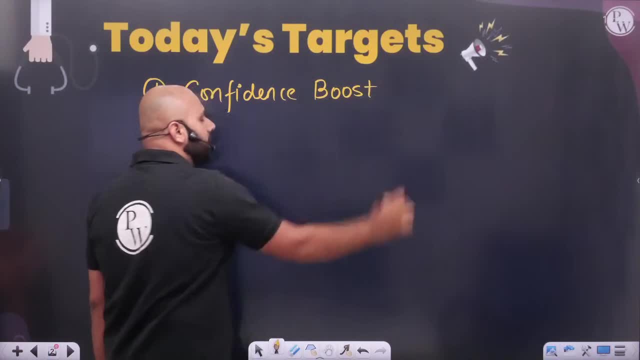 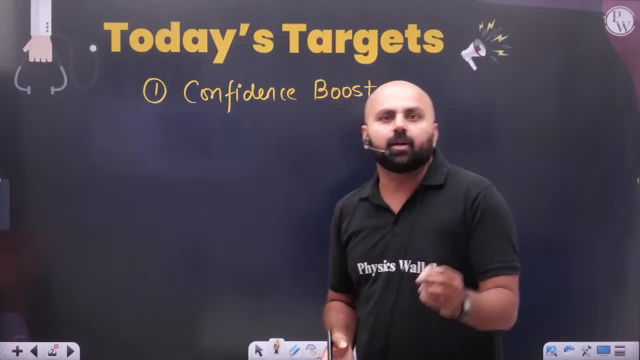 What is confidence? It should boost. My today's target is this: That you feel that you can do this topic. The first thing is that your confidence should boost Reason: Even today, you know formulas, But you are not able to use the right formulas at the right time. 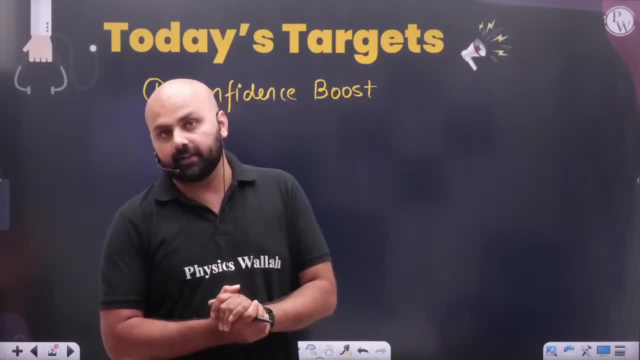 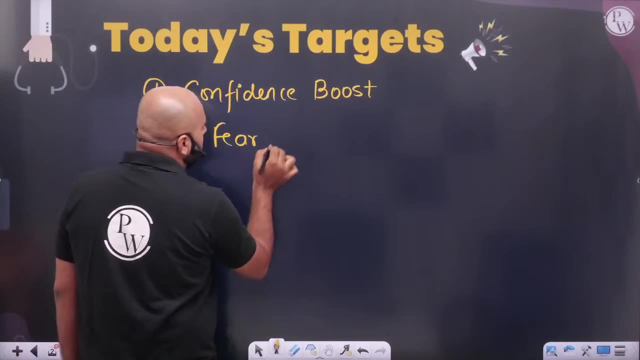 So today's target, The first target, is that your confidence should boost on the topic. Second, Sir, looking at the questions, the fear of questions, all of them. What is the fear of questions? What is the fear of questions? 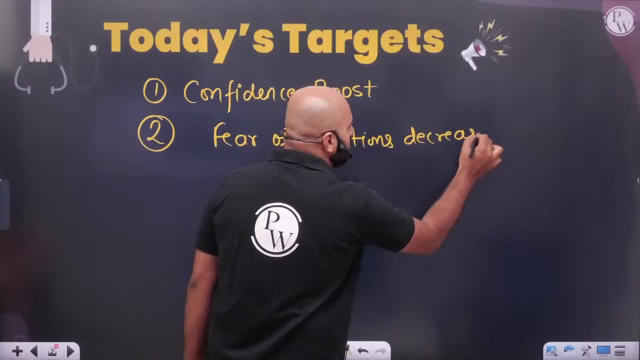 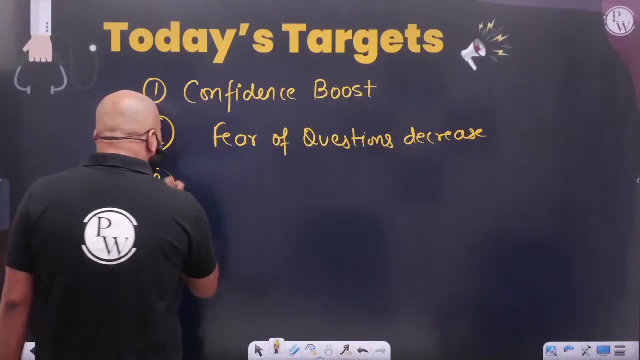 Decrease. The fear of your physical chemistry questions should decrease. Okay, So take it. My target is clear. Third thing, Sir, you have to secure today's selection. First, Sir, all this will happen. After that, You have to secure today's selection. 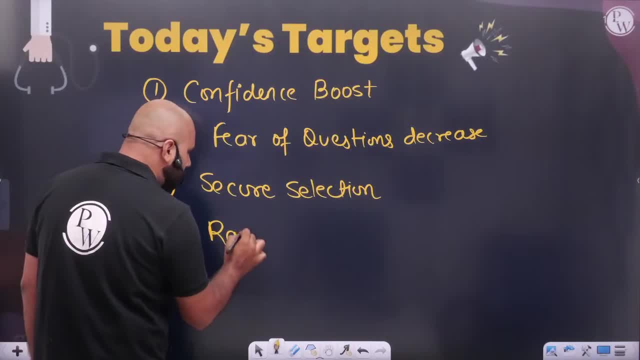 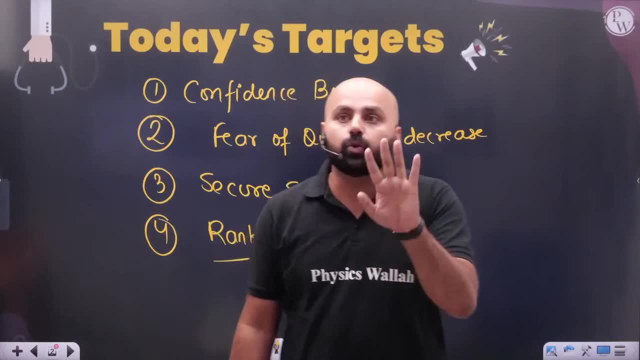 And fourth target: You have to increase the rank, You have to boost the rank, You have to boost the rank. My today's target, Four targets, And I want you all to have this target. These four targets should be there, Sir. first, 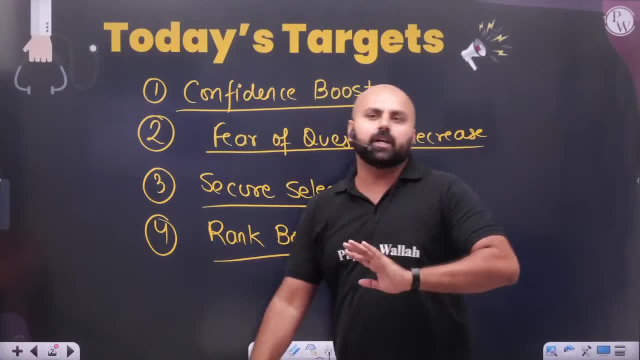 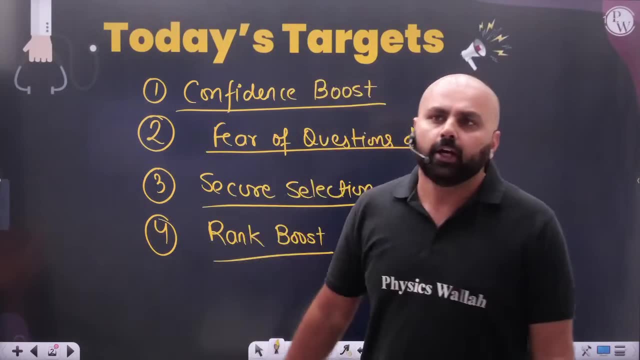 All the topics will come. We will do it like this: That brother, this. It can happen that someone's confidence is good from the beginning, So we will finish the fear of questions. If someone's selection is secure, Then we will rank it. 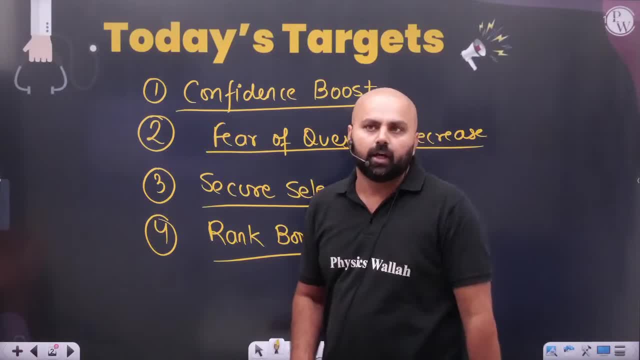 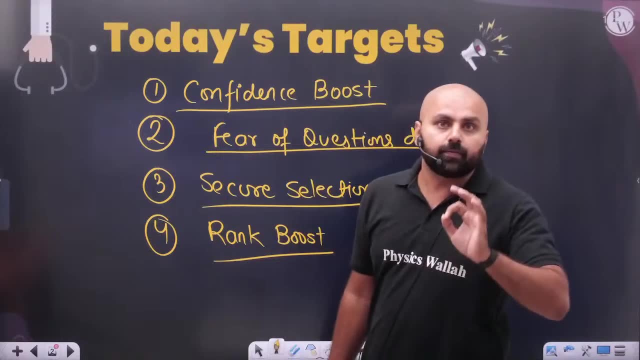 That brother, all these things, We will finish it today. Reason that brother Here, Here Now: Inorganic is finished, Organic is finished. Last Last Physical chemistry: Chemistry: One hundred and eighty. One hundred and eighty questions. 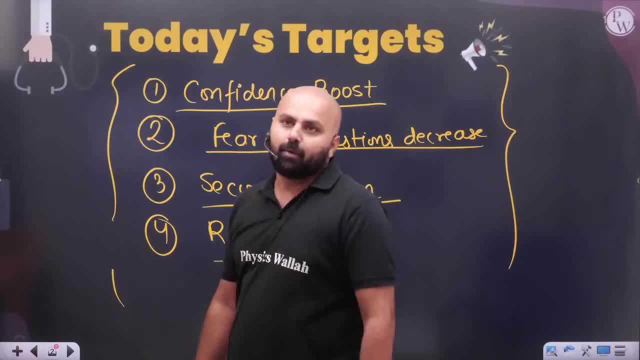 Talk to you about marks. So from this Now we have to take care of these four things. You already know the rest of the target. You already know the target That brother. What to do? You already know the target That brother. 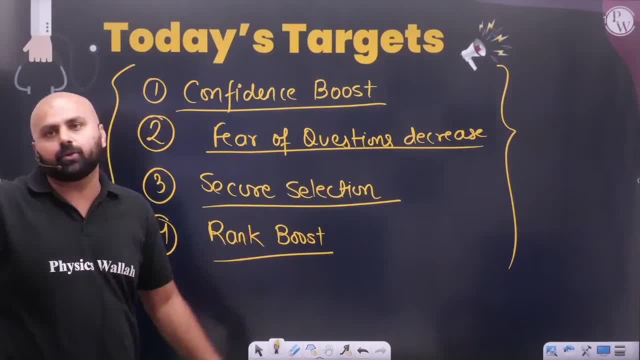 You have to secure the selection As much as possible. Let's improve the rank. How will we do, Brother, Full This whole Twelve chapters Next, Next With us. I don't even know how long, But yes. 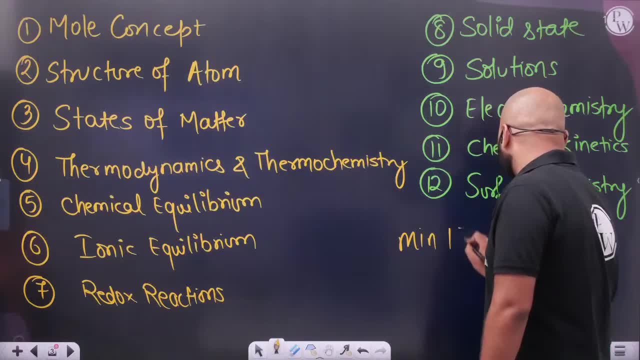 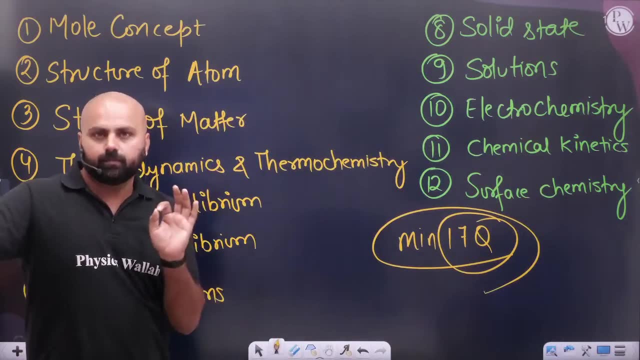 These whole twelve chapters With which Minimum Minimum seventeen questions. Minimum seventeen questions. We will take ourselves to the selection. Minimum seventeen questions. If you see Five Last five years, If you take out the overall average, Then minimum seventeen questions. 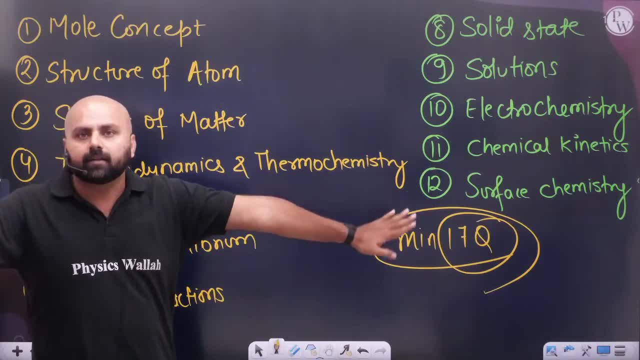 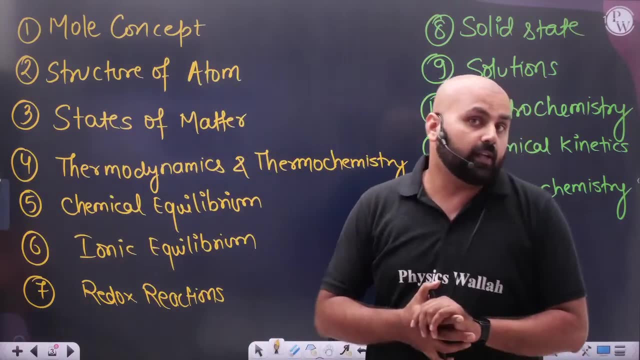 Means If you connect it correctly, Then we will secure seventy and eighty marks. today. We will secure seventy and eighty marks. Yes, It will be done from the basics, But Basic, Basic, Basic, Basic Rest Is That is what it is damaged. 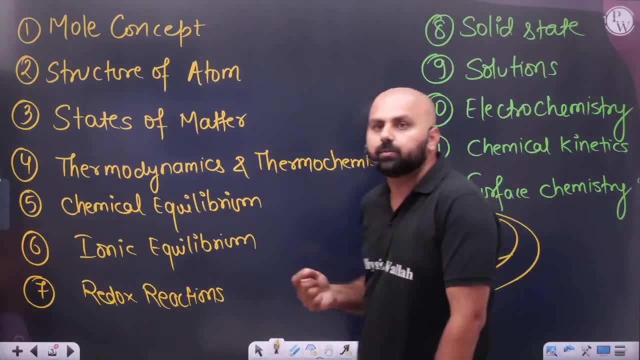 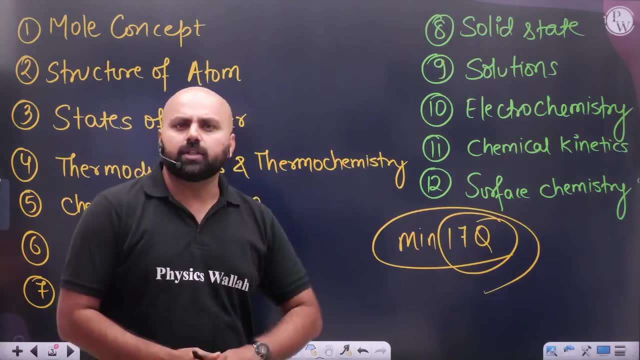 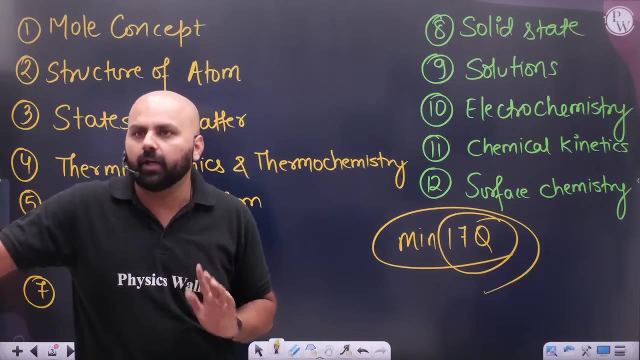 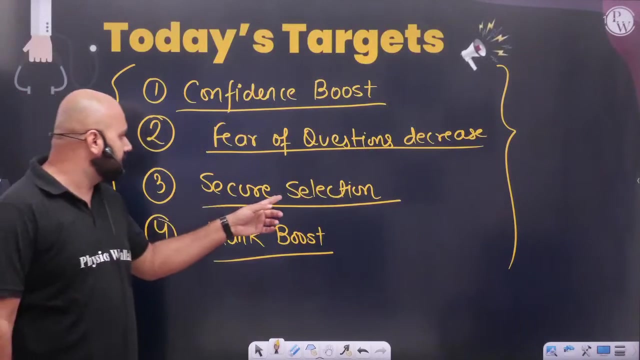 Is that there is the problem. ergo, By that The way, It's very difficult. So The, That means, If you have this, That means and then you have to increase your rank slowly. People who are asking about duration of class. 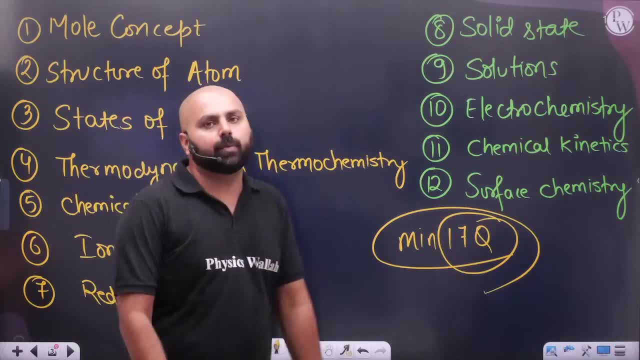 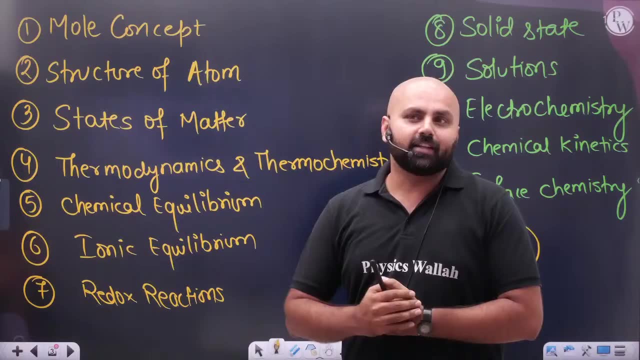 you are asking the wrong question. Coming to this channel, coming to this topic, coming to this class- duration of class break- you have to ask all these things. You think you will become a doctor. The preparation for becoming a doctor is going on. 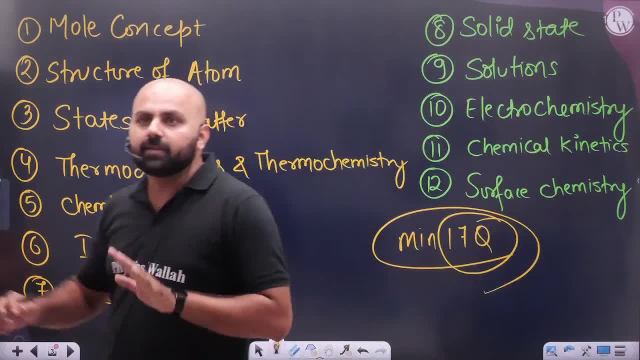 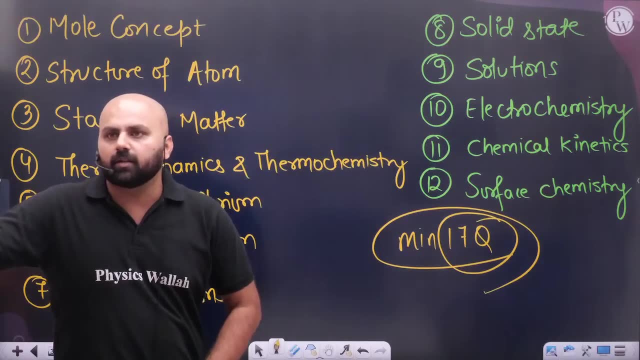 What does duration of class mean, Brother? you should not care about this at all. You study very easily. As much as it will be done, it will be done. Class for 18 hours? No, sir, not even that much. It was physics, it was physical chemistry. 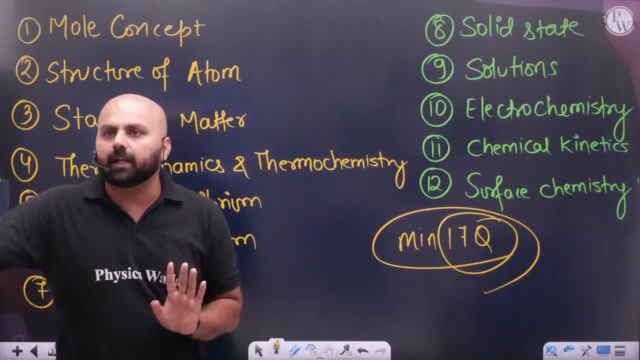 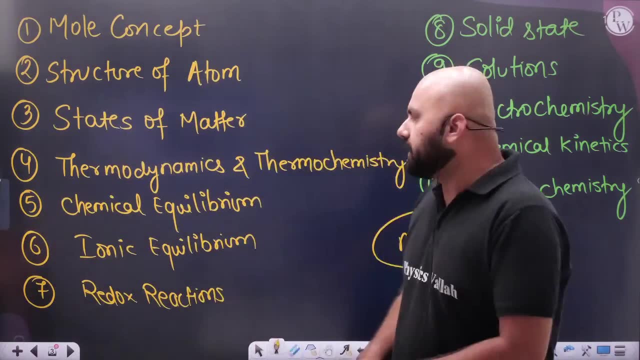 It will be done. It will be a chapter for you. Okay, don't worry about it Now, mentally get prepared. Mentally get prepared. You have to do 12 hours or 12 chapters, As long as it takes, as long as it takes. 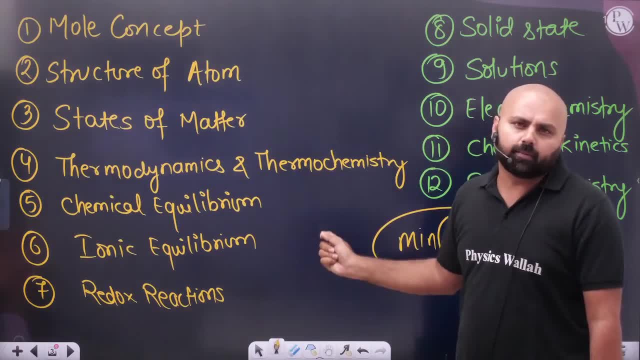 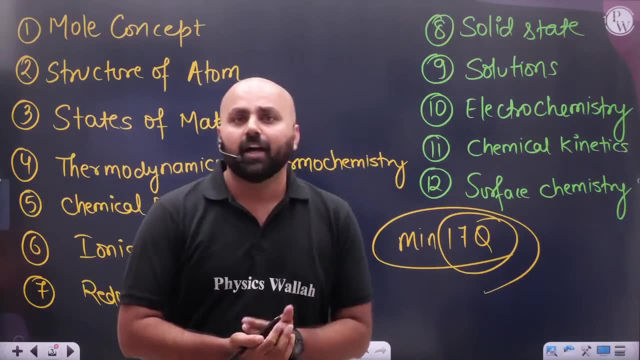 We will keep doing it until we get the confidence We know our target for today, What all we have to do. We will start. Okay, let's go Now. let's start today's story. What is today's story? Today's story is the most wonderful story. 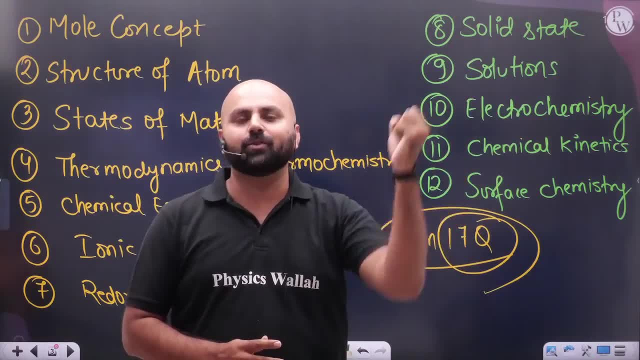 The reason is that the whole year, the whole year of studies. today he is revising it. Someone says that I want to study from here for the first time. Son, please don't watch this video, Because if you study for the first time, 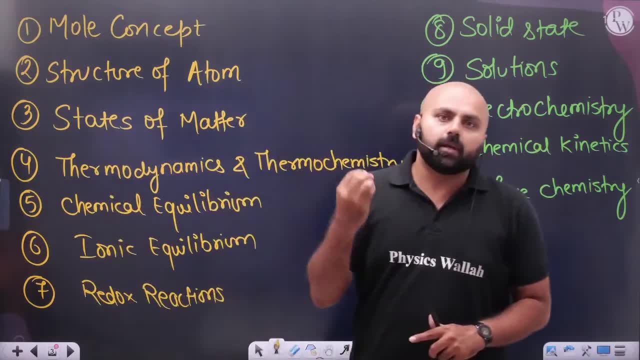 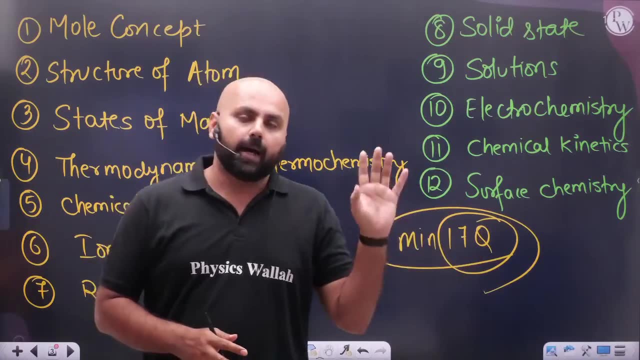 then it is possible that you will vomit, Because it is obvious that this child, the same child, can digest this thing. who is working hard all year round or is knowing a little bit of the topics? You should know a little bit. Yes, we will do revision. 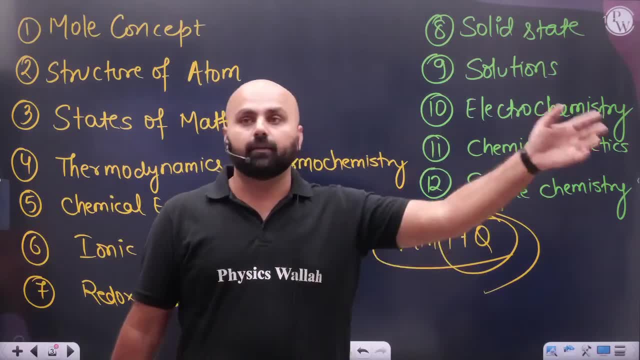 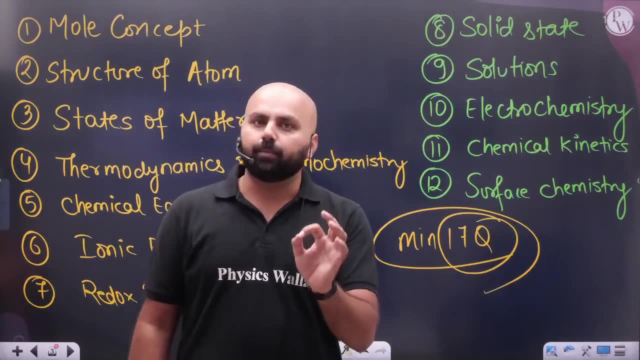 we will do questions, your things will happen, Okay, but yes, by some 11th mistake that no, brother, we have to comment here. then you comment: But yes, those who have come to study, son, you get ready with a rough page and page. 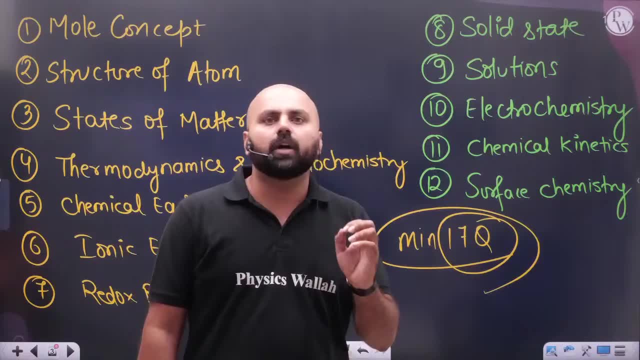 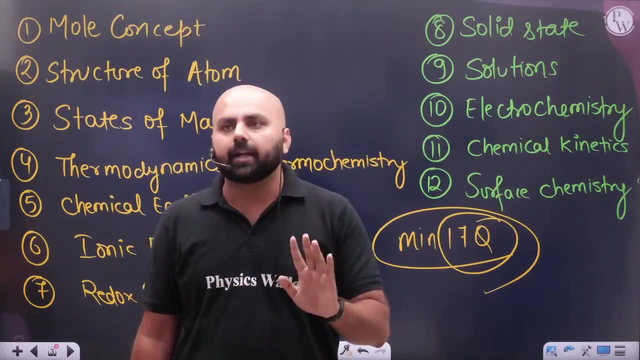 keep taking screenshots of the formulas, whatever things I will tell you. you think. tomorrow the PDF will be uploaded. see from the PDF. if you think, then I will be side. you take a screenshot and keep it. Try to do this much. 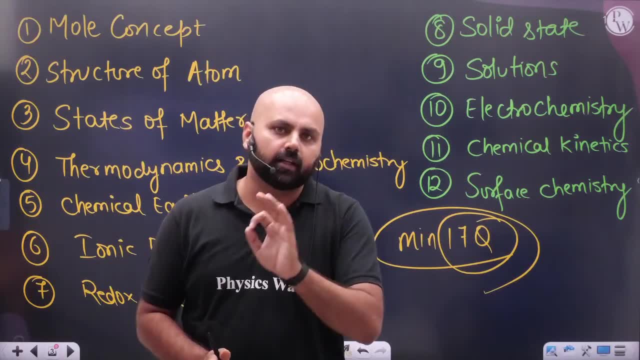 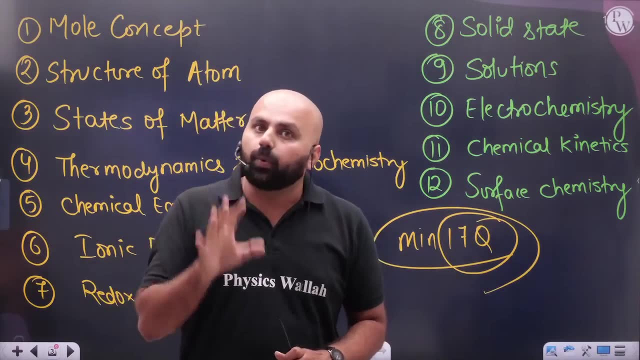 by revising this much in the next 12-13 days when we reach the exam hall, then there will be no problem there. What we will do today, I can't say out of it, but, yes, all the stories based on it. 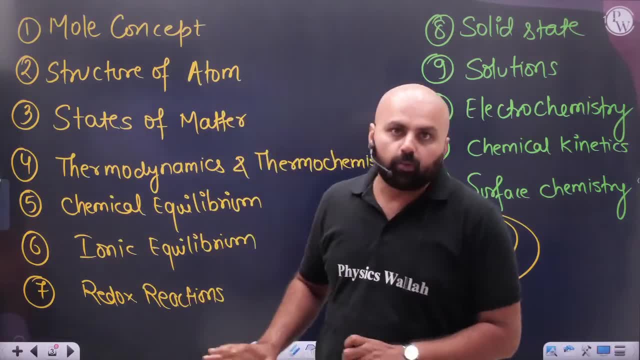 will come in your exam hall will not come out of it. Okay, I can't say that all the questions we will do today will come there only. No. no, this will be a little more, but, yes, all the questions we will do today. 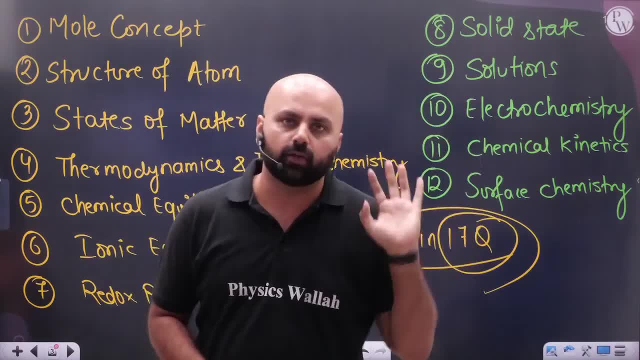 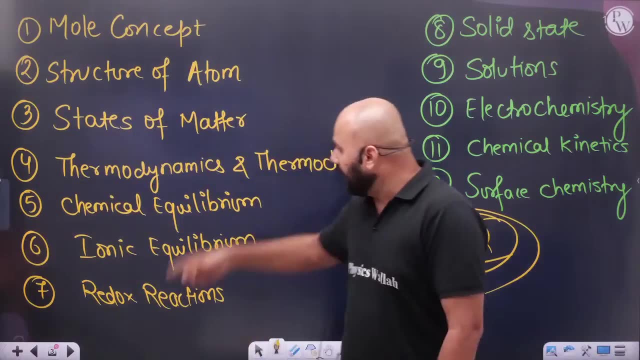 on their concept, the whole story will be on your 7th of May 2023.. So now, what is going to happen on 7th of May 2023? How is it going to happen? So we will start. no son. 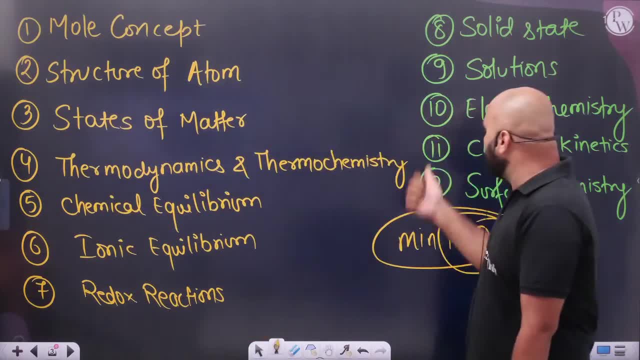 first we will do 11th, because 11th is more physical. then we will do 12th, coming to the last of 12th, coming to the surface. okay, we will finish first. we will start 11th. 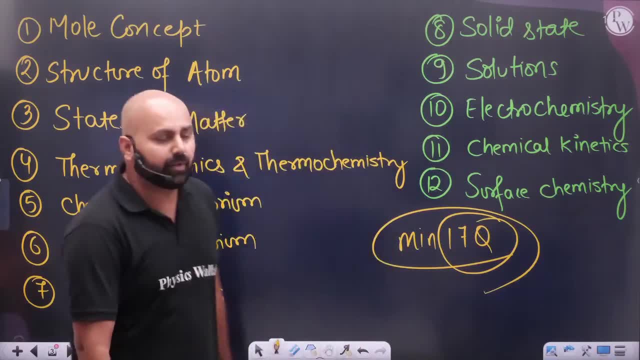 then we will do 12th, because the reason 11th is more important as compared to 12th. in 11th, these 3-4 portions which will come continuously, that is a little more important as compared to 12th. 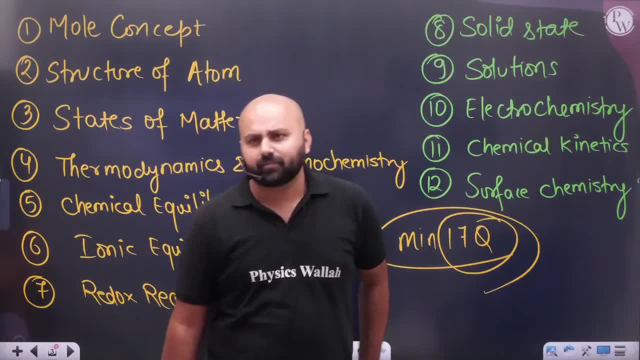 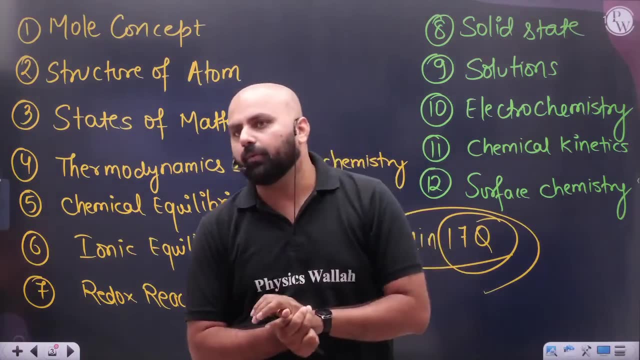 okay, so let's start. let's start with ourselves. okay, let's go, brother. so now let's start. let's start the first chapter in today's Maha revision in the marathon, the first chapter which we will bring. 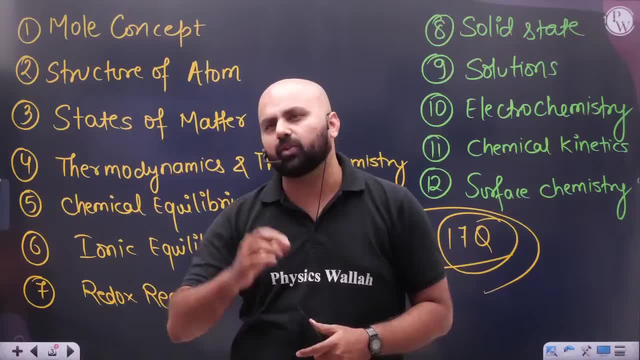 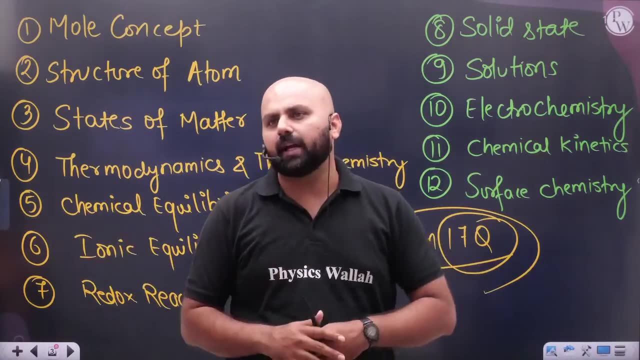 you will get the PDF there. please don't try to write, because you have to write a lot, okay, so please don't try to write. if I will write the formulas, you will get the PDF tomorrow. don't worry, you will go to the app. 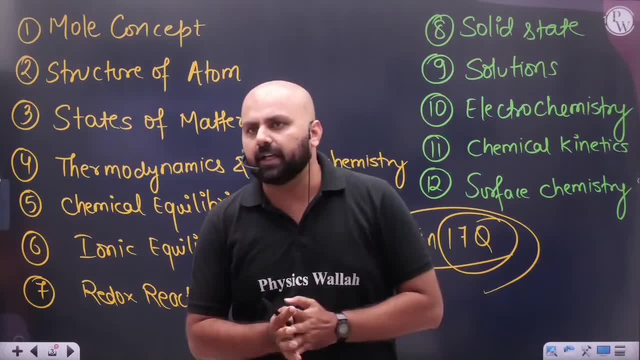 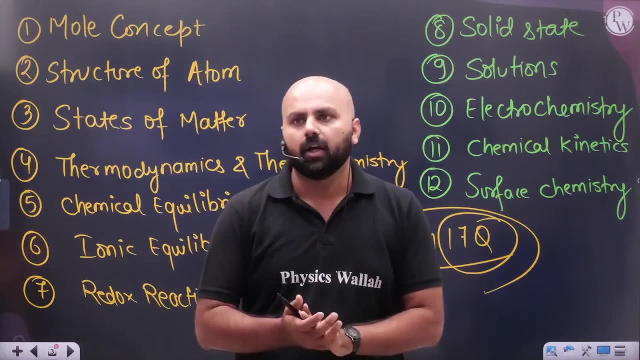 you will get the PDF there. okay, you will get the formula sheets. now, brother, who has not been uploaded, of physics or botany. I mean, I will also forward your message. you will get it, okay, so let's start. 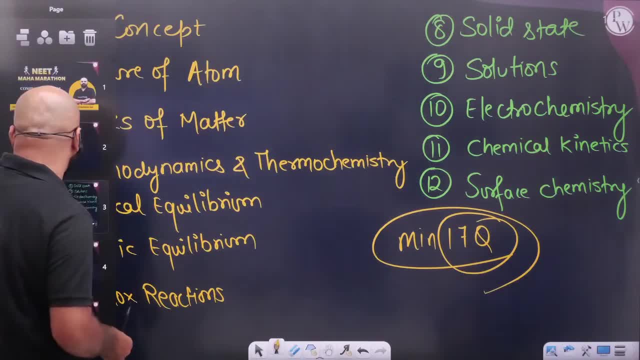 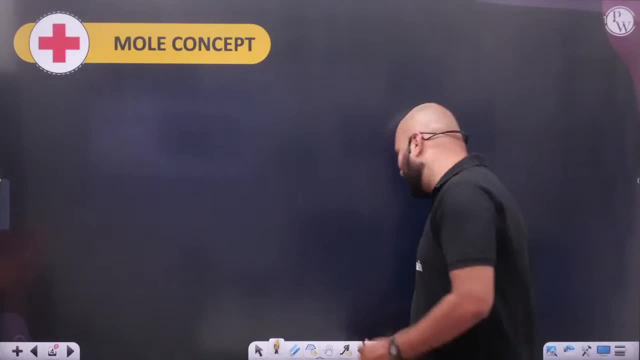 so let's start today's story, and today's story is a very beautiful chapter. the first love means the love of childhood. now, those who are going to give the reneed, this is the love of their childhood. this chapter, the most basic chapter. 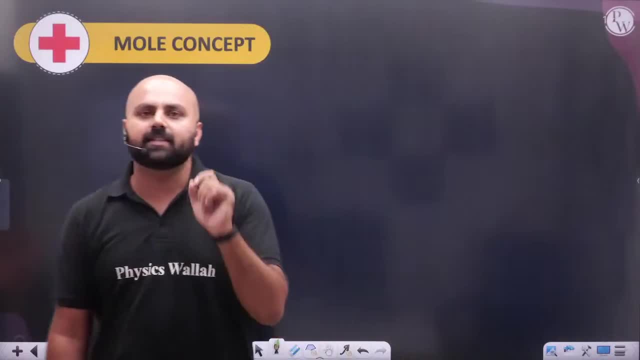 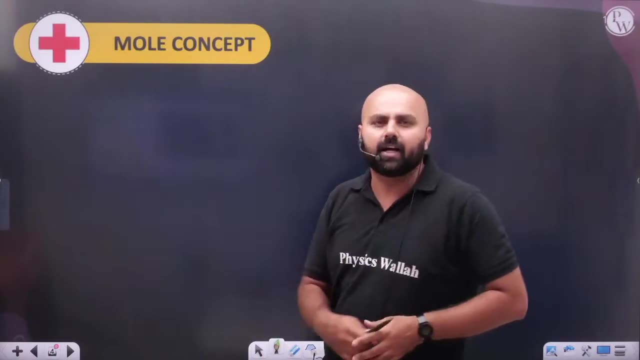 the first chapter and that is the basic concept, the most basic chapter, the first chapter, the basic concept, the basic concept in today's time, you all, I am talking directly. this was the chapter in the eleventh class. 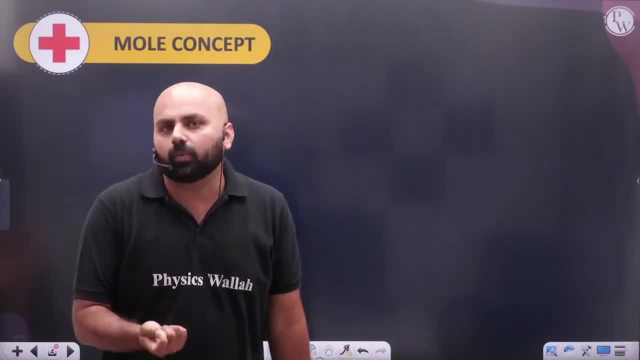 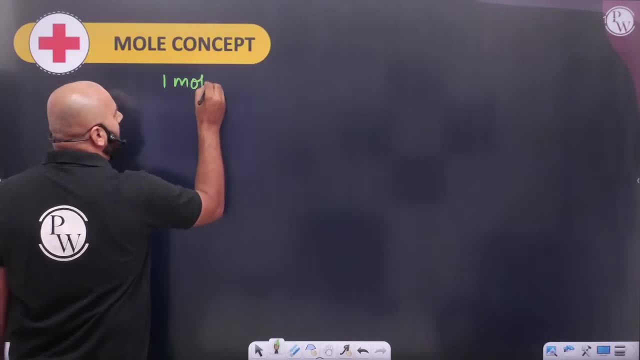 where our life started. we started with atoms and molecules, and from there we went ahead. so now we came to the basic concept. I am not saying anything simple to you. what is a basic for you now, sir, for your exam hall? 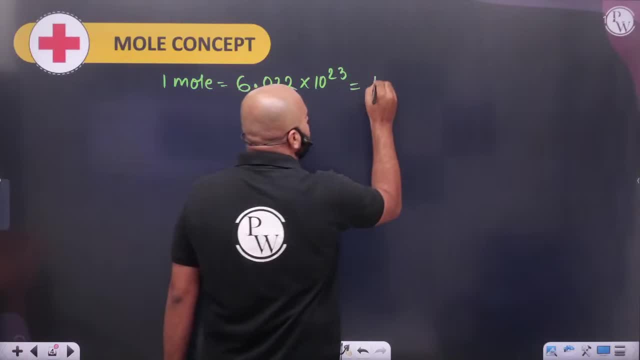 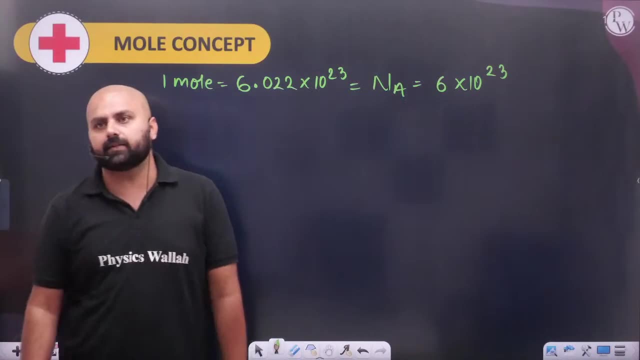 this is just a number which we can write it Avgadro number. or if you want this in the exam hall, then you can write: 6 into 10 to the power 23,. 6 into 10 to the power 23,. 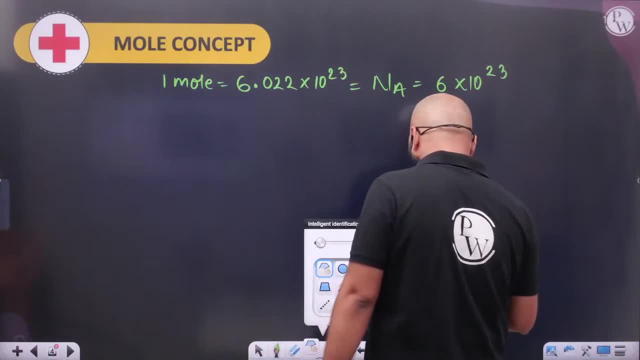 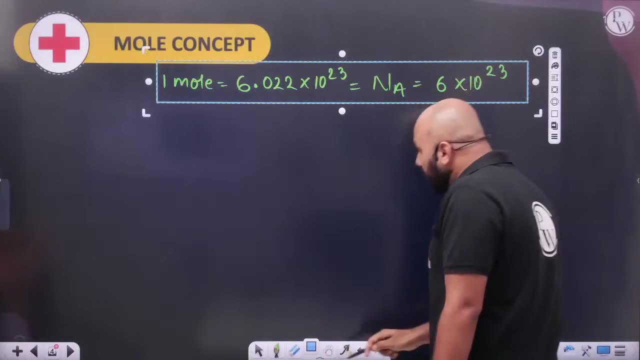 and you have to keep this number in your mind. you have to keep this number in your mind, that brother, this Avgadro number and this one. while doing the calculation, Avgadro number will also change. today, many things are going to be done. 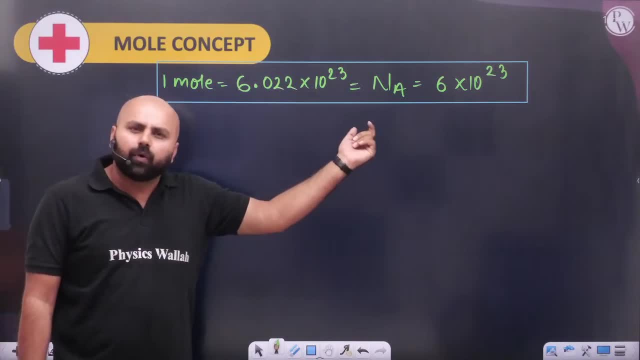 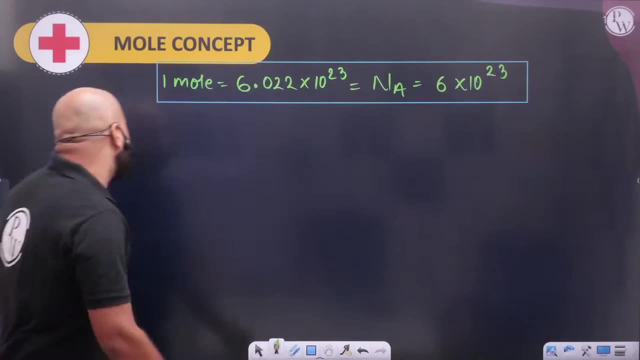 the most basic thing of a simple mole concept is one mole. what is one mole? it is a prefix which will be used anywhere. what will its value do? it will do it so many times. you all know number of moles. 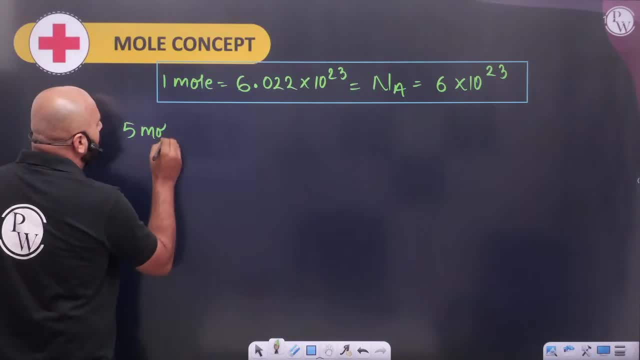 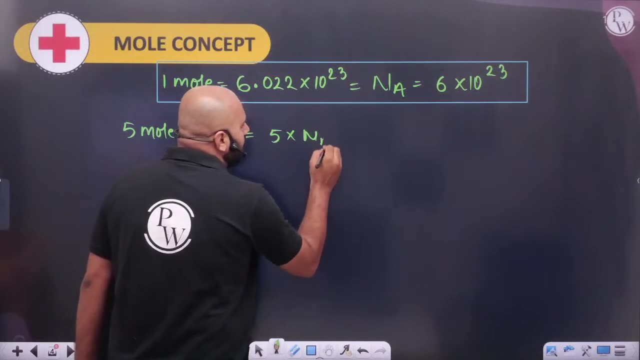 if I say somewhere, if I say somewhere five mole, then you all know its meaning, because now its story will start after a while, sir. what will it mean? 5 into n protons will be mole, is nothing a prefix. 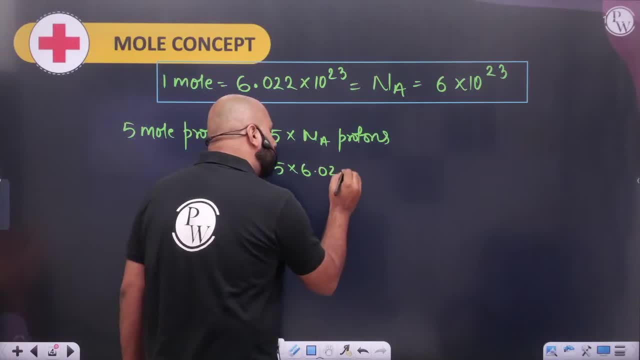 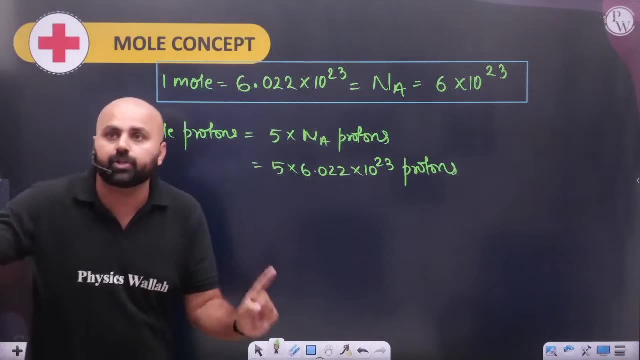 that means what? how many protons are there? 6.022 into 10 to the power, 23 protons are there. I have to tell so many basics, because now questions will come and according to that we are going to do. 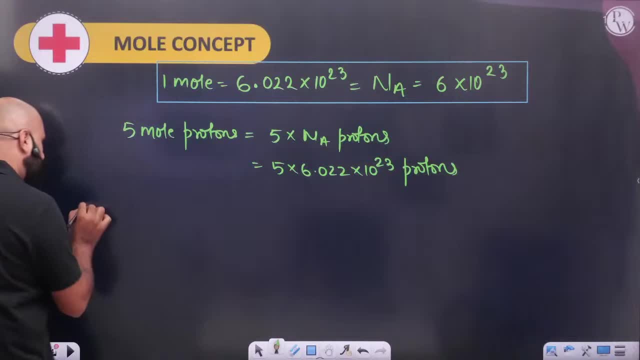 one more thing, sir. if you see the calculation of the mole, then the number of moles, the number of moles if you go to get it. number of moles of x. go to get it, then you get the number of moles of x. 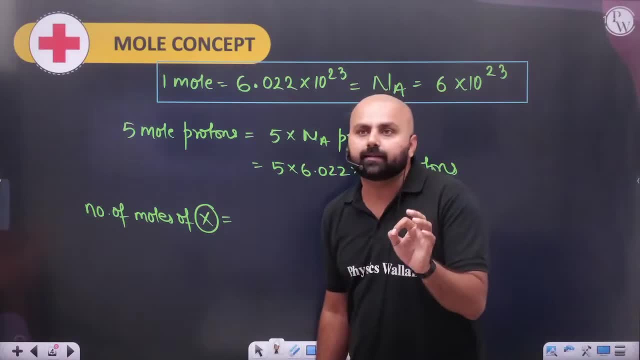 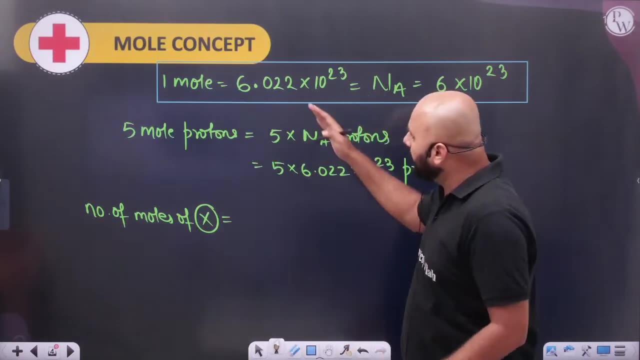 the way to get the number of moles. if you have to get the number of moles of x, there will be question practice. listen properly. there will be question practice just one more day. what you have to do first, you have to understand the theory. 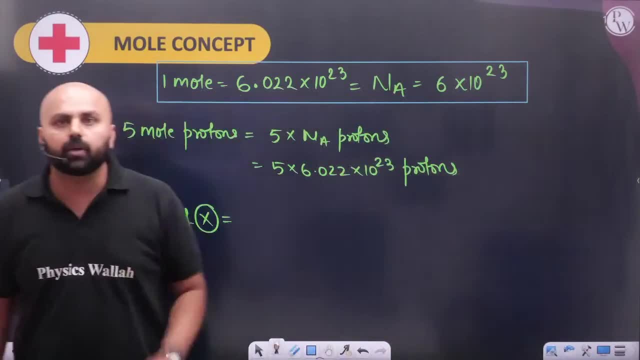 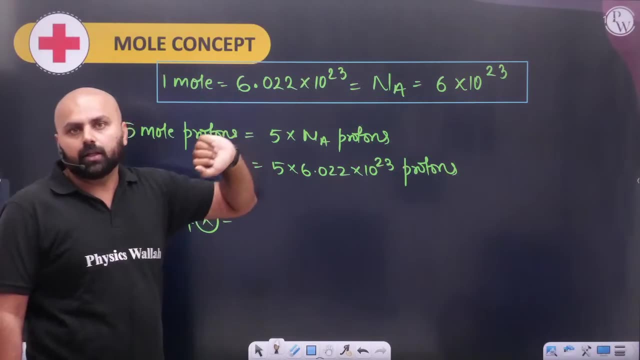 then you will do the questions based on it and you will do it and show now the basic means. that, brother, the more basic. you are thinking that I will not show you the whole definition of the mole. okay, So let's talk about number of moles of x. 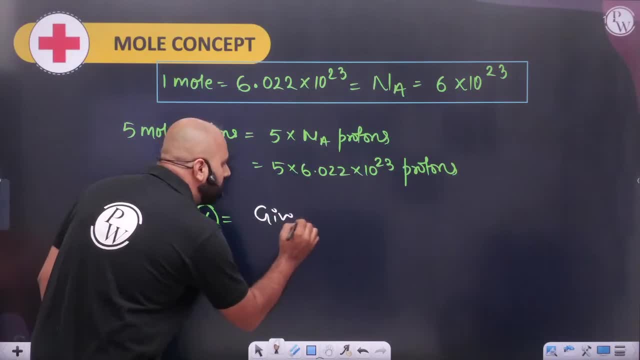 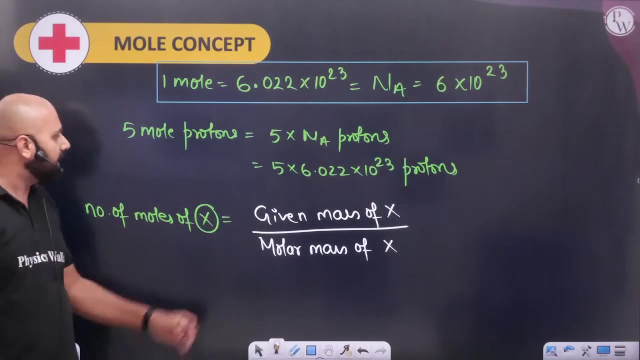 how to calculate the number of moles of x. If you are given mass of x Divided by molar mass of x. So the first formula is given: mass of x molar mass of x. This formula is given mass of x molar mass of x. 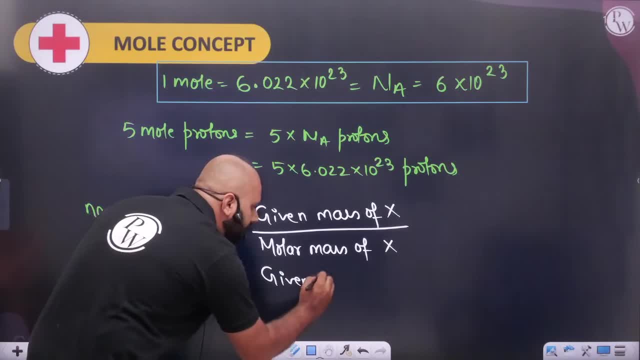 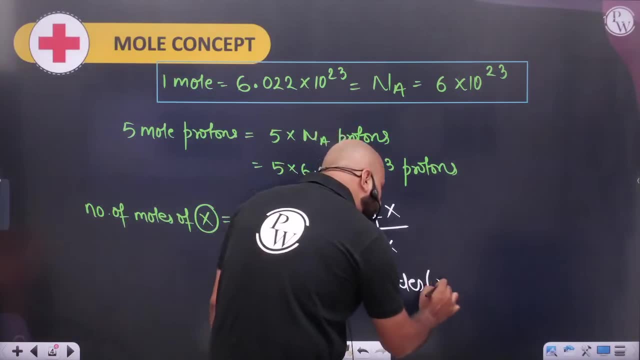 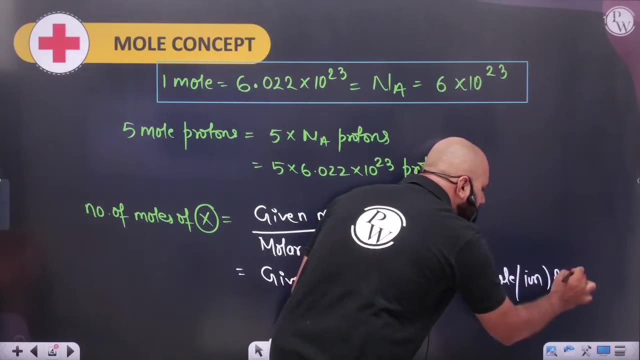 Then the second formula is: given number of particles, given number of particles, anything can happen in particles. it depends, listen carefully, it depends. there is an atom, there is a molecule, there is an ion. whose is it means? how is x divided by Avgadro number? 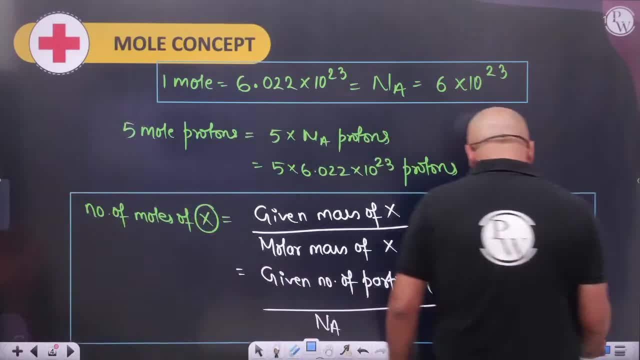 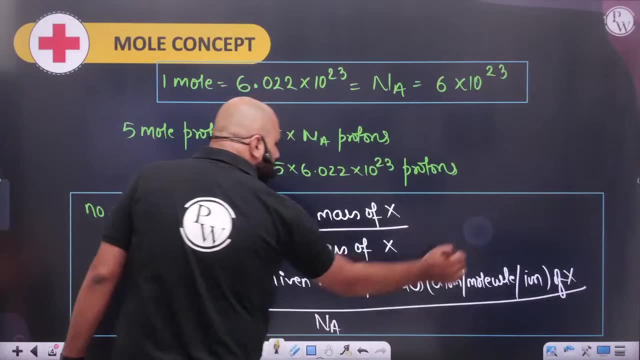 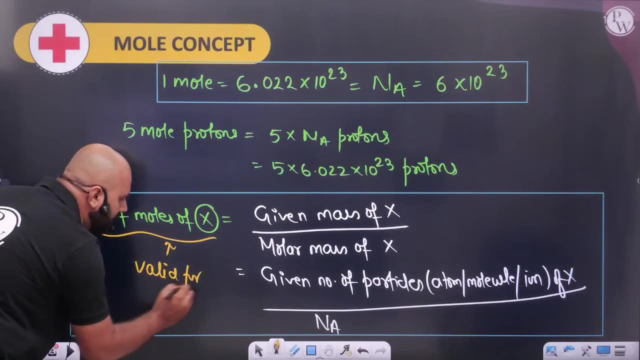 Sir, I am writing this formula because I will tell you a limitation with this formula. this formula will be valid for everyone. this formula will be valid for everyone. this formula is valid for solid liquid gas. it will be valid for everyone. you take solid, take liquid, take gas. it is valid for everyone. 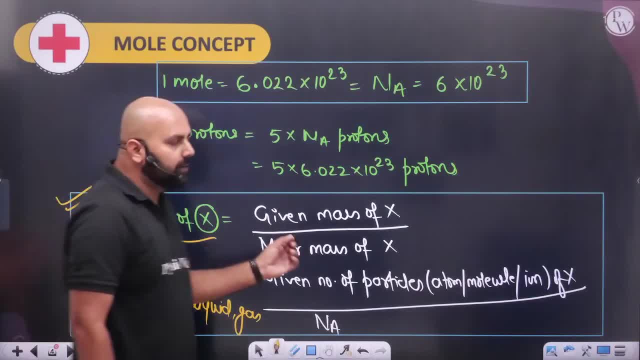 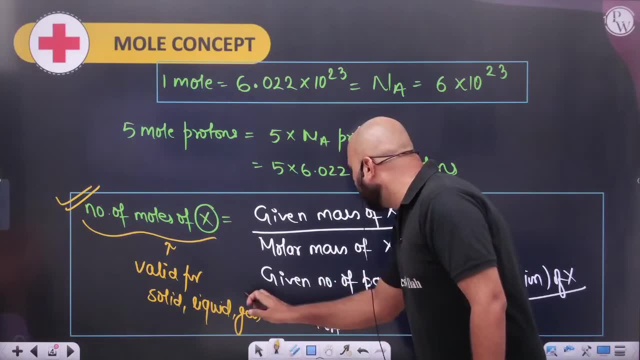 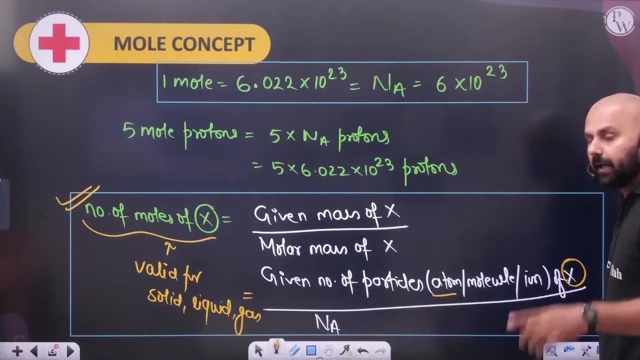 This formula is the number of moles, given mass upon molar mass, given mass upon molar mass, divided by Avgadro. Or, if I talk, given number of, given number of particles. particles can be anything. if there is x atom in front, look carefully. if there is x atom, if there is x atom, then what will happen to the x atom? if there is x atom, then divide the atom. if there is a molecule, then divide the molecule. if there is an ion, then divide the ions, sure? 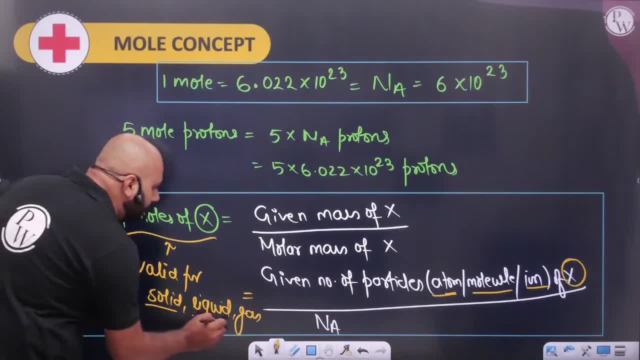 Sir, this formula to get the number of moles is valid for everyone. solid liquid gas is valid for all three. why am I making you write like this? see a little, see yourself talk about solid liquid gas. 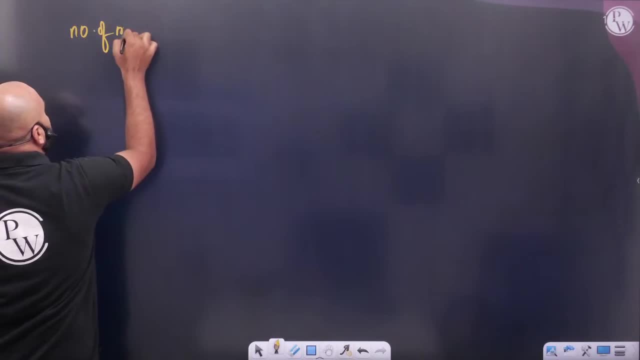 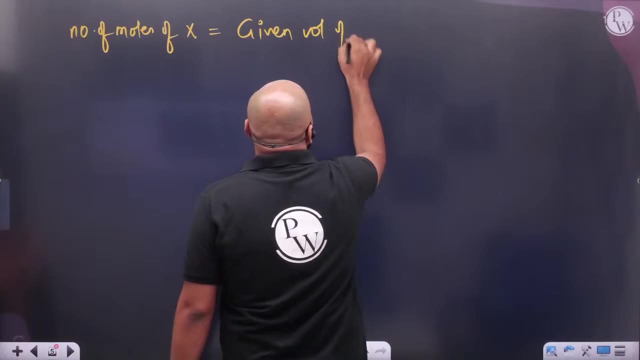 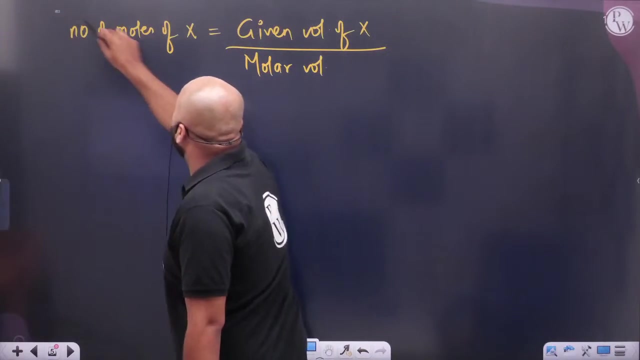 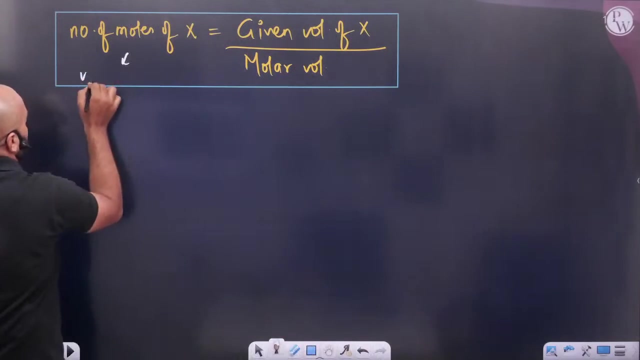 Sir, there is one more formula. and what does everyone do to get the number of moles of x? then there is one more formula: given volume of x divided by molar volume, Sir, this formula, that's why I am writing separately, sir, this formula will be in your life. this is only known. this will only be valid for whom? valid only for gases. 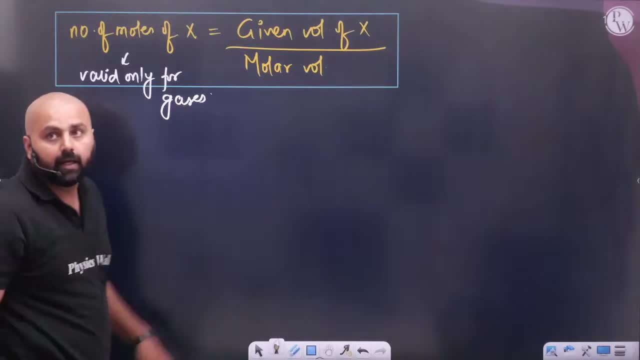 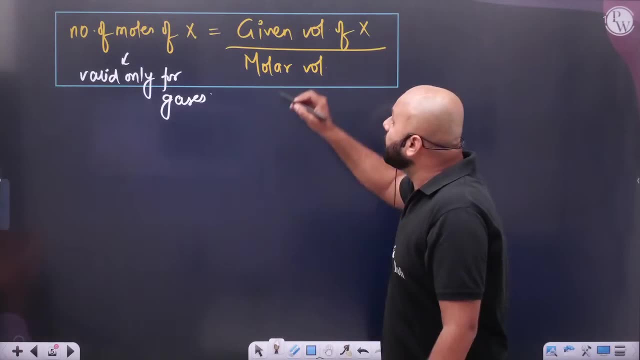 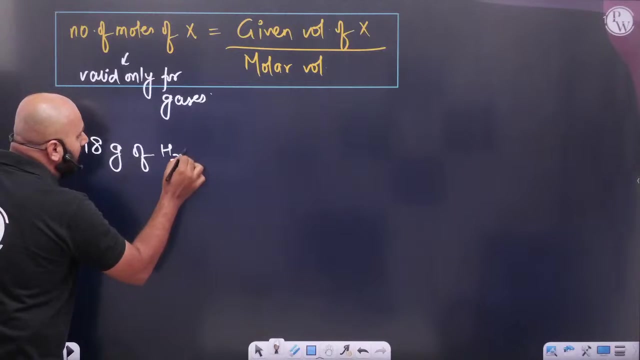 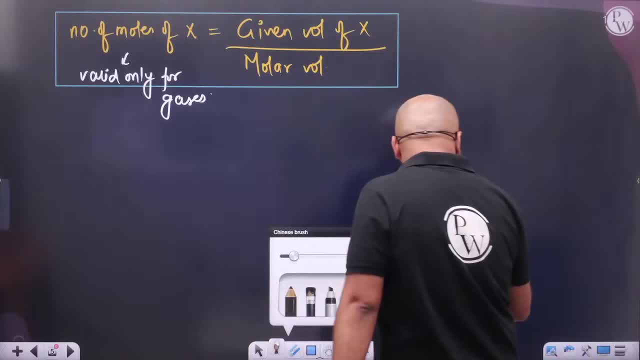 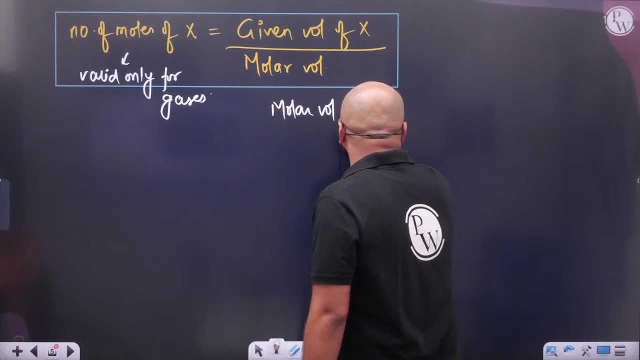 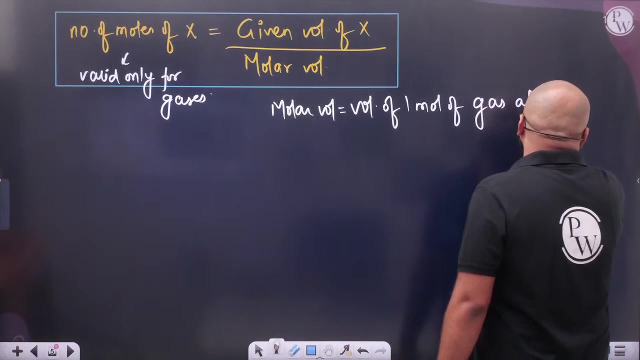 What is molar volume? What is molar volume? See how much is molar volume. molar volume is nothing. molar volume is nothing, son. all the formulas have to be revised. and the same thing: volume of 1 mole of gas at 273 kelvin and 1 bar, or then molar volume works for 1 minute. 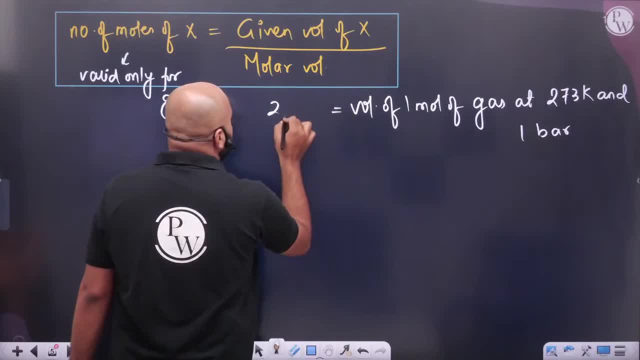 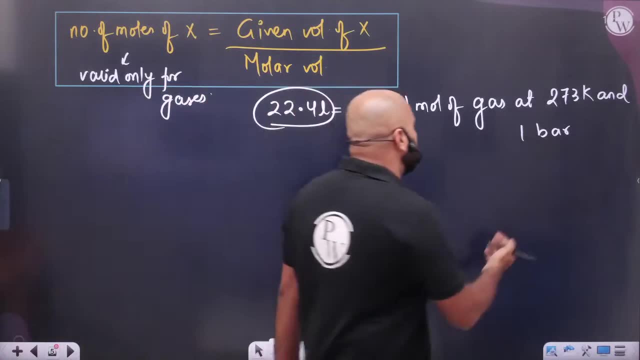 How much molar volume will you use for calculation now? How much will you use? How much will you use? 22.4 liters. this is the molar volume, the calculation we will use in our molar volume. we will use this much. 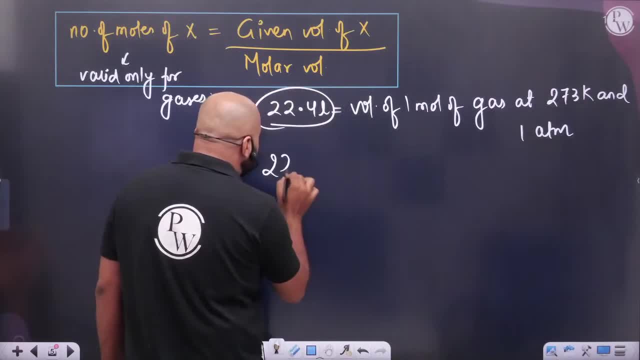 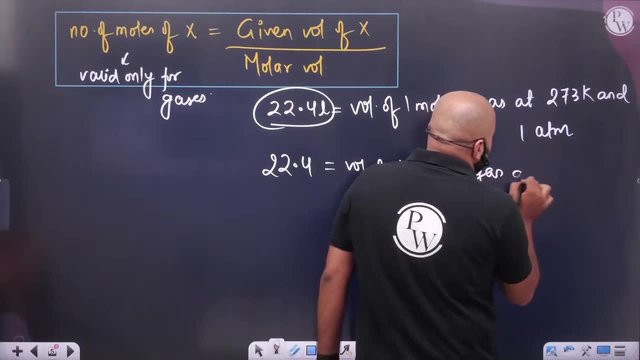 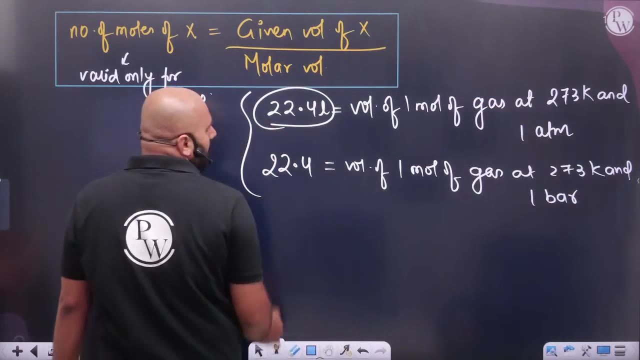 But nowadays in NCRT its value has been changed a little. That is what Volume of 1 mole of gas at 273 kelvin and 1 bar. But don't be afraid in the exam hall don't think all of these. why did just a little change come? 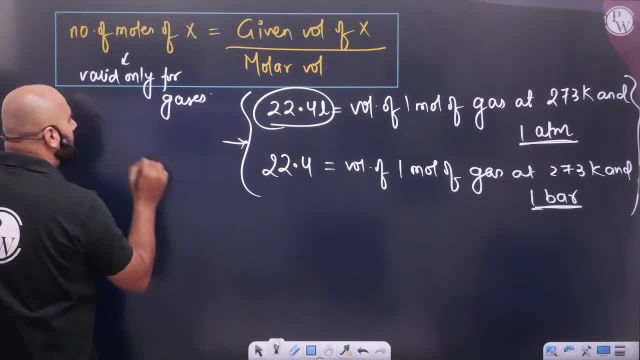 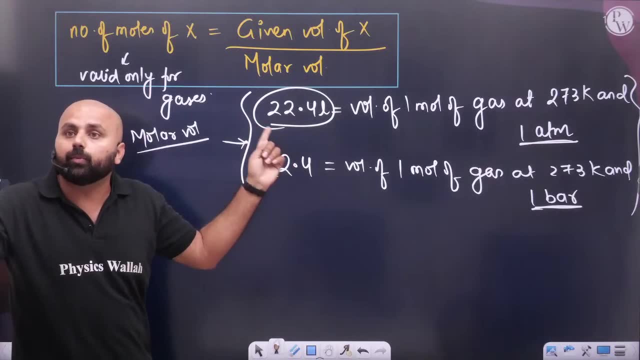 Because here, what has happened to 1 ATM, 1 bar, And what is this for me? Molar volume. Now, whenever you get to calculate the question in the exam hall, whenever you get to calculate the question, you have to take 22.4.. 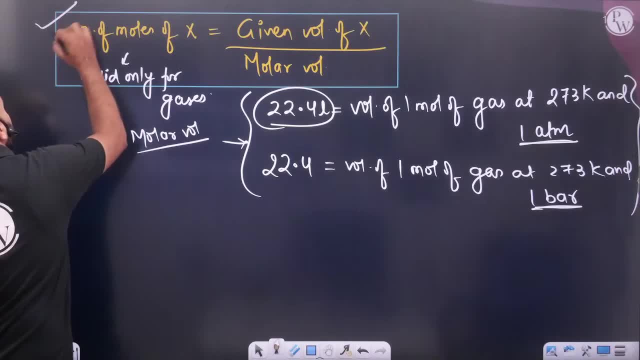 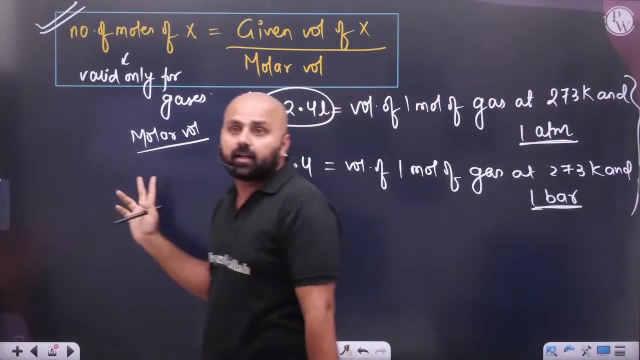 Take care of yourself, Sir. for whom is this formula? For gases? Just for whom? For gases? Don't put it apart from that, brother. That's why I have written differently: 22.7.. Why does 22.7 change? 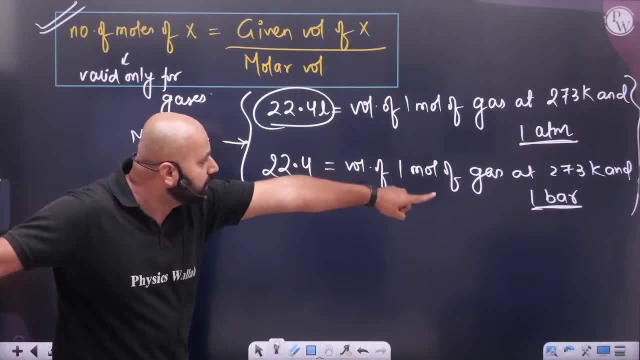 Because you have changed the pressure a little. Why? Because you have changed the pressure a little. What did you put in place of 1 ATM, 1 bar Gas? Yes, If there is water vapour, it will be different, right? 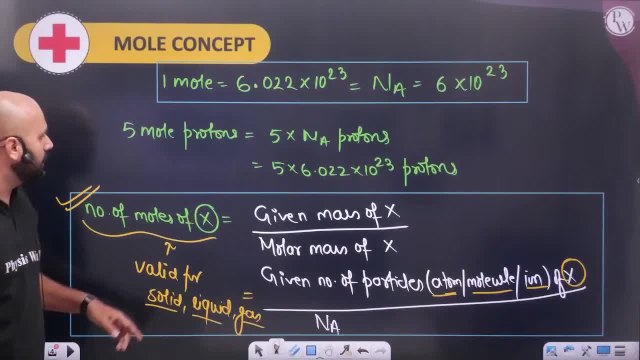 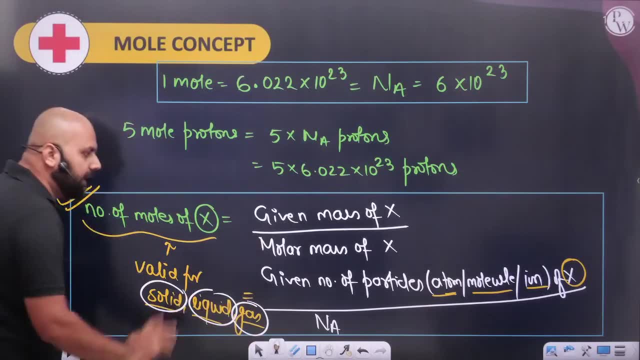 If there is water vapour, then there will be gas. So it is simple. See this formula with yourself. On water- Sorry, I am saying water- This solid liquid gas is valid for all three. These two formulas are valid for all three. 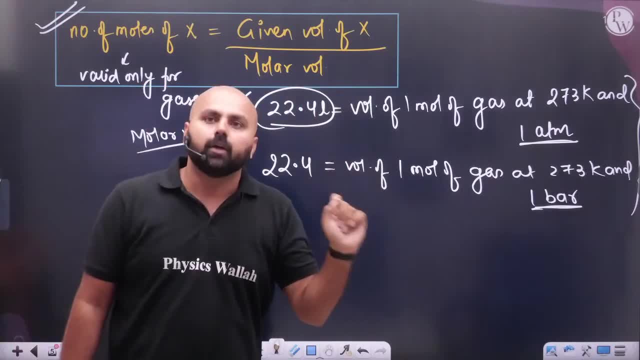 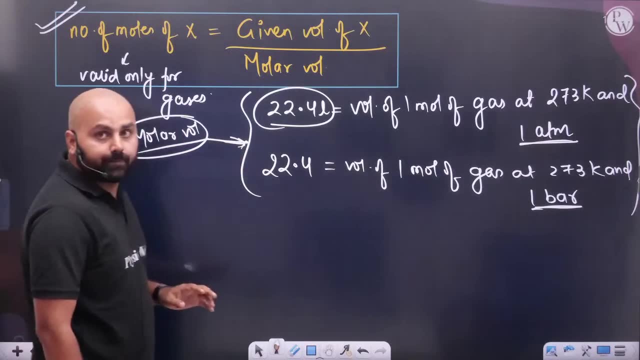 But a lot of people make a lot of mistakes, So don't make this mistake. Whenever it is said to calculate the number of moles of x, you have three formulas And try to run the opposite. Try to run the opposite. A Y map is made on it, son. 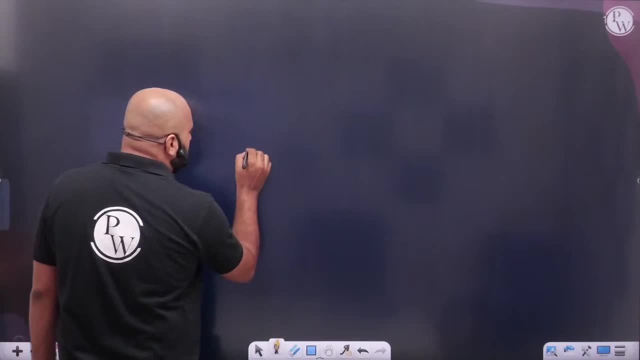 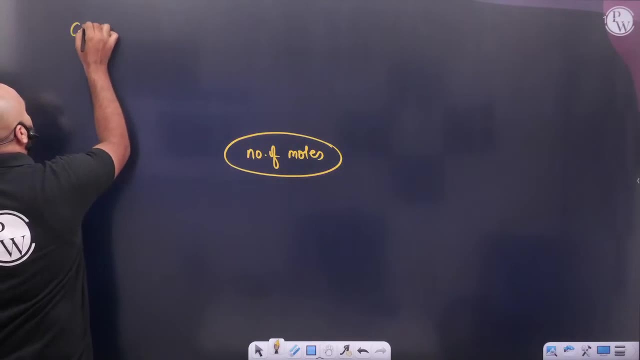 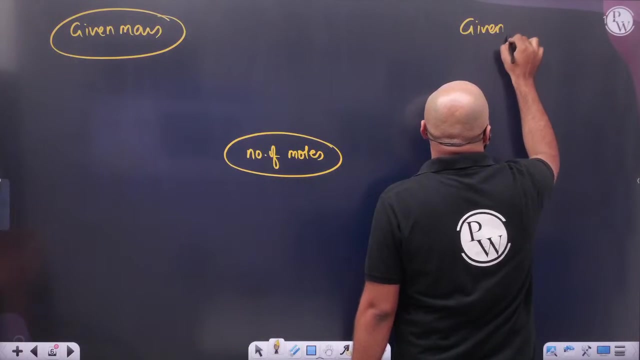 Look carefully, Look carefully. Its Y map is made. The most question that comes with the time of the mole is See that If what is given to you, Given mass, is given, Look carefully, son. Given mass is given If you have given given number of given particles. 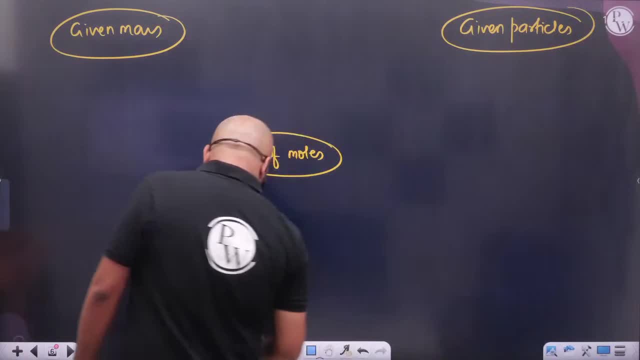 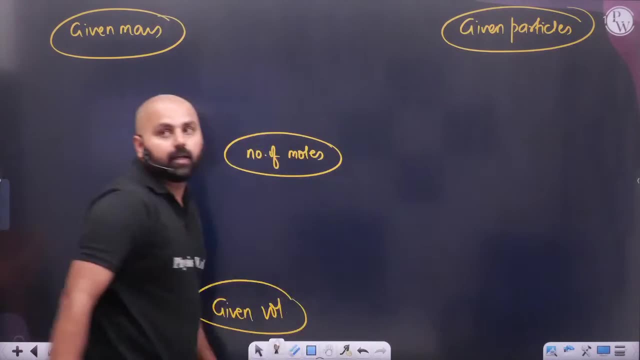 Check this thing And If there is gas. So here you have given a given volume. Son, I am making a mind map for you to see carefully What is going to happen here If I am told, given mass, number of moles have to be taken out from given mass. 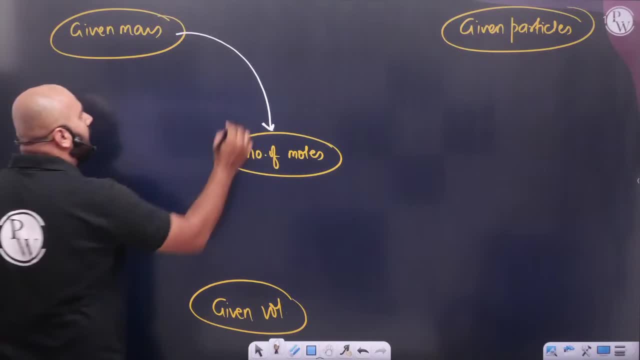 See this carefully. Number of moles have to be taken out from given mass. So what will you do? What will you do by dividing? You will do molar mass. Sir, what will you do with molar mass? You will divide it. 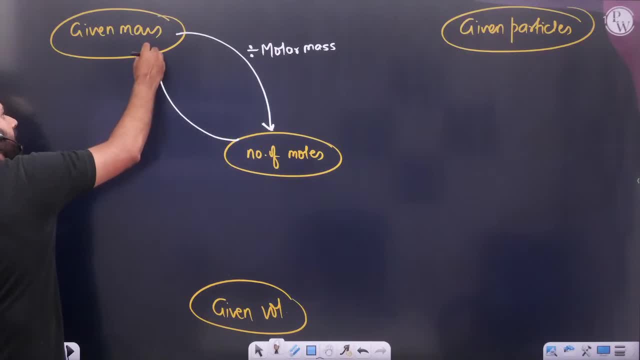 But if you have to take this number of moles in which, If you have to take mass from number of moles, what are you going to do? You are going to do multiplied by molar mass. Remember if you divide while going. 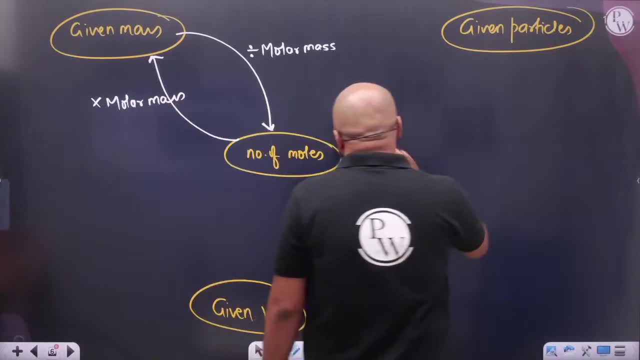 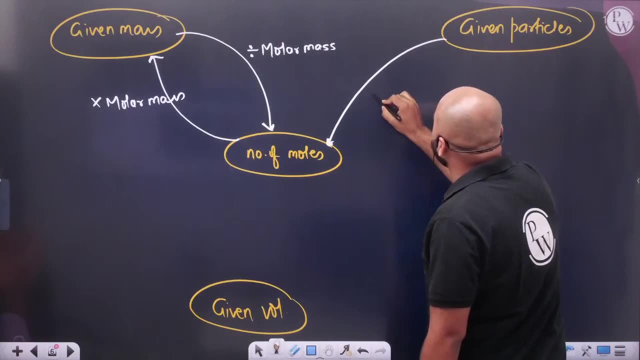 then what will happen while coming? Multiply, Sir. see this with you. See this with you. What will happen? Number of moles: if given particles are given and you have to take out number of moles, then what will you do? by dividing? 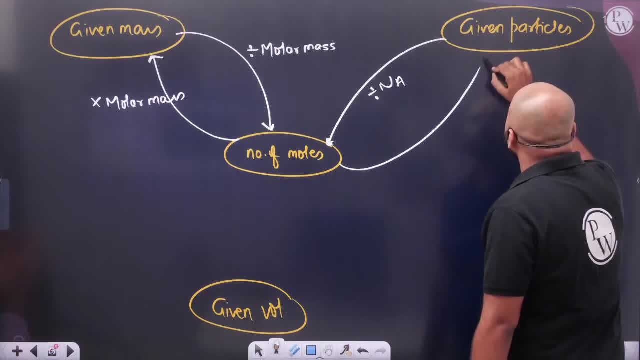 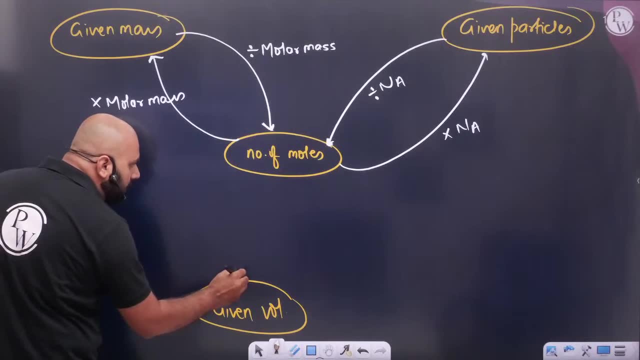 Avogadro number. And if you have to go back, then from here we will multiply Avogadro number. Similarly, given volume is there, Given mass is there. If you have to take number of moles from given volume, then what will you do? 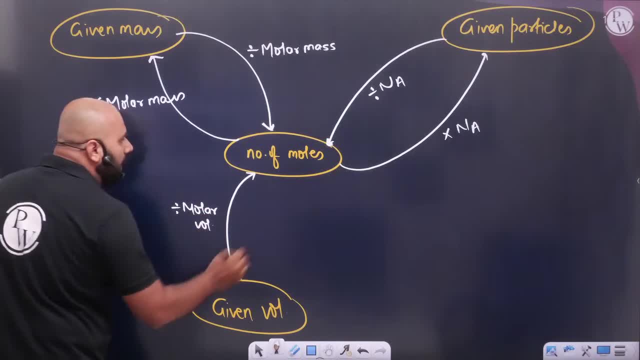 You have to divide molar volume by molar volume And if you want to go back, then what will happen, Multiply by what will happen Molar volume. So this will be my complete Okay. There is one more question here. 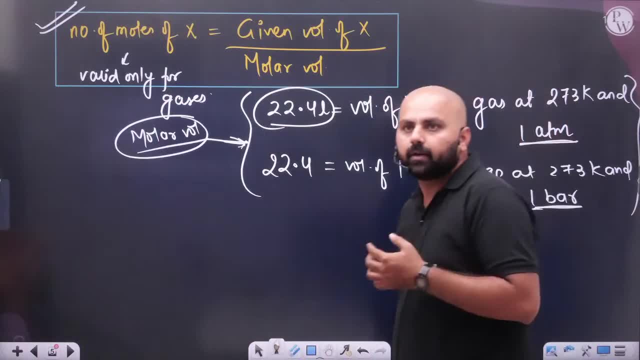 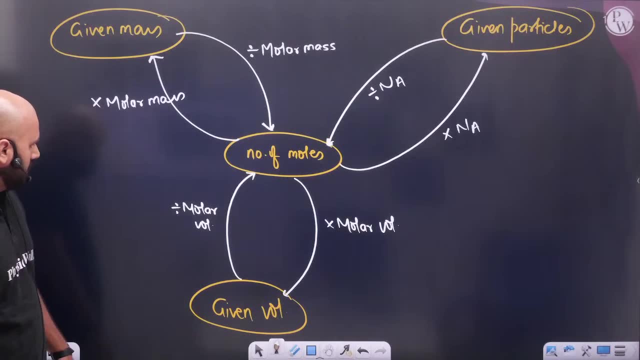 Direct calculation: mistake of number of moles. Direct calculation: mistake of number of roots. Okay, Direct calculation of number of moles. Do you have it? Yes, it is correct. Divide by Where is it? See this? Keep one more thing in mind here. 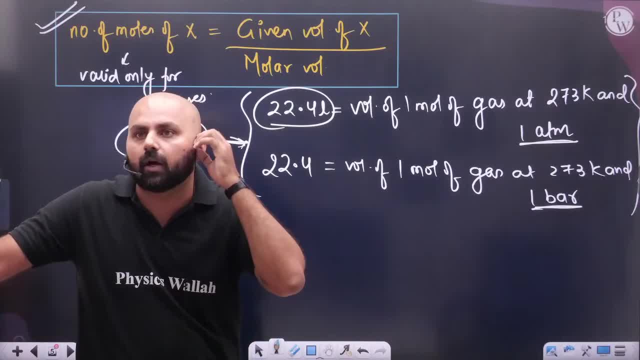 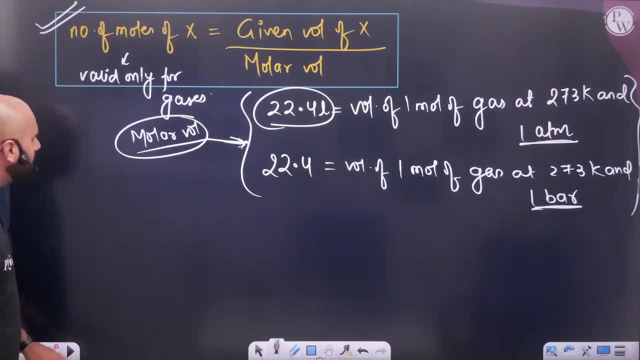 Whenever you have a question of 2020, we will see. now What is printing mistake? Okay, Yes, Of liquid. Do not do with the volume of liquid. Do not do with the volume of liquid. Given particles are there? Divide by Avogadro number. 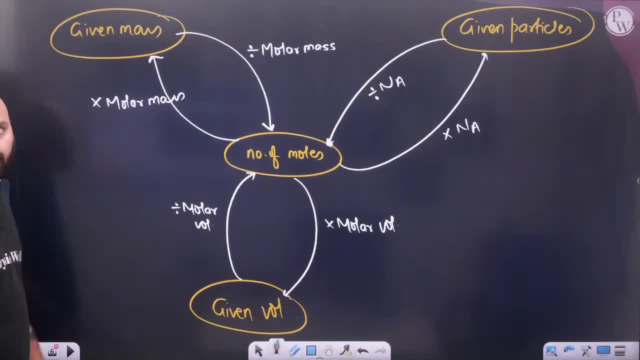 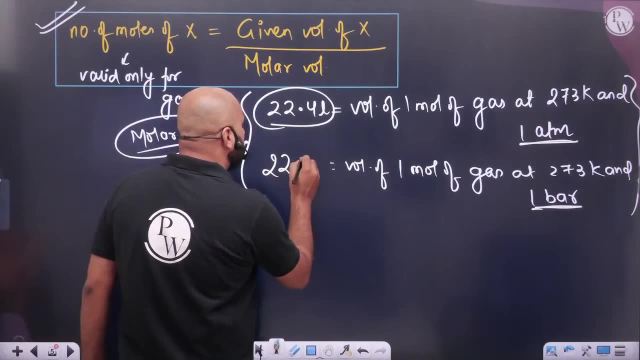 If you go here, then multiplied It is correct. Where are you confusing You too? Okay, 22.7. Okay. 22.7. Okay. 22.7 liter. Okay, This is 22.7 liter. 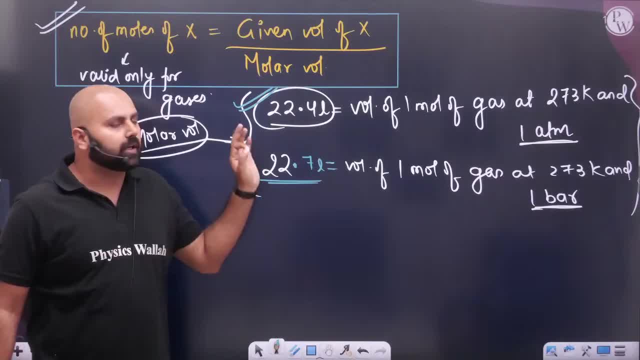 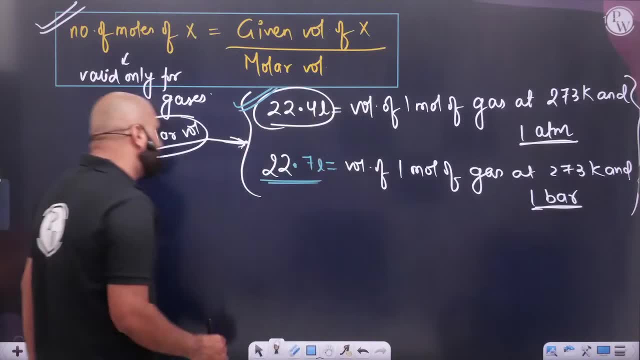 In both of these. You have to use this in numericals. Close your eyes Until the exam hall is not spoken. Until the exam hall is not spoken, Understand the emotions. See this. I will tell you one more thing. One more thing. 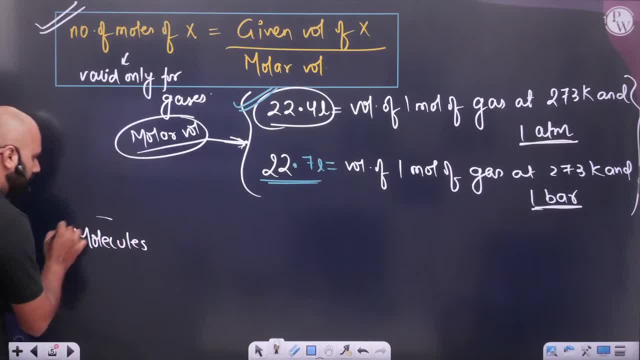 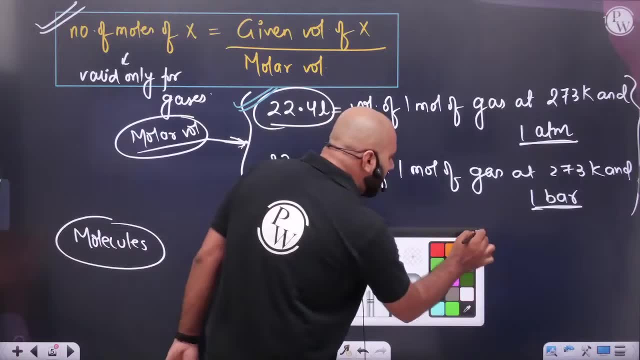 On which most questions are made: If there are molecules, Look carefully. If there are molecules, These are very troubling questions In today's time. It is a very basic thing Which comes from 9-10. But many people make a mistake. 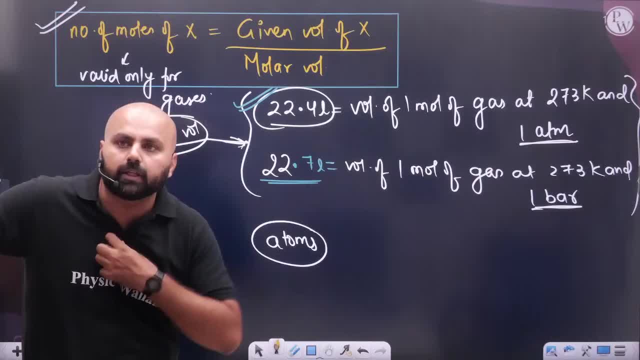 Many people make a mistake. What happens? See this: What happens, Sir? there is a molecule, The atom has to go from the molecule. So from whom do you have to multiply? From the atomicity of that molecule, Sir, from its atomicity. 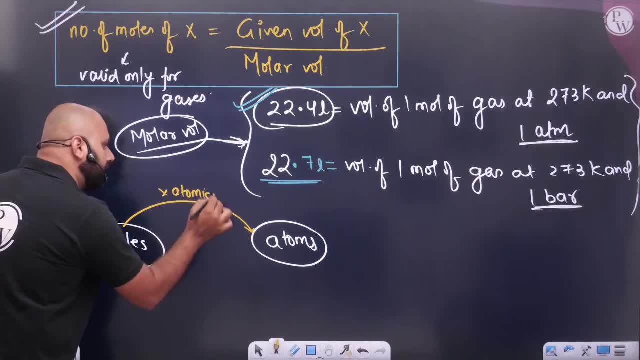 Means, If you have given C6H12O6.. Son see, Can't go more basic than this. See this: You have given C6H12O6.. So, if you want carbon atoms, So you have given C6H12O6. 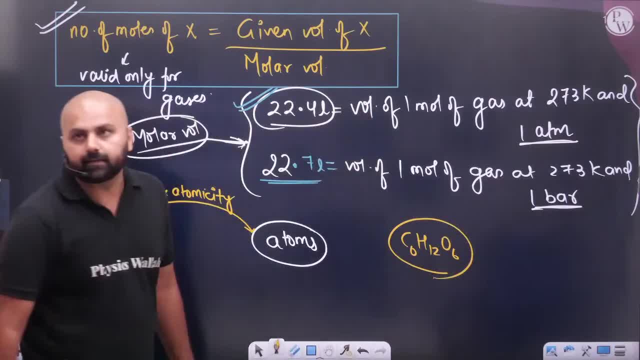 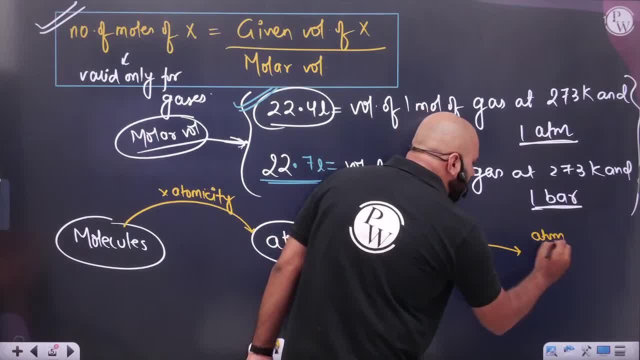 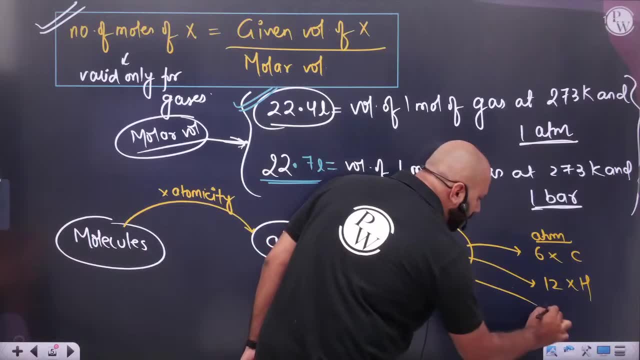 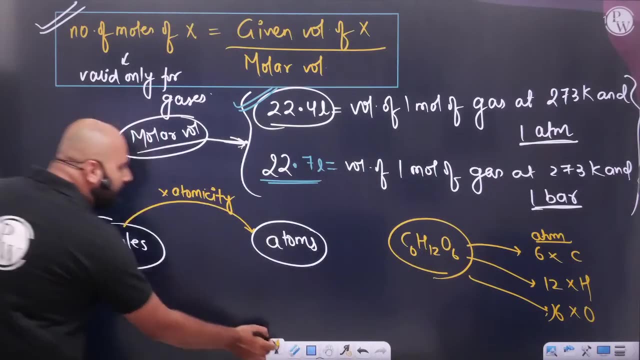 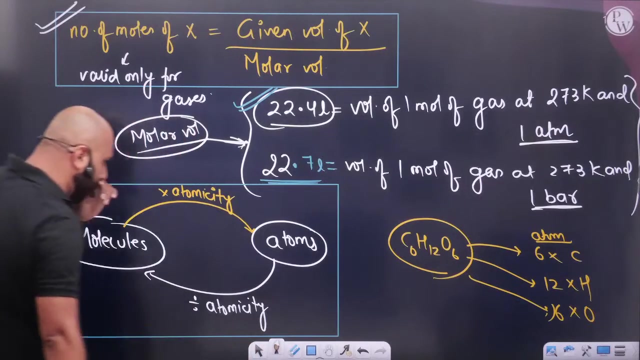 Sur Corv, If you want from carbs will have to divide. So this formula or you can say: this is a basic thing. remember I am telling you a basic thing, Listen carefully, Look carefully at yourself. Molecule from molecule, number of moles. 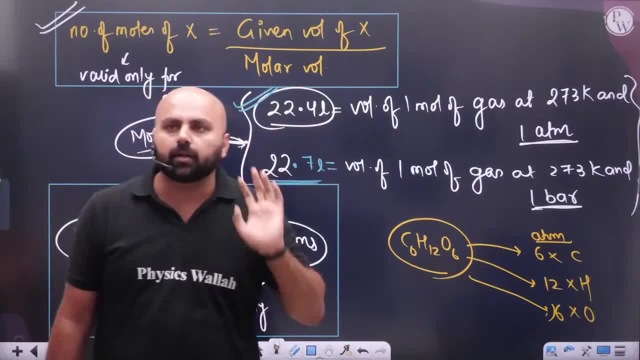 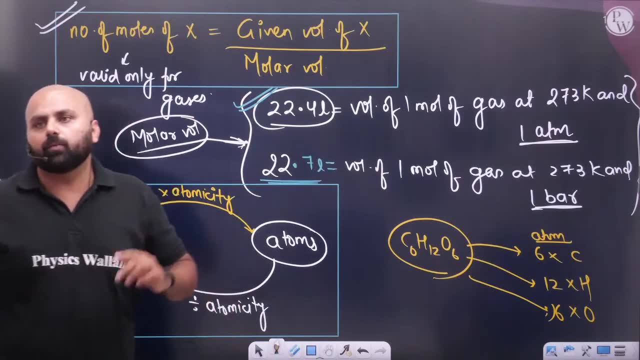 basic formulas, basic things. let's sit on this and do a question. If there is a liquid on it, then the formula of molar volume will not be valid on it. The formula of molar volume will not be valid on it, Okay. 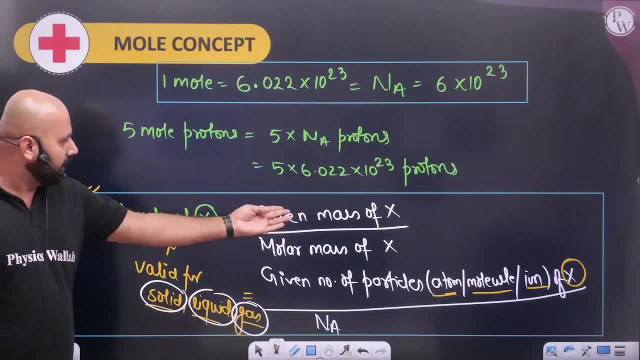 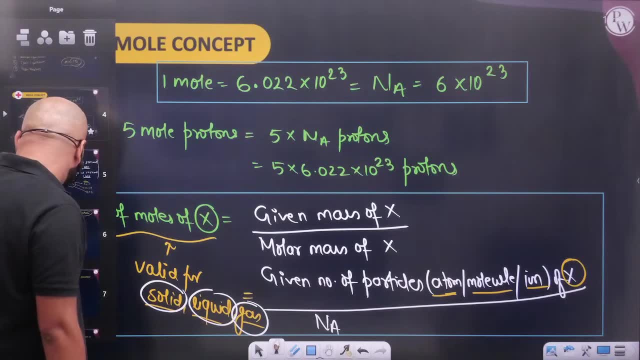 In the case of liquid, these two formulas have been given to you. Given mass or number of particles, It will be done Now, see. Now let's come to the first question. Let's try to come to the first question. Let's try to come to the first question. 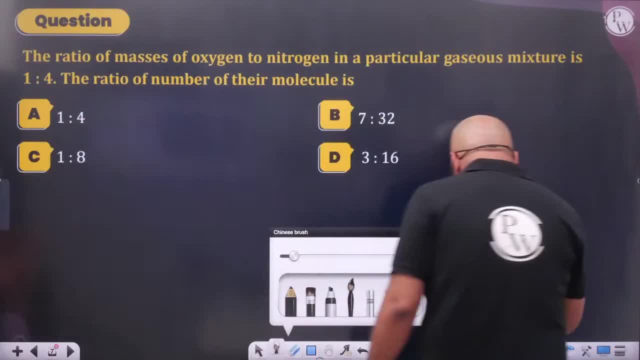 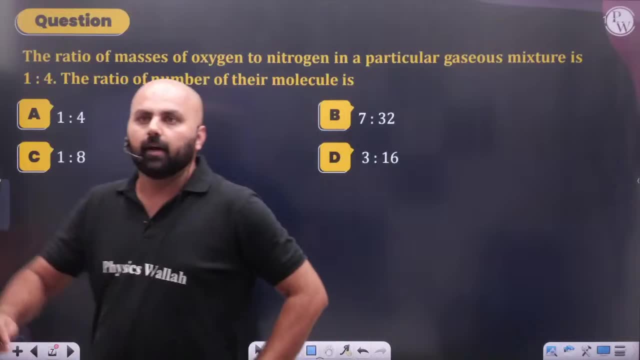 And the first question is for you: Who will become a doctor? Let's start quickly. See this question. If someone has given me that ratio of masses has been given. Please look at yourself fast, Sir. as soon as possible, attempt the questions. 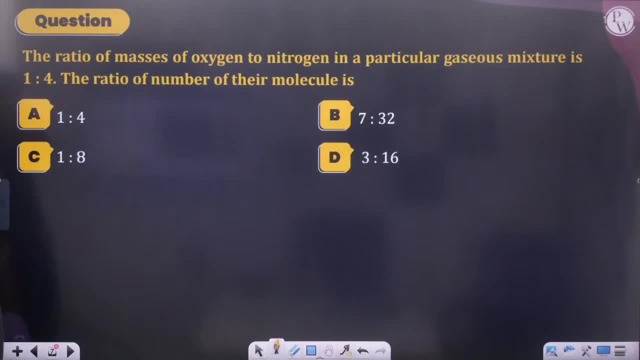 Those who can do it. this question is of 15 to 20 seconds. Please attempt and see. Ratio of masses of oxygen to nitrogen. Ratio of masses of oxygen to nitrogen. Ratio of masses of oxygen to nitrogen: What is it? Mass is given by oxygen and nitrogen. 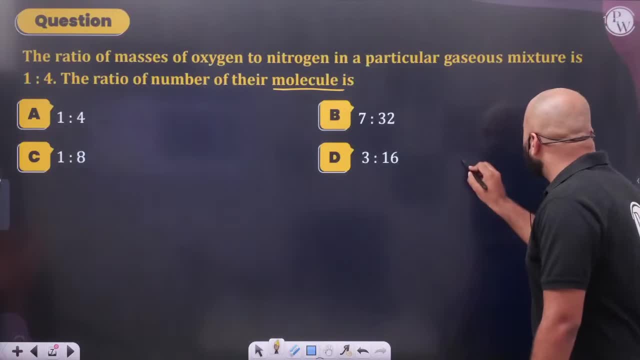 He is saying the ratio of molecules. Sir, given mass of O2 divided by given mass of N2 ratio, What is given 1 by 4.. As soon as it was found in the exam hall, what is its mass? X gram. 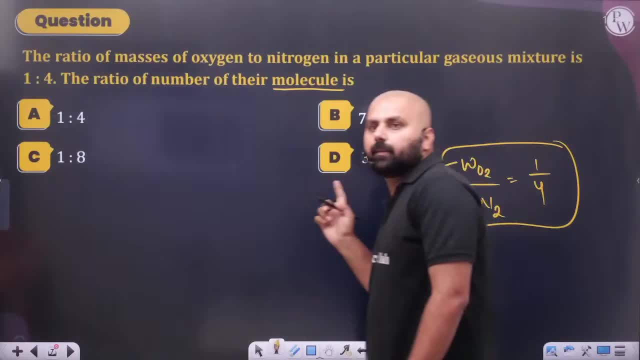 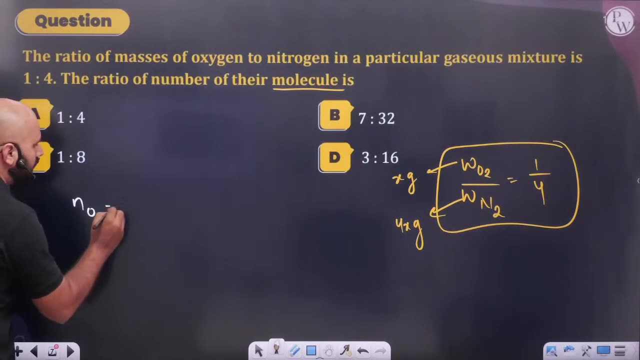 What is its mass 4X gram? What is its mass X gram? What is its mass 4X gram, Sir? quickly see What will be the number of moles of O2?, Sir, X upon 32.. 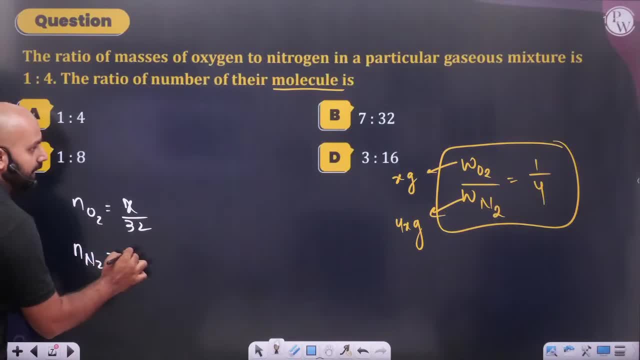 What will be the number of moles of nitrogen, Sir? X upon 32.. What will be the number of moles of nitrogen 4X upon 28.. 4X upon 28.. Sir, talk about molecules, Molecules of. 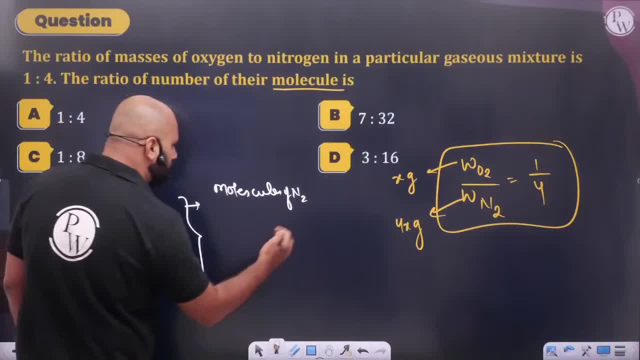 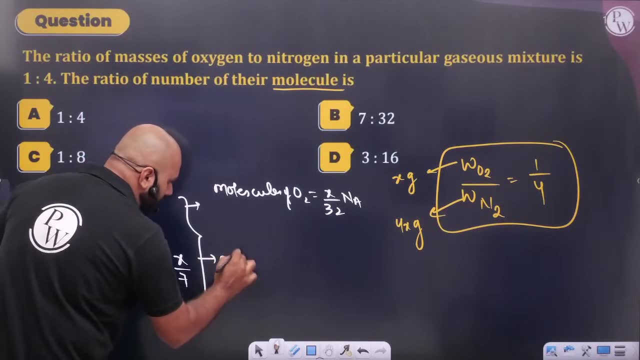 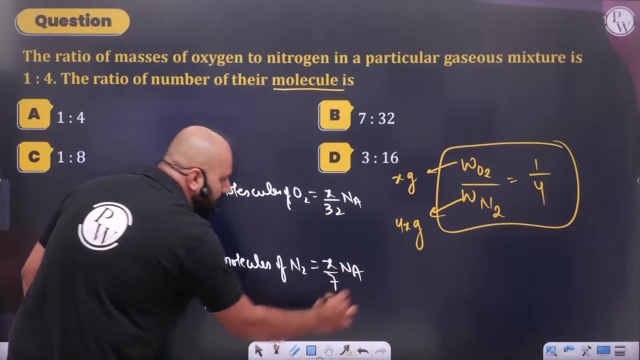 Molecules of nitrogen. If we talk about molecules of nitrogen, If we talk about oxygen, How much will be the number of molecules Into N? Molecules of nitrogen: If we talk about nitrogen, How much will it be X by 7 into N? 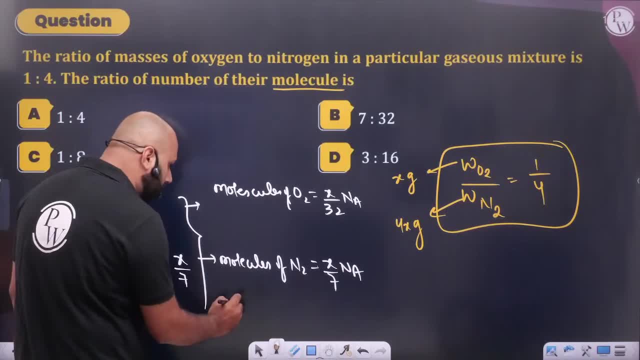 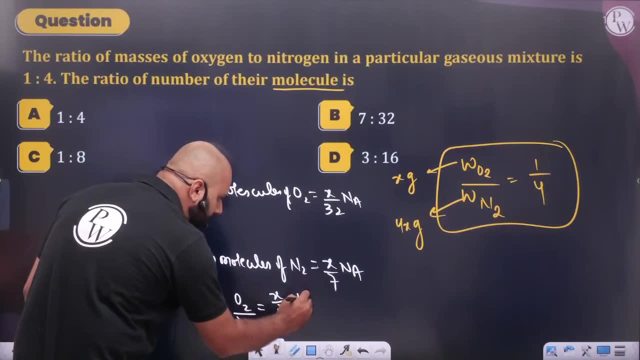 Sir, we have to take its ratio. If we take the ratio of molecules, If I take the ratio of molecules, If I take the ratio of molecules of O2 by N2.. How much will it be, X by 32 N? 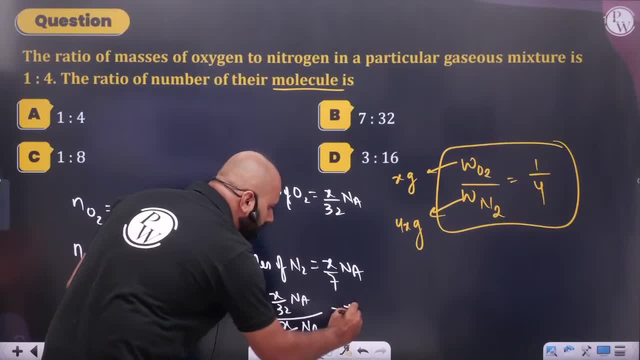 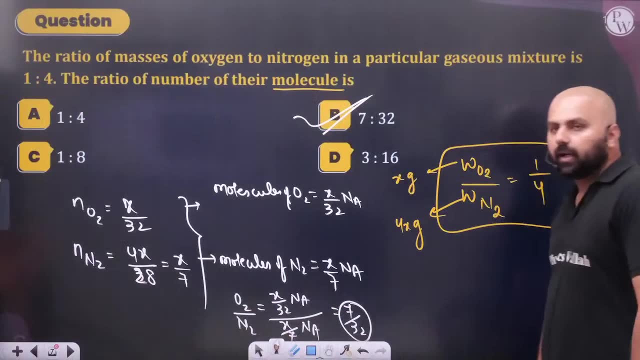 Divided by X by 7 N. As far as I can see, How much will it be X by 7 into N. How much will it be X by 7 into N? Look at it. Let me tell you a simple thing. 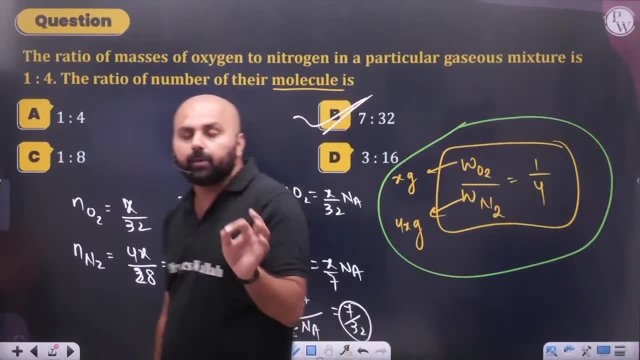 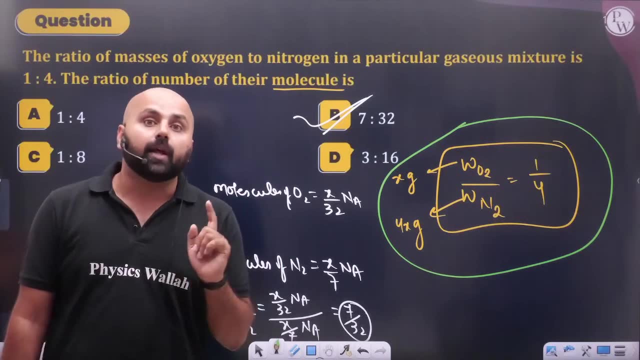 There is no mass in the exam hall. Even if you go to the questions of the solution chapter, there is no mass. It is giving the ratio of moles and mass. That is why I am telling you to be alert. Tell me one thing. 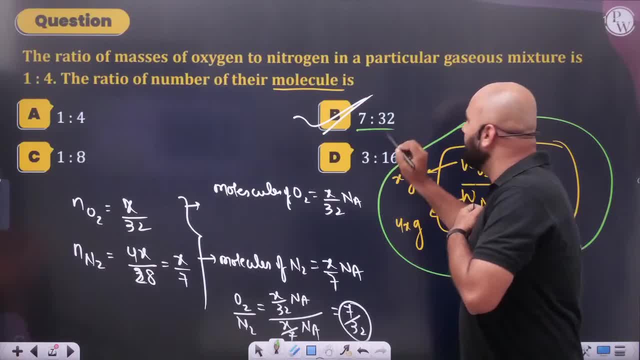 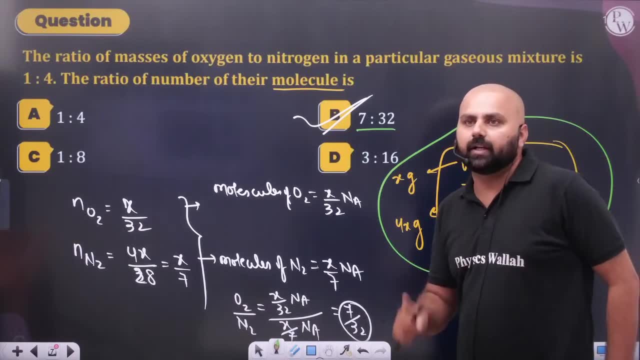 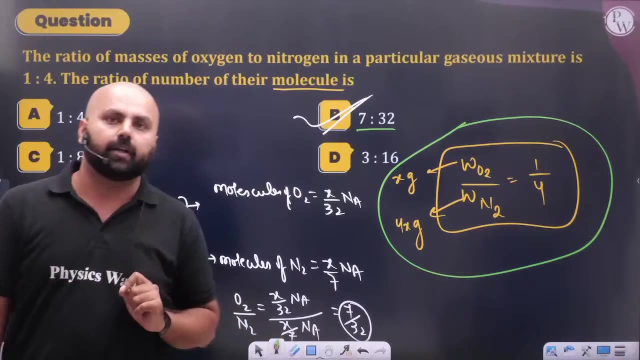 If the ratio of molecules is 7 by 32.. If I ask the ratio of atoms, If I ask the ratio of atoms, How much will it be Same or different? Tell me quickly. If I ask the ratio of atoms, If I ask the ratio of atoms, 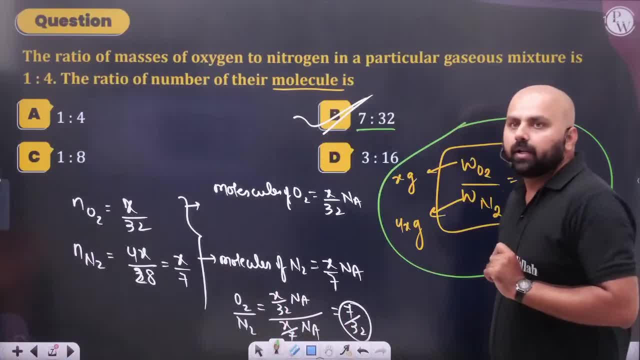 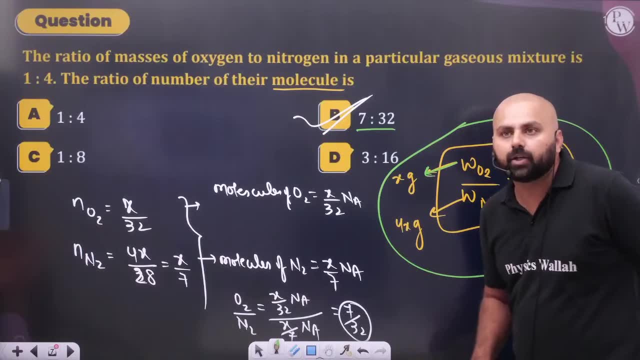 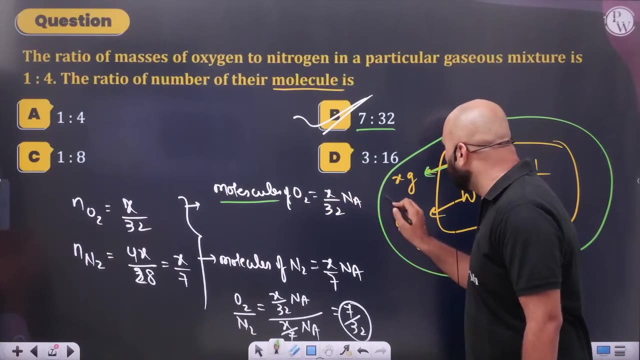 Will it be same or different? Tell me the answer quickly. Will it be same or different, Sir? consider the given mass as X, Because the ratio is given. How much will it be? Will it be same? Why? Because there are so many molecules. 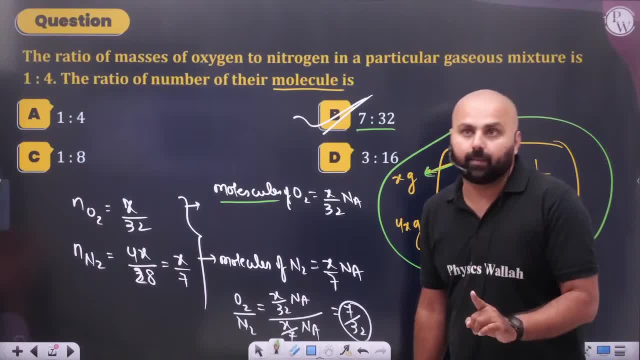 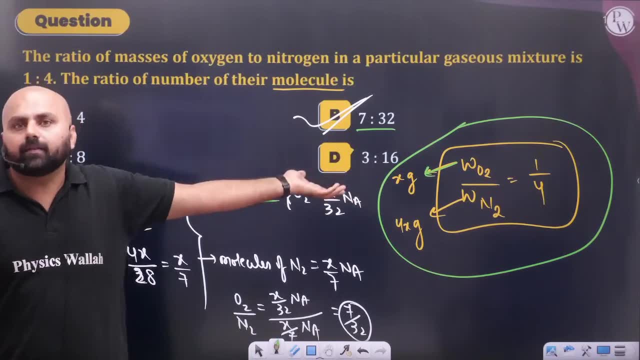 If you multiply it by 2.. What will be the ratio of atoms? It will be same. What will be the ratio of atoms? It will be same. If there is no mass, then the ratio is given, Whatever it is. consider X. 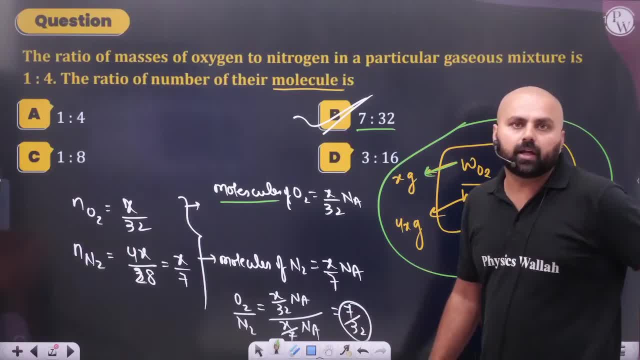 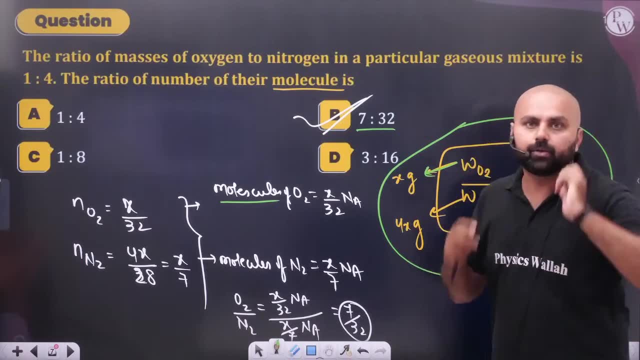 What will be the ratio of X? It will be 4X. What will be the ratio of Nitrogen? It will be 4X. Now you have developed so much basic. Now you have come to the last class. So see, 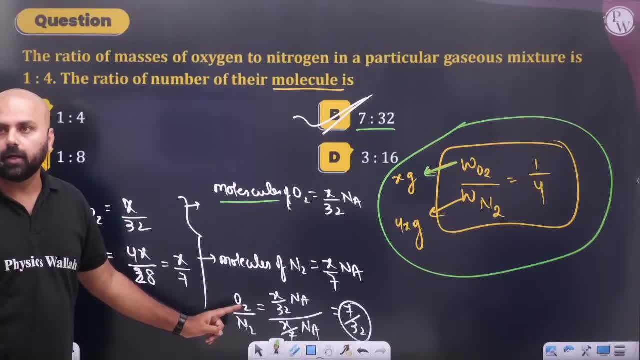 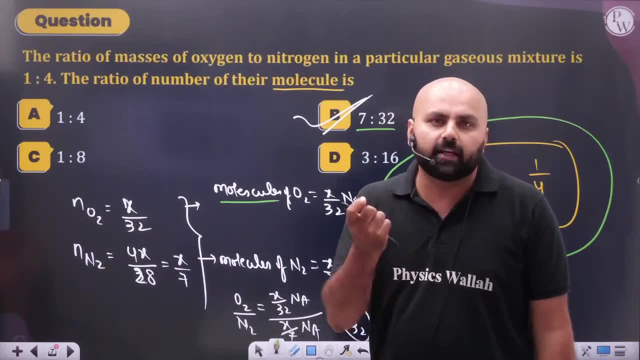 Will it be on molecules? Sure, it will be. Do the next question and show Next question. now a little bit Means 30 seconds Because the exam is from 2 to 5.. Take a pen or a page in 2 to 5.. 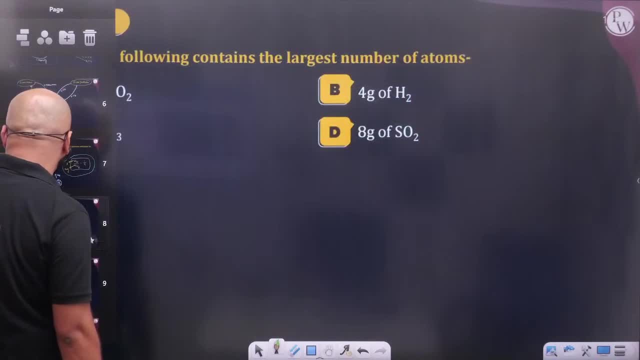 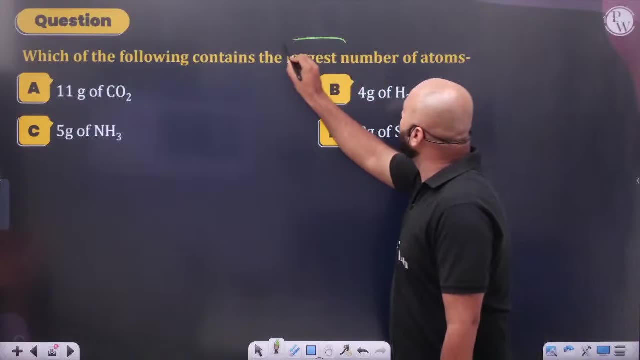 And do the next question and show, It is simple- On atoms and molecules, the probability, The probability of the questions that come. we are talking about them. What do I want? I want the number of atoms in them, Remember, not the molecules. 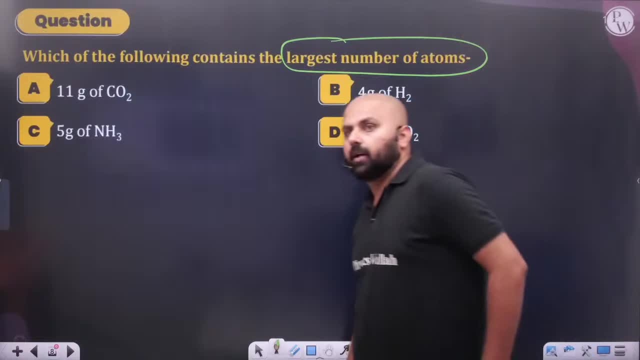 I want the largest number of atoms. I want the largest number of atoms. One is asking: what is Na? Na is your selection, The one who is saying no, no, no, No, no, no, no. What is Na? 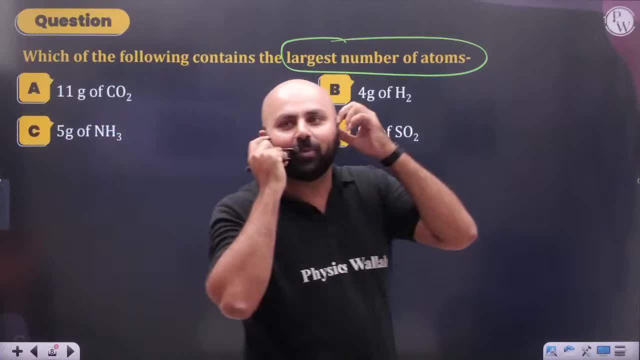 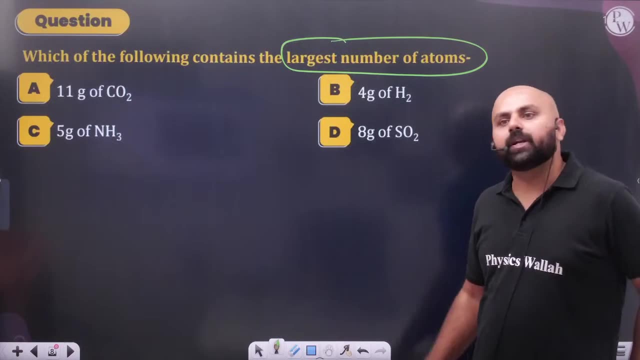 Come on quickly. We are following as largest number of atoms. Quickly Son. these are the chances whose questions will come faster. The chances of getting more and more are of these questions. The chances of these questions are very high. See quickly what will happen. 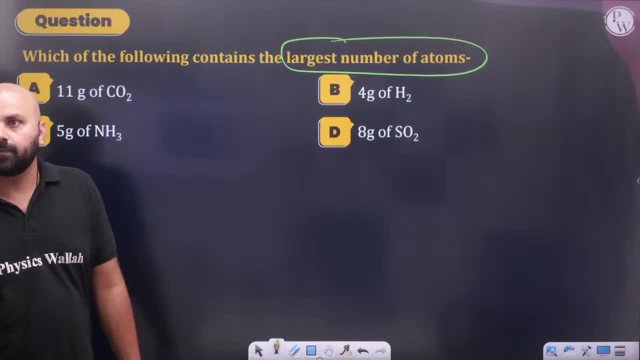 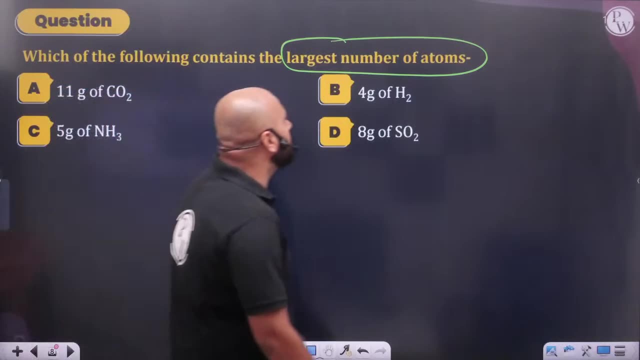 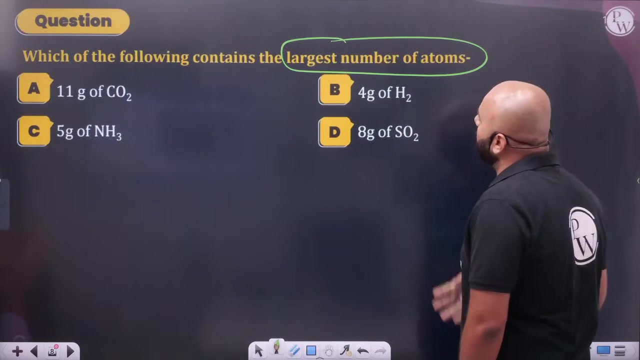 What will happen? Yes, brother, Why did you take the mass of oxygen? 32?? Because O2 molecule means if oxygen was an atom, it would be alone. When we are talking about molecules, molecule means O2.. Largest number of atoms. 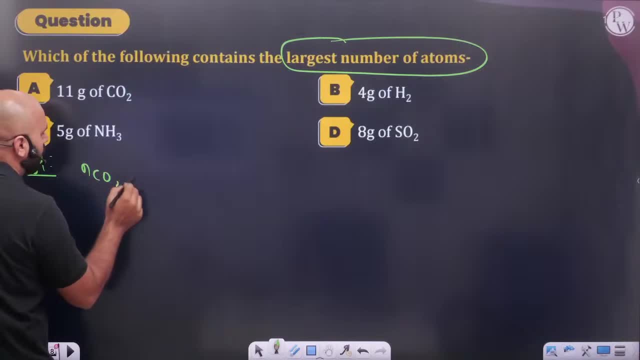 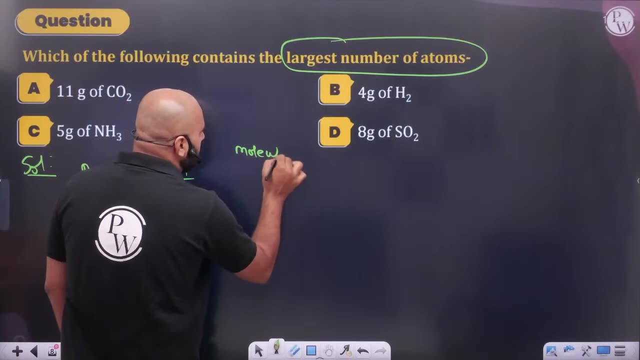 First thing, let me do one thing. Let me take out the number of moles of CO2.. Number of moles of CO2, 11 upon 44,, 1 upon 4.. If I talk about molecules, then how many molecules will be there? 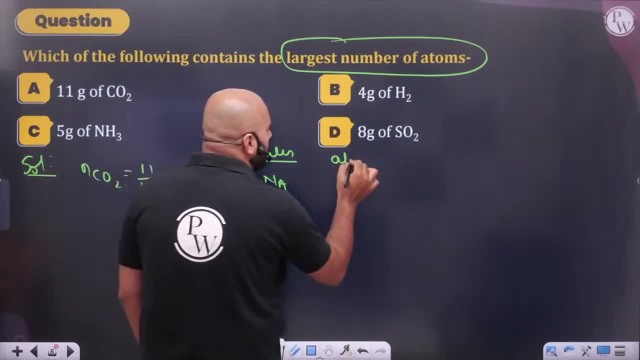 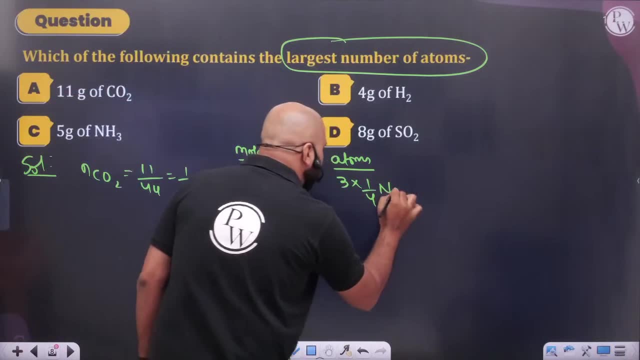 Sir, 1 upon 4 into Na. If I talk about atoms, then in atoms how much is the total atomicity of CO2? 3.. 3 times 1 by 4 Na, This will come. Let me take out the number of moles of H2.. 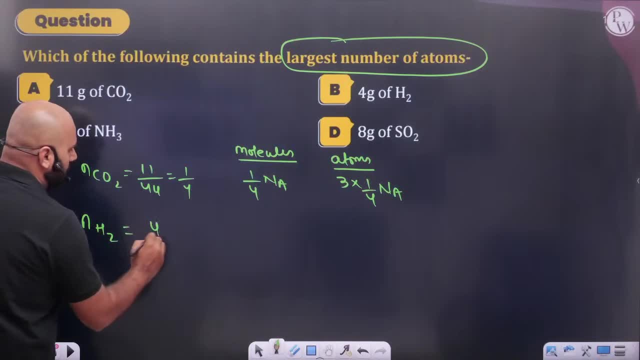 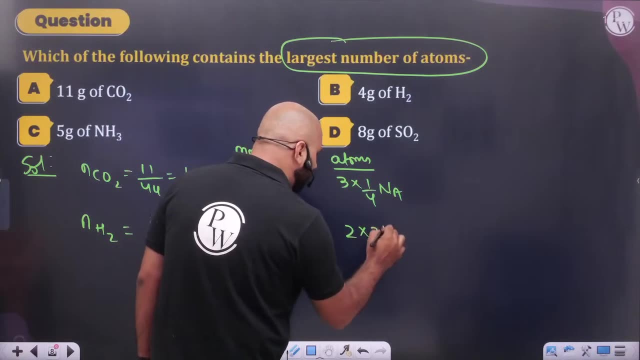 Number of moles of H2.. 4 upon 2.. 2 is there, This is 2 Na And this is 2 times because there are 2 in one molecule. so this is 2 times Na. Number of moles of ammonia. 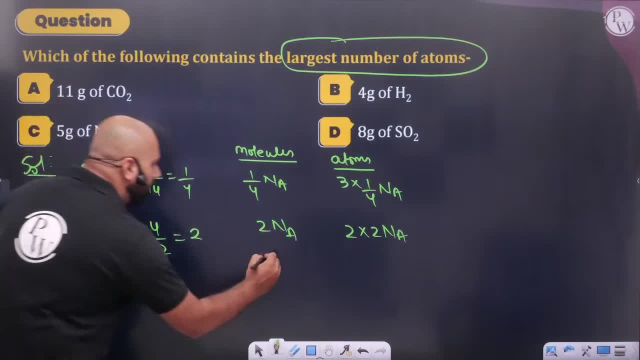 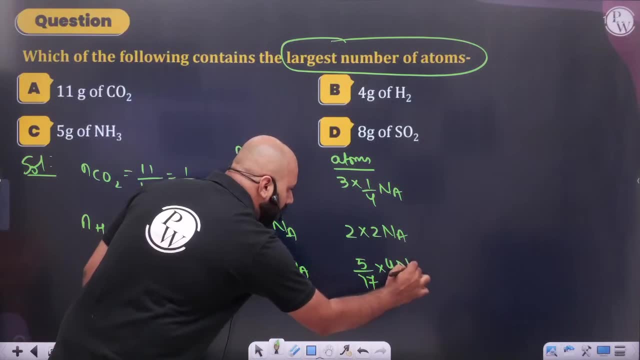 Ammonia in exam hall, those who have a lot of basics. they will have to take it out like this: If you can do fast guess, then you know what to do here. 17 into 4 Na Till now you must have started getting the answer. 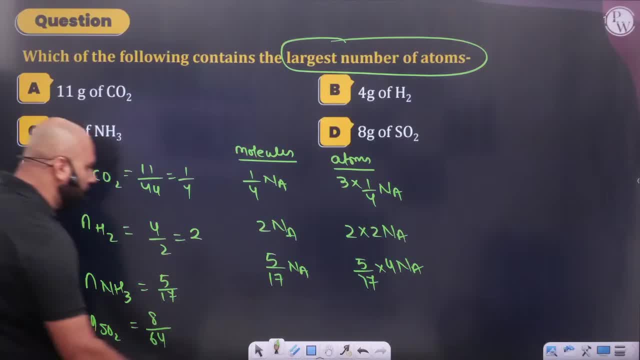 You must have started getting the answer: 8 upon 64. And here: 8 upon 64., That means 1 by 8.. 1 by 8.. 8 upon 64.. 8 upon 64., That is 1 by 8.. 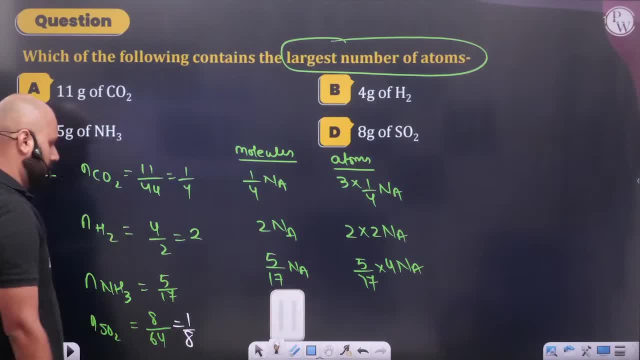 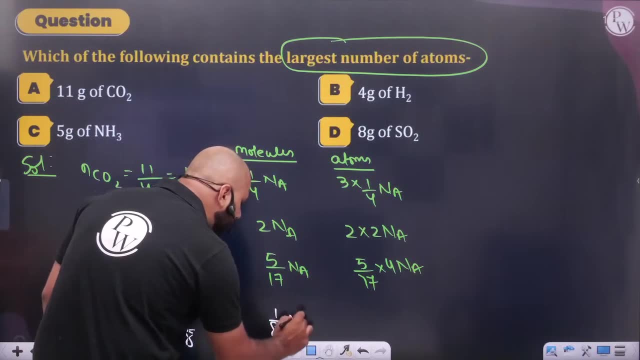 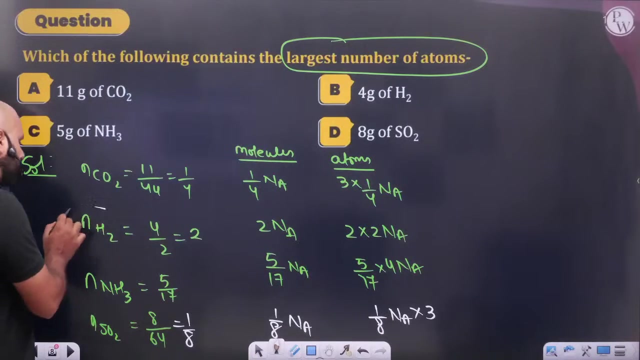 And here 1 by 8.. 1 by 8.. 1 by 8.. Here it is: 1 by 8 into a number. This 1 by 8 into a number, Into 3.. You must be seeing the biggest number. 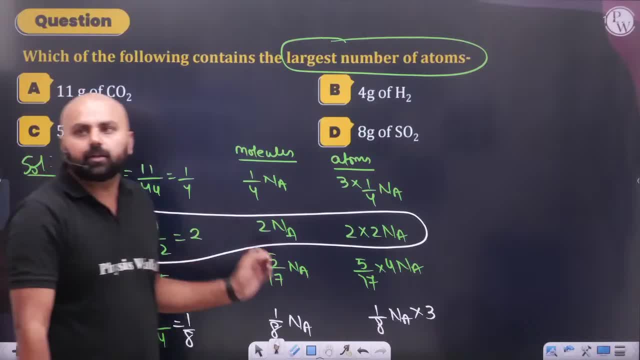 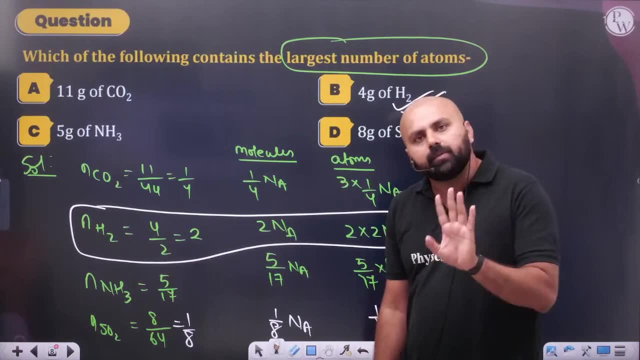 The one who has a big number of atoms- Brother, you don't have to do entire calculation- The one who has the big number of atoms To Hydrogen? So the answer would be Hydrogen. So, brother, look at this. 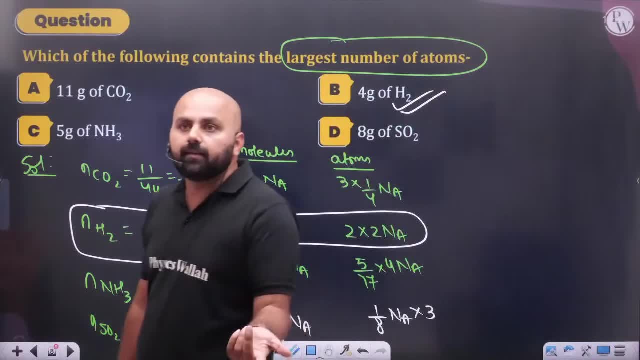 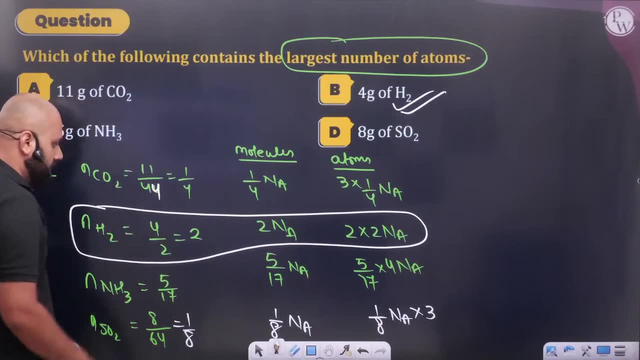 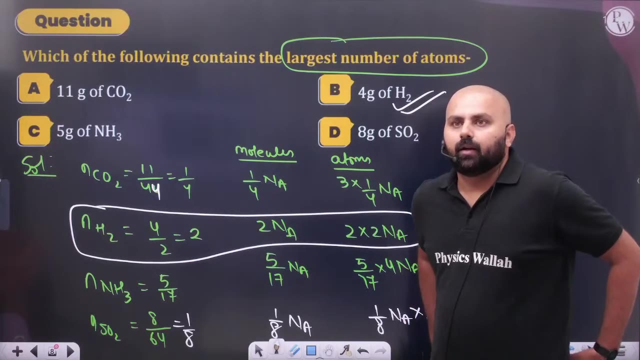 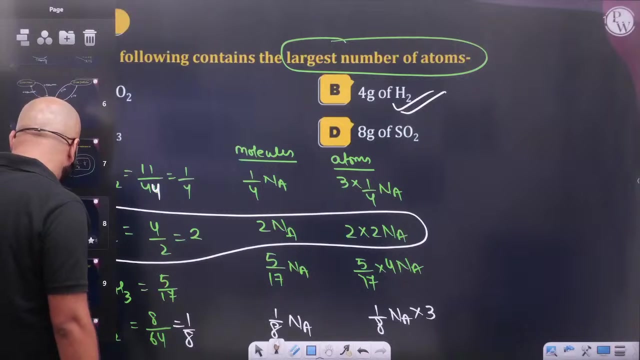 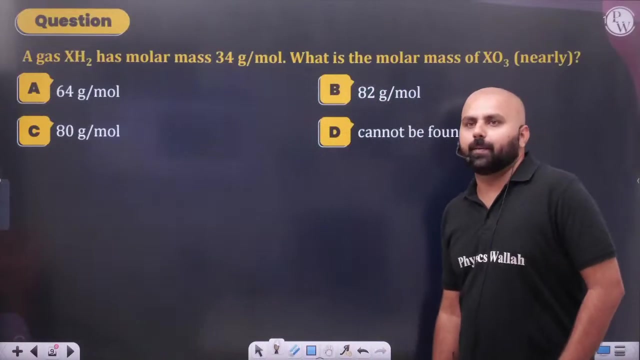 In exam hall, this question will come. the question of atoms, molecules, volume. This is the question to ask here. One is asking: how did you take upon 44? The mass of CO2 is a marathon brother. okay, upon 40, the number of atoms? first take out the molecules, then take out the atoms, multiply by molecularity for atoms. it will happen. come on, look at the next, look at the next. now, someone said that, sir, if you want to ask some such easy type questions, if you want to ask me a simple, a small question, see this, see how good the question is, see what the question is, see what the question is. 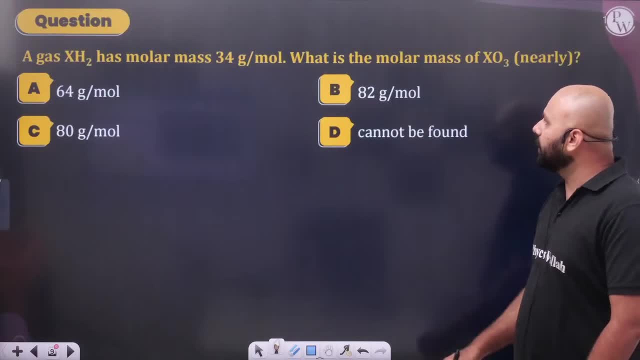 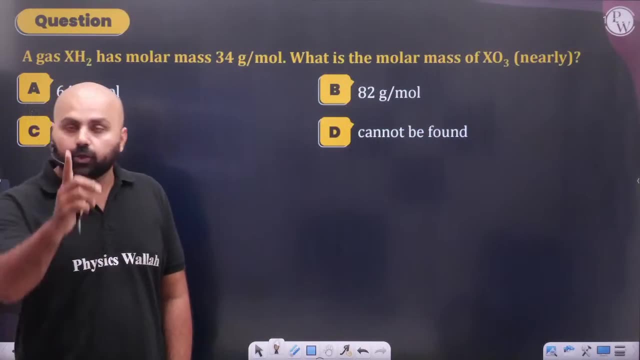 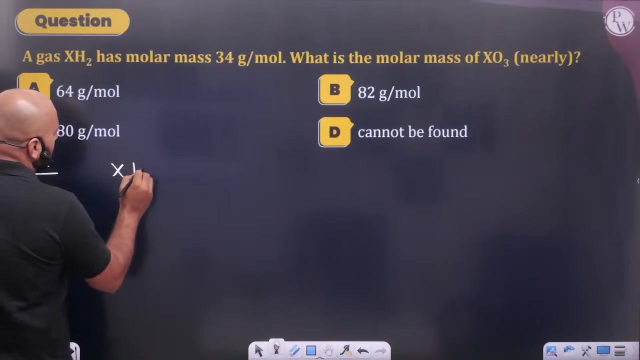 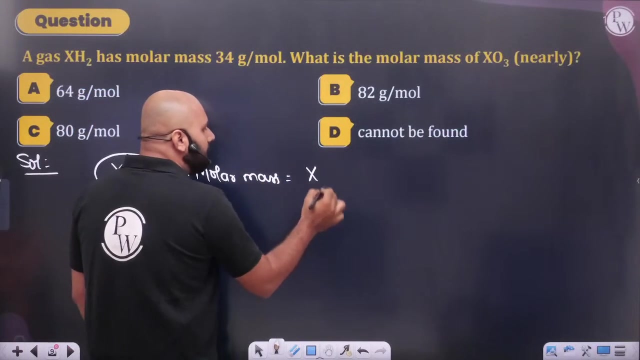 tell me fast: gas XH2 has molar mass 34 gram. what is the molar mass of XO3,? I don't know which is gas, what is X, but if you look at the question it will be solved easily. those who want to do it, do it quickly. attempt, sir. what is he saying? there is a gas mass of XH2, XH2's molar mass. what will be its molar mass? what will be its molar mass, sir? don't know the mass of X. how much is hydrogen, 1, 2 hydrogen and what is its value? 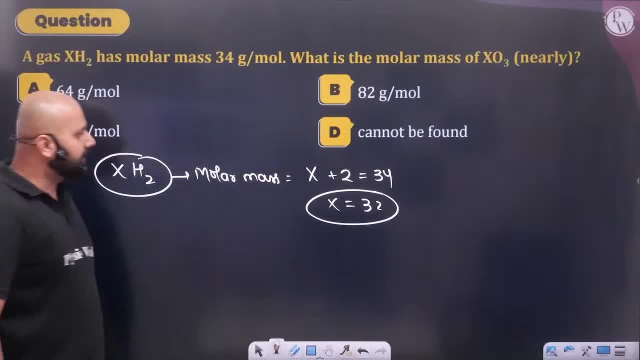 so what is X's mass? How much is the molar mass of X 32.. How much is the molar mass of X 32.. Sir XO3, How much is the molar mass of XO3?? How much will it be? 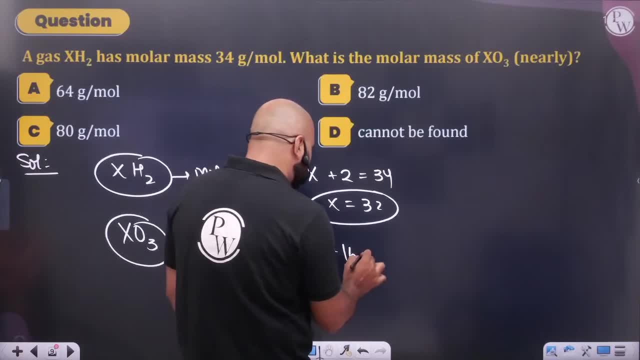 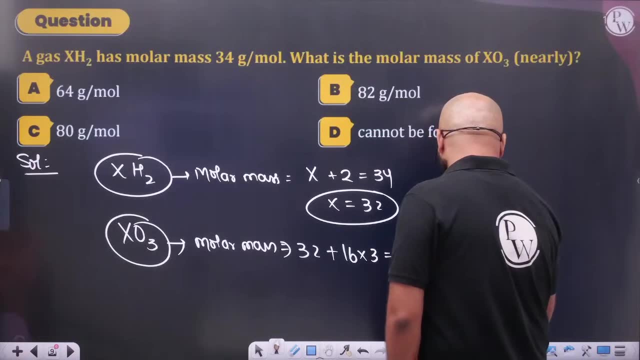 How much is the molar mass? 32.. How much is the mass of oxygen? 16 x 3? How much will it be 32 plus 48? How much will it be 80 grams? See what will be the answer. 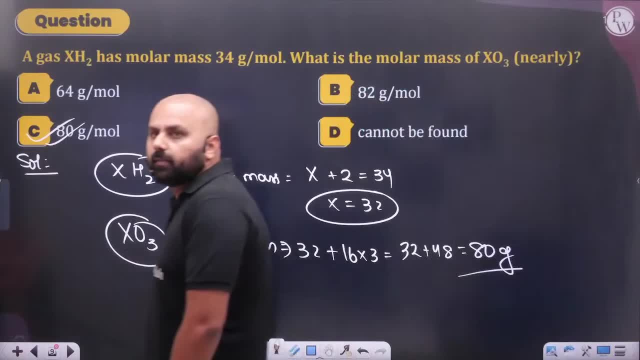 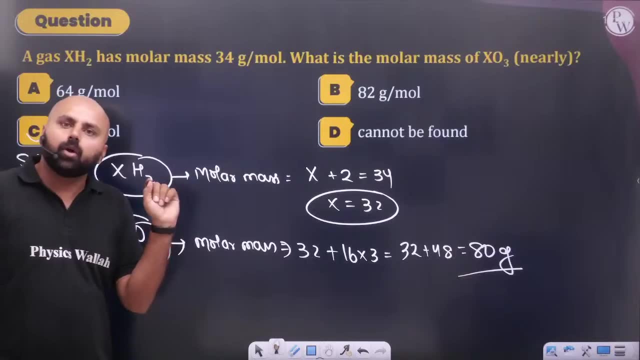 Third answer will come. It is a simple thing. Third answer will come. What did you know from the first one, Sir? how much is the mass of X 32.. After this, see, There will be so many easy questions in the exam hall. 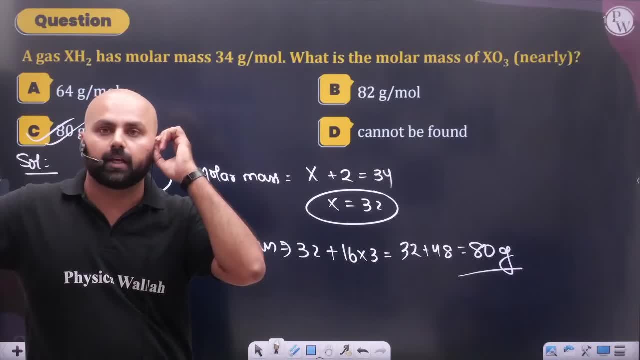 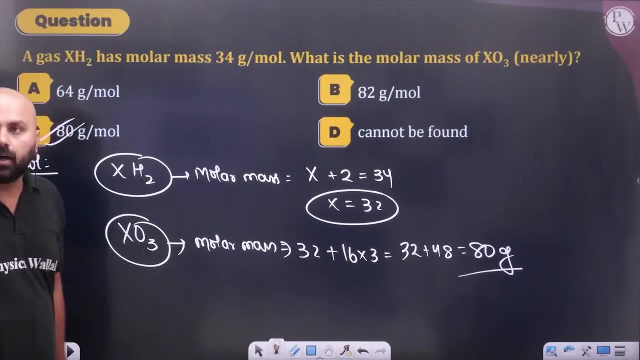 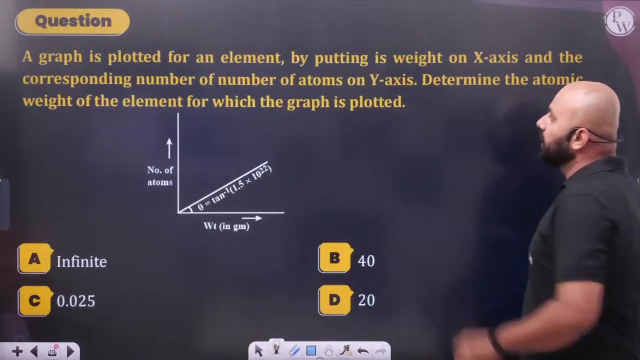 If you have not practiced, then the other person may feel that he has gone. See the same thing here. See the next question. Even better than that, The next question: Those who have practiced. there is no problem for them, Sir. I came to know that. 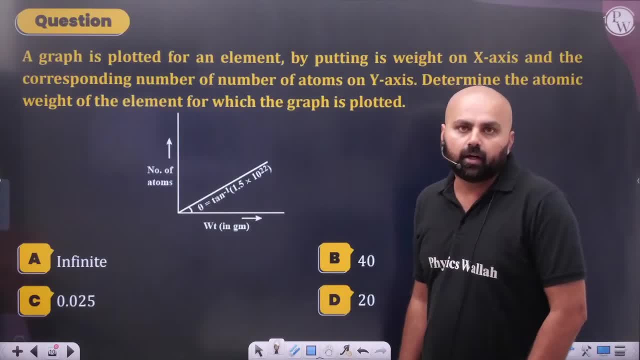 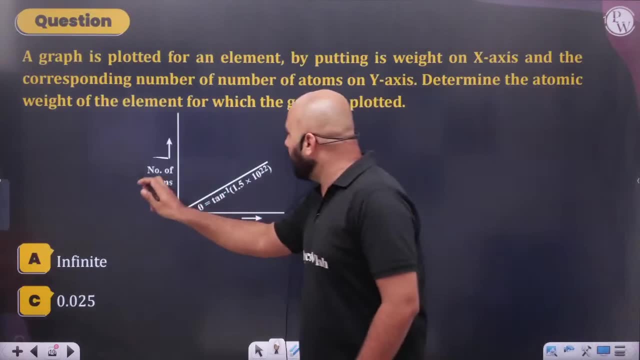 the question of graph came in the mole concept. Sir, the question of graph was given in the mole concept. Now you say that it comes in chemical kinetics. It comes in graph. So how will we do the graph? See this: The graph of number of atoms and mass is being made. 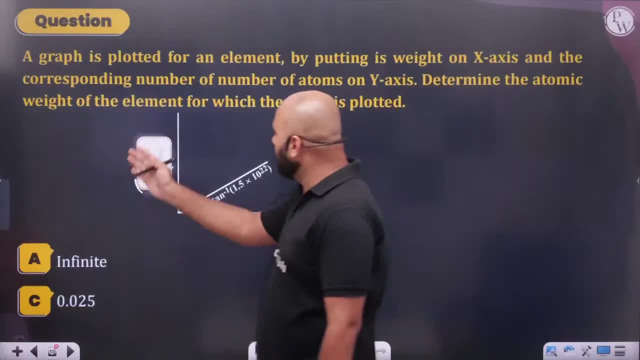 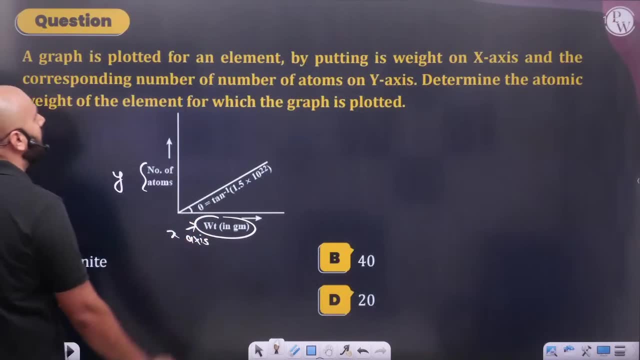 Its tan theta is given. How much tan theta is given, Sir? what is this on the y-axis? This is the number of atoms on the y-axis. What is this? It is the mass on the x-axis. Will you tell? Now, you will tell. 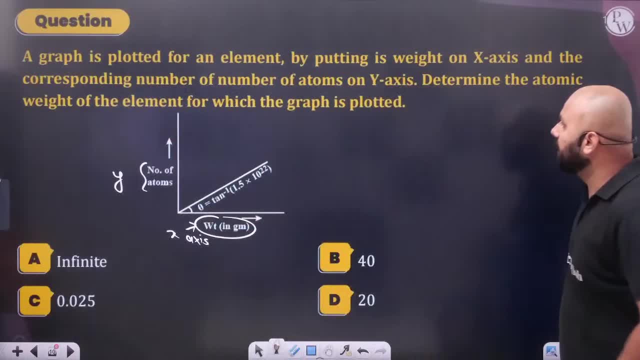 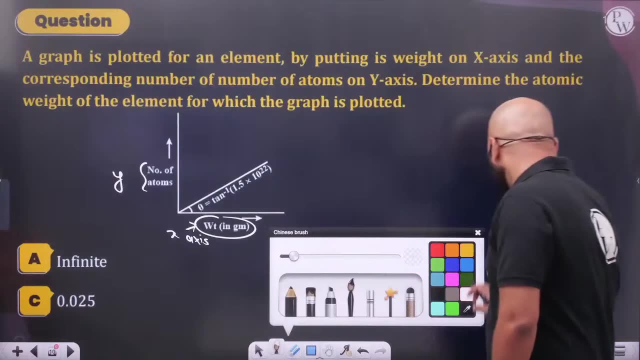 The graph of any element has been made. Determine the atomic mass of the element. Determine the atomic mass of the element. How will we find out? How will we find out? How will we find out? It is a simple story. Tell me one thing. 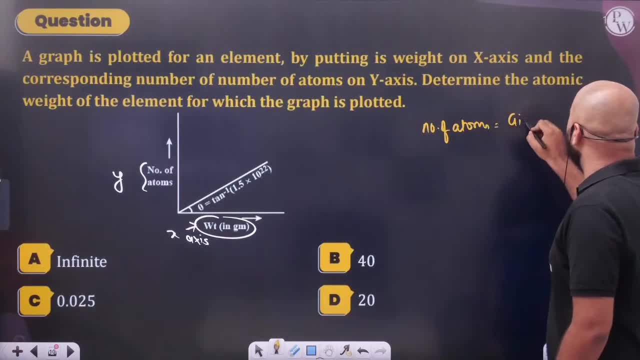 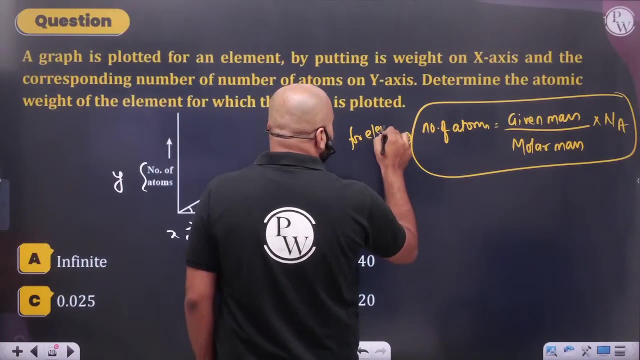 How do we find out the number of atoms? How do we find out the number of atoms, Given mass divided by molar mass? given mass divided by molar mass into Avgadro, number For elements, if we talk about elements For elements, if we take out here: 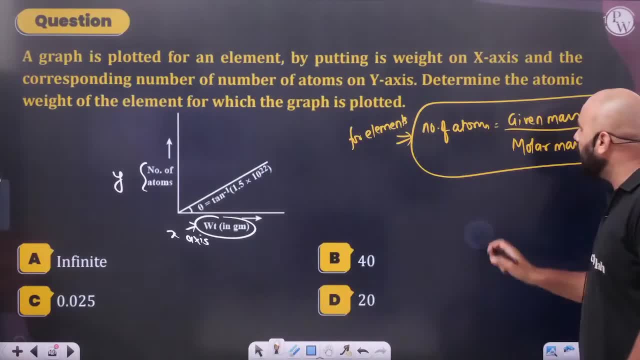 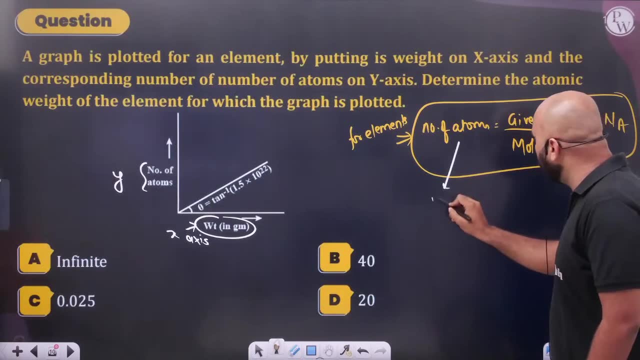 If we talk about elements, then it will come here. For elements, number of atoms is nothing. Given mass upon molar mass into Avgadro number. Sir, where is this On the y-axis? What is this On the y-axis? 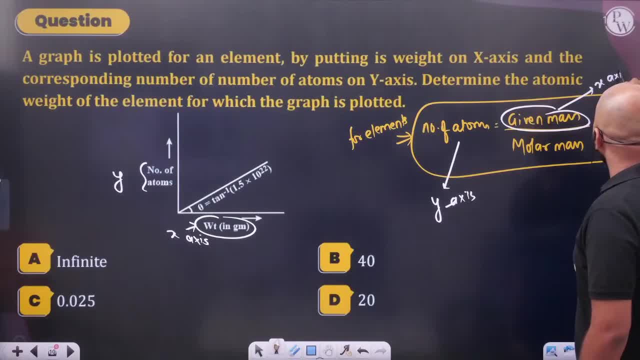 What is the given mass On the x-axis? So y is equal to mx plus mx's graph. How much will be the slope? See the value of the slope. Avgadro number upon molar mass. Avgadro number upon molar mass. 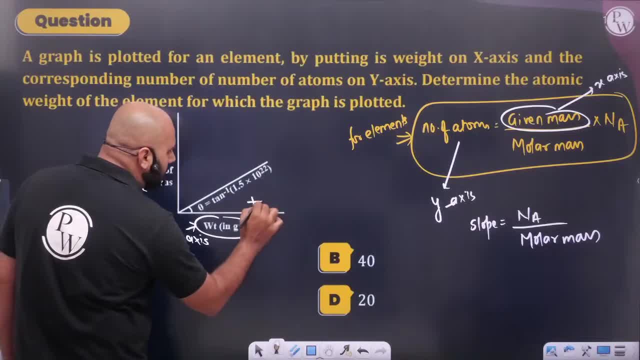 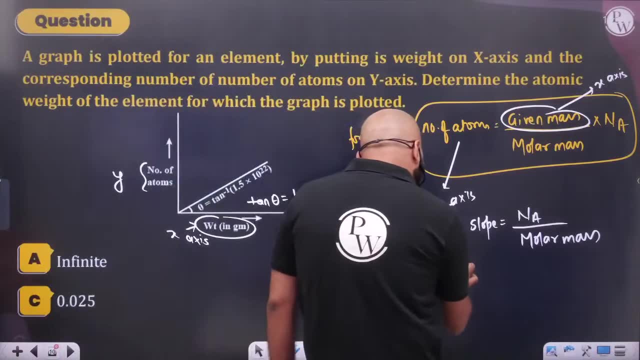 Here we can see the slope. What is the value of tan theta? What is the value of tan theta 1.5 into 10 to the power 22.. You can see the value of the slope. Put it, The answer will come. 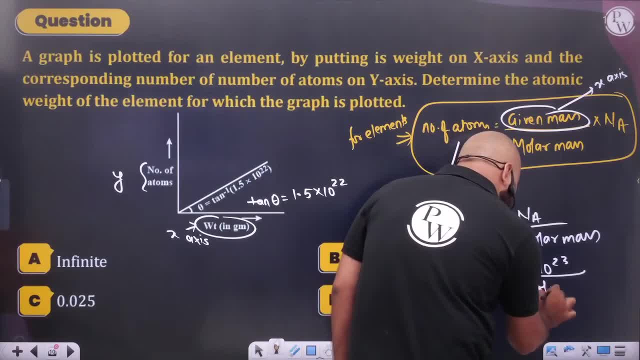 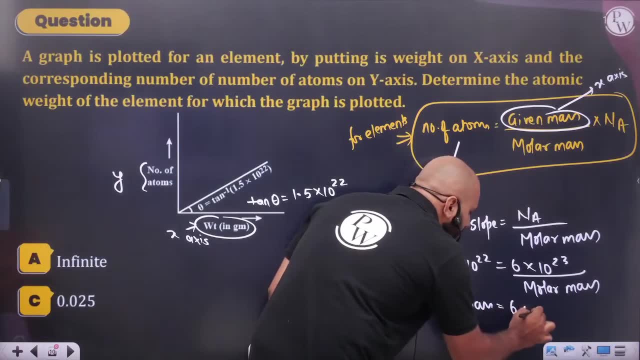 10 to the power 23 upon molar mass. So how much is the molar mass, Sir, if you take out molar mass 6 into 10 to the power 23.. Upon 1.5 into 10 to the power 22.. 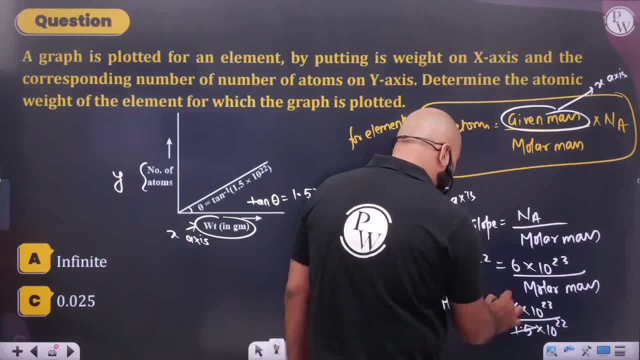 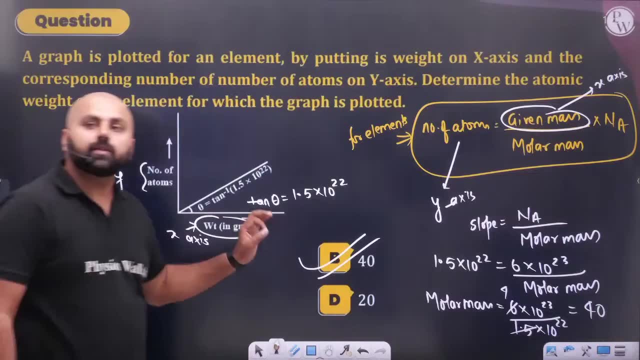 Upon 1.5 into 10 to the power 22.. So this is 4 times 10 to the power 40. What is the molar mass 40. You can easily attempt such questions in exam hall If you have seen it before. 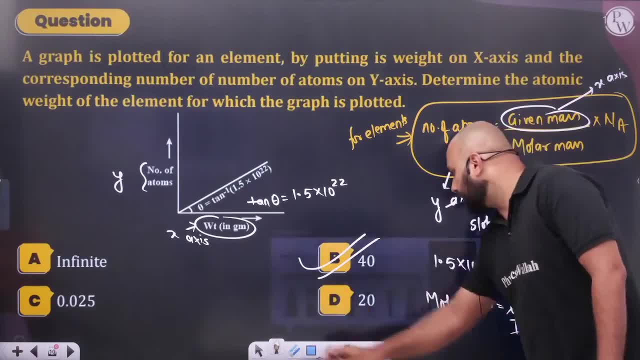 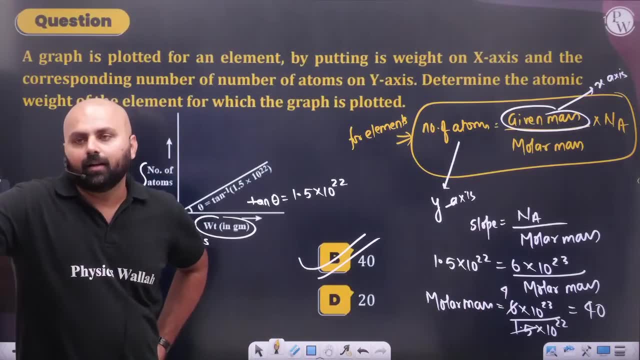 If not, then you can sit and chat, Keep commenting, Keep commenting next year also, Okay. Okay, See you very soon So you can check such questions. You can say this for elements: What will be there in elements If someone says, sir compound? 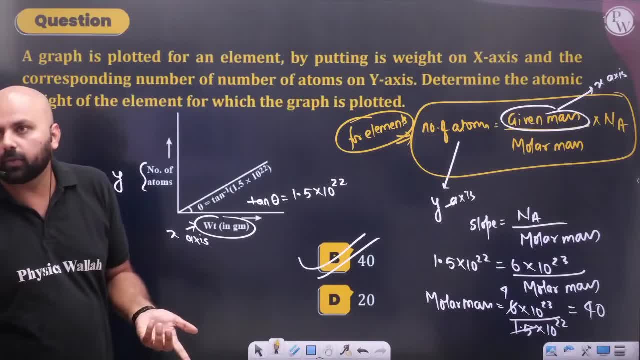 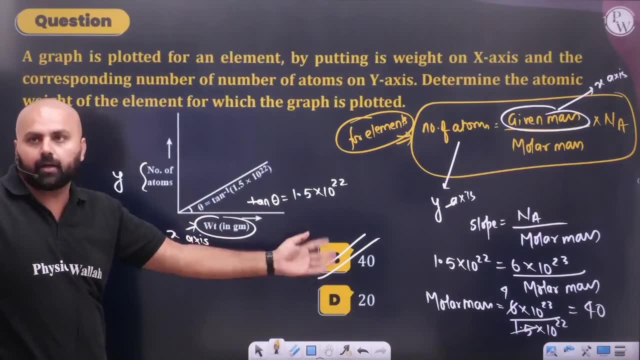 EM is written here. Why do I use Q here? If the EM is written here, then there will be no problem in that. This is the first time one has seen this question. Think like this. Such an easy question will come in the exam hall. 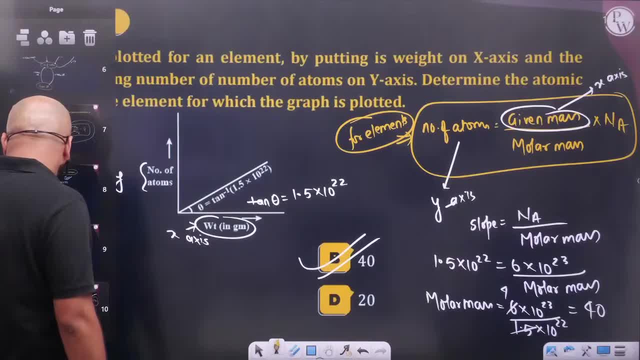 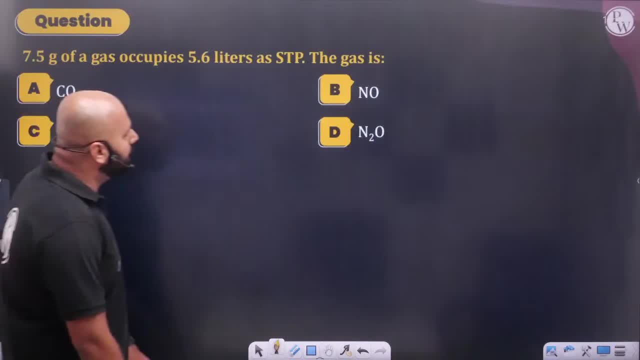 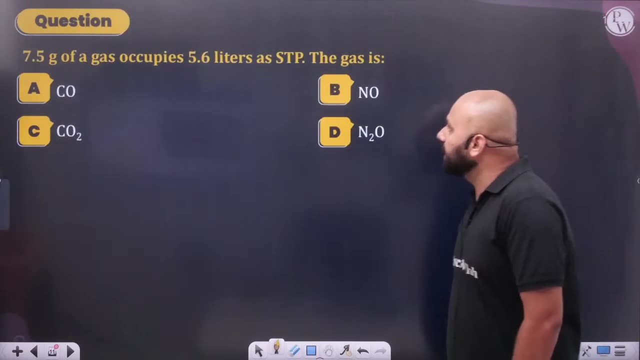 It is better to come to the exam and try this, after looking out and find the solution. Okay, Like this question is given. see, this question is given: 7.5 grams of gas, occupies 5.6 liters of STP. Sir, how much volume of 5.6 liters of STP is given 7.5 grams? 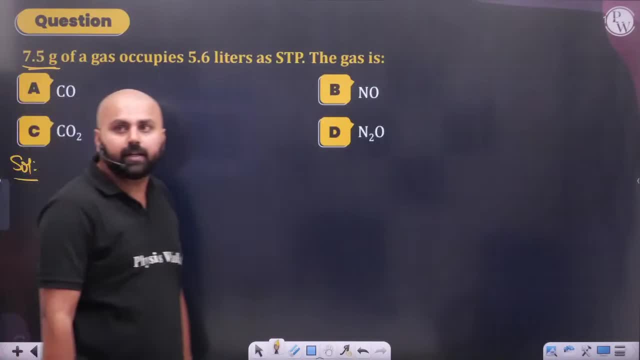 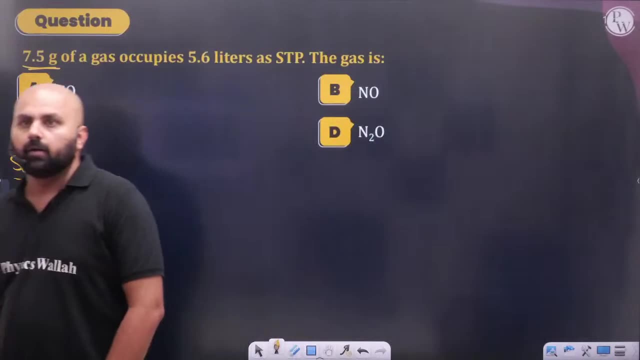 Will you tell me which gas is this, Which gas is this, Which gas is this? Which gas will be there? What will happen? Which gas will be there, Sir? how much is the mass of 5.6 liters? 7.5 grams? 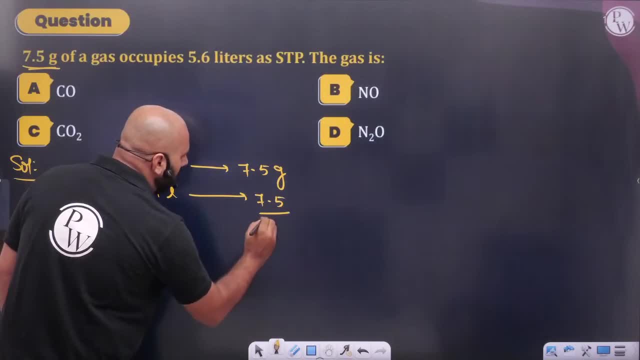 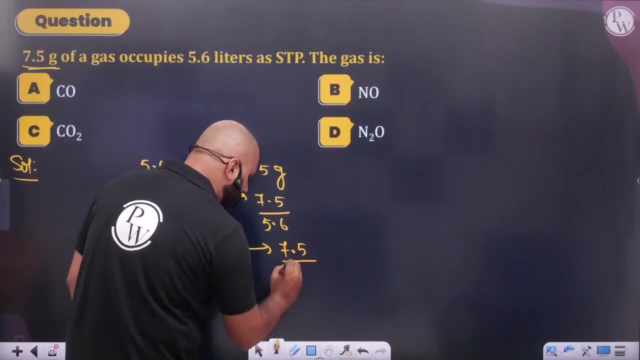 So how much will be the mass of 1 liter 7.5 upon 5.6.. So how much will be the mass of 22.4 liters 7.5 upon 5.6 into 22.4 liters? 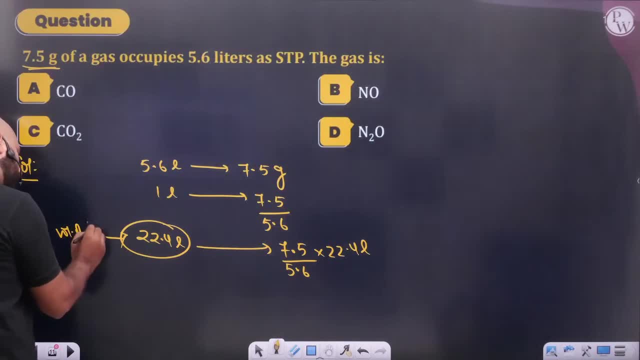 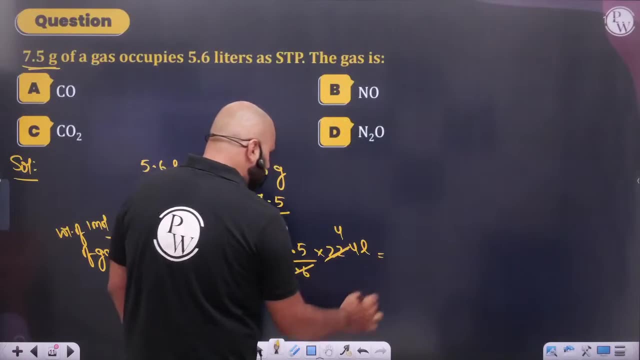 This is the volume of 1 mole right? This is the volume of 1 mole. This is the volume of 1 mole of gas. If you solve this, then how much will be this 4.. And how much will be this 30 grams? 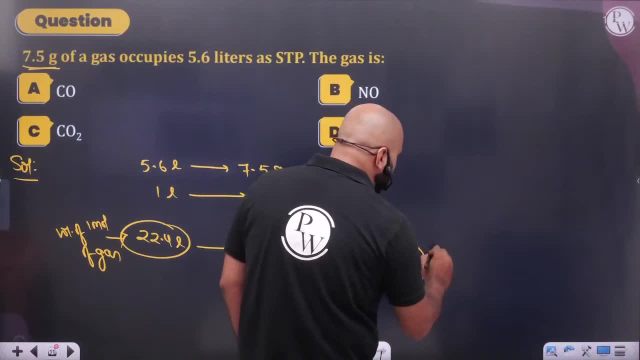 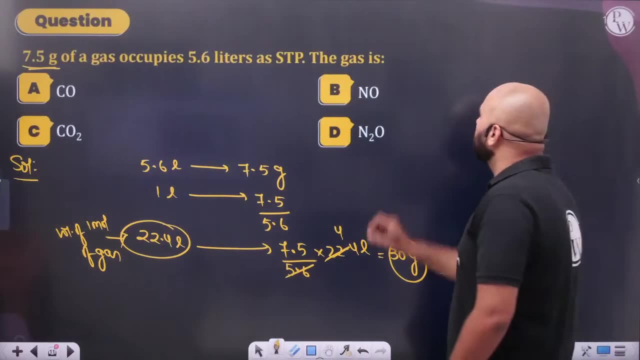 How much will be this? 30 grams. 30 grams, What is this? This is the molar mass. See which gas has the molar mass of 30 grams. Which gas has the molar mass of 30 grams. 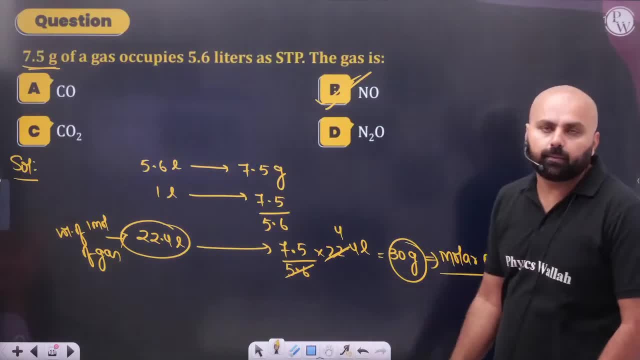 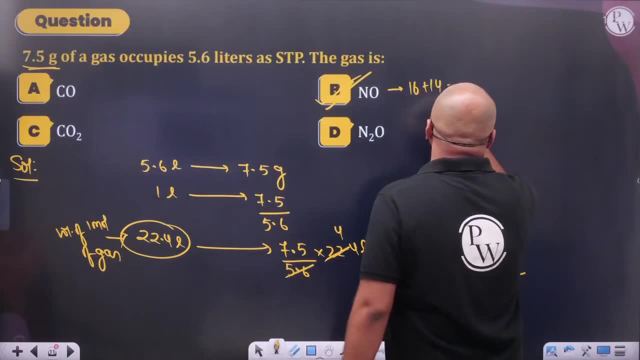 As far as I can see. how much is its molar mass? 30 grams. Why, Sir, calculate the molar mass and see how much it will be, Sir, 16 plus 14,, how much is the molar mass? 30.. 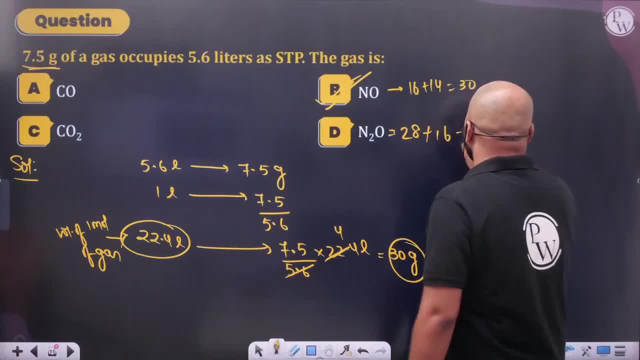 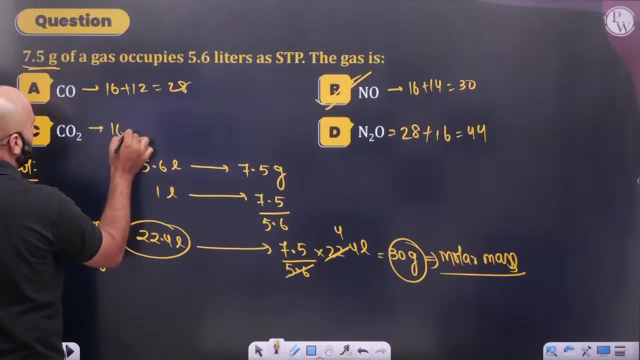 If you see here, then 28 plus 16, 44. If you see here, then how much is it 16 plus 12, 28.. And if you see here, then 12 plus 32,, how much is it 44.? 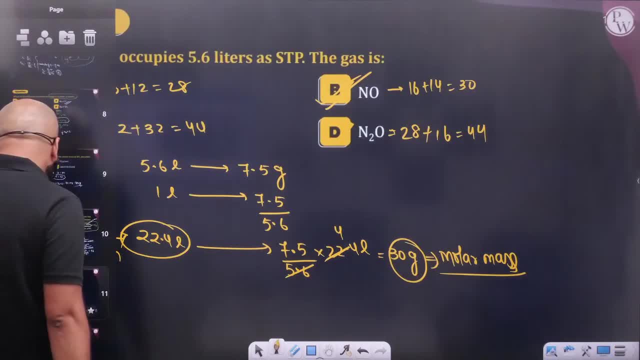 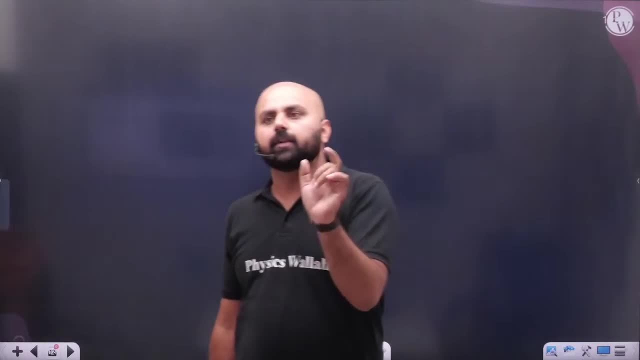 Will you get the answer? Sure, Now we have come to the base questions on these small formulas. We have come to the base questions on these formulas. So the first main thing in the mole concept is that: from where does the mole concept come? 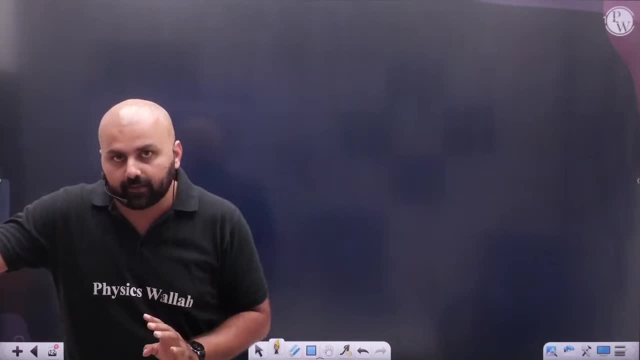 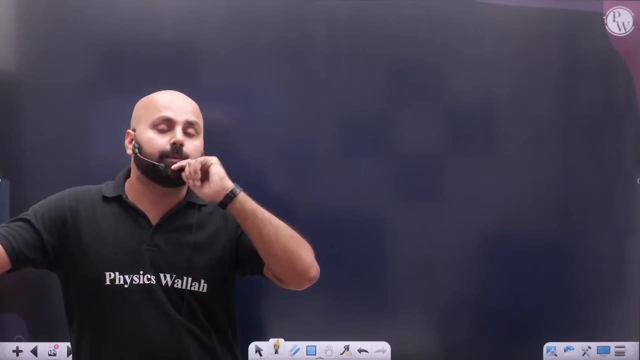 How, How, How are atoms, molecules, volume, related to all this? Second thing. Second thing: In the same chapter, there is one more important thing. This is one more important thing. Do you know, Like the people who have seen the paper? 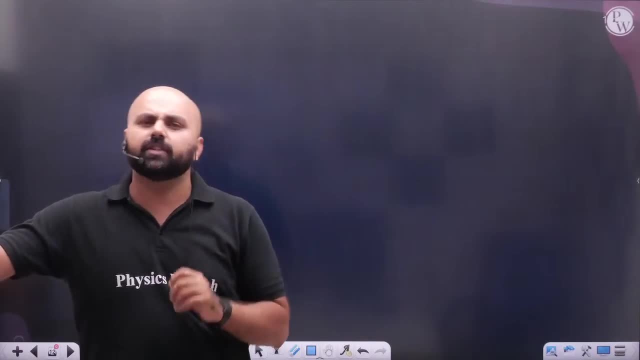 If you have seen the paper of last year, 2022, carefully, There is a small thing. This also comes in physics. This also comes in physics, Like in a paper of NEET 2022, which was done in September, Which was done in September. 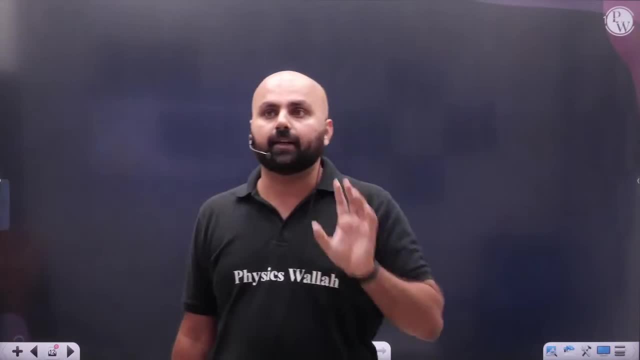 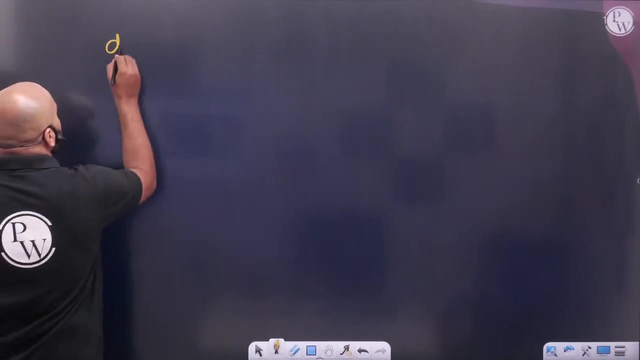 Not the paper of July. There was a paper in September which was done in 2-4 centers only. It was done in 2-4 centers only. Look at that question. You think It is simple than you. If I ask you: what is density? 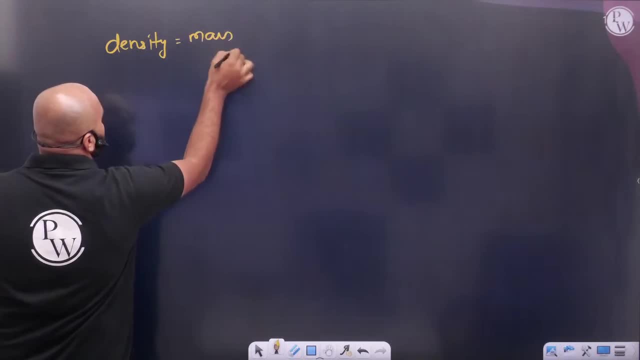 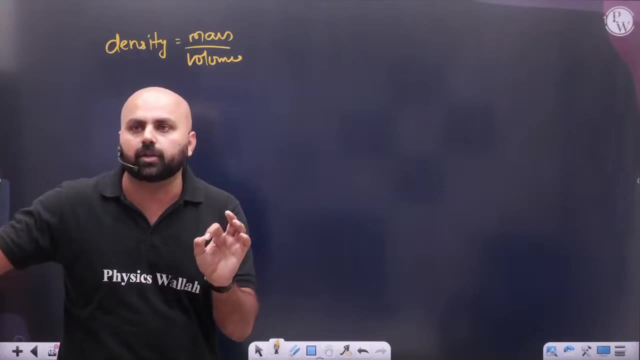 What is density? Then you will say: Sir, what is this? Sir, you are asking such an easy question. You say: mass upon volume. This is what you say. But, yes, The person in front of you asked the right question on this. 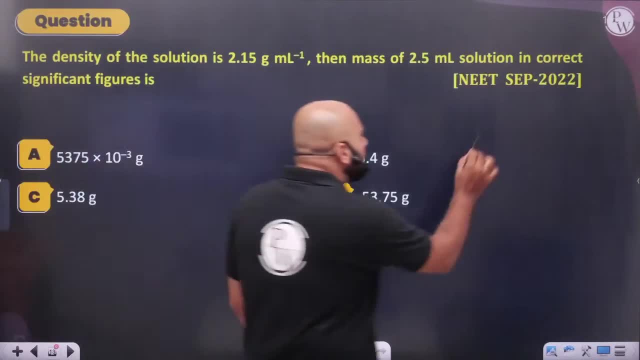 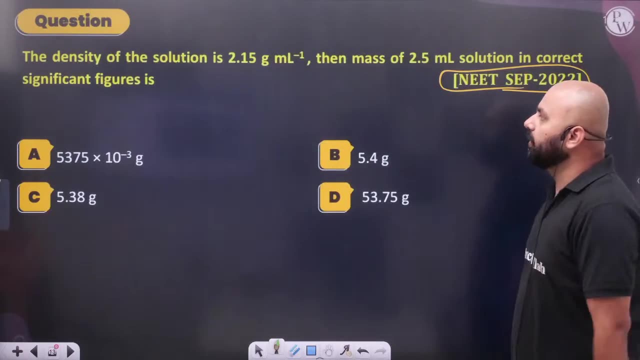 Look at this, Sir. look at this. Look at this question. This is the paper of September 2022.. NEET is a paper of September 2022.. Look at the question Attempt and see What is the question given. 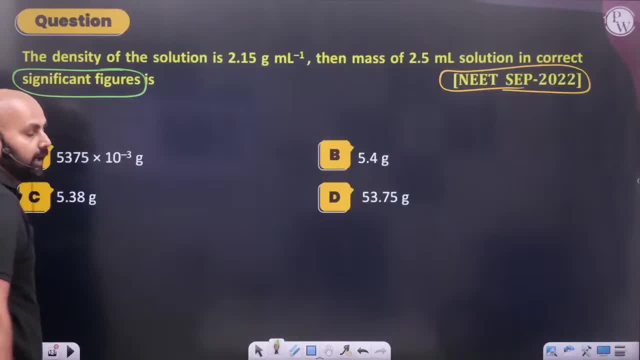 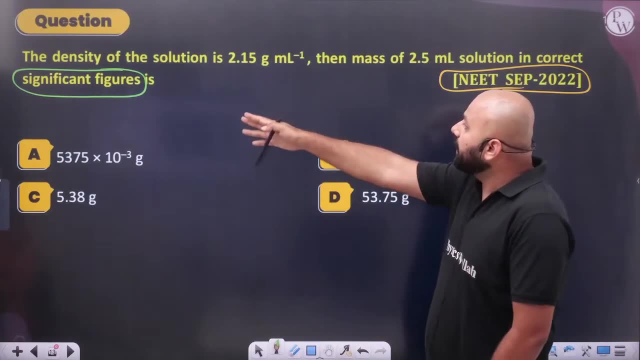 The question of significant figure is given in chemistry. Listen carefully: Significant figure. We leave such a basic thing. The question given on that is given by the chemistry. Ok, The question given in chemistry is this: What is given That density is given? 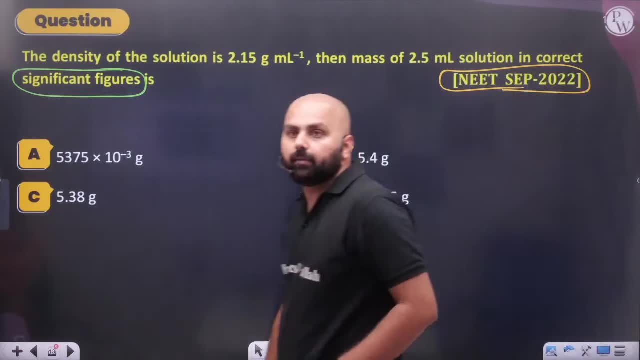 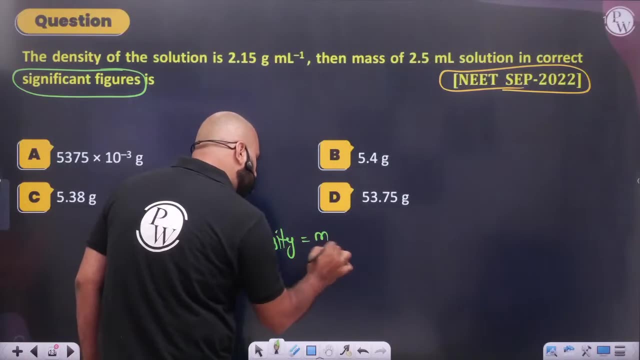 What? to extract Mass? to extract Whose 2.5 ml, Sir? here a simple rule is followed: That whenever you have density, Density is nothing Mass by volume. So if you have to extract mass, Then what will happen? 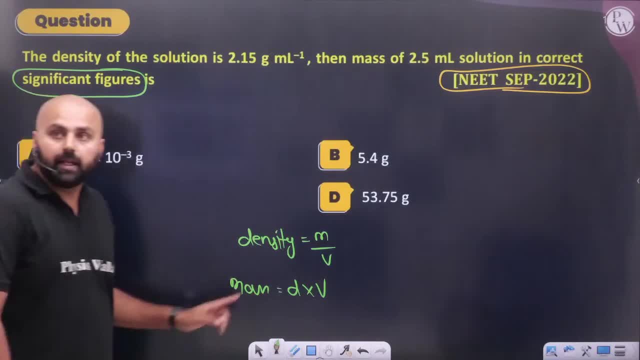 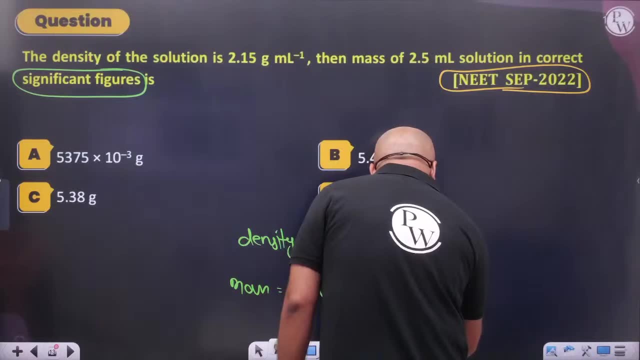 Density into volume, What will happen? Density into volume? But? But, Sir, here the problem is not that He is making you do the calculation. He is not trying to make you do the calculation, Brother, He knows what he is trying to make you do. 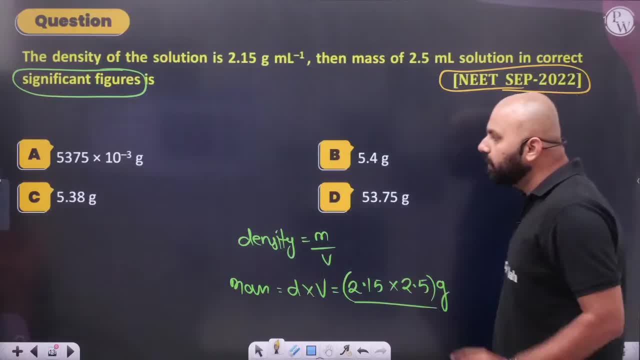 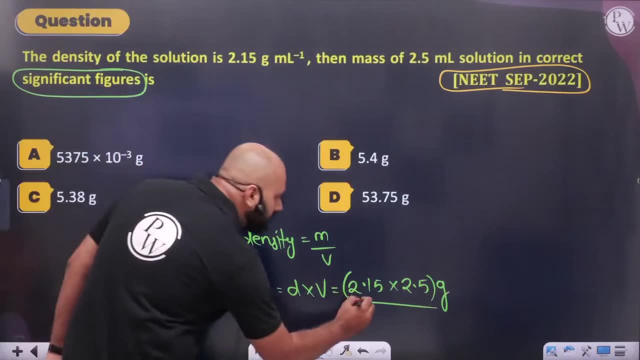 You don't read his calculation. You remember the basic rule of significant rules, The basic rule of significant figures, That if you multiply two people, Then inside you How many significant figures are there in it? There are three significant figures. How many significant figures are there in it? 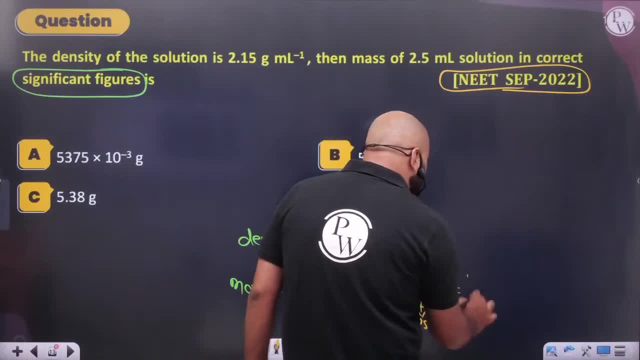 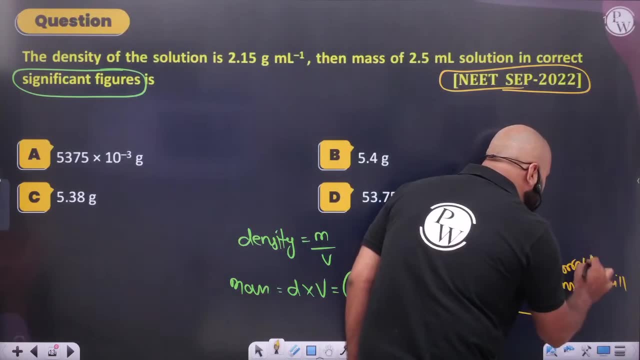 There are two significant figures, No need for multiplication. The answer that will happen, The answer to that Will have The correct answer. Will have The correct answer. Will have Only two significant figures, Sir One, How many will there be? 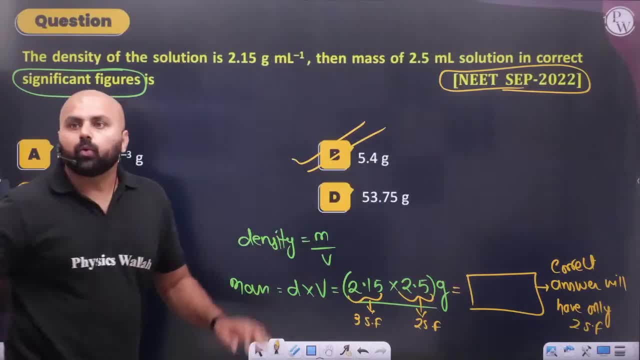 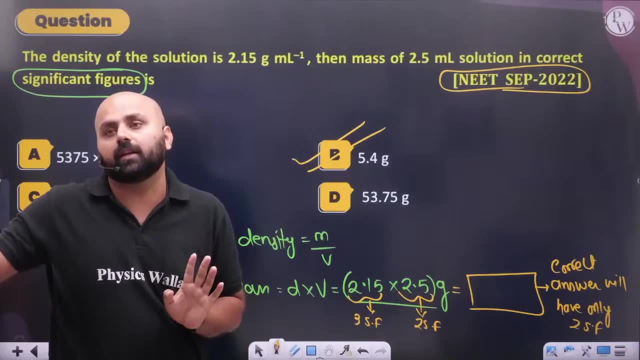 Two significant figures In the whole answer. Which one is there? No calculation, Nothing. When you go to NEET's exam hall, Use common sense, Don't work too hard, NEET is easy. because of that, Why will I multiply? 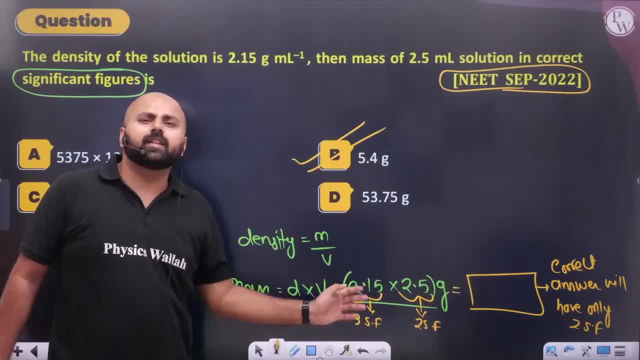 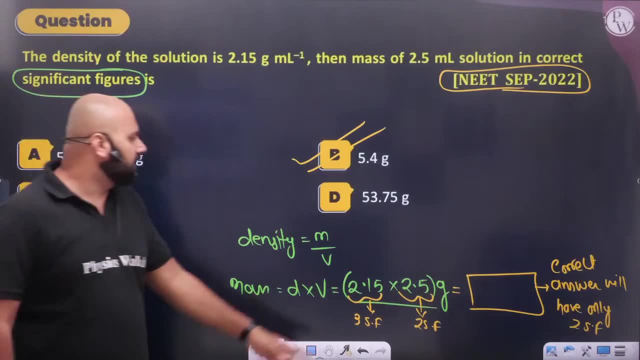 What is the benefit of doing it? Do it. If it is too much, Then do it. See, It will be around 5.375.. But I don't have to do it. The reason is, Sir, See the options. 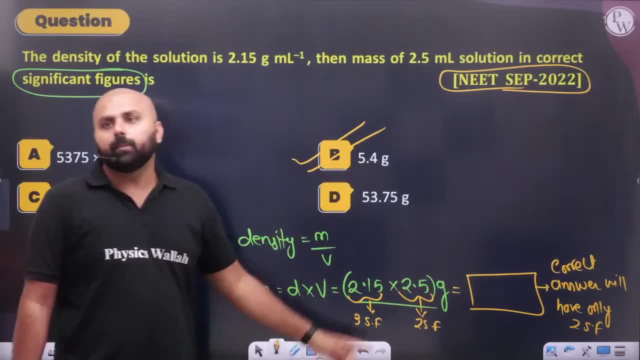 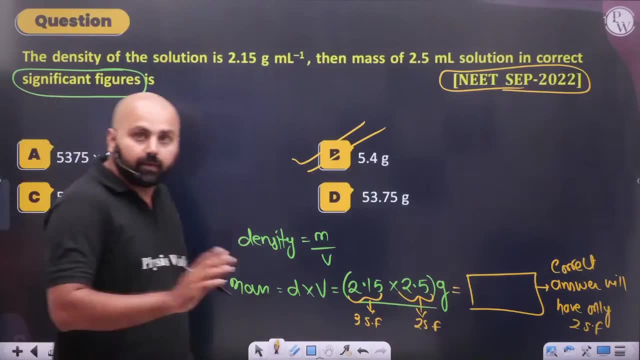 Inside this Four significant figures, Inside this Three, Inside this Four, Inside this Two? My answer will be two. Remember Whenever you do multiplication Of significant figures. Let me tell you a basic rule. You are studying in physics. 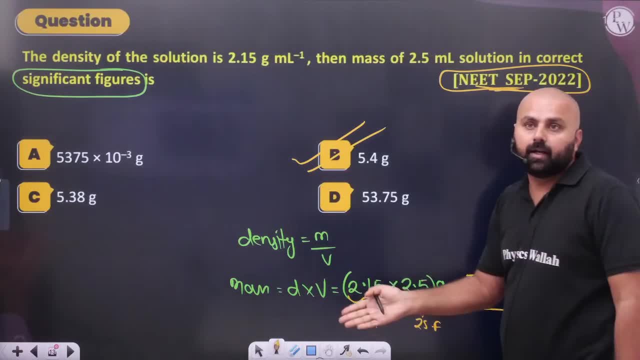 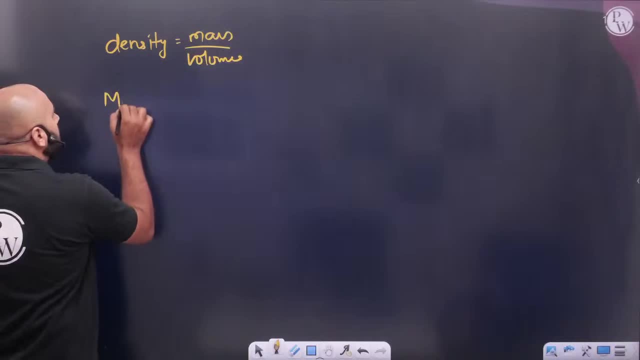 I am repeating it here too: Reason That, brother. There is no trust. This is a side exam. This year, only This year. only Listen carefully What I said. When multiplication or division happens. When multiplication or division happens. If multiplication or division happens. 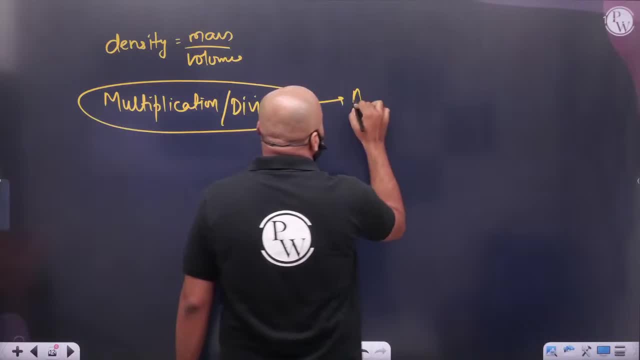 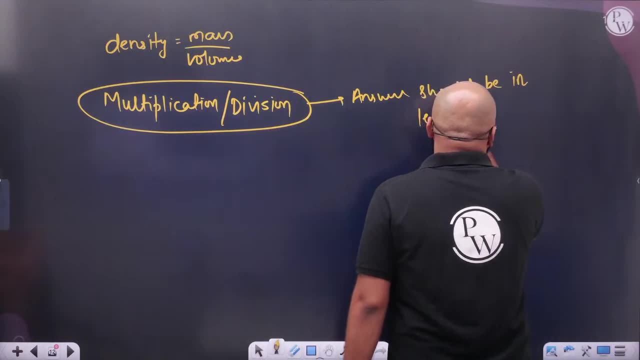 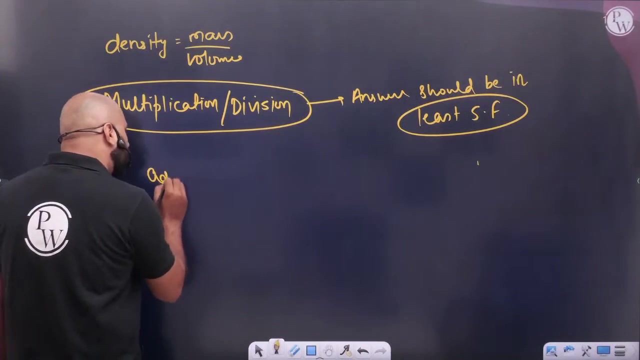 Multiplication or division happens, Answer always happens, in which Answer should be In least decimal, Sir. I am saying least Least significant figure, Significant figure. Try to keep it in the least significant figure. But If addition and subtraction happens, 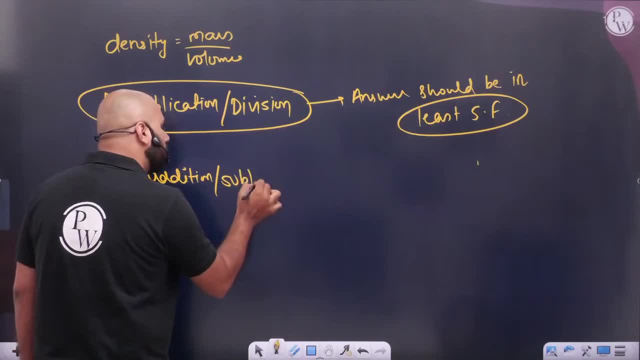 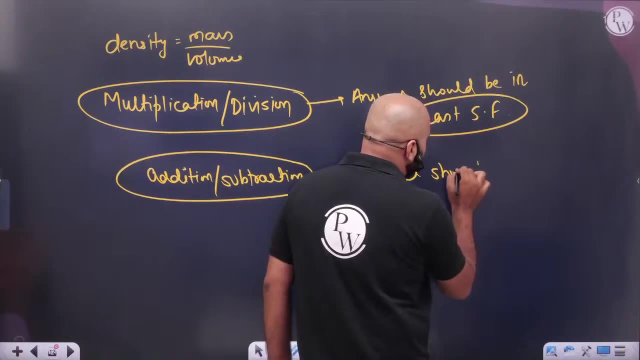 If you do addition and subtraction, Then, brother, Remember, While doing addition and subtraction, That what should be the answer, always Answer should be. Answer should be: Now you must have done in physics, In least decimal place. That is why I am repeating it. 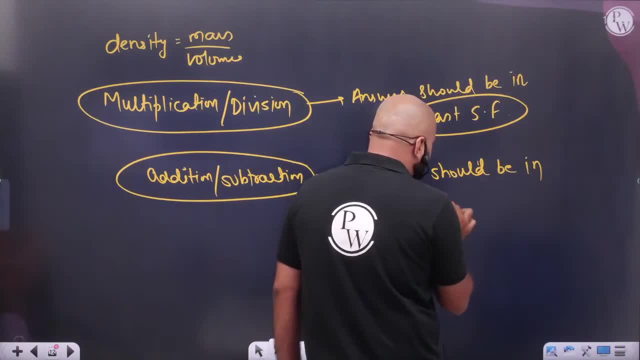 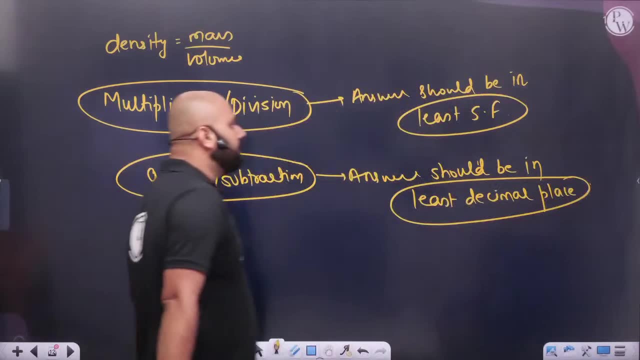 Because, brother, This question In chemistry This year NEET In 2022.. They gave it In September Exam That brother You give this question. So, brother, Significant figure. Work is going on. Minimum significant figure. 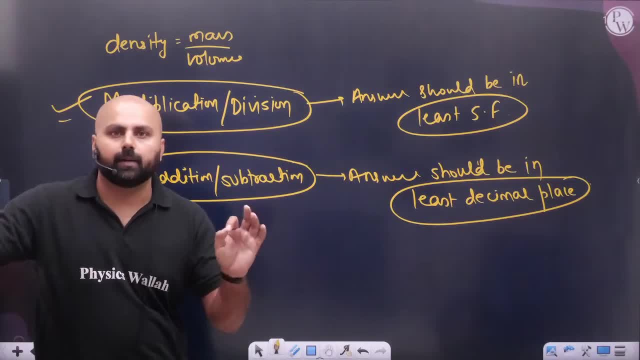 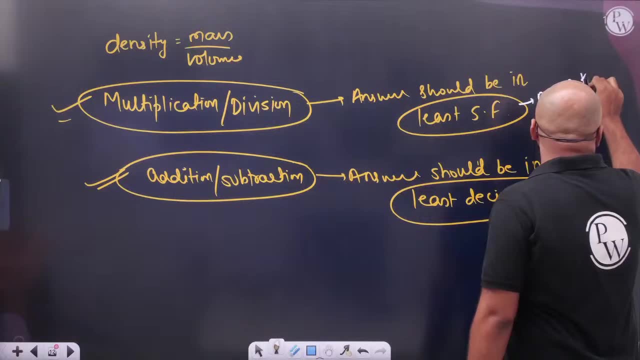 Minimum Least significant figure Means The one Who Who Significant figure Means In between. Out of the given. Out of the given. Not that, Sir, I gave it in one. Out of the given Given. 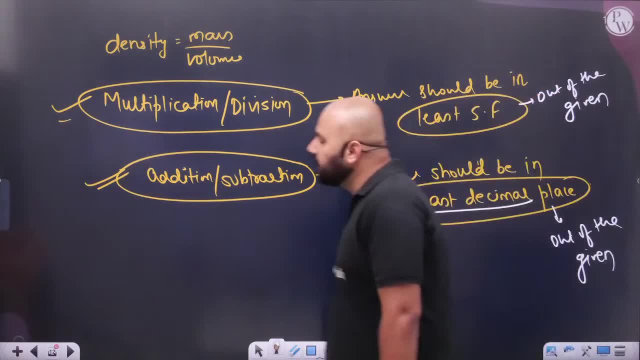 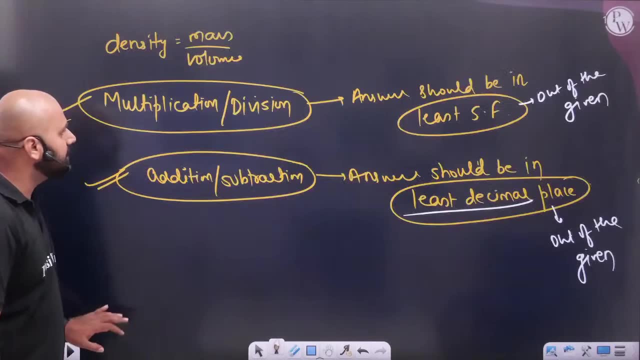 The people who have given. I am saying from that only Least decimal place. You have to take care In addition and subtraction And what happens in this, Okay, It will happen. Okay, Sir, See this With you. I was saying that. 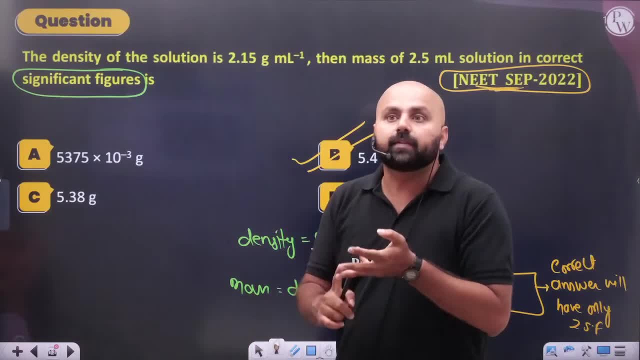 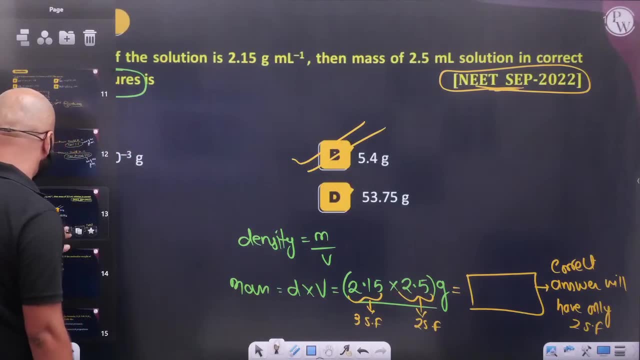 The basic thing is being asked: What, Sir, On you Significant figure? Look at the basic concept: Yes. After that, Who told me? One is saying, Sir, Let's talk about common sense, Sir, Common sense also gives the answer. 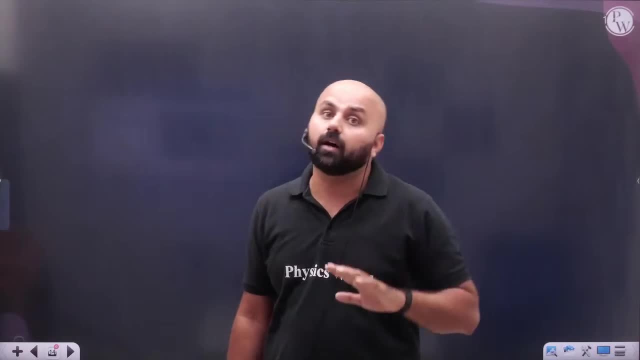 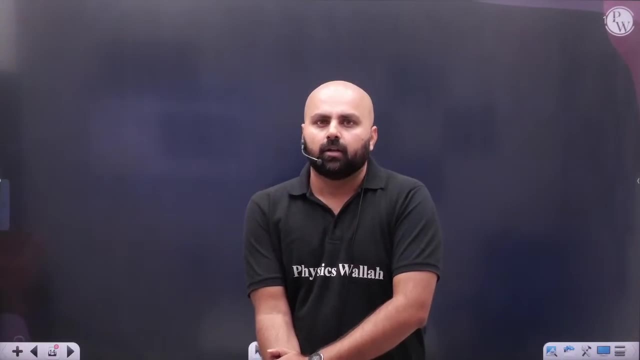 You know When you are sitting in the exam hall. Now, Sitting here and commenting, Sitting here and reading. It is a different story Here. What time is it now? Half an hour has passed In this exam hall, If half an hour passes. 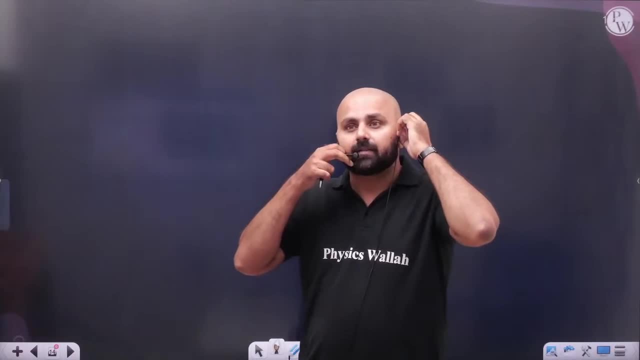 Son, Then it will be known, You will remember Coming on 7th, Remember With you, Remember Exam hall, Different condition Sitting here. There is no option to comment. You can't even say That this question paper is different. 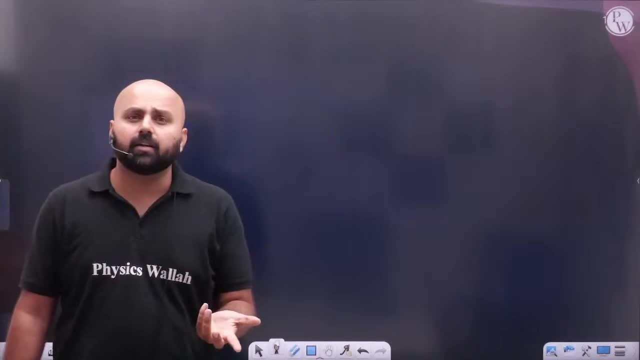 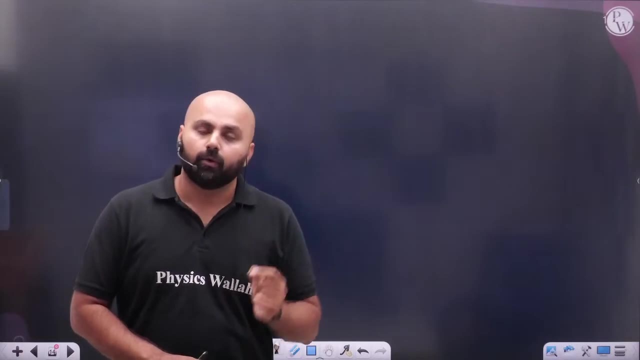 Brother. Okay, Study quietly. Reason That there is still an option to speak here On 7th May 2020.. The person who will be silent from the exam hall- He will remain silent even after coming out- And the one who will come out of the exam hall. 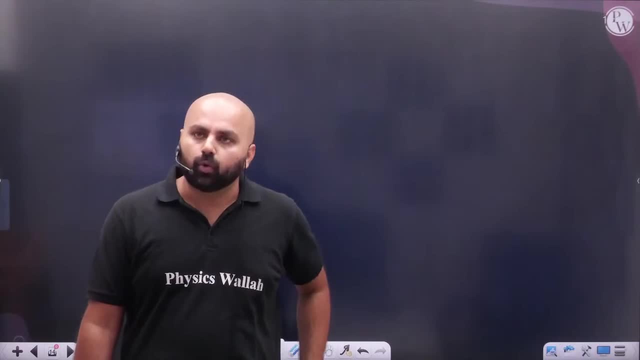 He will come out and keep blowing. Okay, Yes, NEET 2022.. It happened twice, Once in July And once in September. Two, three, four places were at the center. That's why I gave his question Okay. 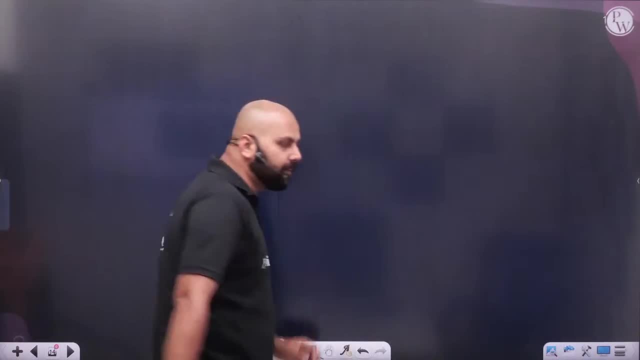 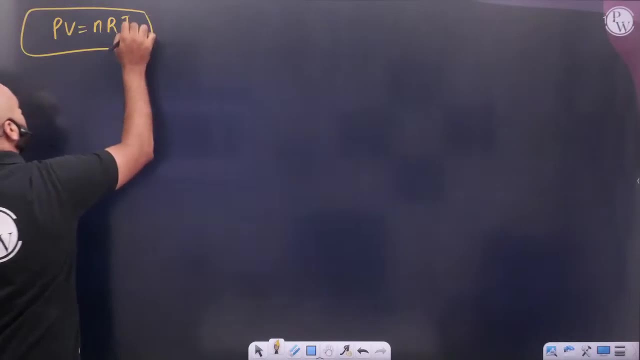 Come on Now look, Sir. What else do you have? What else do you have? So remember, There is another concept in the basic concept And that is equal to PVNRT. Brother, Listen, Because it will repeat again in the states of matter. 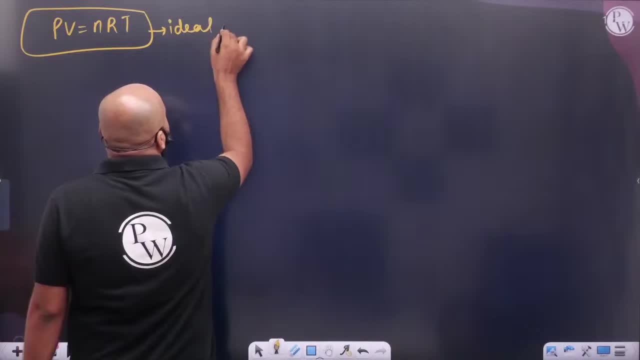 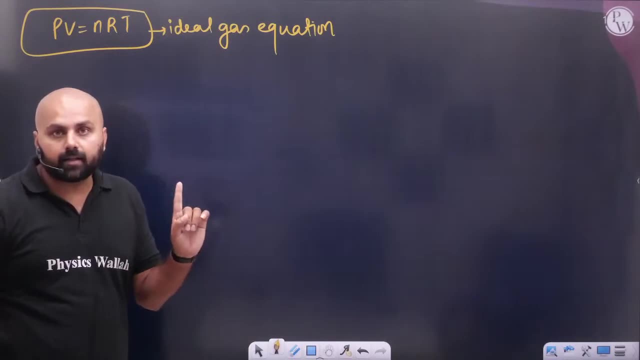 We will read it again there, But there I will focus on its graph. Now I am trying to read it, Remember, Remember. You have- There is no problem with pressure volume here- The R. that happens, Brother, Everyone. revise The value of R. 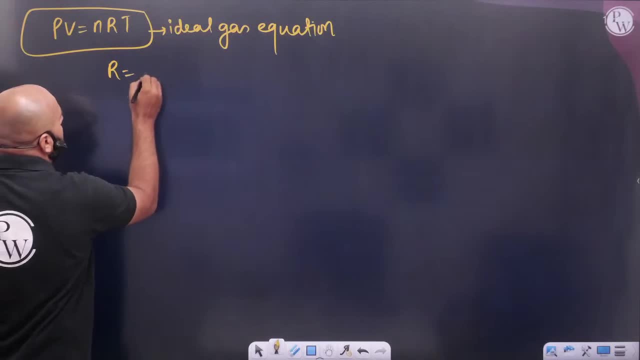 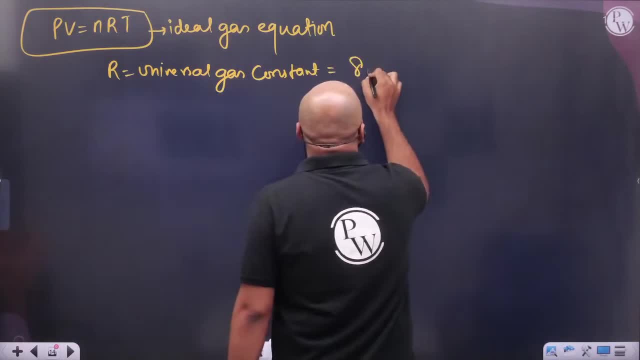 Universal gas constant. But what is the problem? It has two or three values: Joules per Kelvin per mole. It must be written like this: Remember, Apply it only then. Apply it only when, When the pressure is in Newton per meter square. 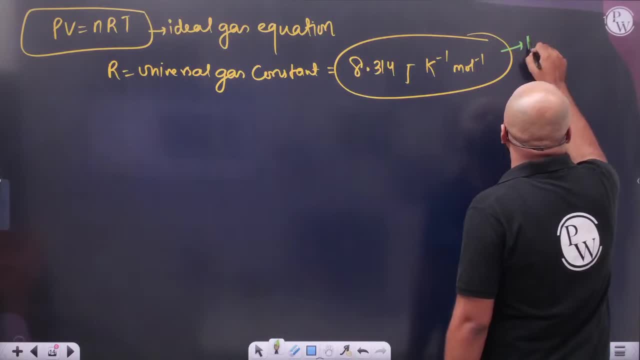 Or when the pressure is in Pascal, And And When the volume is in the meter cube. It is very rare in chemistry. It is very rare in chemistry, Brother. Okay, It is very rare that you get to use this one in chemistry. 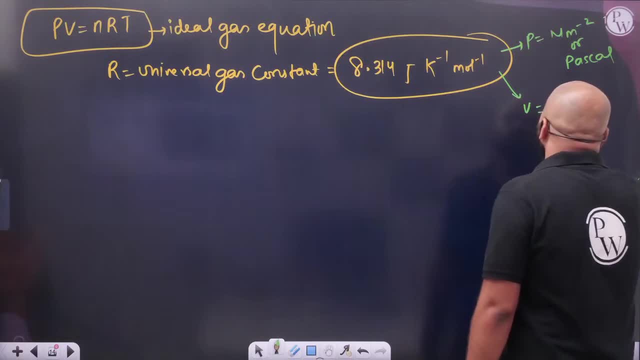 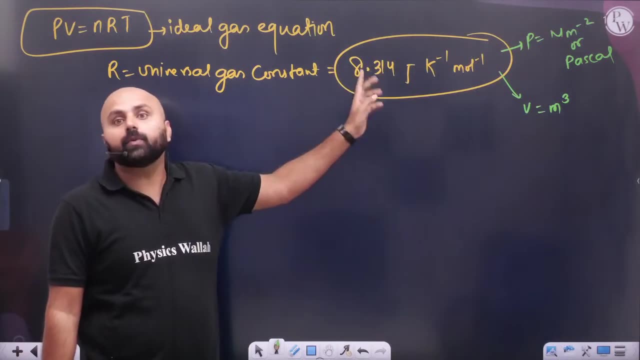 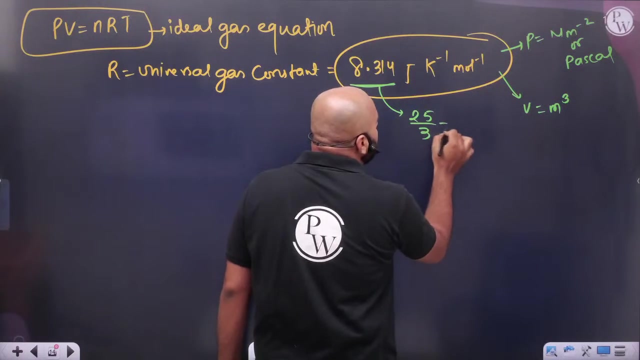 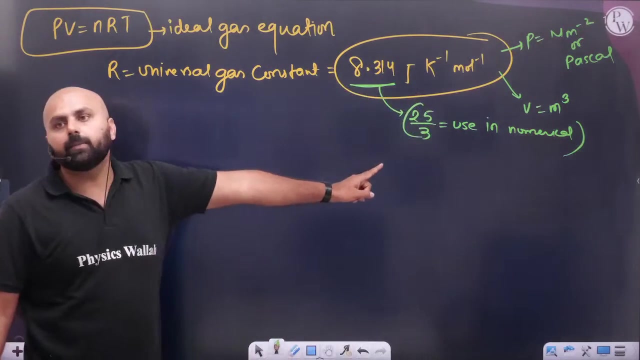 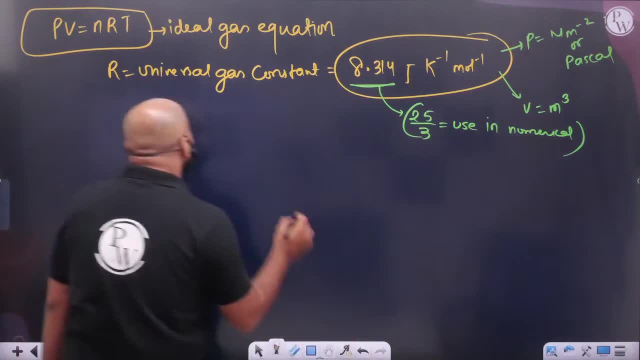 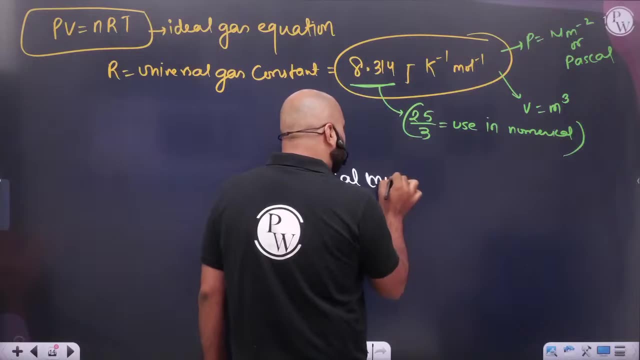 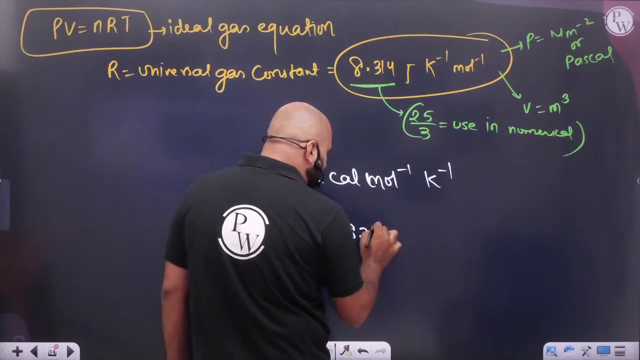 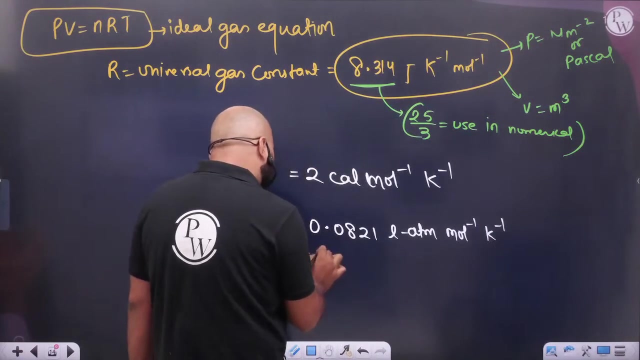 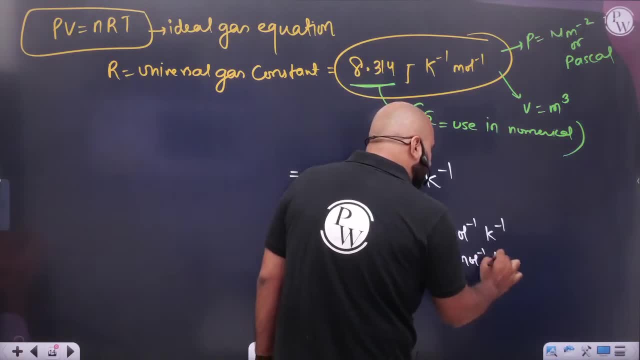 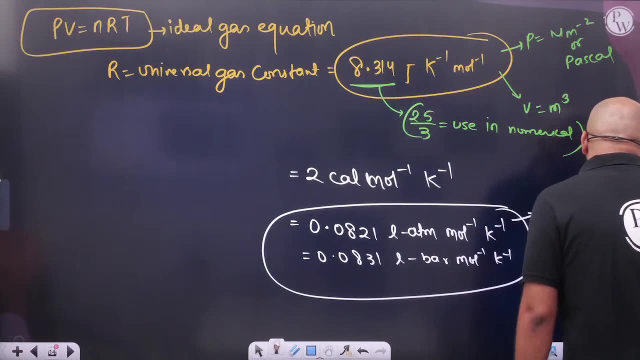 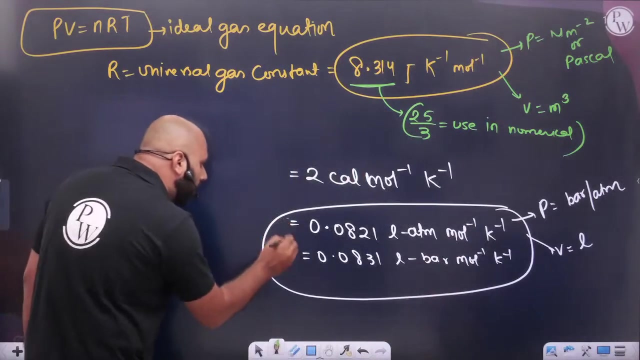 liter bar per mole per kelvin. I am writing these two together. When to use this? When the pressure is in the bar, whether the pressure is in the atm and the volume is in the liter. Look carefully, brother, because this is the most difficult to use the unit and if you want to take these two together, then 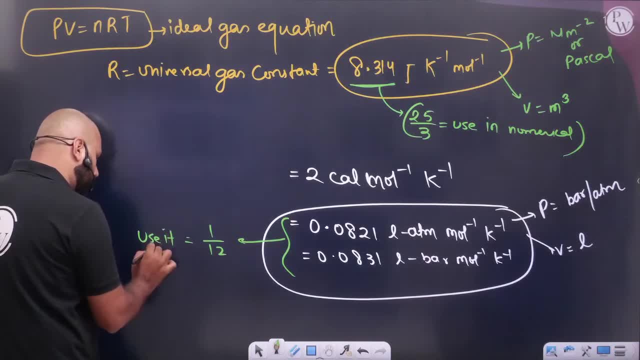 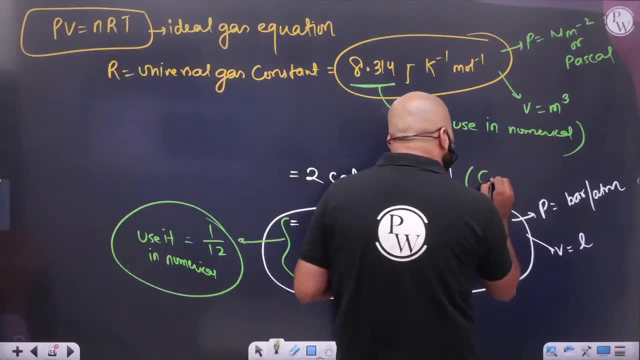 do 1 by 12, use it in numerical. Whenever you have to solve numerical, then you can take its value 1 by 12.. When will this come? This will come when you have a CGS unit. when you have a CGS unit, when the pressure is given in the arg. 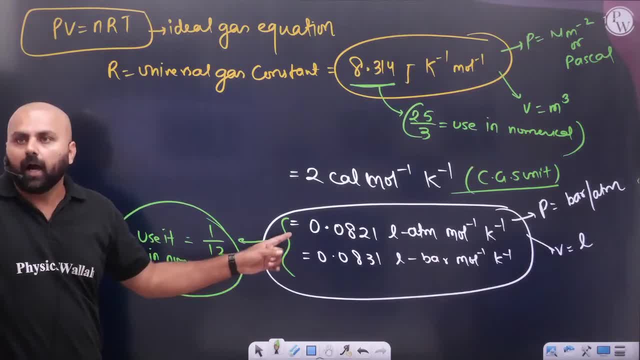 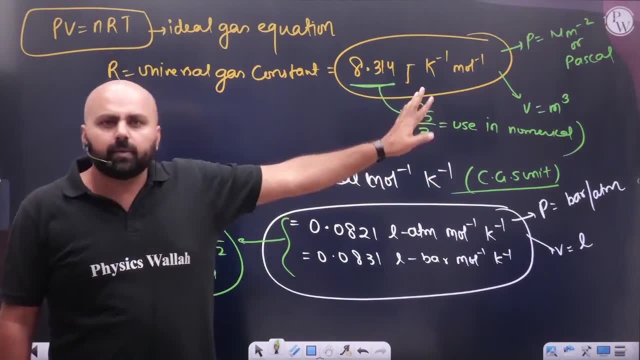 for that. then, brother, see this with you: what will be the value of R? what will be the value of R? see this, take 8.314. when the pressure is very rare, chemistry is very rare. Oh, brother, this will be given in the chemistry. this will not get this in chemistry until and unless it is on thermodynamics. 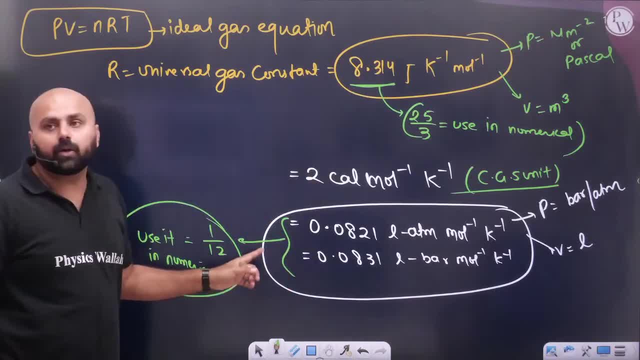 then you don't have to use 8.31 for. but yes, if you will get it to use this one, keep doing it, keep doing 1 by 12, keep doing 1 by 12, keep doing 1 by 12 and keep doing it. it will be done. So use this 1 by 12 in numerical. What is the rest? pressure? What is the number of moles? 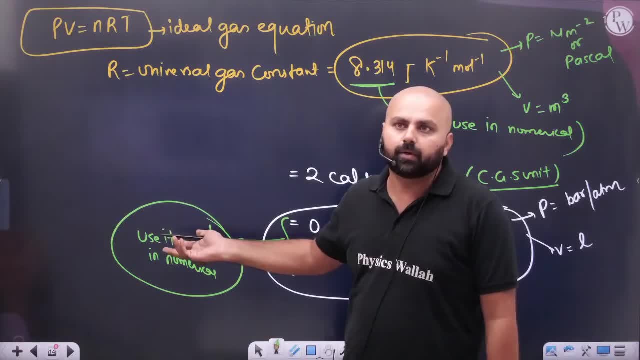 What is R? We always put the temperature in Kelvin. do this to yourself. Okay, We put the temperature in Kelvin. Put it Okay. now someone says 2 calories, brother 1.99,. brother 2 is 4K. brother 2 is 4K. 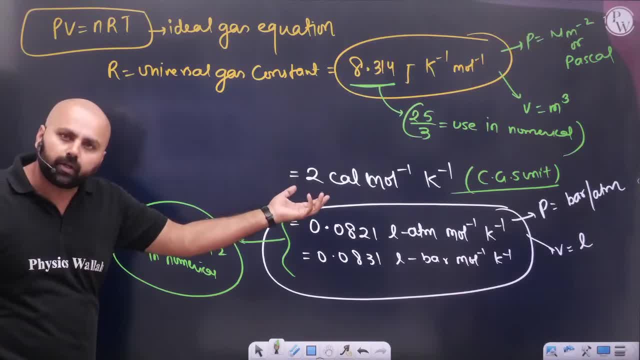 Brother 2 is 4K, Brother 2 is 5.. brother 2 is 5K, Brother 2 is 6K, Brother 2 is 6K, brother 2 is 6K. round off, the use of 2 in chemistry will not come soon, except thermodynamics. 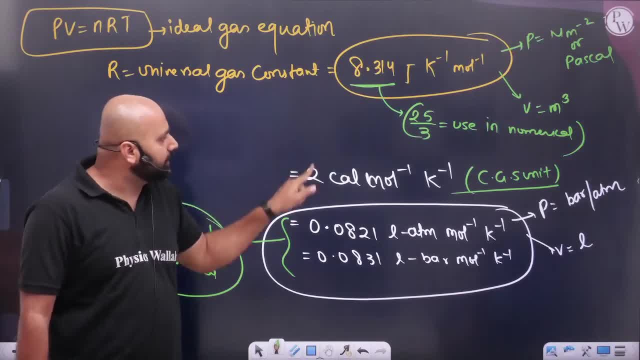 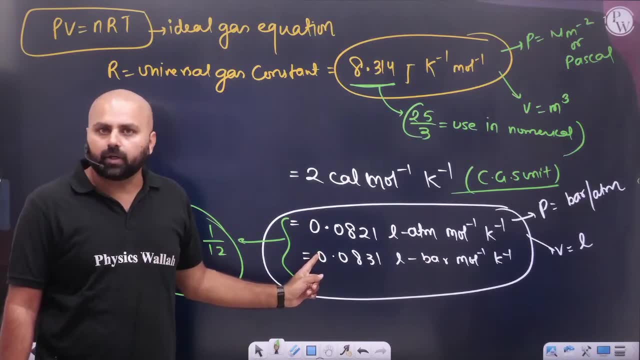 These two will be used in thermodynamics. These two will be used in thermodynamics. equilibrium Rest when you study the gaseous state. whenever you study the gaseous state of the matter. you are going to use only this, Okay. 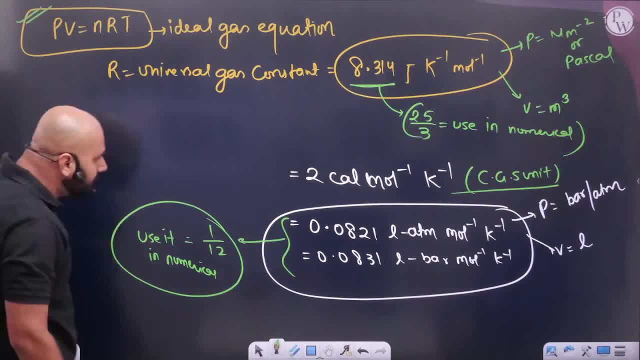 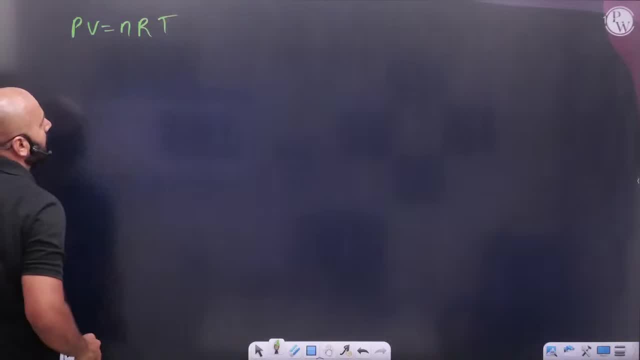 PV is equal to NRT. Sir, I am not afraid of it, but I am afraid of its application. How See this? How is it afraid of the application? Someone said: sir, it is an ideal gas equation. Sir, it is an ideal gas equation. 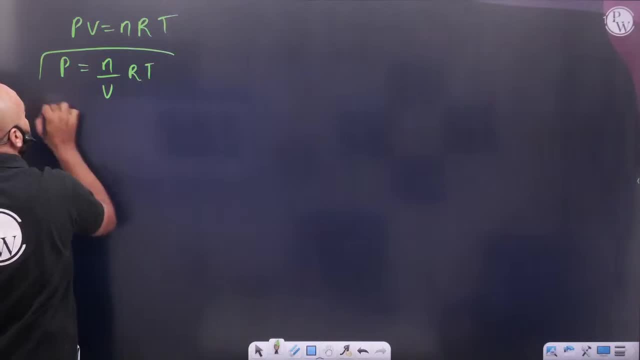 I can write like this too: PV is equal to N by V And N by V. sir, I can write concentration too, C for concentration, Concentration. Or if I want to write this, only then I can write the molarity too. 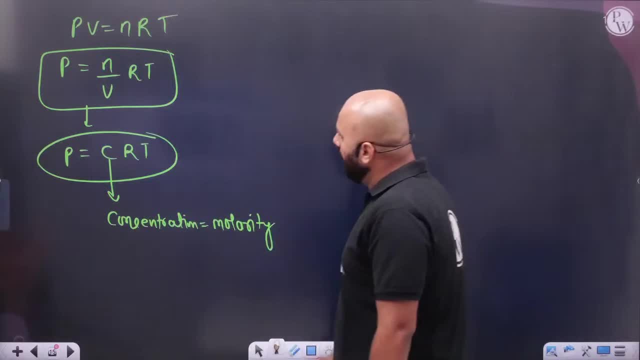 Remember, I can say concentration or molarity too. This is an ideal gas equation. From here, when we will go to chemical equilibrium, I am going to use here the formula of concentration. what happens? PV by RT? How did it come? 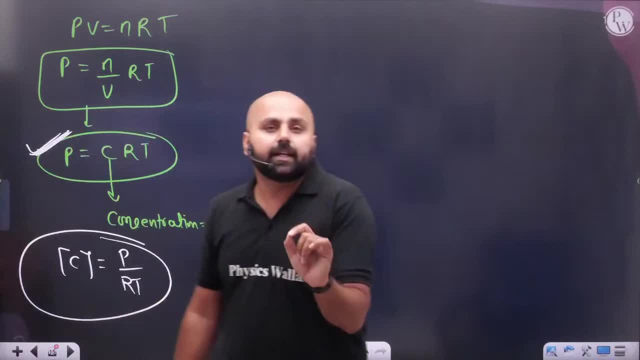 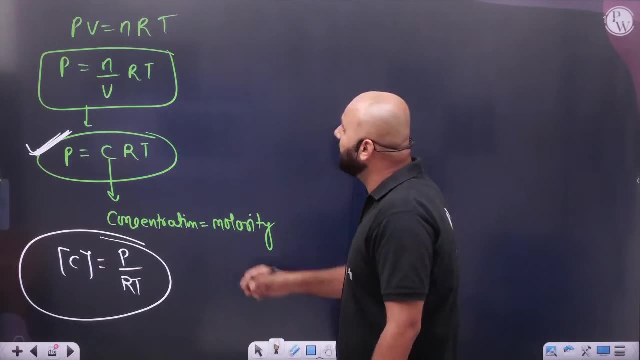 Ideal gas equation. One more way to write this equation- The level of NEET- is that you must be asking these formulas. Formulas are asked. brother, You will not be able to think in the exam hall. You do this. he will not ask you about ideal gas. 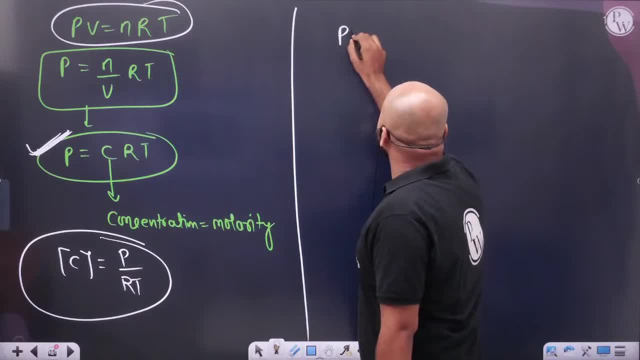 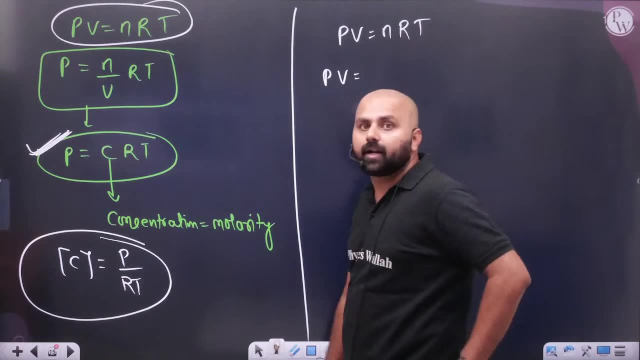 He will say: tell me about this Second thing. who said, sir, we can write it in some other way? Yes, we can write. See, this, PV is equal to. PV is equal to. Okay, those who are remembering: 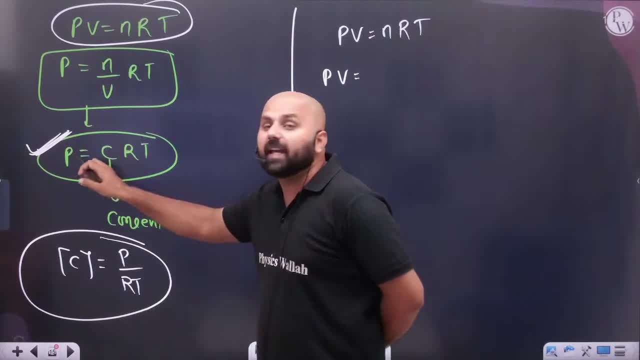 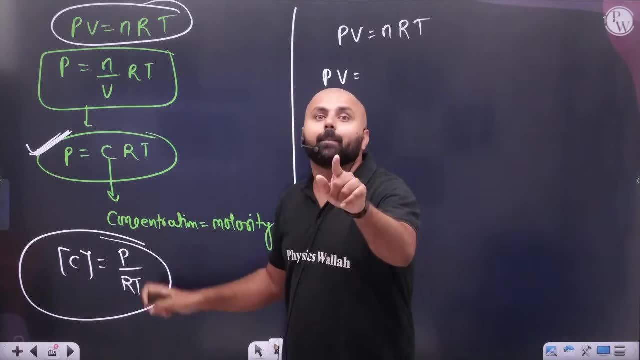 let me remind you one more thing, Because this is a marathon class, Sir. this formula, exactly this formula, is found in the solution: PI is equal to CRT. Remember: PI is equal to CRT. What was PI? It was osmotic pressure. 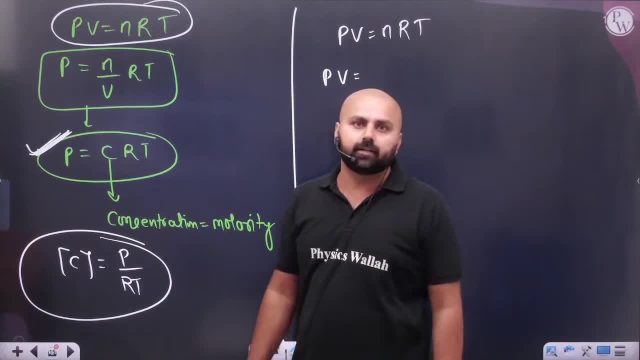 What was PI? It was osmotic pressure. So, brother, keep relating the chapter to the chapter. This is in the case of gas. For whom was it? It was in the case of solution. For whom was it? It was in the case of solution. 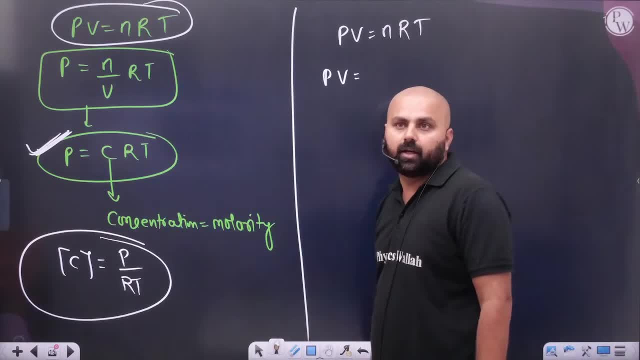 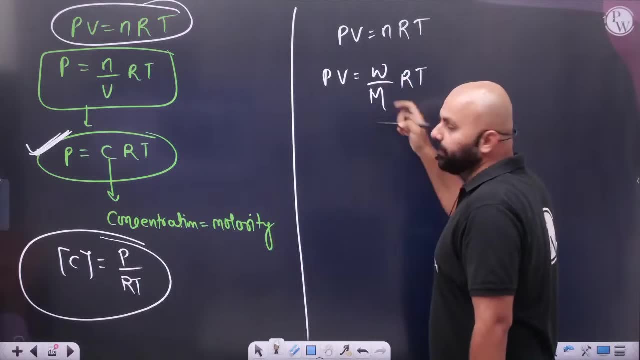 There was PI, It was osmotic pressure. Here is the pressure of gas. Okay, Brother, keep remembering. side by side. See this, Sir, number of moles. I can write this formula: Given mass upon molar mass. 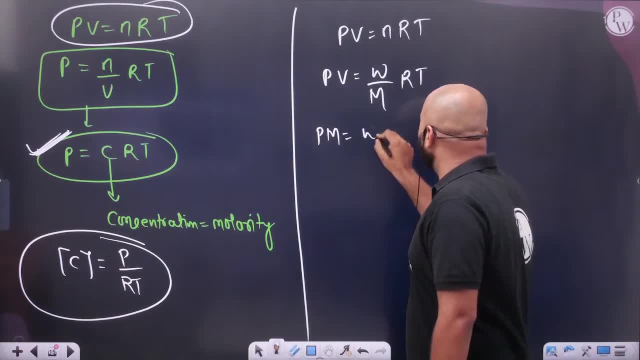 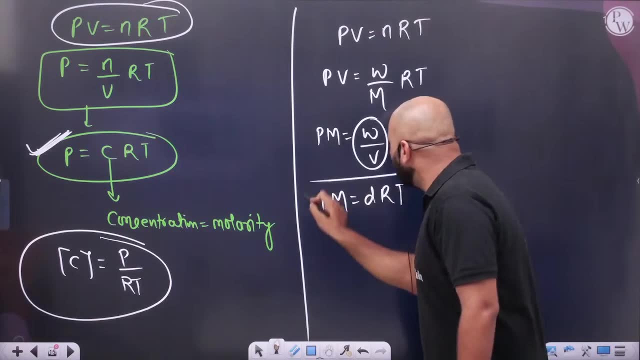 Sir, here PM is equal to mass upon volume RT. And what do we write? mass upon volume, Brother, I am telling you a simple line: PM is equal to DRT. Okay, PM is not scary. Keep remembering, like this. 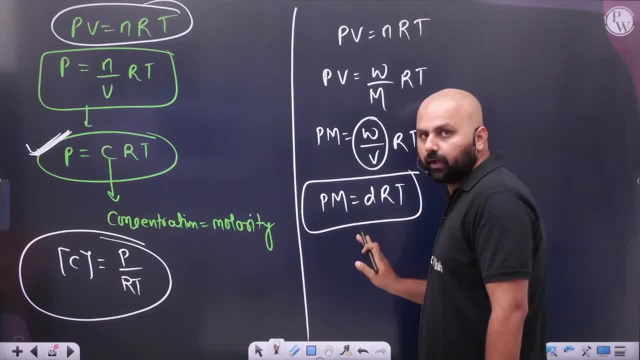 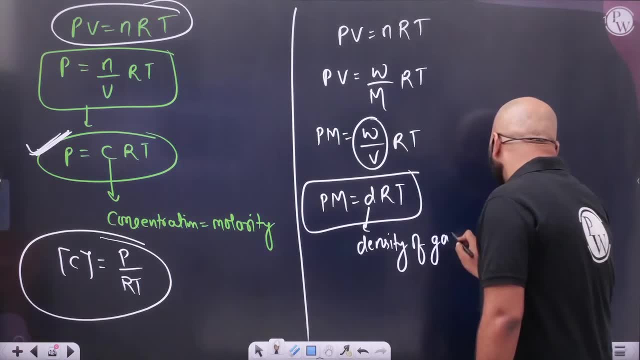 If someone forgets, then PM is not scary. Okay, PM does not get scared. It is a simple thing. So what is D Density? And, brother, if someone asks density of gas, then how much will be the density of gas? 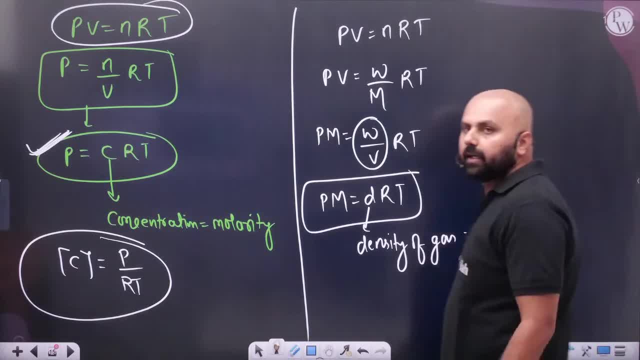 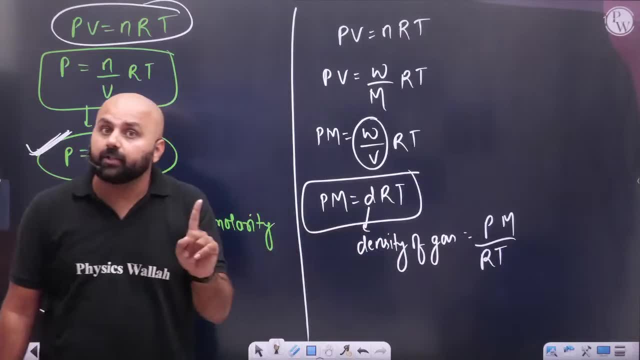 PM upon PM upon RT. What will be the density of gas PM upon RT, Sir? how much will be the density of gas PM upon RT? Listen carefully, Because it is a very important thing. All these things will come in states of matter. 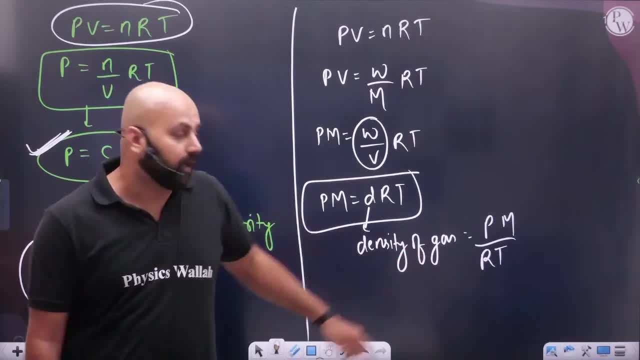 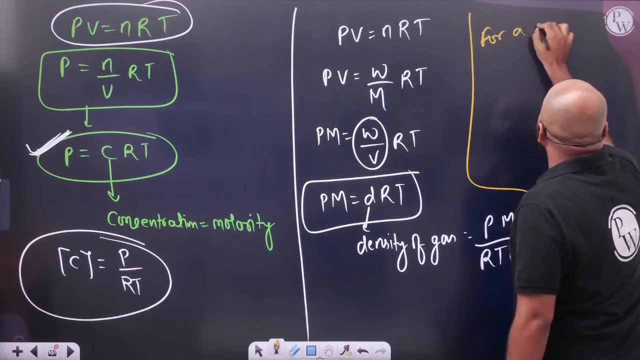 Today, the whole marathon is there. Get ready to run. I will not repeat there. See this: Tell me one thing about density of gas For a gas For a gas. I am asking you a question, Brother. tell me the answer. 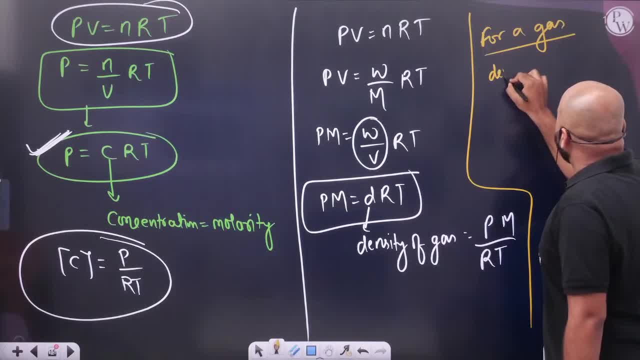 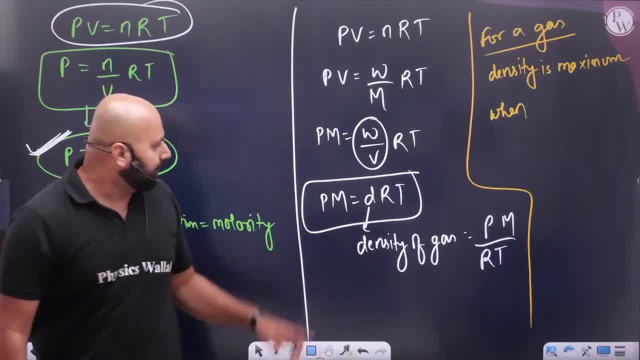 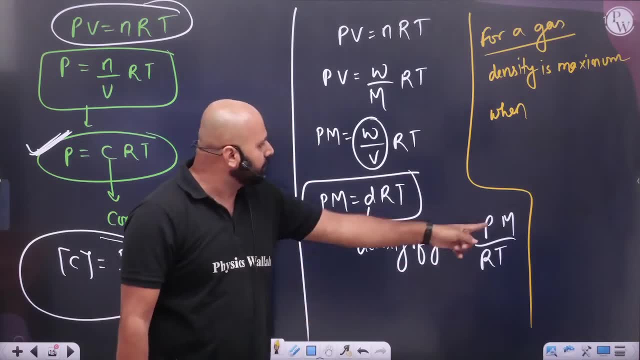 Tell me, It should be more pressure or less. It should be more temperature or less. If the density of any gas want to be more and to make density of gas maximum, then, sir, fix it like the gas. fix it like the gas. 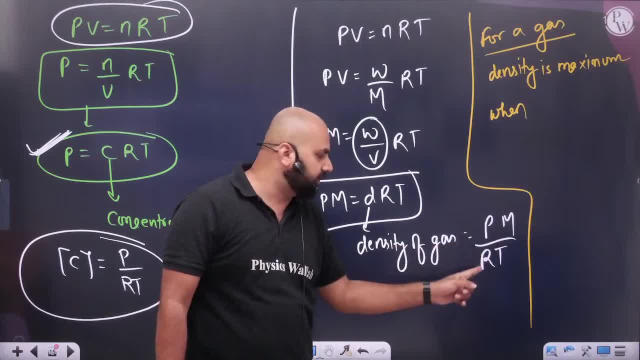 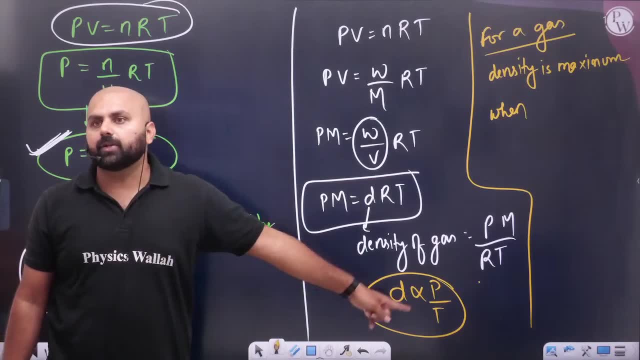 Sir, fix it like the gas. The molar must is fixed, the hour is fixed. I can say here that density is pressure by density is direct proportional to pressure by temperature. density is direct proportional to pressure by temperature. And when will the density of gas be maximum? 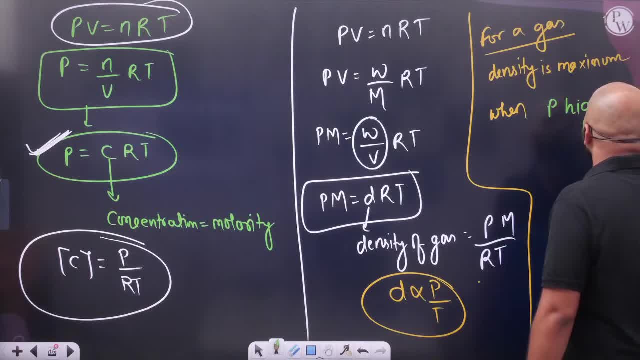 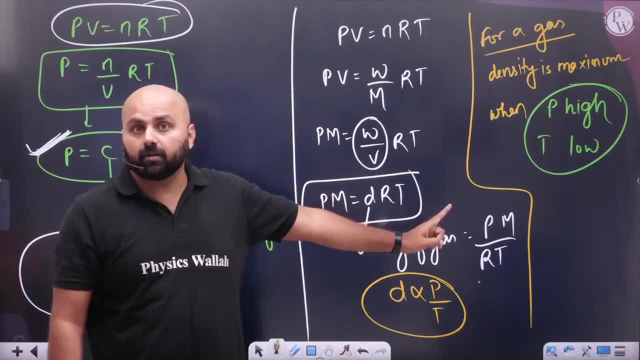 When will it be maximum? When the pressure is high and the temperature is low? When the pressure is high and the temperature is low. See, in the whole concept, straights are matter, Because this is a marathon. there is no boundary here. 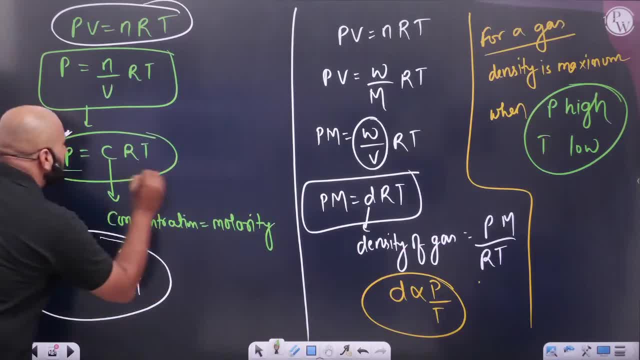 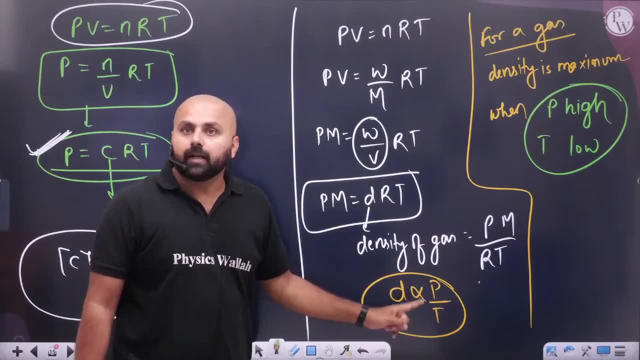 There is no boundary in exam pass, Sir. see, P is equal to CRT. Whom did I remind you of osmotic pressure? See there. when will the maximum and minimum of the density of a gas be? When will the maximum and minimum of the density of a gas be? 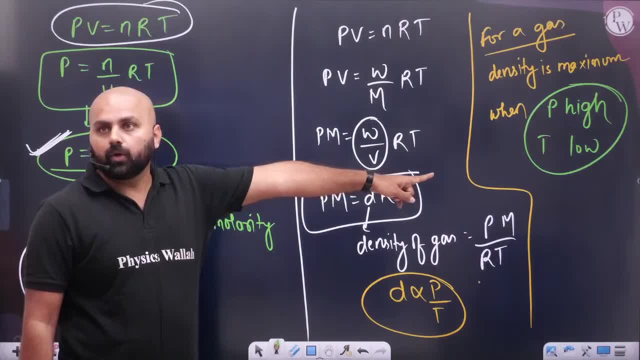 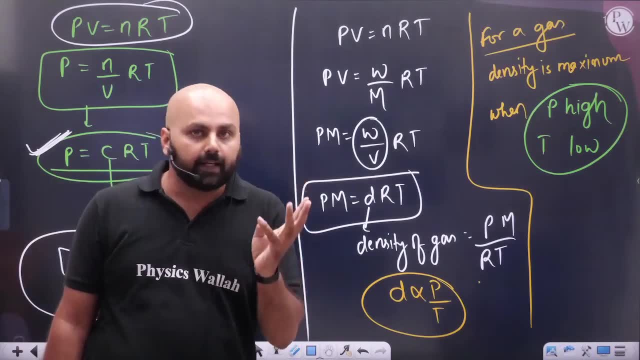 When the pressure is high, what should be the temperature? It should be low. Okay, Okay, This is for a gas, this is going on. Who said, sir? there is one more concept: Density is done. See, the ideal gas equation came. 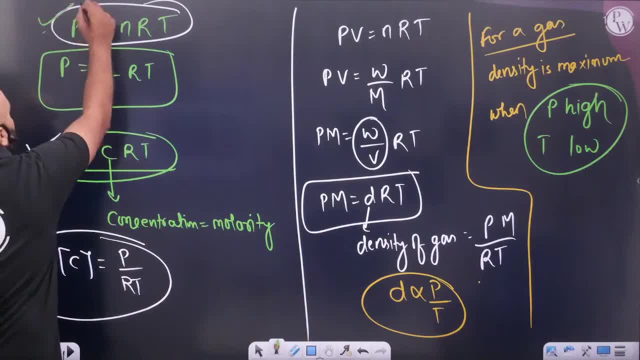 I wrote the ideal gas equation in different ways. This was the ideal gas equation. Then I wrote it like this. Then I wrote it like this: PM is equal to DRT. After that, after that, who told me, Sir, there is a term whose name is vapor density. 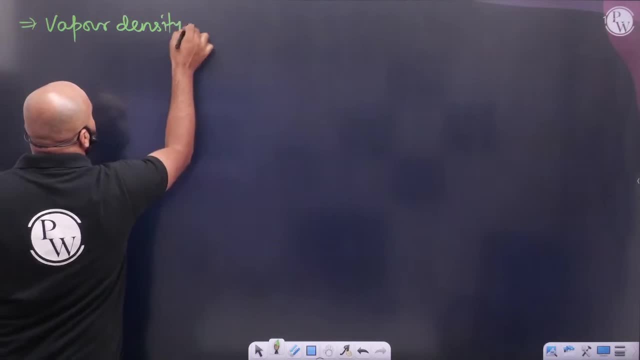 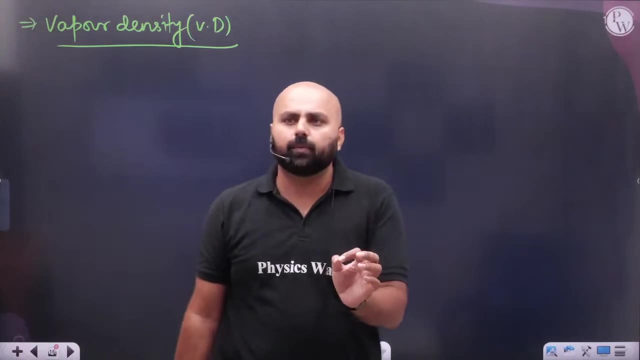 There is a term whose name is vapor density. Brother, listen carefully, Because there is a very basic thing in the exam hall: Vapor density. But should I ask a simple thing, Brother, if I want to ask a simple thing here: Vapor density in the exam hall. 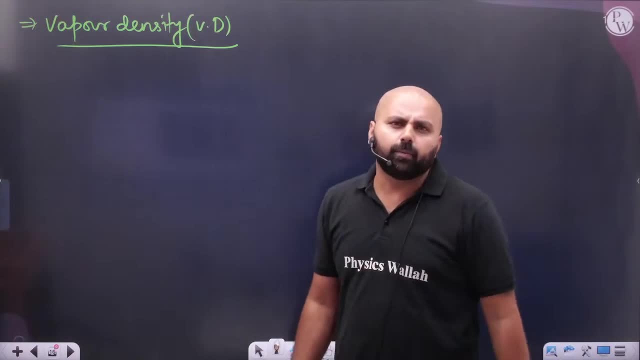 And people do not know the definition. People are sitting in a hurry. Vapor density is nothing. Molar mass by 2. Molar mass by 2. Brother, molar mass by 2 is not fixed. What is vapor density? 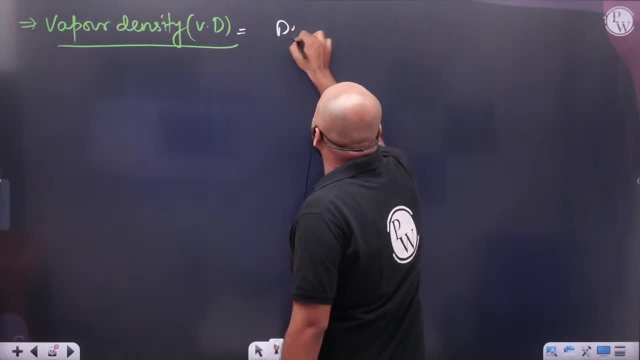 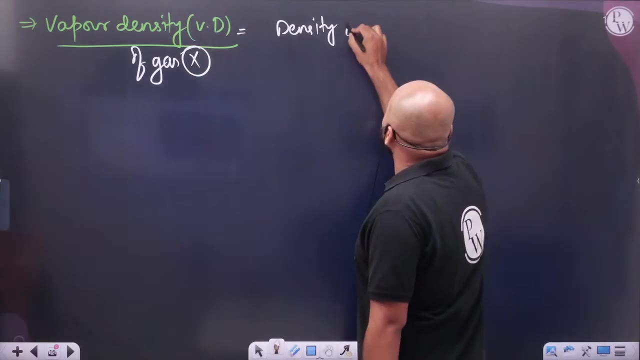 What is the ratio, Sir? density of gas- Density: You are going to remove the vapor. density of a gas, If suppose there is a gas X. So density of gas X, Sir, at same temperature and pressure. At same temperature and pressure. 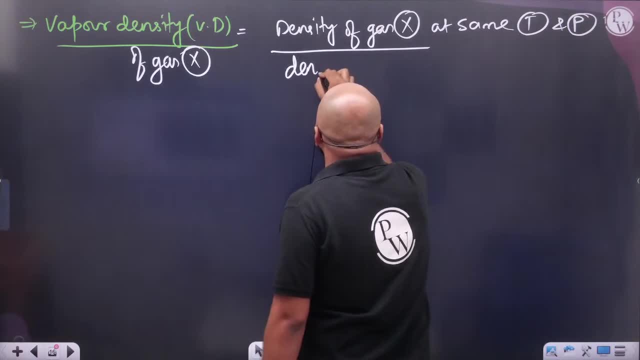 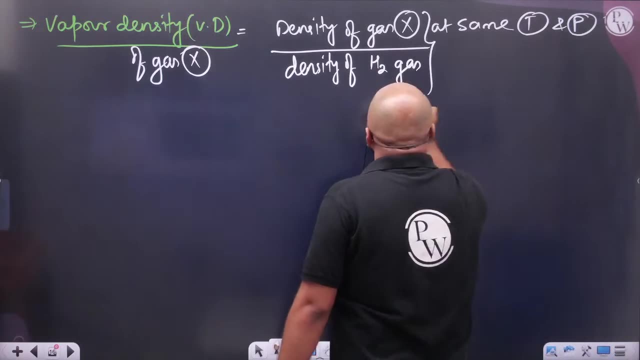 See this Density of gas, Sir. that is why do not go by dragging anything, Brother. see this in the exam hall, Sir. density is vapor. density is nothing. Relative quantity is there. Listen carefully. Vapor density is nothing. 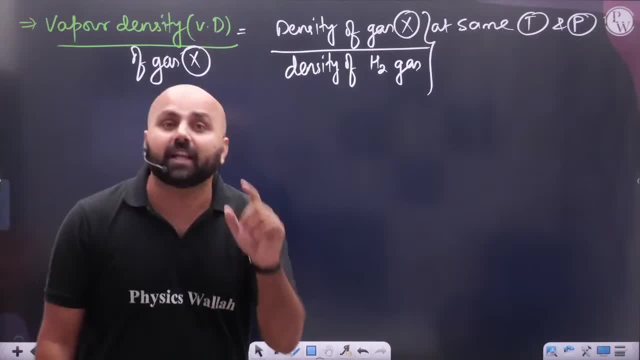 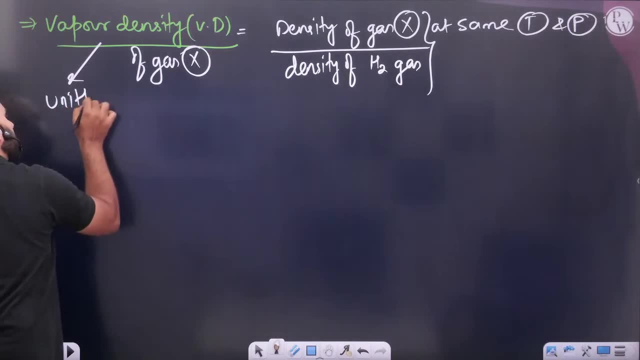 Relative quantity. Relative quantity, There is a ratio. That's why there is vapor density. Vapor density never comes in units. Vapor density never comes in units, Brother, it is unitless. Listen to the story, Because the problem is in the exam hall. 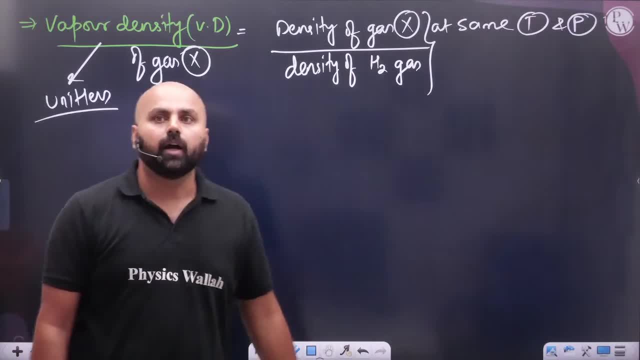 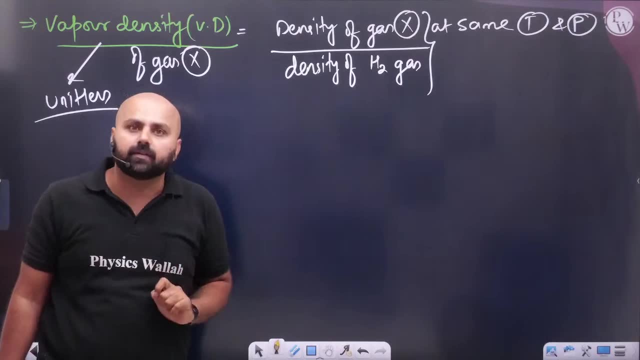 These small questions. What will happen? It will be unitless. What happens? Density of gas X Divided by density of hydrogen gas. Sir, what is the ratio of density? Vapor density. Why hydrogen gas? Because hydrogen is the lightest gas. 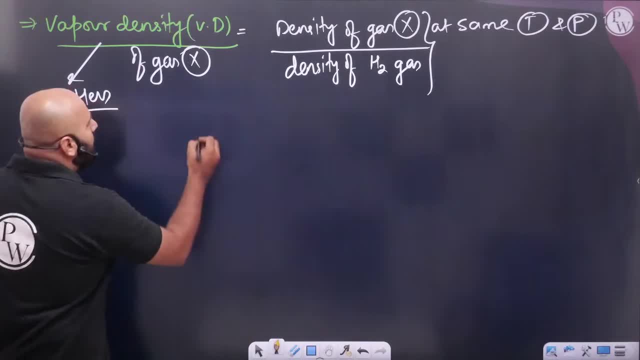 Now it is my wish. In the exam hall, Sir, see it. I said vapor density of gas. Whose to be removed? What is the formula of density? PM upon RT, Sir, what will happen? Pressure of X. 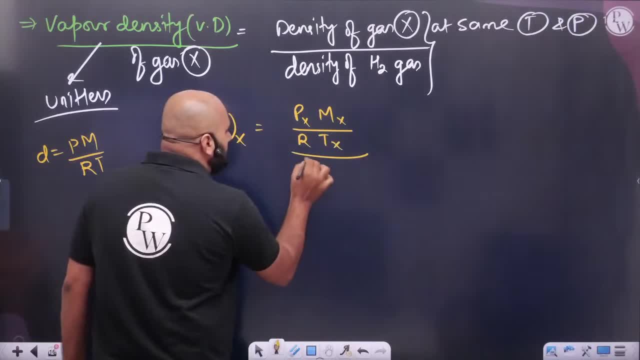 Molar mass of X- RT of X, Divided by pressure of hydrogen. Molar mass of hydrogen Divided by RT of hydrogen. See this. You will write this only, But, sir, you also know Temperature and pressure are same. 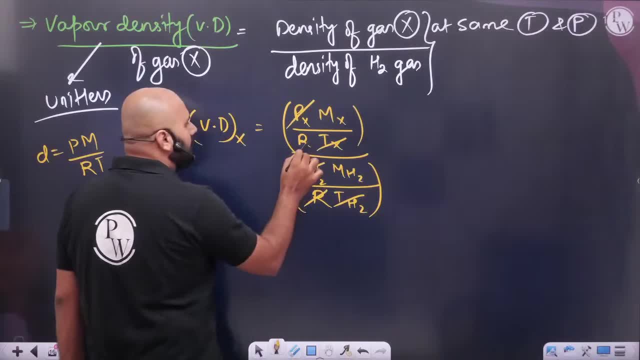 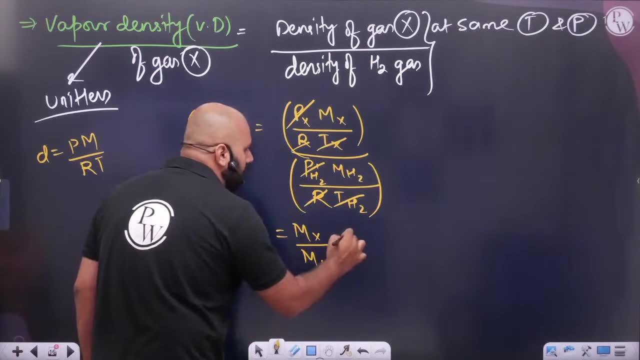 So, sir, what will happen? It will be cancelled. R to R will be cancelled. Vapor density of X is nothing. Molar mass of X Upon molar mass of hydrogen, And that's why Molar mass upon 2 comes. 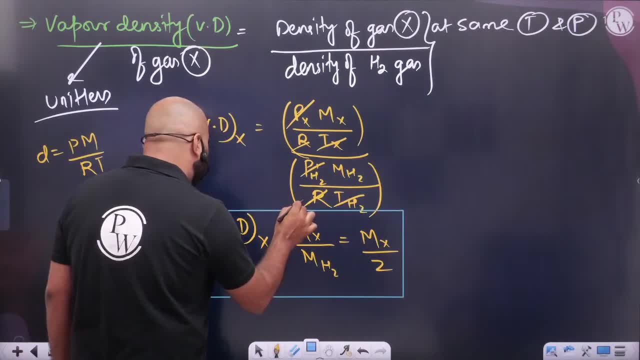 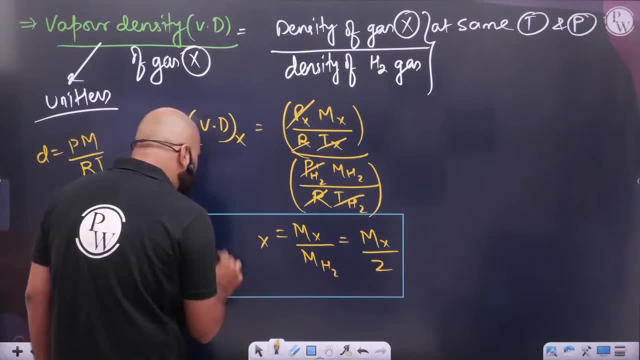 Brother, the formula. How did this formula come? Learn this? Because this formula is very useful. This formula is very useful, Brother, See how will I make the question. I have given you the formula. Vapor density is nothing. Molar mass of X upon 2.. 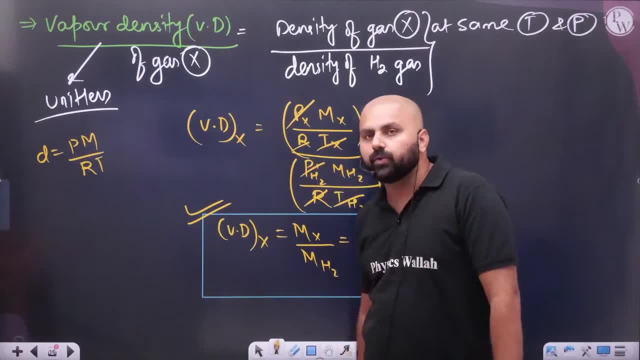 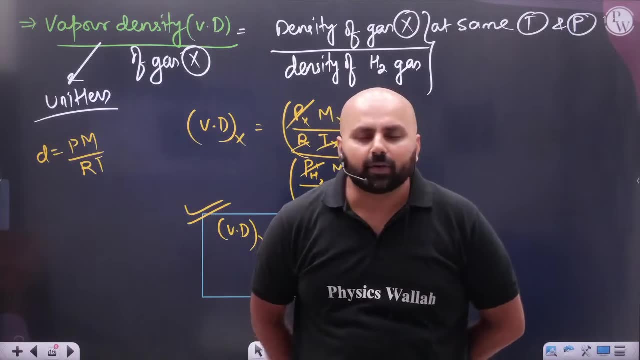 Do you know what will be asked in the exam hall? What is the unit of vapor density? Many people Do you know what will be written in the unit of vapor density: Gram per centimeter. Why gram per centimeter, Brother? why not gram per centimeter? 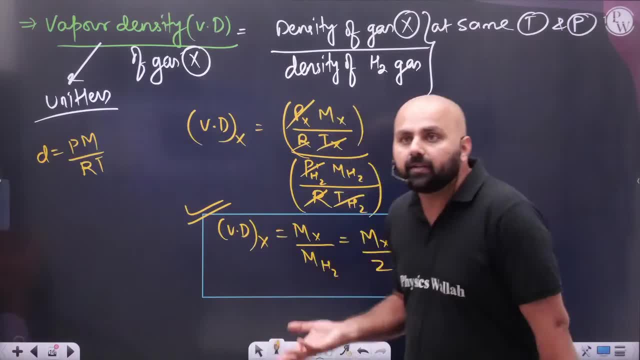 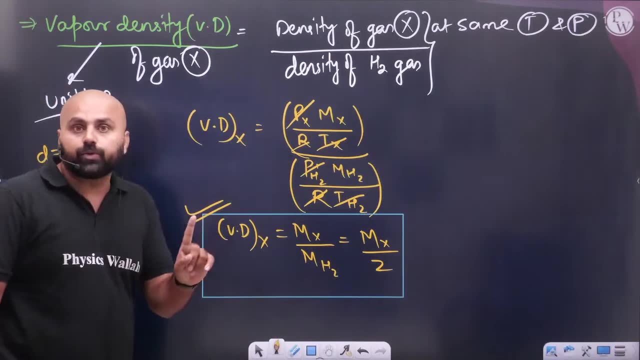 Vapor density is the ratio. It is the ratio, brother. What is vapor density? It is the ratio. If it is the ratio, then what will happen? in that case? You will not get any unit, Okay. Second thing, Second question: 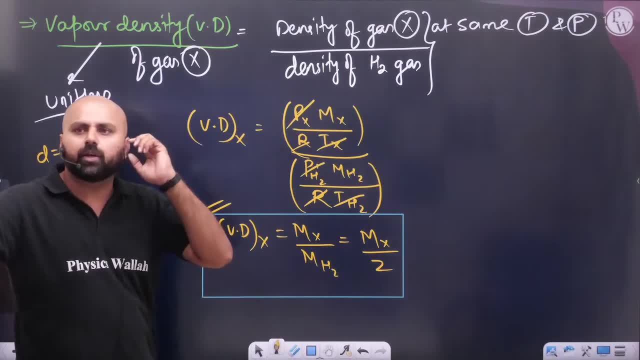 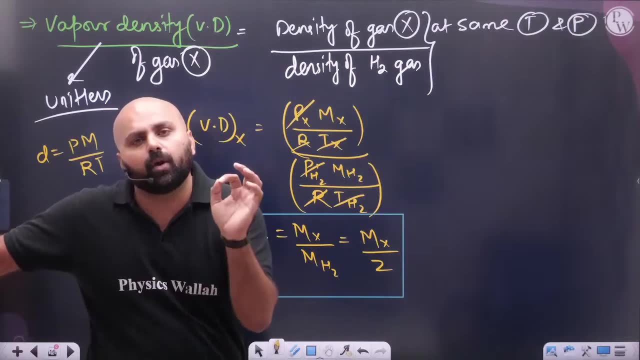 Sir who said that from today, Vapor density. From today, The lightest gas, The lightest gas From today, Let's assume oxygen. If I assume, Let me change the definition. Let me change a simple thing in the exam hall. 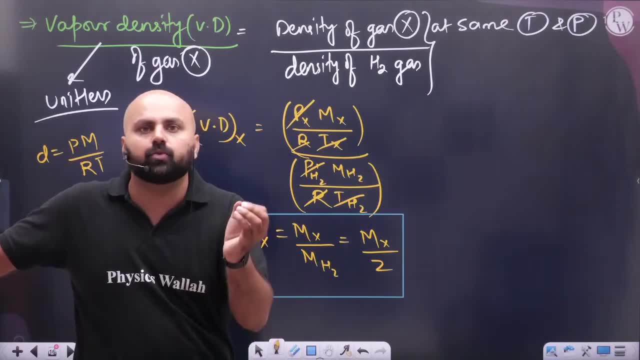 I say From today, Who will be taken as the lightest gas, Oxygen, will be taken. Will you tell me what will be the change in the formula? What will be the change in the formula, Sir? what will be the change in the formula? 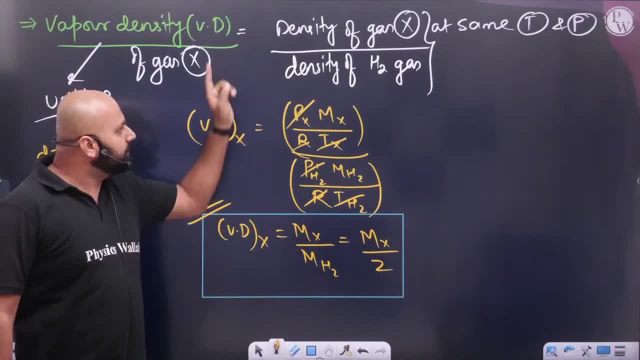 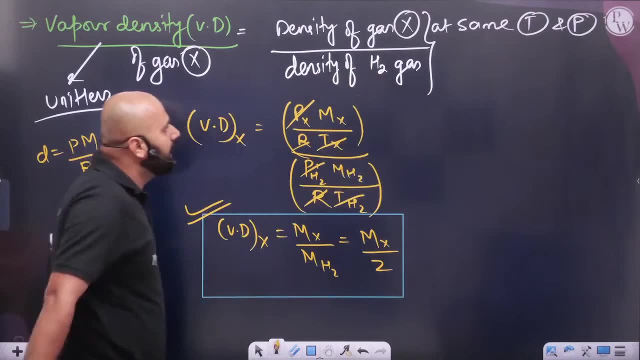 If I said today, Sir, in the ratio, When you take the ratio, So which will be the lightest gas? Oxygen gas will be Brother, if there will be oxygen gas. So density of oxygen gas. Here we will write density of oxygen gas. 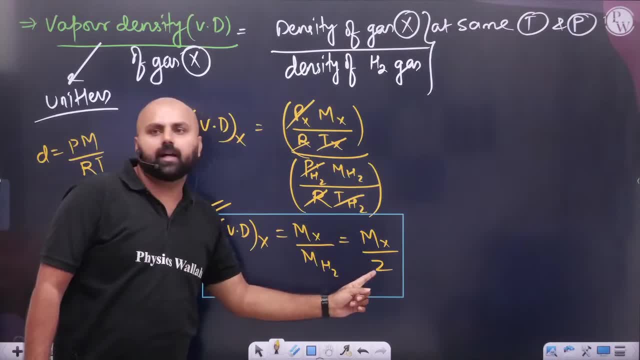 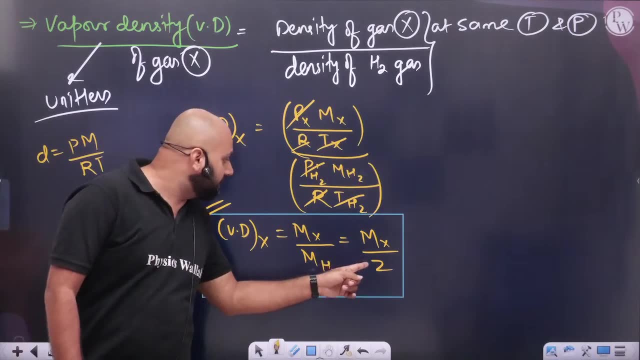 We will write O2.. We will write O2 here, And how much will come here? Thirty-two will come. How much will come? Thirty-two will come If oxygen will be the lightest gas. So what will come here? How much will come instead of 2? 32.. 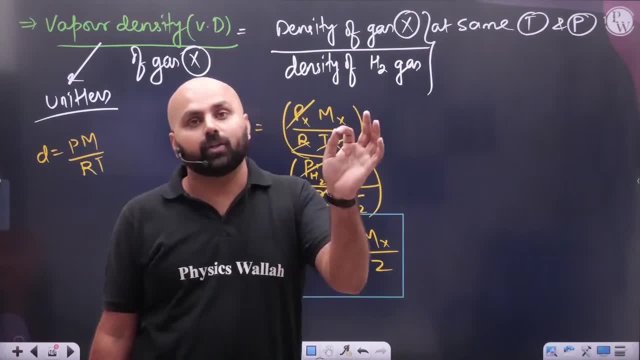 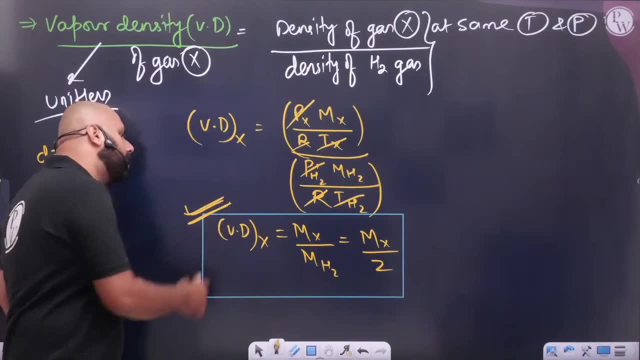 So the ratio of vapour density is a relative quantity Which depends on whose ratio This one. So, brother, just change it. If someone asks you something normal in the exam hall, then obviously you are always in respect of hydrogen, Because it is in respect of lightest gas. 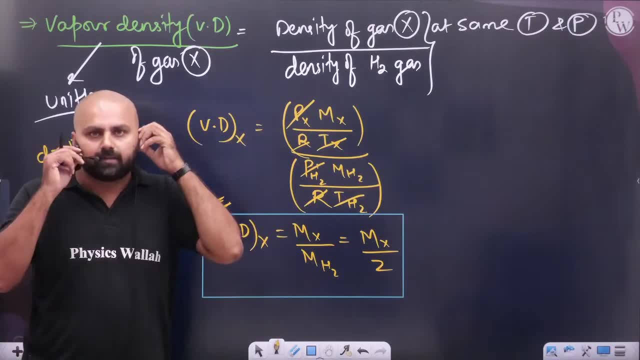 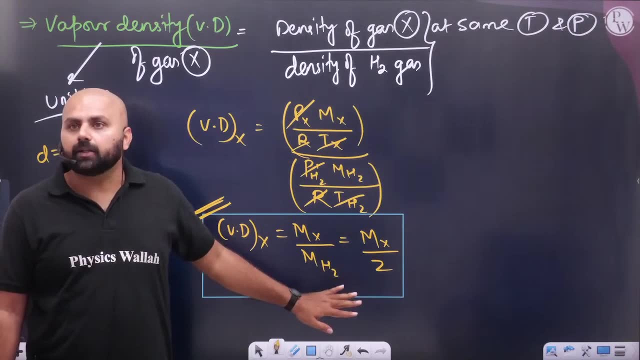 Brother molar mass of oxygen gas is 32.. Brother, oxygen is gas, It is O2 gas, It is not oxygen atom. It will definitely happen. It will be divided by 32.. Sir, the ratio of vapour density with molar mass? 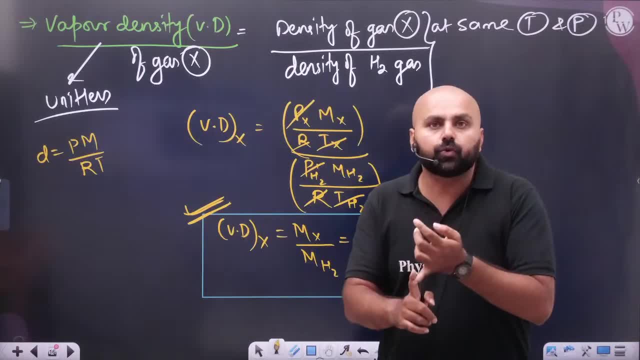 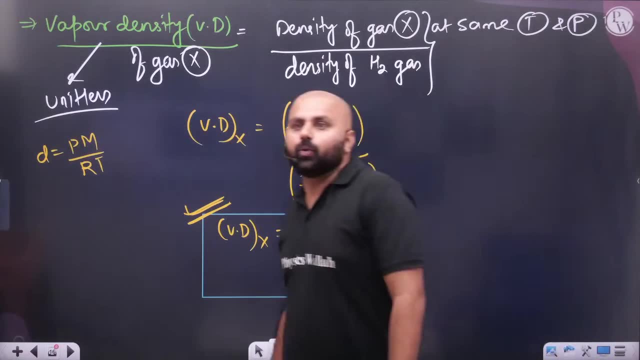 Okay, vapour density is done. Pb is equal to nRT, Pm is equal to drT, P is equal to crT, Apart from vapour density. Now look at the question. Now look at the question. What happens? 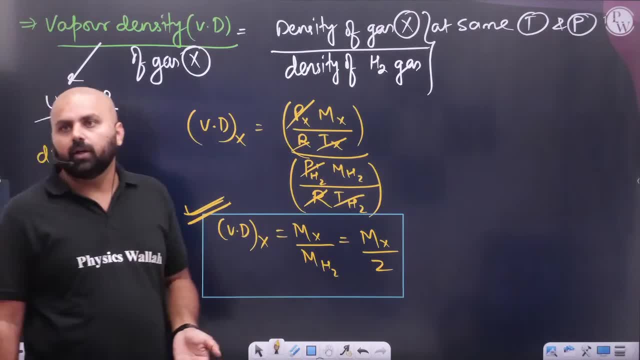 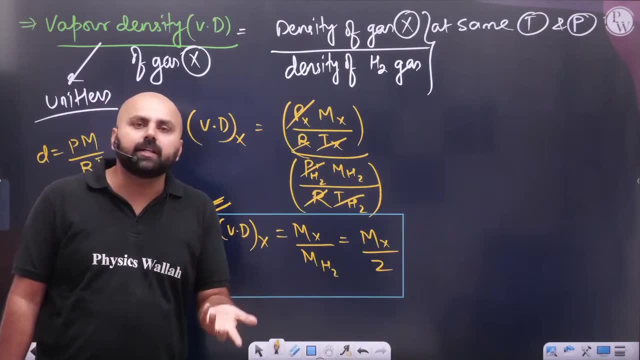 Now look at it. Specific gravity is nothing. It is a ratio of density. That is a different thing. You will study specific gravity in physics. It is a ratio of density. Yes, you have a ratio of density. In which respect? In respect of water? 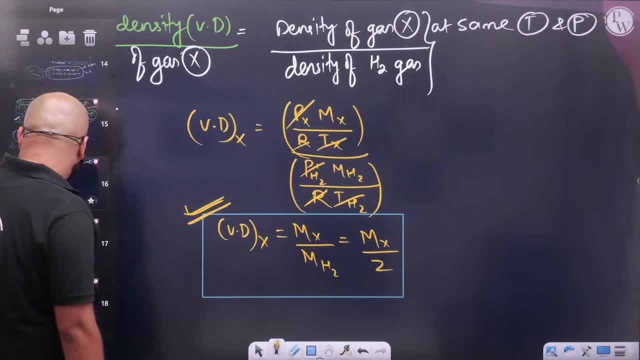 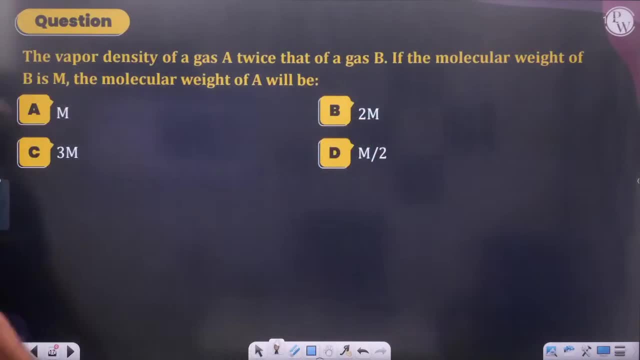 Okay, Now look at the question. Now look at the question. Now look at the question. It is a simple, formula based question. Those who want to attempt Vapour density of a gas x: Quickly attempt and see. Quickly attempt and see. 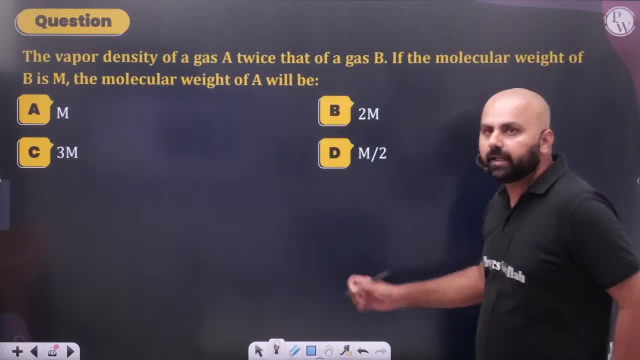 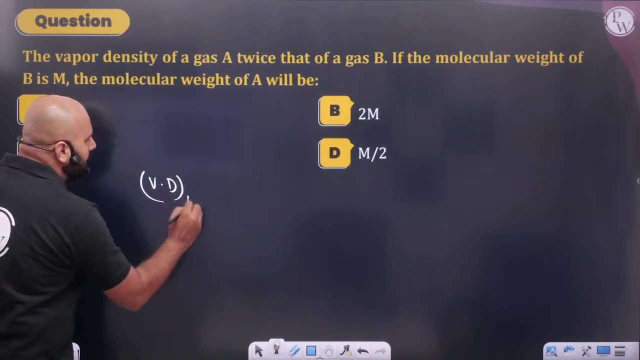 Quickly attempt and see What will happen. Who will be? How will it happen? What will happen, Sir? vapour density of a gas x is twice than Vapour density of Brother whenever you sit in exam hall. Many people's English is a little weak. 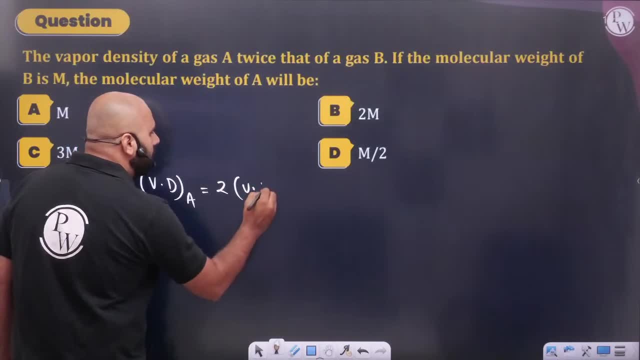 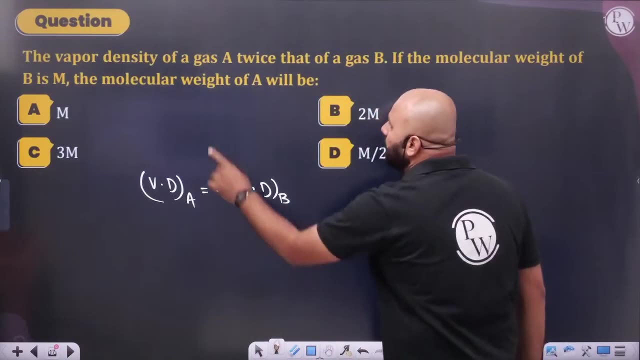 They are not able to write. Brother, look Whenever you feel, If you feel that my English is very weak in exam hall. So, brother, what to do? quietly, Start writing like this: Vapour: density of a twice that of of b. 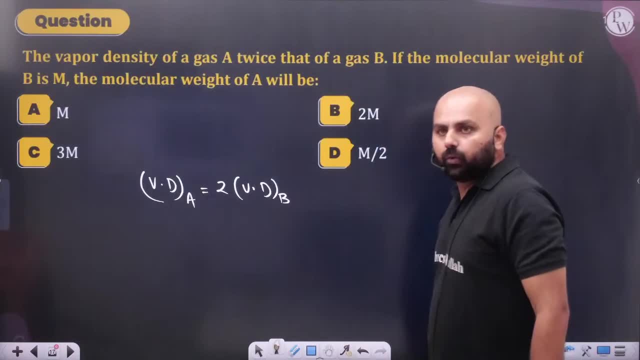 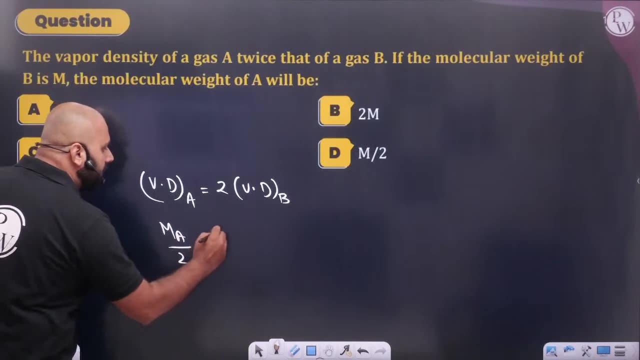 Means b will be twice. Who A After that? someone said that sir its molecular mass. So what will be the vapour density of a Molar mass of a divided by 2.. How much will this be? 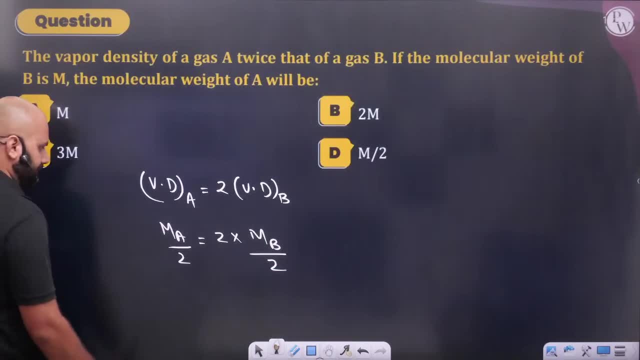 Sir, what will be the vapour density of b: 0.2.. Sir, this, So this 2 to 2 is cancelled out. Molar mass of a is nothing. 2 times molar mass of b May be. our answer will come. 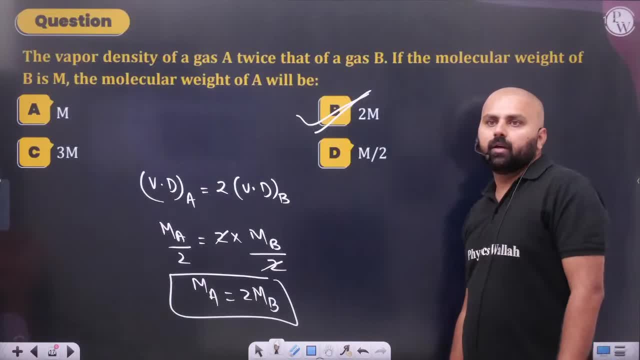 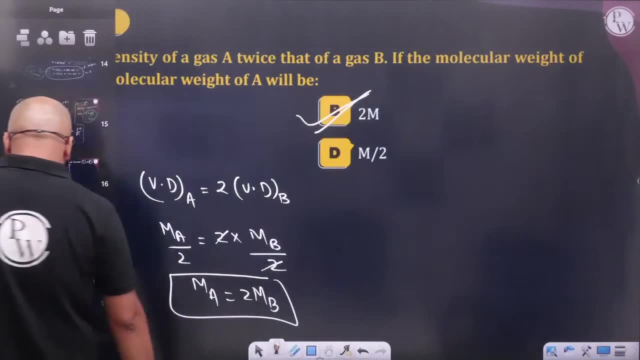 What will be the molar mass of a 2 times molar mass of b? You keep doing Vapour density Relation according to that. Whenever you will get a question, Whenever you will get questions, You get answers according to that. 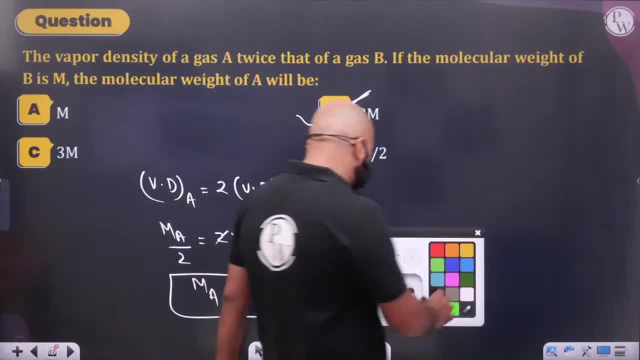 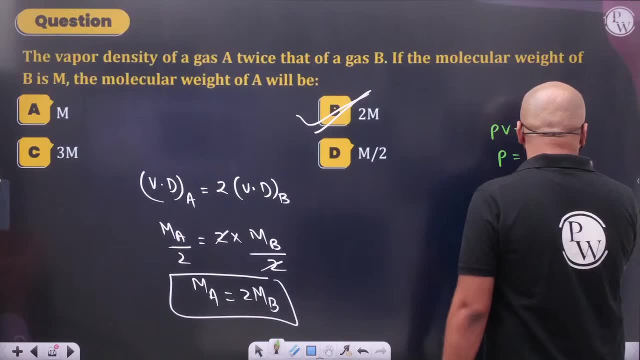 Sir, these are small questions. I am saying again and again. See, I will write all the formulas together: PV is equal to NRT. P is equal to concentration into RT. Sir, we have: PM is equal to density into RT. 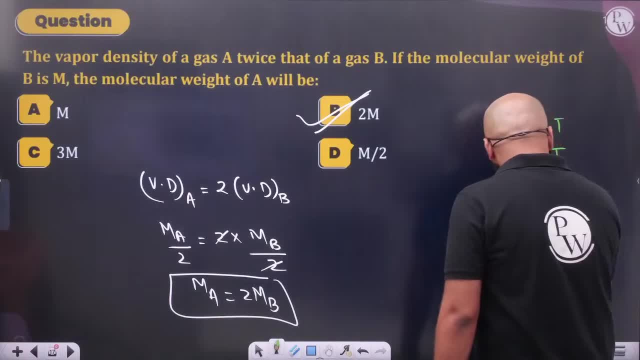 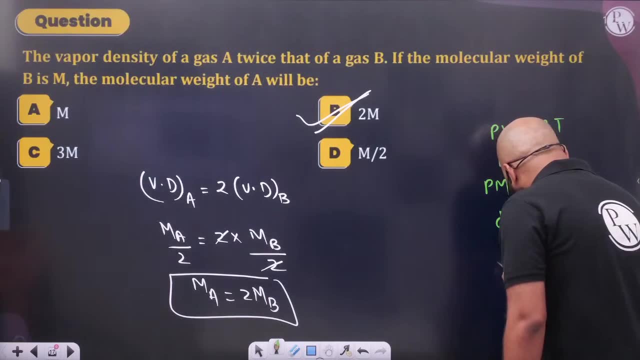 Sir, we have, PM is equal to density into RT. Sir, we have PM is equal to density into RT. If we say density of gas, Density is nothing. PM upon RT. And, brother, look at yourself, What did you get in the end? 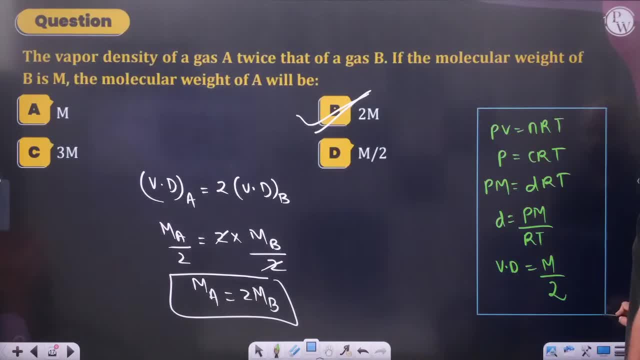 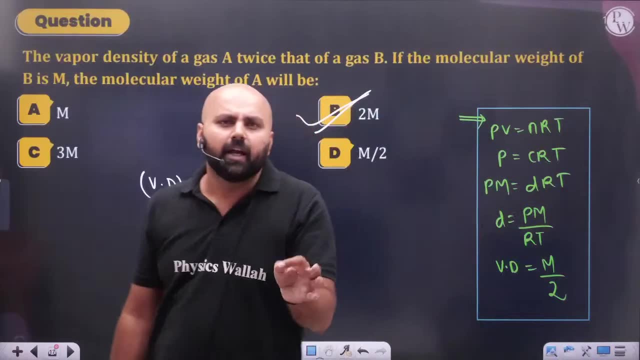 Vapour. density is nothing. Molar mass by 2.. Who is all this for? Don't apply it for liquid and gas. I know such people. They do such things. They will apply this formula on water. They will apply this formula on water. 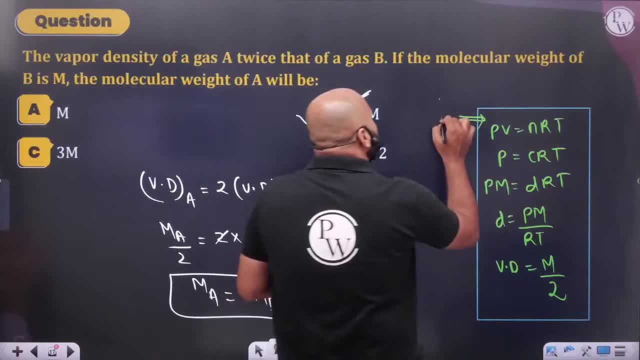 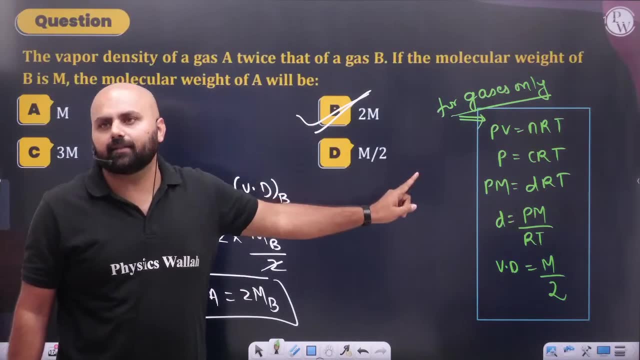 Sir, vapour density of water is asking: Let's remove it. Now, who is all this for? For gases only. There is a difference in both. This is what is fun in exam hall: What happens only for gases. What happens only for gases. 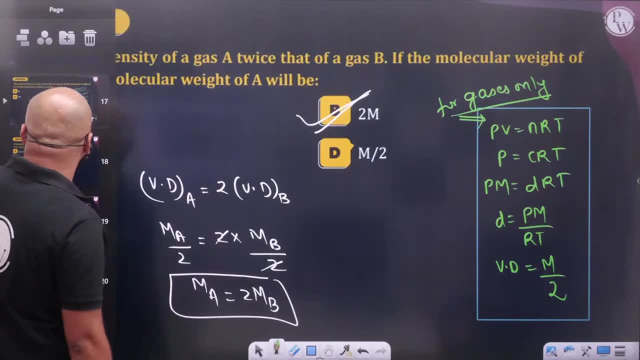 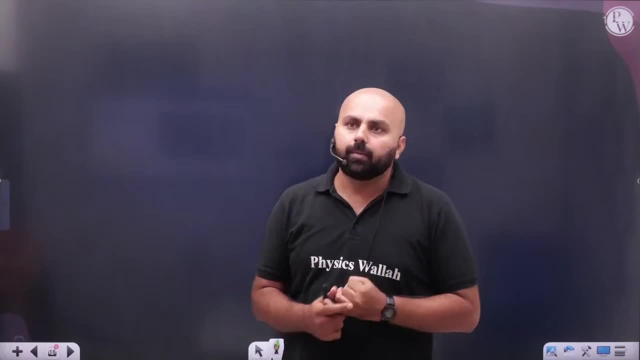 Will you take care of this? Vapour density is done. Now see what else comes in this chapter. Vapour density is done. This is done. Ideal gas equation is done. We talked about this. Now see what else comes. 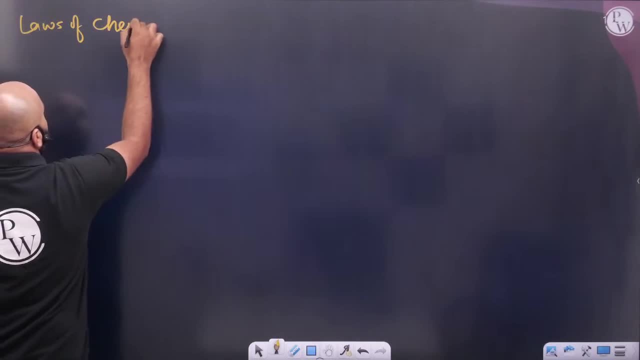 Who told me to do one more thing, Sir. we have laws of chemical combination. Laws of chemical combination is given Brother. all these laws end on one page today. Laws of chemical combination, First, laws of conservation of mass. First laws of conservation of mass. 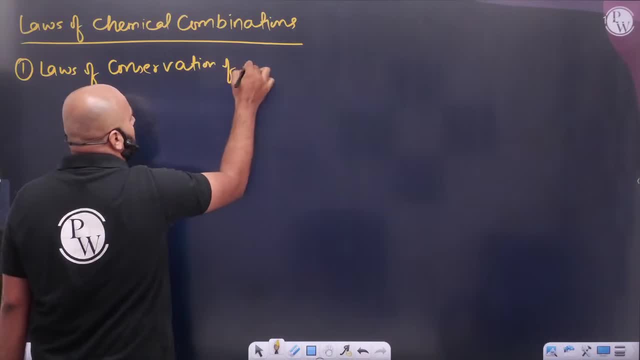 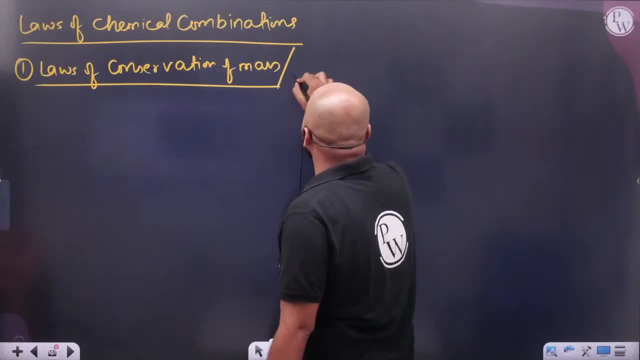 Let me tell you a simple method: Laws of conservation of mass, The way to identify all the laws. Sir, if you go to any chemical reaction, Law of conservation of mass, only Law of conservation of mass, only Call it law of conservation of atom. 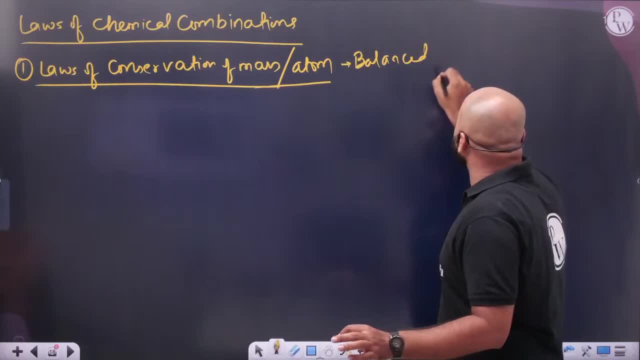 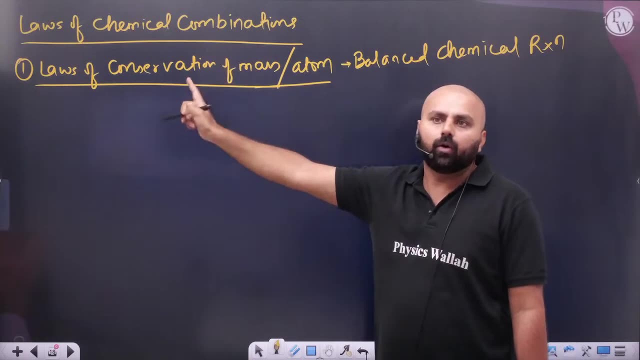 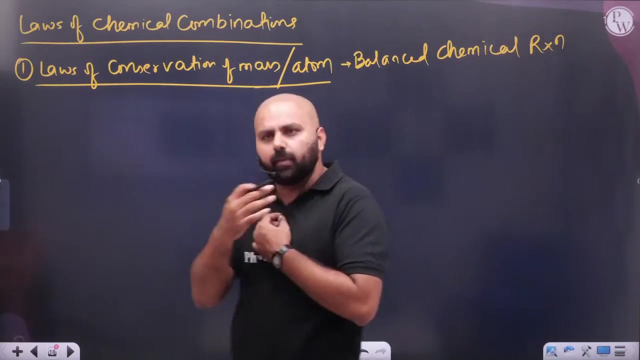 Sir, all the balanced reactions, Balanced chemical reaction, Balanced chemical reaction For whom it happens, Balanced chemical reaction For whom it is valid, For law of conservation of mass, For law of conservation of atom. In this, all the classes, I will upload them. 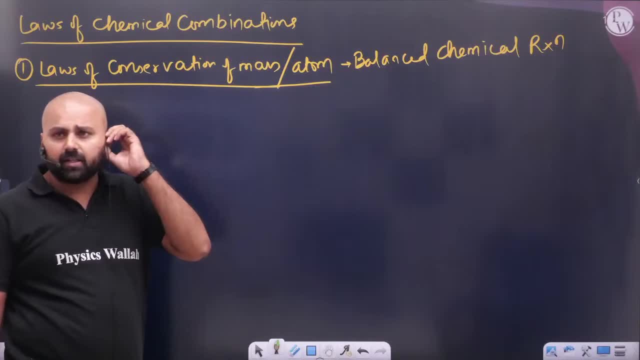 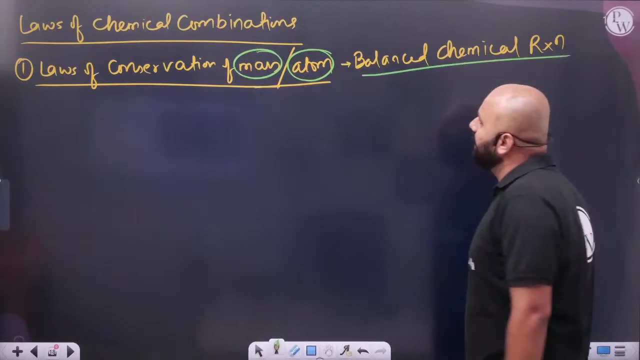 Do not worry, See. See this. I am talking about law of conservation of mass Or law of conservation of atom. All the balanced reactions are based on this. In chemistry we have the mass and atom. Second thing: When we conserve mass and atom, 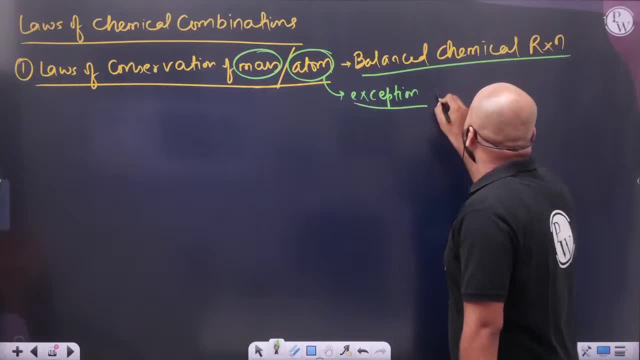 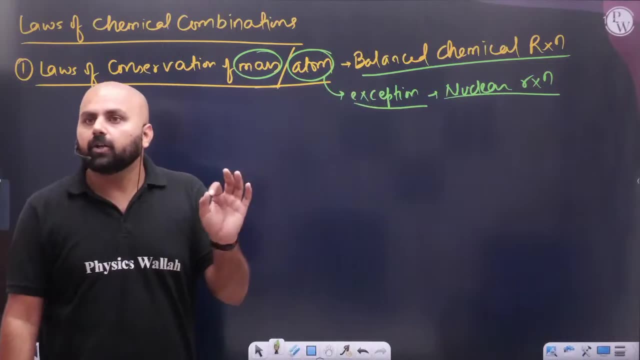 What are the exceptions? Remember What is the exception? Nuclear reaction. What is the exception in this? There is no base on nuclear reaction. Look at yourself in this period, Look at yourself. Valid is not valid in nuclear reaction. After that, who said again? 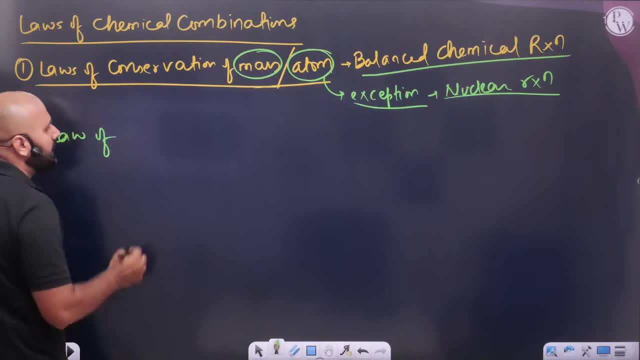 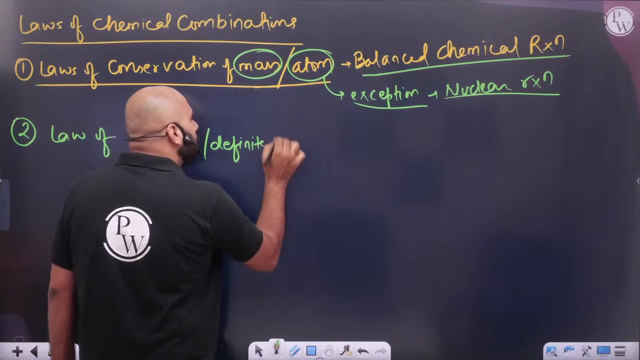 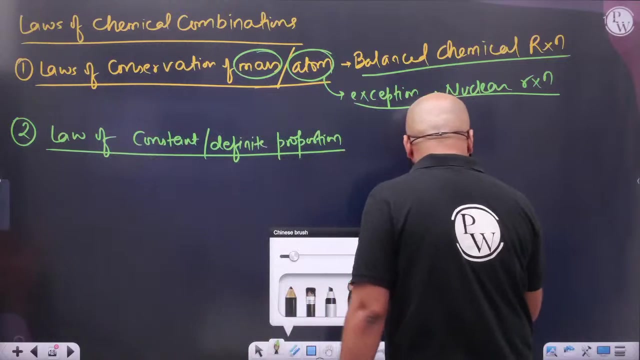 That brother law of law of? If someone tells me that law of constant proportion, Law of constant or definite proportion, Let's talk, Sir. look, it is very simple to question. Law of definite proportion or constant proportion Means if there is a compound, If there is a compound. 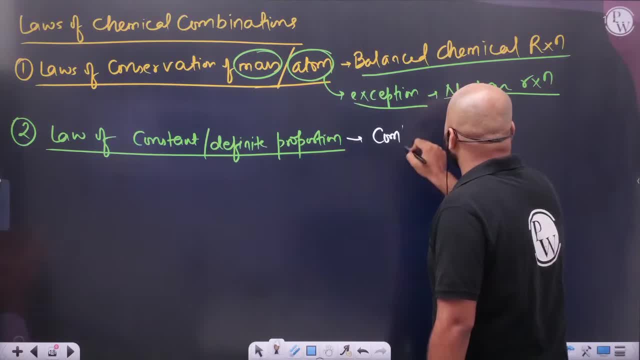 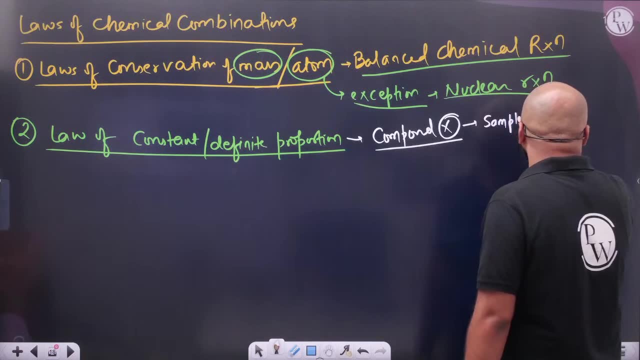 If there is a compound x. If there is a compound x, Keep this in mind. If there is a compound x, Sir, bring its sample, one Sample, from somewhere. Assume that you brought it from Patna. The ratio of the sample is one is to two. 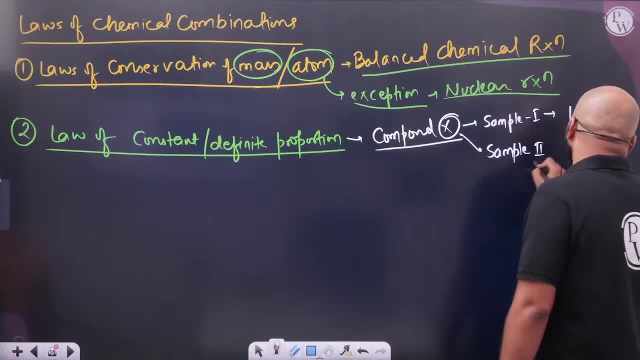 Bring sample two. He will deliberately write this in the exam hall: Sample two must have been given, Sir. what is its ratio? Two is to four. Sample three must have been given. Sir will say: look in different samples, The ratio of mass. 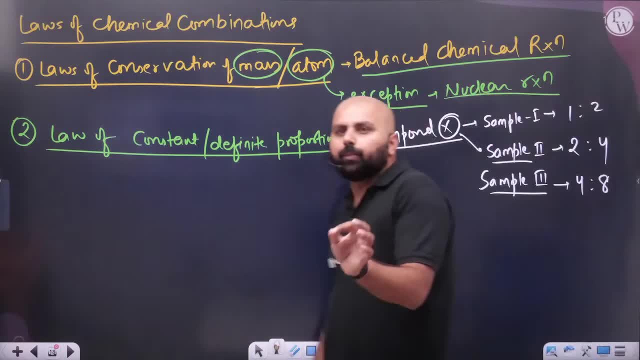 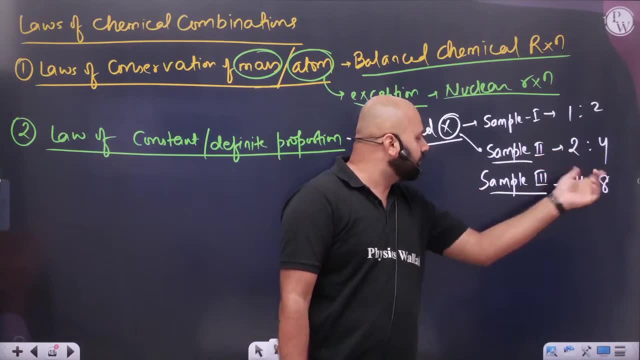 The ratio is like this: Four is to eight. If there is any compound. If there is any compound, Then brother, look at this with us. Okay, look at this In sample. one: one is to two, Two is to four, Four is to eight. 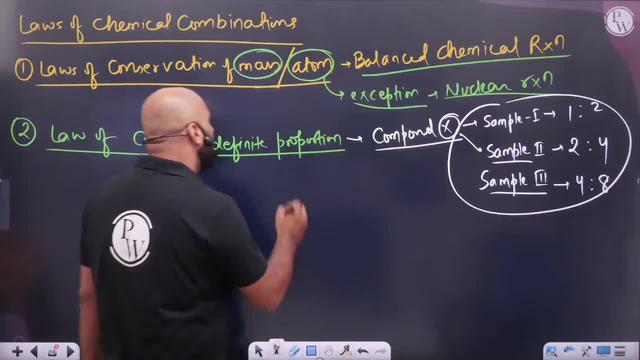 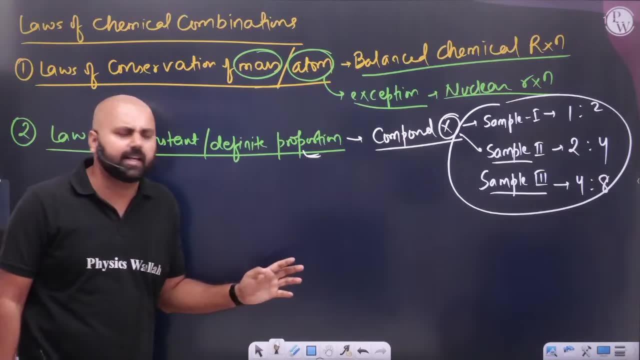 If such a ratio is given. So what is this ratio? It is a fixed ratio. Which one will? we call it Law of definite or constant proportion. We have the same proportion. Bring it from any source, anywhere. Bring it from any source If the ratio of mass is the same. 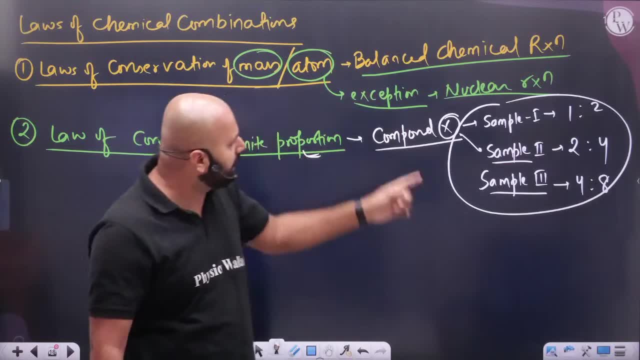 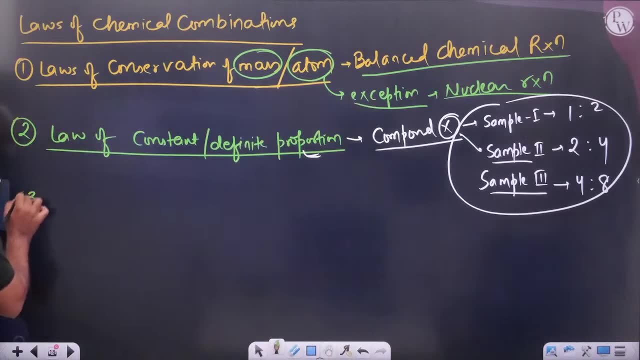 Remember the ratio of mass, Not the ratio of moles. If the ratio of mass remains the same, Then what will happen to us? Law of constant composition. Okay, after that, After that, Who told me? Third one, Sir: law of Law of. 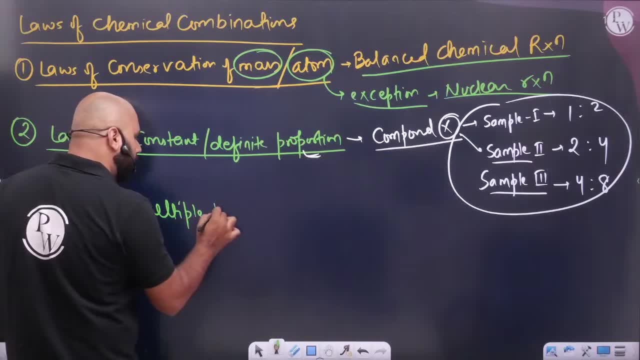 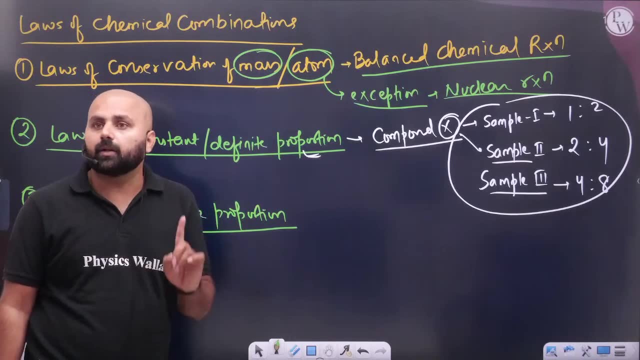 Let's talk about multiple proportions. Let's talk about the law of multiple proportions. Law of multiple proportions: Many people have a headache. Nothing Remember. Let me tell you a simple way You have to remember. Okay, if you want to remember its exception. 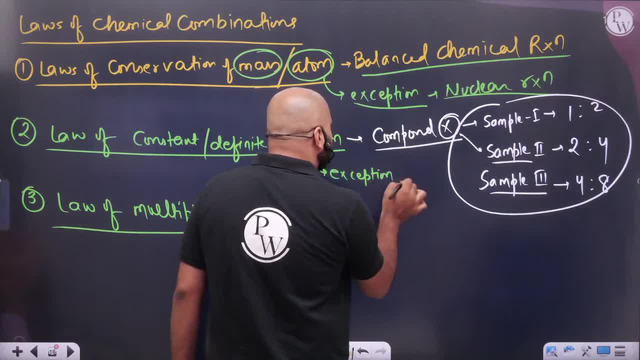 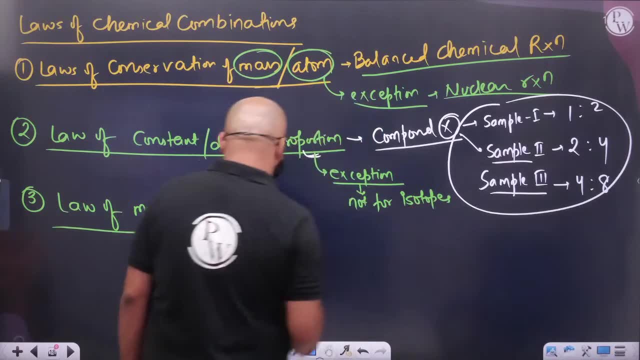 Someone is saying exception, Its exception is not valid in isotopes, Not for isotopes. It is not valid in isotopes. It is not valid in isotopes, Sir. law of If we talk about the law of multiple proportions, What does the law of multiple proportions say? 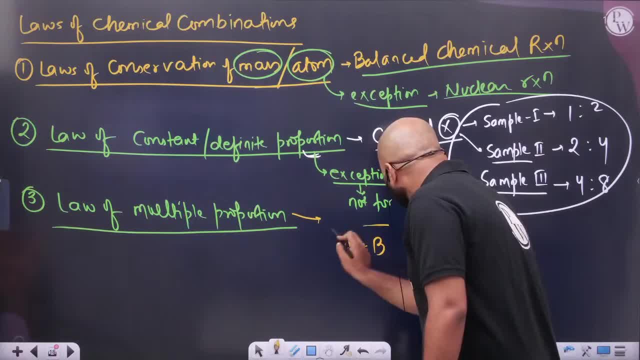 Look carefully If two elements. Look carefully If two elements, If two elements, If two elements, If we have two elements, Sir, if two or two elements, If we make more than one compound Brother, leave the whole story. Leave the whole story. What will be written in that statement? 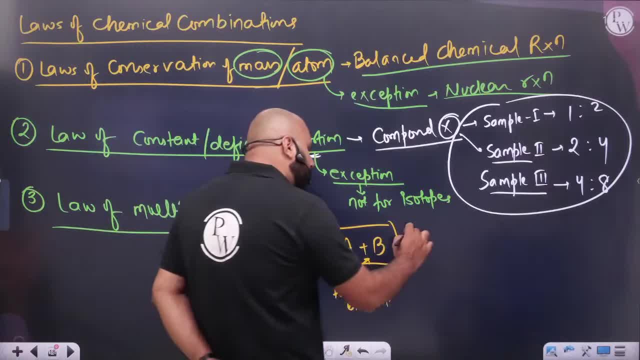 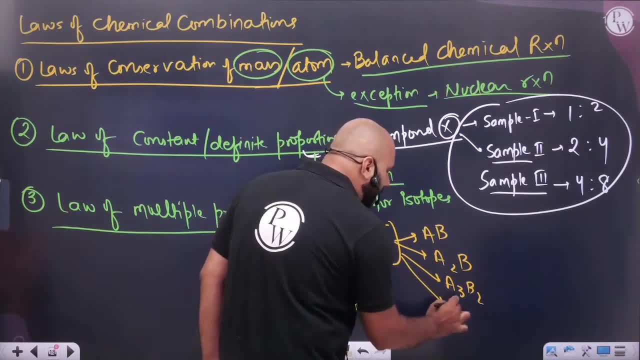 Just understand a basic language. If two elements, If we make more than one compound, It is also known like: If two elements make like AB, If two elements make A2B, If two elements make A3B, If two elements, If two elements make B2, Make anything. 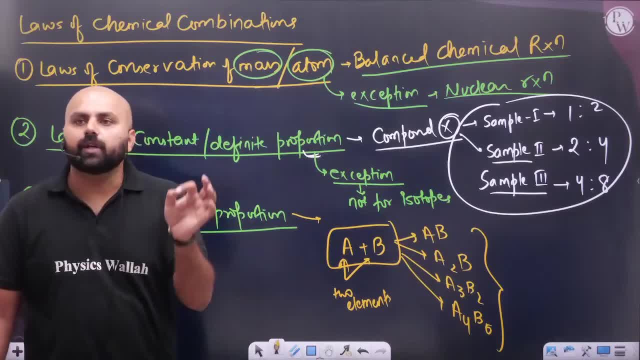 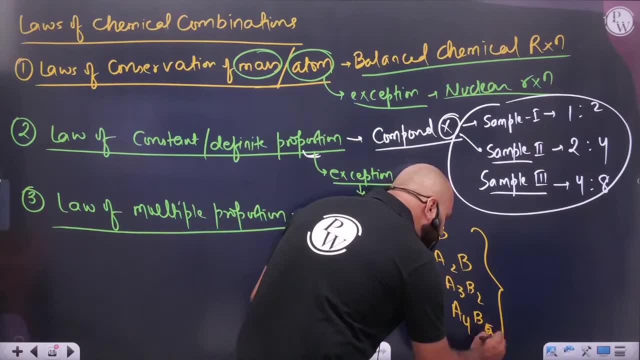 Sir, all these ratios, See, what is all? Whole number, ration, Means. What is the ratio of atoms? Whole number ratio, See this: One is to one, Two is to one, Three is to Two, Four to Six. Sir, this is all. Four is to five, Means It is possible. 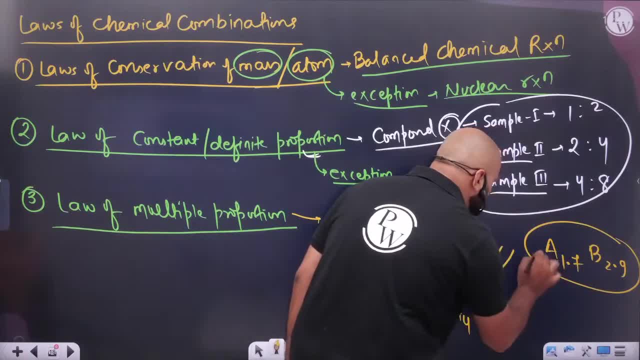 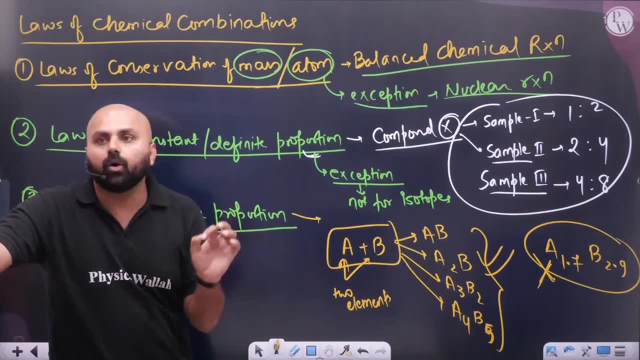 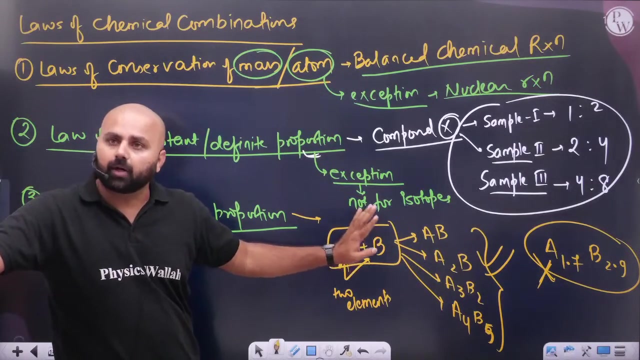 But it can never happen That you get this. This can never happen. This can never be made, brother. this can never be made. this ratio will never come. this ratio will never come. keep this in mind. law of chemical composition. law of chemical composition. you will get the notes in the morning, brother. you look at yourself. tough chapters will not come in the last. my energy is maintained. you look at yourself, brother. okay, okay, look at yourself according to yourself. how to read: you have to read, then sit, otherwise okay. your comment: those who are reading. please, brother, when I say the question will come, then you have to come to the comment section. those who are reading. please turn off the comment section, because it is very important. 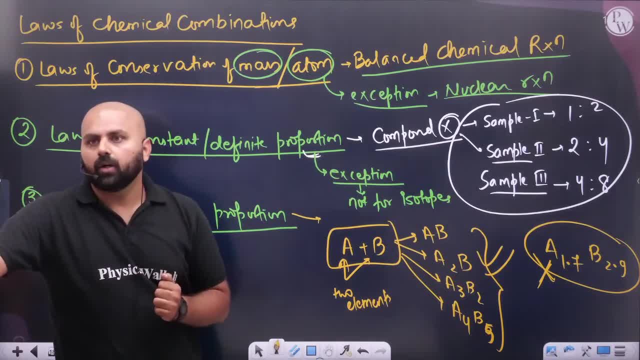 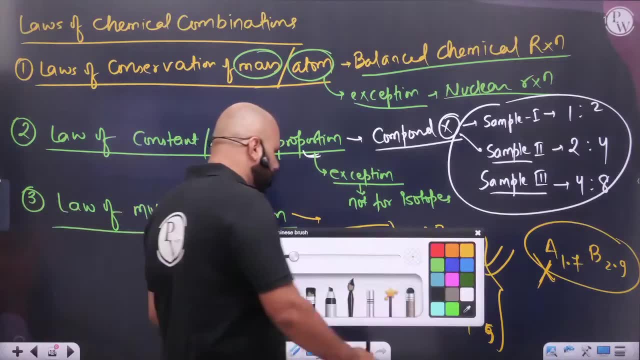 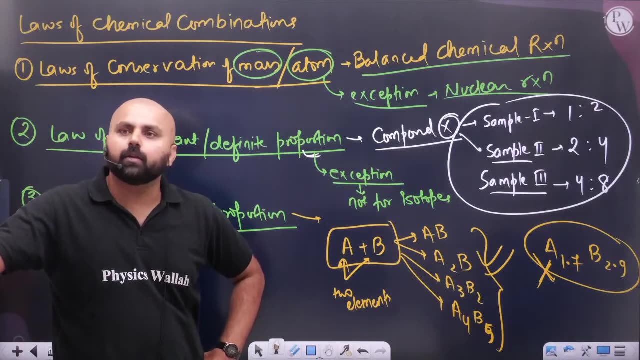 There are a lot of people sitting, okay, so they have come. so let them come, okay. yes, those who are reading. look at yourself quietly, keep revising, keep turning your copy side by side, keep trying, okay, that? yes, brother, they like that thing. they like to do it all day, so let them do it okay. one person is writing- I am just looking at him in the day. there is only one comment, sir, make it a little fast, make it a little fast. he will not understand anything. he just has to write one message. he will get the money for that. go, brother, just write this, just write this, just write this. he does not even know. 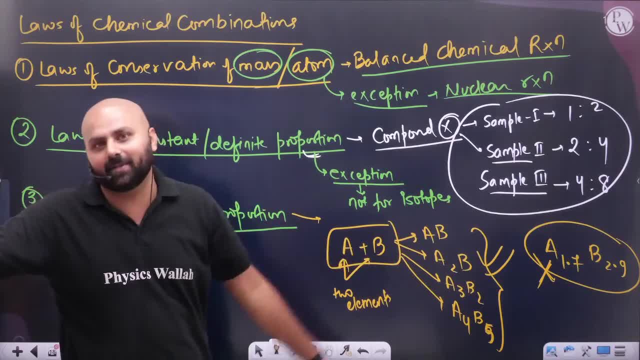 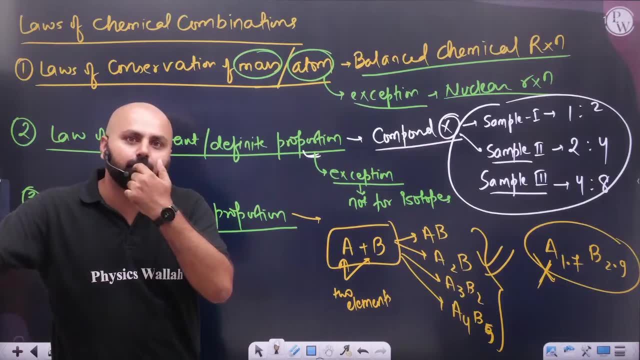 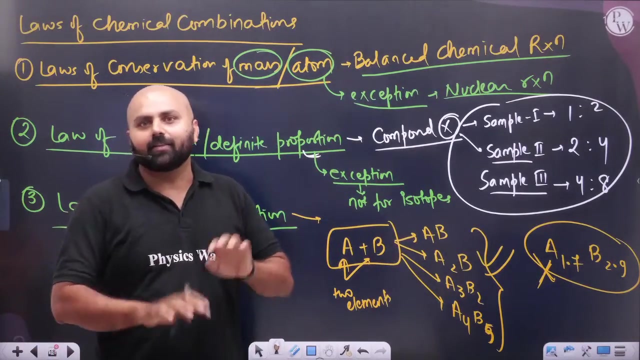 okay, brother, what is so important teacher is giving. why is he giving? I am telling you the reason for that: because the questions have not come, and if they have not come, then they can come. brother, as far as I am concerned, we will do it. you are sitting because you have to sit. you have to finish the chapter, you have to do revision. whatever work you do in two or three days, you have to do it with the head for one day. okay, yes, it has no meaning. from the beginning I have been putting the message continuously, from 2 o'clock to 10 minutes. just fast, fast, fast, fast, fast. nothing comes, but now a little fast. it is going on like this: 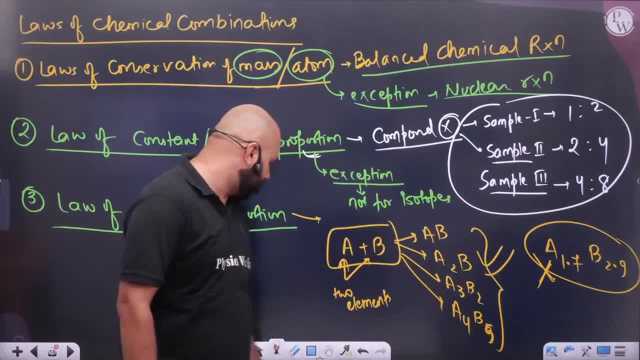 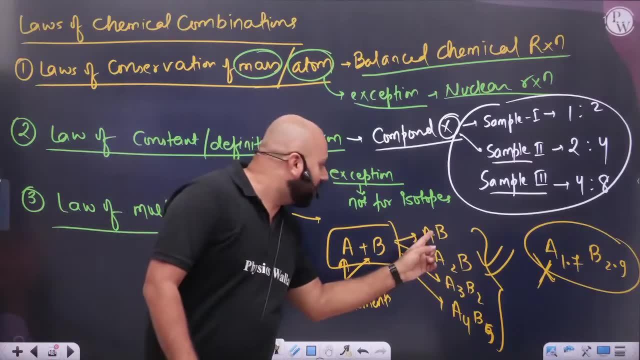 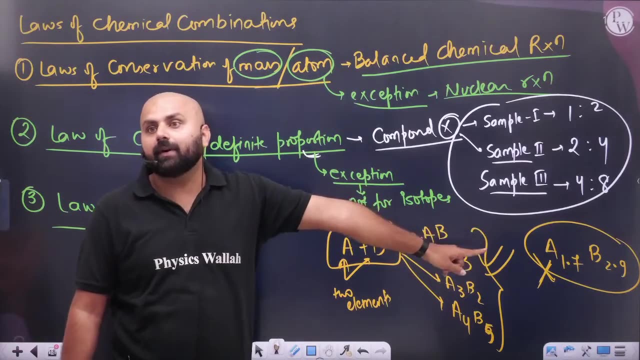 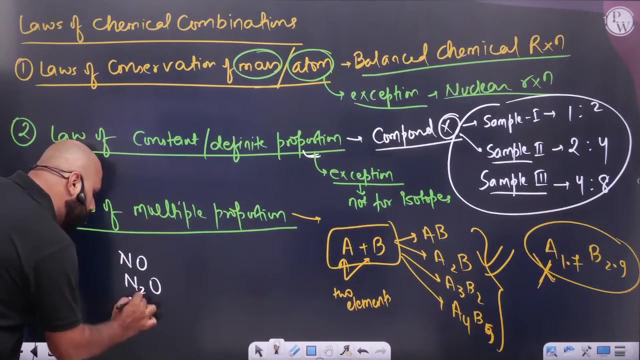 a little fast. hey, read it, brother, ask this question. look at yourself. I am talking about AB. I am talking about AB, okay, yes, I am talking about AB. okay, that what happens to AB. anytime a compound becomes such a compound, don't understand whose violation is it? whose violation is it law of multiple proportion? whose violation is it law of multiple proportion, like I give you this compound? see this, sir. this is NO, this is N2O, this is N2O3, who is this following? this is following the law of multiple proportion. 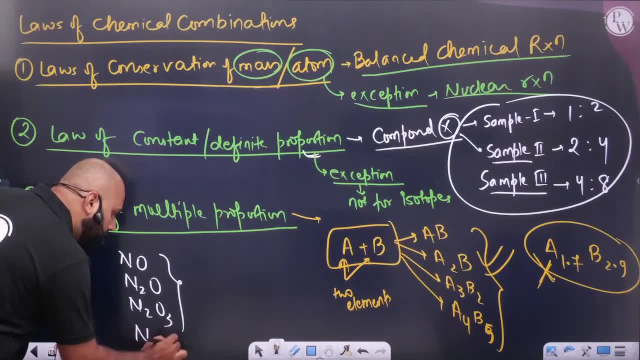 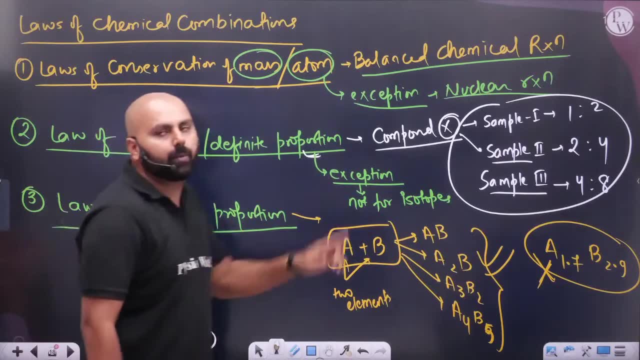 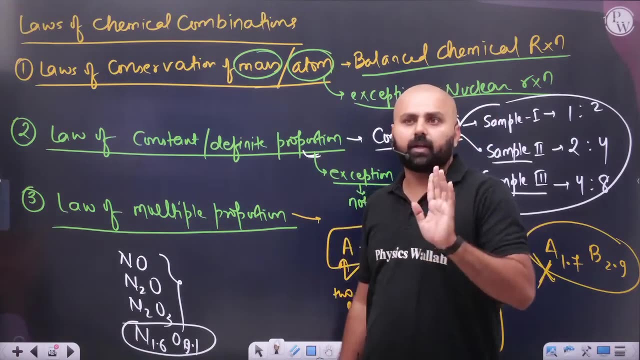 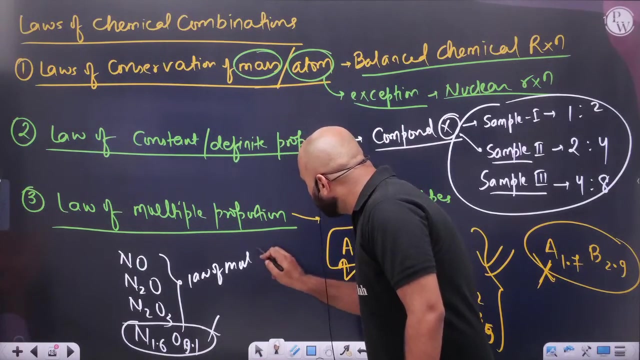 but if I write an example here: 1.6, oxygen, 9.1,. write like this: sir, who will not follow this law of multiple proportion will not follow this law of multiple proportion will not follow. keep this in mind, okay, keep this in mind, okay. this law of multiple proportion, who is this following law of multiple proportion? just a simple thing. reciprocal proportion is not in NCERT at the time. there is no need to read it. 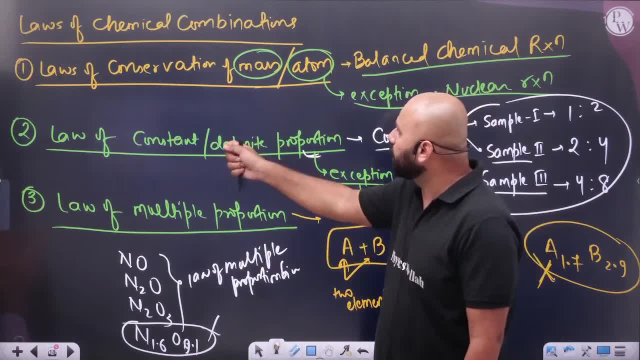 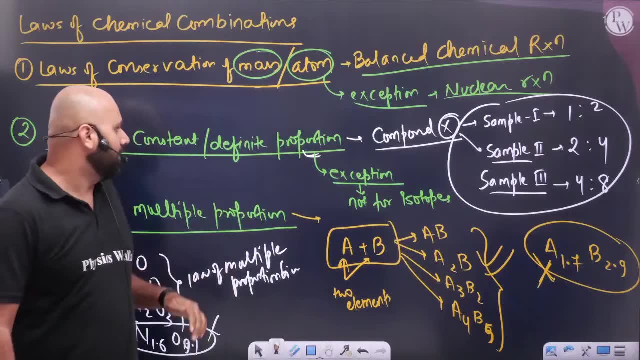 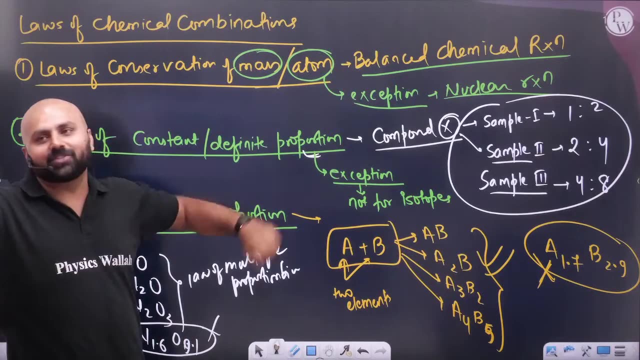 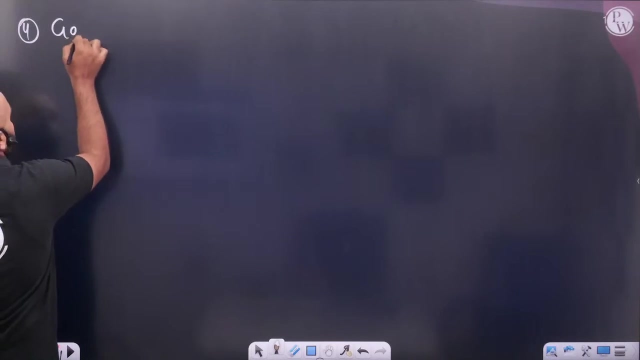 but yes, you just need to know this. multiple, constant conservation of mass. these three laws should be well known. okay, you don't get 300 rupees per comment, brother? okay, yes, we know the rate. okay, so I was saying this law of multiple proportion, law of constant proportion, law of definite proportion, all these things are clear. after that, two more laws come. two more laws come. those are with us. Geluzax law. what does Geluzax law say, brother? what does Geluzax law say? Geluzax of? 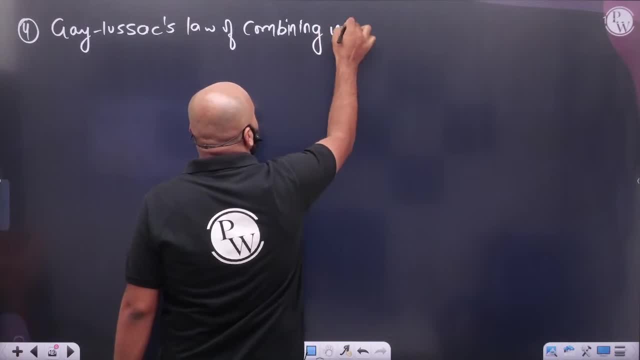 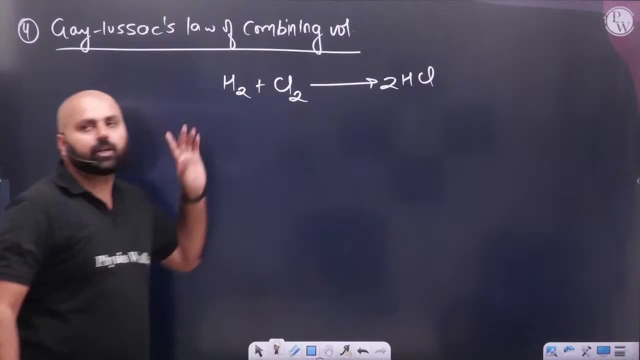 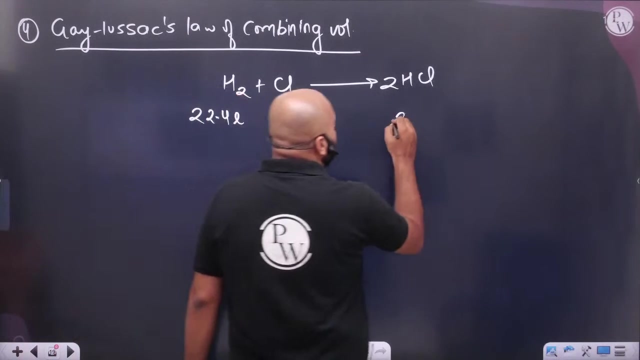 combining volume. that, brother, if you see the ratio of volume, if in any reaction, if there is any reaction, H2 plus Cl2, 2 HCl, then brother, if you see the ratio of volume, then that ratio, volume of ratio, don't take volume, brother, I am saying the ratio of volume. if you see the ratio of volume, then how much will it come, sir, 1 is to 1 is to 2,. 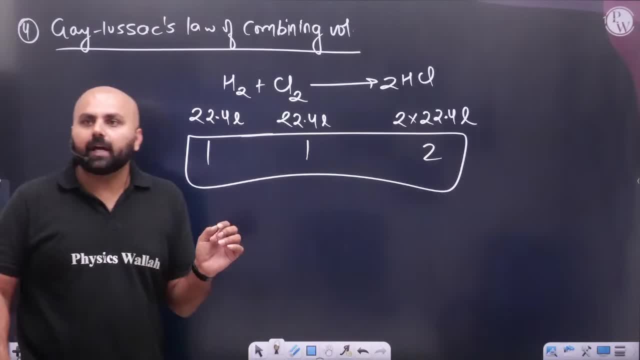 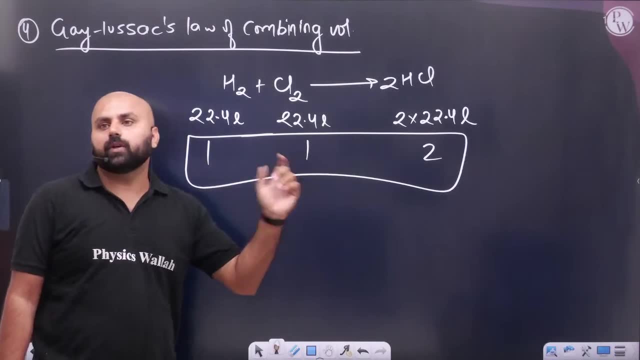 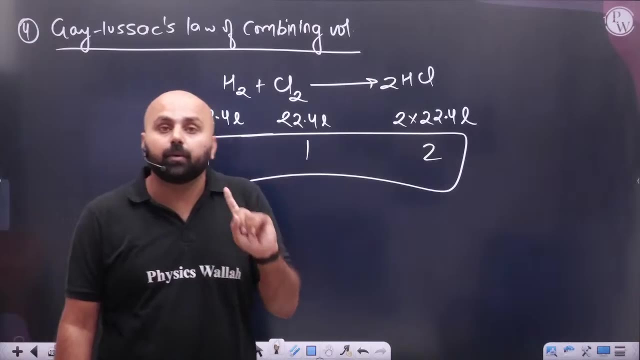 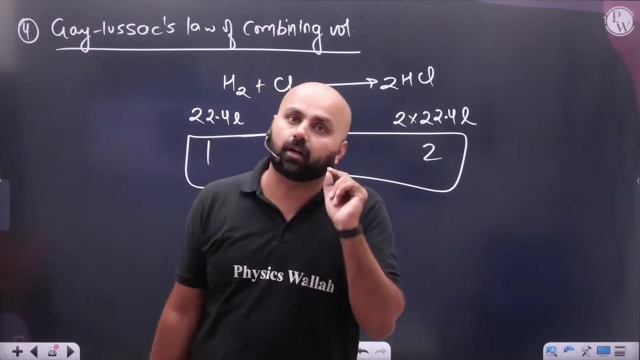 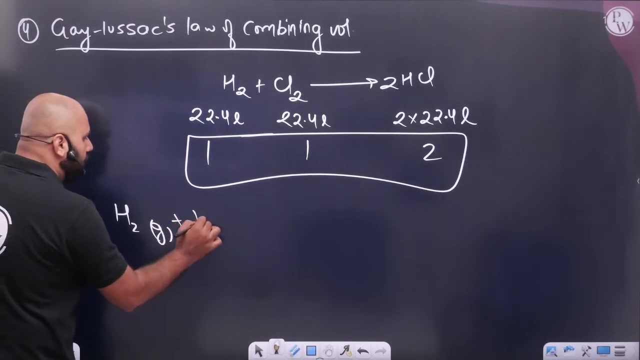 volume of ratio will also come in this, because as much as your reaction is balanced- look carefully- as much as the reaction is balanced in all of them, sir, whenever you take the ratio you will get- 1 is to 1 is to 2, in any case simple- according to which the ratio of volume will also work in the ratio of moles. that's why we never multiply by half in the reaction. we don't take half fraction. reason: the freedom to take half and fraction is only in chemistry, in thermochemistry. you can't write like this anywhere else, sir. tell you somewhere that sir H2 gas is there, write half O2 gas, you write H2, brother, this will be very dangerous. 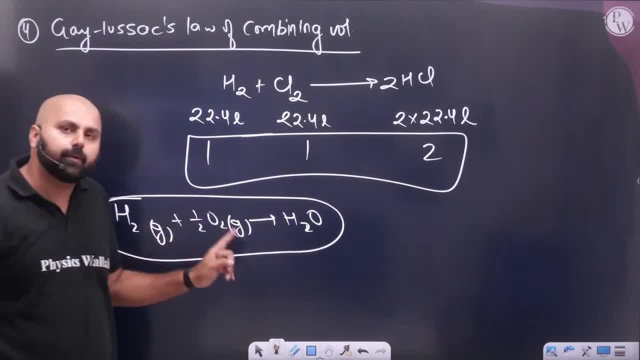 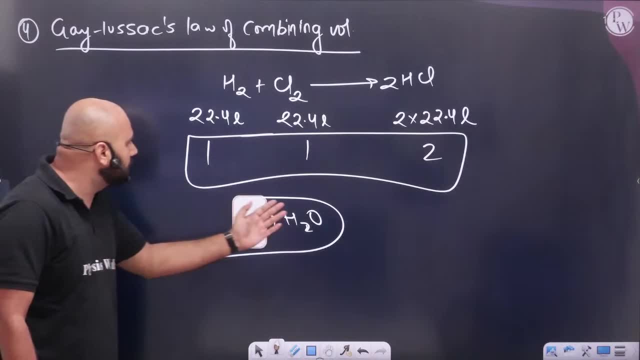 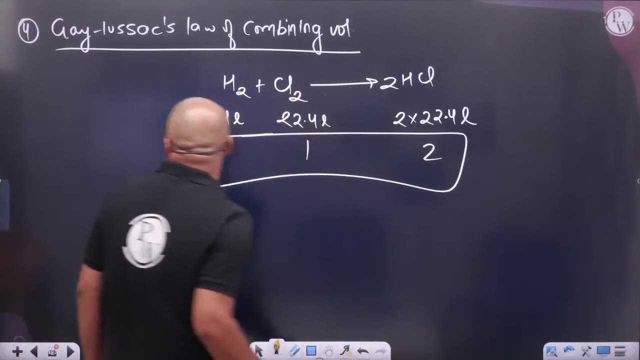 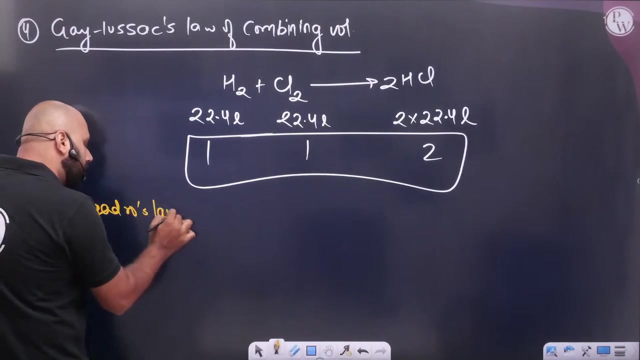 This is not valid. where can it be valid? this reaction can be valid only where the energy is, because what is energy? you can multiply and divide it. half of the molecule is not balanced in the reaction. that is why I am telling you, whenever the ratio of volume will come, it will come, in which ratio after that? after that, brother, brother, I have the last law. what was said F Gatrow's law? what was said F Gatrow's law? what is the F Gatrow's law? if the volume is equal, if the volume of gas is equivalent, then case A in it is the sample of rice, for example, outfall or downfall, it is the same because of the volume of skim corn which comes in the ratio of black rice. the same ratio. this is valid. if you look fully, you can see there is no, sir, if not the black. 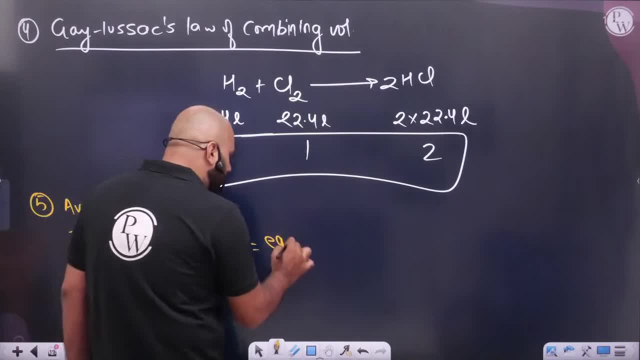 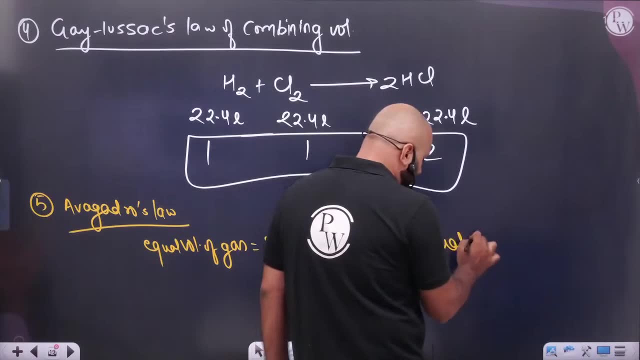 If volume is equal, then it means there will be equal moles of gases, And if there are equal moles, then there will be equal molecules. If there is equal volume, then there will be equal moles. There will be equal molecules. 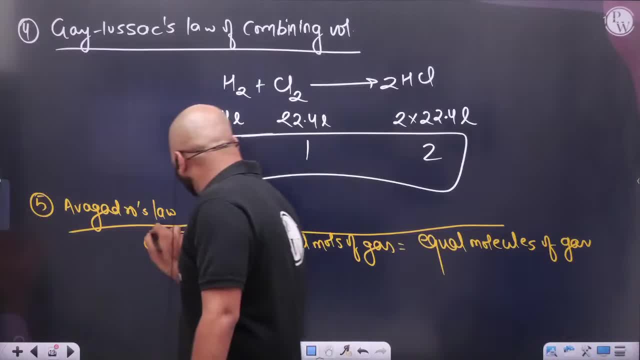 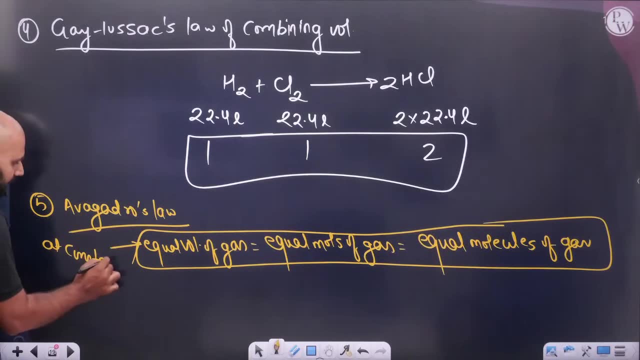 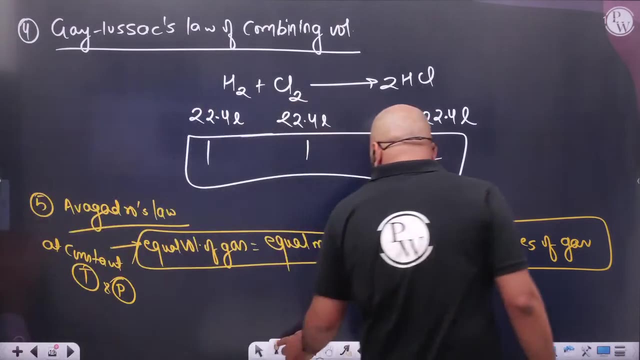 And, sir, this means now we can have look carefully at us when this at constant temperature and pressure, Go to any constant temperature and pressure, Go to any constant temperature and pressure. Equal volume means equal moles, equal molecules. Atom can be and can not be. 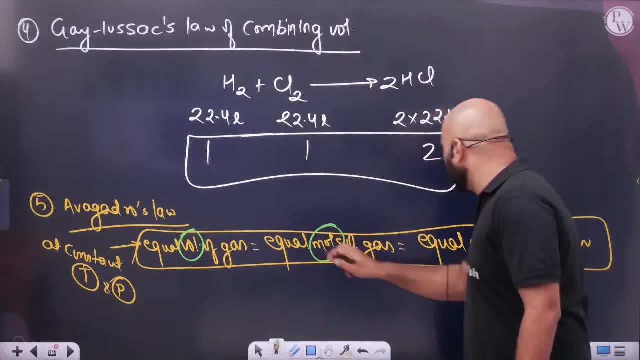 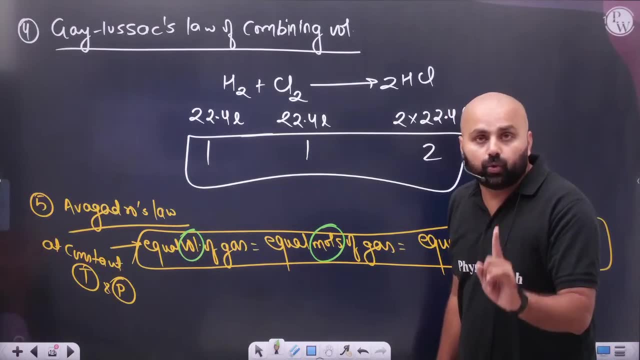 Remember: if volume is equal, then what will be equal? Moles will be equal And whose will be? Molecules will be equal. These last two laws that we have told for whom are they valid? These last two laws that we have told for whom are they valid. 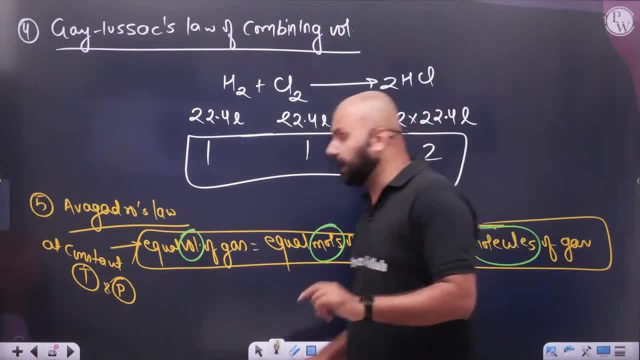 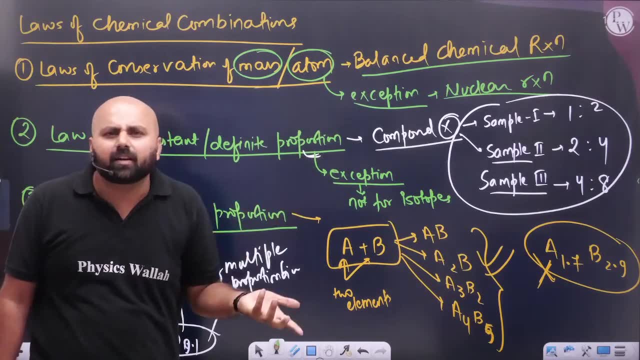 For gas. Remember: these last two laws are for gas. Look at this, brother. Look here we have these. normal for any compound. These are for any compound. We were not even talking about gas and liquid. The first three laws are general for everyone. 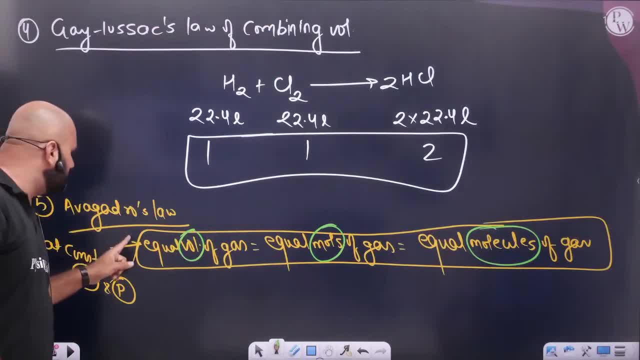 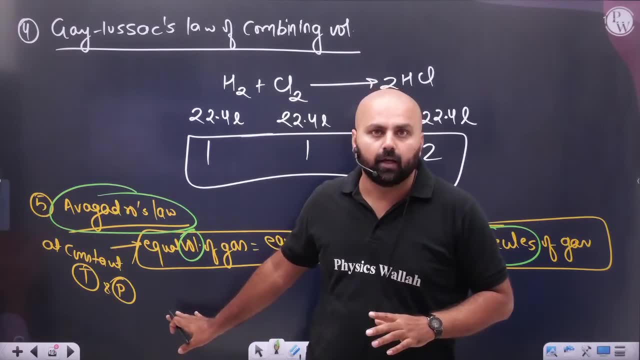 But the next two laws, Gay-Lussac's law and Gay-Vegadro's law? for whom are they? for, Sir? for whom are all of them valid? All of them are for this. For whom? For gases? Are you sure? 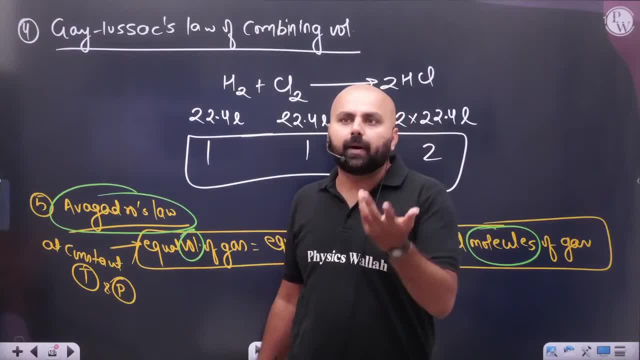 So these will be the laws. Come on, do the question Now, when you have done the laws. there are five laws. Son law of reciprocal proportion is not in our syllabus. that's why we don't have to study. 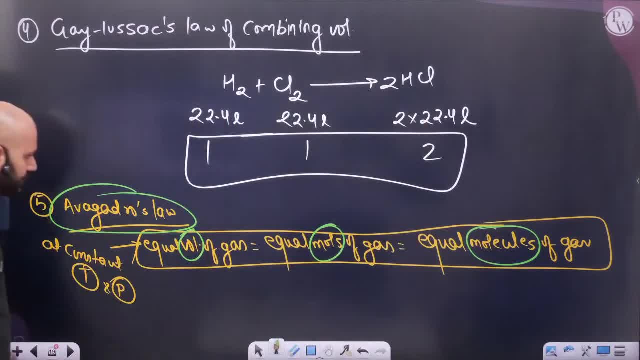 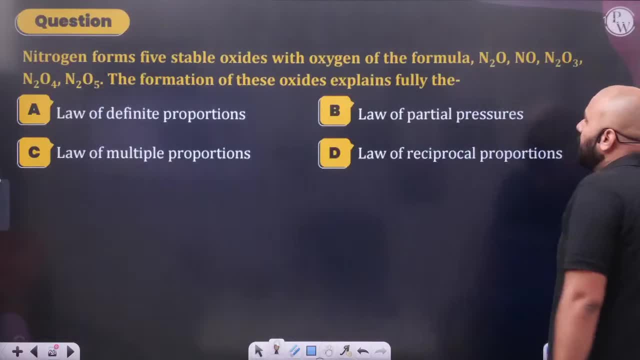 Okay, now look at yourself. See this. whenever you get a question like this, question was given. What will happen, Sir? close your eyes and answer directly. What do you have to think? in this, Nitrogen is becoming a different oxide. 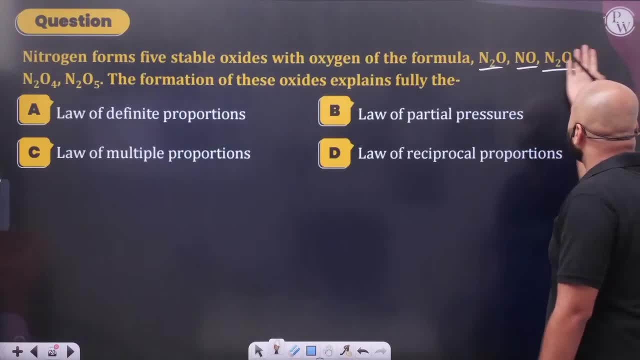 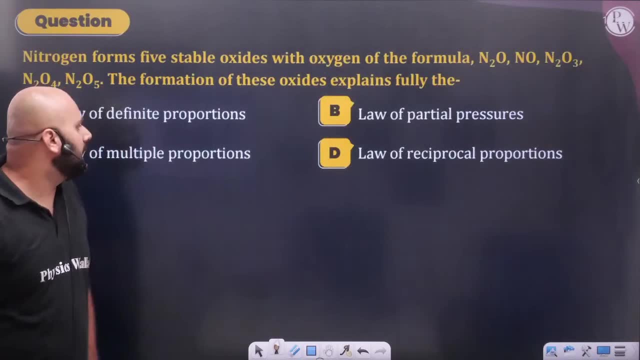 What is the ratio of all? Is the whole number visible? What is the ratio of all? Is the whole number visible? What is the ratio of all? Is the whole number visible? And when the whole number is visible, then what will be the answer? 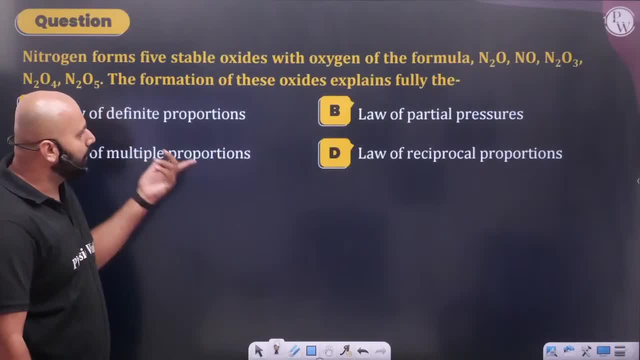 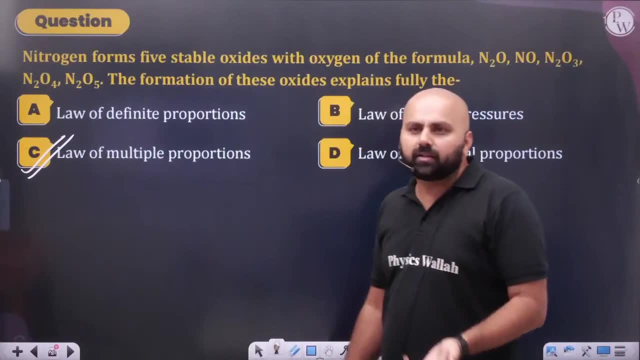 Sir, law of multiple proportion. There is a definite proportion. there is no logic. There is a law of partial pressure. there is a law of Dalton's law. It won't happen here, Sir. reciprocal proportion- If someone thinks that it is reciprocal proportion. 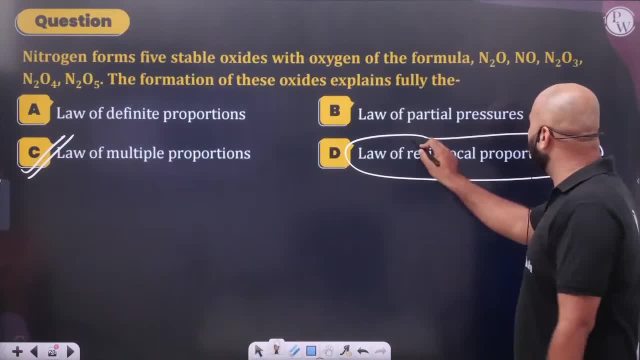 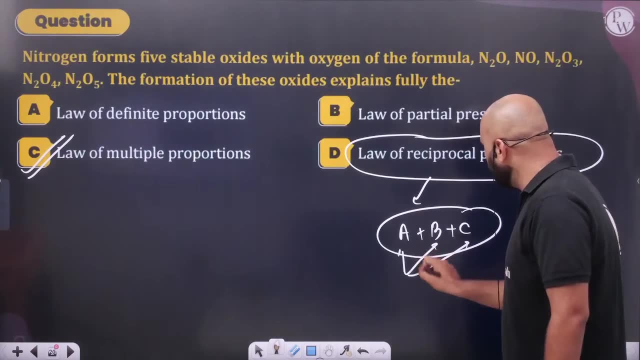 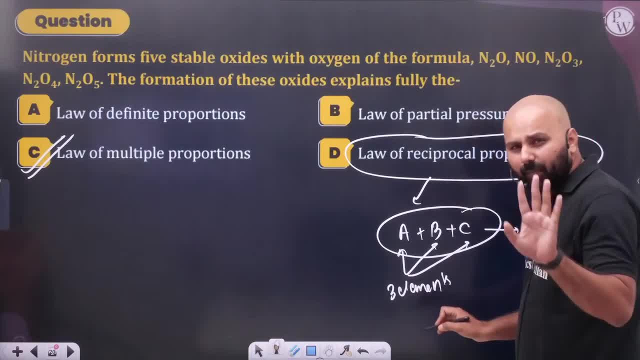 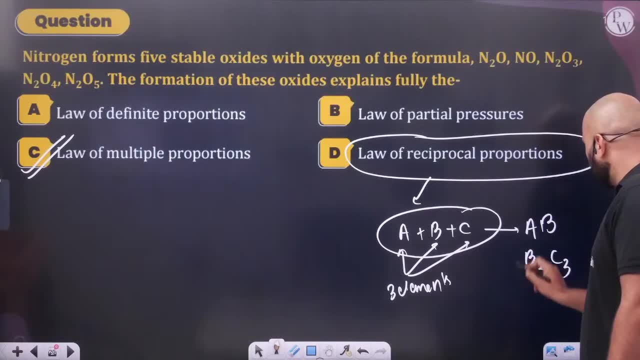 And in between them. if you are afraid in the exam hall, let me tell you a simple way to remember. One compound should be in between A and B. Second compound should be in between B2 and C3.. And the third compound should be like this: 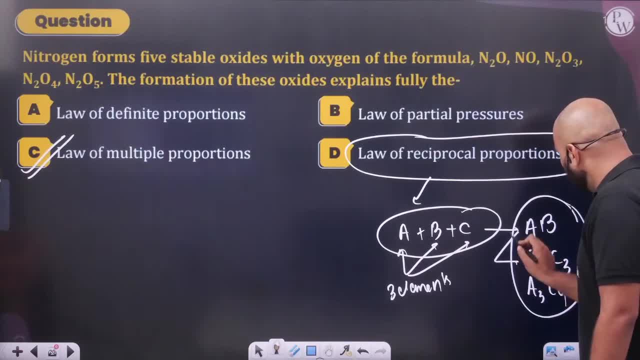 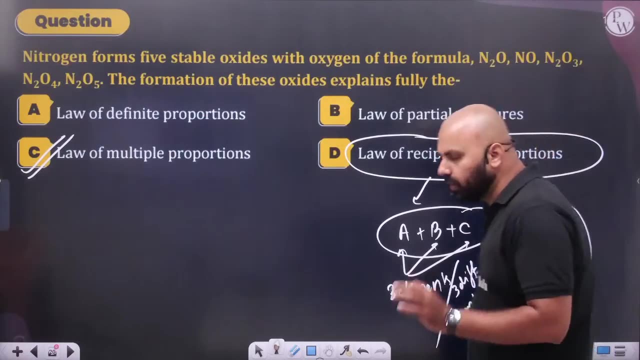 There should be three elements and three, three, three. there should be different compounds, between different compounds. That's it, Close your eyes. between A, B and C. That's it, Close your eyes and follow these two conditions. This is called the law of definite proportion. 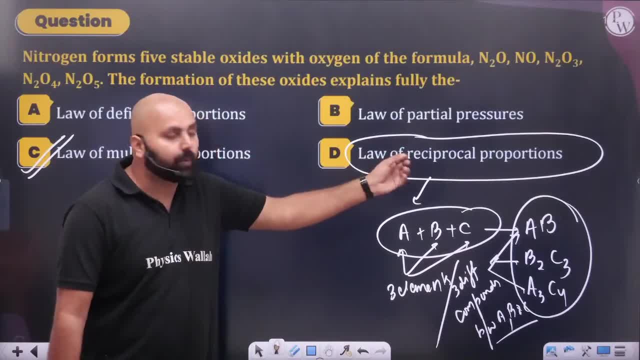 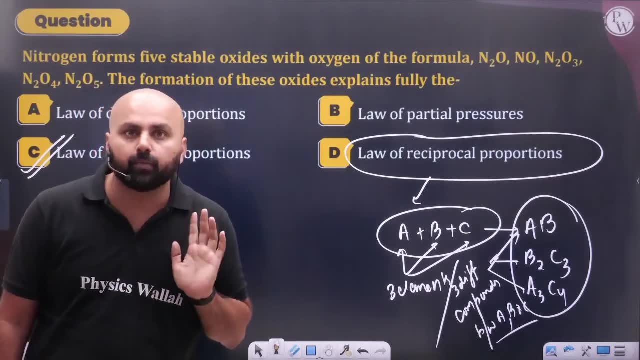 Don't do anything else In the law of definite reciprocal proportion, in the law of reciprocal proportion. don't know more than this, because it is not in your syllabus. Okay, it is not in your syllabus, So just know this much. 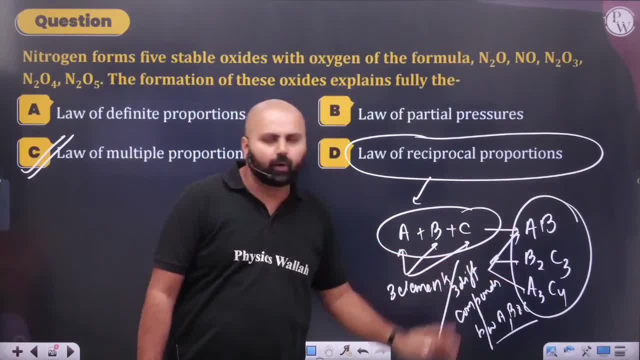 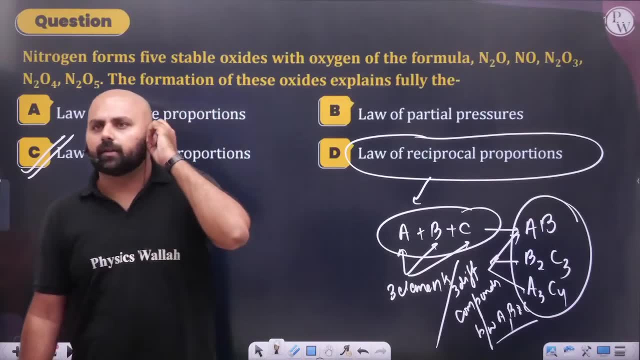 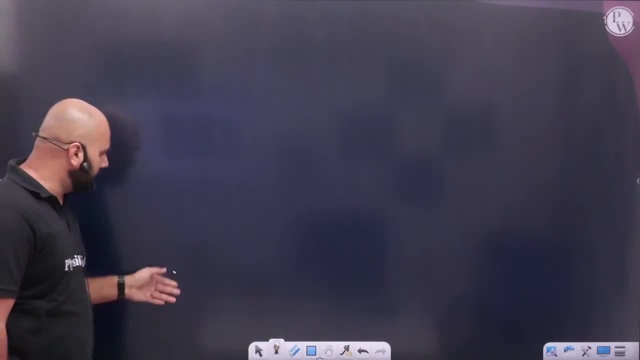 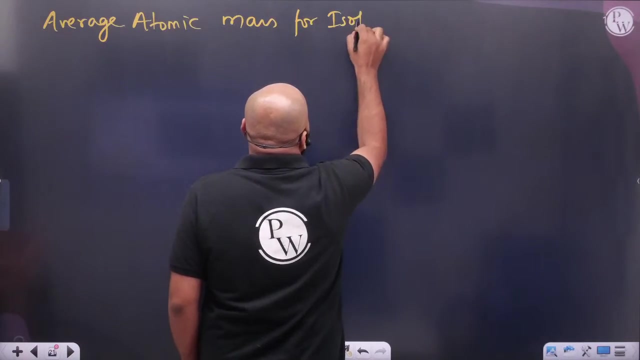 There should be three elements and there should be a compound. There should be a compound. close your eyes about them. it's done, no problem, okay. close your eyes about them, no problem, okay. second thing, sir, if we talk about laws, then talk about laws after that. after that, see, son, laws are done. after that, two more concepts come. one comes, the concept of mango. for whom average atomic mass brother? I will tell you a simple thing. for whom? for isotopes. in the case of isotopes, sir, 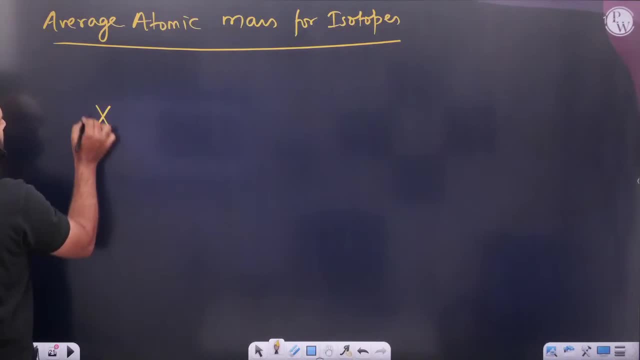 if someone says: remember one thing: if there is any element, see this, I will tell you a good statement. this is my sorry, it turned upside down. what happened, this is with us. z. what happened? a sir, what is this number of protons? what is this number of protons? what is this proton plus neutrons, or what is this called mass number? and what happens atomic number? I will write a line. see carefully that, sir, whether number of electron, proton, whether neutron, 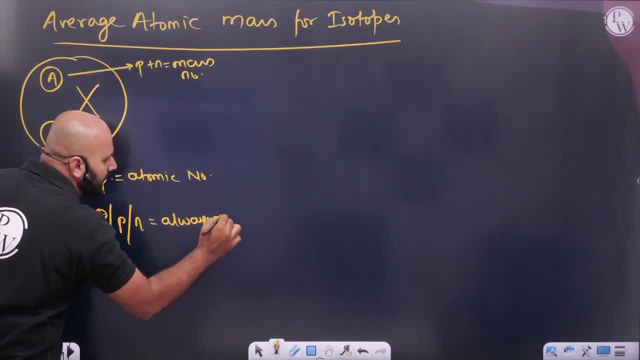 always a whole number. this will never be half complete. this statement is small, small statements, but exam hall can be asked: atomic number or mass number? atomic number and mass number? atomic number and mass number- what will always be? always whole number? somebody will say always. 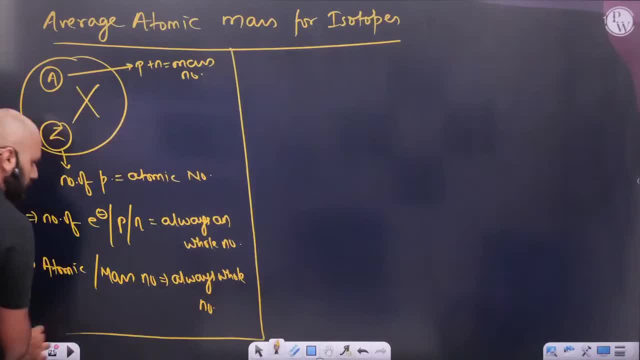 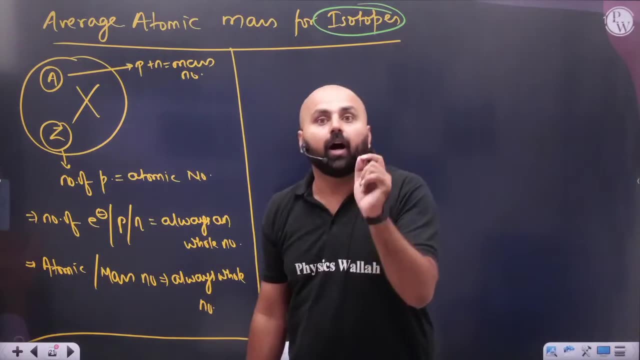 whole number. so, brother, why does this happen that you get chlorine mass thirty five point five? because what happens in that? isotopes? if someone has a mass in a fraction, if someone has a mass in a fraction, If someone's mass is in fraction, it means it will be an isotope. 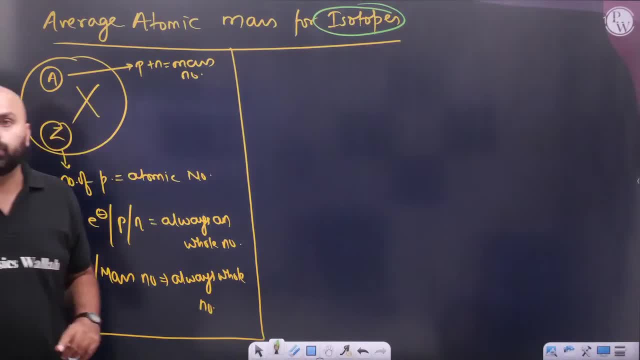 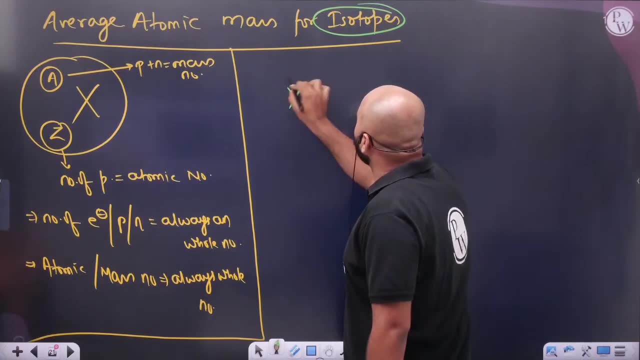 If someone's mass is in fraction, that means it will be an isotope, And if your mass is in fraction, then it will be an isotope. Suppose there is an element x. there are 2-3 isotopes of it. 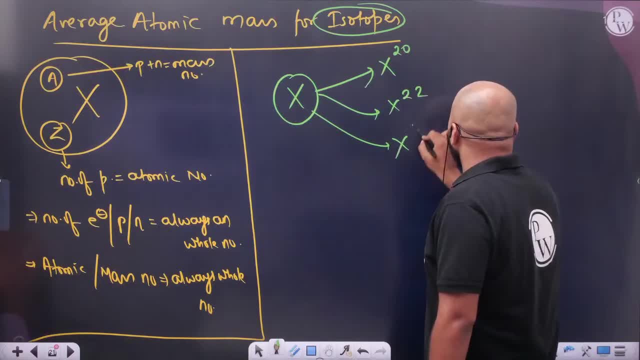 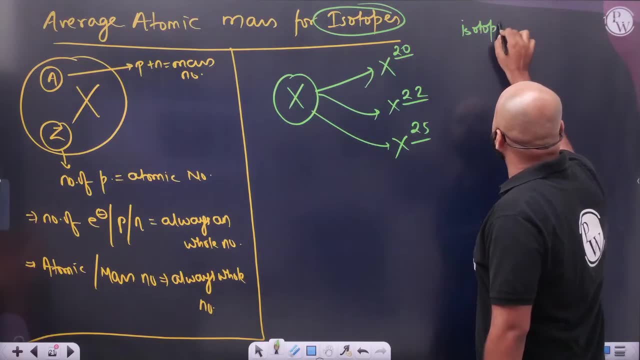 The value of x is 20,, the value of x is 22,. the value of x is 25.. Sir, if you have given isotopic mass above, what is its isotopic mass? See how it is taken out. The isotopic mass is given How much. 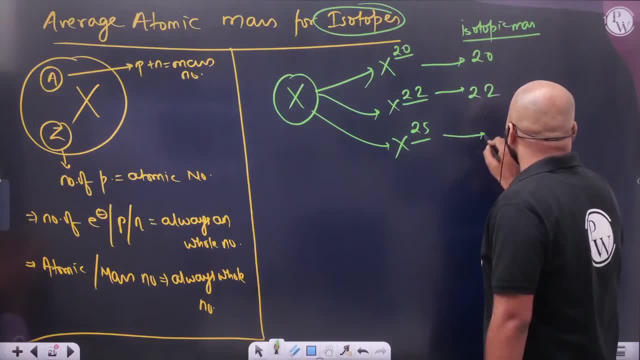 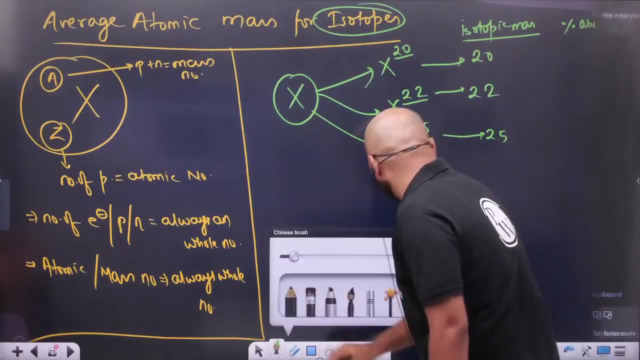 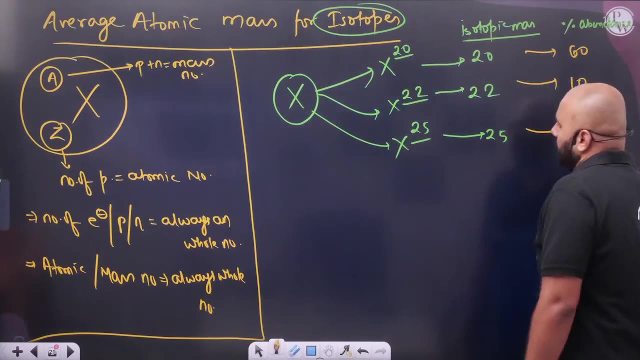 The value of its seed is 22,. the value of its seed is 25.. You just have to do one thing: You have to see the percentage abundance. Take out the percentage abundance, Percentage abundance. Suppose it has given 60%, 10% and 30%. 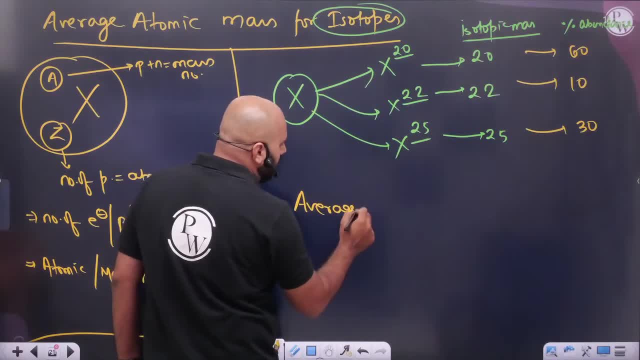 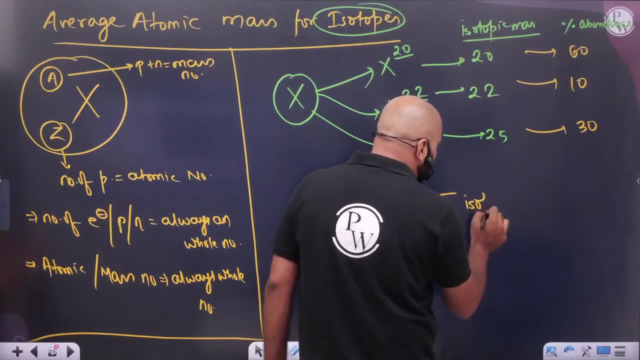 Nothing. Average atomic mass. If you talk about average atomic mass, then taking out the average atomic mass is the easiest thing. What do we do? The isotopic mass? With whom do we multiply the isotopic mass? Multiply it with its percentage abundance. 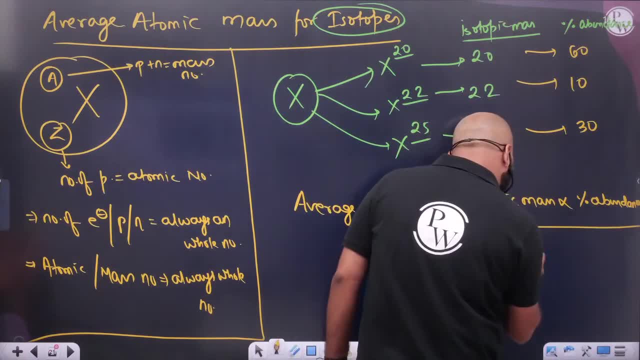 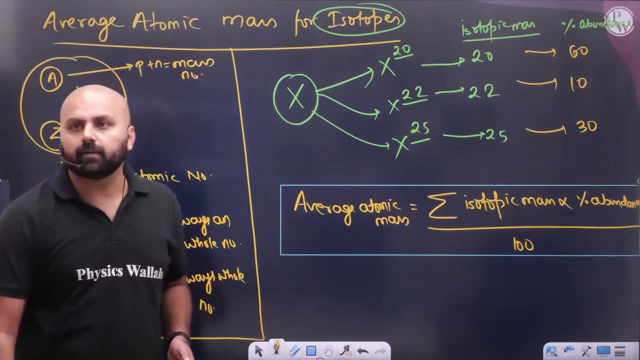 Multiply it with its percentage abundance. Divided by what do we have to do? 100.. Divided by what do we have to do? 100.. This is my formula. What do we have to do? We have the formula. 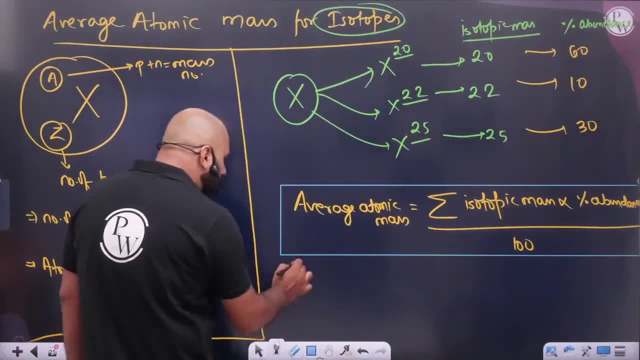 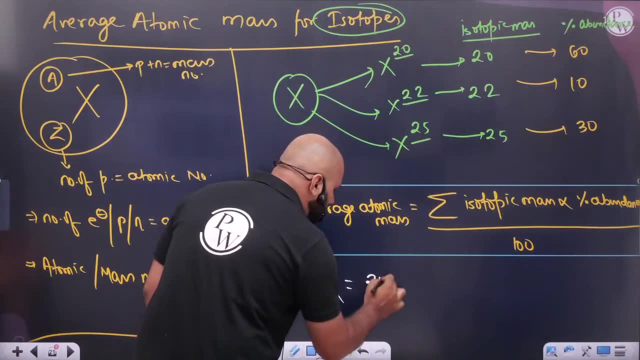 Sir, see what will happen. See what will happen. If I want to take out the average atomic mass of x, then what will be the average atomic mass of x? With whom do we multiply 20? With 60.. With whom do we multiply 20?? 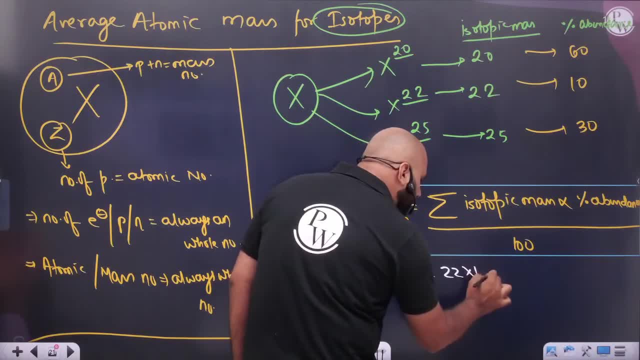 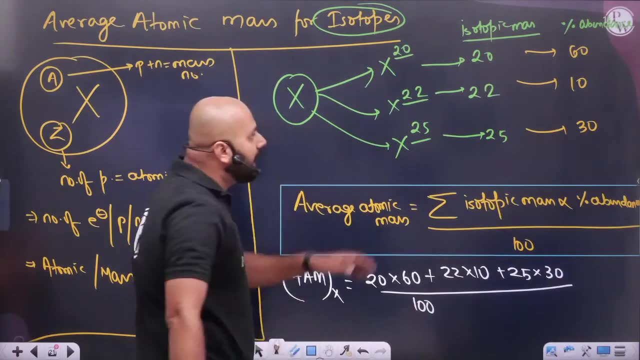 With 60.. With whom do we multiply 22? With 10.. And with whom do we multiply 25?? With 30.. Divided by what do we have to do? 100.. This concept can be used in the exam hall. 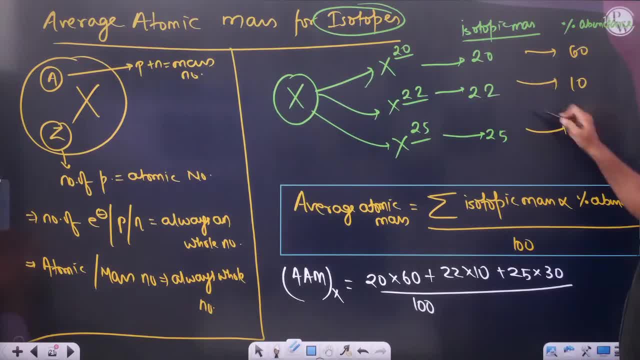 Let this concept disappear here. Give 20,, give 22,, but not 25.. So look in the exam hall: 60 and 10,, 70% is done. So how much is left? How much is left? 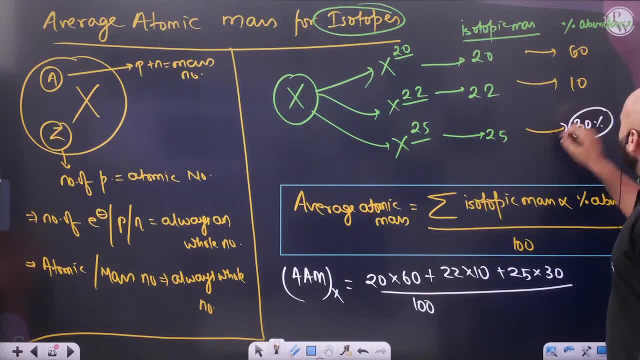 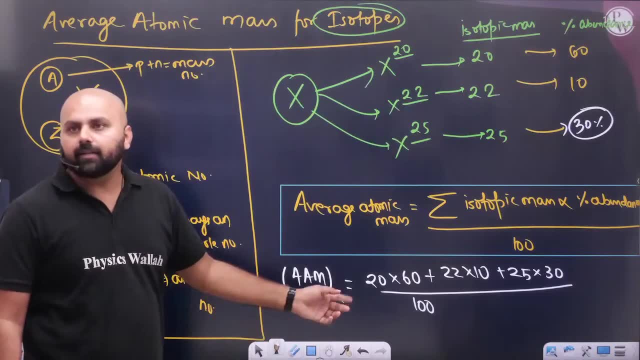 How much is left? 30%, Sir, if there is 100%, if 100% is the public, then from that sir see 60,, 10, and how much is that 30. Take out the answer and see. 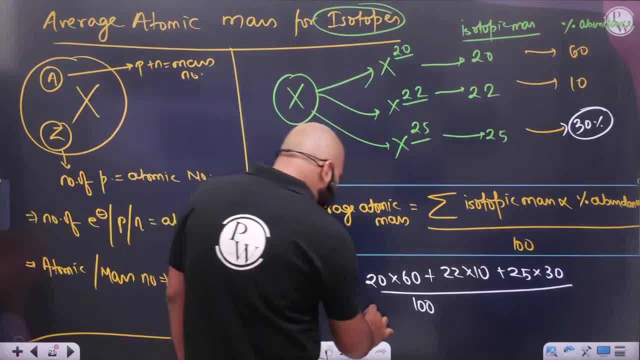 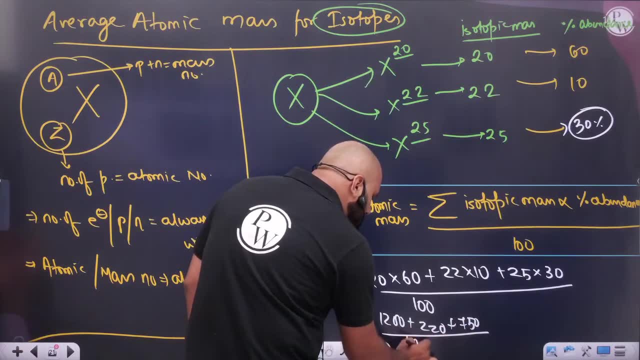 Take out the answer from here and see, Brother. these are the answers. these are the questions that will come. Why are you taking tension, Brother? now just revise all these things. Those who think: oh sir, this is very easy. 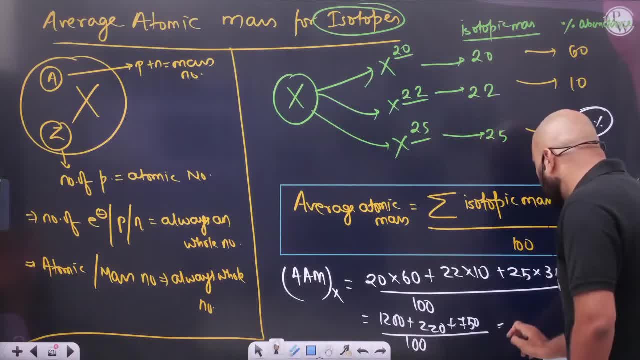 This is what you will get in the exam hall. You will get it in the exam hall. This is 220.. How much is it? 70. And 7 to 9,, 9 to 11.. And how much is this? 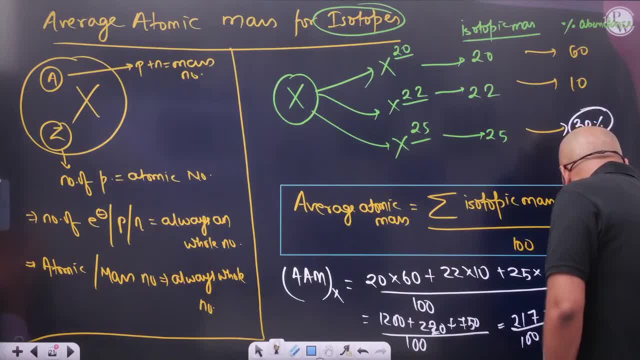 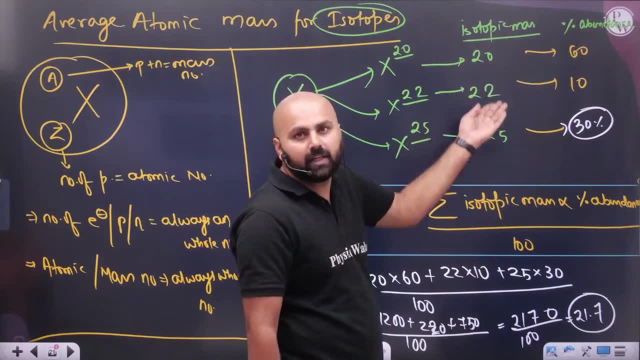 Take out the answer. How much will come? How much will come 21.7.. 21.7.. Okay, Why will you give mass instead of abundance? Brother, mass has already given its isotopic mass. Isotopic mass has been given. 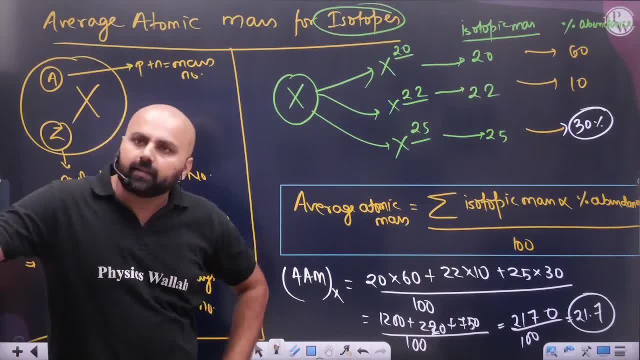 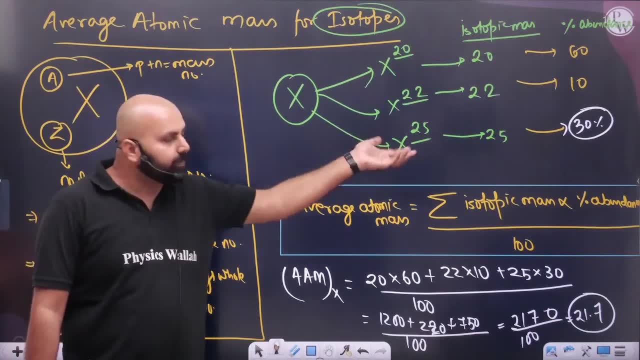 You will have to give isotopic mass, Okay. So, yes, do it like that, No problem, It is your choice, You do as you like. Okay After that. after that, Sir, it is easiest if you give such a question. 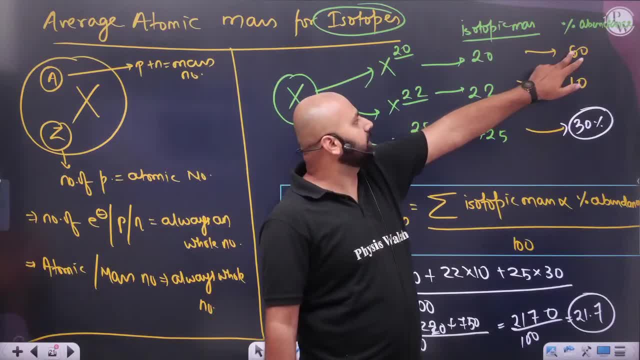 Okay, one or two questions are also like this. Suppose there are only two people, So you have to take its percentage x. What will be the percentage of the other 100 minus x? Take one percentage x, What will happen to the other? 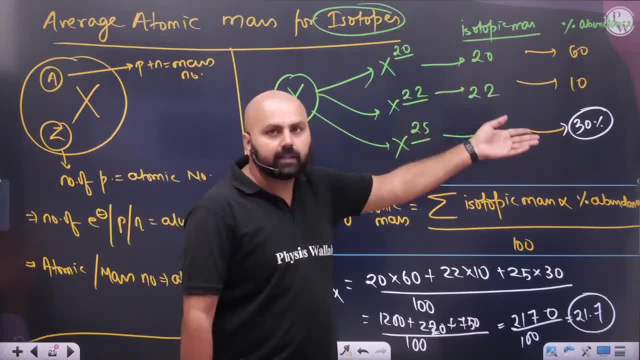 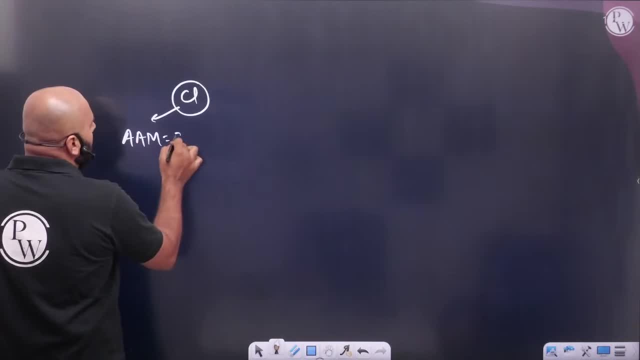 Take 100 minus x. If there are only two people, then take any one percentage, Like the famous example, is chlorine. What happens in chlorine, Sir? the average atomic mass of chlorine, if you see the value of mango, how much is the? average atomic mass: 35.5.. Chlorine has two isotopes: One is 35 and chlorine has 37.. Someone said, sir, tell me the percentage abundance, Tell me the percentage abundance, How much of this will be, and how much of this will be. 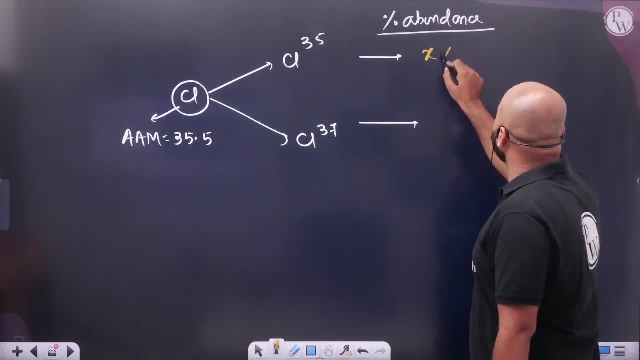 Nothing. You just have to do this much in the exam hall. Take its x, And how much of this will be, Sir? if you don't know, then take any one x. How much of the other will be 100 minus x. 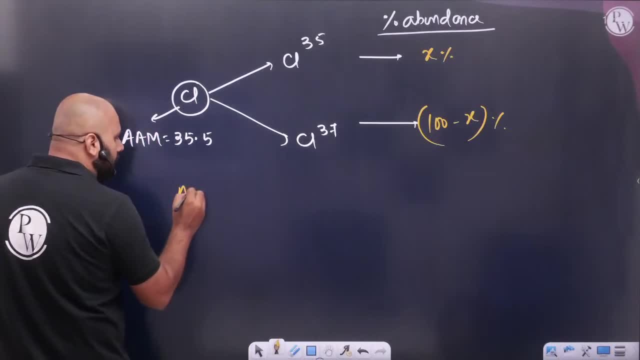 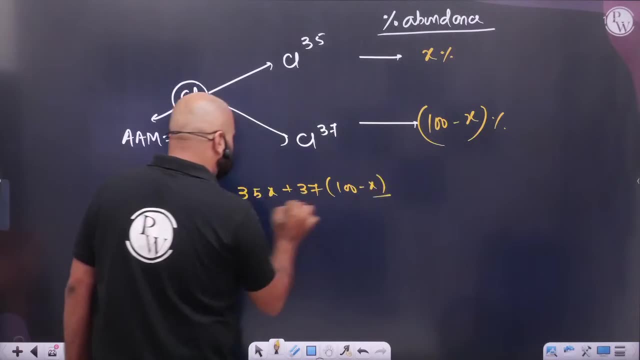 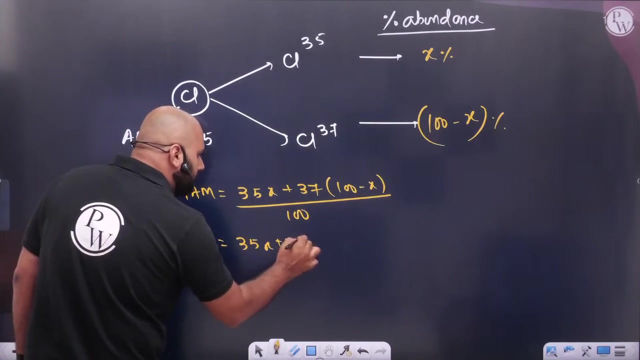 Okay, And see this: what will be the formula of average atomic mass, Sir, 35 into x plus 37 into 100 minus x, divided by how much will be 100.. How much is this? 35.5 is equal to 35 x plus 37 hundred minus 37 x divided by 100. 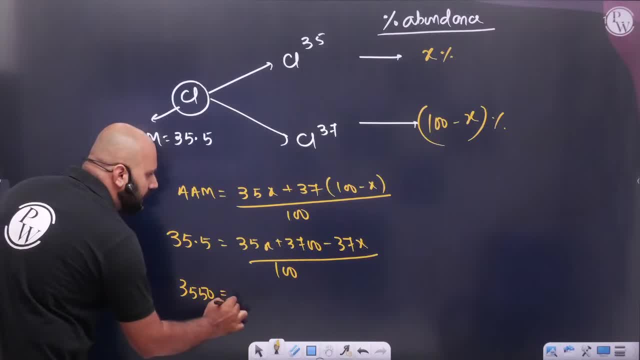 It will come here. If you solve it, it will be solved 37 hundred minus 2 x. If you go to get the value of x, how much will it be? 75 percent? 150 will be 75 percent. 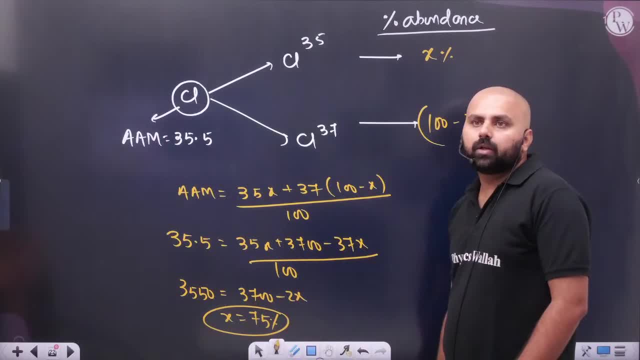 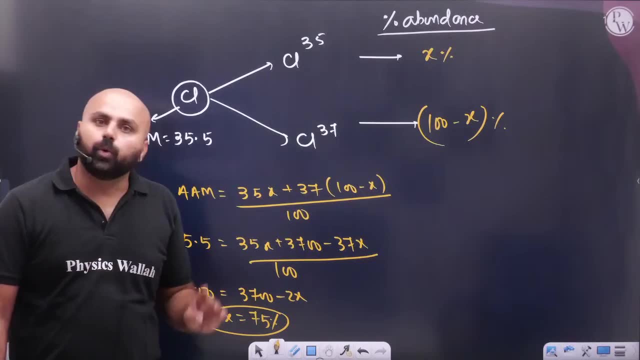 And how much will it be? 25 percent. Keep doing it, No problem. Okay, So you must be getting such questions. Keep doing it, It will be done. Now you people attempt the next question, Because the next question is a good one. 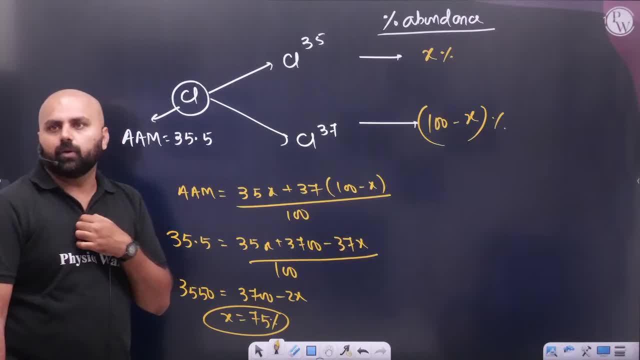 The next question is a good one. It is a good question. Try it. See the percentage abundance. If you have not given the percentage abundance, it will not work like this. If you have not given the abundance, then its value. Two out of three things must have been given, right. 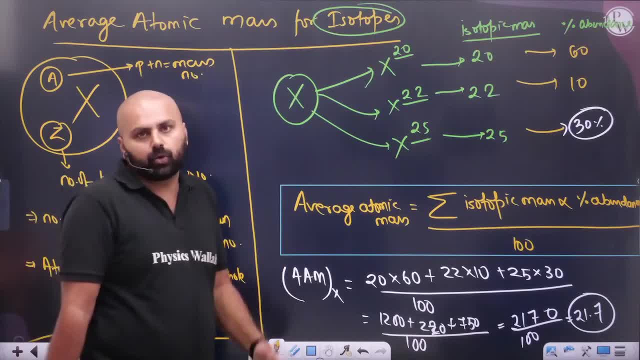 Some two things Now. it is not like that. If you do not give everything, then it will not be fun to take it in the exam hall. Everything must have been given. It will not be like this: Yes, one or two things will be missing. 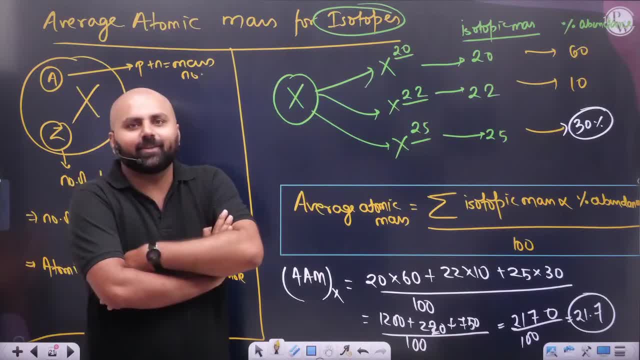 Take that out Now in the exam hall. he is saying that I will give the answer. Tell me the question. It does not happen like this. The NTU people will not joke like this. Okay, Come on, Look at this. 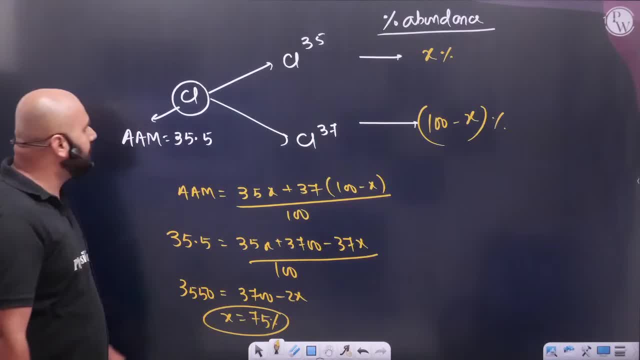 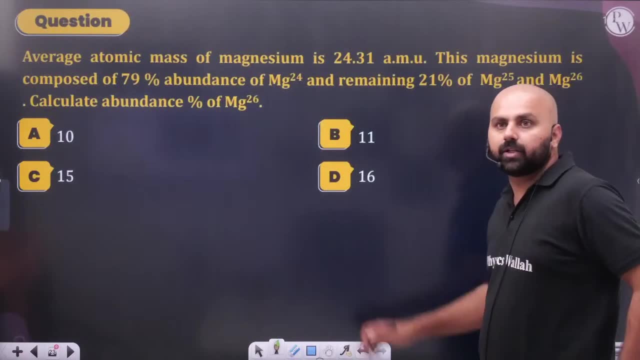 Now look at the percentage abundance. Now do a good question. Try to attempt this. Try to attempt this question. Sir, I have brought so many topics and so many questions. I am trying to do it together Quickly. The first chapter is very simple. 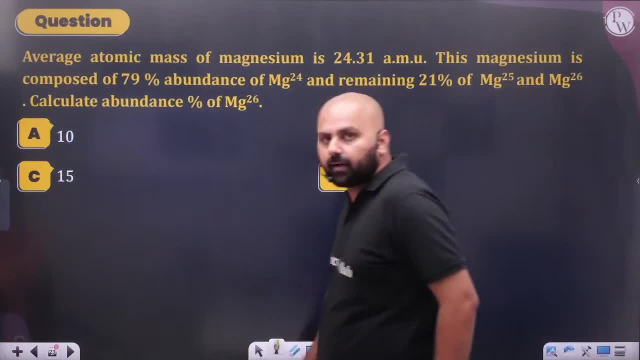 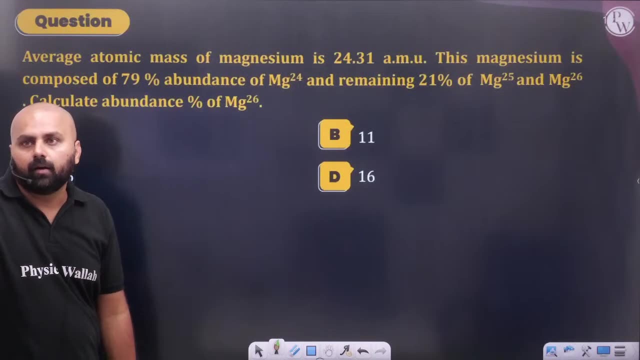 That is why we are tensed. The first chapter is done. In this, the state of matter is half covered. That is why we do not get tensed Quickly. What will happen? Tell me about this. What will happen Quickly? 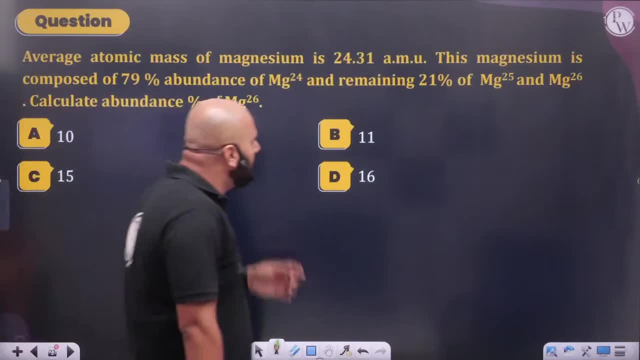 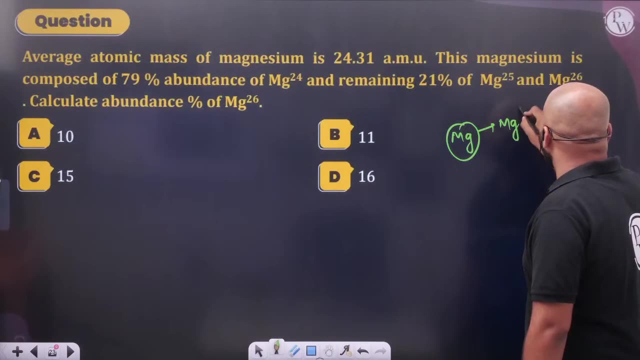 Take it out. What is he saying? The atomic mass of magnesium is given 24.31.. He is saying that there are three isotopes of magnesium. Look at yourself. If I want to make an exam hall, I will make it like this. 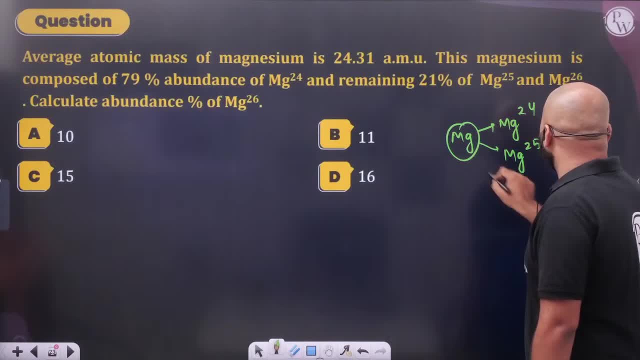 24.. Magnesium 25. And magnesium 26.. What will I do? I will do these two. The percentage abundance of 24 is given. These people do not know, Sir, what is he saying. I will take out the value of this. 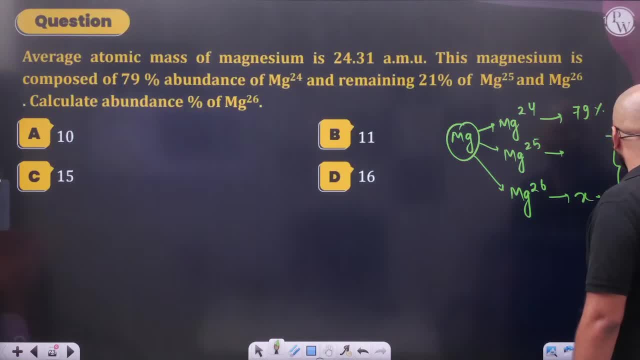 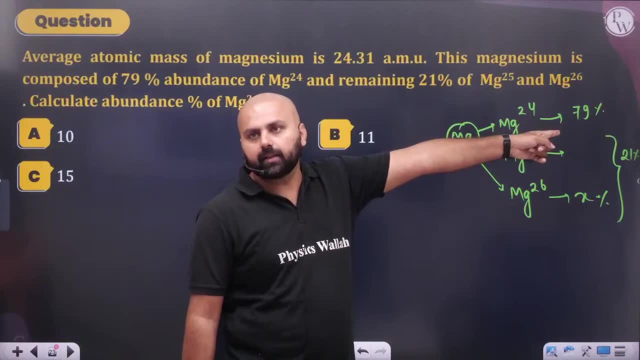 X. How much will it be by combining these two? 21 percent. How, Sir? how much should be the total? 100.. How much is a person alone in 100?? 79 percent, How much is alone? How much is alone? 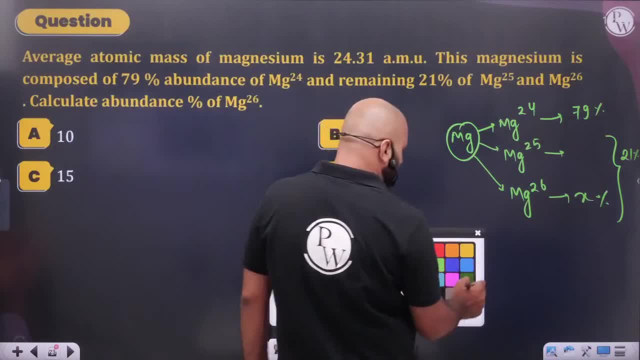 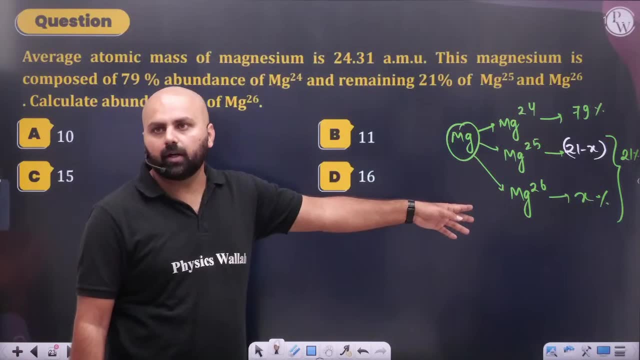 79. Sir, how much will it be by combining these two, It will be 21 percent. So how much should I take the value of this? Take 21 minus X, See, It will be 21 minus X, Sure. 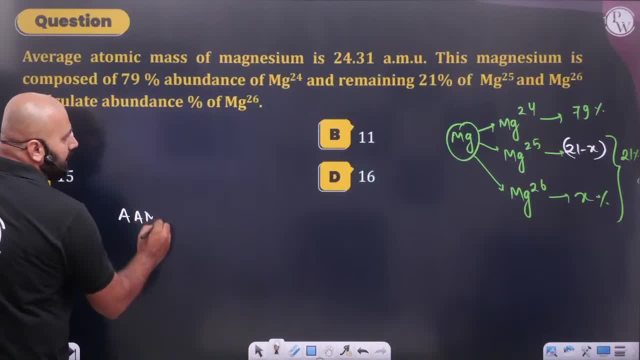 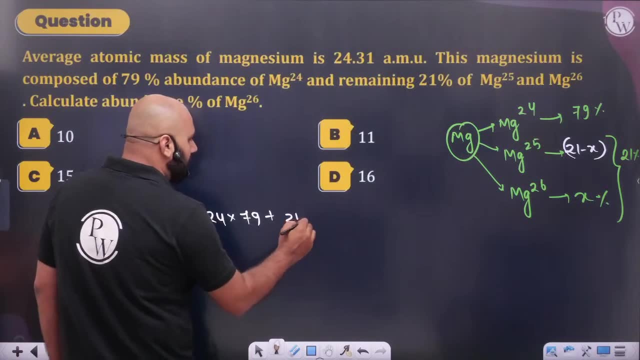 So see this Sir, see the value of this mango. If I go to take out the value of the atomic mass of magnesium, then how much will it be? 24 into 79 plus 25 into 21 minus X plus 26 into X divided by 100. 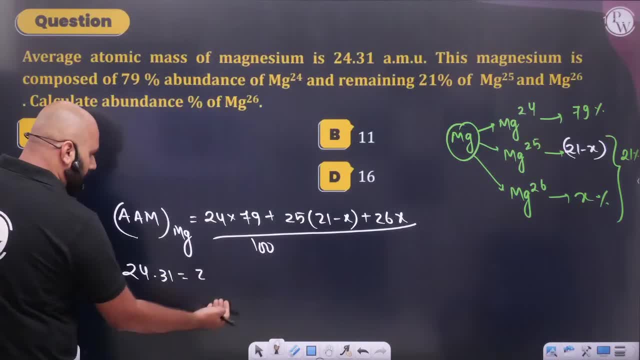 Brother, let's practice together, Because now you will not be able to practice more than this: 24 into 79.. Sir, calculate quickly. You have to do it in the exam hall. Okay, I don't have to do it. 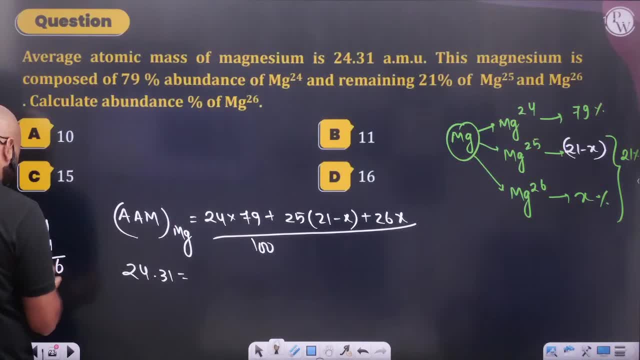 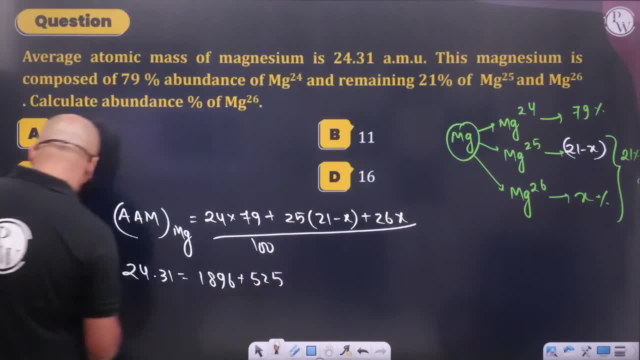 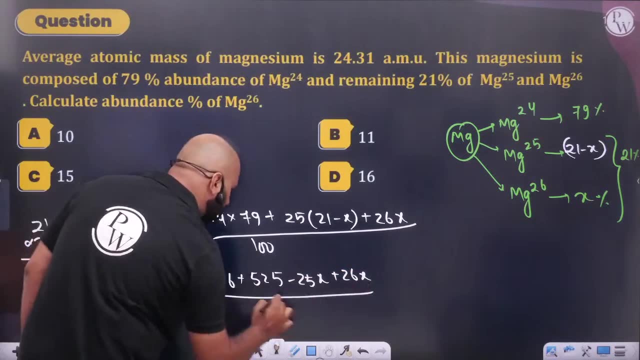 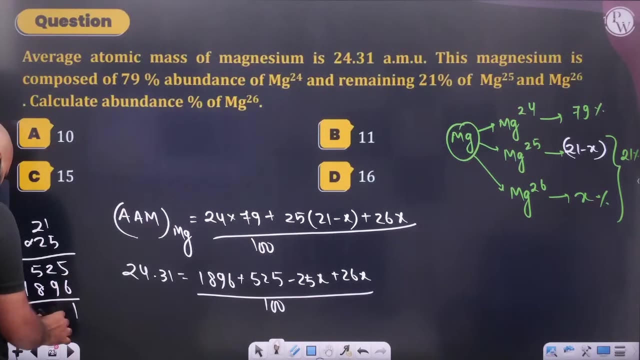 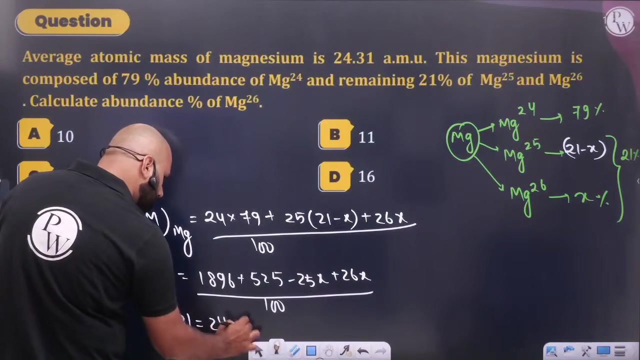 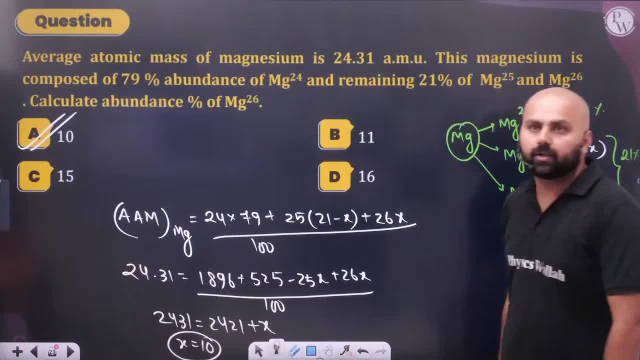 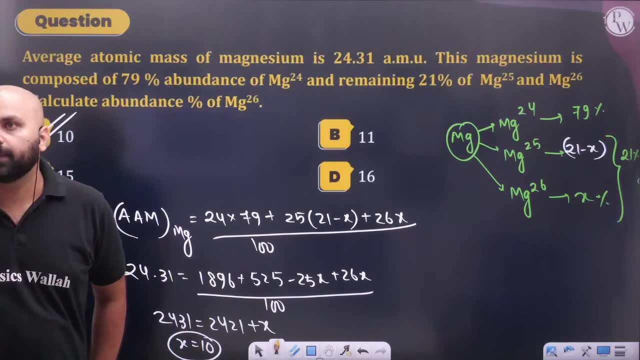 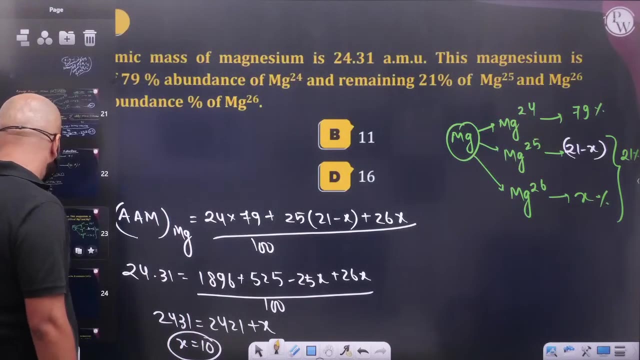 Sir, let's do the calculation together in the exam hall. only this much time has to be given to the calculation, Sir, how much is the value of x? 10 percent has come. if you calculate how much will be, the value of x, 10 percent will come. ok, it will be done, be sure. come on, brother. now see, sir, we have the question of average atomic mass. the question of average atomic mass has been done. after this: 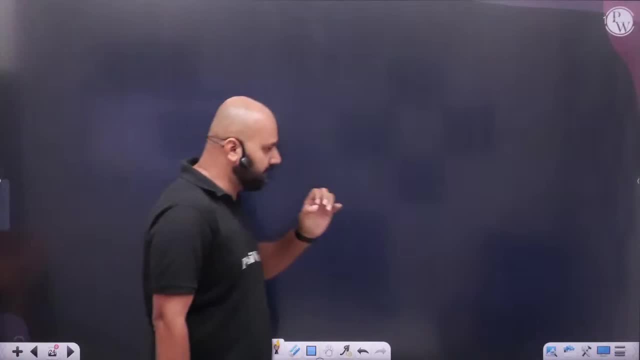 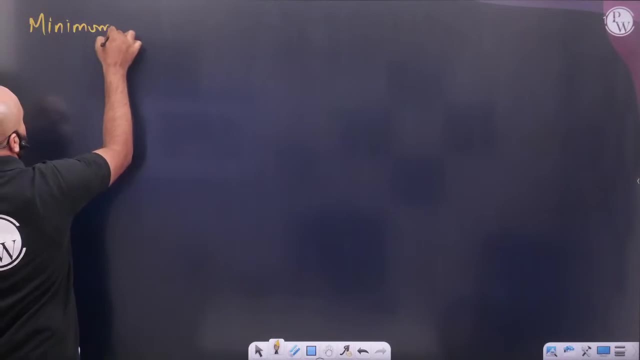 Now see as much as the question. more or less a lot of theories will keep a cover along with it. material, average atomic mass. after that a concept comes that is known as minimum molecular mass. remember always with us: there is concept comes, minimum molecular mass. 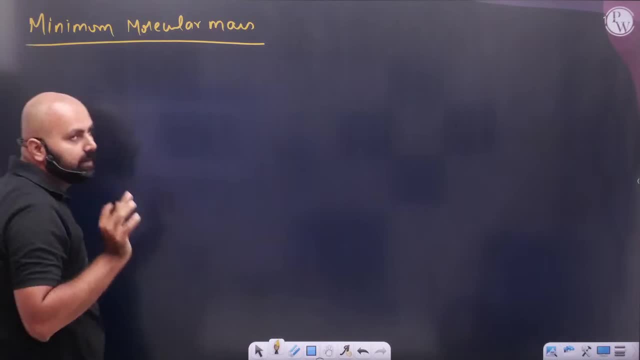 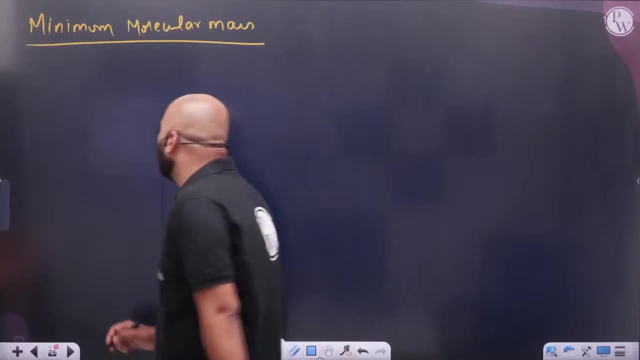 If someone has to get a minimum molecular mass, then remember his concept in his mind what the minimum molecular mass will be. Ok, the meaning of minimum molecular mass will be, sir, if you have a compound, let's say there is a compound x, it is saying, sir, it is not inside. 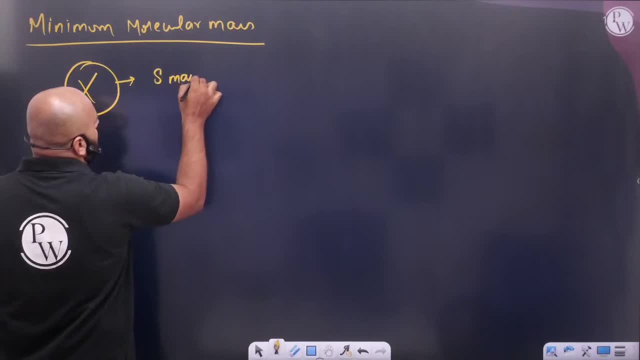 sir, in theços on sulphur, mass percentage is given. Sulphur's mass percentage is given 3.0 point is given 0.32 percent. He is saying that what is the minimum molecular mass of x? What is the minimum molecular mass of x? 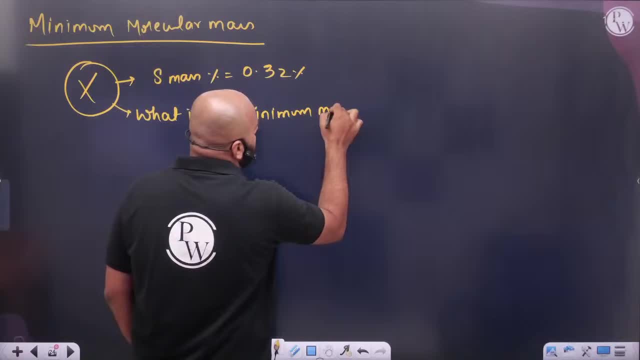 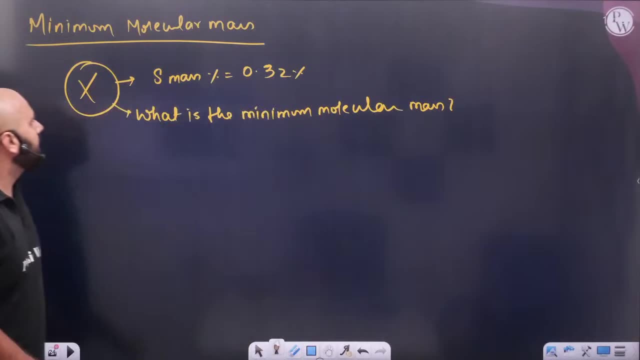 Brother, there is no shortcut, Nothing. You use a basic math. You will always get the answer. Remove the concept of minimum molecular mass. How will you remove it? See, How will you remove it. Sir, the mass percentage of sulphur is given. The mass percentage of sulphur is given. That means: 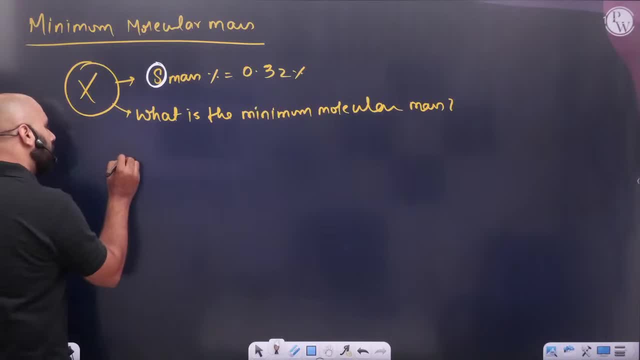 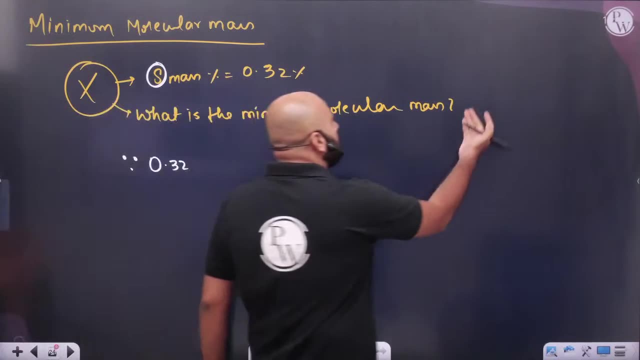 what That means. what That means. what Brother this 0.32.. See this carefully. See how I am writing, Sir. I don't know. Minimum molecular mass of x to be removed. What is in x? What is in it? 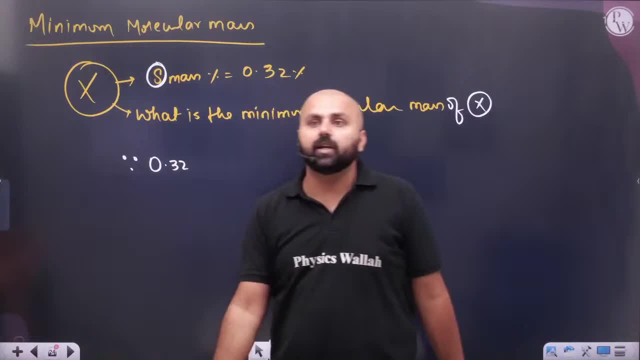 I don't know, There is sulphur in x. Apart from that, what else is there? I don't know. You look like MR sir's brother. Yes, he is a brother. The reality is that our house is nearby. I am also from Bihar. 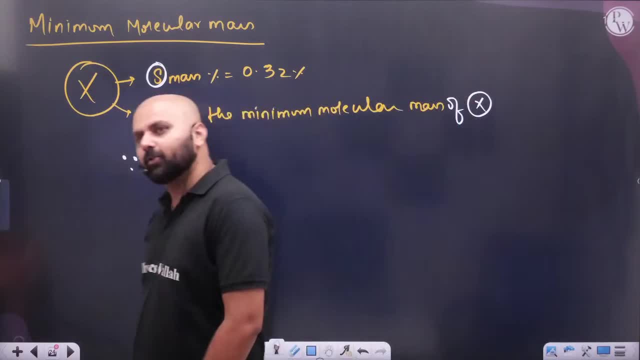 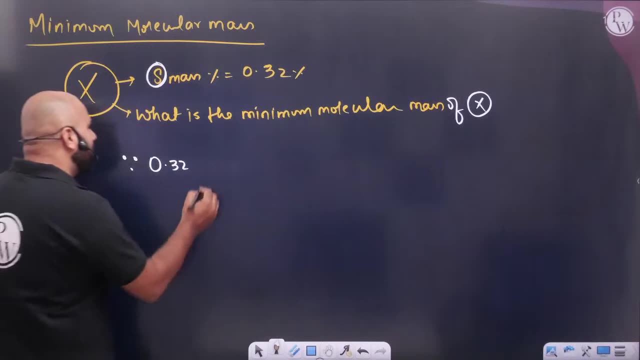 He is also from Bihar, sir, And we are from nearby. Okay, So, brother, your soul is done. You keep on thinking. I don't know what MR. MR is going on in it. Okay, See, See carefully. 0.32 gram Brother, take it a little seriously. I don't know what doubt it is. I don't understand. 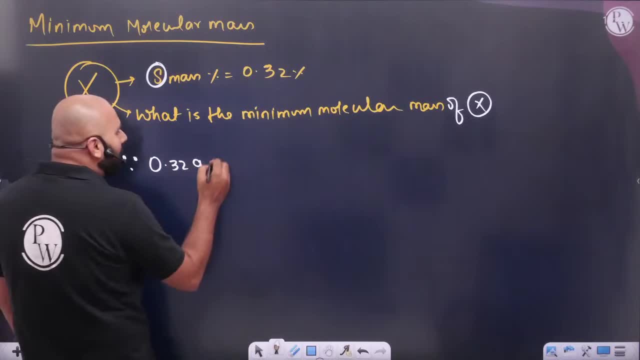 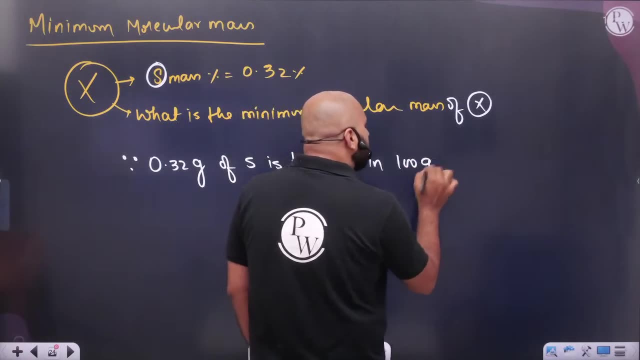 Maybe it can be Okay. See this, 0.32 gram of sulphur is present. You just have to do one thing: Write this, brother, Write this. I am telling you the question of basic math. 100 gram of x. 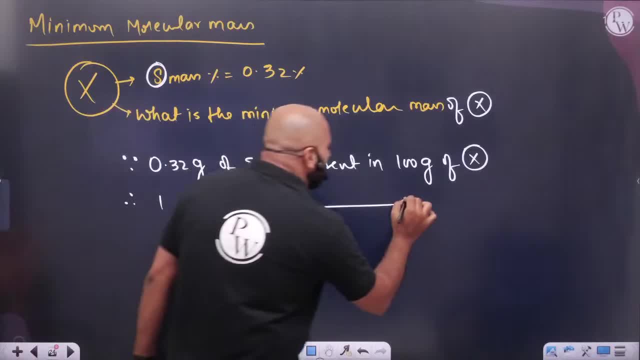 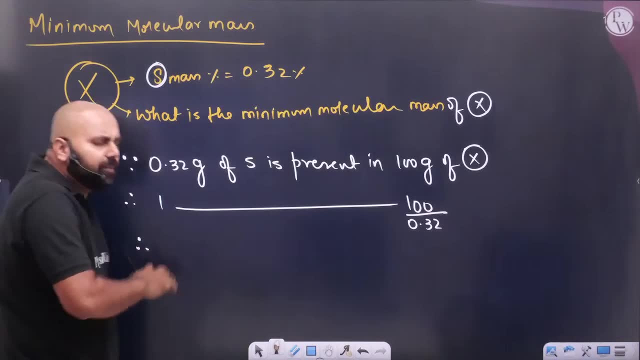 What will happen in a second 100 gram of x? And now, what am I doing? So, sir, we have all learnt the unitary method. We have all learnt the unitary method. And look here, Sir, I don't know what sulphur is and what is not in x. 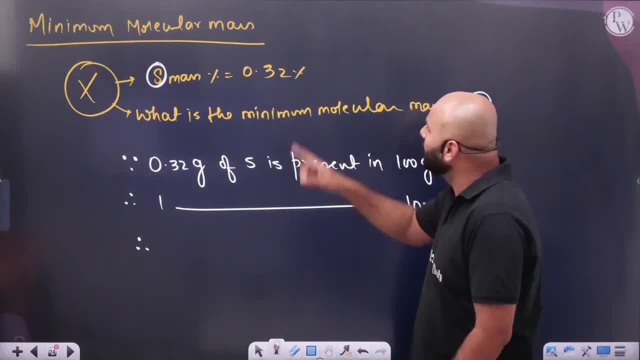 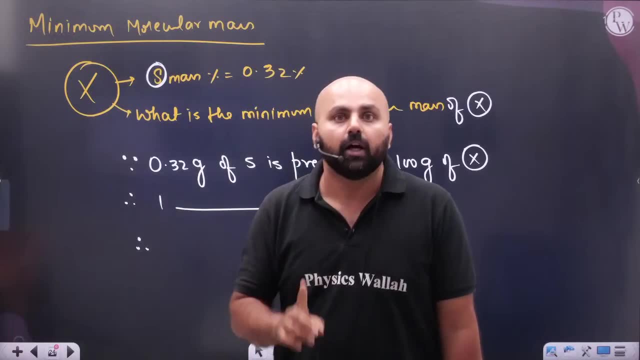 But I don't know what is there or not in x. But apart from that, one thing I know: The minimum of sulphur, No matter which compound one atom will be. at least What will be the mass of one atom of sulphur? What will be the mass of eight atoms of sulphur? 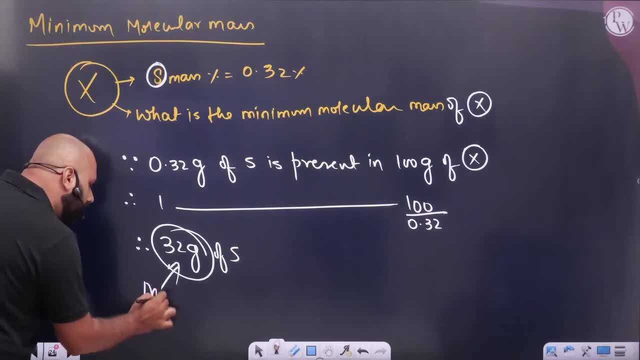 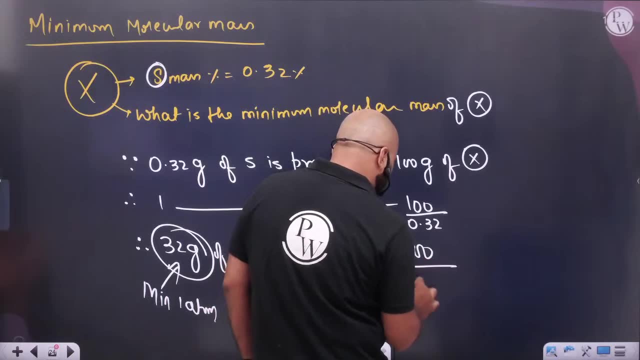 32 grams of sulphur. who is this representing, Sir? there will be at least one atom. There will be at least one atom. So, sir, here it is. If there is at least one atom, then put this, Put this and get the answer. 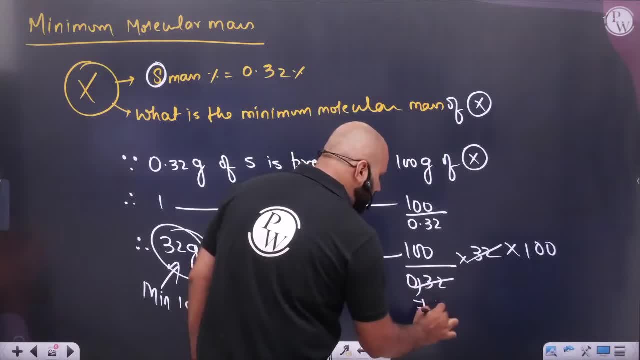 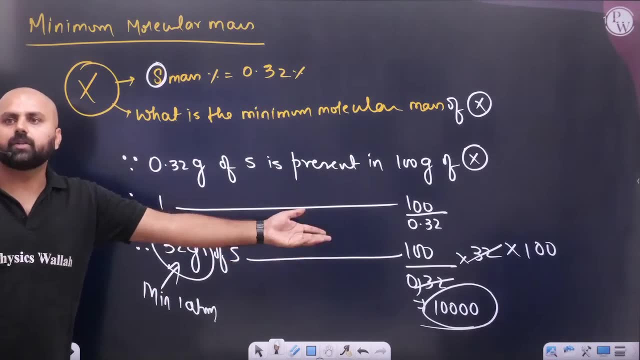 100 and get the answer. How much will it be? How much will it be 10,000 grams? Sure, It will be done, sir. So these are the small things. This is nothing. Don't remember any formula. 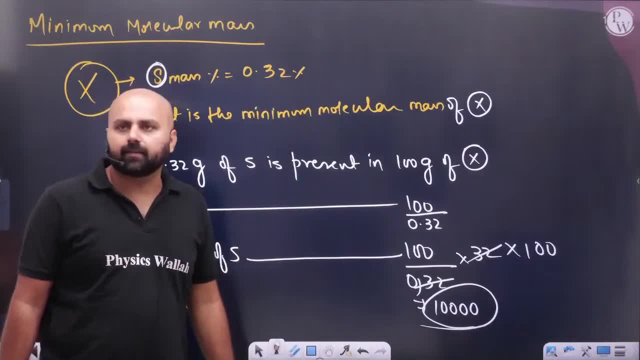 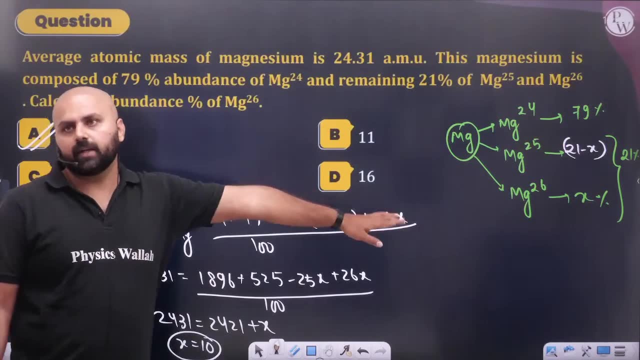 Use simple logic and get the answer. Use simple logic and get the answer. Who said, sir? the answer to the last question will be 11%. Son, I have taken an X for you. Look at yourself properly. Look at yourself properly. 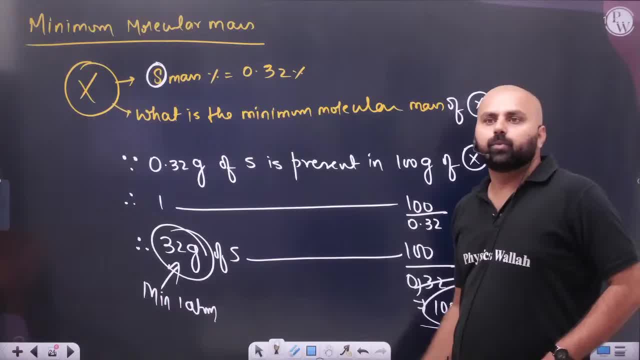 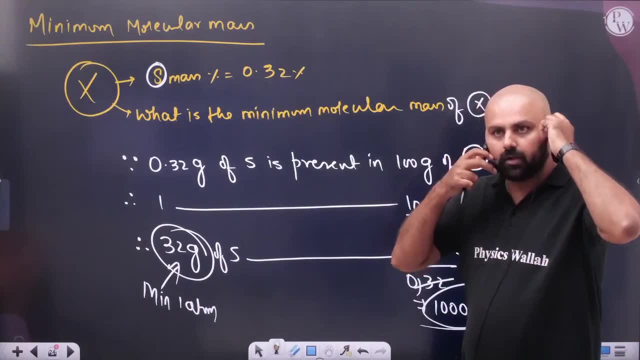 Before questioning me, do check once. Look at this. It will be useful for 10,000.. I don't know which one is from where. Okay, Yes, brother, we are from Motihari, Anyone else? Okay, Okay, now look. 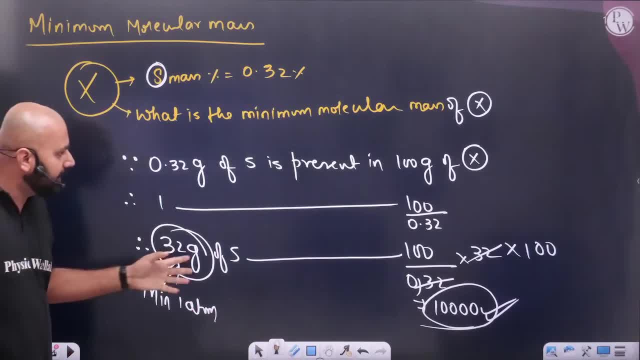 Whenever there are such questions now do the next question Now. I have told you this question. Now think about the next question yourself In the exam hall. there is a question in AMES. There is a question in AMES. 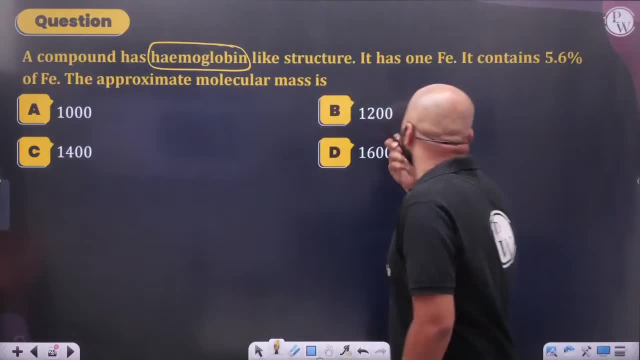 One is saying Hemoglobin. Everyone knows about Hemoglobin compound. He is saying, sir, there is some compound in it which has a structure like Hemoglobin. It has only one iron And it has 5.6% of iron. 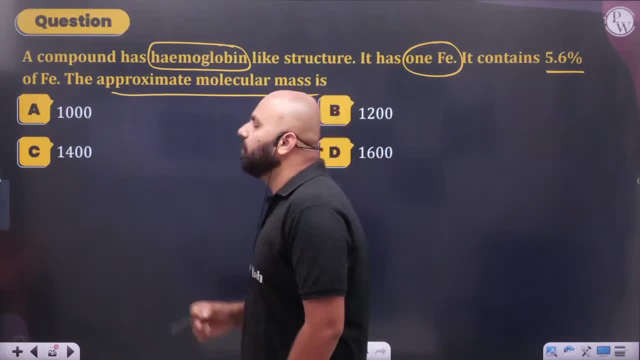 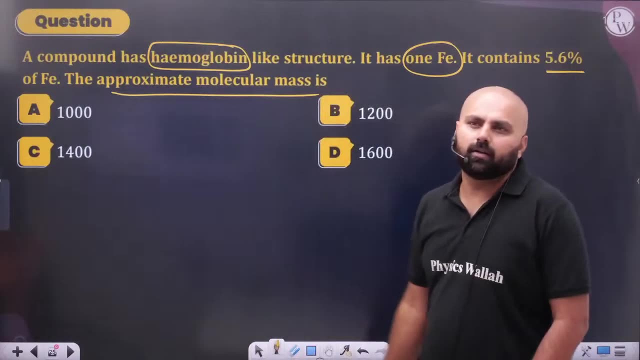 Sir, how much will be the approximate molecular mass or how much will be the minimum molecular mass? How much will be the approximate molecular mass or how much will be the minimum molecular mass? How much will be the minimum molecular mass? What will be? 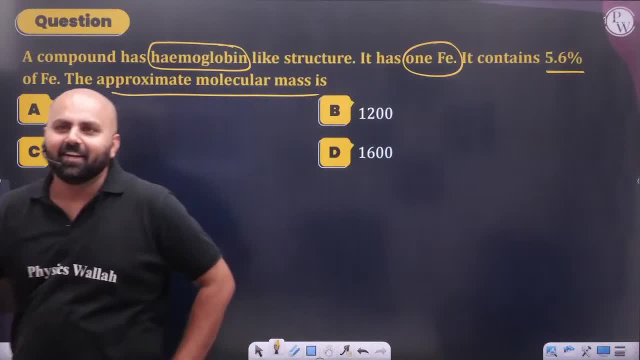 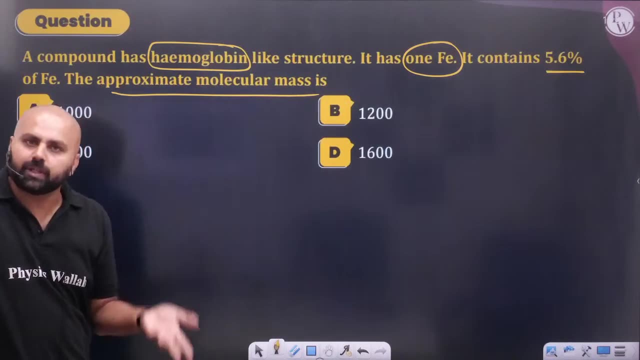 Sir, 32.. Okay, 32.. It is the mass of one atom of sulphur. If you are taking grams, if you are taking grams at the top, then also at the bottom. Use the unit dimension, brother. Use the unit dimension. 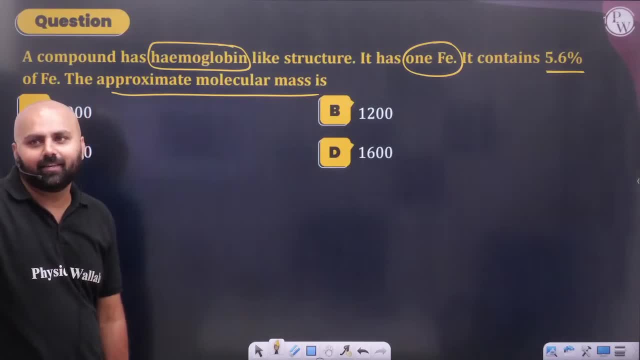 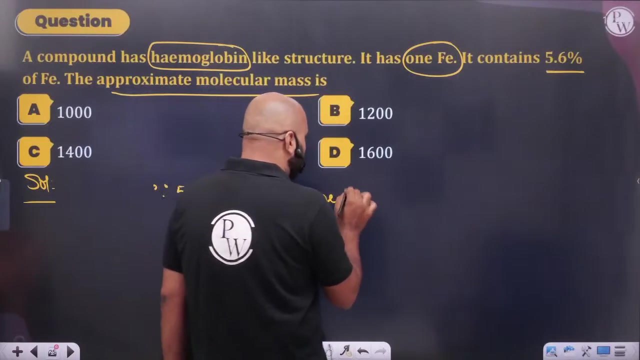 Come on, Yes, quickly, See this. What will you do, Sir? nothing. Use the same unit dimension again. 5.6 grams of iron is present in 100 grams of compound. 5.6 grams of iron is present in 100 grams of compound. 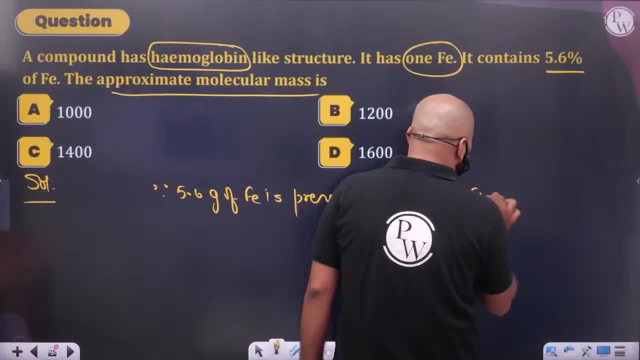 5.6 grams of iron is present in 100 grams of compound. I don't know which compound it is, But I know that it has 5.6 grams of iron, But I know that it has 5.6 grams of iron. 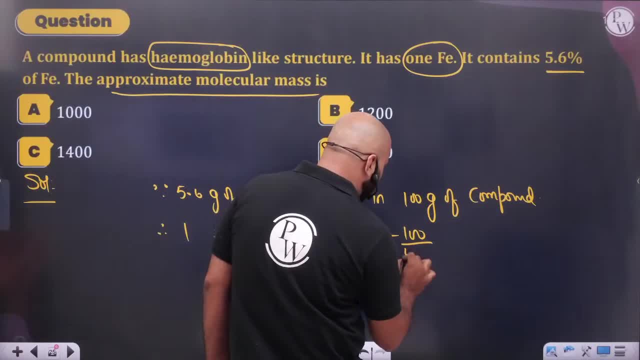 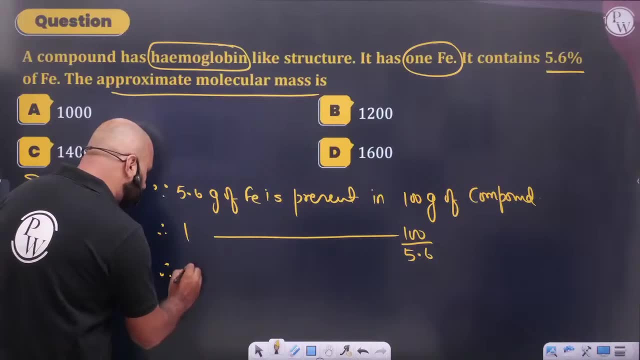 So what will happen for 1 gram of iron, 100 upon 5.6.. And if I say what will happen, See here What will happen in this, Sir. what will be the mass of 1 iron? What will be the mass of 1 iron? 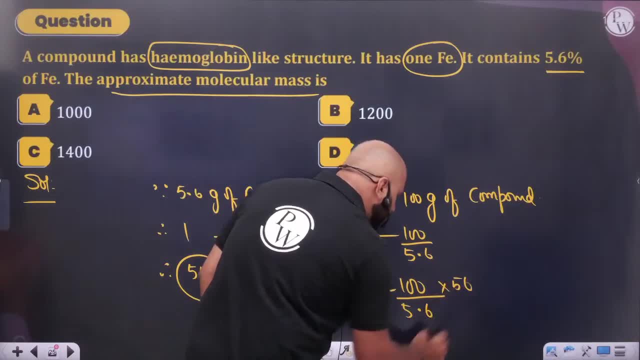 100 upon 5.6 into 56.. Okay, If I am taking grams at the bottom, then also I will take grams at the bottom. Only then it will be cancelled out. So see here, 0 has gone up. 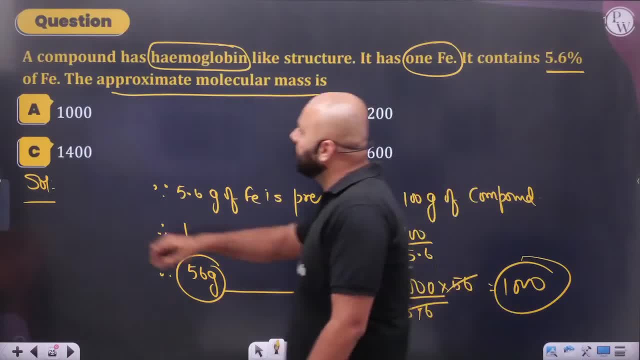 56 to 56.. How much is the answer? 1000 has come. How much is the answer 1000 has come. How much will be the answer? 1000 has come. So just keep doing it, Keep doing it. 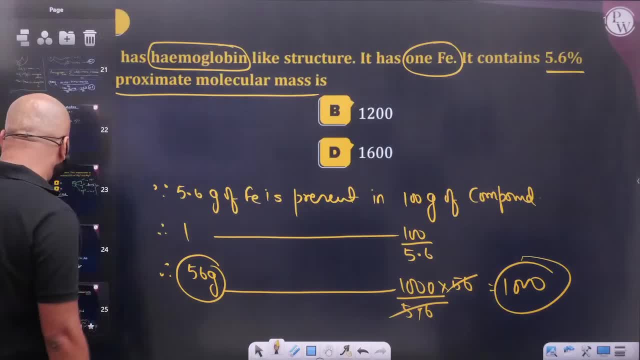 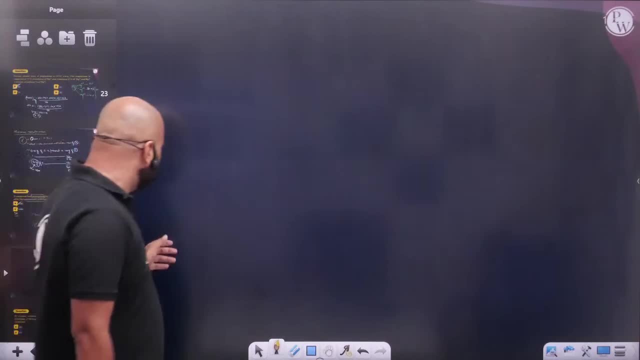 Keep doing such small questions, Questions like this are filled in this chapter. Why? Because, sir, such questions are asked here. Such questions are asked here. Next question will be seen. Next question will be seen: The concept which will come after Minimum molecular mass in our life. 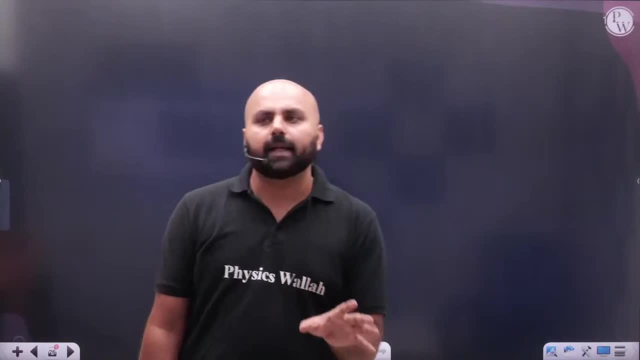 That will come. Which one Empirical and molecular formula? There is a reason to take more time in this chapter Because this is the most basic chapter. It will take a little more time Where we can save time. we will take less time in states of matter. 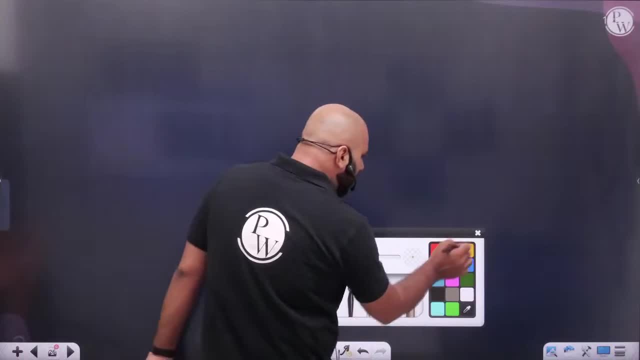 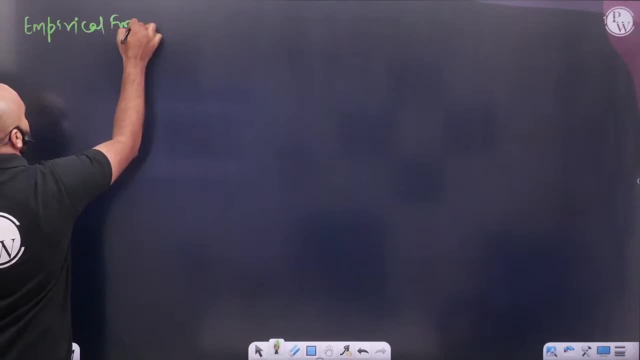 Because we must have already done a lot. I am saying: see, in this chapter We have one more concept That is known as empirical formula concept. Hey, talk about empirical formula. If you talk about empirical formula, If you talk about empirical formula, 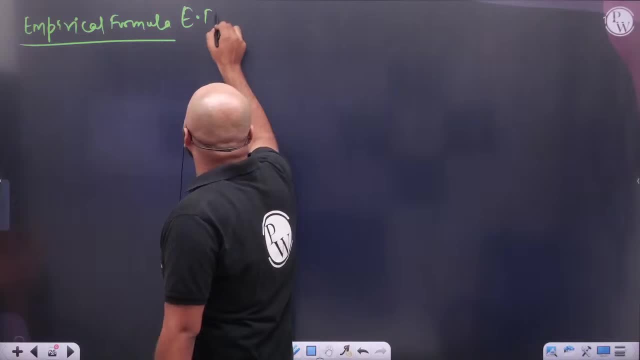 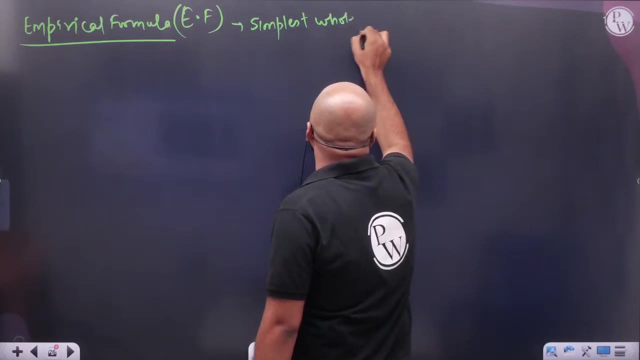 If I write empirical formula in short cut, What will be empirical formula? Empirical formula is nothing. Simplest whole number ratio. Simplest whole number ratio. Whose Sir? whole number ratio? Whose Atoms, Sir? take simplest whole number ratio of atoms. 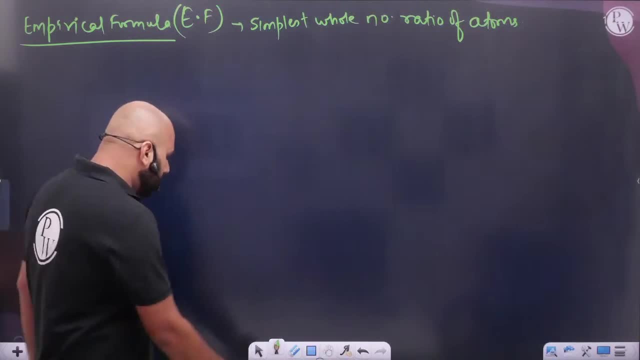 What do they call that Empirical formula, Sir? see this with yourself. See this: In empirical formula, molecular formula, There is a multiplication factor. There is a multiplication factor. He uses both of them, Sir. he relates both of them. 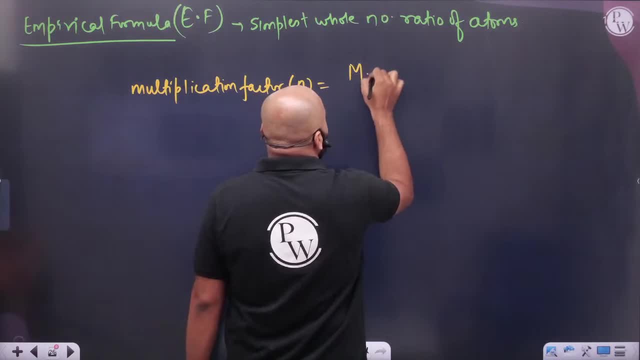 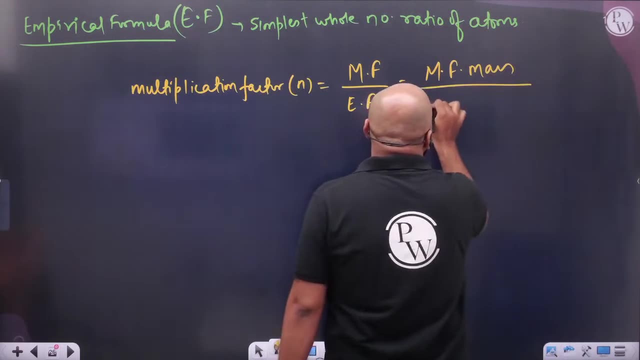 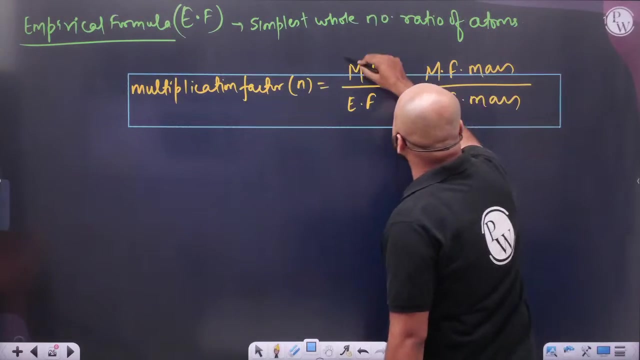 The value of n. What is this? Molecular formula divided by empirical formula Or molecular formula mass? Molecular formula mass divided by empirical formula: mass. We have this formula, We have this formula And we are using this formula. See this Multiplication factor. 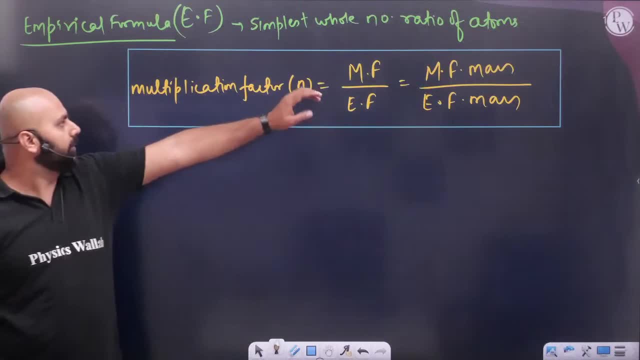 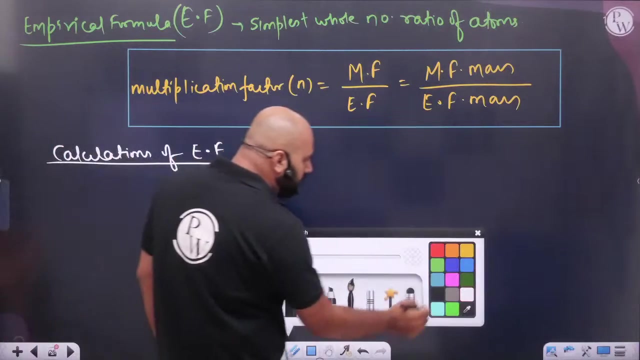 Second, Who told me, Brother, molecular formula and empirical formula, mass ratio. Okay, Sir, how will we do the calculation? Look carefully In exam hall. no one can tell an easy calculation of empirical formula. Remember, we have to calculate. 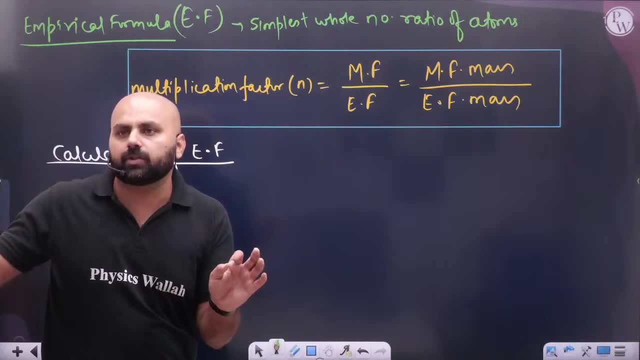 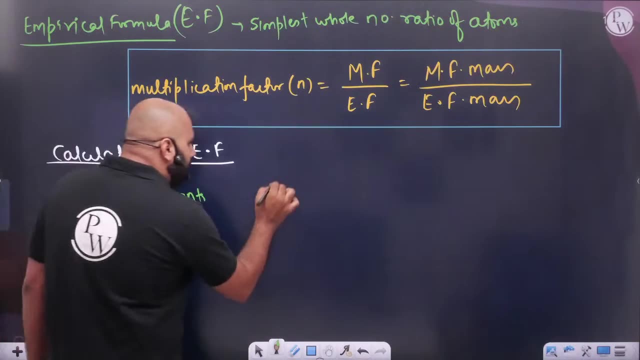 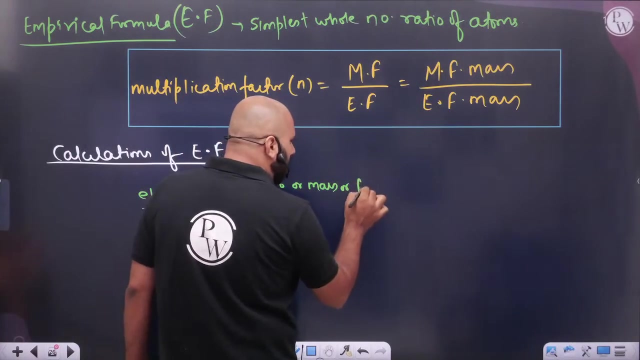 empirical formula. I will tell you the easiest way to calculate empirical formula. See this: What to do in exam hall? Write elements Here. if percentage is given, Whether it is mass or fraction, Whether it is mass or fraction, Whatever it is, 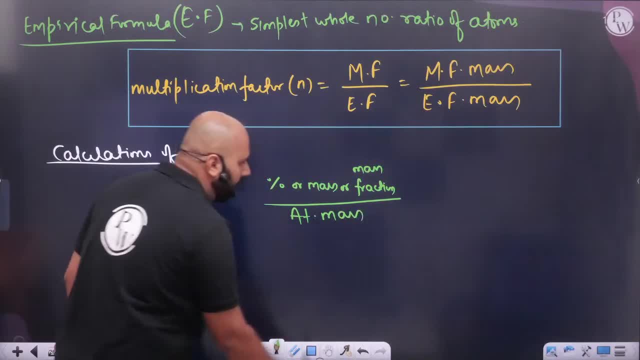 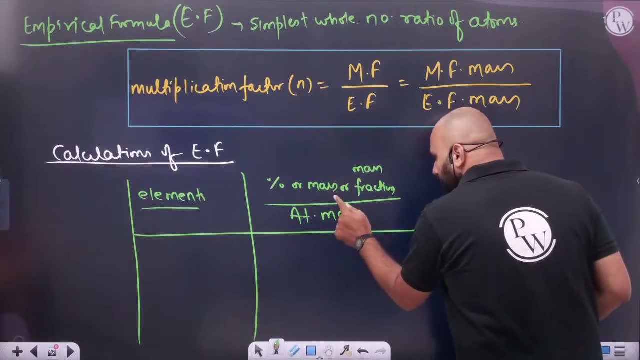 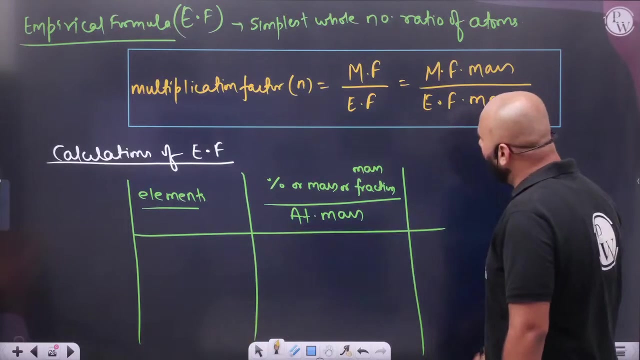 From whom to divide From atomic mass, Sir. what will we write first? We will write elements After elements. what will we write, Sir, whether it is percentage, mass, mass, fraction, Whatever it is, From whom to divide? 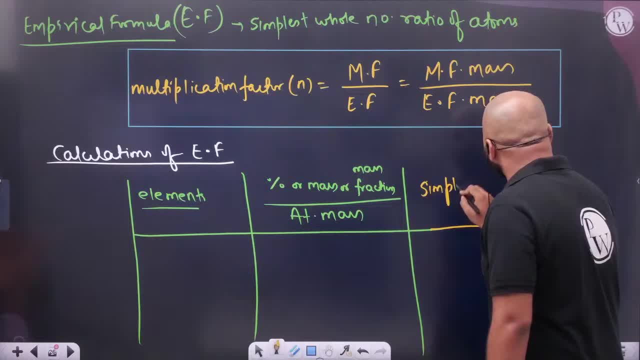 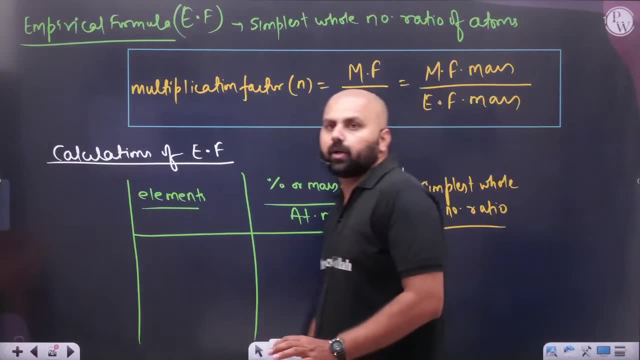 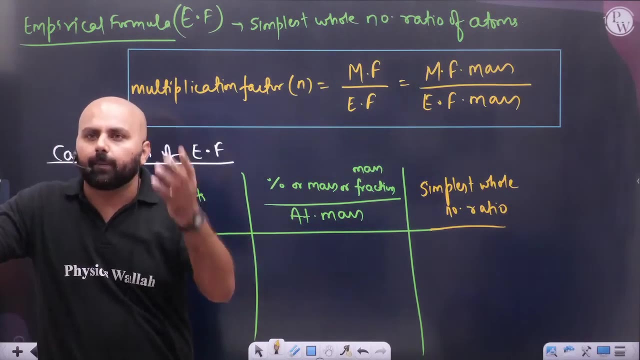 From atomic mass. Whatever it is, You will get the answer in 3 steps: Simplest whole number ratio. Simplest whole number ratio In empirical formula. Sir, you should know about iron Molecular mass Already. you have passed 12th. 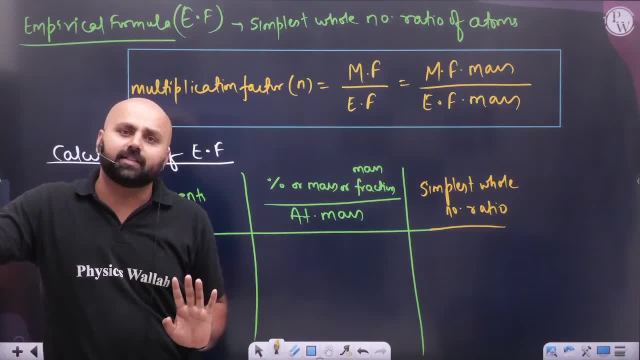 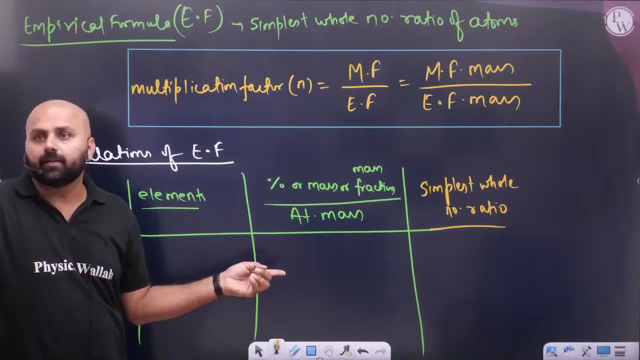 You have chapter Brother. this chapter is the most important chapter. Reason: All the chapters have small concepts and questions. You know the question on empirical formula. Okay, Keep in mind, These are small questions. These are questions for 2021.. 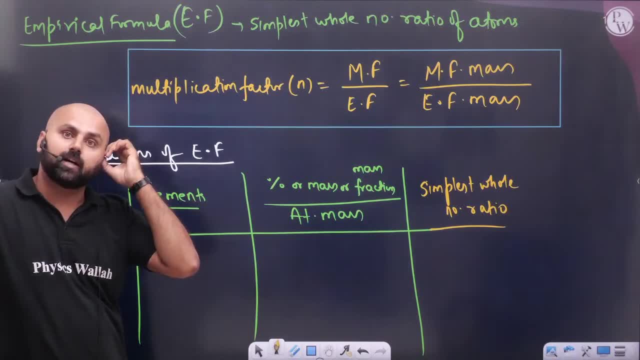 For me as a teacher. I always say in class: on 7th May, I will come and say in the evening of 7th May 2023. That this thing should be taught Whether it is marathon or normal class. That's why every point is being covered. 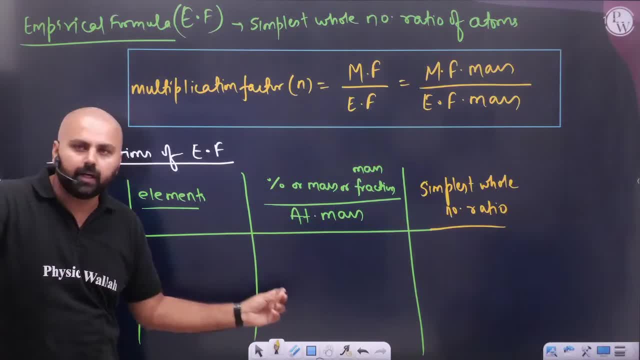 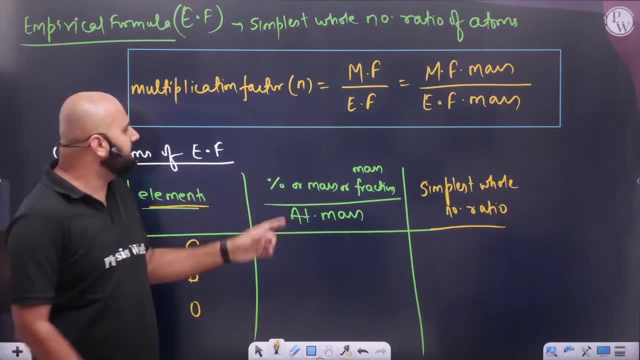 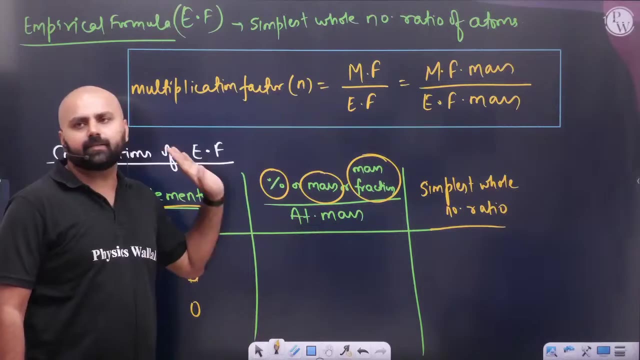 It is being covered only for you. Try as much as possible. Try as much as possible. Hold these small questions. Write any thing Like carbon hydrogen oxygen, Whatever percentage is given, Whether it is mass or mass fraction, Whatever is given. 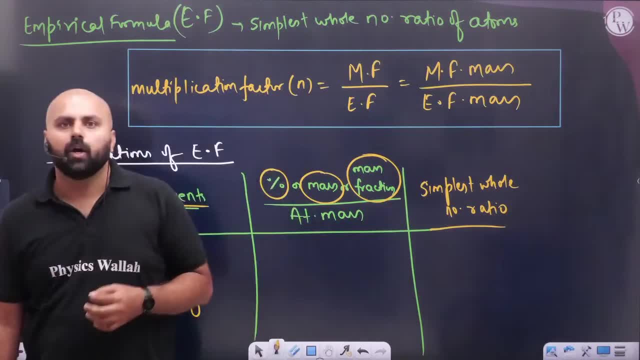 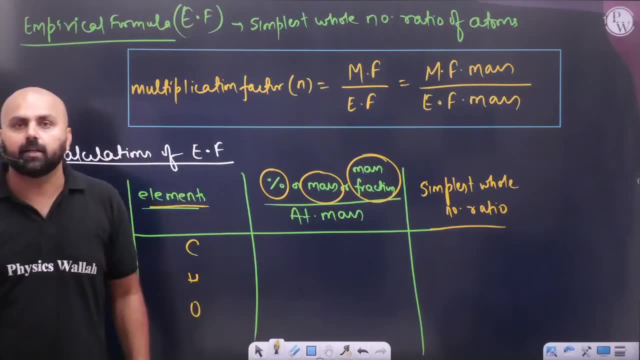 Divide it with atomic mass And in the next question Do the simplest whole number ratio. It is a very simple method. That's all you have to do in exam hall. But in exam hall the other person enjoyed. In exam hall the other person enjoyed. 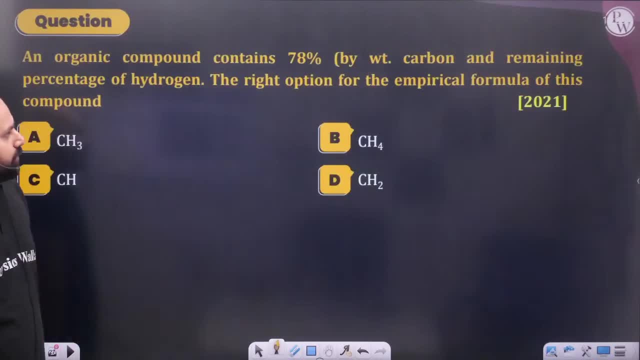 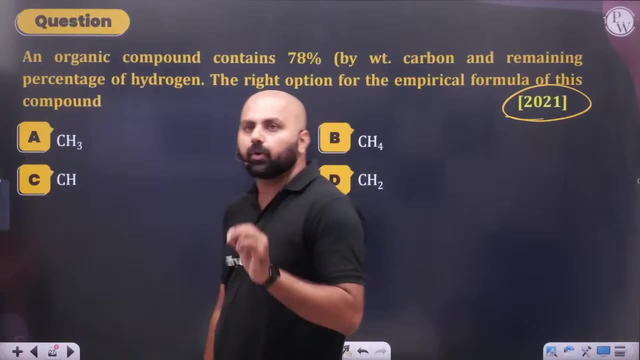 Do you know how? I will show you the question of NEET 2022.. I will show you the question of NEET 2021.. There was a question in 2021.. There was a question of 2021.. Very beautiful question. 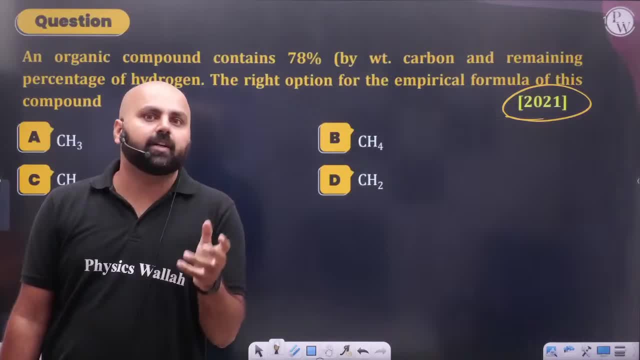 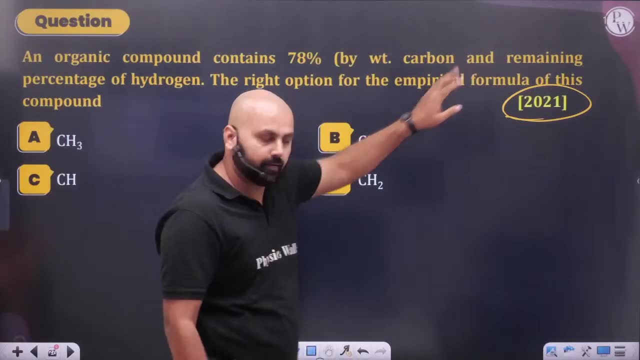 That's why we say: look at yourself How pressure is put on the exam hall. How pressure is put on the exam hall. Look at this. There is an organic compound What is 78% by weight? There is carbon. There is nothing. 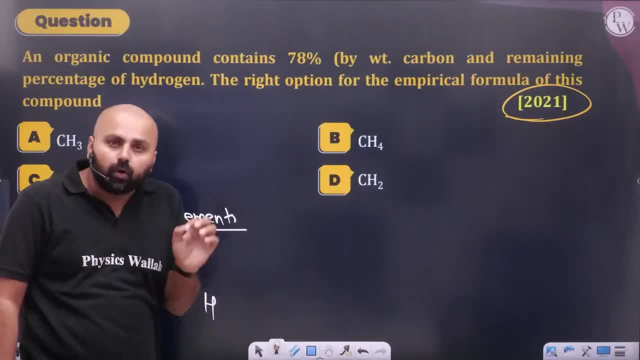 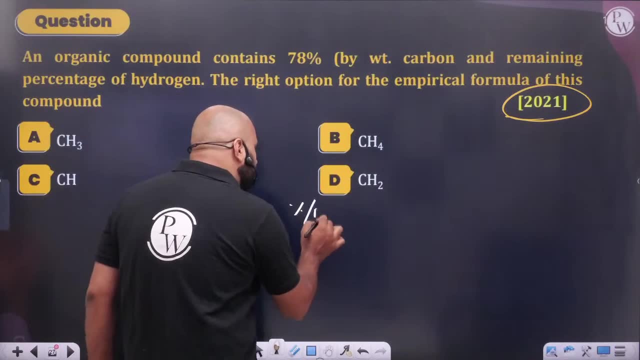 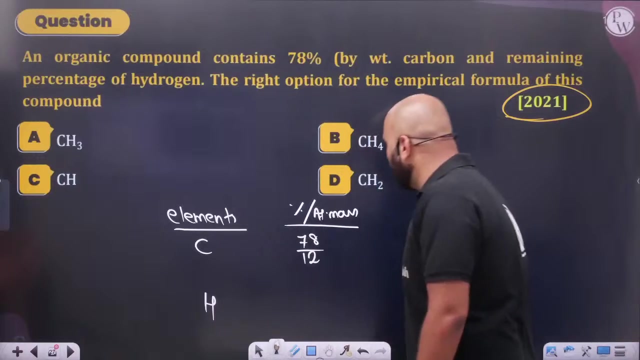 What do we have to do? What have we learnt? Look at the exam hall. What you are studying, Go and apply in the exam hall. It will be so difficult. Atomic mass: What is the percentage of carbon? 78. 78 upon 12 is the atomic mass of carbon. 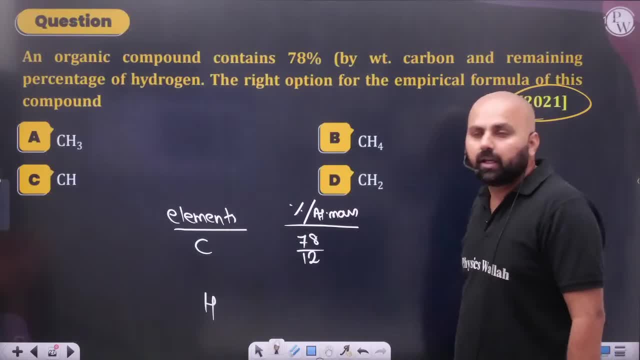 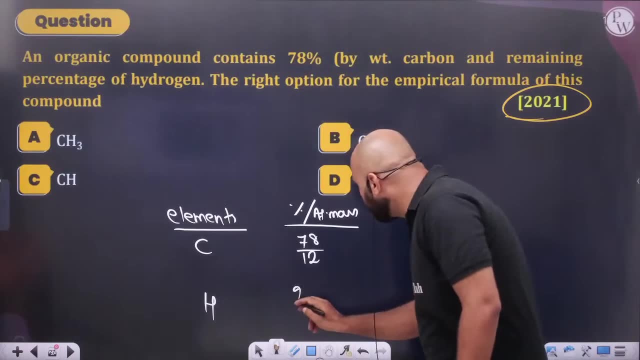 The answer of hydrogen is not there. I am just showing. I am talking about hydrogen. How much hydrogen will be left? Carbon and hydrogen are in the organic compound. How much hydrogen will be left? 22 will be left, Sir. divide it. 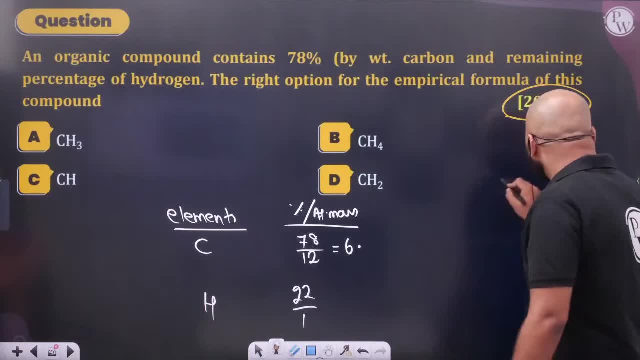 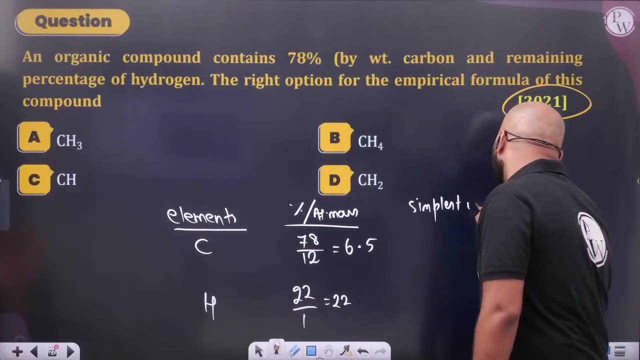 Take it out in the exam hall. How much will it be? 6 points, Sir. how much is this 72.. 6.5.. How much is this 6.5.. How much is this 22.? 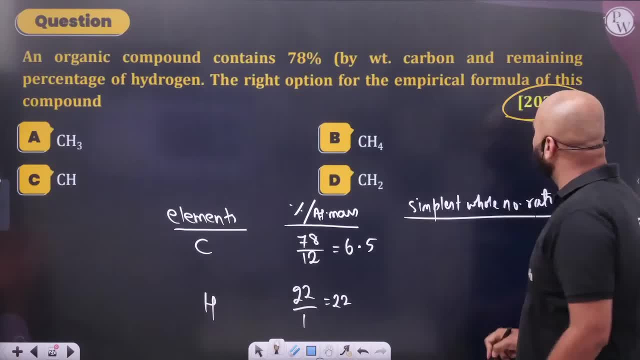 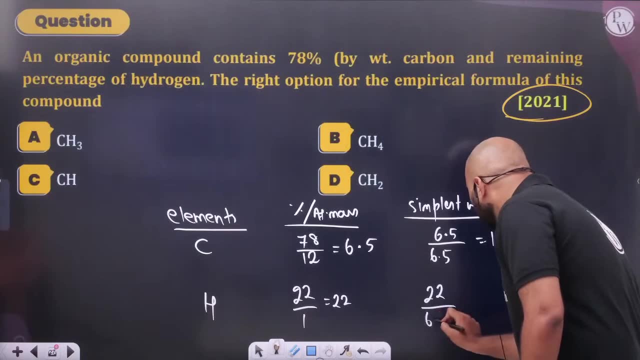 What is the next step? Simplest: whole number ratio. When this paper came, many people made a mistake. Divide everyone from the smallest number. This is 1.. If you divide 22 by 6.5.. If you divide 22 by 6.5.. 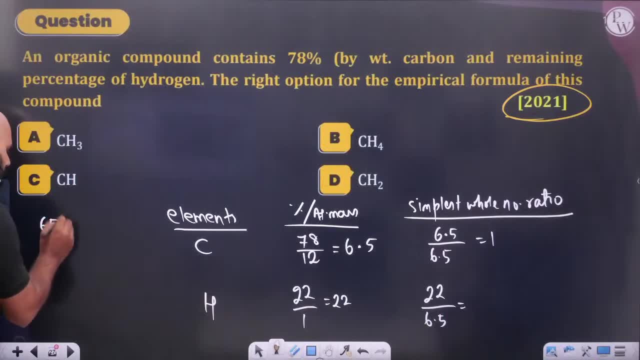 How much will it be? If you think, then do it, Do 65 upon 220.. You will know How much will it be 3.. This is 5.. And how much is this? 195.. Sorry, How much is this. 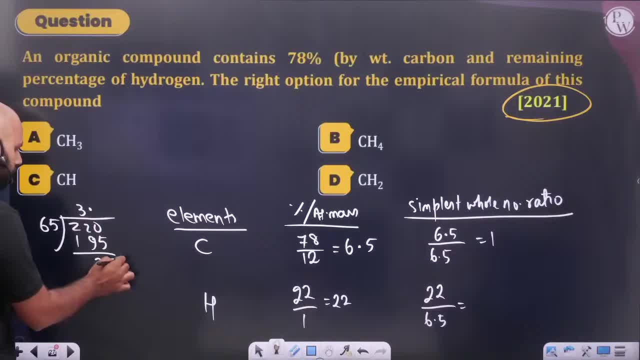 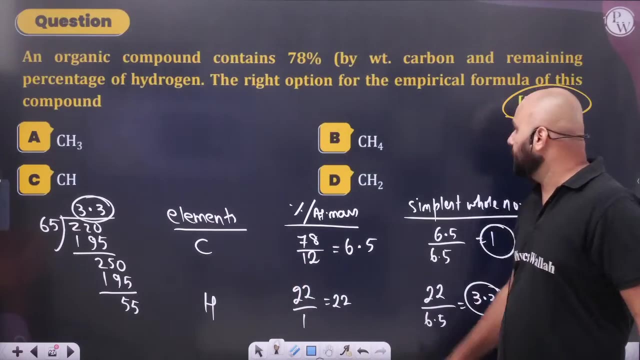 22 is 0.. If I do it again, 3.3 will come. 195 will come. How much is this? 55.. How much is this answer? 3.3.. Son, when people reach here in the exam hall, 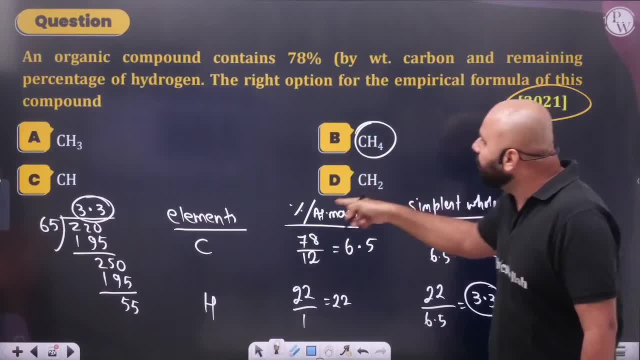 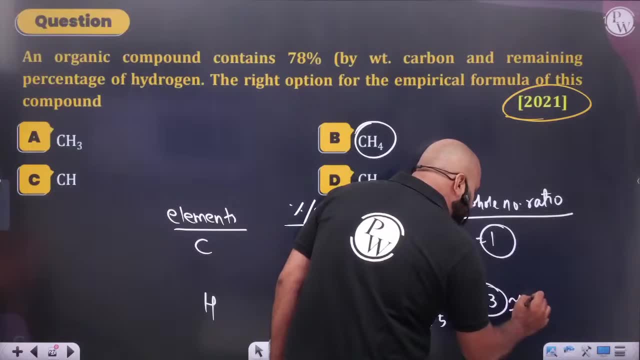 That's why the roundup is told. Do you know what some people did? They ticked this. This option is given because of this. People had no doubt in this. That's why people are saying Confidence will only come in the exam hall. 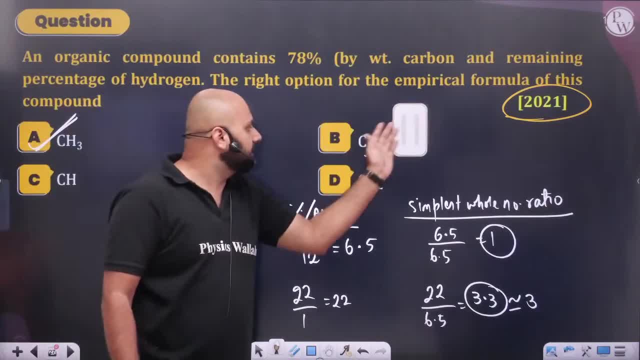 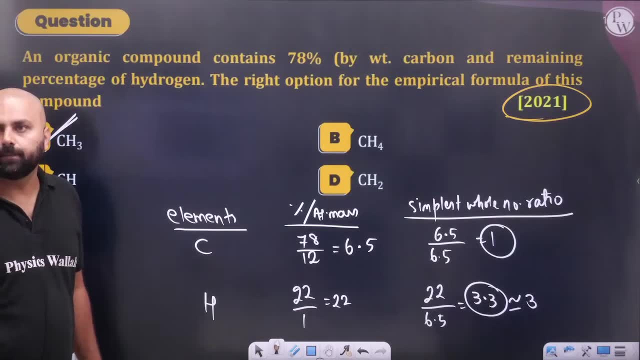 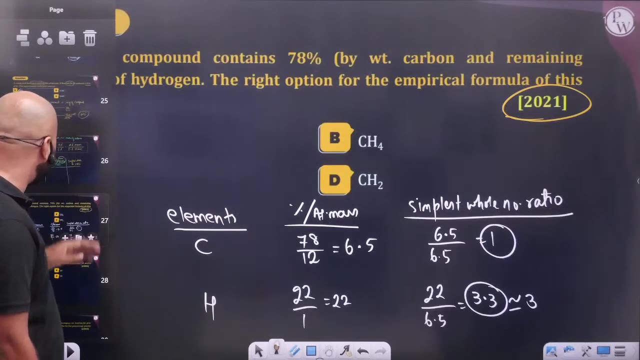 When you do it. Don't make this mistake in the exam hall. Take the simplest ratio, Take the whole number ratio. Okay, It will be done. Are you sure? Done? Obviously, if you don't have confidence, What can you do? 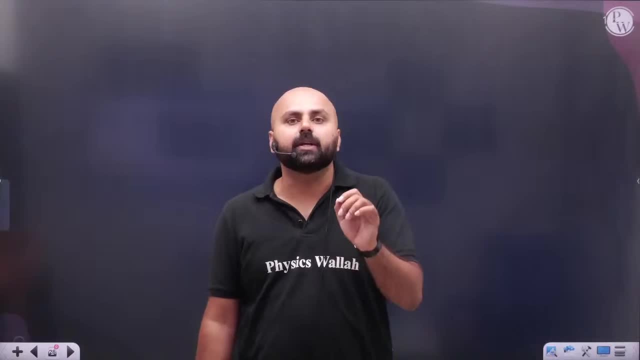 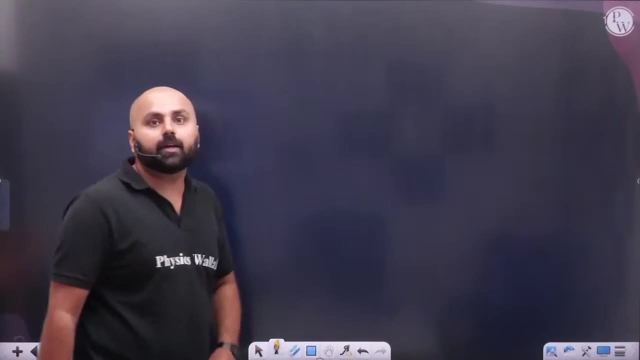 If you don't have confidence, Then the problem will come. Now this chapter is reaching the end Because only one thing is left: Stoichiometry. After that, the terms of the solution are left. I am taking so much time in this chapter. 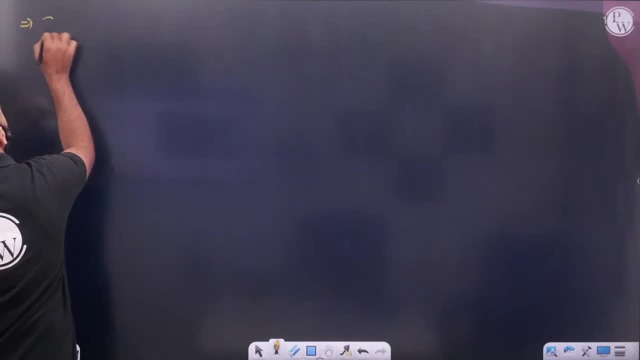 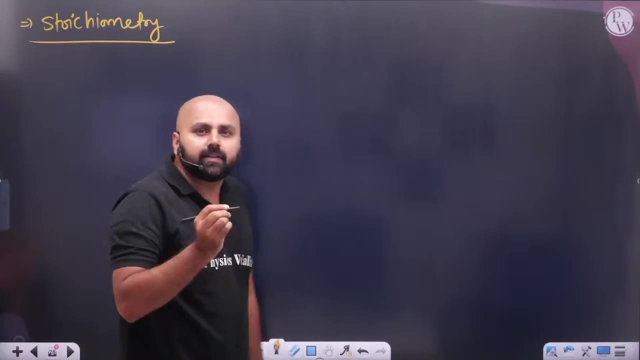 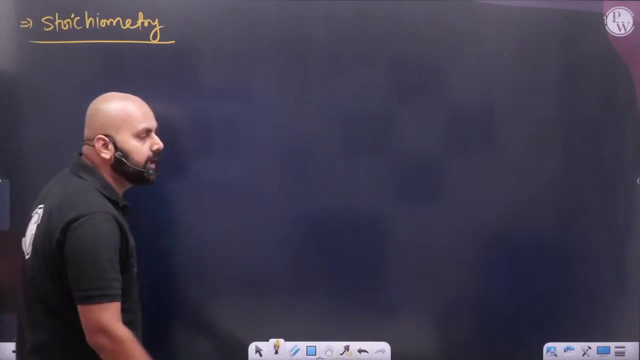 Look at this, Look at this: In stoichiometry, Sir, we have stoichiometry, Stoichiometry. Whatever you say, as you say Nothing, I will tell you a way to write any reaction. I will tell you a way to write any reaction. 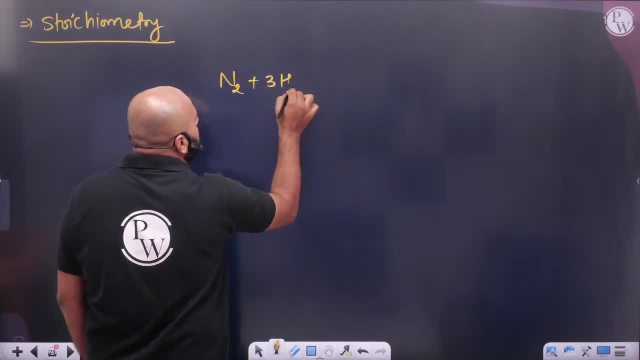 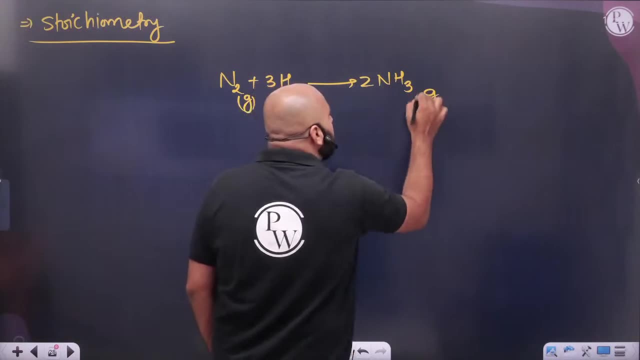 Keep sitting on it and keep questioning. Sir, if suppose somewhere such a reaction is written: N2 plus 3H2 gives 2NH3. Then, brother, see the way to write this reaction. How can I write If I want to read this reaction? 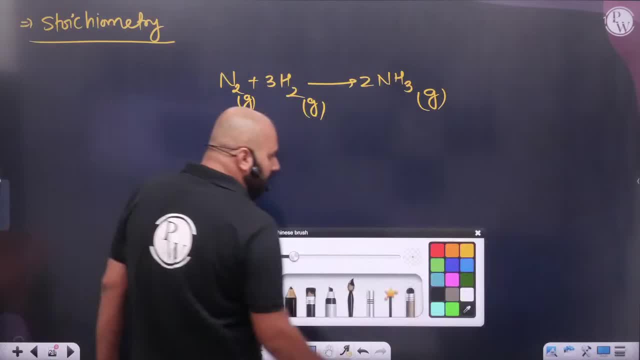 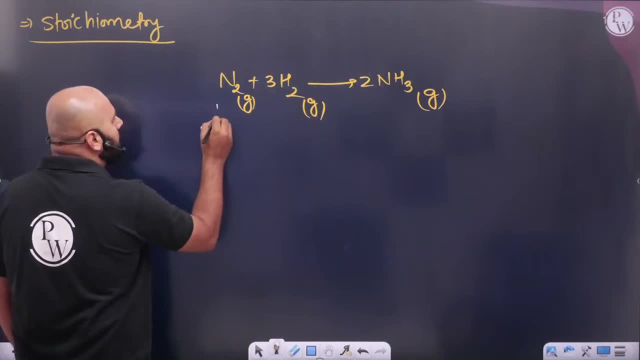 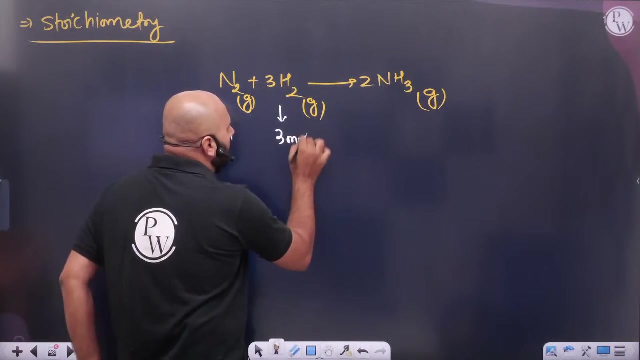 If I want to write, Then how can I write this? See this: What will be the answer to this reaction? See this: I can write this: One mole of nitrogen. One mole of nitrogen. One mole of nitrogen Is reacting with 3 moles of hydrogen. 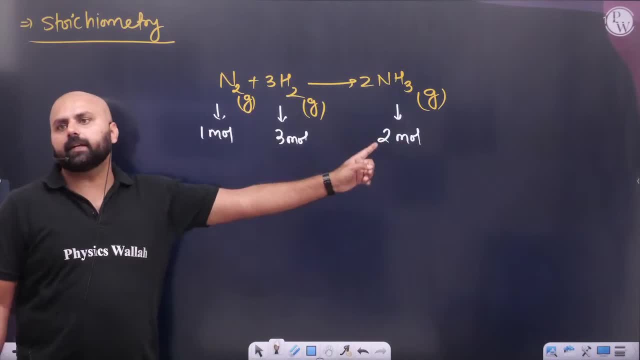 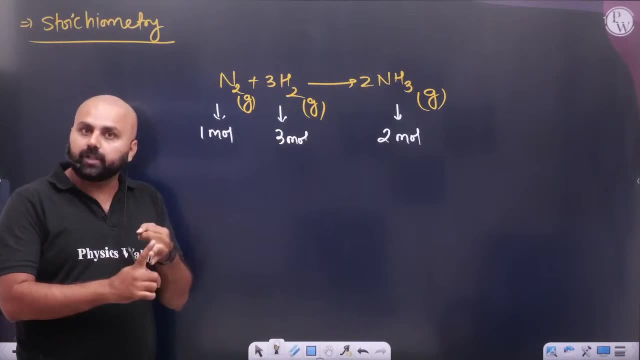 And how much is it getting? 2 moles of ammonia. One mole of nitrogen Is reacting with 3 moles of hydrogen. I will explain everything. Listen carefully. We will revise different concepts together. See this: This was written in the term moles. 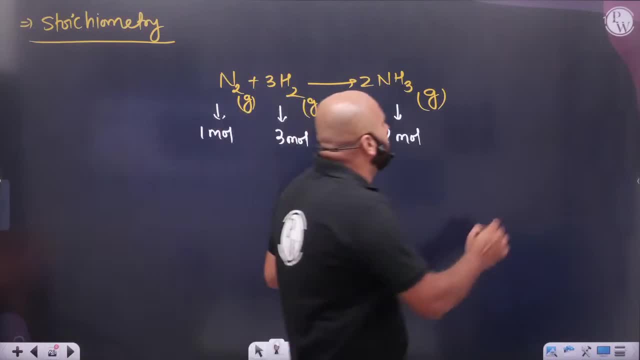 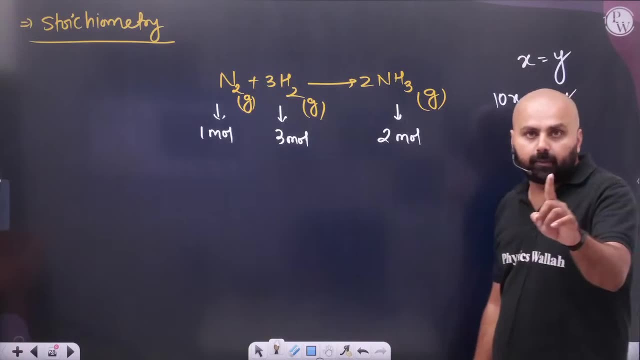 See carefully what happens. I will tell you a simple mathematical equation: If X is equal to Y, Then multiply it with 10 on both sides, Sir, will be same. Multiply it with 10 on both sides Will be same, If anywhere in the questions. 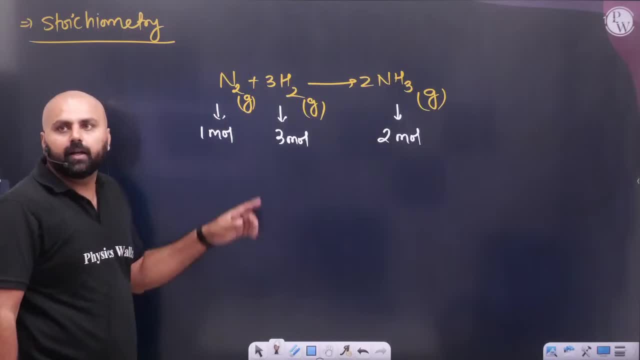 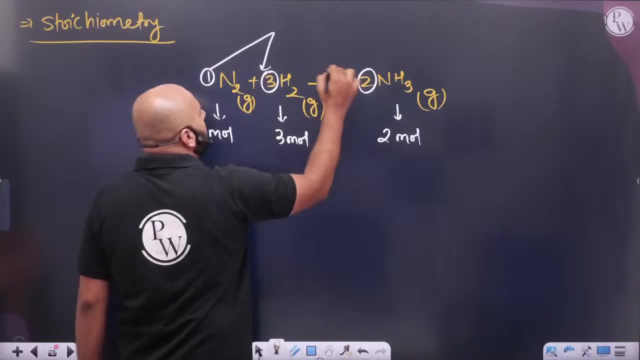 Then there is nothing. If I want, sir, Is there anyone saying how to write it? Look at this: there is 1 in front of it, there is 3 in front of it, there is 2 in front of it. What do we call these? 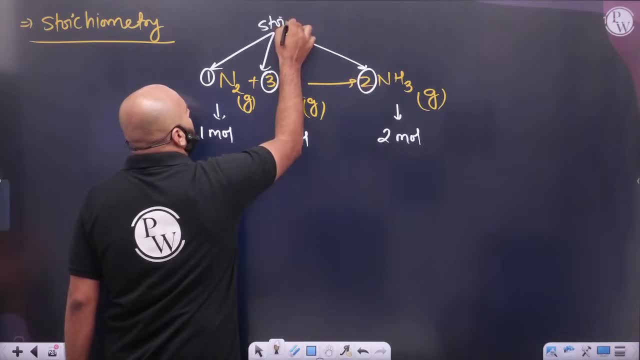 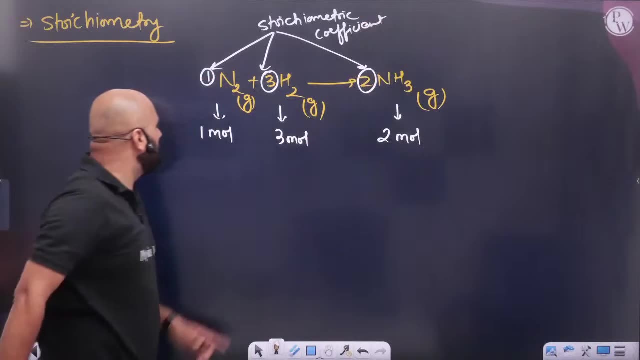 What do we start calling these? We call it stoichiometric coefficient. What do we call these? We call it stoichiometric coefficient. This is what we decide. So look at this. what will happen? 1 mole, 3 mole, 2 mole. 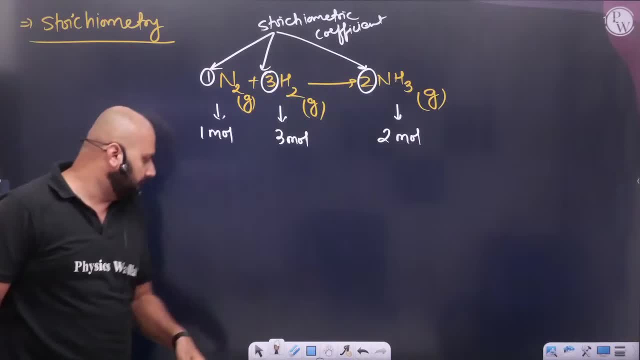 Look at this: If it was 3.9 in the previous question, then we would have taken 4.. But it was 3.3. So obviously I had rounded off. Look at this Now. I will tell you a simple thing. 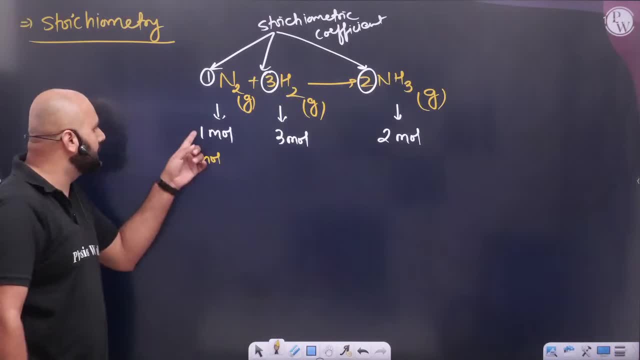 Remember, if I want this, what did I do? I multiplied it by 10.. If I multiply it by 10, listen, If I multiply it by 10, then what did I say? If x is equal to y, then if you multiply both the sides by 10, there will be no difference in the reaction. 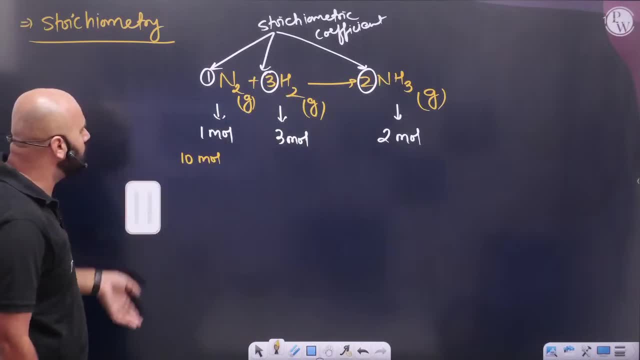 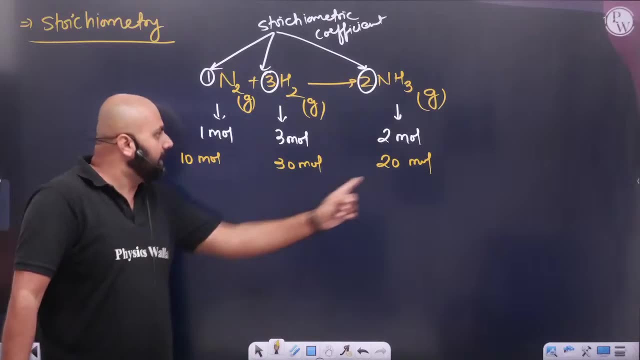 Same thing applies for reaction. If it is your wish, I said, sir said, multiply it by 10.. Take it, Multiply by 10.. But yes, multiply in all, Not just half and half. This is freedom in reaction. 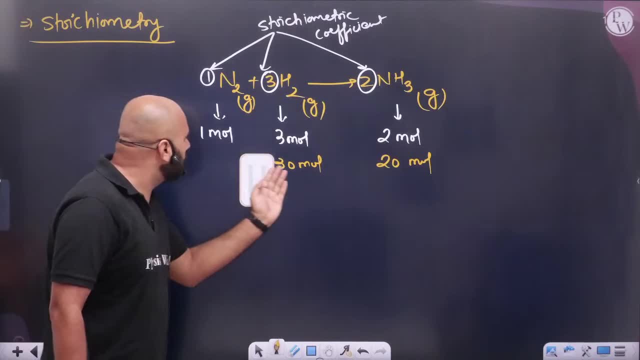 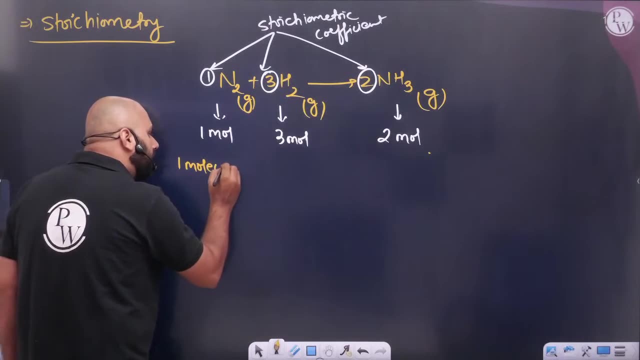 Whatever you do, you will do it for everyone. Okay, Whatever you do, you will do it for everyone. Similarly, who said, sir, let's do one thing, Let's divide it by the F-gatter number? If we divide it by the F-gatter number, then what will this be called? 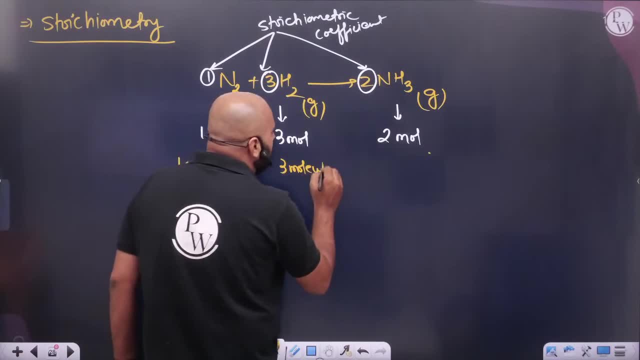 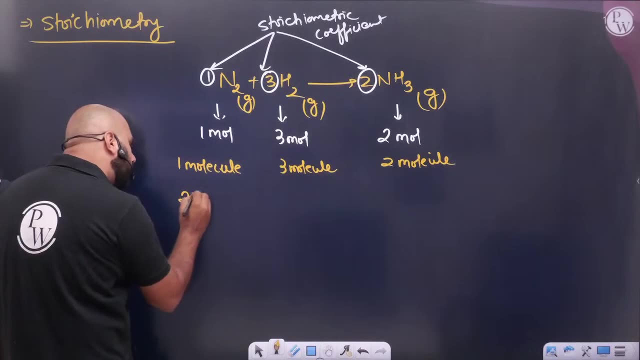 How is one molecule reacting From 3 molecules? And how is this reacting From 2 molecules? Okay, How is this reacting From 2 molecules? Similarly, sir, its 1 mole volume is 22.4 liters. Sir, how much will it be? 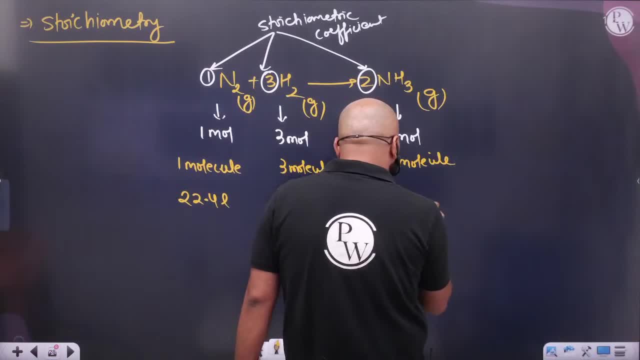 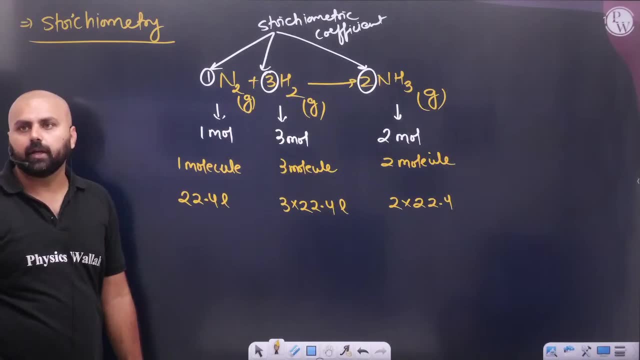 3 x 22.4 liters. And how much will this be, 2 x 22.4 liters, Sir? who said: put the volume instead of the mole. Put the volume. With whom did you multiply everyone With 22.4.. 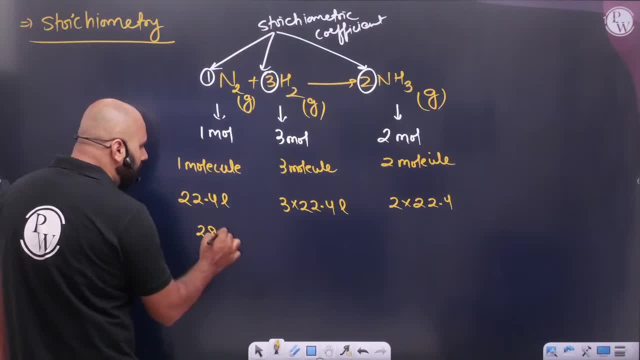 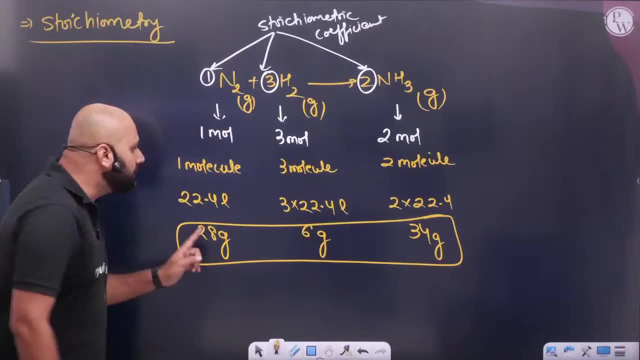 Second thing, Sir, last one, If we see the mass, then 28 grams, How much of this 6 grams And how much of this 34 grams. Remember, in the whole reaction there is conservation of mass. 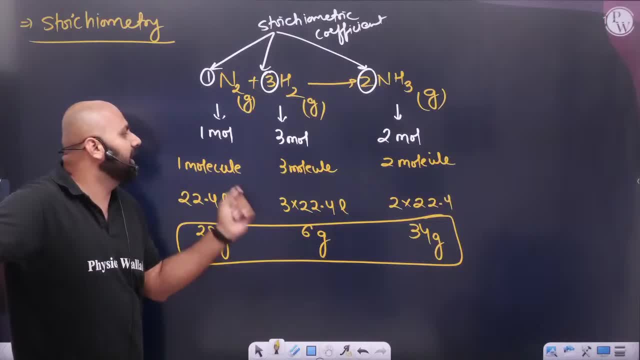 Mass is conserved, Mole is not conserved, Molecule is not conserved. Mass and atom are conserved. That's why listen carefully. What does stoichiometry mean, Sir? moles are not conserved, Molecule are not conserved. 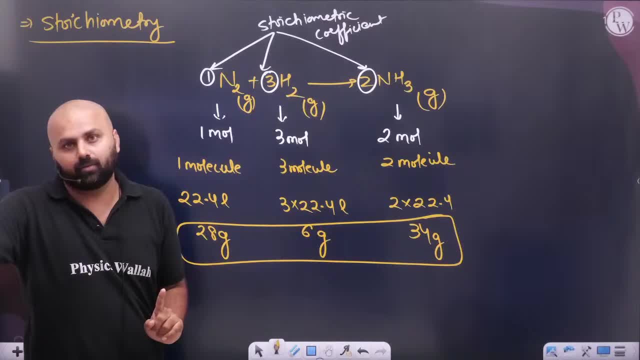 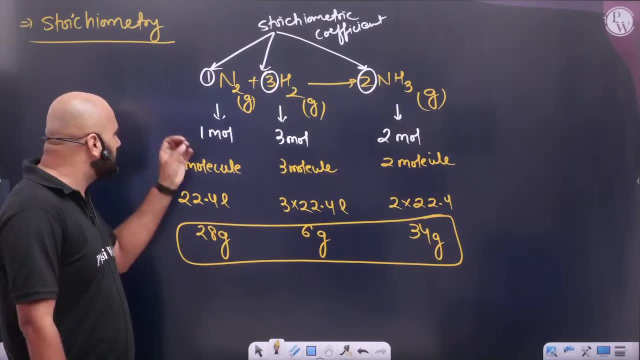 What is conserved? Atom and mass are conserved, See volume is not conserved, So volume is not conserved. You have to keep this in mind, Sir. volume is not conserved. Molecule is not conserved. 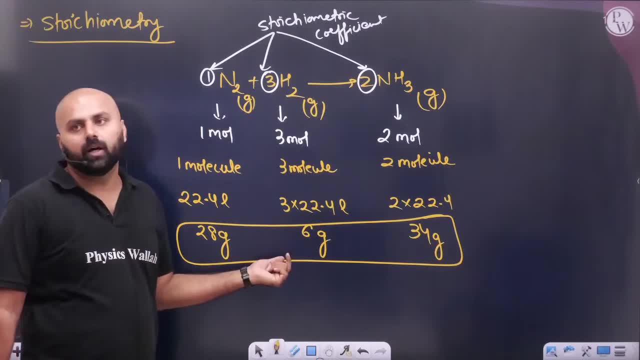 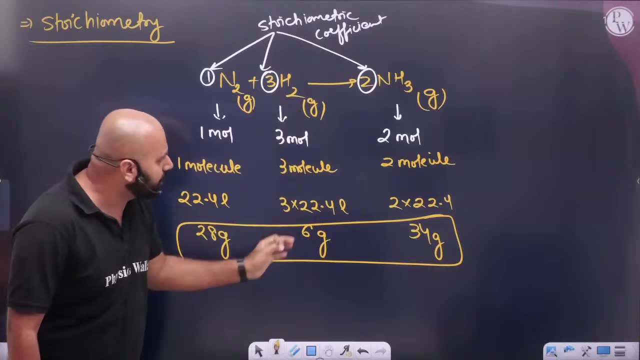 What is conserved, Left and right side will be equal. Mass will be conserved. Molecule will not be conserved. Atom will be conserved. If you learned to write this, if you learn to write this, sir, looking at any reaction, I can write these words. 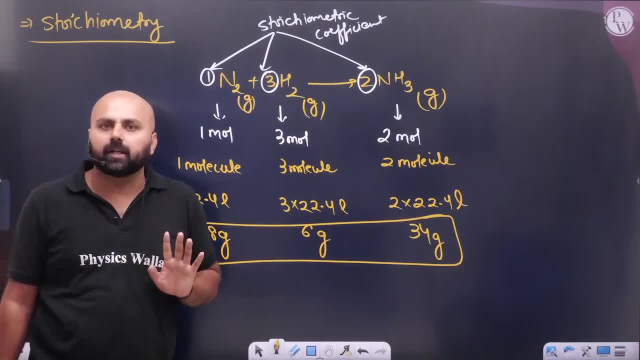 I can write this word by looking at the equation. So I will tell you a simple trick. Stoichiometry is as easy as that. Stoichiometry is as easy as that. What will happen? Stoichiometry is as easy as that. 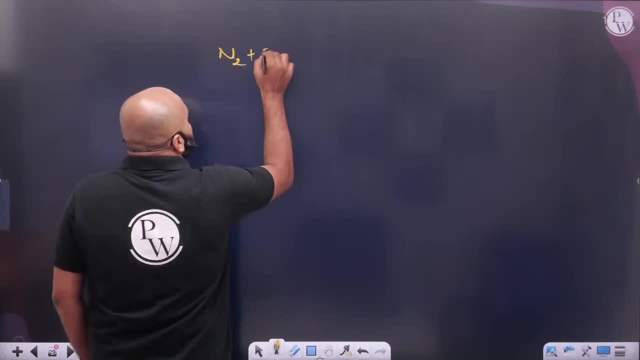 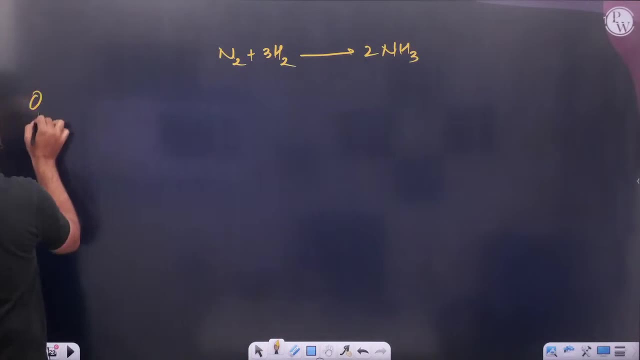 How See this? Someone has given you, No matter how the question is written in the language, it will be very easy in your life. You don't have to do anything. Suppose I have given such a question, If 10 mol of 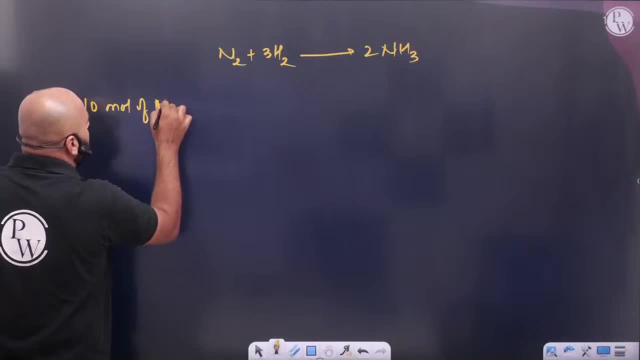 Hydrogen is 10 mol of Nitrogen is used in Haber's process. Everyone knows the name of this process. If you are using 10 mol of Nitrogen in Haber's process, then now see what will be asked in the exam hall. 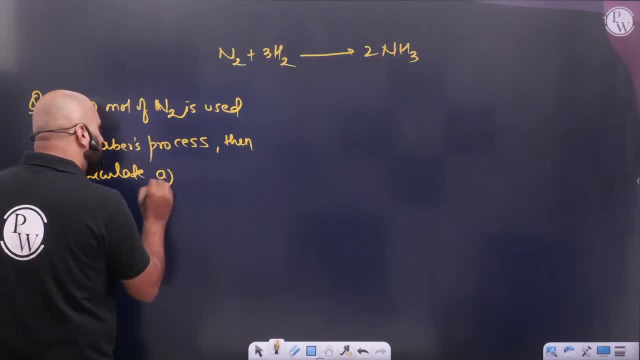 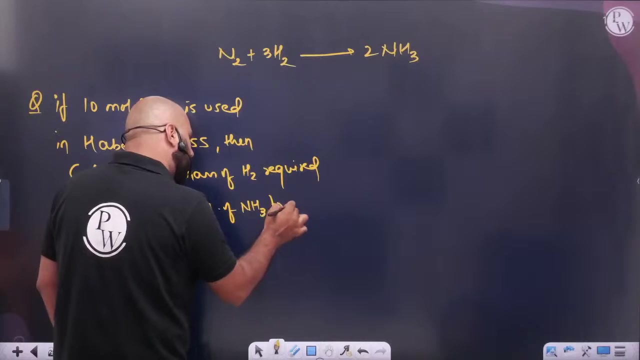 Calculate. Who asked you Mass of H2 required. Mass of H2 required. Second one: Who asked you Volume of Ammonia produced. Brother, don't do anything. I will tell you a simple method. We will use that method to answer the questions. 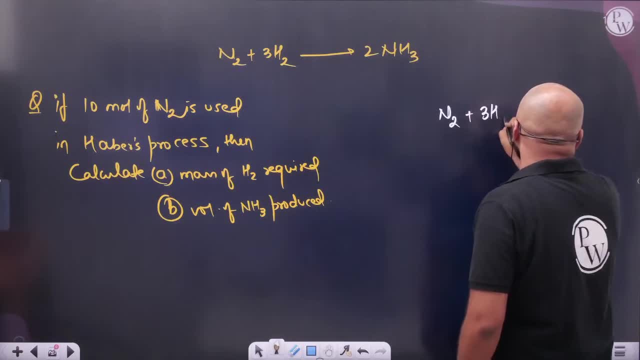 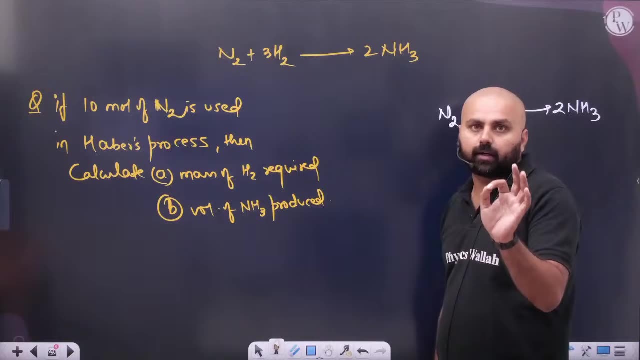 Within seconds. There is no reaction written. You will get the reaction written in the exam hall. If you don't get it, then write it on the side. Nothing. I will tell you a simple method: Listen to the story. What is given in it? 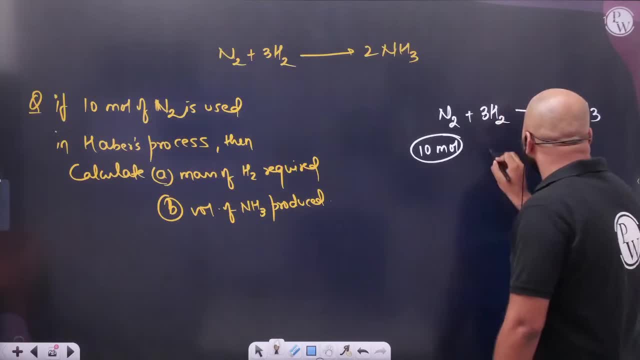 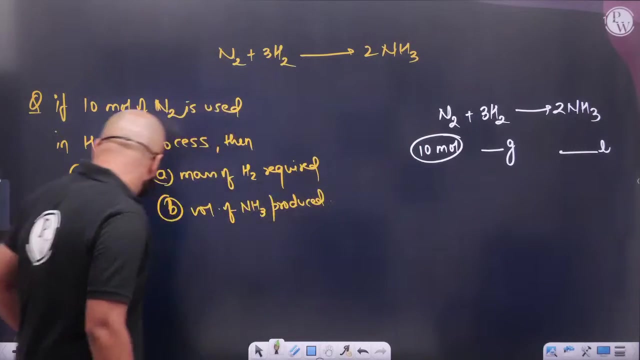 10 mol. I will write the given below. This is my given. What do I have to get out of it Mass? What do I have to get out of it Volume Calculate Now, see carefully The standard given above. 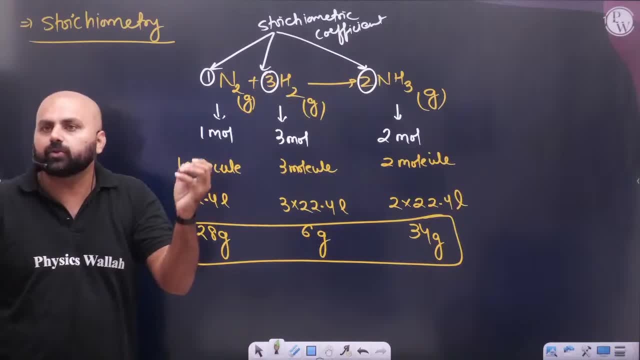 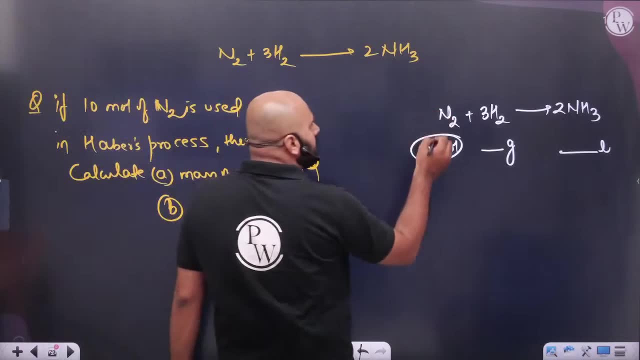 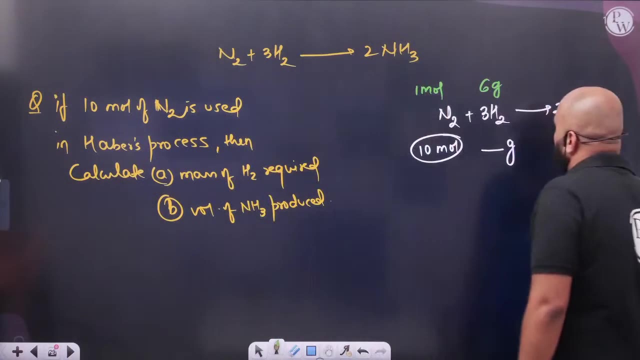 Standard means the reaction. without thinking, Without looking, You saw the reaction. The same thing, The standard. you could write How many mols are reacting. One mol is reacting. How much mass is being produced With 6 grams? If you want mass, then what is written above? 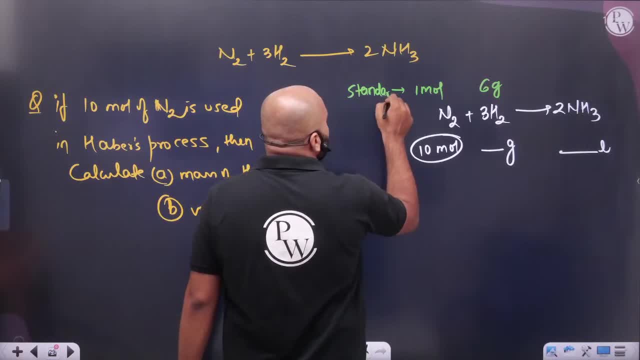 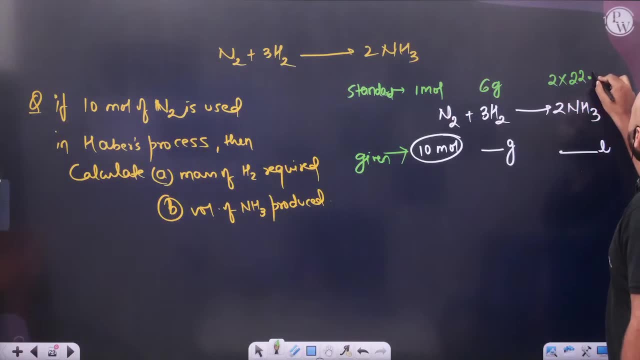 Mass? How? Standard way, Standard way. And what is this Given, Sir? what does it require Volume? So what does it require Write volume? What does it require Write volume? How did you know It is 2 mol, So this is the volume of 2 mol. 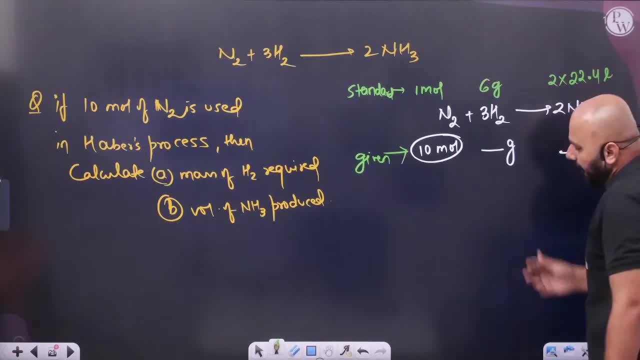 Sir, how much is its mass? 6 grams. How much is its mol? 1 mol. You write the standard And do you know how you can get it out within seconds? Do you want to get the value of this? Nothing. 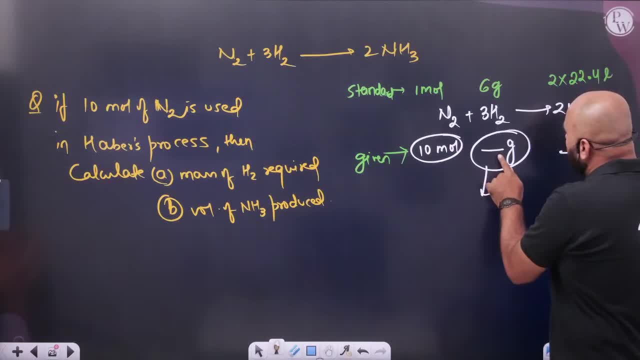 I will tell you a simple method: Nothing, It is given. Do you want to get the value of hydrogen? Nothing, 10 into See. Do you want to get this out? Nothing, This The given. Multiply it with its standard. 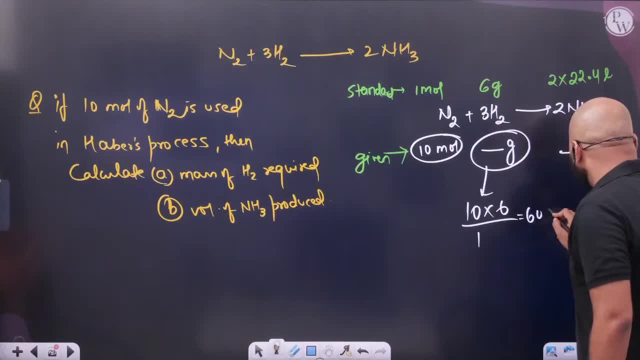 Divide it by. Divide it with its standard. How much will it be? 60 grams, Sir. if you want to get this out, then nothing. Do it again. 10 into. How much will you do? 10 into? 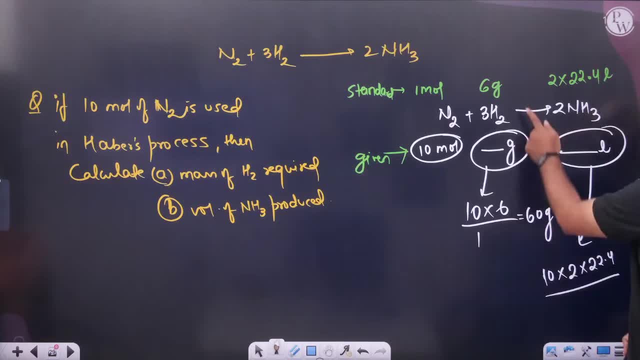 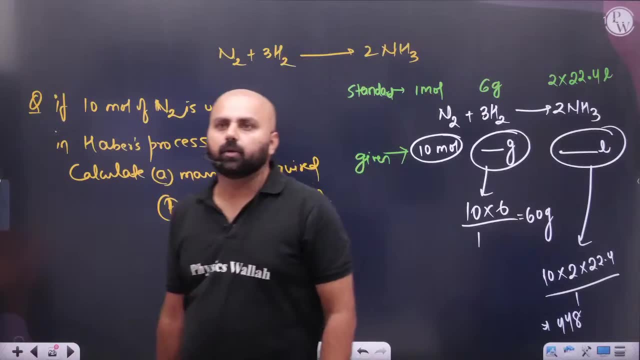 2 into 22.4, divided by How much will you do 1.. How much will it be 44.8.. This will be the result. This will be the result. Keep doing. You are being told a simple. 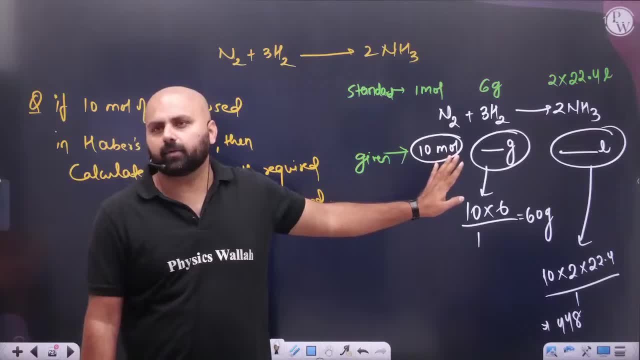 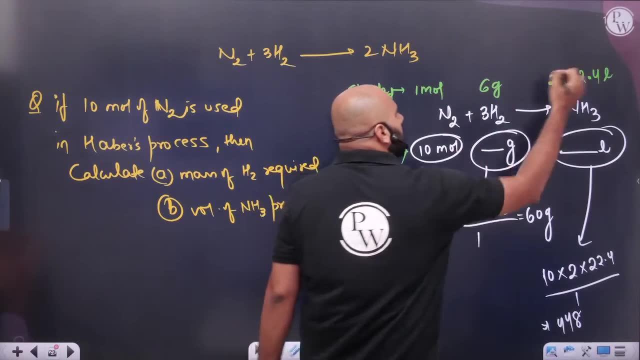 shortcut. You just have to do this much in the exam hall. Just keep this in mind: This given: Multiply it with the standard of the other person. Divide it by this. Multiply the given with this. Divide it by this Within seconds. the answer will start coming. 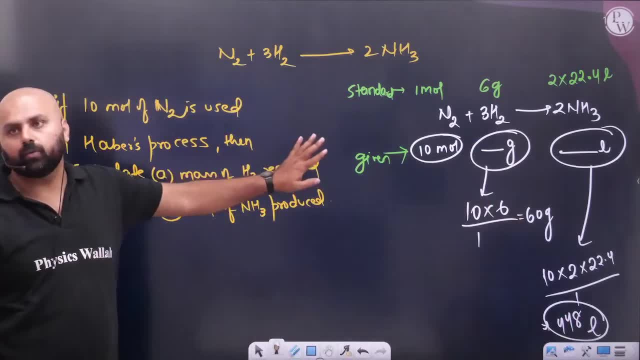 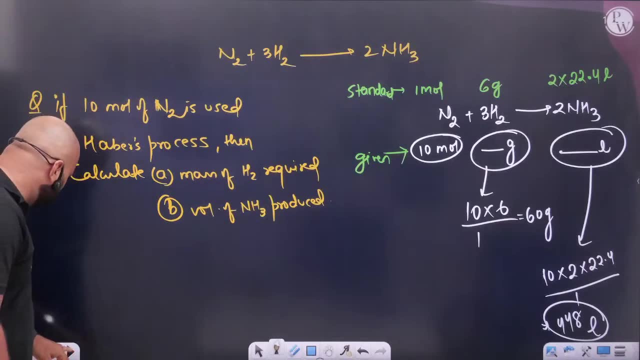 Within seconds, the answer will start coming. So this is my basic concept of stoichiometry. Now different concepts will come in this, But first let's see one more thing. What is that? The question of NEET 2019.. The question of NEET 2019.. 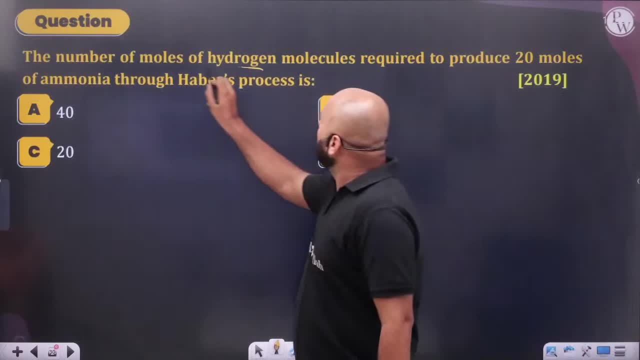 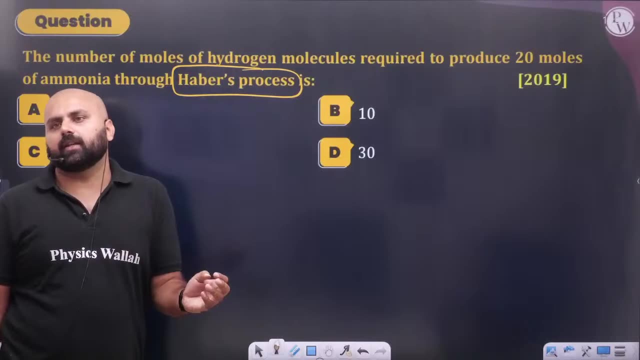 When will there be a reaction in this? It will never be given. Everyone knows the Haber's process. This reaction is a previous year question, Very easy In the exam hall. only easy questions come. Remember, Only easy questions come. It is just on you. 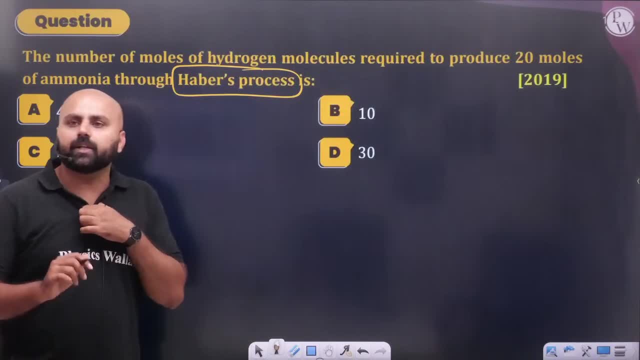 How are you looking at it? How are you looking at it? Don't worry about the exam hall. The same questions will come in the exam hall. Okay, See this. What to do. What is being said in the Haber's process? 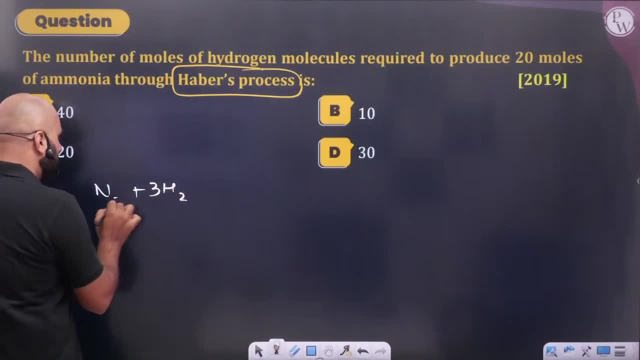 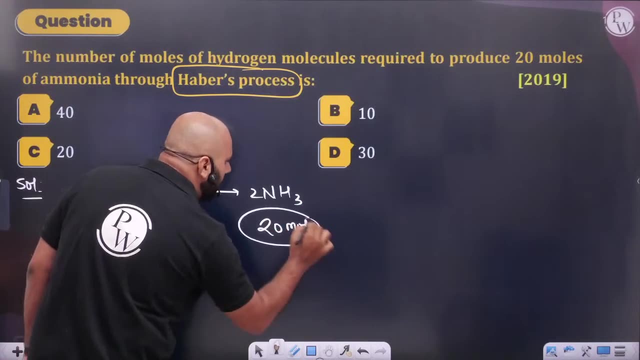 See again H2.. 3H2 plus N2.. What is being made? 2 ammonia. What is being said, Sir? 20 moles of ammonia has to be made. This is given in the exam hall. This is given. 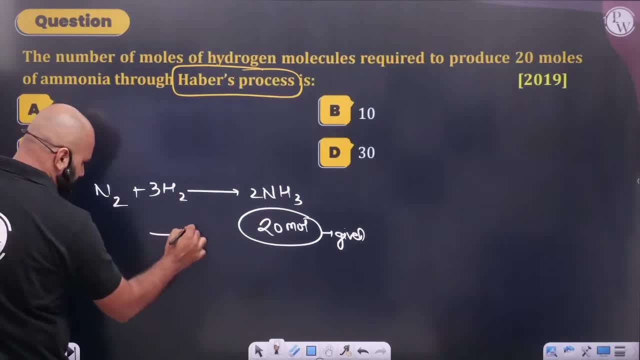 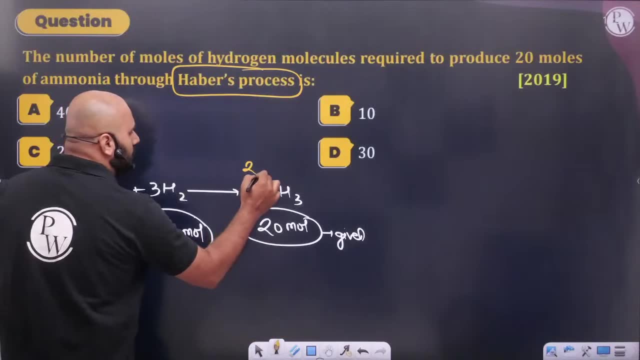 What do you want? The exam hall is saying: we need hydrogen moles, We need hydrogen moles, Nothing. If you don't want nitrogen, then don't even write. Just see this: 2 moles are reacting, 2 mole formation. 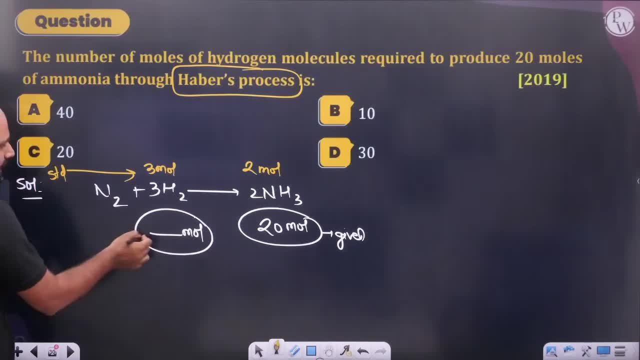 Why is it happening? 3 moles. Did you write the standard? Write the standard above. This has to be taken out Nothing. With whom to multiply the given. With whom to multiply the given? How much will it come? 30 moles. 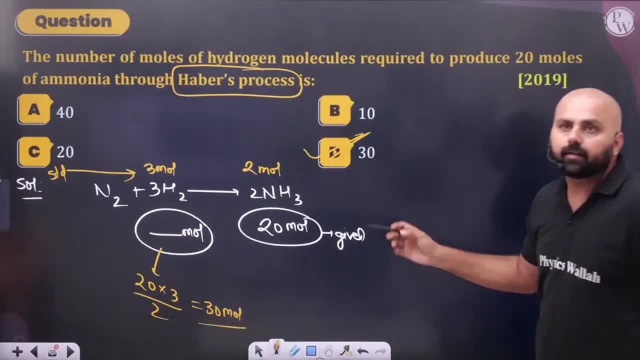 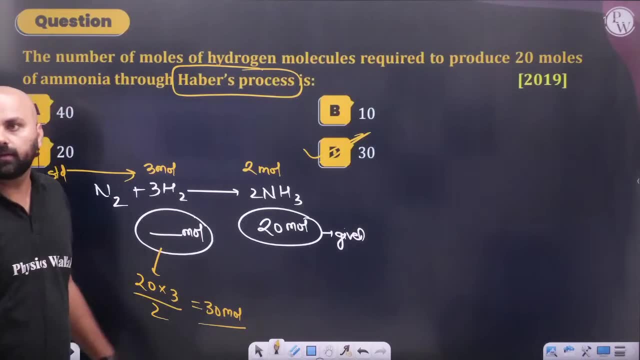 In the exam hall. you just have to give this much time and get the answer. What will be the answer? 30 moles. Just keep doing it. Okay, It will happen. If you are sure, then it will happen. You have to do the questions. 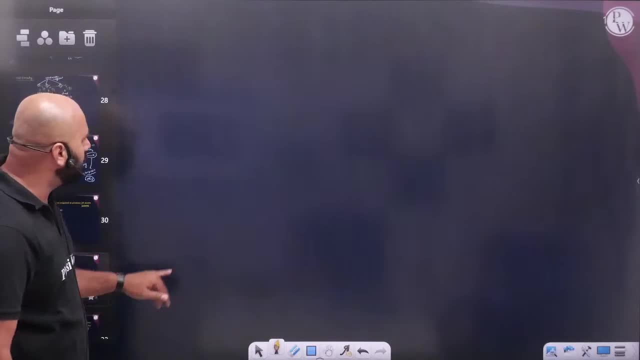 If you do the questions, you will start knowing. If you see the concept of purity, what happens in purity. There is only one problem in purity, In the concept of purity and in the concept of yield. If the concept of purity is being given. 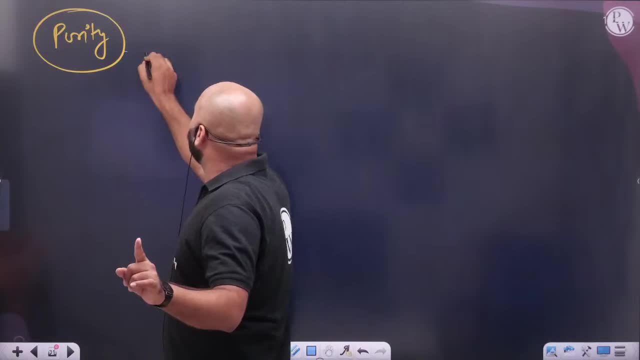 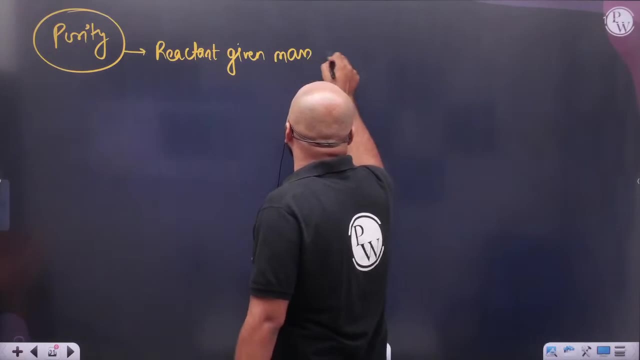 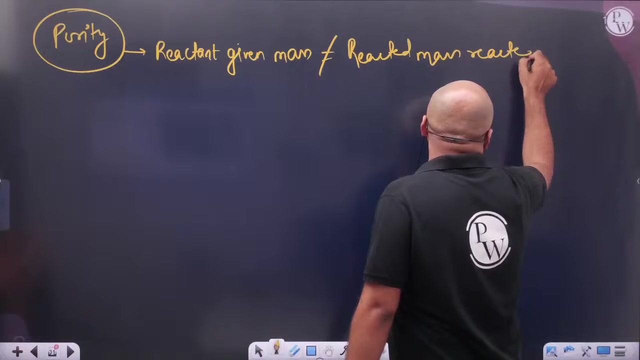 if the concept of purity is ever asked, then remember of reactant, remember the given mass of reactant. the given mass of reactant that is not equal to reactant's mass reacted. Sir, remember, Just remember one thing in your mind: 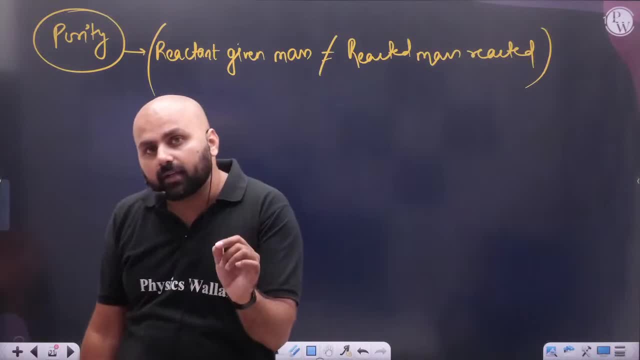 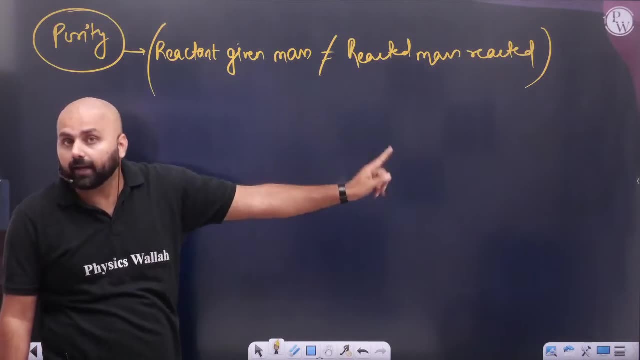 If the concept of purity is given in the question, then you have to remember that the mass given in the sample of reactant, the given mass, will not be equal to the reacted mass. Why not? Because it is obvious If you take 100 grams of calcium carbonate. 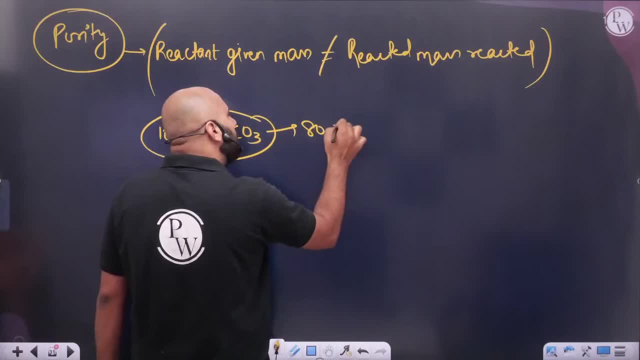 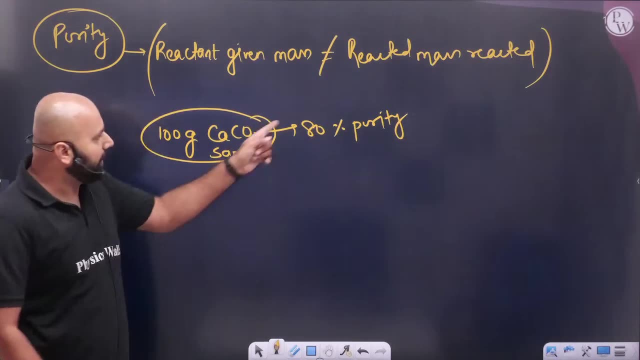 and write next to it that it has 80% purity, It has 80% purity. If I take 100 grams of calcium carbonate sample and write next to it that it has 80% purity, What does it mean? That 100 grams of calcium carbonate 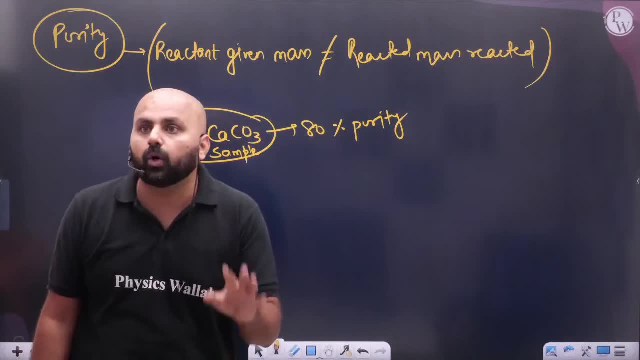 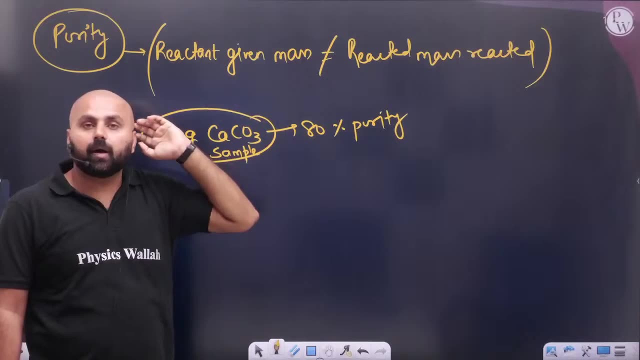 will not react fully Whenever you sit in the reaction, then what will happen? Reacted mass will be different. Reacted mass will not be 100 grams If you keep this concept in your mind, that whenever purity is a concept, the given mass of reactant. 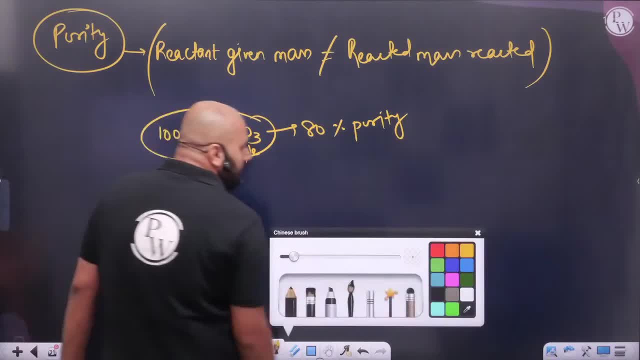 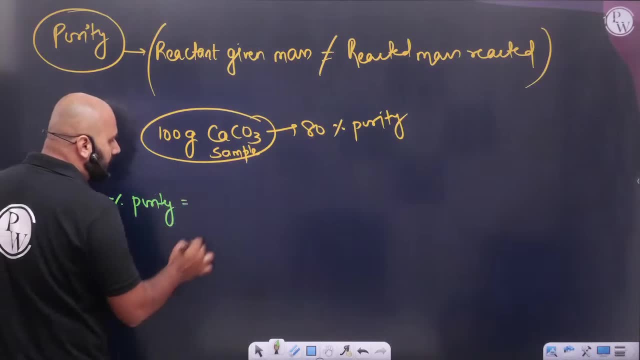 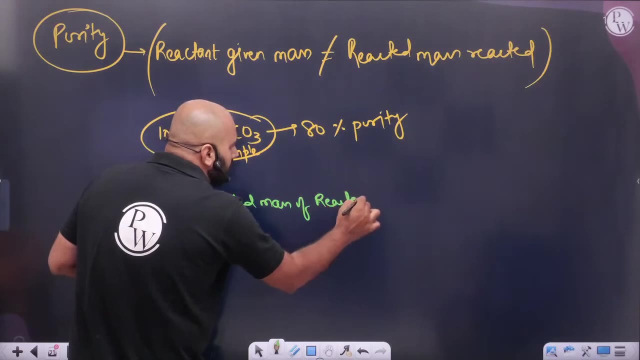 that is not equal to reacted mass. Second thing: How do we find the percentage purity of the reacted mass? How do we find the percentage purity? You have to find the percentage purity, So the reacted mass of the sample of reactant divided by 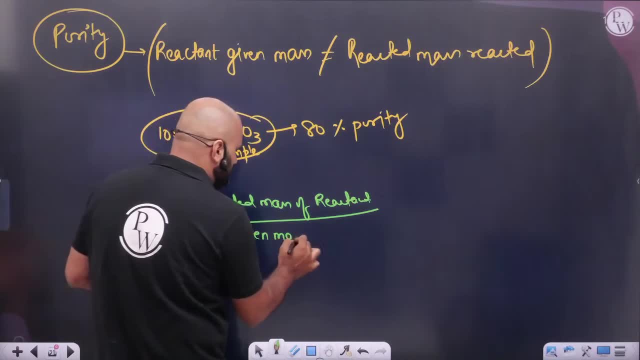 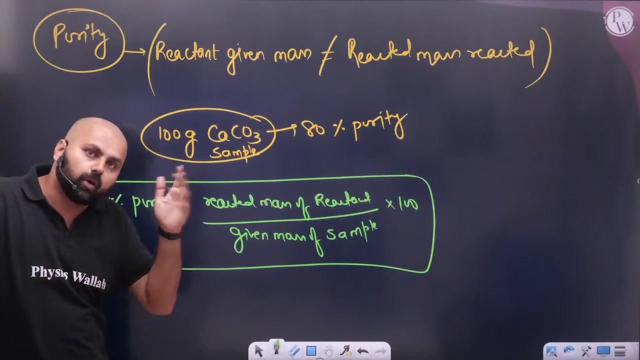 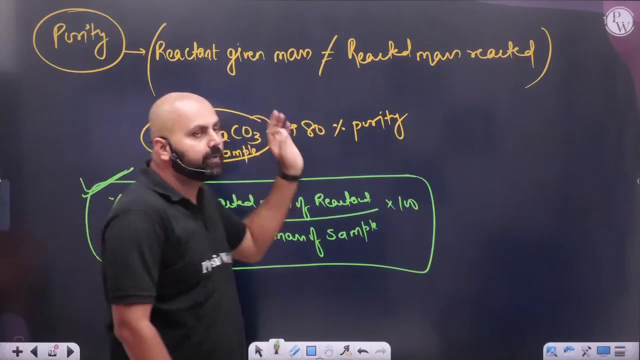 given mass of sample into What do you do? Do 100.. You will get it. Do 100.. Keep finding the percentage purity. Just remember that never take 100% in purity questions. If you take 100%, why? How did it go? 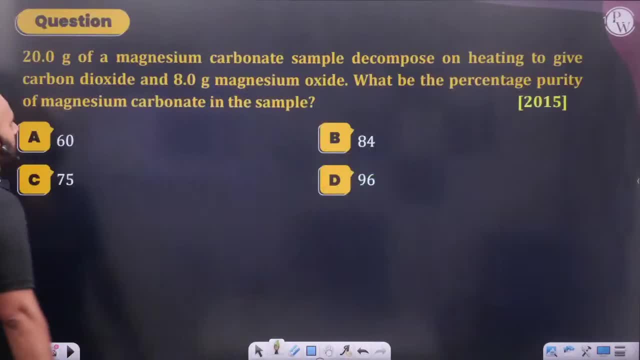 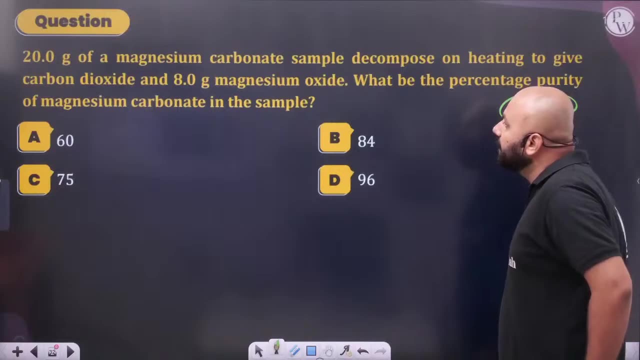 You will get to know Now. you will see the question. Whenever the percentage of purity comes, you will get to know In 2015,. a question was given. Magnesium carbonate is decomposed. Magnesium carbonate is given 20 grams. 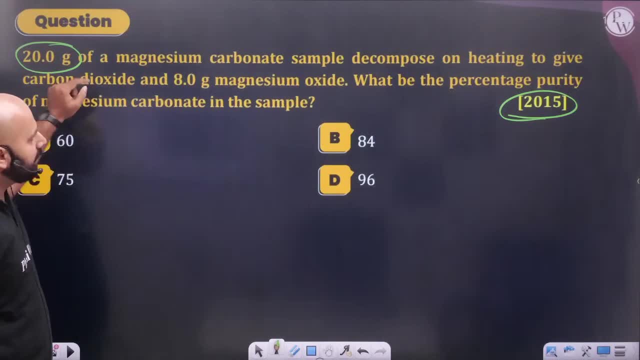 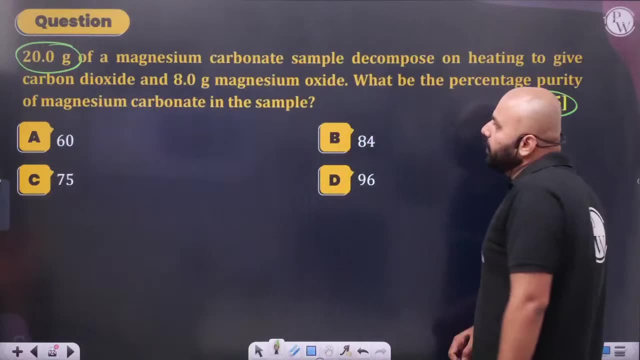 I can't say in the question that it is a purity question. But how do we know? It is decomposed, What is given on heating Carbon dioxide and 8 grams of magnesium oxide? What will be the percentage purity of magnesium carbonate? 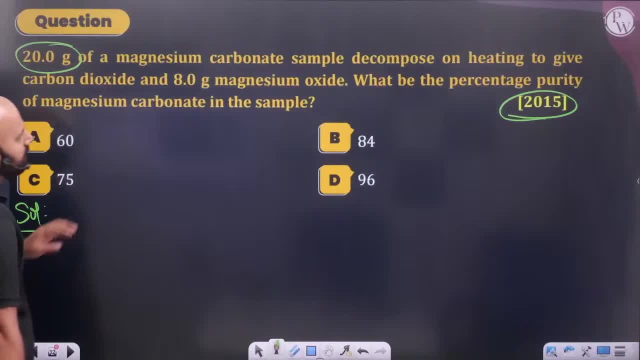 As soon as it was said, understand that 20 to 20 grams of magnesium carbonate is not reacting. 20 to 20 grams of magnesium carbonate is not reacting. 20 to 20 grams of magnesium carbonate is not reacting. We have magnesium carbonate. 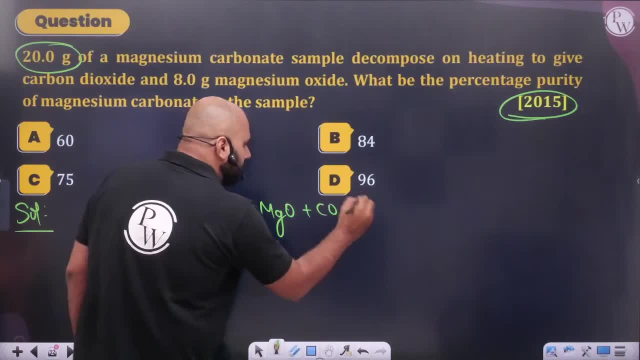 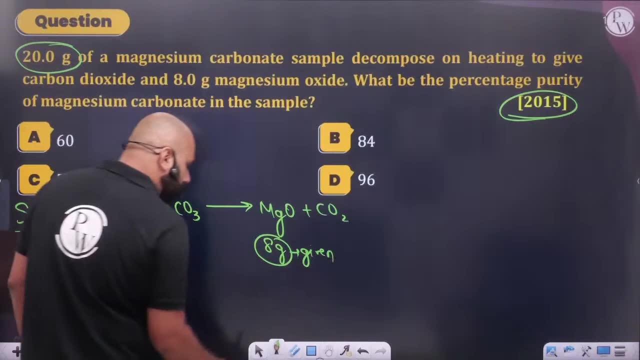 Magnesium carbonate is decomposing. It is written in the reaction. You see it like this: One thing has been told to you: What is given to you. You are given 8 grams of it. What you have to do? Take out pure magnesium carbonate. 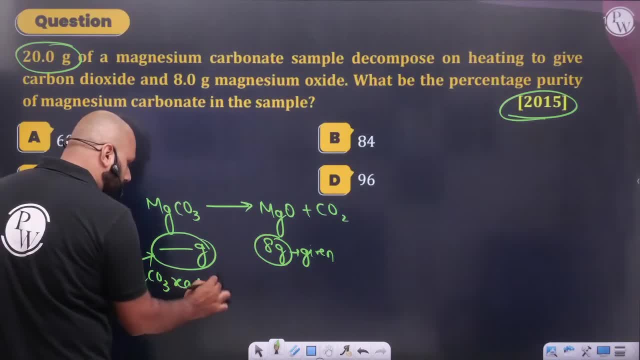 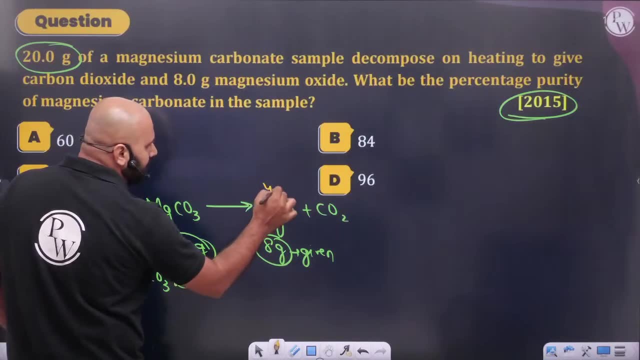 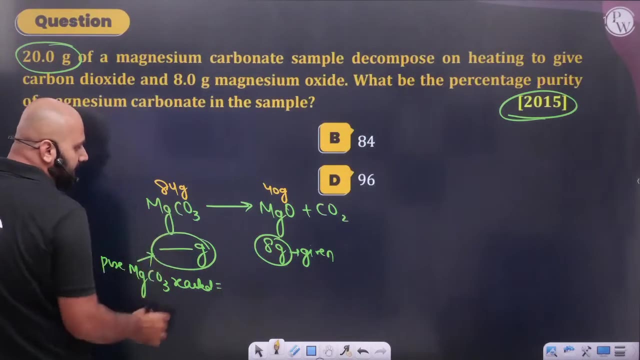 which is reacting. Take out pure magnesium carbonate, which is reacting. How will you take it out? Nothing. You see What is the mass of this Magnesium: 24.. 40 grams. What is the mass of this Magnesium, 12 plus 60.. 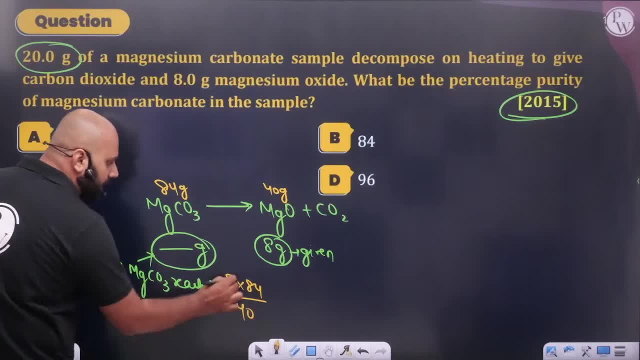 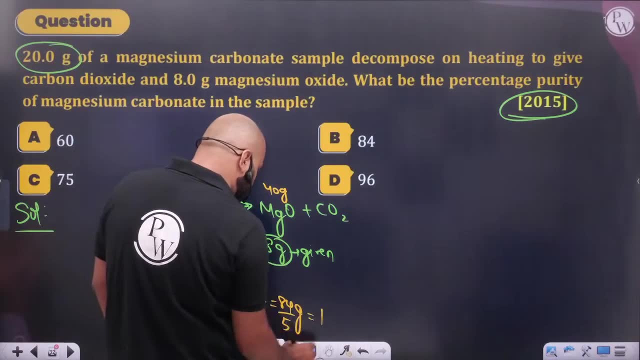 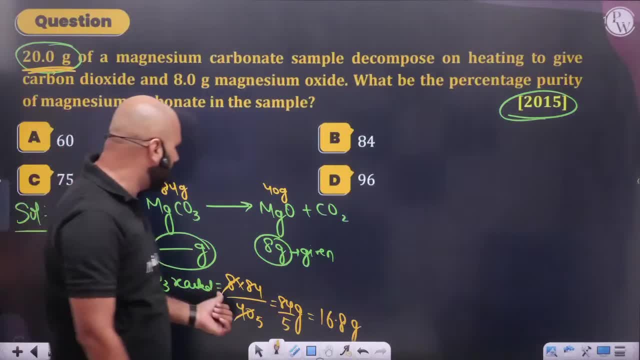 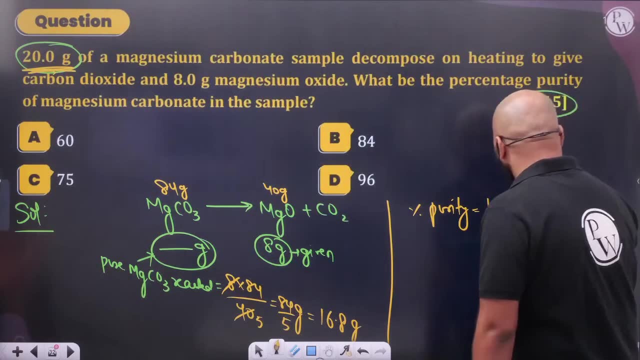 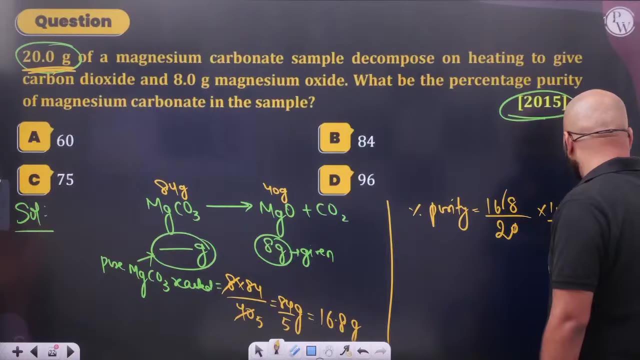 You had 20 grams of magnesium carbonate, But magnesium carbonate is not reacting. If you take out percentage purity, 16.8 divided by 20 into 100.. If you take out solution, How much is this 10.. And this goes from 0 to 1.. 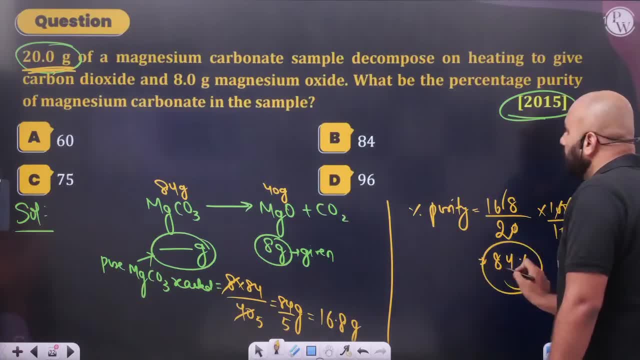 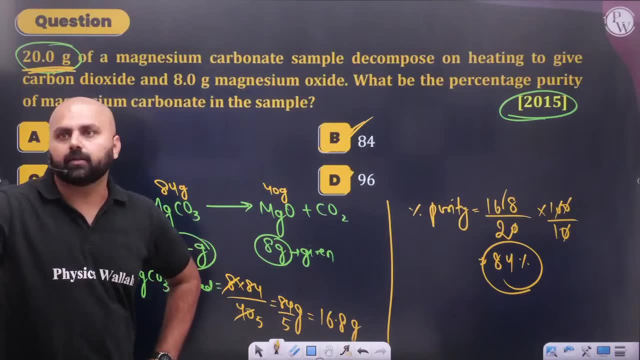 168.. How much will it be 84 percent? How much is purity 84 percent? Keep taking out. Keep taking out 84 percent. Are you sure? Then you have to do this work. You are only asking questions. 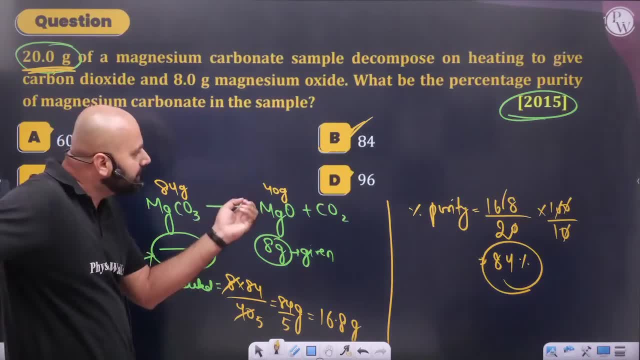 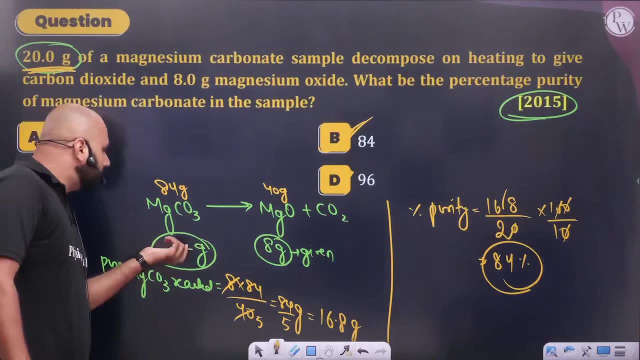 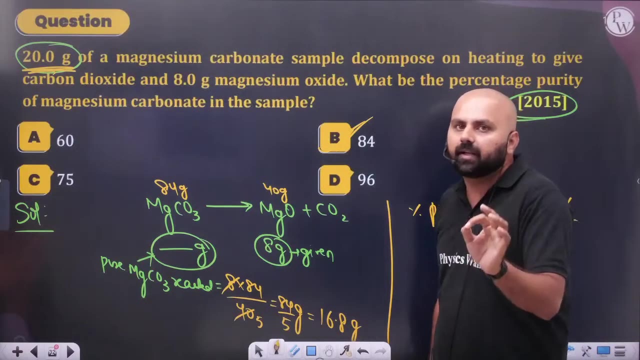 Whenever you are asked a question, then you have to take care of one thing: My percentage purity. Whenever someone asks you to take 20 grams of its mass, You are making a mistake. The concept of purity is that the given mass of reactant 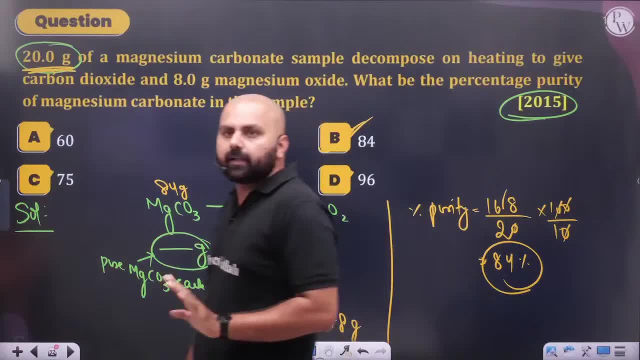 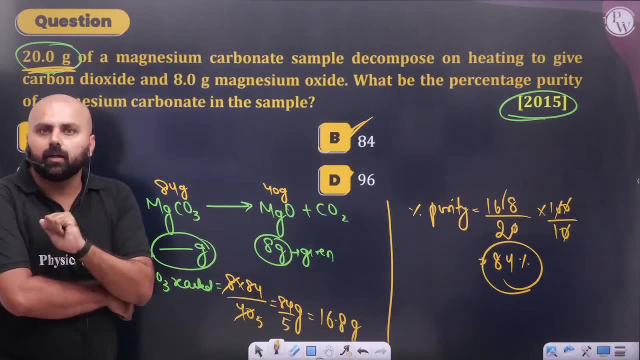 cannot be taken in reactant. It is the same way. You should never take the mass of reactant. If you take 20 grams, Then how will you know? Then what will you know? It is better to take it once. What do you get out of this? 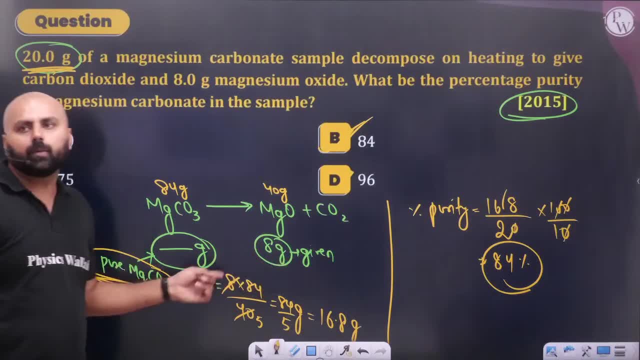 Pure magnesium carbonate. It must have come from this position. Then take it out by opposite. Take it out by opposite. Take it out by opposite. How much magnesium carbonate came from 8 grams of MgO. As soon as you get to know. 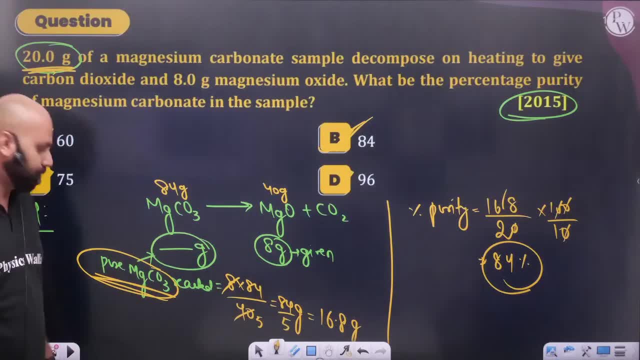 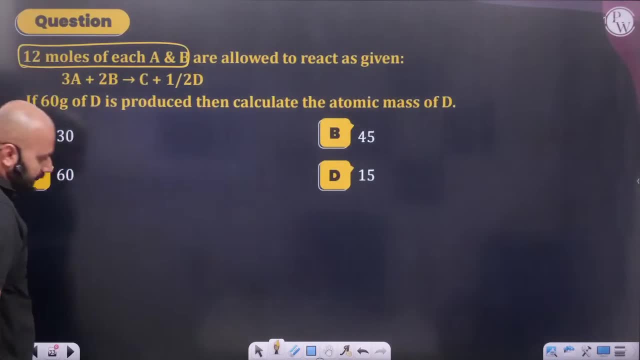 Brother, what does this mean? Only this is in the 20 gram sample. Then just do it, It will be done. Now look at the next. Now I am telling you the concept of limiting reagent. The concept of limiting reagent. 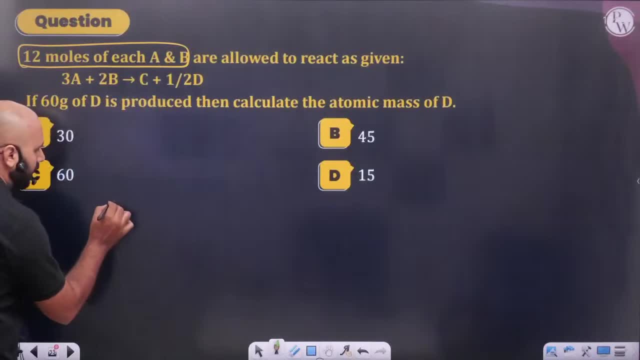 If you are very afraid of limiting reagent, Just do one thing in the exam hall: Write two extra lines. If you do not have a question of limiting reagent, Then you just write two lines. What is given? Both the moles are given. 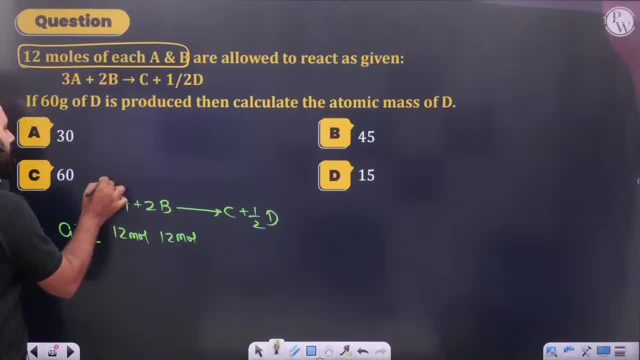 How much are its moles? 12 moles And how much are its moles 12 moles? See this: If you write the standard, Then its 3 moles, And how much will it be 2 moles? 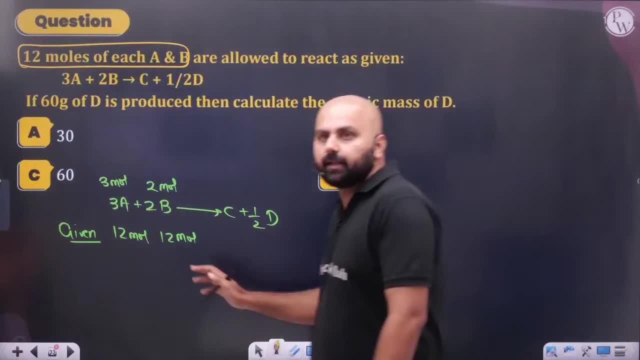 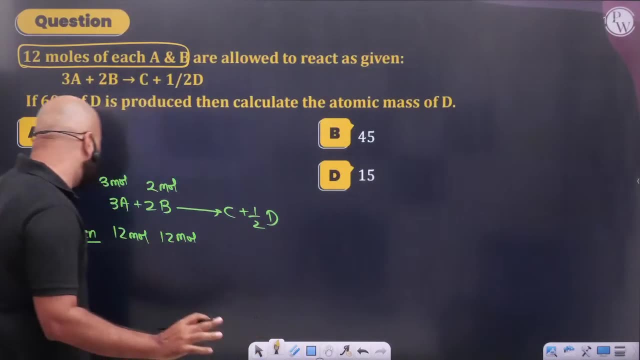 Its 3 moles. How will it be? See this, How will you do the question? If you have any problem in limiting reagent, Then just write one or two lines, Then the answer will come. I will write For complete reaction of 12 moles of A. 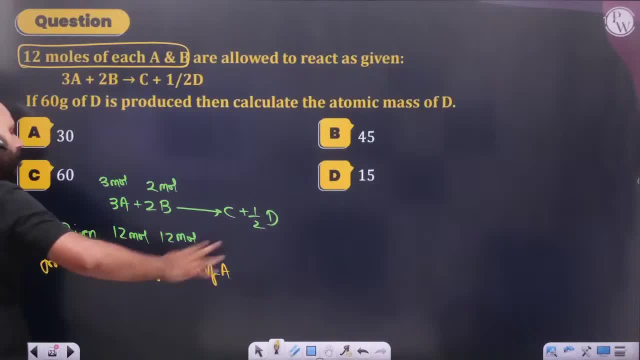 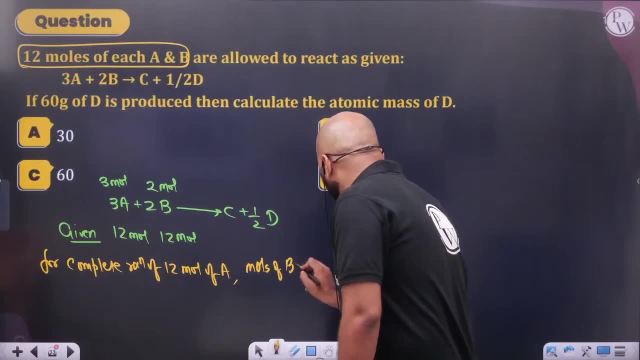 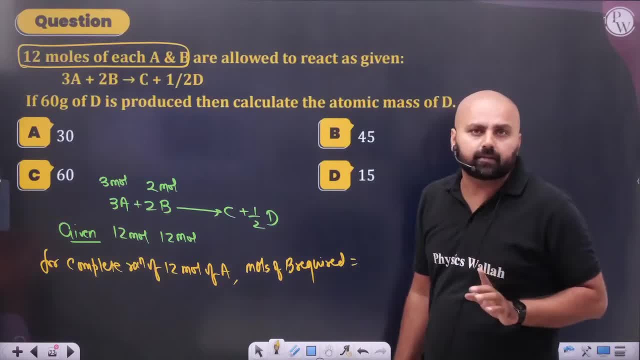 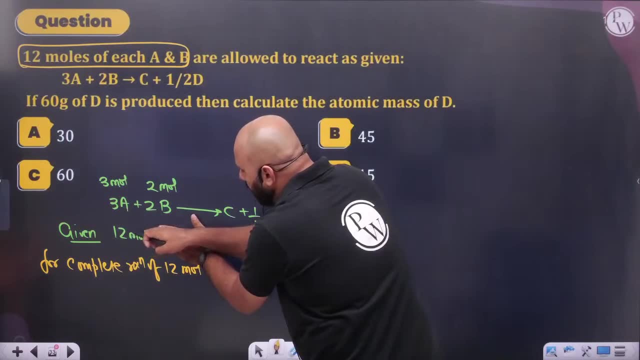 Because if you are still confused Then you will not get any shortcut. It is better to do one thing quietly, Sir. if 12 moles of A, If 12 moles of A, If 12 moles of A, Then what will come out of the unitary method? 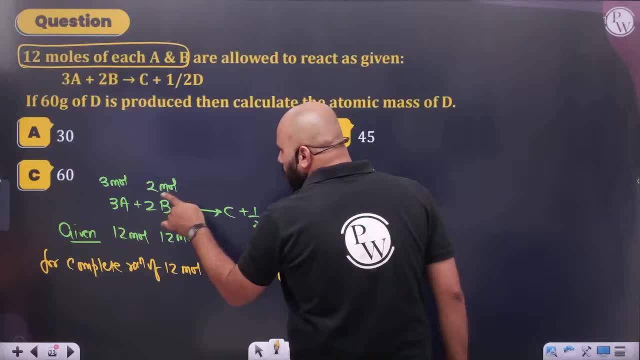 How many moles of B will be required? Sir, for 12 moles, how many moles of B will be required For 3 moles? 2. Sir, for 12 moles, how many will be required? 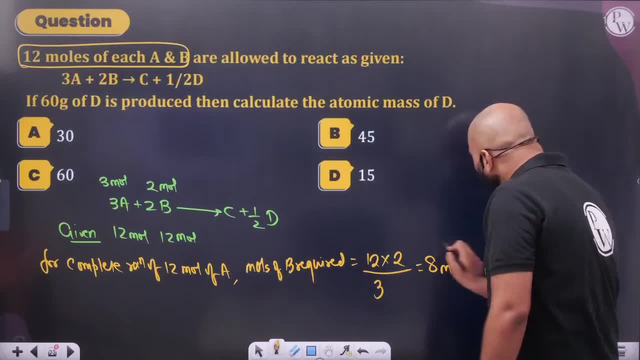 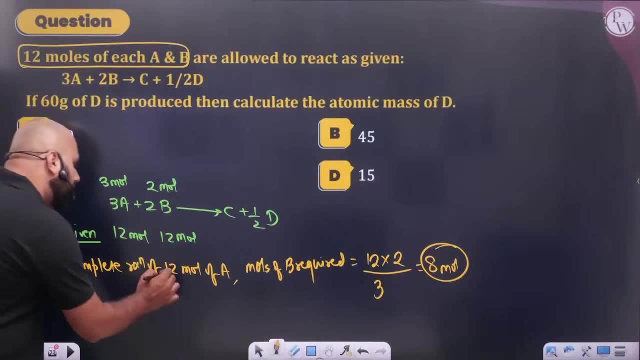 Sir, for 12 moles, how many will be required? How many will be required? 8 moles? Is 8 moles is given in the exam hall? If 8 moles are given in the exam hall, Means What happened to my A. 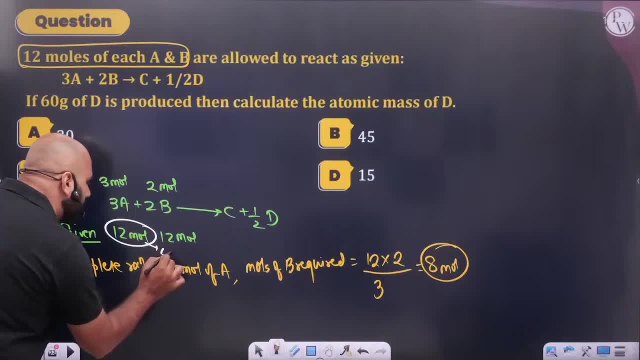 Meaning Laimiting Reiesent, Because A is completely react. How many are the moles of B? 8 moles will react, Sir. how many those who are un-reacted? How many are those who are un-reacted? How many are the moles of B? 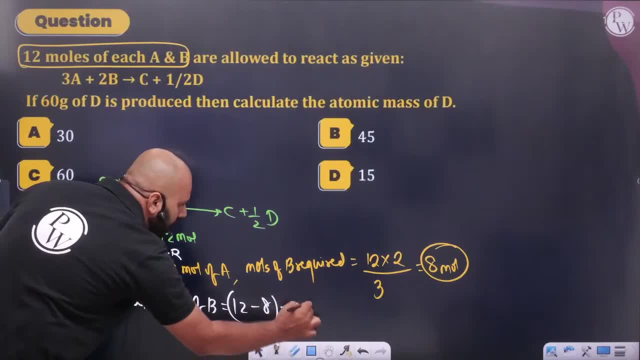 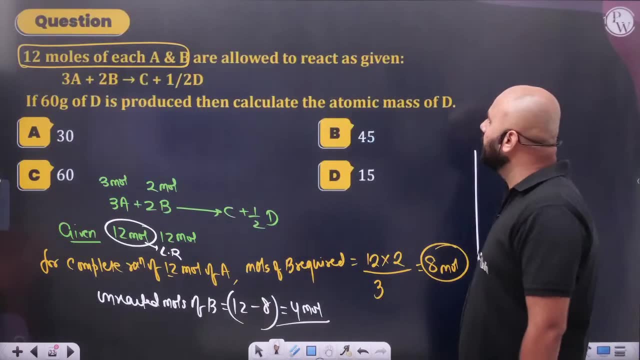 Sir, out of 12 moles, 8 will be react. How many of those who are 4 moles of B? They will be un-reacted. 4 moles of B will be unreacted. I don't want to extract the unreacted moles of B. 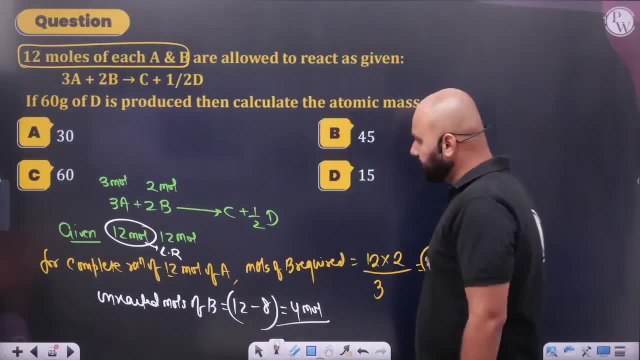 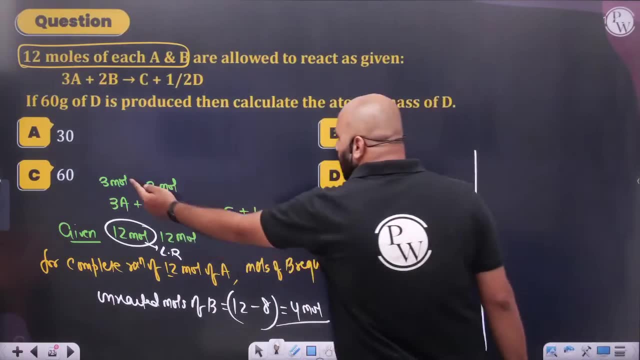 In this question. it is saying that 60 grams of D is produced. Tell me one thing, Sir: what does limiting reagent do? What does limiting reagent do? It decides the entire reaction. So look at the limiting reagent. 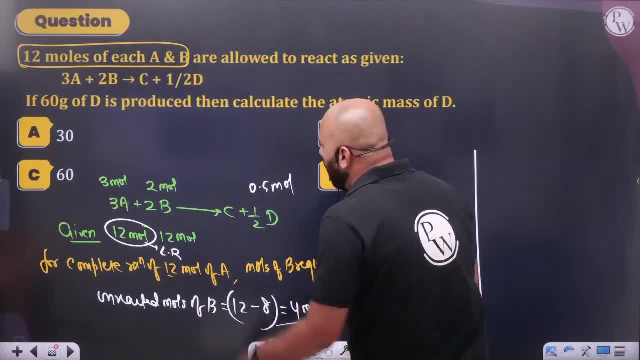 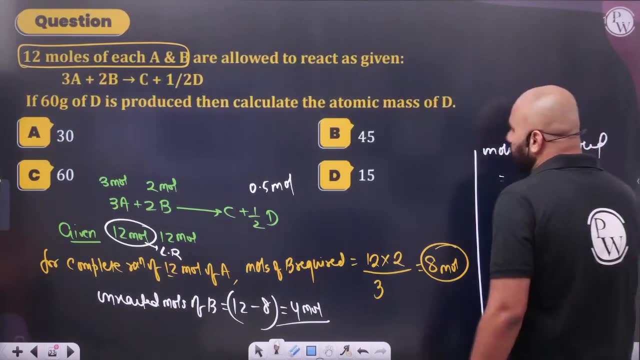 How much is being produced from 3 moles? 0.5 moles, Sir. then how much will be produced from 12 moles? Moles of D produced. You will go to extract moles of D produced. You will go to extract moles of D produced. 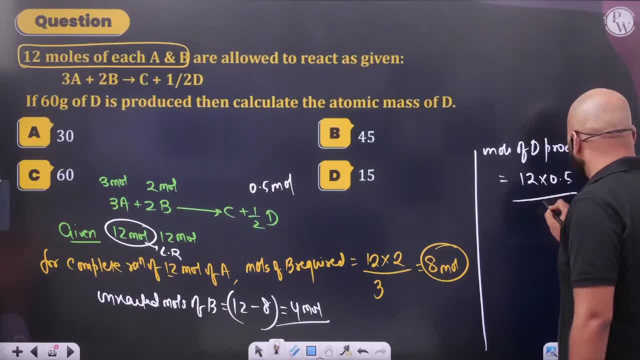 How much will it be? 12 into 0.5 divided by 3.. Divided by 3. How much will it be? 2 moles will be produced. And how much is the mass of 2 moles 60 grams? 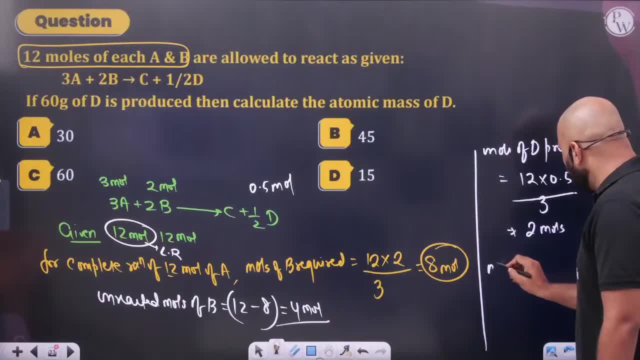 So how much is the mass of 2 moles? Mass of 2 moles. How much is the mass of 2 moles? Mass of 2 moles is 60 grams. So, sir, how much will be the mass of 1 mole? 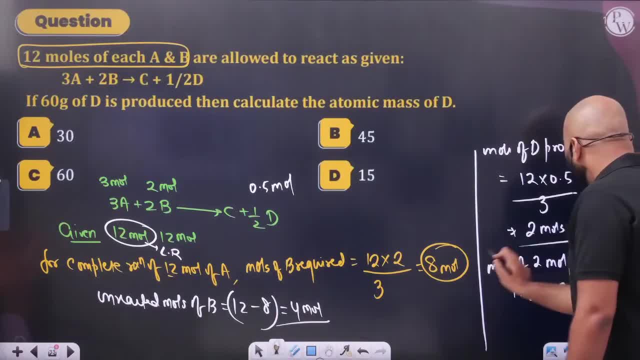 How much will be the mass of 1 mole 30 grams? If the mass of 2 moles is 60 grams, then how much will be the mass of 1 mole 30.. Take out the answer. A answer. 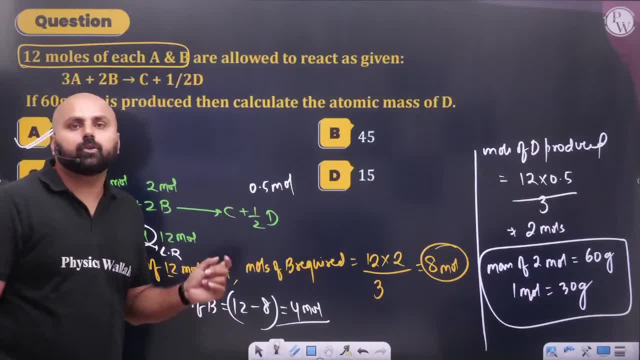 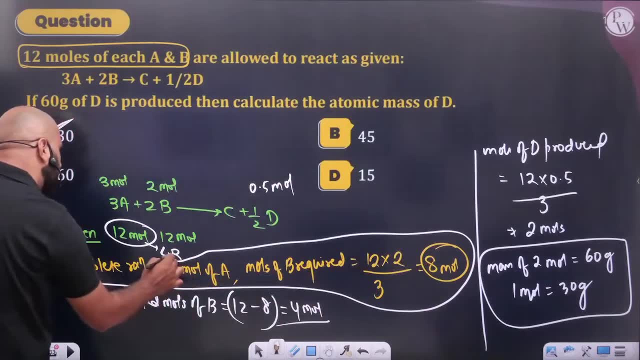 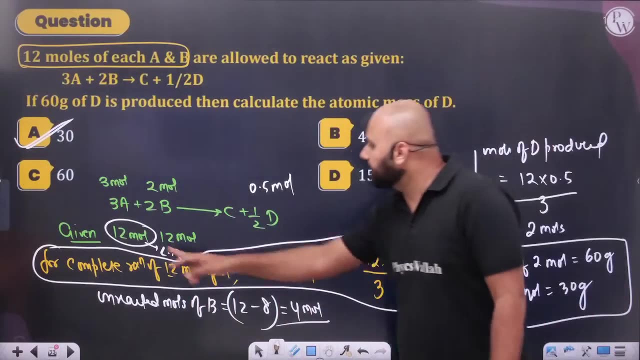 Whenever you have to find the limiting reason in the question, then write a simple line. If you write this line, then you will know that. if this does not happen, suppose someone is saying that: when did you get fit? If this does not happen, suppose here 20 comes instead of 8, then I would have assumed that this will not be able to react completely. 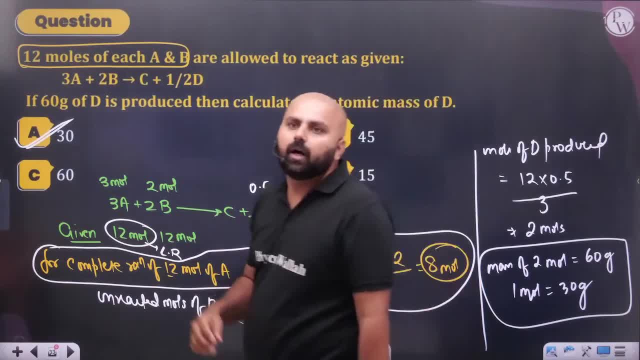 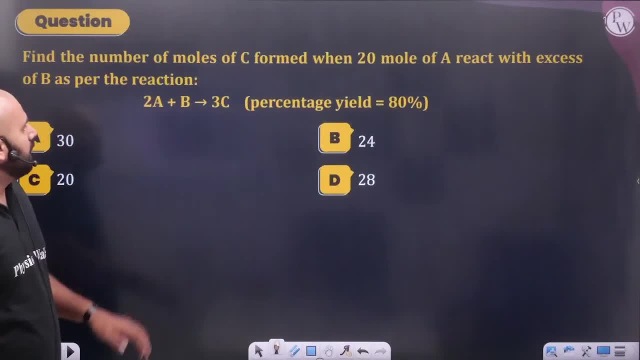 So, obviously, if this will not be able to react, then the next limiting reason will be there. If this will not be able to react, then the next limiting reason will be there. Keep doing the question, Sir. after limiting reason, see the concept of yield. 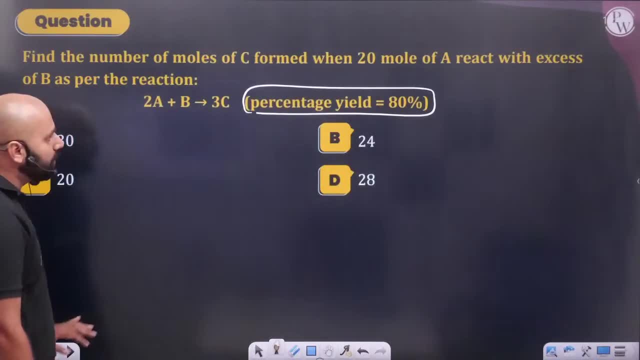 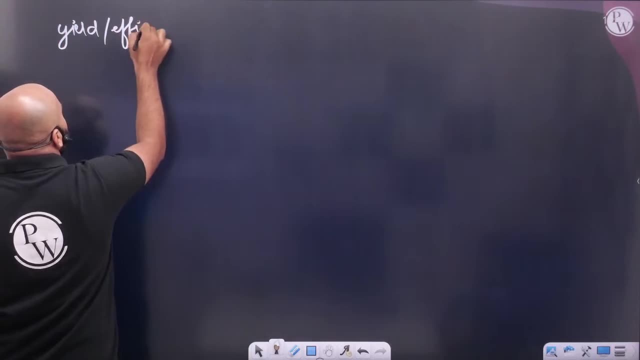 See, in the concept of yield, there is a difference between purity and yield. There is a difference between purity and yield. What is the difference between purity and yield? The meaning of yield is nothing. It means efficiency. What will happen to you? 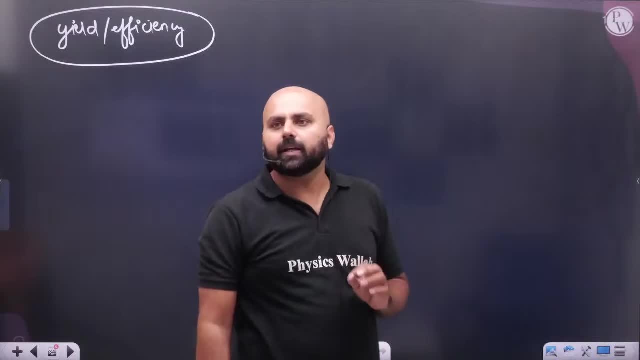 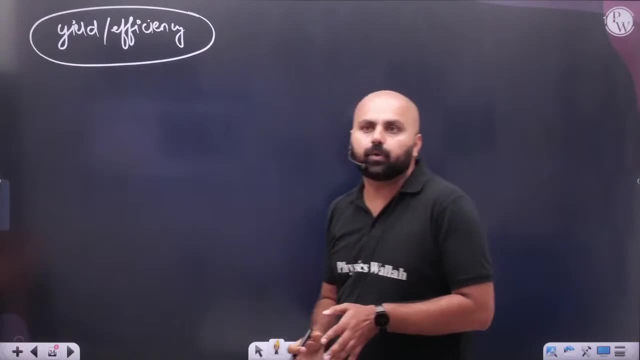 Efficiency will happen. Efficiency means that you are taking the reaction in. You are taking the reaction in, You are taking the reaction in. It is possible that the reaction will be old or the machines will be old in some time. So there, There. 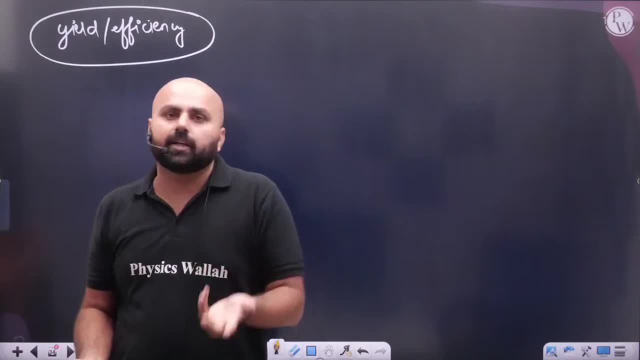 The one who knows how to do tricks. he can do tricks. Why? Because you will get the answer from the trick as well. But the person who is trying to learn- at this time he does not have any option. He will be able to do it by writing one line. 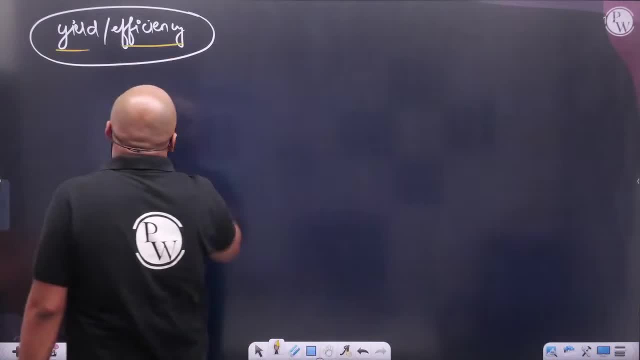 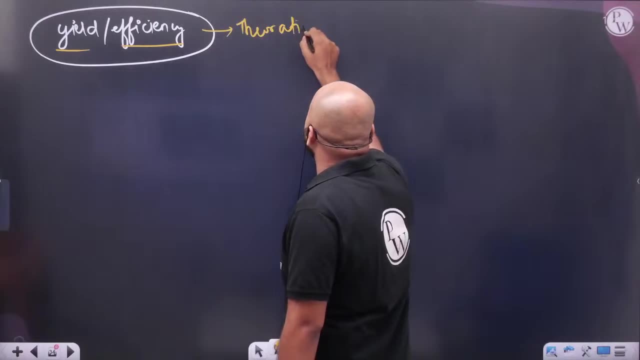 After that, I am talking about yield and limited efficiency. What is yield and efficiency? Just remember here that there are two types of things. One is, like you study, theoretical. There is theoretical yield, And one is observed yield. Theoretically, what do you think? 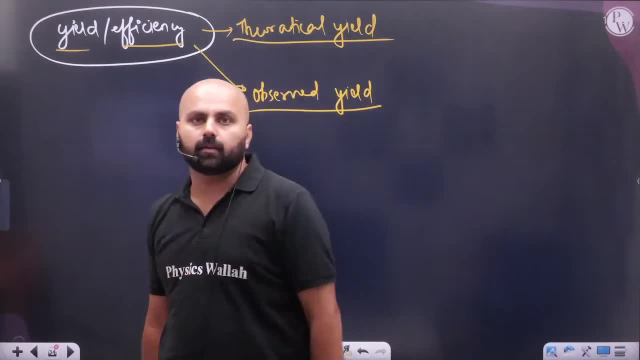 Sir, we will not be able to do it in 2.5 to 2.5 hours. Then a message comes, Sir, give me a break Why You will get the exam in the afternoon. You will not get it. 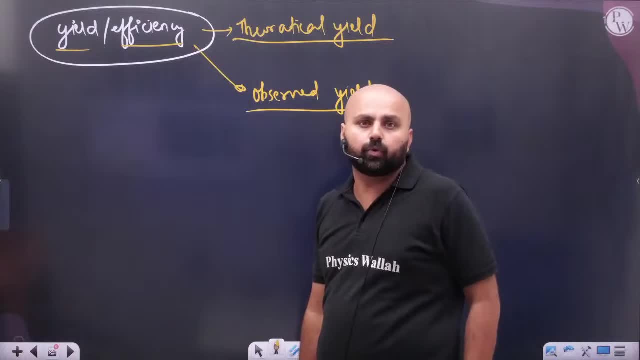 Till 2.5 to 2.5 hours. Just think about it. I go to sleep in the morning. The office class is over Today again, I will sit in the evening and study chemistry. Theoretically, I thought that I will wake up at 2 o'clock and study. 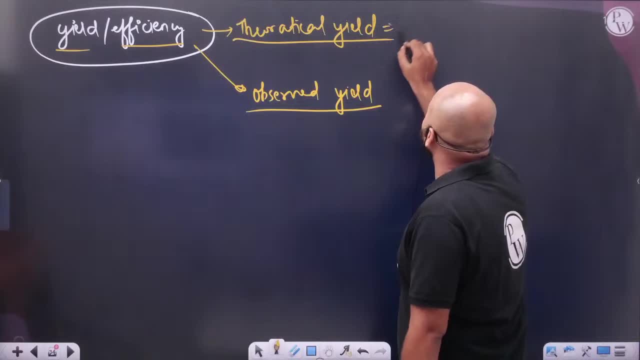 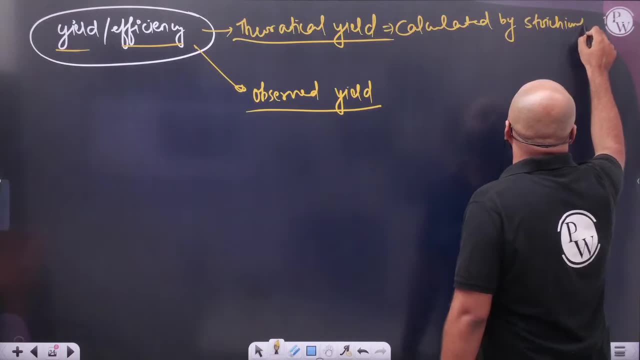 But I did not sleep. What is theoretical, Sir? where does it come from? Calculated by stoichiometry. From whom do we calculate? We calculate from stoichiometry. From whom do we calculate? We calculate from stoichiometry. 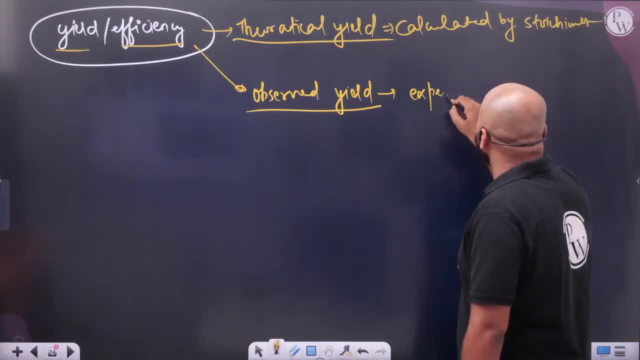 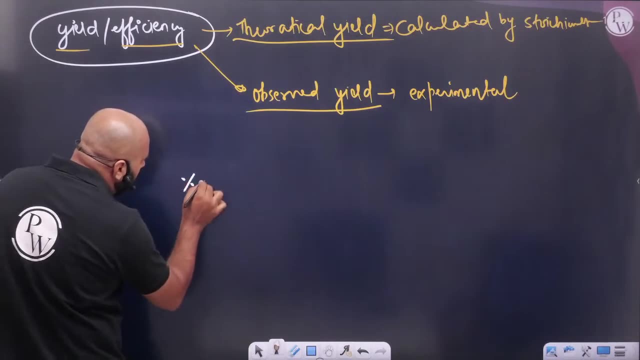 What is observed, Sir, it is experimental. You will be told in the exam hall Or you will have to calculate. Sir, see, You have to get the percentage yield at any time. To get the percentage yield, there is a formula for it. 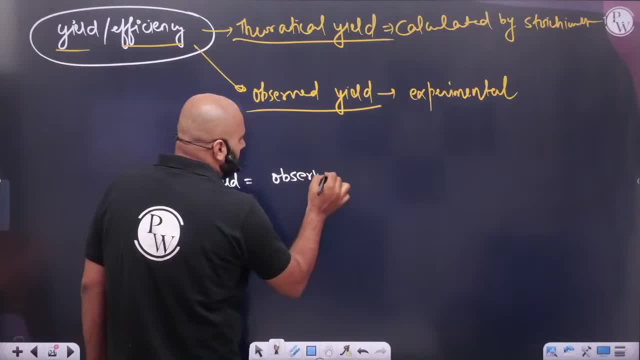 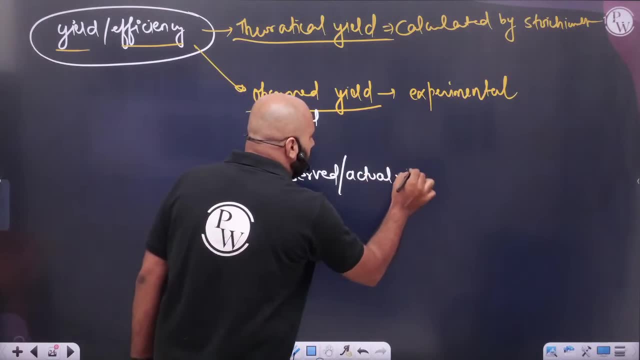 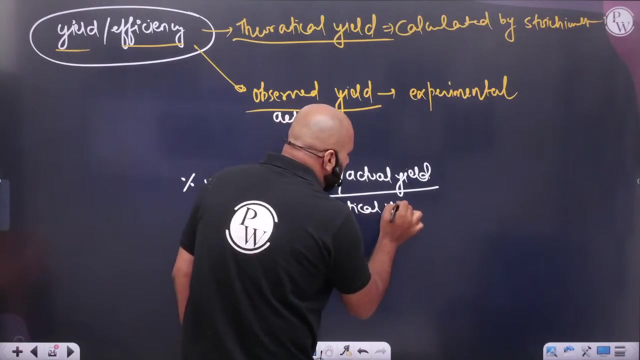 Sir, observed yield. We have observed yield, Or let's call this actual yield. What do we call observed Actual yield? Which is reality And divided by, Divided by What will be observed, divided by Theoretical, And how to multiply this? 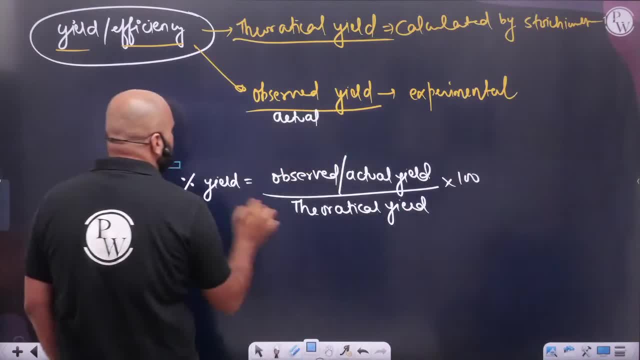 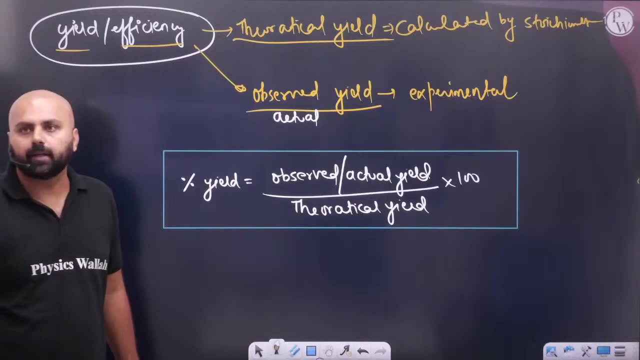 How to multiply this From 100.. So what will happen? The formula of percentage yield. It is on you. I am writing all the formulas. You will get the notes. Do it Okay, See brother. Sir, this question is given. 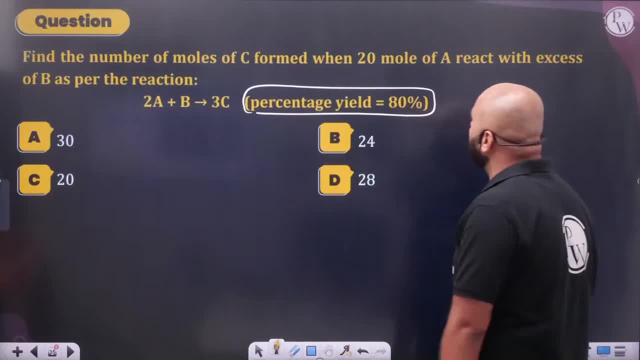 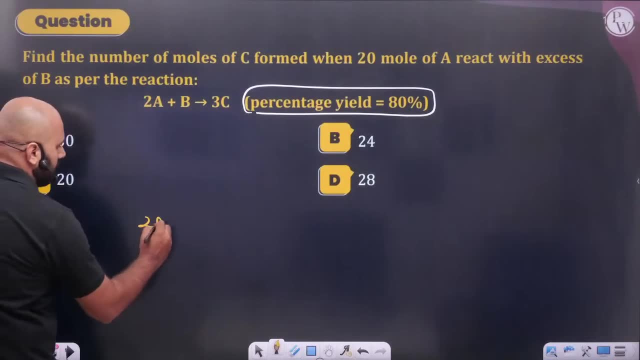 The question of percentage yield is given. How will you do the question of percentage yield, Sir? B, small a, Is reacting with the excess of B. No problem, Tell me a simple thing, Sir. there is 2a. 2a is reacting with B. 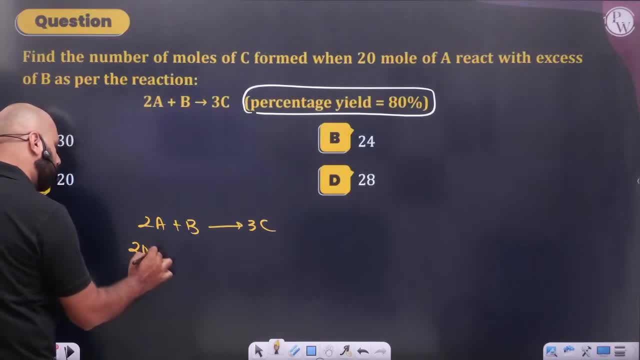 What is it making? What is it making with 3c, Sir? it has given 20 moles. Its 1, 2 moles. Its 2 moles, Sir. we don't know about B, But from its 3 moles. 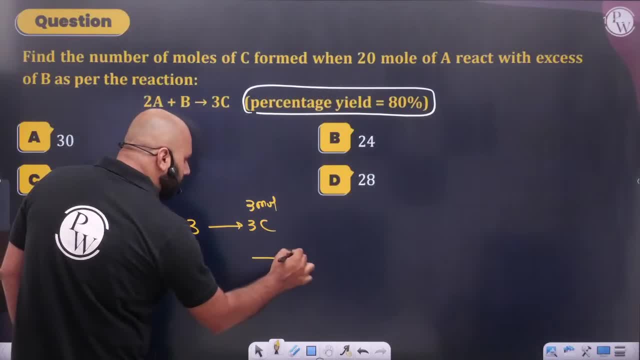 It produces 3 moles. So how much will it produce? 20 moles, If I have to find out. So what is the shortcut, Sir? with whom will we multiply this 20? With 3. Divide by 2.. 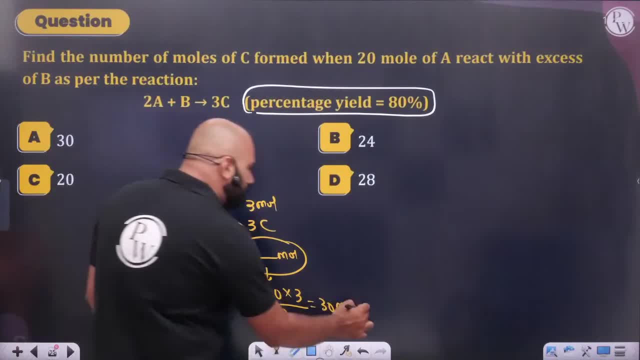 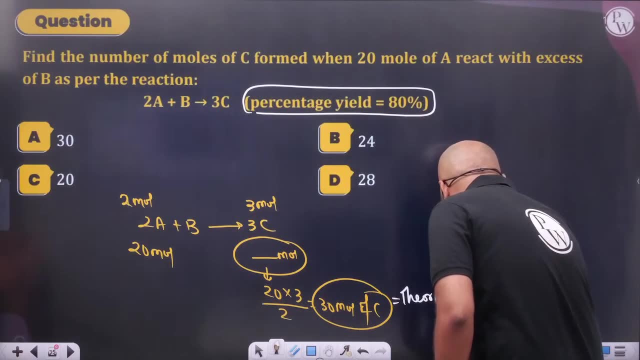 How much will it be? 30 moles, But this 30 moles of C. This is not actual, Sir. what is this? This is theoretical yield. Why? Because, sir, you have taken this out on copy Right. 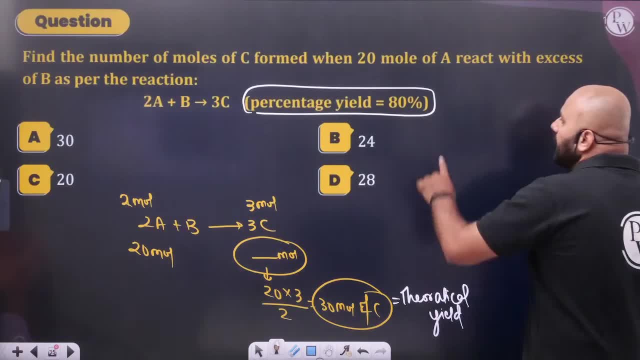 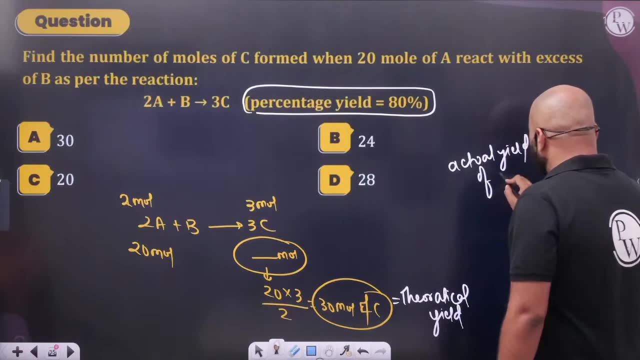 You have taken this out on copy- that theoretically it will be 30 moles, But in reality what is the percentage yield? What will be the actual yield? What will be the actual yield of C? Nothing, Sir. how much will we have to take out of 30 moles? 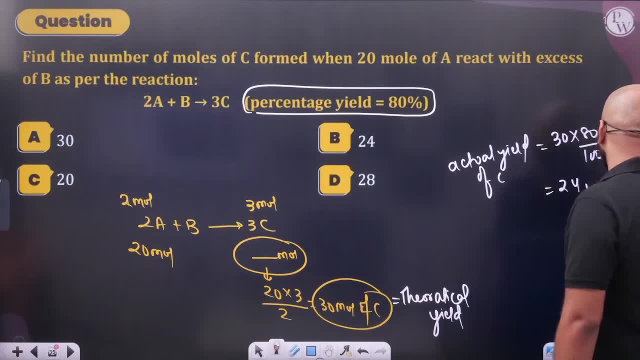 80%, How much will we have to take out of 30 moles? 80%, So it will be 24 moles. So what will be the actual yield? 24 moles. That's it. You have given 30 moles answer. 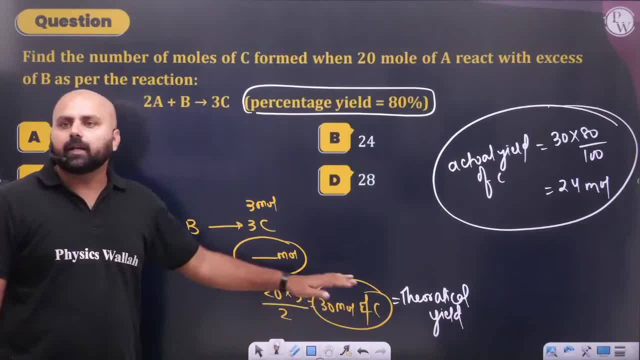 You don't want to fix that. You have taken this out on copy. Theoretically it will be this much, But in real life it will not be this much. In real life it will not be this much. So we have 34 moles. 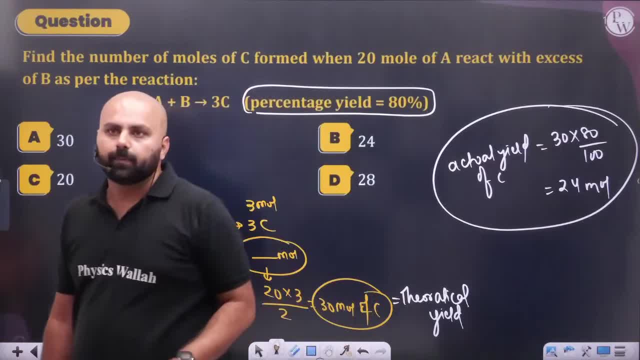 What will be the actual yield? instead of 30 moles, 24 moles. Are you sure, Sir, it will be. So let's go Now in my stoichiometry. the concept of Limiting Resonance Purity is finished. 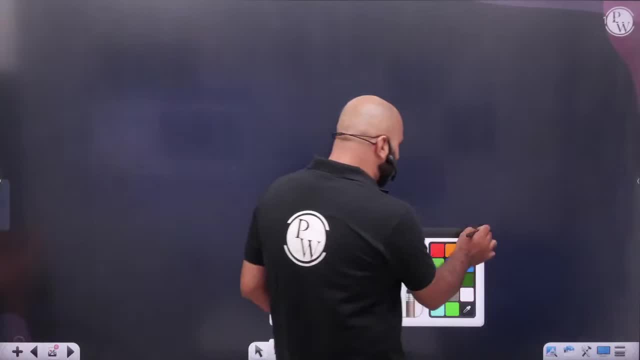 So now I am doing one thing right now, Because I don't want to go to the solution and waste time, Because by that time everyone must be tired. So I am telling you right now, And that is Concentration Terms: 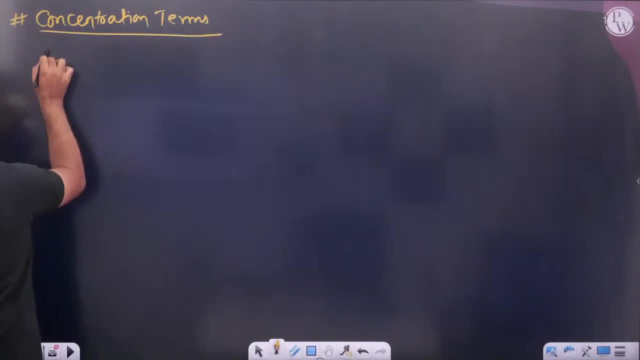 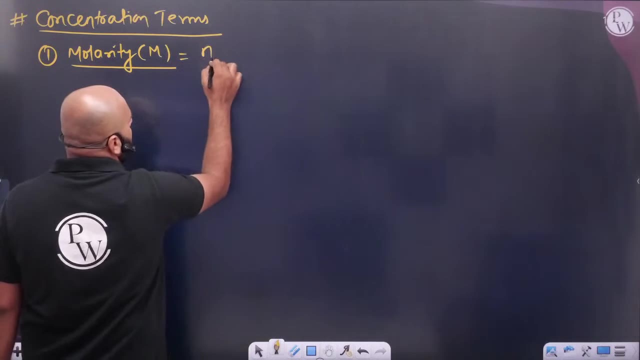 That is Concentration Terms. What are the major things we have in Concentration Terms? There is Molarity. Take a look at Molarity. The formula of Molarity: Number of moles of solute divided by volume In which? In liters. 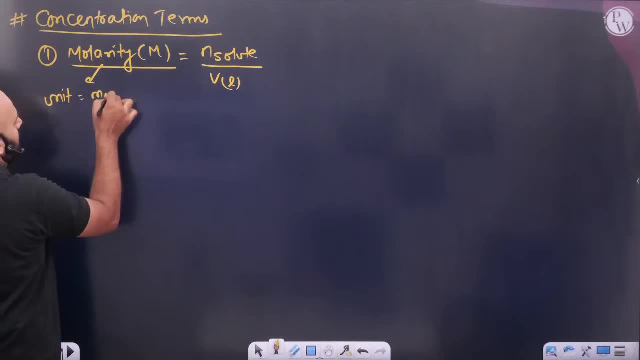 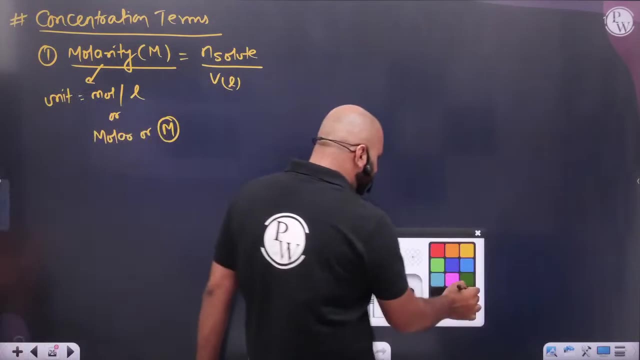 Remember, Remember its unit, Sir. what is it? Moles per liter? Or what do we call it Molar, Or we call it capital M Who said, Sir, I don't want to use this formula, So nothing. 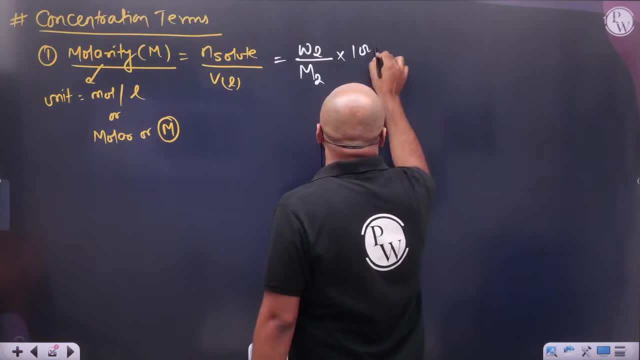 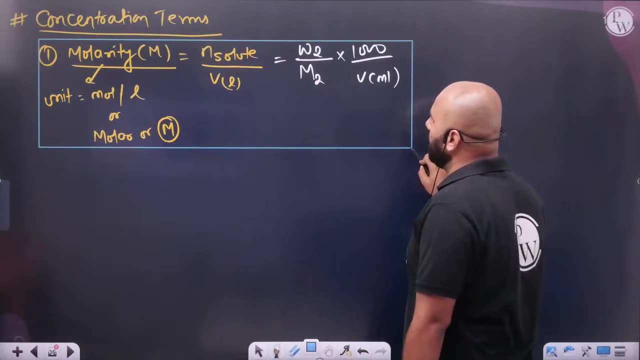 Given mass of solute, Molar mass of solute into 1000 upon volume, In which In ml. Okay, You have to remember this formula of Molarity. You have to keep this formula of Molarity in your mind. Two is nothing. 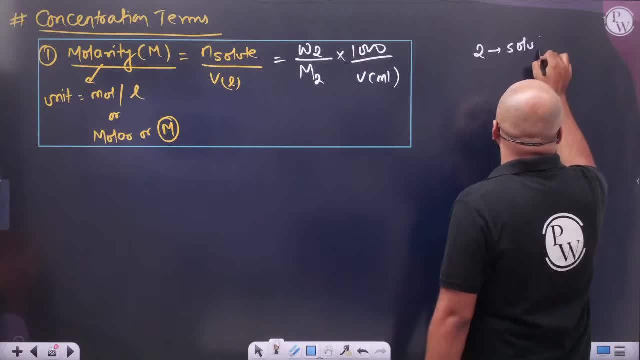 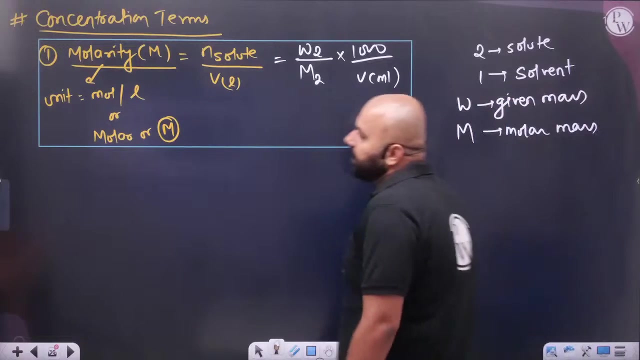 Sir, remember: Two represents solute And one represents solvent. W represents given mass, W represents given mass And capital, M represents molar, mass. Molarity is the most highlighted thing we have. Molarity is the most highlighted thing we have. 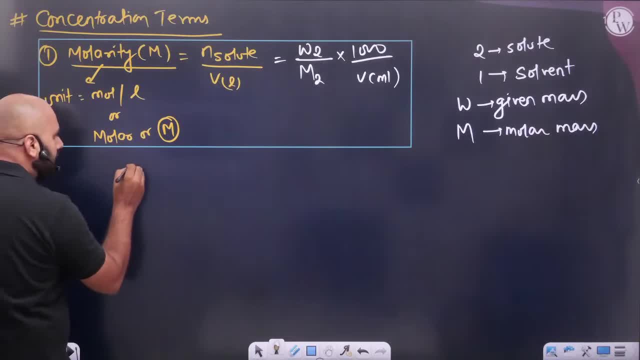 Okay, See this. See in Molarity. What is the important thing that comes in Molarity? If somebody asks you number of moles of solute, then either you do Molarity into volume in liters And if you give Molarity into volume in ml. 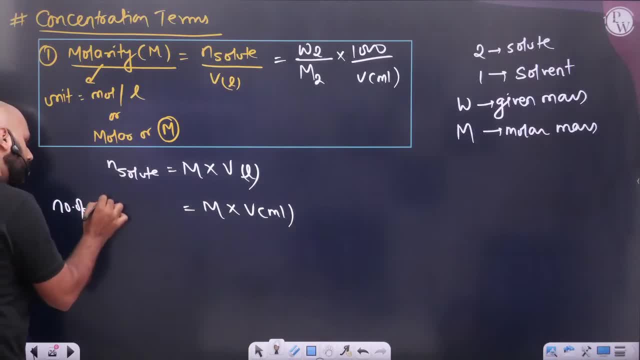 then, without giving the number of solute, what will come? Number of millimoles of solute will come After that, Sir, if you are doing dilution or concentration, If you are doing dilution or concentration, the formula of that time is: M1- V1 is equal to M2- V2.. 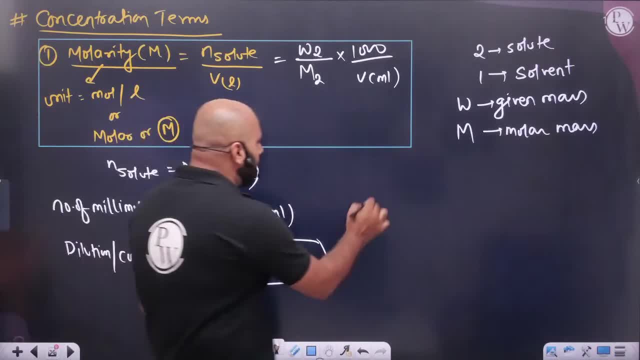 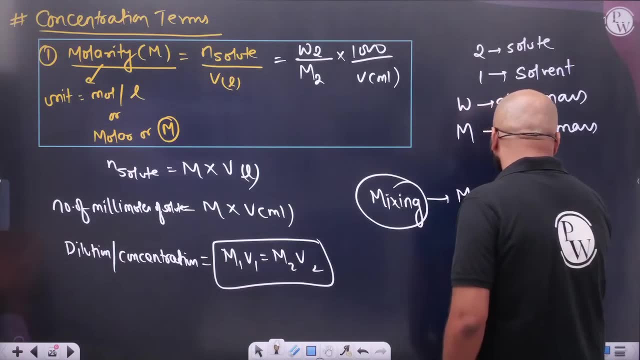 M1 V1 is equal to M2 V2.. And the last one, the concept of molarity, also says that if you are doing mixing, then in the case of mixing, the molarity of mixture is nothing: M1 V1 plus M2 V2 divided by volume of mixture. 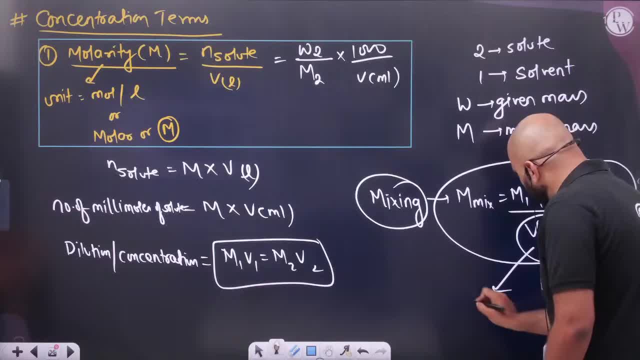 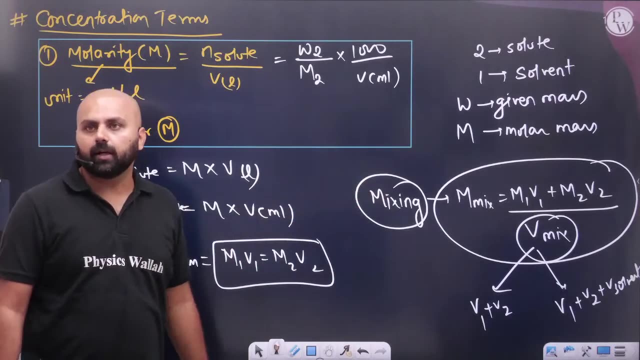 Volume of mixture can be anything. pay attention in the exam hall. it can be V1 plus V2 and it can be V1 plus V2 plus volume of solvent. So this is the formula of molarity. The formula of molarity is done by molarity. 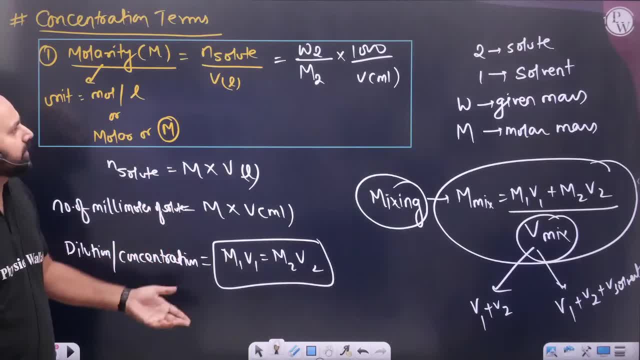 Now look at this, this molarity we have. 2 is what Solute. 1 is solvent. its mixing formula, dilution formula. pick it up, keep doing it. After molarity: if we talk about the most, okay, we have molarity number of most. 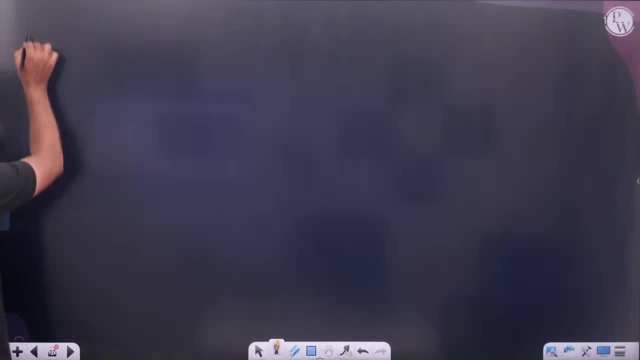 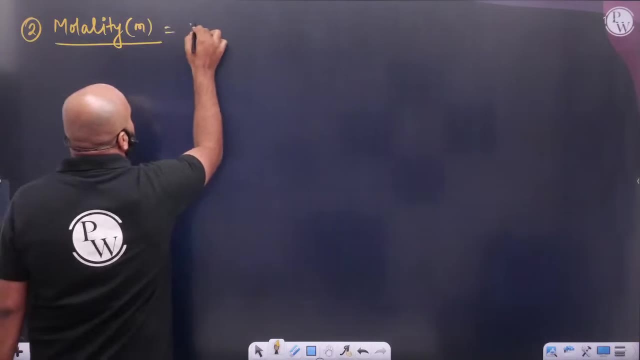 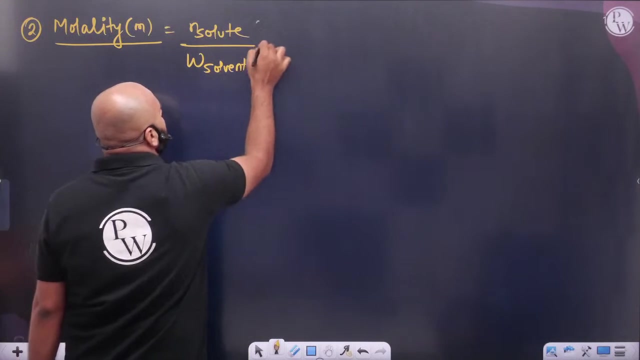 divided by volume. if you look at the exam hall, then its second formula, the second person who comes, molarity comes. What is molarity, Small m? what does small m say, Sir? the number of moles of solute is divided by sir. what is mass of what is solvent? this person is given in mole and this person comes in kg. 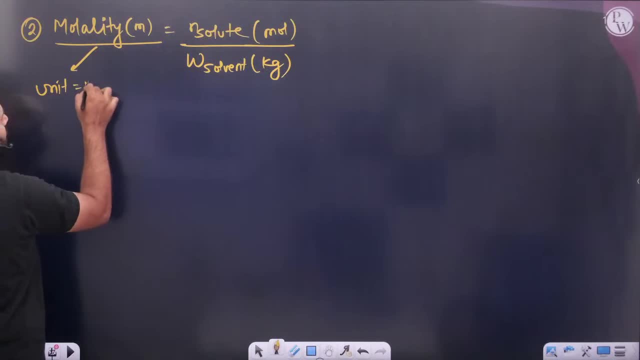 That's why look at its unit. what happens to the unit? Kg is done on moles, or what do we call this? We call it molal. Or what is molal? We call it small m. Molality is done, we call it molal. 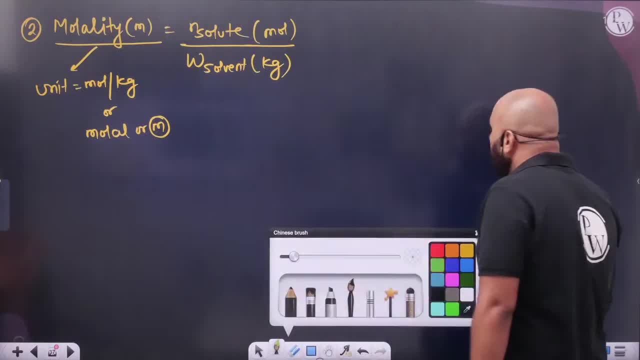 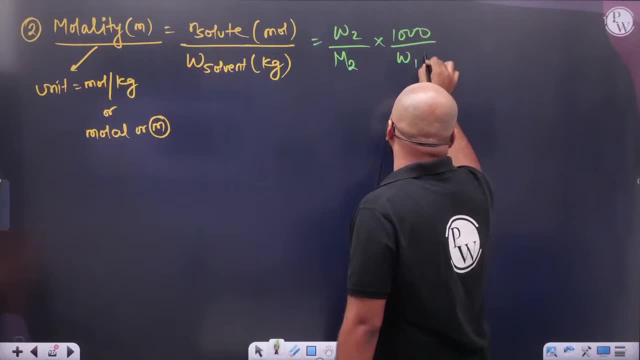 Okay, Look at this molality. look at its formula: w2 by m2 into 1000 upon sir, what is its mass? If I take it in grams, then this will come. its formula will come. You will do questions, you will see it now. 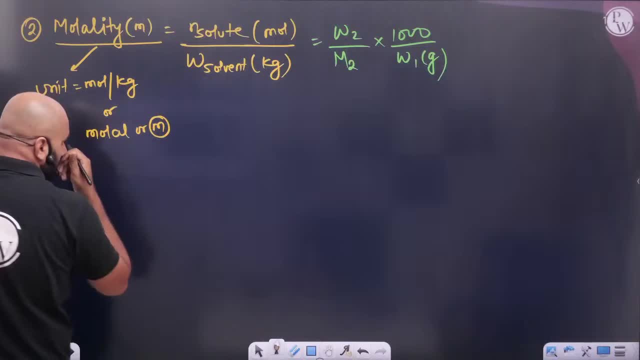 Molality in molality, this person. if you see the molality, then he is talking very simple things. He is talking very simple things. Okay, Look at this. what is more important than molality? So one or two more things will come, like strength. 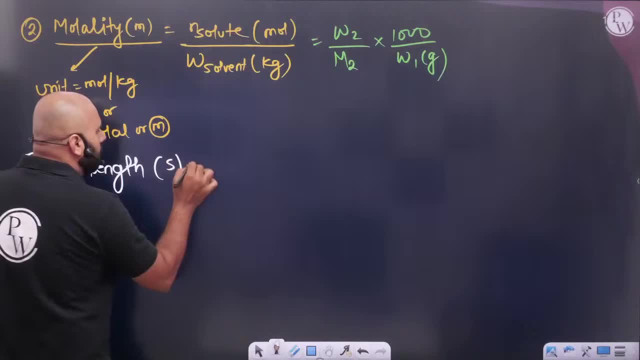 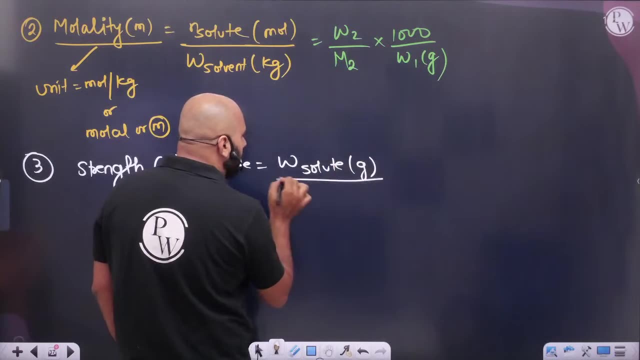 Strength of solution. strength of solution. what does strength of solution mean? Nothing, Given mass of solute. given mass of solute in grams divided by volume whose Of solution In which, In liters. Volume of solution in which. 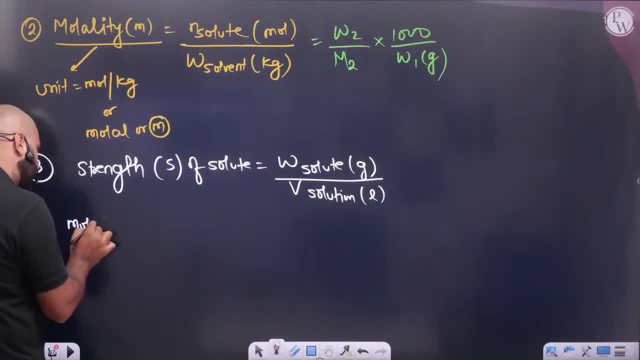 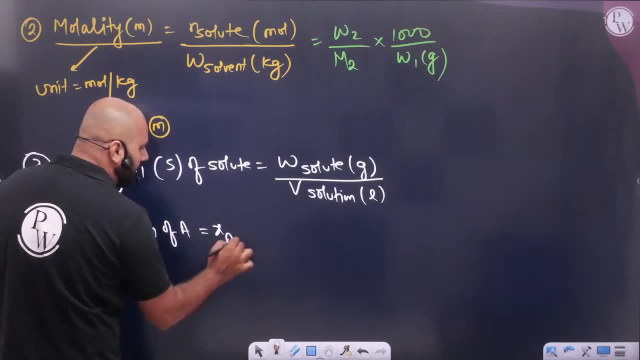 In liters. If someone is asking you about mole fraction. if someone is asking about mole fraction, then if you are asking about mole fraction of A, then how will you represent it? Chi A, and that is number of moles of A divided by total number of moles. 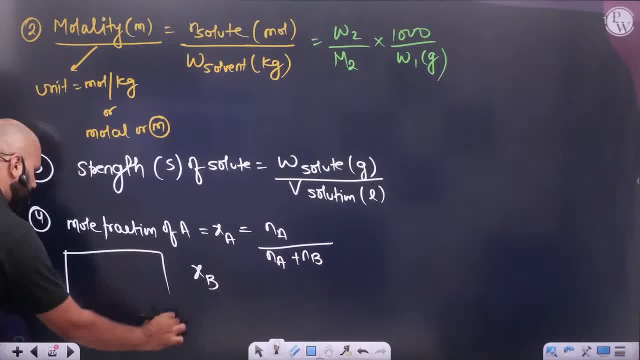 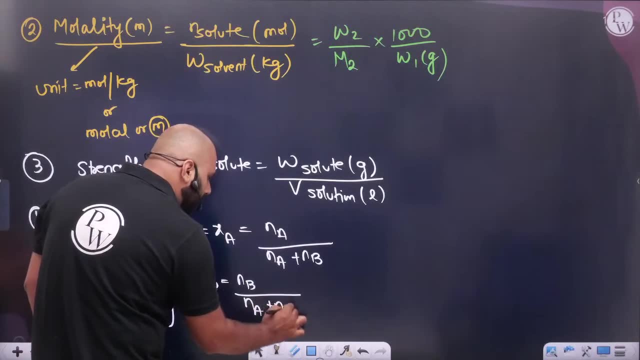 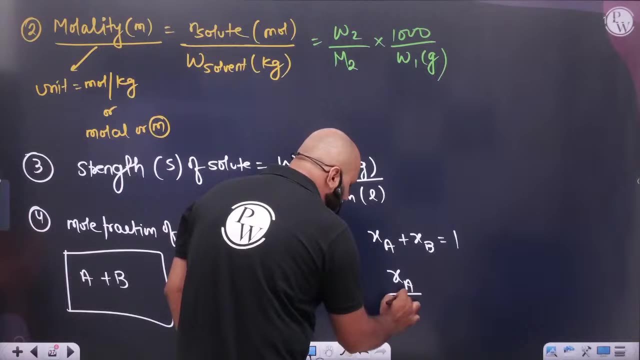 If chi of B is asking: there are only two people. if there are only two people in your life, A and B, then number of moles of B divided by N A plus N B. In their case, remember one thing: the sum of mole fraction. the sum of mole fraction will be 1, and the ratio of mole fraction will be equal to number of moles. 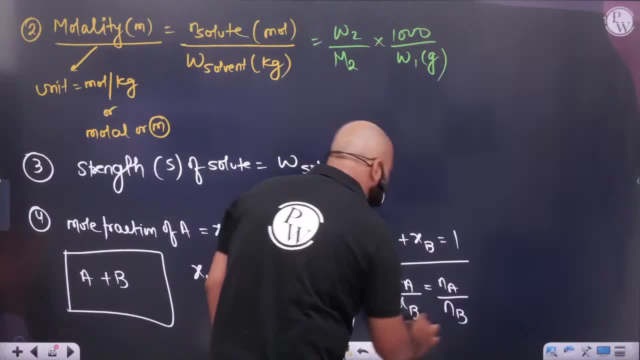 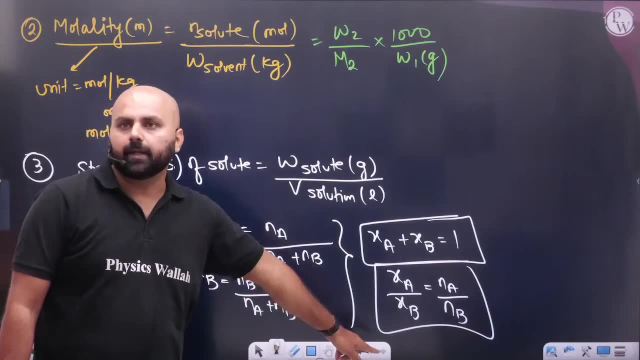 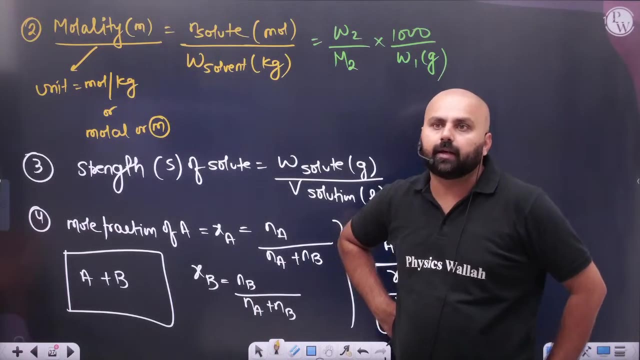 It will be equal to the ratio of number of moles, The sum of mole fraction will be equal to 1, and the ratio of mole fraction will be equal to this. Okay, So see, Now, see here, brother. Now one is saying: sir, the formula, brother, you will remember the formula, right. 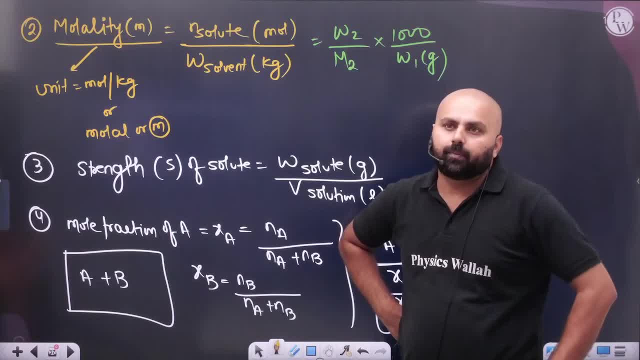 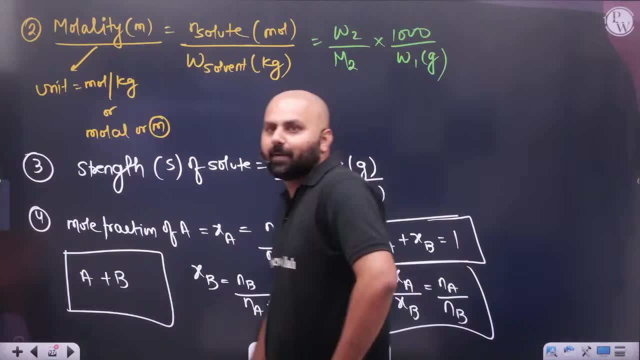 Okay, Yes, It was with us. Come on now, see Now, now say Earlier, he was saying sir, when they were small, then, yes, Okay, Now I will tell you. I will tell you the trick of concentration. 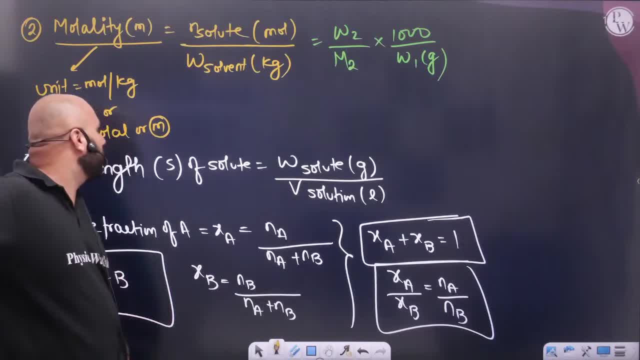 Okay, I will tell you the trick of concentration. Now this is done. Wait Now, the formula of strength is done. The formula of strength is done, The mole fraction is done, The molality is done, The molarity is done. 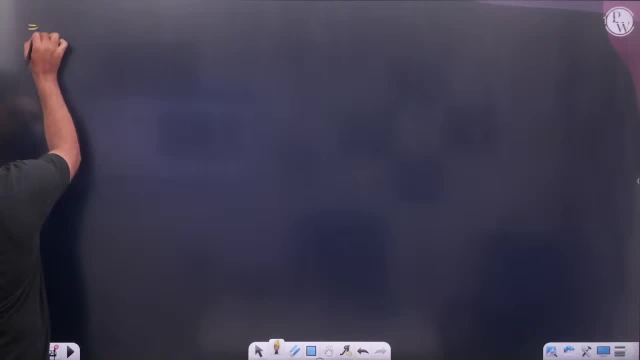 See the relation between them a little. Remember the interrelation. What is interrelation, Sir? one formula of molarity is a shortcut. One shortcut of molarity is 10 times X D, 10 X D, 10 X D, divided by molar mass of solute. 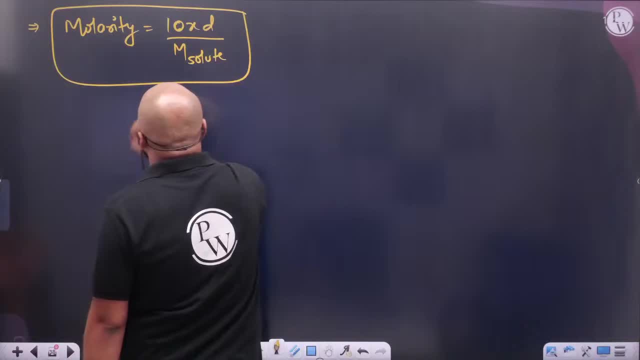 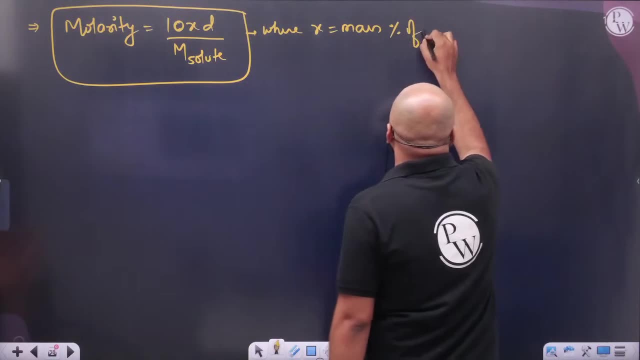 There is one formula of molarity capital M, that is 10 X D, 10 X D. Where Where X is mass percentage of, Where X is mass percentage of solute, D is density of solution. It is direct formula. 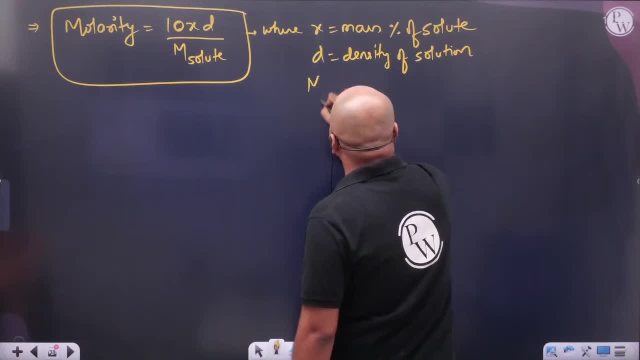 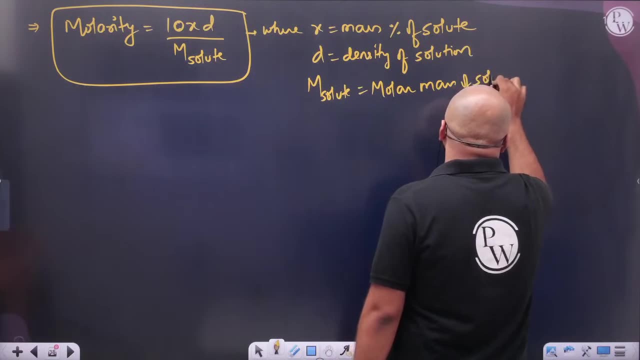 When you will put it directly, the answer will come: Density of solution M- molar mass of solute. M is nothing. Molar mass of solute, The first relation which you can use directly in the shortcut to solve your numerical sounds. 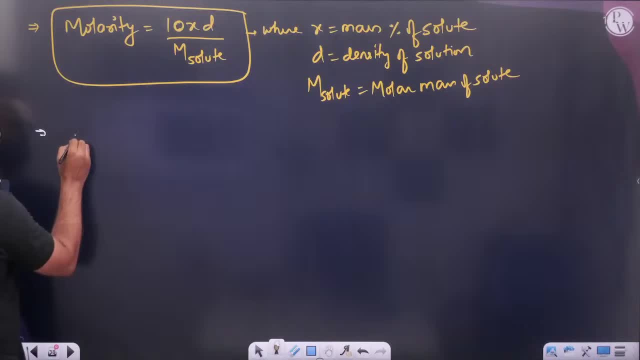 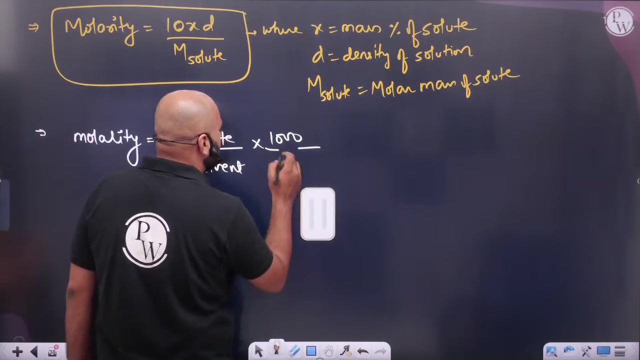 This formula is directly based here. If you see here, If you see here, the formula of molality is very famous. The formula of molality is known as mol fraction of solute divided by mol fraction of solvent into thousand upon thousand upon molar mass of. 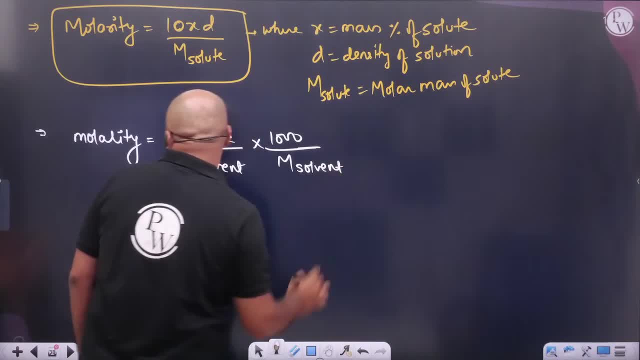 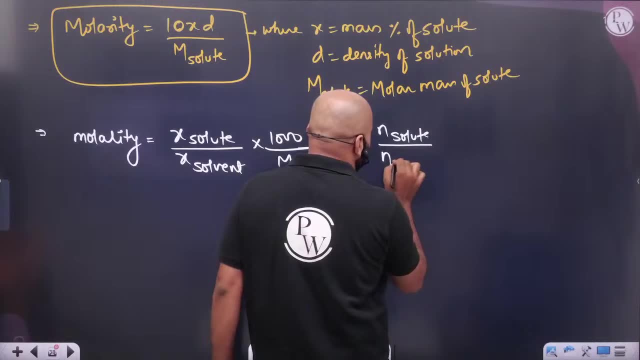 thousand upon molar mass of solvent. So this is the formula. If you want this formula of molality, then you can write it like this: Number of moles of solute divided by number of moles of solvent. You can write it in terms of number of moles of solvent. 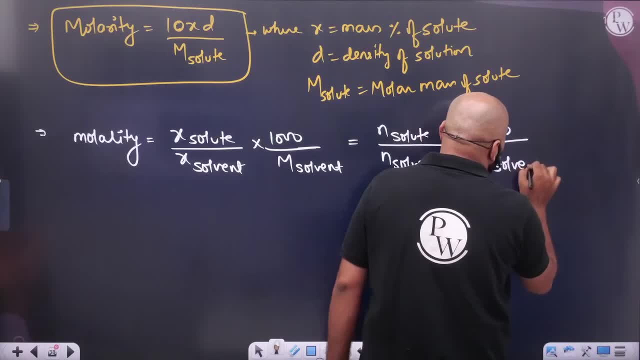 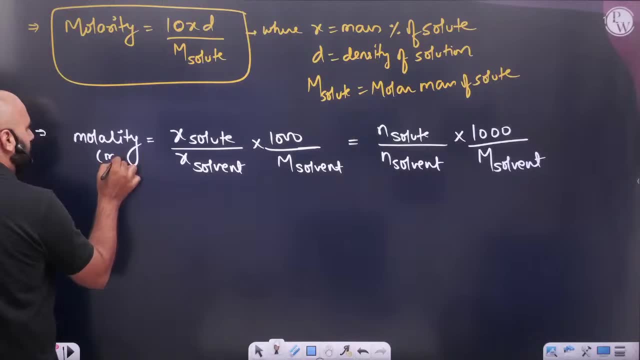 because the ratio of mol fraction will be equal to the ratio of molar mass of solvent. After that, if you talk about molality according to small m, then there is one more relation. Strength is nothing, Strength is nothing. Molarity into molar mass of solute. 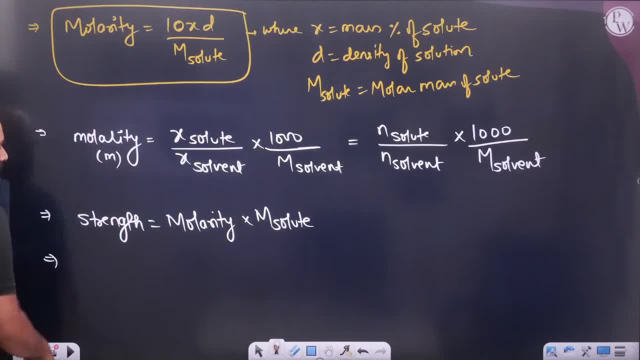 Molarity into nothing, Molar mass of solute. And the last one, the ultimate relation is the one which was given in NCRT, The one which has the most chances of coming. This question used to be asked in M's earlier. 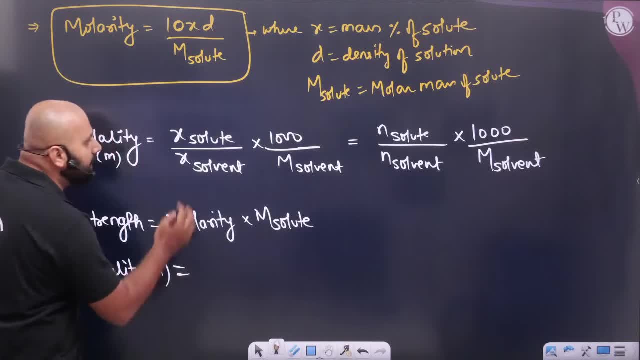 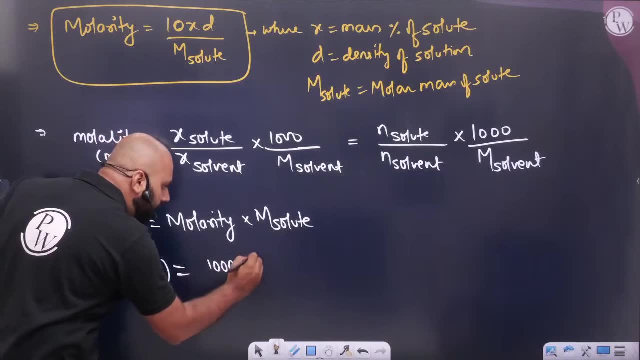 But now they have stopped asking this question. M's exam is over. That's why we don't get this question. This question is good if it comes, but it is in NCRT and it has 14 chances. Thousand times molarity. Thousand times molarity. 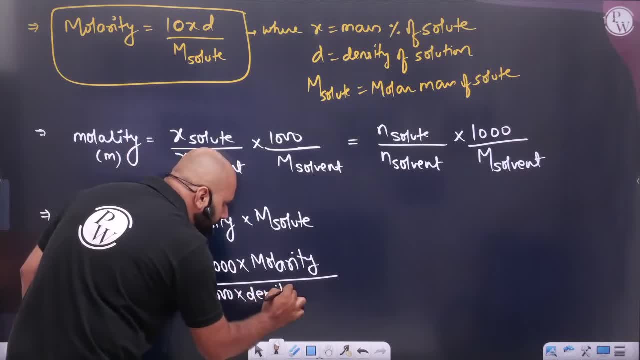 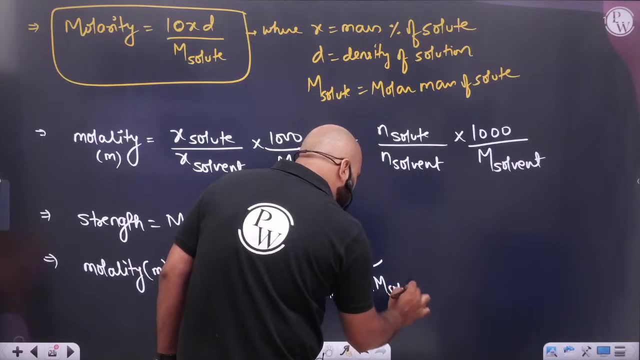 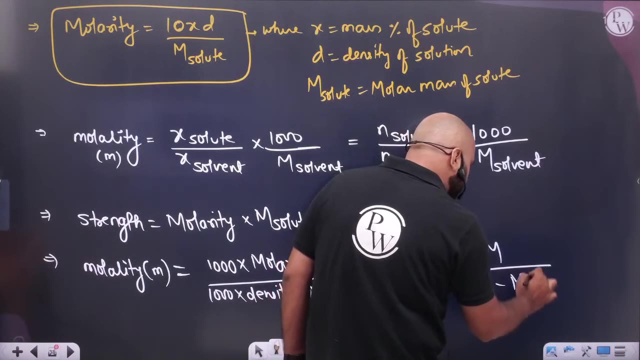 Thousand times density. Thousand times density minus molarity, Formularity into molar mass of solute. Brother, I don't want to write such a big formula. I want to write it straight: 1000 times capital M, 1000 times D minus M into molar mass of solute. 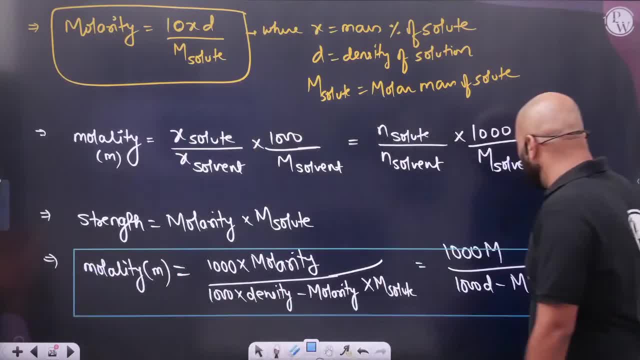 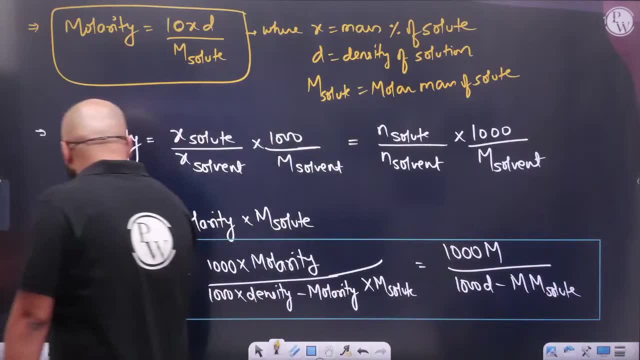 Brother, this formula. now we should remember this formula. Reason is that in exam hall in NCRT there is a base question on it. So in NCRT there is a base question. So this formula, if someone asks me, then these four formulas the most used formula, 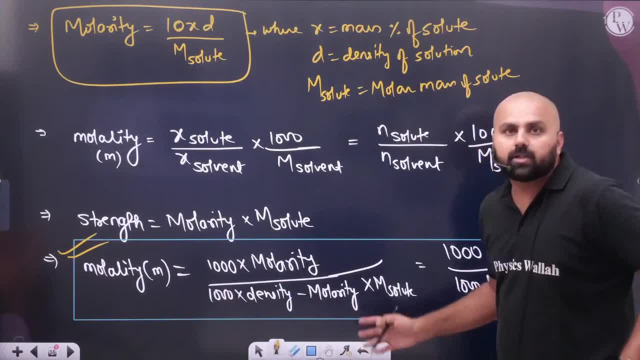 and the most used formula, and in this there is no need to understand. This class is not like that, that brother. now I will derive one thing and show you. Then it will not happen in 12 hours. then we were doing this all year, right? 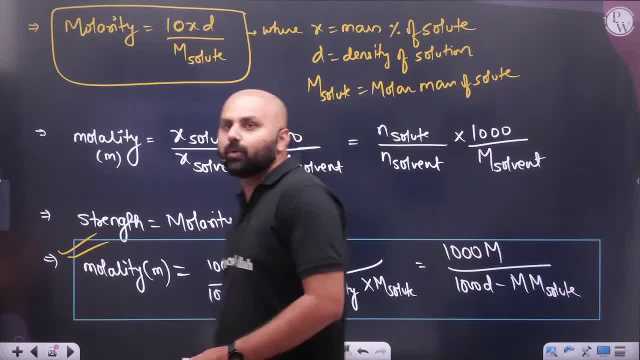 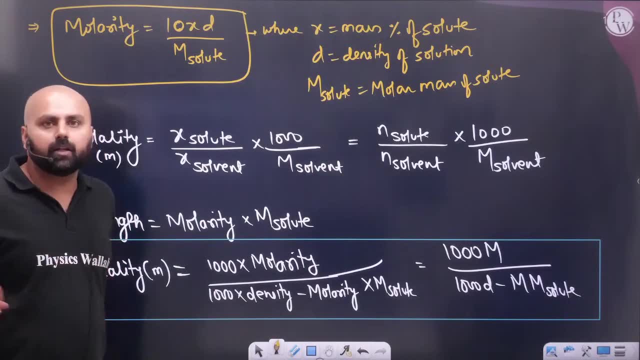 We were driving, okay, Yes, if there was to understand, to understand. now I don't have it with me. okay, Now I will not derive this. I will not show you for that. son, believe batch or Lakshya batch, or come in that, okay. 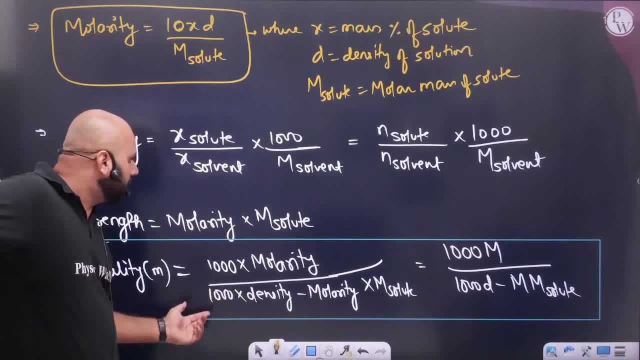 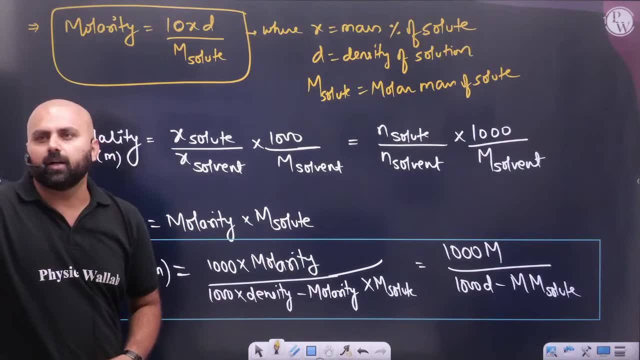 Yes, So this is the formula. So this is the formula. So this is the formula, This is the formula of molality. use it, brother. Yes, boss, great. Now here are simple, simple, simple ways to put formulas. 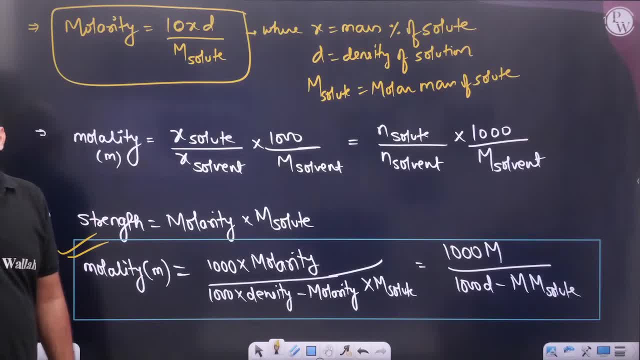 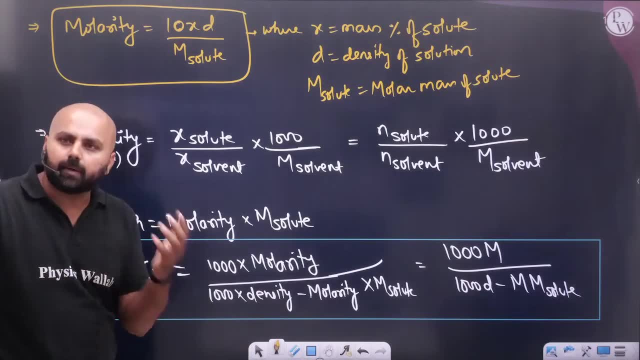 Answer keeps coming out, brother, Quickly, quickly come out. okay, Okay, Which one? If the formulas are done for the first time, then, brother, if they are done for the first time, then there is no problem. No problem, brother, you keep it with you. when you get your PDF, do it with PDF, brother. 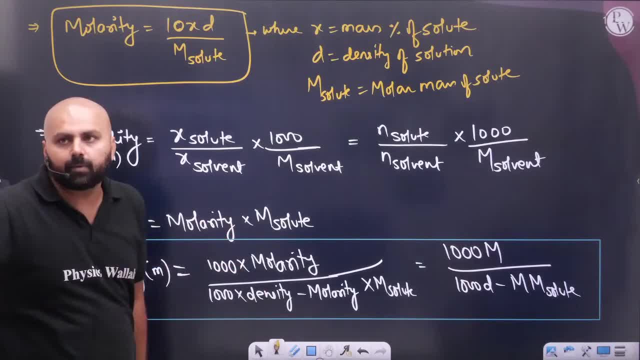 Put it with the PDF. you can do it with it. You can do it with the PDF, you can do it with it. Now, you can't do derivation at this time. I am doing derivation to make you understand. I am already going late. 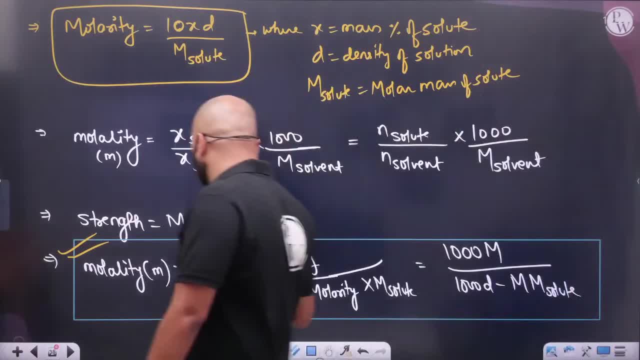 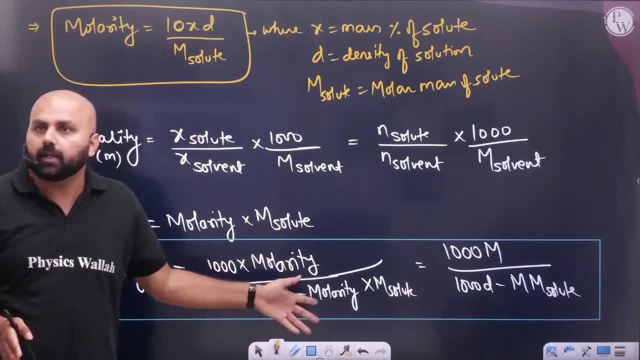 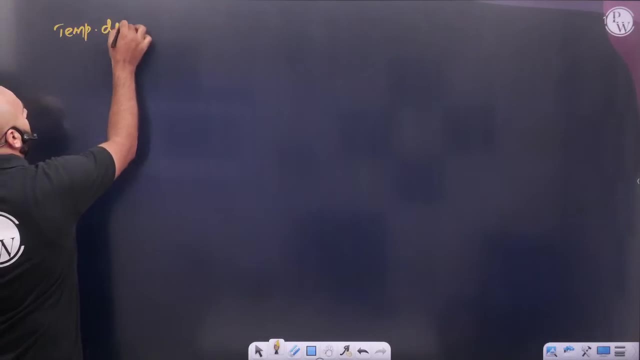 In order to make you understand. I came to know that I am doing derivation Now that much time is not gone. if you want to do something for 12 hours, then write the formula After that. one more thing: remember here who will be temperature dependent. 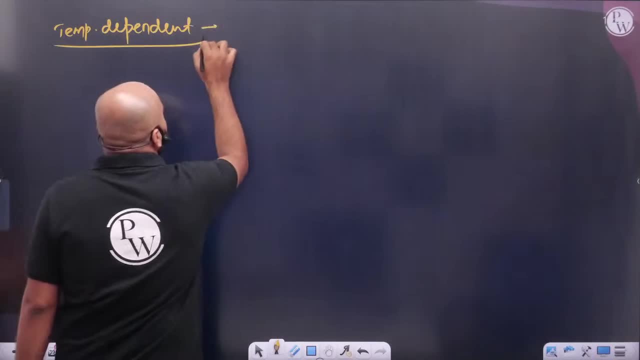 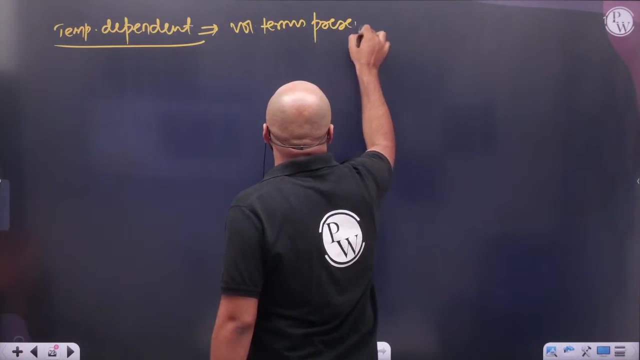 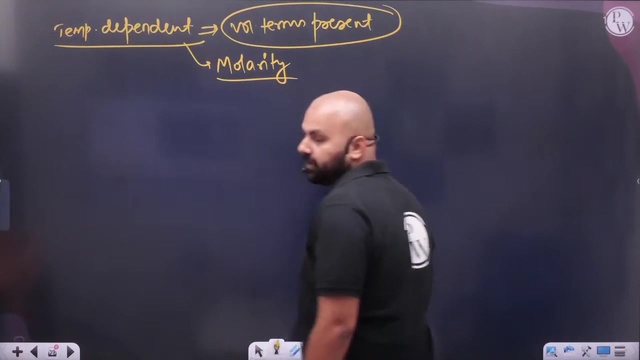 The question of temperature dependent is asked. Temperature dependent means that remember where volume is present. wherever the volume term is present, he has it, whatever that be the molarity. Look what is molarity. It has become temperature dependent Where the volume is present. 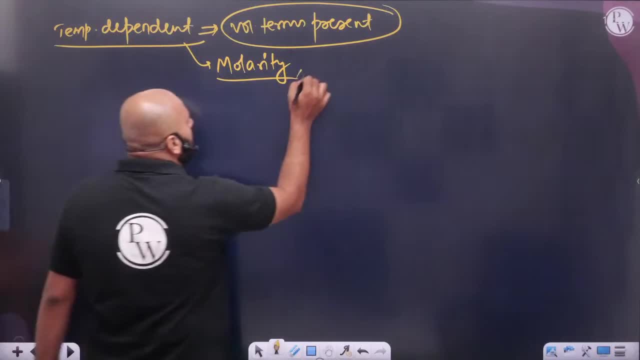 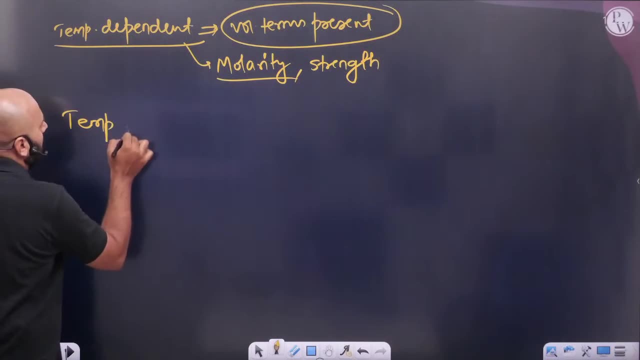 Where the volume is present, it will become temperature dependent. Molarity has taken place, Strength is there. This all has become temperature dependent. But if I talk about temperature independence, If I talk about temperature independence, If the temperature is independent, then where there is no volume, like there is a mole fraction. 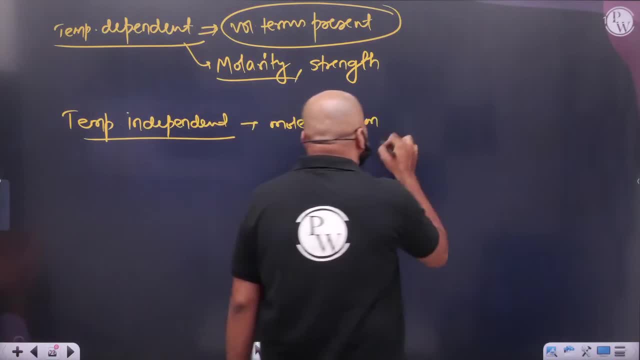 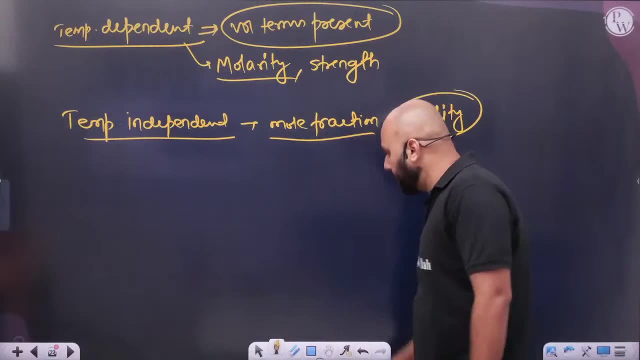 That's why you will see in the solution chapter when we do experiments, When you will see in the solution chapter, molality, Sir, see this molality and mole fraction. What is all this? Temperature is independent. You consider them as temperature independent. 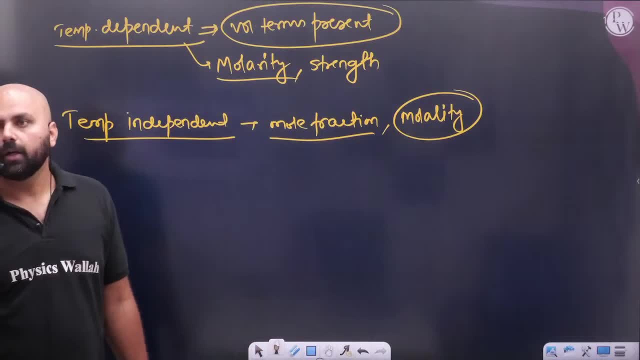 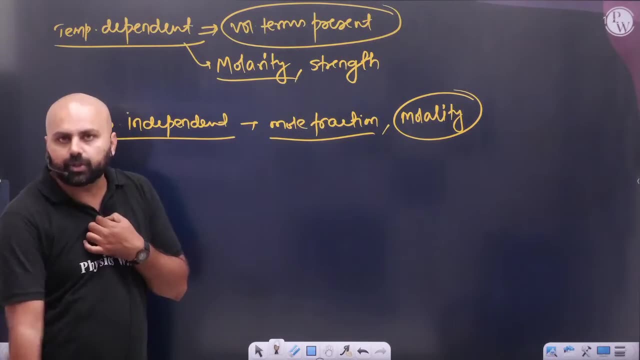 It will happen, sir. Okay, So do these things. Okay. So this Now: who has normality Son? it is not in the syllabus now, But first let's do the question of molarity, Which was the question of this year, NEET 2022. 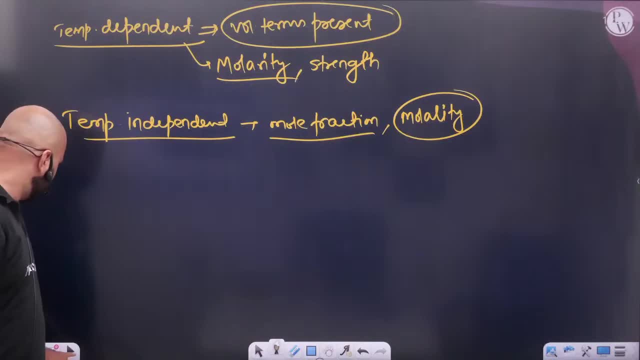 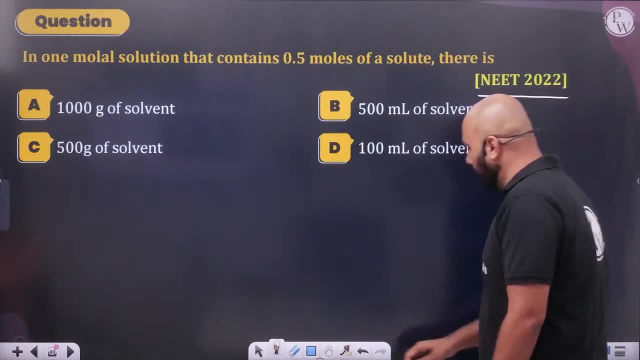 Do that, Okay. Okay, Let's go In one molal solution that contains- this is the question of this year, 2022.. If there is one molal solution, how much is there in it? There is 0.5 moles of solute. 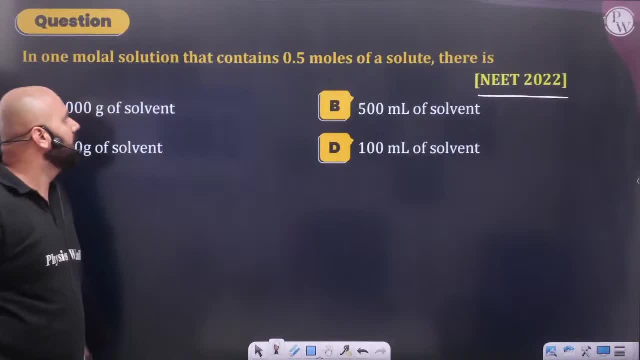 In one molal solution where there is 0.5 moles of solute, what will happen? There is: If you have one molal solution, molality is given to you. What is molality? Number of moles of solute divided by. 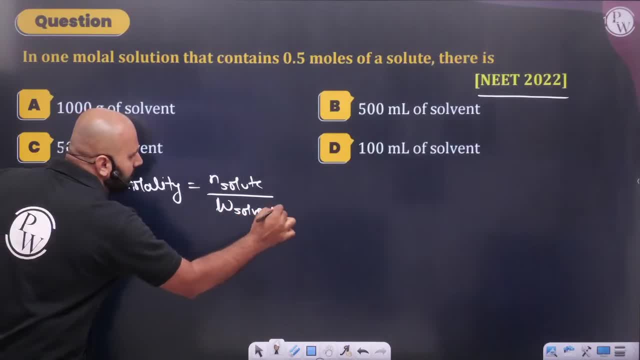 Mass of solvent In which In kg. So, brother, take mass of solvent in kg, What will happen? Molality is 1.. What are its moles? 0.5.. How much will you take mass of solvent? 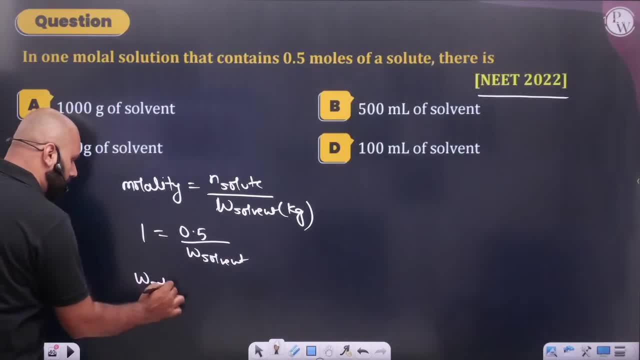 Sir, how much came in mass of solvent in kg? If you see mass of solvent in kg, then how much will come 0.5 kg? And how much can we call 0.5 kg, 500 grams? Now look here. 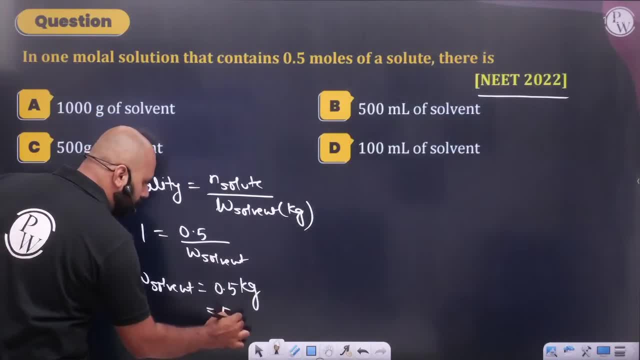 500 ml. 500 ml. 500 ml of solvent, 500 ml. We do not take it from the volume. Molality or concept is not depending on the volume. So what is the mass of solvent? Mass of solvent. 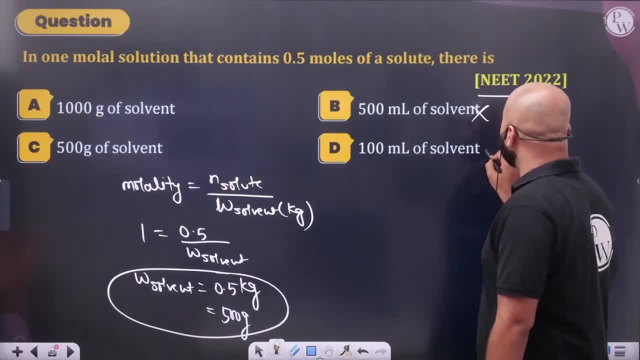 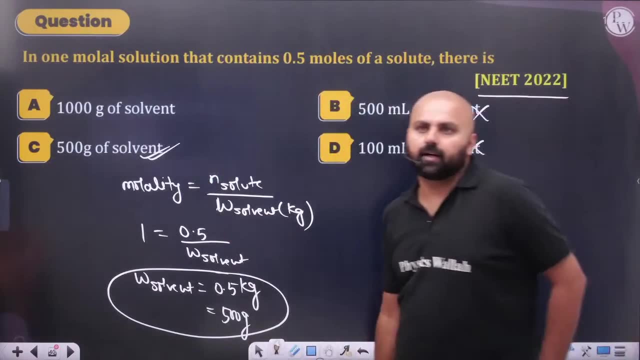 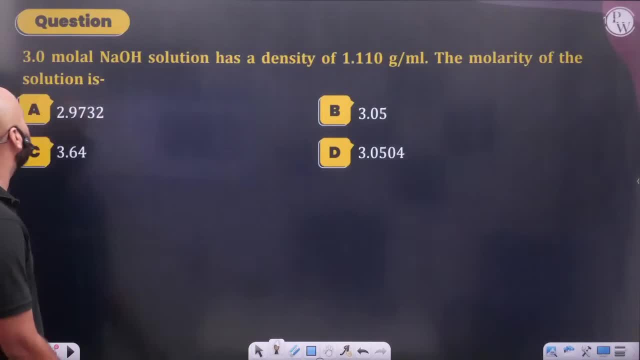 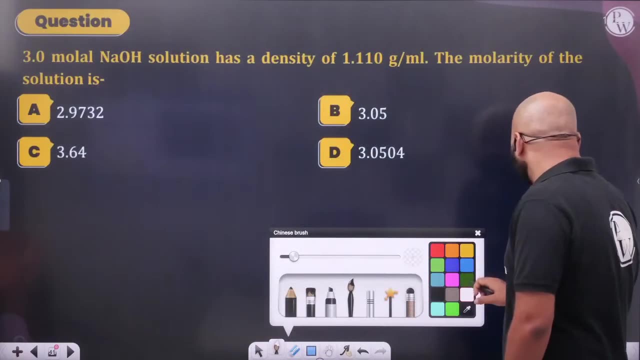 Now just do all these things. This question is given in NCRT also. Look at this type of question. That is why I told inter relation. Inter relation told it Because you have enough time to do this question. See these: You can get such question in exam hall. 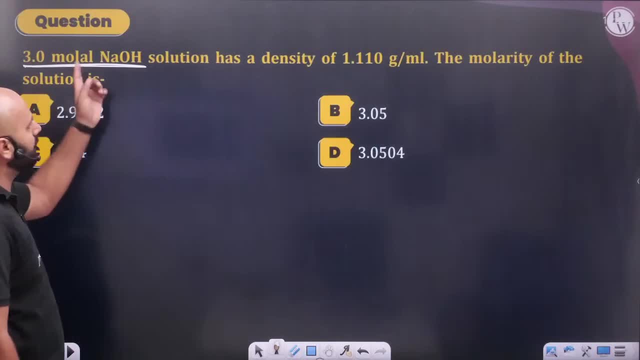 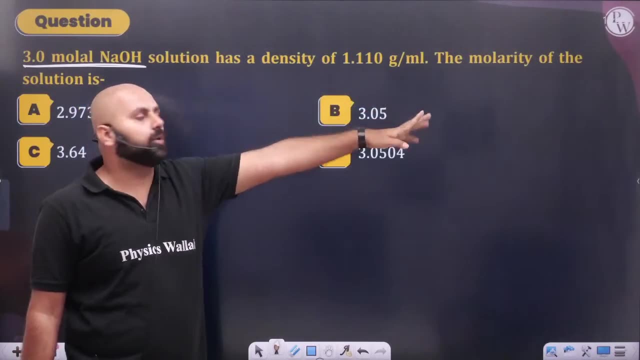 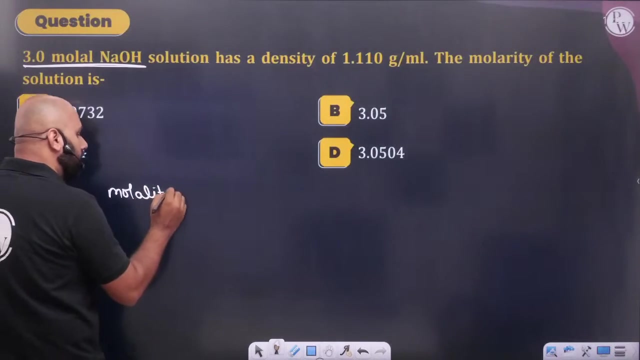 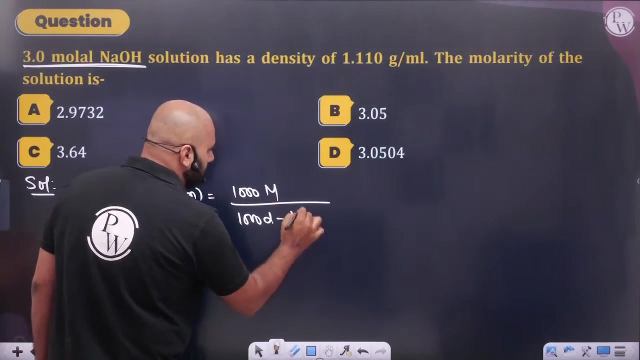 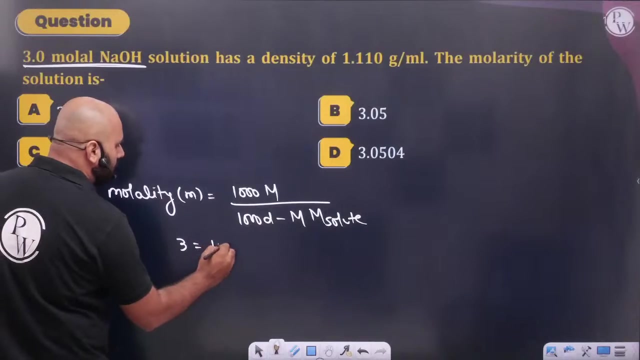 Because if you check in NCRT then you will get it. Last example is given here: 3 molarla flesh solution. Check, we have given the molarity density. what is being asked? what is being asked? take out the molarity. how will you take out the molarity? nothing, the formula of molarity. the formula of molarity, just now it was written the formula of small m. brother, put the direct, direct formula 1000 times d, 1000 times d minus m, into molar mass of what will happen, solute 1000, what is the molarity of this? 3, how much is this? 1000 times m? divide by 1000 times density. 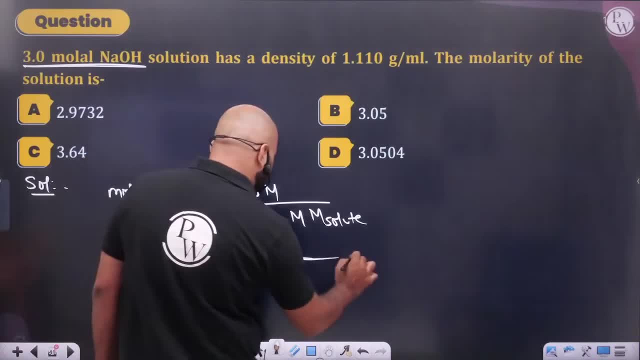 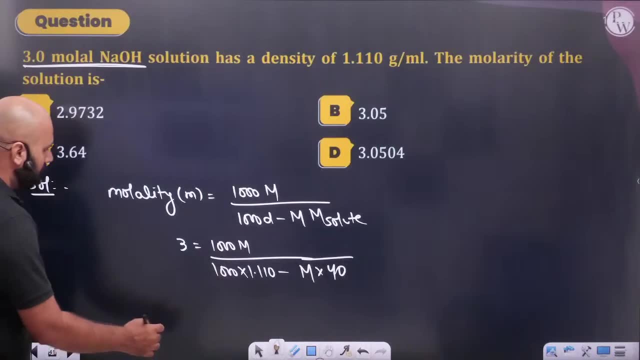 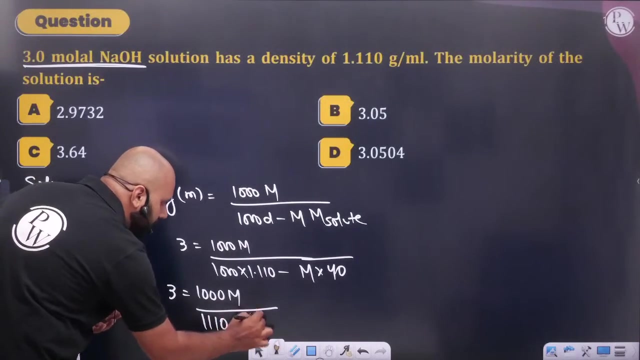 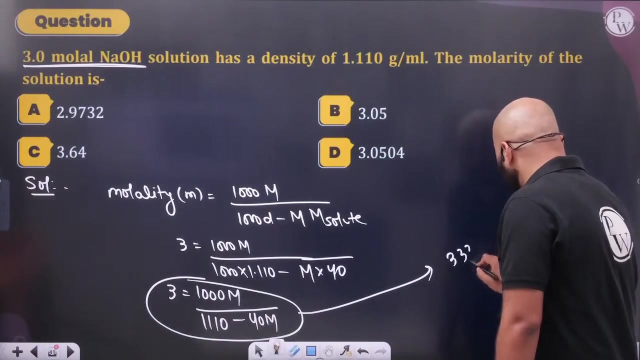 1000 times 1.110 minus- we don't know- the molarity, molar mass of solute. how much is the mass of NaOH 40,? how much is the mass of NaOH 40,? we will solve. how much will this be 3000 m? how much will this be 110 minus 40 m? how much will this be 40 m? I will come to solve. so, while solving what will happen, 3330 minus 120 m is equals to 1000 m. 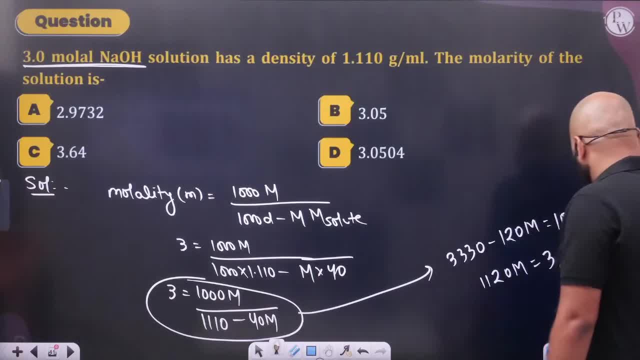 so what will happen? you will see the value of m 3330 upon 1120,. its value is approximately. how much will sido do be less then 3? only 2 points will be less than 3.. The only value seen is less than 3.. 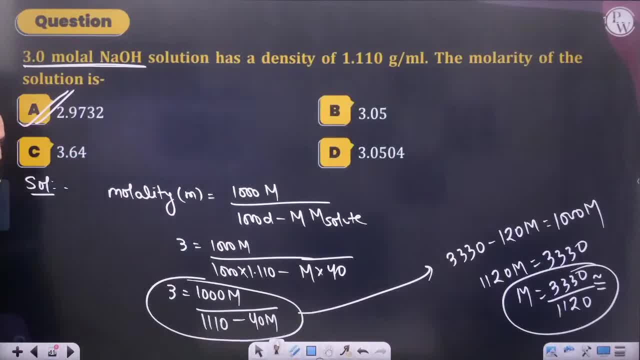 So what will be the answer in the exam hall? a answer will come. What will be the answer in the exam hall? a will be received. Okay, so let me see it for once. what will be the answer in the exam hall a and why there will be only less than 3.. 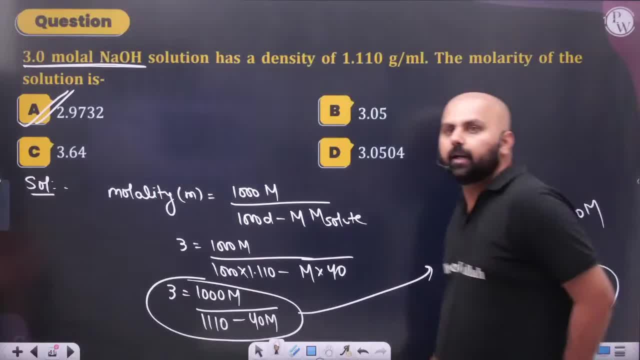 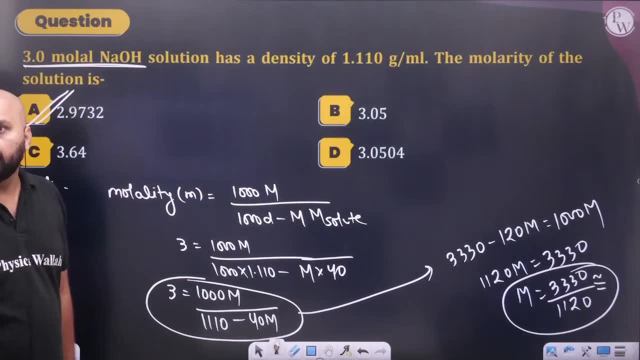 Why it is the 33 of 11,, 20 of 20. 3 will be too much. it should be above 60, then the answer will be less than A in the exam. Sorry, if it will be less than 3, then put the answer. this one is sure. who is there for boards? then there is no one for 11th and 12th. 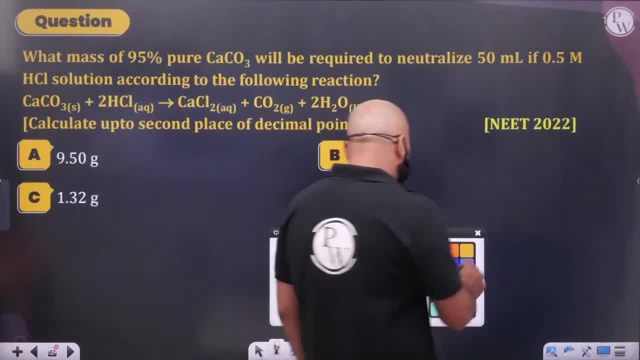 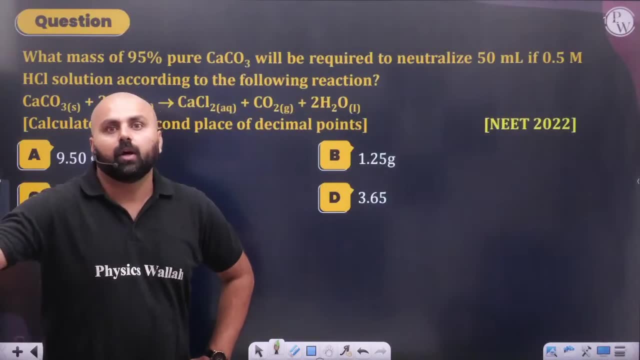 See the question of this year in NEET 2022,. how was the concept of purity given? See the ones who were doing purity again and again. what is the concept of purity? I am telling you again The concept of purity. is said that the mass of reactant which is reacting, that is not the actual mass. that is not the actual mass. it will have to be taken again. 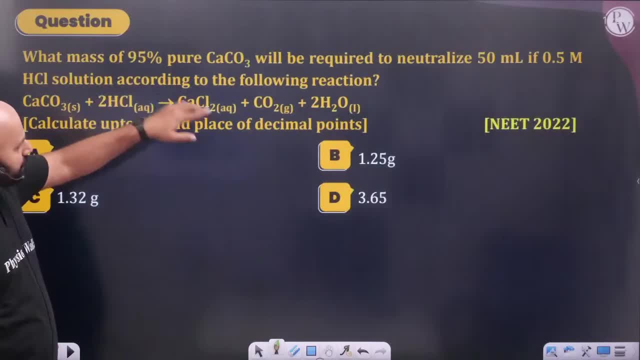 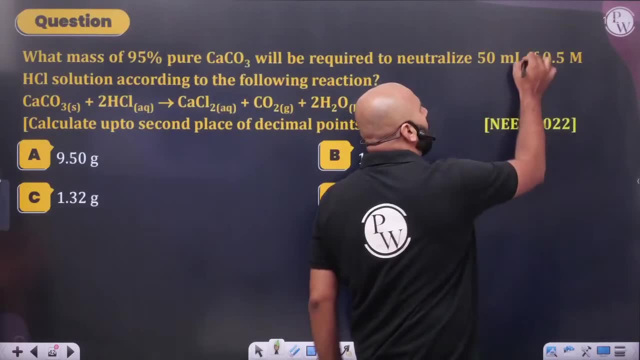 See what happens. I am saying this question is of NEET 2022, he is saying that, in this reaction, 50 ml of this, sir, 50 ml of neutralize, whose 0.5 ml, 0.5 ml of HCl, in accordance with this reaction. 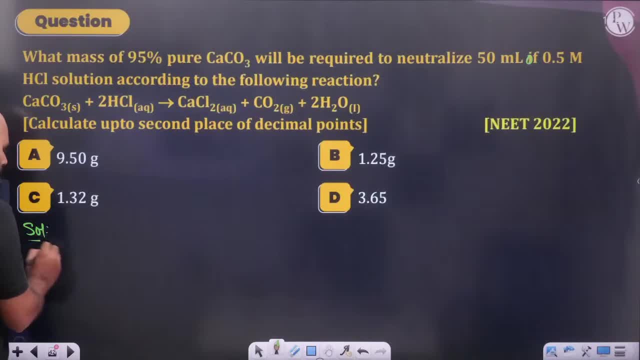 Tell me once, if I talk, if I talk about moles of HCl, then how will I take out the moles of HCl? How will I take out the molarity into volume in liters? How will I take out the moles of HCl? 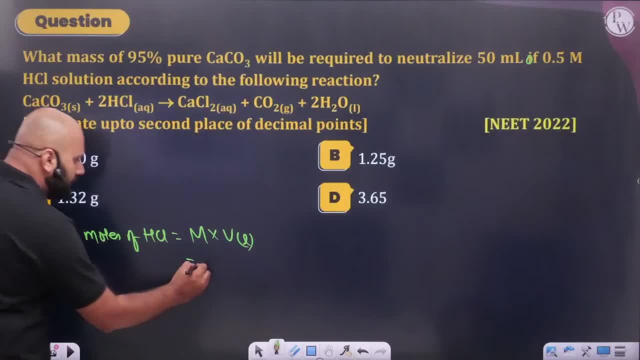 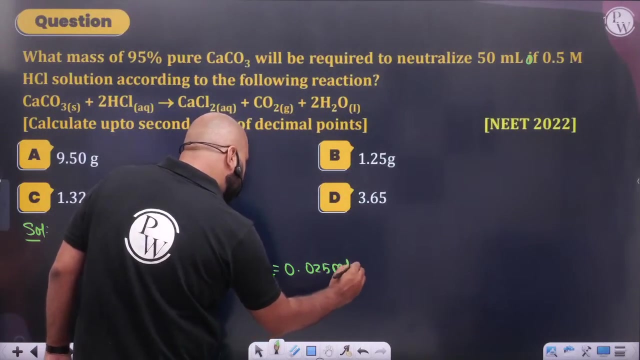 HCl's moles. 50 ml of this. so, sir, 50 ml of this, 0.5 into 50 upon 1000,, 50 upon 1000, how much is this? 10, see this 0.025,. so many moles are there. so many moles are there whose HCl's. 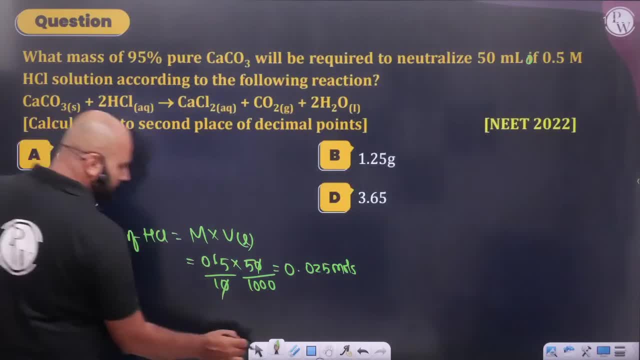 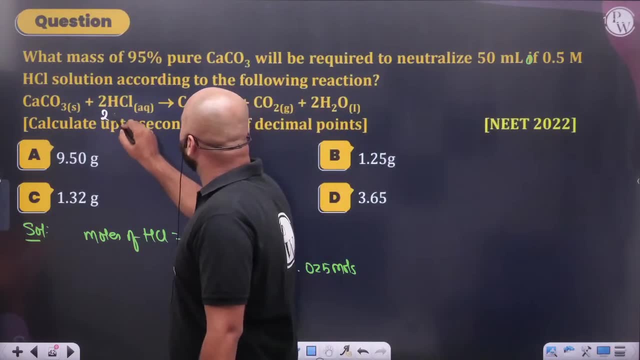 Sir, see the reaction from its two moles, from its two moles, from HCl's two moles, from HCl's two moles. how many of its moles are reacting? One mole, So, sir, what does this mean? 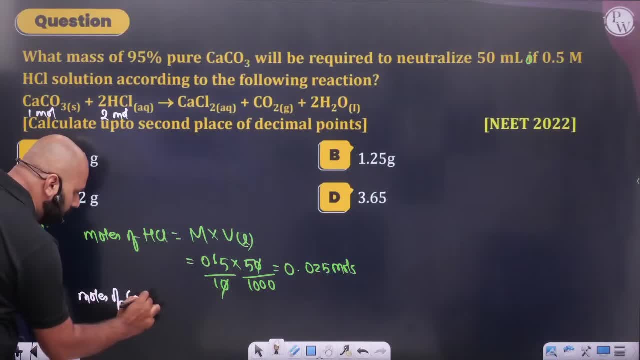 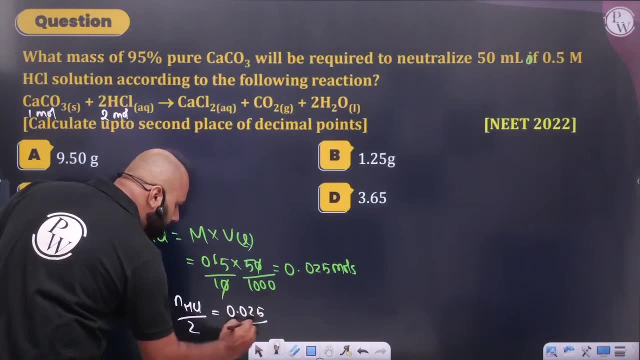 Moles of calcium carbonate. what will be known in the exam hall? Sir, halve the number of HCl's moles. How many moles are there? 0.025.. How do you divide this From 2. How much will it be? 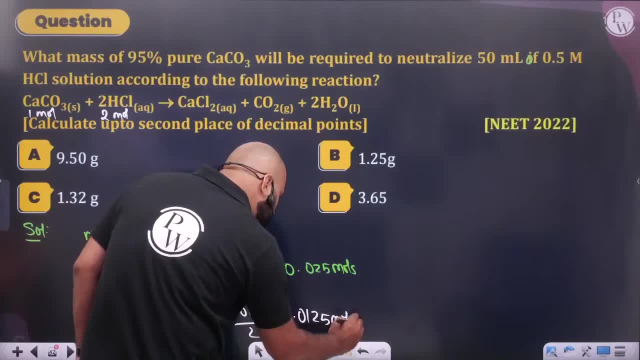 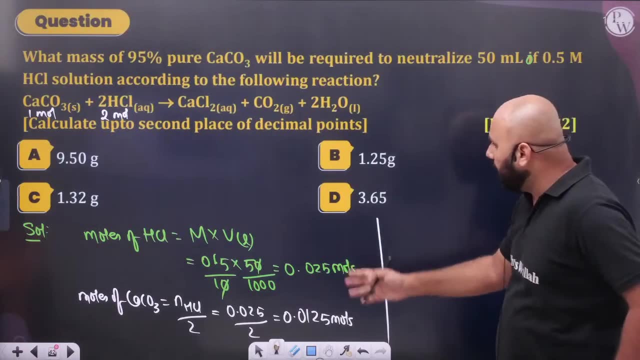 0.0125 moles. How many are the calcium carbonate's moles This much? How did you find out? Nothing, brother, Okay, nothing. What are you doing? I will tell you the normality. I will tell you the redox reaction, not now. 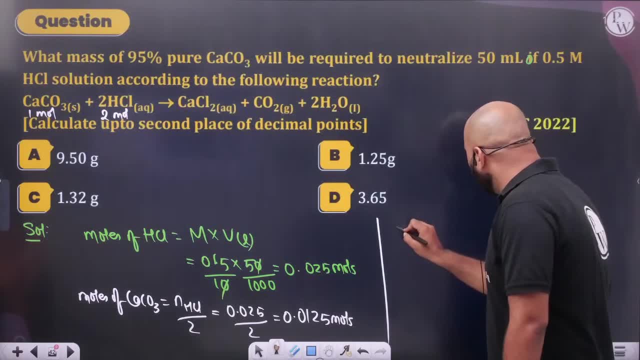 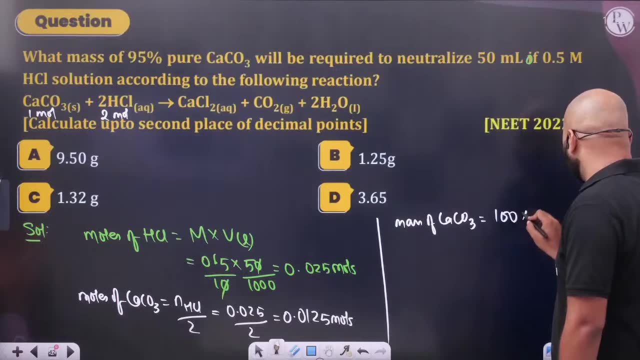 See, I am talking about moles of calcium carbonate. If moles are there, then how much is the mass of calcium carbonate? How much will this mass of calcium carbonate be? How much is the mass of one, 100 of one mole? 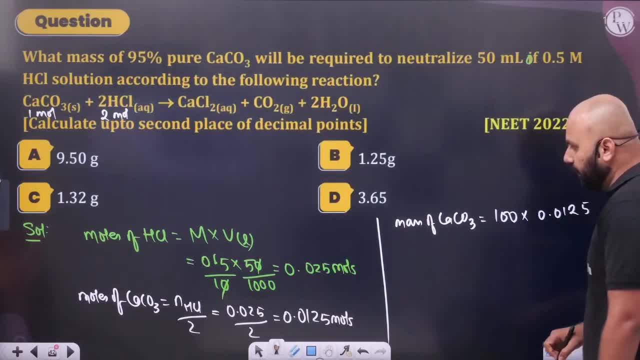 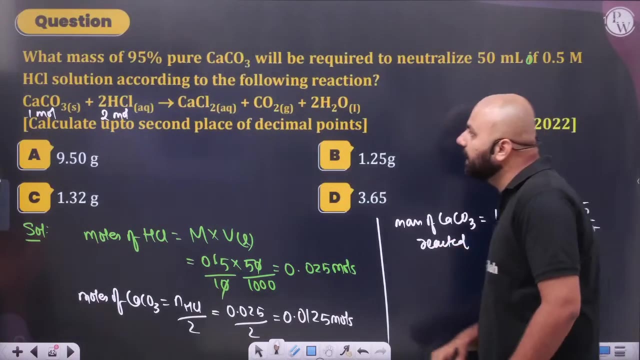 0.0125.. 0.0125, divide it, How much will this be? How much is the mass? 1.25 gram: This is the mass of calcium carbonate which has been reacted right. How did you find out? 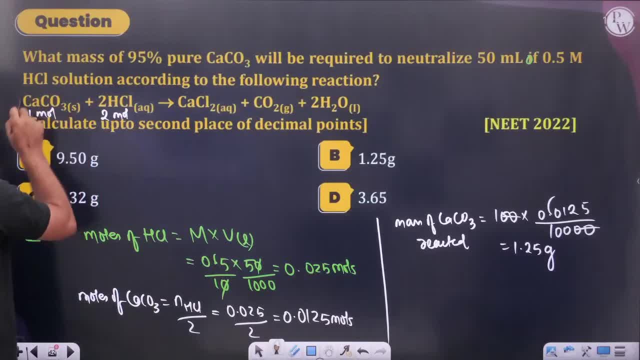 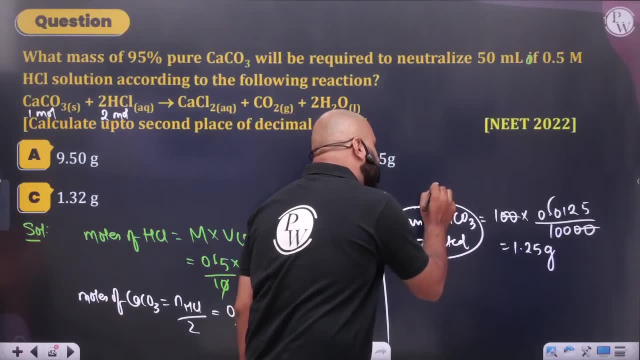 Because who will react with HCl? Who will react with HCl? Pure calcium carbonate. So the mass of calcium carbonate which was reacted, we can say that this is pure calcium carbonate. How much is pure calcium carbonate? 1.25.. 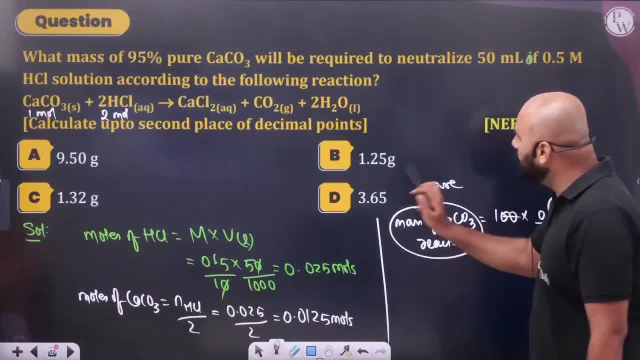 What is being told to me, Sir? don't tick 1.25. answer 1.25 will not be the answer. Don't make this mistake in the exam hall. Don't make this mistake Why? Because I am telling you again and again: 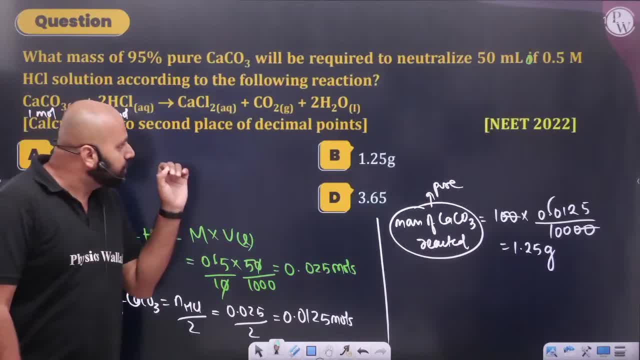 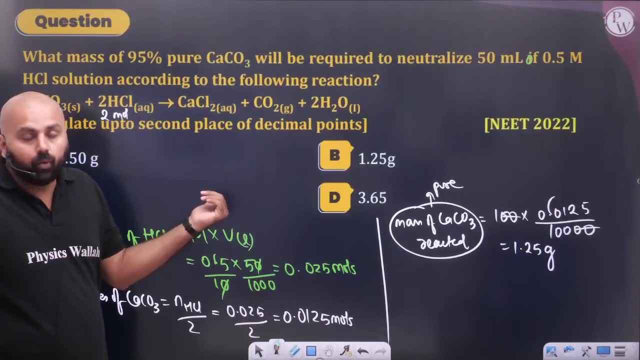 What does purity of concept say, Sir? the mass which will react, the mass which is reacting, what will it start doing? It will not be equal to the taken mass. It means the mass which will react will not be equal to the mass of reactant sample. 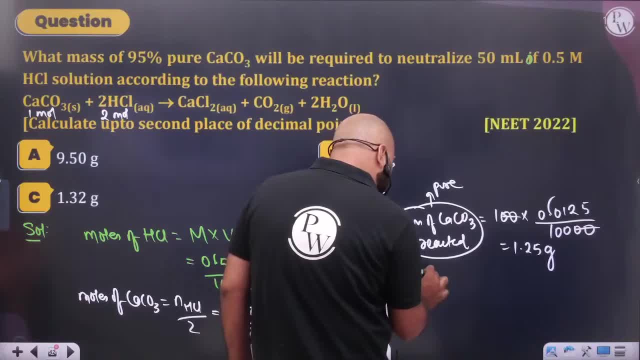 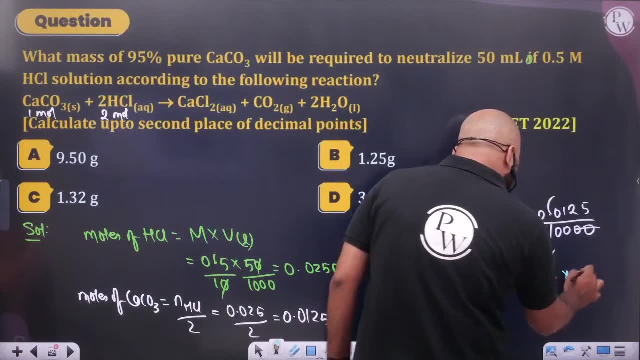 So it means this answer will not be there. Let mass of calcium carbonate sample. Calcium carbonate sample: How much will be the mass of calcium carbonate sample X? So, brother, let's do one thing: How much will be pure calcium carbonate? 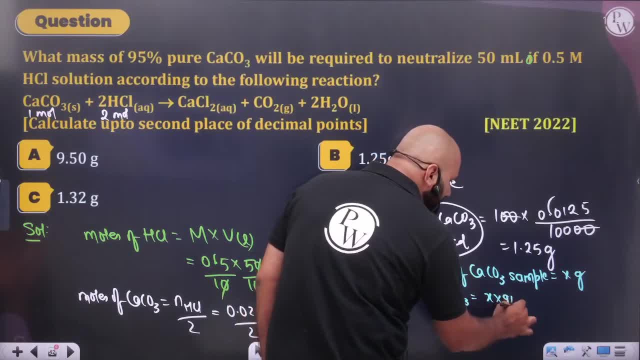 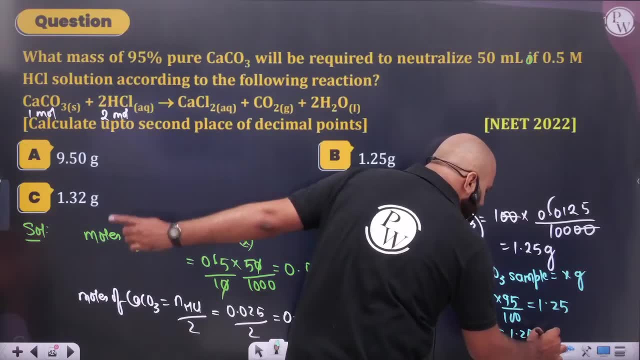 Pure calcium carbonate, 95% of X, and that must be equal to 1.25.. Sir, you will find the value of X, Sir, the value of X, In the given option. see whose 95%. you are getting 1.25.. 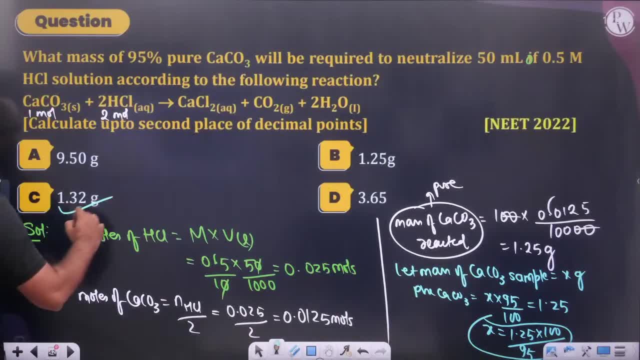 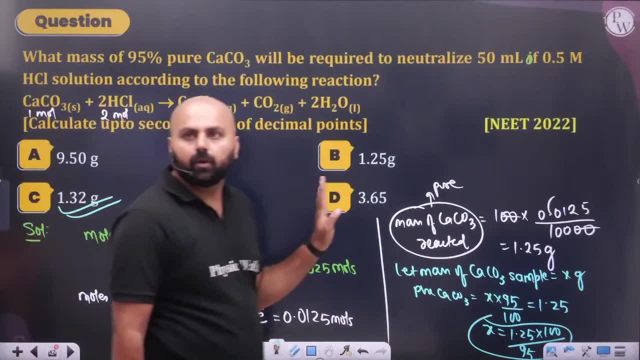 Whose 95%, you are getting 1.25.. Sir, as far as I can see, 95%. If you take 95% of this, then it will be 1.25.. See in the exam hall. Don't do this work in the exam hall. 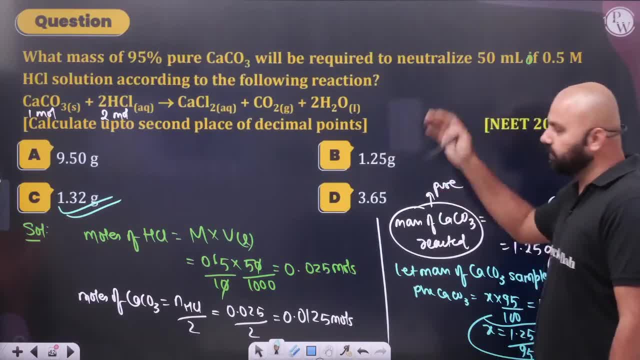 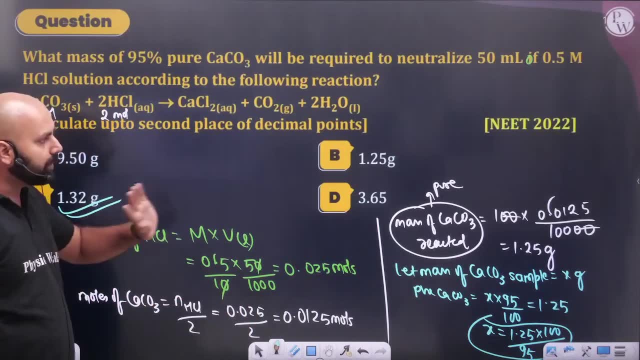 Don't tick this option. This option was given for this only, So that those who are weak-hearted quickly tick and go. So don't do this work, It will be done, Be sure. So, brother, this is my whole first chapter. 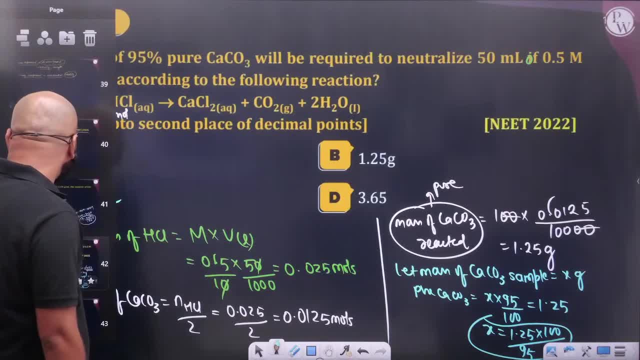 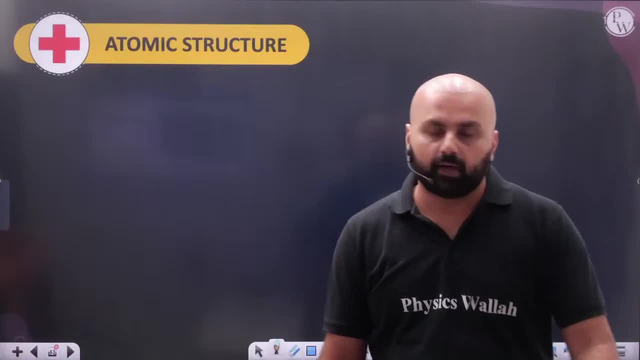 We revised the whole concept in two hours. Reason is that there are many concepts in it. There were many concepts where I will revise the normality part. I will revise the normality part. I will revise the normality part. There will be the normality part. 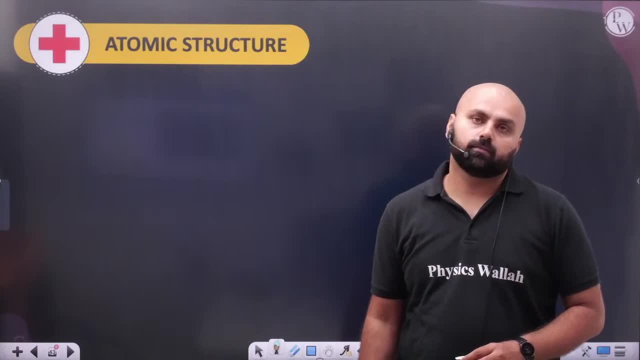 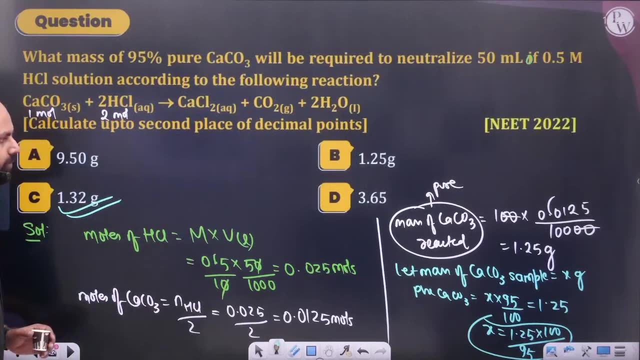 Okay, The normality part will come in the redox reaction. We will talk about normality redox reaction. Okay, Brother, you practice at home also. I have told you a little while ago. Okay, Tell me once What is written. 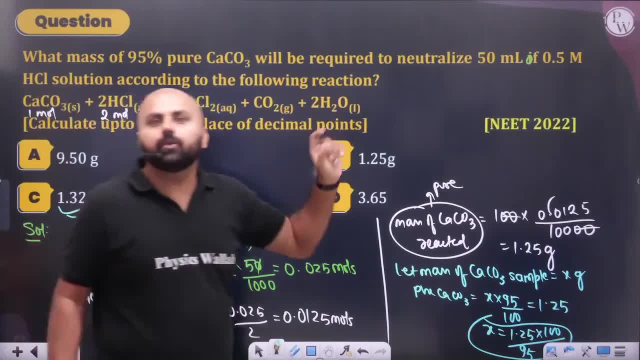 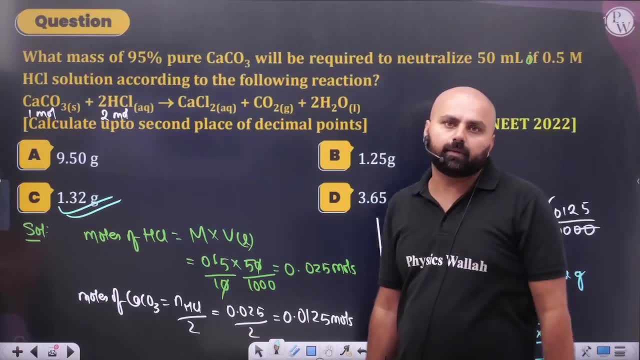 What mass of this will be required? That means the sample taken has only 95% purity. How much calcium carbonate is reacting? I am saying that only 95% of my marks come. So if 95 comes, then how much will be the total mass? 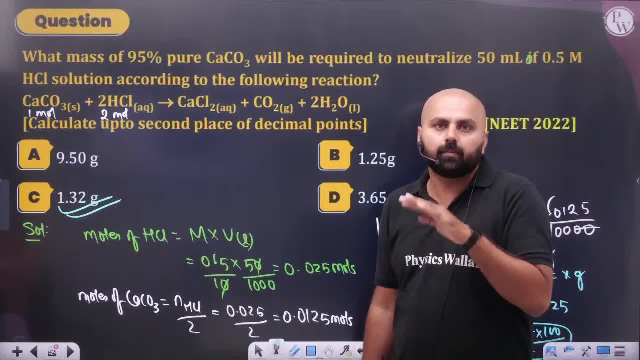 It will be 100, right. If my 95 marks come, then it means how much will be my marks? 95.. So how much will be the total? 100.. So he is saying that, sir, how much is the pure? 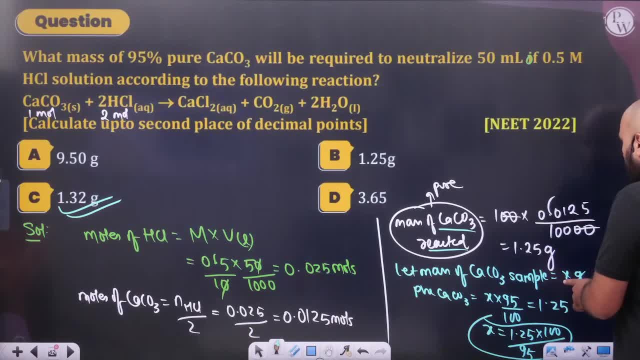 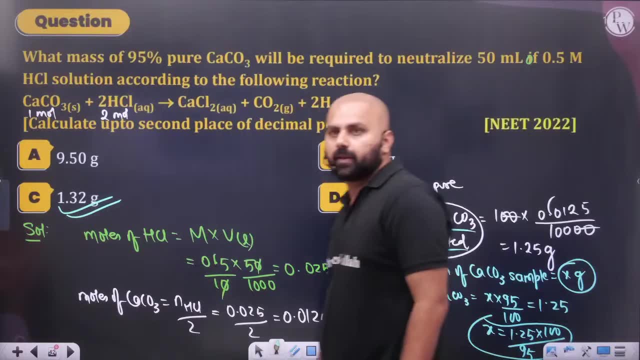 95% Suppose how much calcium carbonate of the sample is taken. How much mass of the sample is taken- X gram. How much 95% of X gram should come Purity? Do it Okay. See this brother. 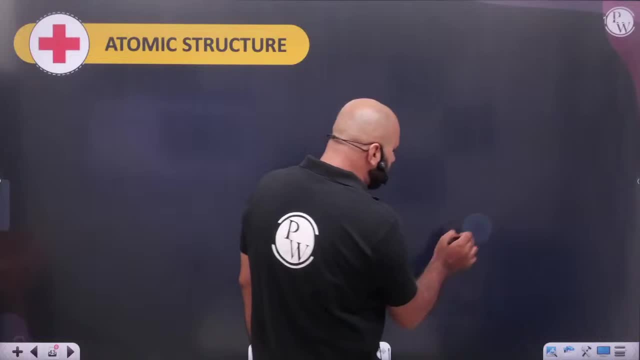 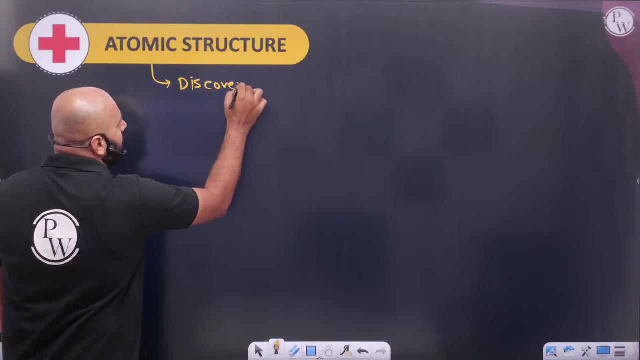 In the atomic structure. In the atomic structure you can directly take the mass of the sample. Okay, In the atomic structure you have three things. In the atomic structure you can talk simply. If someone tells me that let's talk about the discovery of electron and proton. 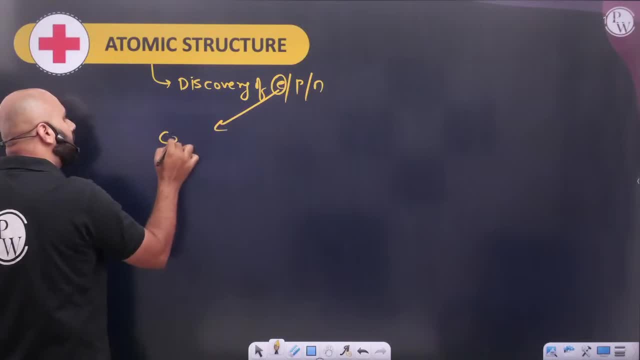 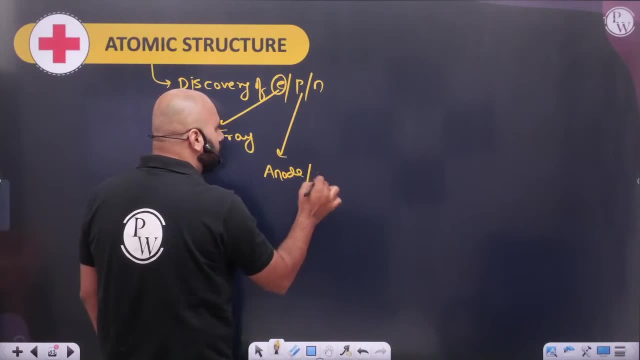 Electron, proton, neutron. So what did I have for the discovery of electron? I had cathode ray. It was a cathode ray experiment. What was there for the discovery of proton? It was anode ray. Or what did we call anode ray? 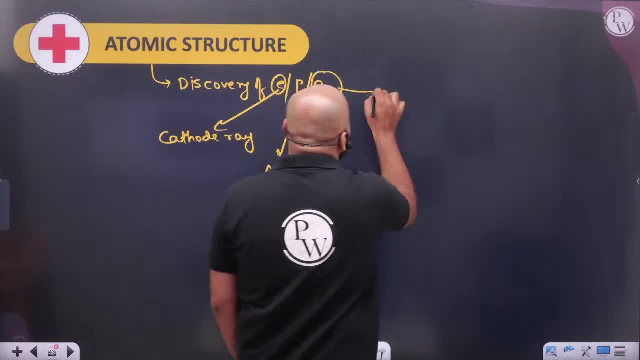 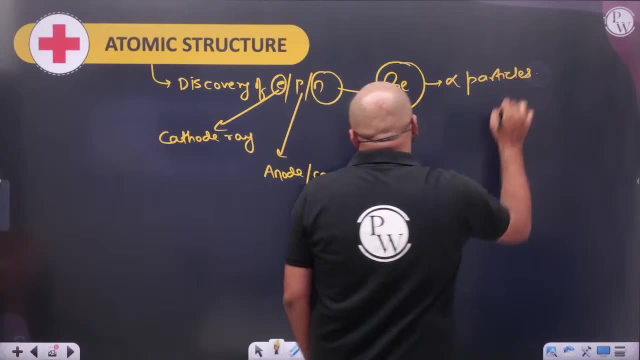 We used to call it canal ray. And what did we do for the discovery of neutrons? We used to bombard radioactive alpha particles on beryllium. This is what used to happen. Okay, Sir, what was the difference between cathode ray and anode ray? 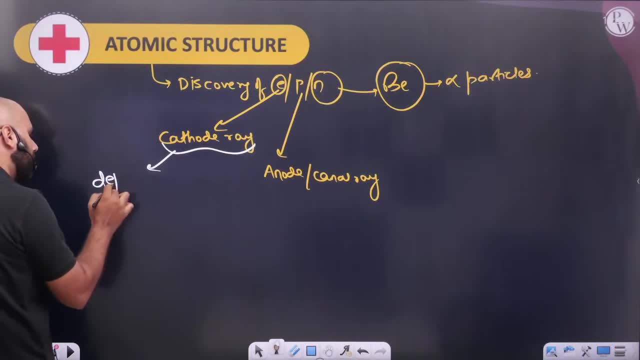 If you talk about cathode ray, then it does not depend on whom Not dependent on Not depends on Gas. It does not depend on whom On the gas, What is the gas And who is the material of the cathode? 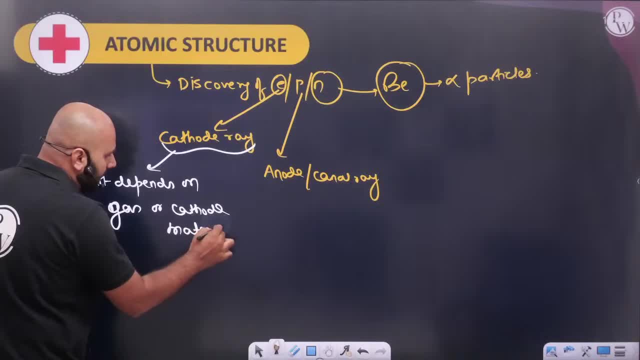 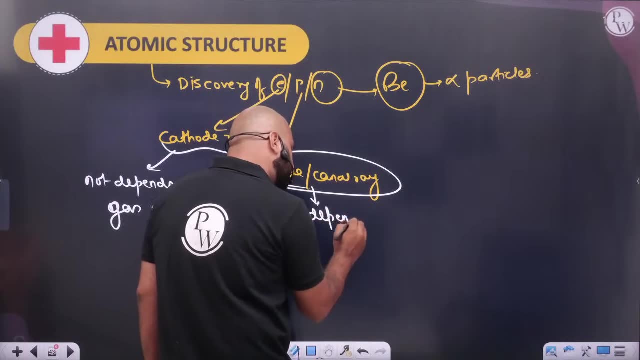 The material of the cathode does not depend on all this, The most basic thing to talk about in the atomic structure. If you talk about anode ray, then on whom does anode ray or canal ray depend? Depends on, Depends on. 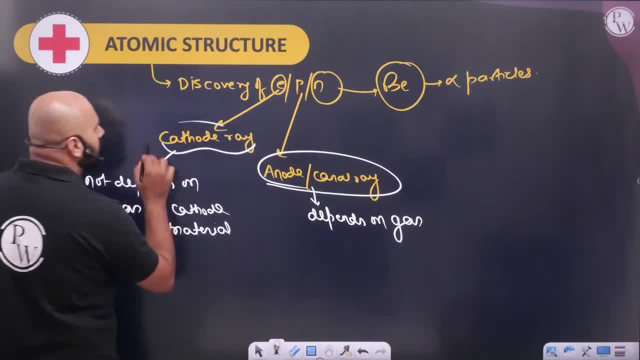 Gas. After that, all these cathode ray, whether it is canal ray or anode ray, all these radiations of anode ray, cathode ray, all these air conduct, whose example was this Of air Conduction of air. 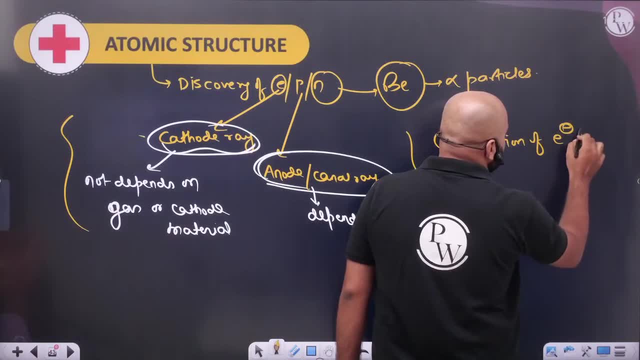 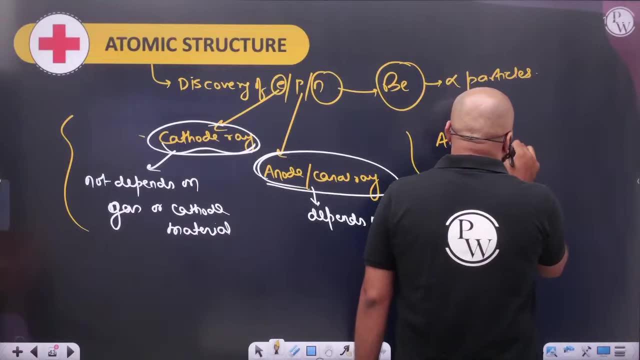 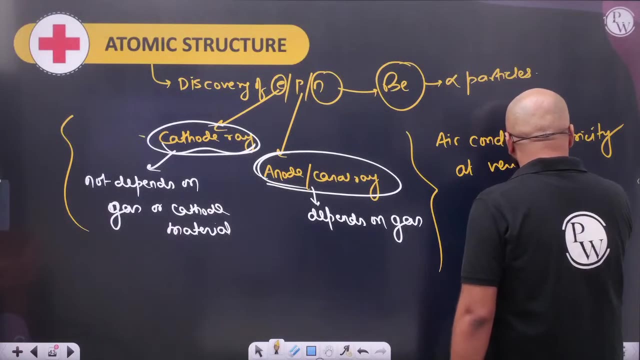 Conduction of electron in air, Or talk about conduction, Conduction in air. If the conductivity of air, Air conductivity, Air conducts electricity, All this, All these stories on which we were talking- Air conduct electricity at very low pressure. 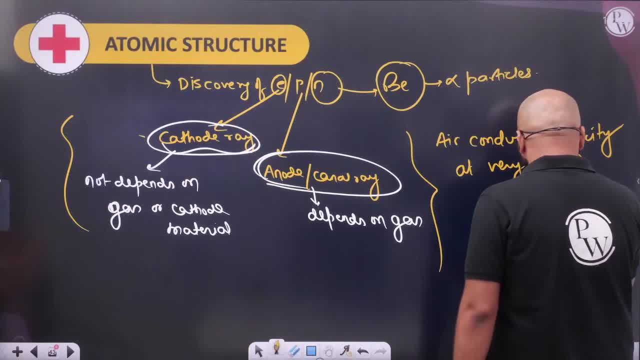 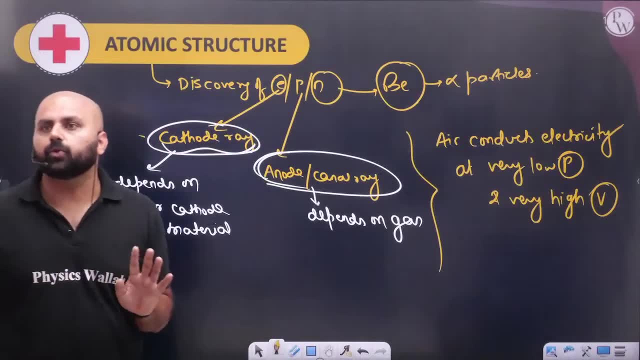 Very low pressure and high voltage, Very high voltage. This was the basic story. You will see this little things in the NCRT. You will see these little things. The break will be 5.5 now 5.5.. Atomic structure is a small chapter. 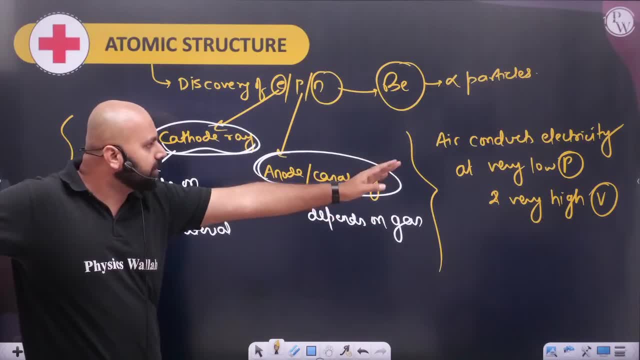 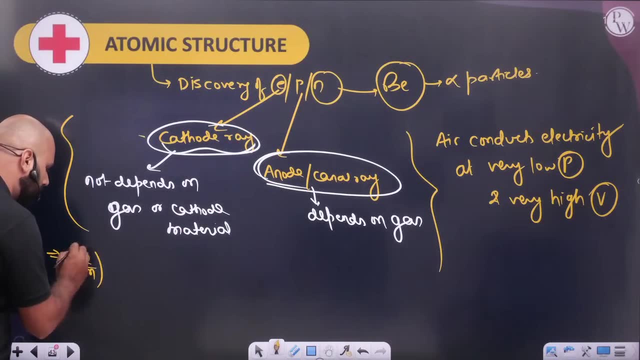 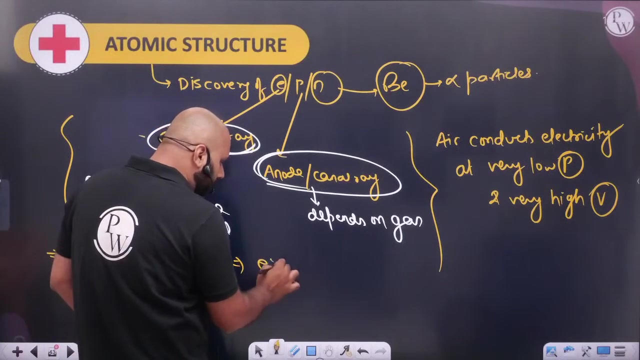 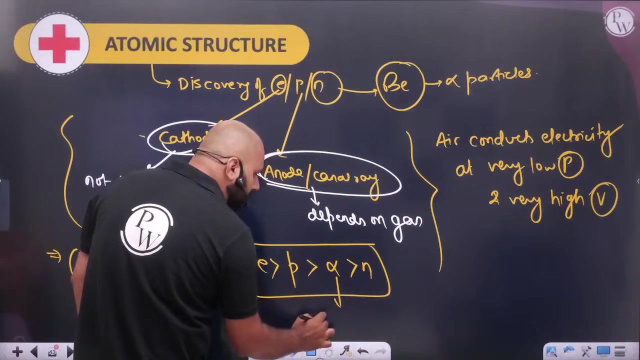 It will be done soon. Listen to the story. Air conduct, electricity at very low pressure and very high voltage, Anode ray, cathode ray, canal ray. Here we will have 2-3 things. first, see the ratio of E by M, E by M ratio, or we call it specific charge. what is this Specific charge ratio? you will see the ratio of specific charge, E by M ratio, whose ratio is more. if we talk about the most, then electron, then proton, and then alpha particle, then neutron. remember that the ratio of alpha particle is E by M ratio of- if I am writing alpha particle, 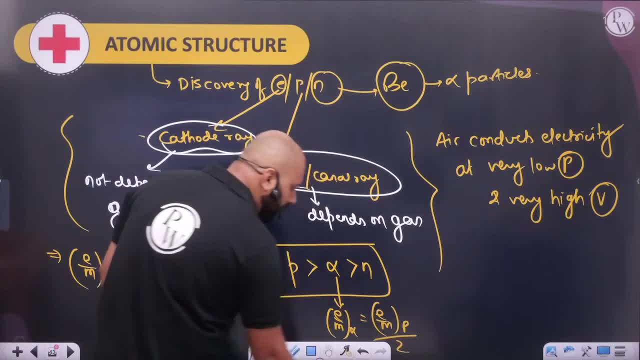 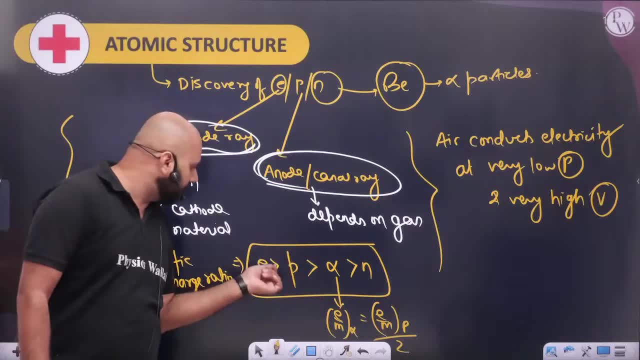 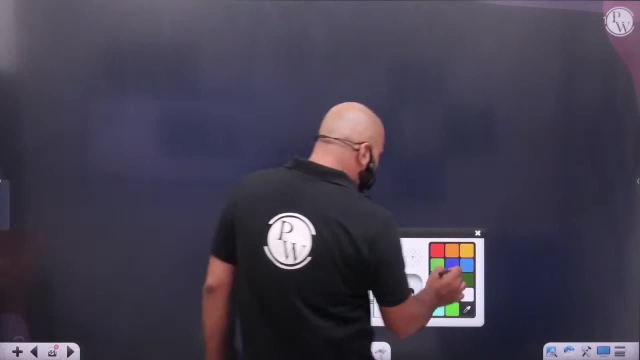 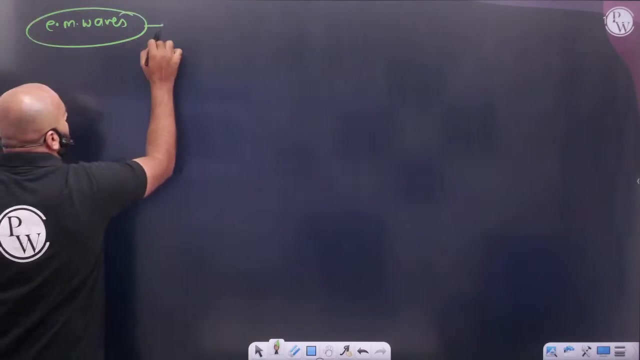 then E by M, ratio of proton is just half. whose is the most electron? then proton, then alpha. then whose is neutron? okay, electron, proton, alpha and then neutron. do it according to this. okay, see this: electron, proton, neutrons. after that we have electromagnetic spectrum. when electromagnetic EM waves are talked about, let me tell you all the charged particles. charged particles, charged particles, are never part. 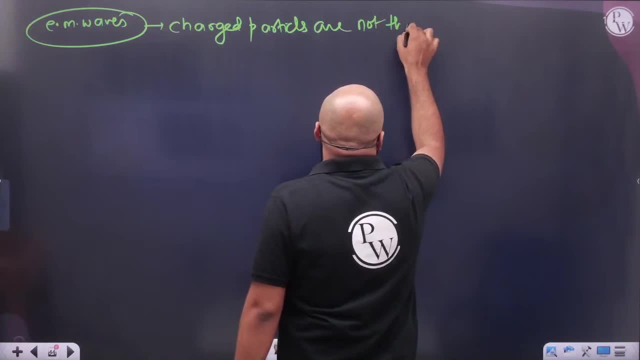 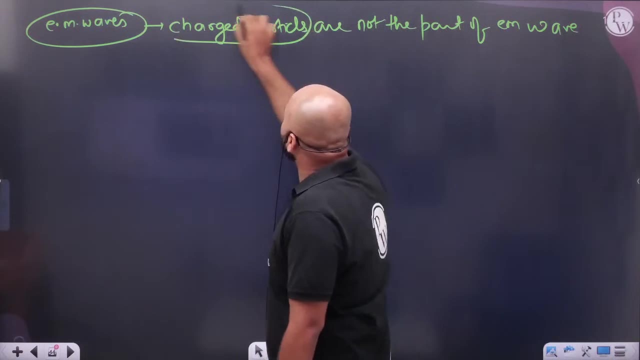 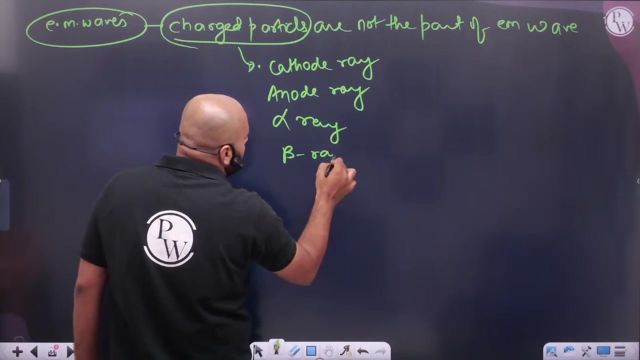 are not the part of, are not the part of EM rays, whenever you see the waves generated by electrons, then it will never do, sir. charged particles will not happen. why, Sir, electromagnetic waves? remember cathode ray. cathode ray will not happen. cathode ray, anode ray will not happen. cathode ray, anode ray will not happen. alpha ray will not happen, beta ray will not happen. they are not the part of, they deviates. 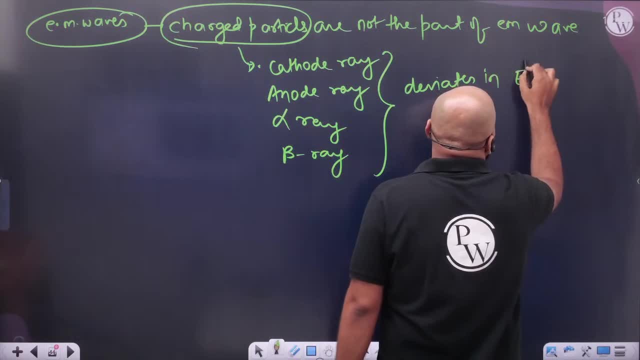 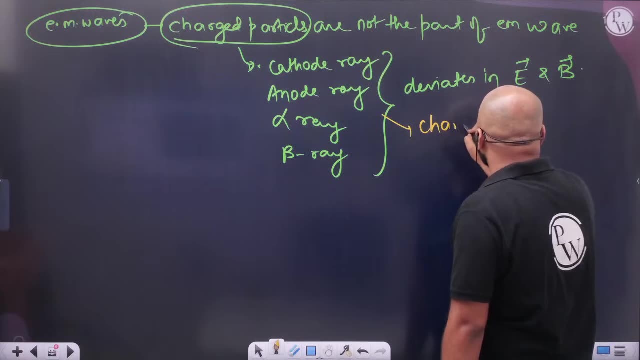 deviates in electric energy, magnetic field. They deviate in electric and magnetic field. Why? Because they charge on themselves. They are charged, So that's why they deviate And that's why they are not the part of EM waves. 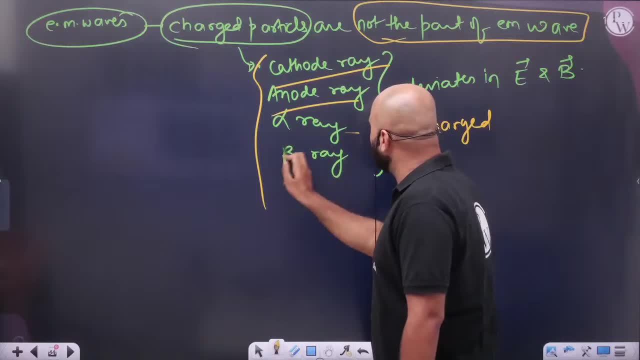 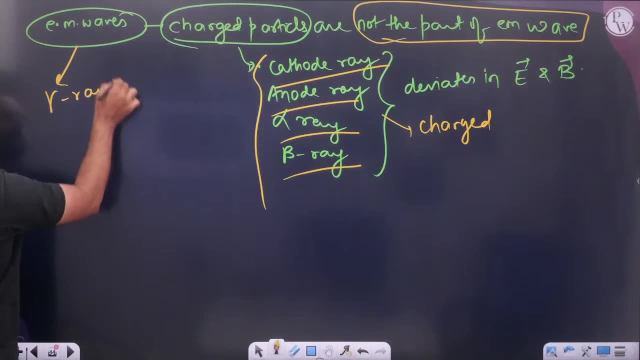 They are not part of EM waves. Cathode ray, anode ray, alpha beta are not part of EM waves. If you want to remember, then remember that you have gamma ray, which is the part of alpha ray, Or x-ray, which is the part of alpha ray. Now, when it comes to x-ray, remember how x-ray is produced. 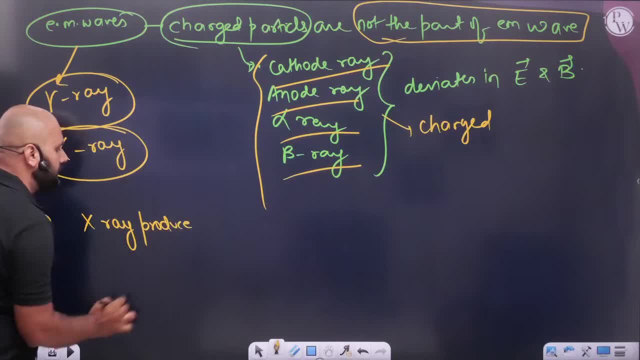 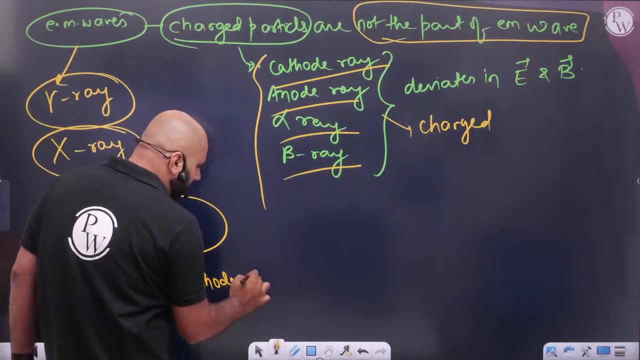 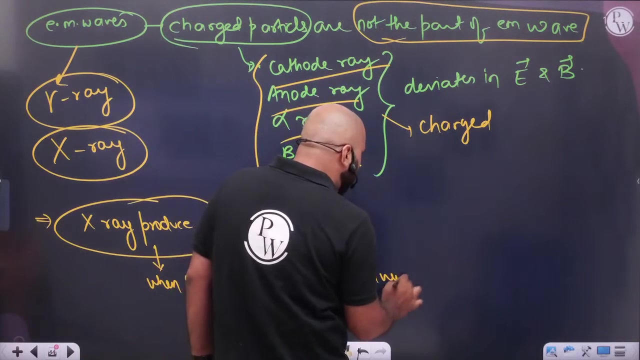 To produce x-ray. x-ray is produced when x-ray is produced When cathode, when cathode ray, when x-ray is produced, when cathode ray falls on cathode ray falls on heavy metal. If any heavy metal like platinum falls on them, then what will be generated? X-ray is generated. 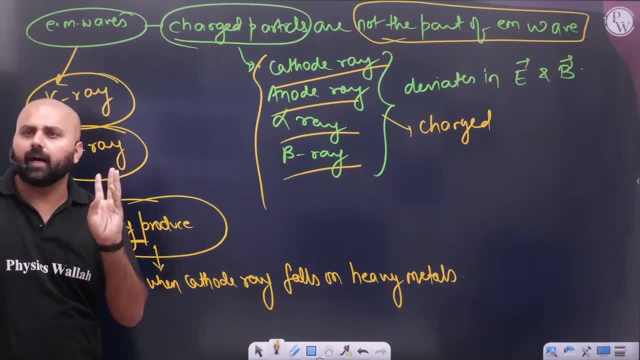 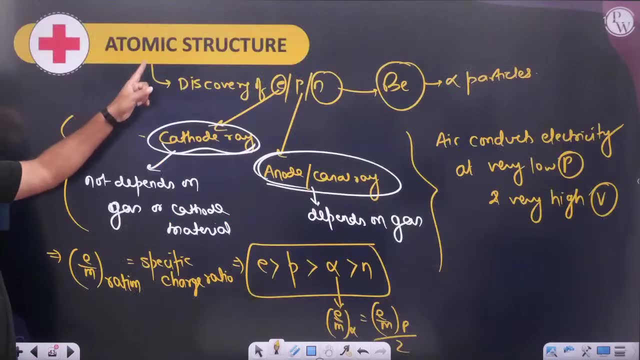 Again, these are small things, small, small things. See, let's talk about atoms. If we talk about atoms, then catch these small things. Okay, We have atoms, cathode, anode, air conduct, electricity, specific charge, electron, proton, alpha, neutron. 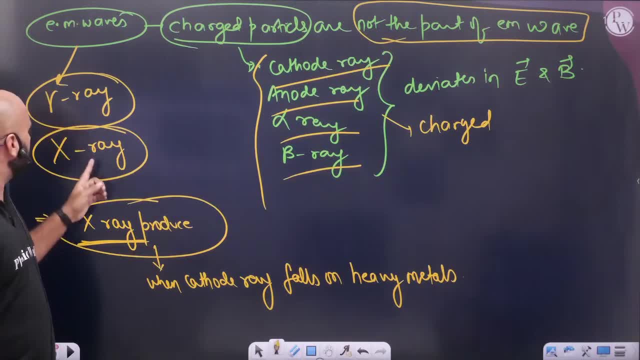 We are talking about all these. Whose part is this? It is not the part of EM waves. This is the part of alpha rays, gamma rays. We had done different experiments. We have seen all those experiments. For example, a question was given like this: 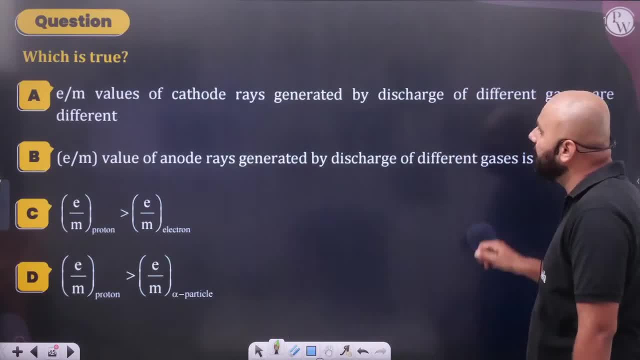 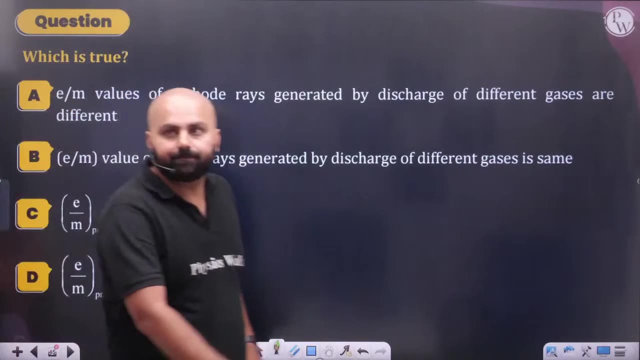 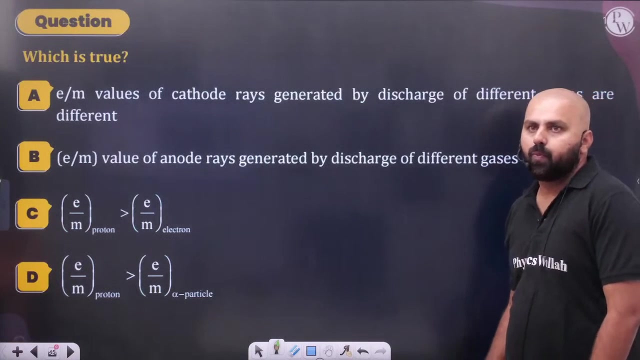 See this. A question was given like this, Where all the concepts are mixed. Which is true, Which is true? Will you tell Which will be true, Which will be true, Which will be true? You will get the PDF, brother. 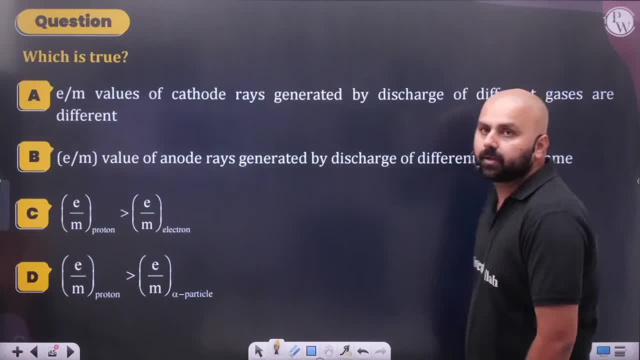 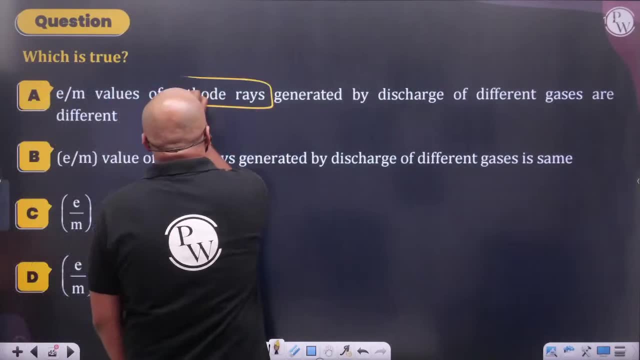 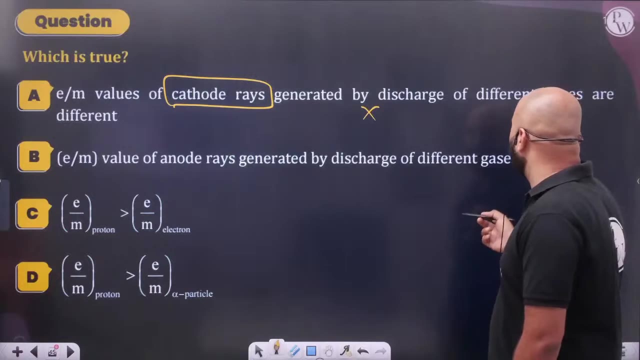 Quickly, What will happen, Which will be true? Quickly tell the answer. Who will have the em value of different gases? The cathode ray never depends on the cathode ray gas. Then this statement will be wrong. What will be the anode ray? It depends on different gases. Then what will be this? This also will be wrong. 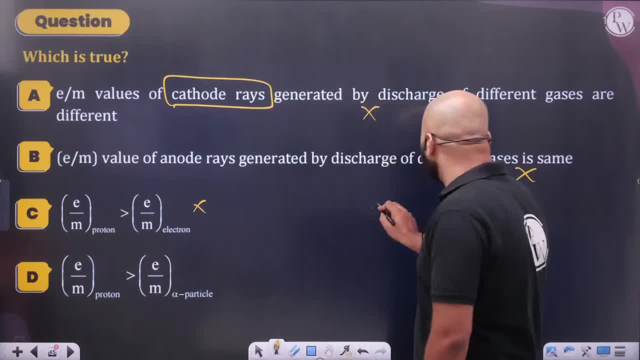 E by M ratio, with proton electron. No, Who has the most electron Then? who has proton? Then? who has alpha particle? Then who has neutron? Who will have more electron? What will be the right statement? What will be true? What will it be? It will be D. Keep this in mind. 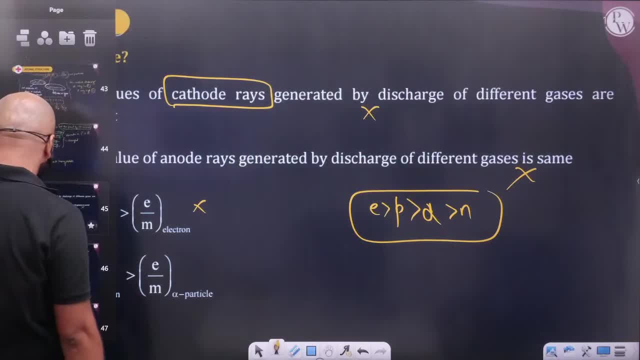 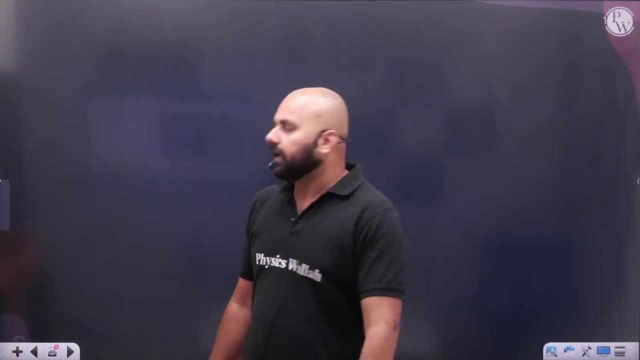 If you look at the second one after this, if you look at it now, like there are electromagnetic radiations. So what is the way to remember EM waves? You must have done it in physics too. Here we try to remember again and again. 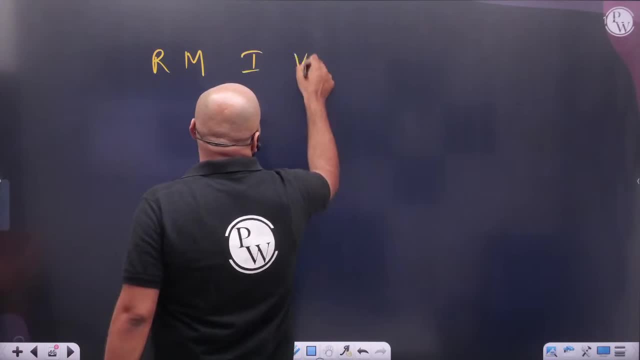 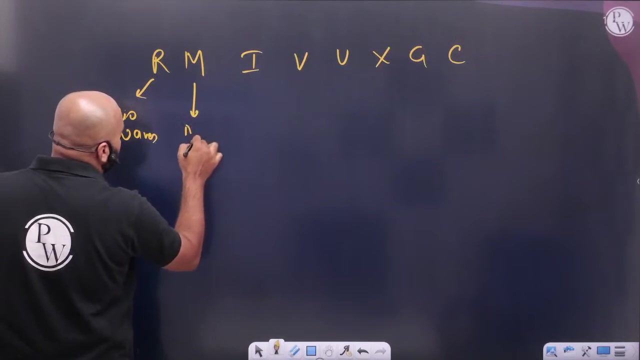 that in radio. I promise, I vow you, I vow you, I will not chat with my ex-girlfriend Means. these radio waves have happened. What has happened? Radio waves have happened, Sir. remember a simple trick to remember In radio: radio waves, radio waves. 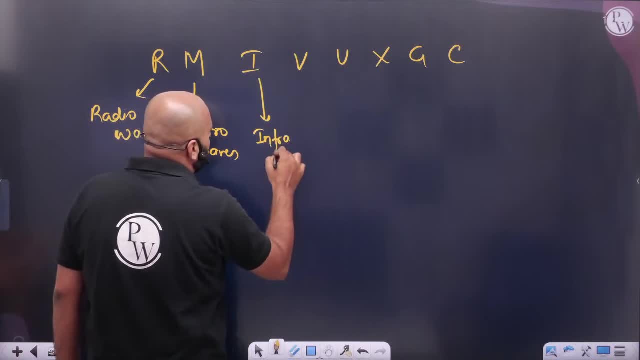 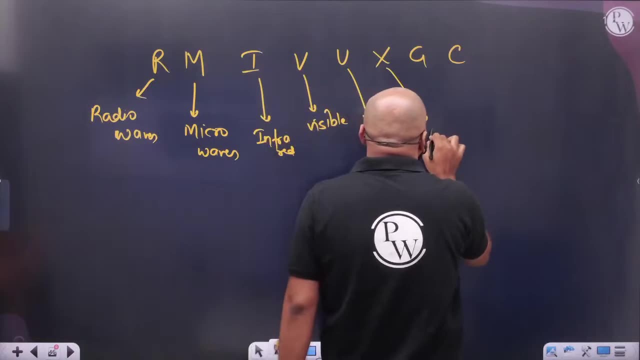 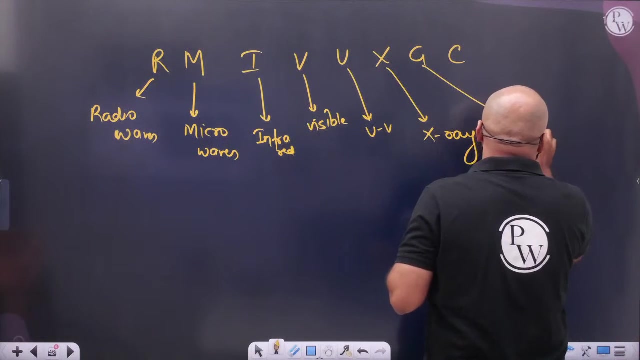 microwaves. infrared, infrared- What has happened? Visible- What will happen? Ultraviolet UV radiation, X-ray In radio- I promise I will not chat with my ex-girlfriend. Gamma rays: What will happen? Gamma rays? 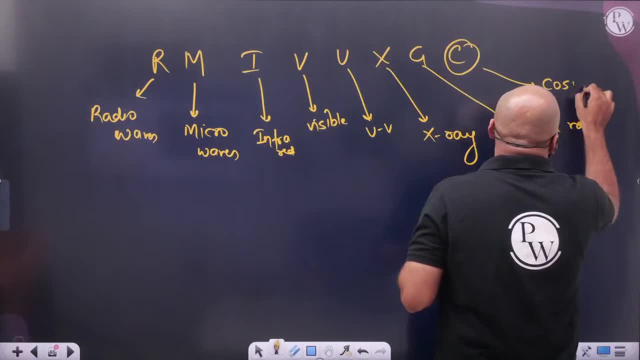 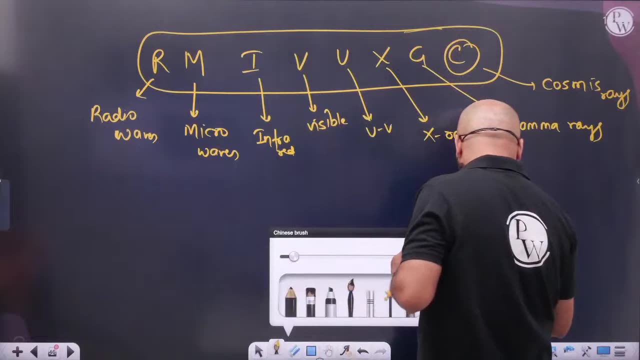 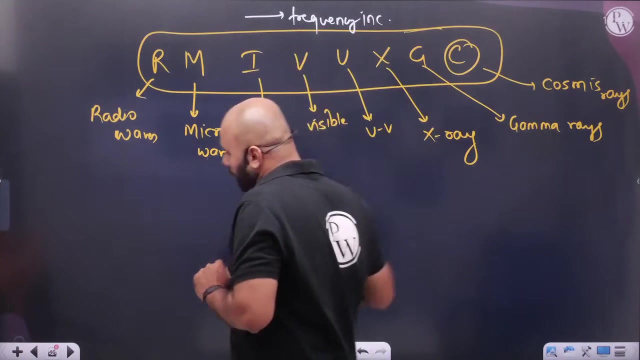 And what will happen? Cosmic rays, Sir generation. OK, Try this. I will teach you this too. Sit down, Don't actually stand here. There is no problem. The problem is that if I tell you this to me, then you will get a chart. 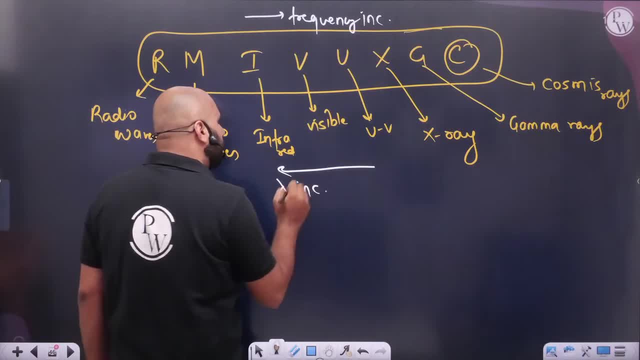 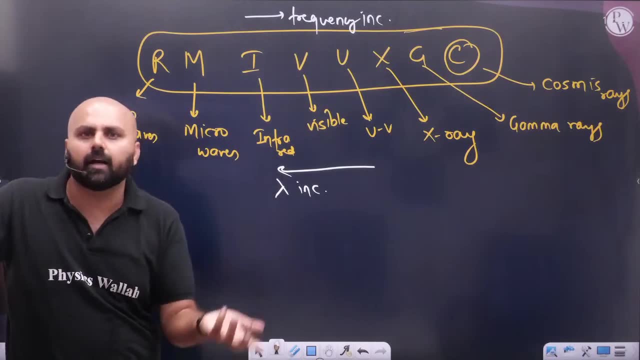 now, the way to remember is: brother, you go from here to here. when you say this, what will happen to you? How will the frequency be? what will be the frequency If you go here, from here? You have to remember the questions in your own way. 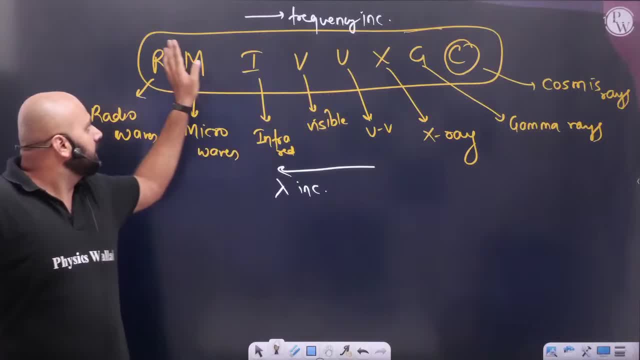 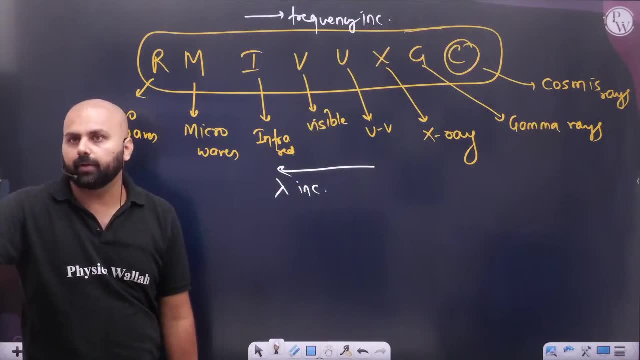 Questions should be attempted from you. The way to know the frequency is that as soon as you give a promise on the radio, you know what is going to happen with you. I won't chat with my ex-girlfriend, Okay, As soon as you remember. 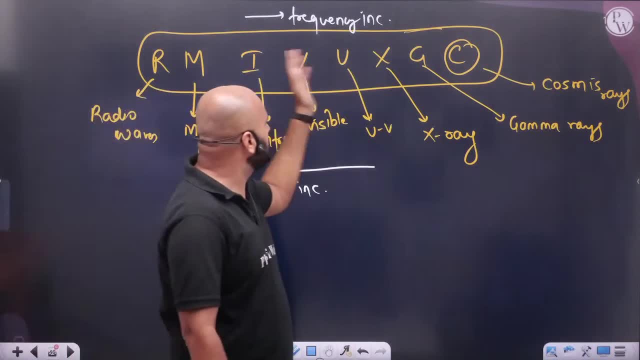 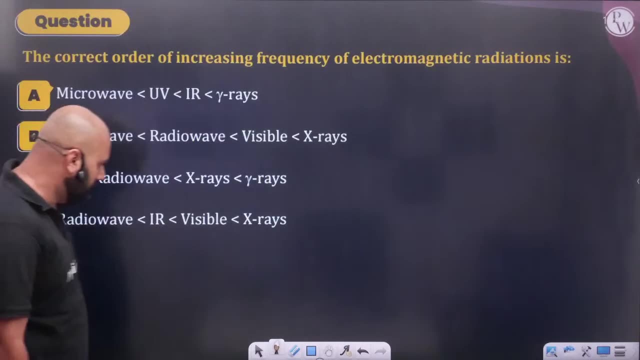 Okay, you can remember as soon as you remember. I promise on the radio, I promise I won't chat with my ex-girlfriend. This is the way you can remember EM waves. If you remember, then tell me the answer to this question. 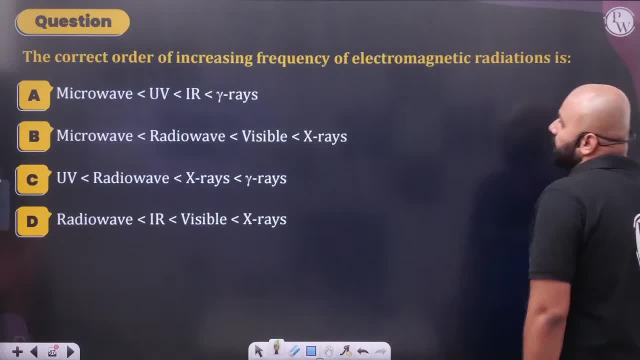 If you already know, then tell me the answer to this question. Tell me the answer to this question. Tell me the answer as soon as possible. See for yourself- You have to see this in the exam hall- What will happen, What will be the answer. 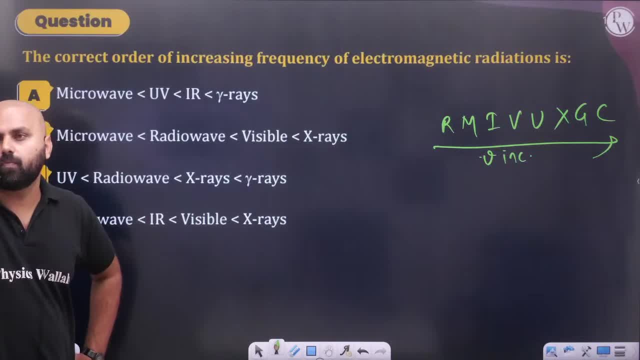 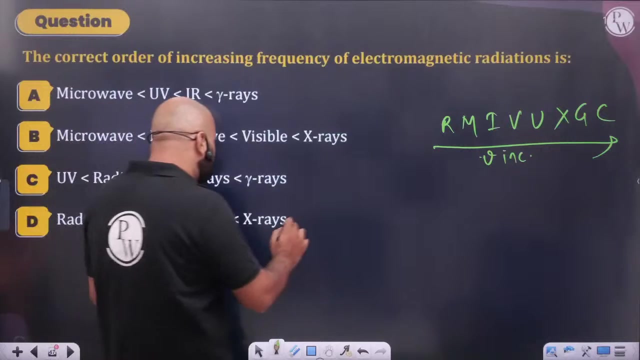 Okay. What will be the answer? What will be the answer? What will happen? What will be the answer? What's the answer? Radio order- Micro order. Which answer will be correct? D option will be correct. D option will be correct. 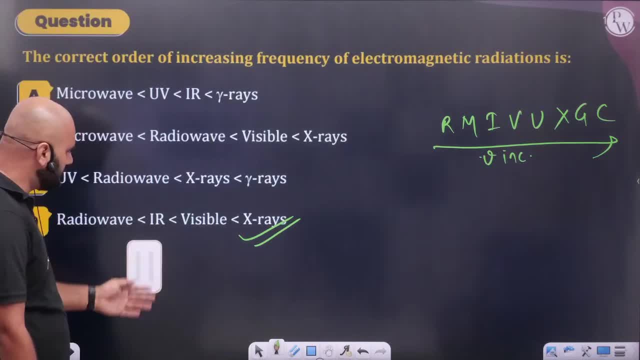 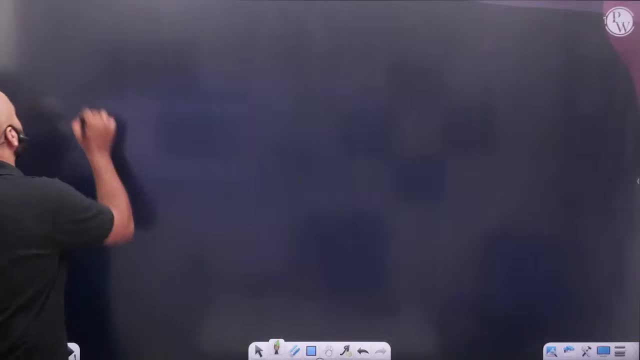 This is what you are talking about in the electromagnetic spectrum. This is what you are talking about in the electromagnetic spectrum. See the basic things. See the basic things you have. Okay. Who asked me about Planck's Quantum Theory? If we talk about Planck's Quantum Theory, 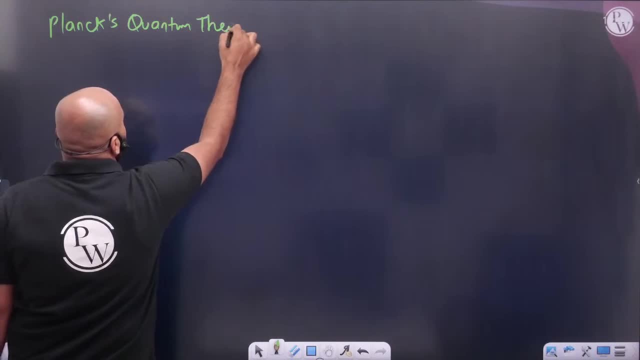 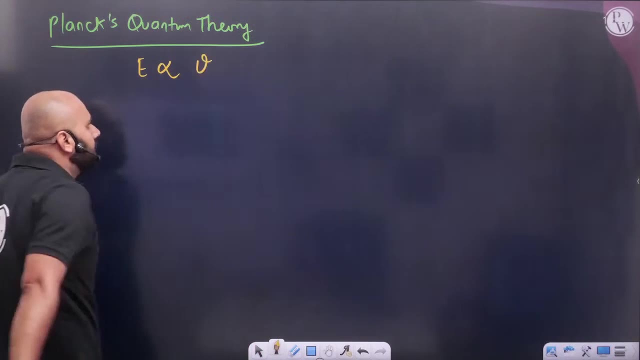 If we talk about Planck's Quantum Theory. What will happen in Planck's quantum theory, Sir? you already know What does Planck's quantum theory say, Sir. the energy of any photon is directly proportional to the frequency. So energy is equal to h into nu. 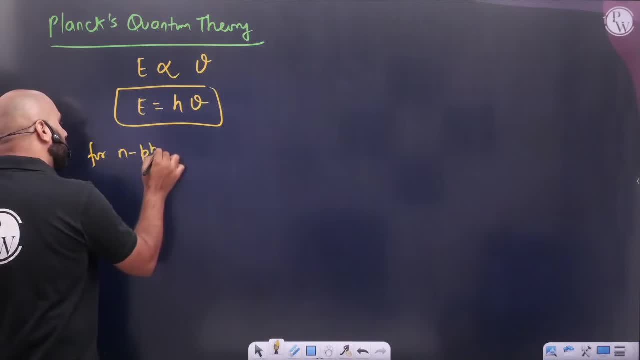 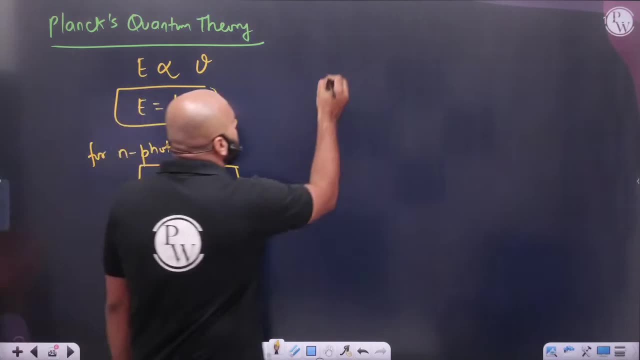 Okay, And if there are n photons, then what will happen for n photons? Energy is nh into nu. Energy will not become nh. Then we know that. sir, the frequency is: if I talk, c is equal to nu into nu, into lambda. 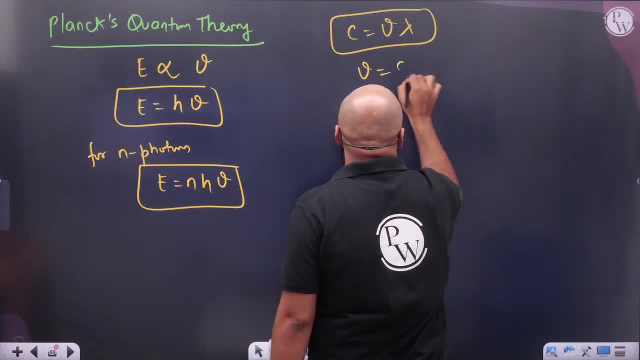 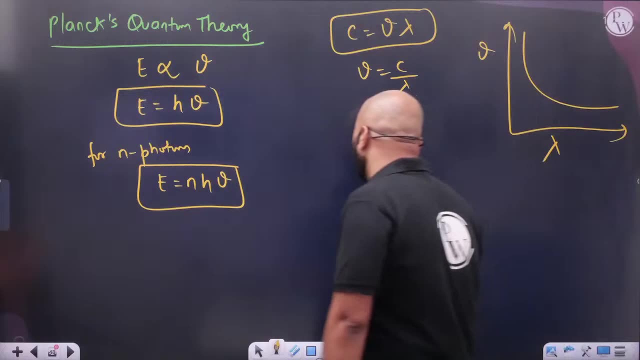 This is what we have studied in physics. So here, what can I put in place of nu c by lambda? Remember, if someone asks about the graph of frequency and lambda, then it will be an inversely proportional graph. If I am told this formula, then I can write it as hc by lambda or nhc by lambda. 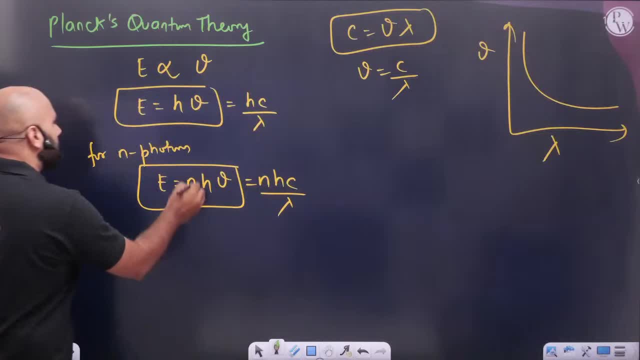 If I am asked these formulas, remember the number of n. What is n? Number of photons? And what will always happen? It will be a whole number. What will always be the value of n? It will be a whole number. The reason sometimes: 1 photon will come, 2 photon will come. 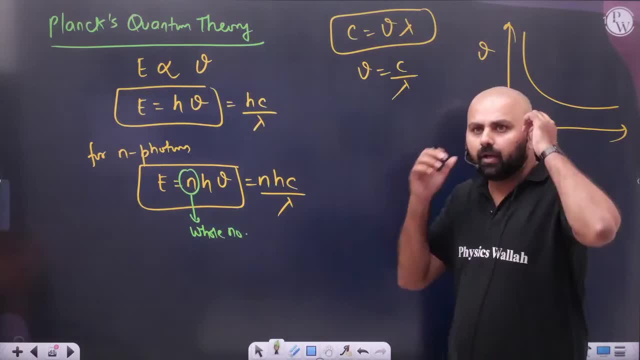 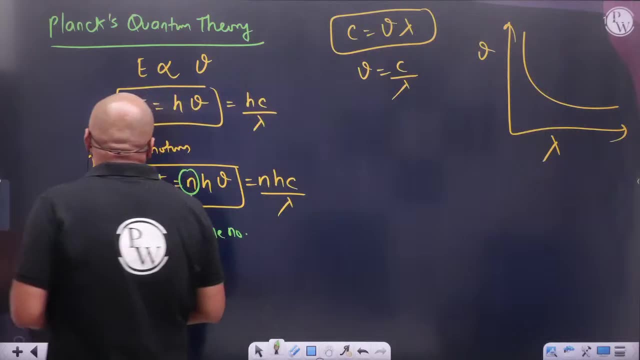 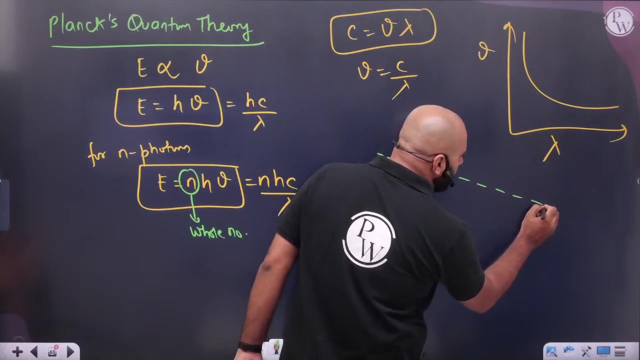 3 photon will come, 4 photon will come. Okay. So here sometimes a whole number will come, sometimes nothing else will come. Okay, We have obviously packets of energy. Planck's quantum theory was saying that any energy that comes, any radiation that comes, that is not a continuous form of energy. 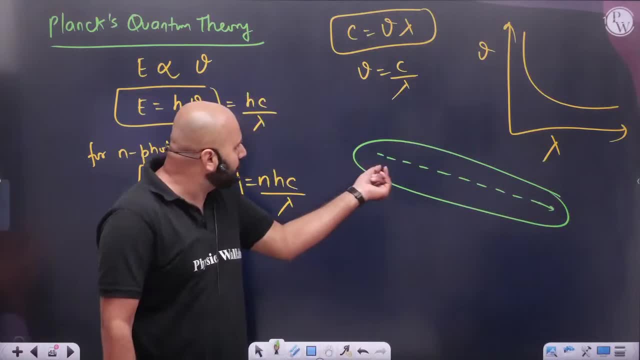 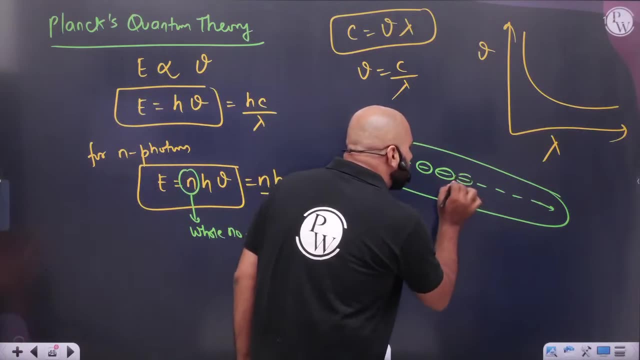 What is it? It is a discontinuous form of energy. What are the small things in it? Small small quantas, Small small quantum That they have packets of energy. He has energy. He has energy. Discontinuous form of energy. 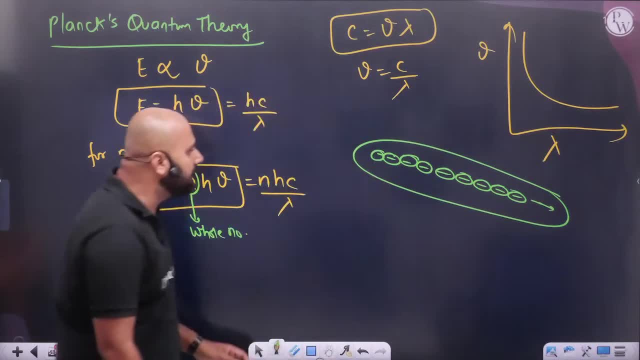 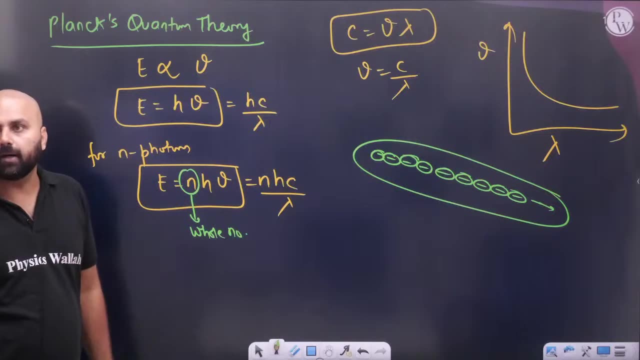 And if you see the discontinuous form of energy, then how much will be there in 1 photon h, nu or hc by lambda, Sir, what will happen in n photons, n, hc by lambda? Second thing, second thing: brother, look at this. second thing, look at this. if you have any person, look at this. if you have, if the new frequency absorbs and new 1 and new 2, if it releases, then the energy will be directly additive. 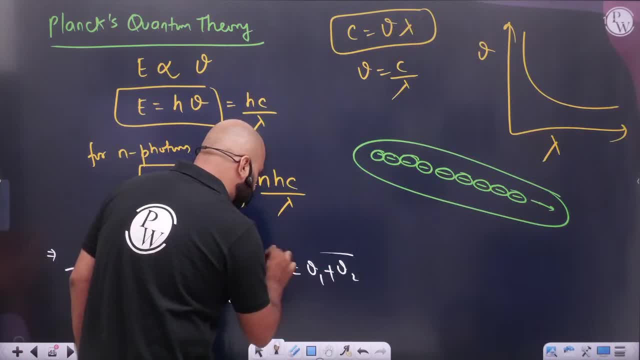 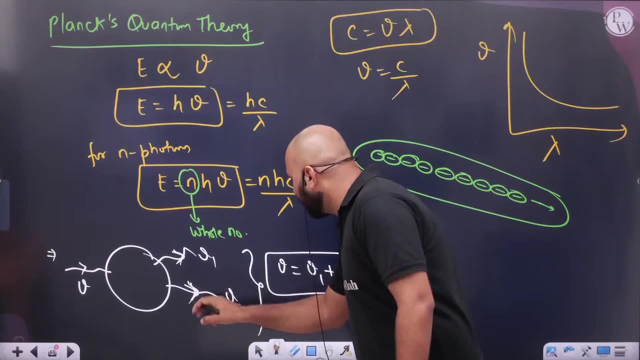 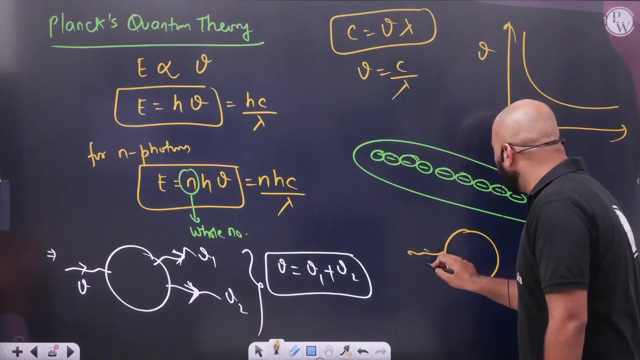 Here. new is nothing New: 1 plus new 2, you can use. Because what is the energy? It is absorbed, You are absorbing energy, you are absorbing frequency and releasing frequency. But if the same thing happens for whom? if the same thing happens in wavelength, sir, you are adding lambda wavelength, you are absorbing, you are releasing lambda 1 with you, you are releasing lambda 2, so the energy that will be inversely proportional, then 1 by lambda is equal to 1 by lambda. 1 plus 1 by what will happen. 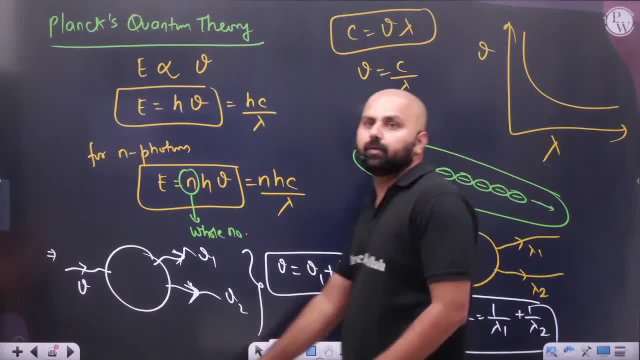 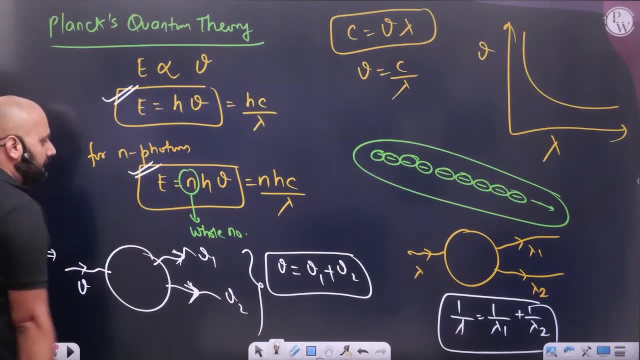 This formula will come: 1 by lambda 1 plus 1 by lambda 2.. Keep doing this. Listen to the story. In Planck's quantum theory, this formula came By using this. what are we doing? If there is a body, if it is absorbing? 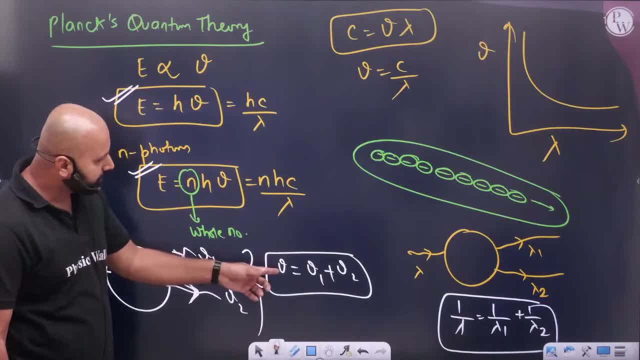 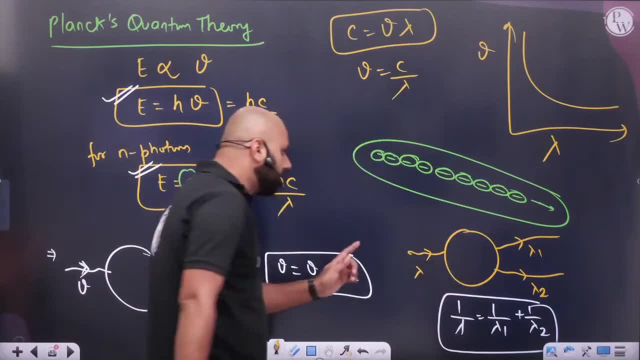 new frequency, if it is releasing new 1 by new 2, then frequency will be directly additive. Frequency will be directly additive. Frequency will be directly additive. But if lambda 1, lambda 2 is happening, then in its case 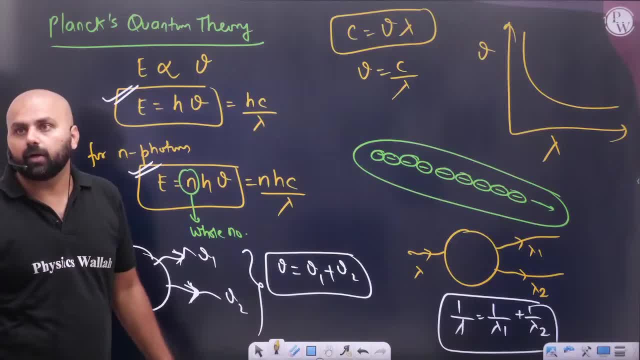 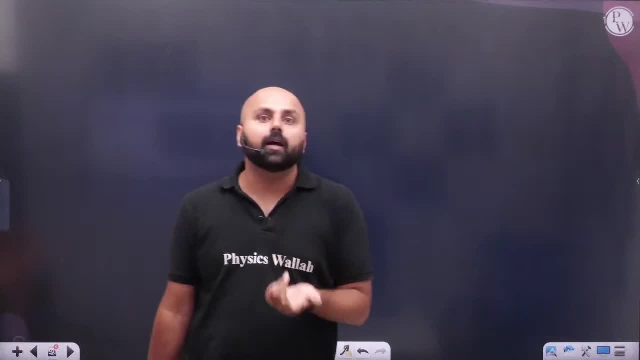 what will happen? Inversely proportional, Because the energy will be inversely proportional. What will be the energy? It will be inversely proportional. Second thing: if someone tells me that, what was the next application of Planck's quantum theory? 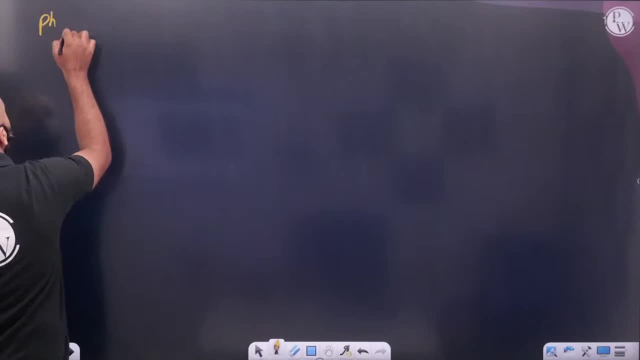 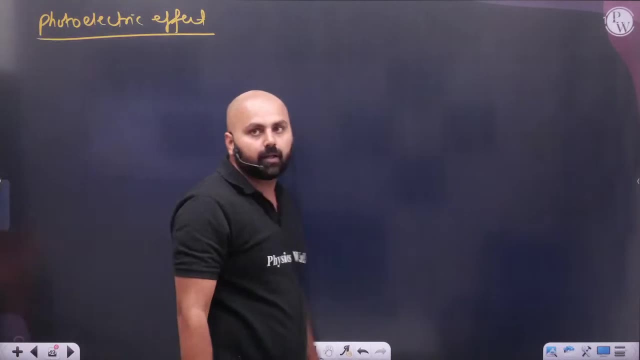 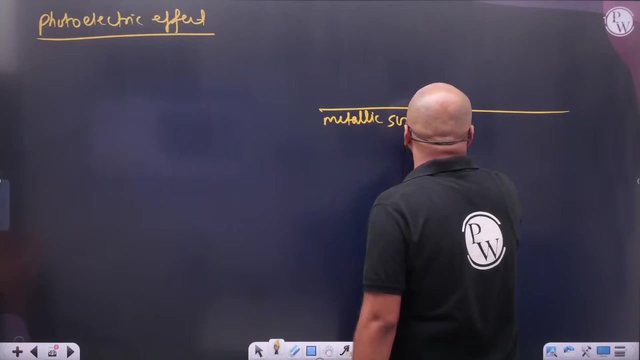 What was the next application? The most important application was in photoelectric effect. In photoelectric effect. Einstein got the Nobel prize for this. only What does photoelectric effect say? That there is a metal, a metallic surface. Remember for whom this is for Photoelectric effect. 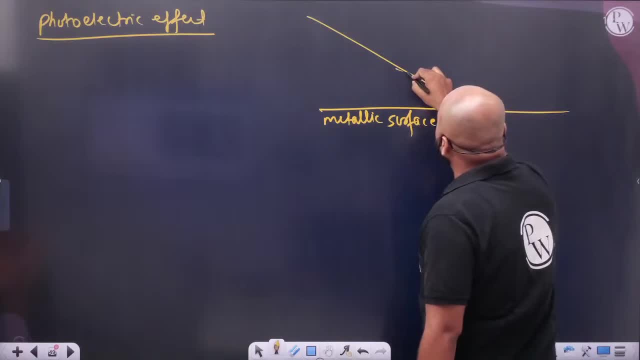 is on the metallic surface. If you have read this chapter in modern physics again and again, all these things are being repeated: If there is a metallic surface. if, from any frequency incident frequency is this: if your incident frequency is this: if your incident. 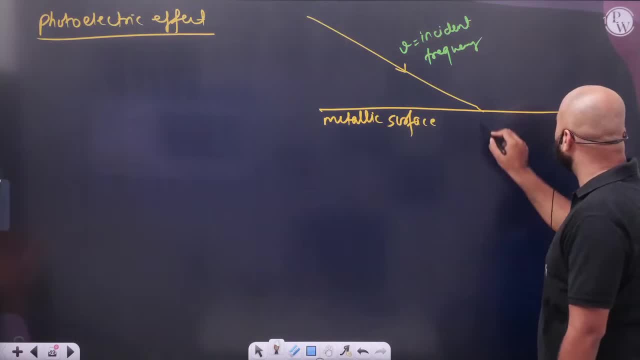 frequency is this, then you do not release electrons in the beginning itself. Where do you give energy for a while In the work function? Where do you give energy for a while In the work function As soon as your energy is released from the work function? 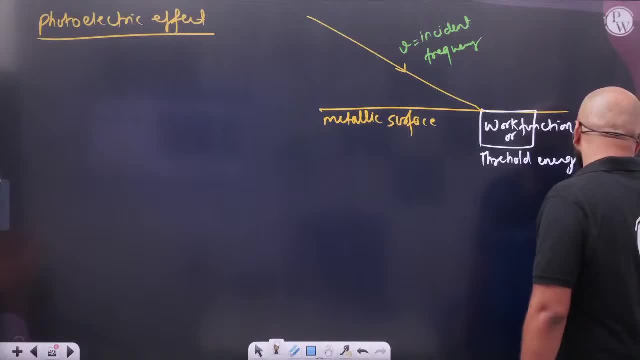 or more than the threshold energy, or more than the threshold energy. what is going to happen here? What happens here? Release of electron will happen. Electron will release. This is what happens. What is electron? It is released, So in photoelectric effect. 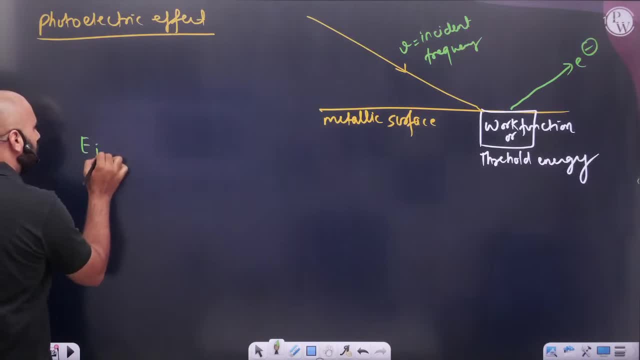 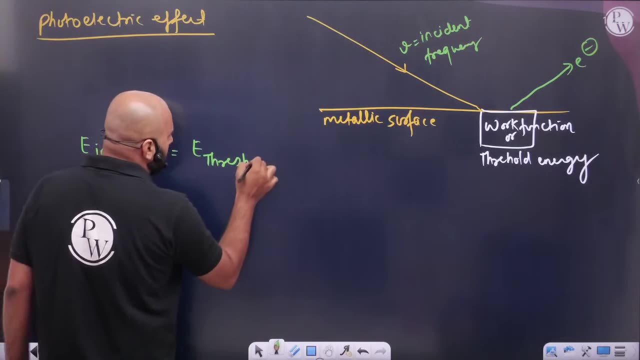 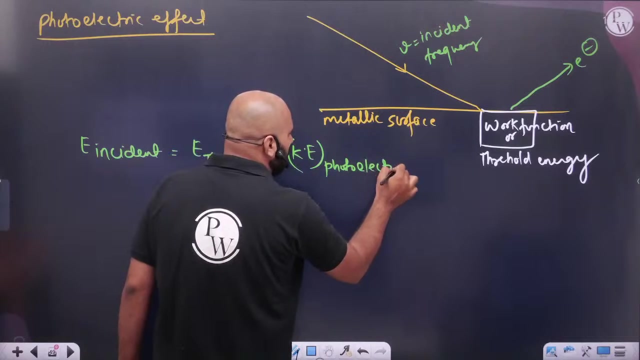 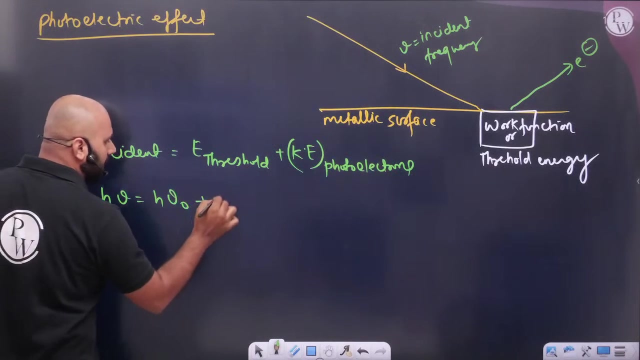 what is the formula? The incident energy will be equal to threshold energy plus kinetic energy of photoelectron. Kinetic energy of photoelectron will be: So, sir, what is the incident energy? h? nu, and that will be h nu naught minus plus kinetic energy. 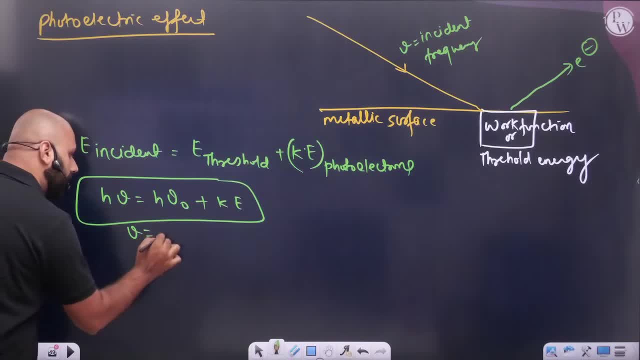 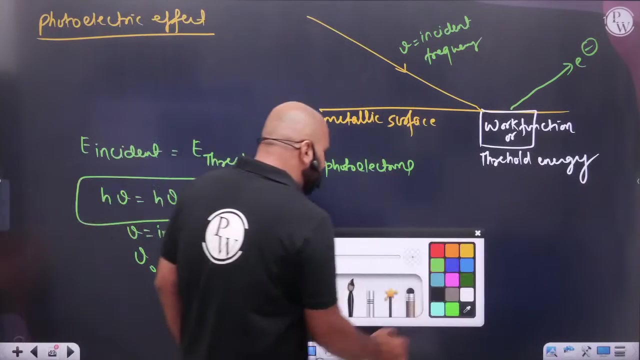 Sir, remember one simple thing: Nu naught What is nu Incident frequency? What is nu Incident frequency And what is nu naught Threshold frequency? What is nu naught, Threshold frequency And threshold frequency? See this: The force of kinetic energy. 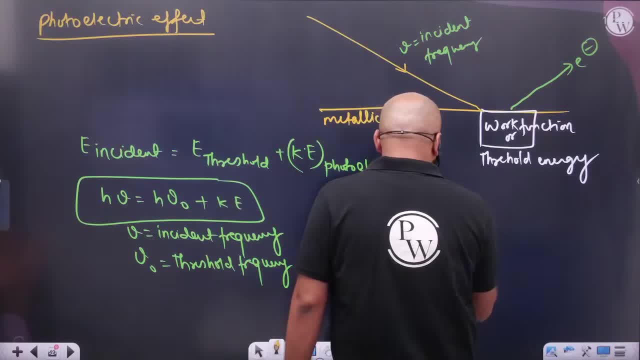 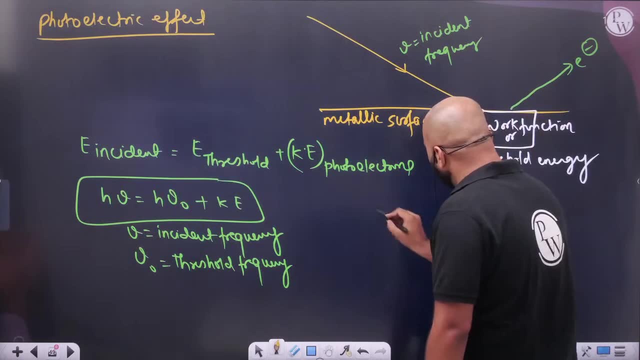 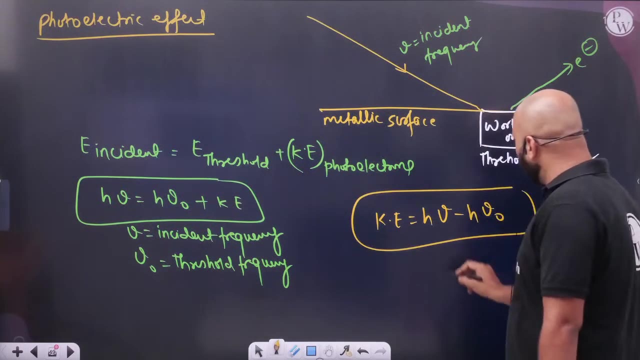 is equal to h nu minus nu naught. If you want to get the formula of kinetic energy, if you want to get the complete kinetic energy, then h nu minus h nu naught. Remember one simple logic: Kinetic energy y is equal to mx. 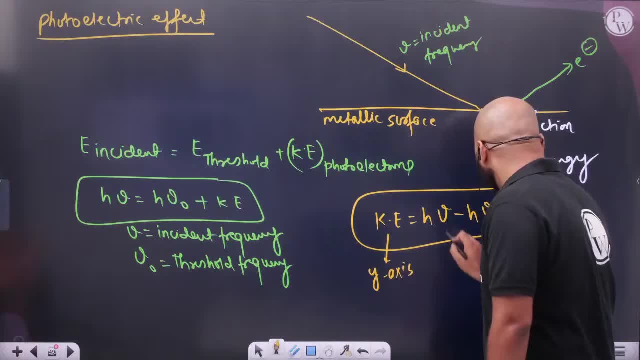 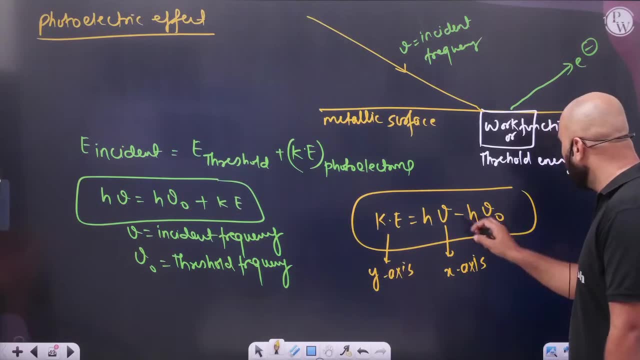 If we take it on y axis. if we take it on y axis, if we take it on x axis, then it will not be directly proportional. If we see the graph, then what is this Threshold? If you make a graph of this? 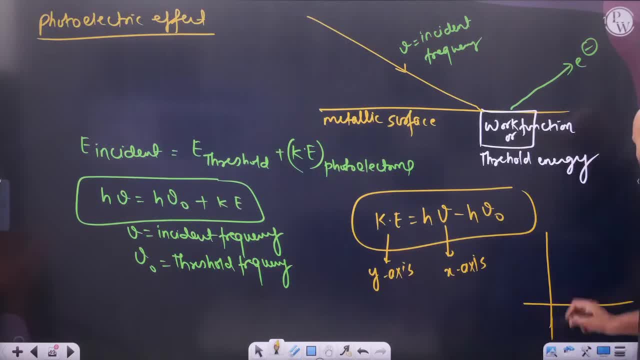 what kind of graph will it be? See this: If you make a graph of kinetic energy and its frequency, then what kind of graph will it be? y is equal to. we have seen the graph of mx plus c. We have seen the graph of mx plus c. 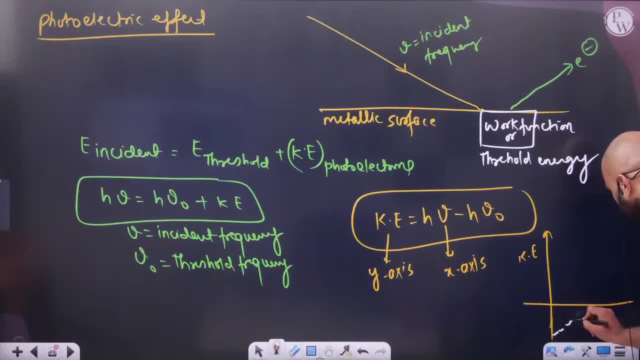 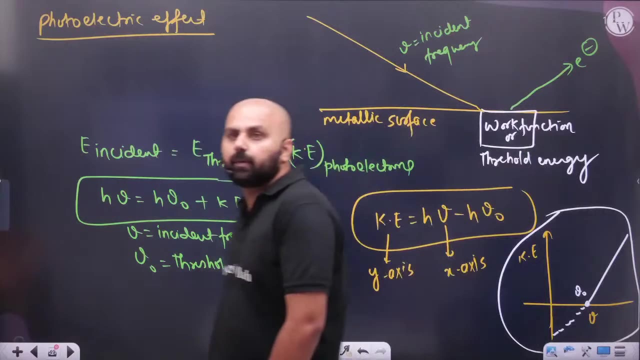 Sir, from here the negative will be negative. We do not have negative kinetic energy, So this will happen And this frequency we have will be equal to nu naught. So remember this graph, The graph of kinetic energy with frequency. You must have done this in. 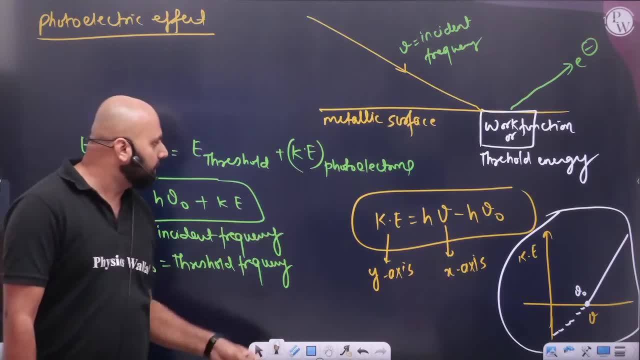 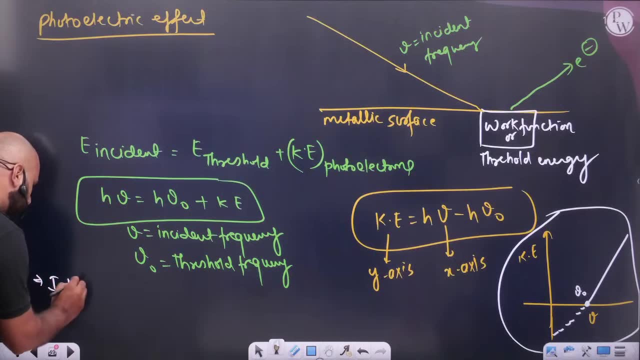 physics also. So see this. The graph of kinetic energy with frequency is like this. One more thing: If you increase the intensity- remember this is also written in physics- If you increase the intensity, then the number of photons increases. If you increase the intensity, 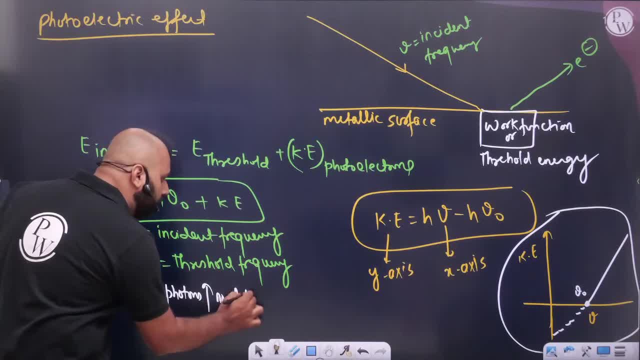 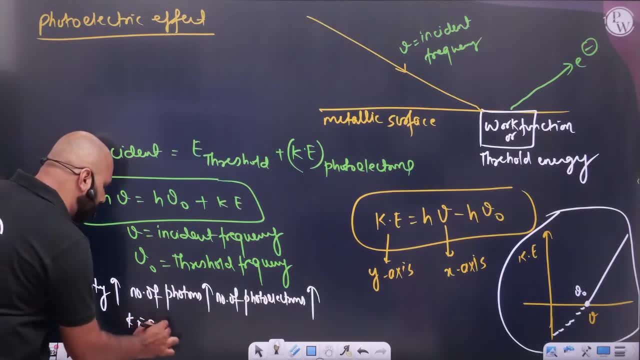 then the number of photons increases. If the number of photons increases, then the number of photo electrons increases. If the number of photo electrons increases, Kinetic energy will be the same. What will be the Biology of kinetic energy? What will be the change? 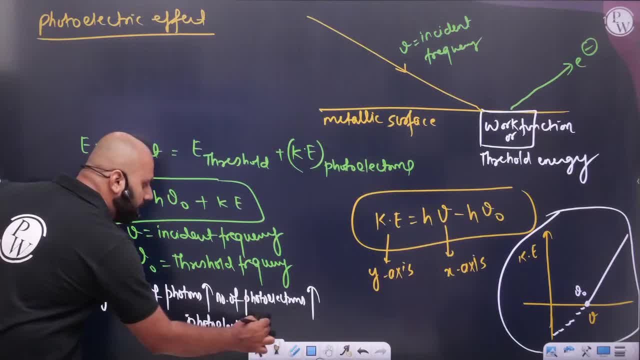 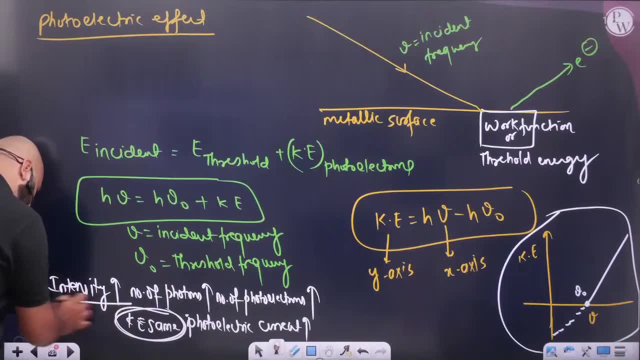 the photoelectric current will be increased. What is photoelectric current? What will be the increase in the photoelectric current? Kinetic energy has nothing to do with intensity. Increase the intensity means the number of photos. If you increase the number of photos, there is no kinetic energy. 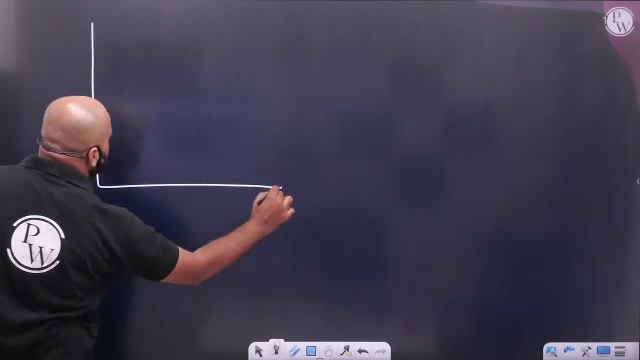 There will be no difference in the kinetic energy. Look at this, Sir. if we talk about intensity, then you will see the graph of intensity and kinetic energy. Sir, you will increase the intensity. What will be the kinetic energy? It will be constant. 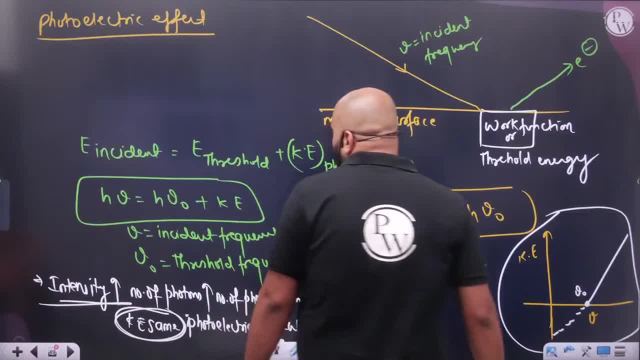 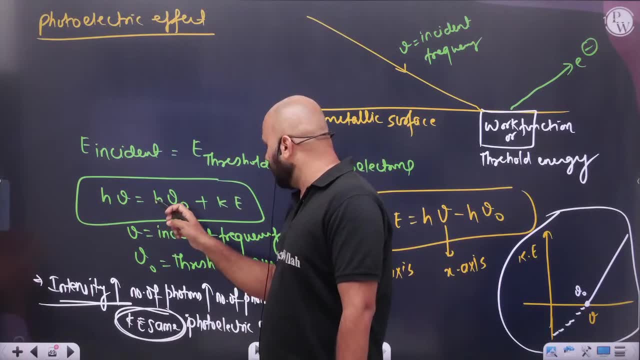 Why? Because the intensity has increased. Sir. the intensity has increased. Do one thing: Multiply these two sides with n. Because the number of photons increased. so this became n times. Obviously, the threshold frequency became n times for everyone. What will be the kinetic energy? 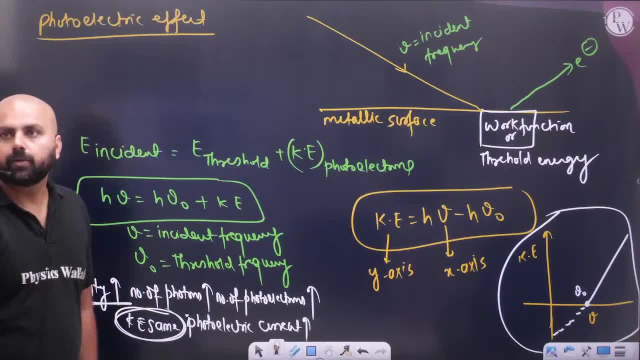 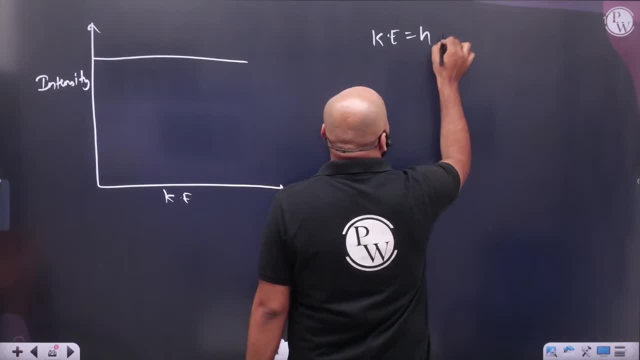 It will become n times. So do it like this: Sure, Come on Now see. u see, in this photoelectric effect kinetic energy which came in the photoelectric effect h no minus h no come. or if you talk about kinetic energy, then when you talk about this, 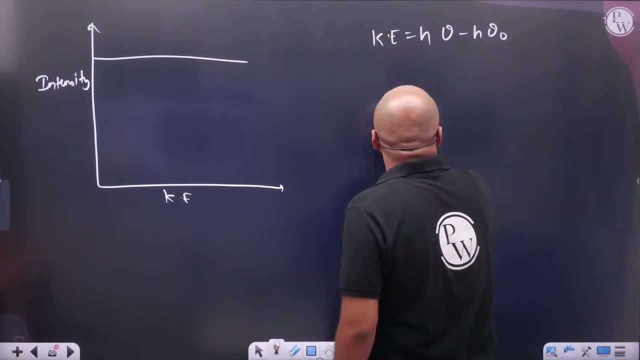 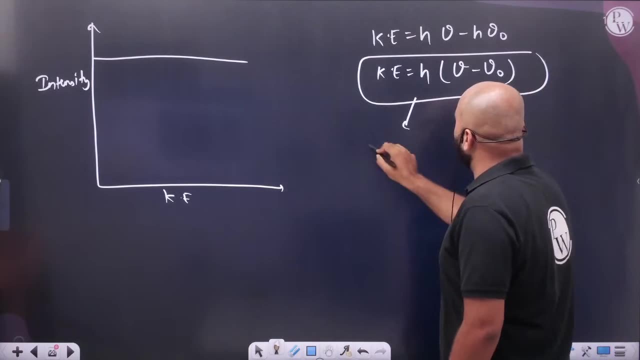 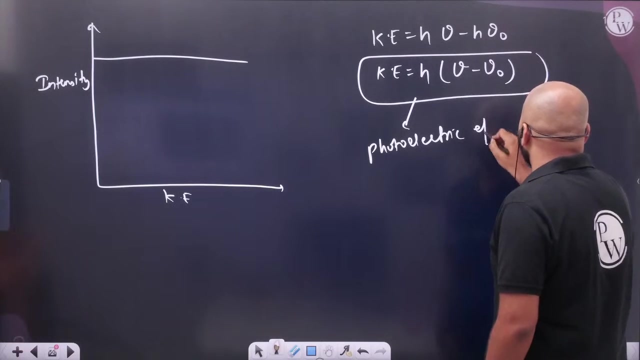 kinetic energy. look at this. Kinetic energy: h, no minus, no, Sir, when is this photoelectric effect possible? When is a photoelectric effect observed? Hmm, When will the photoelectric effect be observed? When will it be observed when it is absorbed? then, for that the story comes that, brother, when new greater than what, 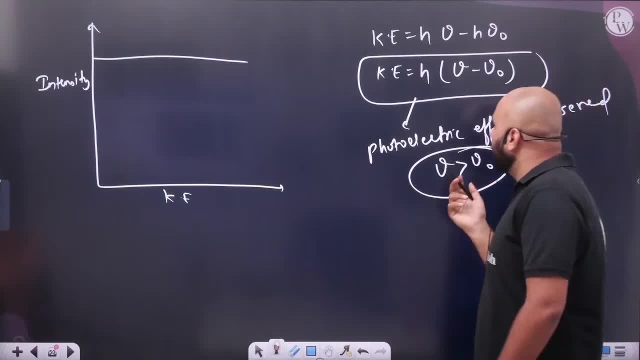 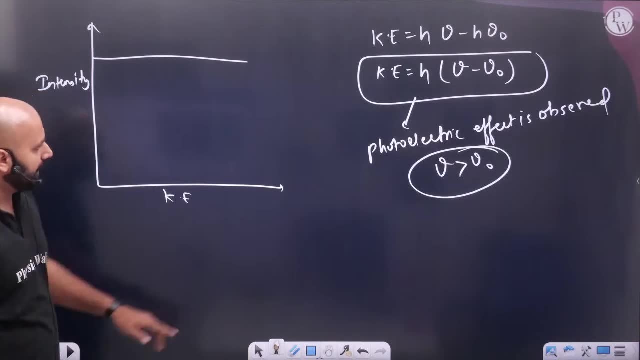 happens new not happens. if otherwise it is equal, then kinetic energy is zero and less than happened, then it is gone. okay, if you increase the intensity in the graph, then what will be the kinetic energy? same. and remember this graph of kinetic energy because 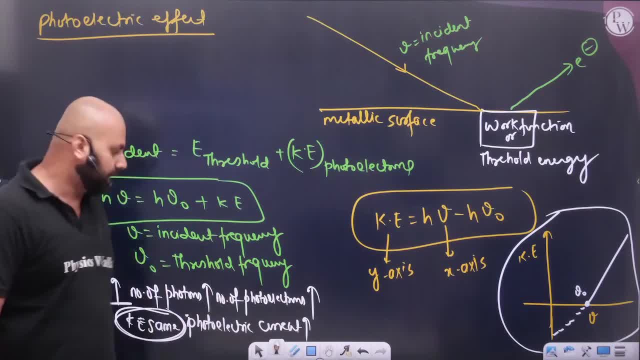 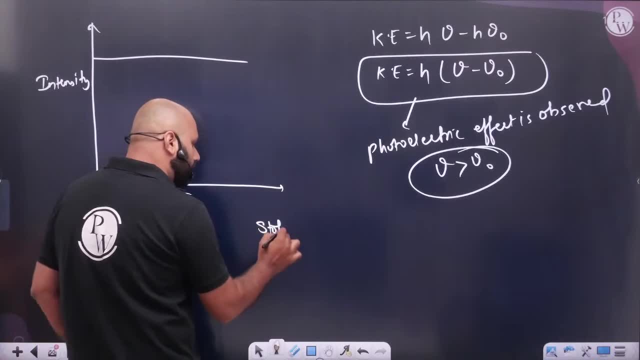 this is a lot of trouble, okay, okay, see this, brother. we have this photoelectric effect. there is nothing else in the photoelectric effect. one word is stopping potential. stopping potential is nothing. stopping potential is nothing. you have a simple stopping potential. 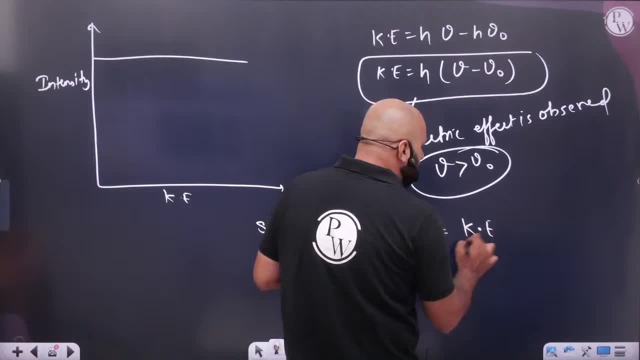 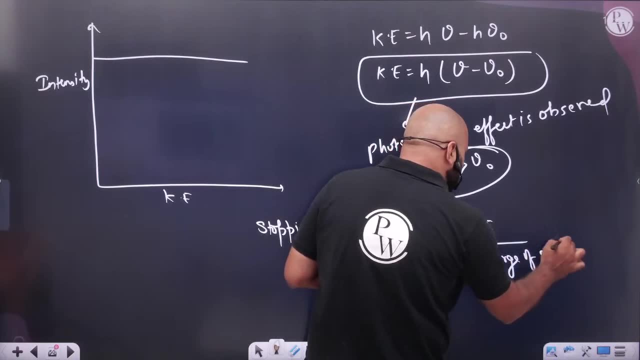 is vs. stopping potential is nothing. how to divide kinetic energy? how to divide kinetic energy from charge of electrons? how to divide kinetic energy from charge of electrons, sir, stopping potential, if you have to remove it quickly, then if kinetic energy is in joules, 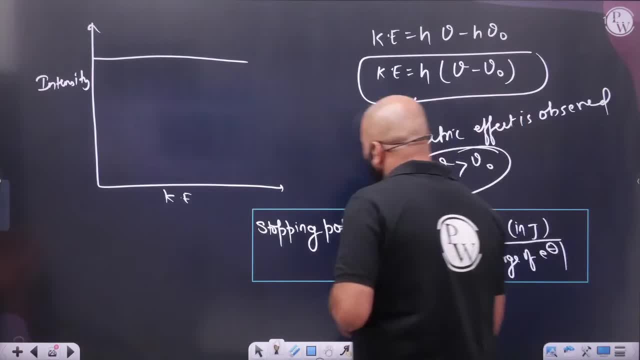 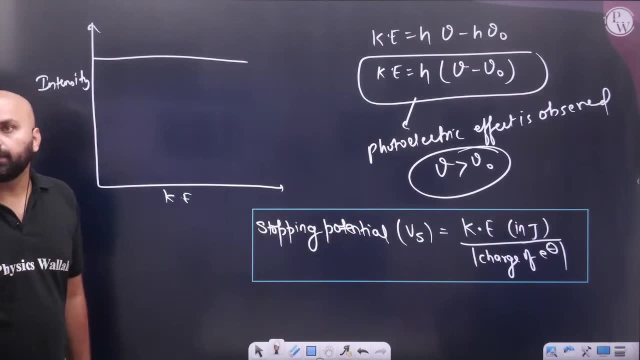 if kinetic energy is in joules. if kinetic energy is in joules, then stopping potential. What will you divide it with This? Ok, This is kinetic energy. Now you will get this question, Sir, tell me this Number of electrons. 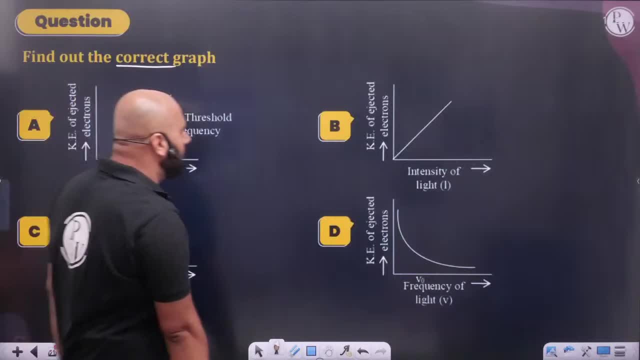 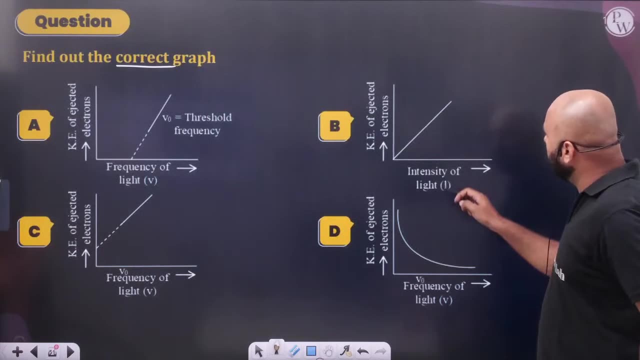 Frequency. Which graph is the correct graph? Which is the correct graph? So how will you find the correct graph? Kinetic energy does not depend on the threshold frequency. It does not depend on the intensity of light. Kinetic energy does not work with the frequency of light. 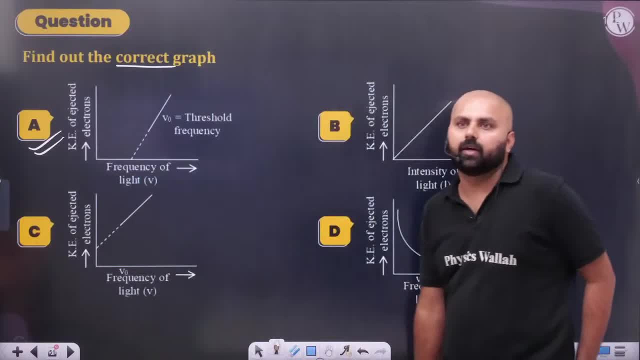 Which graph will be the correct graph? First one is the correct graph. First one is the correct graph. What will be the first one? It's going to be the correct graph. Ok, What is the first one? It will be the correct graph. 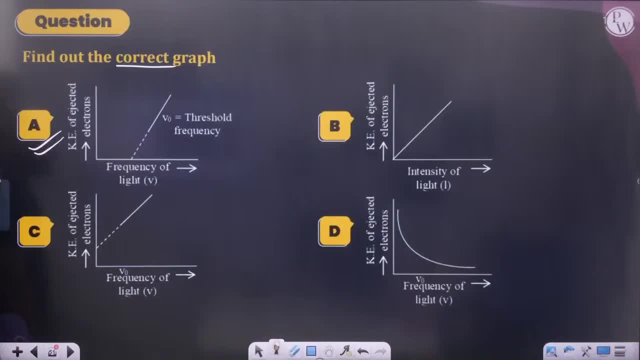 Why will kinetic energy work with the frequency? Why it will ok. Inversely, motion only will not be ok, Obviously. What will happen? How will the kinetic rendered work with the frequency? Frequency is here only. It will work only above this. 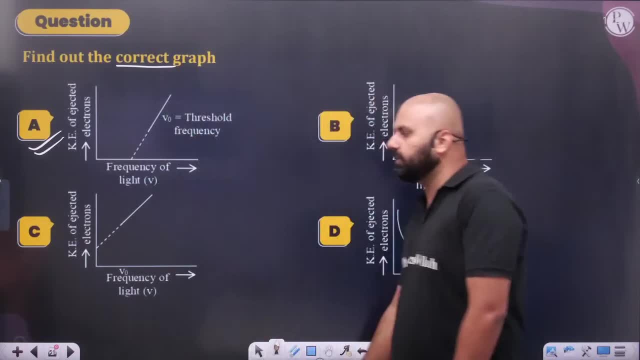 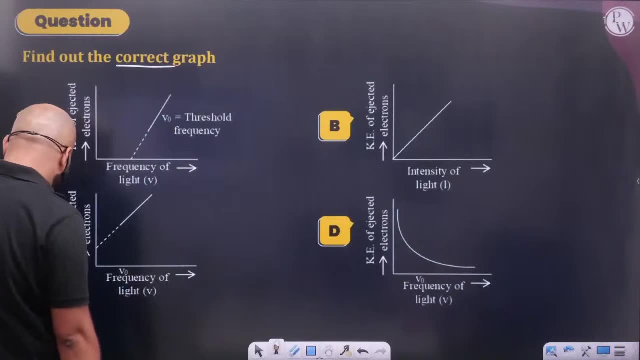 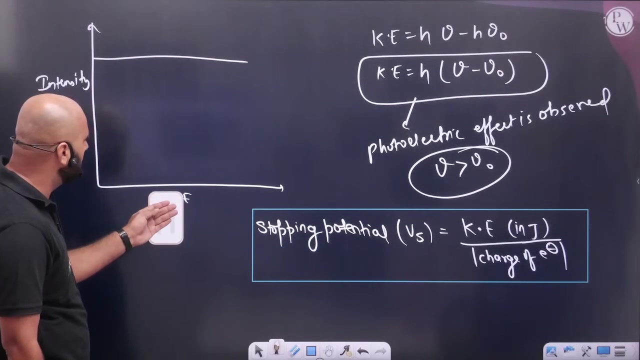 Cross the threshold frequency, only then it will go up. It will pass the threshold frequency, only then it will go up. Ok, Cross the threshold frequency, only then it will go up. Ok will pass. then only we will have ok here. it is fine to understand the emotions. this will be kinetic energy and this will be intensity. 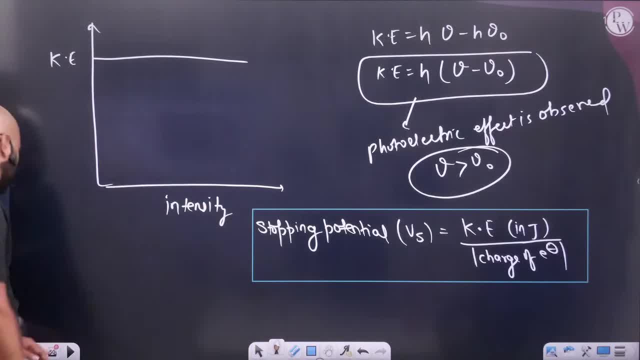 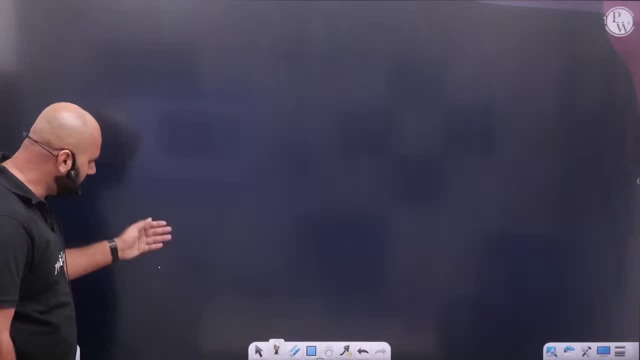 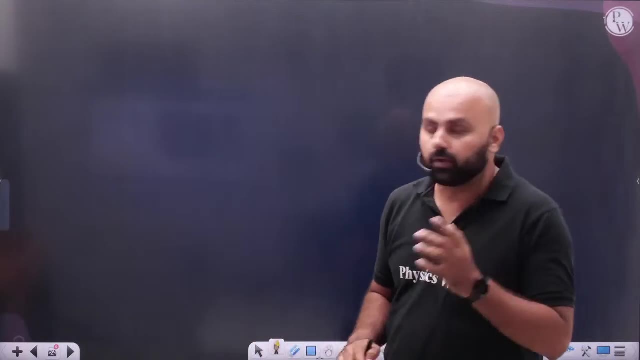 See, the intensity will increase. kinetic energy will remain the same: See the next question whenever you get a question. so now see, after photoelectric effect, the major thing that comes to me in atomic structure, Einstein's Planck's quantum theory- the major part that comes to photoelectric effect is Bohr's theory, Bohr's model. 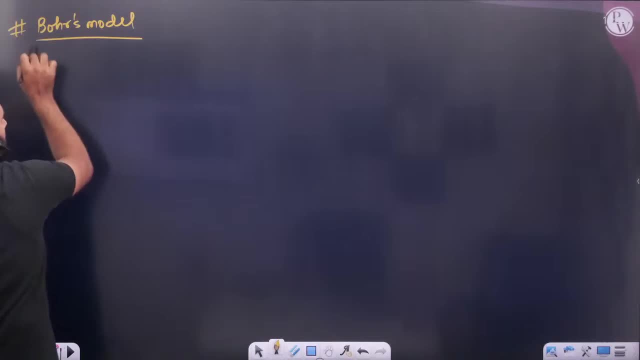 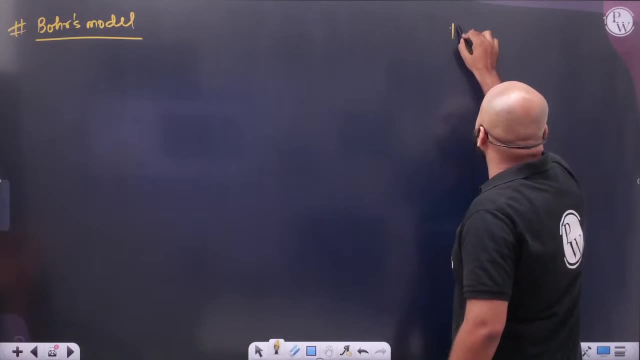 Sir, you will talk about Bohr's model now. don't ask me about Thomson model and Rutherford model. you have already done Thomson model and Rutherford model in physics, Even apart from Thomson and Rutherford in Thomson model and Rutherford model. 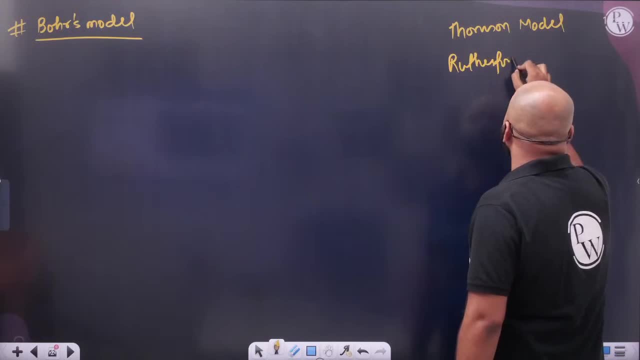 when you do Rutherford model in physics, then you get to know that in physics you also get to know the distance of closest approach. What is the distance of closest approach? All these things have happened in physics, so there is no point in wasting time on it. 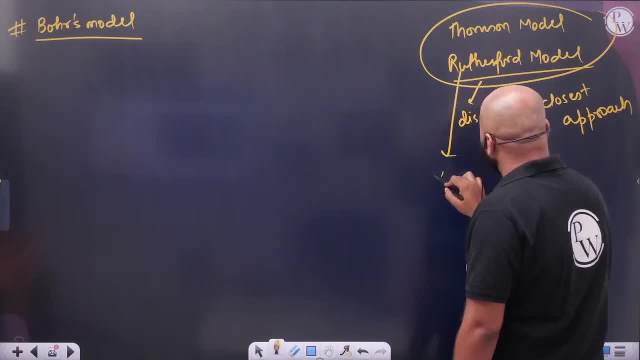 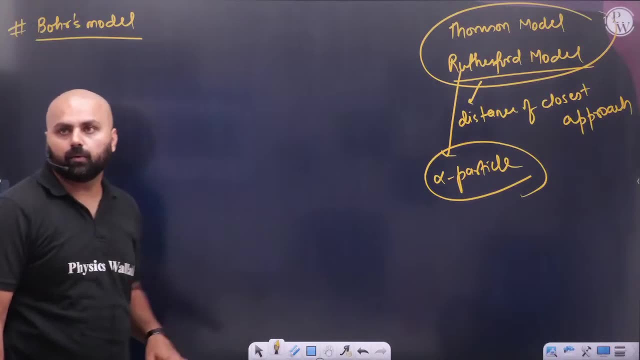 What is the distance of closest approach? What happened in Rutherford Alpha particle scattering experiment happened Now. I will repeat the same thing here. there is no point. See what is useful now. see what is useful. What is useful: Sir Bohr's model. 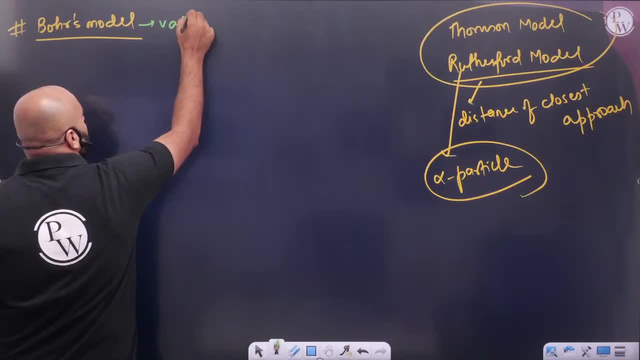 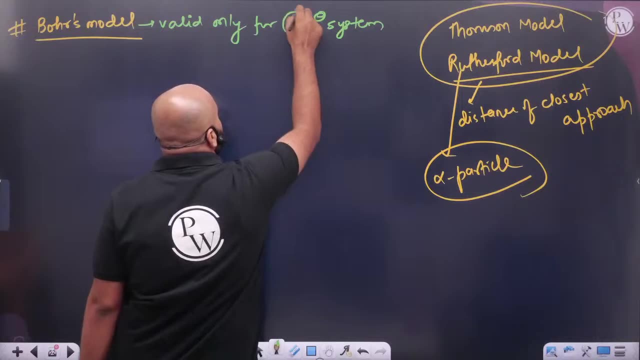 What is in Bohr's model. It is valid only for, valid only for one electron system, One electron system. It is valid for one electron system means it is valid for hydrogen. it is valid for helium plus, it is valid for lithium plus 2.. 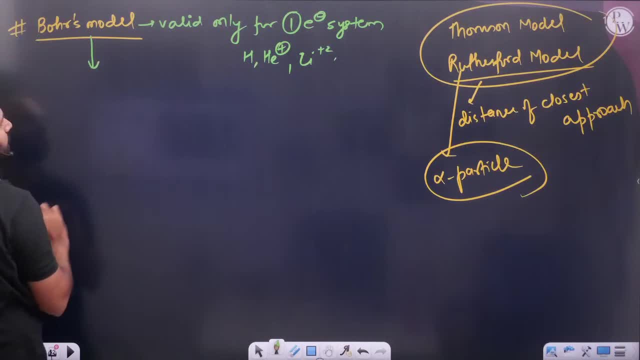 It is valid for all these. What happens is, according to this: there were some postulates in some postulates. the first postulate was that, Sir, the electrostatic force of attraction, the first postulate, the electrostatic force of attraction between two people. 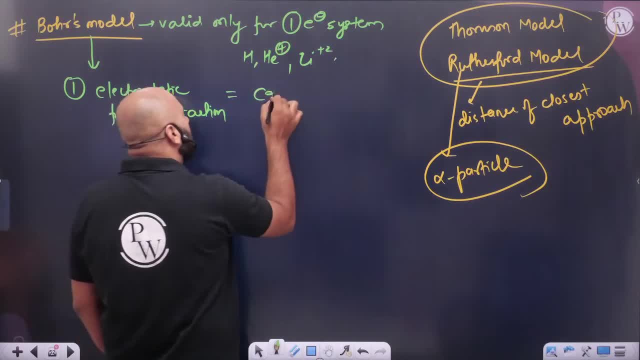 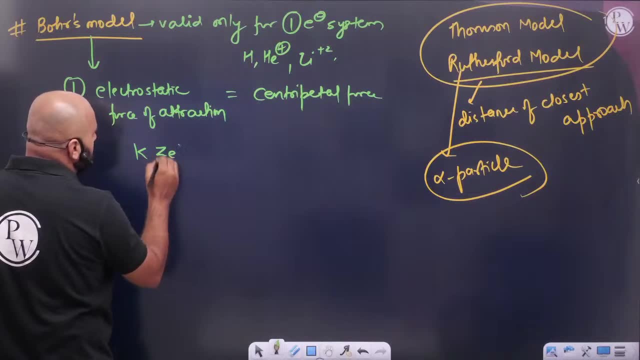 the electrostatic force of attraction will be equal to whom? Equal to centrifugal or centripetal force? With us, Sir, you do not go above physics. you see, this simple kz into e upon r square is nothing. centripetal force mv square by r. 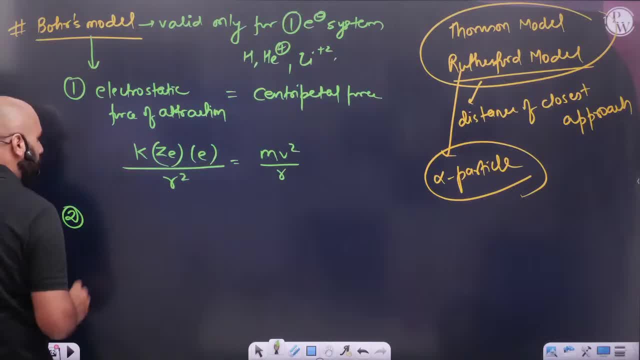 What was the second postulate, which talks about the major postulate. So in Bohr's orbit, what was said in Bohr's model? If we talk about Bohr's model, the second postulate was that the angular momentum 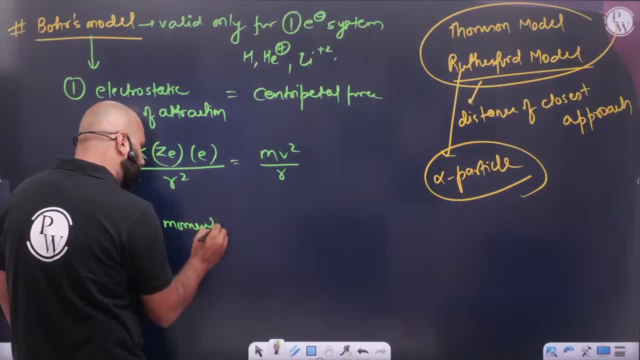 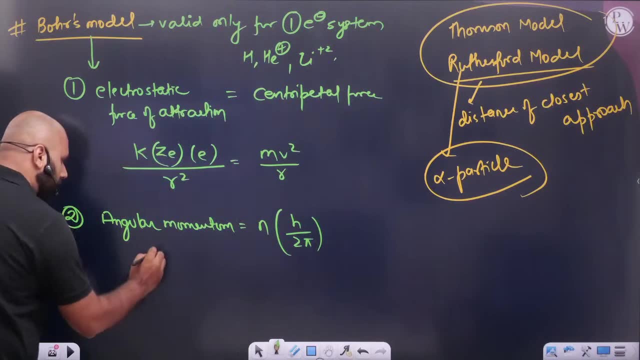 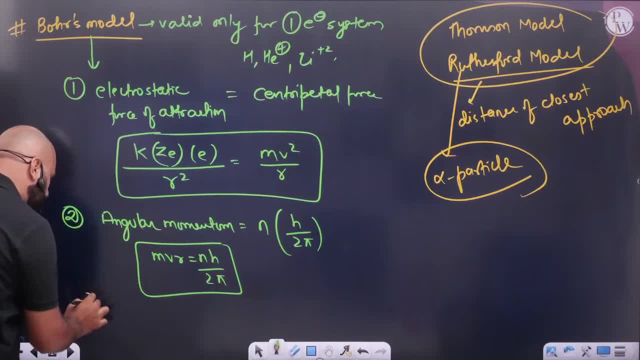 We take these two major mathematical expressions. Apart from this, you will see they said that when will the electron lose or gain energy? When will the electron lose or gain energy? What is it going to do When they make a transition? 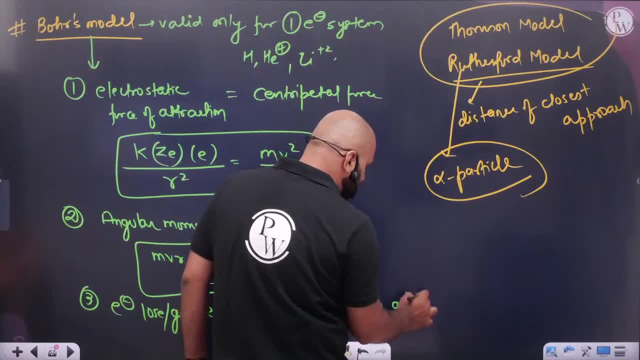 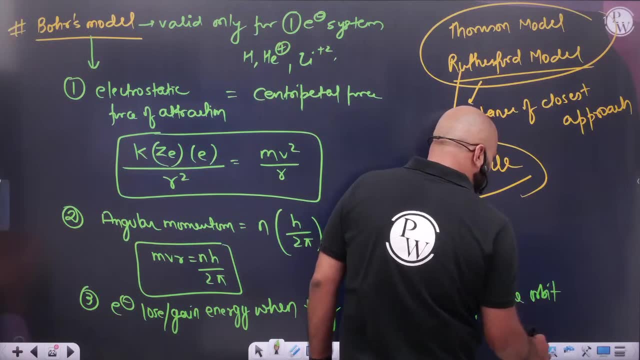 What will it do? They are making a transition, They are going somewhere, Transition From one orbit to other, one orbit to other orbit. The electron will only lose or gain energy when it goes from one orbit to another orbit. 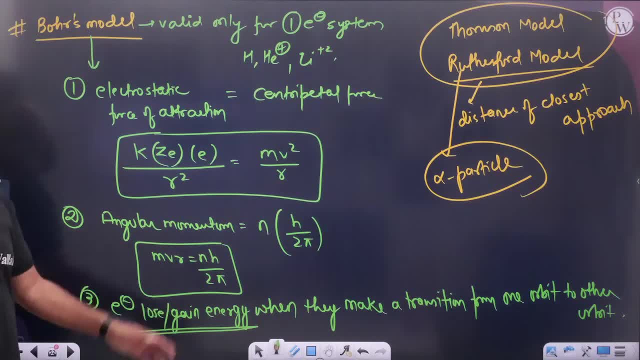 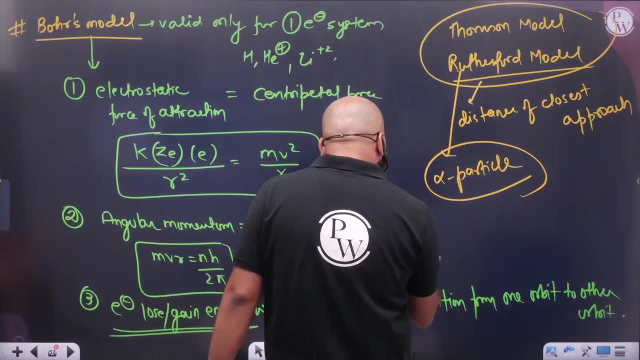 It may gain energy, it may lose energy. So keep this in mind. mvr is equal to nh upon 2 pi. mvr is equal to nh upon 2 pi. h by 2 pi. we write h by 2 pi somewhere. 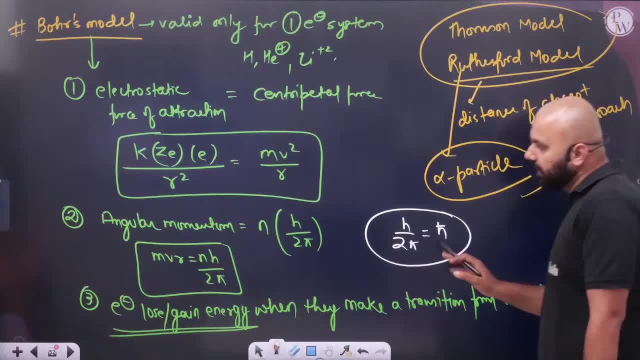 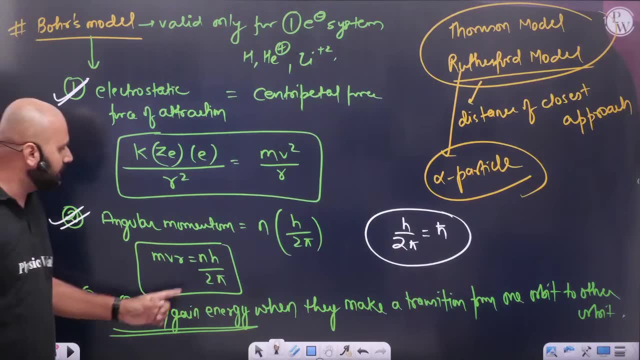 h bar, also h by 2 pi. we write h bar somewhere, h bar also. These are basic postulates, basic important postulates, basic important postulates that when does energy lose or gain energy? When does it transition? What will transition mean? 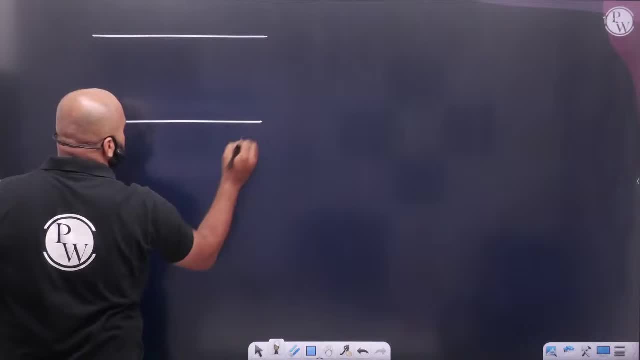 What will transition mean If you are at a lower energy level? If you are at a lower energy level, if your orbit is fixed, if you are at a lower energy level and if you are at a higher energy level, then when you jump from top to bottom, 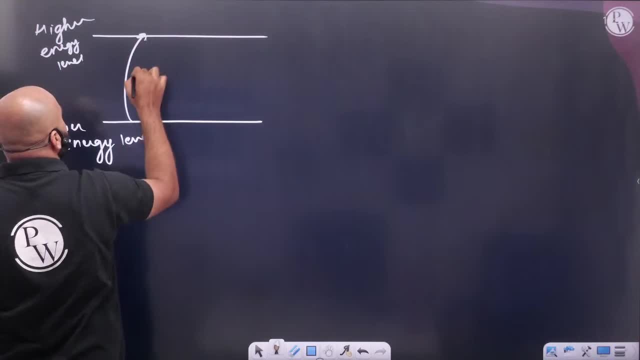 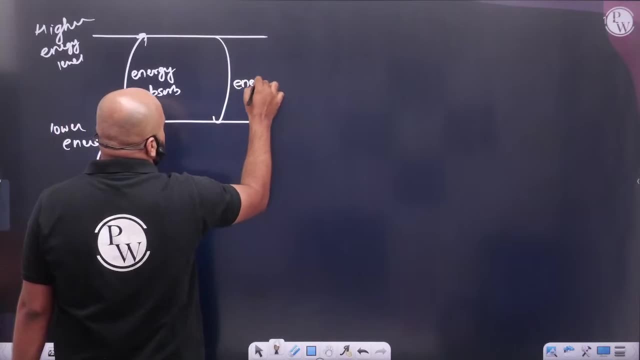 higher energy level. if you go from here to here, then what will you do? You will absorb the energy. What will you do? You will absorb the energy. And if you come from here to here, then what will you do? You will release the energy. 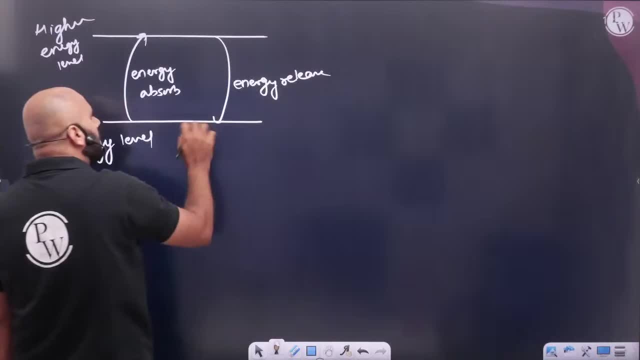 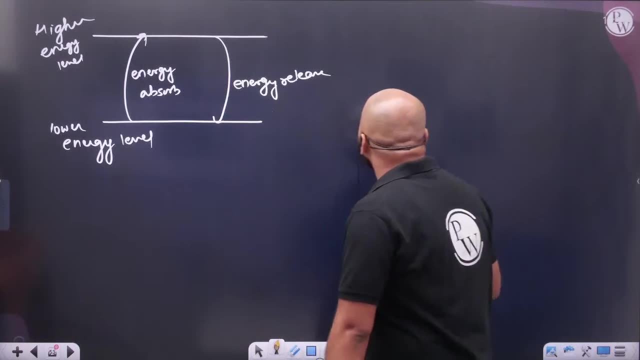 But if you are in the same orbit, if you are here, then here the energy will neither lose nor gain. So the drawback of Rutherford is closed here. If you are here, then your energy will not lose or gain. Then who said 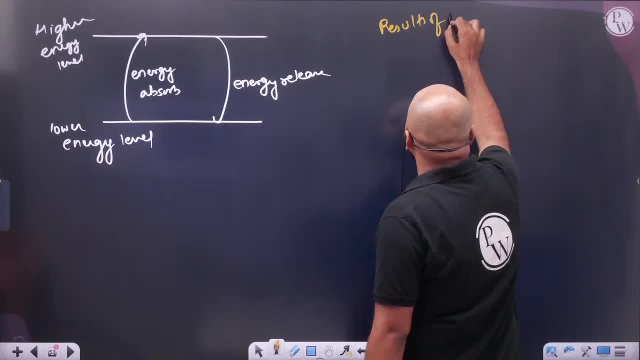 Sir, tell me the result, Or do you have results of Bohr's calculation? Let's see the results of Bohr's calculation. Bohr's calculation, and what results did he get. So what is the result? Radius of nth orbit. 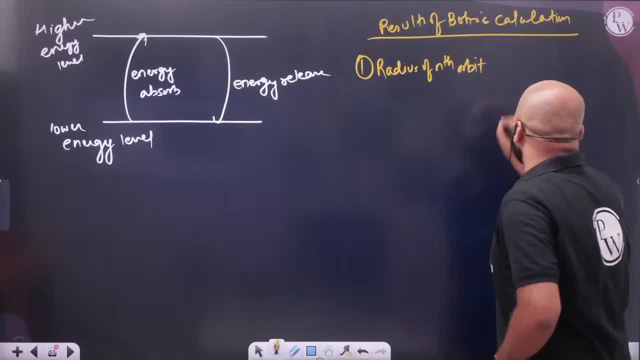 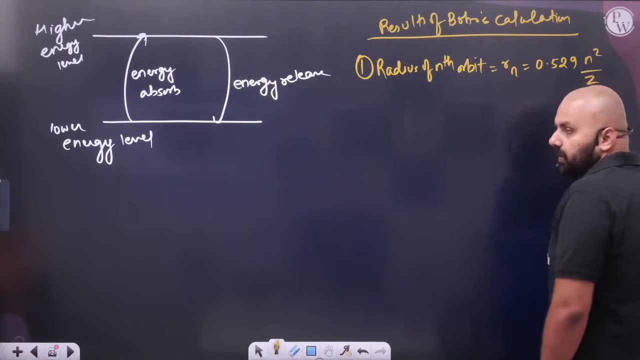 in any orbit. if you want to find the radius of nth orbit, then Rn is nothing: 0.529 n square by z. 0.529 n square by z. What will happen, Sir? what will be the radius of nth orbit? 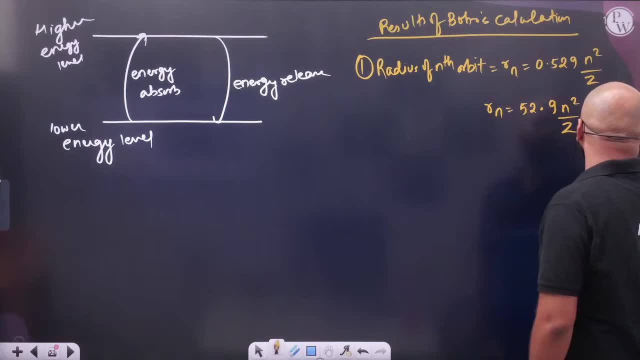 52.9 n square by z Picometer. And what is this Angstrom? So, sir, the first and the most basic thing, what did he find? The formula of radius? Before this Thomson and Rutherford, what were they doing? 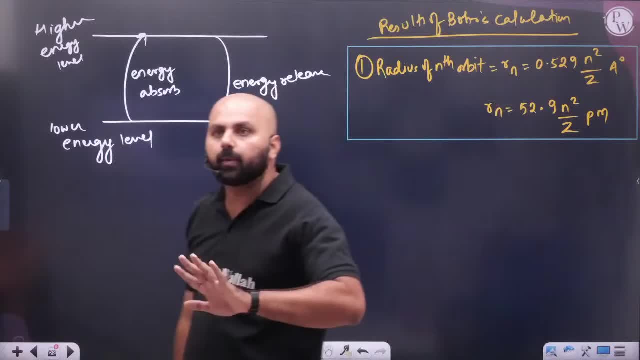 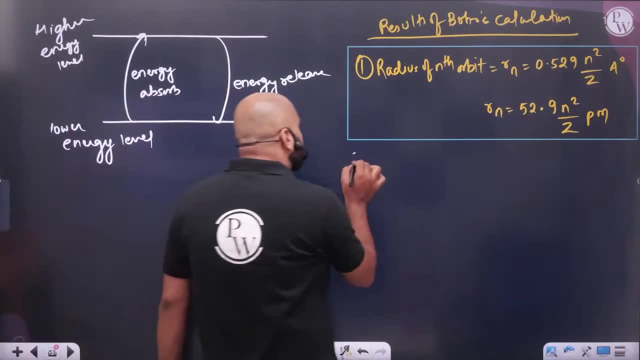 They were simply telling that this is like this. this is like this. We don't have any problem here. Okay, With us. see this radius of nth orbit. this came Then. who said, Sir, velocity of nth orbit? velocity of nth orbit? 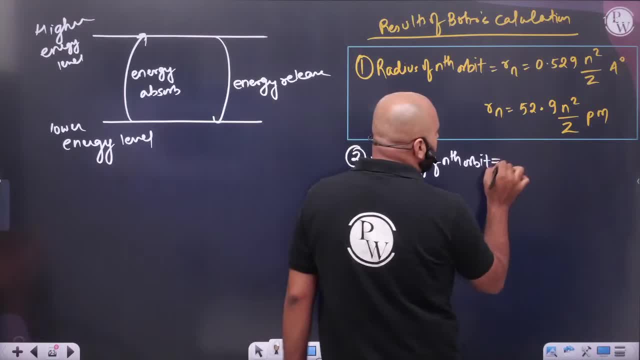 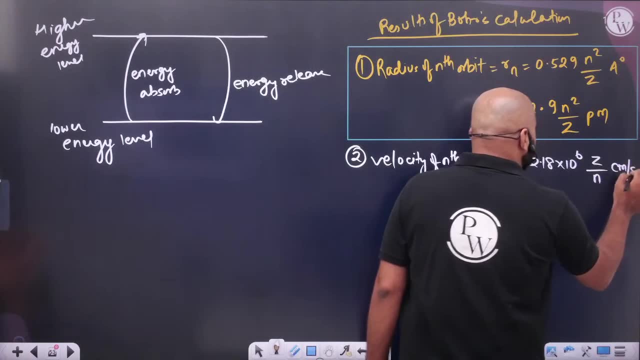 if you take it out and see, then velocity of nth orbit. if you see Vn, then what is Vn? 2.18, power of 10,, 6, z by n centimeter per second, Or if I talk. 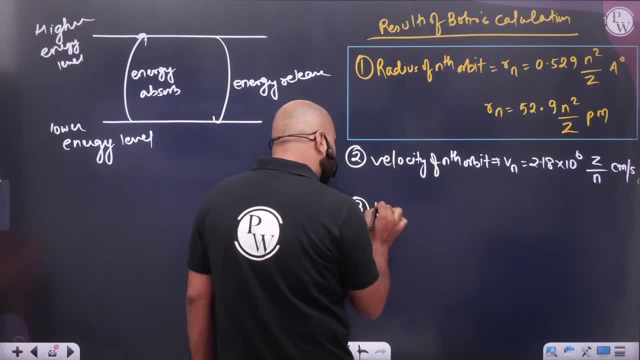 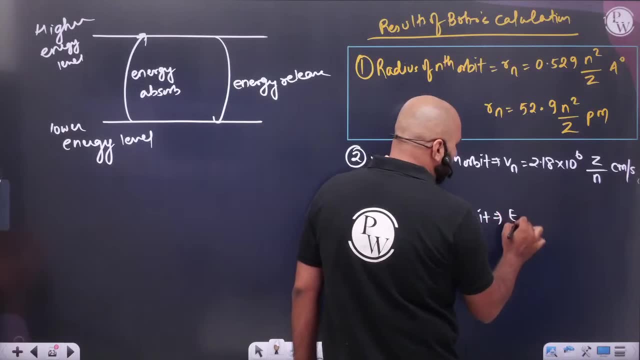 after this third one, energy of nth orbit is talked about. Energy of nth orbit is talked about. So how much energy of nth orbit will come? That will be En is nothing. What will happen Minus 13.6,? 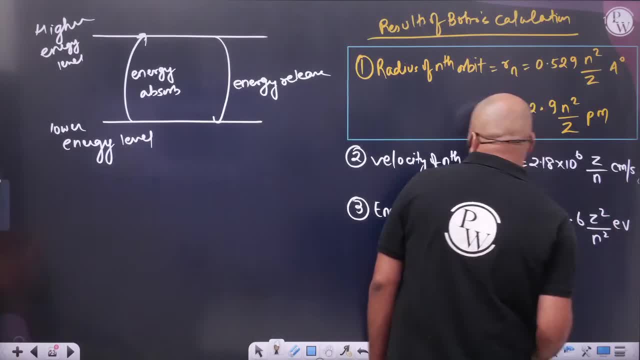 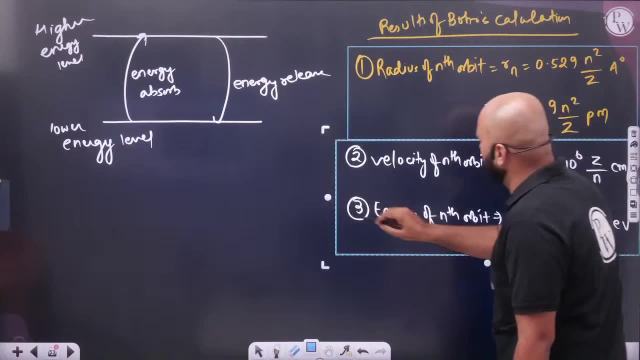 z square by n square electron volt. So I have these two small small formulas which I have derived, which I have derived from where, From me, from there, Which is Bohr's model. This formula came from Bohr's model. 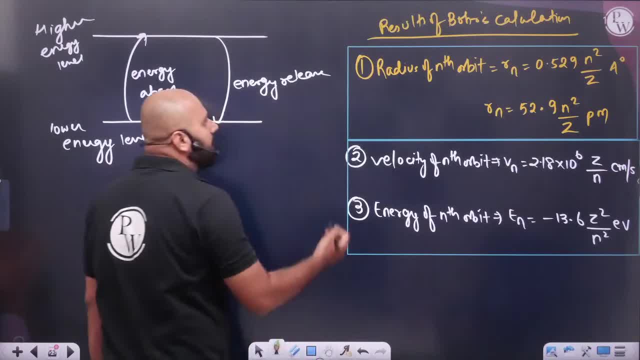 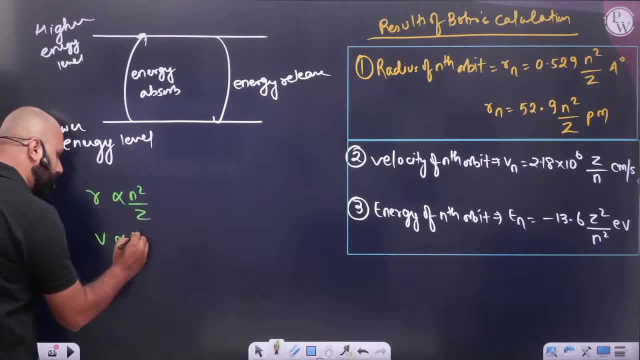 I don't have to remember all the things with this. Okay, if you remember the formula, then it's a good thing. No, you at least remember this much: that n square by z radius, n square by z velocity, z by n. 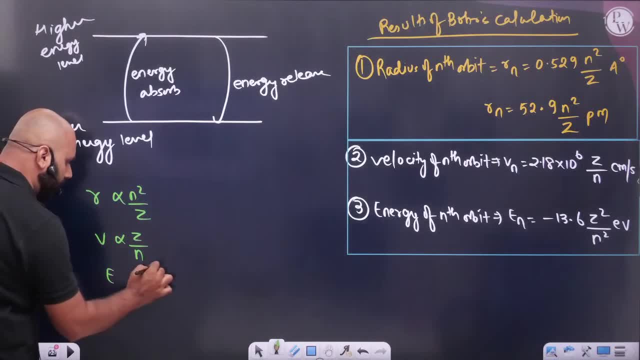 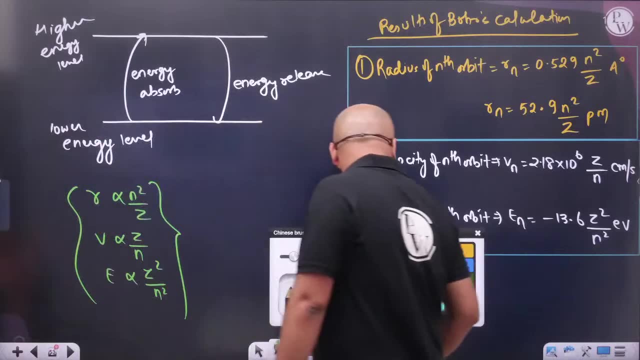 directly proportional and the energy that is there, that will be directly proportional to what z square by n square. So radius will depend on this, velocity will depend on this, energy will depend on this. Keep doing Radius, velocity, energy. 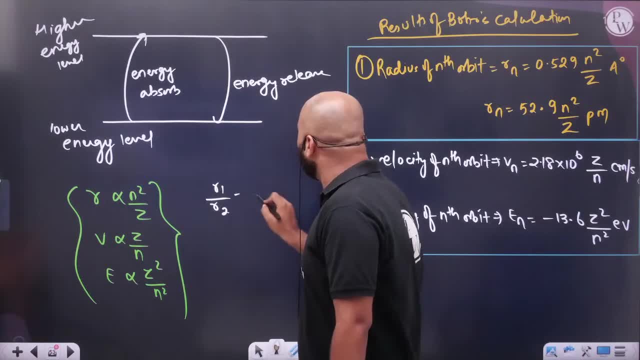 keep taking it out like this. After that you will see: remember n 1 square by z 1, you can take it out quickly by doing this. according to me, There is no need to take out the whole value If you want. 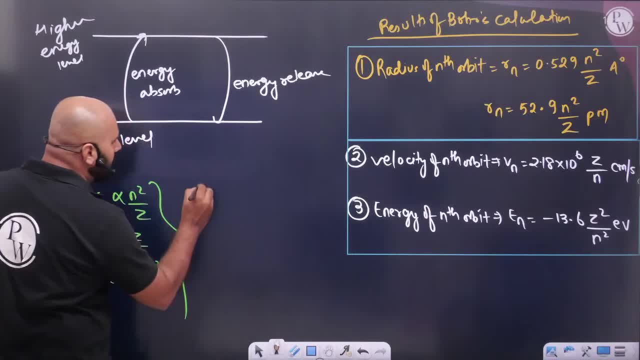 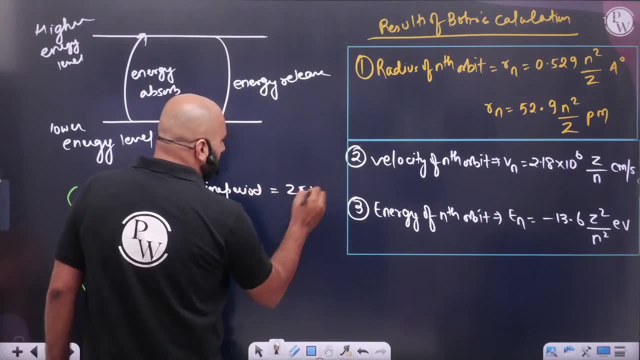 you can take it out like this. Here two more things come. One is time period. What will be time period, Sir? how will time period be taken out? So time period: 2 pi r upon v. So time period will be directly proportional to r by v. 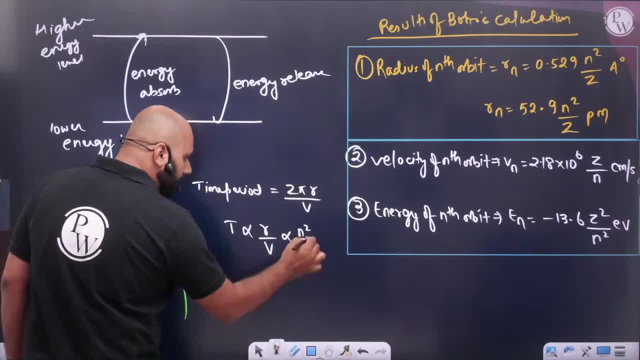 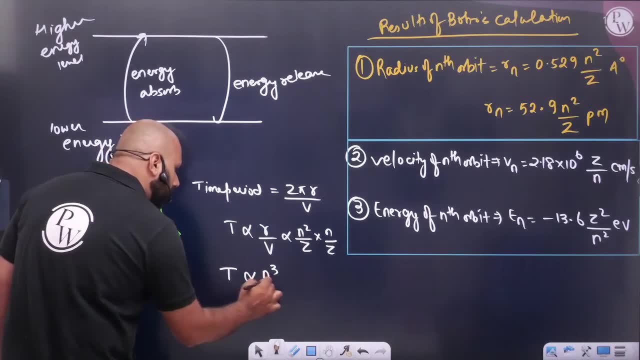 Whose r is directly proportional to n square by z, Whose velocity is directly proportional to z by n. So, sir, time period will be directly proportional to n cube by z square. So if you want to remember this formula, 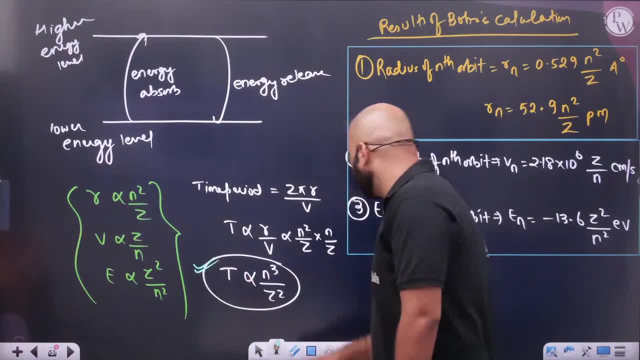 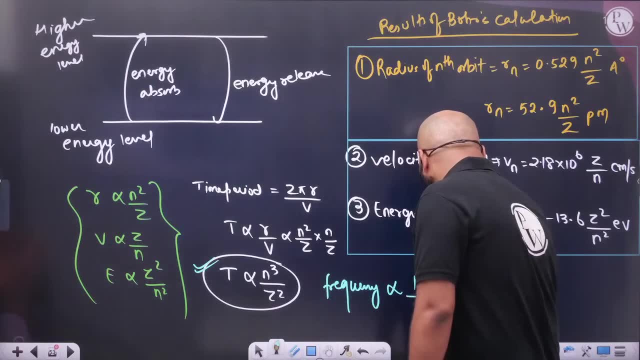 then remember it, Otherwise you can also derive it. This will be the formula of time period. If someone asks about the frequency, if someone asks about the frequency in nth orbit, then what is the frequency? 1 upon time period And on which frequency will it depend? 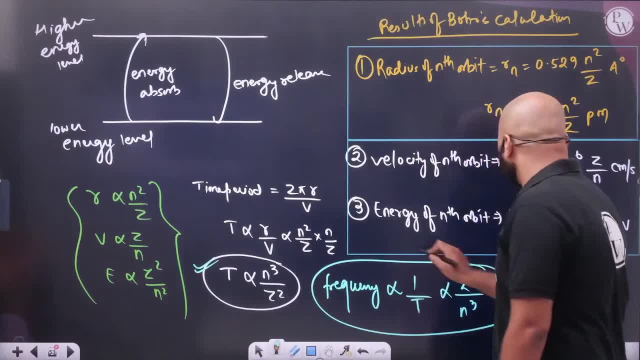 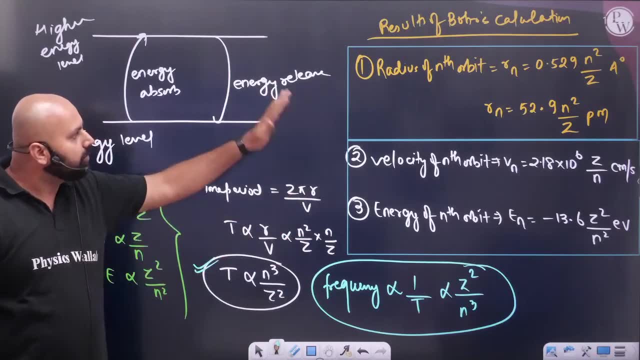 z square by n cube. On which frequency will it depend? z square by n cube. Okay, so do these small formulas Now. you don't have to derive it by sitting. If you want, then do it slowly Whenever you give the question of Bohr's model. 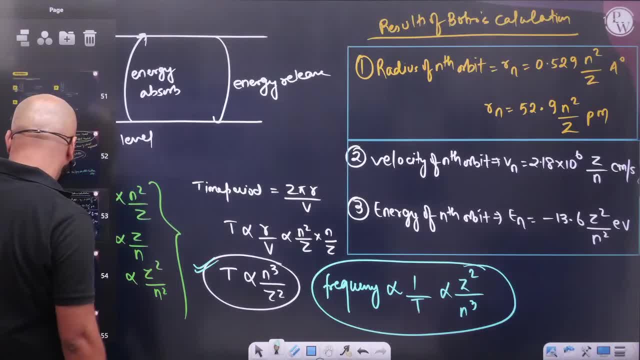 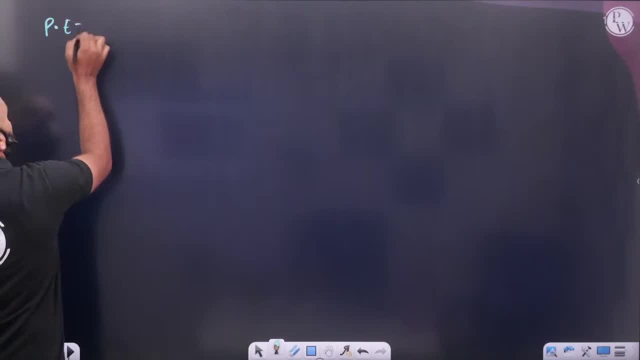 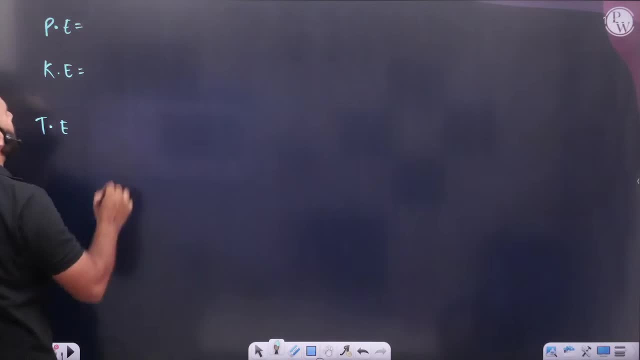 Potential energy, kinetic energy and total energy. What will be the potential energy? k z square by r minus. Kinetic energy will be 1 by 2 k z square upon r. Total energy will be minus k z e square upon 2r. 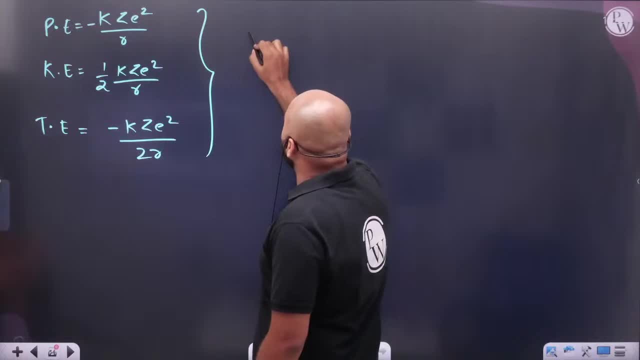 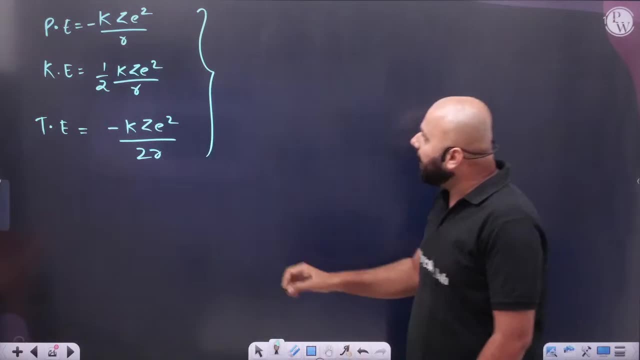 So the relation between them can also be asked, Sir, the relation between potential energy and total energy, The relation between them. You will remember this statement of physics: There is plus z on the nucleus. How much is outside? There is minus e. 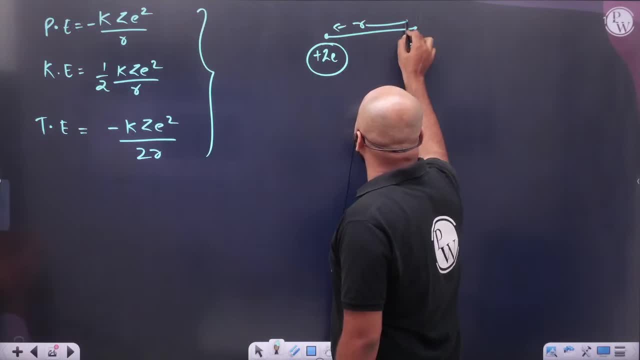 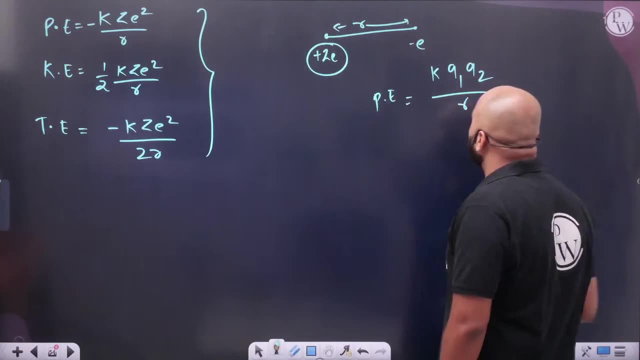 So if there is r distance between them? If there is r distance, then what is the potential energy? What is the potential energy k, q1, q2 by r? If we take out the potential energy in physics, then what will be its formula? 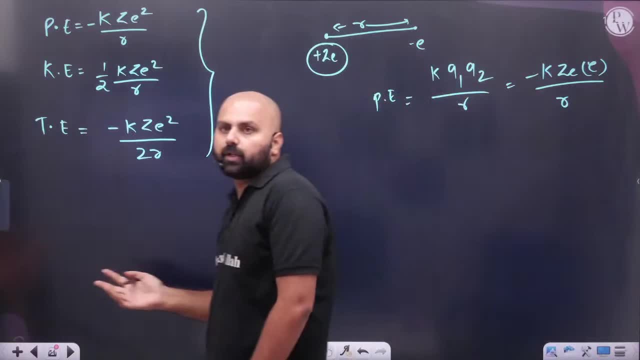 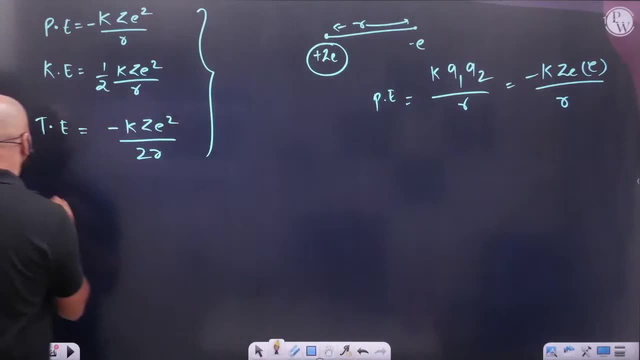 We will get r. So take out the potential energy, total energy, kinetic energy between them. After that, if we talk about Bohr's model, then in Bohr's model two more things are said. What else is said in Bohr's model? 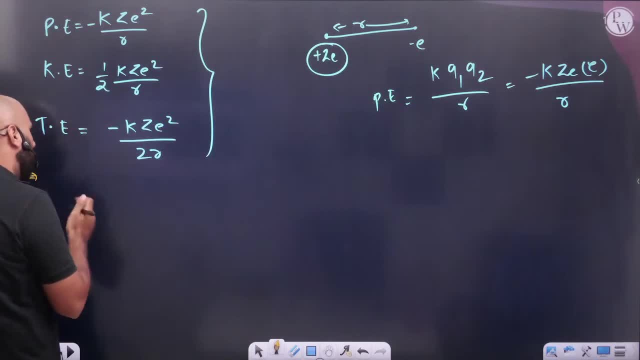 Sir, potential energy, total energy, kinetic energy. If you are simple in this, the orbit of each energy gets fixed. If you want the orbit of energy, then first do a question. Look above it. These are the formulas in front of everyone. 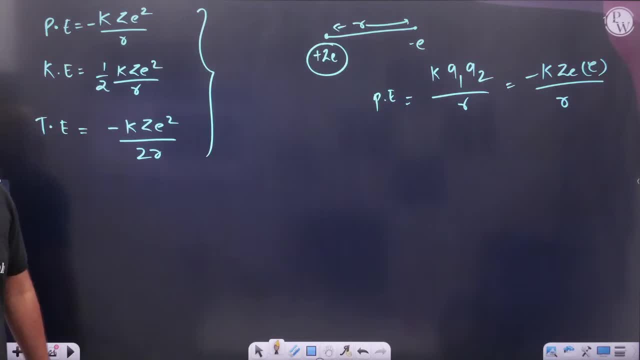 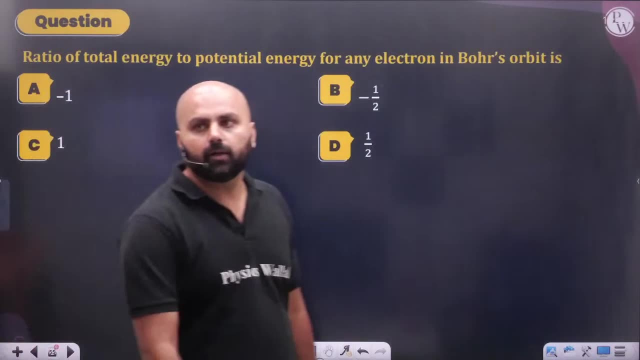 These are the formulas in front of everyone. Now, do a work and see. Do a work and see. Ask this question, Tell this question. Tell this question. What will happen? Tell this question: What will happen with you? A question is asked. 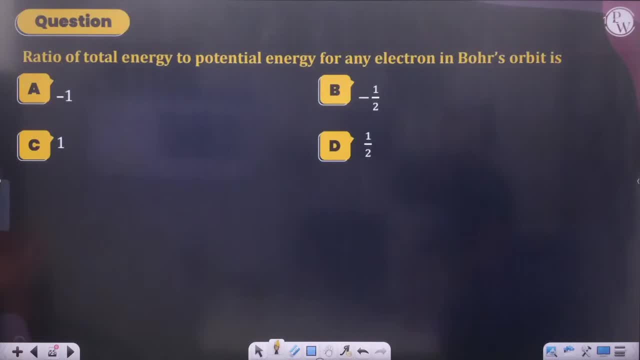 What will be the ratio of total energy and potential energy? So what will be the potential energy Minus k z e square by r? The formula of total energy was written Minus k z e square upon 2r, So it will not be minus, minus, minus. 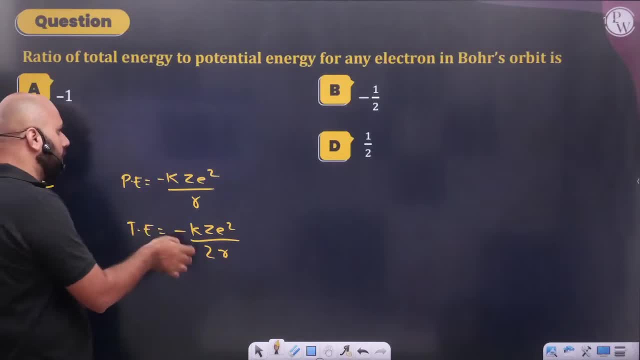 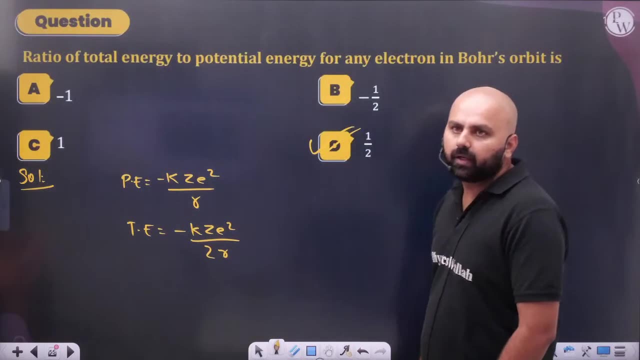 So remove the first and second option. See the ratio of these two. How much ratio is coming with us? One ratio will not come. Which ratio will come? D answer will come. One ratio will not come with us. D answer will come. 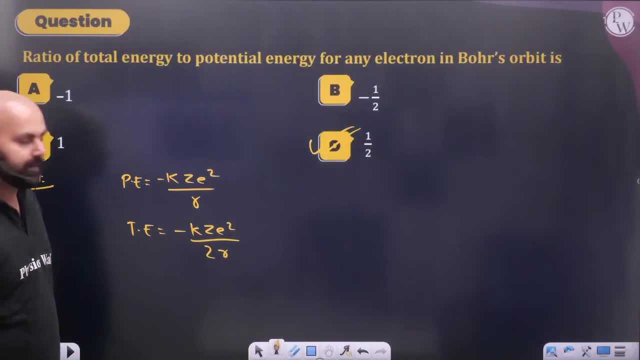 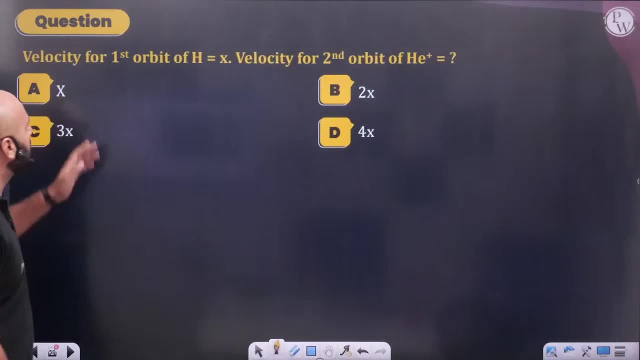 Okay, That's it, Brother. let's revise it quickly. Let's revise it quickly, Let's finish it. See this: This question is given, Sir. velocity of first orbit of hydrogen. Remember this. Let me tell you a simple thing. 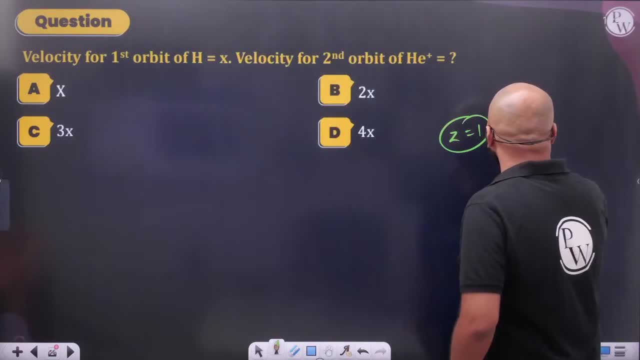 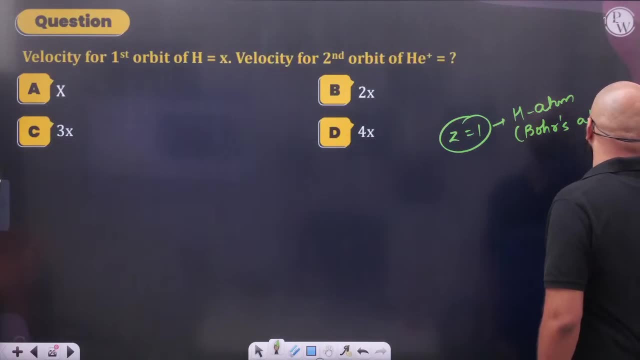 Sir, z is equal to 1.. This hydrogen atom will be given to us. What do we call it? We call it Bohr's atom. What do we call it? We call it Bohr's atom. If z is equal to 1, then we call it Bohr's atom. 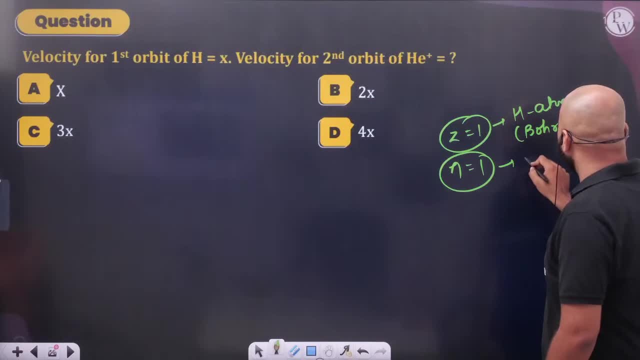 And n is equal to 1.. So what do we call it First orbit, But we call it Bohr's orbit. So whenever you are told something, remember that Bohr's atom or Bohr's orbit is not a different thing. 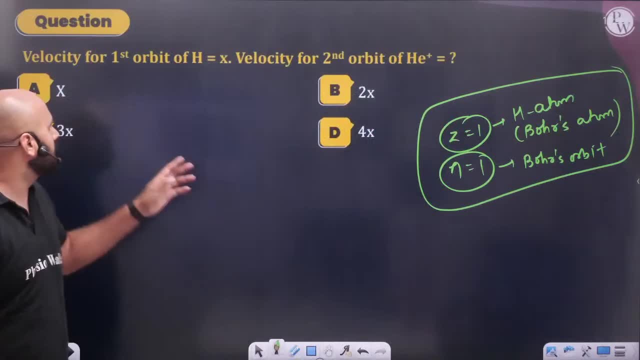 It is telling the same thing in a different way. See in this question. What is it saying? On which velocity is it directly proportional z by nk? On which velocity is it directly proportional z by nk? See the writing method. See the writing method in the exam hall. 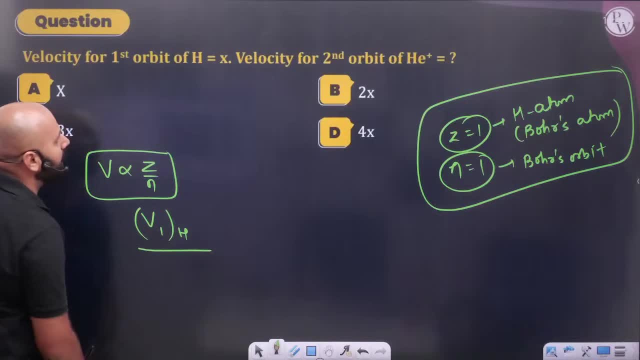 Velocity of first orbit, Whose Of hydrogen Divided by velocity of second orbit? Whose? Whose is to be taken out Of helium, Sir, whose velocity is directly proportional to z by n, z by n? In the case of hydrogen, it will be 1 by 1.. 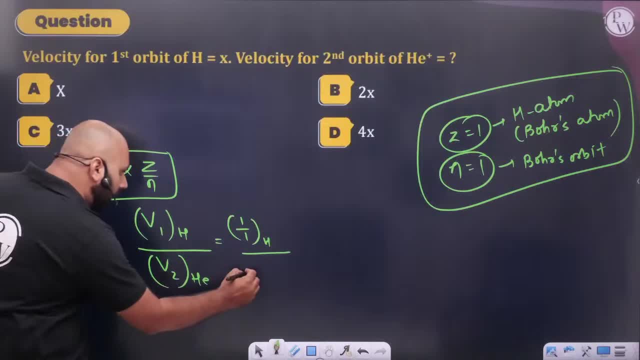 Because sir z is also 1. Number of orbit is also 1. What will happen in the case of helium? here, Atomic number is also 2.. Here is also 2.. So in the case of hydrogen and helium, you will see both. 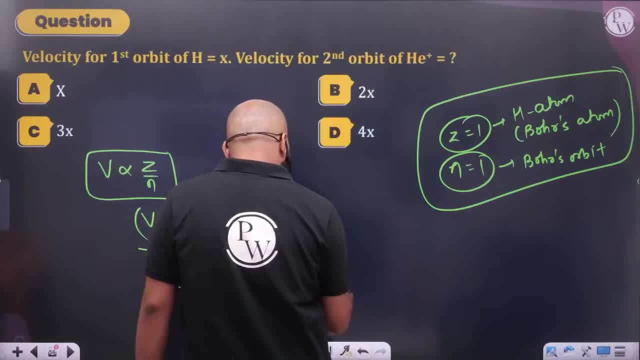 Sir, what is the velocity? in both cases, 1 is 2.. Ratio is 1.. Ratio of 1 is 2.. Ratio of one is 1.. What iselling the velocity of orbit? It will be XE. What will be the velocity of orbit? 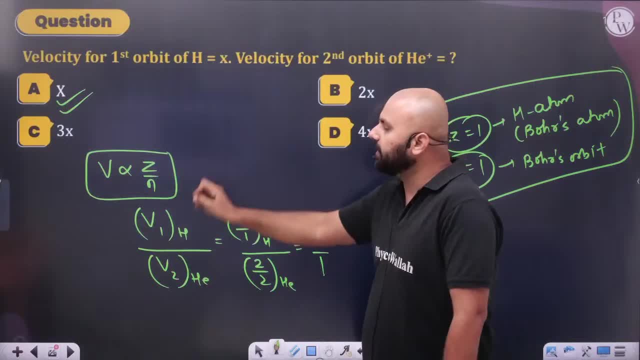 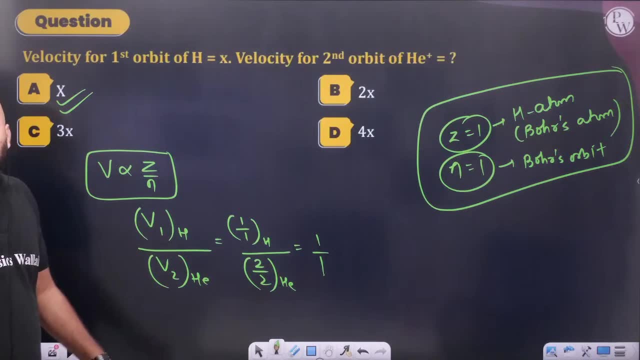 Gate isω. Why, Sir, ratio of 2 is2.. Z by n. What will happen z by 2. Sir, we don't take atomic mass right Atomic mass. Who are getting b option? Have you taken the ratio of atomic mass? 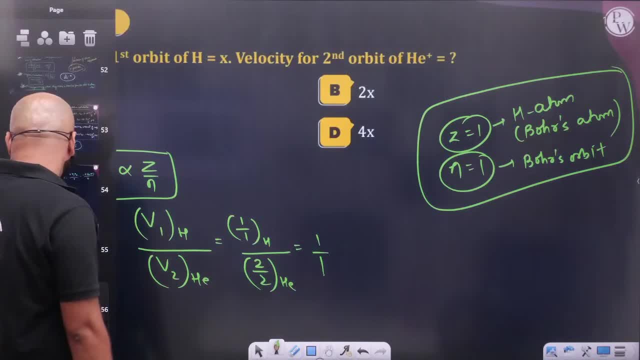 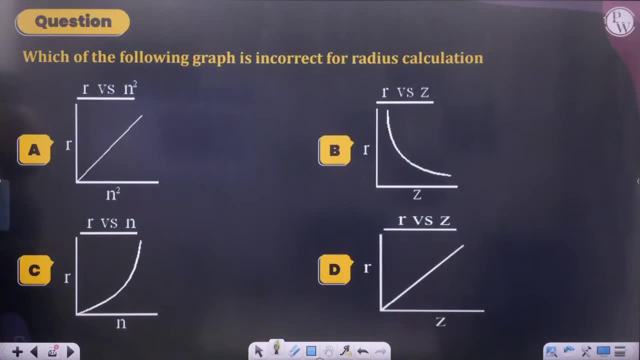 We don't take the ratio of atomic mass Strictway. it's a simple thing: velocity of z by n. See, if someone is asking a question graph wise, how will we find z by n? He is asking which is the incorrect graph. 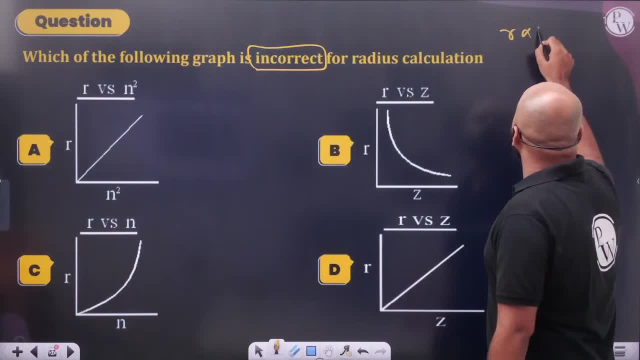 The radius is of n square by z and the velocity is n square by z. Sir, see the inverse proportional of radius and z. This graph is correct. The radius directly proportional to n? square. This is also correct. The radius directly proportional to z. 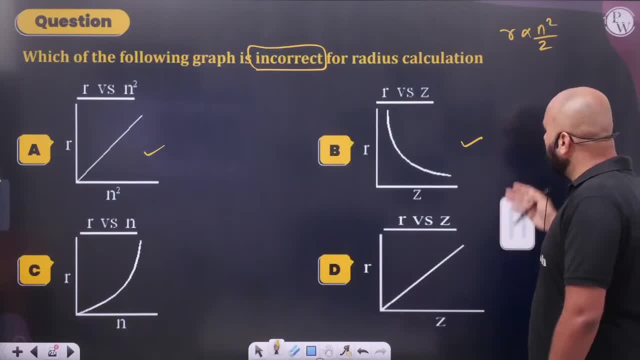 What is this graph? It is wrong. The radius directly proportional to z. What is this graph? It is wrong. What is the answer? It is d, The radius directly proportional to z. What is this graph? It is wrong. This graph is wrong. 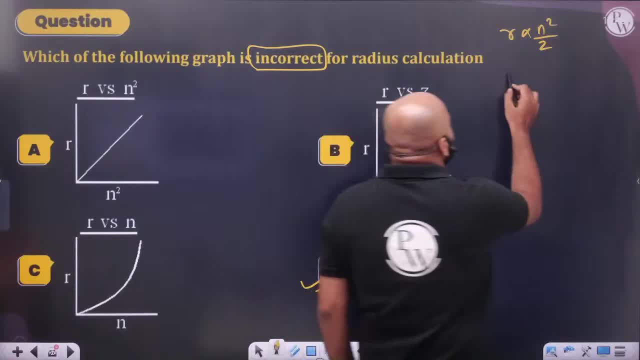 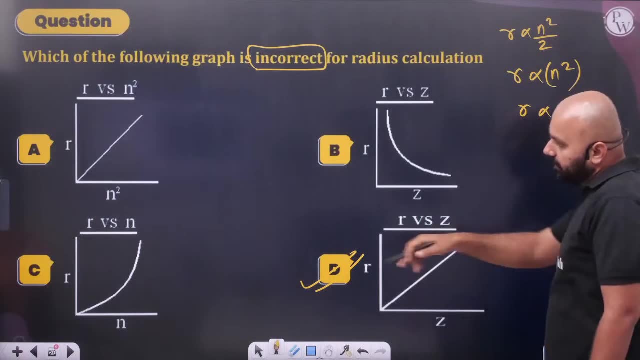 Because the radius of n square by z means the radius is directly proportional to n square. The radius is inversely proportional to z. If the radius is parabolic then obviously in respect to n it will be parabolic. Someone will say c. 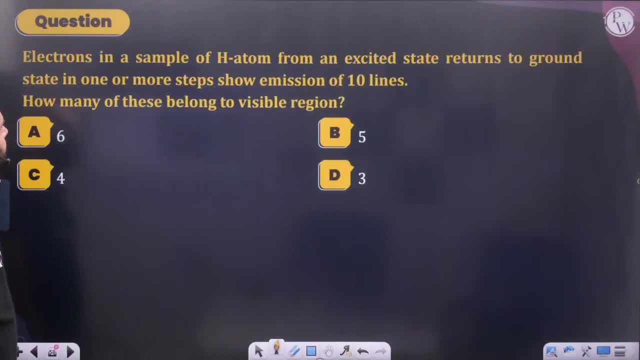 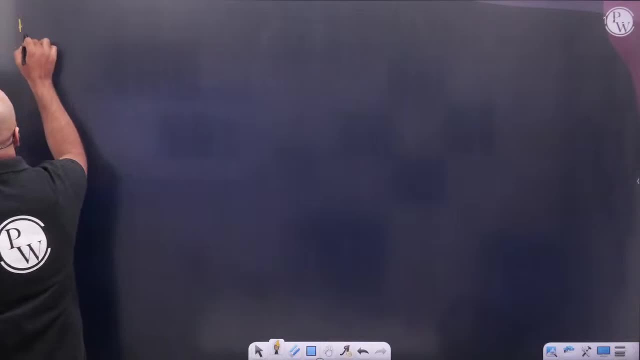 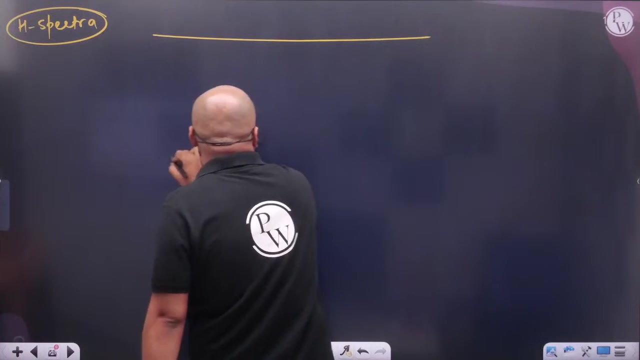 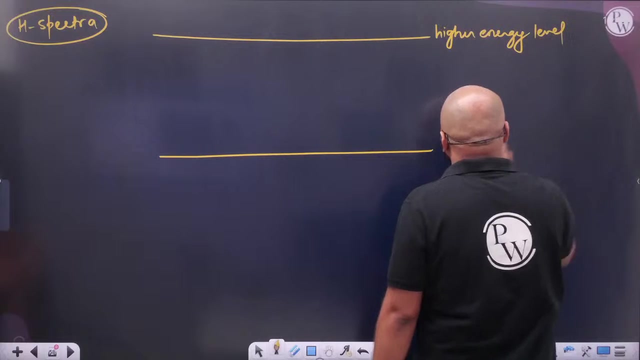 Sir, it is parabolic. Okay, Now see. Now let's talk about hydrogen spectra. Hydrogen spectra- What is hydrogen spectra? Remember hydrogen spectra. There are 2 types of spectra: One is absorption and the other is emission. If you are at higher energy, you would lose energy. 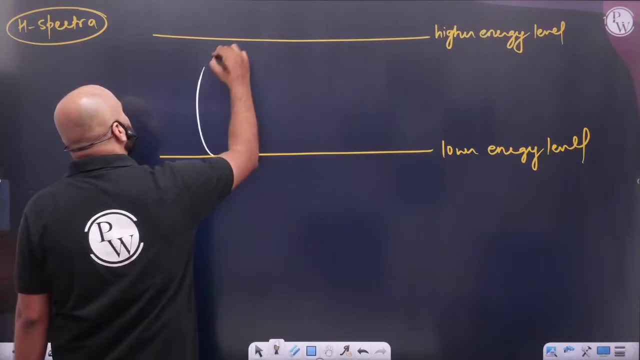 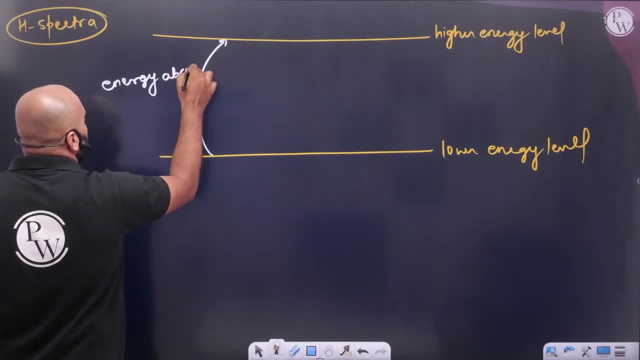 Watch this, Watch this. We will go from here to here, sir. So you absorb energy. If you go from here to here, then you will lose energy. energy is absorbed. What is the spectrum on this side? It is called absorption spectrum. 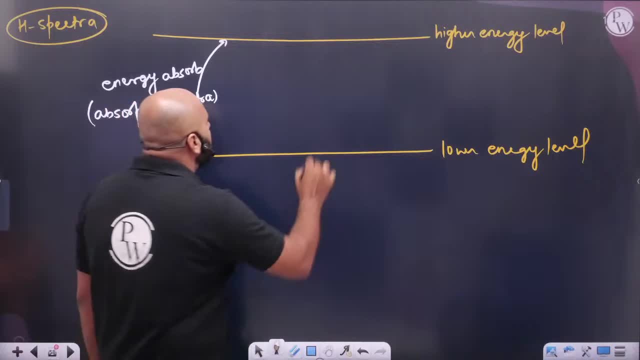 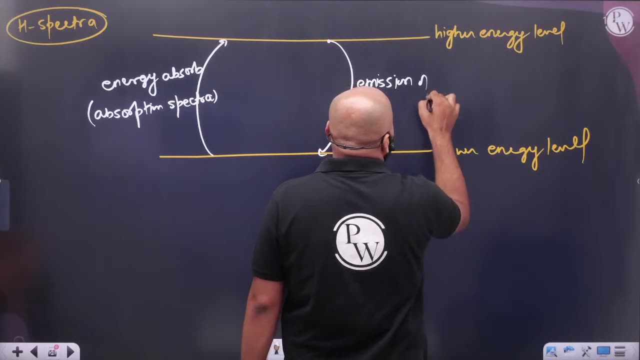 What is the spectrum on this side? It is called absorption spectrum. If you go opposite side, it will become emission spectrum- Emission of energy. and what it will become Emission spectrum? What it will become Emission spectrum. In this case you can use the direct Rydberg formula. 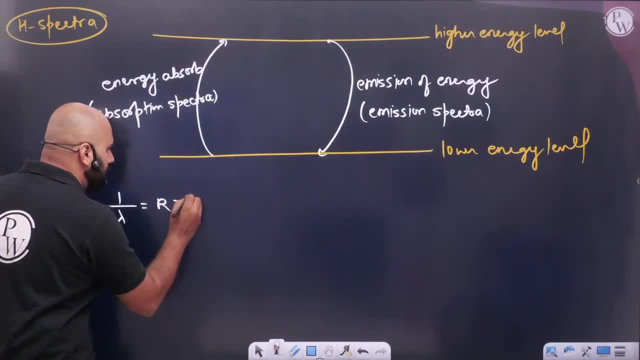 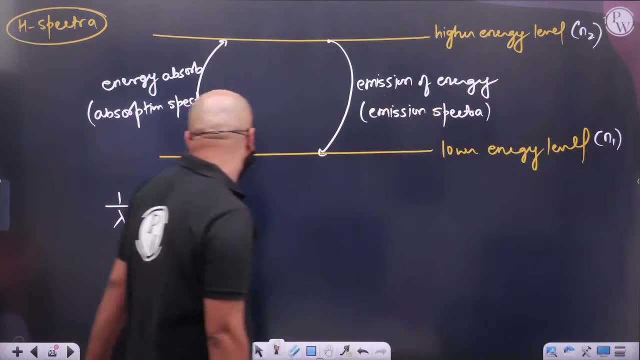 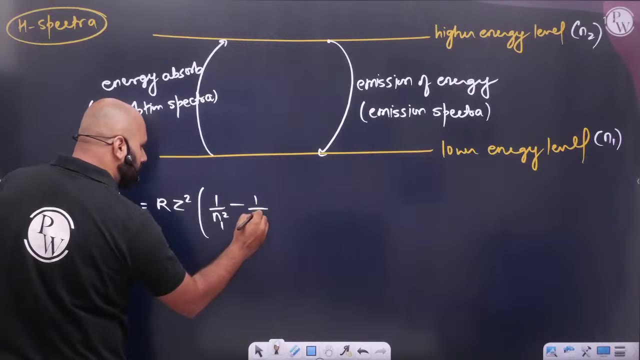 and that is what. 1 by lambda is nothing. r z square. 1 by n2: higher energy level means n2, lower energy level means n1.. See for yourself: 1 by n2 minus 1 by n1 square minus 1 by n2 square. 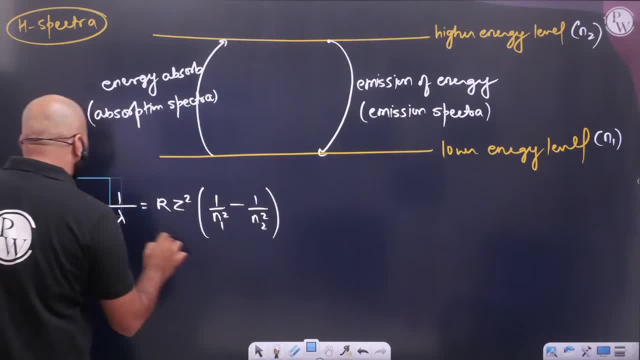 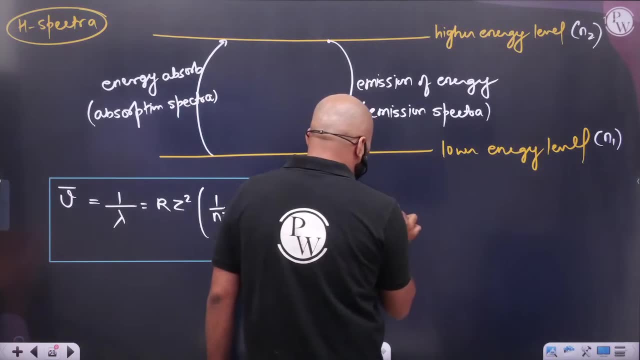 What do we call 1 by lambda? We call it wave number, So you can use this Rydberg formula. In this formula, what is the value of R Where R is 109678 centimeter inverse, or if I say directly, for numericals? 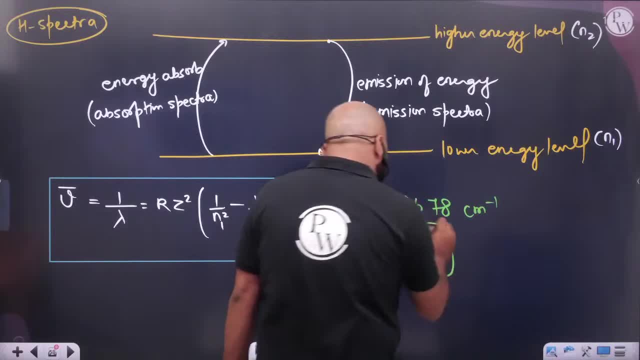 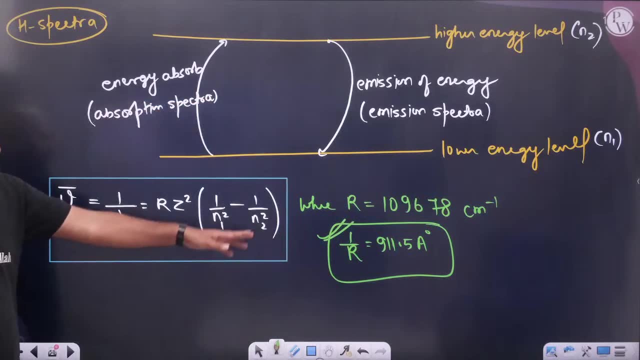 then you can use this for numericals. What is the value of 1 by R 911.5 angstrom? If you are talking about numericals, then what is the value of 1 by R 911.5 angstrom? 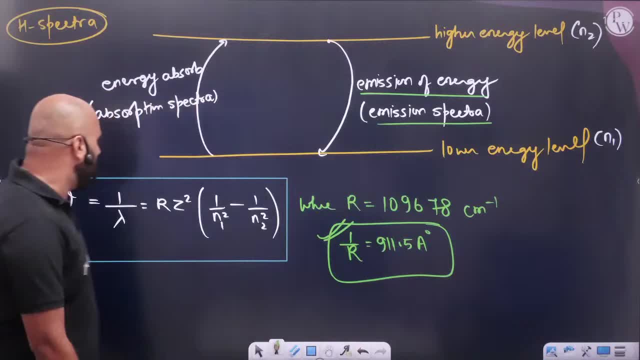 If you go from higher to lower- we always talk about emission spectra- If you are coming from n2 to n1, if you are coming from n2 to n1, if you want wavelength, then what will you do For wavelength, you will use this formula: 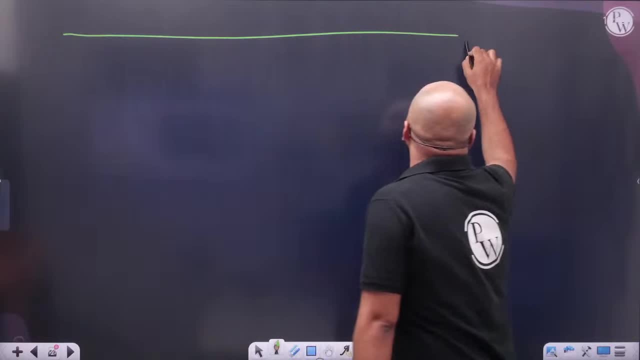 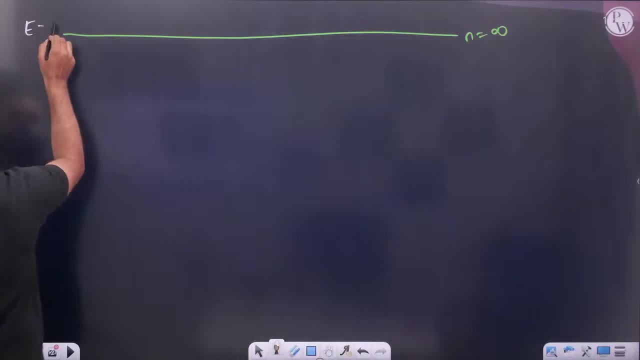 After that, why is the hydrogen spectra unique? Because there are a few things in the hydrogen spectra. If n is equal to infinity, then how much energy will it have? Sir? if I come from below, I take n is equal to 8.. 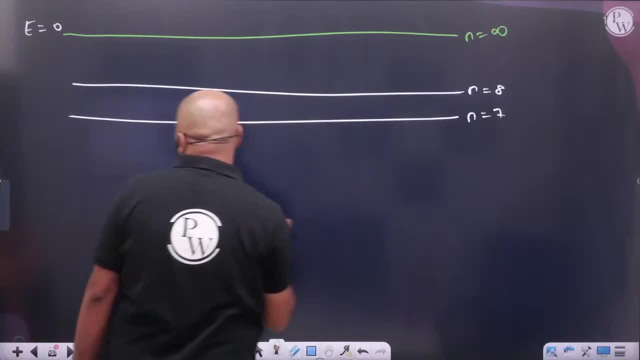 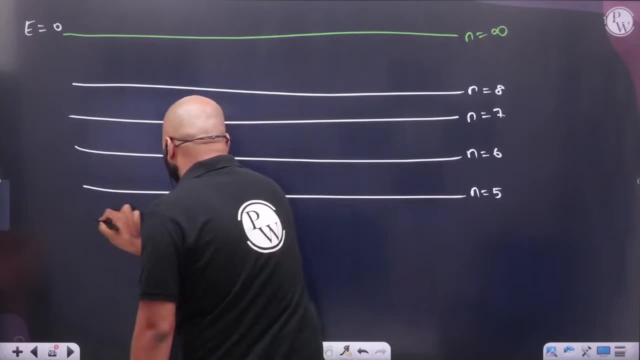 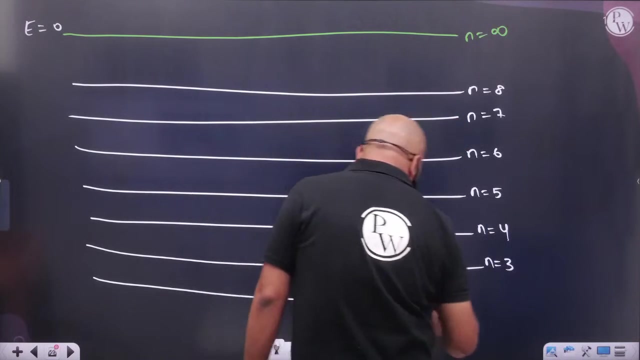 If I take n is equal to 7.. If I take n is equal to 6.. If I take n is equal to 5.. If I take n is equal to 5.. If I take n is equal to 4.. If I take n is equal to 3.. 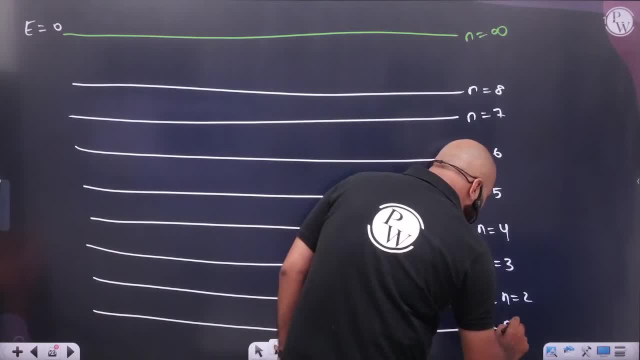 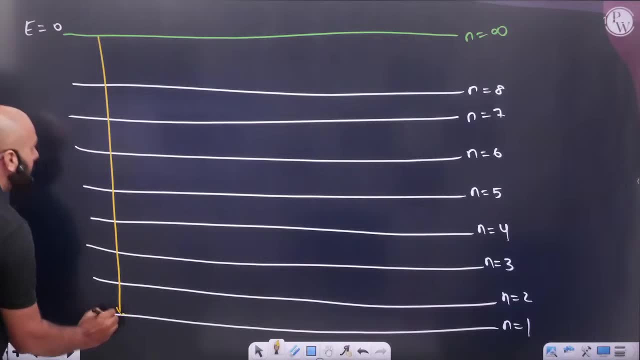 If I take, n is equal to 2.. And the last one, n, is equal to 1.. At the very end we have ground orbit. Now, if I jump electrons from here, from anywhere from anywhere, if you jump directly at the first, 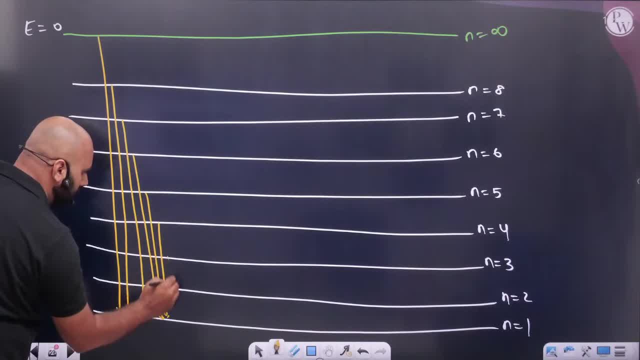 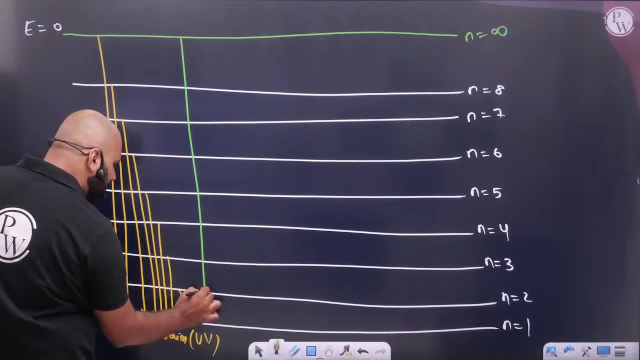 whatever lines and lights you will get, all of them will be called Lyman series. And the lines of Lyman series, all of them, are of UV radiation. If you jump at any second, remember all these small things. you will practice again and again. 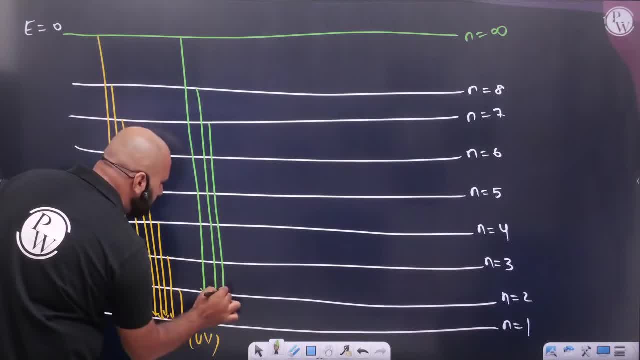 you must have remembered, but I am reminding you at the last time: if you jump at any second, at any second, then what you have to do. if you jump at any second, then what you have to keep, that which series is this: 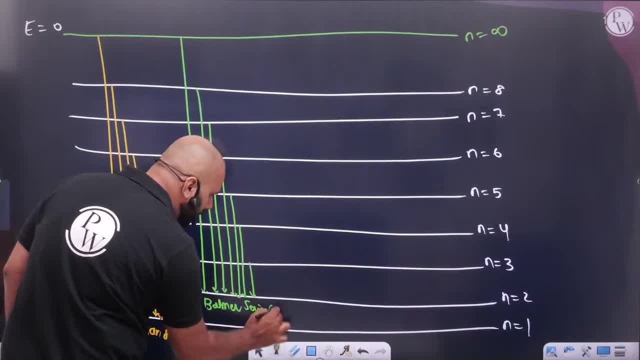 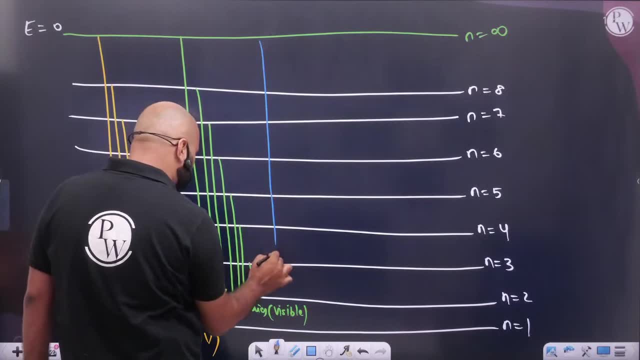 it is a Balmer series. Balmer series means what has happened, visible, what has happened, it has become visible. And tell yourself: no, sir, I do one thing, I jump at third. I jump at third from anywhere. 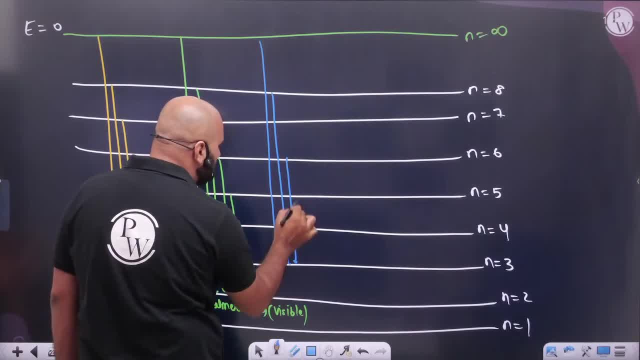 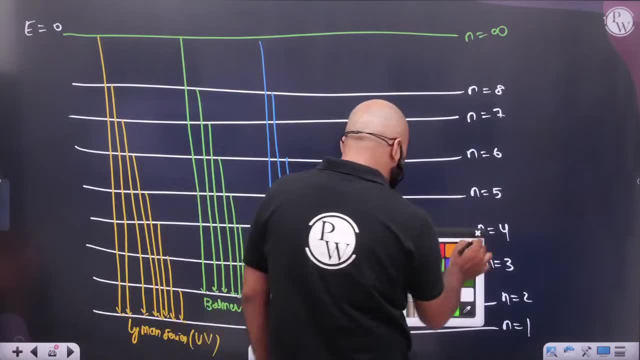 if you jump at third after this, wherever you jump after Lyman, Balmer will come, after Balmer. what will come? Paschen will come. it will keep going like this, like this: you jump on the fourth from anywhere. 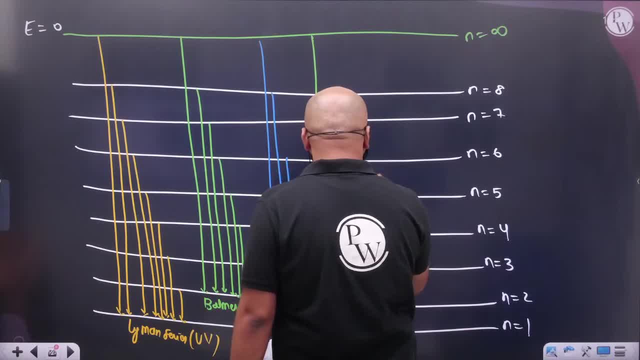 you jump on the fourth from anywhere, from anywhere, you jump on 4,. so what will happen? this bracket will be created Lyman Balmer Paschen bracket, And if you jump on 5, all of this, as many people as possible. 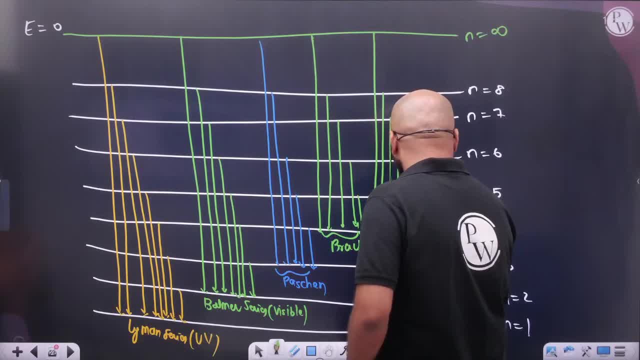 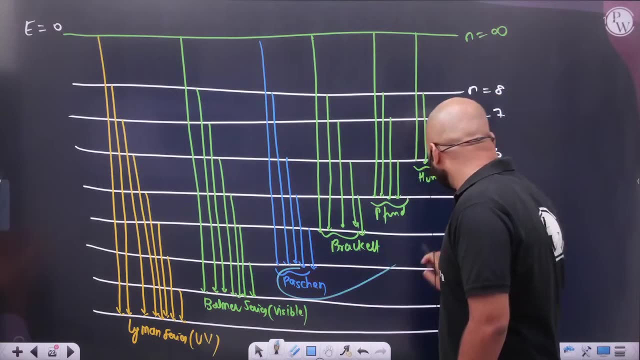 Lyman, Balmer, Paschen, Pfund, and if you come on 6, then what will be called Humphrys? This will be called Humphreys. All these after this, after Balmer, all these will be in which series? 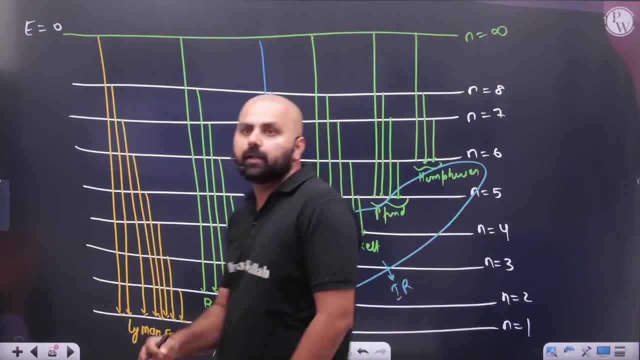 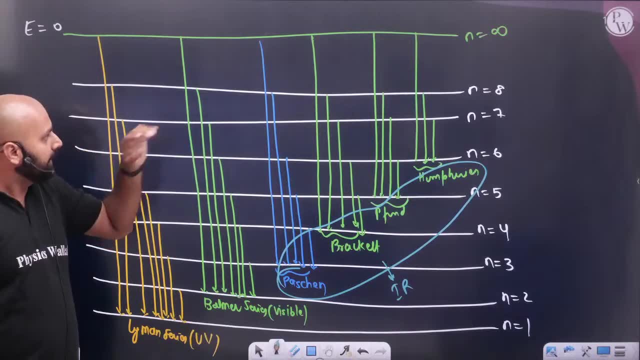 All these will be infrared. All these will be infrared. All these will become infrared. Lyman, Balmer, Pasteur, Braket, Piffen, Humphreys- All these are spectral lines. Here, 2-3 questions are very famous. 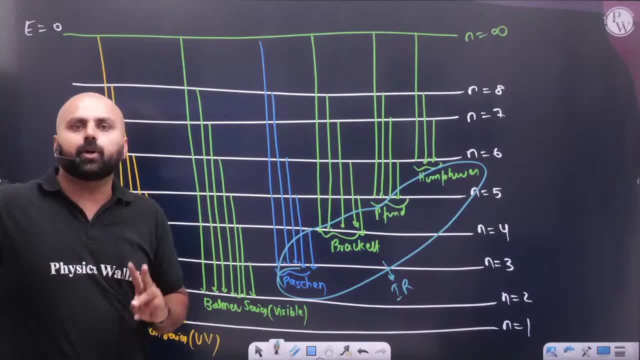 2-3 questions are very famous. If you jump from N2 to N1, then 2-3 questions are very famous. See which ones they are, Because total number of if you are coming from N2 to N1,. 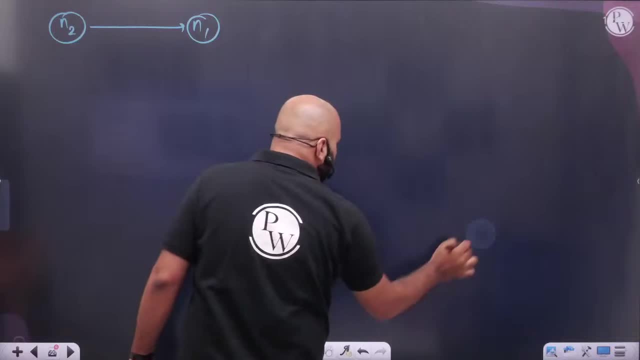 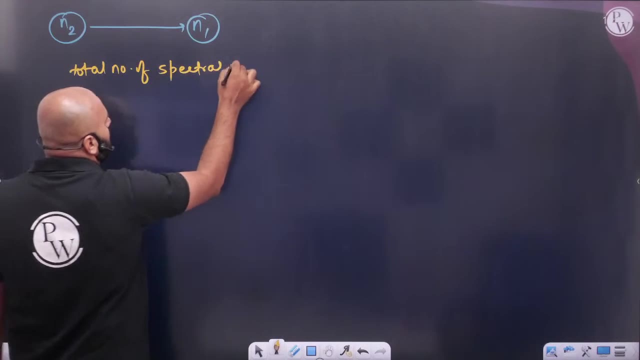 if you are coming from N2 to N1, if you are coming from N2 to N1, then the first question comes: total number of spectral lines. You have the first formula: total number of spectral lines. What will happen? N2-N1,, N2-N1, plus 1,. 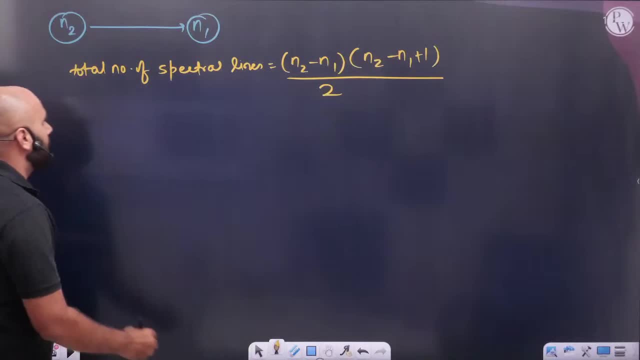 divided by 2.. And if someone asks, Sir N1 was going from N2,, number of spectral lines. number of spectral lines, number of spectral lines in that particular series in a particular series means in Lyman or Balmer. 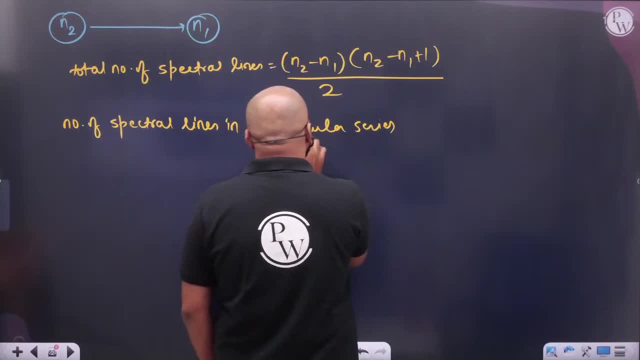 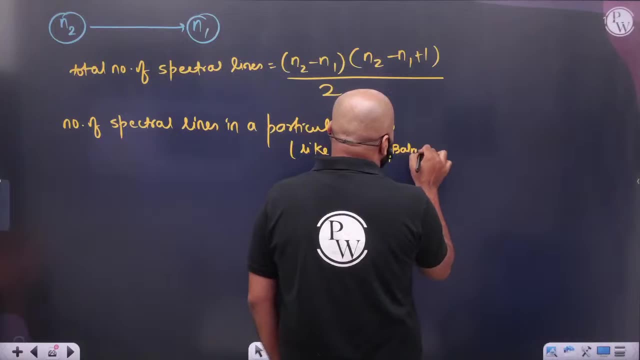 or in particular series. particular series means like Lyman Balmer. if someone asks something like this: Sir, tell me in Lyman, how much is the series of Lyman Balmer, etc. If someone asks something like this: 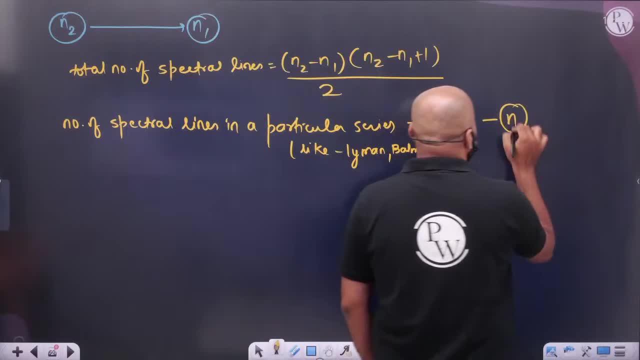 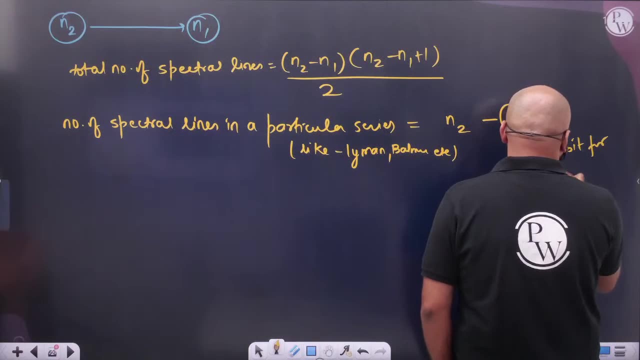 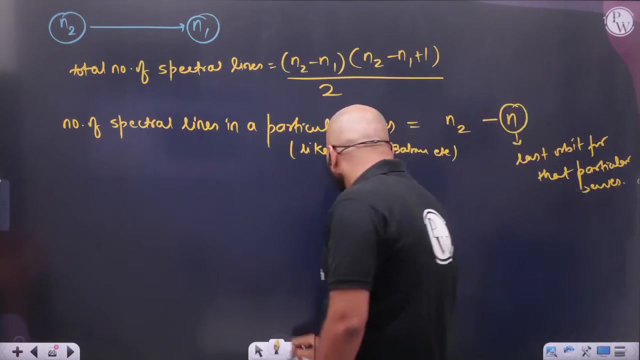 then remember in that case, N2-N, and N is the orbit for that particular series, The orbit in which you have to come First thing. keep this in mind. After that, suppose if someone is talking about Lyman series. 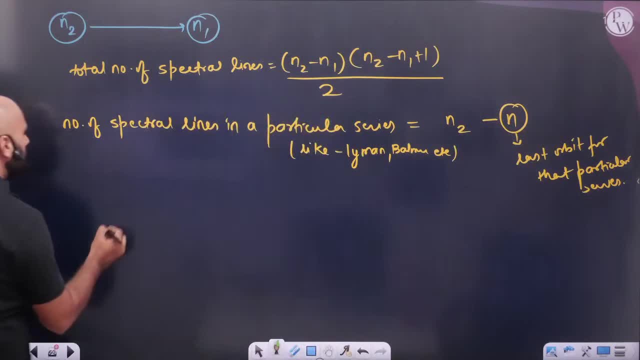 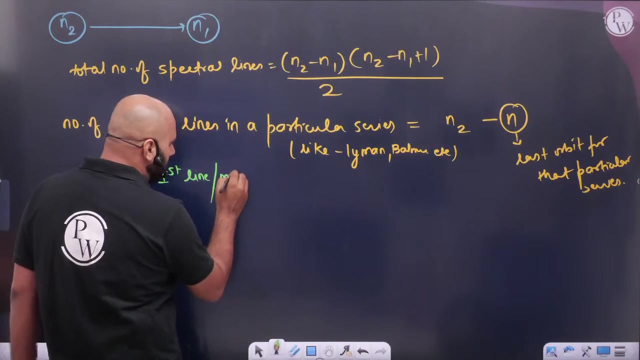 look carefully at yourself. if someone is talking about Lyman series, any series is given suppose there is Lyman series. so if someone says in Lyman series, Sir, the first line, or what do we call the first line, the first line will be of minimum energy. 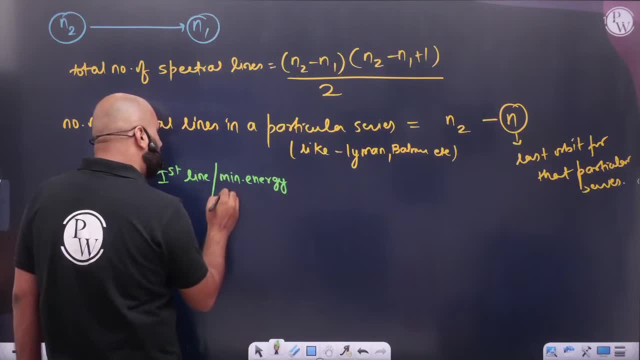 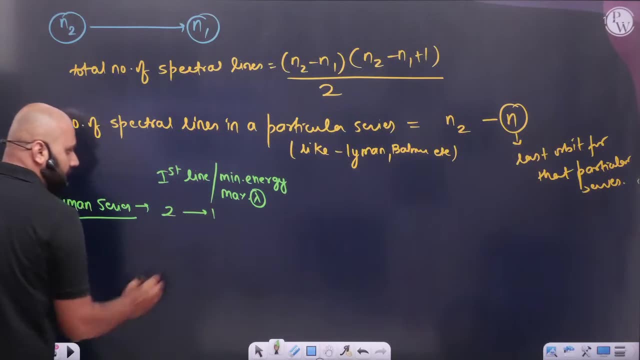 first line will be of minimum energy. where minimum energy, what is the maximum there? Wavelength. Minimum energy, maximum wavelength. Where will the first line of Lyman series come from? From 2 to 1.. If someone says the last line, 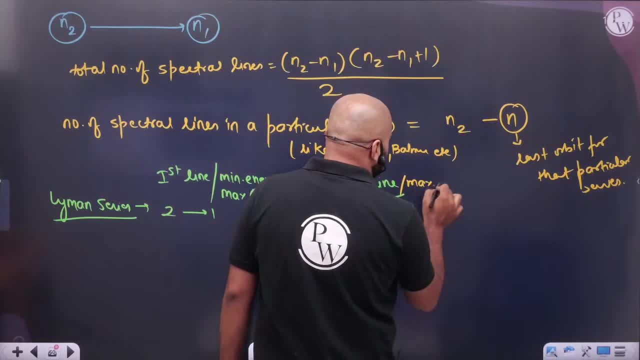 Sir, where will the last line come from? So, where will the last line come from? Obviously, from infinity. Last line means maximum energy, and that's why minimum wavelength Last line has maximum energy, and that is minimum wavelength, Sir, after Lyman. 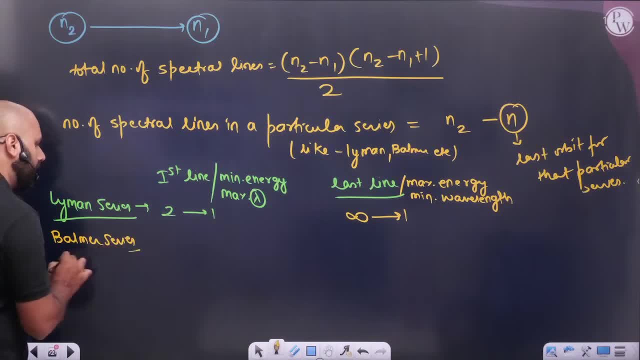 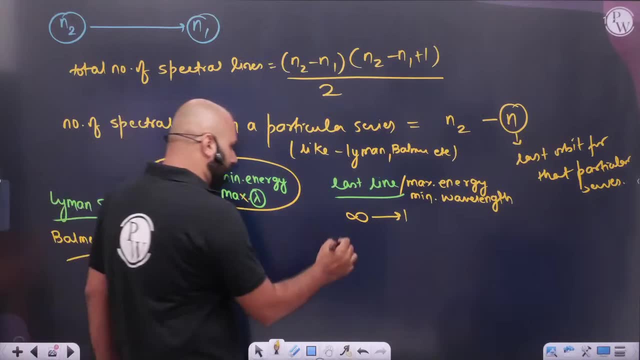 if someone asks about Balmer, then in Balmer series, where will the first line come from? From the person next to you And the person next to you. what happens in the first line- Minimum energy gap and what is the maximum? 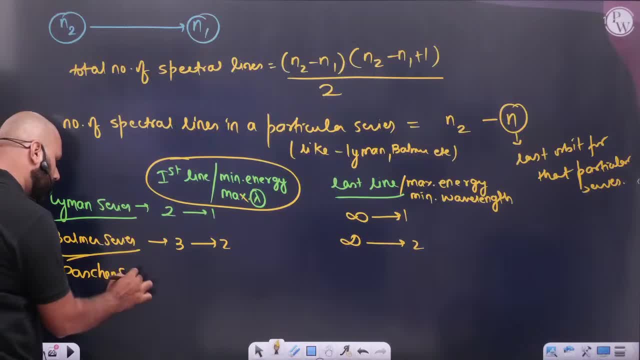 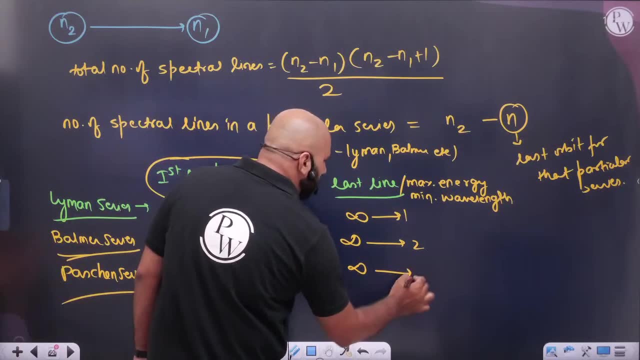 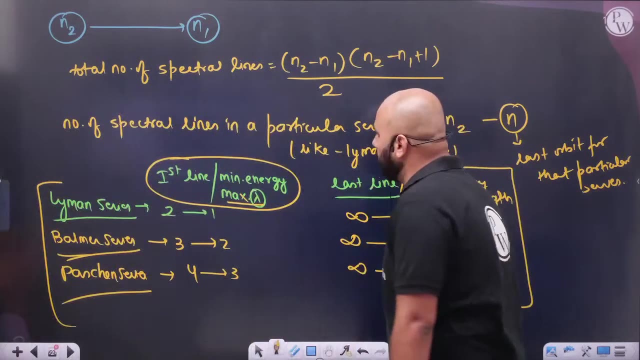 Wavelength And what will happen From infinity to 2.. After Lyman Balmer? what will happen after Balmer? Like this: Lyman Balmer, 1st line, 2nd line, 3rd line. 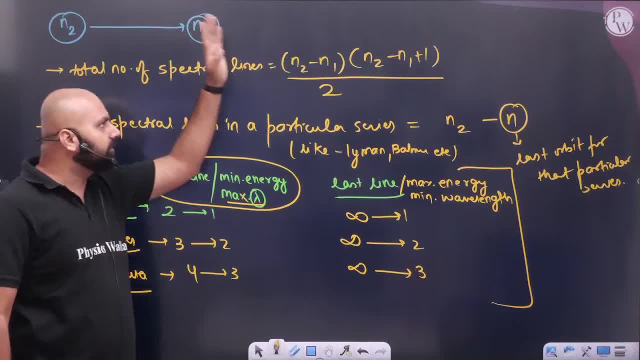 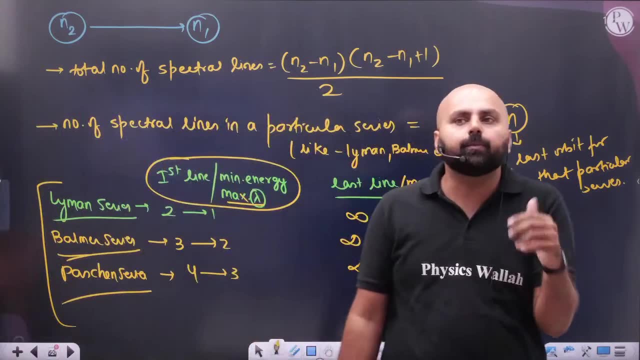 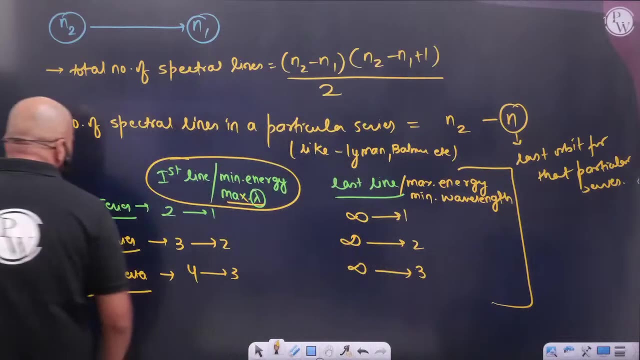 These two formulas are different. This is the total number of lines And this says lines of a particular series. What will happen? Particular series means lines of Lyman Balmer. See this, See this question In this sample of electrons. 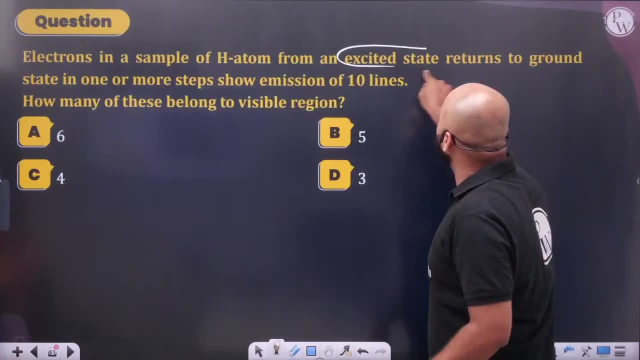 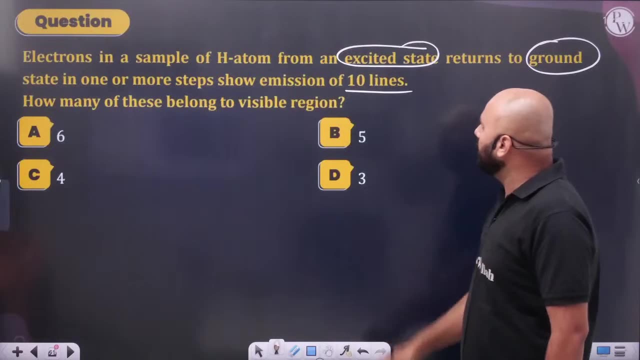 from the excited state it is coming to the ground state, From the excited state it is coming to the ground state. Ground state means total number of lines is 10.. Total number of lines is 10.. How many lines are there in visible region? 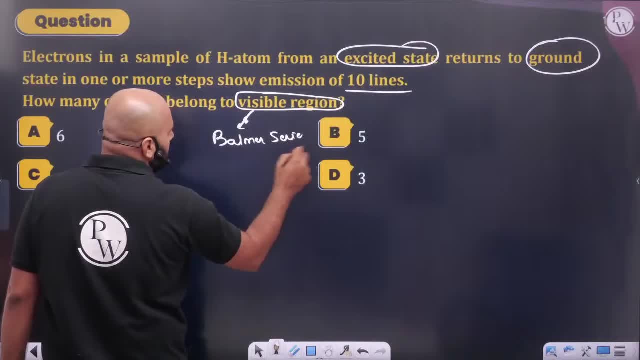 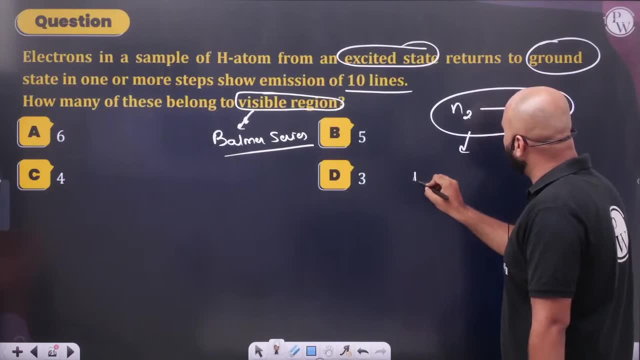 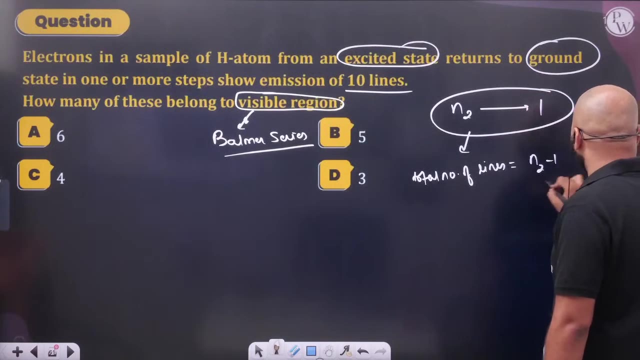 Visible region means: whose line are you asking? Feasible region means whose line are you asking? Balmer series line. Balmer series line: See this. These are the questions. What will be the formula of total number of lines? 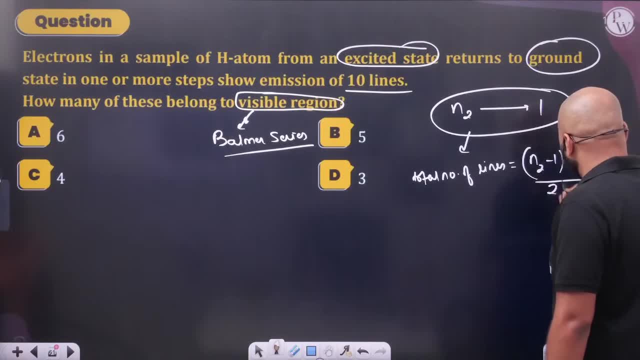 N2 minus 1.. N2 minus 1 plus 1.. Divide by 2. Total number of lines is 2.. 10. N2 divide by 2.. See this Minus 1 plus 1.. Sir, how many will be divided by 10?? 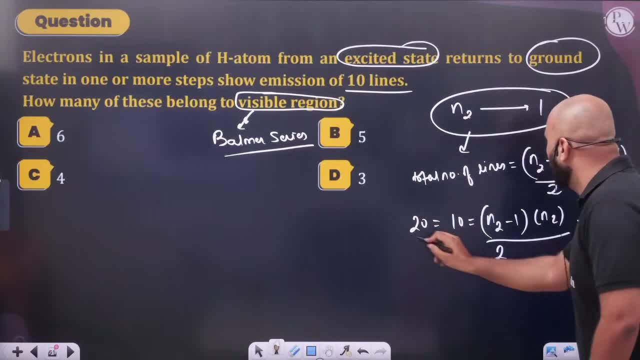 I can write 20.. What can I write? 20 by 2.. N2 value should be 20.. When can it be? When can it be, Sir? what will happen to us? What will be 4 times 5 by 2?? 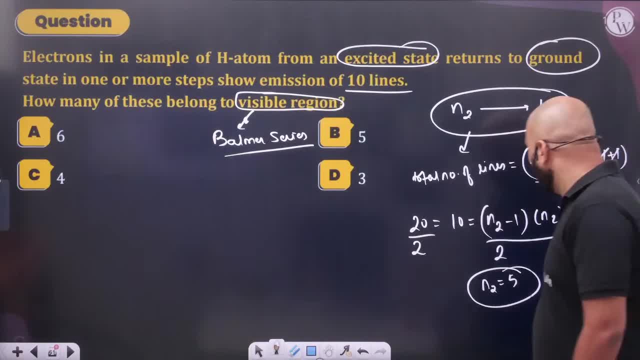 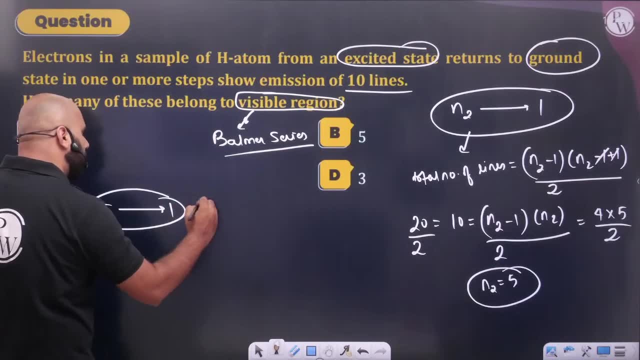 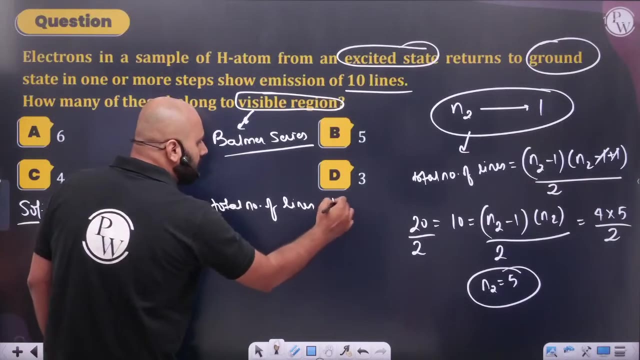 This only can happen. What is the value of N2? It is 5.. What is the value of N2? It is 5.. When you will come from 5 to 1, total number of lines: total number of lines will be 10.. 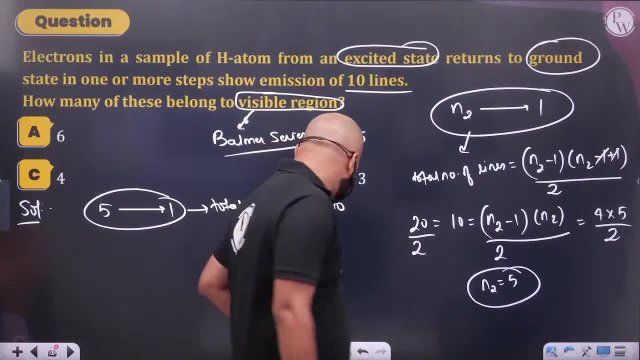 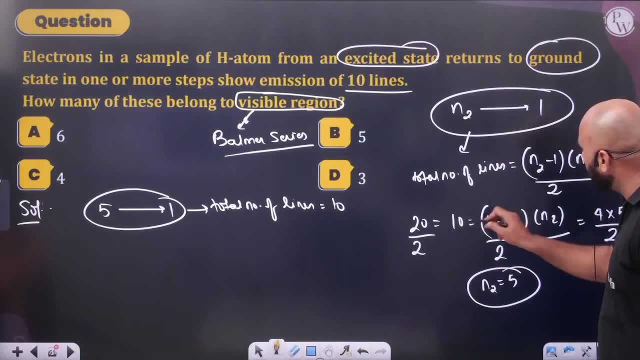 How did you do 4 times 5?? This is a simple method. See what you have to do. This is 20.. When can it be 10? If someone is divided by 2 and the answer is 10.. What should be above 20.? 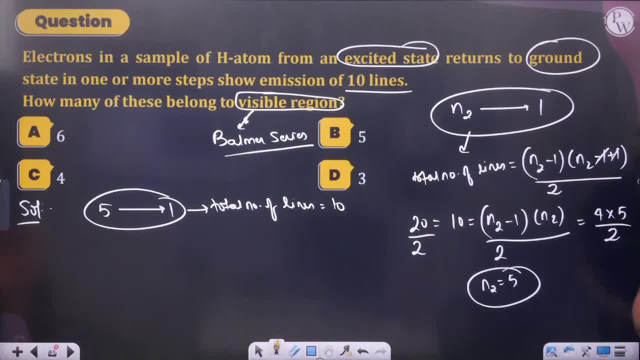 When can it be above 20?? One number is just a big number. When can the multiplication of 2 people be like this: 4 times 5.. From here I have the total number of lines. What will be the lines of the Lyman series? 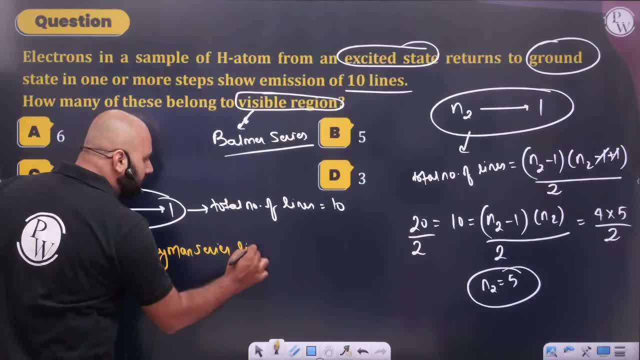 How will we get the lines of the Lyman series? How will we get the lines of the particular series? How will we get the lines of the particular series, Sir? that minus Lyman series means, Sir, we have to get the lines of the Balmer series right. 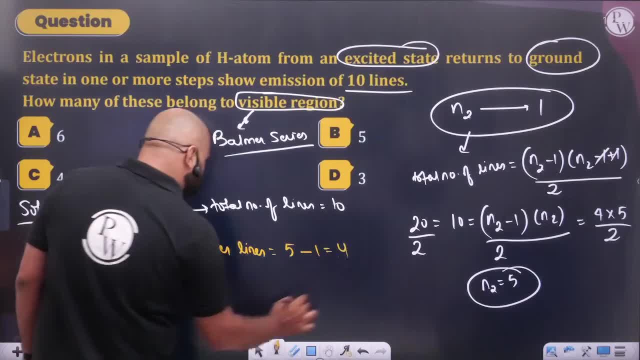 Sir, we have to get the lines of the Balmer series right. What will be the lines of the Lyman series 4.. I have to get the lines of the Balmer series. What will be the lines of the Balmer series for me? 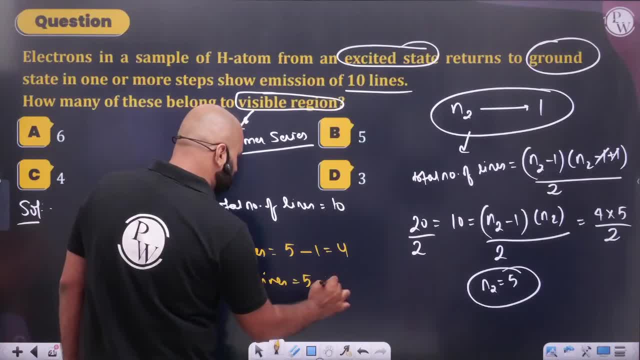 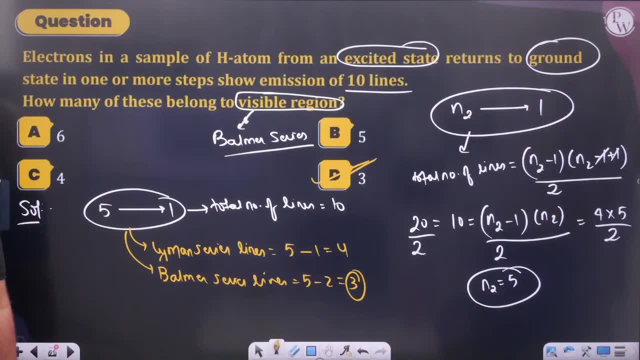 What will be the lines of the Balmer series? This will be 5 minus 2.. How much will it be 3.? And that will be my answer. How much will it be 3.? Ok, Ok, So this will be the answer. 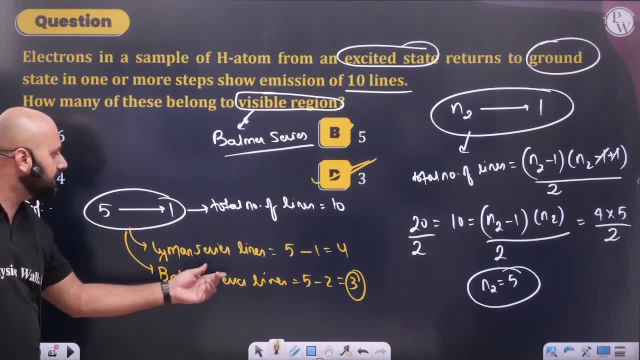 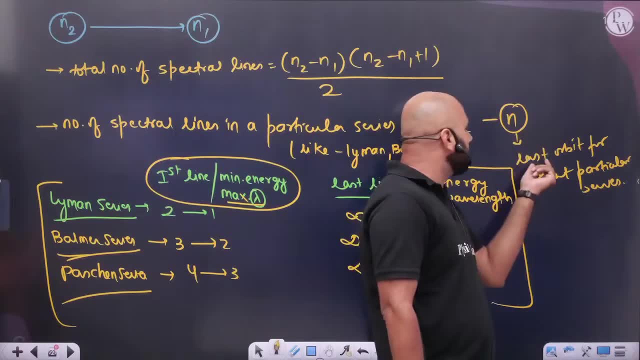 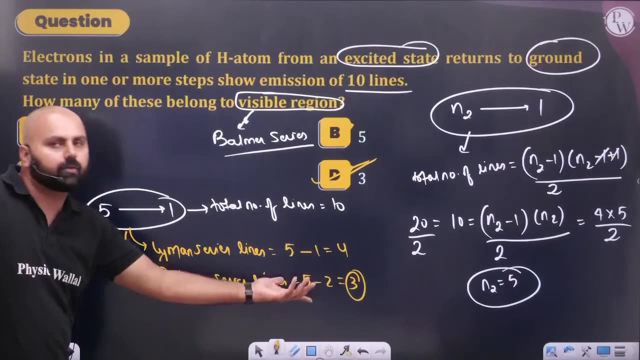 Now how many lines will be there in a bomber series like this? it has come in Lyman, it has become a bomber. see, the particular goes in a series, it goes in a particular series then, from N2,. where is the last orbit of that series, of the particular series, like in the case of Lyman? what is the last line of Lyman? it is 1,. what is the last orbit of the bomber? it is the second orbit. do it with yourself, keep doing it. bomber, Lyman, bomber. how much has become 2, Lyman? if it will be of the past, then how much will it be brother? what does the past mean? the last series means on which it is defined. 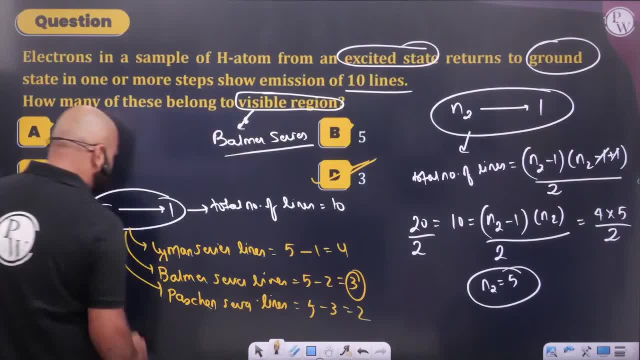 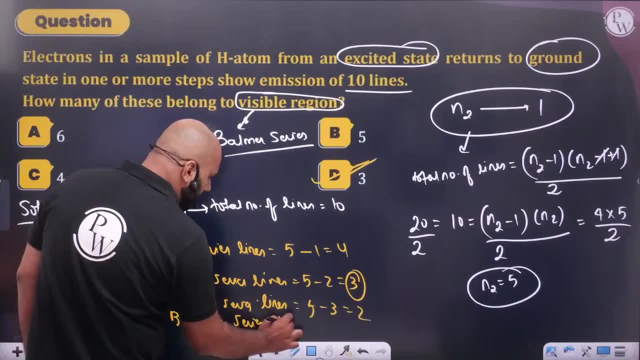 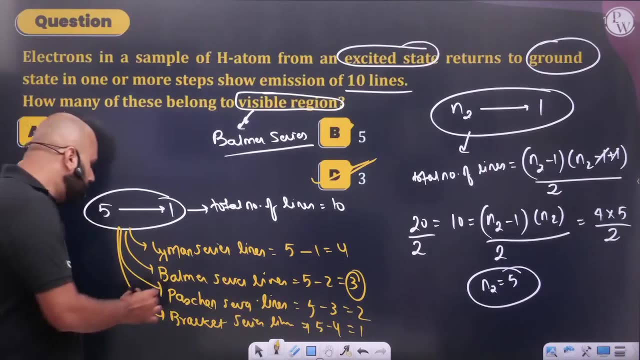 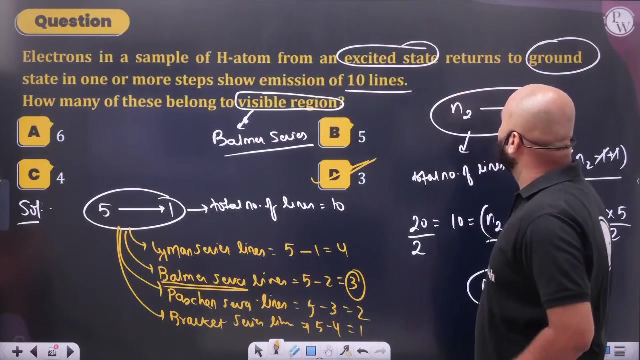 last means 5 minus 3, how much has become 2,? sir who said, sir, tell me about the bracket, then how much will become in the bracket? how many lines of the bracket series will become 5 minus 4, 1, see, the total number of lines is 10, which of those 3 is visible? line which was visible? it was a bomber series. after Lyman, it was a bomber. do it with yourself, okay. so 5th excited state. what will be the excited state? what will be the value of N2,? 5 only came. 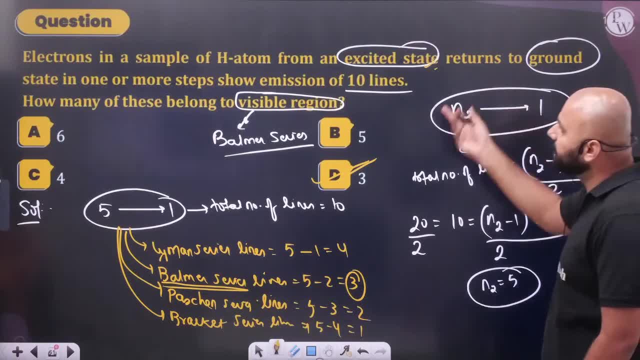 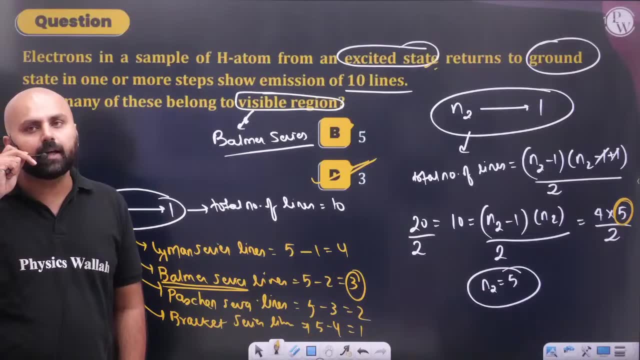 the value of N2 is 5,, 5 into 4, so the excited state will be 6th state. it will not happen. the value of N2 will be 5,. brother, okay, what line will be coming to us? what will be the total number of emission lines? it is coming to the ground state. ground state means what happened. it will come to 1, we will not say 0,. 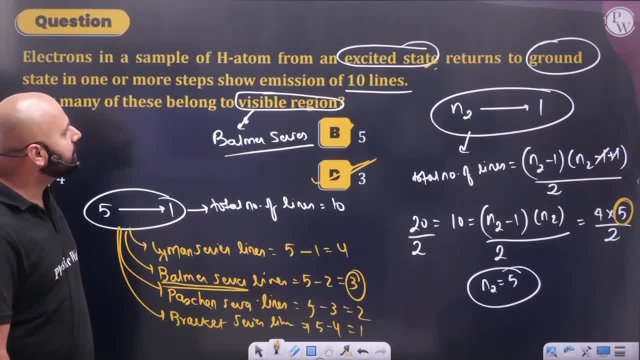 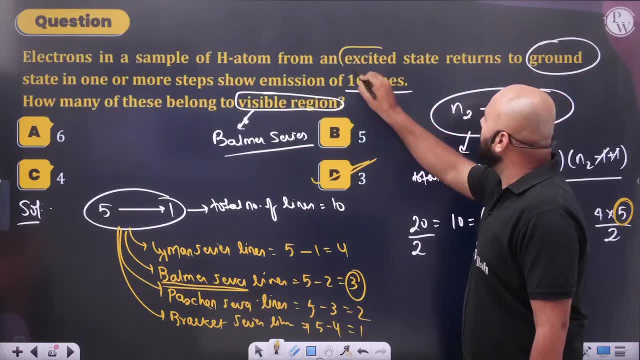 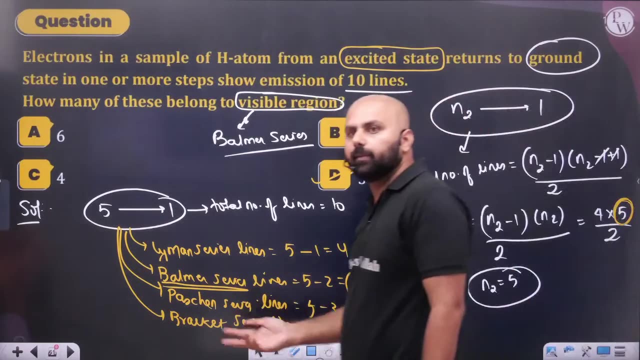 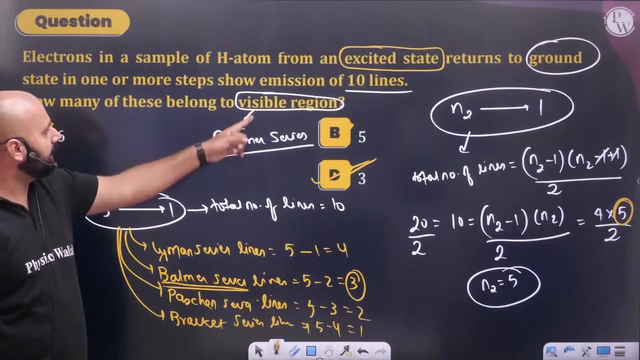 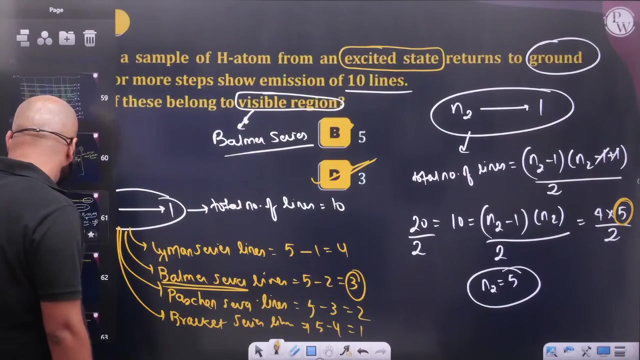 we will not say 0,. 5th excited state. it will not happen. brother, what value of excited state have I taken here? I have taken N2, so why do I add it myself, brother? how much the value of excited state has come now, any orbit will happen. this is the 5th orbit. it will come on 5th, 6th, 1st, where did it come on? 6th, 7th, on its own? okay, it will not happen on its own. it is coming in the ground state. on which will we take visible light? on the bomber series, nothing else. okay, see this with you. whenever such questions are asked, like this question is given. see this shortest wavelength. 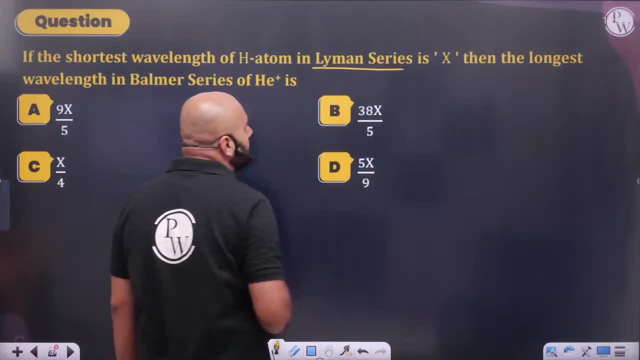 the shortest wavelength of Lyman series. What does the wavelength mean? where the energy gap is should be less. when the energy gap will be less, where will the energy gap from 2e it will be came on? 1, shortened wavelength of hydrogen. 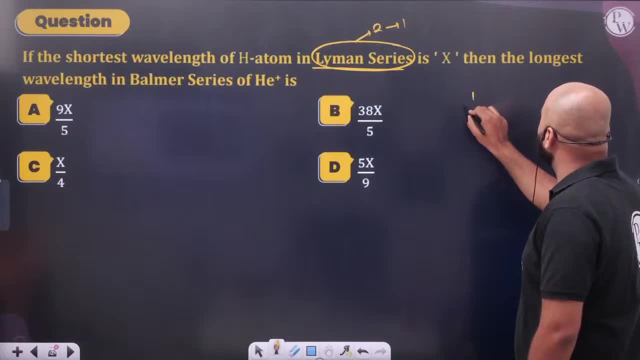 is given. the shortest wavelength of hydrogen is given, it is 1- Lives under 2涉1. Too much came to solve it: j1x Minus 1 bai2, How much will it be? 1 by lambda minimum, and that is equals to 3r by 4.. 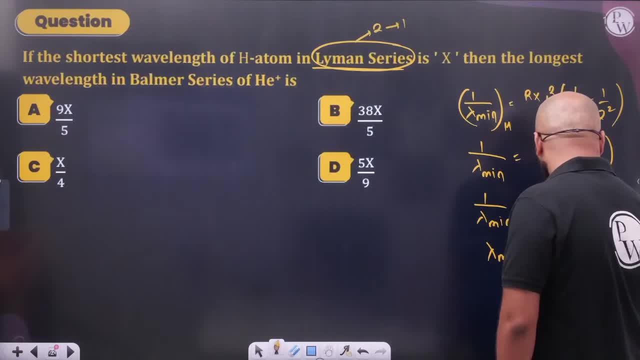 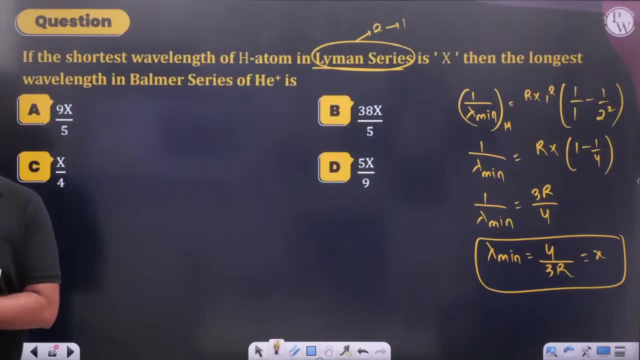 The value of lambda minimum is 4 by 3r and the value of this is x. The value of lambda minimum is x. What is the value of lambda minimum? It is x. I have come to know about this. He is saying: tell me the Balmer series of helium plus. 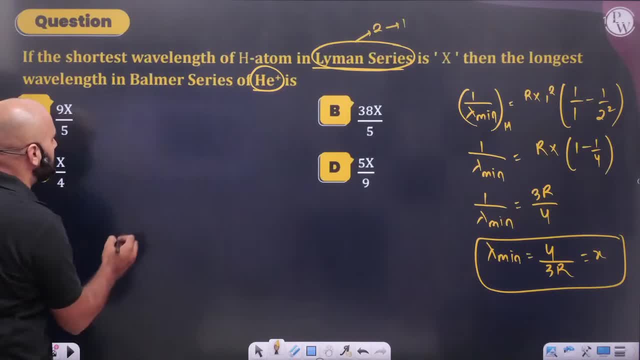 I have come to know the value of lambda minimum x. Now let's do one thing: The Balmer series of helium plus Which one? The longest wavelength. When does the longest wavelength come? When does the shortest wavelength come? If we have to find the lambda, then the energy is coming. 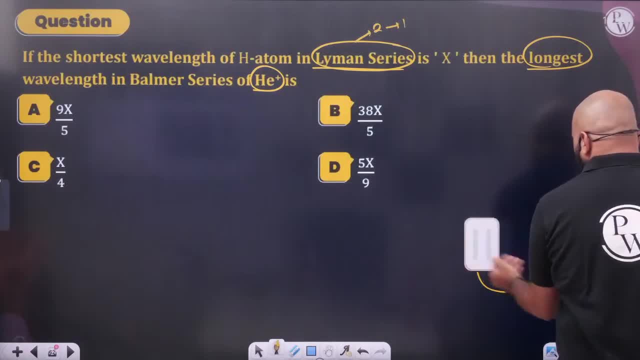 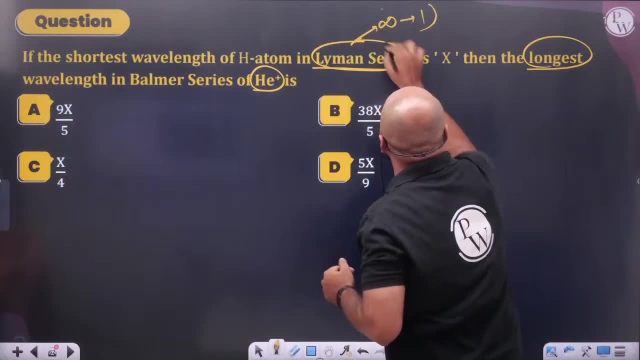 I made a mistake. We have to find the lambda minimum. in the first case, Lambda minimum means the maximum energy gap. When will the maximum energy gap occur? When you will come from infinity to 1.. When you will come from infinity to 1.. 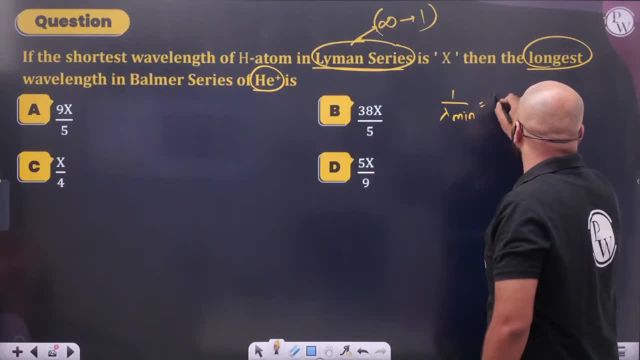 When you will come from infinity to 1, then 1 by lambda minimum, that is, r Into 1 by square, 1 by 1 minus 1 by 1 by square of infinity by square. So 1 by x is going to be r. 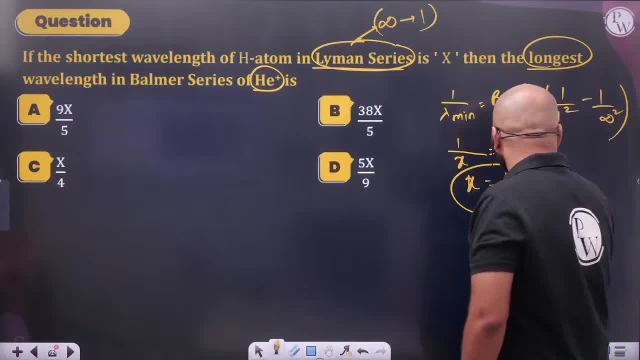 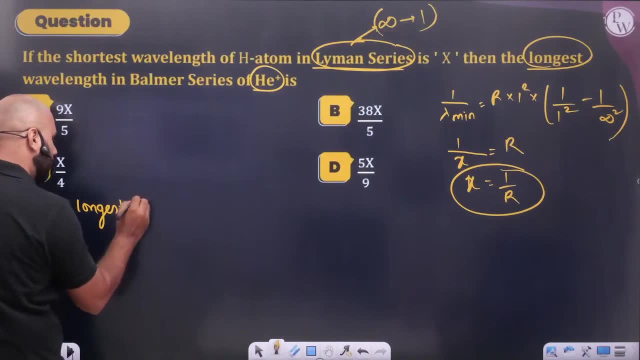 What is the value of x? It will be 1 by r. What is the value of x? That is 1 by r. The longest wavelength has to be found from the Balmer series. When will the longest wavelength come? The longest wavelength of the Balmer series. 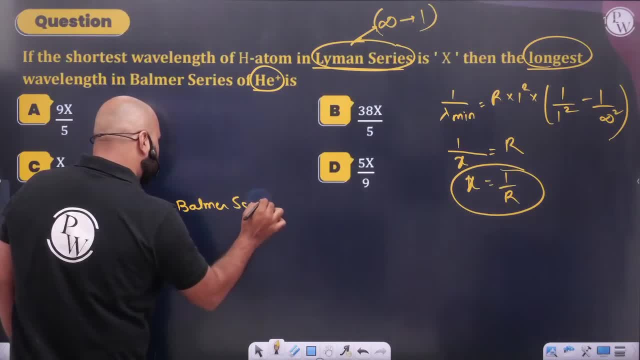 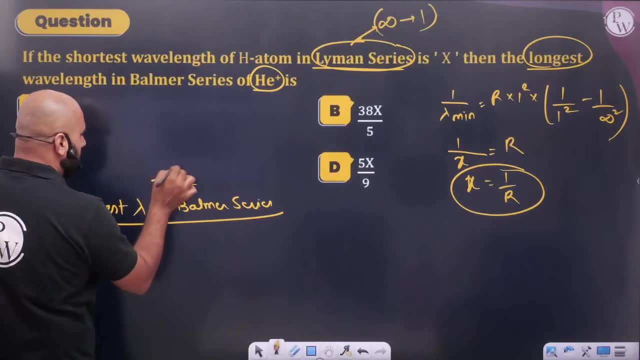 We will talk about the Balmer series. So when does the longest wavelength come? What will be the energy? It will be less. Energy will be less. That means from Lyman-Balmer series, from Lyman-Balmer. where will it come from? 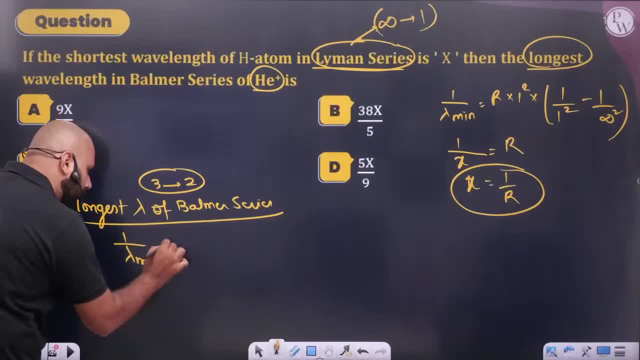 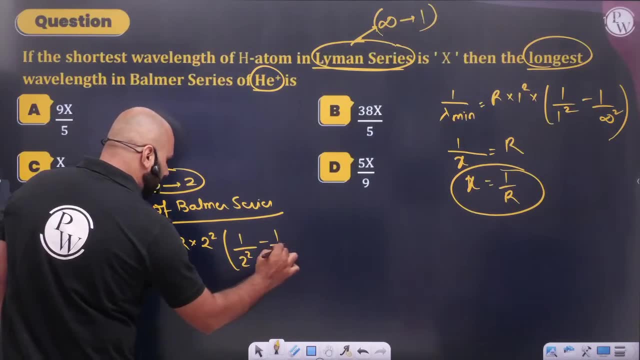 On 2.. So you want to get 1 by lambda max. That is R Z square. Z means square of helium, 1 by 2 square minus 1 by 3 square. We will solve. We have to get 1 by lambda maximum. 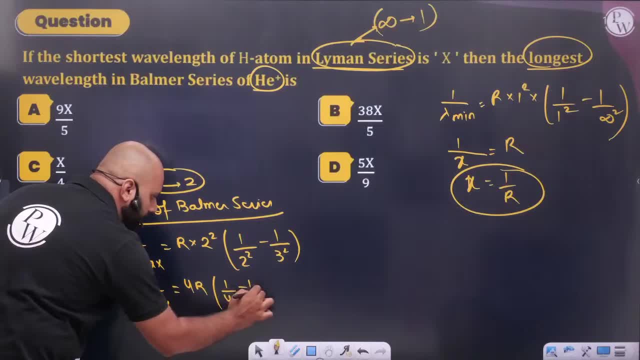 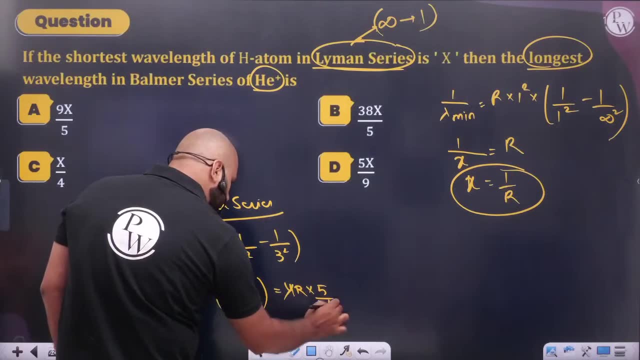 4R into 1 by 4 minus 1 by 9.. How much will you solve? We can write this 4R into 5 by 36.. That is 5 by 9.. What will be the lambda maximum? 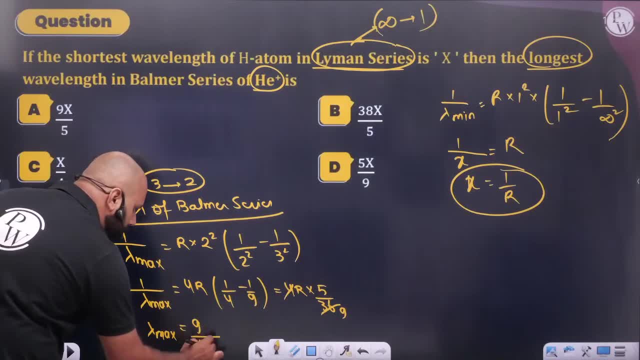 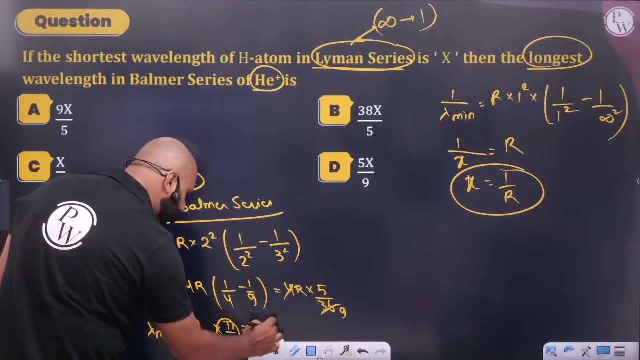 What will be the lambda max? 9 by 5 into 1 by R will come, And what is the value of 1 by R? What is the value of 1 by R? It is X, So 9 by 5X. 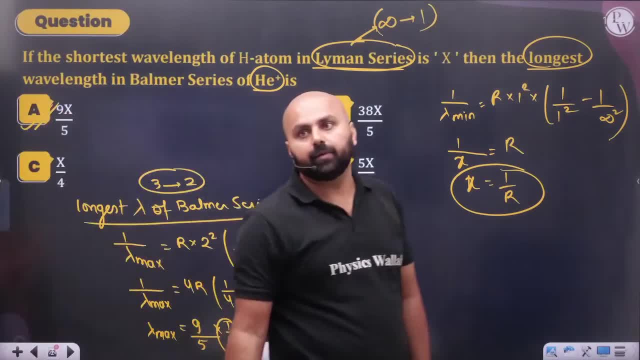 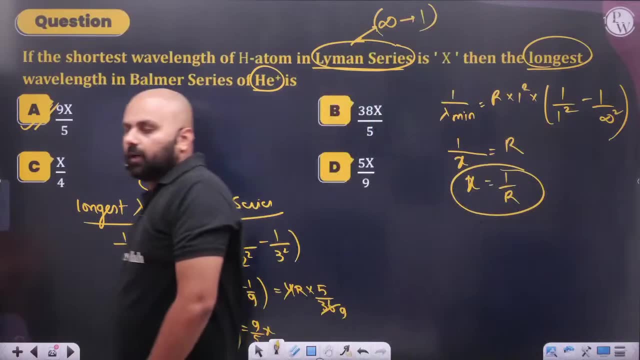 What will be the answer? 9 by 5X will come. 9 by 5X will come. So do it. 9 by 5X will come. Keep doing it, Keep looking at it. Okay, 9 by 5X will come. 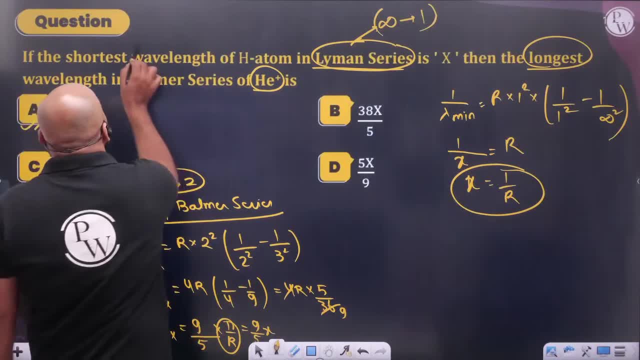 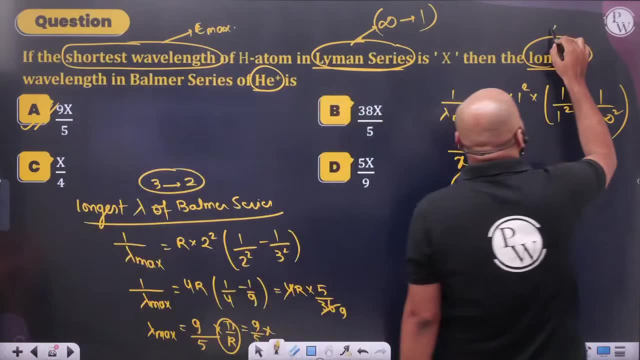 9 by 5X will come. 9 by 5X will come. Now see Shortest wavelength. Shortest wavelength means what should be the energy. Maximum should be Energy should be maximum. Longest wavelength means what should be the energy. 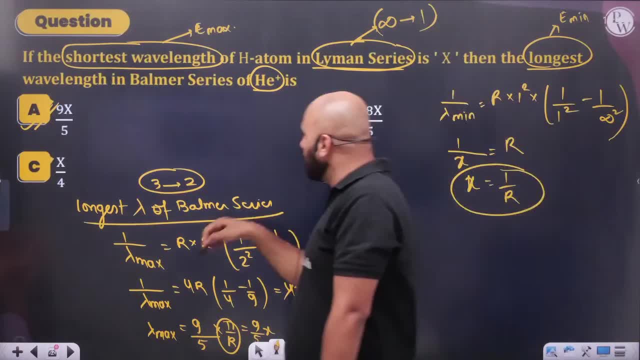 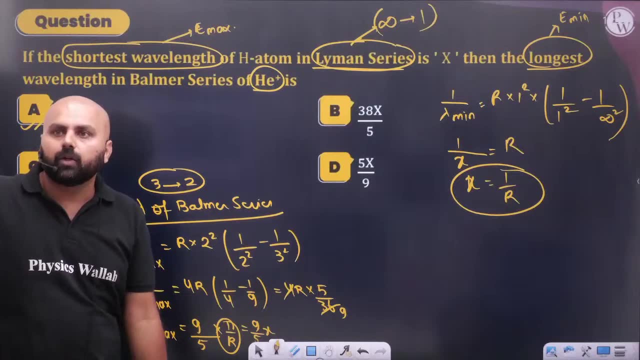 Minimum should be Energy. minimum means jump from the side. Maximum means jump from infinity. What happens from infinity? Jump. So keep doing it. These are the small things. Keep doing it. It has questions of Lyman series and Balmer series. 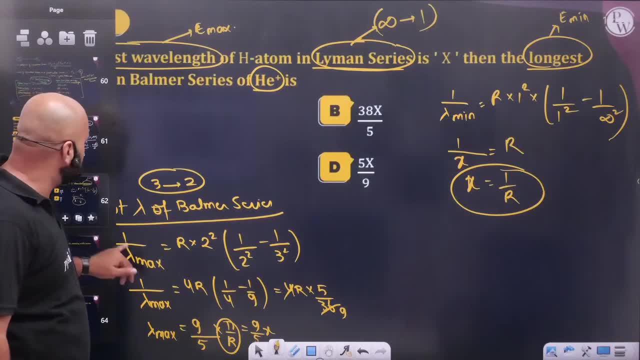 After that, see, If someone asks me that, Sir Balmer series and Lyman series. Sir Balmer series and Lyman series. If we talk about this, in Bohr's model, Hydrogen spectra is there. Bohr's model is there. 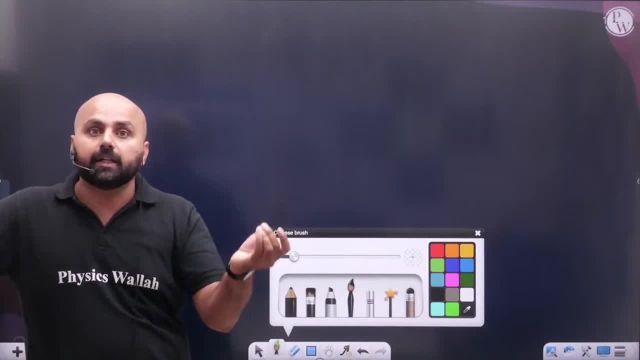 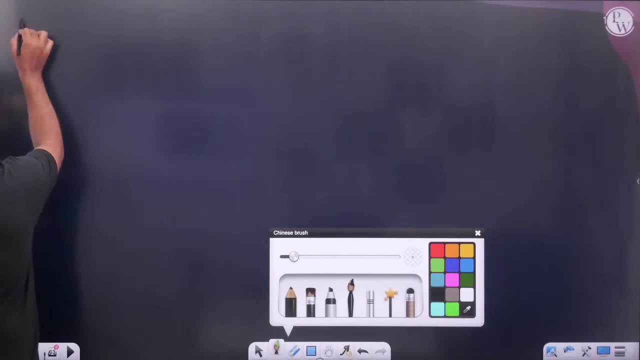 Electro energy velocity radius. these are the talks in Bohr's model. So before going to quantum mechanical model, from Bohr's model, who comes in our life in the middle? Who comes in our life in the middle? One comes De Broglie. 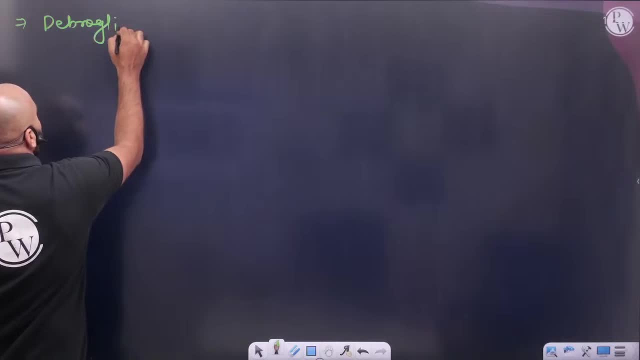 De Broglie's wavelength comes. De Broglie's wavelength comes. What does De Broglie say? That brother De Broglie has to say hypothesis. De Broglie is writing all the formulas of hypothesis together. Remember what is the formula of lambda? 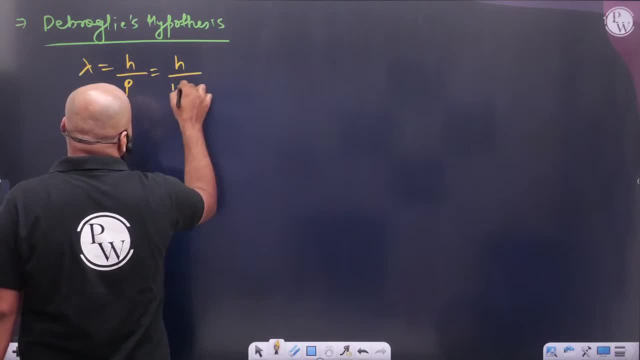 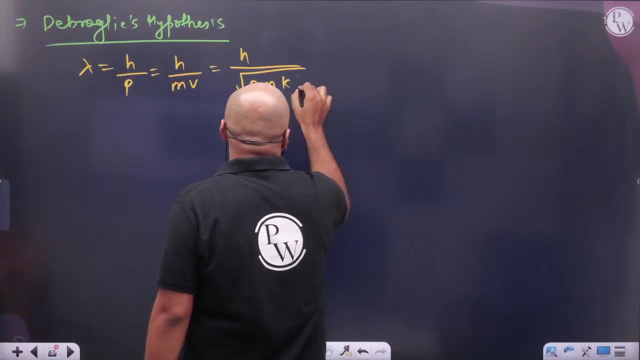 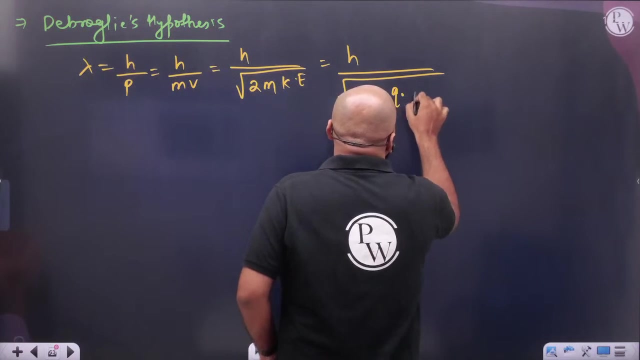 Lambda is nothing: h upon p or h upon mv, or remember this. We want to write this: h upon under root 2 times m into kinetic energy, or h upon under root 2 times m into Sir charge, q into stopping potential. This formula is completely of lambda. 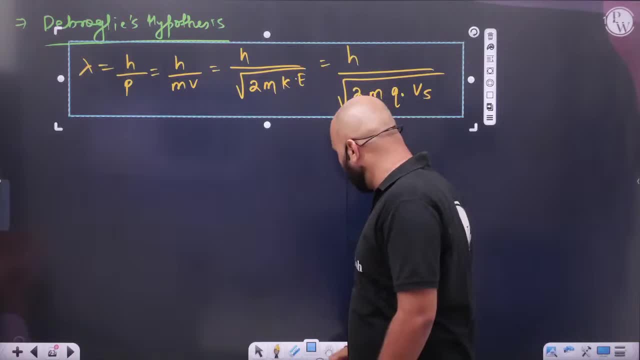 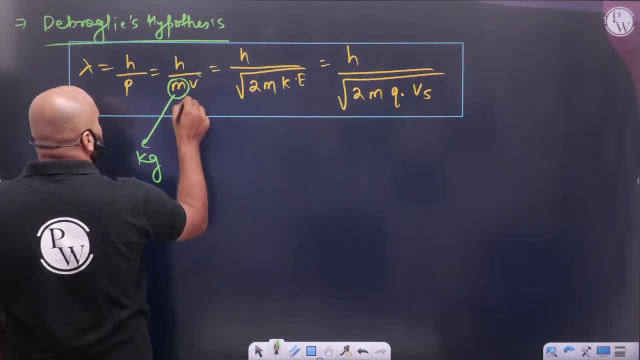 What is this lambda? So these are matter waves. Matter waves means anything. Remember here, Whenever you are putting the formula. So remember m, In which you have to put In kg And in which velocity you have to put. 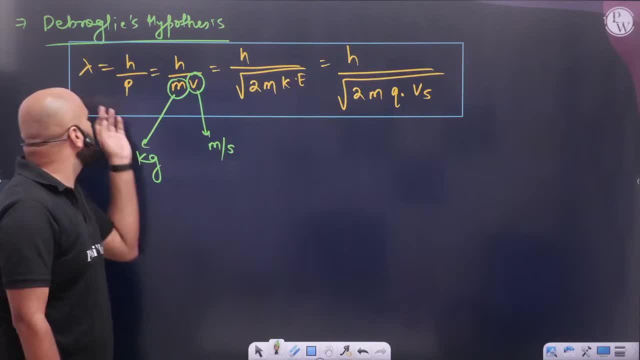 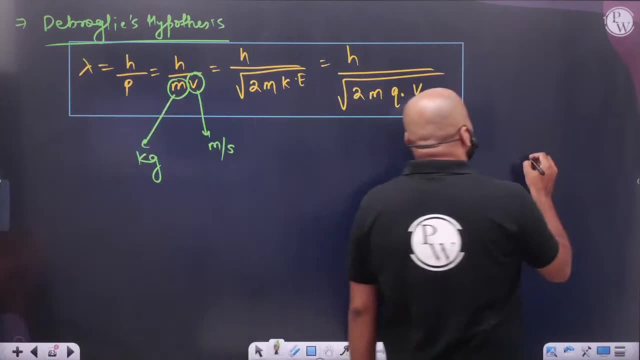 In meter per second, In kinetic energy joules. So remember, Lambda is directly proportional to, inversely proportional to momentum. What did De Broglie hypothesis say? That, brother, if any person moves, then inversely proportional to what will happen. 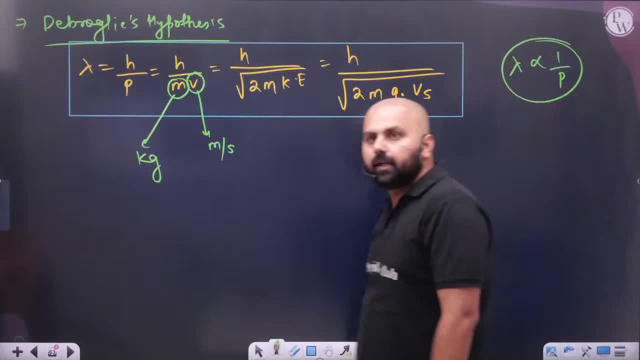 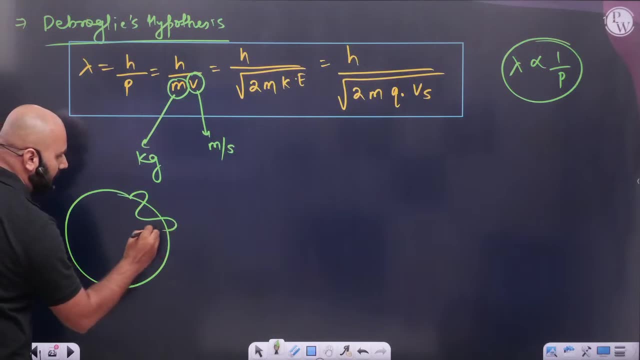 Momentum will happen. That's it. Keep this in mind. Keep this in mind. After that, one more thing: De Broglie had proved one more thing Which Bohr did not prove. What did De Broglie say? That, brother, the motion of electrons will be like this. 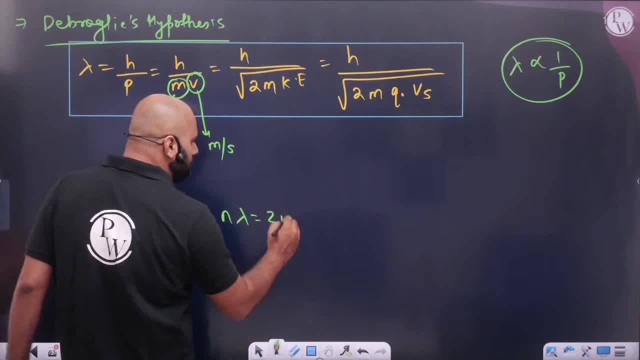 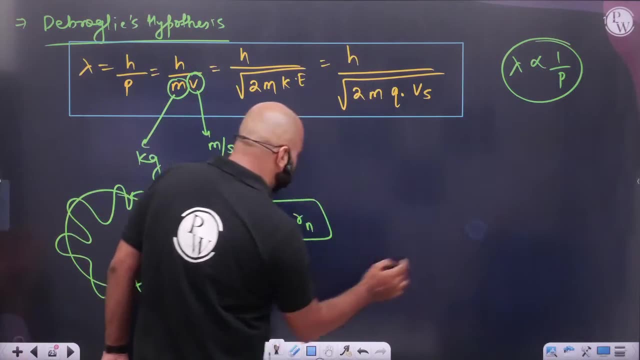 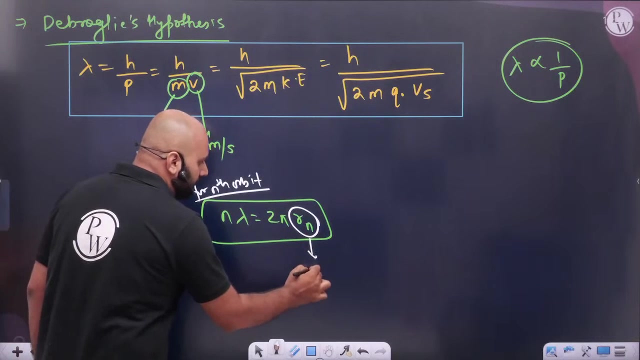 So here n lambda is equal to 2 pi r of radius of nth orbit. Remember n lambda. n lambda is nothing. 2 pi r of radius of nth orbit, n lambda for nth orbit. If you go to nth orbit then n lambda will be the radius of nth orbit. 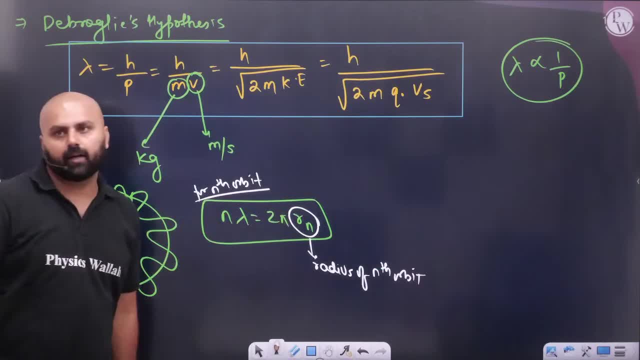 If you go to third orbit, then 3 lambda is nothing. 2 pi r into n- Okay. So 2 pi r n lambda will happen. So keep doing this. Okay, Keep doing this, It will happen. So pick this up with you. 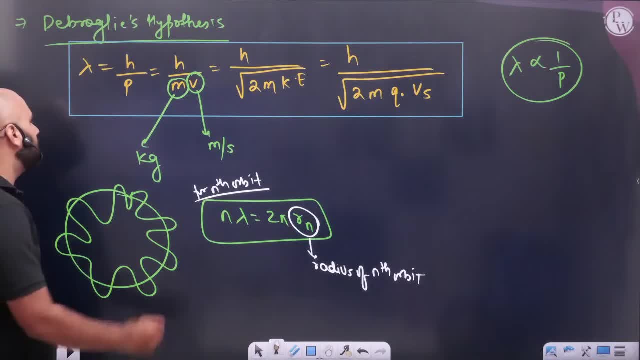 Do it. There is nothing in De Broglie hypothesis. Just remember: Whenever you put mass here, you will put it in kg. When you put velocity, you will put it in meter per second Second. Sir, who comes just after this? 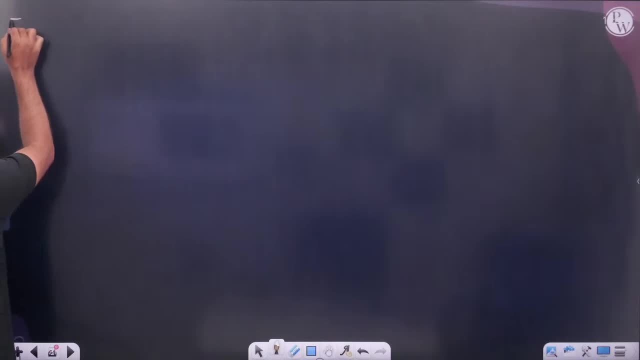 Heisenberg. Heisenberg said: brother, I don't care. Heisenberg, uncertainty principle. What does he say? Brother, you are saying wrong Those who do microscopy. Sir, you are saying wrong. Sir, you are saying wrong. 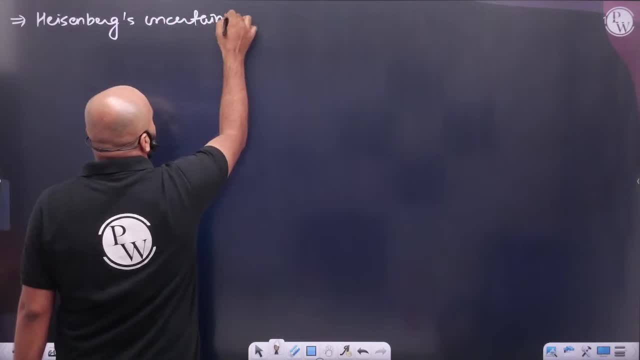 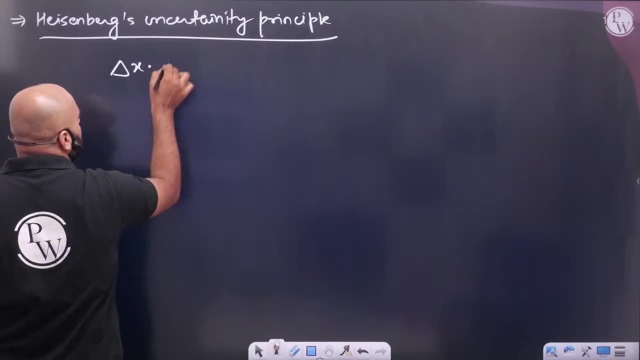 Sir, you are saying wrong. Whatever you do about these microscopic objects, no matter how much you do, you can't find their position exactly and in the same time you can't draw the momentum. Their value will always be more than h by 4pi. 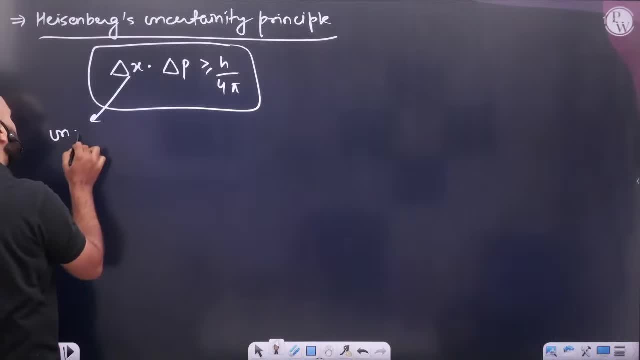 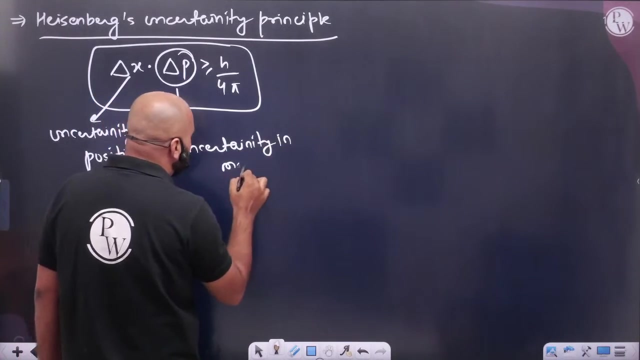 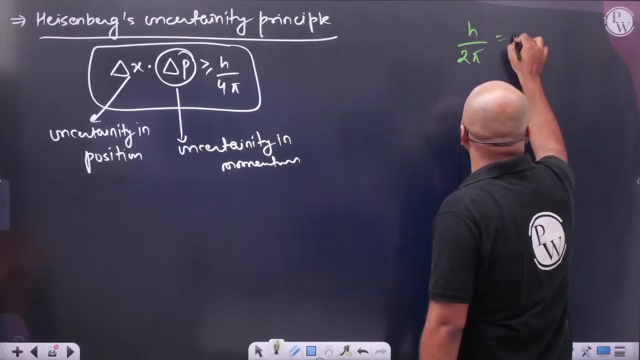 Uncertainty is uncertainty that will be inside the position. Uncertainty in position, Uncertainty in position And uncertainty in momentum. Uncertainty in momentum. What will this be? in momentum? it will always be greater than or equal to, or what we have called h by 2 pi is h bar. 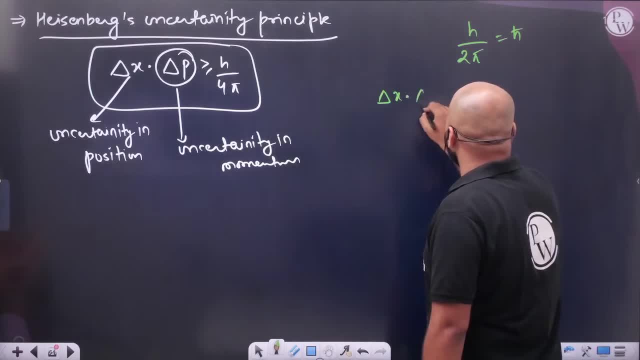 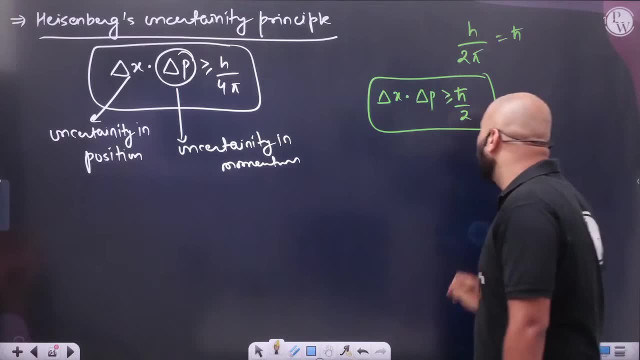 so remember it can be written like this too: delta p is equal to h bar by 2. if you get it like this too, then don't be scared. it has different expressions written like somewhere. it can happen that delta x- the change in momentum- will come due to delta v. 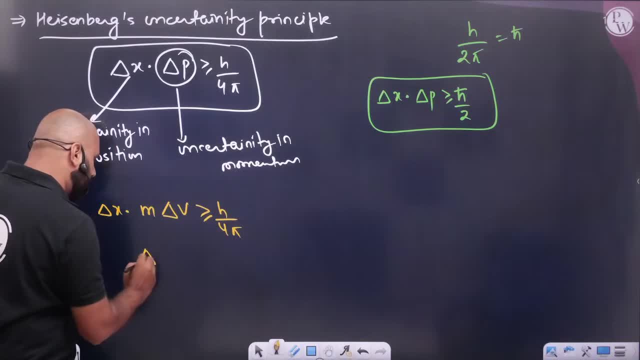 so h upon 4 pi. somewhere. it can be written like this too: delta x into delta v, h upon 4 pi m. this formula can also be obtained somewhere. it can happen that, sir, let's do one thing, let's do one thing. we know the momentum. 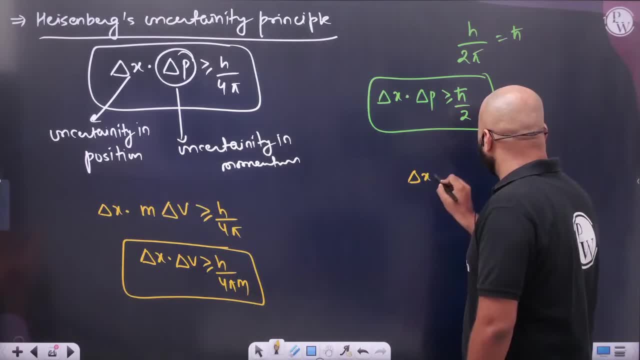 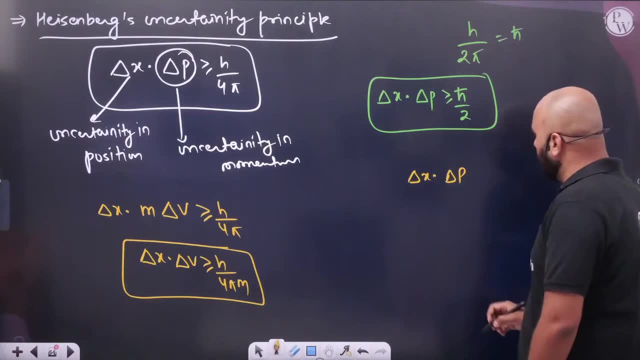 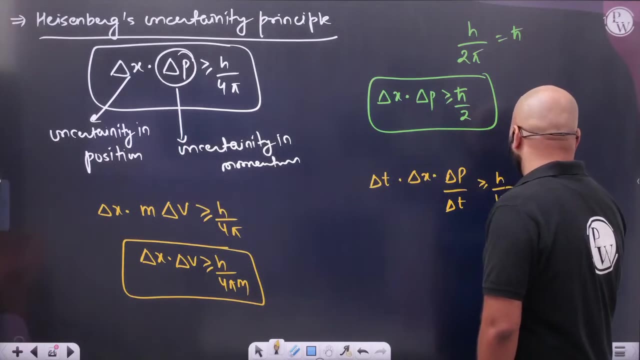 so what do we do? delta x into delta p? let's do one thing. delta p: we know the momentum. so what do we divide the momentum by time and multiply it? what do we divide by time that is equal to h upon 4 pi force? what is momentum by time? 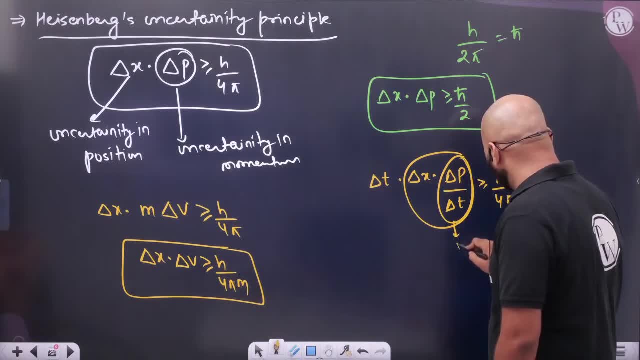 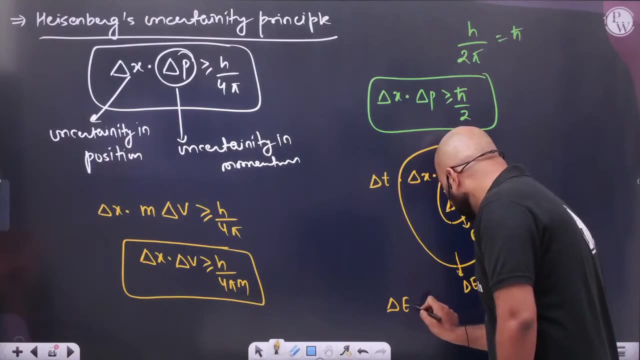 force. what is force into displacement? what is this force? what is force into displacement, energy? so let's see how we are doing. what is this force? force into this, one is known as energy. so we can also write a formula: delta e into delta, t, h upon 4 pi. 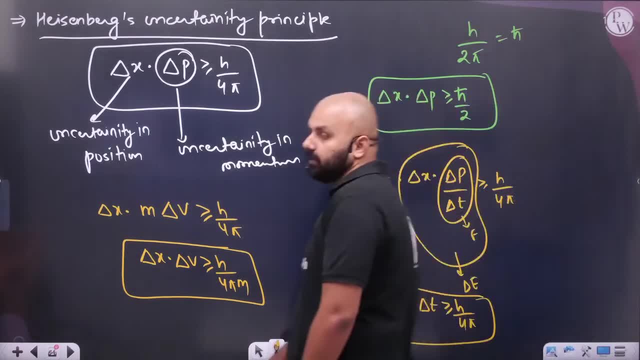 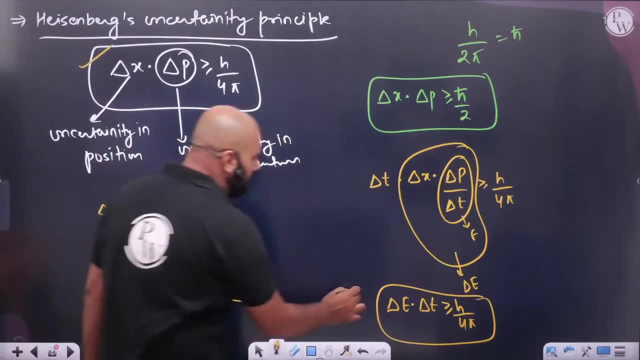 we can also use this formula for this, for Heisenberg's uncertainty principle. so let's get this answer now. there are different expressions like this: this expression, this expression, this expression: whatever is given in the exam, it can be given in the exam hall. this expression: pick it up. 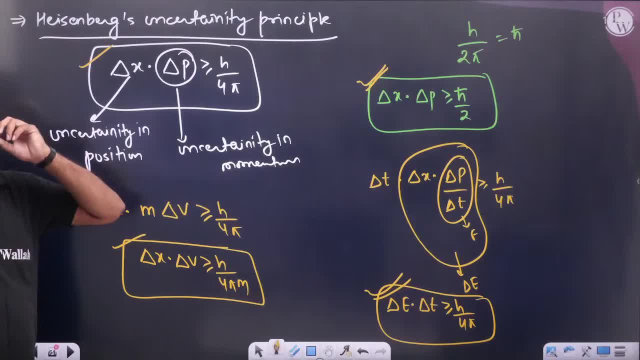 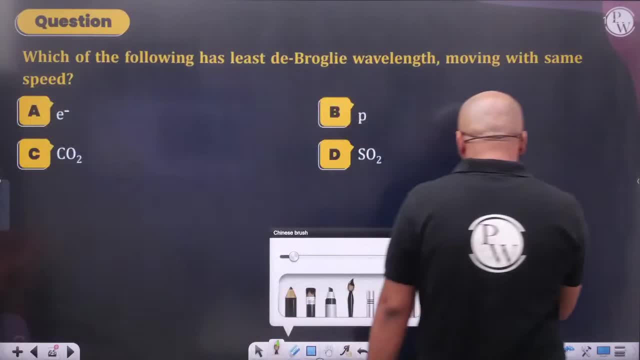 keep doing angular, momentum, momentum positions, uncertainty will always be greater than this. ok, see this. someone asked me, sir, how this question will be de Broglie wavelength. what is de Broglie wavelength, sir? it is the same speed if the speed of de Broglie wavelength is same. 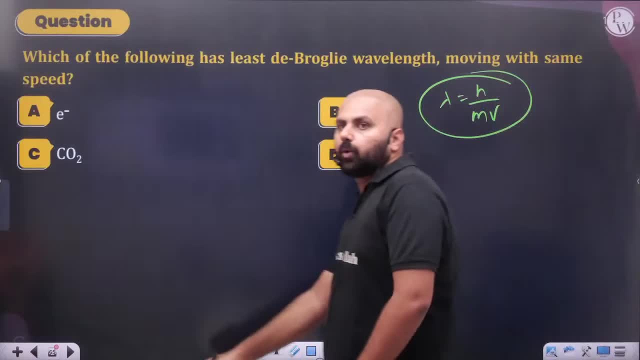 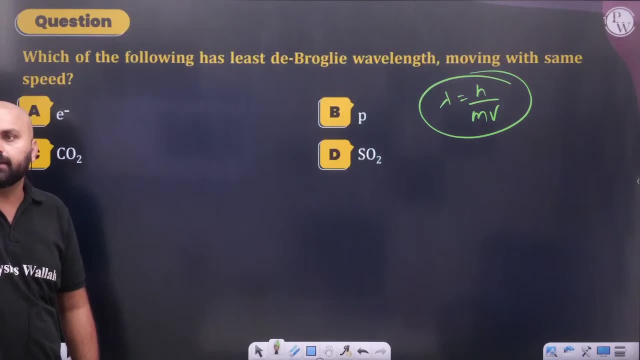 then on which will it depend? people who are studying quickly. tell the answer: de Broglie wavelength. if it is the same speed, then on which will it depend? on which will it depend? quickly? tell the answer fast. what will be the answer to this? what will be the answer to this? 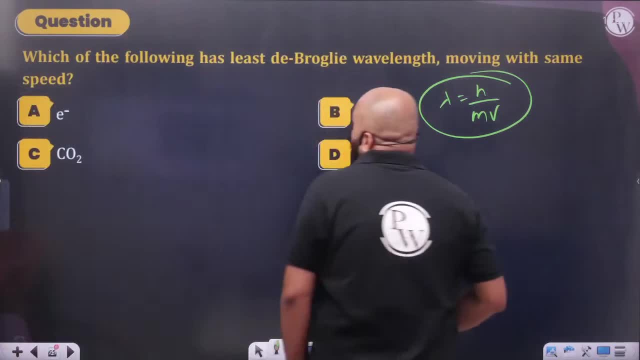 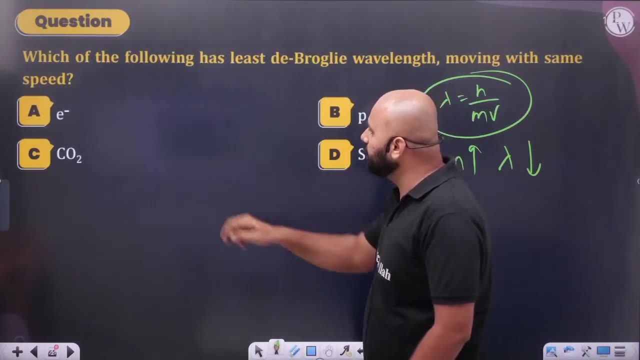 what will happen? obviously, whose mass, whose mass will be more. if the mass increases, then what will happen? wavelength will decrease. electron is given, proton is given, CO2 is given, SO2 is given. what is the mass of SO2, the maximum? if the mass of SO2 is more? 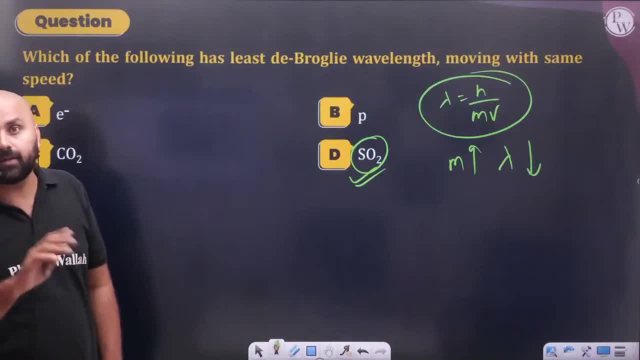 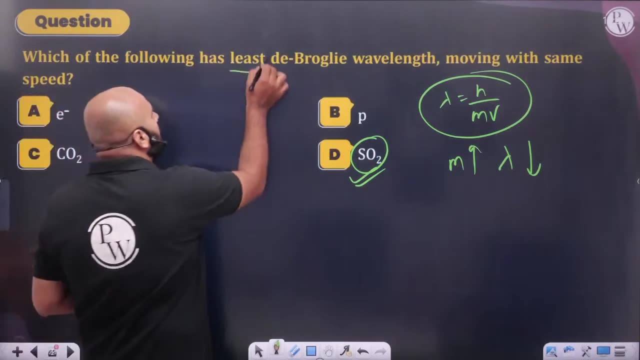 then what will happen to its wavelength? it will decrease. see carefully. now many people are giving one answer: whose mass will be more, then its wavelength will decrease. sir, you are thinking the opposite. list is said. list is said. see, this is what they are saying in exam hall. 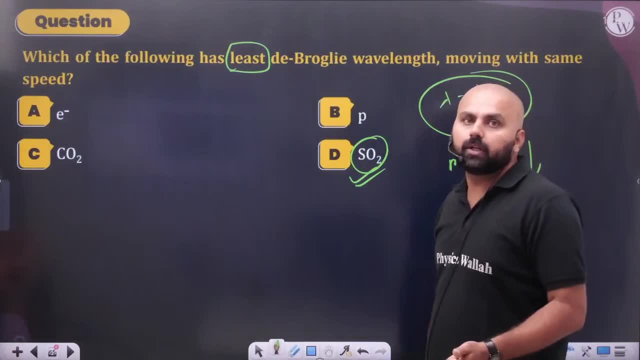 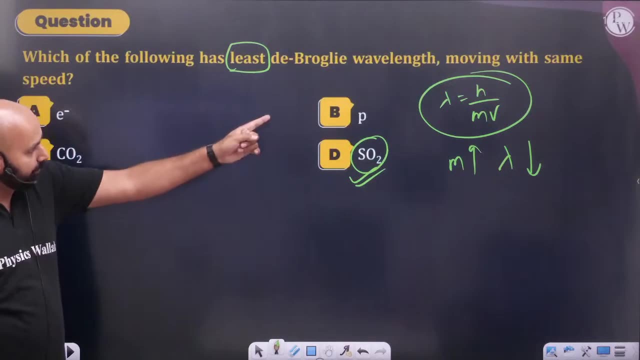 you don't have to make this mistake. you don't have to make this mistake. you all see here. only some people gave the first option in exam hall. everyone can make this mistake. try as soon as you do on mass: mass increased, wavelength decreased. I want a list. 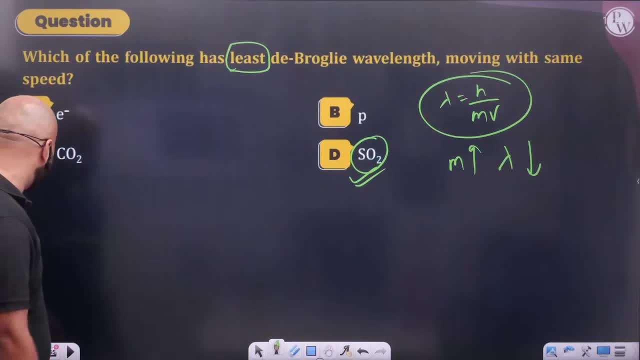 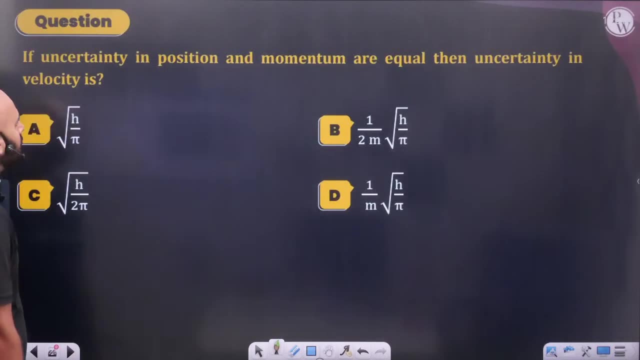 so obviously we need mass. whose mass is more SO2? whose mass is more SO2? see this question. uncertainty in position is given and momentum are equal means. delta x is equal to delta p. I am being told, sir, tell me the velocity delta x into delta p. 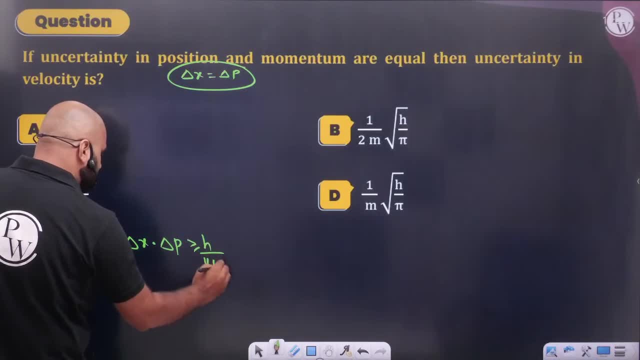 see this. we have very correct question. h upon 4 pi, sir. what can we write? delta x, delta v, m. what can I write, sir? delta x, what can I write delta p, delta p into delta p greater than h upon 4 pi? so what happened? m, delta v. 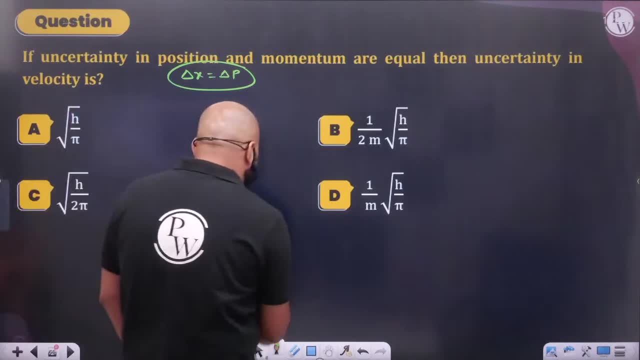 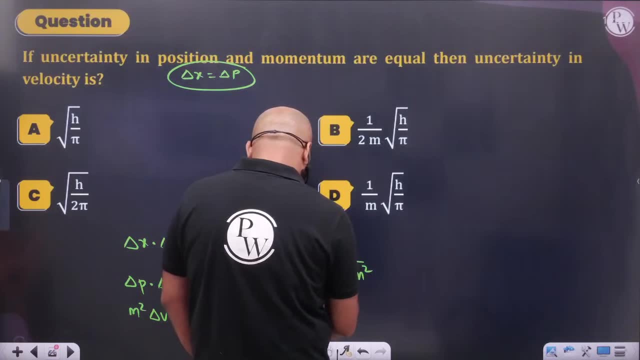 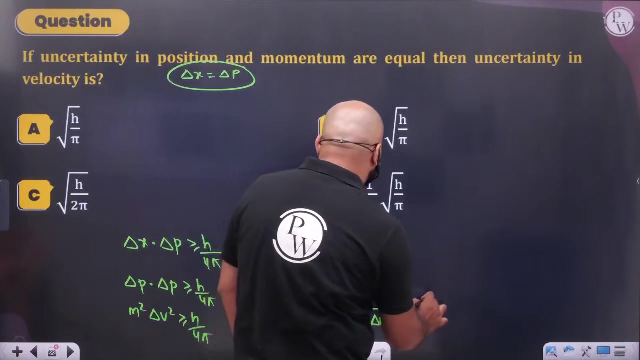 m square. delta v- whole square. that is equal to h upon 4 pi. see from here what can I write? delta v, whole square. h upon 4 pi. delta m- whole square. delta v under root: h upon 4 pi. sir, delta m is being written bhai. 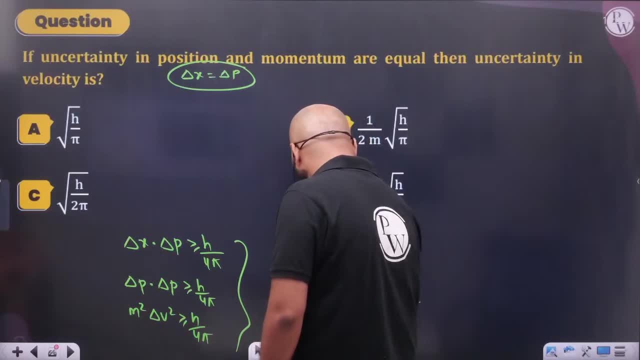 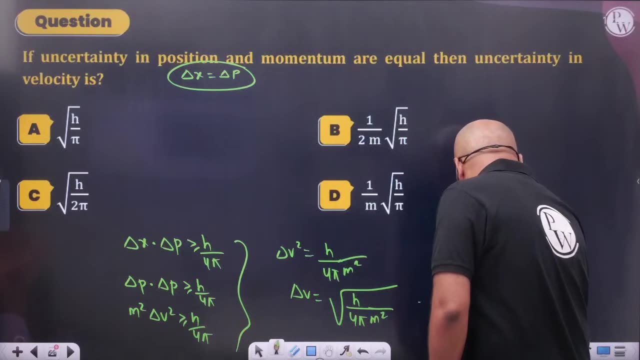 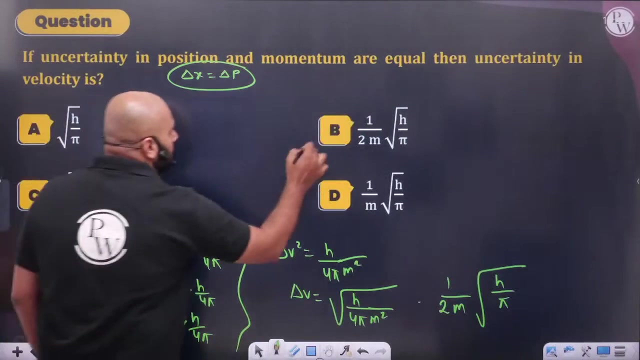 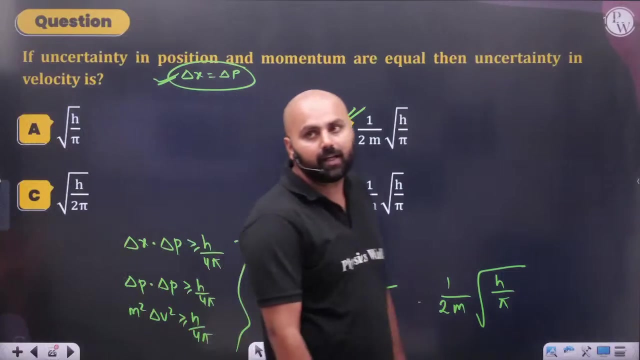 v delta m r. what is delta m write s c m m r, v m m M s M is delta M. what delta m wr? so see this: 4 pi m witch 1, 4, 4, 2 m, 2 n. below what have to see the question yourself. Yes, these are the questions. I will have to think like this: 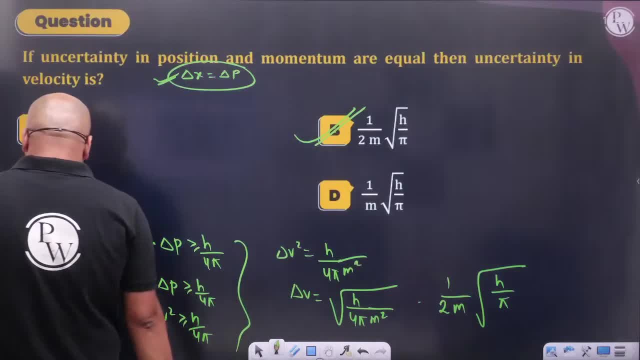 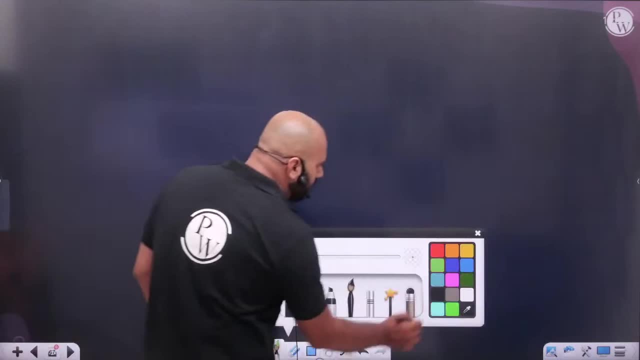 I will have to do like this. Okay, Look at this brother, Look at this. Now quantum numbers. come on Schrodinger equation. Let's talk about Schrodinger equation. Let's see Schrodinger equation. What was the Schrodinger equation? It comes on Schrodinger equation and quantum. 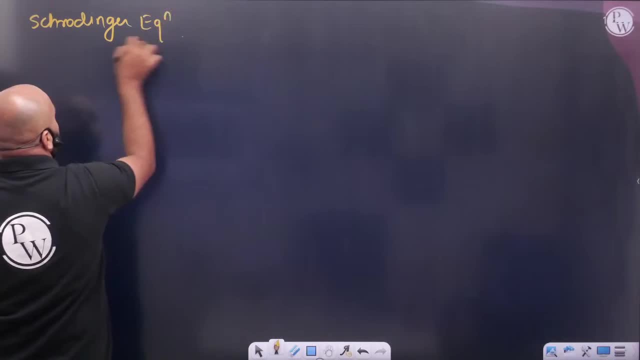 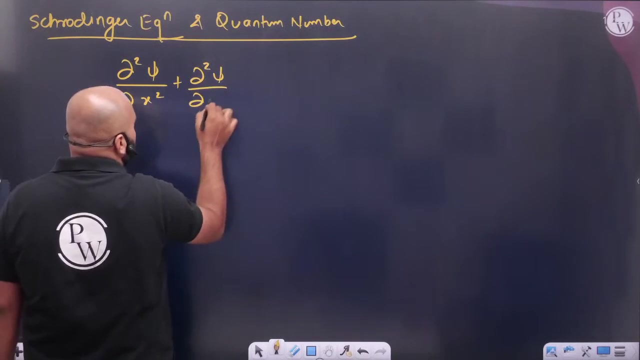 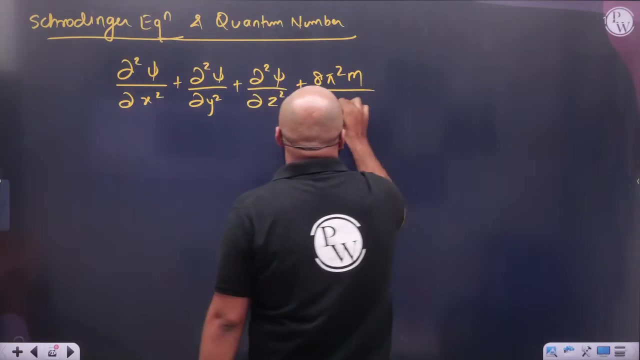 equations, Schrodinger equation and quantum numbers. Let's see what the Schrodinger equation was. So nothing Del square psi upon del x square plus del square psi upon del y square plus del square psi upon del z square plus 8 pi square m upon h square e minus v into. 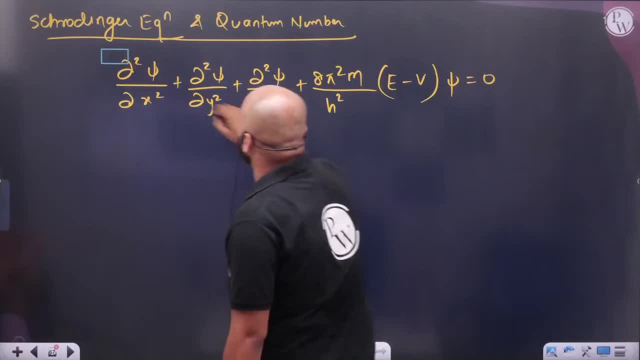 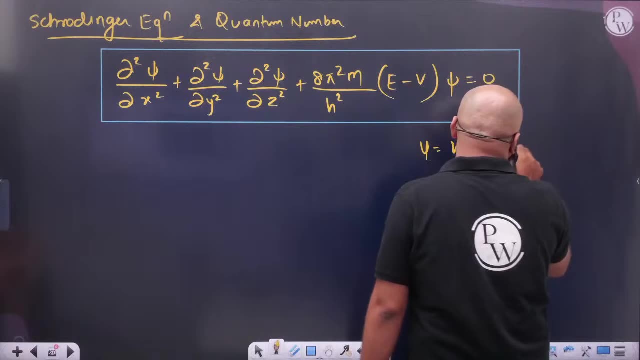 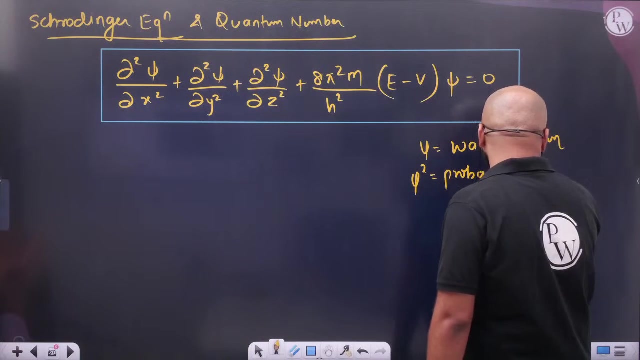 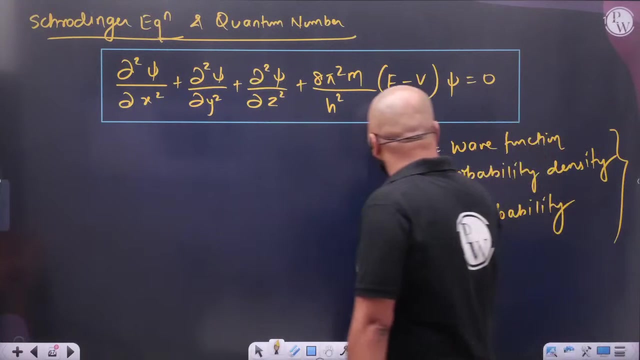 psi is equals to 0.. This is my Schrodinger equation, Where psi represents the wave function, The psi square represents the probability density, The probability density represents the probability density and psi square into dv represents the probability. This is all you need to know for now. The psi and psi square are obvious. You don't need to go into. 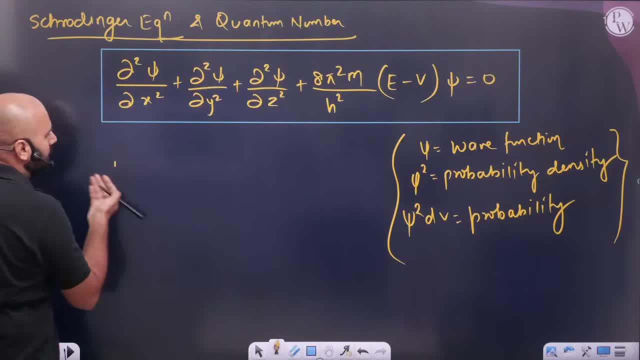 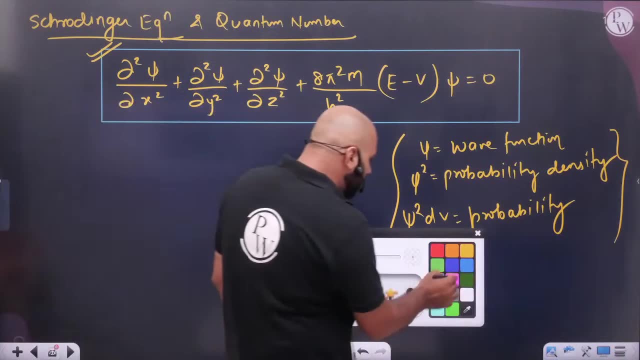 that, If you look at it according to Schrodinger, Schrodinger wrote the equation that, brother, if there is any electron, then it fluctuates in different axis, like this. So this is the equation, Sir. the second thing: what did Schrodinger say here? that you will solve this equation? 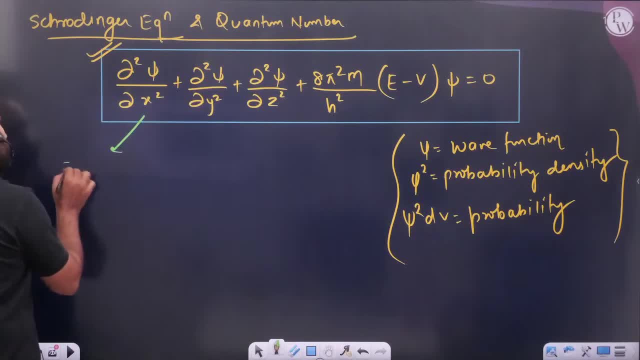 If you solve it, the solution of Schrodinger will come out In your syllabus. the solution means it is not written to solve The solutions that will come from Schrodinger. the solutions of Schrodinger equation are represented like this: The value of psi is nlm Three quantum. 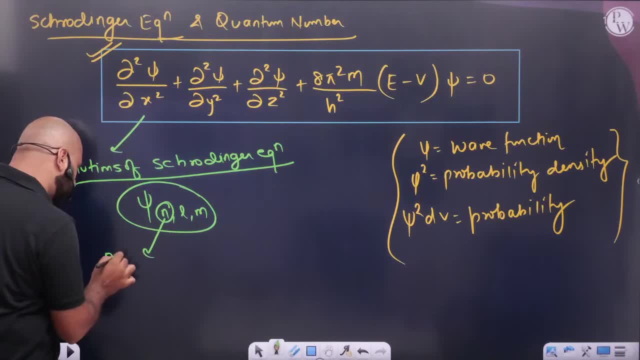 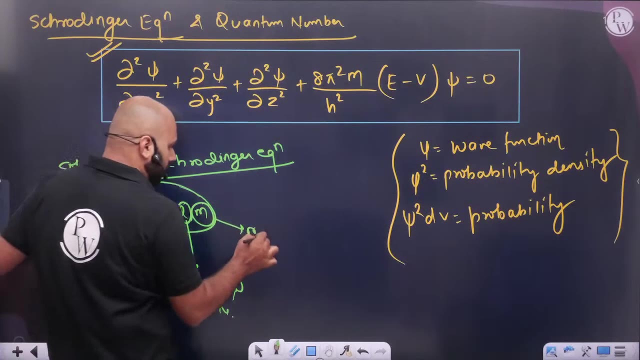 numbers come out. Where n is known as principal quantum number, n is known as principal quantum number, L is known as Sir as a principal quantum number, n is known as as a principal quantum number and we have m is known as magnetic quantum number. What did we say? m is called. 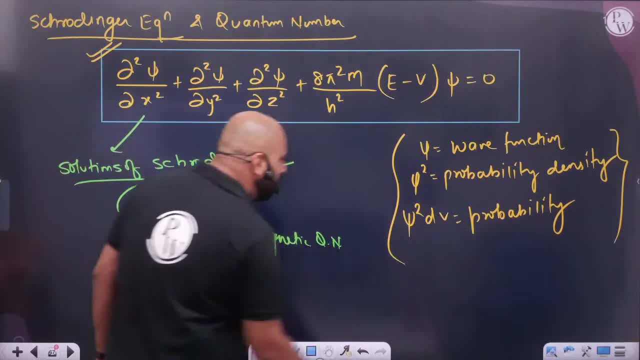 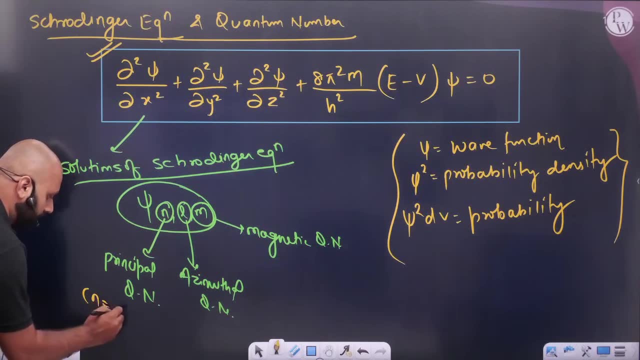 Magnetic quantum number. Sir. see this. with this, the limitation came with it. Sir, the value of n will always be 0,. sorry, I am telling the value of n is 0.. What will be the value of n, 1,, 2,, 3,? DOS does, does The value of L? from where does it happen sometimes? from zero to n minus zero. Sir, this value of n is always 0.. Sir, this value of l is always 0,. do you understand, Sir? this value of l is always 0,. D-D-D-D. Sir, this will always signify the. 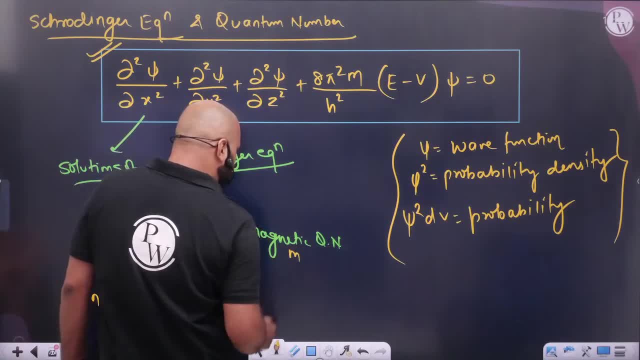 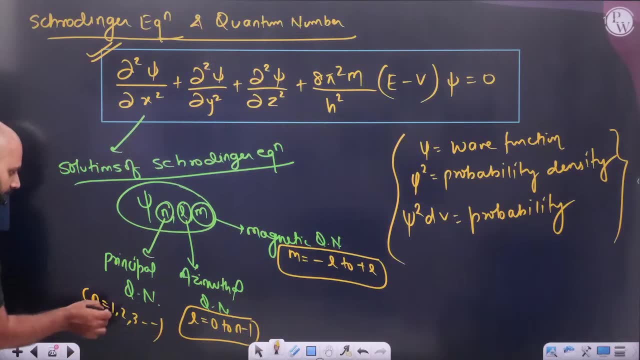 value of n as the value of n, which is the minimum number of m. Sir, this is the number of m, Sir, this value of l is always, And the value of magnetic quantum number M will be minus L2 plus L. Meaning, Sir, L depends on N and M depends on this. 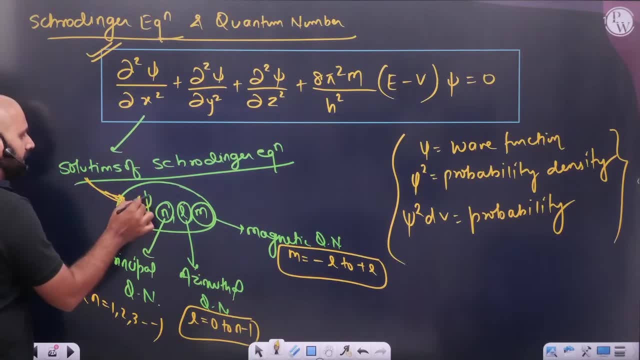 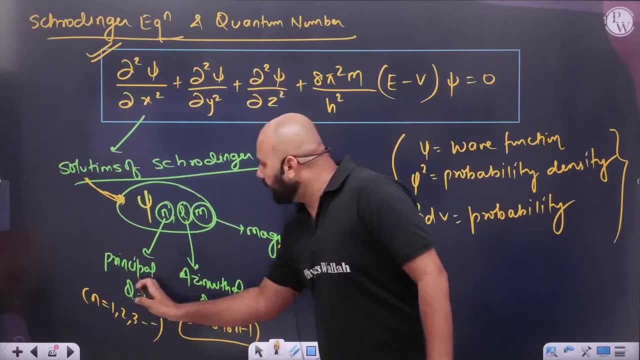 So in solution we got three values of psi from Schrodinger's wave equation. We got three values of psi: N L M. Okay, N L M First one is principal quantum number whose value starts from N, 1,, 2,, 3,, 4.. 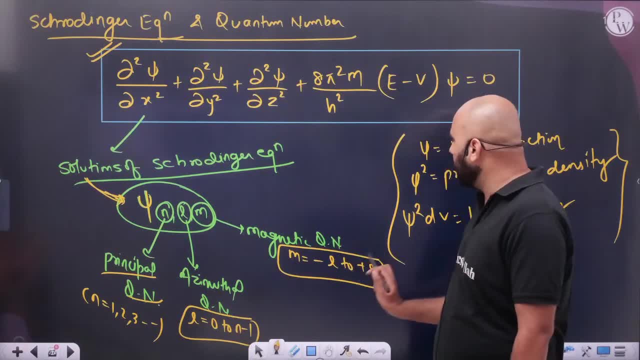 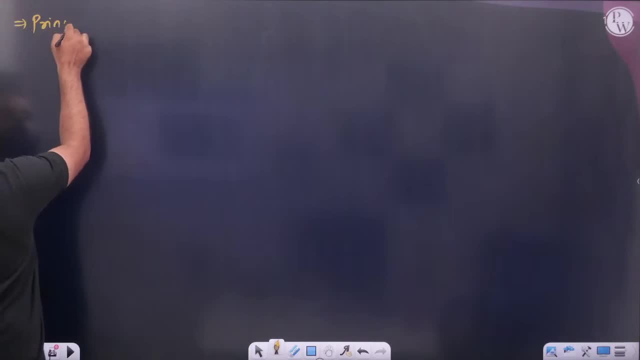 As usual, quantum number L is from 0 to N minus 1.. Magnetic quantum number is from minus L2 to plus L. Sir, if we talk about quantum number, then first of all the principal quantum number comes. If we talk about the principal quantum number, then see who does it represent? 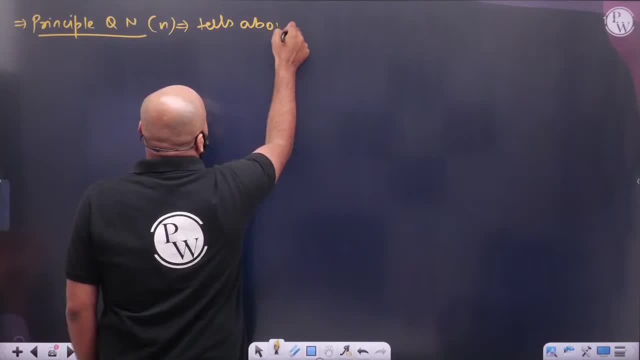 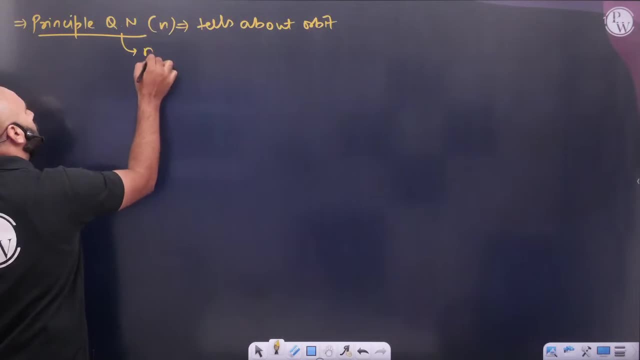 Who does it represent? It tells about cell. Who does it tell about? It tells about orbit. It tells about orbit Meaning. it will tell about the orbit in which it is. Sir, the value of N can be anything: 1,, 2,, 3,, dash, dash, dash. infinity can go. 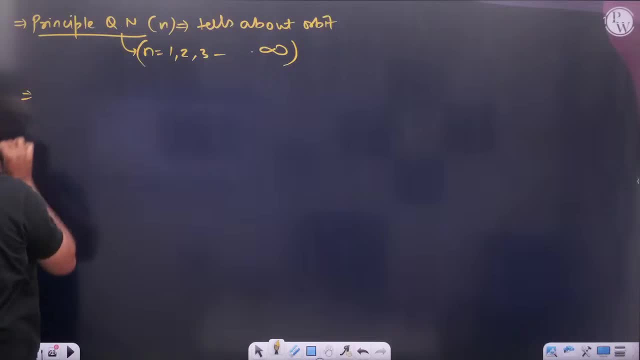 There is no tension, Sir. there is no tension From this. you were also taking out Bohr's orbit. Okay, whatever you are taking out, M V R is equal to N H upon 2 pi. Whatever you are using, who does N belong to? 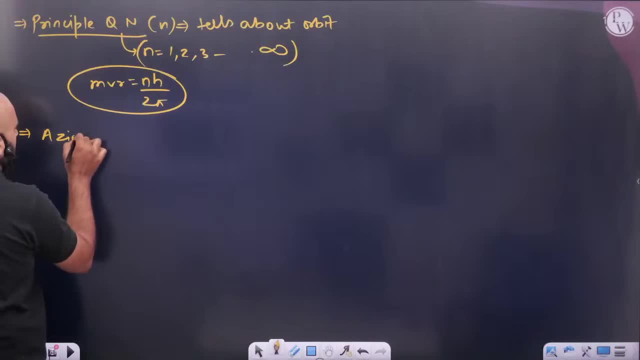 It belongs to this, only Then. who does it belong to Asimuthal quantum number? Actually, asimuthal quantum number is a little different from quantum number. What Asimuthal quantum number is L? Who does it tell about? 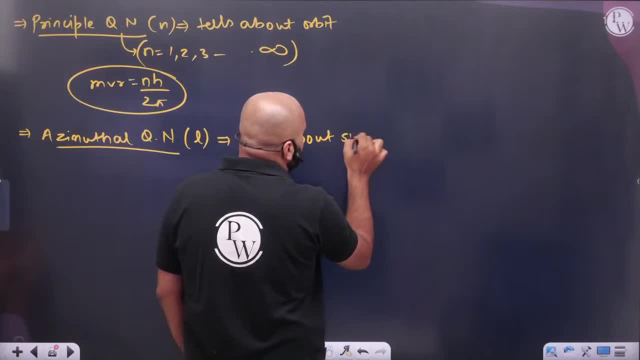 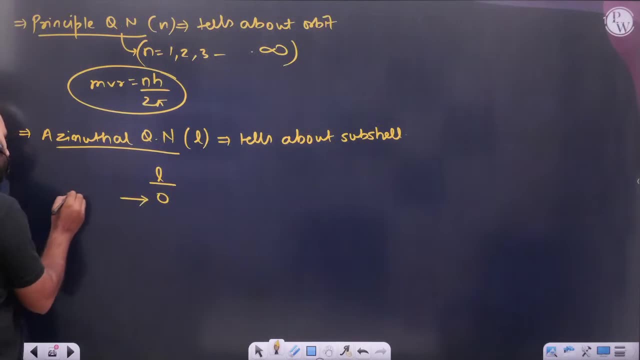 It tells about subcell. It will tell about subcell Meaning. you go inside the cell subcell. You will see the value of L. If it is 0, then which subcell is there? It is S subcell. 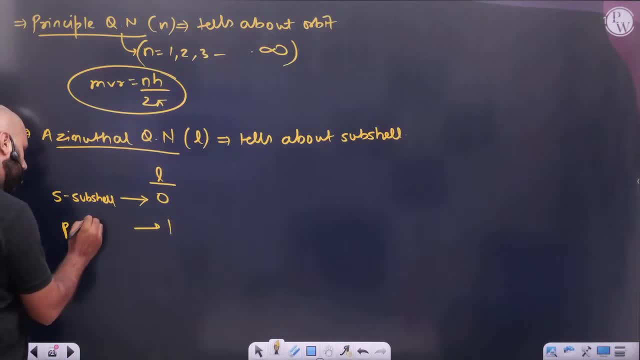 If the value of L is 1,, then P subcell is there. If the value of L is 1,, then P subcell is there. If the value of L is 2, then what will happen? D subcell will be there. 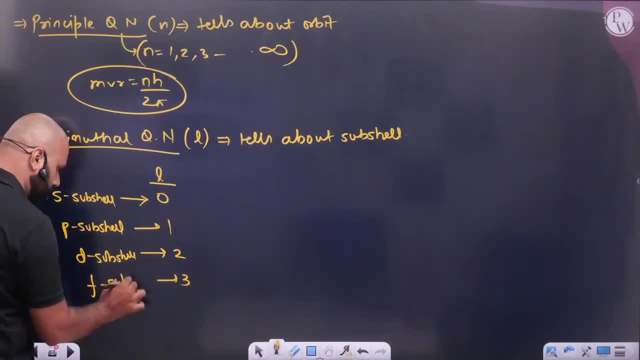 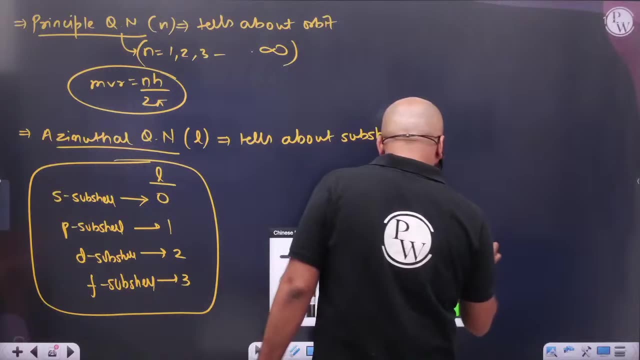 And if the value of L is 3, then what will happen? F subcell will be there. So, by doing this, S P, D and F, Who will tell this Asimuthal quantum number From which? from where does the value of L go? 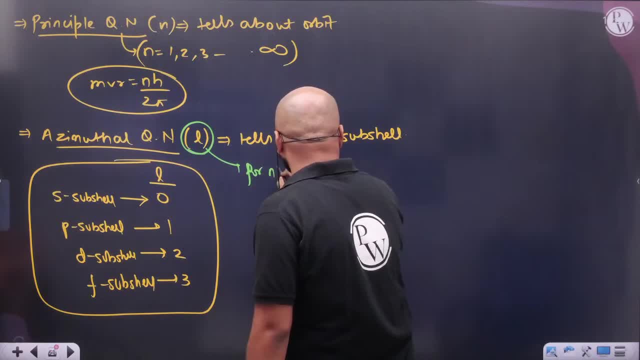 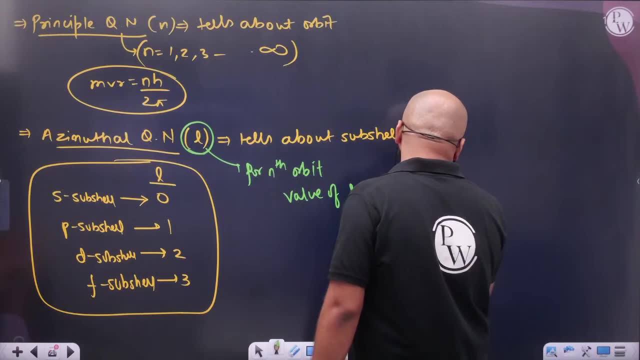 From where does the value of L go For an orbit, an earth orbit? If we go to an orbit, then the value of L, the value of L will be from 0 to n-1.. The value of L will be from 0 to n-1.. 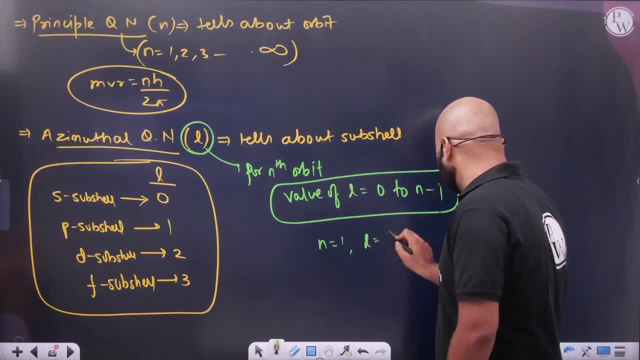 Meaning: if n is 1, then what will happen to the value of L? 0 means 1S. If the value of N is 2, then 2 values of L will go 0, L's value is 1.. 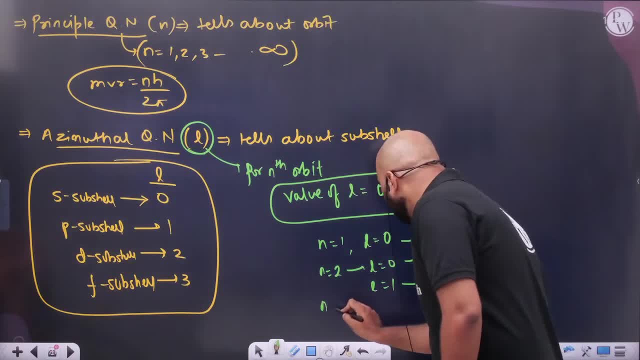 This is 2S. What will happen? This will be 2P. If the value of N is 3,, then what will happen, Sir? the value of L is 0.. L's value is 1.. L's value is 2.. 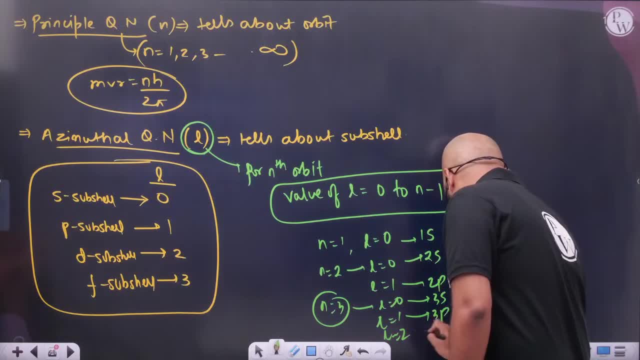 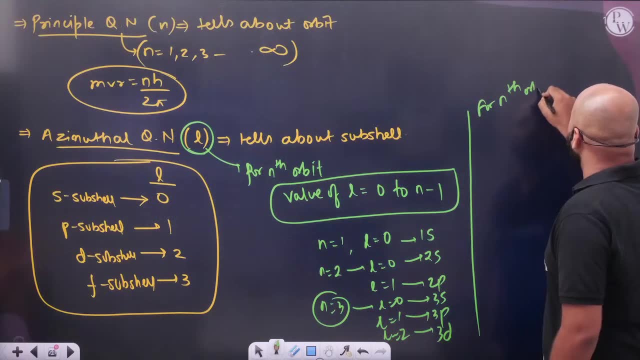 What will happen 3S? What will happen 3P? What will happen 3D? So do it like this and take it out. Meaning here is a simple: for nth orbit. remember, for nth orbit. 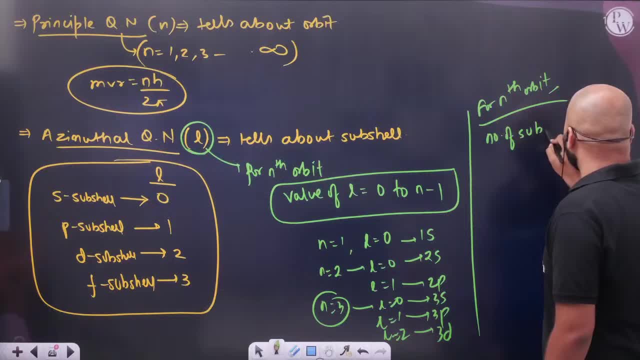 the number of sub-cells will be. the number of sub-cells will be how many possible will be. its direct formula is n, Because how many sub-cells are there in the first orbit, 1.. In the second orbit, 2.. 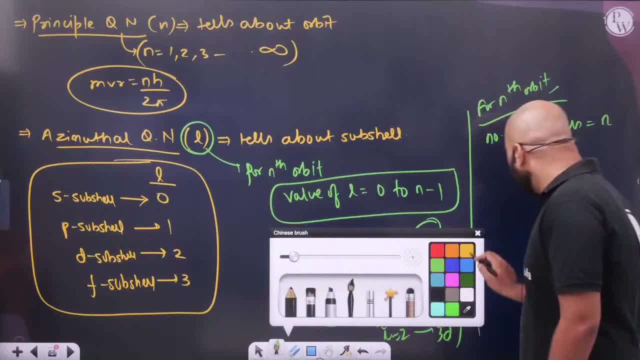 In the third, orbit, 3.. So do it like this and go Go on Here. I will write all the formulas as well. The number of orbitals will be. so if we talk about orbitals, then n square will be. 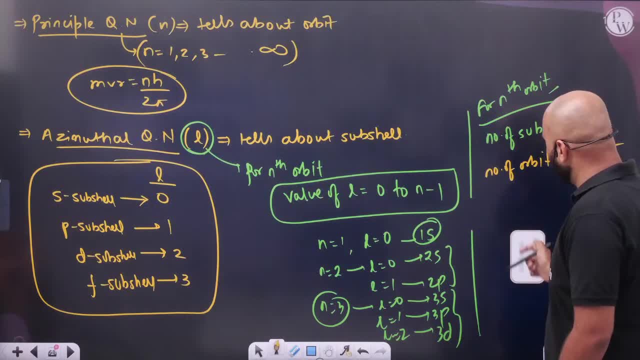 number of what will be the maximum number of electrons. I will write all this on here: What will be the maximum number of electrons? So what will be the maximum number of electrons 2n square If we go to any orbit? 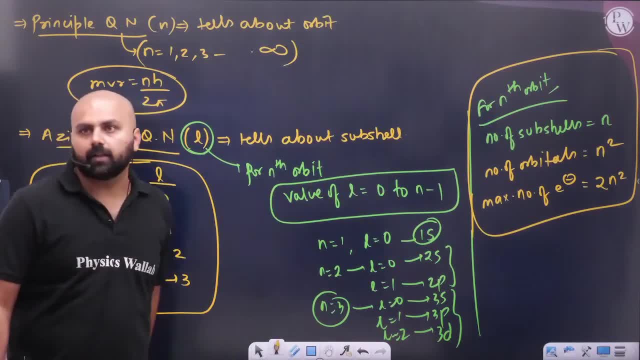 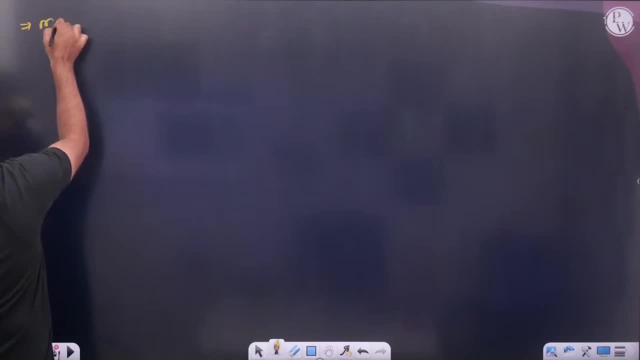 then you get this. If we go to any orbit, then these things come. Now, these are simple things. Just keep revising the formula together, Then we will see. One last thing: we have magnetic quantum number. What does magnetic quantum number say? 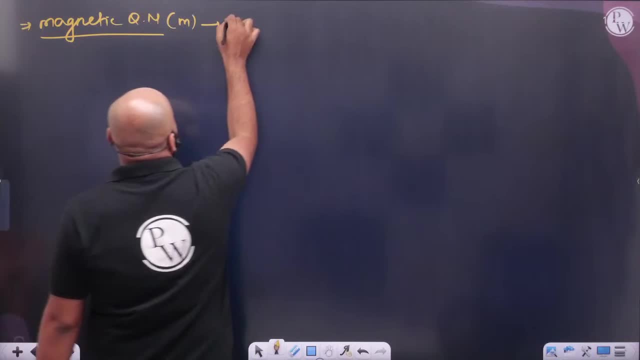 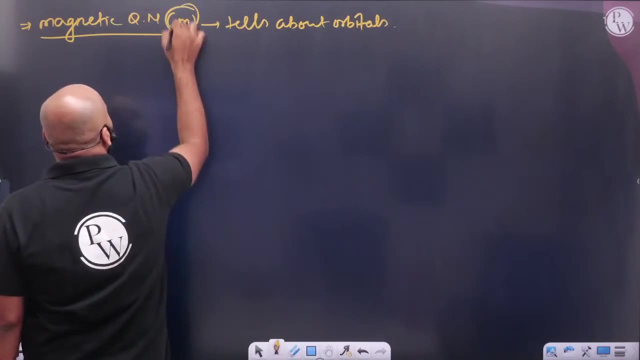 Sir, magnetic quantum number m. what does it tell about? So, what does it tell about About orbitals? What does it tell about About orbitals, Sir? its value, what is the value of m From minus l to plus l? 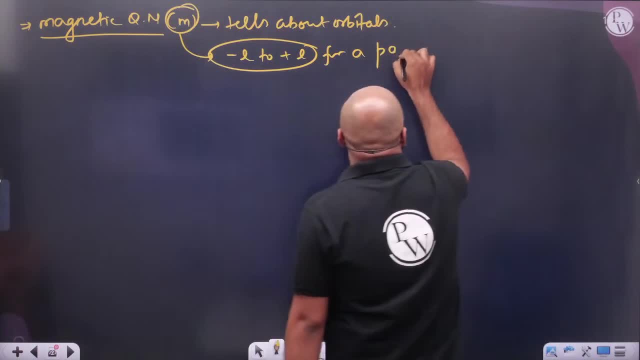 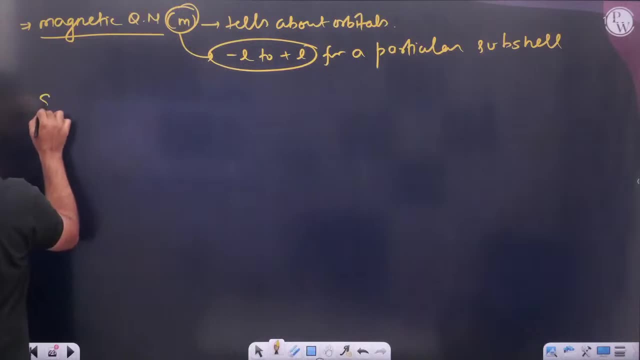 Keep in mind for a particular sub cell. Each sub cell will be different. Remember this thing. I have made it the same for all. Each sub cell will be different. This is S sub cell In S sub cell, if you see. 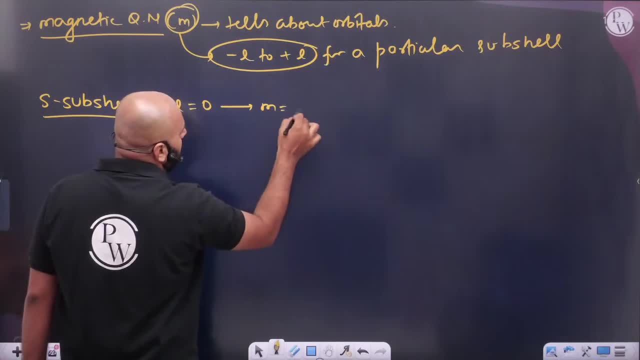 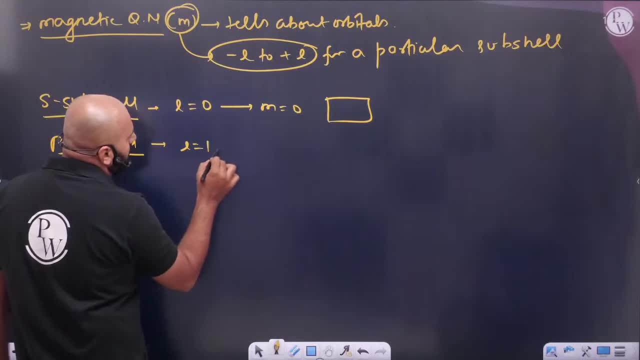 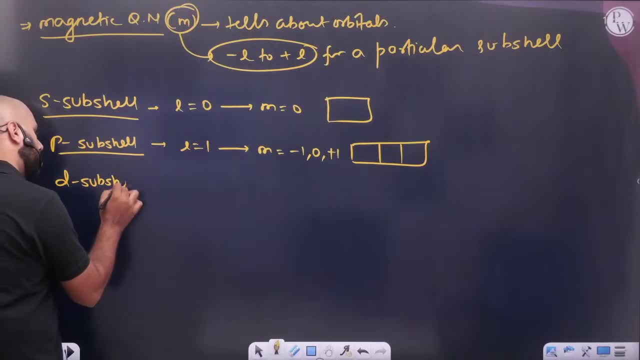 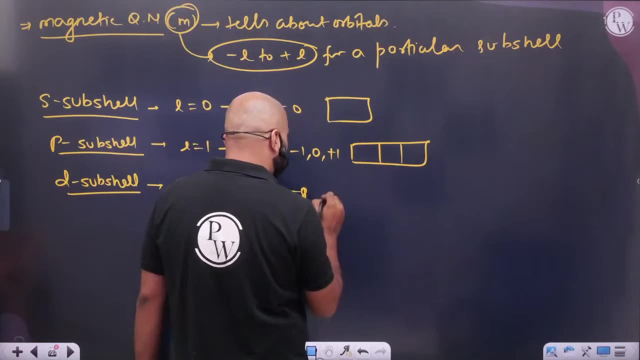 Similarly, if you talk about D sub cell, then in D sub cell what will be the value of L 2.. What will be the value of M Minus 2, 0,, sorry, minus 2, minus 1, 0, plus 1, plus 2.. 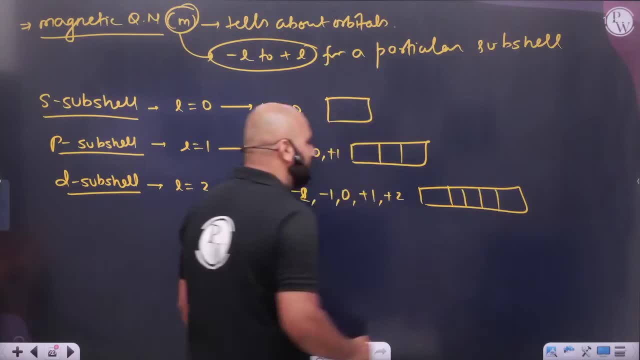 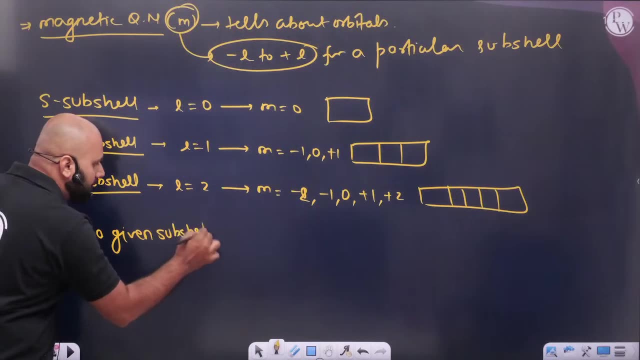 So keep going like this. See here for given sub cell, for a given sub cell. if someone asks you there is a given sub cell, there is a given sub cell, then in its case, what will be the number of orbitals? 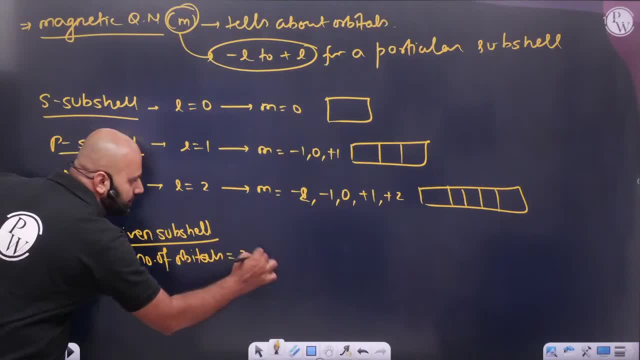 What will be the number of orbitals you will have? That is 2L plus 1.. And how many maximum electrons can come in it. How many maximum electrons will come 2 times 2L plus 1, and that is equal to 4L plus 2.. 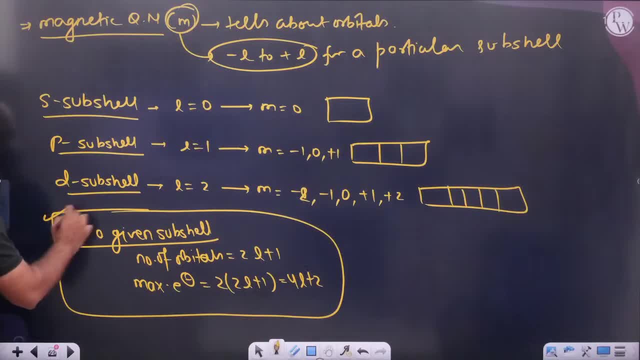 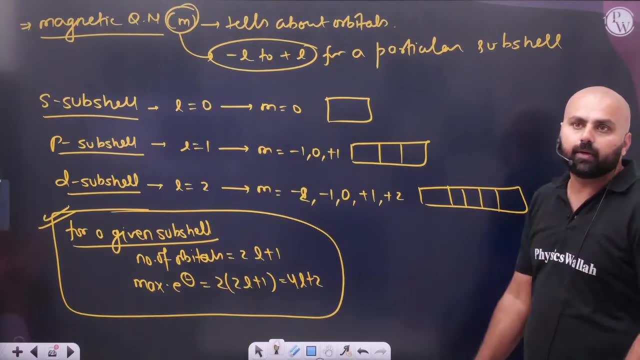 Remember these small formulas somewhere in the exam hall. you will get to do the direct match the column. You can do the direct match the column. Everything is decided by coming to the magnetic quantum number NLF straight. Everything is decided by coming here. 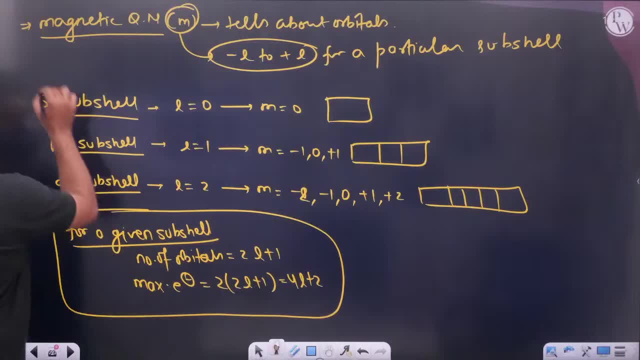 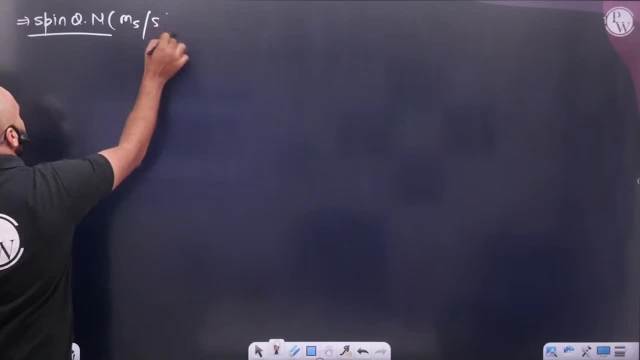 What else comes in quantum numbers. So a spin quantum number comes, which is very simple. What will the spin quantum number tell? So this is nothing. Remember this spin quantum number. remember this was not the solution of Schrodinger. 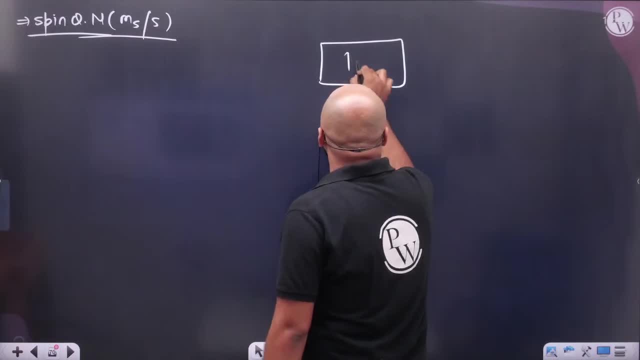 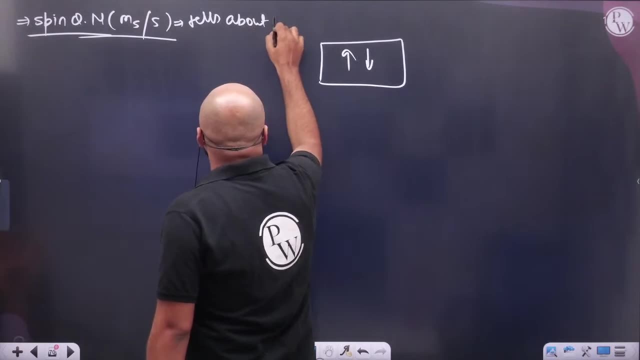 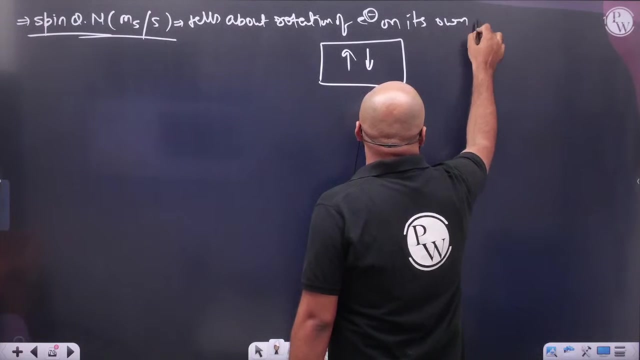 Why did the spin quantum number come? Because the electrons are of opposite spin. So the spin quantum number is nothing. It tells about the rotation of. tells about rotation of electron on its own axis. How is it doing on its own axis? It will tell about that. 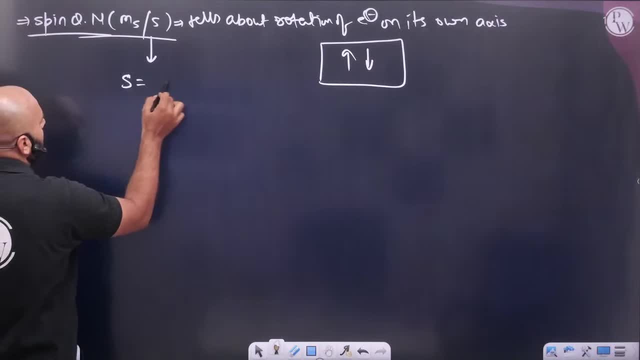 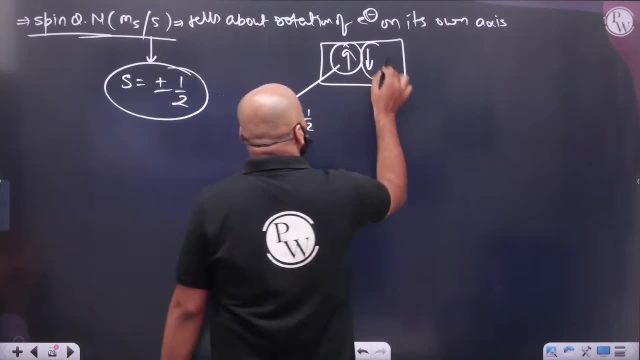 Meaning it has only two values. If it has only two values- plus minus half or plus half- Suppose you gave it plus half. If you gave the value of spin plus half, then how much will you have to give the value of this spin? 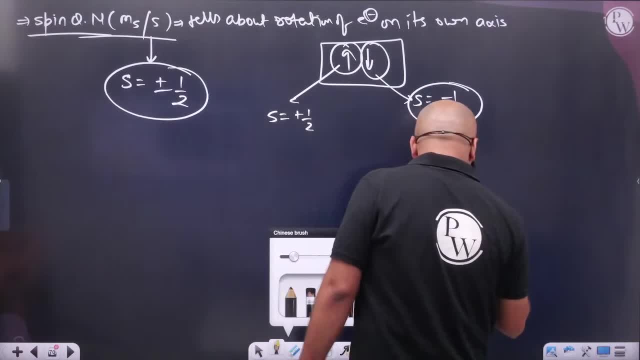 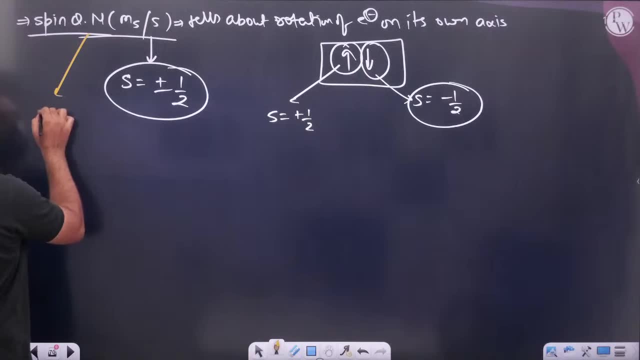 You will have to give minus half. How much will you have to give the value of this spin? You will have to give minus half, You have to give minus half. So the spin quantum number is only this much. only Just remember. it is not the solution of the Schrodinger equation. 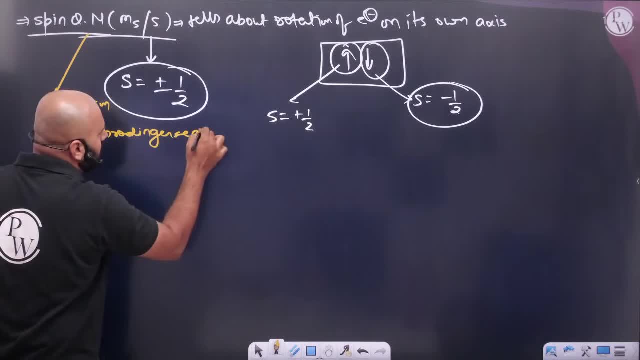 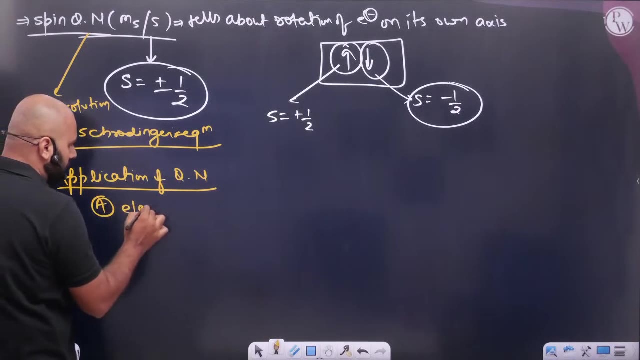 It had no relation to the Schrodinger equation. If someone is asking you what are the applications of quantum numbers, If you see the very first application of quantum number, then that is Electronic configuration, The very first application of the electronic configuration, Electronic configuration. 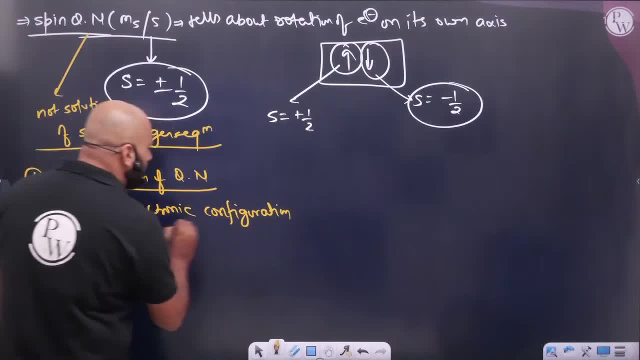 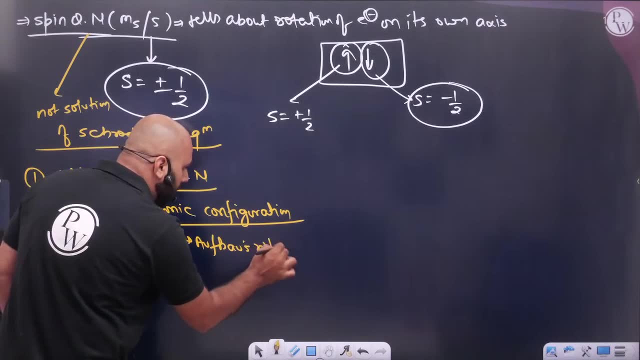 Here we can say: above principle, If we try to write electronic configuration, then three rules follow, Three rules follow Which one One above rule follows. What does above rule say, Sir? what does above rule say Higher n plus l value? 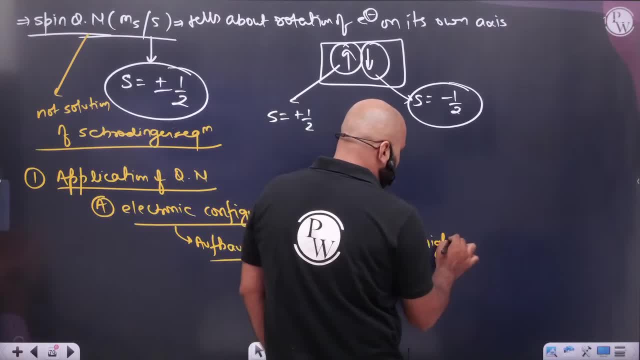 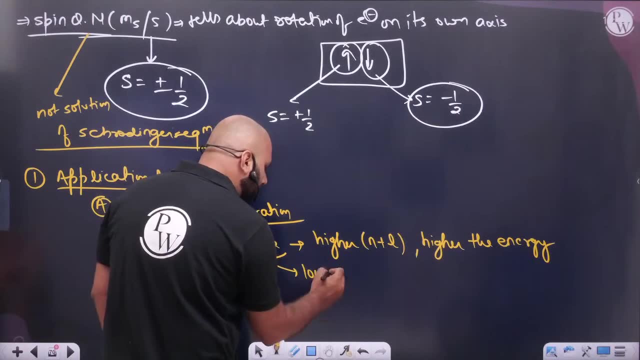 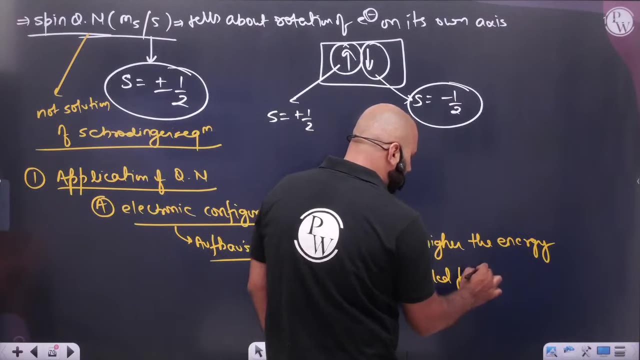 Higher the n plus l, higher is the energy. Higher the n plus l, higher the energy. What does above rule say, Sir, which one will we fill first? First, lower energy, Lower energy. Lower energy is filled first, First we will fill lower energy. 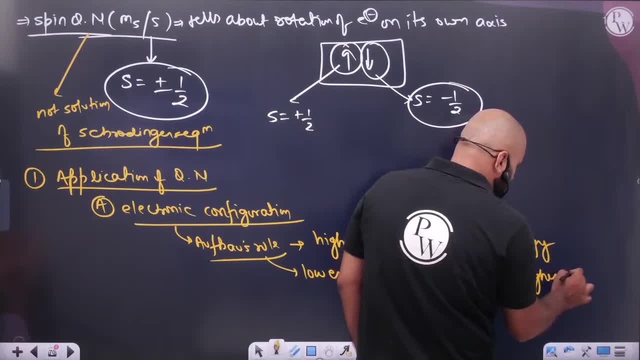 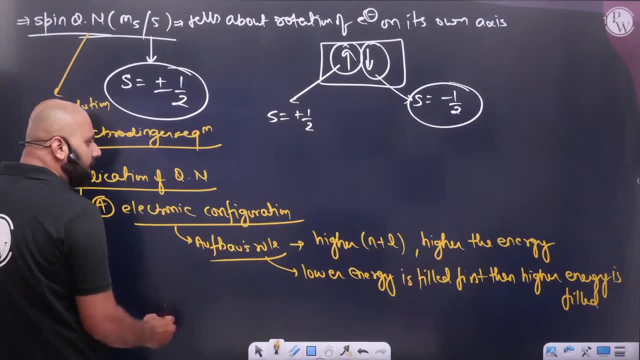 Then higher energy level, Higher energy is filled. Sir, in this way we will be filling everyone. See this, Sir, in above principle: this will come If same came. Someone said: sir, same n plus l came, Same n plus l came. 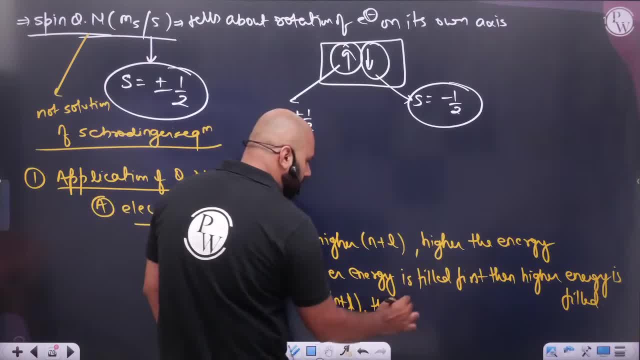 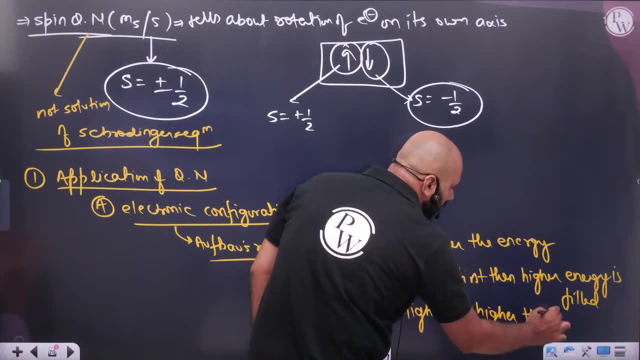 So in that case, same n plus l came. Then Higher n, The higher the n value. what will be the energy value? Higher is the energy, Higher is the energy. So see the value of n plus l near you. After that, what comes second? 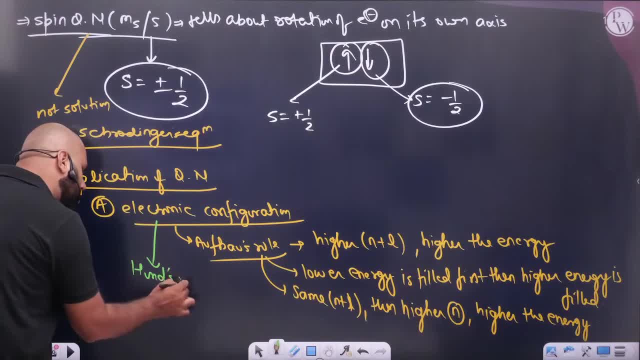 Hund's rule. What does Hund's rule say? Whenever you will fill electrons, what will you do? If we talk about P4, then you cannot fill P4 like this. You cannot fill P4 like this. Remember in Hund's rule. 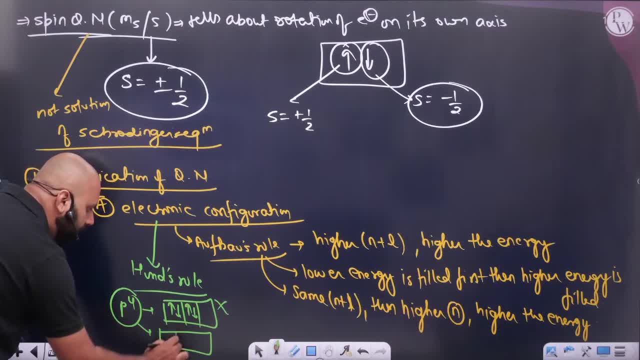 It will not be filled like this. How will P4 be filled? What will you do to all of them? You will fill one by one. you will fill one by one, then after that you will fill. this Hund's rule tells, in a way, that the fully filled is more stable. fully filled is more stable. then who is more stable? half filled is more stable. 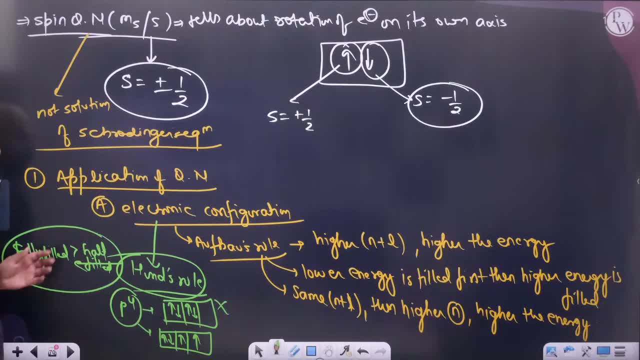 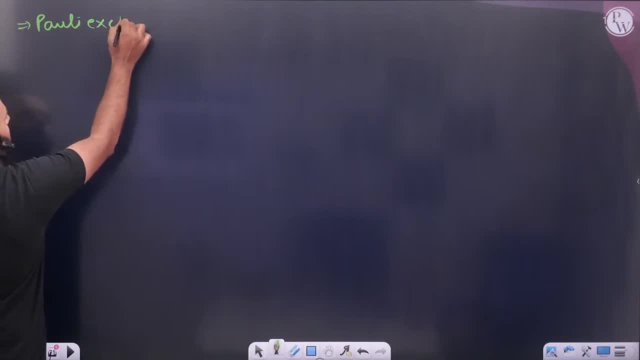 Who will be the most stable after fully filled, half filled will be. So this is used in electronic configuration. Then you will see that you have a principle of poly exclusion. What does poly exclusion say? Remember, different people have different ways. Poly exclusion says that never two people can live like this. 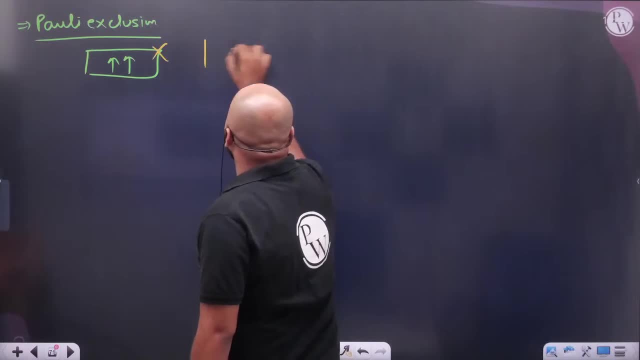 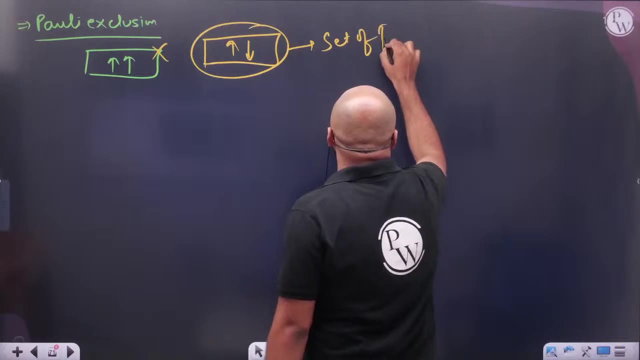 If you are living in the same house, then never two people will live like this. How will it be? always One will be up, then one will be down. Means, sir, all four. set of four quantum numbers. set of four quantum numbers can never be the same. 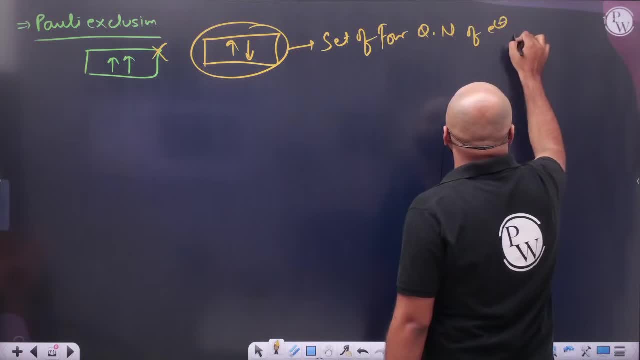 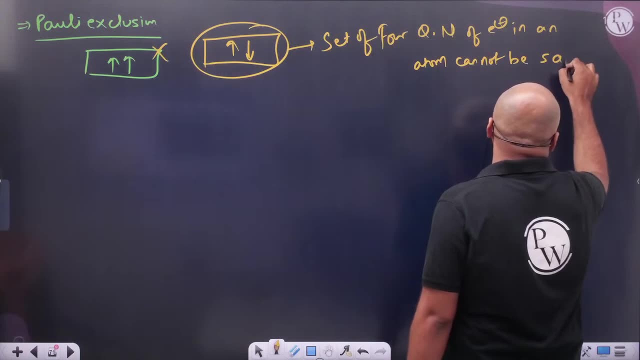 Quantum numbers of electrons in an atom. in any atom, the electrons cannot be the same, Never can be the same. All four, three can happen, no problem, But all four can happen. All four quantum numbers will never be the same for anyone. 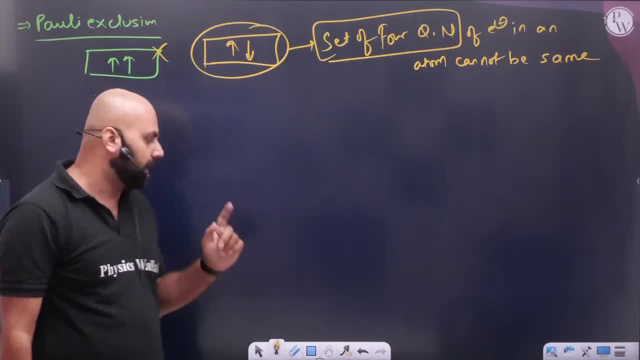 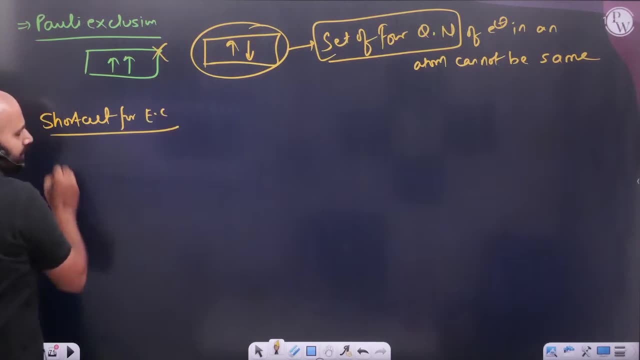 Okay, Never will be the same for anyone. So this is the principle of poly exclusion. Now slept. We all know the shortcut of electronic configuration, Shortcut for electronic configuration. You all probably know from the beginning that- how to fill electronic configuration. What is the way to remember anytime? 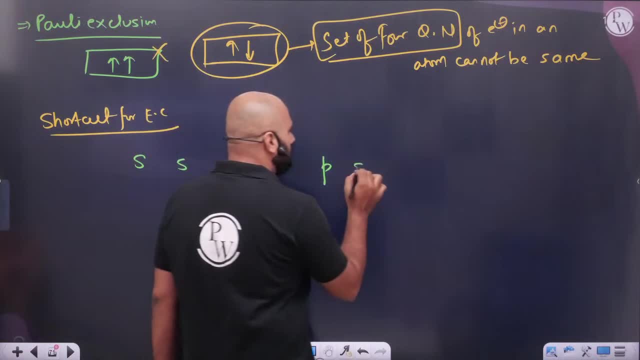 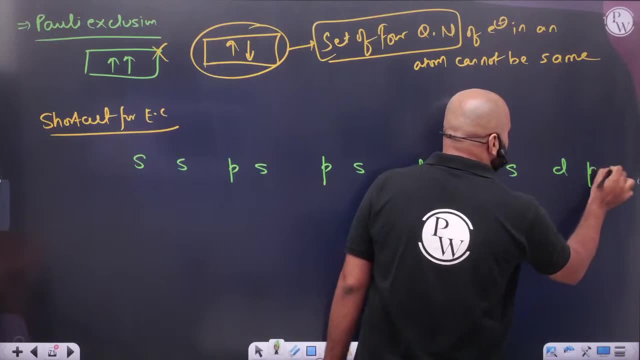 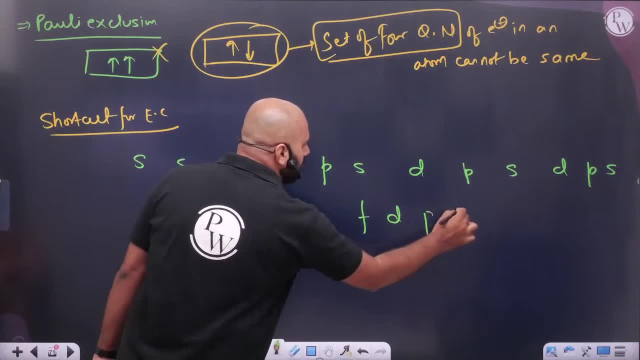 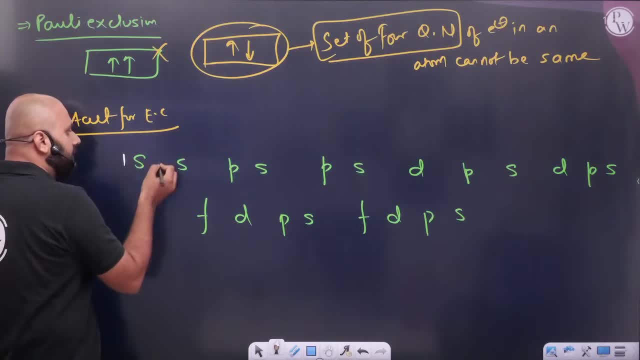 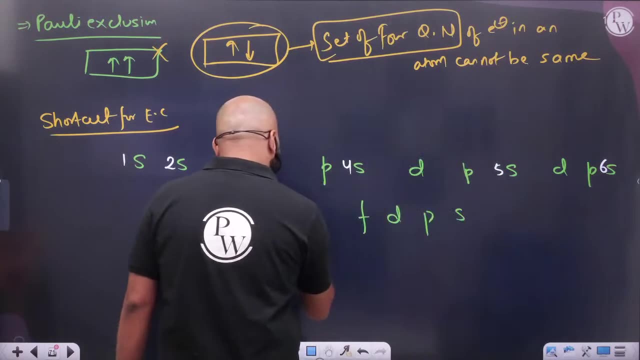 Electronic configuration cannot be written more easily than this Simple Look at this. where will the numbering of S start from here? S survival starts from 1st, So S will start from here. Look at yourself. 5, what happened? 6, how much did this happen? 7, how much is this 8.? 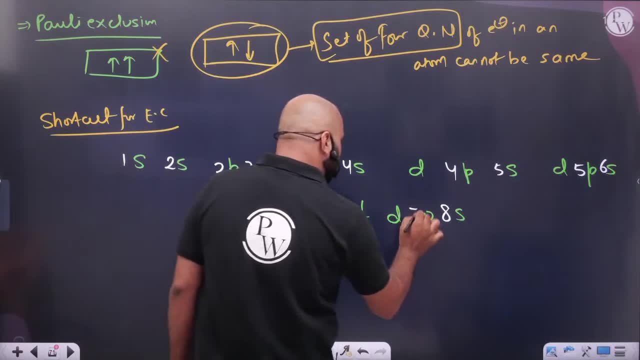 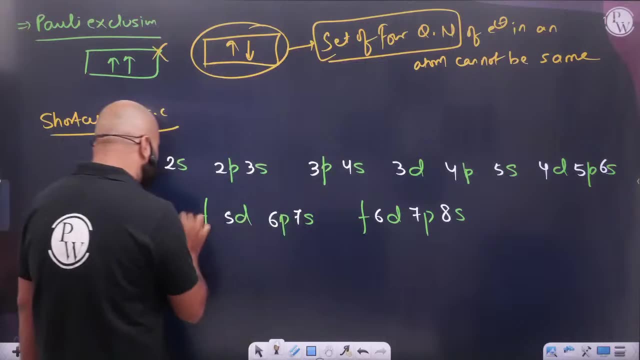 S, Sir, where does B sub cell start from 3?? So where does it start 3,, 4,, what is this 5,, what is this 6? And where does the numbering of 4 start from 4? 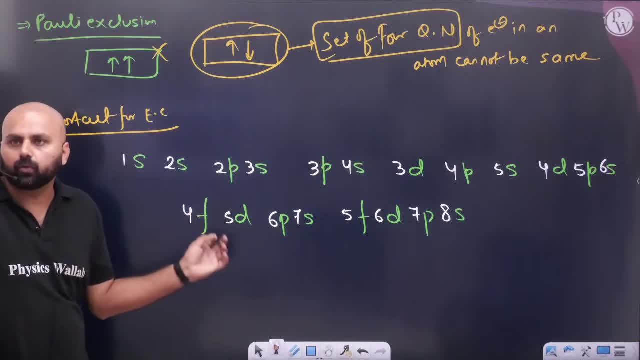 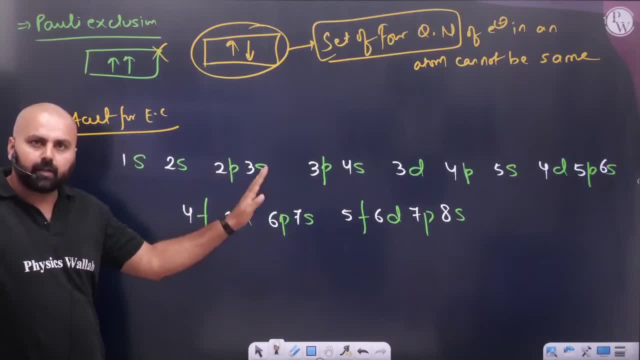 So, sir, first we wake up from sleep, Then we study and sleep, Then we study and sleep, Then we study and sleep. So it is like that. Some people are so dangerous. So it is like that. See this: Whenever you want to fill electronic configuration, If someone asks you sir, where will you recognize inert gas? 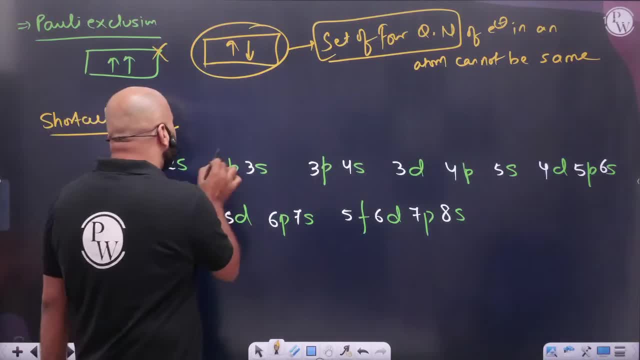 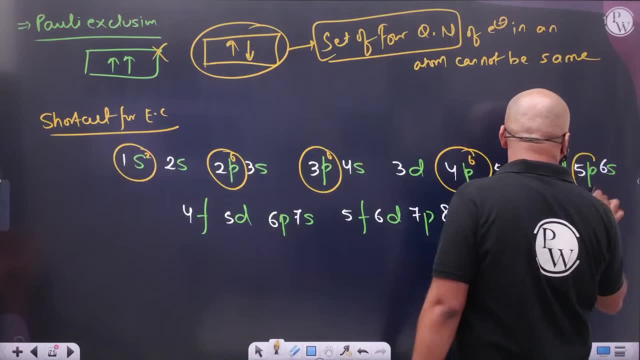 Inert gas is here. Where is inert gas? It is here. Whenever 6 comes in it, inert gas will come. If you want to write electronic configuration in inert gas, Then write this with you. If you want to write the configuration of inert gas, Then here is the inert gas. 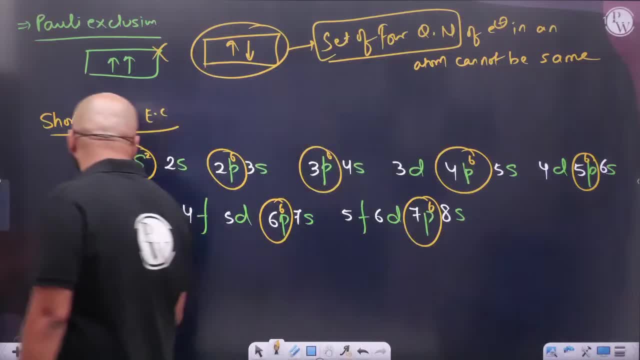 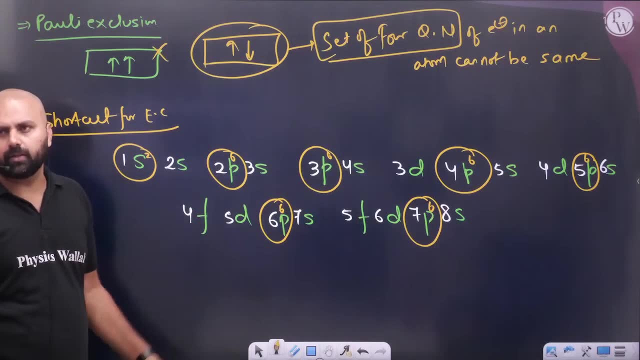 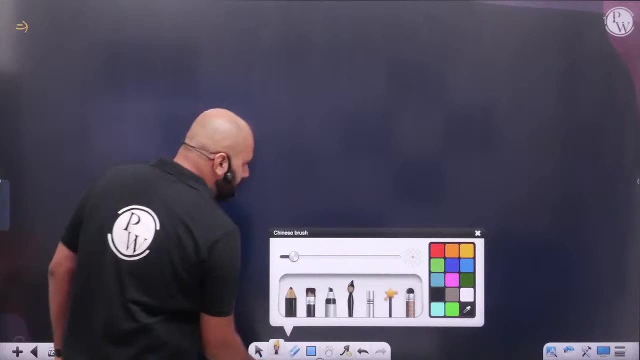 Inert gas. What is inert gas? It is P6. Leaving one helium Rest, you keep filling it. All the rules will be followed. Ok, All the rules will be followed. So do such things. Shortcut of electronic configuration. After that in our life Which comes in electronic atomic structure. 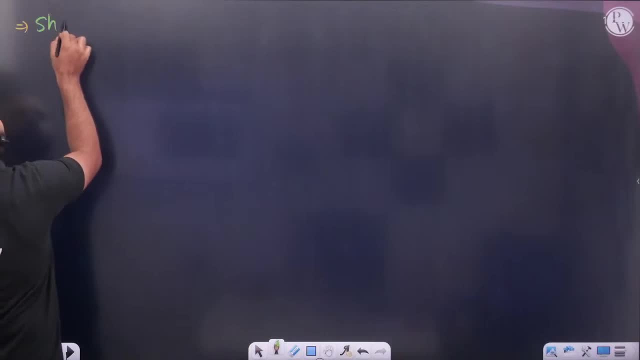 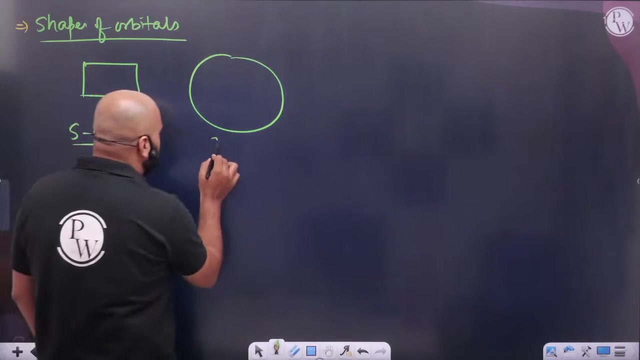 After quantum numbers. Saves of different people, Saves of orbital, Saves of orbital. What are the saves of orbital? So, brother, see, In S There is only one orbital. So the save of S is spherical, The orbital of S is only one. S will be spherical, S will be spherical. 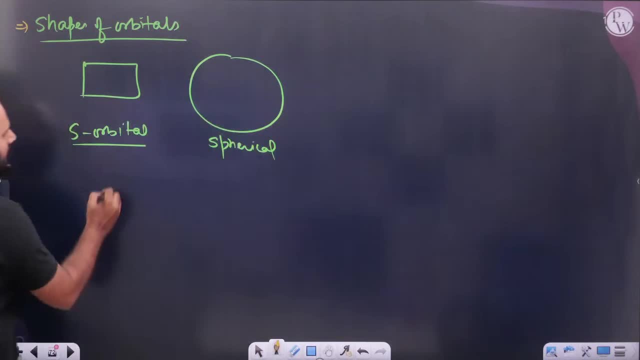 If we talk about P, Then different people come in P See here: Any electron can be found anywhere. In this case there is no nodal plane. There is no nodal plane. But if we talk about P- orbital See in P subcell- Then PX, PY, PZ. 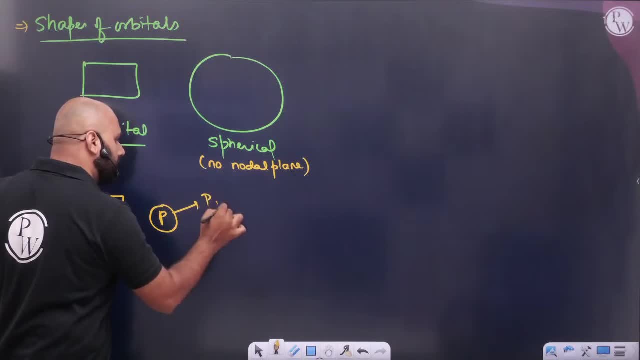 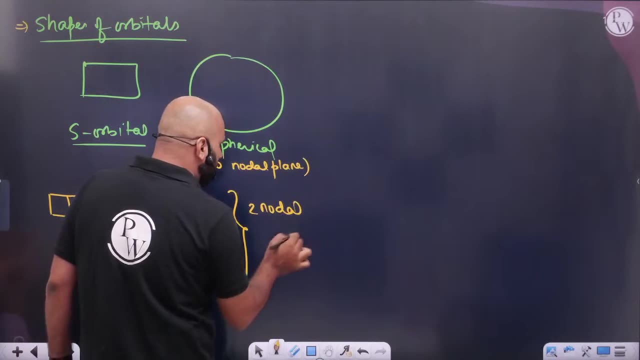 There are three. There are three in P, Which are PX, PY and PZ. You have to remember That, sir. These three have two nodal planes. Now you will start to see Two nodal planes. If you talk about PX, Then nothing. What does PX mean? 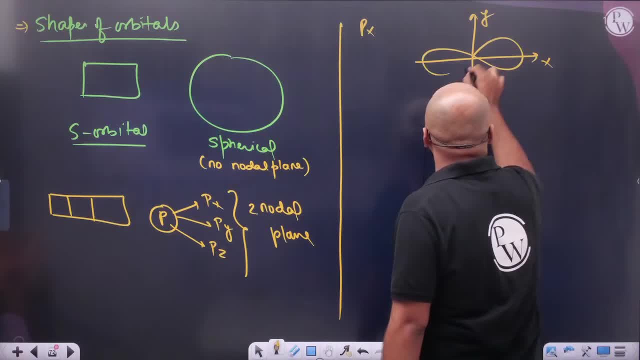 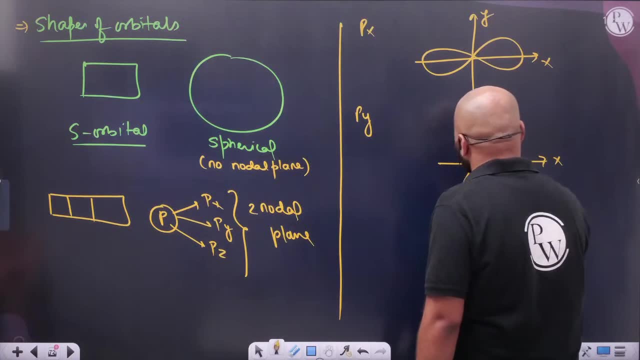 If this is the X axis, This is the Y axis, Then where to make PX? Make this: If you talk about PY, Then what will happen to PY If it was on the Y axis? This is the X axis, Then make PY like this: If you talk about PZ. 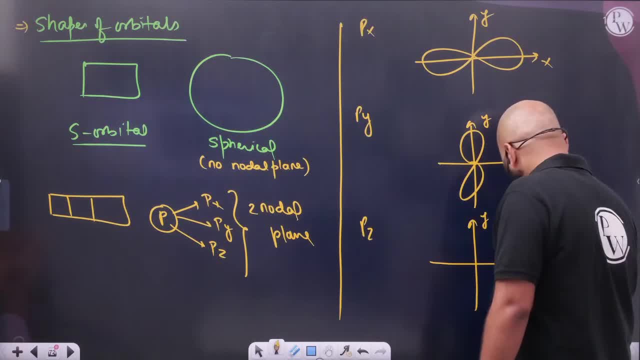 Then, sir, this was the X axis, This was the Y axis. There is one Z axis. There is one Z axis. There is one Z axis. What happened? There is one Z axis. So, sir, make it like this: on Z axis, Electron cloud. So see this: All of them have two nodal planes. 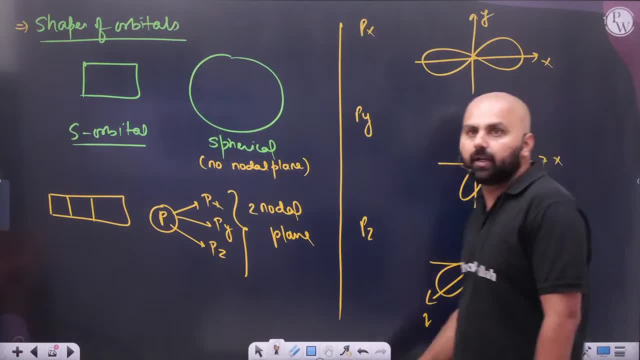 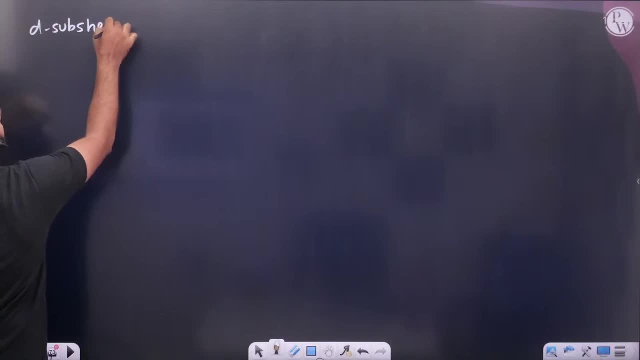 Like, if you go to PX, Then YZ and its nodal plane will come. So like this: If I talk about D, If I talk about D subcell, If I take D subcell, Then in D subcell, How many are there in D subcell? 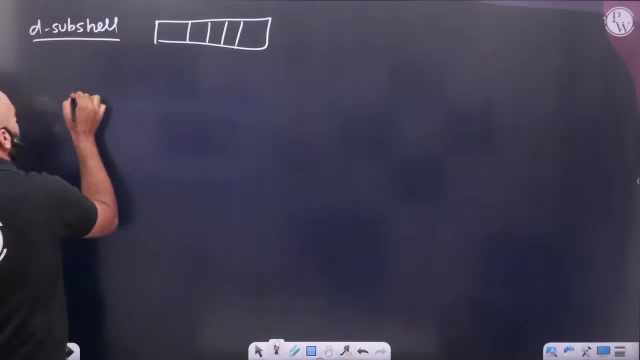 There are five. How many are there in D subcell? There are five. See which ones: DXY, DYZ, DZX. This is what happens. Where are these? They are in between the axis. Where are these? They are in between the axis. And if I talk about DX square minus Y square, 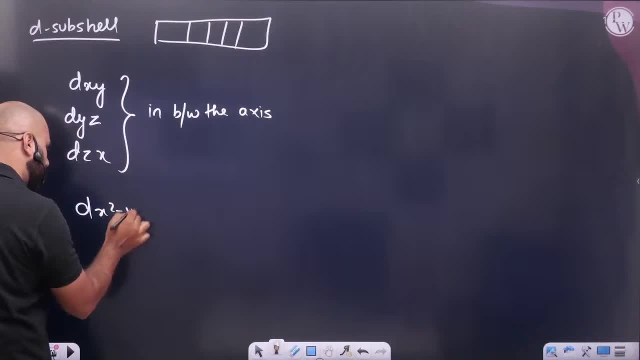 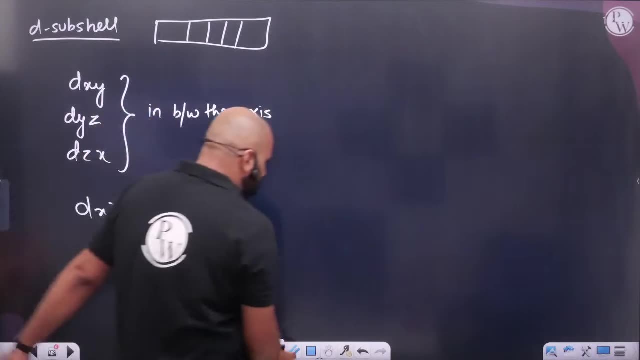 DZ square. What are all these? They are on the axis. What are all these? They are on the axis. See the first one of these three: DXY. There is no problem. Take X and Y And make a double flower. If this is X, This is Y. 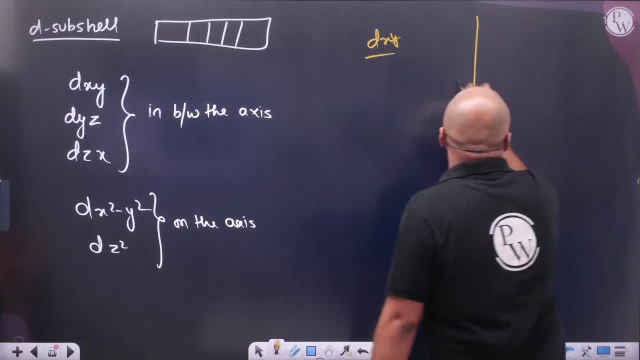 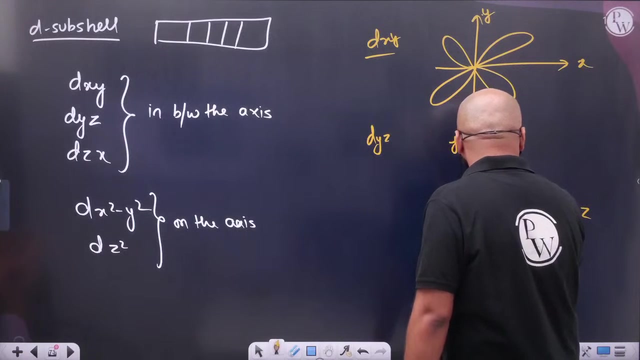 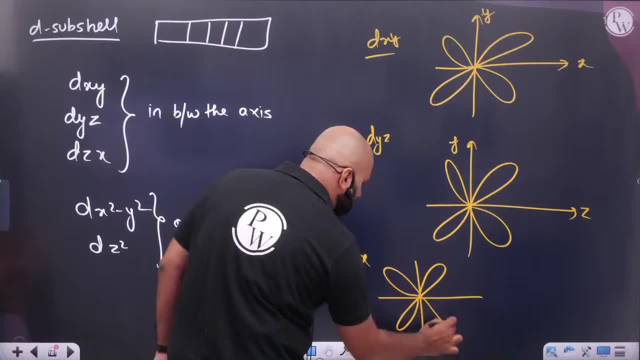 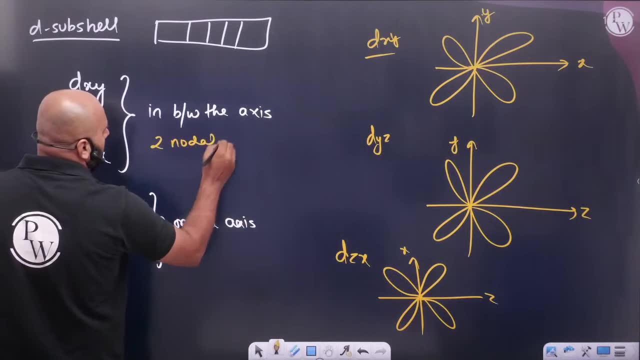 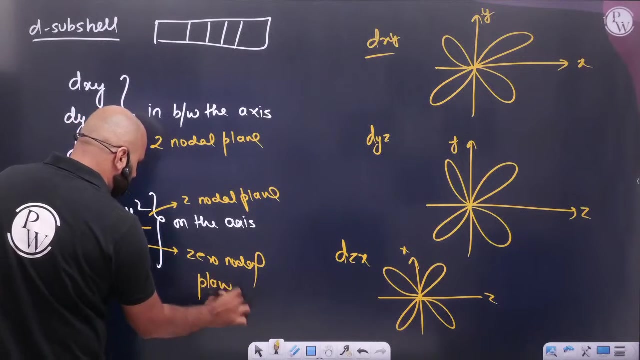 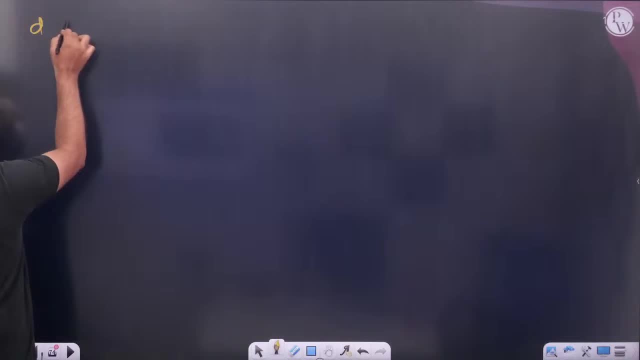 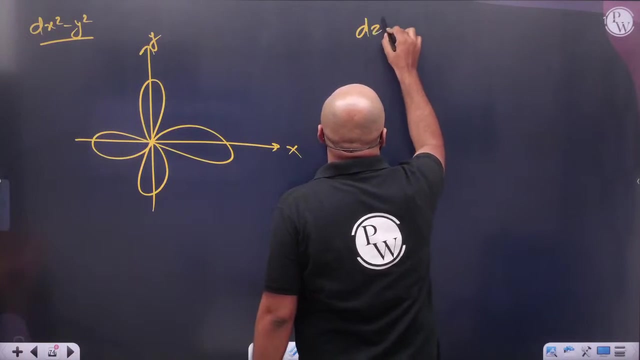 See the structure of dx square minus y square. see the structure of dx square minus y square. how will it be? This is x axis, this is y axis. the structure of dx square minus y square will become like this: it will become on the axis, and that's why, when you study the coordination compound, 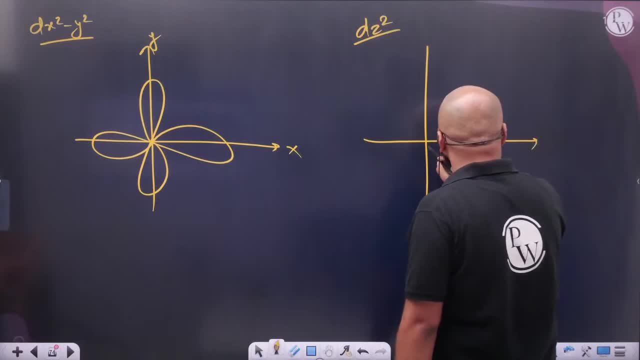 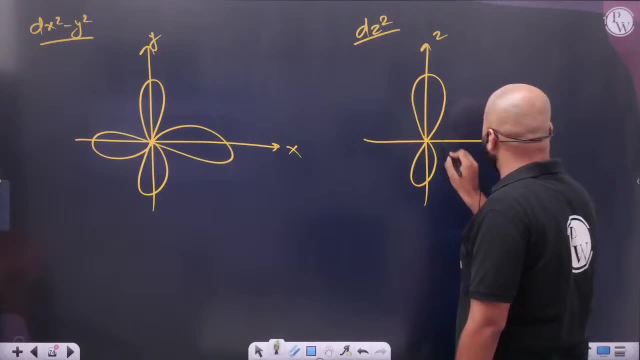 you will come to know that. what are these people you will see in dz square? this is z axis in dz square. See this. the question can come on its shape. the question can come on its shape. The electron here, this ring is in xy plane. this ring is in xy plane. this ring is in xy plane. 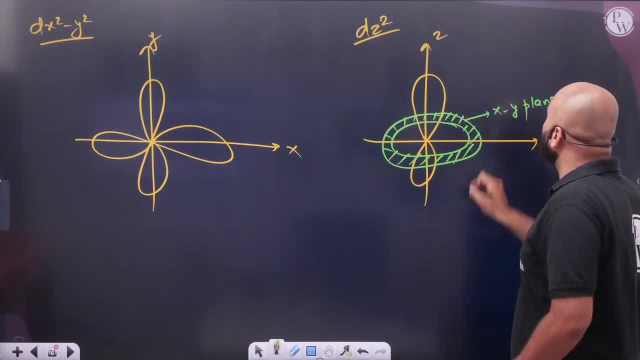 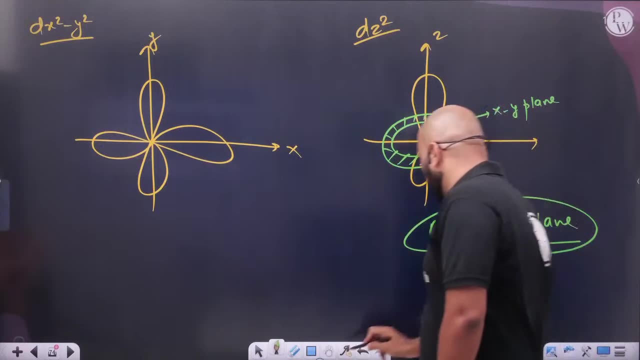 so here, electrons are in every plane. that's why it does not have any nodal plane. no nodal plane, there will be no nodal plane. In the case of this, there will be no nodal plane. Okay, so see this with you. 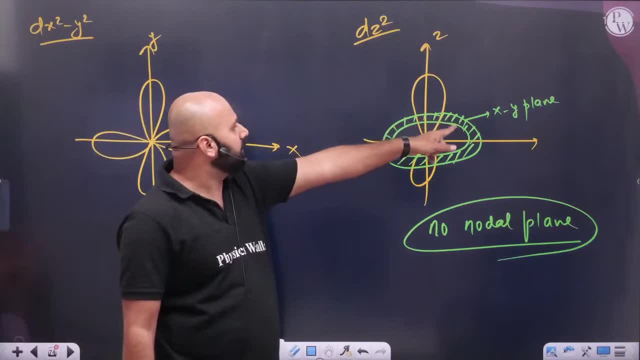 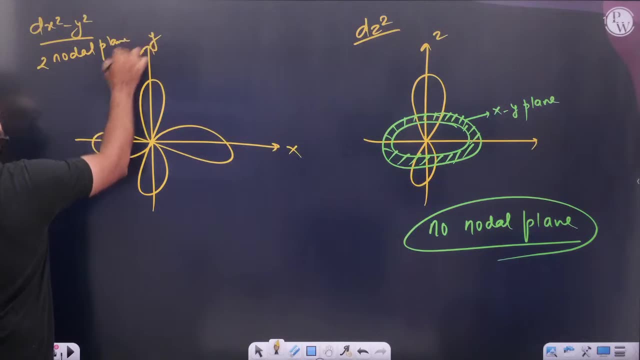 Now see this ring. it has three axes: x, y and z, on all three. that's why it has no nodal plane. it will have two nodal planes. it will have two nodal planes. Someone says, sir, what are nodes? 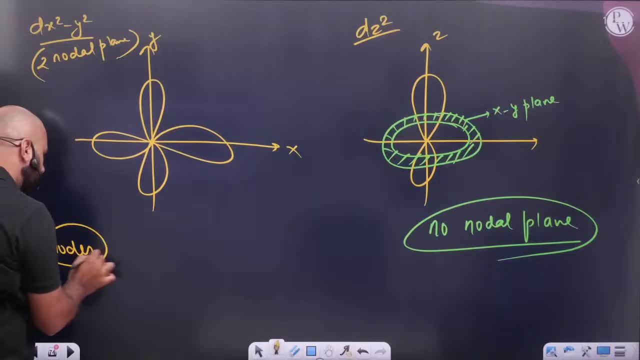 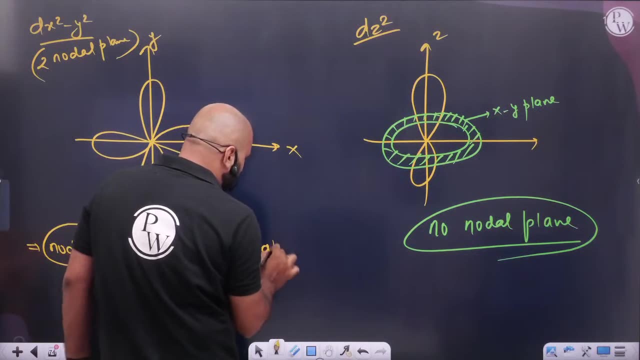 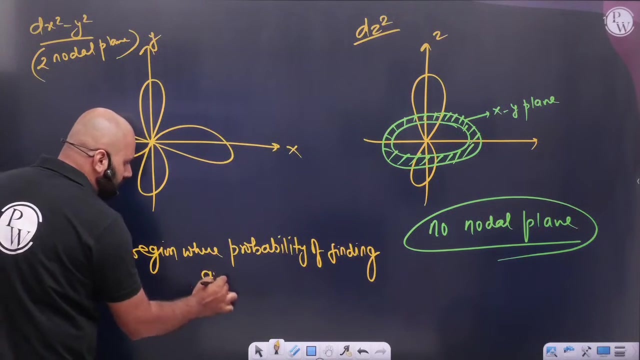 So, brother, the node is that: what are nodes? So what are nodes, Sir? the reason where you get, the reason where probability of finding an electron, probability of finding an electron, where the probability of finding an electron is zero, 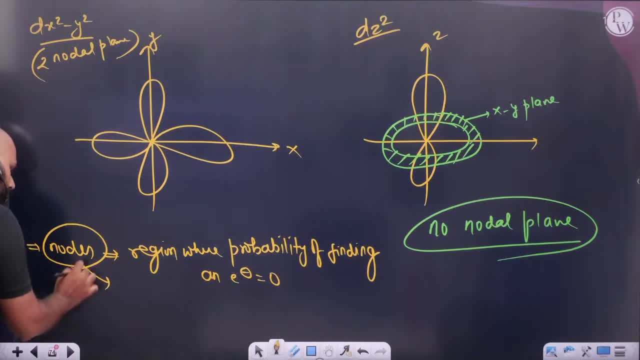 where the probability becomes zero. If you see the nodes with you, there are two types. one is radial nodes. radial nodes, we write this n minus l minus 1, calculate directly. and one is angular nodes. what will be the angular nodes? 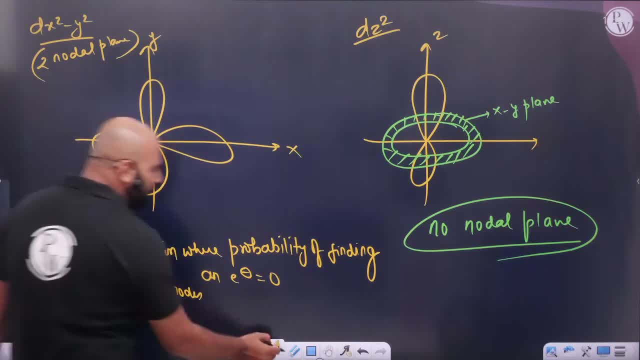 Sir, it will be equal to the quanta number. If someone asks you tell me the total nodes, then what will be the total nodes? Add both of them, what will be the total nodes? n minus 1.. Radial nodes. angular nodes. 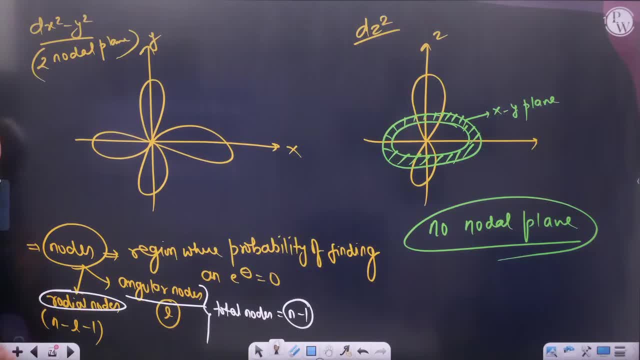 Radial nodes are also called spherical nodes. What will be the radial node? How much will it be? n minus l minus 1.. What will be the angular node, l? What will be the total nodes? n minus 1.. Radial means to see the distance on the radius, nothing else. 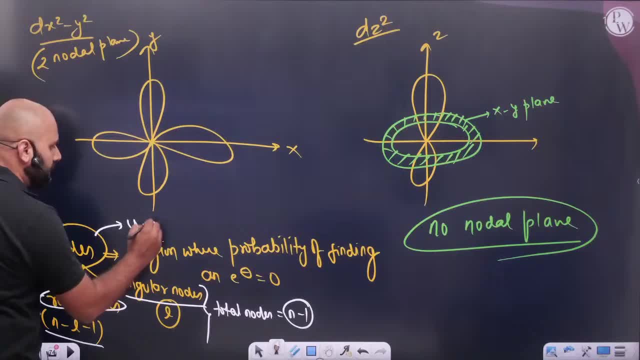 Nodes means where the value of psi is zero. If the value of psi is zero, then the value of psi square is also zero. Where the value of psi square will also be zero, What will be the value of psi square? db Zero? 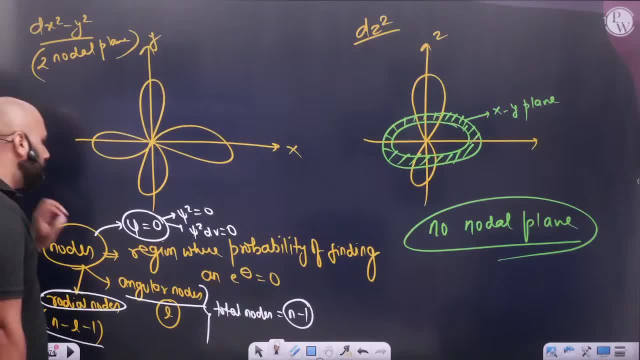 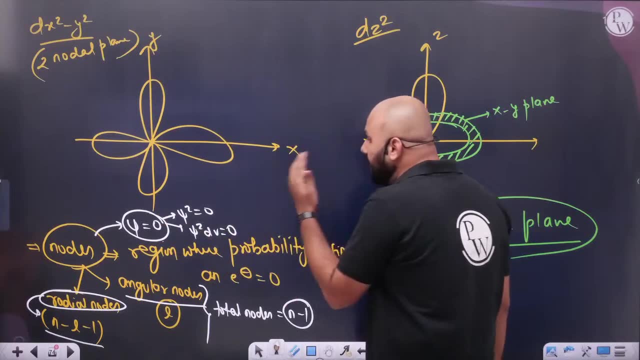 What will be the value of db Zero? Remember nothing else. If someone wants to give a graph-wise question, if someone will give a graph-wise question, then see in the graph that nodal plane where the value of psi is zero. what is the node? 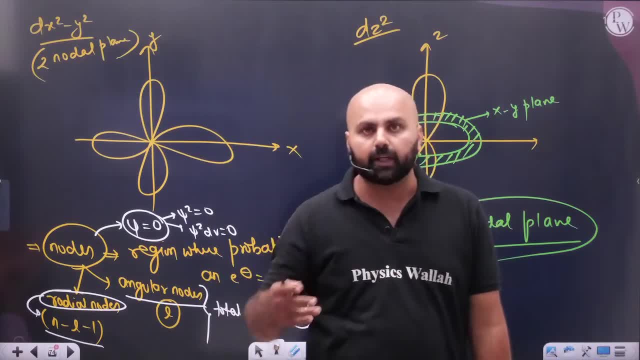 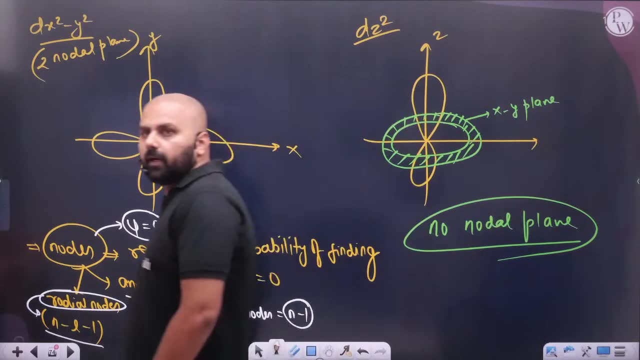 Radial means to see the distance on the radius, And one is angular means what will happen to us? It will be straight. Look at it. look at the angle. Okay, look at it according to that. Come on, look at the question. 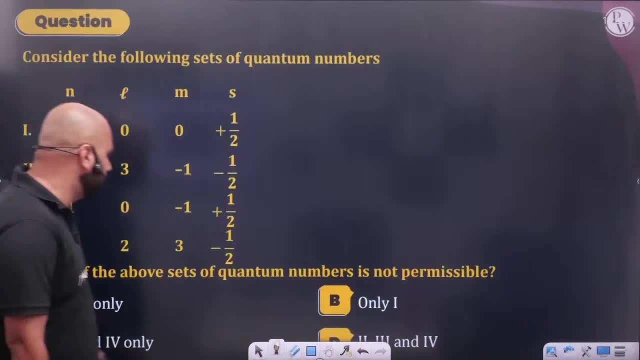 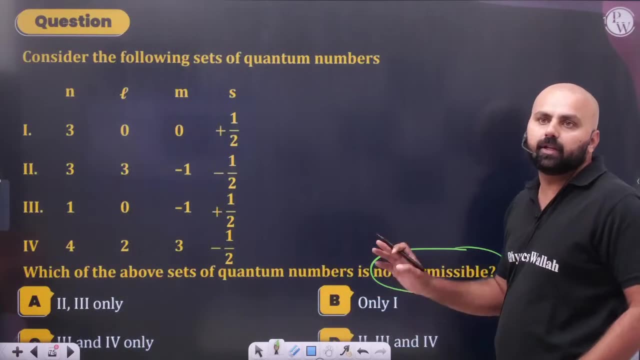 Look at this question: Which quantum set of numbers is not possible? This question also comes a lot, Sir. which one is not permissible? Which one is not perfect? Which one is not permissible? Let's finish this chapter. I will give a break after that. 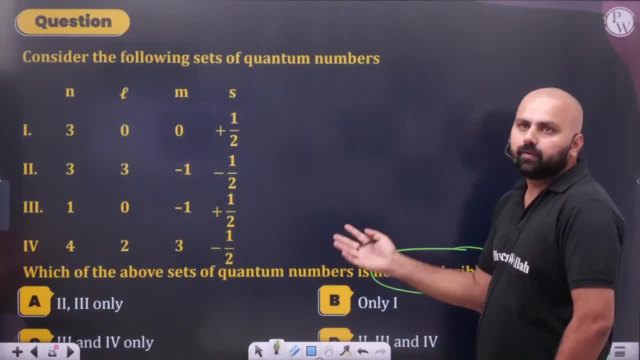 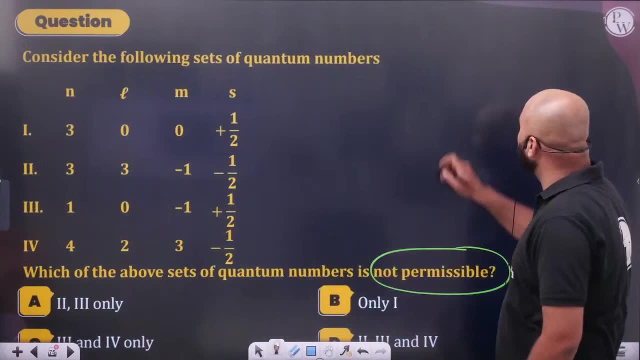 I am doing revision. Where am I studying? I am doing revision. Okay, The value of n: Yes, the topic to be taught. It is not enough to teach in one day For the whole year. How will you become a doctor like this? 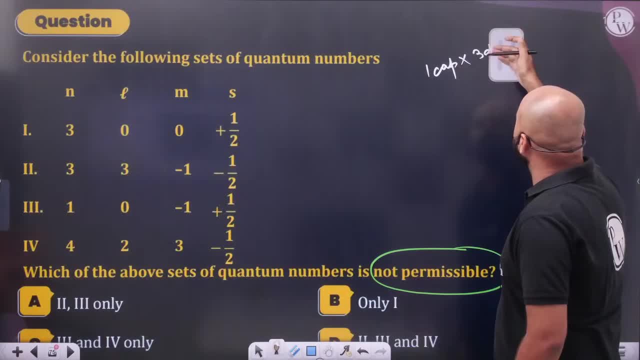 One capsule in three days, Three times, Three times into five days. One patient: You wrote to one patient like this And that patient said: sir, I will do one thing: Fifteen capsules. If I eat it at one time, then the thing will be equal. 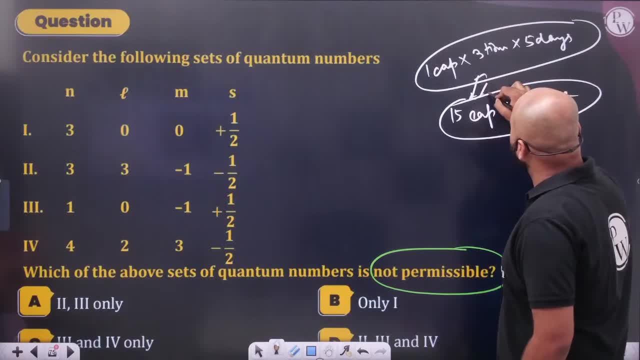 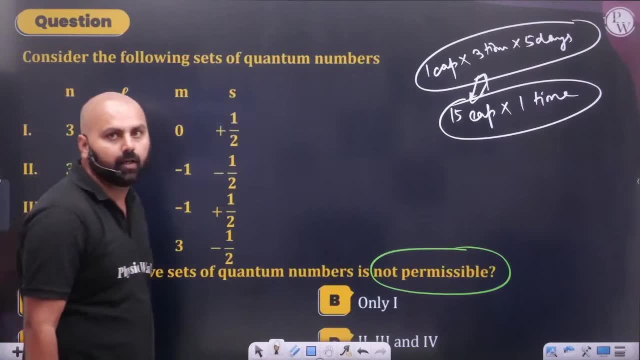 You only know Both are equal, right, sir. Sir, you will write the medicine after becoming a doctor: One capsule. One capsule has to be eaten three times, Have to eat for five days. You will write this as a doctor. The patient will come and say: no, sir, let's do one thing. 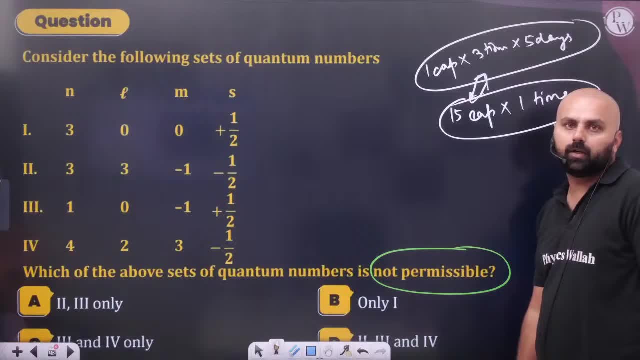 Fifteen capsules have to be eaten. I will eat it once. I will eat it at any time. You think he will remain alive. And how much fun will you have, Brother, at this time we are reviewing, So in revision, you will think that now one thing. 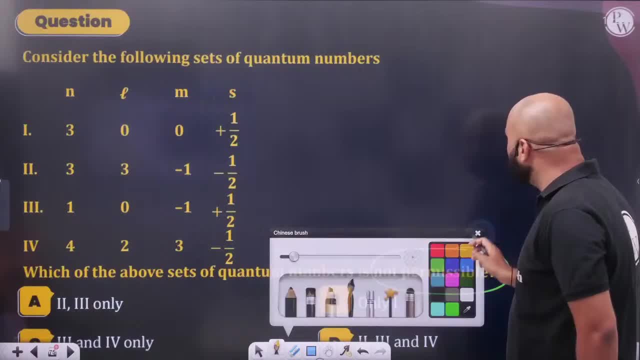 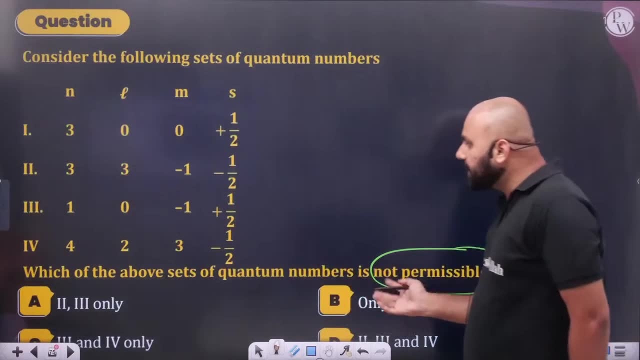 Brother. now someone is saying derivation, Brother, why will I do derivation in revision? Okay, There is no derivation in revision. man, Where were you before? It's just that the selection people are sitting. Just revise them quickly, Finish it. 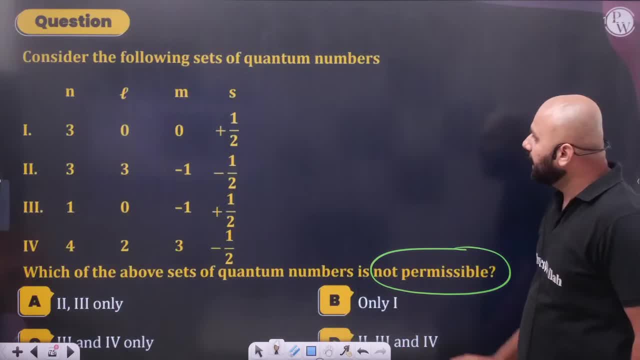 Okay, What will happen? See Which is not permissible here. See this: What is he saying, Sir? the value of N is three. See, The value of N is three. The value of L is three. No, How far does the value of L go? 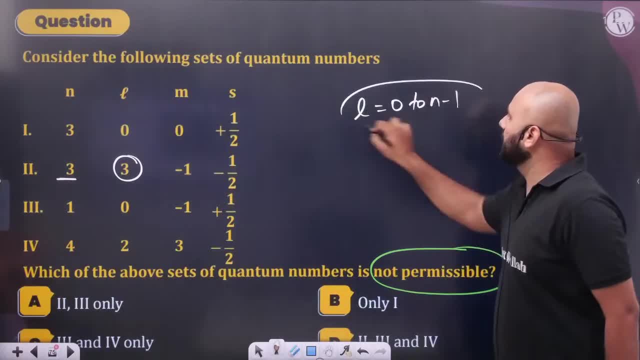 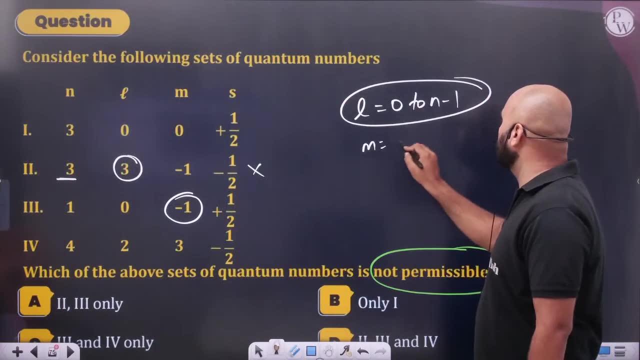 G From zero to N minus one. So, sir, this will not happen. Second, one will not happen. Sir, the value of L is zero. And how much is this Minus one? Where does the value of M go? 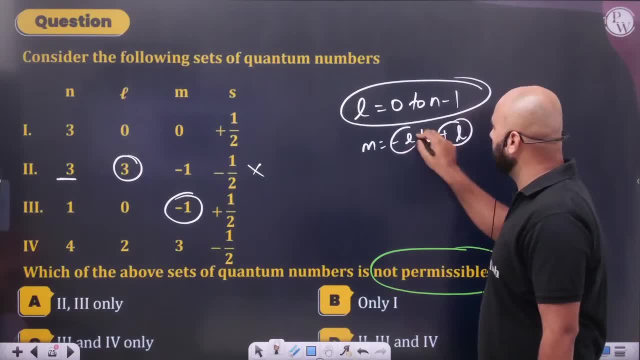 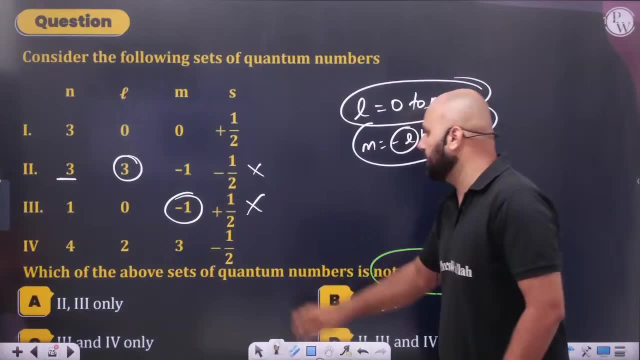 Minus L2 plus L, Minus L2 plus L. Sir, this depends on this, This depends on this. So, brother, this is also not possible. So, this is also not possible. Third is also not possible. Four, two, three. 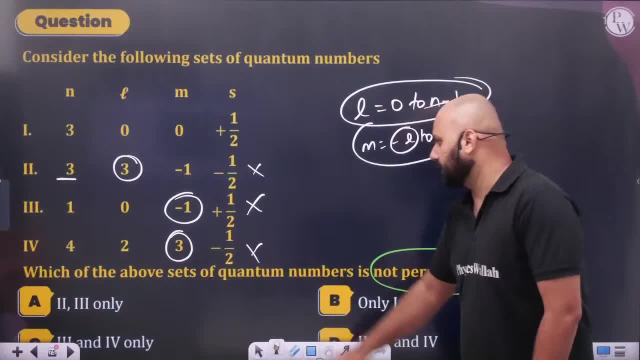 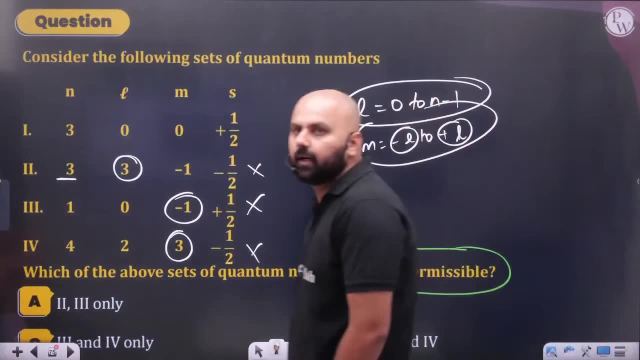 Again. this is also not possible. So what happened? Cancel out, Which is not possible, Sir. second, third and fourth. What will be the answer? Second, third and fourth. D answer will come: Second, third and fourth. 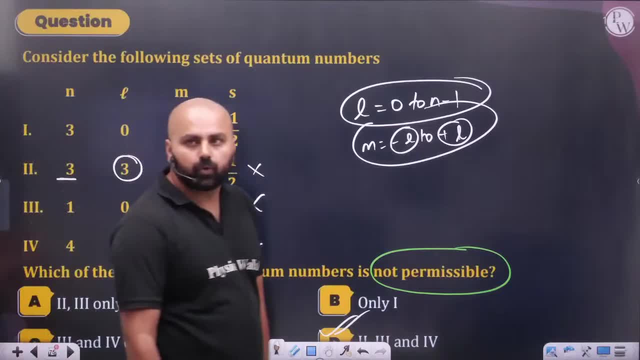 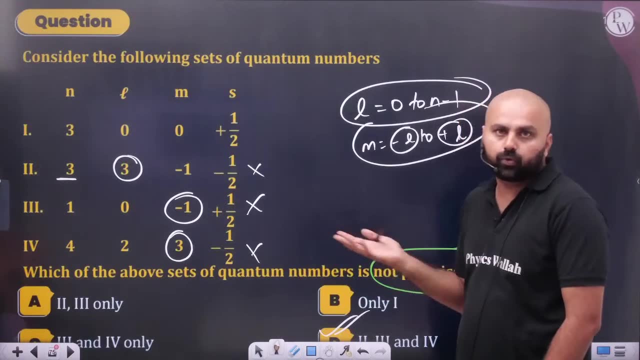 D answer will come Sure. So, brother, the people who are doing the calculation are saying that: yes, brother, Brother, this is what revision means. So I am also revising the theory, If you ask me, then already you have done a lot of things. 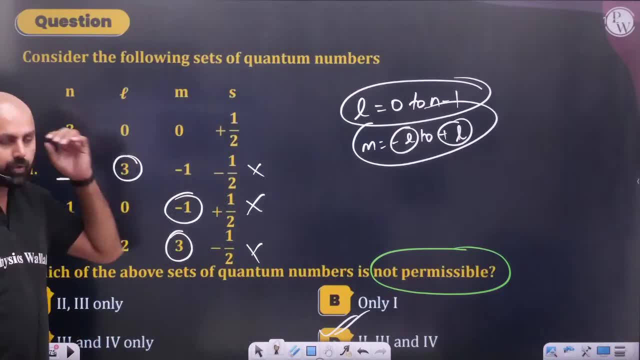 Brother, the theory is getting late. You could have asked questions directly, But no problem, Let's do it. You are meeting last time. Let's do it. Okay, See this. See this, This has been asked. Yes, angular momentum. 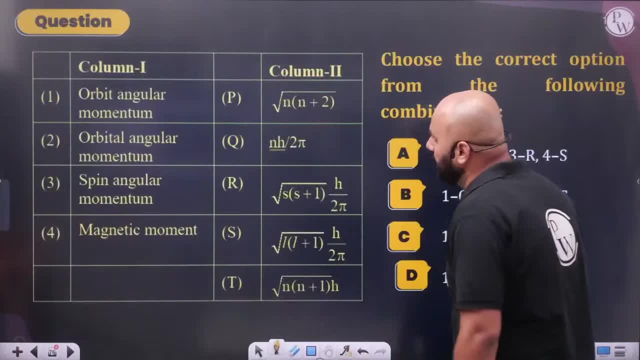 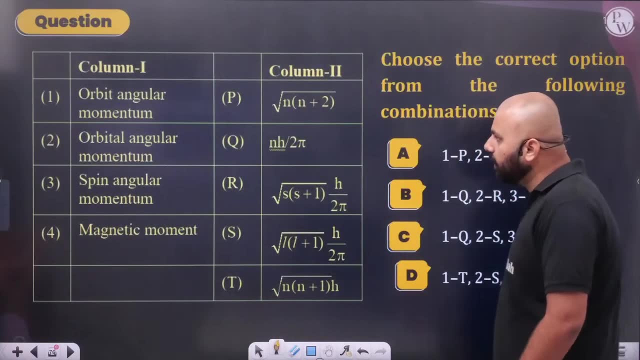 This is a good question, brother. This is why all formulas will be revised. Look, how do you extract the magnetic moment. How much is the magnetic moment? How much is the magnetic moment? Look carefully, Whose will be, Sir? if you want to extract the magnetic moment, then what you do. 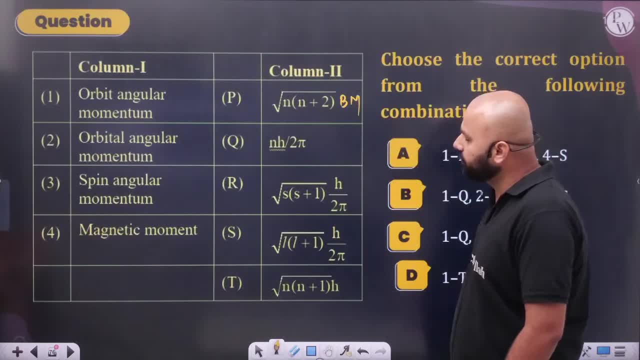 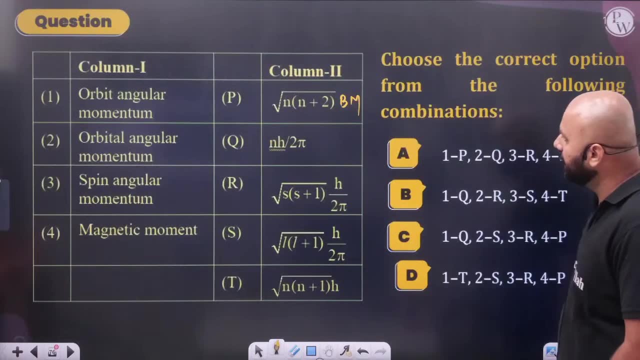 Magnetic moment is extracted like this: N into N plus two, BM is done. So what is the answer for four? One, sorry. What will come for four? It will come p, N into N plus two. What will be the spin angular momentum? 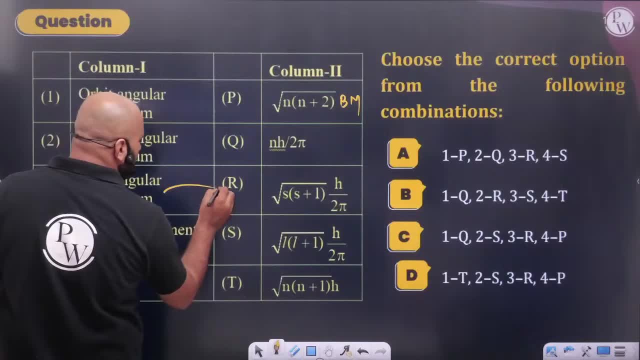 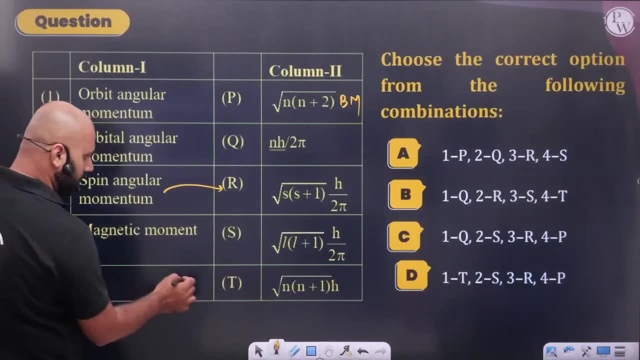 Sir, what will happen to three? It will be r Spin angular momentum. This is how we extract. How do we get orbital angular momentum? Magnetic moment n plus 1.. How much is orbital angular momentum? How much is orbit angular momentum? 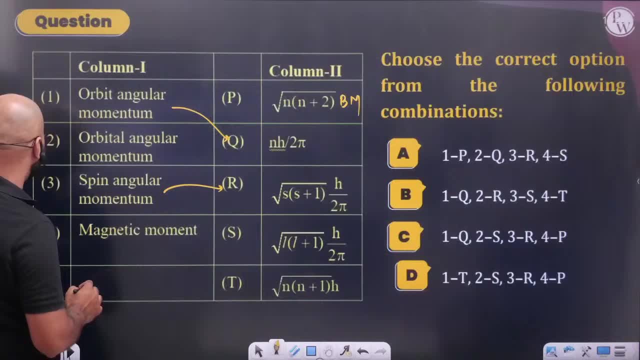 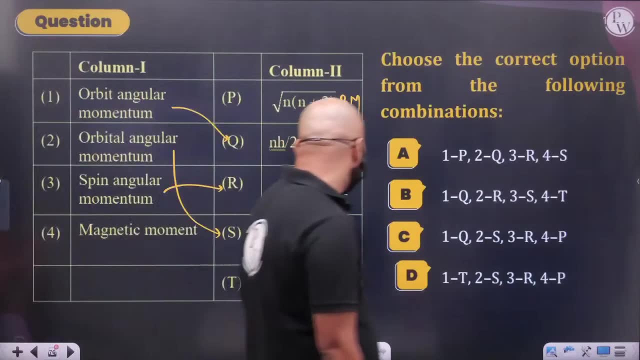 Q of 1. Q of 1 is 3. Where is orbital angular momentum Into this S of 2? S of 2 is S. Q of 1 is Q. R of 3 is R. P of 4 is P. 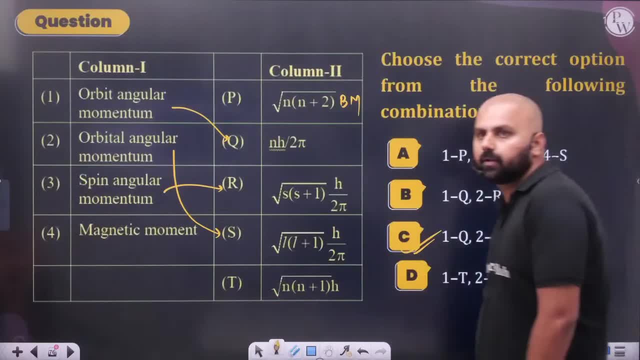 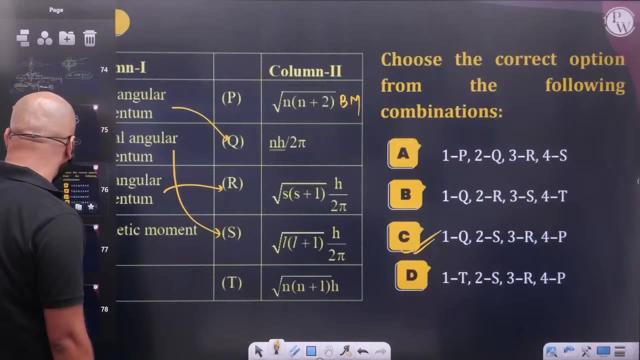 What will be the answer? Keep doing such questions. These are small questions. Now see, some questions will be revised. This will be revised, Will it be done? These are small questions. Our quantum numbers are finished. We have these states. 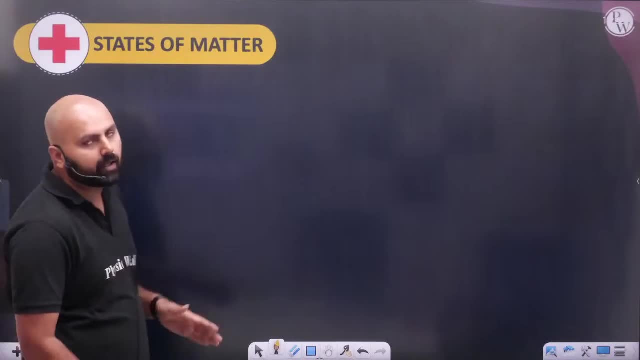 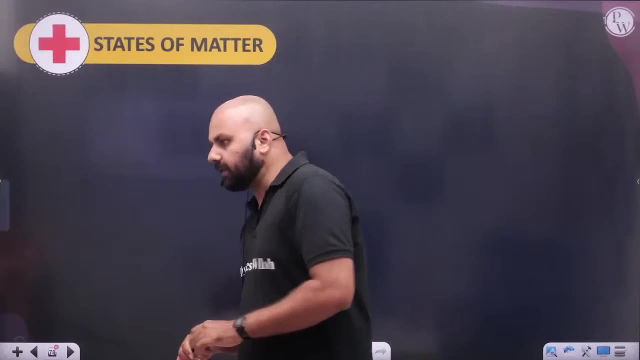 See, we are trying as much as possible. Now let's see the states of matter. This is a small chapter. Let's do one thing Now: our exam is going to pass From 2 pm to 5.30 pm. I had kept it till 5.20 pm. 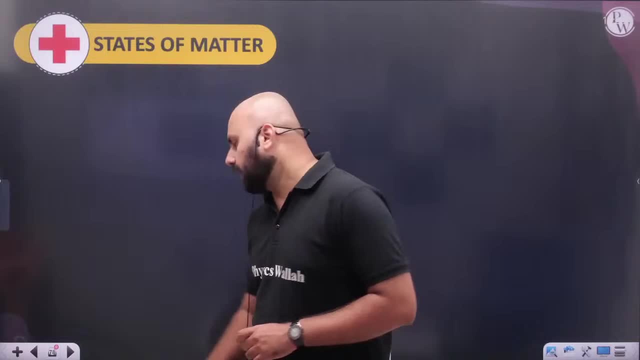 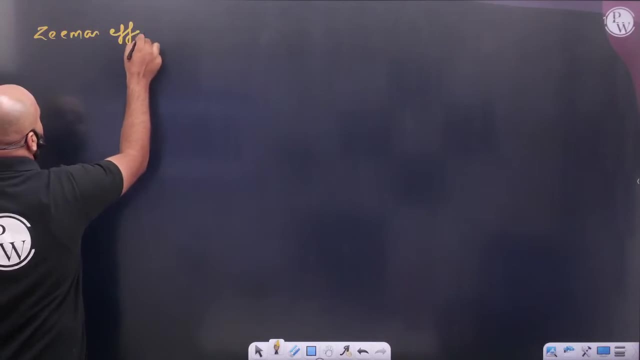 No problem, Let's do one thing. Someone is asking about Zeeman effect and Stark effect. I will tell you Zeeman effect and Stark effect. There is nothing in Zeeman and Stark. What is Zeeman effect and what is Stark effect? 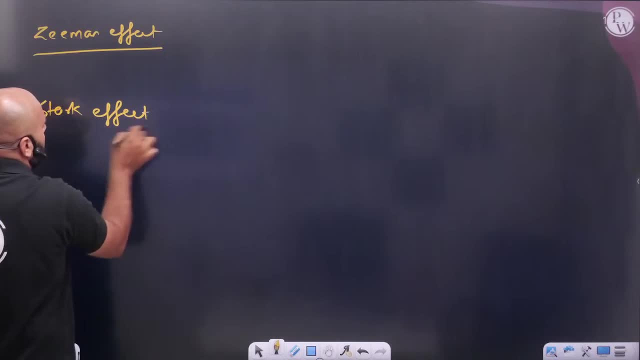 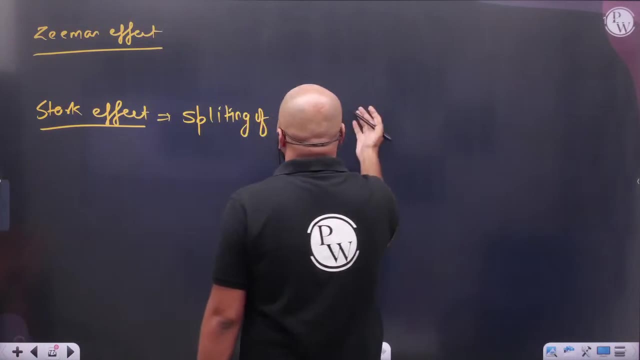 Stark effect means splitting of spectral lines. There is splitting of spectral lines in all. Here too, splitting of spectral lines is happening In both cases, in presence of electric field. in presence of electric field, we call it Star effect. In presence of magnetic field: 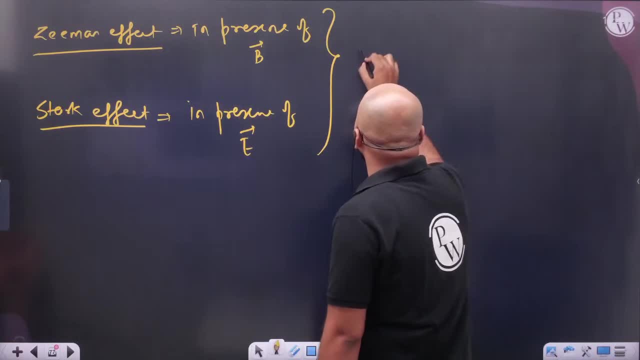 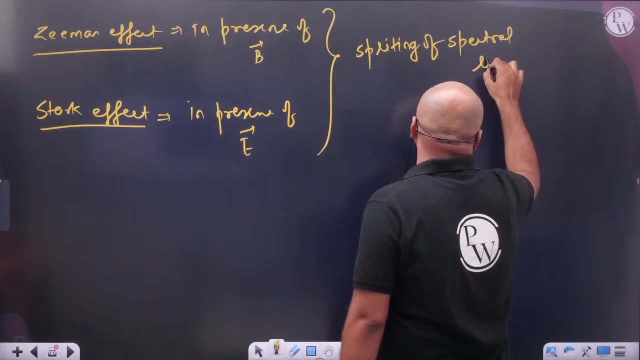 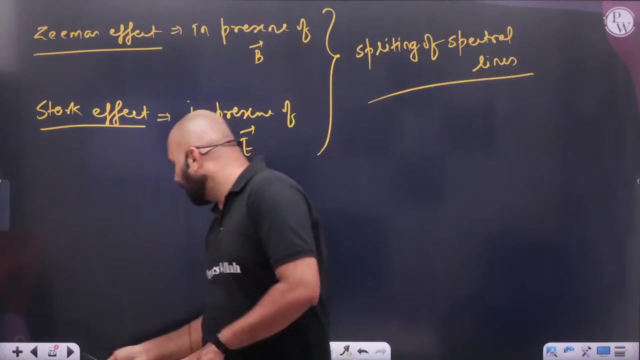 we call it Zeeman effect. In both cases, there is splitting of spectral lines. There is splitting of spectral lines. There is splitting of spectral lines. These are small things. Now, who breaks the lunch break? Let's take a break. I will not give more break. 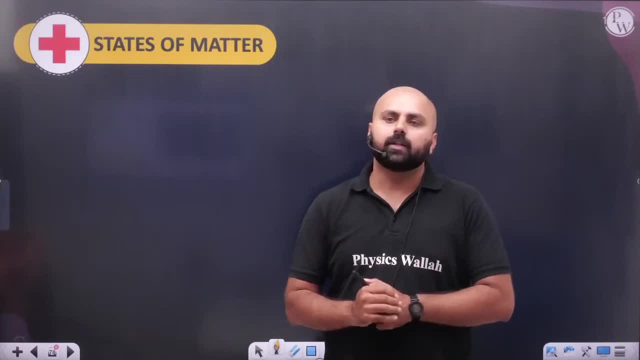 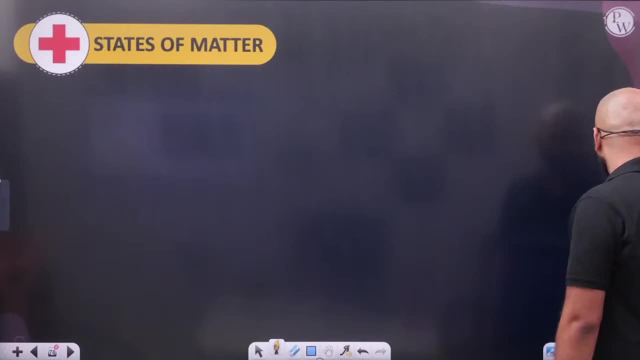 If I give more break, the momentum will disappear. We will get 30 minutes break at night when it will be time to eat. Now we will take 15 minutes break and then we will start the states of matter. Let's start the states of matter after 15 minutes break. 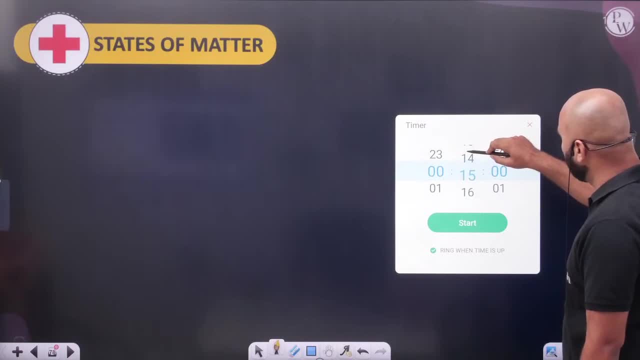 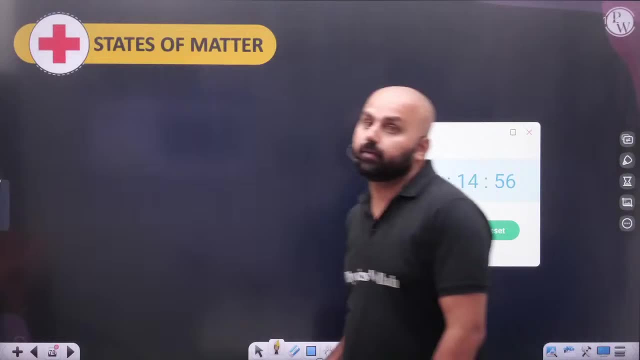 Let's take 15 minutes break. Maximum 2 chapters are over. This is a big journey. Let's try a little. Let's meet after 15 minutes break. Everyone get ready quickly After 15 minutes break. You can remember Stark from Tony Stark. 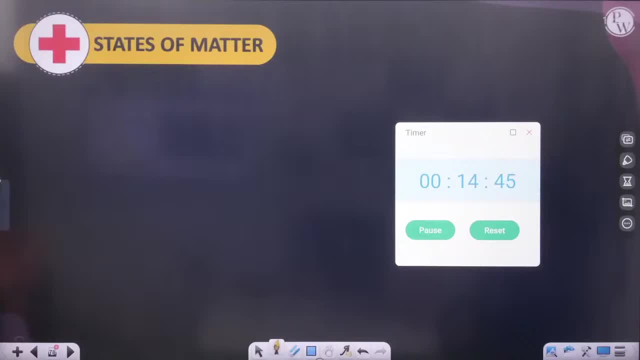 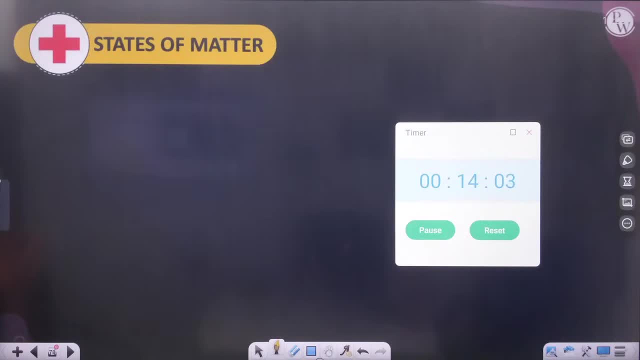 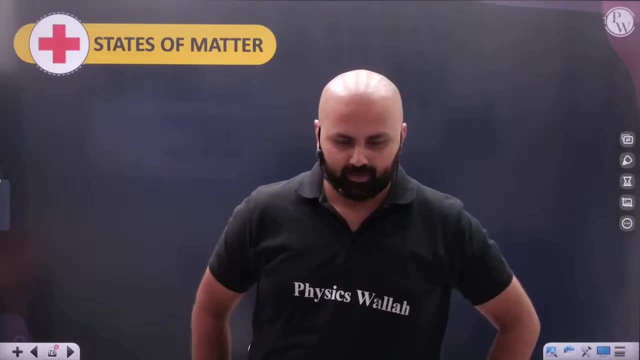 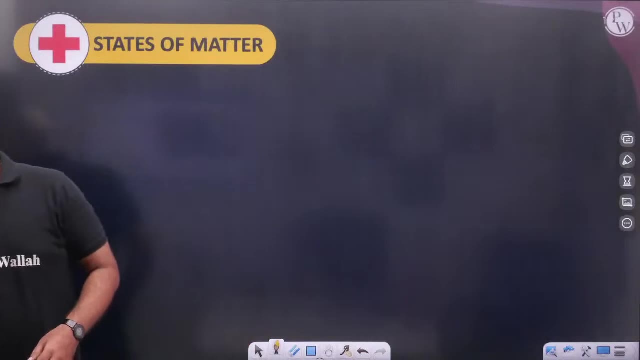 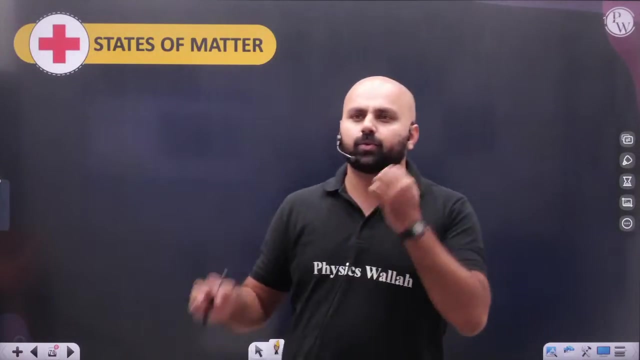 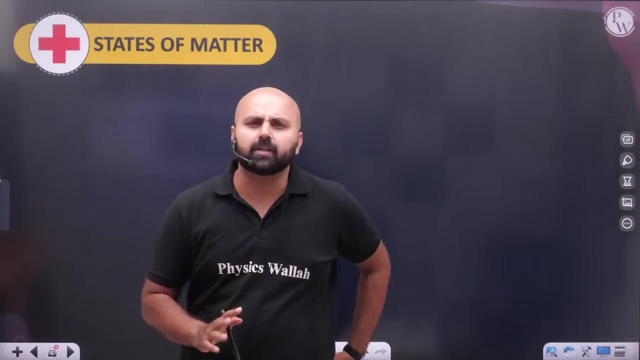 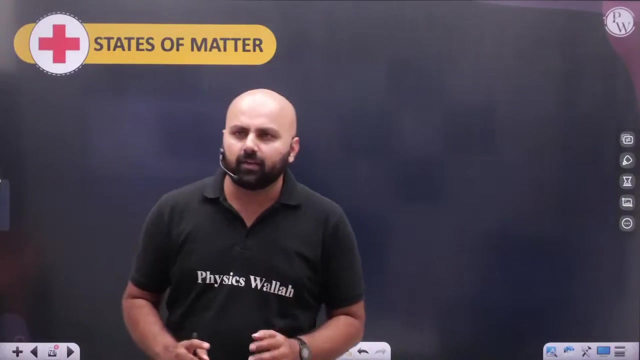 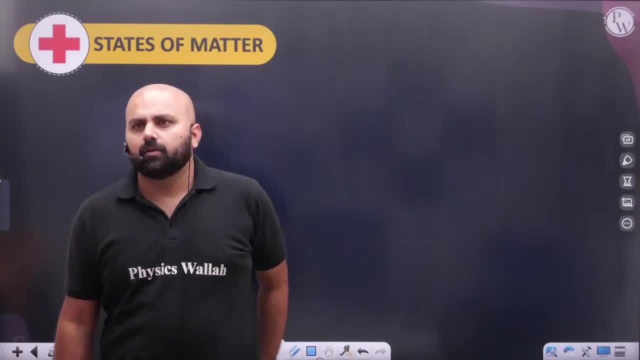 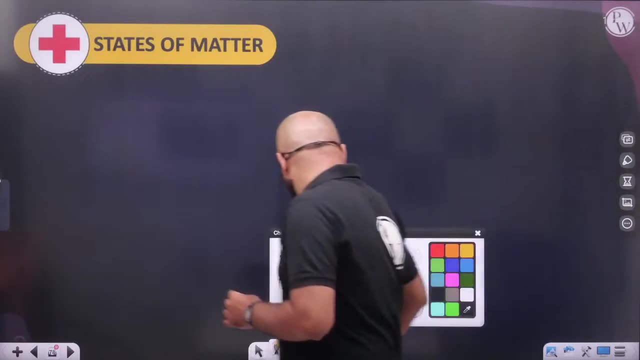 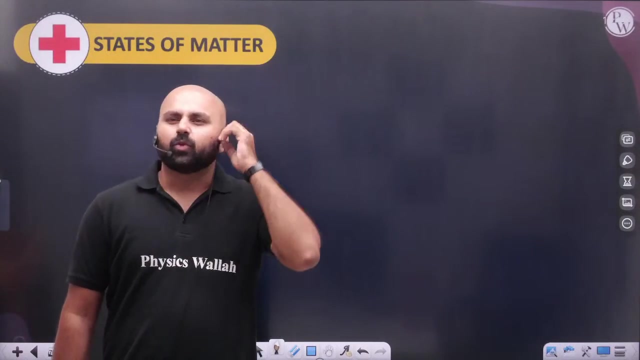 Okay, okay, Arjuna brother, what are you doing here? there is a lot of things left in your life. you wait now. when your time comes, then we will talk about your time, okay? Yes, let's balance both as much as possible. let's do formulas and theory and let's keep a little time limitation in mind, because then it is the same thing that if it is too long, then there is no use. I was talking about the state of the matter. let's define simple things in the state of the matter. 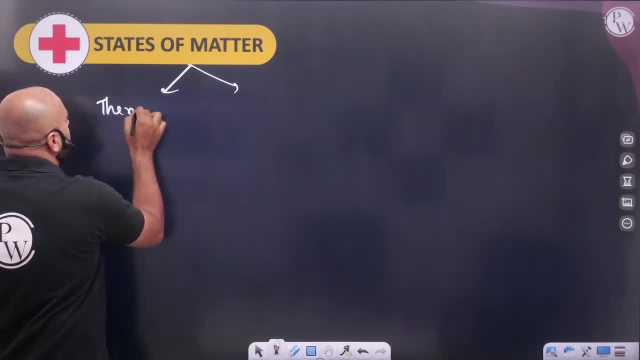 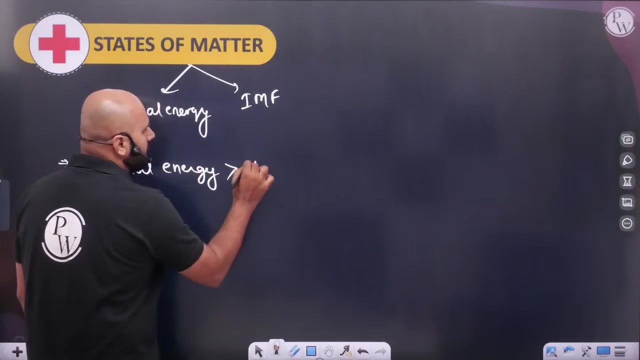 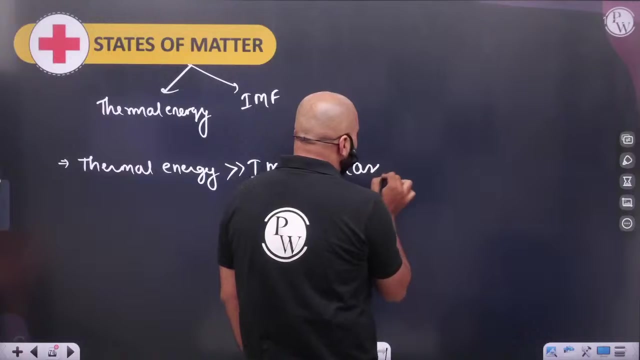 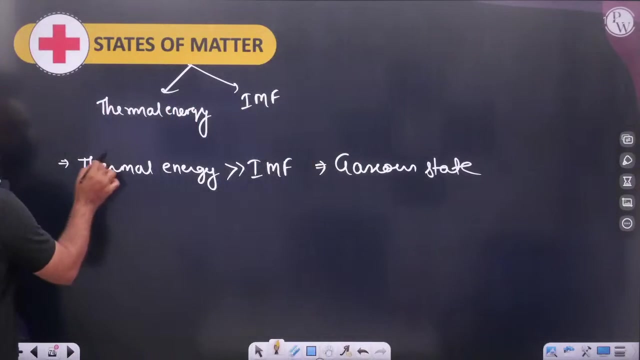 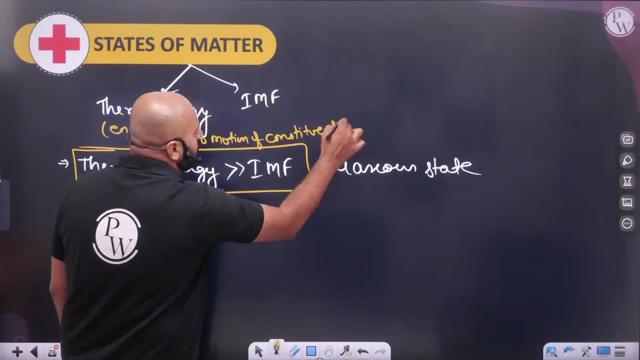 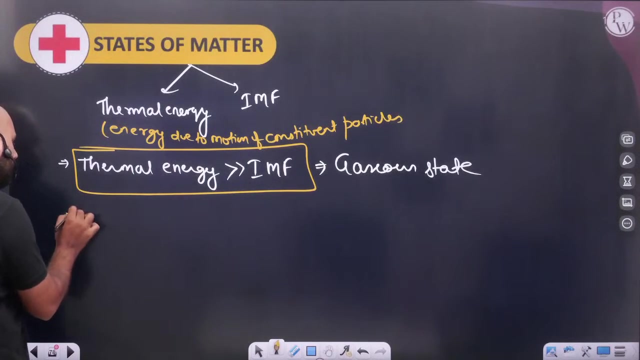 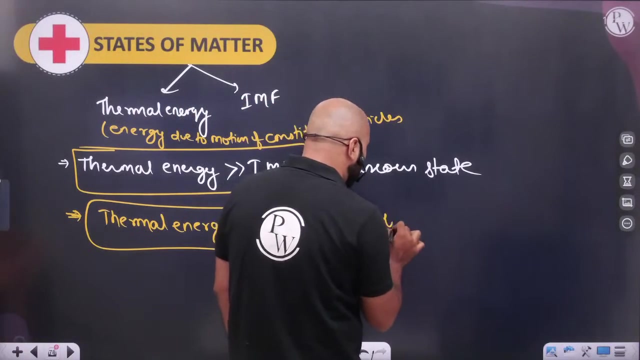 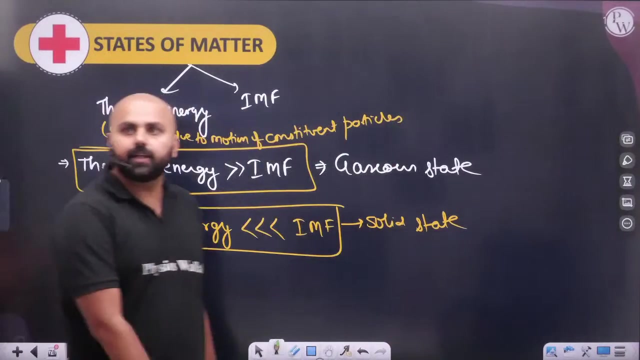 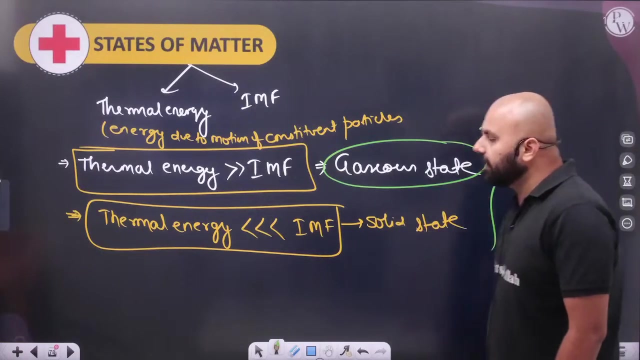 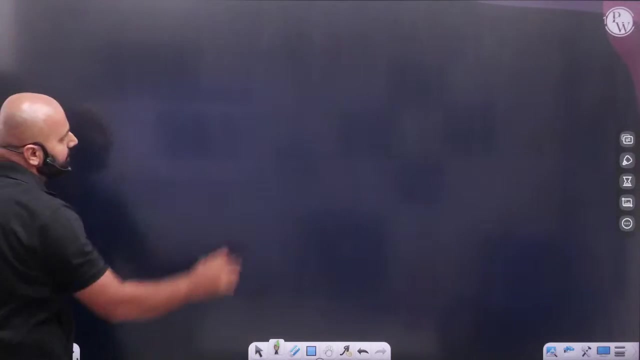 Okay, So in this case our next chapter of the twelfth will come and that will be called solid state. brother, the first thing that is defined in the state of the matter, it is defined here, solid state, and this liquid state. then after that, if we talk about thermal energy, intermolecular force, then we come to the gaseous state. now in the gaseous state I have four gaseous laws. there are four gaseous laws, but if we talk about gaseous laws then we will try to read all the gaseous laws together. how then see? 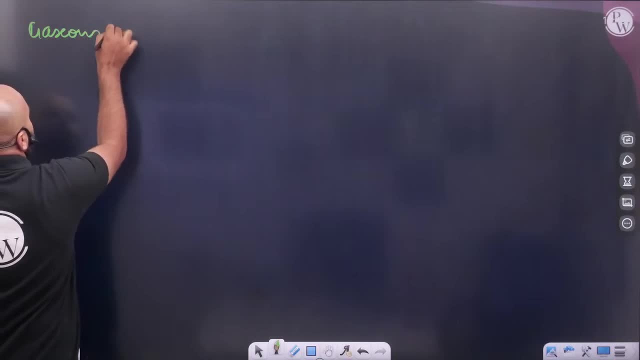 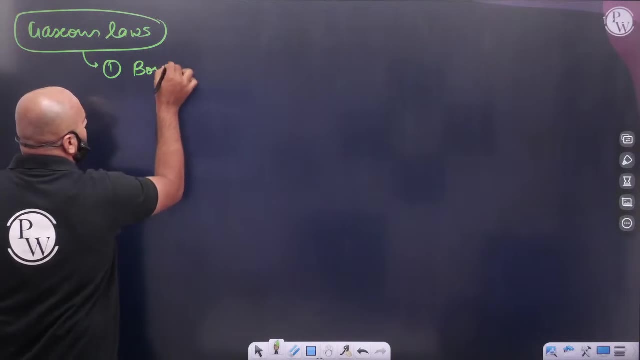 okay, Then we will talk about gaseous laws. so, guys, Gaseous laws. what will I get? see what you will get in gaseous laws. first, wilds, what is called by this wilds- nothing. if you are a wilds, what is in the world, the one who stays constant, is the temperature. 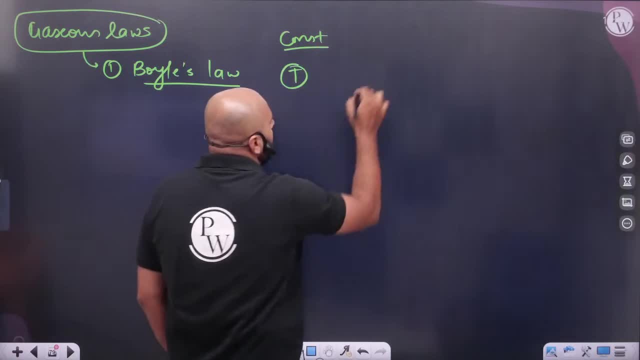 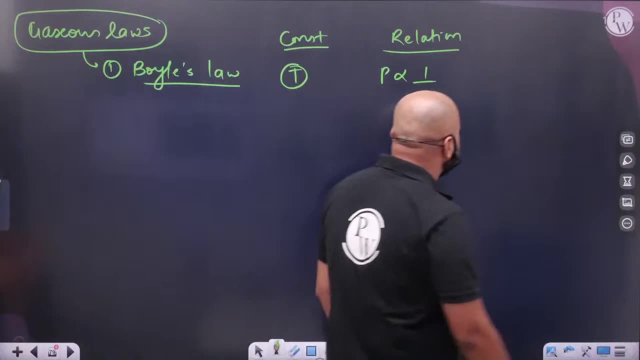 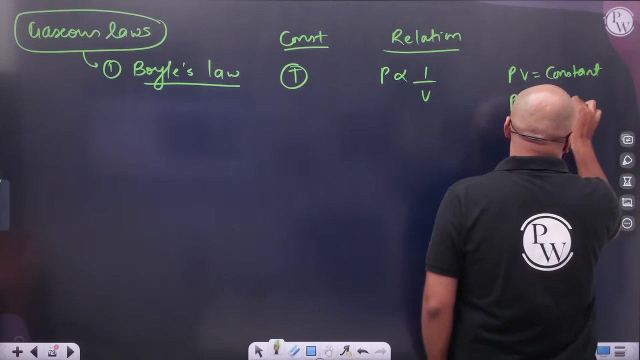 Generally temperature. The temperature is constant, then what happens? the relationship you will see here? Then what will happen? relation pressure En Glasgow và Pia, supposed two after your Pia, spaces are three As equals to 2 Const constant. P1- V1 is equals to P2- V2.. This formula comes to us: PV is equals to constant In. 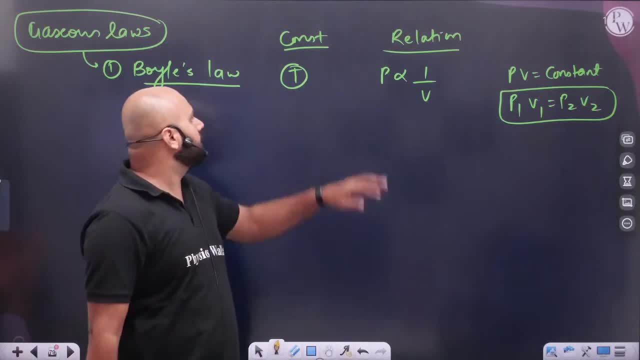 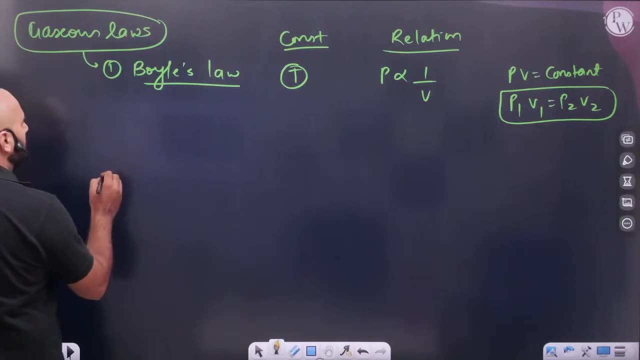 Weyl's law. this is what we have to say For sure. See this In Weyl's law: temperature constant P is inversely proportional to volume. PV is equals to constant P1- V1.. If I talk, 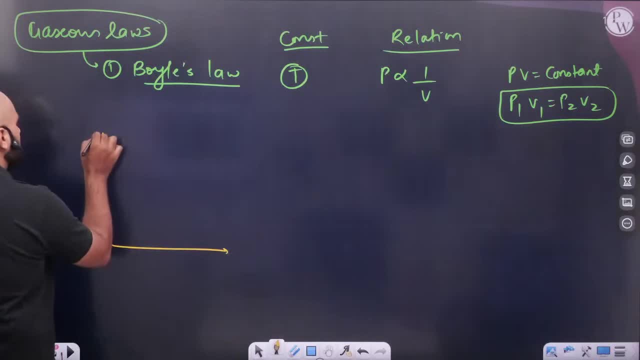 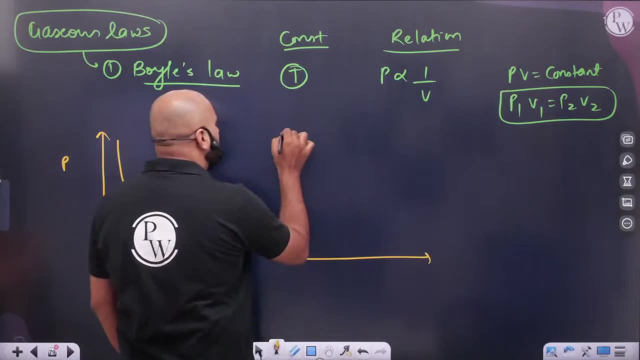 about graph, then pressure versus. if you make a graph of pressure versus volume, then inversely proportional graph will be made. If you make a graph of pressure versus 1 by V, pressure versus 1 by V, then directly proportional graph will be made. PV. if you. 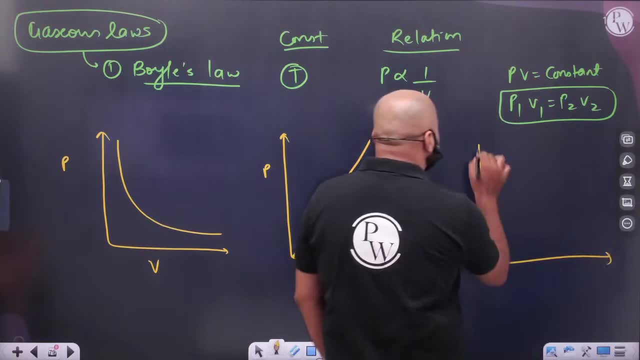 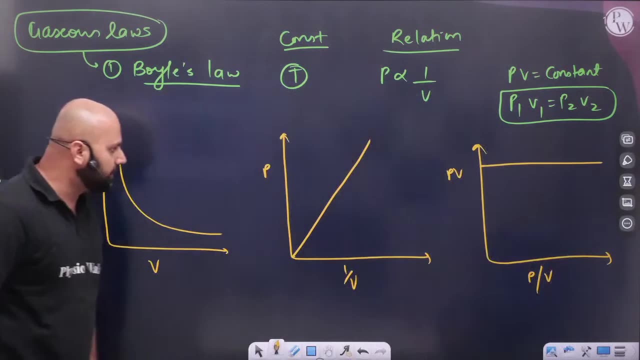 look carefully at all the graph of PV in R, visibility per se, inamat of P and V, the constant will come. Why? Because if you change the pressure, the volume will adjust itself. If you change the pressure, then the volume will adjust itself. So see this: If you change, 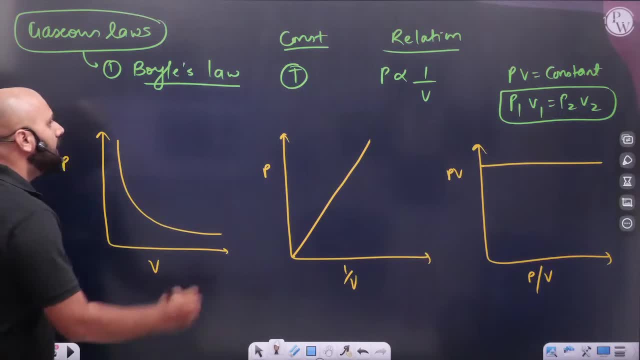 the pressure, the volume will adjust itself. So the graph of PV is equal to constant. Let's take out one or two more things from here. Sir, if I want to take out the slope, then dP by dV, if you see, in isothermal condition. 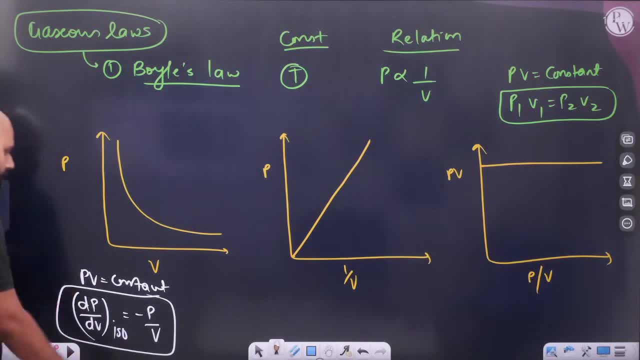 then what happens? It becomes minus P by V. If you see, in isothermal condition then it becomes minus P by V, Or if I want to write this correctly, then I can write this also: Log P plus log V is equal to log K. 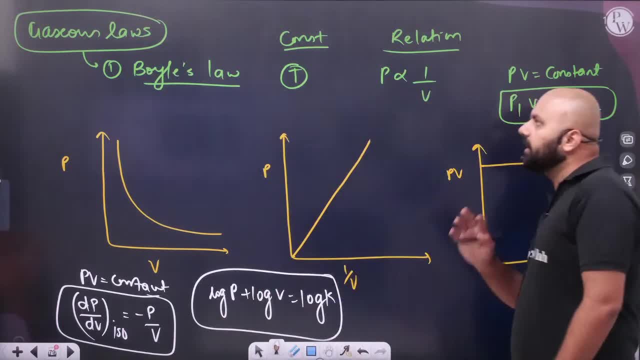 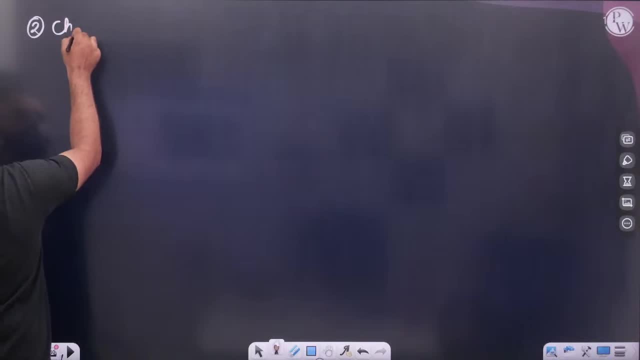 So this equation can also be written. The graph of this can also come. So this happens in Boyle's Law. This is seen in Boyle's Law. If we talk about Boyle's Law in Charles's Law, If you see about Charles's Law, 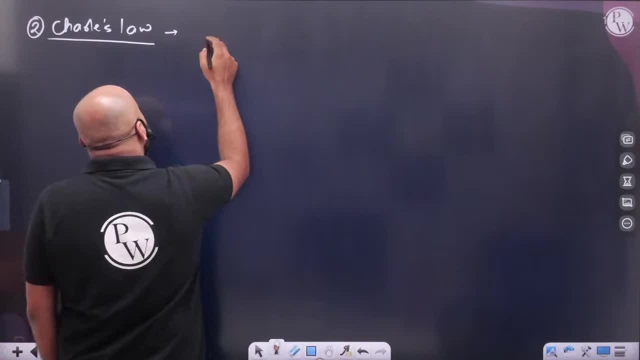 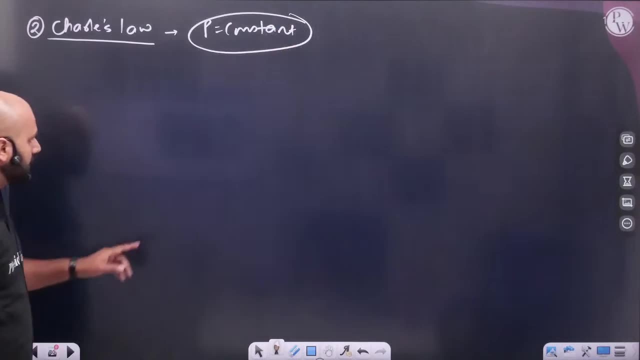 then Charles's Law says that: Sir, what will be your constant? Sir, what will be your constant? The pressure will be constant If pressure is constant. all these graphs that you have created, all the graphs that you have created, temperature constant graphs that you have created. 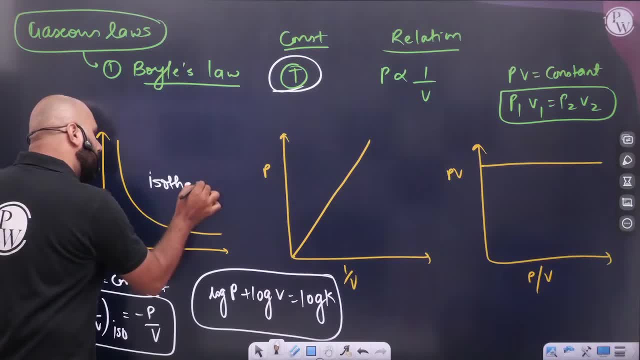 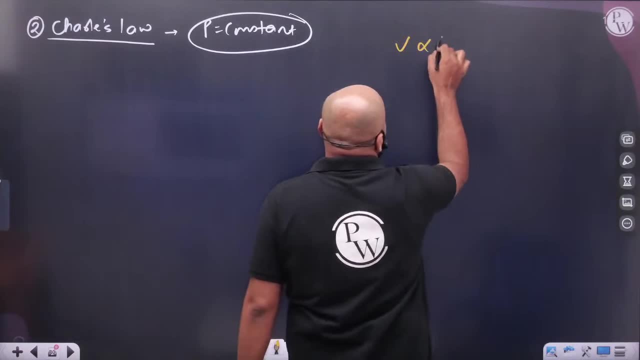 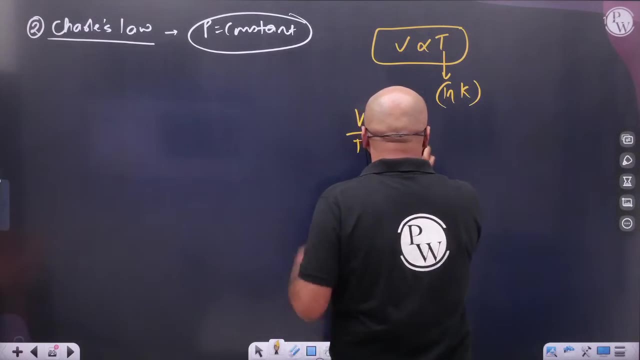 then all these graphs are isotherms. All these graphs are isotherms. Similarly, here you can see, is constant and here it is seen that volume is directly proportional to temperature. Just remember that the temperature should always be in Kelvin, Sir. V by T is constant. V by T is constant, and 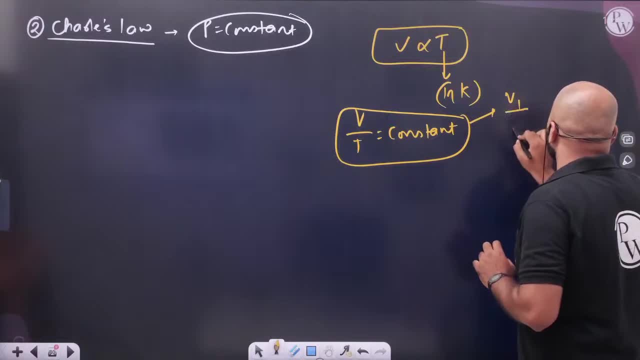 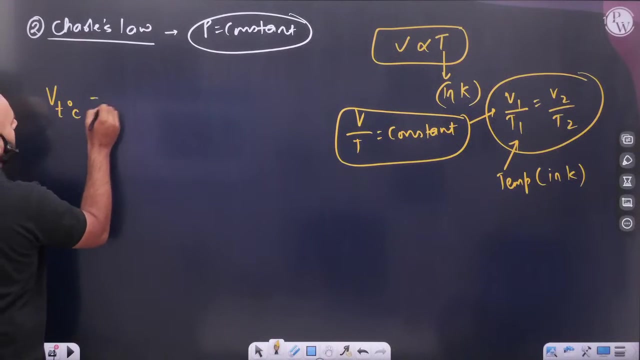 if V by T is constant, then a relation comes here: V1 by T1 is equal to V2 by T2.. In all these, the temperature should always be in Kelvin. The temperature should always be in Kelvin. Remember one relation: VT degree Celsius is nothing. V0 degree Celsius plus V0 degree Celsius. 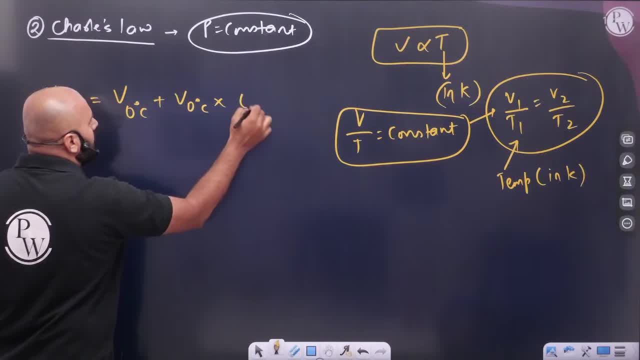 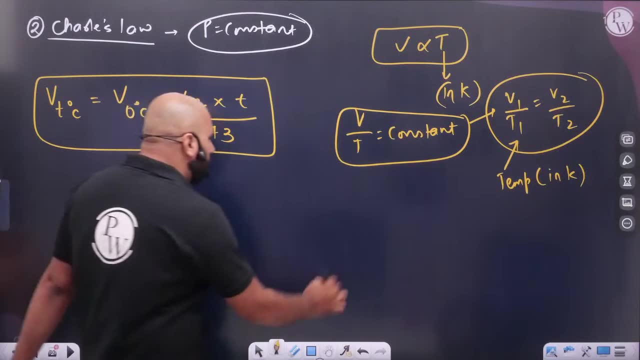 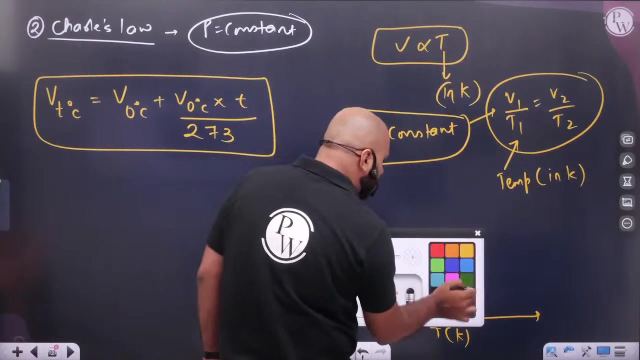 into T degree Celsius or T divided by 273.. If someone asks in degree Celsius, then he will have the option. Remember, when you make a graph of V and T, if the temperature is in Kelvin scale, then a directly proportional graph is formed. A directly proportional graph is formed, but 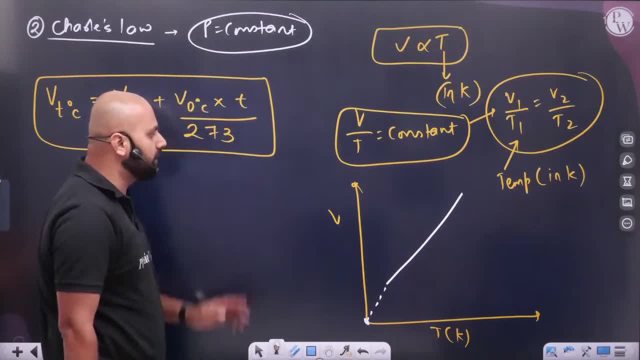 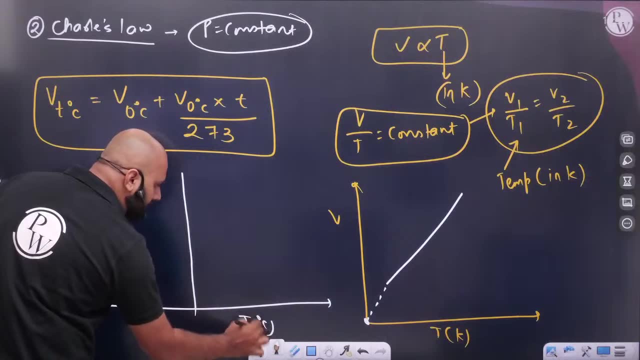 it starts from the origin. Why? Because zero Kelvin is not the possible temperature. But if the same graph is formed, behind whom? If the temperature is formed in degree Celsius, then if you see the graph of its volume, then the graph will be here. How will it be? If the graph is seen, then you will see here: This is minus. 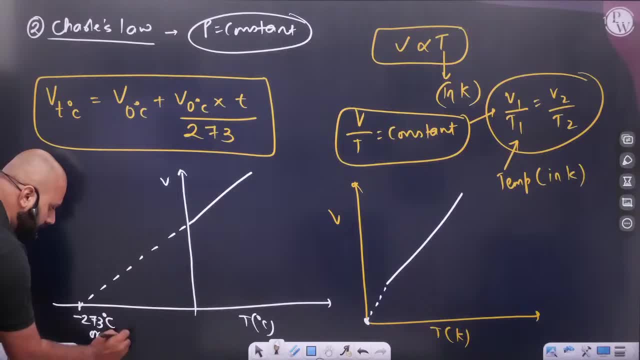 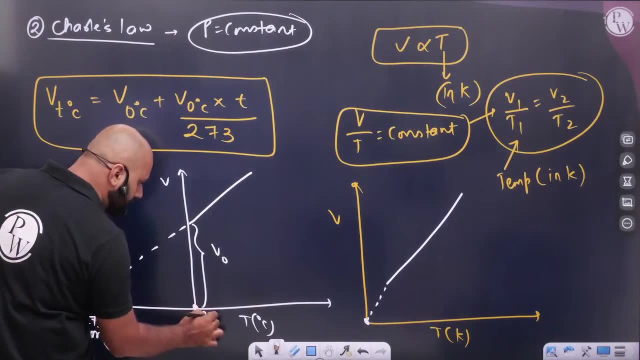 273 degree Celsius, or what do we call this? Zero Kelvin, This intercept. what do we call this? We call it V naught. This is 0 degree Celsius. this is zero degree Celsius. Remember the difference of both the graphs. 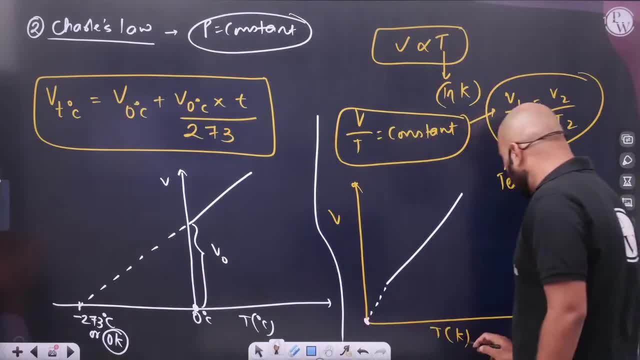 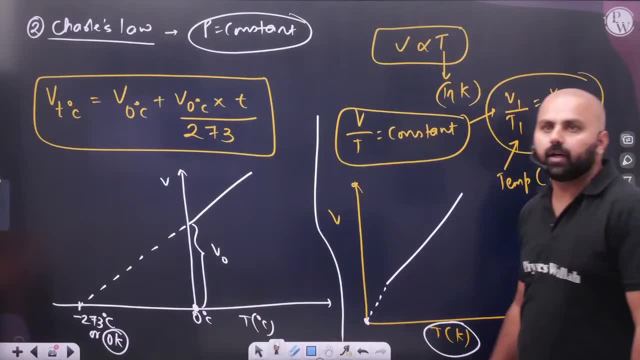 remember the difference of both the graphs. if you make a graph of volume and temperature in its Kelvin, then straight line. If you make a graph of it, it will not pass through the origin, but it will pass through it. It will surely pass. So you have this Charles law In Charles law. we know this comes after that, if you. 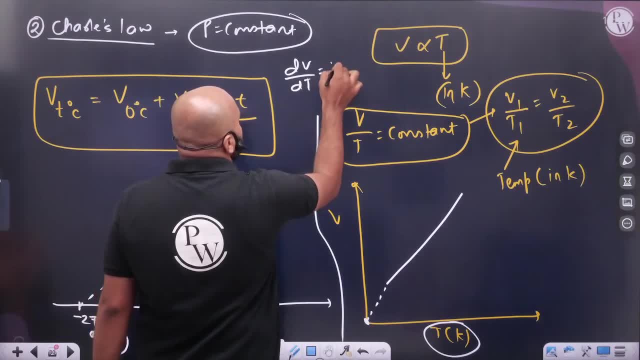 want here, then DV by DT. DV by DT is nothing. V by T will come. If you want to calculate, do it yourself. Who comes after Charles law's just? If you want to calculate, do it yourself Who comes just after Charles law. 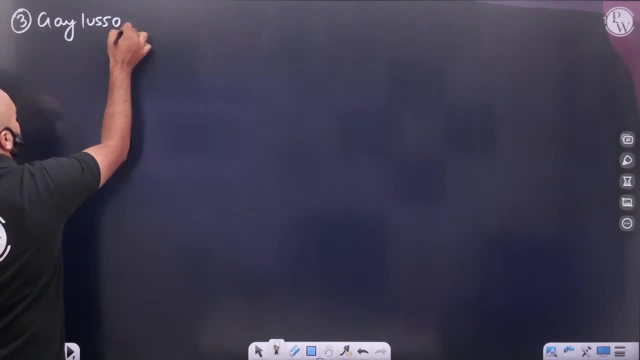 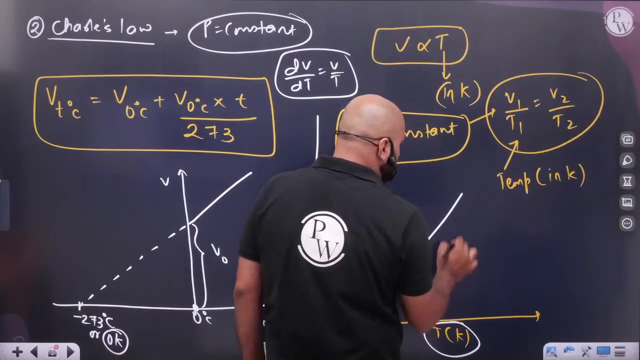 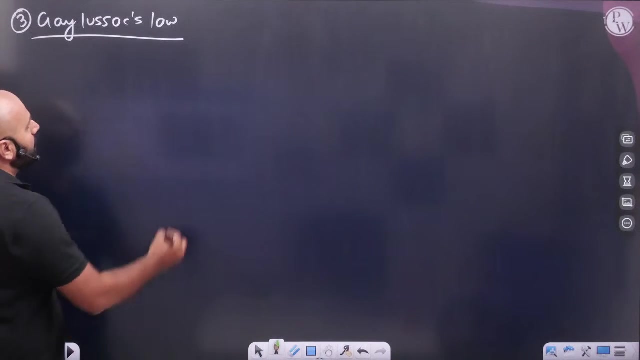 In Charles law and Geluzak's law. there are a lot of similarities. In all the graphs, pressure will be constant. In all the graphs, pressure will be constant. These graphs are called ISO bars. Where pressure is constant, there is an ISO bar. 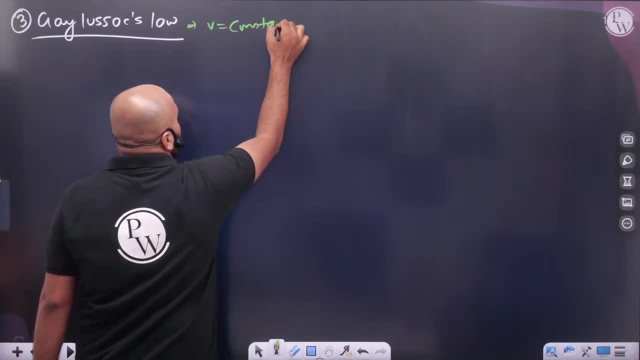 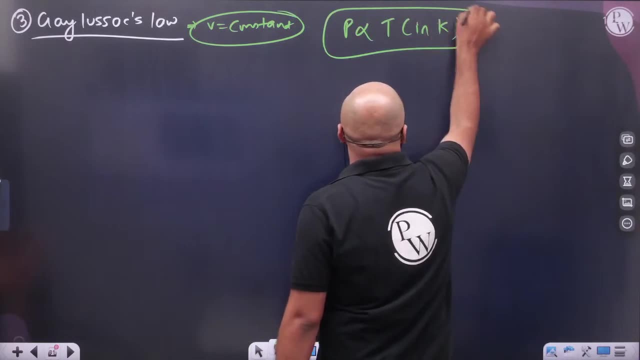 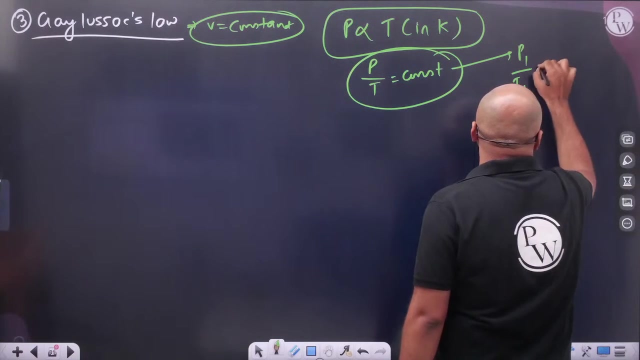 In Geluzak's law, volume will be constant. Pressure is directly proportional to temperature. Pressure is directly proportional to temperature. Remember temperature is always in Kelvin scale. P by T is constant. P by T is constant. P1 by T1 is equal to P2 by T2.. 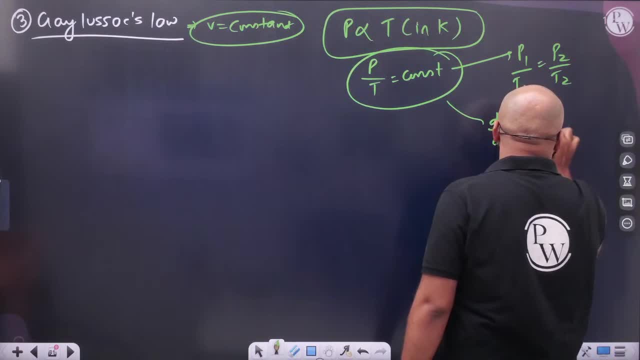 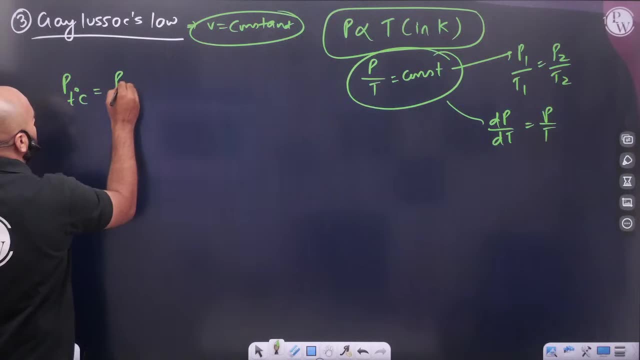 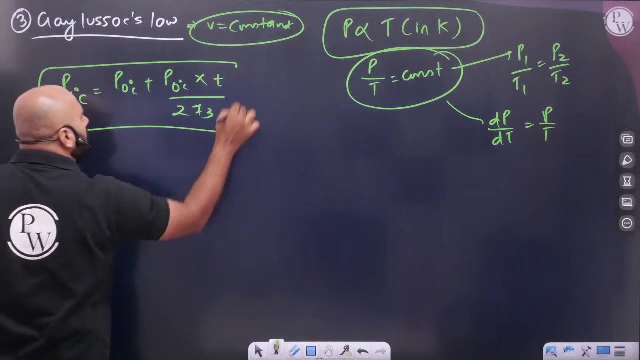 Or we can say: Dp by Dt is nothing, P by T, Again, if I talk about pressure directly proportional to. Again, if you want to calculate P at T degree Celsius, then we will take P by P0 by T into T by T2 by T3. 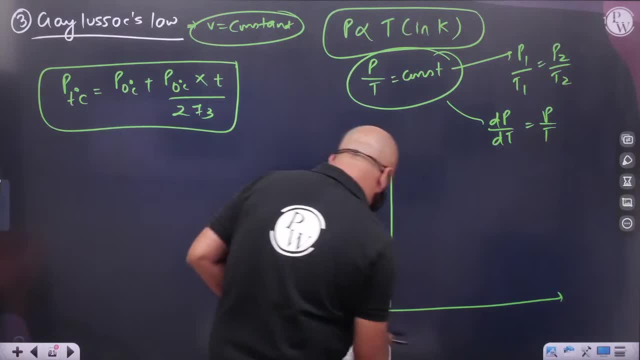 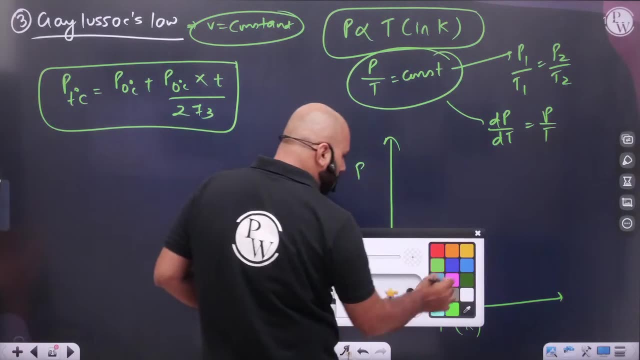 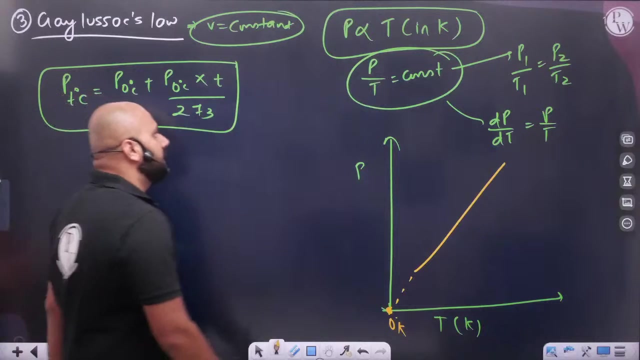 The similar formula which was there Here also. if you see the graph, it will be like this. If you see the graph, you can get this: Take temperature at Kelvin. If you see graph, then how it will come. Sir, it must be coming like this: 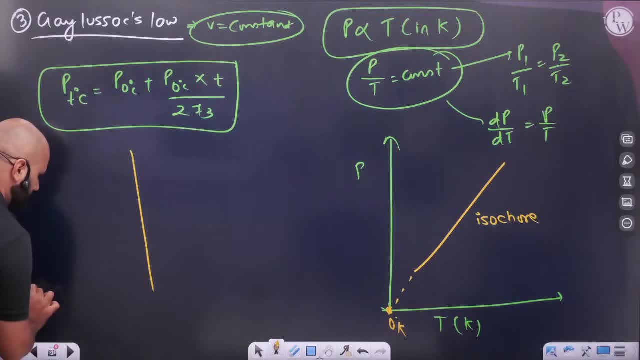 isochoric graph. and here, if someone told you that no, sir, temperature is to be taken in degree Celsius, pay attention to the temperature. when it will be in degree Celsius, then the graph will be minus 273 degree Celsius, or 0 Kelvin, or 0 Kelvin, then we have a pin of 0 degree Celsius. 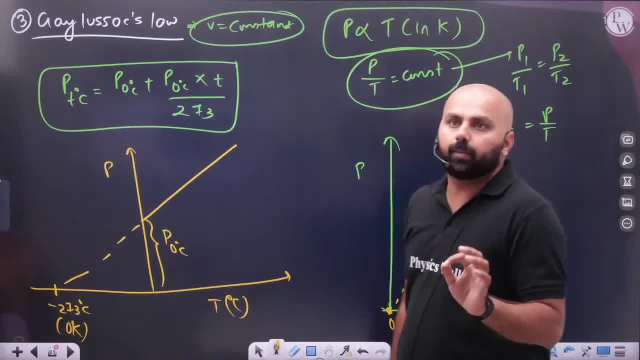 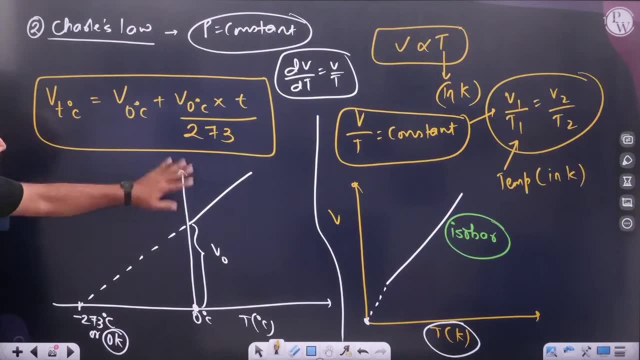 this will be such a graph. keep in mind, keep in mind the graph of both. remember, in the graph of both, brother, these things will happen. see this with you all these constants are V by T, volume, temperature. take the constant of all these. work according to this. the rest are these three laws. 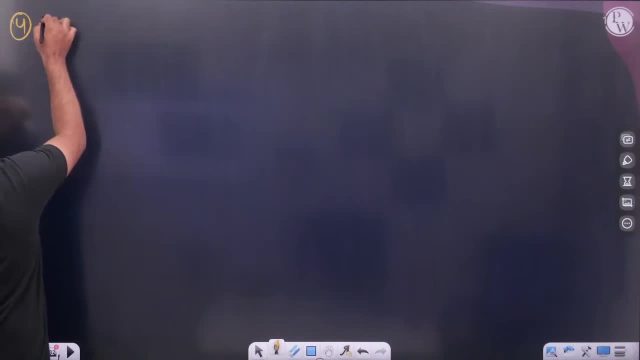 these are the three laws, and above them, the fourth law is the easiest: the FGadrow's law. the FGadrow's law is the easiest, that brother, if the pressure and temperature are constant, if the temperature and pressure are constant, if the temperature and pressure are constant. 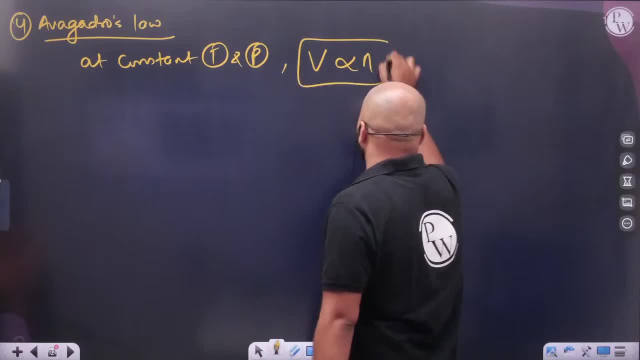 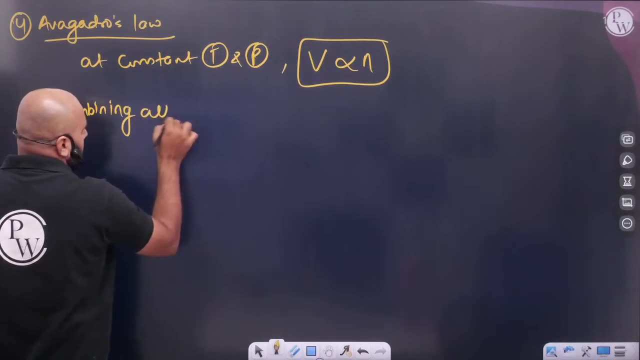 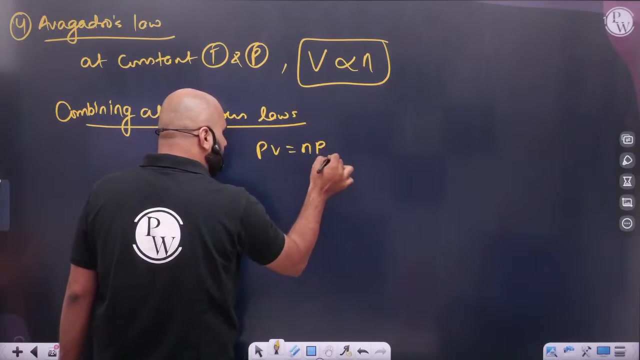 then in that case the volume will be inversely directly proportional to number of moles, with all of them put in. all the laws combining the gaseous laws of all are gaseous laws. so finally, what we get is that PV is equal to n RT. 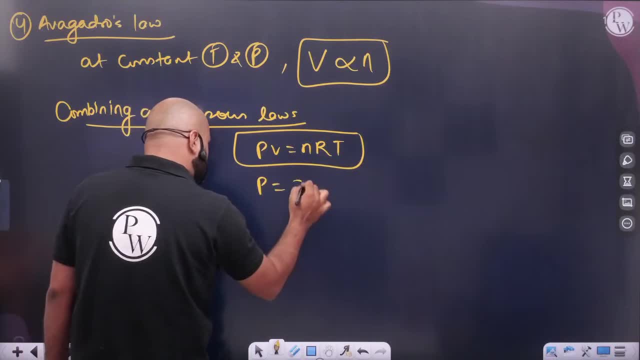 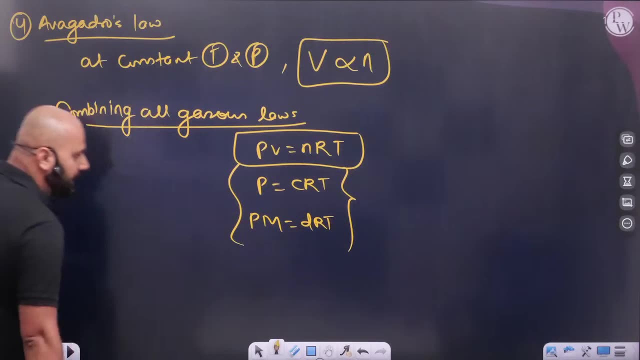 it is a little earlier explored, P is equal to CRT or PM is equal to DRT, then I said this in by just that recent basic concept. then I also Krishnaier also that it is nothing. molar mass of the gas is divided by 2. 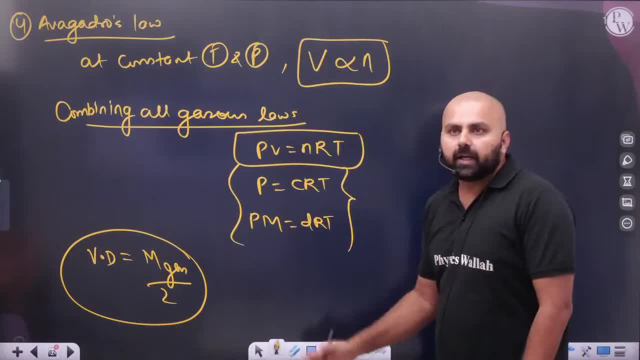 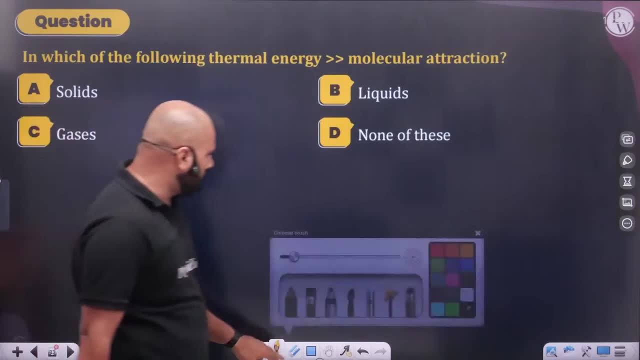 So keep doing the ideal gas equation vapor with yourself. Now look at the questions. Look at the questions. What will be the questions Like this question is given: Quickly tell the answer. Quickly tell the answer. What will be its answer? 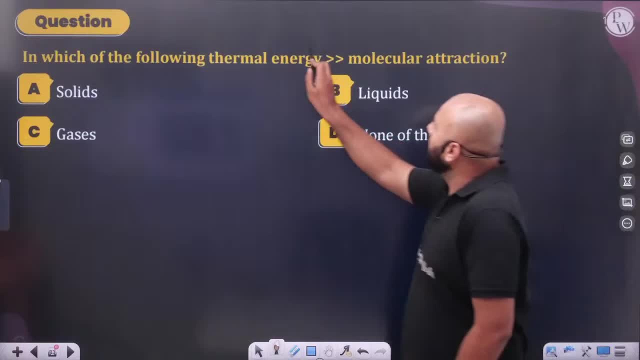 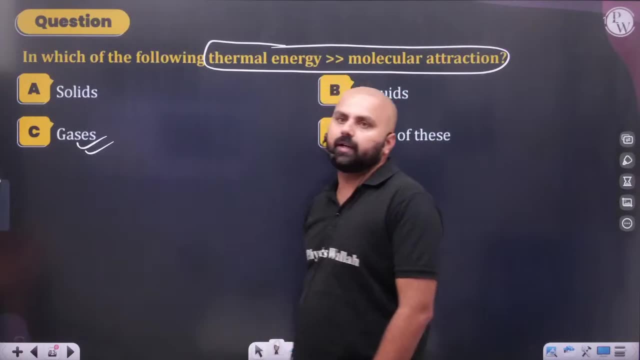 What will be its answer? What will be its answer? What will be the thermal energy Greater, greater than molecular attraction? Who has more Thermal energy is more. What will happen? Who are you In gaseous? Who are you? 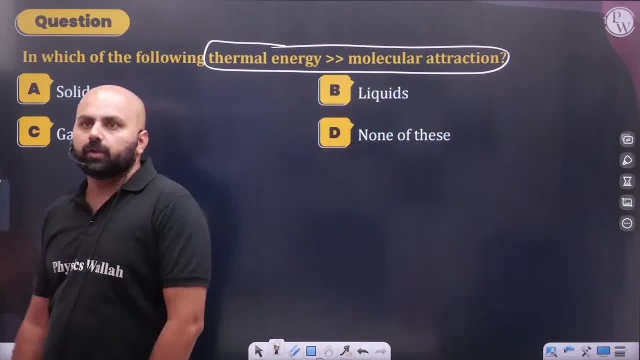 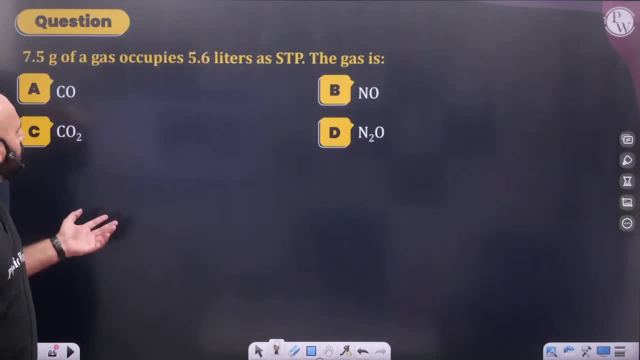 In gaseous. Okay In gaseous, Nothing else. Okay In gaseous. Look at the next question. Look at the next question Again. this question is repeated. Quickly remove it. This is repeated. The original concept. 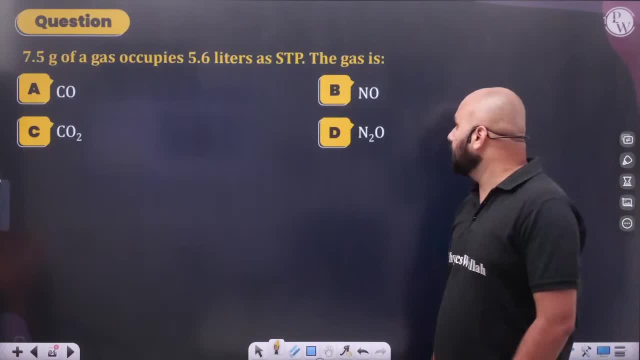 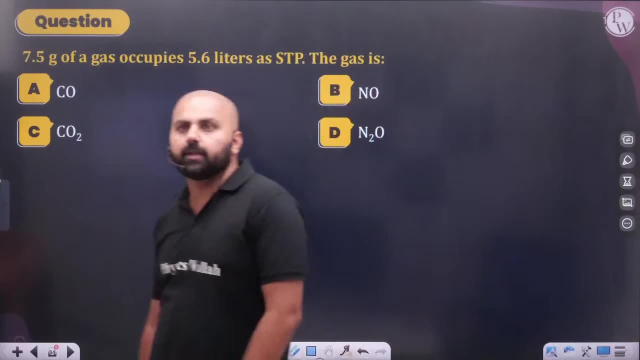 This is repeated, But no problem, Remove its answer. What will be its answer? What will be its answer? You all know the molar volume. You all know the molar volume, So remove it according to the molar volume. 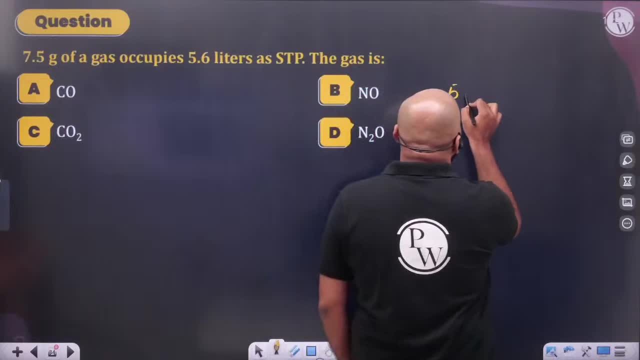 What will happen? See, Sir, 5.6 liters, 5.6 liters. How much is that? 7.5 gram, Sir? how much will be a liter? 7.5 upon 5.6.. How much for 22.4 liters? 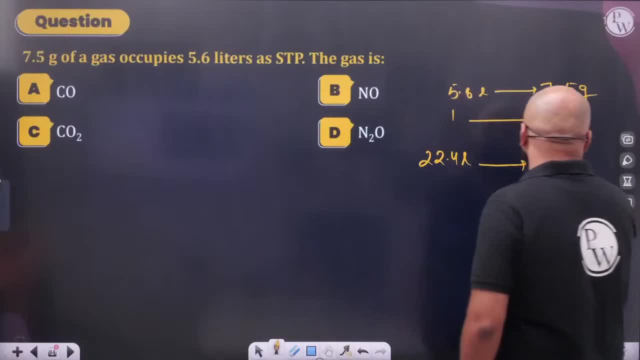 7.5 upon 5.6.. How much for 22.4 liters, 7.5 upon 5.6.. It had been done right at the start. it was done at the start. 30 gram, 30 gram molar mass has come. 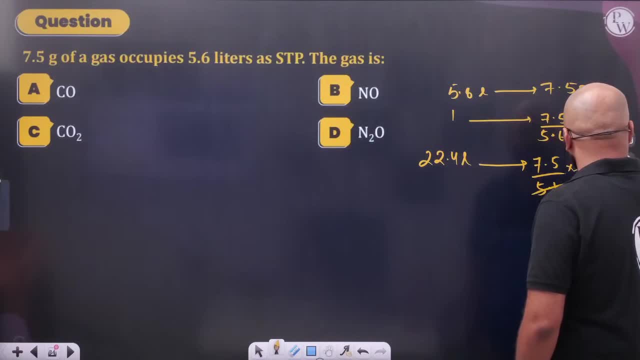 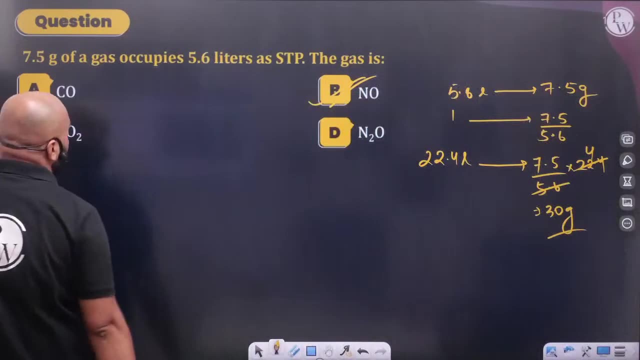 30 gram molar mass is using B. Okay, Do the next question. Do the next question. The curve of pv and p is slow. Pv and p have not given edeflate like indic minorities at present. CThe curve of pv and p is slow. 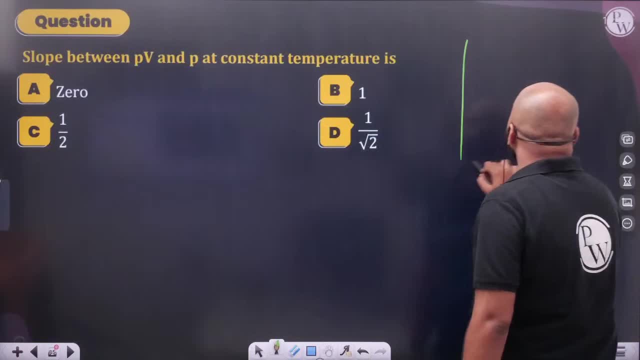 And now pvi and p p. Neither slog of p or p, or p or na�lui. So we have applied this curve Pv and p is curve. how would be Think for yourself how would be. pv and p is curve. 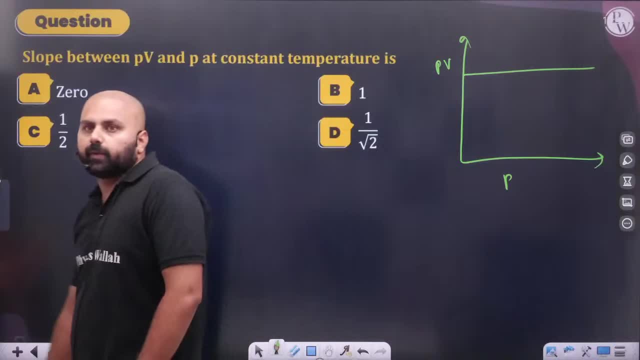 How would be? pv and p is curve. What would be its slope? Pv and p is curve's slope would be: How much would be the slope of pv and p? What would be the slope? How much would the slope be? Slope between Pb and P at constant temperature. 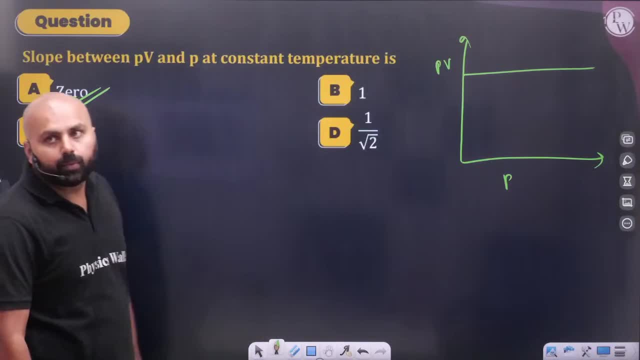 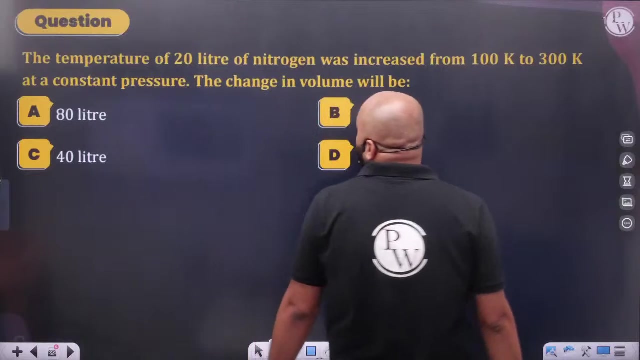 Sir, please look at the slope. what will be your angle? How much will be the slope? It will be 0. Slope 1: How will it be 1?? It will be 0. Look at yourself. Look at the questions. What is being said? 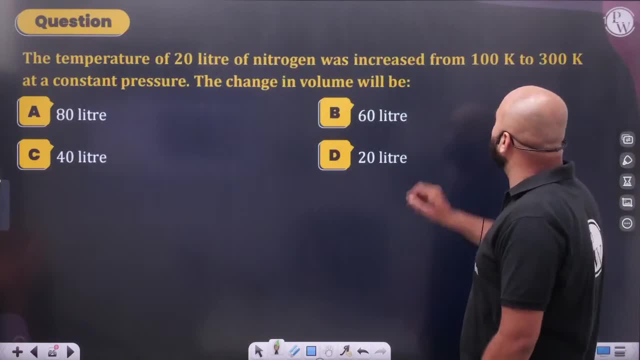 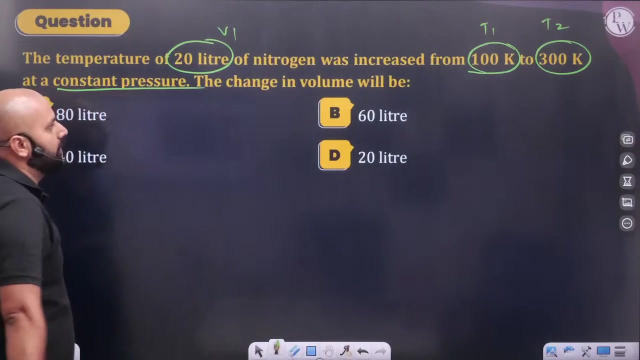 Look carefully. Temperature of 20 degree L of Nitrogen Increased from 100 Kelvin to 300 Kelvin, From V1 to T1. This is T1 and this is T2. Sir, your volume is V1. What is being said? You are doing it at constant pressure. 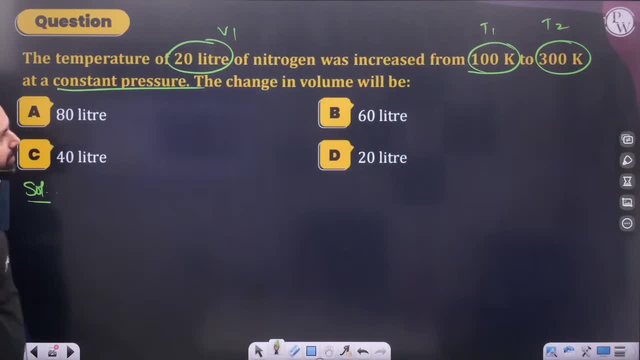 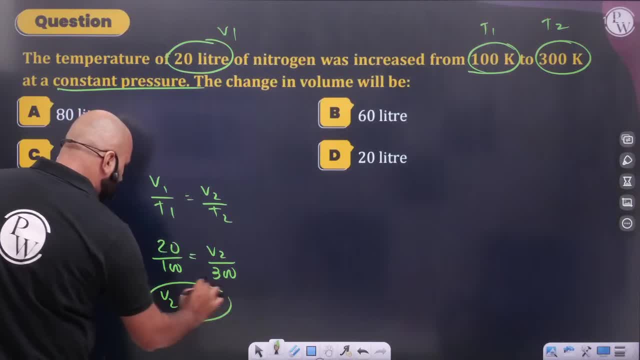 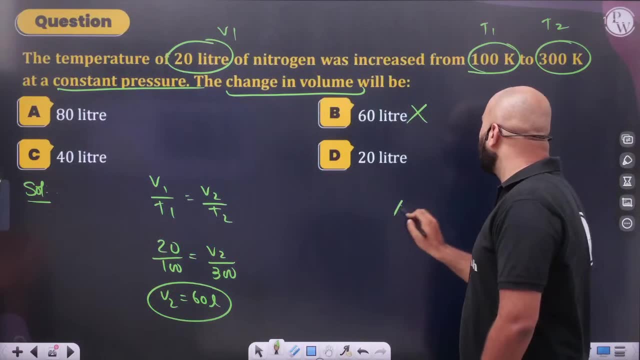 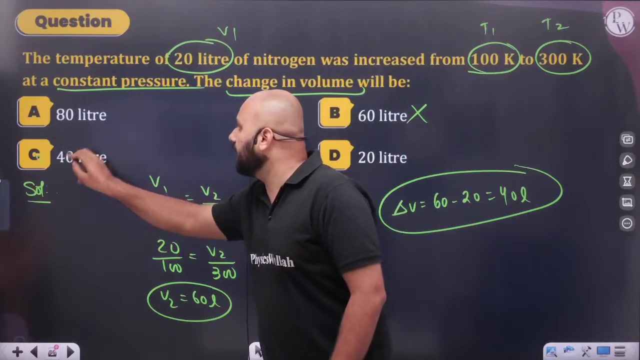 What will happen to V2? 60 liters? Now, here there will be no 60 liters option, Because look at the question, It is asking change in volume. It is asking change in volume. It is asking delta V. What will be delta V 60 minus 20, 40 liters? 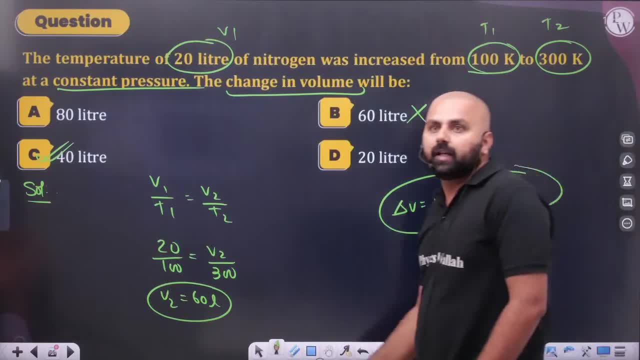 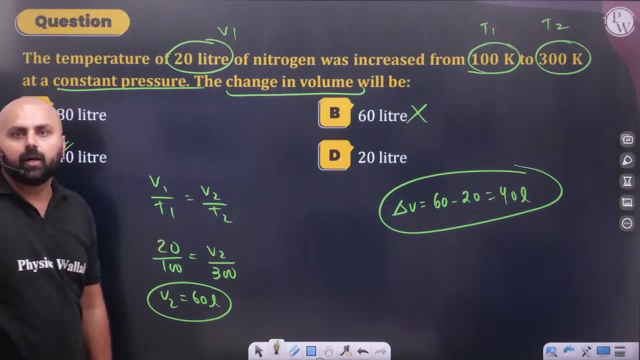 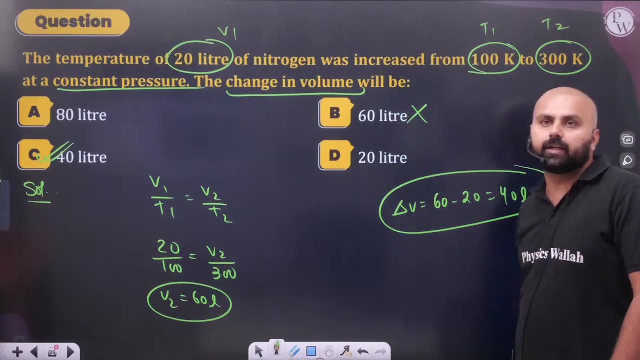 Brother. see the question. What will be the answer? C will be the answer. What will be the answer? C will not be the answer. Look carefully. It is asking change in volume. Don't get stuck here. Don't get stuck here. It will not be 60 liters. 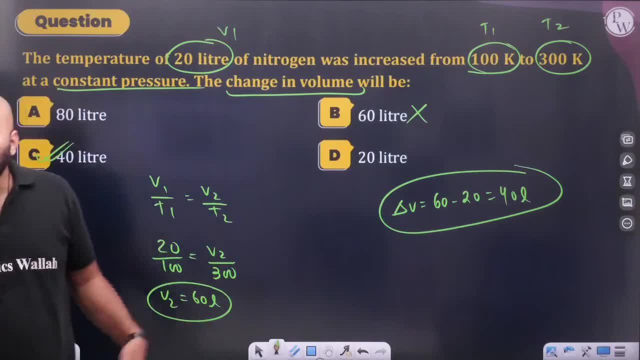 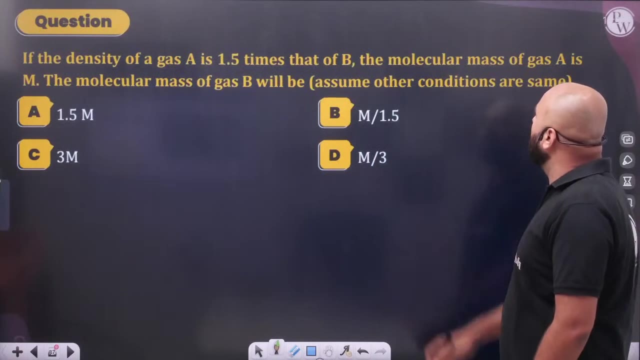 It will be 40 liters, Nothing else. It will be 40 liters. How will you know It will be 40 liters? Look at this. Look at this question Again. Density of a gas is given Molar mass of A, Molar mass of B. Other conditions are same. 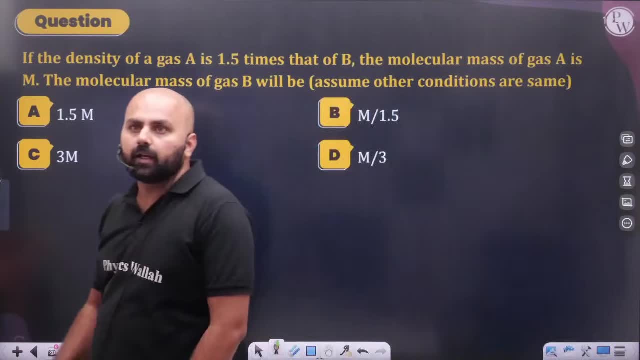 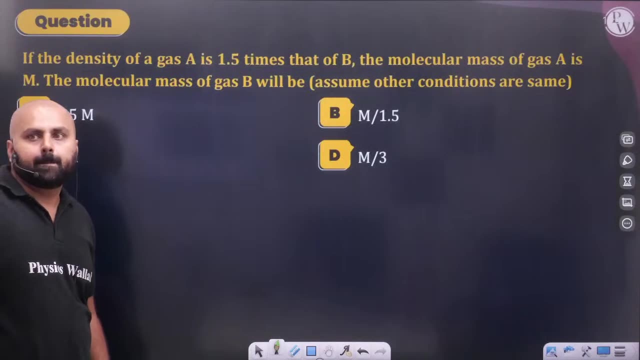 Will you tell what will happen? How will you find Molar mass of B? How will you find Molar mass of gas Fastly? What will happen Fastly? What will happen, What will happen, What will happen. What was the formula of density? 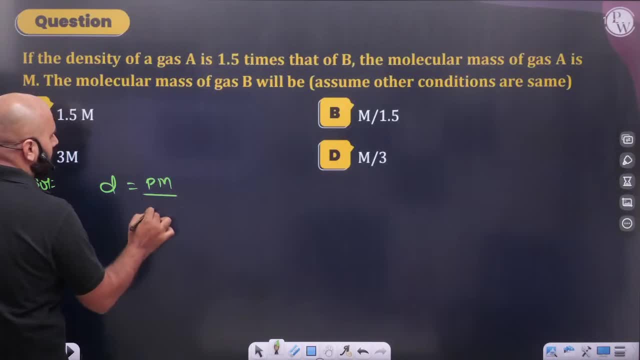 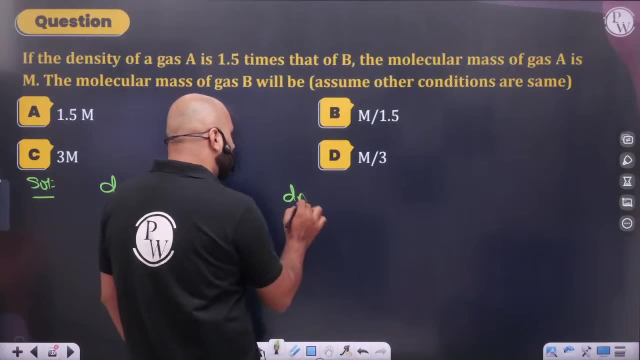 What was the formula of density? PM upon RT. Sir, if everything is same, Then density is directly proportional to Molar mass. Rest are same Density of A upon Density of B. What can I write? Molar mass of A divided by Molar mass of B. 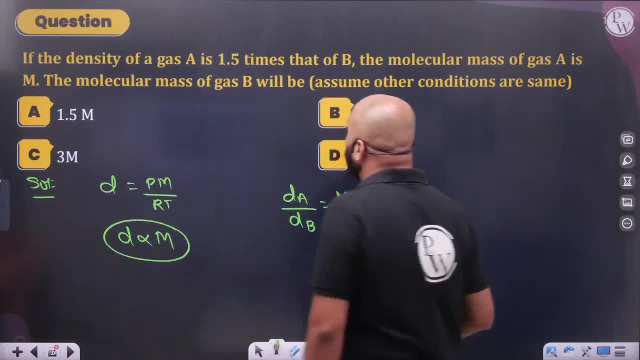 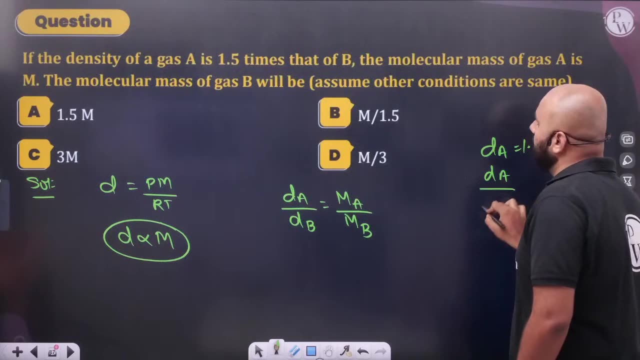 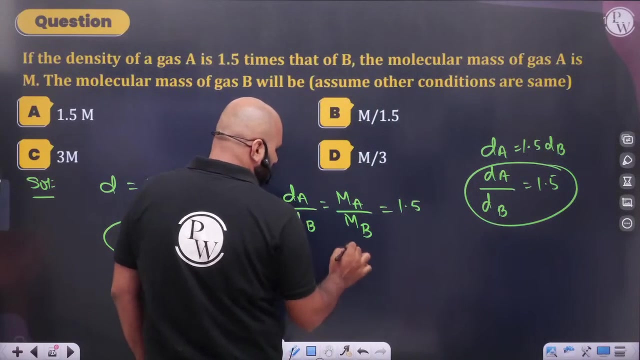 What can I write? So Molar mass of B. What did you write? Density of A is 1.5 times Density of B. Density of A upon Density of B. Density of A upon Density of B is nothing. Now put it 1.5. 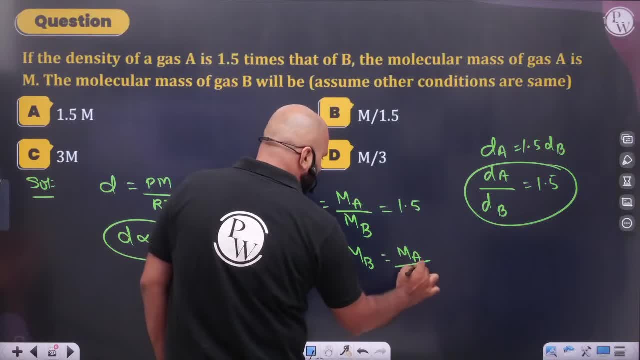 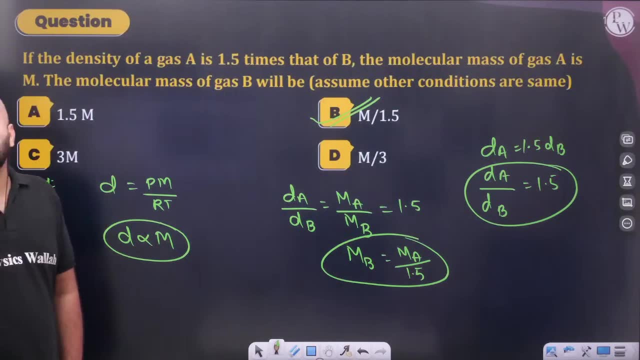 Molar mass of B is nothing. 1.5 Molar mass of A upon 1.5, How much will it be? B option will be. What will be the option? Density is seen directly. Rest of the conditions are same. So what will be the density? 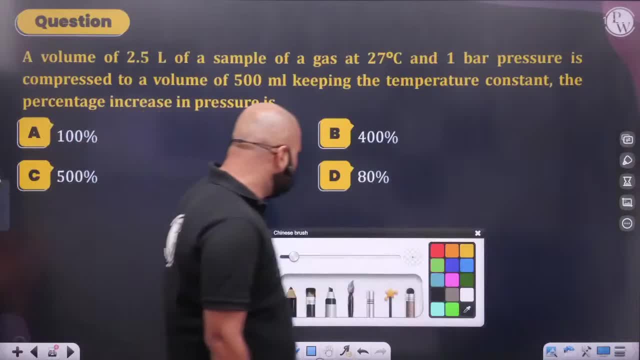 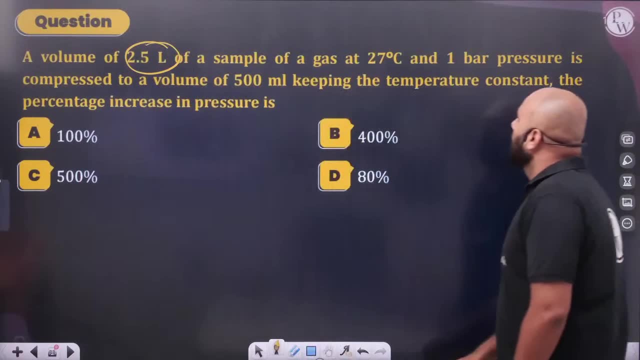 Molar mass. Look at this, Look at this question. Sir, 2.5 liter gas. Sir, 2.5 liter gas At 27 degree Celsius, At 1 bar pressure. Its volume is increased. Sorry, volume is decreased. 500 ml. Temperature is constant. Take percentage increase. 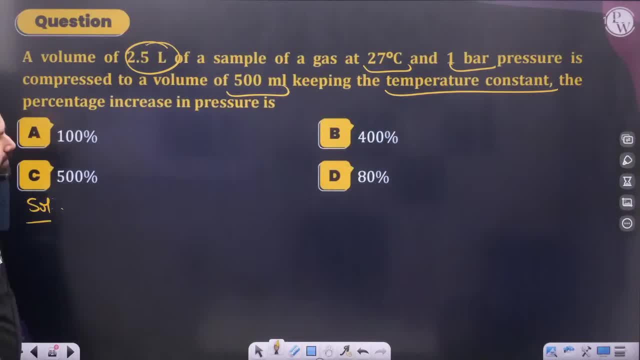 Take percentage increase. What will be the percentage increase? What will be the percentage increase? What will happen? V1- P1- V1 is equal to P2- V2. P1- V1 is equal to P2- V2. Pressure is 1- Detholder is 1. 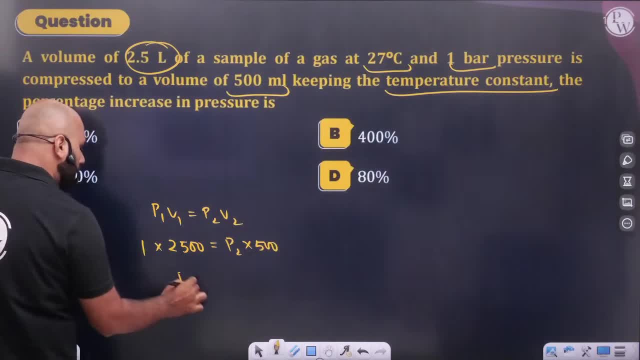 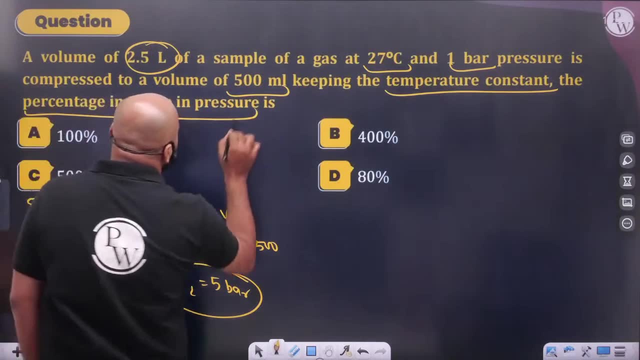 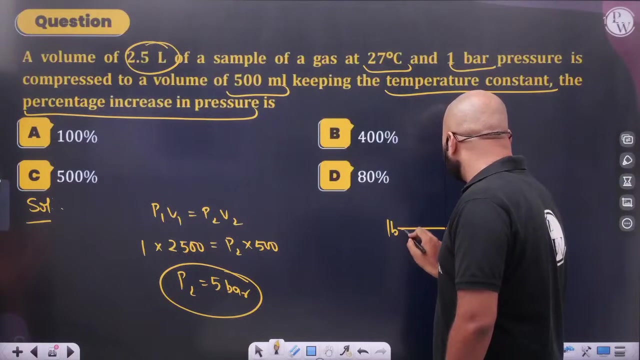 Convert these two, Else the wrong answer will come. The value of P2 will come. It will be 5 bar. Now here there will be one mistake. What is being asked? Percentage increase in pressure, Sir, where are you going from 1 bar? It is 5 bar. 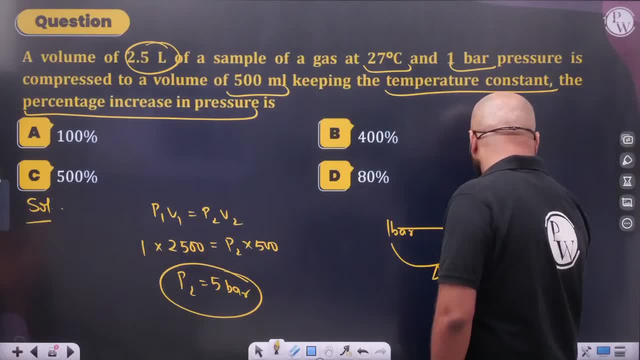 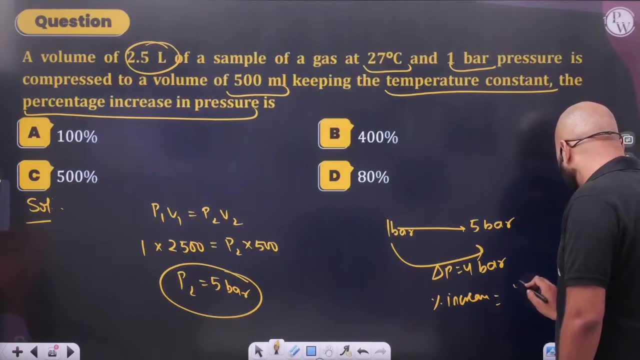 Sir, how much increase you are doing. What is delta V? delta P is 4. How does the percentage increase come? Don't write 500% by mistake. Don't write 500% by mistake. 4 upon 1 into 100.. 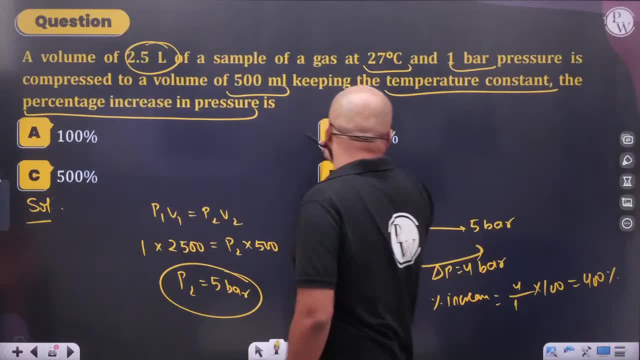 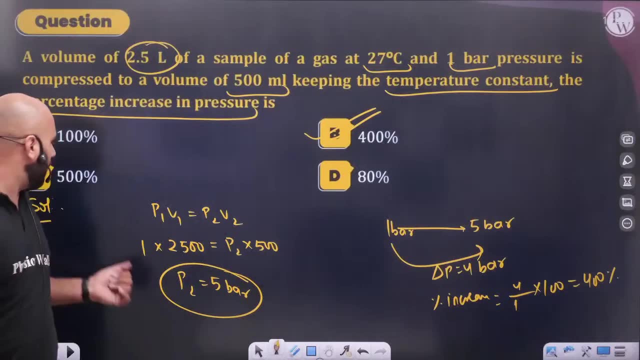 How much will it be 400%? To find the percentage, Sir, what will be the percentage 400%? C will not come. It's not that if 1 to 5 is happening, then answer C. Answer of 500% increase is not of 500%. 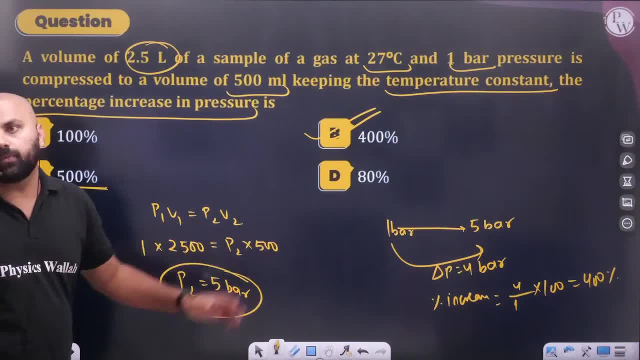 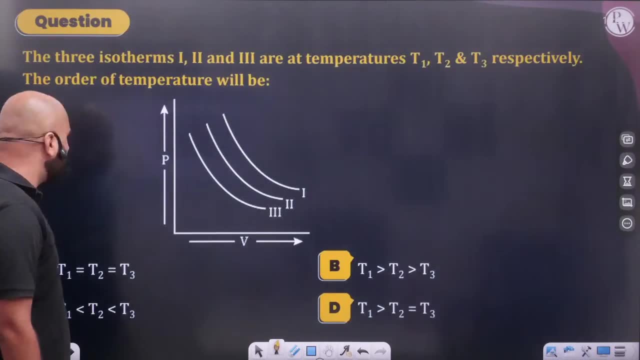 What is the increase? It is of 400%. What is the increase? It is of 400%. That's it. See these small questions. Now see, Before doing these graph questions, I will tell you a way to do graph Whenever graph questions are made. 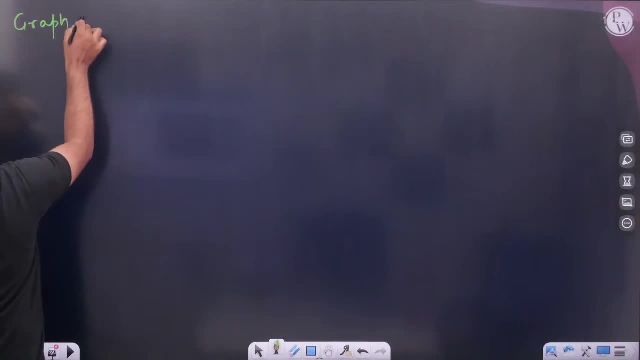 Whenever graph questions are made, Suppose graph questions are said. If graph questions are given, then remember a simple way: Never write that, sir. this is pressure and volume Then in its graph. If you write it, then it will work. But yes, if the other person wants. 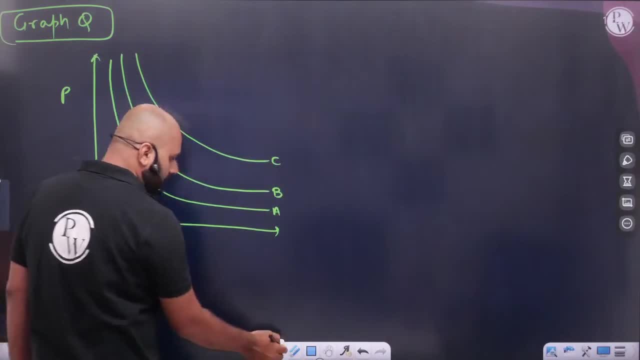 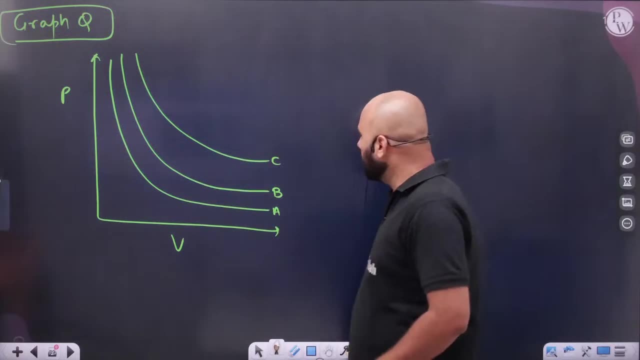 then he can do it. If temperature A, temperature B, temperature C, Different temperatures are given, Sir, tell me the relation between these three. Nothing, Try a simple method. Pull a constant line, Vertical or horizontal. pull a constant line. 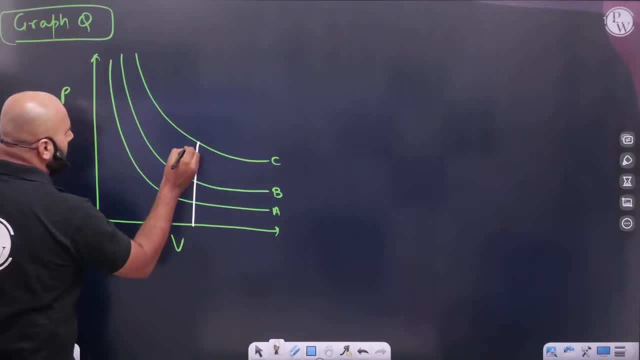 In this respect, see Sir different temperature A. Sir different temperature A, temperature B and temperature C. See carefully. As soon as I pulled this line, What did I feel? What did I do to the volume Constant? If the volume is constant, 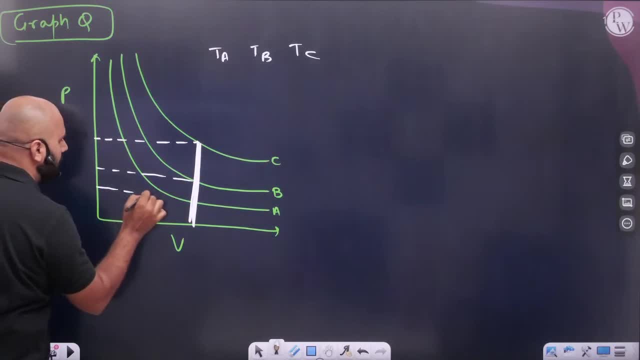 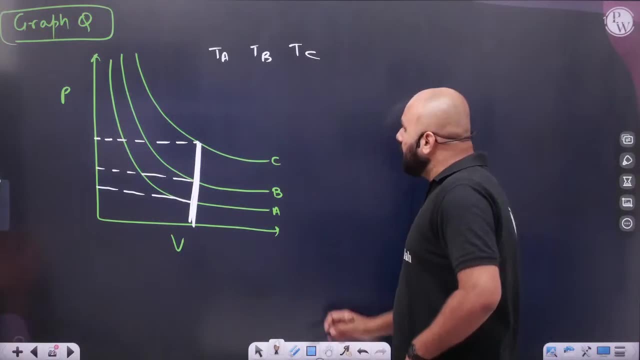 then, at this point, how much pressure is coming? At this point, how much pressure is coming? How much is the pressure? The pressure is coming for different people. This will happen. See, how much pressure is there at this point, Sir, if the volume is constant. 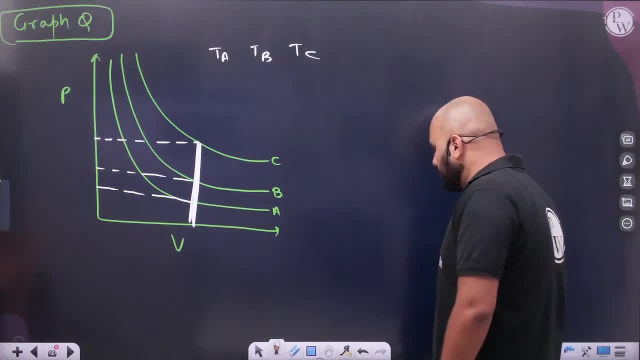 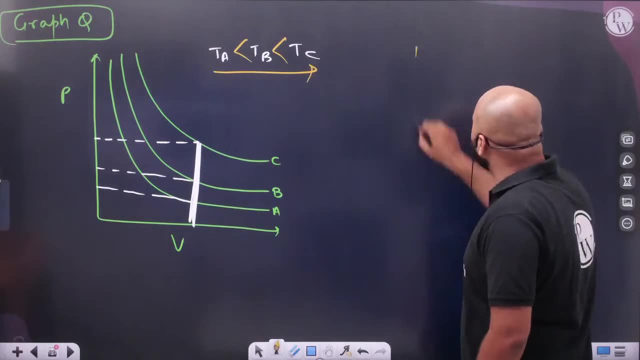 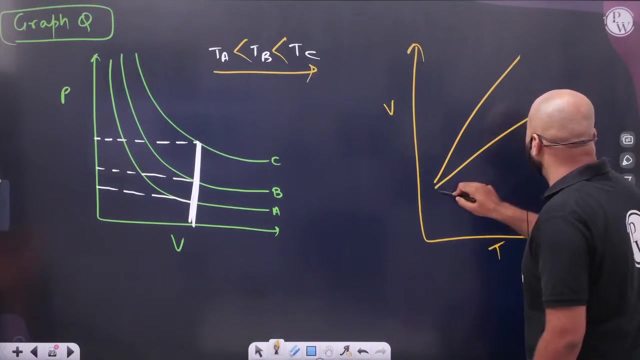 then what will be the directly proportional to When the pressure is directly proportional to Temperature? Sir, the one who has more pressure has more temperature. Ask any question. You have to pull a vertical line. Assume that you have drawn a graph of volume vs temperature. 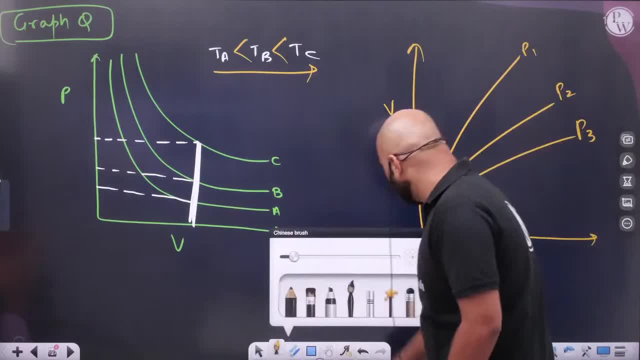 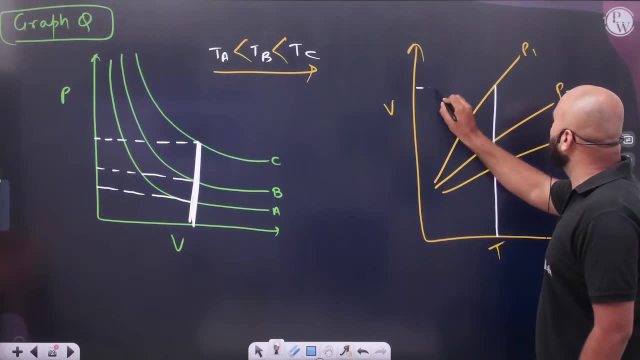 This is P1 pressure, this is P2,, this is P3. Don't mess with it. Use a simple logic Draw, a simple vertical line. Temperature has become constant. Look at it. There is no need to make it in exam hall. You can see it. The one whose volume is more. 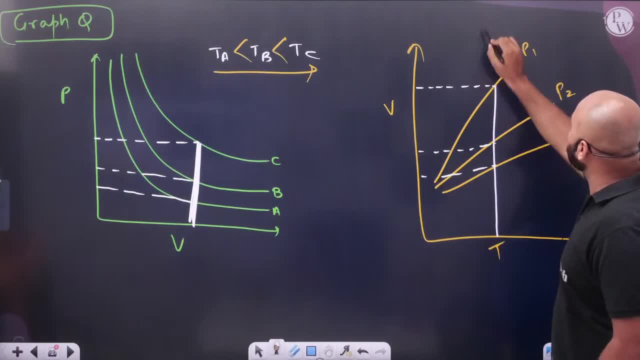 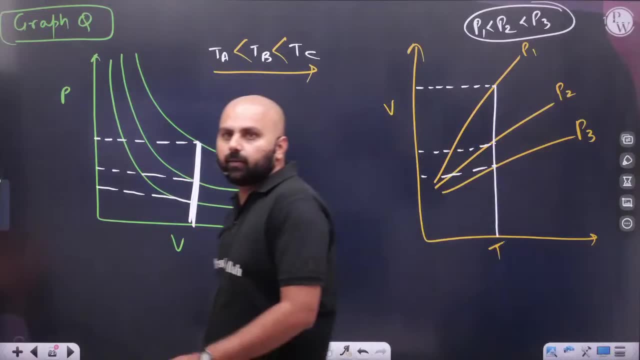 Temperature is constant. The one whose volume is more: What will happen to its pressure? It will decrease. The one whose volume is more: What will happen to its pressure? It will decrease. Use a simple logic. You don't have to draw a vertical line. Draw a vertical line from here to here. 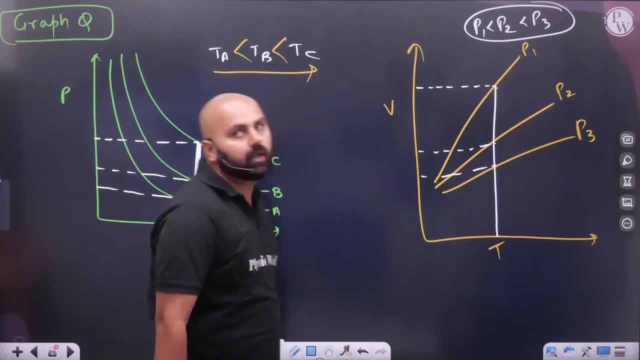 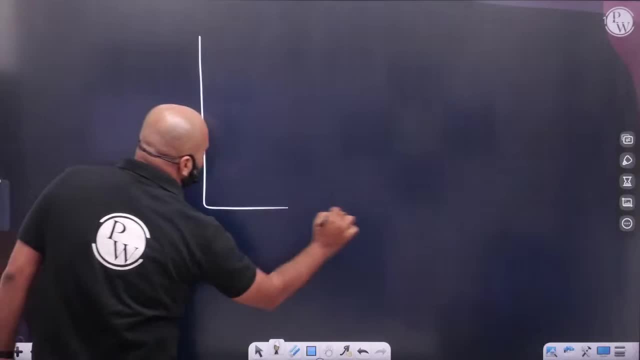 Look at it, Its volume is more. It means its pressure has decreased Because it is constant temperature. This works Wherever the question is given, Wherever the graph questions are given, Wherever it is given, Assume it is given like this Pressure vs temperature graph is given. 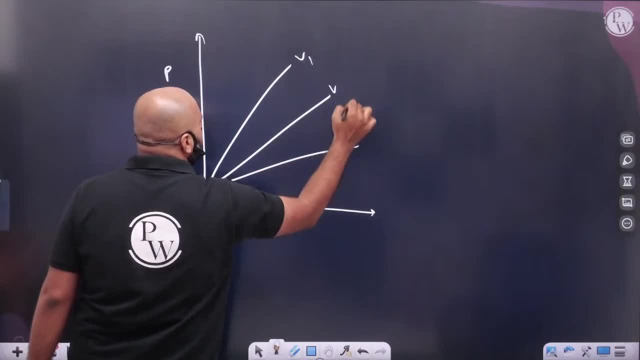 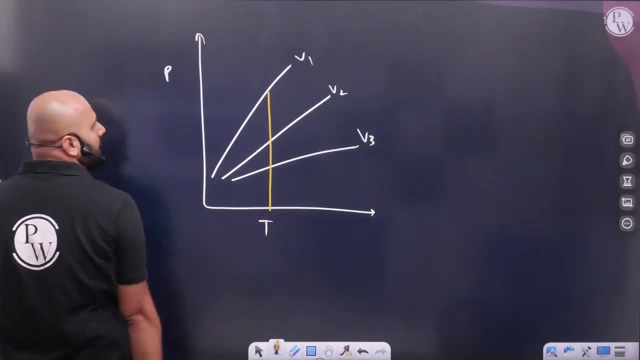 Sir, it is given differently: This is V1,, this is V2,, this is V3. Who said, sir, tell me this. Nothing You have to understand. It is very simple. You always have to draw a vertical line. Draw a vertical line, Look at it according to this. 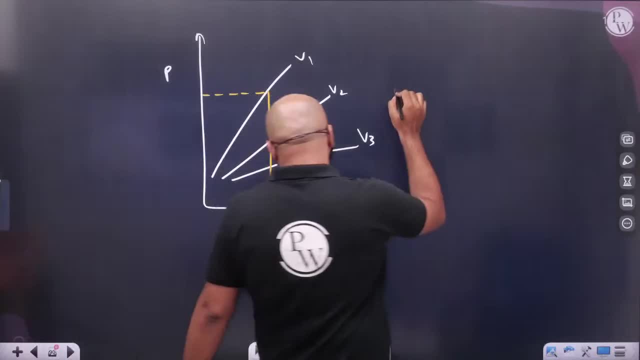 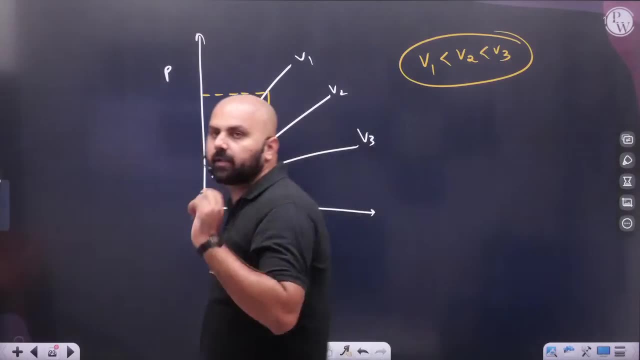 Its pressure is more. What will happen to the volume? It will decrease. Why? Because the temperature is constant. So what will happen to V1? The lowest? Then what will happen V2, Then what will happen V3? So everyone has. This is the best way to solve the graph. 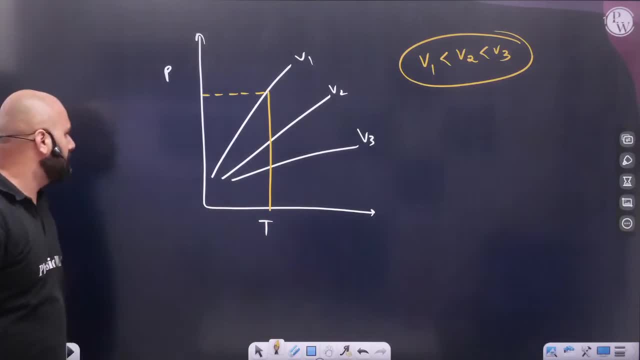 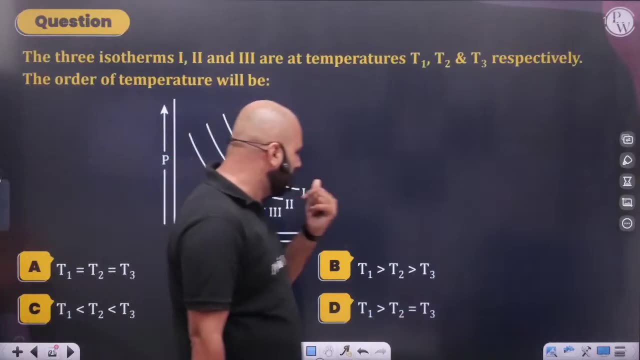 This is the best way. Okay, That's it. Keep doing. We have small questions Like now this question. Now this question is very simple for you. Some people sit remembering, So they know. Otherwise, you pull the vertical line. You pull the vertical line like this: Sir, this volume has become constant. 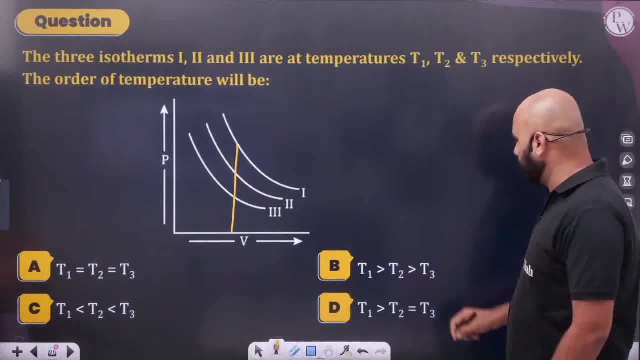 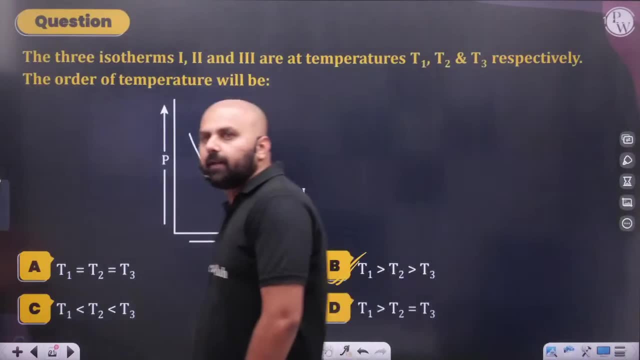 Whose pressure is high? What will be the temperature there? High? So who will be the most T1, Then T2, Then who will be the most T3? What will be the answer? What will be the answer? B will come. What will be the answer? 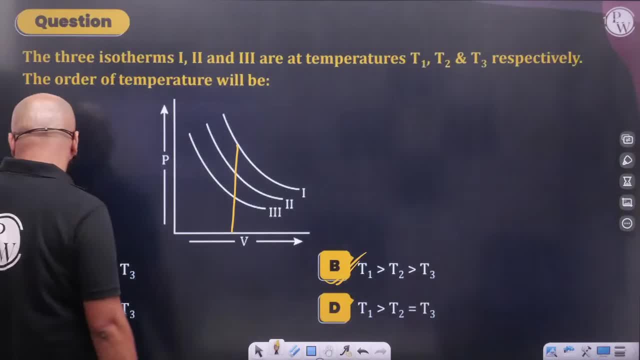 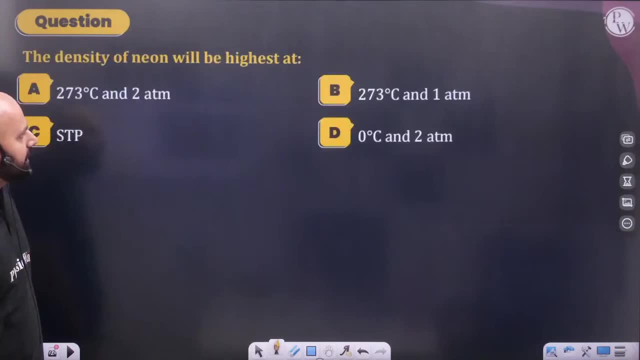 B will come, Keep doing. Okay, What will be the answer? B will come, Keep doing. Then who said, sir? Now see what is the good question. We have the ideal gas equation. See its application. Density of neon gas. Density of neon gas will be highest. What is the density of any gas? 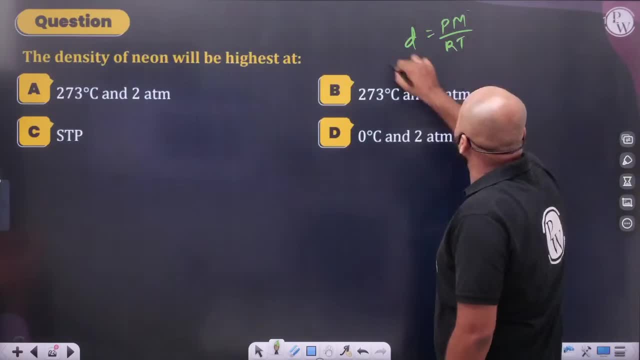 PM upon RT. Like neon gas Means, molar mass is fixed. Density will depend on, Directly proportional to pressure. Inversely proportional to temperature Where the pressure will be high, See the pressure. STP also decreases. Pressure is high here, And what should be the temperature? 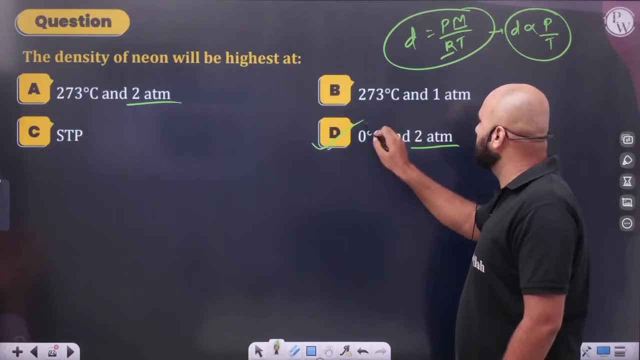 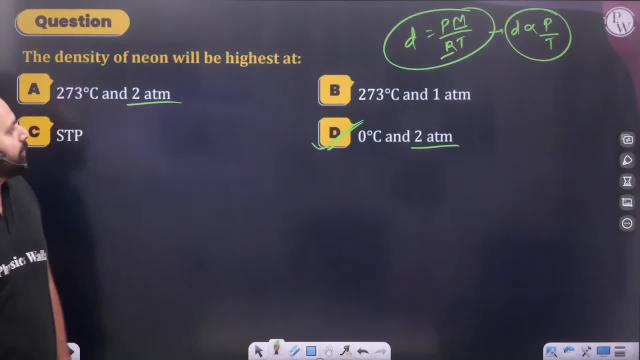 It should be low, Temperature should be low. So what temperature will you take? 0 degree Celsius Or 2 degree? Density will be high only When your temperature is low. And what is the pressure High? Then what will be the answer? D: What will be the answer? 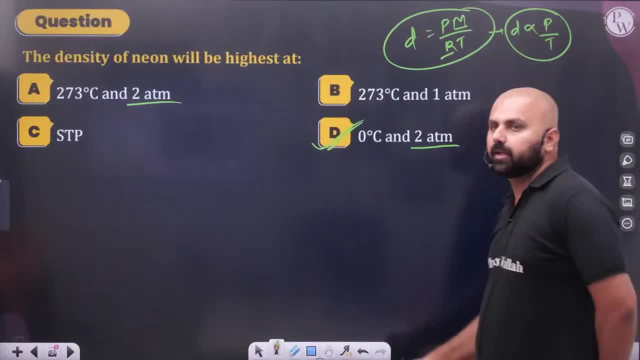 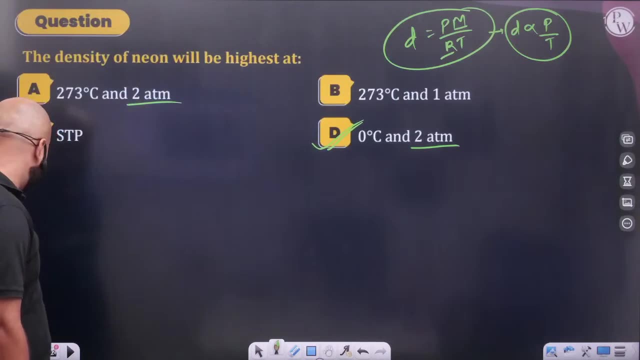 D Density. When we started a little while ago, That's when we studied, So we did like this. Then see Who told me Sir Dalton's law of: Oh, Now see what is in between here. Now let's revise the theory a little Above Dalton's law, Dalton's law of partial pressure. 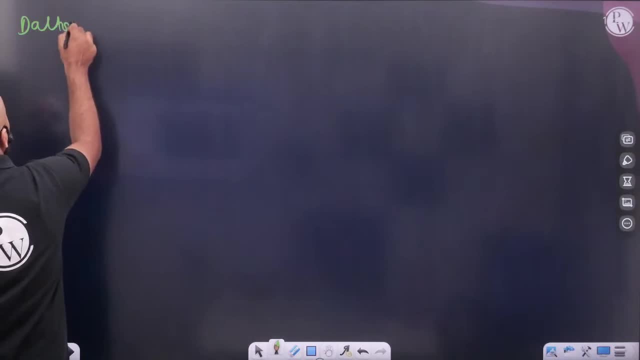 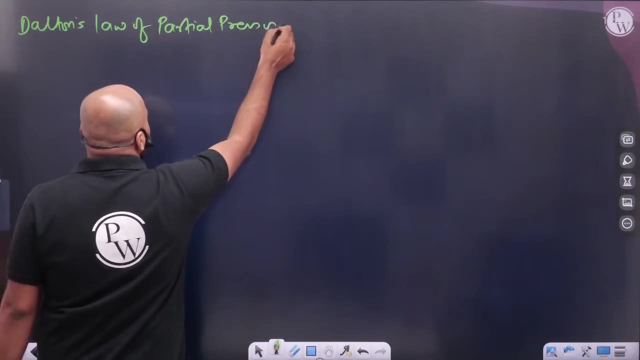 Dalton's law of partial pressure. Brother, This is being asked a lot At this time But yes, Now it has been 2-3 years, So now a little. I think This year Will not make so many mistakes That the same topic. Keep asking questions. But yes, Should know. 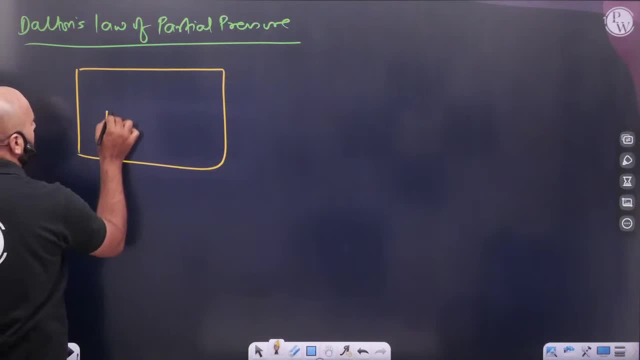 What is Dalton's law of partial pressure? Dalton's law of partial pressure Is the story of the middle of two gases, And what are? both of them Are unreactive. What should be? both of them Should be unreactive. Should be unreactive. 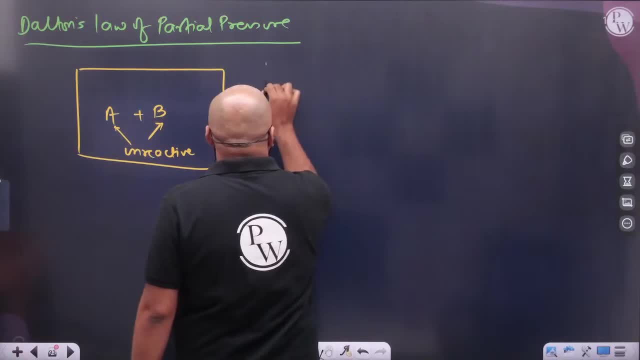 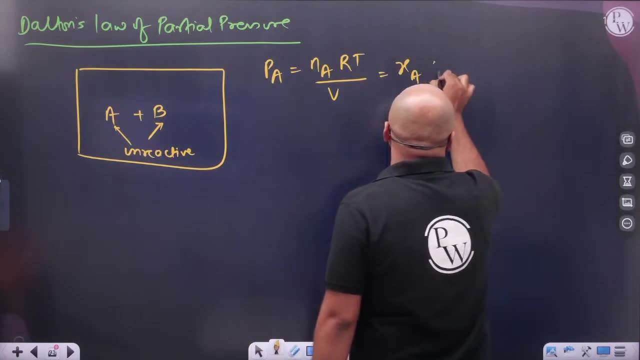 Should be non-reactive If we talk about them. So what is the pressure of A Number of moles, RT by V? Either write it like this, Or Mole fraction of A. Into What can you write? P, total. Similarly, Pressure of B To remove. So number of moles of B. 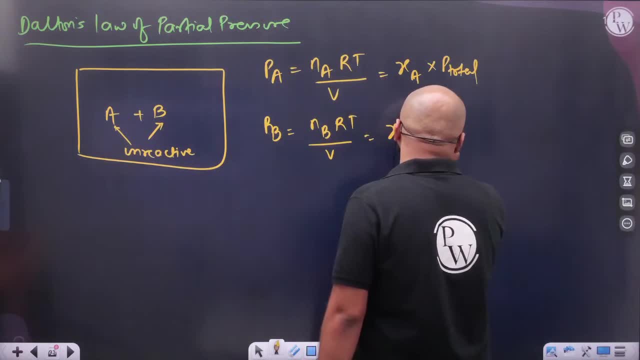 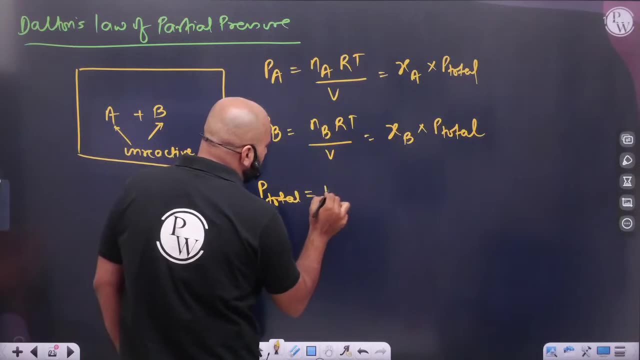 RT by V. And what will happen? Mole fraction of B Into What will happen P total? And here If we talk about P total. So P total is nothing PA plus P total is nothing PA plus PB. What will happen? NA plus NB Into RT by? 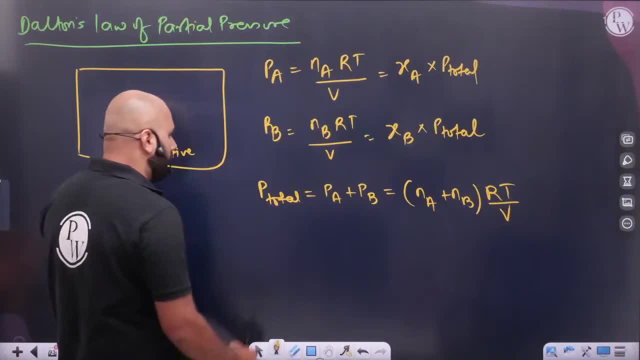 NA plus NB, RT by V, And by doing this You can remove everything. Sir, According to Dalton's law, Partial pressure Pressure is inversely proportional to Mole fraction Directly proportional to Mole fraction Directly proportional to What will happen. Mole fraction Directly formula. 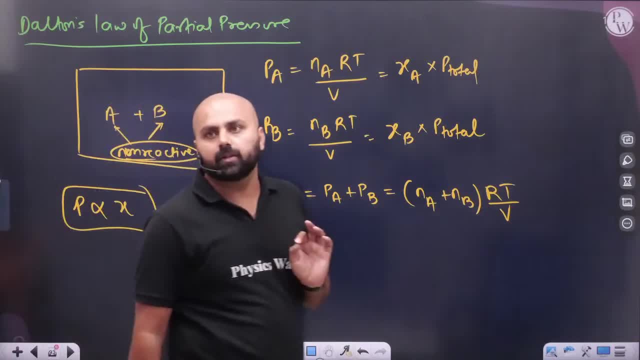 Add everything For non-reactive gases. For non-reactive gases, Use Dalton's law, Partial pressure, Directly formula. Any problem. Dalton's law, Partial pressure, Very simple concept. Just keep in mind: There should not be reactive gas. There should not be reactive gas After this. If you see the story, 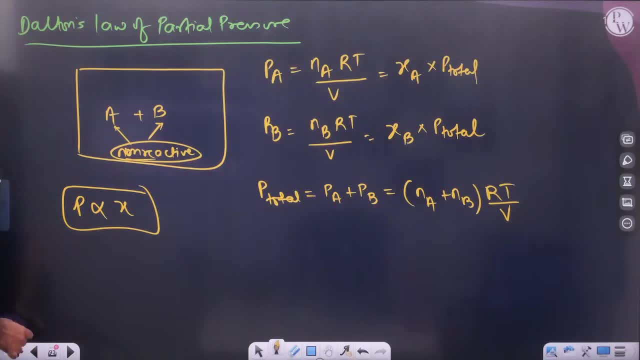 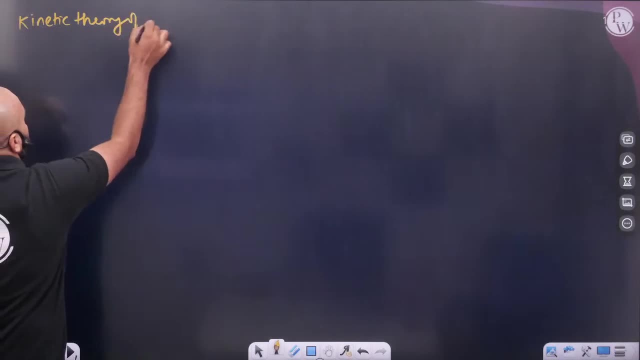 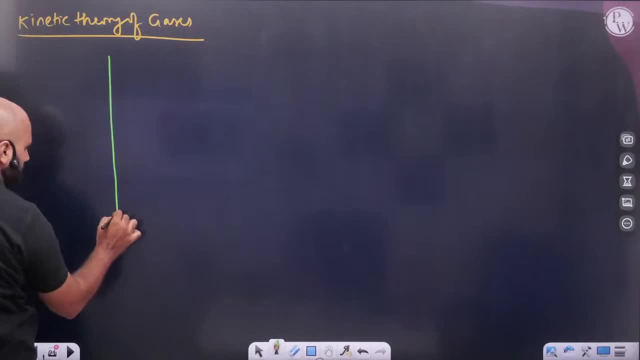 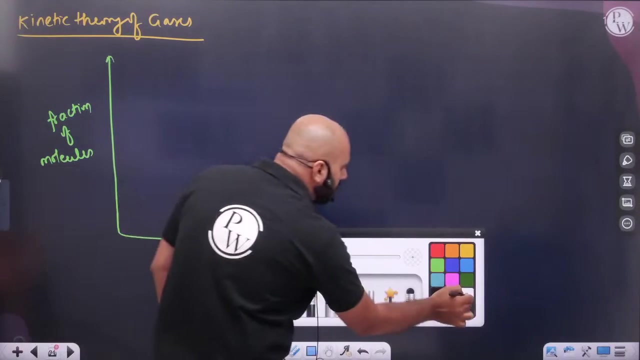 Kinetic theory of gases, What we talk, That the Gas molecules, If we Start to see their variation, If I Start to see variation, Speed, Fraction of molecules, If Start to see variation, So They Speed With variation, So will be of different types and its graph becomes like this. its graph becomes like this: this point: 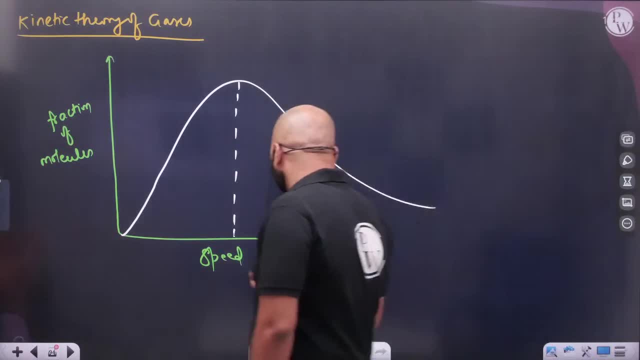 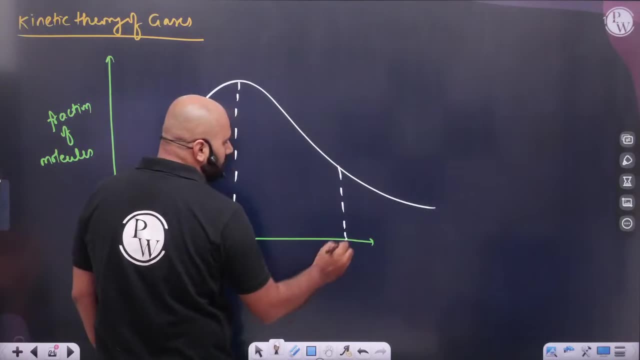 happens? this point happens where there are maximum people. what do we call this speed? we call it most probable speed, the highest speed that comes in it. what do we call it? we call it vrms and the average speed of the in-between. what happens? it becomes v average, then it comes out of 3 speeds. 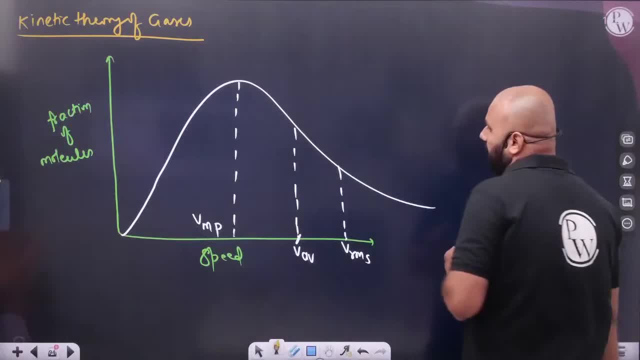 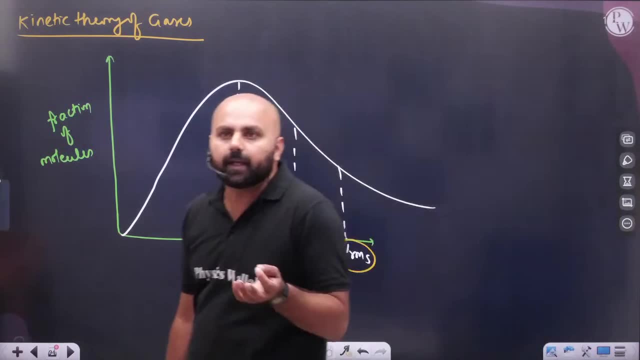 if we talk about speed of gas, if we talk about speed of gas molecules, then I have 3. speed comes out, most probable average, and vrms is a kinetic theory of gases. brother, what was the kinetic theory of gases? what was the thing in the kinetic theory of gases? if you want to take the intermolecular force of 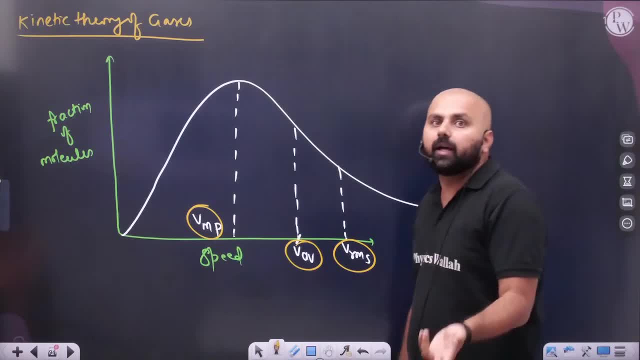 this zero size of gas molecules. what you have to do is to neglect what gases do do: elastic collision. now just study physics. so there is no theory here. if you have a formula of vmp, then what is coming if vmp? 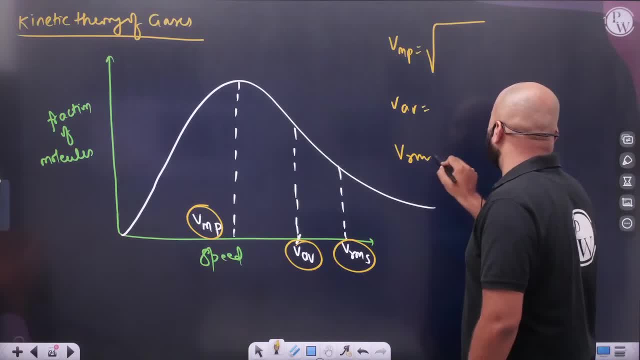 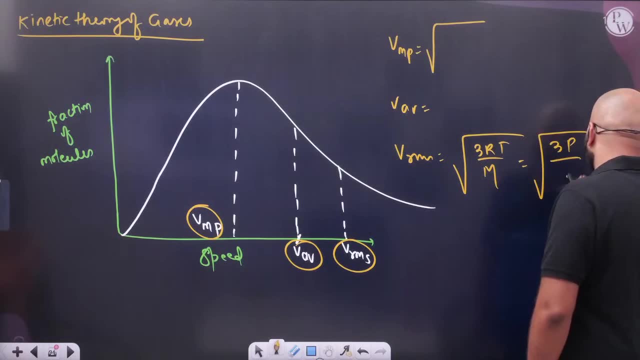 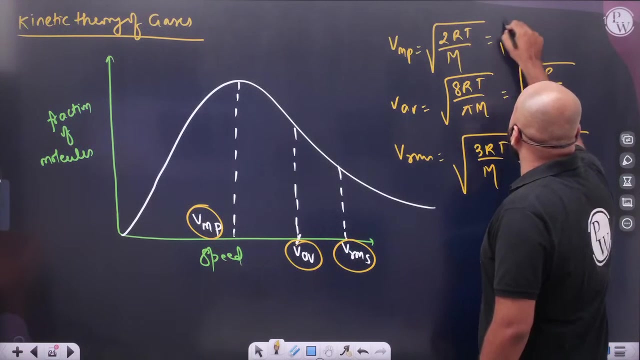 If we talk about V-Average, V-RMS, then V-RMS is the highest speed: 3 RT by M, 3 RT by M or 3 P by D. we can call it density. We write this as 8 RT by Pi M, 8 RT by Pi M or 8 P by D. we write Pi D and we talk about this as 2 RT by M or, under root, 2 P by D. 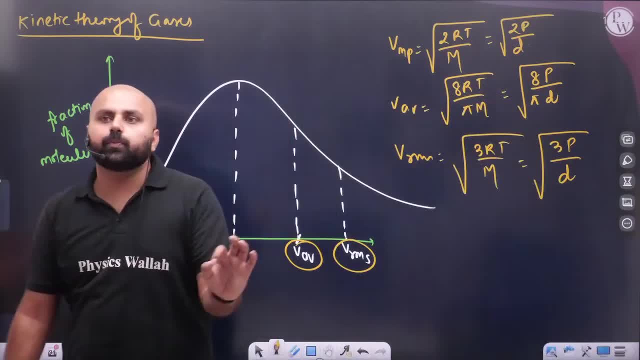 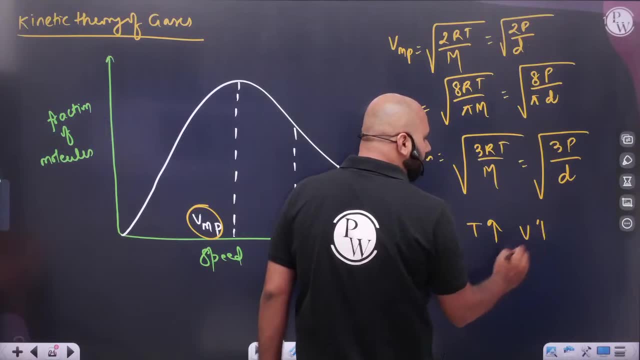 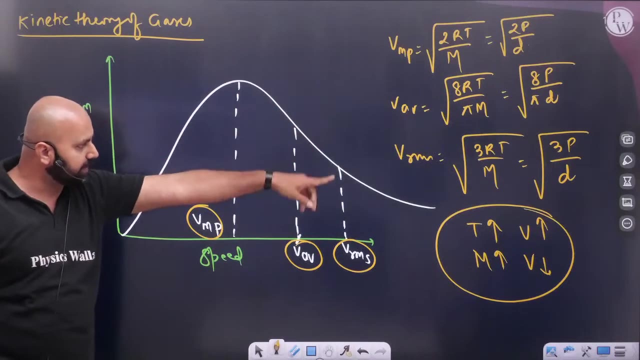 What do we have to do with all this? pick it up. pick it up any speed, any type of speed. remember, if you increase the temperature, if you increase the temperature, any speed, the velocity will increase. if you increase the molar mass, the velocity will be less. keep this in mind. any speed, be it most parallel, be it average, be it RMS. now look at the graph. if you increase the temperature, the graph will shift to the right. if you increase the temperature, the graph will shift to the right. and if you decrease the temperature, the graph will shift to the left. if you increase the molar mass, the graph will shift to the left. 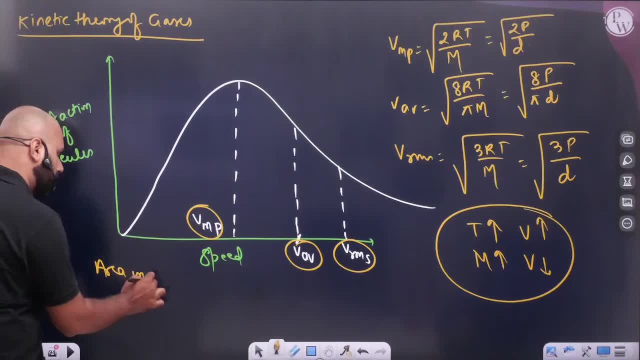 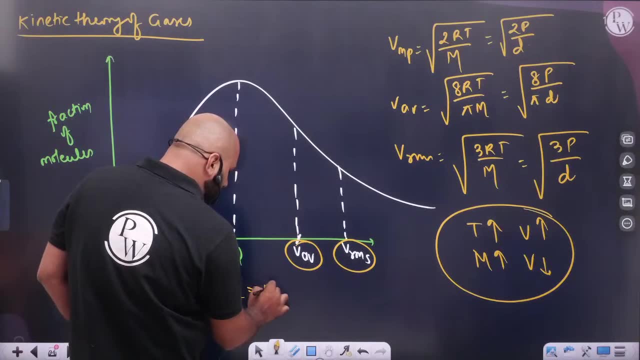 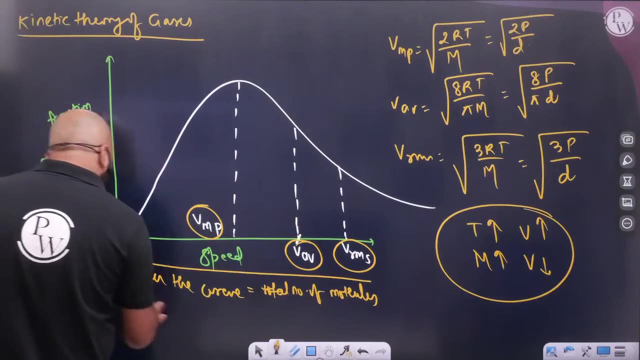 The area under the curve is equal to the total number of molecules. Your graph will go up and down, no problem. Your temperature will go up and down. let the graph go up and down, But what is the total number of molecules? It has to be the same. 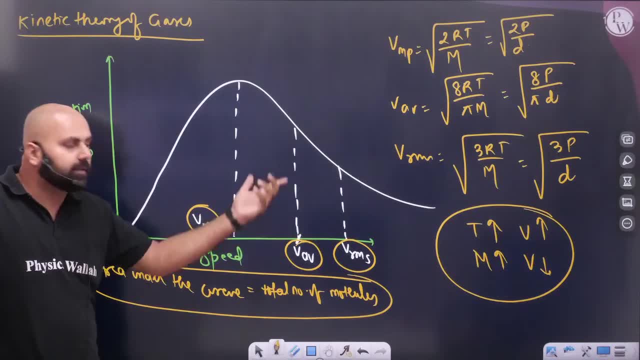 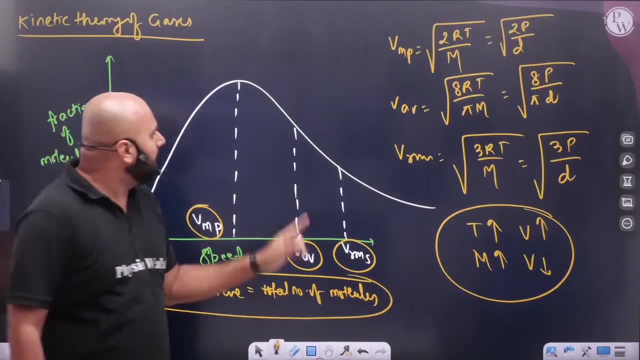 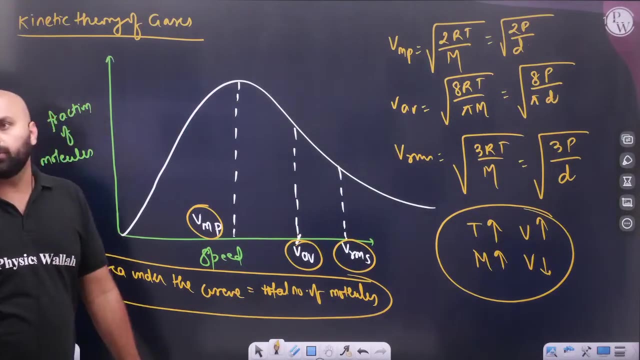 Total number of molecules has to be the same. So keep this simple thing in mind. We have V, most probable V, average V, RMS. Take out the answer like this: Kinetic theory of gases is done: Area under the curve is equal to the total number of molecules. 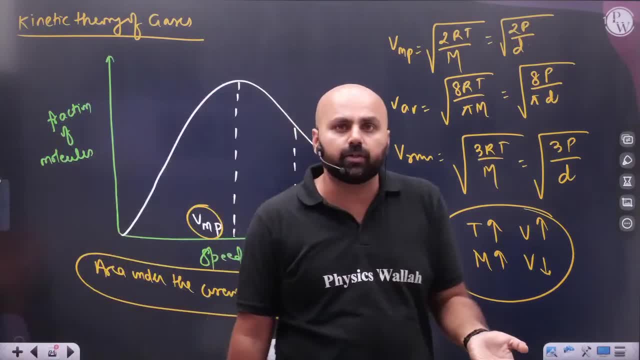 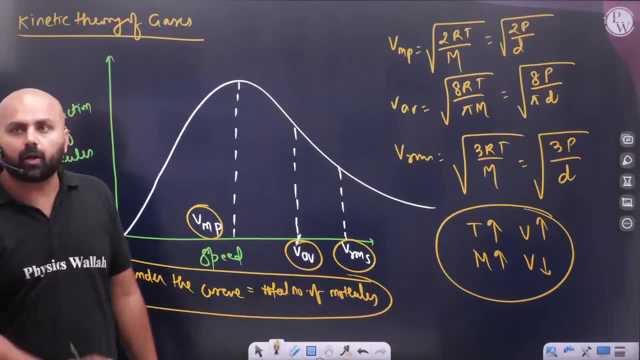 What is the other collision frequency? Collision is elastic collision. You have already studied physics, You have done derivation, So I am not giving more on this. Do a basic work on this. What is the area under the curve? We will increase the time temperature. 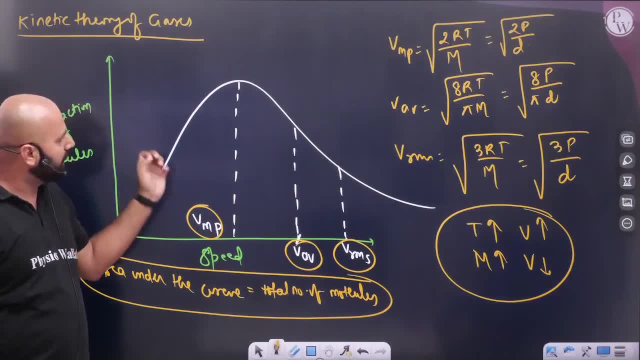 It will go towards earth. We will decrease the temperature. It will come here. We will increase the molar mass. It will come back. We will decrease the molar mass. It will go forward. So this is how V RMS works. 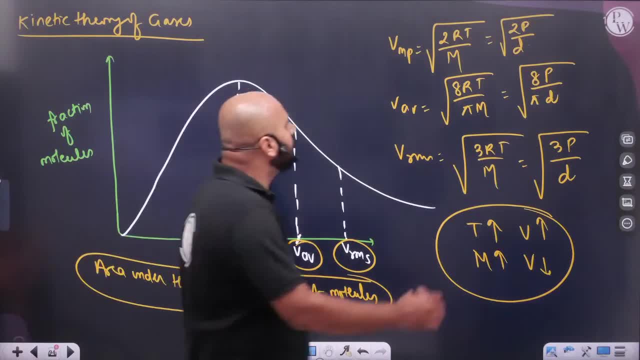 This is what we are talking about in kinetic theory of gases. Apart from this, whenever we have to find the values in this, we put the mass in kgs. Remember, whenever we put the mass, we will put it in kgs. 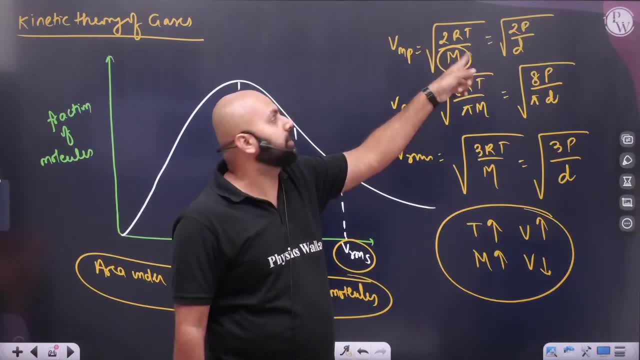 Why in kgs? Because what is the velocity required? It is required in meter per second. So what is the mass to be put in kgs? What is the temperature In Kelvin? What is the value of R 8.314? 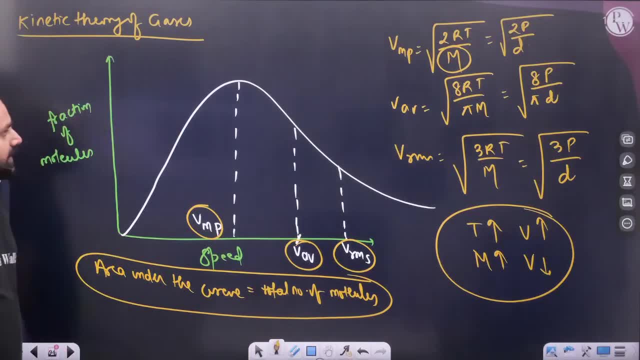 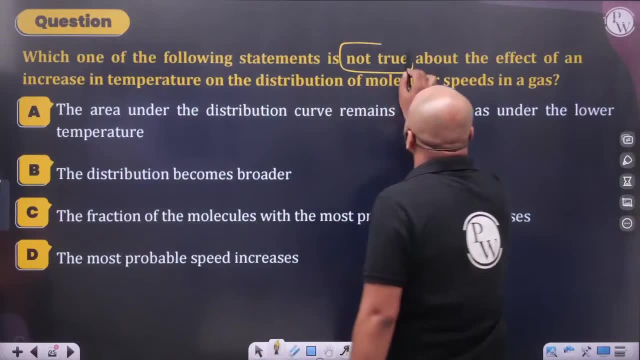 Sure, Sir, it is the value of R. So this is done. Now see the question given by this is this: What will happen? No true must be told. It is not true. Which statement is not true? If, what do you do? 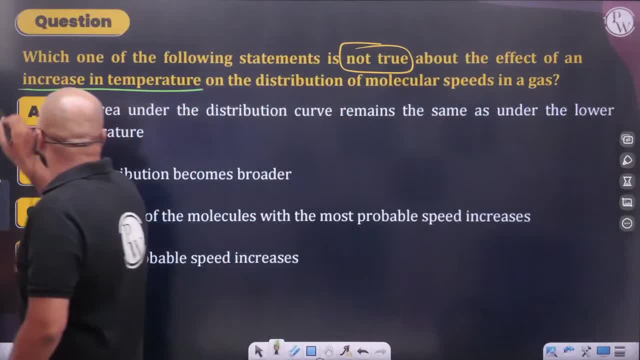 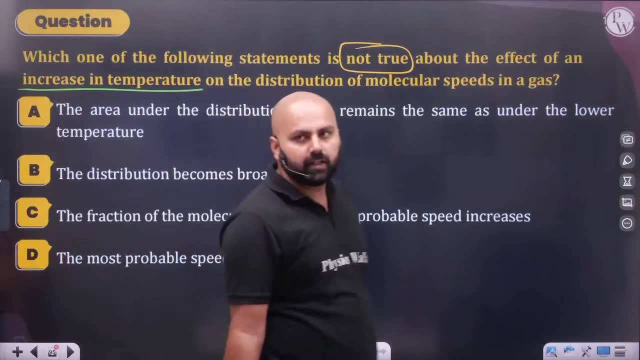 If you raise the temperature, You will raise the temperature. You will raise the temperature. What happens, Sir, if you raise the temperature? then what will happen, Sir? area under the curve will remain the same. Obviously, the area under the curve will remain same. 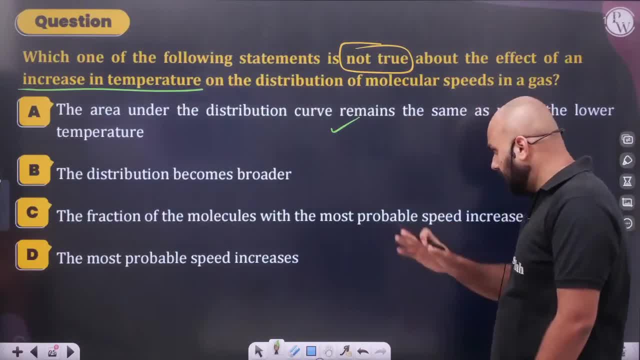 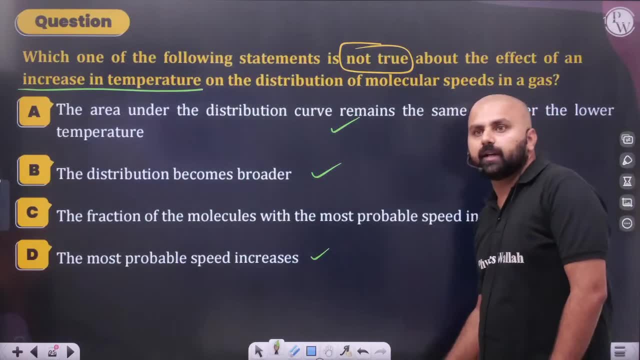 Okay, The area under the curve will remain the same Because the number of molecules is same. becomes broader, obviously it will become wider, The most probable speed. obviously, if you increase the temperature, all types of speed will increase. All types of speed will increase. But 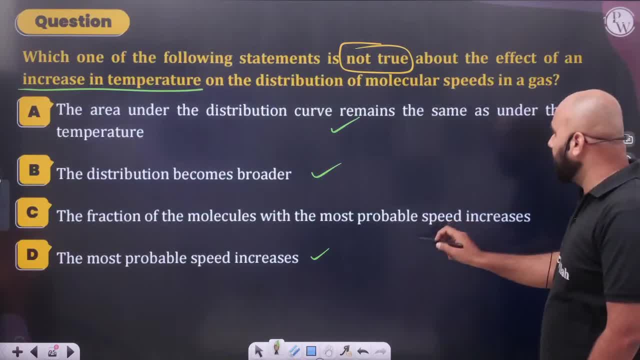 all types of speed will increase. See this with you. Fraction of the molecules with most probable speed increases, Fraction of the molecules will not increase. The graph will go here. If we talk about the graph, it was like this, So how will it be going? It will be going like this. So what will happen to the fraction of the molecules? 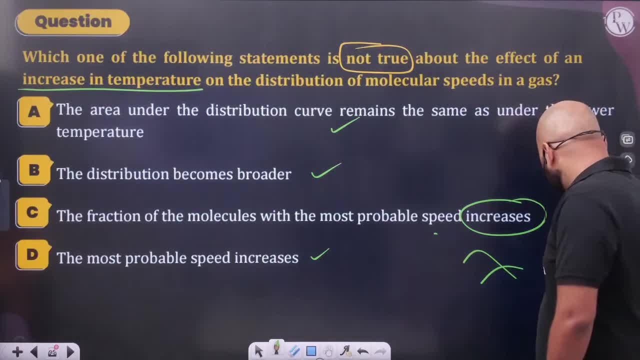 With most probable speed, it will start decreasing gradually. So what will be the answer? What will be the answer of this? What will be the answer of this? C will come. We will get the wrong answer. This is not the true answer. 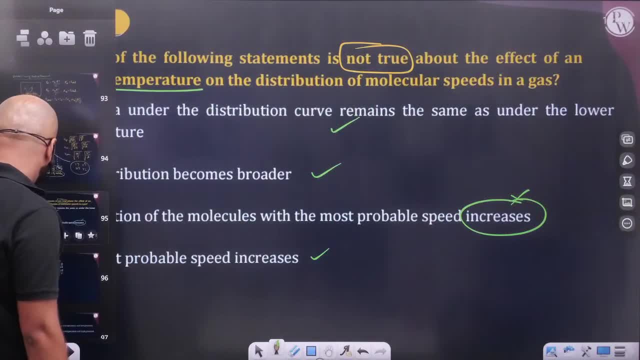 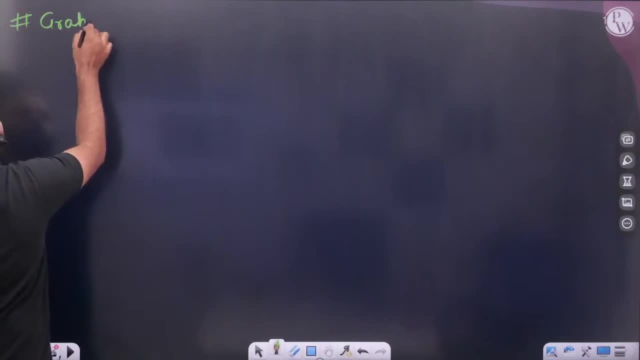 This is not the true answer, So this will come to us Then. who said that, sir, after kinetic theory of gases, we have a simple. I will not take much time. this is not with us for long. it is out of syllabus. 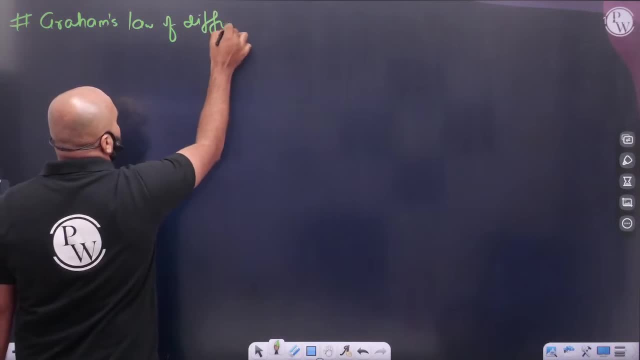 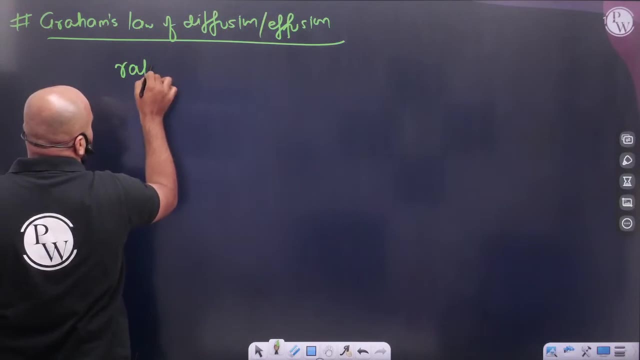 Graham's law of diffusion or effusion. In diffusion or effusion keep a simple logic: That whenever there is diffusion or effusion, in that case the rate of diffusion, rate of diffusion or effusion. rate of diffusion or effusion. 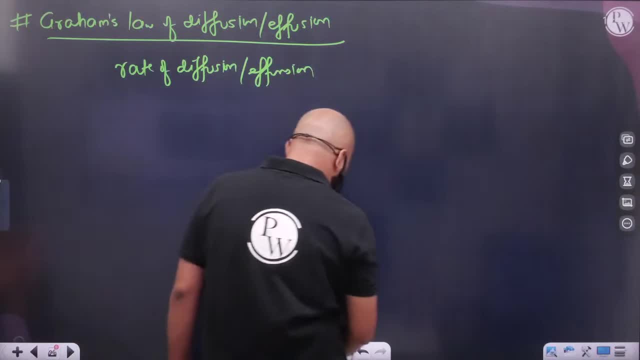 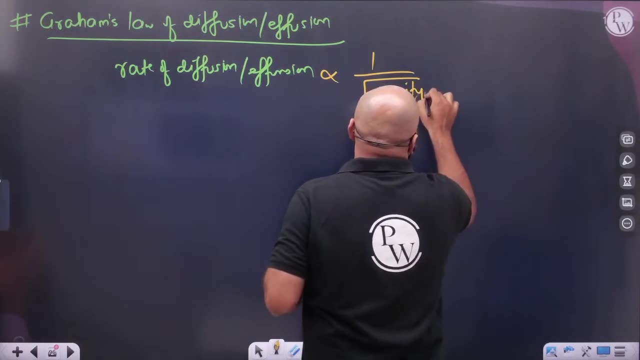 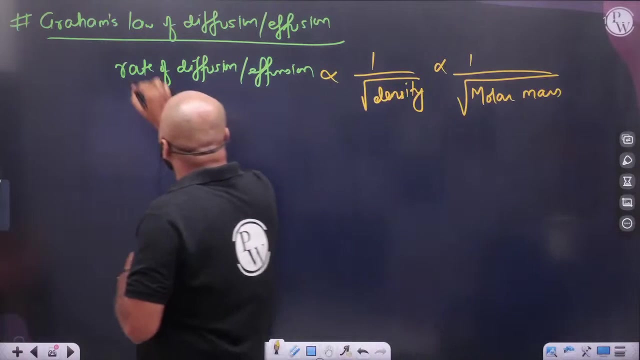 what does Graham's law say? That the rate of diffusion or effusion will be inversely proportional to under root density. and because everything is common, so what will be inversely proportional to Molar mass will be at constant temperature and pressure. 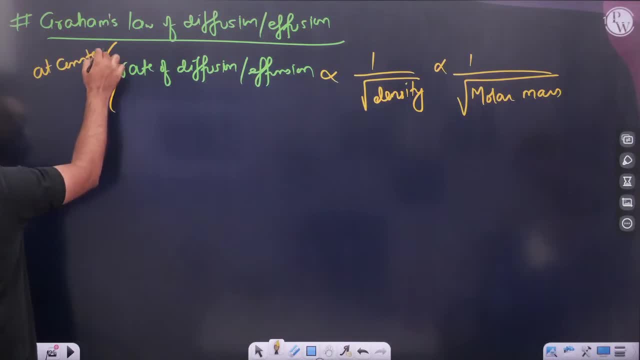 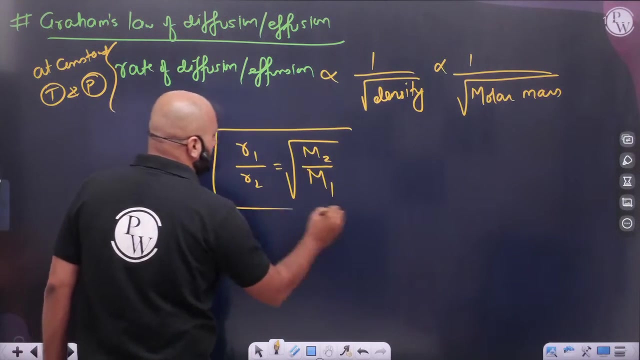 At constant temperature and pressure. At constant temperature and pressure, The rate will be inversely proportional to molar mass. Means R1 by R2 is nothing. Molar mass will be M2 by M1.. This will be our formula. 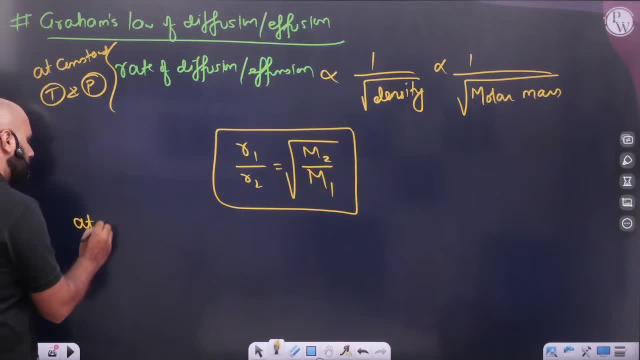 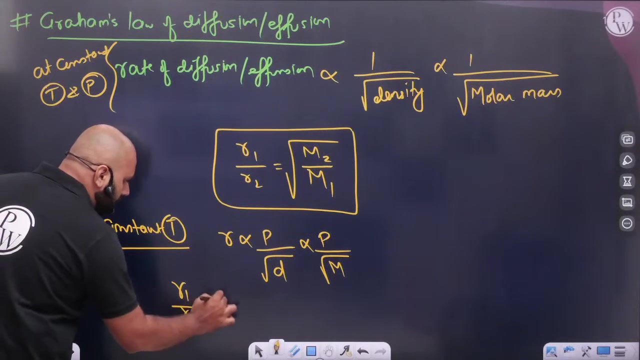 Who said that, sir? if there is no constant temperature, if there is no constant pressure, if the temperature is constant, then the rate will be P by under root, D Or P by under root. what will happen? R1 by R2 is nothing. 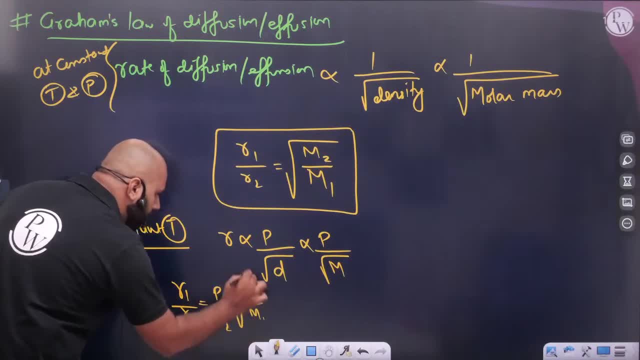 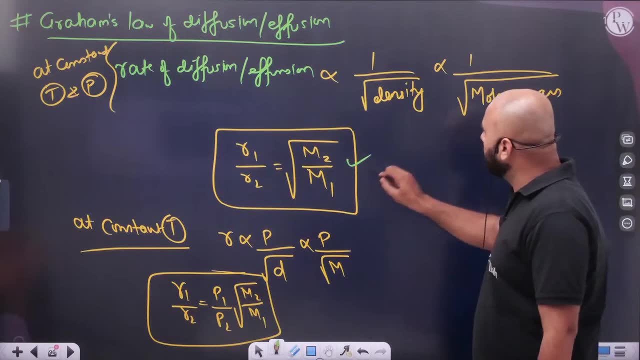 P1 by P2, under root M2 by M1.. Sir, this will be the formula of rate Whenever we define the rate of diffusion or effusion. see Graham's law says that, sir. the inversely proportional to molar mass. 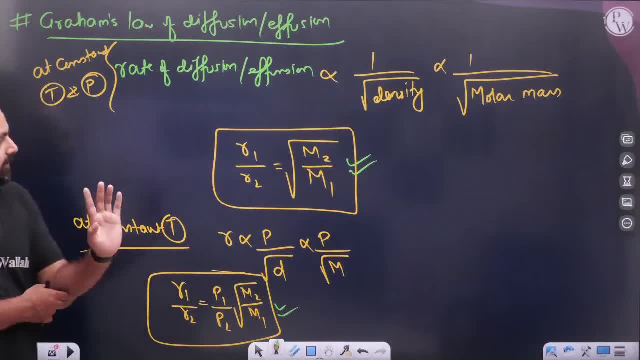 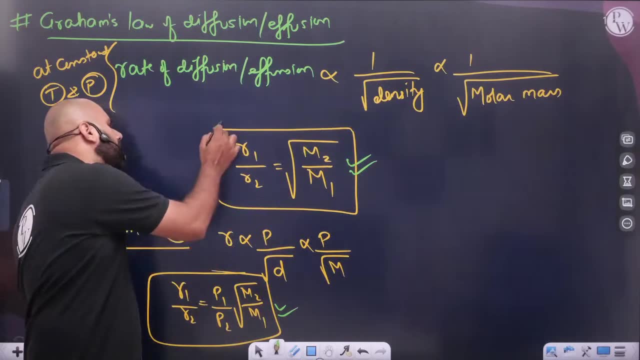 All your questions will be on molar mass only. But but, brother, what is the problem? How do we define the rate here? The problem is not that you are using this formula. You will get this ratio anywhere very easily- But how do we define the rate? 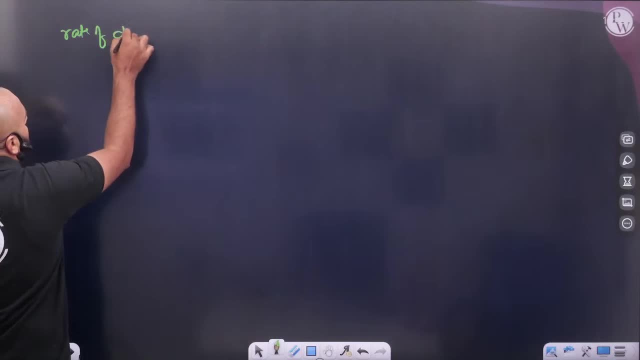 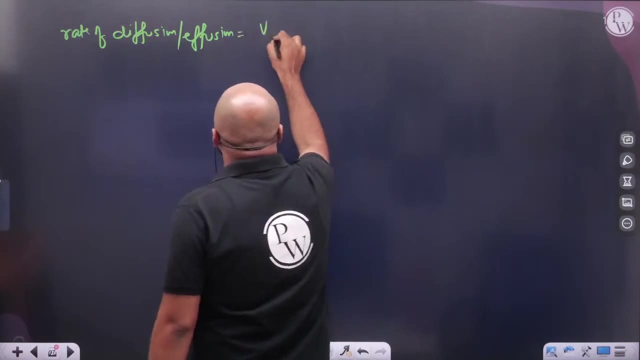 So the rate of diffusion, the rate of diffusion, do you know? whose is equal to whose? Whose definition is equal to whose? So this is, sir, how much volume was diffused: V2 minus V1.. Or volume diffused divided by time. 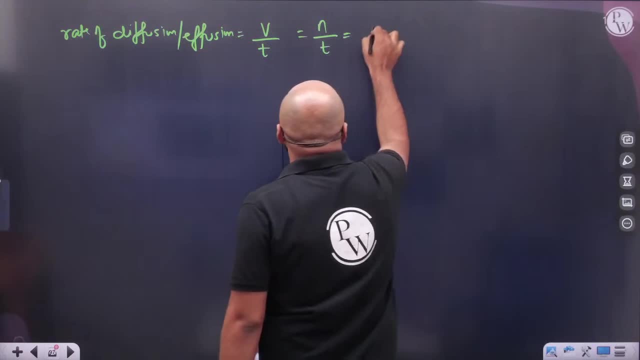 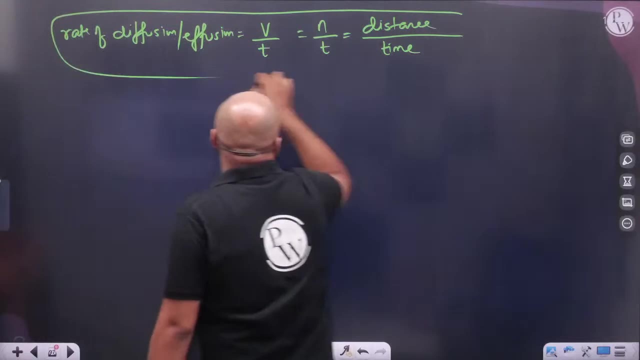 Or number of moles diffused divided by time, Or distance travelled by gas. distance travelled divided by time. Because what is he trying to tell? Rate of diffusion or effusion? Who is moving at what speed? See carefully. 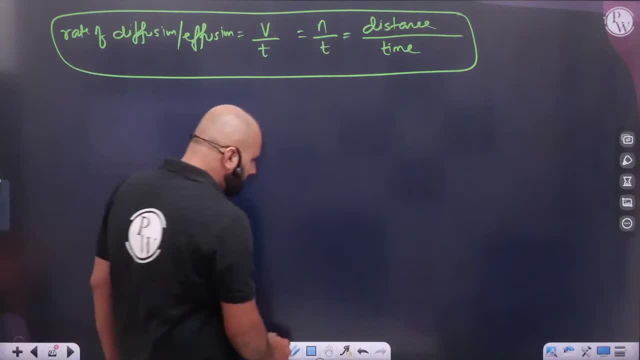 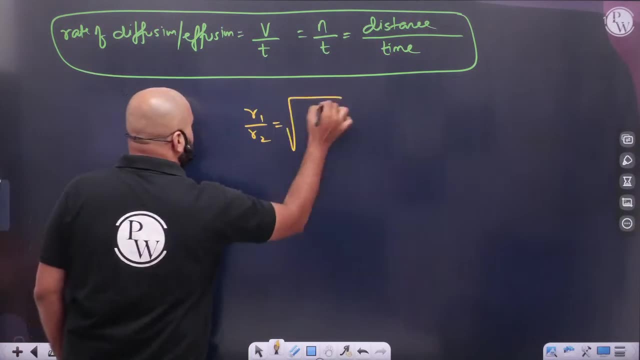 Who is moving, at what speed. It is being told for this. So, brother, if someone asks, you, tell me R1 by R2.. So R1 by R2,, according to Graham's law, will be equal to M2 by M1. 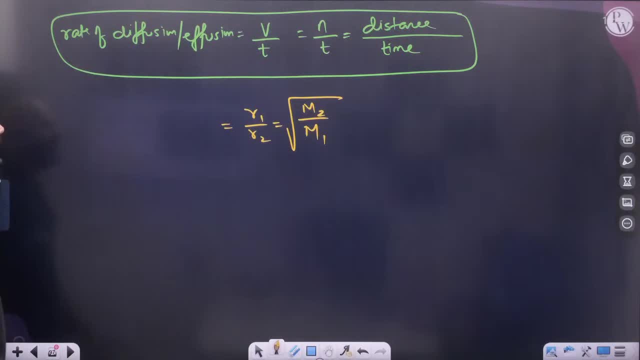 But, sir, how to measure R1? So what can you write for R1? N1 by T1.. What will this be? N2 by T2.. Or we can say here, not saying number of moles. 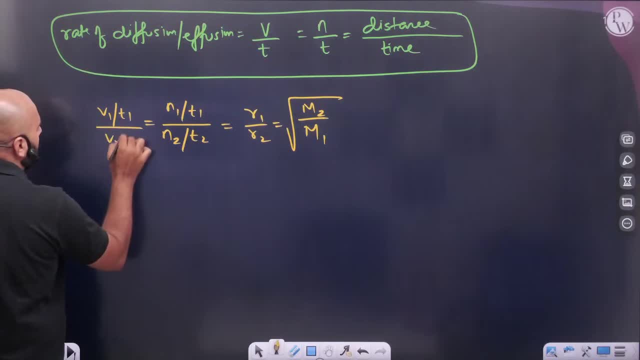 V1 by T1. Is equal to V2 by T2.. Or if I talk about distance, D1 by T1 is equal to D2 by T2.. You will put this formula directly, This formula at constant temperature and pressure. 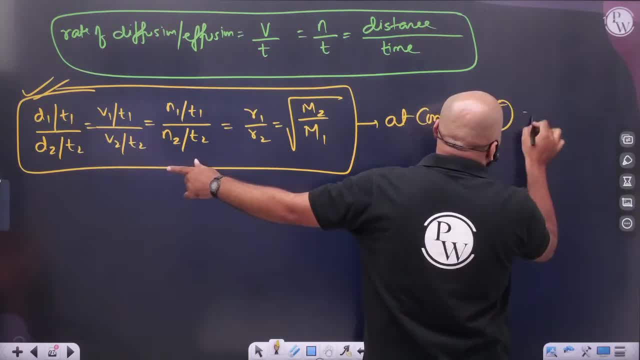 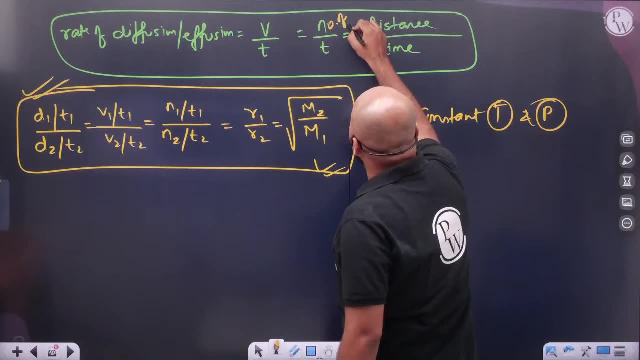 The numerical that will come in your exam, maximum to maximum. Today the chances of it coming are less, But maximum to maximum this will come. N is number of moles. How many number of moles are these? What is this Volume? 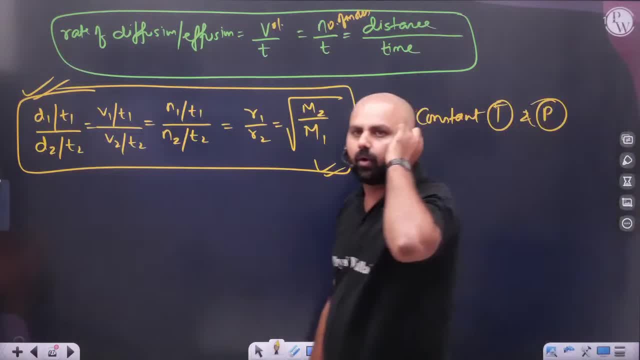 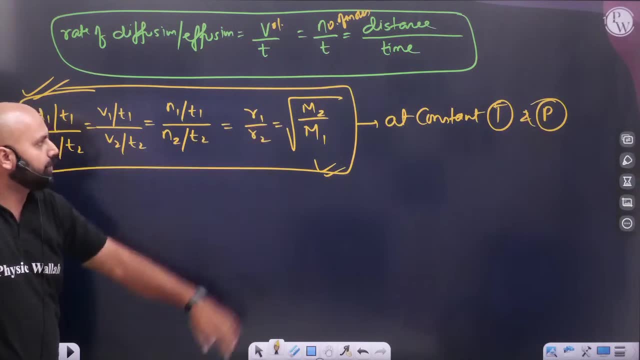 Volume divided by time, Directly: N2 by N1.. That's it, Nothing else. Okay, You have to put this directly: At constant temperature and pressure, R1 by R2, inversely proportional to molar mass, In respect of N1 by T1. 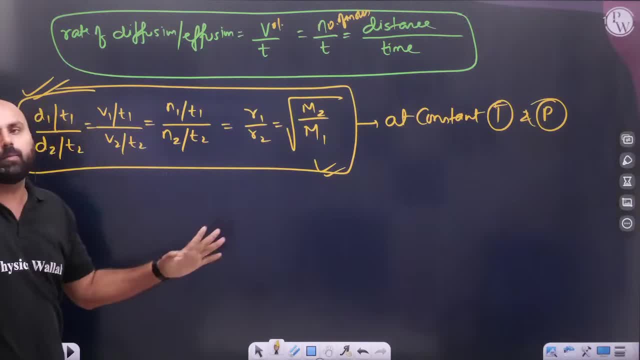 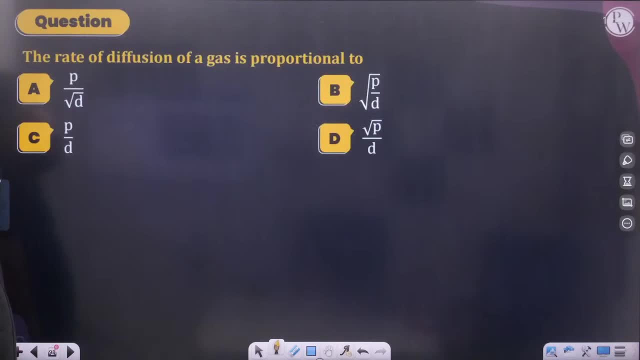 In respect of volume Or in respect of distance Measure from anywhere, There will be no problem. Okay, Let's go Now see the question of rate of diffusion. So this question was asked: Rate of diffusion of directly proportional to. 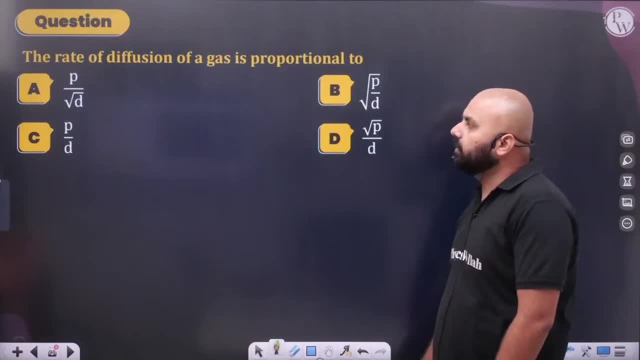 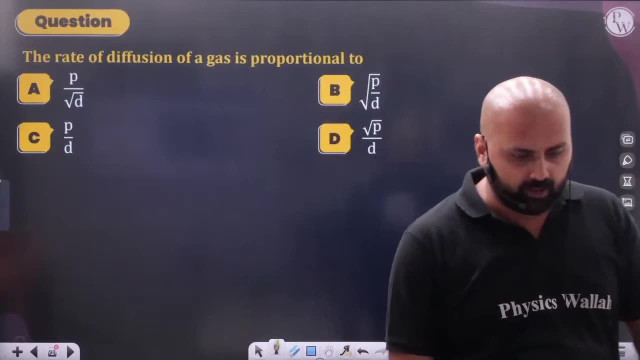 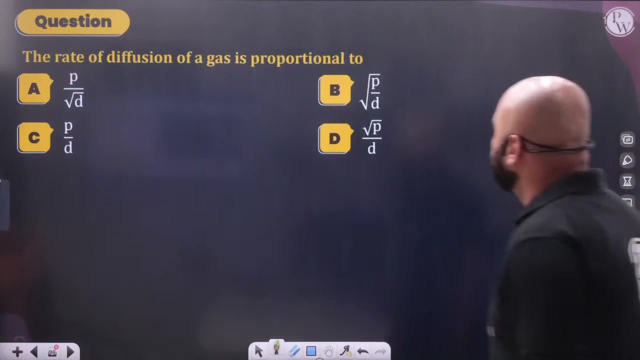 What will happen? What will happen In PYQ, since all-indialible exam has been completed. it has been removed. What will happen? What will happen? A will happen, What will happen, A will happen. It is a simple thing. 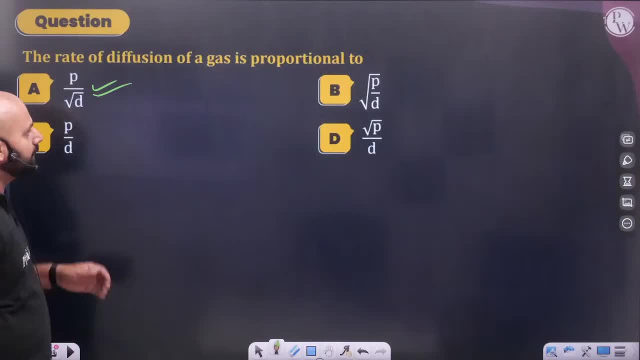 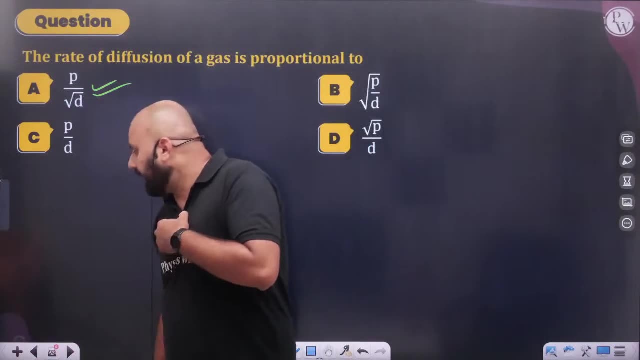 What will happen? A will happen. I have learnt to take values of R earlier. Okay, I have learnt to take values of R earlier. So, after rate of law of diffusion and effusion, if we talk about it later, then one more thing comes in our life. 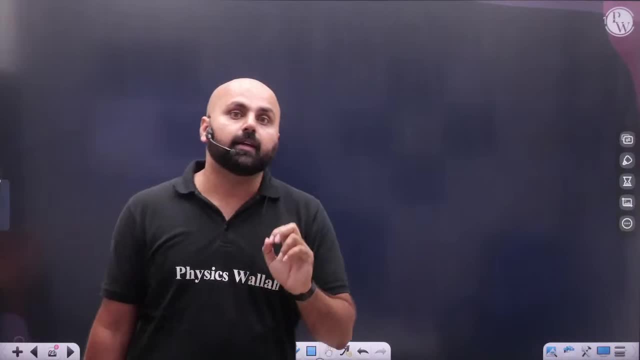 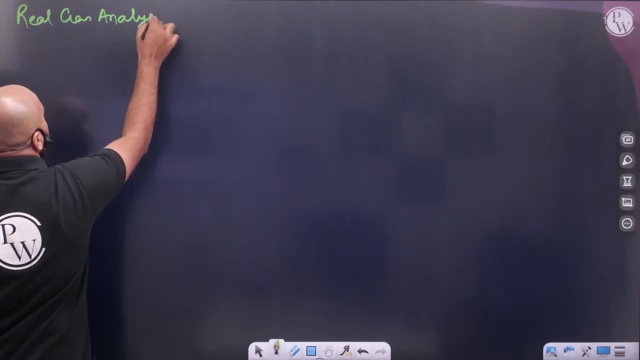 After doing rate of law of diffusion and effusion in our life, comes real gas analysis. What is real gas? So, brother, he is living a different life. What is real gas? He is living a different life. He is saying that, brother, the curve of pressure and volume that you make, 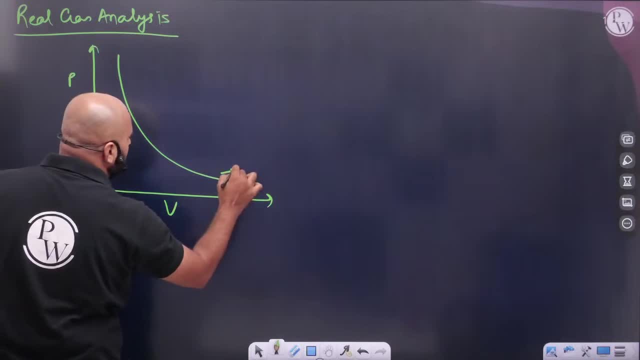 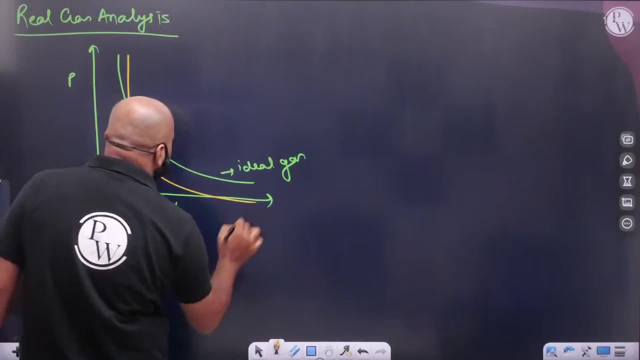 the curve of pressure and volume. if you have made it of ideal gas. if you have made it of ideal gas, then real gas says that I will walk separately. I will not talk like this. I will walk like this. I will walk like this. 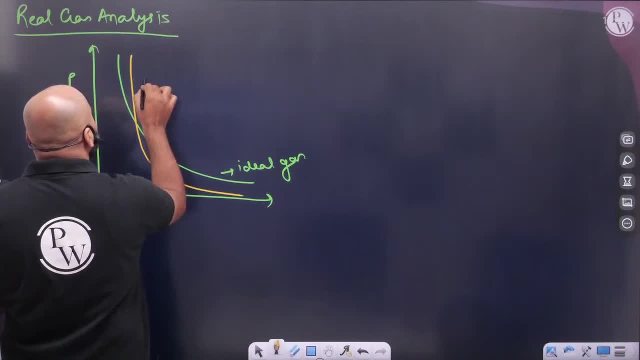 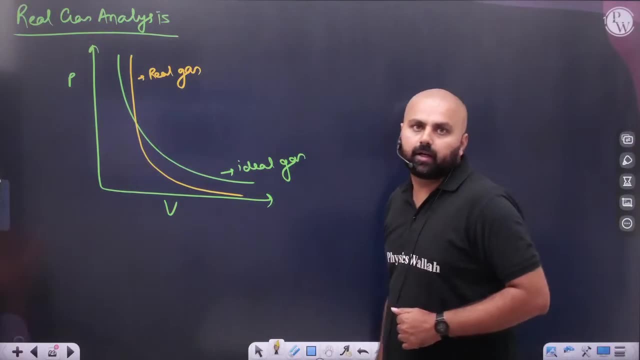 I will walk like this: Okay, This real gas fluctuates like this Means: if you make the graph of pressure and volume of ideal gas, then it becomes different of real gas. And what is real gas? The one who does not fulfill the condition of ideal gas. 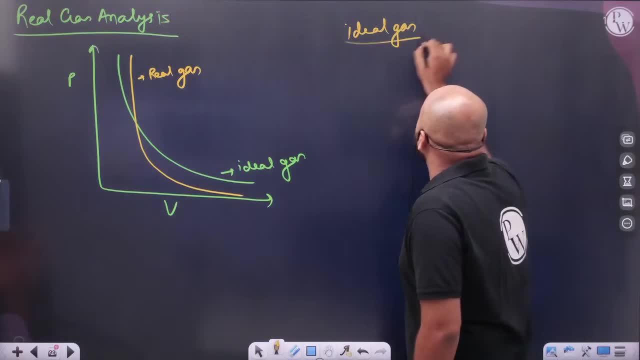 What is ideal gas? The one who listens to you, Who is following- PV is equal to NRT, Real gas- is saying that. I will not listen to him. I will not listen to him. PV is not equal to NRT. Okay. 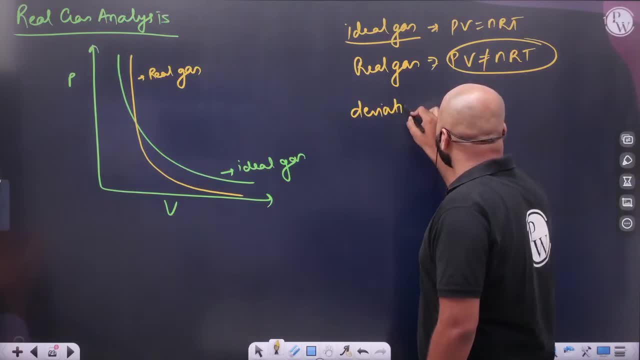 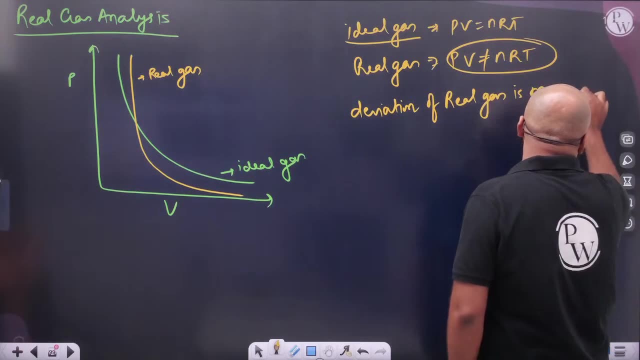 Then, who said, Sir, these people will deviate. So how to measure their deviation? We measure the deviation of real gas. Deviation of real gas is measured. In which term do we measure this? Measured in terms of? In which term do we measure? 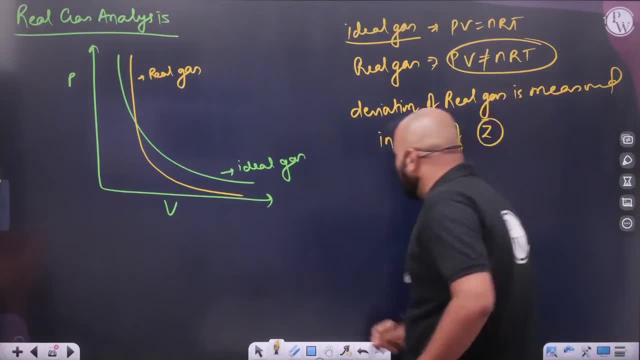 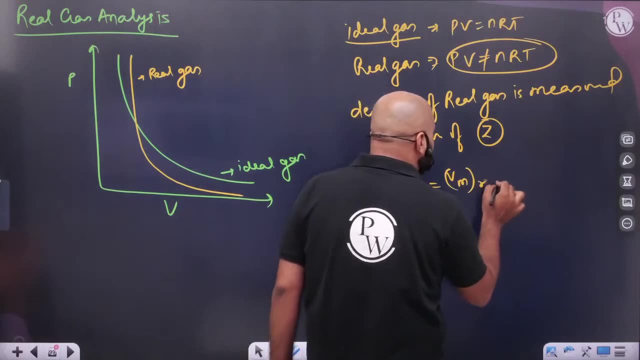 Sir, in terms of compressibility factor, In terms of Z, What is Z? So see this with you: PV upon NRT, Or we call it volume: Whose Volume of real gas, Volume of molar, And divide by the volume of ideal gas? 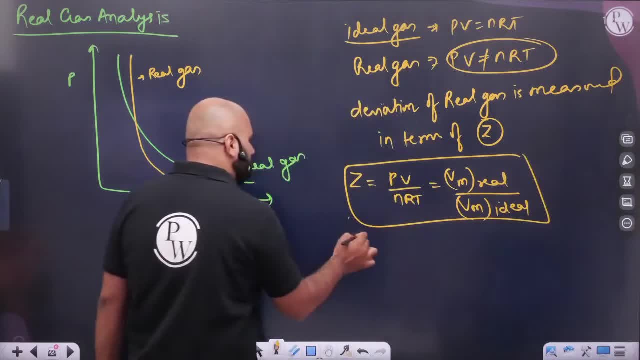 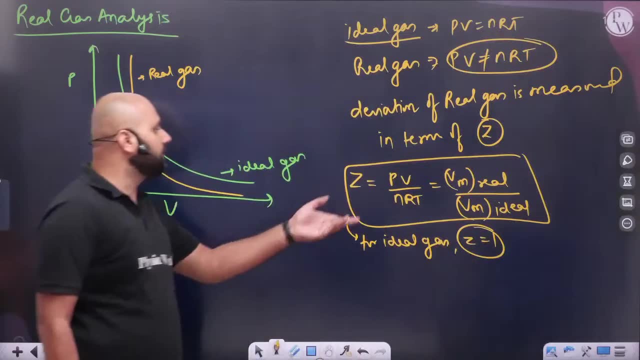 We will see The value of Z in ideal gas. For ideal gas, For ideal gas. What is the value of Z? 1 will come. Why? Because, sir, PV is equal to NRT. In ideal gas we have, PV is equal to NRT. 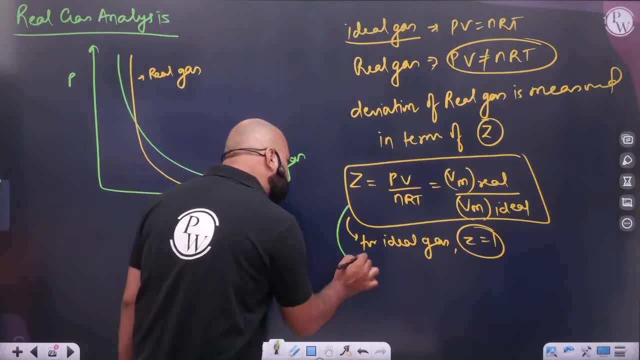 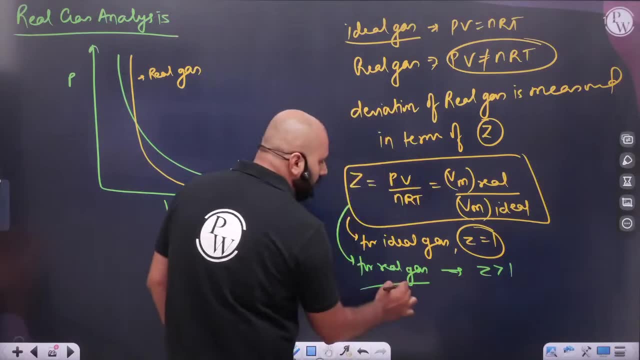 In ideal gas, PV is equal to NRT. But if you talk in real gas, If we talk in real gas, Then Z has two values. Z will be either greater than 1. Or Z will be less than 1.. Look carefully. 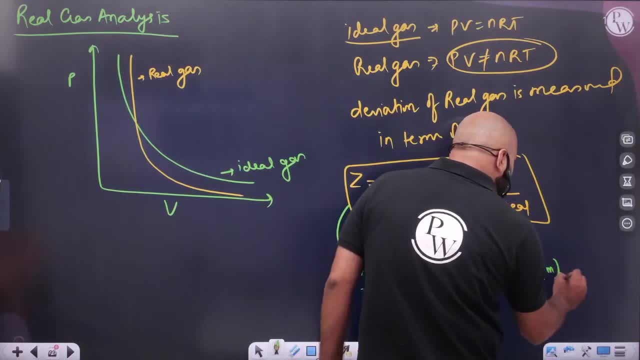 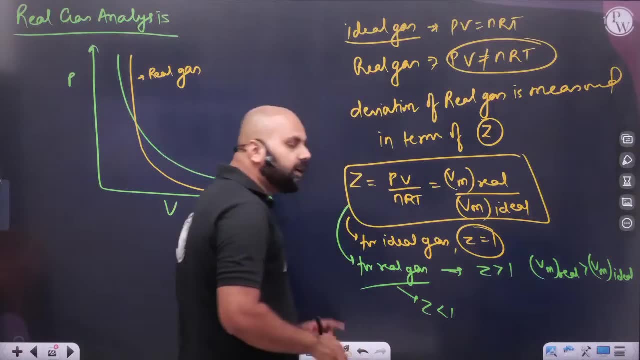 If it is greater than 1. Means volume of real gas. Volume of real gas Is more than the volume of ideal gas. When can this happen? When your molecules are far, far away? When can it happen When which force dominates in you? 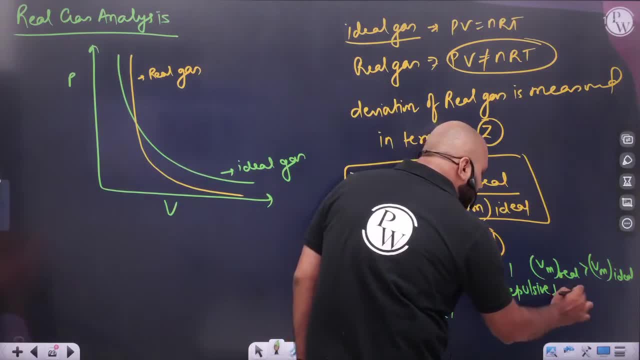 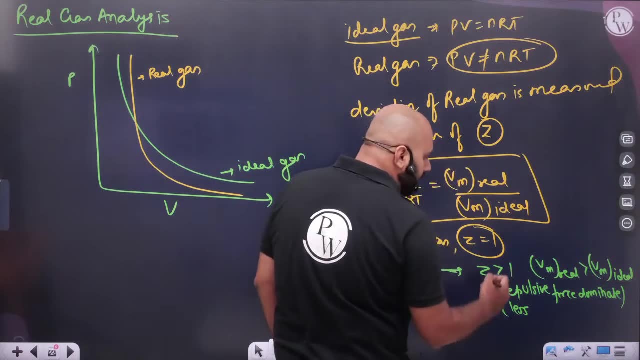 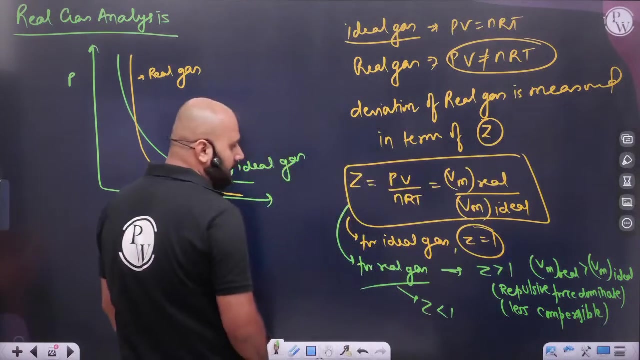 Repulsive force dominates. When which force dominates in you, Repulsive force dominates. And when repulsive force dominates, It means your molecules Don't want to come close and it will be difficult to compress, Less compressible Or we can say, difficult to compress. 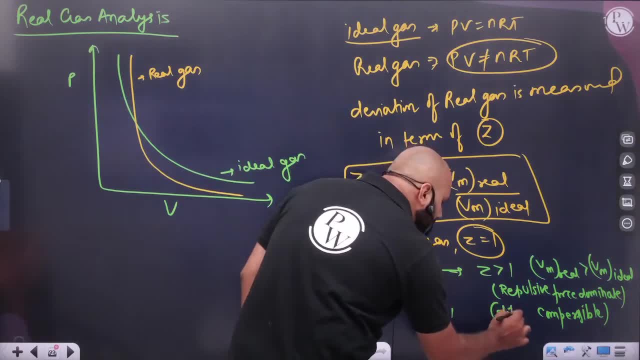 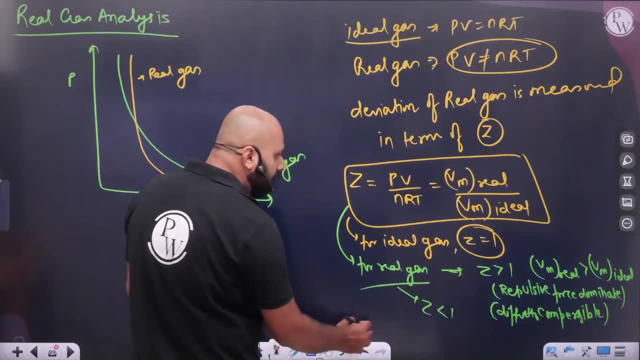 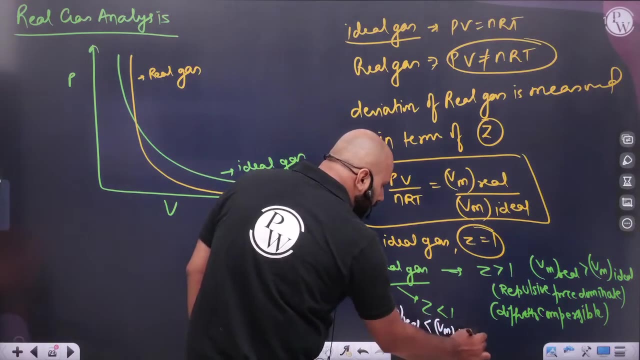 It is difficult to compress because it has repulsive force, Difficult to compress. But if the value of Z is less than 1, then what will happen? The volume of the real gas will be less than the ideal gas. It means attractive force is more. 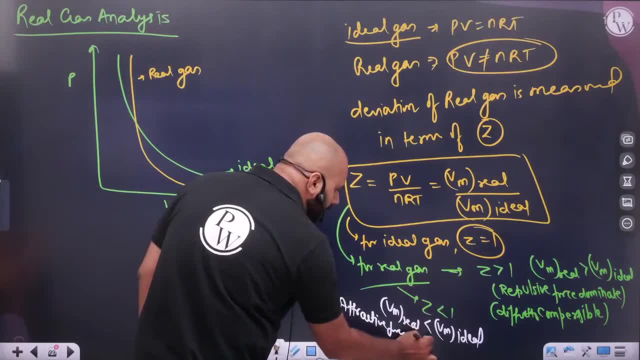 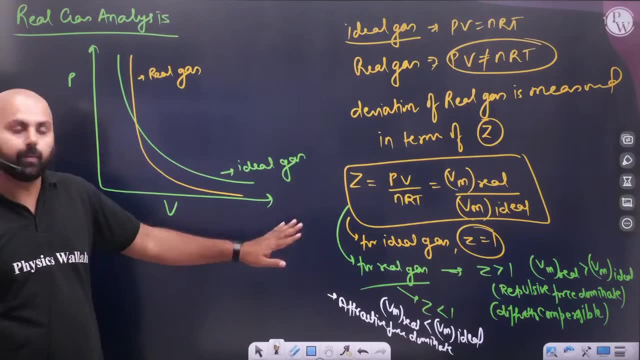 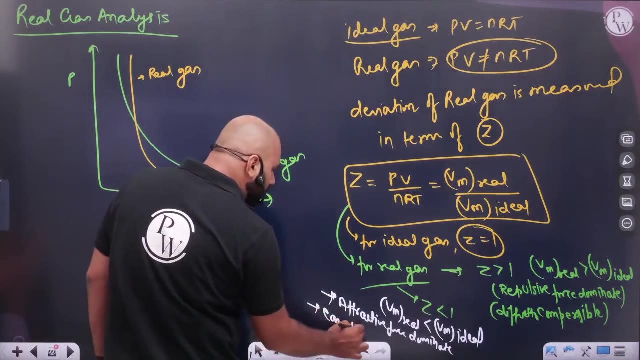 Attractive force is dominating. See, the questions are like this. We don't know numerical from this portion, Only theory comes from this portion. Here attractive force will dominate. Attractive force means easy to compress. You can compress it easily. So Z value is 2.. 1 is greater than 1 and 1 is less than 1.. 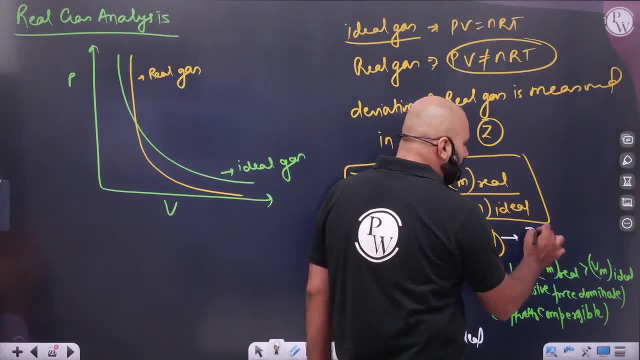 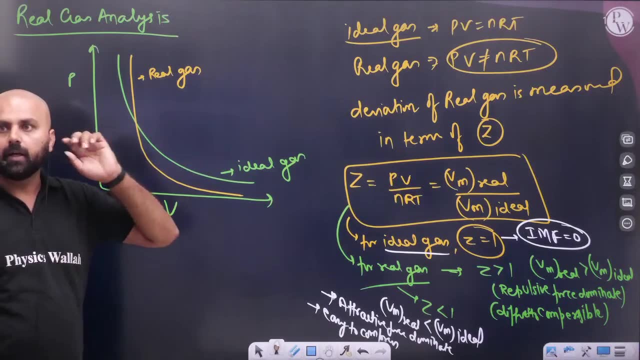 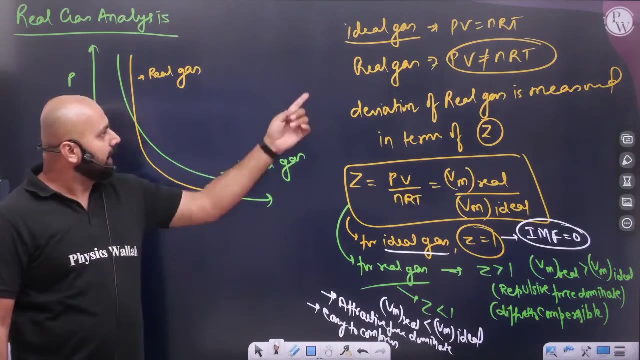 Someone said: in ideal gas There is no attractive force. Intermolecular force is 0. in ideal gas, Intermolecular force is 0. Remove it in that case. So all these things happened: Ideal gas, real gas, Real gas analysis. 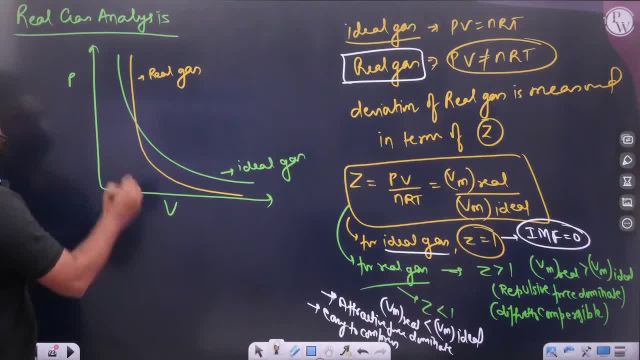 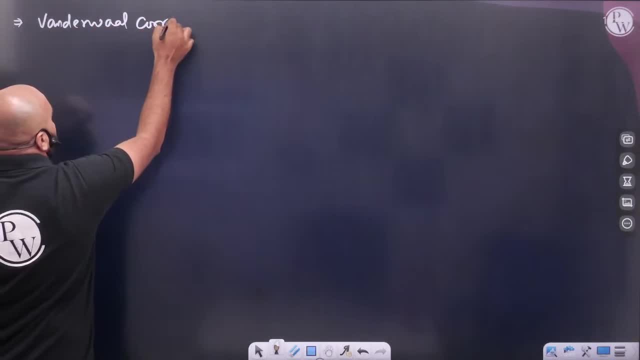 Ideal gas, real gas. Then who said: what happens in real gas? What happened in real gas? Vanderval correction came in real gas analysis. It was said in pressure correction. What was said in pressure correction? You are making a mistake, You are neglecting this. 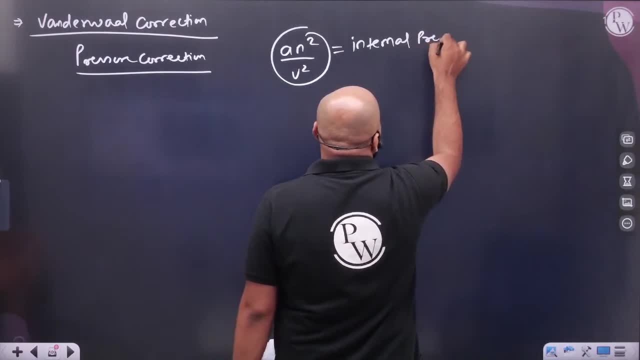 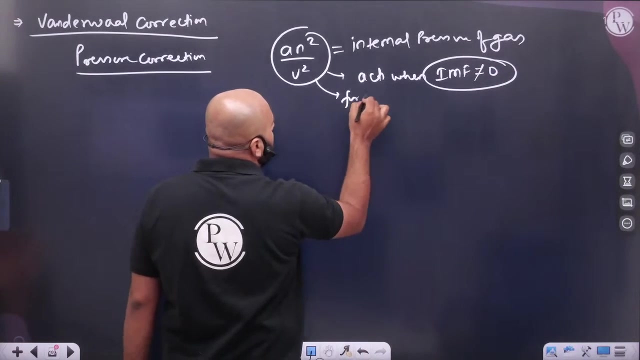 AN square by V square is internal pressure of gas. Sir, when will this come? When will this come When intermolecular force is not equal to 0.. Intermolecular force is not equal to 0.. For whom? For real gas? 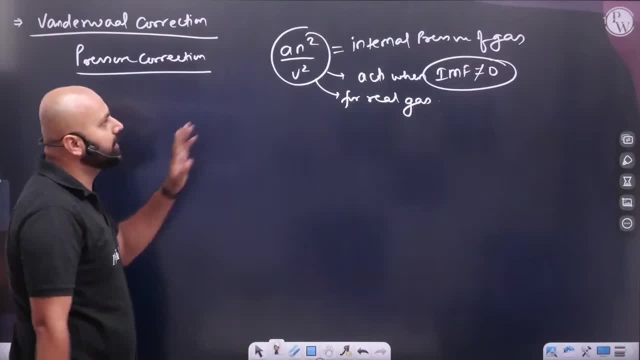 This is for real gas. This is correction term. This is internal gas. What will be your pressure? P plus AN square by V square. If someone asks you Pressure of ideal gas, Then pressure of ideal gas is nothing: Pressure of real gas plus AN square by V square. 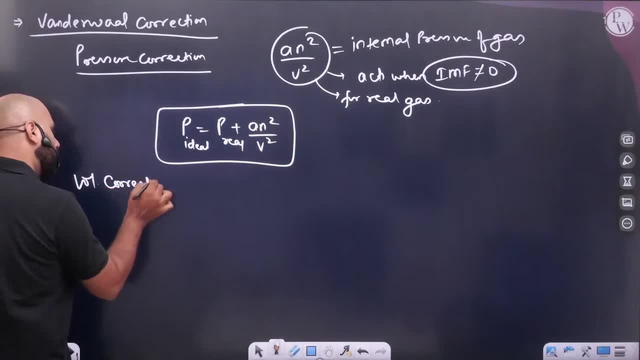 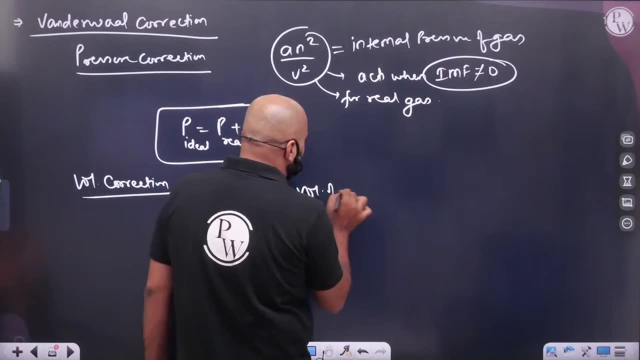 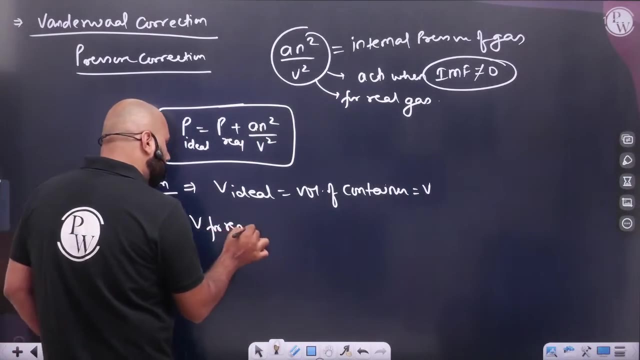 Similarly in volume correction. In volume correction also 2 corrections were done. Sir, what was the volume for ideal gas? Volume of container? Why? Because sir volume of container V, But sir volume for real gas was taken. So what will be the volume in real gas? 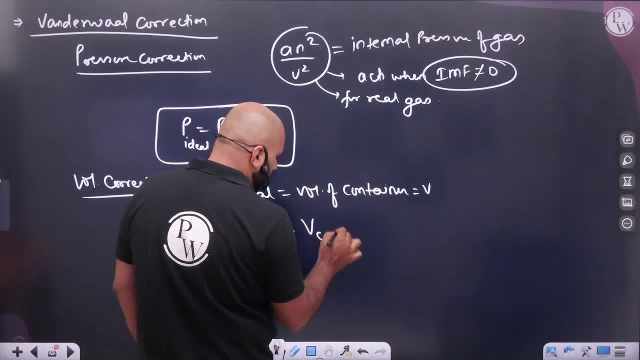 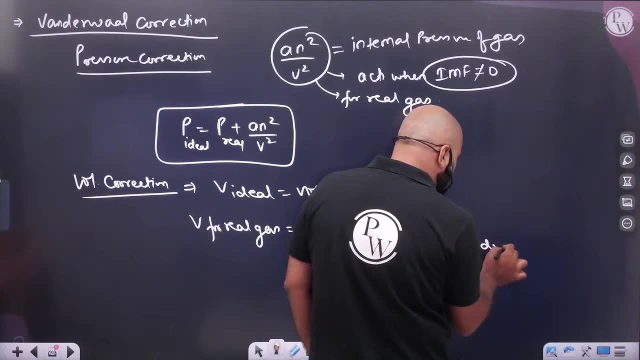 Sir, volume of container Minus V, minus V minus NB, Where NB is known as excluded volume. What do we call NB, Excluded volume, Or what do we call Co-volume? What will NB come to us, Co-volume? 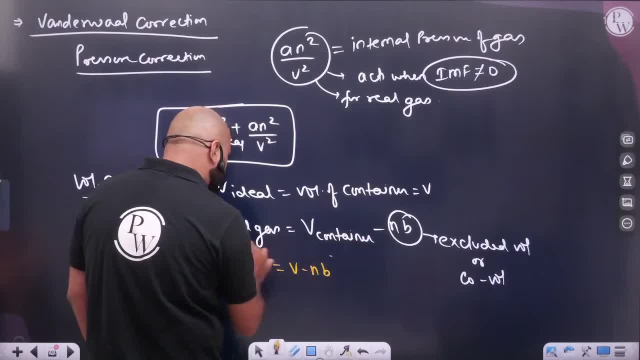 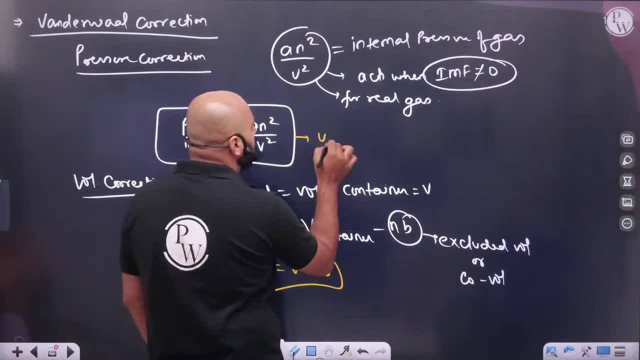 What is the value of V, V minus NB came? We use this. Remember, guys, If you know unit dimension, Then you can calculate units. If we want to say unit of A directly, Then what will be unit of A, Sir? unit of. 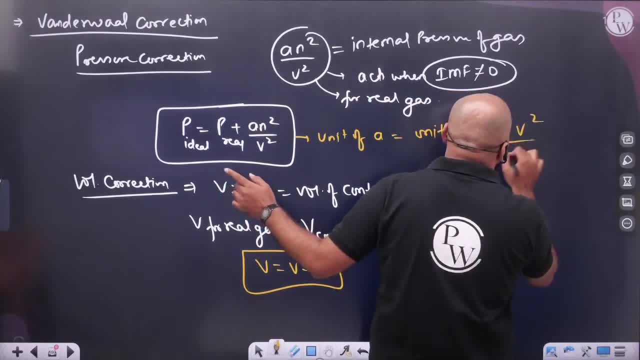 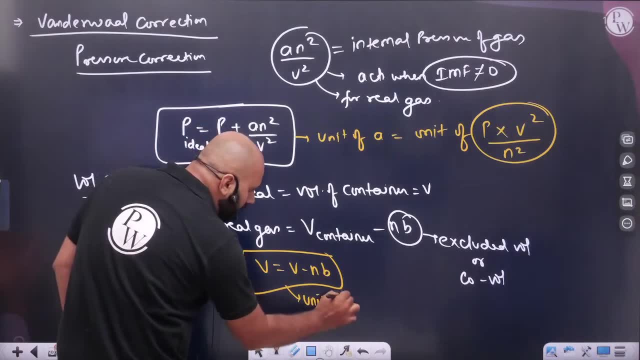 See how I am writing: Pressure into volume square upon number of moles. How am I writing? You are wise, Keep understanding. If I talk about unit of B, Then unit of B is nothing. Unit of Unit of volume divided by number of moles. 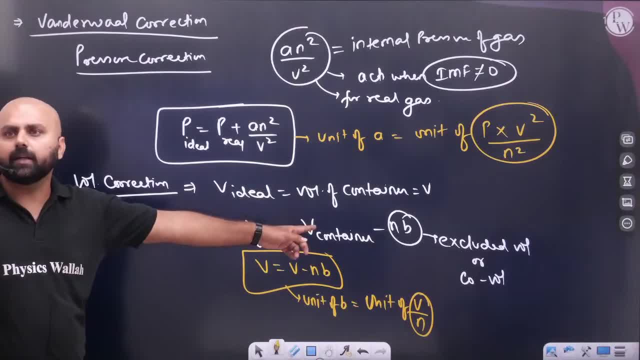 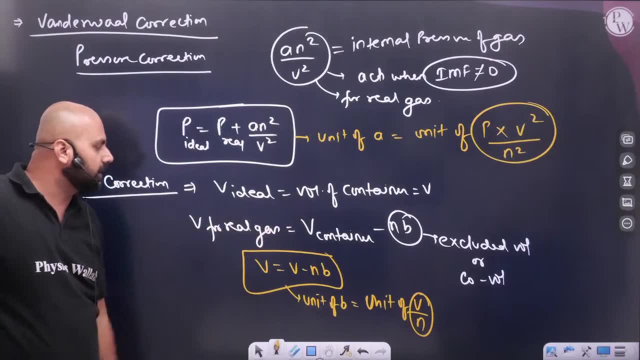 Calculate unit like this: Okay. Calculate like this, That's it Okay. So pick up small things like this. This is what happens in ideal gas. What do we reduce in real gas from container? What do we reduce from container Excluded volume? 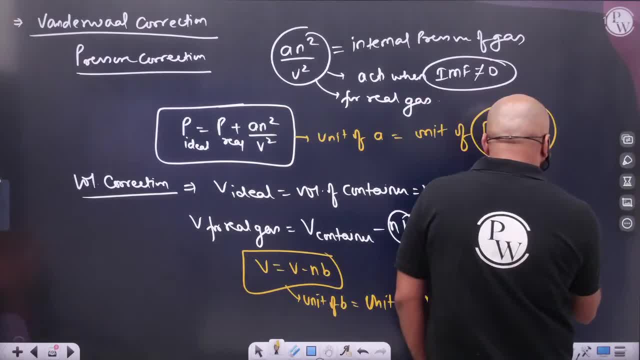 This is what we call volume occupied by. This is what we call volume occupied by gas molecules. What you used to neglect, What you used to neglect, That will come in our life. What you used to neglect, Like: what is A? What does A represent? 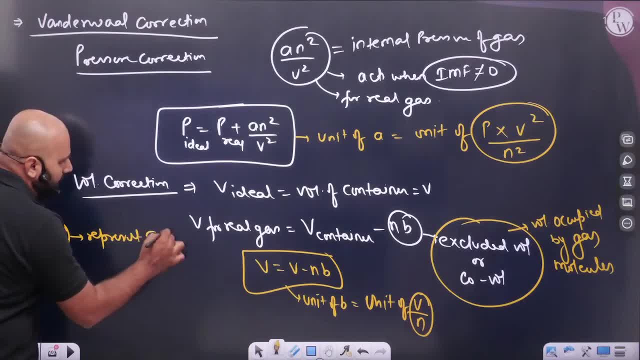 A represents intermolecular force. A represents intermolecular force, Sir. we have A as intermolecular force. What does B represent? Size of gas molecules. Size of gas molecules Means where the size of gas molecules will be bigger. 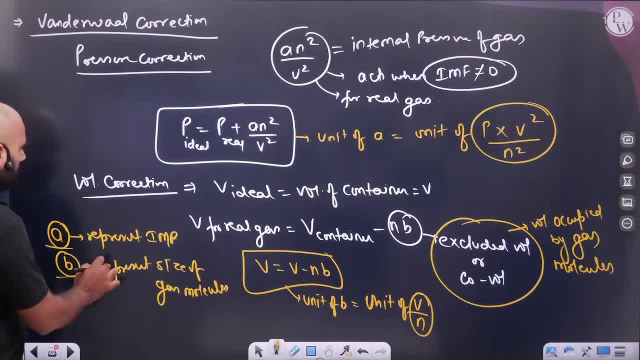 There, the value of A and B will be bigger. What will be the value of A? It will be small. So this will finally come to me after correction. This will finally come after correction. Okay, After that, See this. See this. 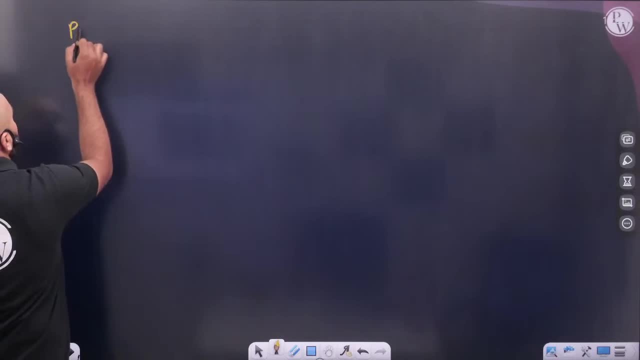 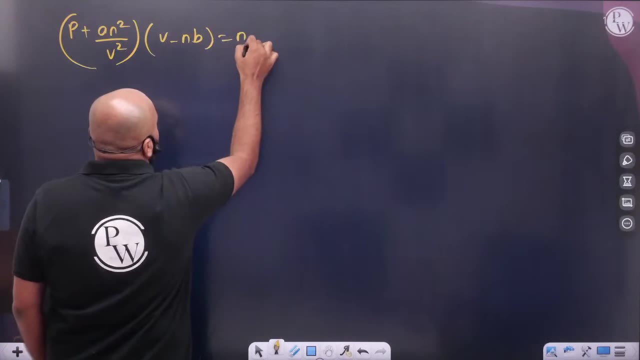 We have. Who told me, Sir, what will come to us? finally, B plus AN square upon V square, P minus V minus NB is equals to NRT. This is the equation which who follows. This is the equation which who follows. 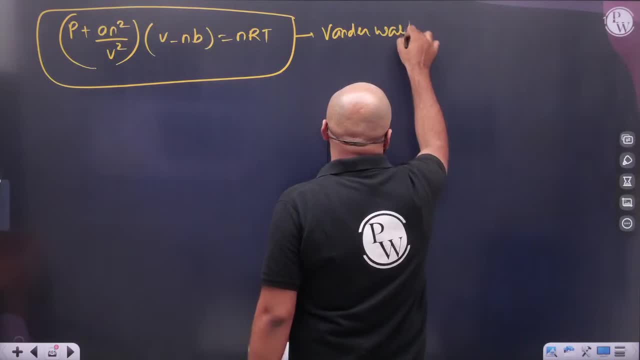 We call this as van der Waal equation Or real gas equation. Van der Waal gas equation Or, if we want to call this, So we can call it real gas equation. Where A and B are. Where A and B are van der Waal gas constant. 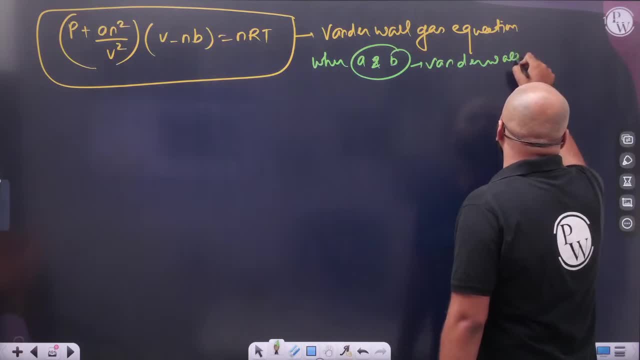 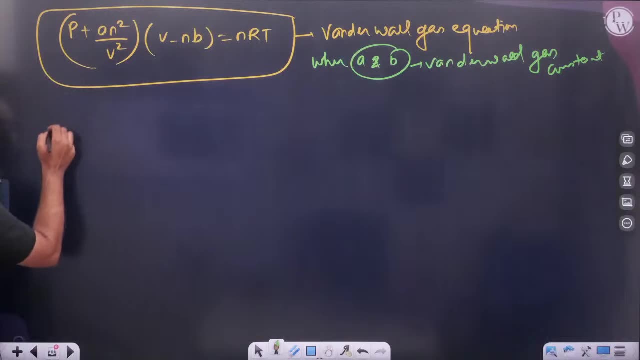 What do we call this? What is A and B Van der Waal gas constant? What is this? Van der Waal gas constant A and B. After that, If different conditions are taken in this, What condition is taken, Sir, if very high pressure is given? 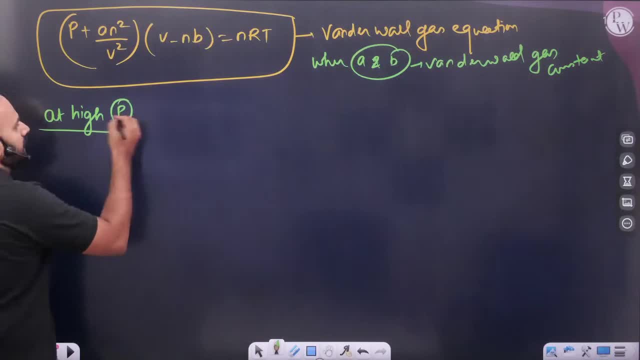 At high pressure is given. So what happens on high pressure? See carefully. What will happen on high pressure, Sir, on high pressure, If pressure is high, Then what will be the volume? It will be low. Volume will be low. 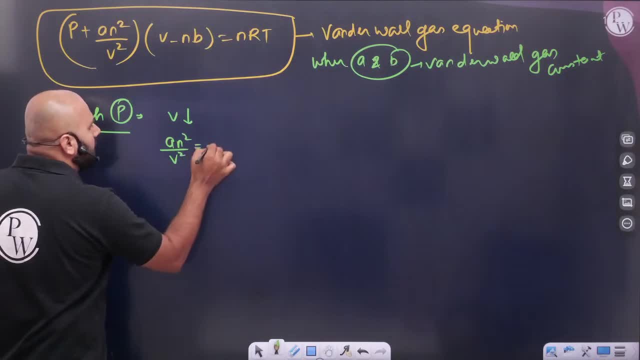 On high pressure, AN square by V square, What will be the value of the value Negligible? So, the value which I have on high pressure, The value which I have on high pressure, The value which will come on high pressure. 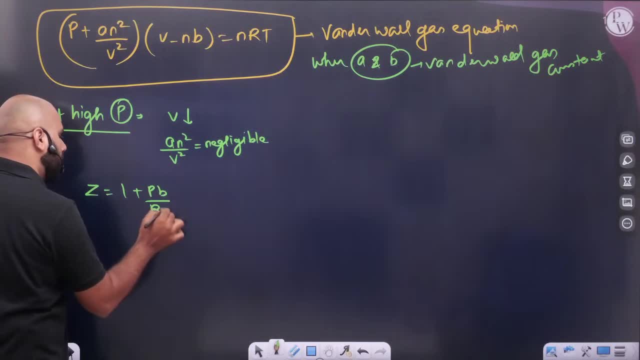 One plus. If I solve this, Then how much will come? One plus Pb by RT will come. If I say at very low pressure, At very low pressure, If I do very low pressure, Then in that case What will be the volume? 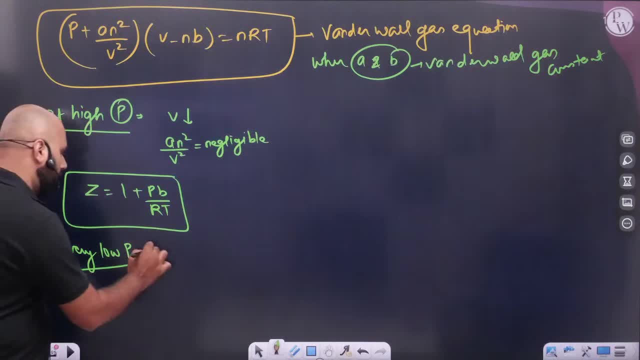 High. In that case, What do we do with Nb- Negligible? I am not doing derivation, I am just coming How it will be Negligible. So what is the value of Z One minus A upon VmRT? 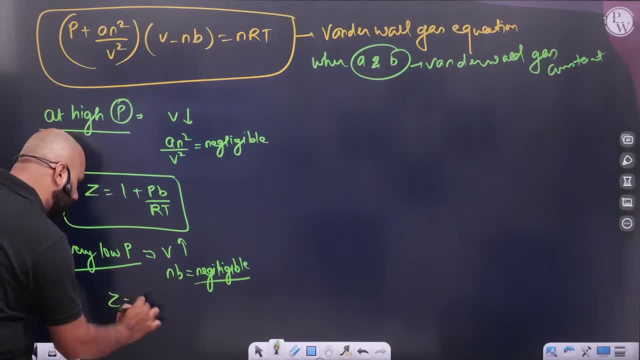 So see the value of Z. The value of Z is different. So what is the value of Z? What is the value of Z? One minus A upon VmRT. So what is the value of Z? Negligible How it will be. 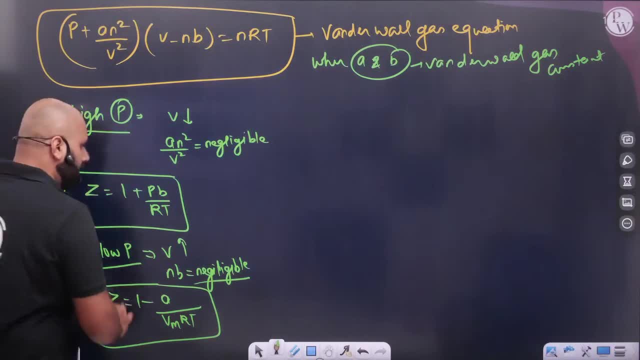 The value of Z is different, Then how it will be Negligible. So what is the value of Z? One minus A upon VmRT. So check the value of Z. The value of Z fluctuates at different kinds of places. 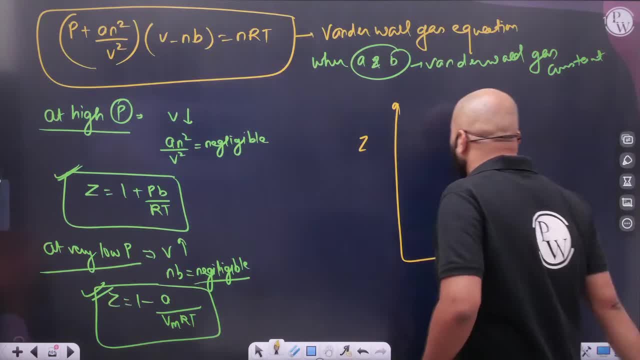 That's why. That's why, if you look, If we will make Z's graph, If we make Z's graph, If we will make Z's graph, If we will make Z's graph- nieles 9 to 17- making Z's graph in respect of pressure. 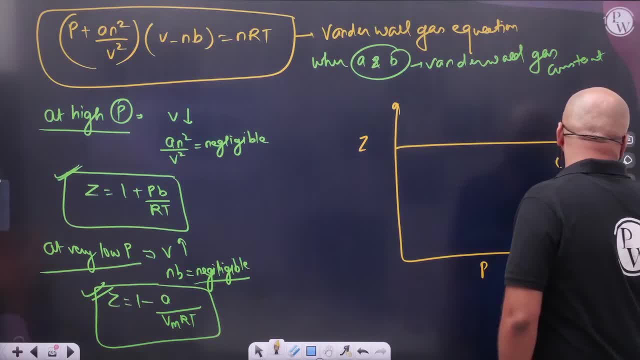 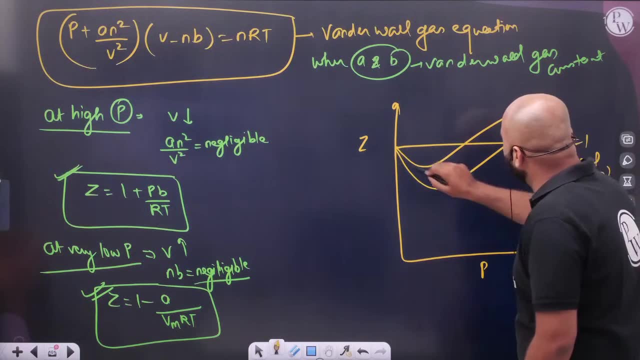 Then all that equals to 1.. For whom, For ideal gas, Z equals to 1, is 1 for ideal gas As the real gas comes, The real gas at low temperature, There is no difference. Look at it at low pressure. 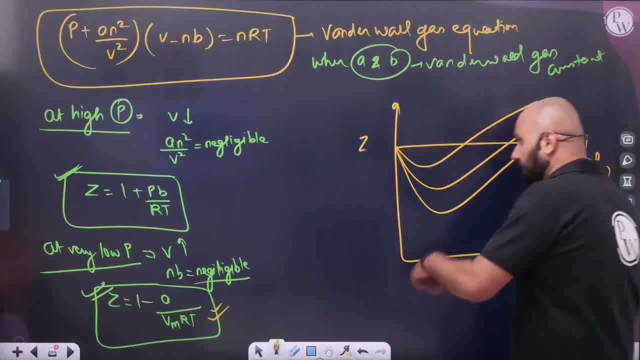 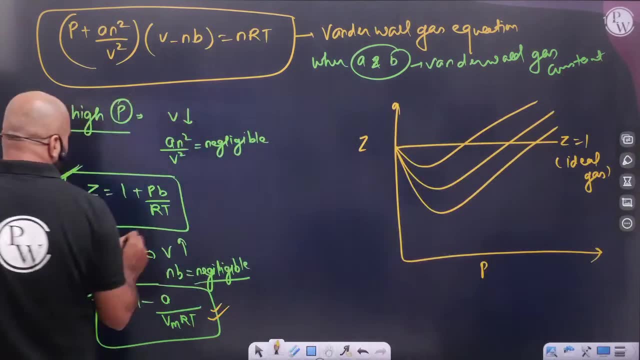 So what is less than 1 at low pressure? As soon as there is high pressure, what is the value of Z? It is passing. So any gas, real gas. what happens at high pressure? This happens. What happens at low pressure? 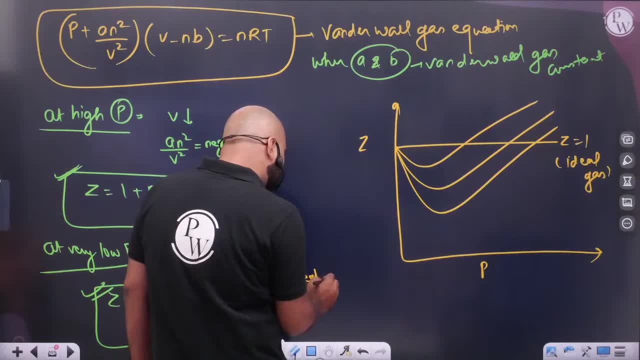 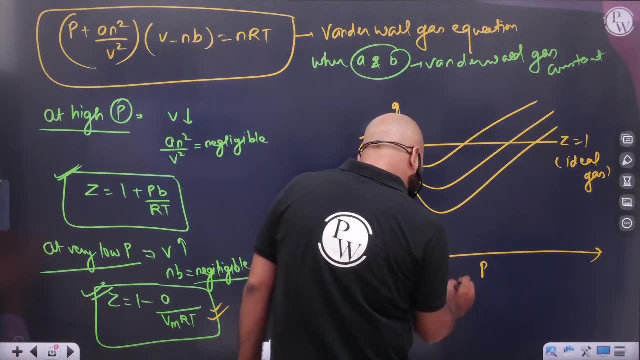 This happens And if there is a real gas, when will the real gas behave like an ideal gas? VHF says ideal gas. When Sir VHF says ideal gas, or you can say at ideal gas, at Boyle's temperature, It starts behaving at Boyle's temperature. 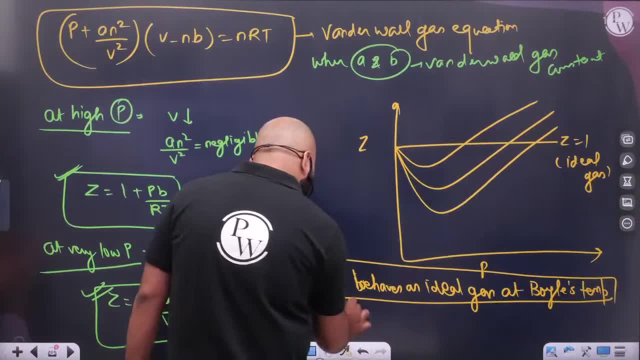 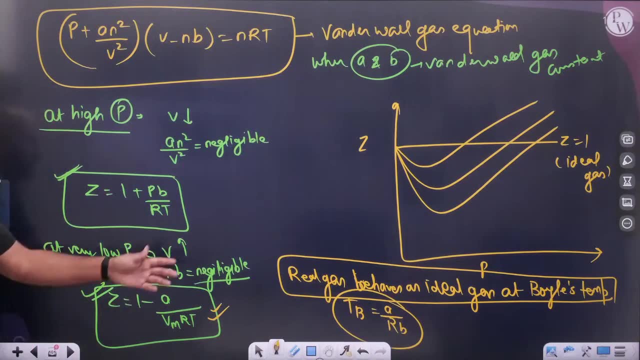 And how does this temperature come? How does Boyle's temperature come? Tb is nothing A upon What will happen. Rb will happen. Tb is nothing A upon What will happen. Rb will come. A upon Rb will come. 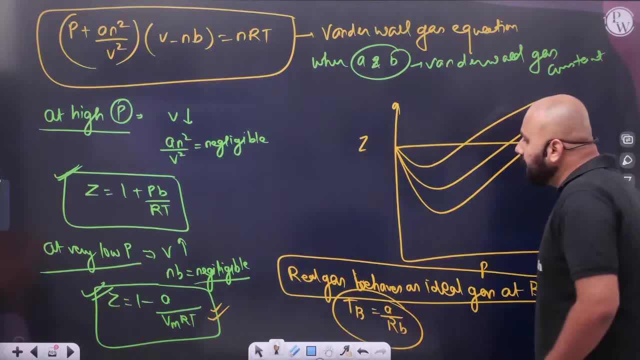 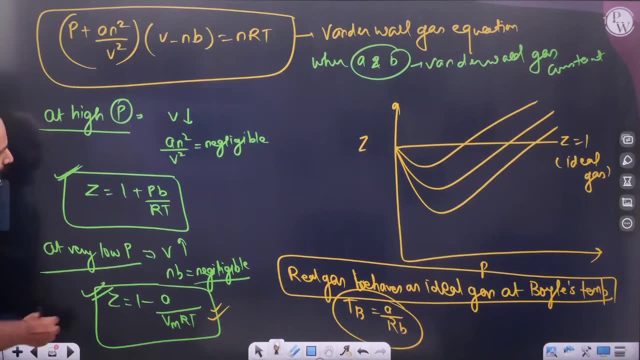 See this with you, See this, Tell me this thing. Who said, sir, when will this real gas start going towards ideal gas? When the value of Z becomes 1.. When will the value of Z become 1? When the pressure is low. 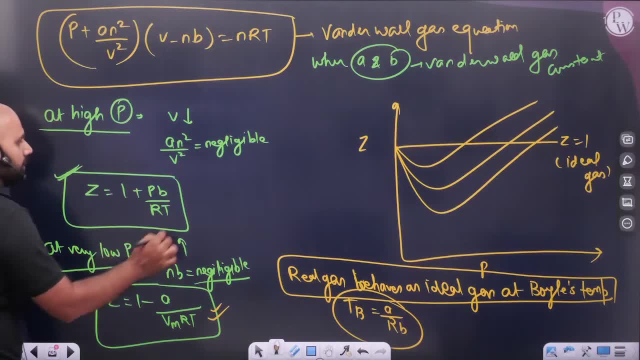 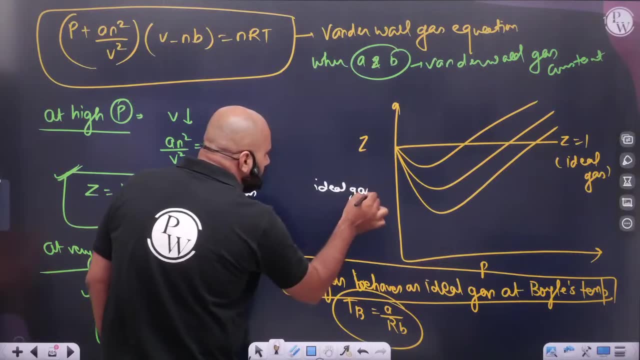 When the pressure is low, What is the temperature Low And what is the temperature High? So it means real gas is real gas. When will it start going towards ideal gas, Real gas. When will the deviation be less Deviation? 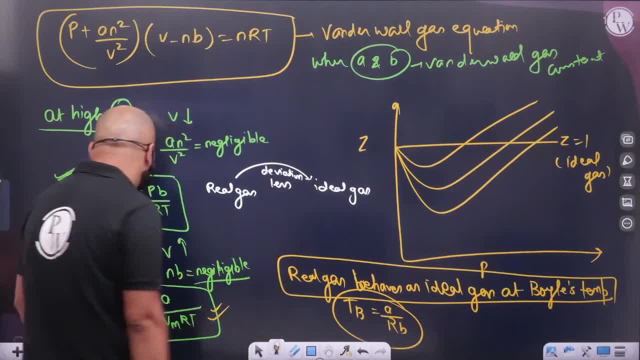 It has to be reduced. It has to be reduced. When will the deviation be less? When the pressure becomes low. What happens to the pressure Low And what happens to the temperature High? So this formula comes. If you see in this, one more condition comes. 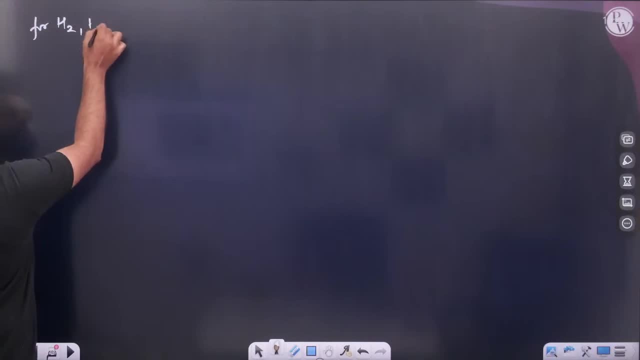 For hydrogen and helium. For hydrogen and helium intermolecular force, what is the value of A Zero? So the value of Z is 1 plus Pb by RT For hydrogen and helium. always, In the case of hydrogen and helium, the value of Z will always remain high. 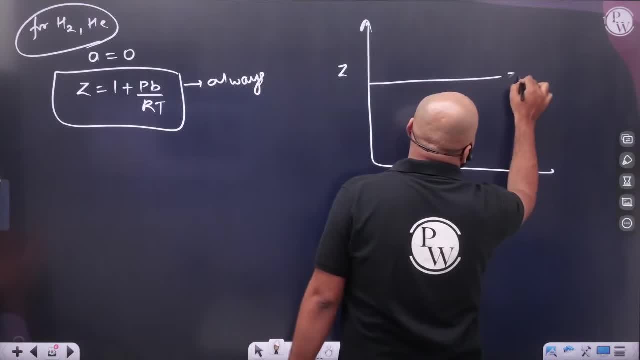 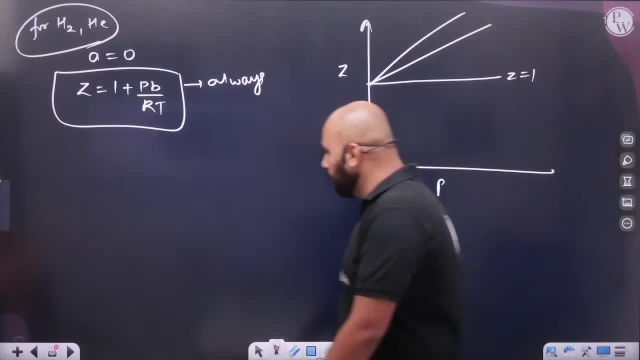 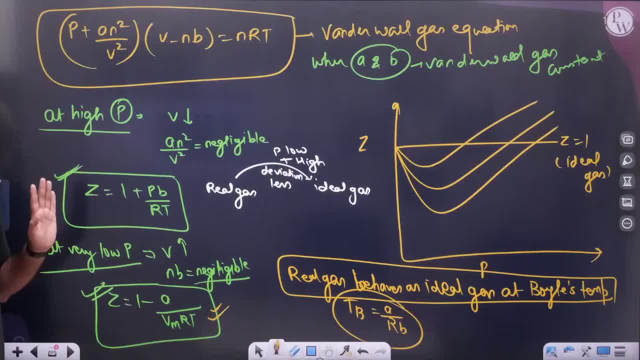 Real gas, ideal gas. Here, the entire theoretical portion is there. The entire theoretical portion is there. Okay, Yes, the entire theoretical portion is there. You have to keep in mind: Real gas behaves like ideal gas Where, At the boil's temperature, 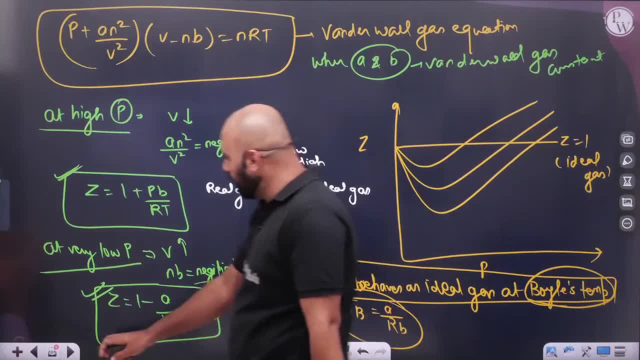 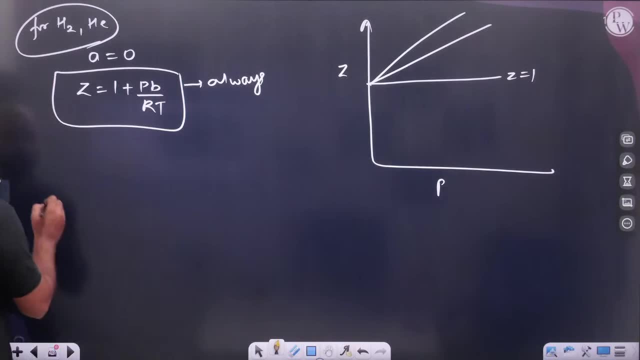 It behaves at the boil's temperature. That's it. At the boil's temperature. Tb is equal to A upon Rb, And that's why we consider this gas as real gas and ideal gas. Now, if you see, we have more small things. 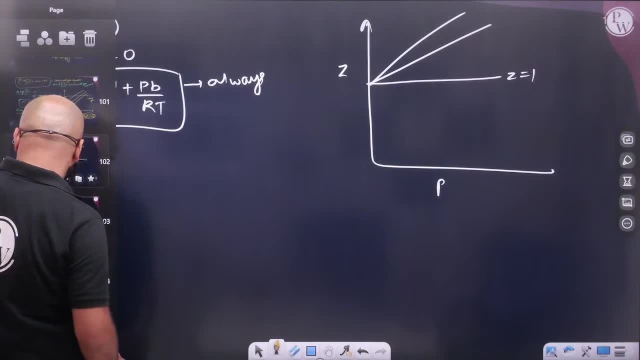 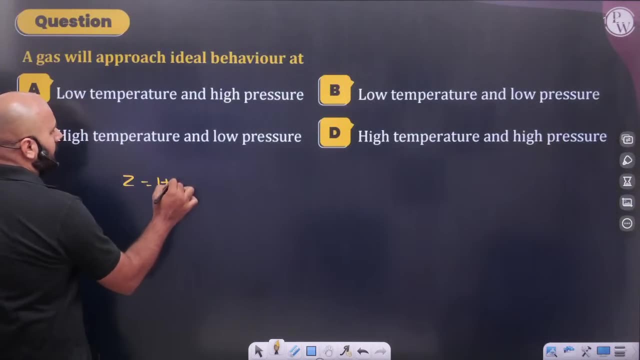 Let's first look at this. Let's look at its questions. See this: A gas will approach ideal behaviour. When will gas approach ideal behaviour? See this: This equation is written. Ideal behaviour means what should be the value of Z. 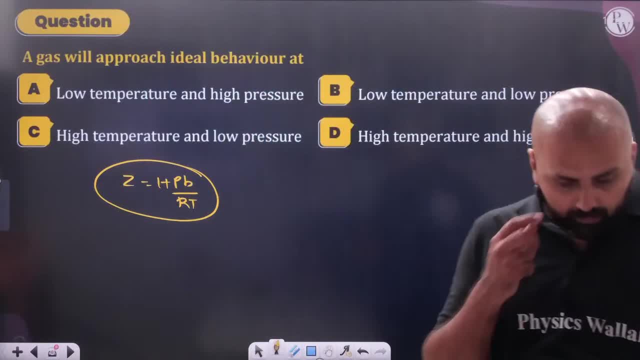 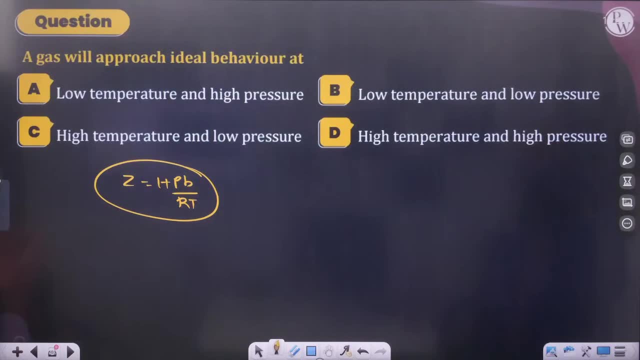 It should be 1.. What should be the value of Z? It should be 1.. So the value of Z is 1.. What will the value of Z be? Will you tell me When will the value of Z be 1?? 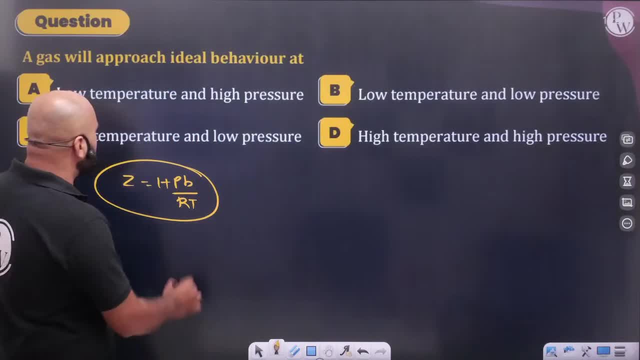 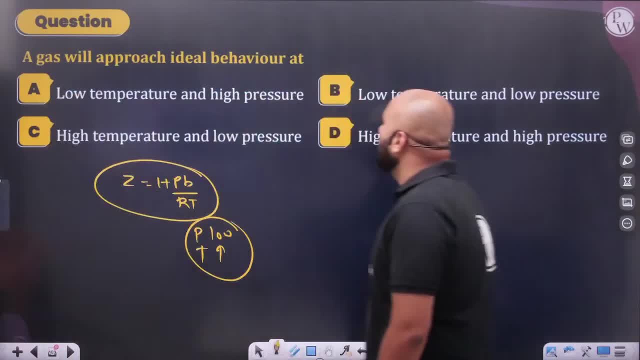 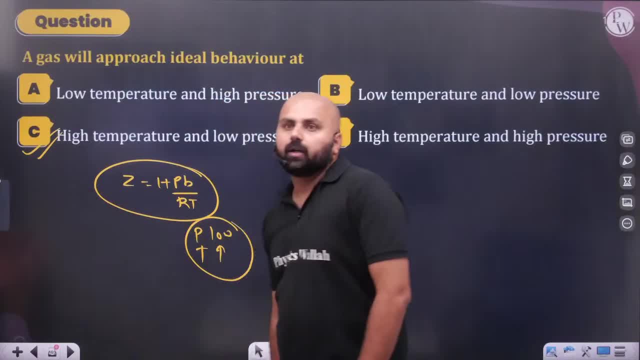 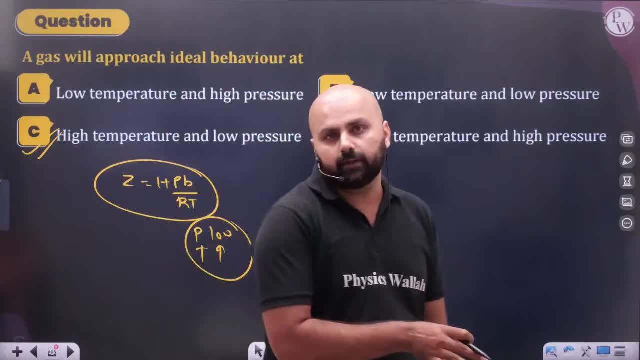 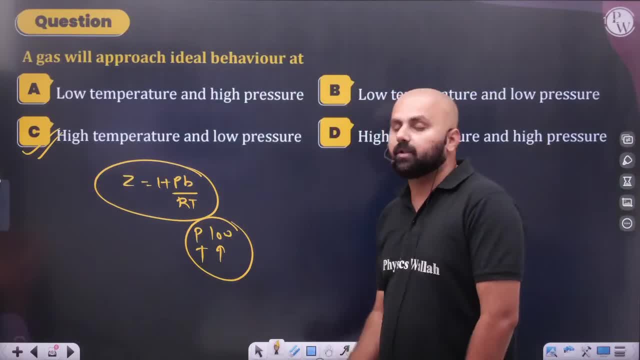 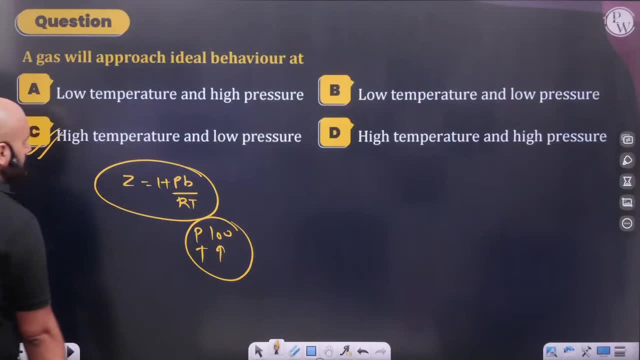 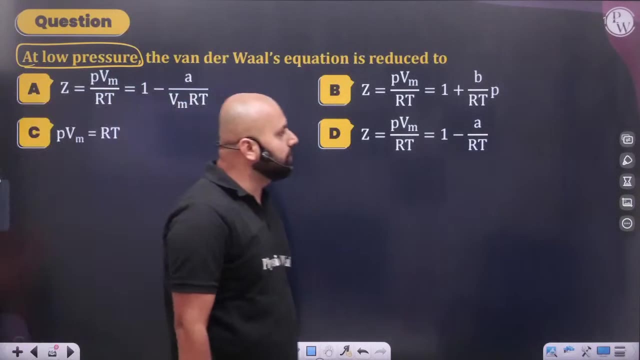 you can do it from the competition, Because everything is mentioned here. That's why I am saying Theory plus questions. If you know the theory, then it's a good thing At low pressure. which equation will be followed? Which equation will be followed at low pressure? 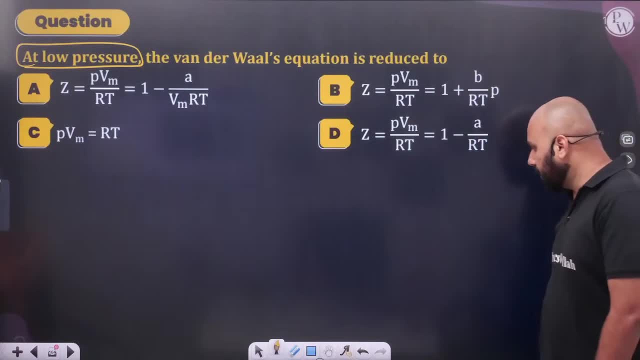 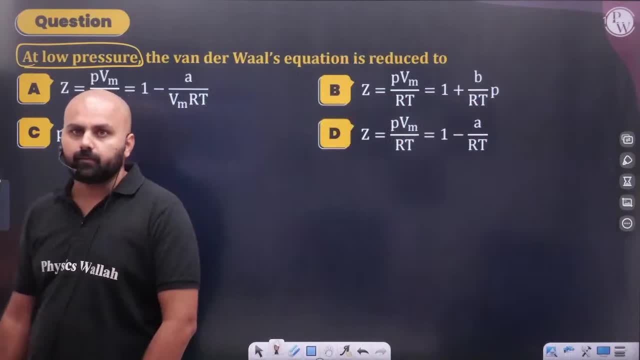 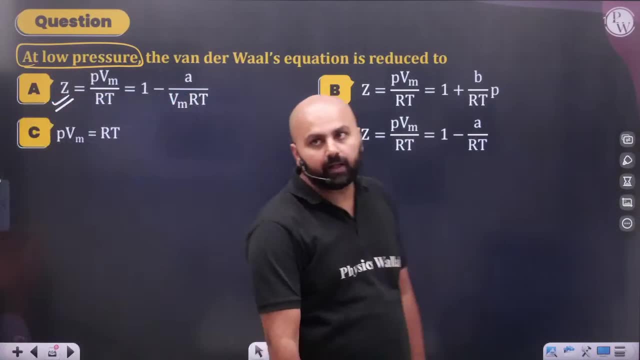 Quickly, What will be the answer. at low pressure, The value of Z will be 1 minus A by VmRT. At low pressure it will be less than 1.. We will have it later. Where did D come from? Vm is releasing the molar volume. 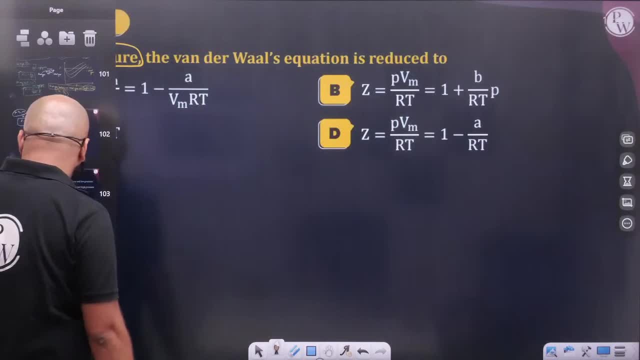 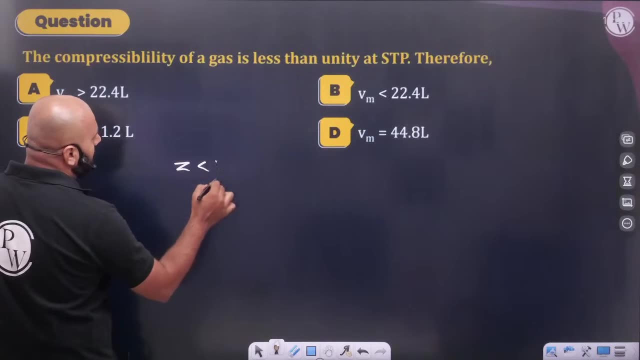 So we will have it later. Then someone said: let's do one thing. Look at this. It's talking about compressibility. The value of Z is less than 1.. So what will be the volume? What is the value of Z? 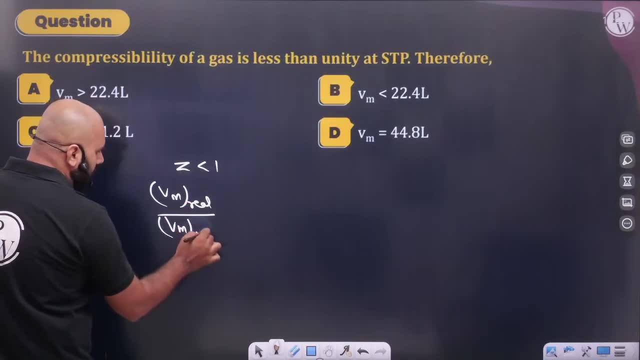 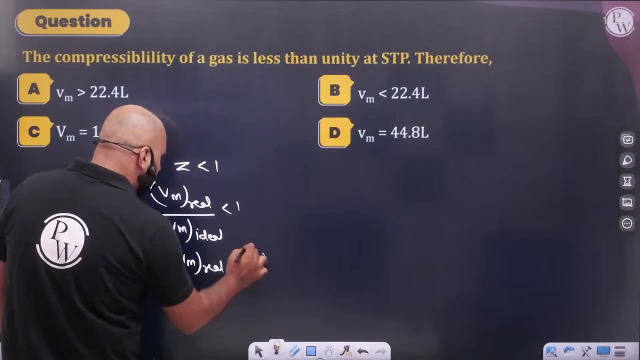 Real gas upon molar. volume of ideal gas. What will be Less than 1.. So what will be the volume of real gas? It will be less than the volume of ideal gas. The value of Z is less than unity, So what will be the volume? Less than What is the molar volume of ideal gas: 22.4.. So what will be the volume? It will be less than 22.4.. What will be the volume? It will be less than 22.4.. 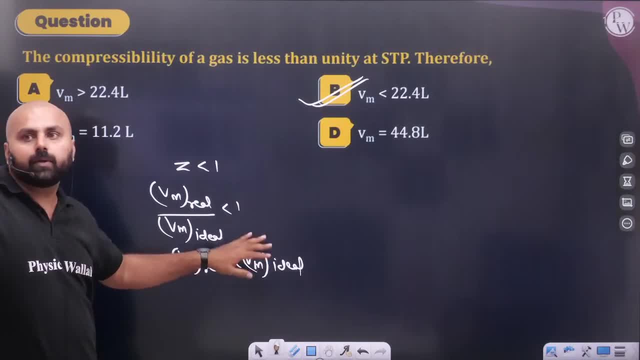 Sir, it's a simple thing. Compressibility is less than 1.. So, real upon ideal, What will be the ideal gas? Big, So what will be the molar volume? Real gas, What will be the ideal gas? 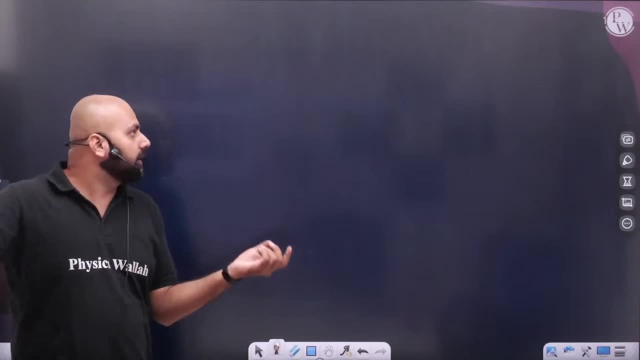 In fact we were talking about the Real gas, the ideal gas, we were talking about the kinetic theory of gas, the speed we saw, the rate of diffusion and diffusion. Then if someone asks us in the state submitter, a simple thing comes. 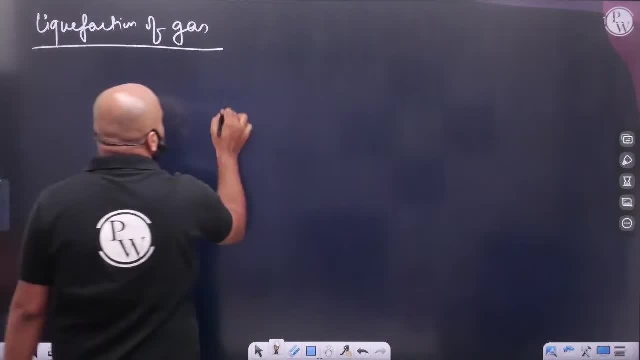 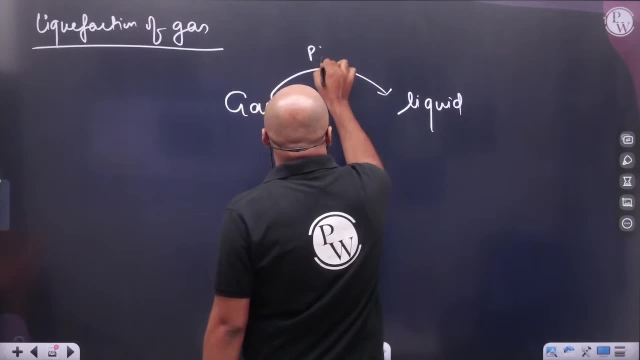 that is known as liquefaction of gas. What is liquefaction of gas? That is, to liquefy any gas. Remember, I am writing a direct line to liquefy gas. Pressure should be greater than critical pressure and temperature should be less than critical. 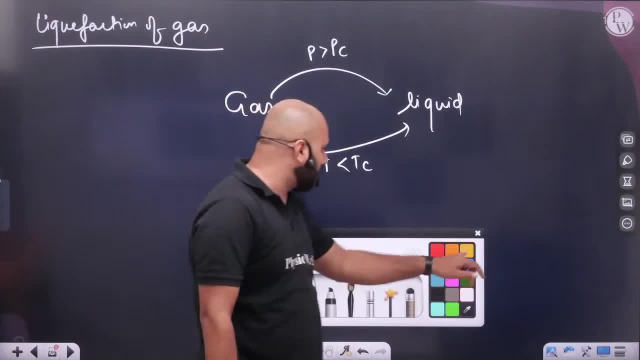 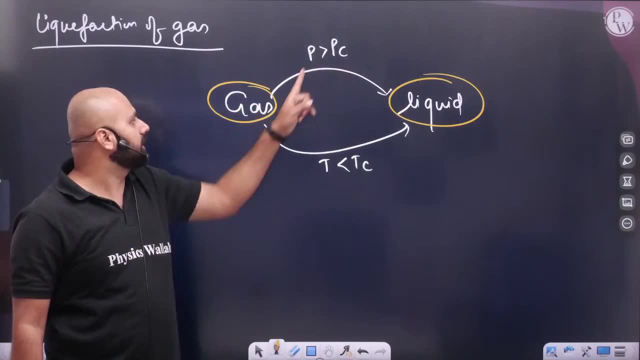 temperature. Remember two conditions: gas has to be liquefied. if you want to take the gas in liquid, then remember the condition to take the gas in liquid. Pressure should always be greater than critical pressure and temperature should be less than Tc. 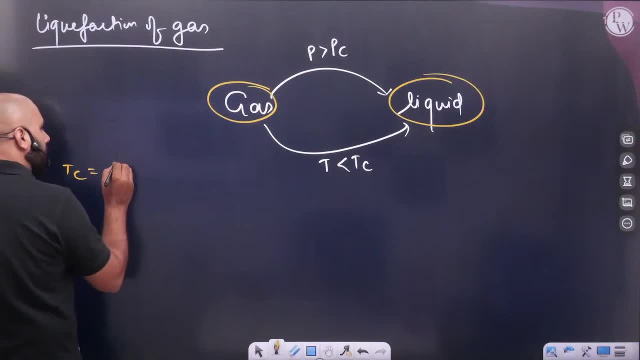 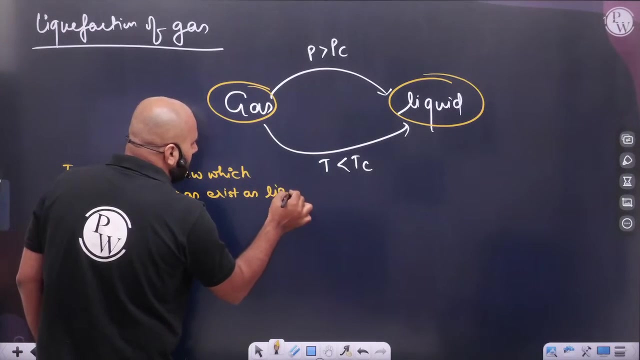 Sir, what is Tc Critical temperature? Where, Sir, if you see, above this temperature, temperature below which this gas will exist, in whose form? In which form? Temperature below which gas exist as Gas exist as liquid, The gas which exist in which form? 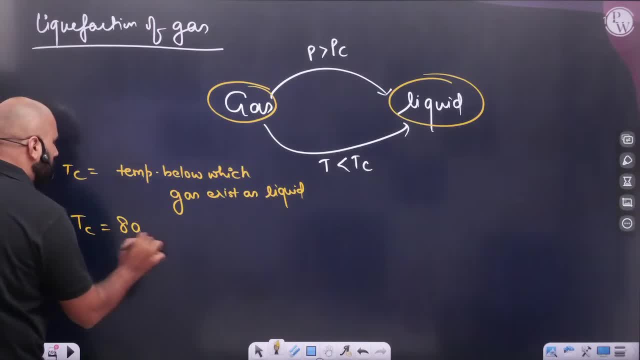 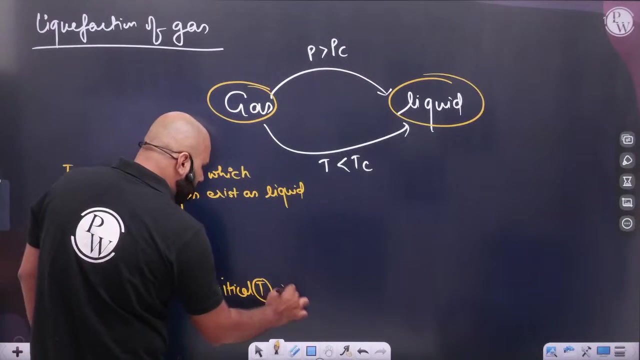 Like liquid. So if you see the formula of Tc, then what will happen? 8a upon 27Rb. is there Critical temperature? this happens, Sir. what is Vc? Volume at volume, of volume at critical temperature and pressure? critical temperature and pressure. 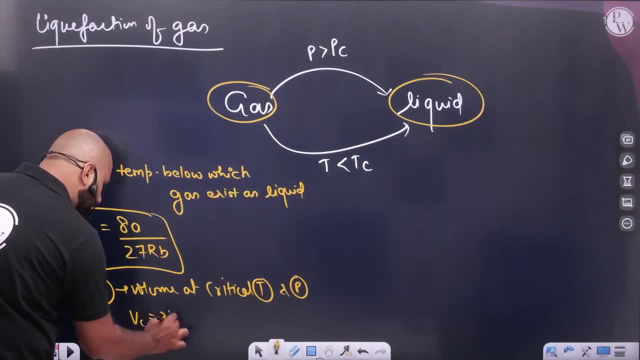 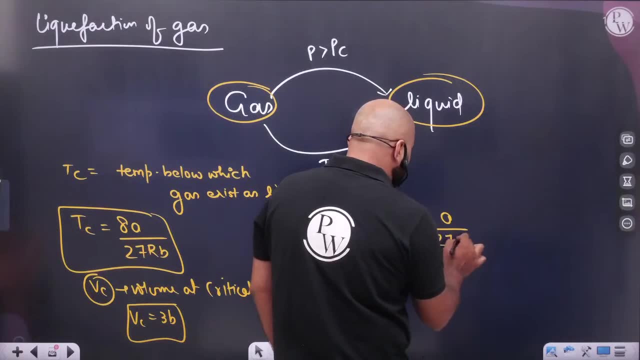 Sir, if you see its volume, what will be the value of Vc? 3 will also be there. If you see the value of critical pressure, then it will be a upon 27b square and even if you take out the compressibility factor at critical time, if you take out Pc, Vc upon. 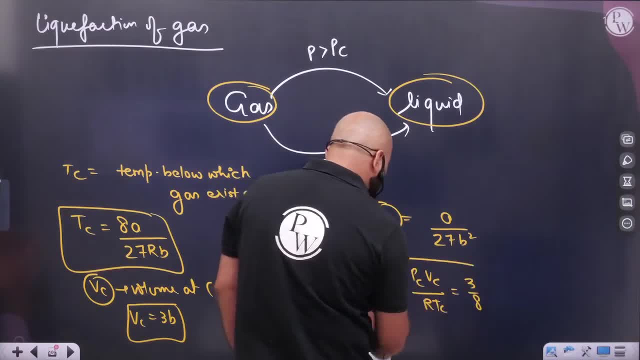 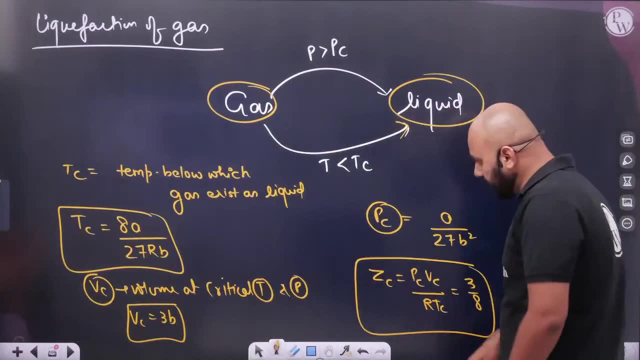 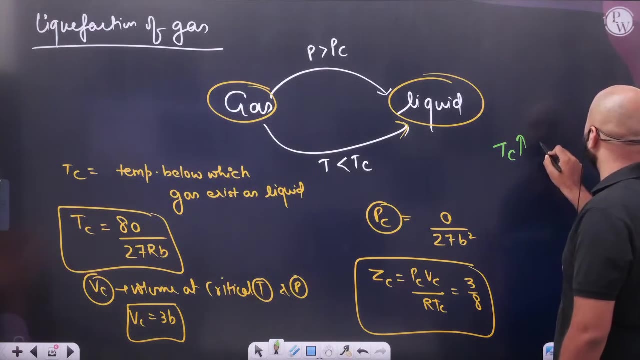 R Tc, then how much will it be? It will be 3 by 8.. So remember, if you want to liquefy the gas, then temperature should be less than Tc. If you want to liquefy any gas, its Tc will be as high as Tc will be as high as the intermolecular. 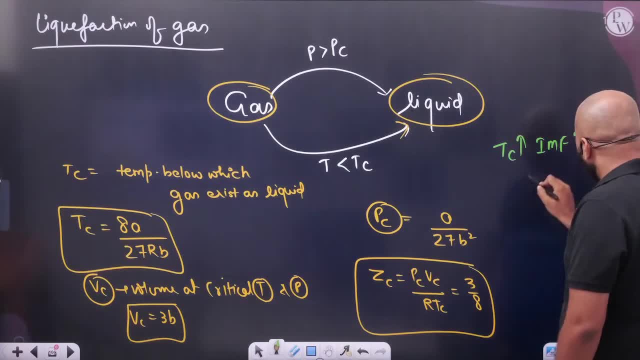 force. What will be its intermolecular force? It will be high. Intermolecular force is high means the ease of liquification: you liquefy it easily, it is easy. What is the ease of liquification? it is easy. 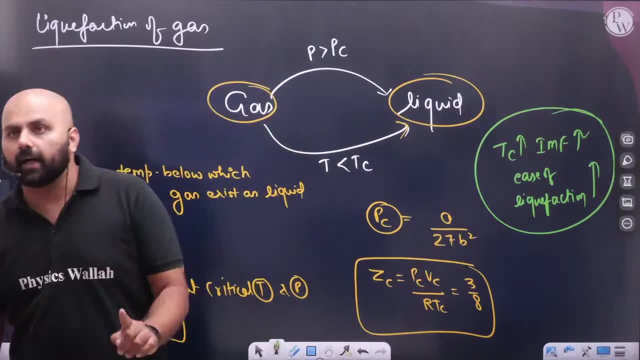 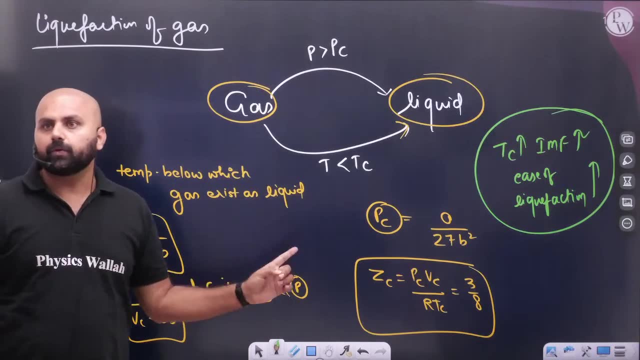 Remember, the higher the critical temperature, the higher the intermolecular force. sir, the intermolecular force will be as high and the ease of liquification will be as easy. Okay, What happens to the equation? with the ease of liquification, it will be easy. 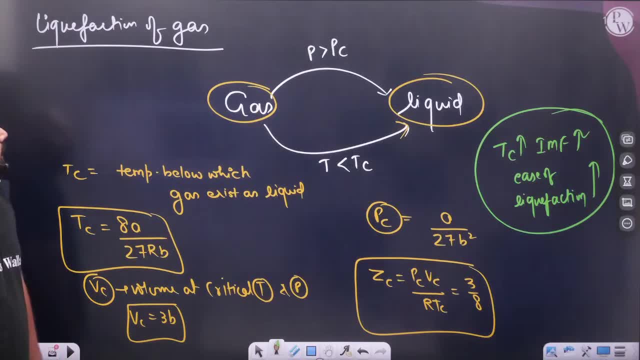 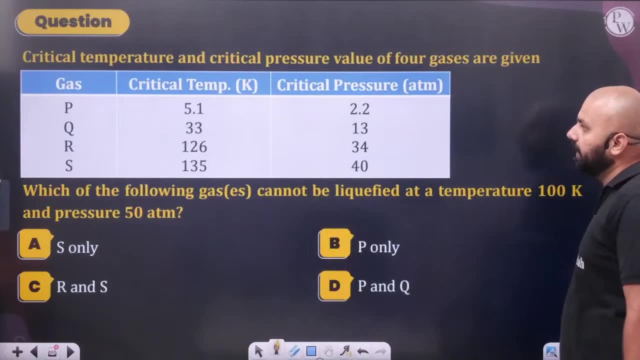 Okay, Now you See, Look at the equation here. it is saying that critical temperature, critical pressure is given critical temperature, critical pressure is given to every gas. PQRS is given critical temperature, critical pressure. It is saying that which gas will not be liquefied if I am keeping the temperature 100 Kelvin and the pressure is 50 atm? 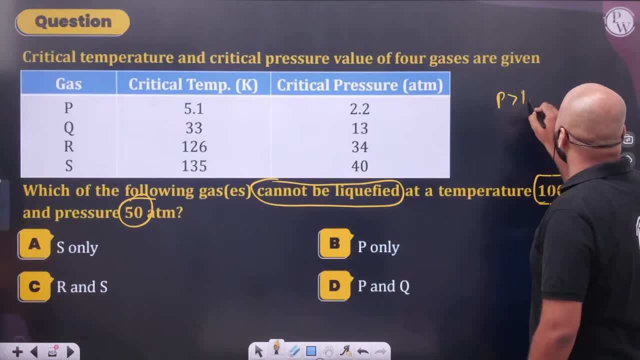 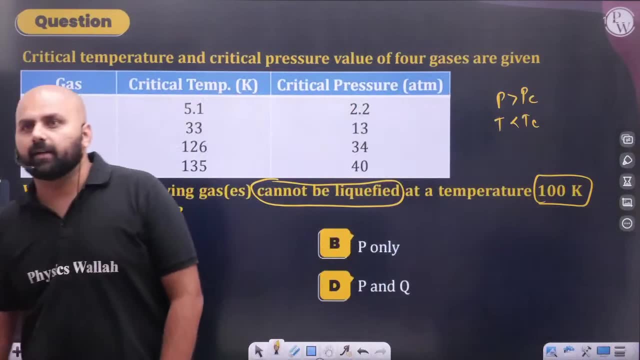 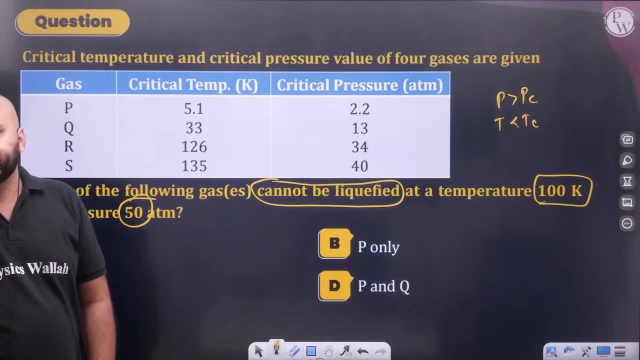 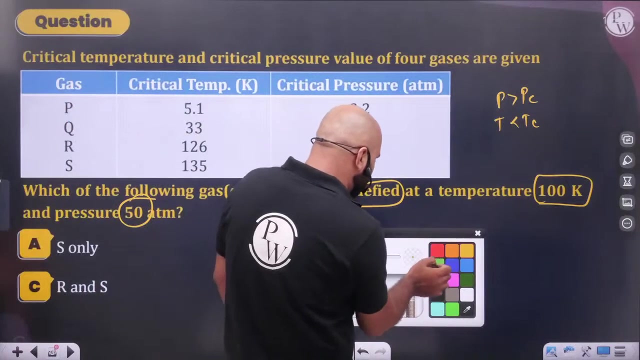 What did I say? Pressure should be greater than critical pressure and temperature should be less than Tc. Look at the pressure. I think the pressure is more for everyone. the pressure is more for everyone. Brother who is reading, reply to the comment section only when you have the option to stop on YouTube. 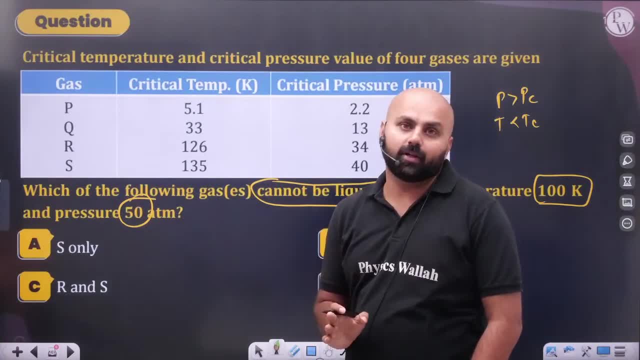 Your time is very important in your life. Don't read about spammers or anything else, Because you know what is going to happen in your life. It's just a matter of 10-15 days. it's a matter of 10-13 days. it's a matter of 13 days. 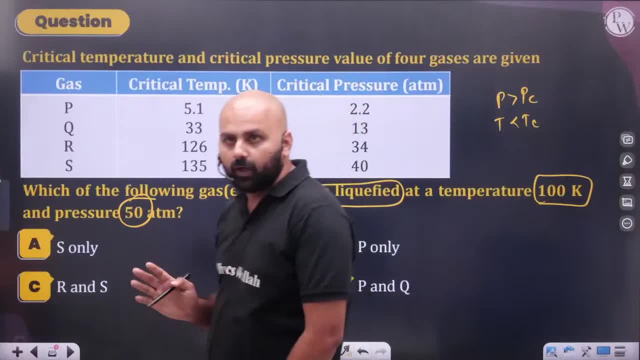 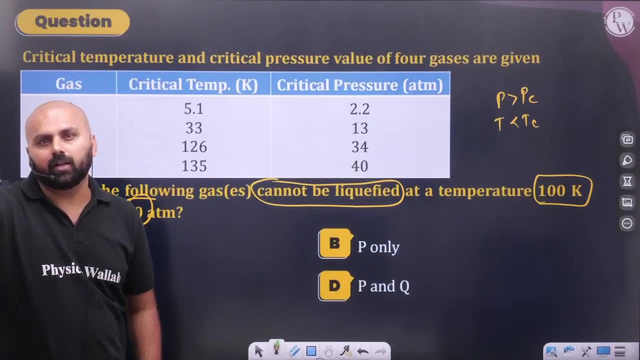 Don't try to explain to them by looking at the spammers. Be on the side quietly, Let them read. let them read. Just try to answer the questions where they have come. Okay, he will give suggestions. he will abuse me, he will abuse you, he will abuse PW, he will abuse everyone. 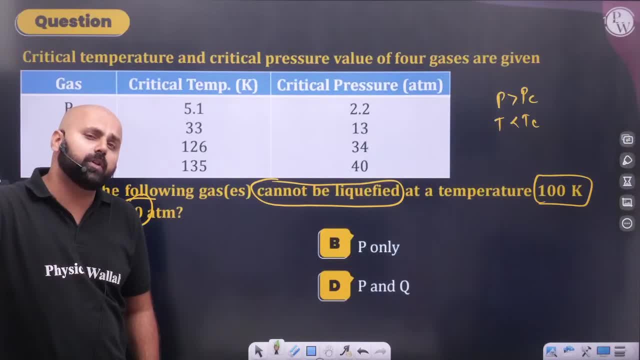 He has come for that. nothing else is left in his life. Think that nothing is left in his life. that's why he is here Now. think about science. if you are preparing for NEET in real, you think that after 7 months he will sit and study physics and chemistry. 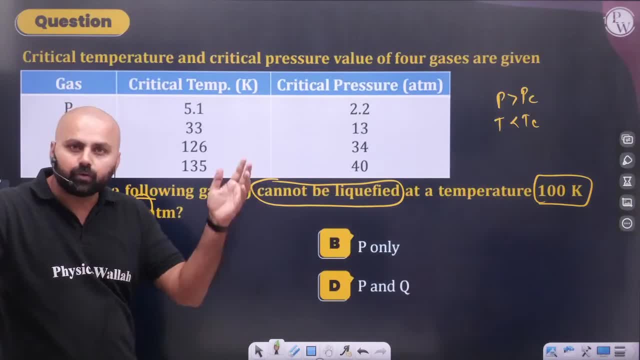 There is so much left in his life. there are so many YouTube videos in his life- on Netflix, on Amazon. he will read all these videos. He will take all the revenge. Think how bad a person he is. He is coming here and spamming you. 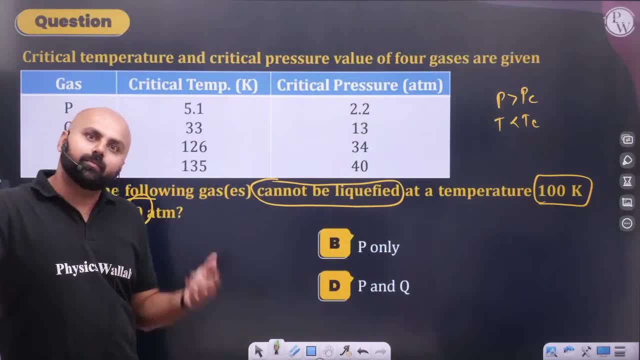 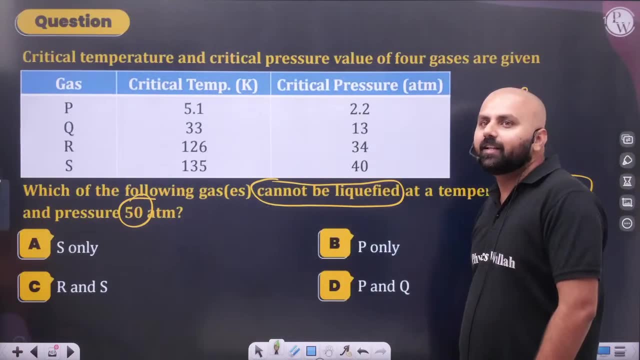 He is coming here and doing this. Okay, He is not recommending any video on YouTube. He is doing this only Go, man. you have so much life, you will get this only, Okay. critical temperature means there is no boiling point. 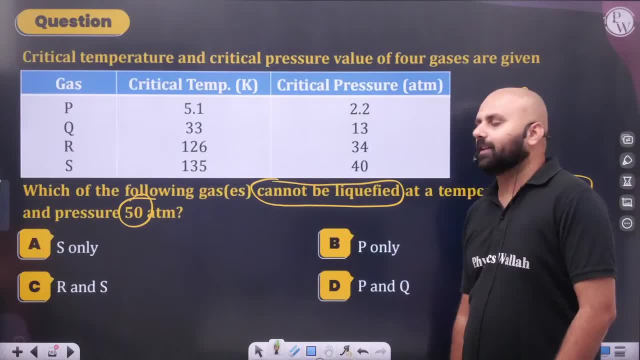 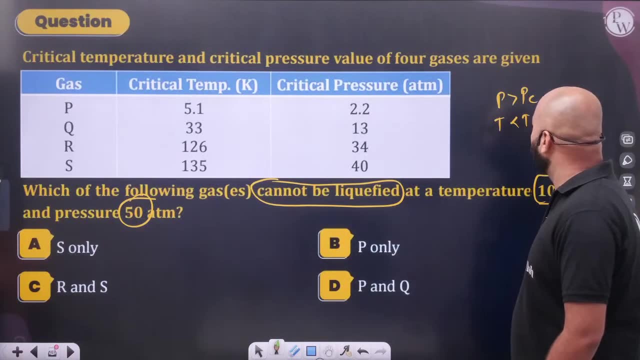 Okay, there is no boiling point. What will happen, Sir? cannot be liquefied. What is the pressure of everyone? Less than PC? What is the pressure of everyone? The pressure of everyone is greater. You have to see the temperature. 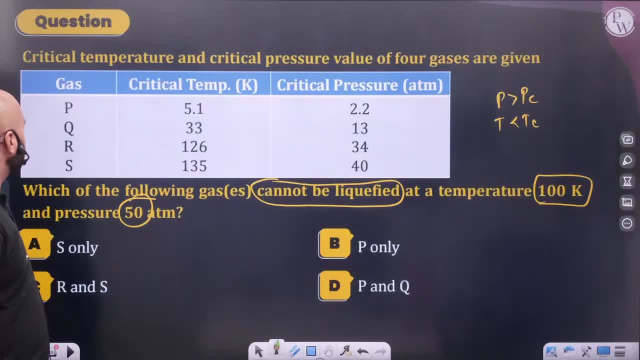 Sir, before 100 degree Celsius. 100 degree Celsius, Sir, 100 degree. look at this: if you go to 100, it will be liquefied. If you go to 100, it will be liquefied. 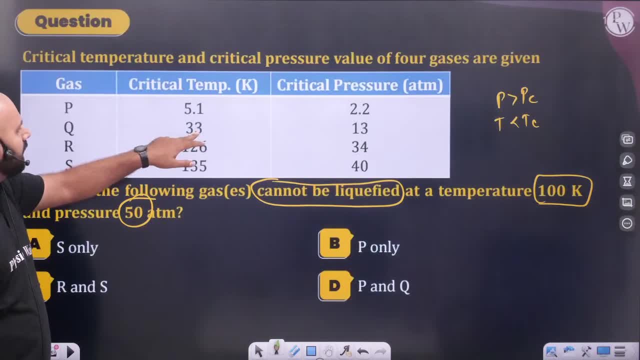 Okay, if you go to 100, it will be liquefied. Okay, and look at this: what will be P and Q with you? They will not be liquefied. What will be P and Q Cannot be liquefied. 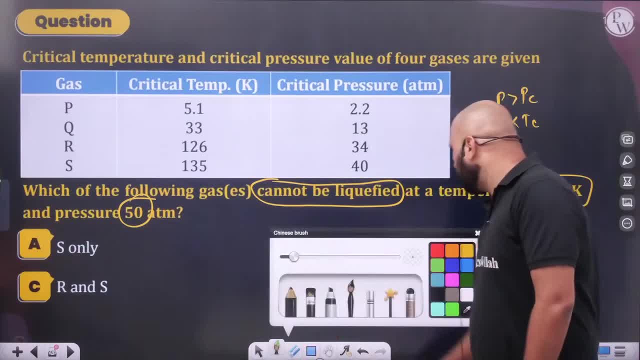 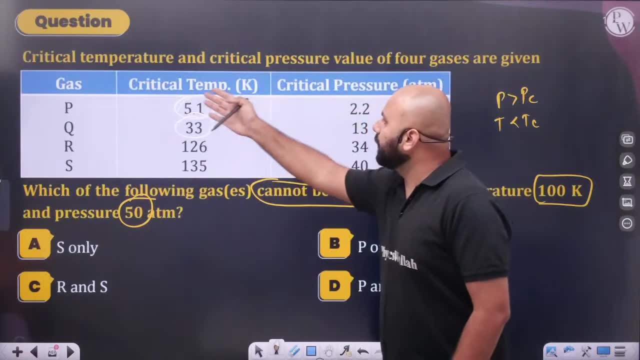 Which will not be liquefied. So the temperature should always be less than critical temperature. Sir, in their case, in the case of P and Q, what is your temperature? It is more than critical temperature. So what will happen to us? 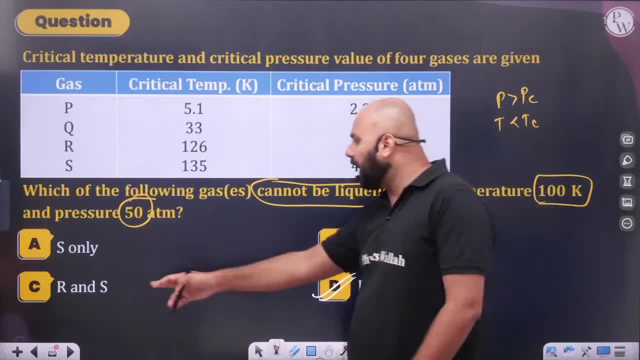 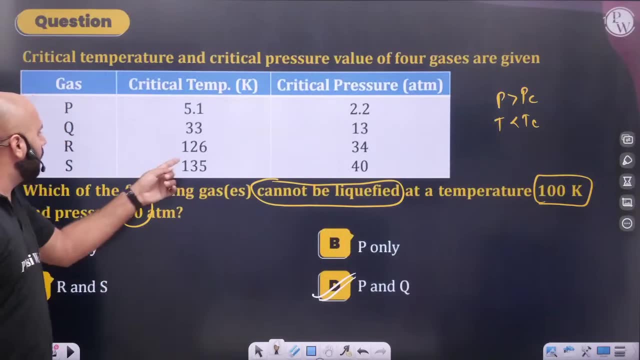 D answer will come. What answer will come? D answer will come. You are misunderstanding Those who are getting R and S. you are thinking the opposite. Critical temperature is 136 Kelvin. How much are you keeping? 100 Kelvin? So if it goes below 135, then it will be converted into liquid. 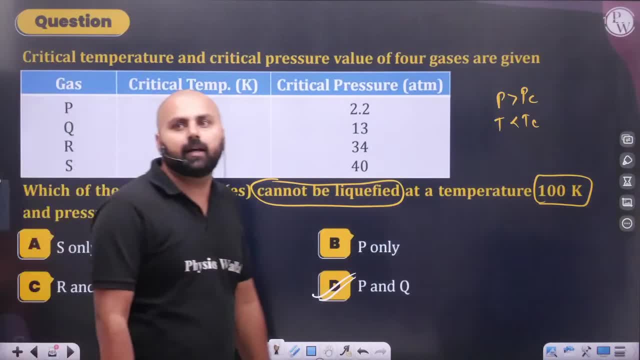 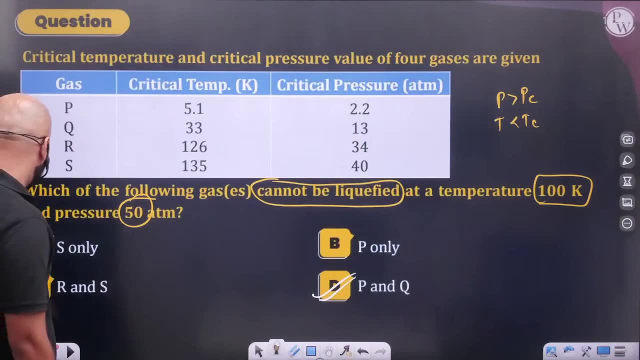 But how will the 33 one be converted into liquid? So listen carefully. Okay, How will the 33 one be converted into liquid? So look at this. Okay, Is it done. Okay, In liquefaction. do one more thing. 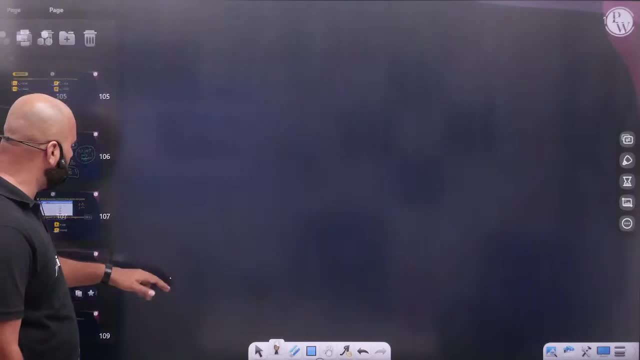 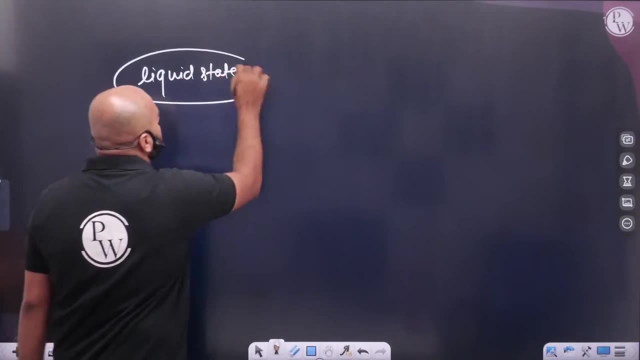 If we talk about liquefaction, then after liquefaction one thing comes. After gaseous state we will talk about a liquid state. So in liquid state major three things come. We read only three things in the liquid state of chemistry. 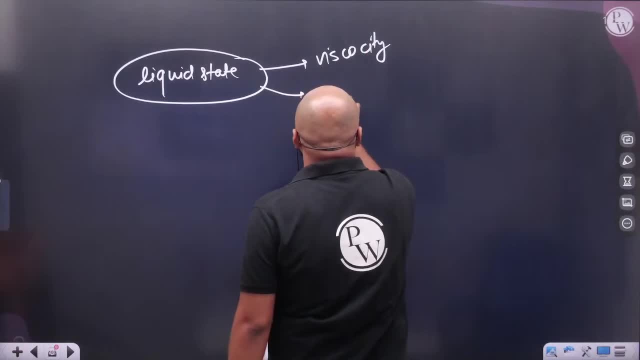 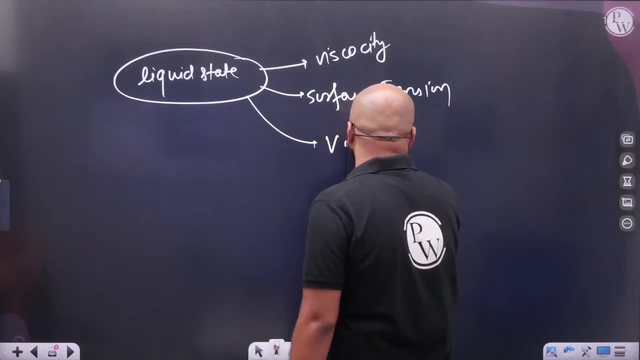 One is viscosity. One is surface tension. Now, in today's time, you have been taught a lot in physics, So you don't need to tell me this, Just remember here. And one is vapor pressure. I want to tell vapor pressure because it will come again in the solution. 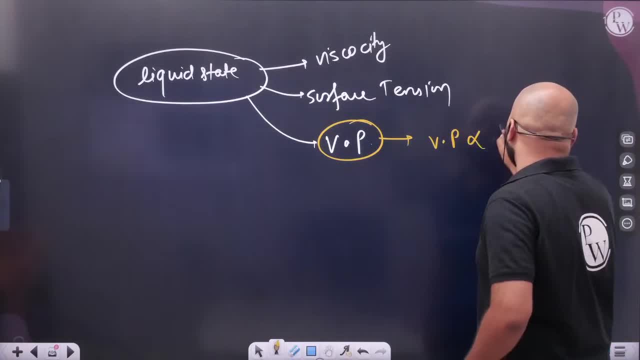 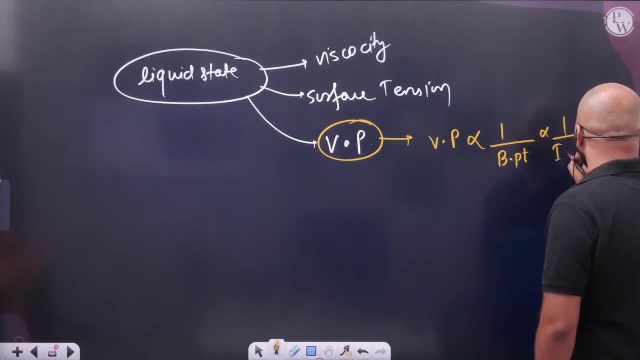 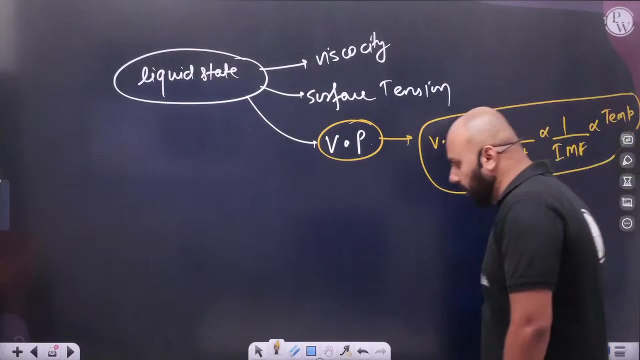 What is vapor pressure? Vapor pressure of any liquid is directly proportional to, inversely proportional to boiling point, inversely proportional to boiling point, inversely proportional to intermolecular force and directly proportional to temperature. Keep this in mind. If you want to remove vapor pressure of any liquid, then, sir, if you have boiling point. 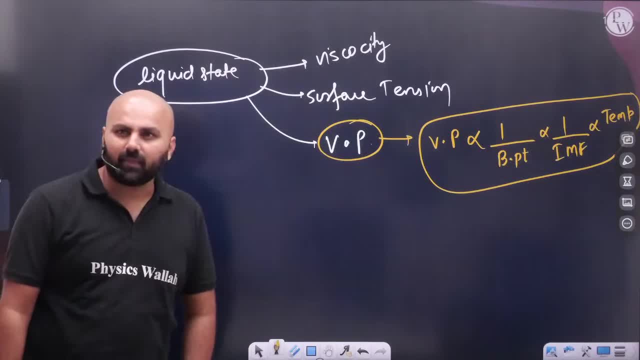 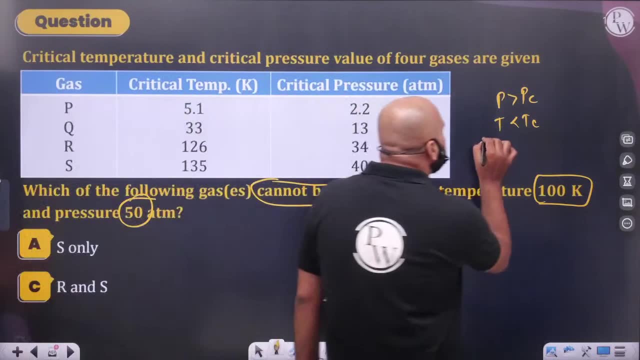 if you have your boiling point. Oh brother, see this. What is the problem? Temperature should be less than Tc. Temperature should be less than Tc. Whose temperature should be less than Tc? Take their critical temperature. how much? 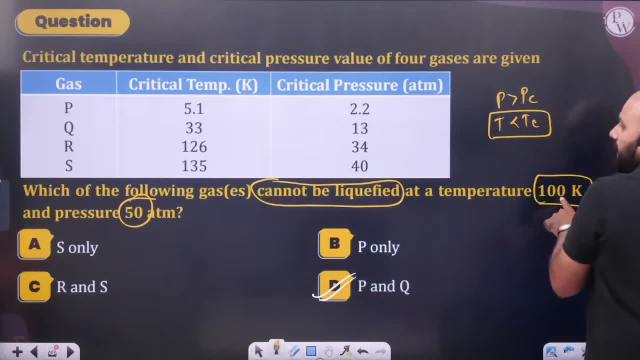 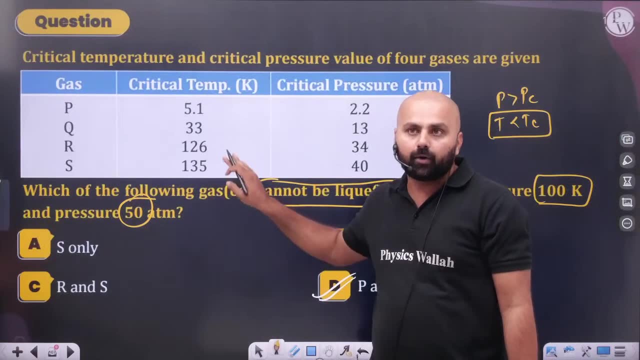 126.. What is your temperature? 100 Kelvin. What is your temperature? Census is less than you. So what will happen to R and S? It will get liquefied. R and S will get liquefied right. What will happen to R and S? 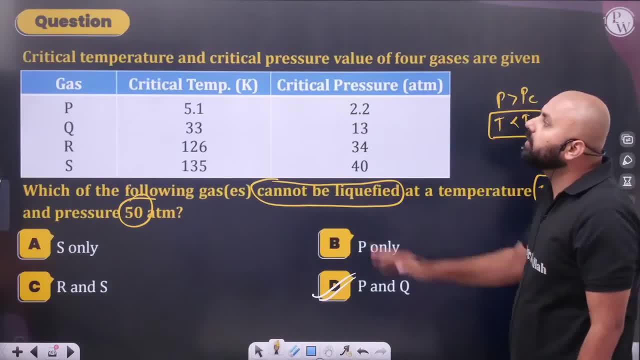 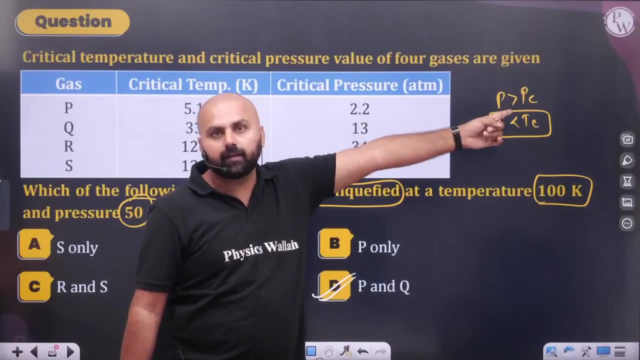 They will get liquefied. Why will r and S not liquefied? What will happen to temperature? What will happen to temperature? It should be less than Tc. See the condition: Everyone's pressure is greater than PCA. coronavirus. shining Peter, destruction your food. 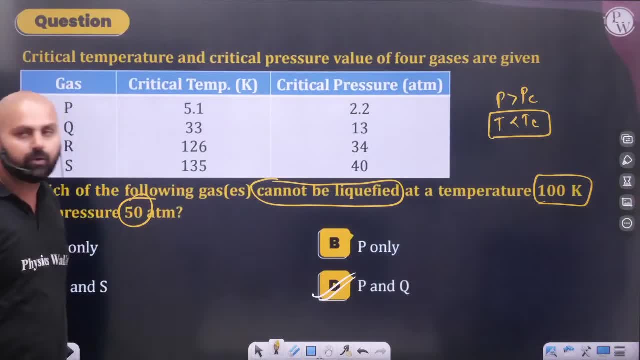 whoever has less than Tc, it will be liquefied. will be 4s liquefied. p and q will not be liquefied. okay, cannot be liquefied what liquefy will not be possible. p and q will not be possible. 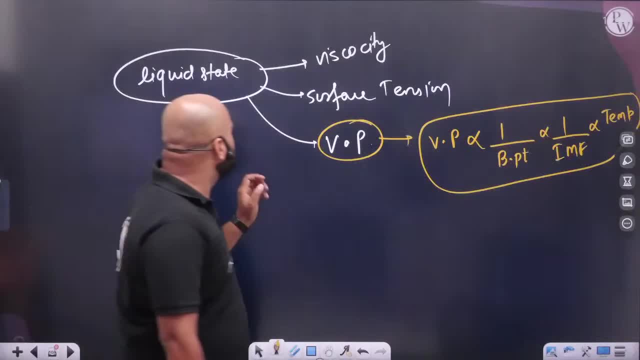 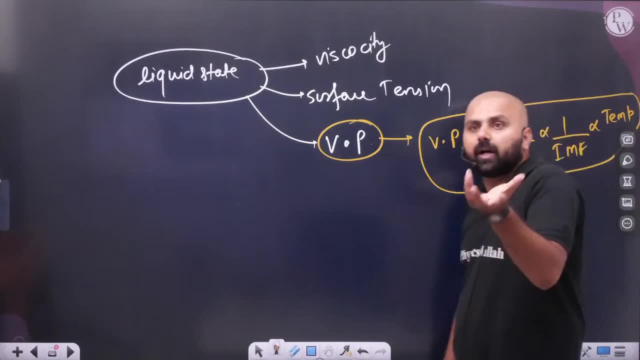 Okay, yes, see, we have. okay, look at this. I am saying: if your boiling point is more, then your vapor pressure will always come down because you will increase the temperature. if you increase the temperature, then the boiling point will become: if you increase the temperature, then what will happen to that boiling point? 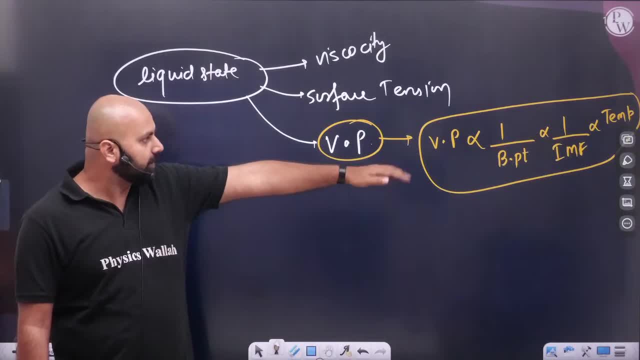 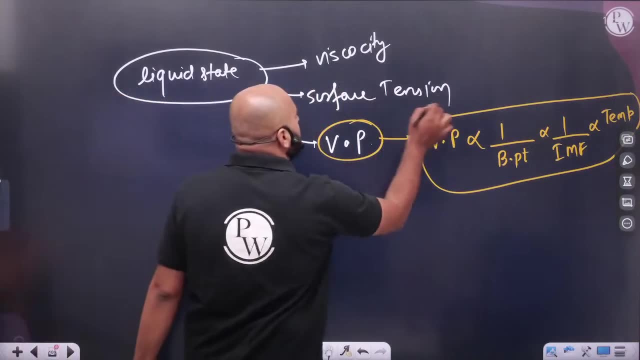 will also decrease. ok, What will happen to the boiling point? We will increase the temperature, or you can say that the boiling point is more and vapors will be less. Second thing: Viscosity or surface tension. Viscosity or surface tension? 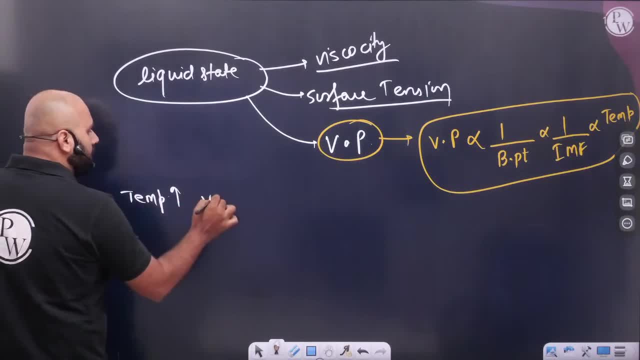 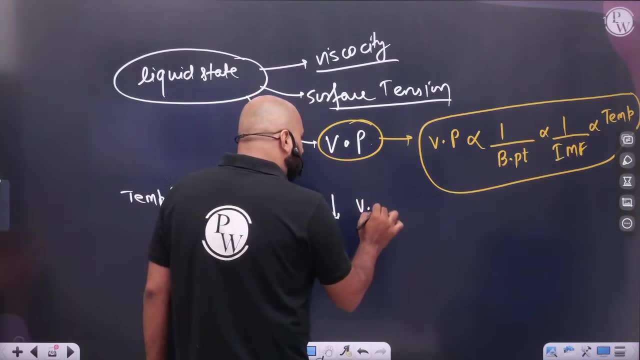 When we increase the temperature, then remember: what is viscosity? It decreases. What is viscosity? It decreases. What is surface tension? It decreases. What happens to the vapour pressure? It increases. So there is a property of liquid which increases itself by increasing the temperature. 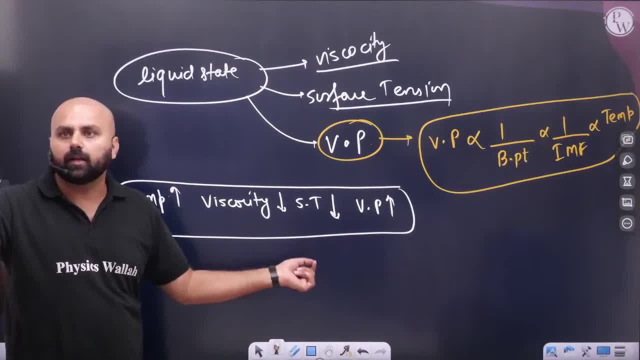 So there is a property of liquid which increases itself by increasing the temperature. Okay, what will it do? by increasing the temperature, It will increase, No other thing. Now, one more thing is defined. on vapour pressure, One more thing is defined. 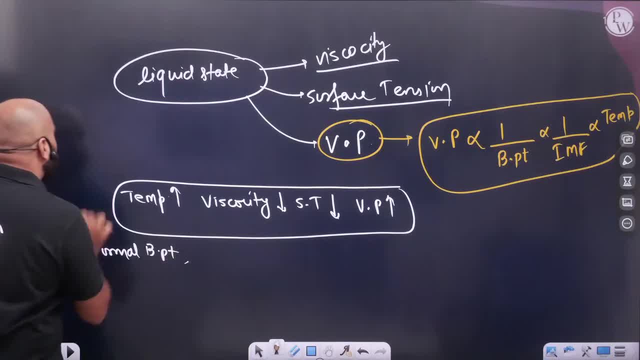 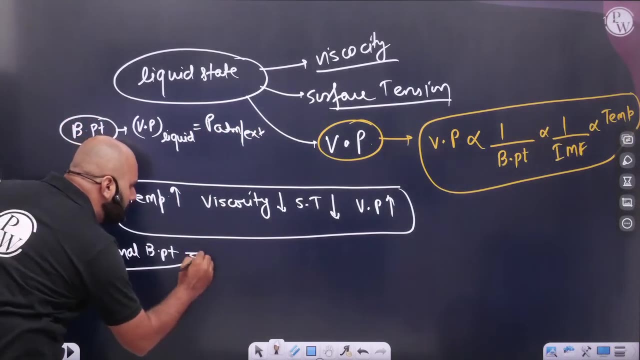 One is a normal boiling point. What is a boiling point? Boiling point is a liquid where vapour pressure of liquid may be equal to atmospheric pressure or to external pressure. Normal boiling point means your vapour pressure of liquid, vapor pressure of liquid will be equal to 1 atm. 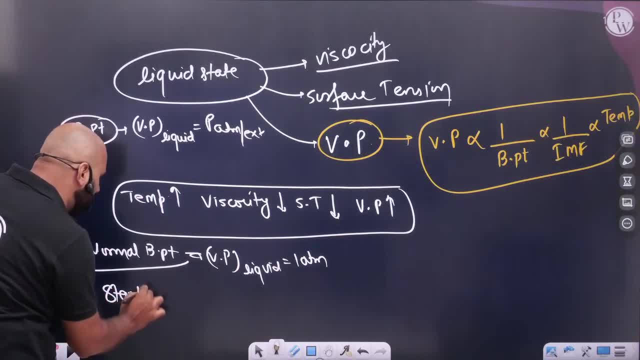 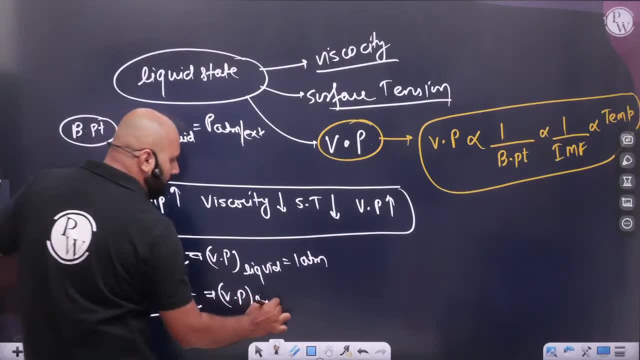 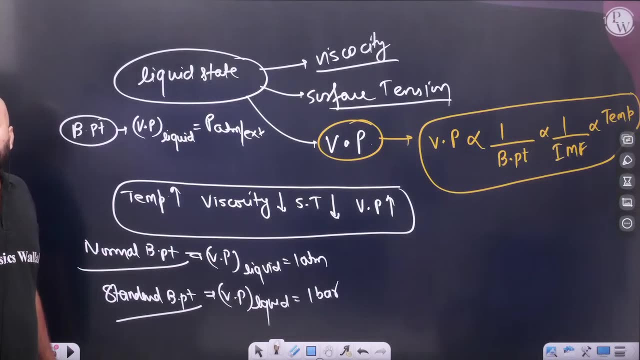 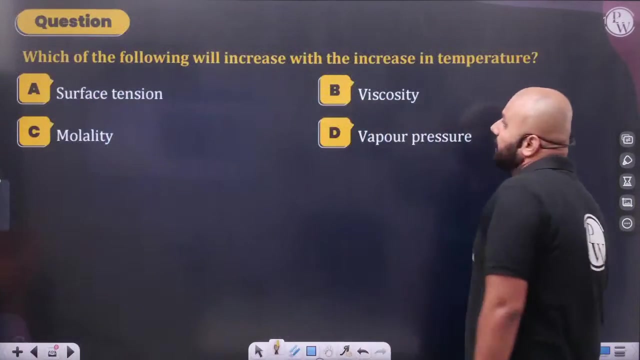 and standard boiling point condition. all this is in ncrt. so when vapor pressure of liquid will be equal to vapor pressure of liquid will be equal to 1 bar. keep on doing. ok, so these are the small things. see here again. question is given. sir, which of the following will: 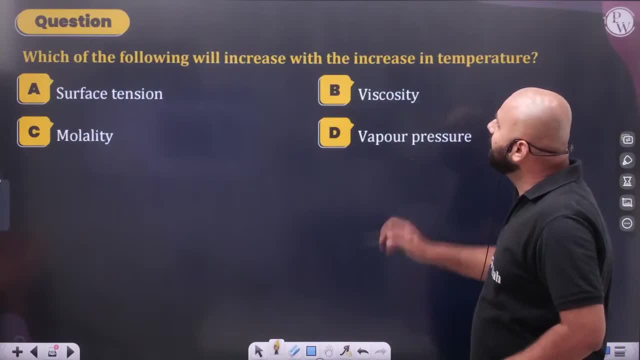 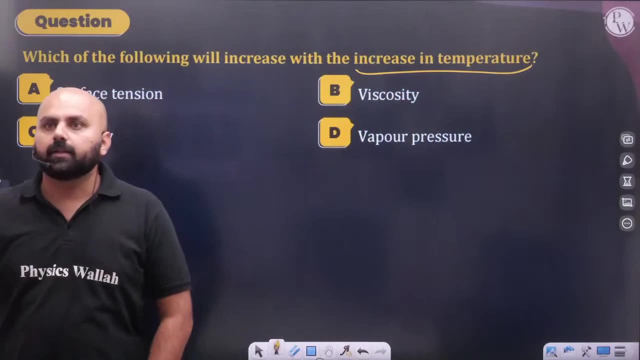 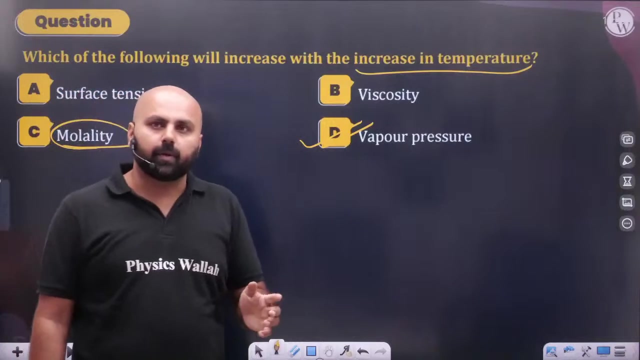 which of the following will with increase in temperature? what will be the answer? quickly, what will happen to us? who increases what increases with temperature? rest, surface tension, molality- molality will not make any difference. viscosity will decrease, surface tension will decrease, vapor pressure will increase. so, if you talk about states of matter, 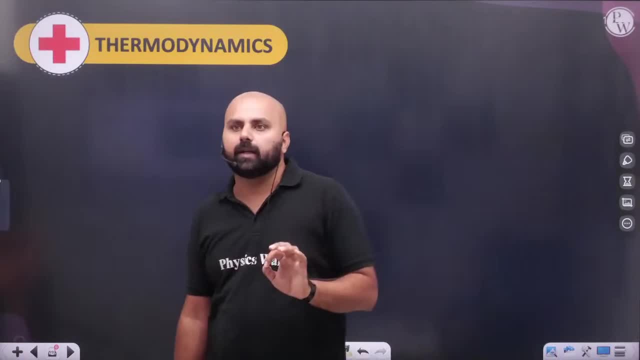 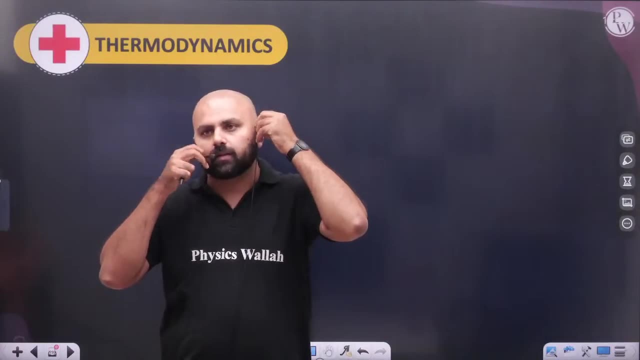 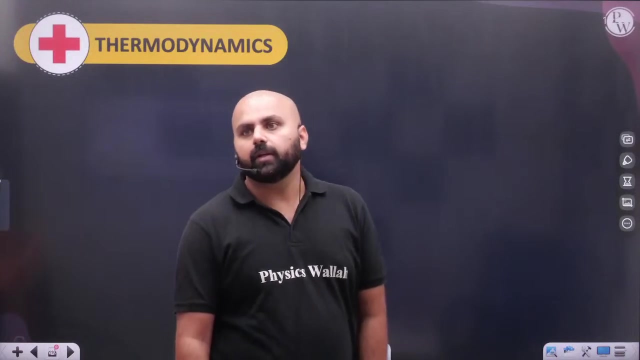 then in states of matter, you will get the same story. 5 gaseous laws are there. there is a story on them. now let's come to thermodynamics. let's talk about it. you will see in thermodynamics. you will see in thermodynamics. you will answer so much. 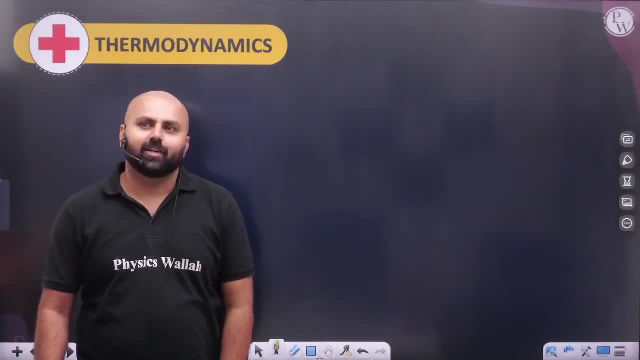 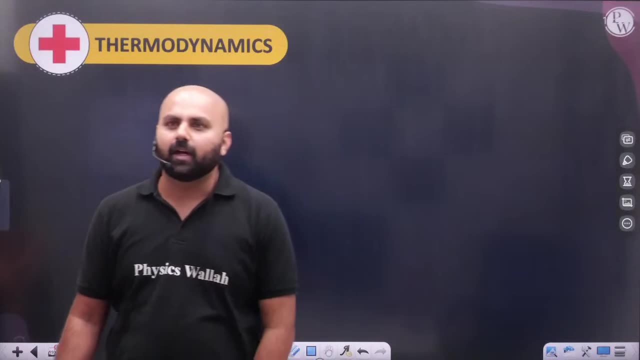 poor one one is Neha Kumari. think she is doing massage by giving punishment. she is doing spam. must be a boy. she is not known and nothing else. we don't need inversion temperature. ok, think how much of a fake person she is. One kid is saying that he is in 7th class. 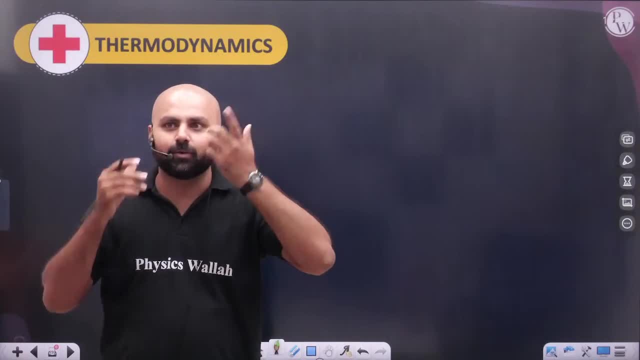 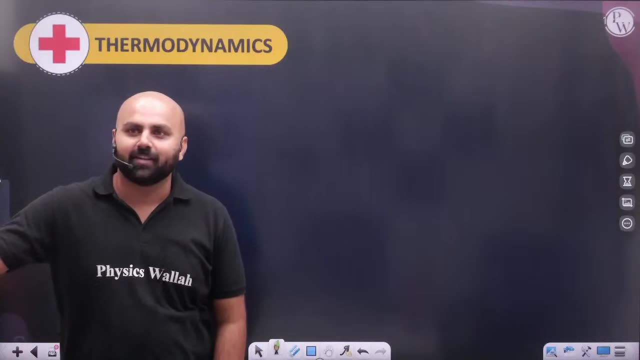 We were in 1st class. you are late. You have done this in 1st class. We are kids of 1st class. you are late, We don't know since when we started preparing. You are watching the video after coming in 7th class. 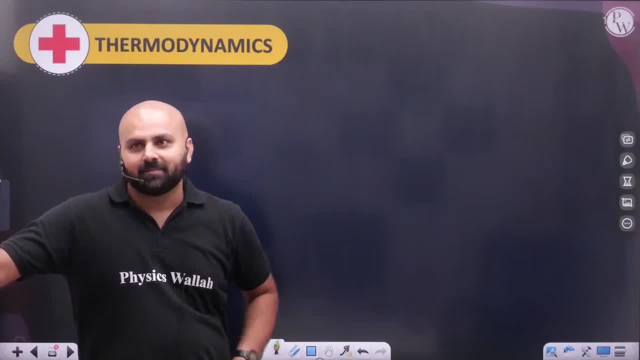 So bad. We are living on a different level. I had no idea. I thought that the kids who come now will come sincerely, Who will come to joke like this. But I don't think so. The boys of Angel Priya exist in real life too. 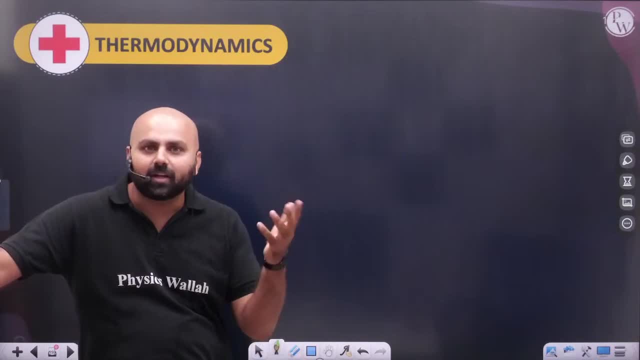 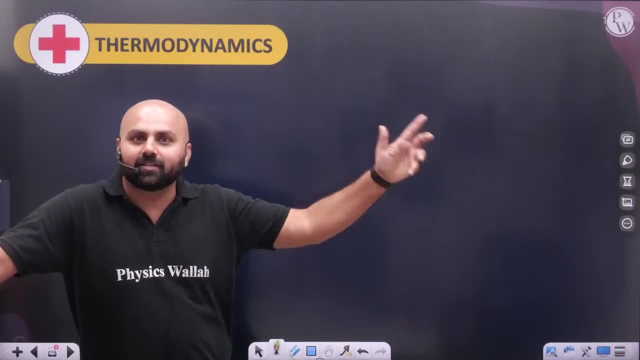 And on the channel of studies. It's okay if a YouTuber is doing it, They are doing it here. They don't know what is fun, They don't know what is going on in life: Liquefication, crystallization, thermodynamics. 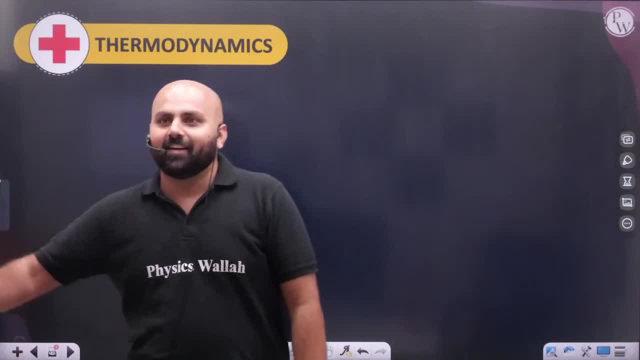 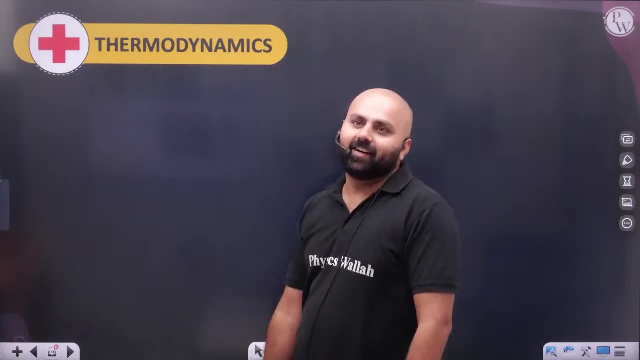 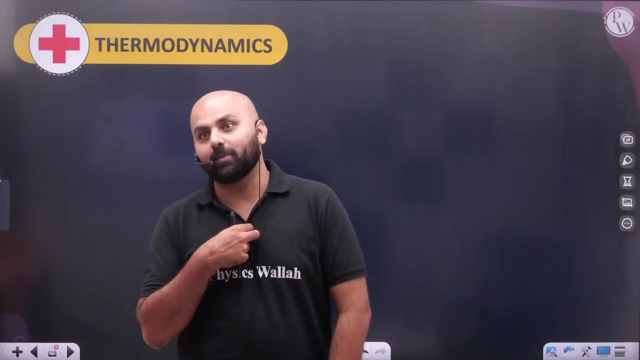 They don't understand what is being studied here. They don't know what is being understood here. There is a crowd here. Let's do it, Let's go. Yes, Let's see, Let's start, Let's give respect. Some people are still here. 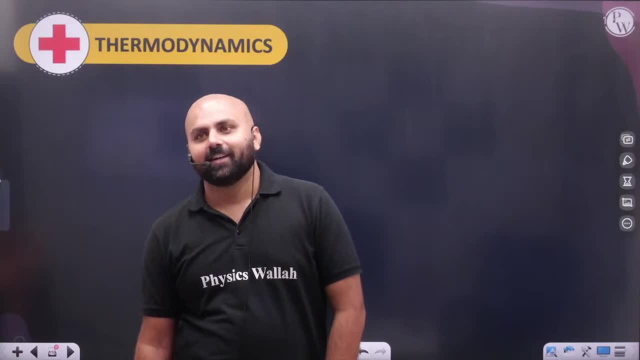 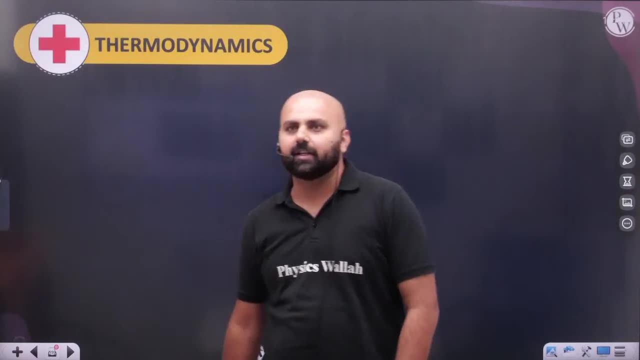 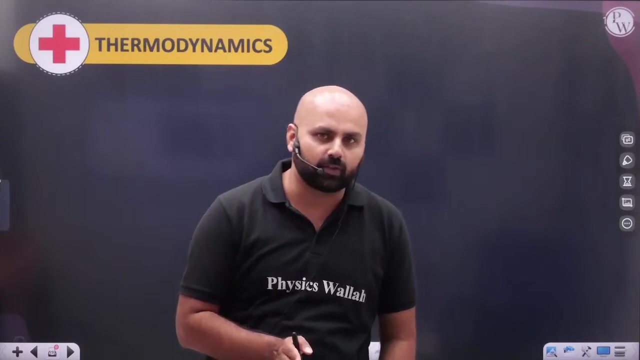 Okay, Let's speed up a little. We will come slowly. Let's talk about thermodynamics. Where does the story start? The story starts with the theory and questions. My theory is that today, the theory is also done. Along with that, the questions are also done. 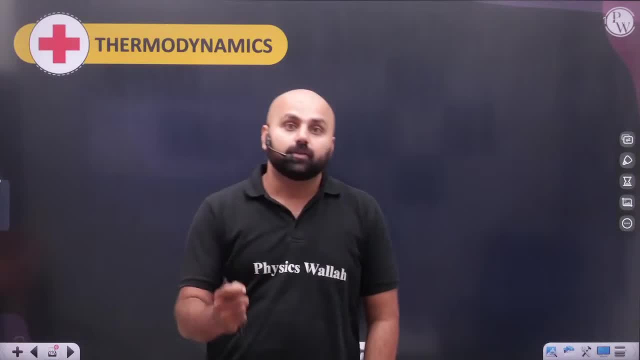 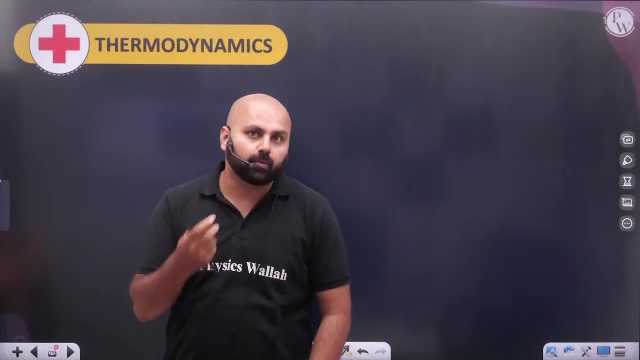 Now, if you are doing theory, Then obviously the questions will have to be compromised. Who wants to do more questions? I am telling you, I have done all the part of doing questions. I have done it in the Maharevision. You think you can do it from there. 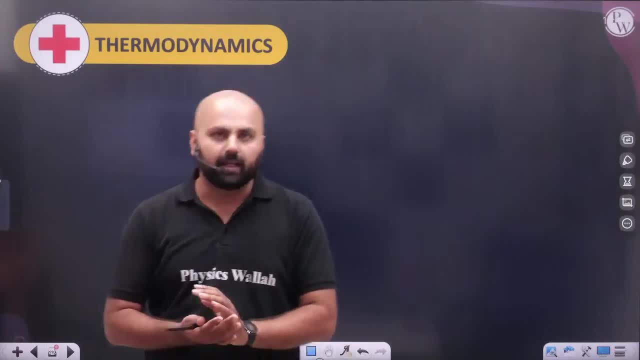 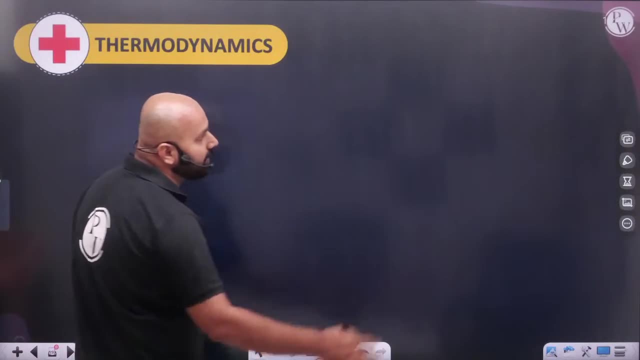 You think you have to do it in hope. But if you want to do everything together, Then let's manage it a little. Let's relate both things together. So don't just do questions. If you know, Thermodynamics runs for 20-25 hours in the class. 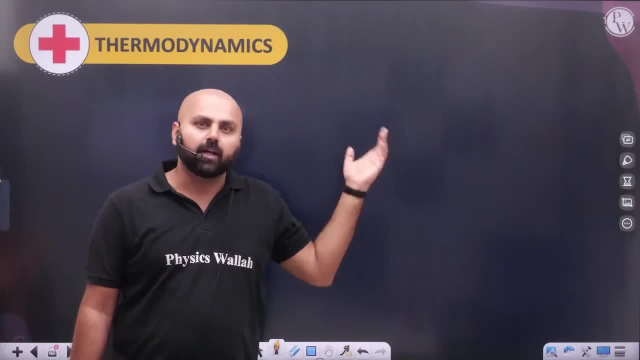 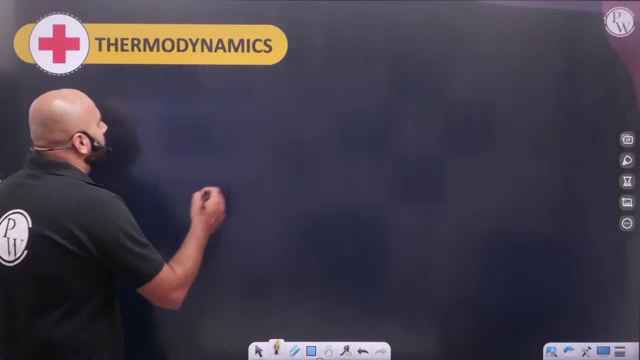 Then obviously it will not be possible In one thing Here. you have to finish it in 1-1.5 hours, So the questions are also not much. Just revise the theory. We started with the most basic thing in thermodynamics. 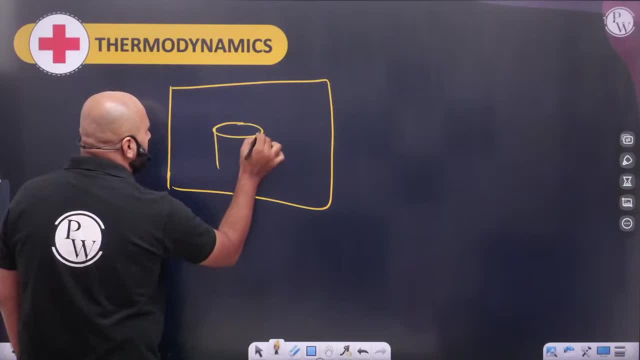 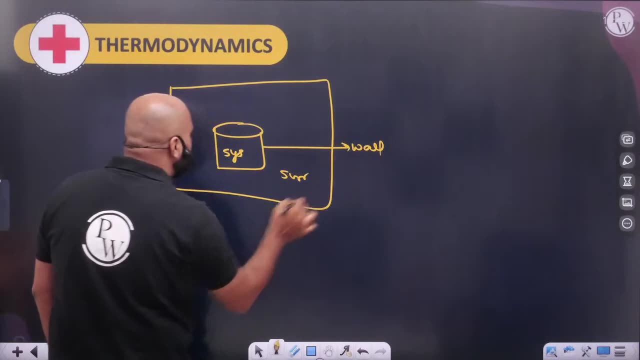 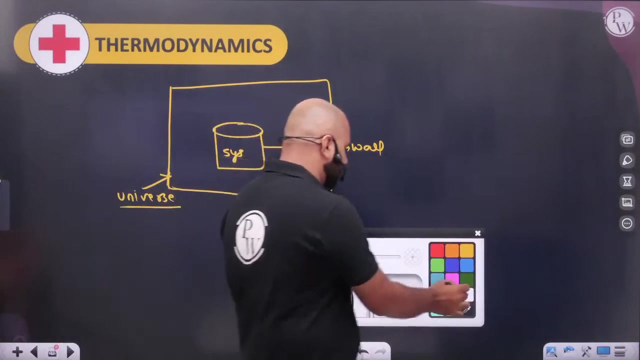 And that is, Let's read, the most basic thing. This is the system, This is the surrounding. Who is there to separate them? It is the wall. What do we call this whole thing? We call it the universe. What do we call this whole thing? 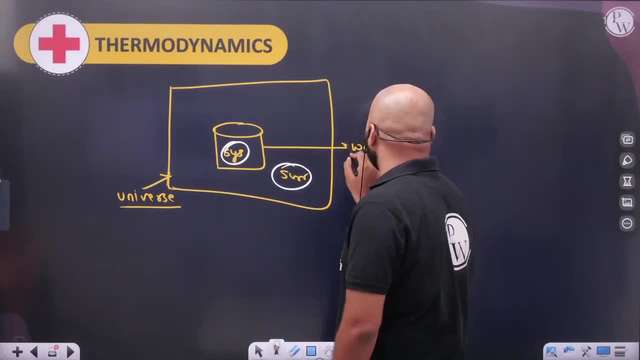 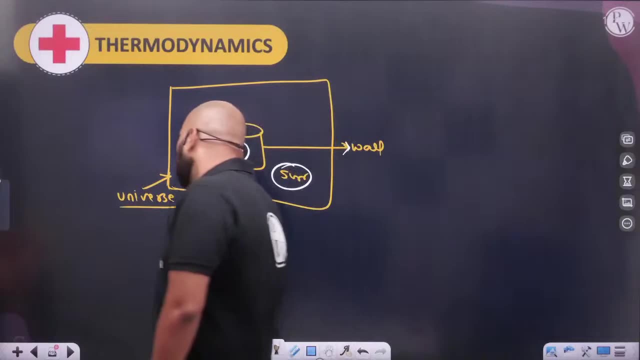 We call it the universe. So there is a system, There is a surrounding, There is a wall to separate it. Who is there on the side? It is the universe. There are 3-4 things. We have two types of walls. 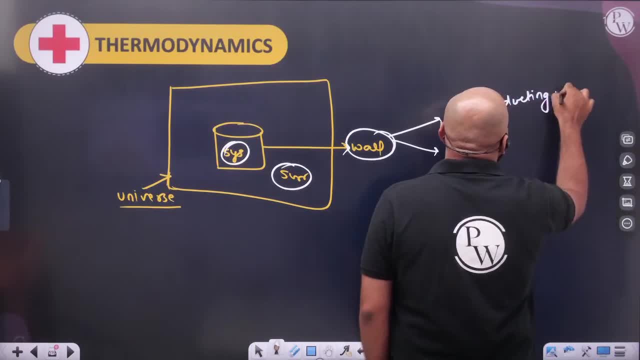 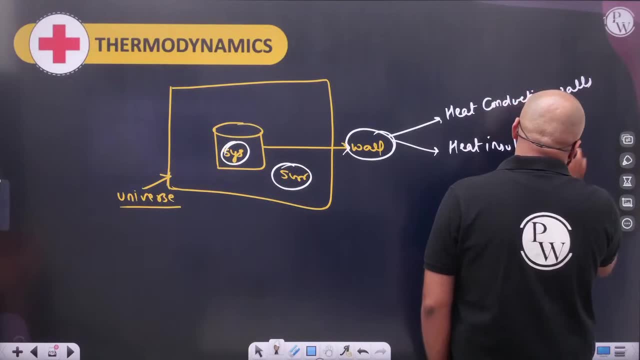 One is heat conducting wall, Which conducts the heat, And one is heat insulating wall. One is heat insulating wall, Or what do we call this? Insulating walls? What do we call heat insulating walls, Adiabatic walls? 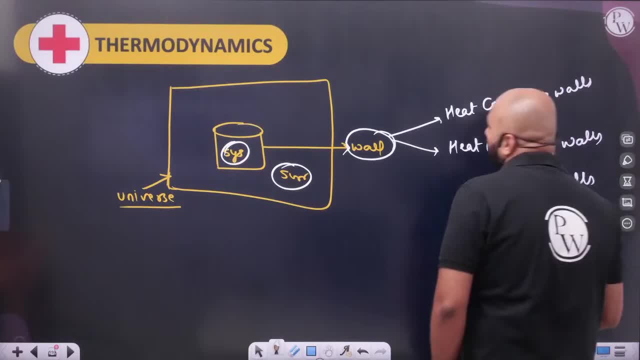 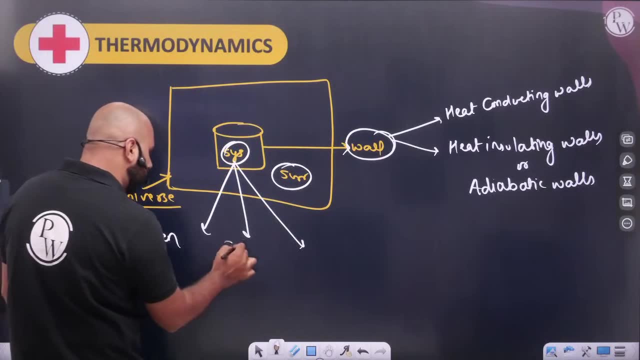 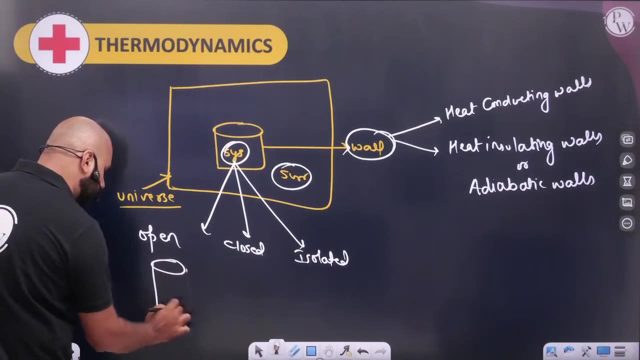 Heat insulating walls, Or we call it adiabatic walls, Heat conducting. We have 3 types of systems: One is open system, One is closed And one is isolated. What does open mean? Open means Energy, Exchange of energy or heat. 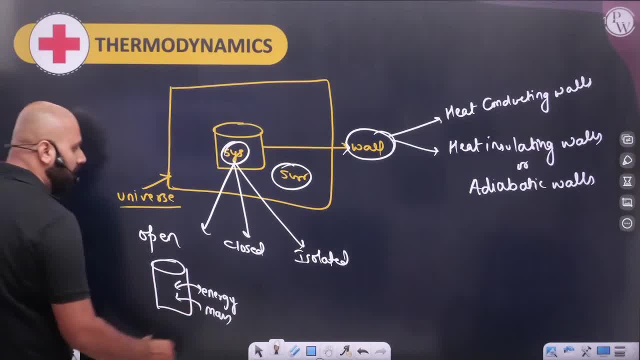 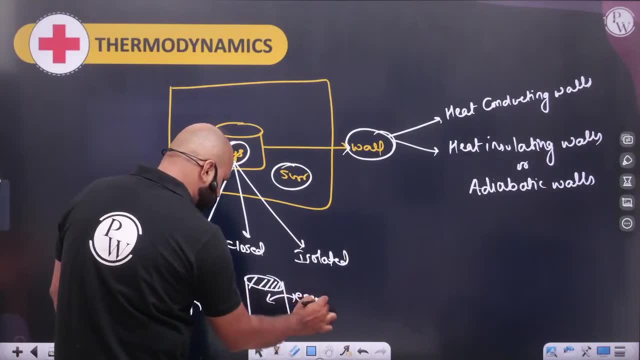 And what is the exchange of mass, Both inside and outside? What does close mean? Close from above? What does closed mean? Energy will be exchanged, But what will be the exchange of mass? It will stop Here. energy is also being exchanged. 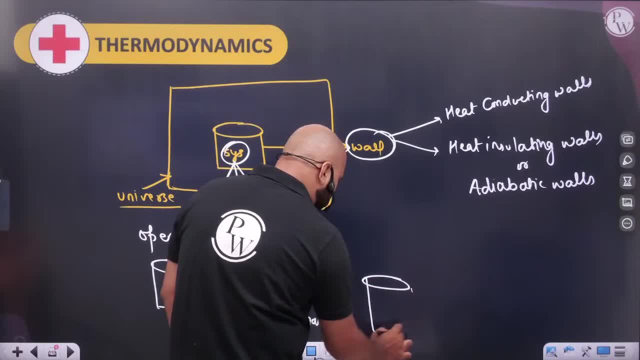 Here, energy will be exchanged, But mass will not be exchanged. Isolated means living at a different level. Isolated means this is going on in their life. They will be running like this. They will be talking in isolated, Closed from above. 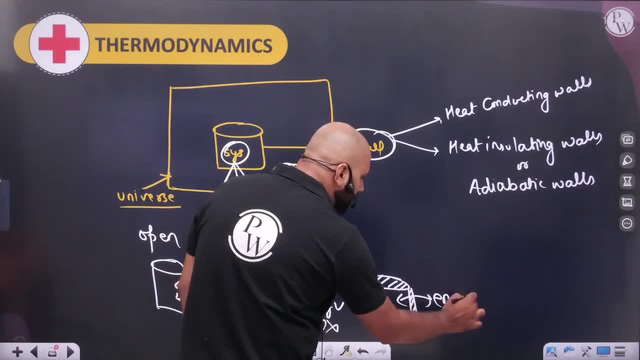 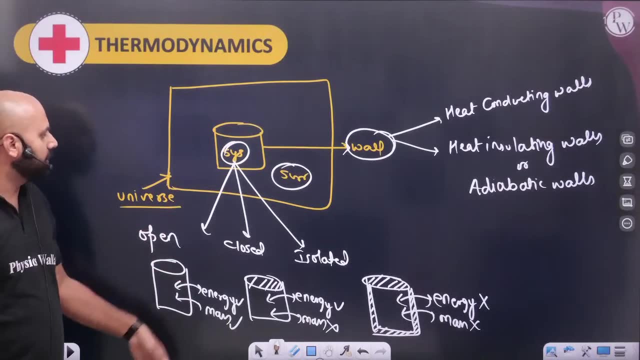 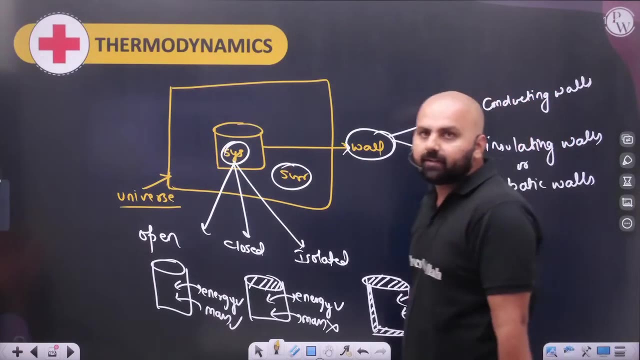 No energy outside, No mass outside, No energy outside, No mass outside. No energy outside, No mass outside. So they have a system Surrounding What is surrounding. If the system loses, the surrounding will be affected. If the surrounding gives, the system will gain. 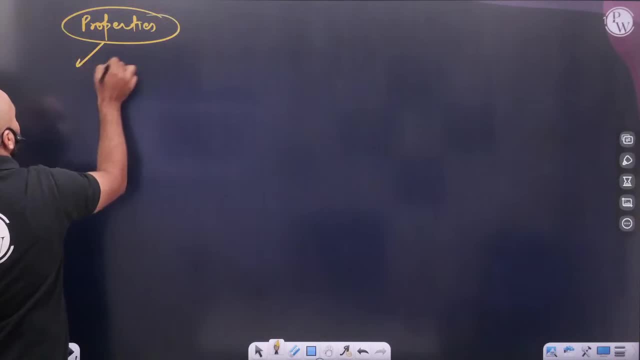 I have two things here. I have properties here. Intensive means: Look here. These chapters are small. These are formula based questions. Intensive means independent of mass. Intensive means independent of mass. Independent of mass. Extensive means depends on mass. 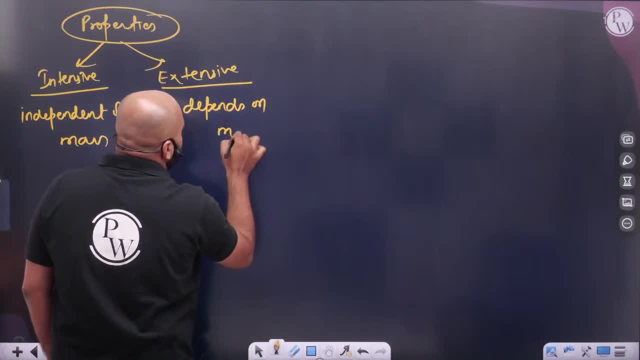 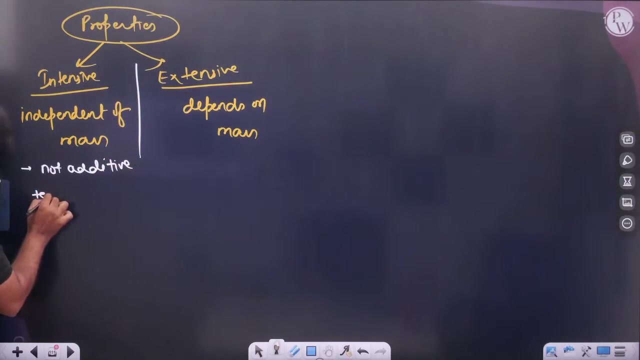 Depends on mass, Depends on mass. So this is intensive and this is extensive, Intensive and extensive. Intensity and intensive: these are independent of mass. These are not additive. You can't add them directly. Like temperature, you can't add them directly. 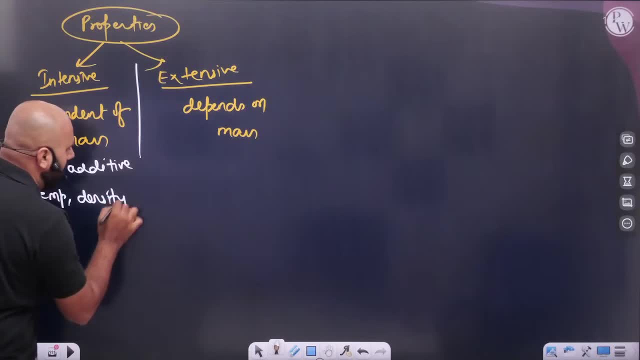 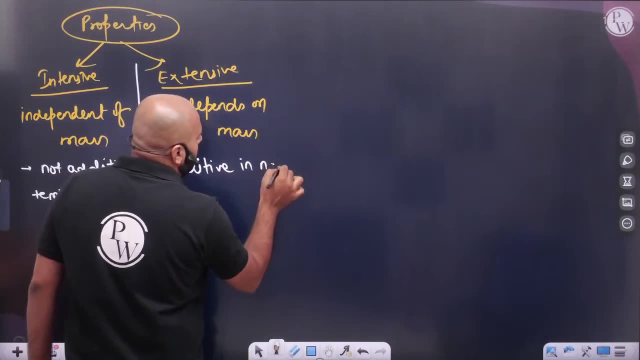 Density- you can't add them directly. Density- you can't add them directly. Extensive is additive. You can add them. Additive in nature If you want to add them, add them Energy enthalpy. all these are extensive properties. 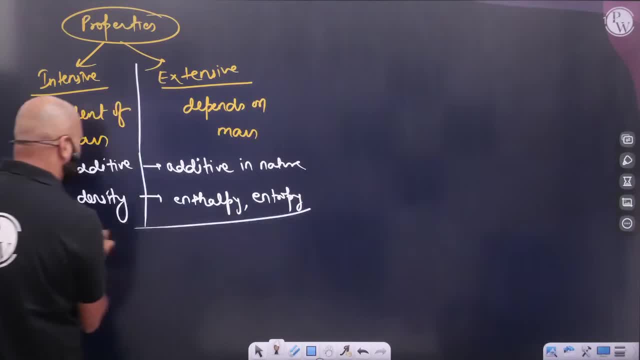 Enthalpy, entropy, all these can be added. If an extensive is converted into an intensive, then extensive upon extensive, then also it is converted into intensive. Extensive upon extensive, then also it is converted into intensive. Or if an extensive 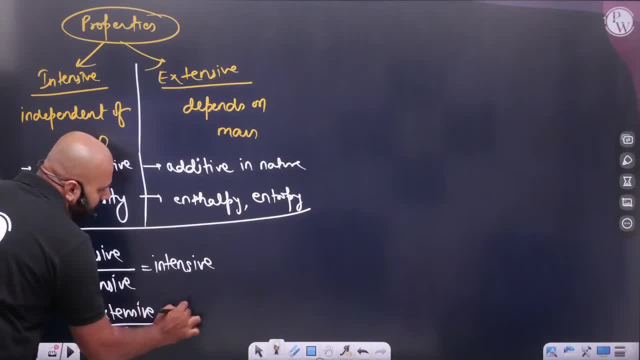 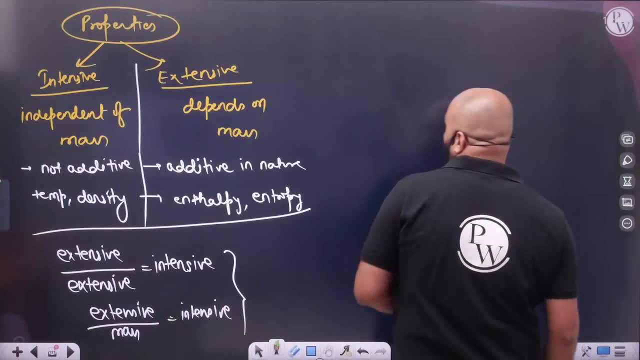 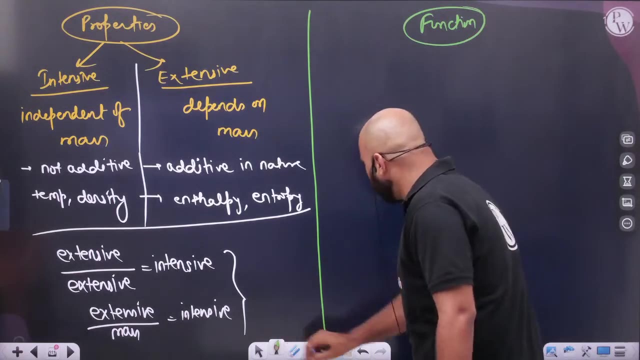 property is divided by mass, then also it is converted into intensive. So remember these basic things. If intensive is intensive, then also you have intensive. Similarly, now we will talk about function. If I talk about function or process, then you will see here. 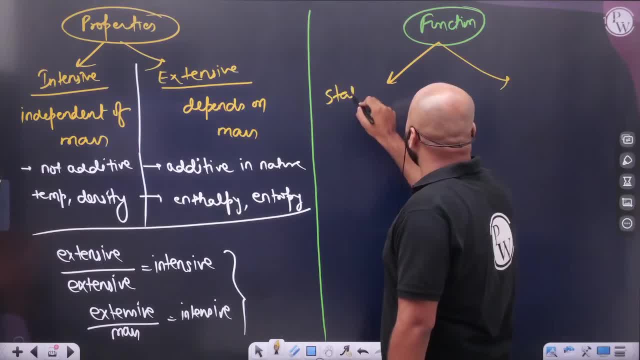 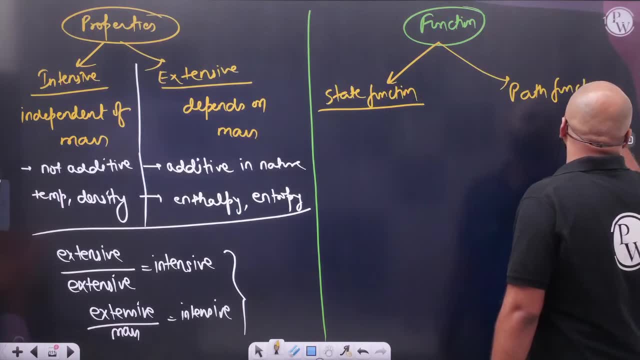 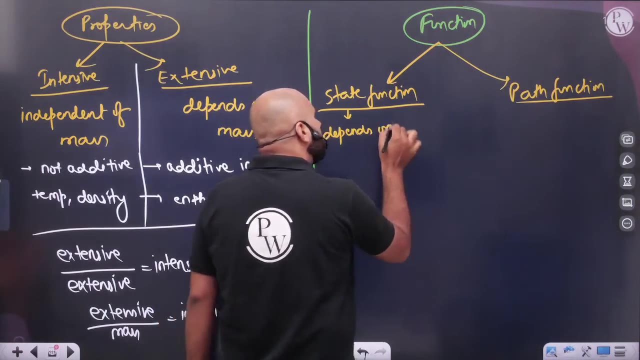 there should be two types of people, there should be two types of function, Which is: One is a state function and the other is a path function. The difference between state function and path function- On what does the state function depend- depends only on. 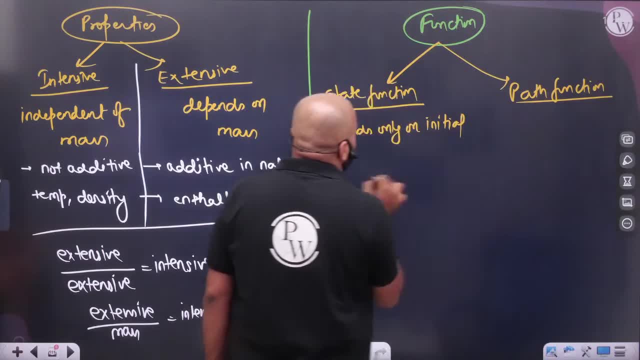 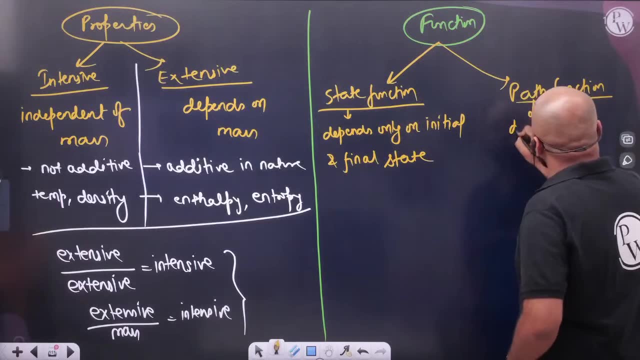 initially and finally. position Only on which it will depend: Initial and final position. Only. on what will it depend? Initial and final state, Sir, it will depend on the path. depends on the path, Sir. remember that we have to study only two path functions: heat and work. 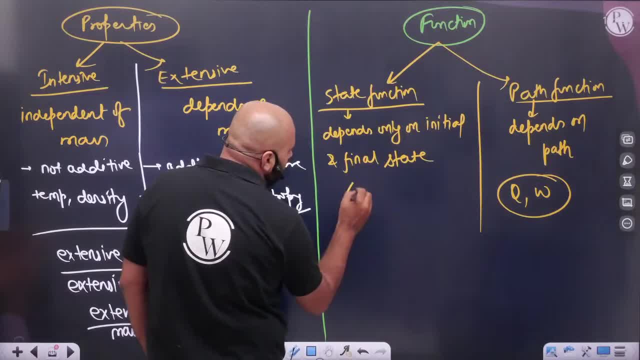 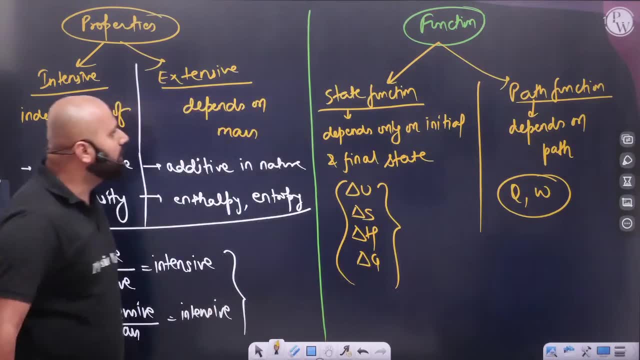 Only two path functions are in our syllabus Rest. all of them internal energy, entropy, enthalpy, Gibbs energy. all of them are state functions that we have to study. Any state function means that we have to study only in the initial and final position. 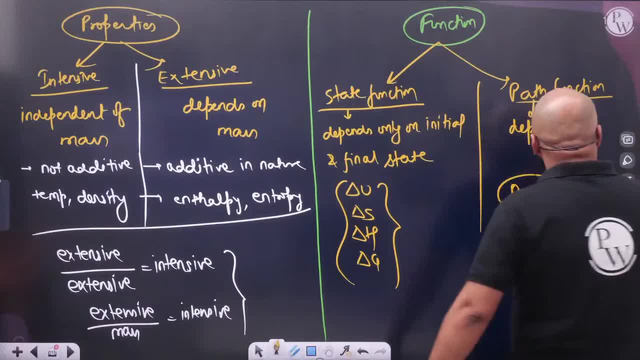 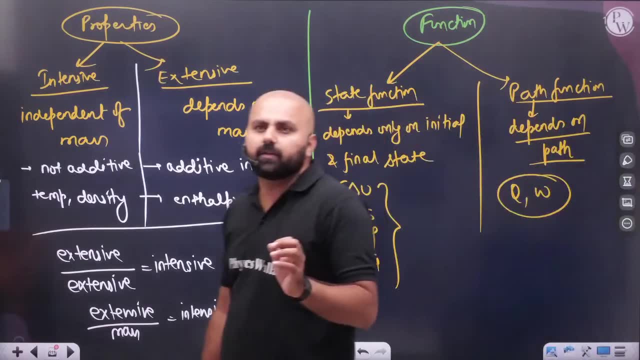 Sir, we have to study in the initial and final position. Okay, See, this path function depends on path. Simple Heat and work depend on the path. So these are the basic things. Now, here you will see. first of all, let's revise the formulas of path function. 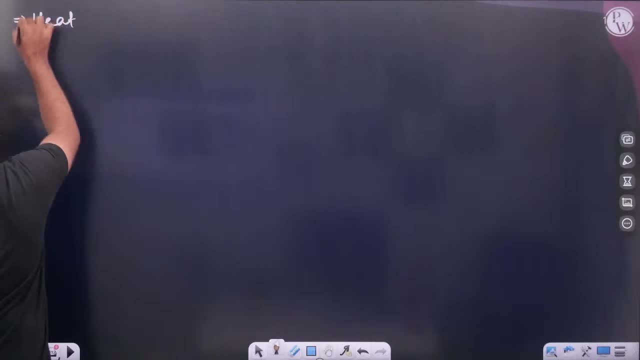 First of all, let's talk about heat. So heat comes in our life of two types: Heat in our life- we represent heat with Q- And heat comes in our life of two types. One is sensible heat, One is sensible heat. 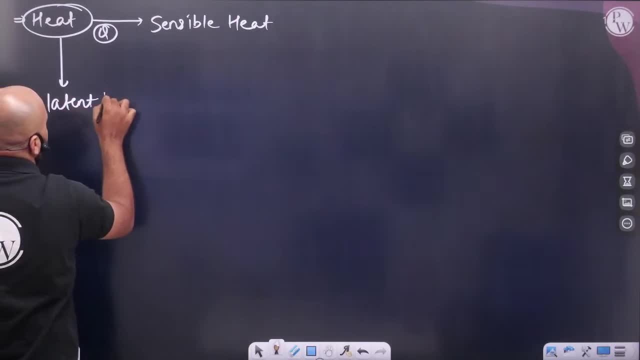 And one is latent heat, Latent heat. If I talk about latent heat, then there are two or three ways to calculate latent heat. There are two or three ways, Sir, here. if latent heat, if its unit is given per gram, per moles, then what will you do here? 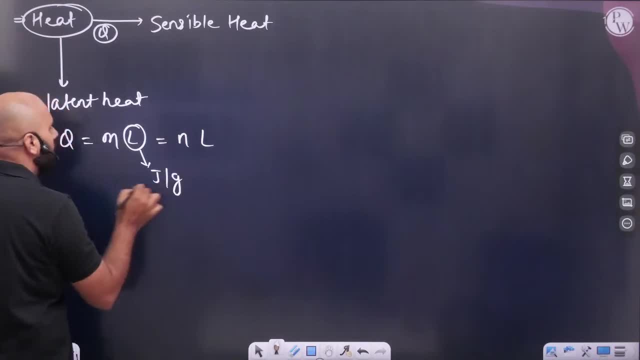 Sir per moles. If gram is given per joules, then what will you take mass in gram? If here, sir, joules per mole is given, then look at the formula. Put unit dimension here, take mole. There is no new formula. 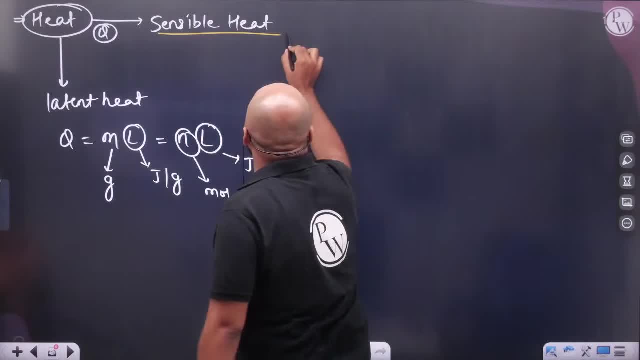 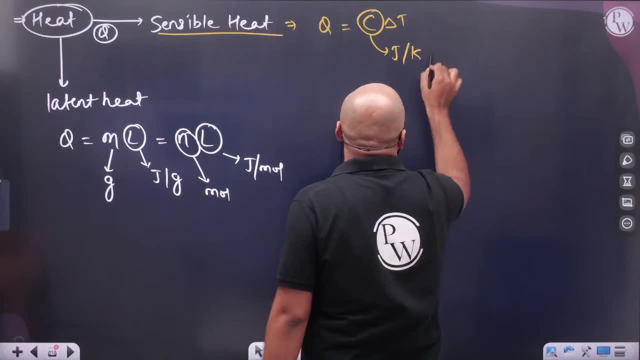 Same formula. What happens in sensible heat is that here three formulas come: Sir, C, delta T, where C is, Look at its unit, Joules per Kelvin, will be written. Or we call C as heat capacity, What we call C as, 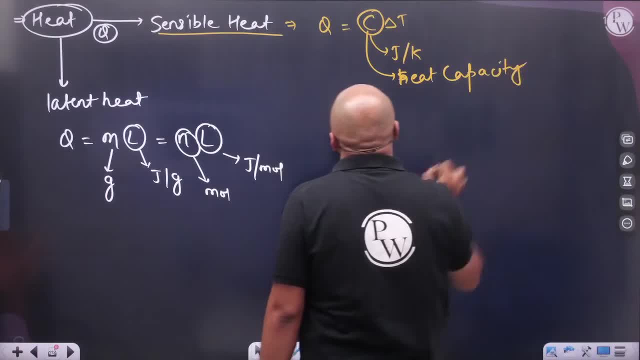 Heat capacity. Brother, don't mess up the formula. You have already done it in physics: Q is equal to M. small c delta T. What happens to small c? Specific heat capacity. Put unit dimension, your answer will start coming. Small heat capacity. specific heat capacity. 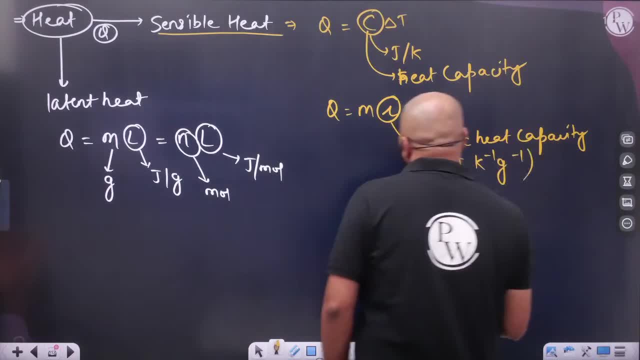 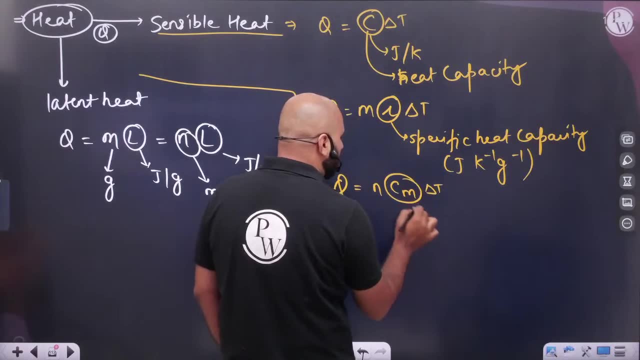 What will be the unit? Joules per Kelvin, per gram. And if you take out sensible heat, then one more formula comes: N, C, M, delta, T. Sir, what is this Molar heat capacity? What is this Molar heat capacity? 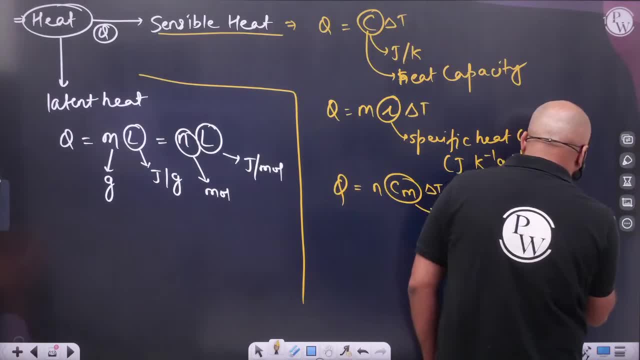 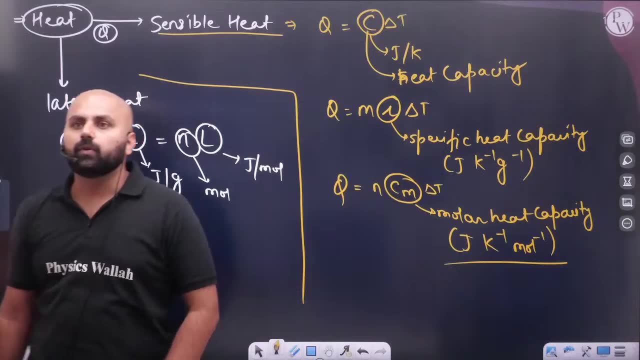 Look at the formula, Put the answer according to yourself. Small, Your Sir, you can get the answer by looking at the unit Joules per Kelvin per mole. So this answer will start coming. So Q is equal to nothing. 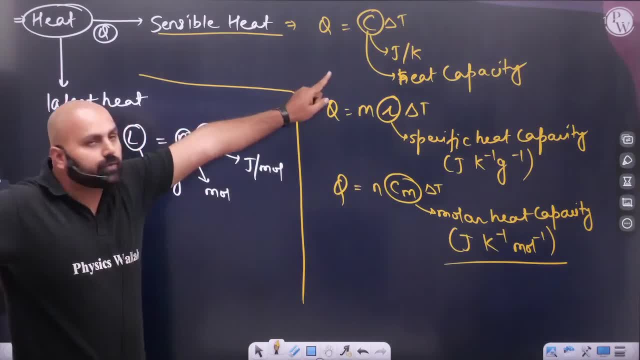 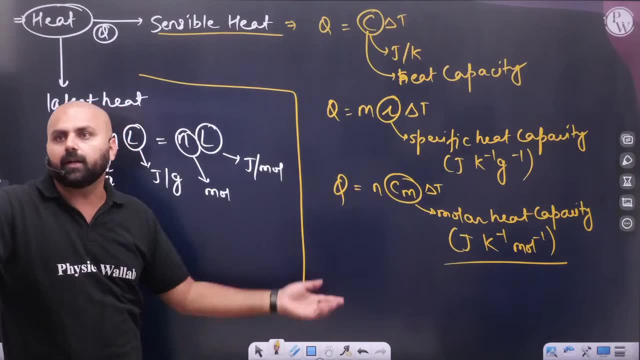 Okay, Look at this: Q is equal to C delta T, Q is equal to C delta T. Okay, We have: Q is equal to M C delta T. Q is equal to N C M delta T. We are doing it like this: 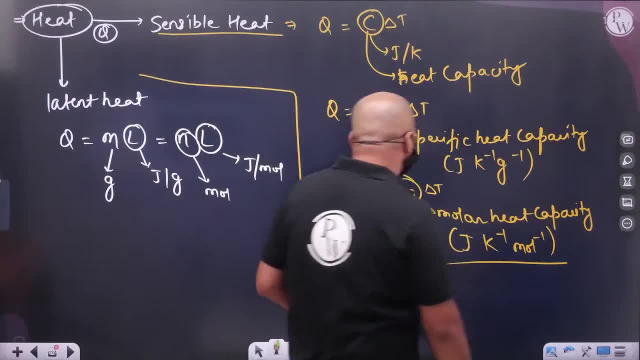 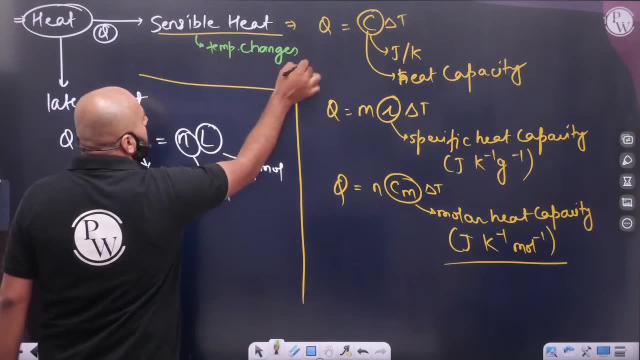 Okay, We have the state function. These are all the path functions. According to them, For whom sensible heat is used When temperature is to be changed, This changes the temperature here. That is why temperature is changing: C, delta, T. What happens here? 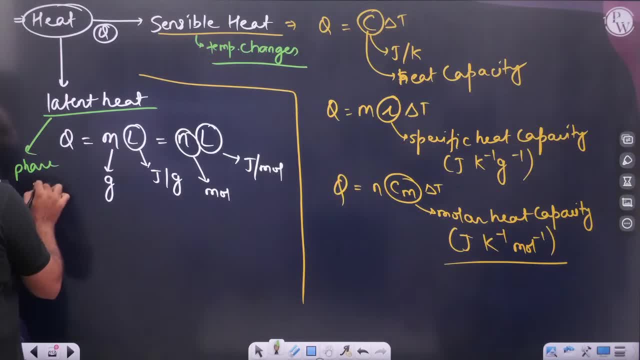 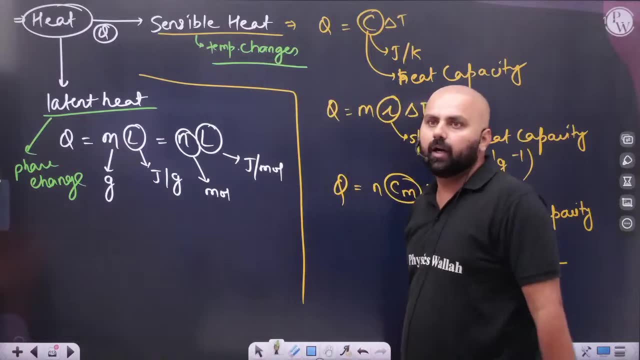 What happens to latent heat? Phase changes, Phase is changing, So what will latent heat do? Phase is changing, So sensible heat will change temperature. Latent heat will change this After that, if someone tells me that sensible heat, latent heat? 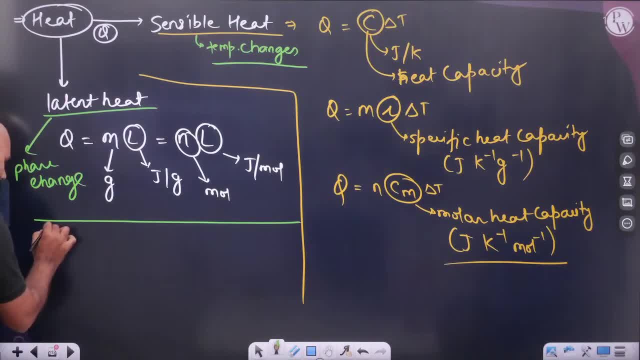 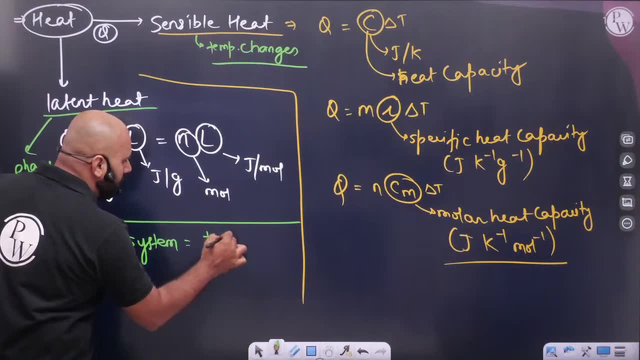 For heat. look at the sign convention, The sign of heat Heat given to system. If you are giving heat to system, then what will you take? Heat absorbed or what will you take? You will take positive Heat given to system or absorbed by the system. 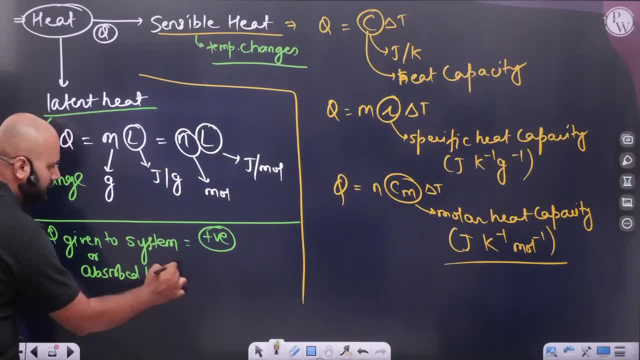 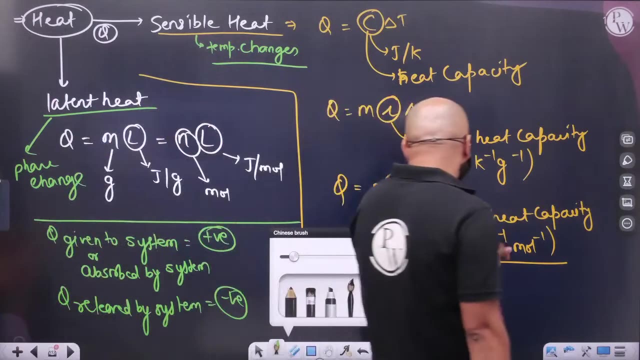 If it is written like this: absorbed by system, then what will be positive? And if I say heat released by system, heat released by system, then what will we take it in the sign convention: Negative. This physics means chemistry is such a chapter. 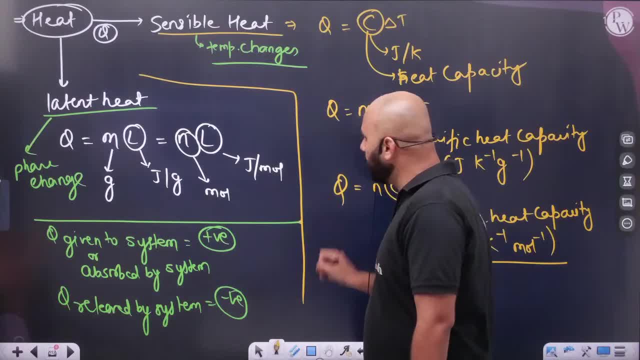 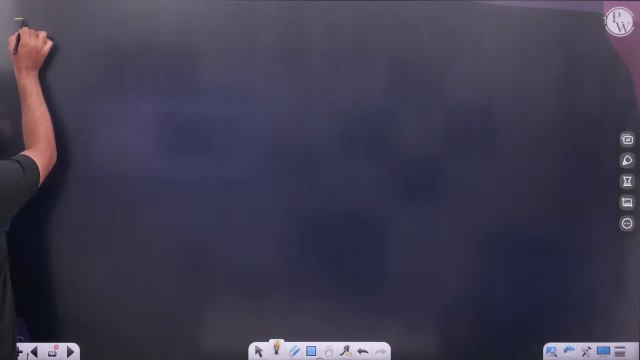 Where we have to follow the sign convention, Otherwise all the numericals can be wrong. So heat released or heat gained, Heat released or heat gained. Similarly, if we talk about work, then if you look at the work, then we have work here. 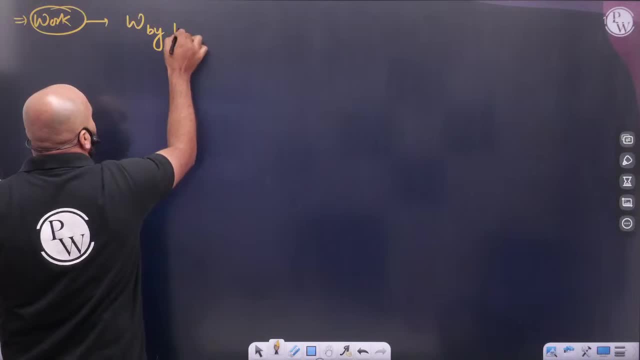 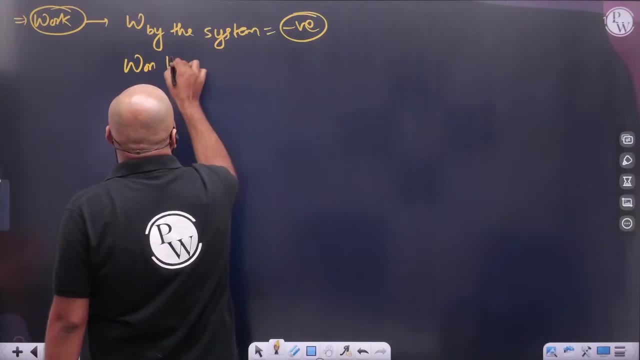 Look at the sign convention of work first. Work done by the system is given. If the system works, that means it will lose energy, it will be negative, And work done on the system will be positive. How will it happen? We will start to see this. 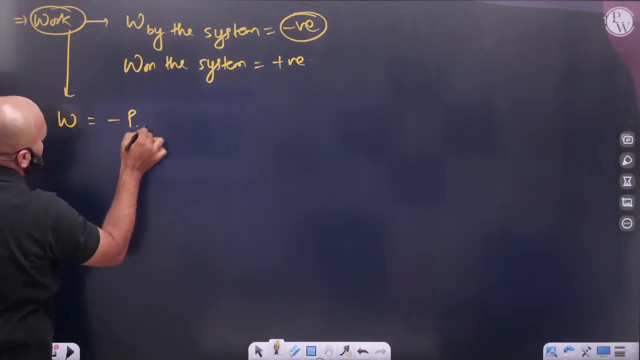 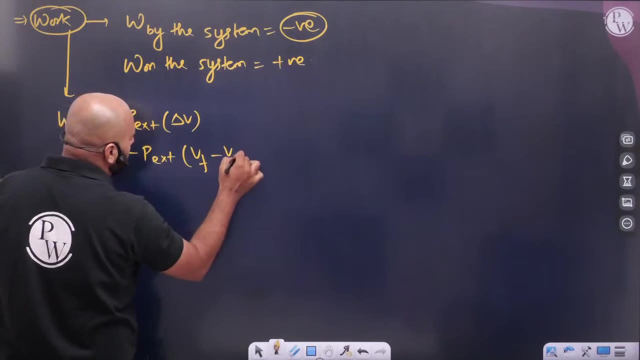 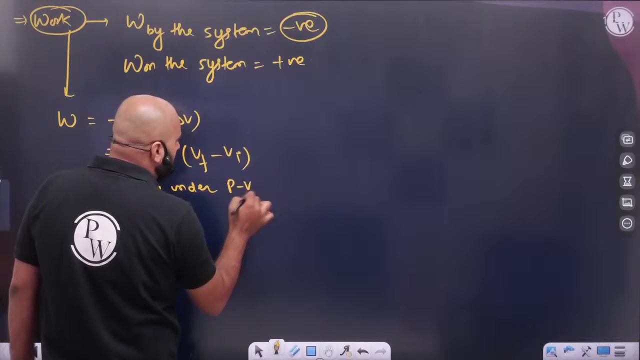 Here the formula of work done is minus p external delta v. or we write: minus p external v final, minus v initial. This will be my work done. Or area under: remember this. Area under pv curve. Area under pv curve. Area under pv curve. 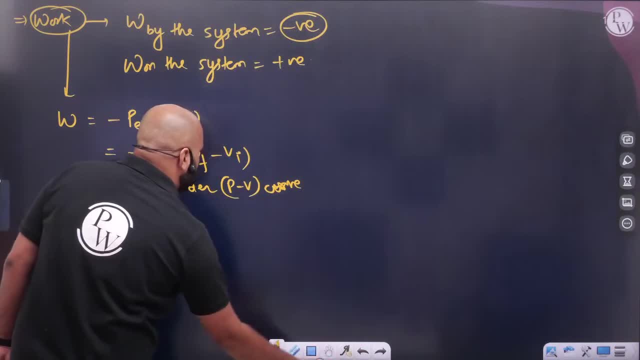 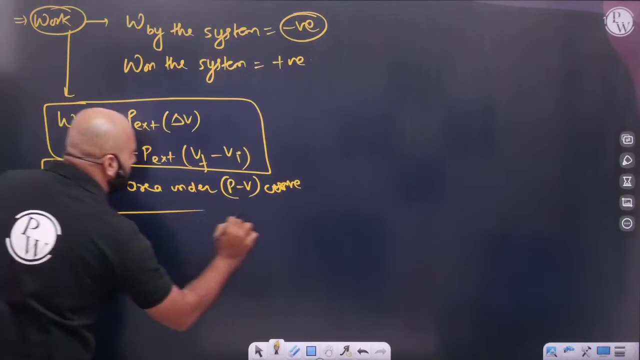 This is its area under pv curve. What does this tell? Sign convention of work done tells: So this is the formula of work done. This is the normal formula of work done. Now look at the work done. Whenever the system works, then we will take negative. 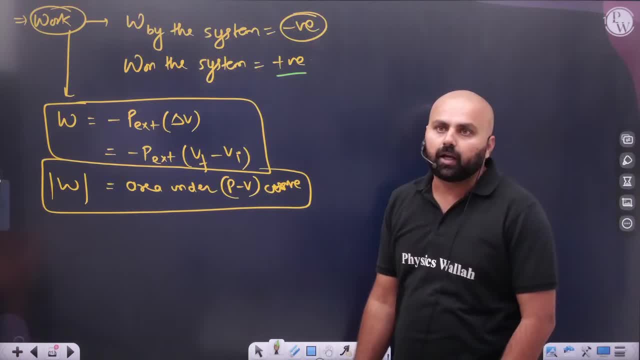 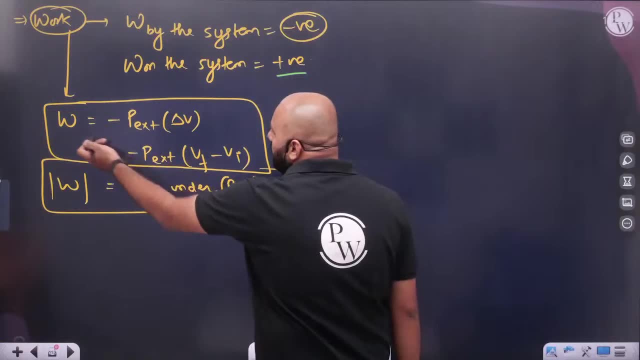 If we take work done on the system, then we will take positive. It is doing expansion. Sir, it is obvious that we do not take work done by the surrounding. We will not take work done by the surrounding. We are taking work done by the system. 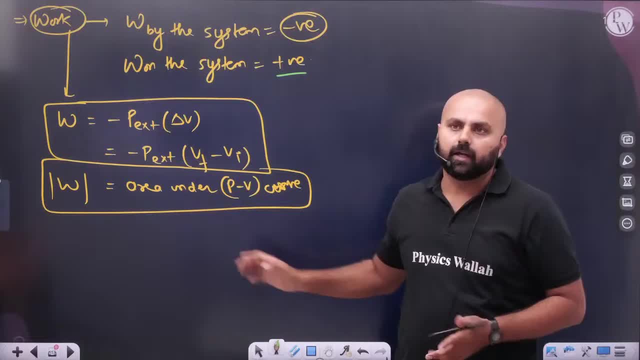 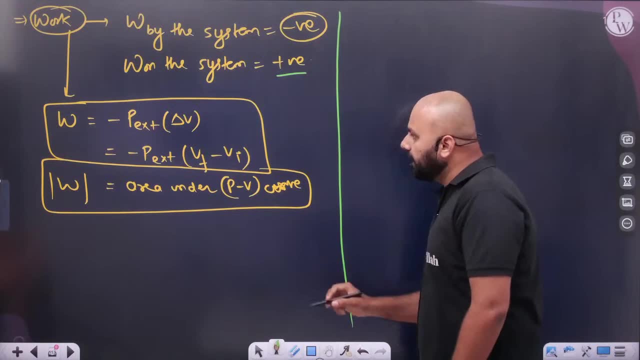 Work done by the system means it must have gone to the surrounding. That's it. So look at this, Look at the heat work. After that, someone told me that, sir, let's do one thing: Work is done, The heat is done. 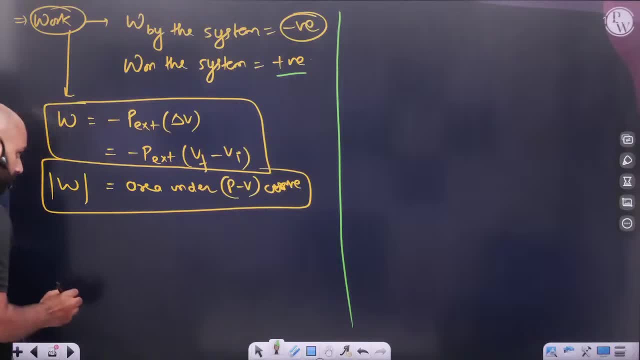 So what will we call the area under pv curve? Now, look here, Now I will talk about everything here Now. I will write it here like this: Now it will come further Work done. formula in isothermal reversible. 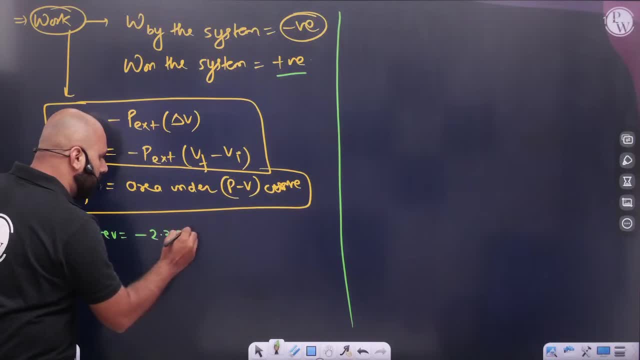 This is valid for all, For all these processes. If you look here, then what will happen? nRT log V2 by V1 will happen. And if you look at work done in adiabatic, then what will happen? P2, V2 minus P1, V1 upon gamma minus 1.. 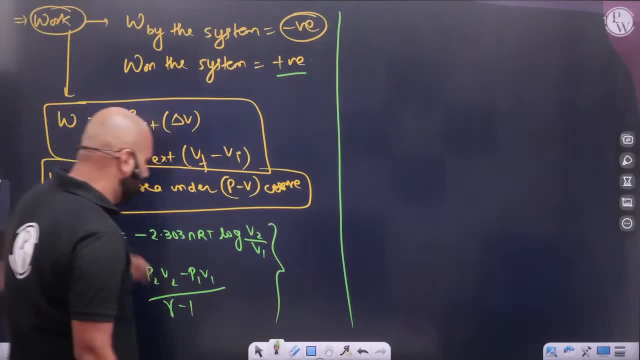 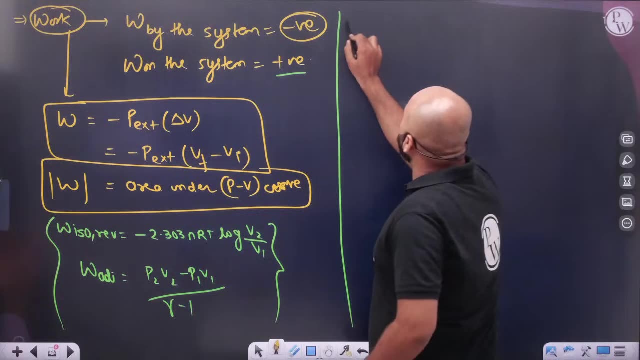 I will write this formula here also so that it will be easy to revise. Sir, both of these are path functions, Work and heat. That's why we are following sign convention. Who will come after that in my life? What comes in my life? 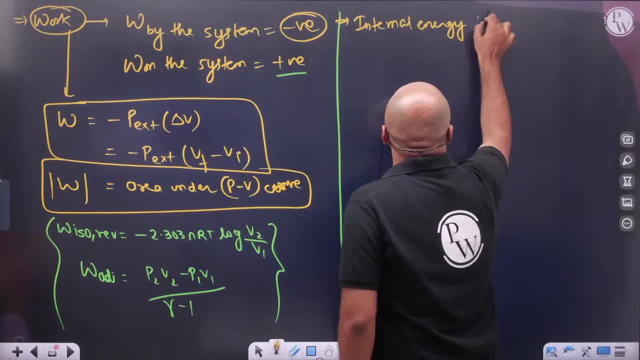 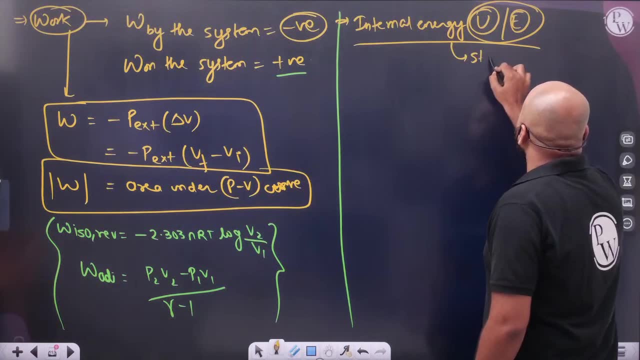 Internal energy. We represent internal energy with U or E, But there is a problem with this. We cannot calculate this exact value. This is again a state function. Look, these were two path functions. Now all of them are state functions. 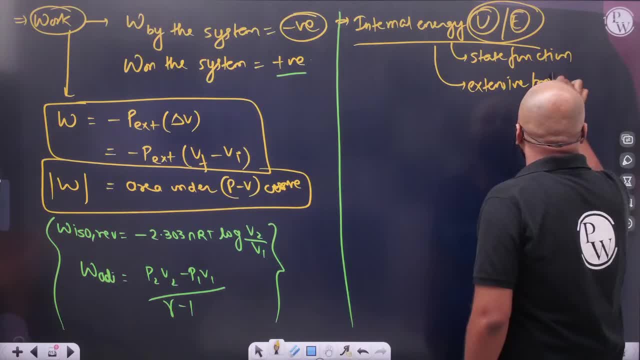 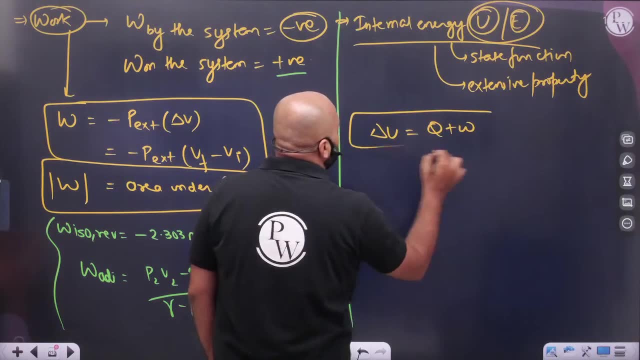 Extensive property. Now look at this case. What you have to do. You can calculate delta U And where will delta U come from Heat plus work done, Where will delta U come from? First law of thermodynamics? What do we call this? 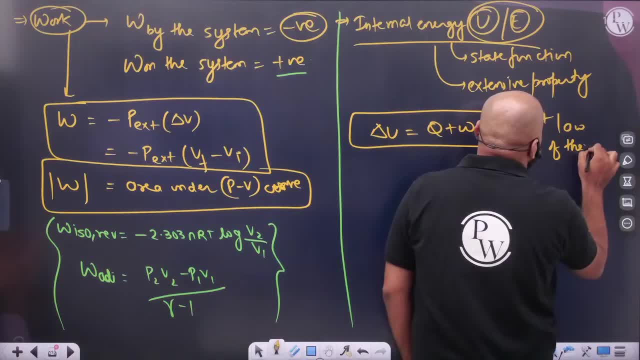 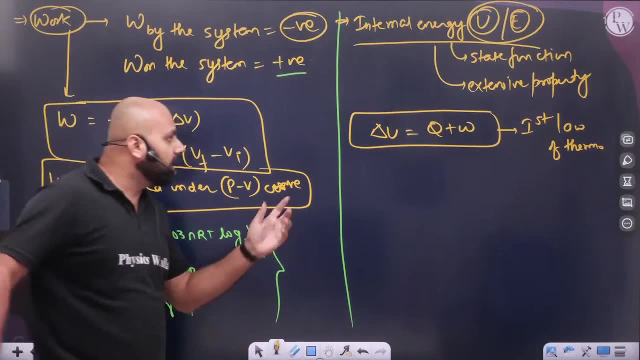 First law of thermo. What does first law of thermo say? Delta U Q plus W will come. Delta U Q plus W. Obviously physics will be different. Sign convention of physics will be different. Sign convention of chemistry will be different. 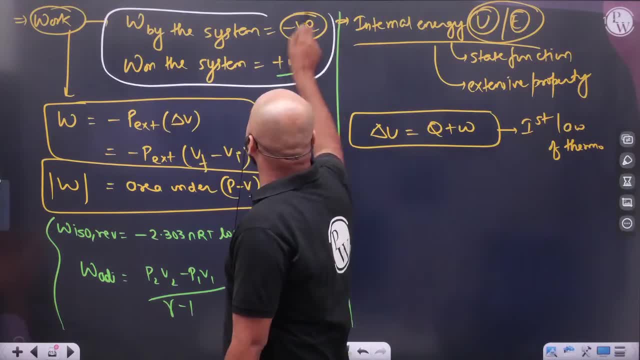 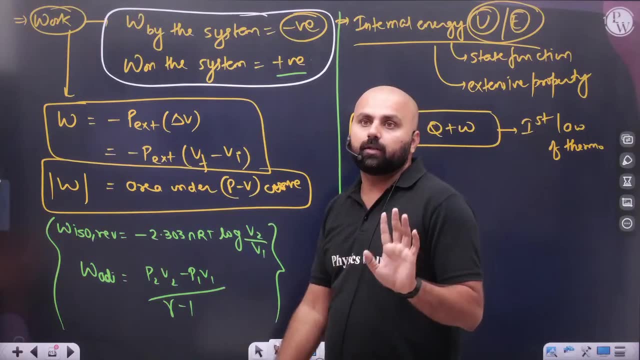 In physics, this sign, convention, Sign convention of work, Sign convention of chemistry will be different. Keep this in mind. This sign convention of physics and chemistry will always be different from work. Work will be different, Work will be different, Not other than that. 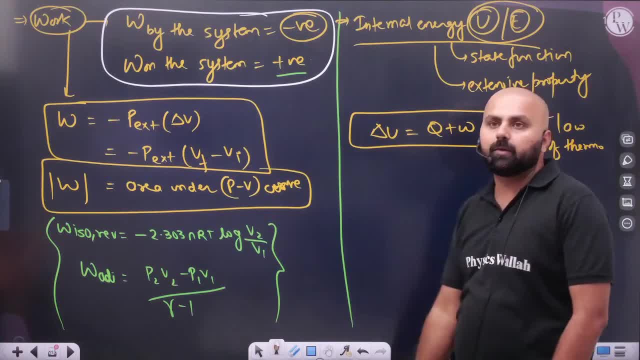 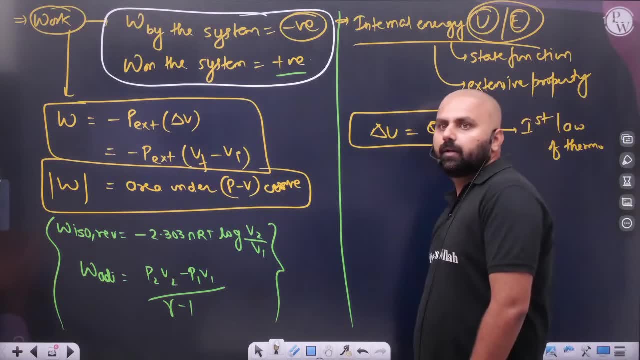 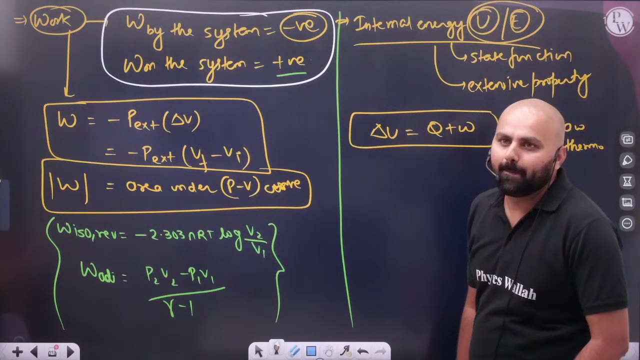 Work will be different. Work will be different. The rest of the heat will remain the same. The rest of the heat will remain the same. Okay, Yes, Look at this. Yes, From next year. Okay, Which is more? Yes, brother. 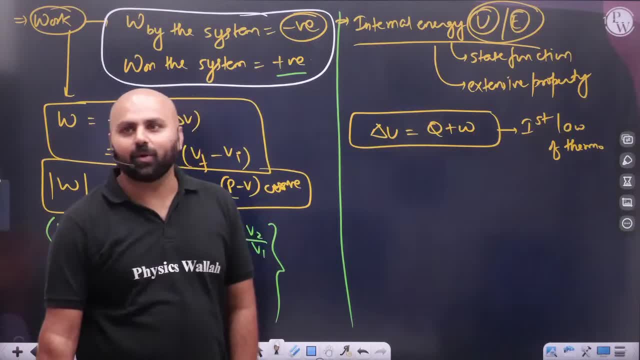 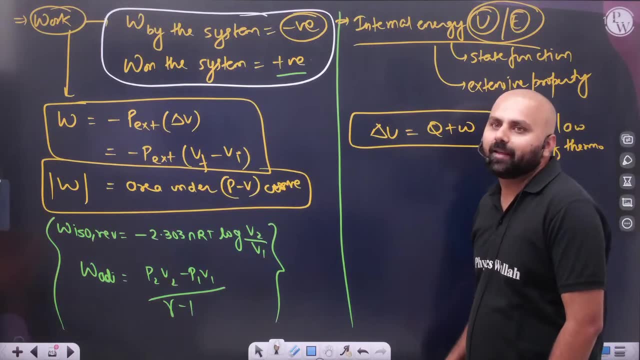 This is the chapter of revision, So now we will not show you derivation here. Okay, Yes, Sign Brother, You can go, No problem. Okay, Now the student is tried to sit down. No, The student is completely thrown away. 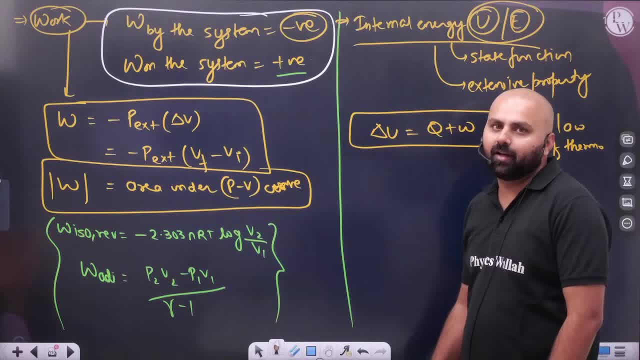 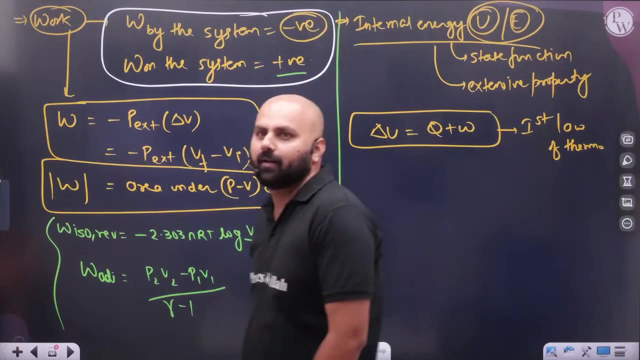 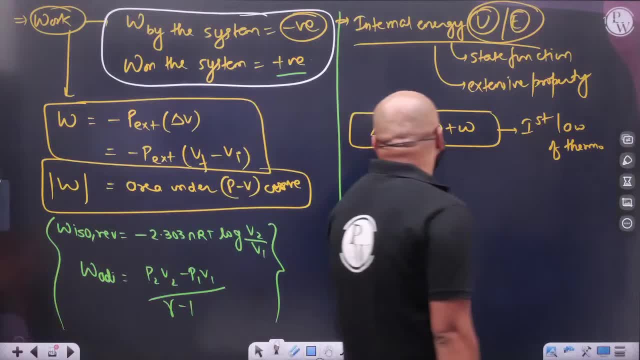 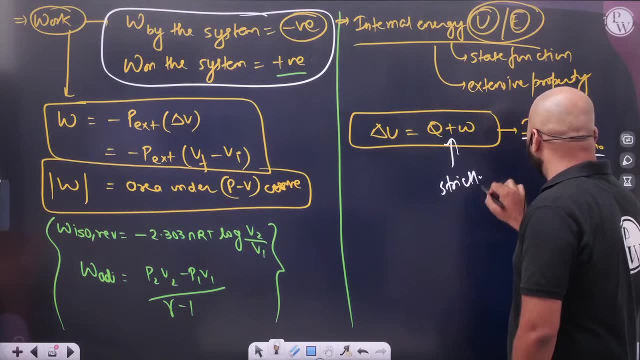 Come on, Let's see What are you talking. Delta U, Let's discuss about the first law of thermo. First law of thermo Only, while using this formula: strictly follow. Remember this, because you keep on saying it repeatedly. people make a mistake repeatedly. 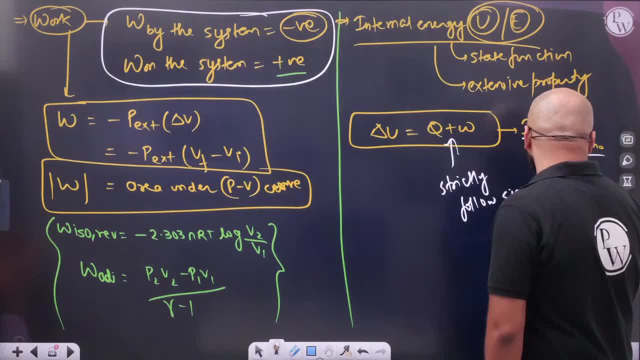 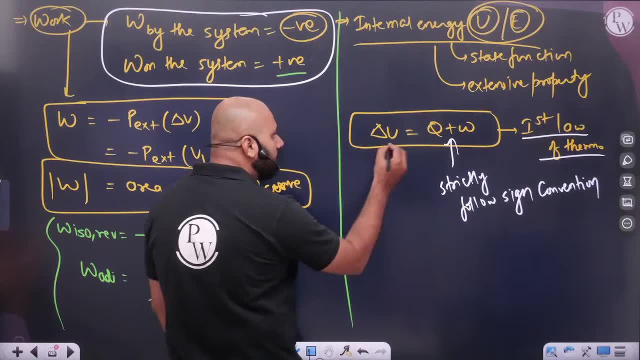 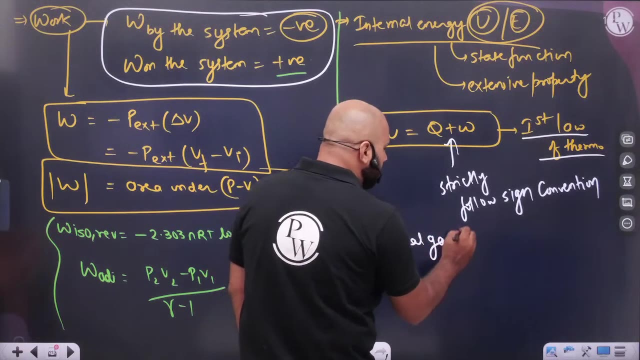 Strictly follow sign convention. Whenever you get a chance, you have to strictly follow sign convention. Next, look at your small things. Get rid of small things, Sir. look at this. If I say Delta U of ideal gas is directly proportional to Delta T. 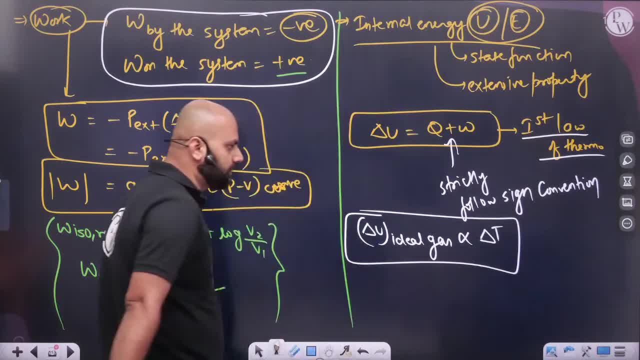 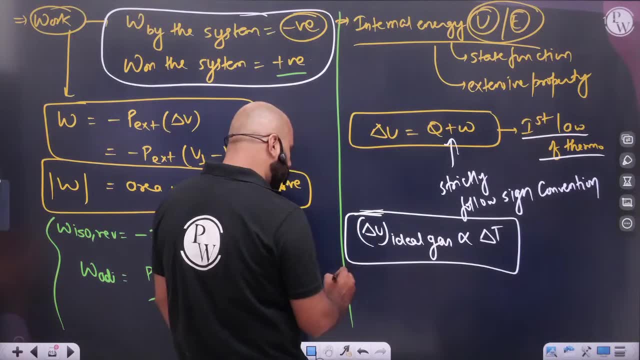 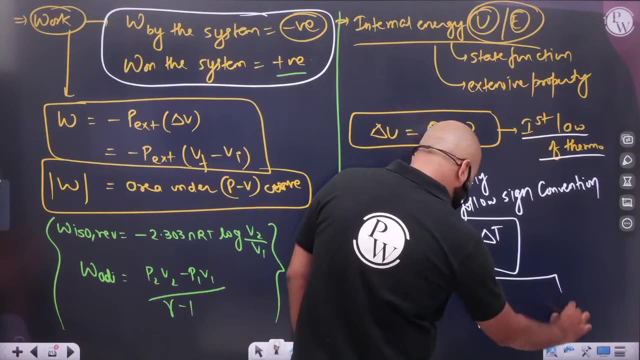 But yes, the temperature of the ideal gas is directly proportional to Delta T. If the temperature changes, then the temperature of the ideal gas will change. Second thing: if I talk about the zeroth law, Now let's understand the zeroth law. The zeroth law of thermonics is so difficult that we can't even imagine. 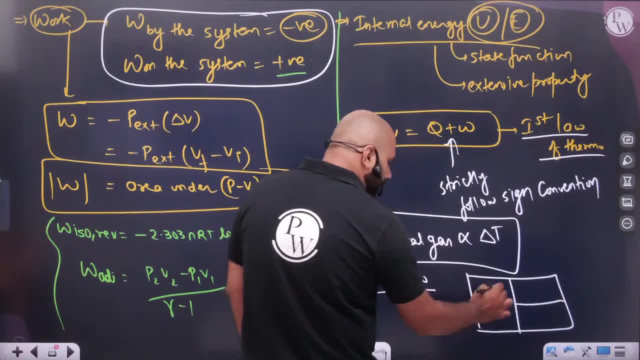 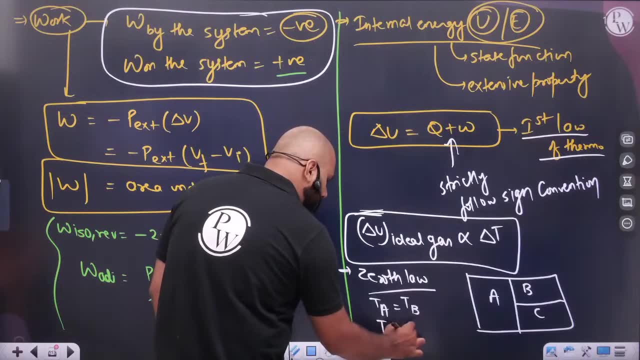 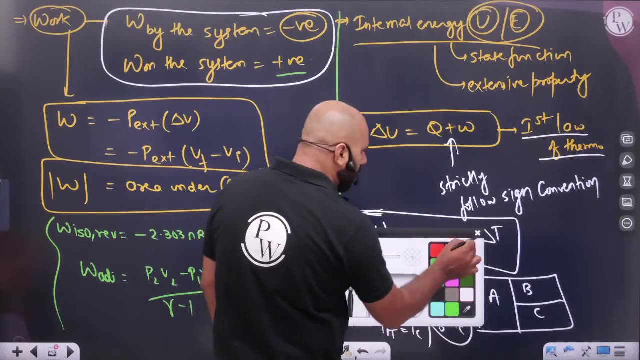 What does the zeroth law say, Sir? if A, B, C is equal to temperature of A and temperature of B, Temperature of A is equal to temperature of C, Then it means temperature of B and temperature of C will be equal. This is what I call the zeroth law. 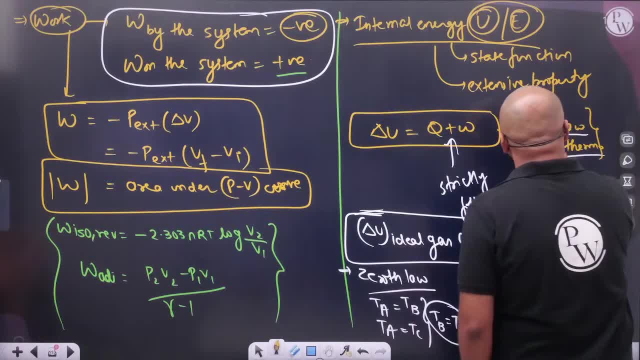 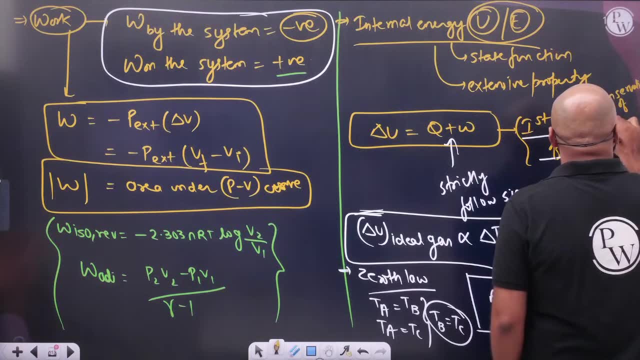 I just wanted to tell you one thing. On which is the first law based? First law is based on the conservation of energy. First law is based on the conservation of energy. First law is based on the conservation of energy And second law is based on the conservation of energy. 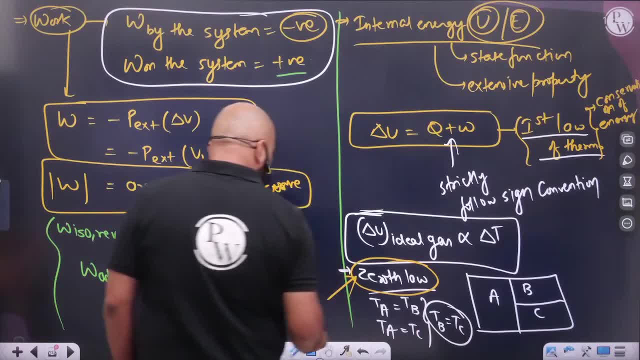 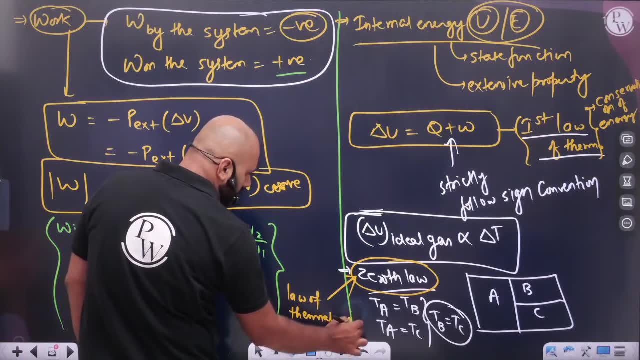 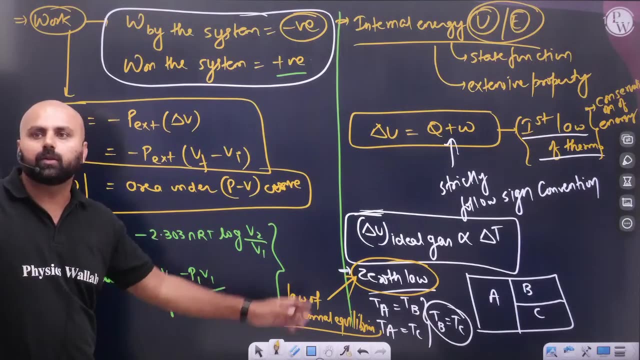 The zeroth law that is based on, from which the law of thermodinamic equilibrium is based, Means temperature of two people is based equal. silly, Now there can only be one question questions on this- That the first law is based on the law of conservation of energy. 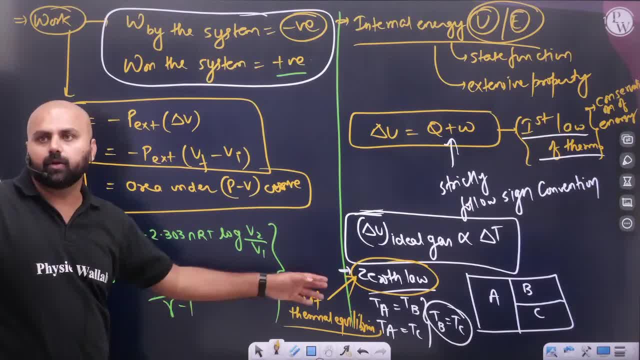 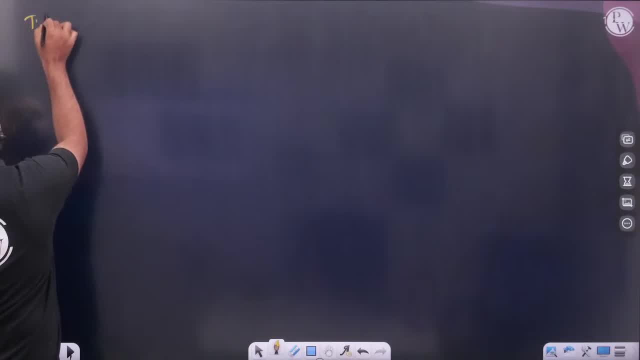 This is based on the law of thermd 너무. This is law of thermal equilibrium. Okay, Okay, Now see First law. as we read, In our life comes types of process, If you see types of process. So what is called in types of process. 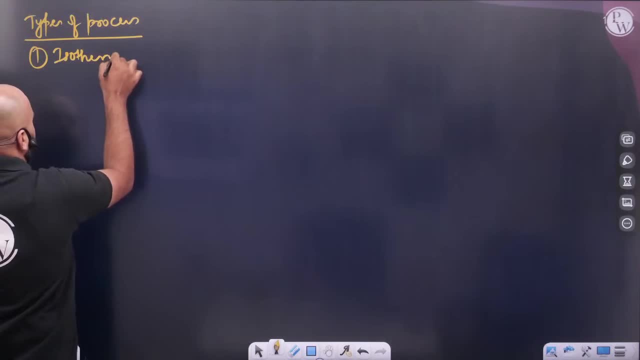 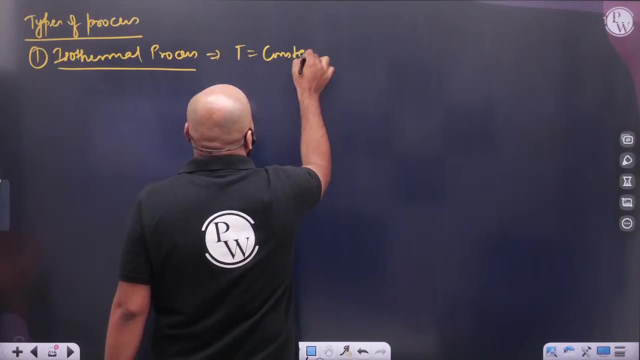 So first process, which is very famous, Isothermal process. In isothermal process, Sir name only knows. Now boil slum, is there? What will be the temperature Constant? Temperature constant, That means delta T 0. And delta U. 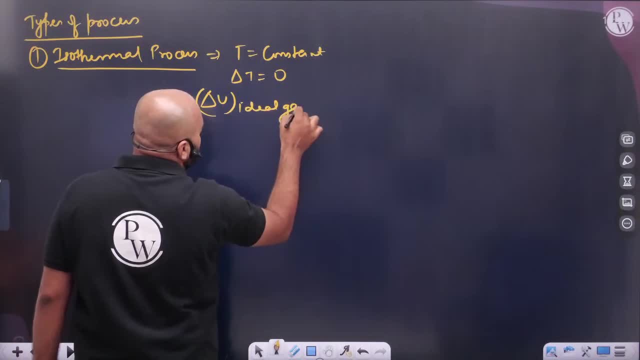 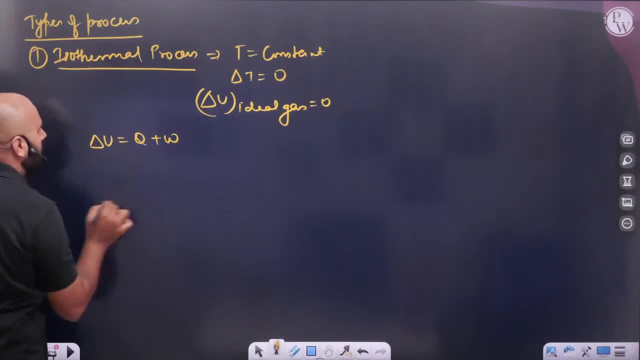 What will happen to the ideal gas? It will become 0.. What will happen to the delta U ideal gas? It will become 0.. So, brother, What does first law say? Delta U is Q plus W. If this becomes 0. 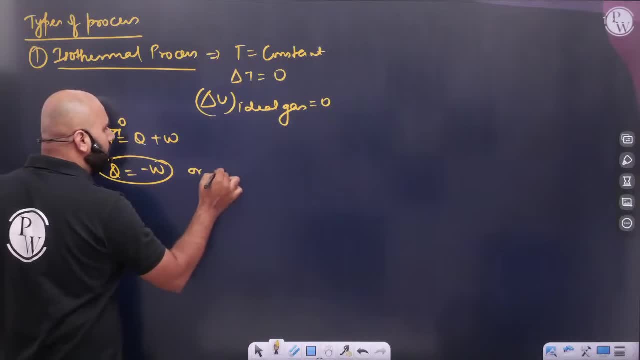 Then heat will be minus of W Or W will be minus of heat. So this is basic thing. PV is equals to constant, Temperature is constant. So here, DP by DV. If you draw graph of P by V in isothermal, Then how much it becomes. 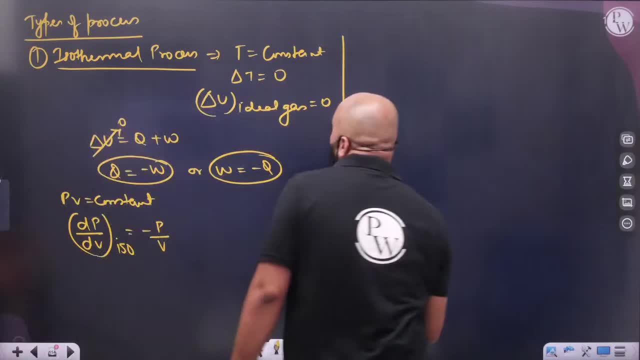 Minus P by V Brother. This is the basic thing. You have already done all these things in physics. That's why you have to see it a little bit. Thermonics has been done in physics. I can take time in thermochemistry. 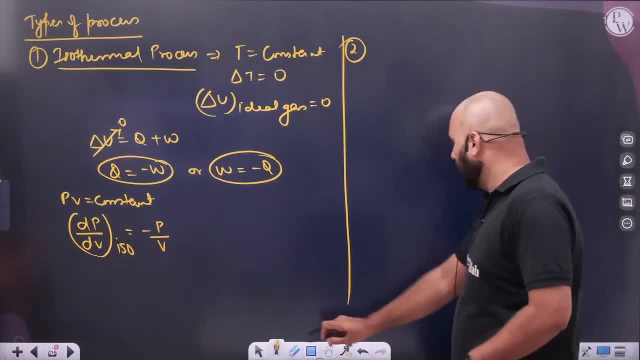 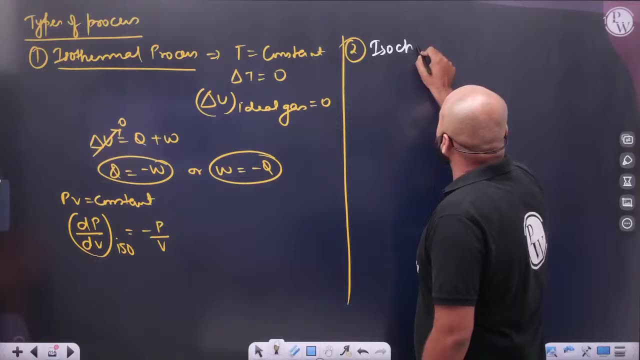 If you have already done thermonics in physics, Then we can do it fast. fast, That, brother. It has already been done in physics. Not many days have passed. The day before yesterday is over. After isothermal, If I talk about isochoric process, 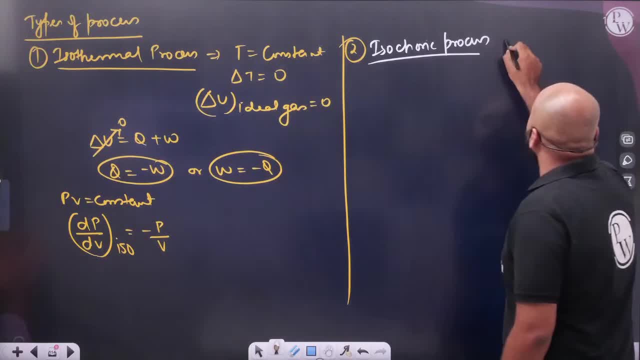 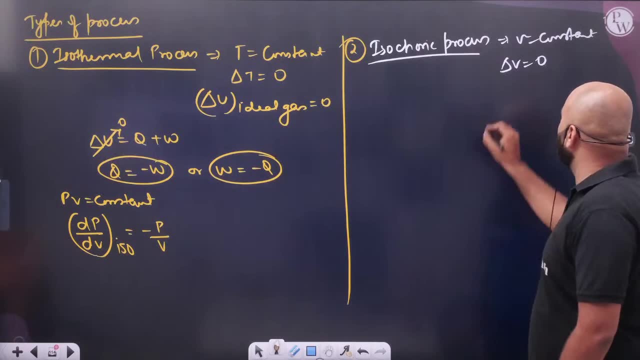 If you see in isochoric process. So what happens in isochoric process? Volume becomes constant. And if the volume is constant, What will happen to delta V Zero? Delta V becomes zero. As soon as delta V becomes zero. 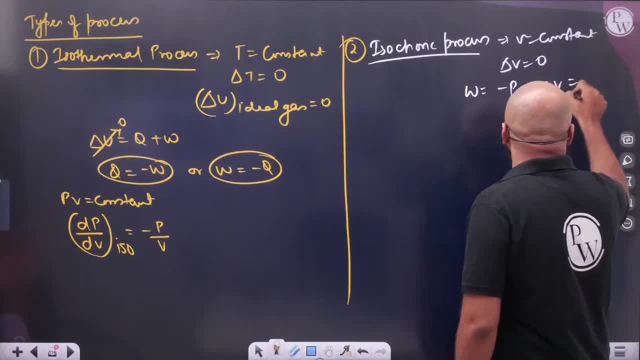 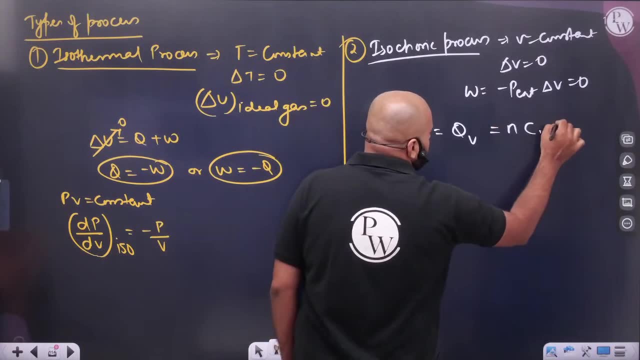 What will be the work done Minus P, external delta V. What will be the work done? Zero Means Whatever. the heat will be at constant volume. Where will all that go To change the internal energy, Sir? See this. 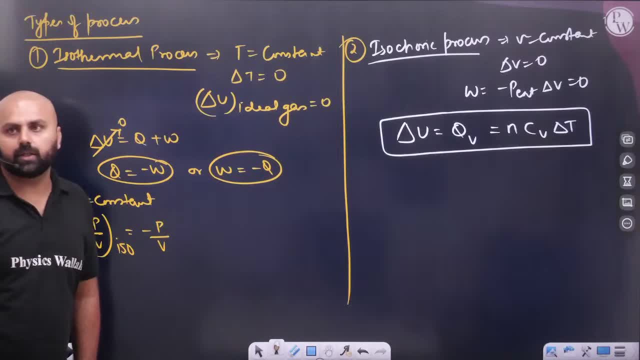 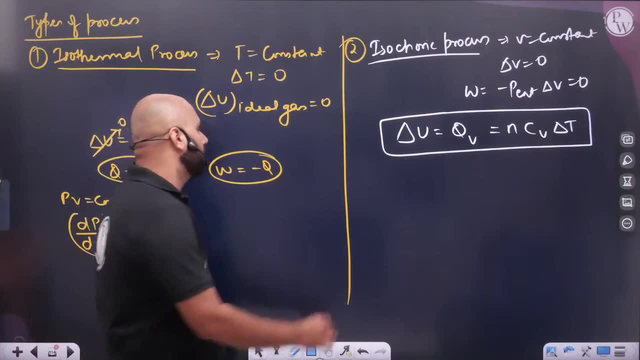 Heat at constant volume. What do we call internal energy change? Ok, Internal energy change, Internal energy change. So see this: What is delta U, Heat at constant volume. Then, sir, Let's talk about third, After isochoric. 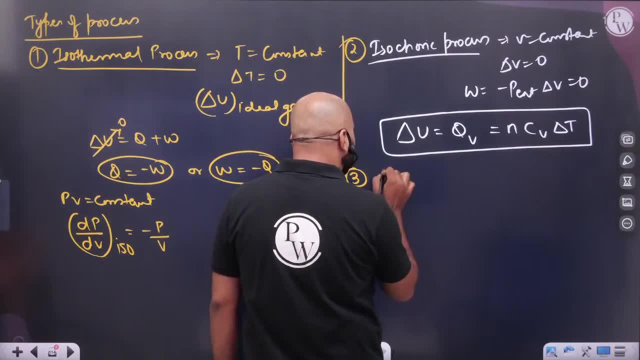 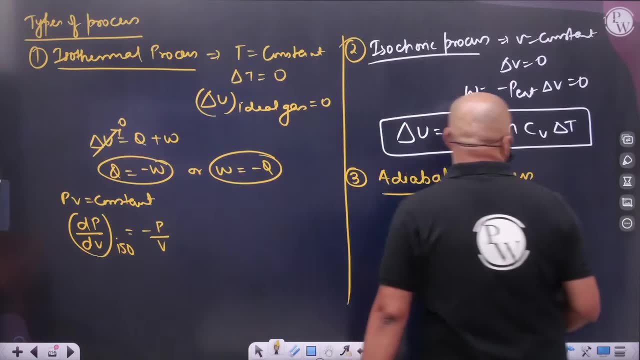 If I talk about adiabatic process, If I talk about adiabatic process, If I talk about adiabatic process, So in adiabatic process, Sir, What will happen? Heat is equal to zero. So as soon as heat becomes zero, 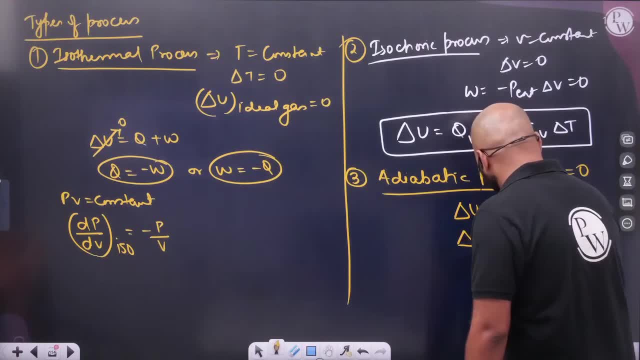 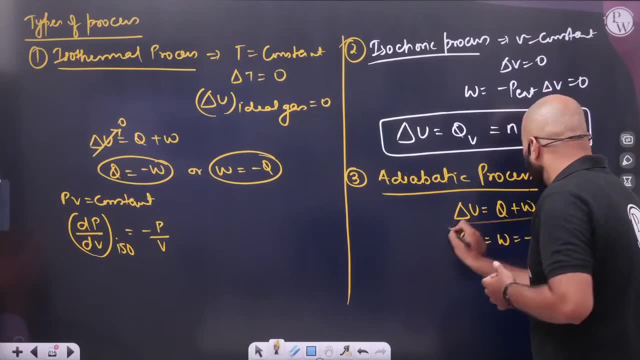 What will delta U become? Q plus W. Delta U is nothing Minus P delta V. Or we can say: Delta U is W Minus P delta V. So this is the formula of delta U, If you see in adiabatic process. 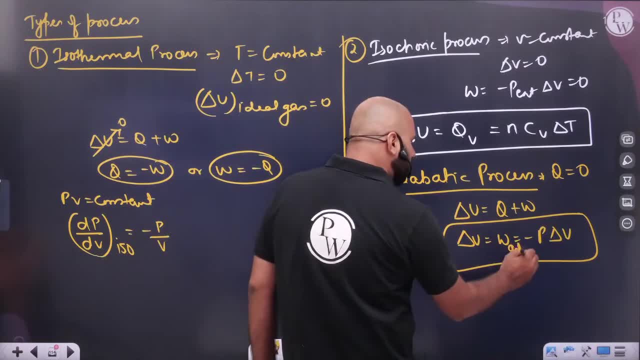 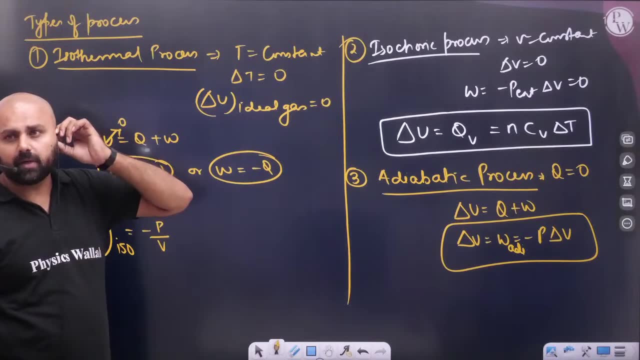 So adiabatic process is nothing. Work done, adiabatic will be equal to NCV delta T. We will pick it up from here. Ok, So see this. See this with yourself. Ok, If I get adiabatic process. 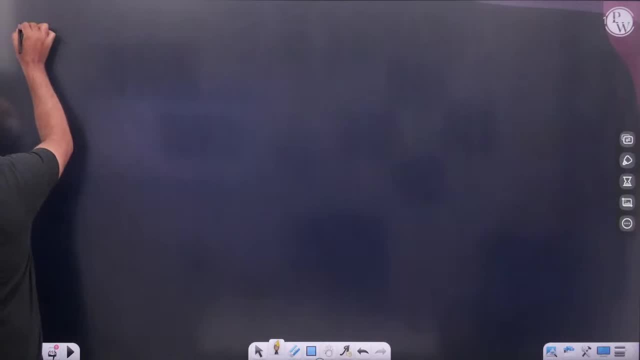 Q zero. Now fourth thing, And here an important thing is going to come, And that is enthalpy. That is known as isobaric process. Brother, quickly, all this Direct questions of this come Isobaric process. Nothing will come separately here. 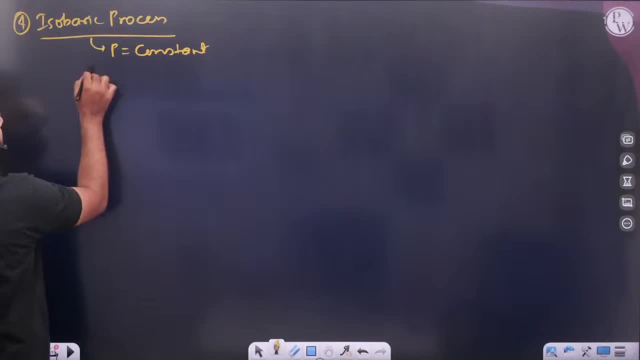 Just these small questions will come Which will trouble you. Pressure is constant. So what will happen? on pressure constant, Nothing will be zero. So what will happen to delta U, Q plus W? And if you see delta U, So Q minus P, delta V? 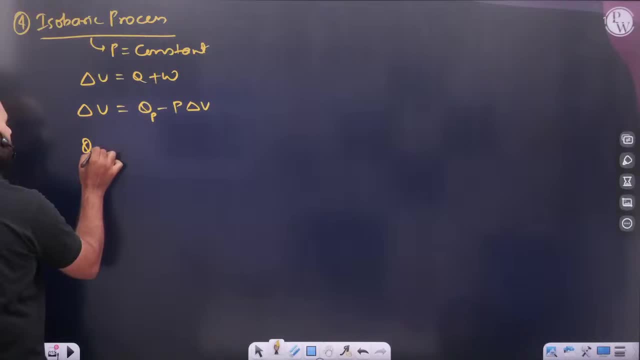 And this is heated constant pressure. So if you want to write QP, So we can write delta U Plus P, delta V, And we give this a new name, Delta H, Where delta H is known as enthalpy Delta. change is nothing. 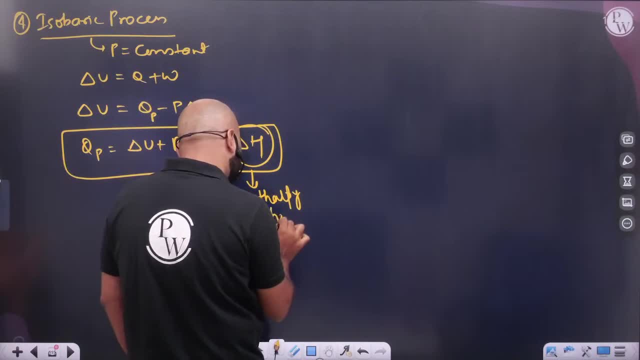 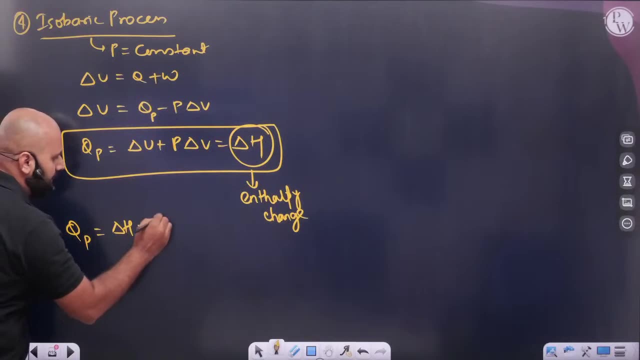 Enthalpy change. What will happen? Enthalpy change, Sir. see this. Heat at constant pressure. Heat at constant pressure is known as delta H. What will be its value? NCP, delta T And heat at constant volume is known as delta U. 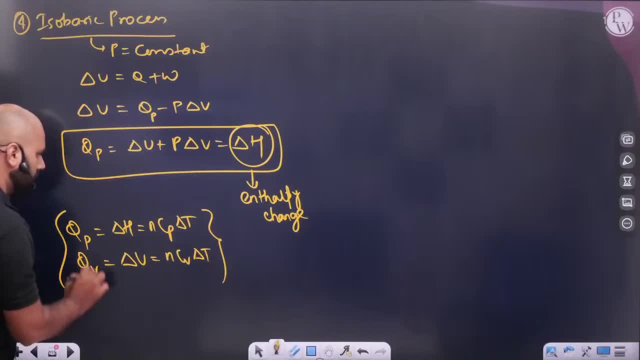 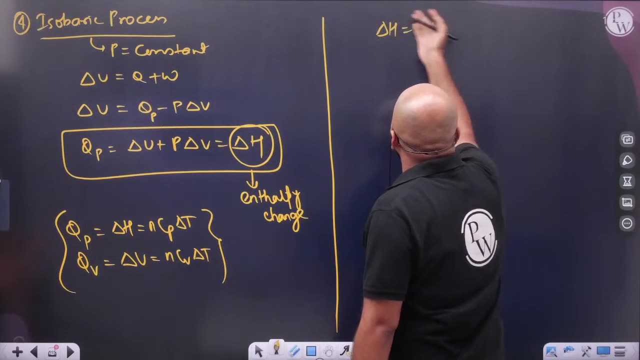 What will be its value? NCP? delta T: What do we start doing from here, Sir? delta H is nothing. Delta U: Now I will talk about enthalpy. I will talk about enthalpy, So enthalpy is nothing. 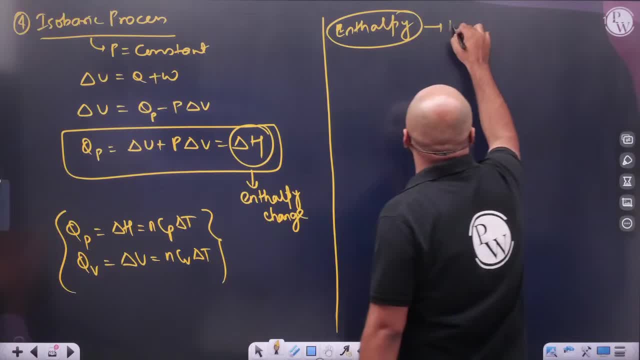 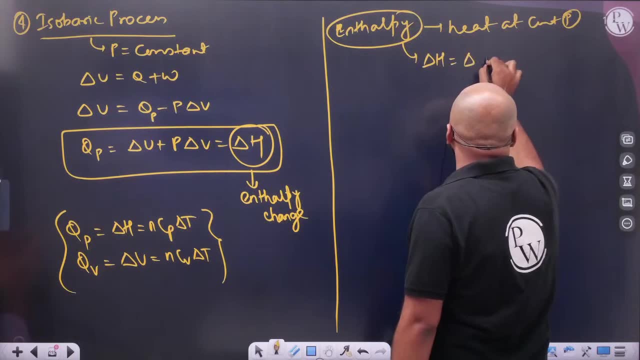 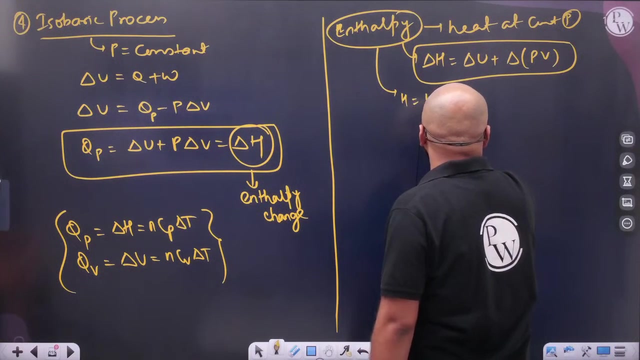 Enthalpy is nothing. Heat at constant pressure, Heat at constant pressure, And if you see here, So what will be delta H? Delta U plus delta PV, Why? Because, sir, what is the value of H? U plus PV? So, sir, the first formula of delta H is this: 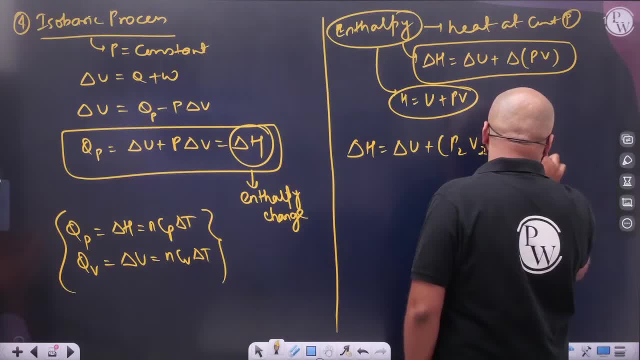 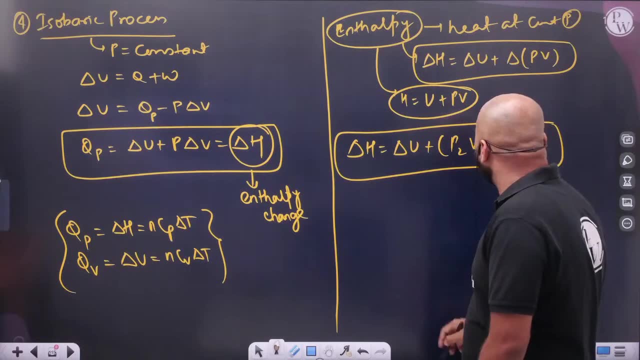 Delta U: P2 V2 minus P1 V1.. Delta U: This formula will come. Then who said, sir, let's do one thing, Let's do one thing. This formula of delta H is coming. So in delta H, If we talk about for ideal gas, 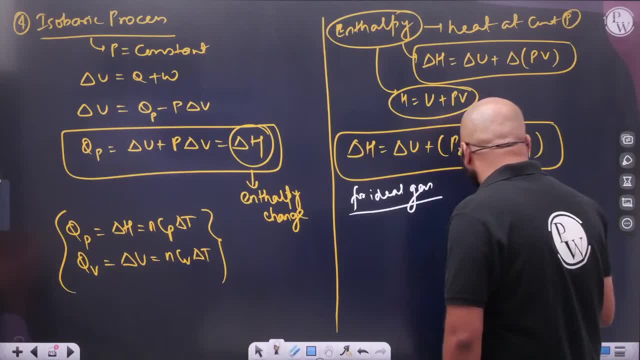 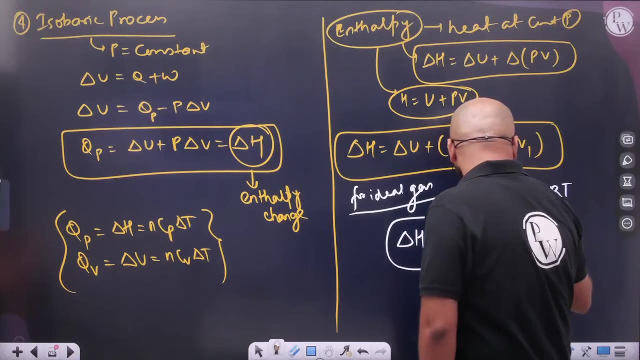 If we talk about ideal gas. So, in ideal gas, In ideal gas, What can we write? P, delta V, Delta NGRT. Sir, delta H is equal to delta U plus delta NGRT. In case of ideal gas, you can write this: 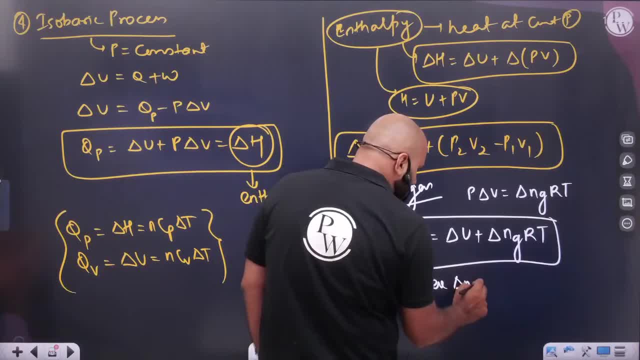 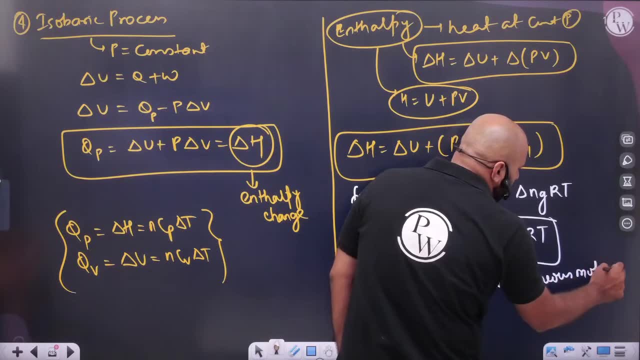 Where delta NG Now? from here, the life of delta NG has started. Delta NG: Number of gaseous moles. Whose gaseous moles? Gaseous moles of product minus. Gaseous moles of product minus. 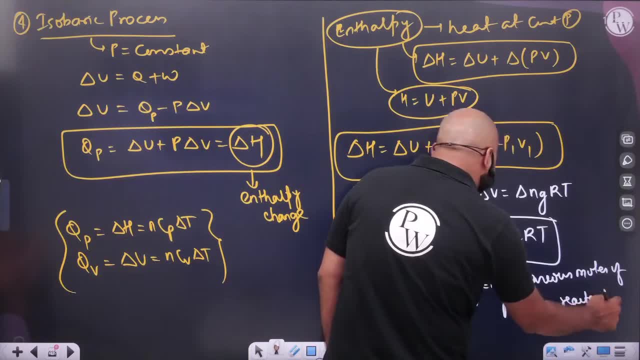 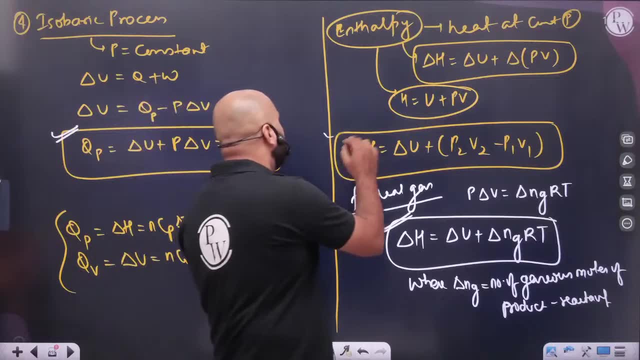 What will happen? Reactant, Remember this. But for whom is this formula? For ideal gas? This formula, This formula is for everyone. This formula is also for everyone. But where is this formula? only For ideal gas? How, Brother, it is simple. 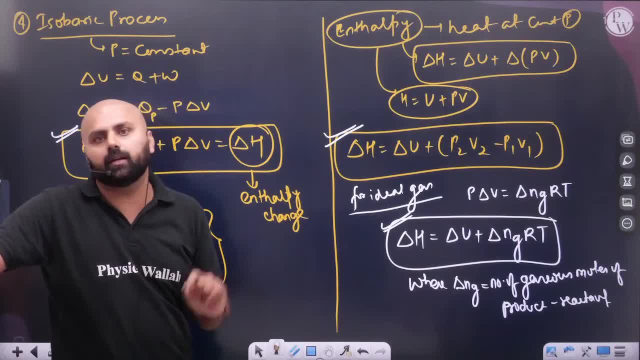 P delta V can only be delta NGRT when there is ideal gas. If there is no ideal gas, Then P2 is equal to NGRT. The�il valid will not be. PV is equal to valid. we won't have. PV is equal to delta NGRT. 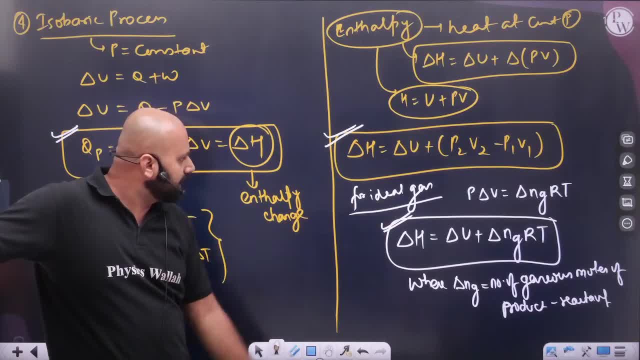 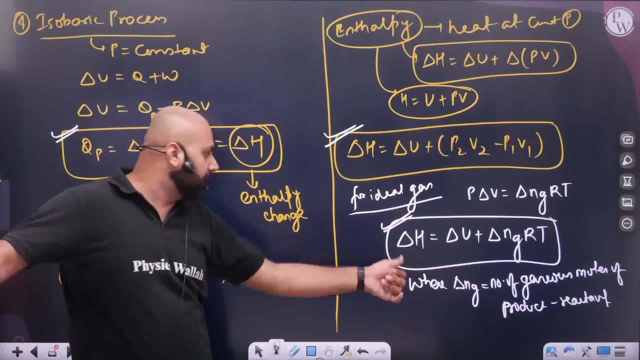 Ok, keep this in mind. With ideal gas- here it will be P, delta, V, delta NGRT. What will the value of delta H be? ZUL U plus. Many questions will arise about this. Many questions will arise Here. we Now here on this. 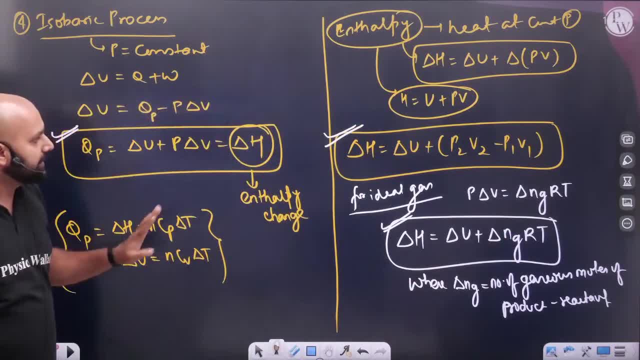 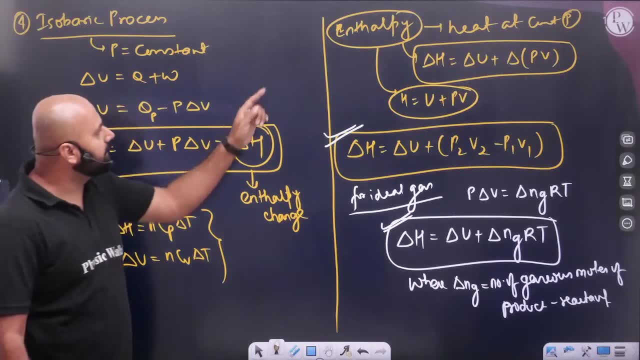 Here: this formula, Then this: The questions will be full of enthalpy above two or three formula. Ok, After that, look, I was told Enthalpy, Enthalpy again, is a state function. What is Enthalpy? It is a state function. 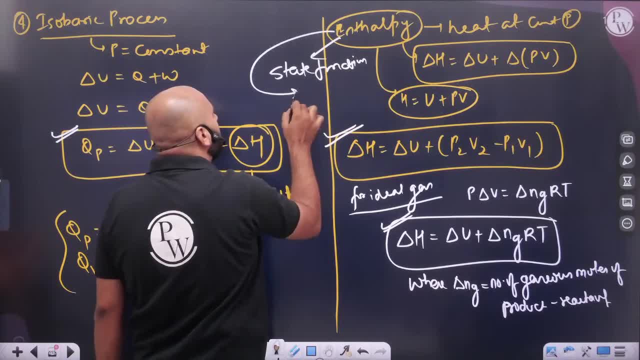 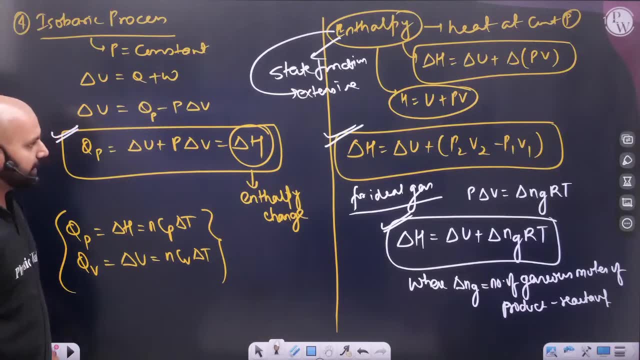 Again, Enthalpy is a state function. It is an extensive property. What is Enthalpy? It is an extensive property. So extensive property, state function. these small things are added. Keep removing yourself. Gaseous moles, delta, H. 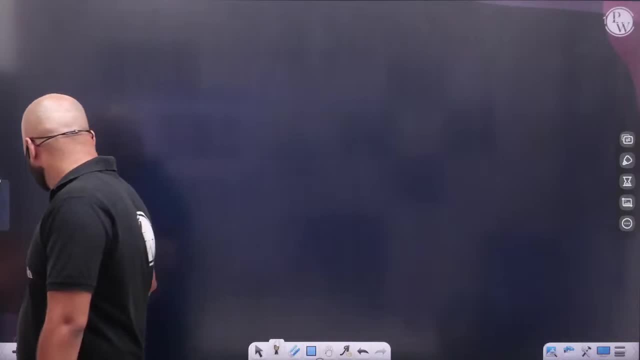 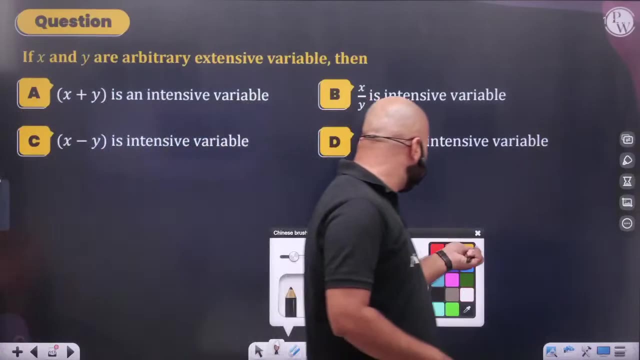 Should we do the question? Let's do the question and see. Let's do the question and see. Here it is. Look at the question with us, Sir. X and Y are extensive variables. Then tell us the answer. Shoot the spammers. 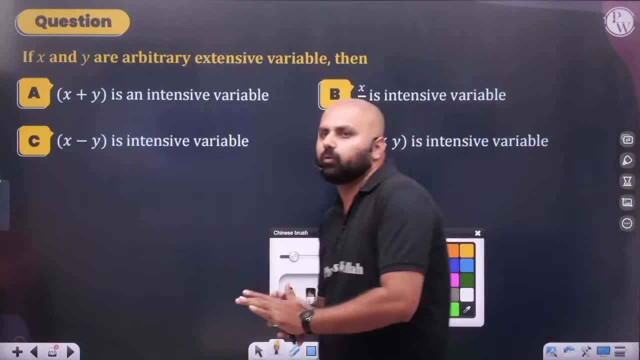 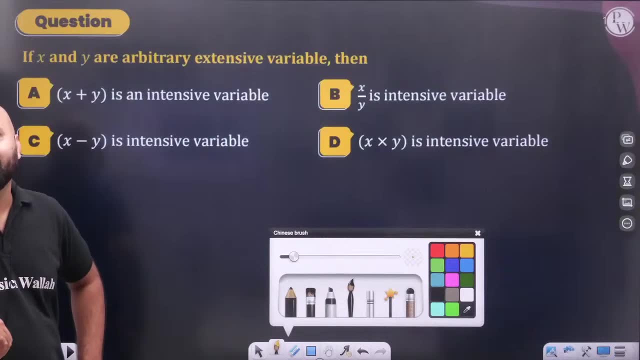 Start telling us your answer. There is no use in blocking them. One name will do it, another name will do it. You do your work, Just put it aside. Okay, Quickly, What will be the answer? What will happen, Sir? X and Y are extensive variables. 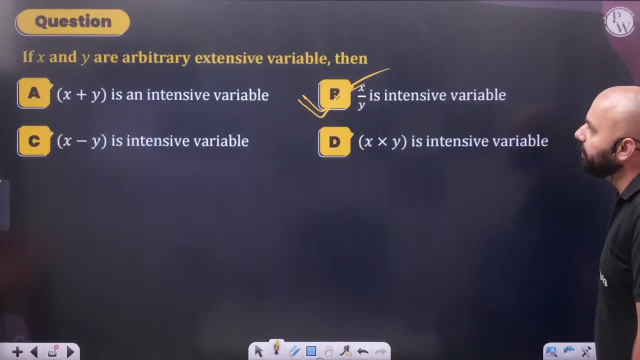 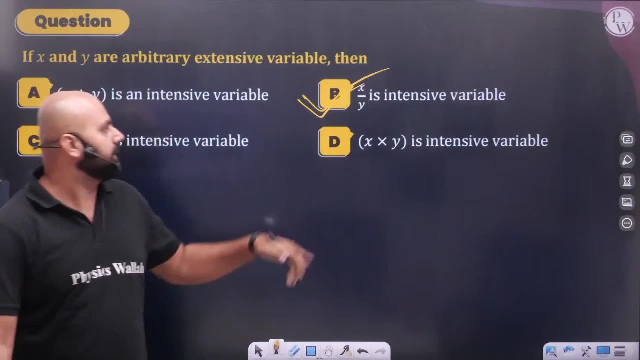 What will be x, y, y Intensive variable? Why? Because if we add Extensive, extensive is not necessary. But if we divide what will be extensive upon extensive Intensive, What will be extensive upon extensive Intensive? 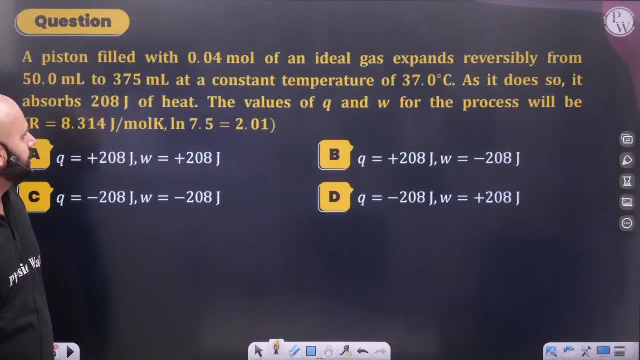 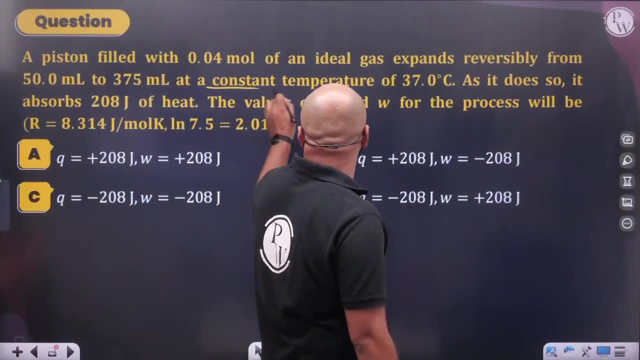 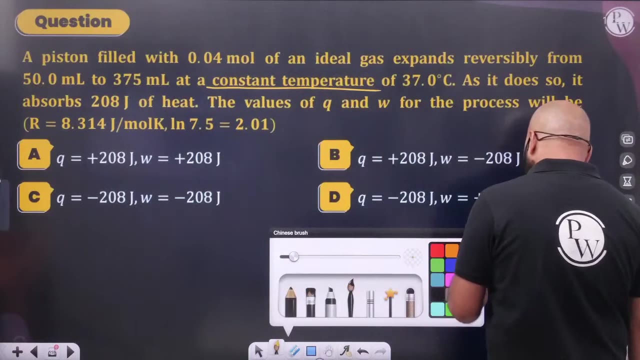 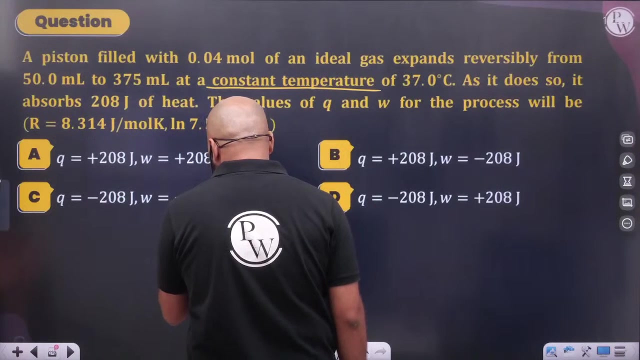 Let's see the next question. What is the gas? What is the temperature Constant? Whenever there is a constant temperature, in the case of isothermal, when the temperature is constant, what will happen to delta U ideal gas? It will become zero. 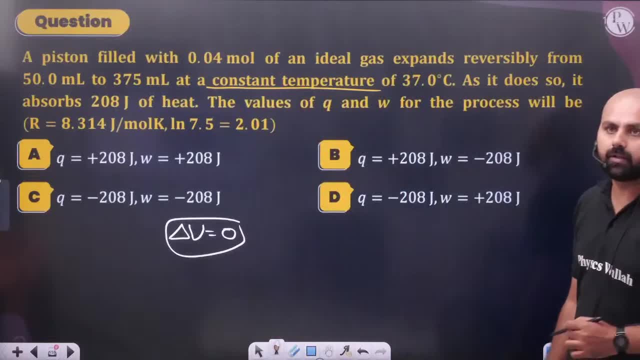 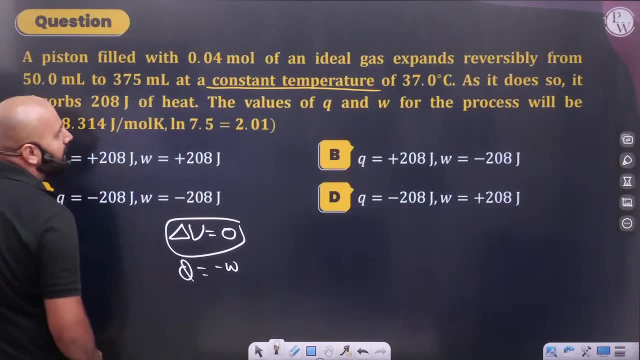 When delta U becomes zero, we don't have to do the calculation. What will happen to delta U? What will happen to delta U? Delta U zero means Q is equal to minus W. Sir, you are absorbing What is your heat? 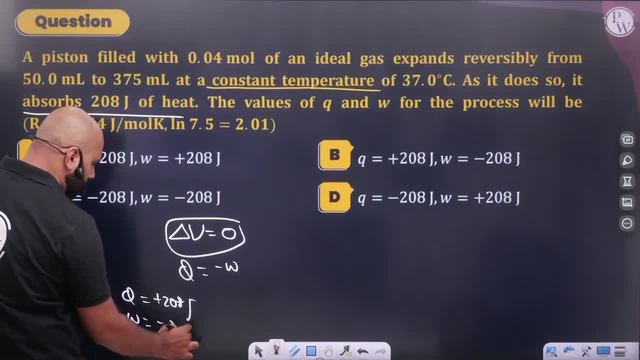 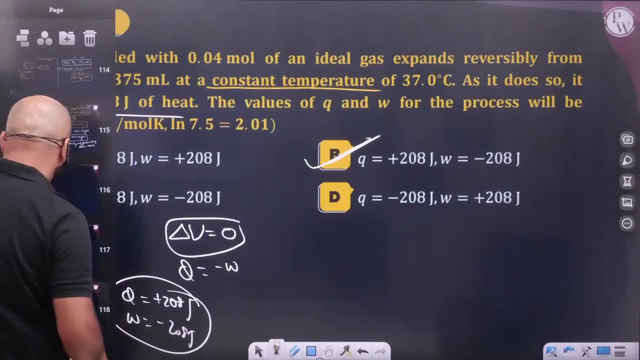 Plus 208.. So what will be the work done? Q is equal to plus 208.. What will be the work done Minus 208.. So do such questions? Look at this. Look at this question. What will happen? 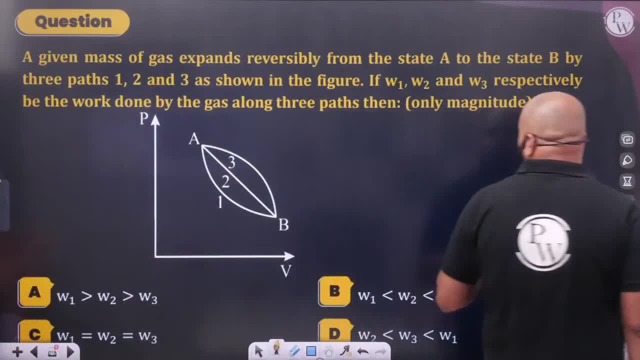 Work done. What will be the work done? Area under the curve. Area under the curve. What is he asking Magnitude? What is he asking Magnitude? Look at the answer to this question. What is he asking Magnitude? 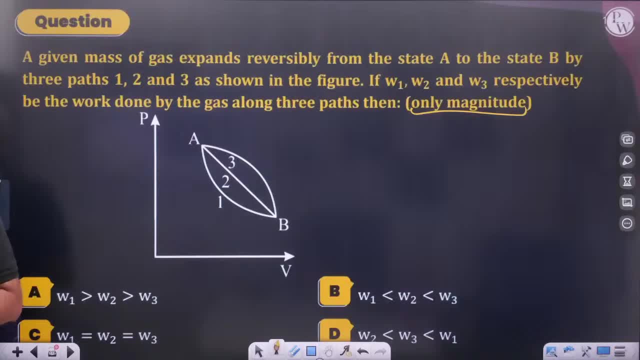 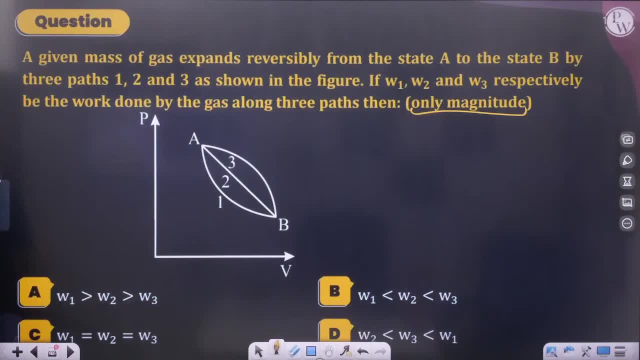 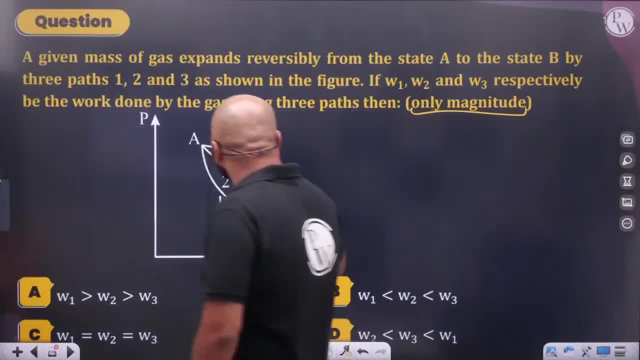 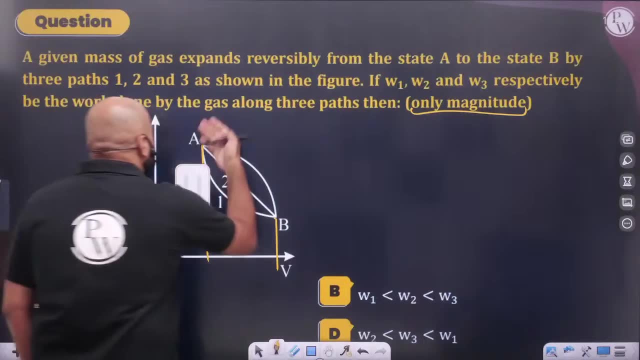 what will happen, Sir? whose work done will be more? See the area under the curve. whose area is more under the curve? If you see the area under the curve, then work done of third, then second, then one. Whose area under the curve is more? 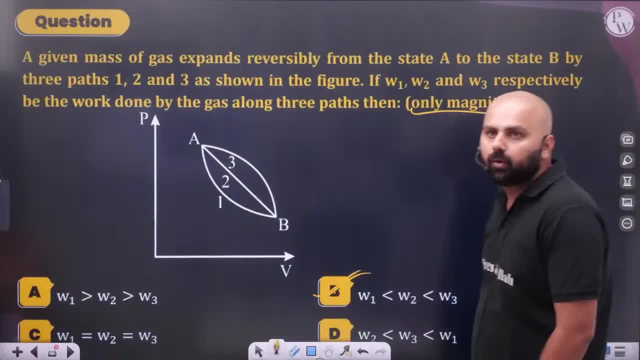 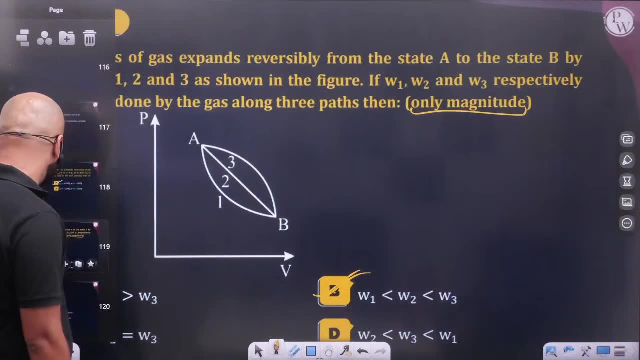 Third, then second, then whose will come? One Keep on taking out, Take out the area under the curve like this. Then who said, Sir, this work done came to us, Work done. area under the curve, Area under the curve. Now see, You have 3 processes, 4 processes. 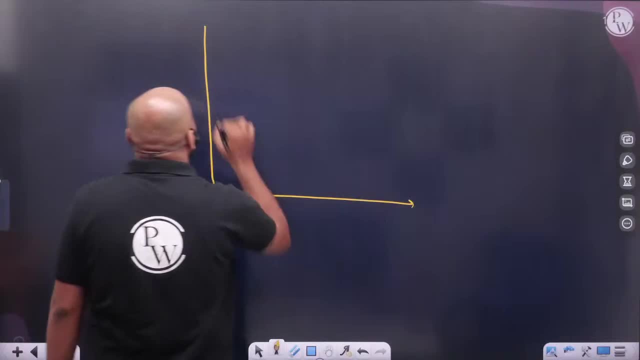 If I mix all the 4 processes, If I mix all the 4 processes, See this: Pressure versus volume. See this. If I mix all the 4 processes, Then See this, Sir: what will be this process called Iso-Baric? What will be this process called? 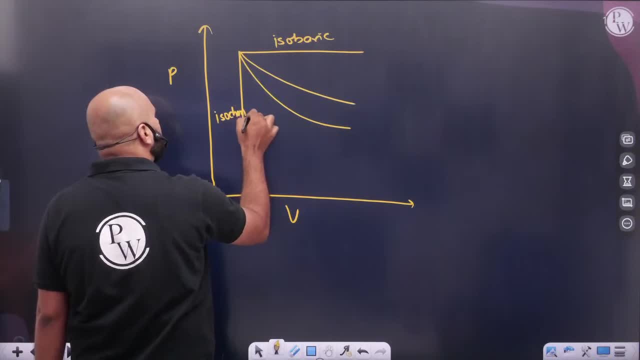 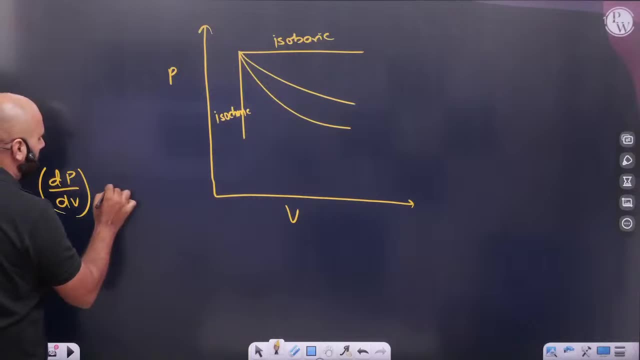 Iso-Baric. What will be this process called Iso-Correct? But Remember one thing: Dp by Dv In the graph of pressure versus volume, What is the value of the graph of isothermal Minus P by V? Its slope is minus P by V. 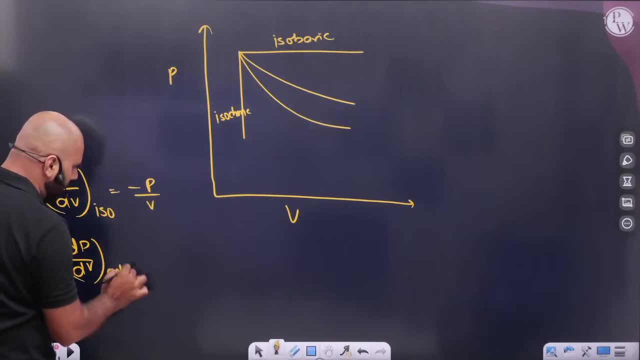 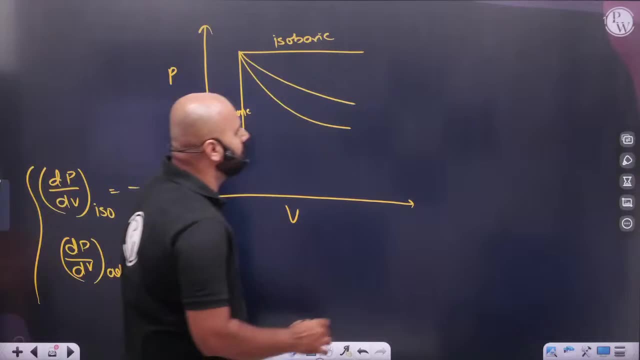 Dp by Dv. If I talk about adiabatic, Then, Sir, everyone has read: Minus Gamma, P by V. What are the values of Gamma? What is Gamma? We all have read: Gamma is nothing. Cp upon Cv. All this has been done in physics just now. 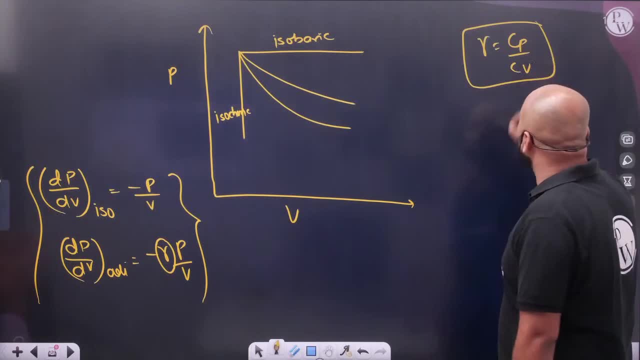 Everyone should come in exam. pass. Gamma is nothing. Cp upon Cv. And if we talk about Cp upon Cv? If we take out Cp minus Cv, What happens? R becomes for 1 mole. If we talk about 1 mole, What will happen For 1 mole? 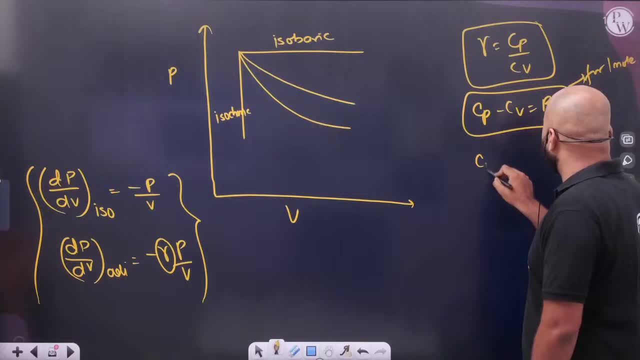 Cp minus Cv is equal to R. So if If you want to take out here: Cp is nothing, Gamma times Cv, Now you can take out by putting here: Cp is nothing, R upon Gamma minus 1. This is the formula of Cv, This is the formula of Cp. 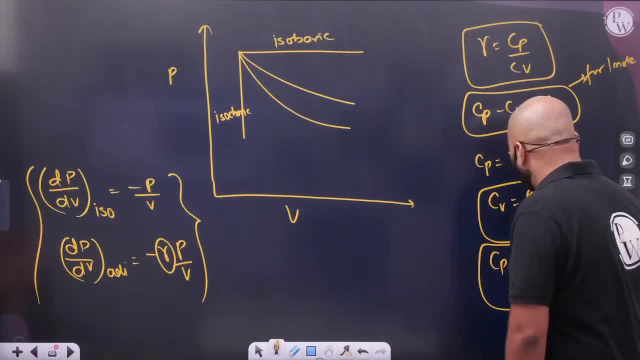 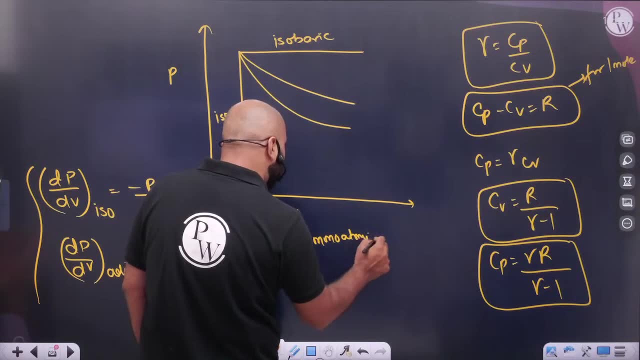 You have done all this in physics, I don't need to tell this. What are the values of Gamma If Gamma is monoatomic gas? If it is monoatomic gas, Then what is the value of Gamma? Gamma will be 5 by 3 If it is diatomic gas. 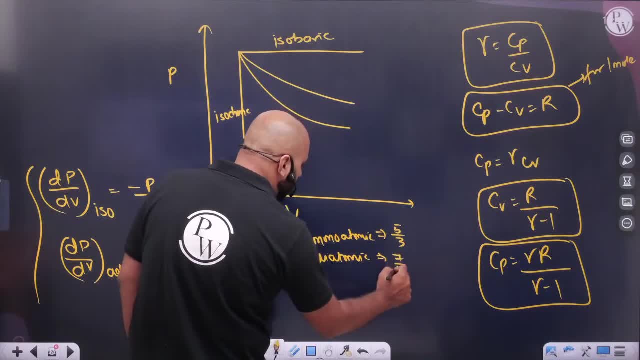 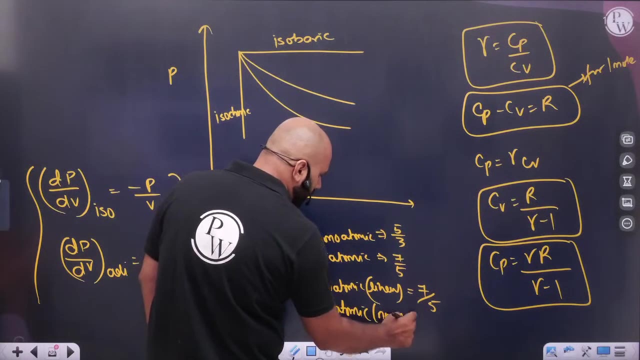 Then it'll be 7 by 5. If it is triatomic linear. If it is triatomic linear, It'll be 7 by 5, And if it is triatomic nonlinear- In this case Triatomic nonlinear- Triatomic non-linear will be 4 by 3.. 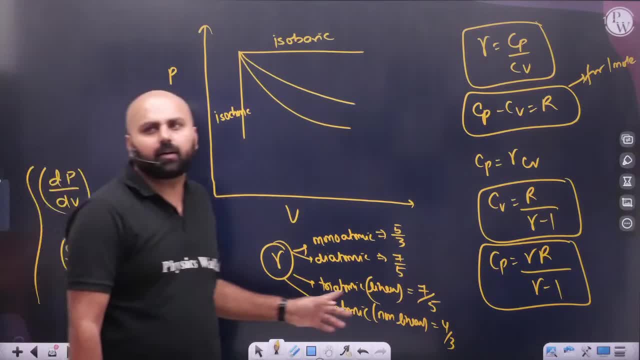 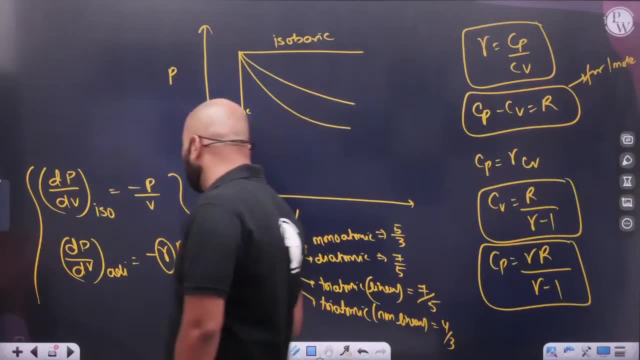 So gamma values, You have done all this in physics. If you have done this in physics, then it is no use wasting time on physics. Okay, No, if there is no sign convention, then we have to see whether it is doing expansion or contraction. 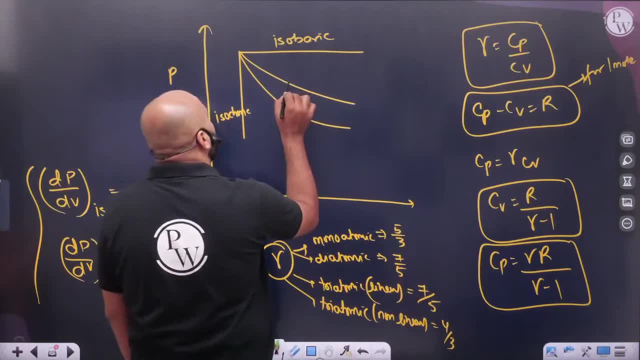 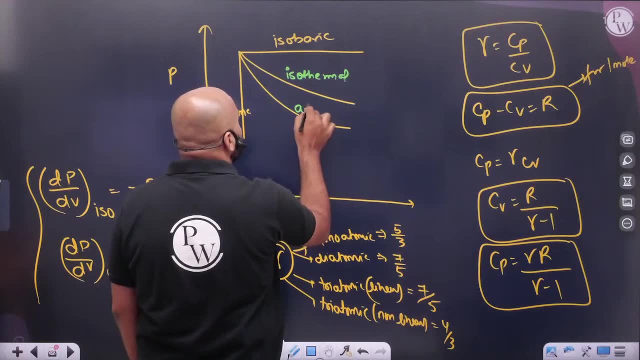 So whenever someone tells you adiabatic and isothermal, then remember always in graph who will be above. Isothermal will be above, Adiabatic will always be below. Adiabatic will always be below. Remember this graph. 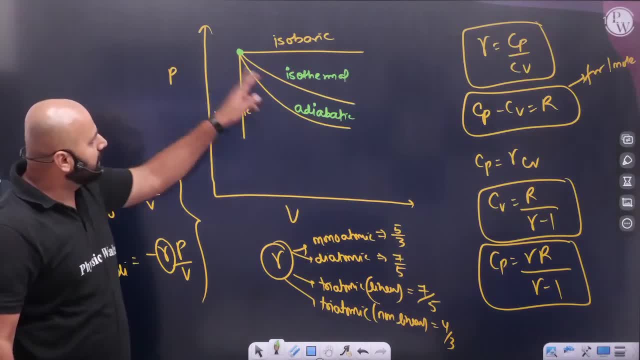 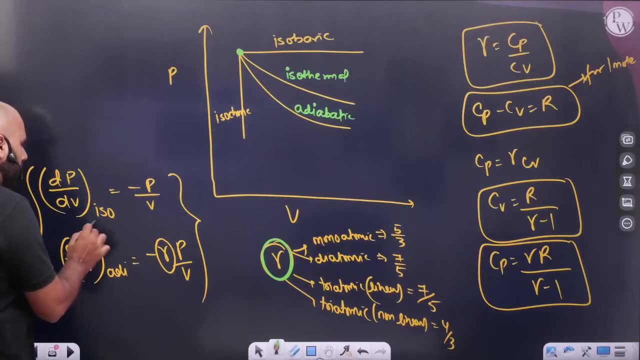 where all four processes are represented together: Isothermal, adiabatic, isochoric, isobaric. This graph is important. Rest see the values of gamma DP by DB. Isothermal's slope is this: Adiabatic's slope is this: 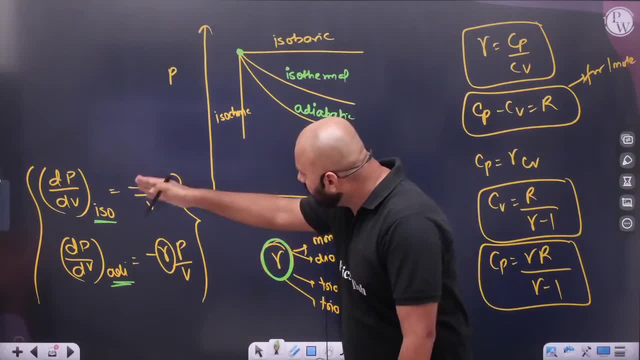 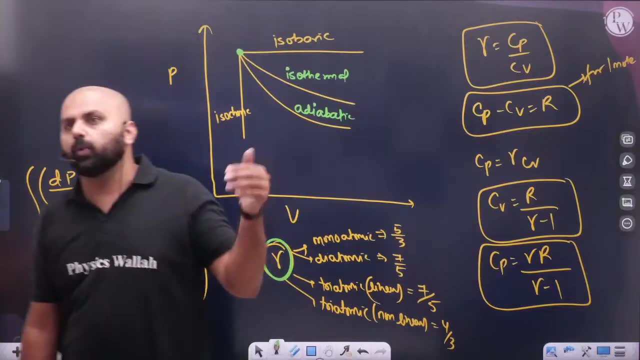 Gamma always. What will happen to adiabatic? Adiabatic will always be below Because it has a negative slope. It will be more negative. It will be more negative than that. Okay, So isothermal will always be above. 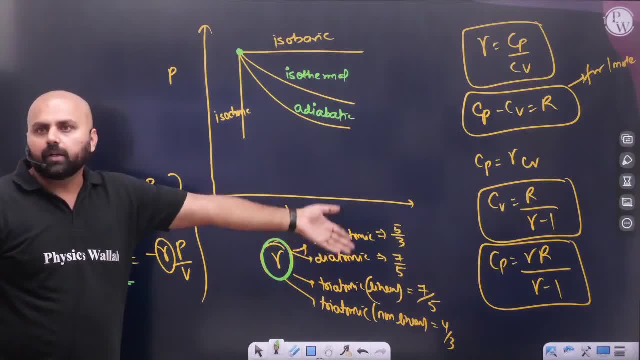 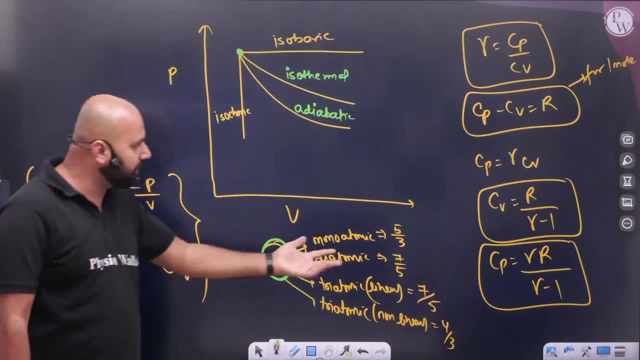 Adiabatic will always be below. So this is the formula sheet. Okay, This is the formula sheet. Keep doing this. Okay, Keep this in your mind. It will be a different formula sheet again and again. I am giving you all the important information today. 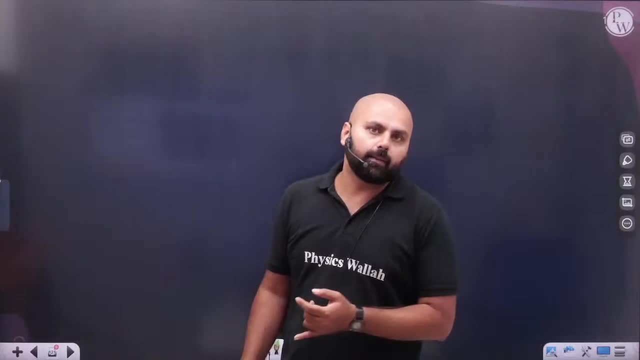 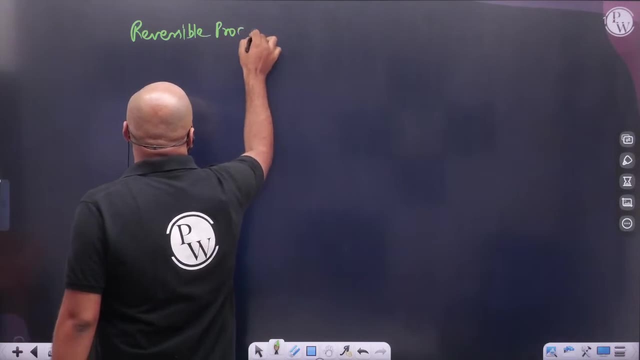 Okay, Keep doing this. Okay, Then I was told that gamma is there. Now there are two more processes here. One is called reversible process. Remember, there is a reversible process And one is irreversible process. Irreversible process means: 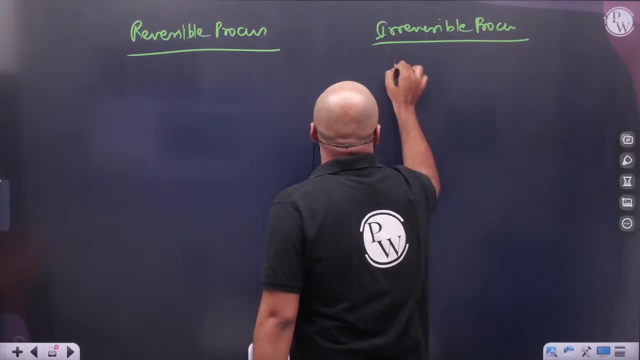 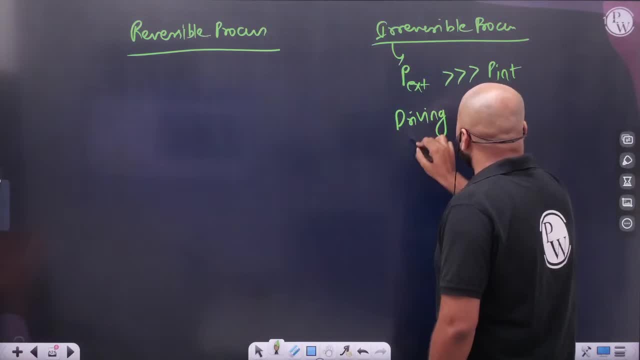 What will happen to the driving force? It will be very strong. From which? From opposing force. What will happen to opposing force? It will be strong Means. it will happen in one jhatka. This is the real process. It happens in finite time. 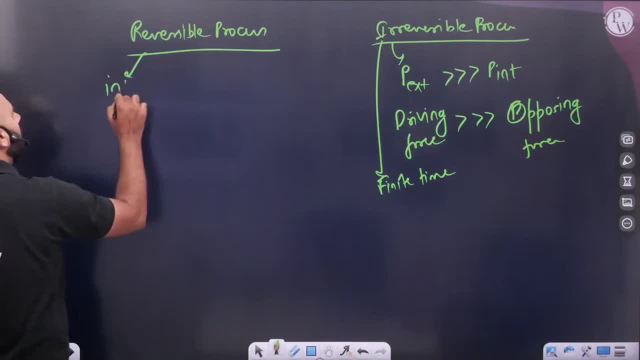 Irreversible. But what is in reversible? It will happen in infinite time. Why will it happen in infinite time? Because this is the ideal condition. It is not possible in real life Because, according to them, external pressure is almost equal to internal pressure. 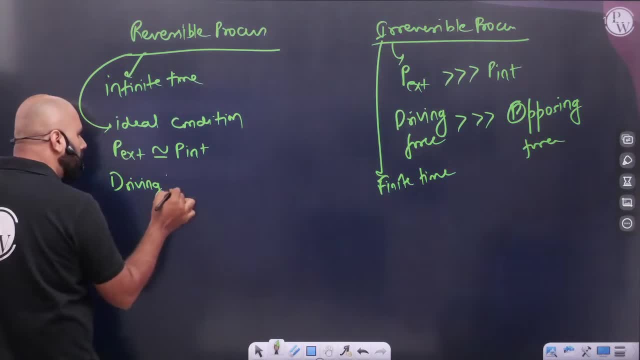 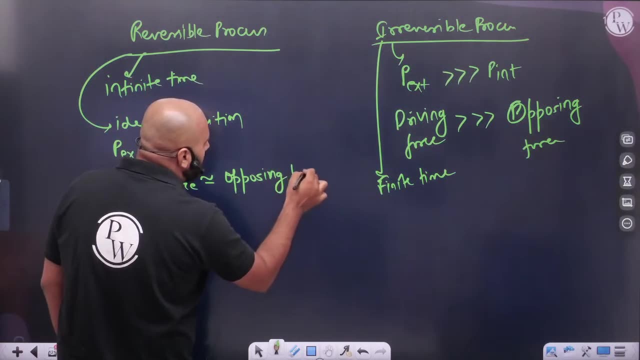 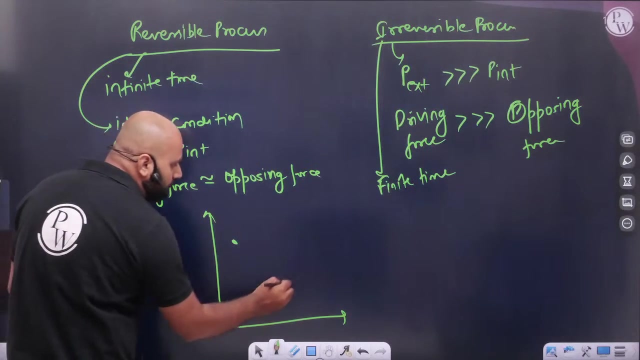 The driving force is almost equal to opposing force. That's why it is called opposing force. Remember, whenever someone tells us if there is an isothermal expansion, There are two ways of expansion. I have to go from here to here. Do you know what an irreversible person will do? 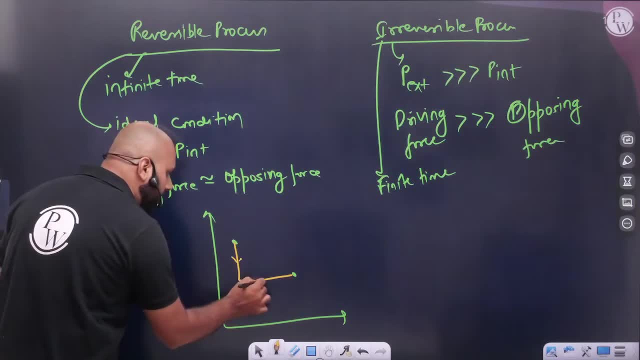 See, Irreversible person will do expansion like this, But the same reversible person will do small steps like this. Where will it go? It will go down. Whose graph is this Of reversible? Whose graph is this Of reversible? 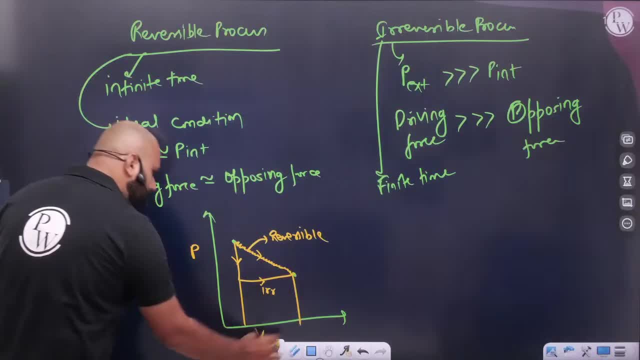 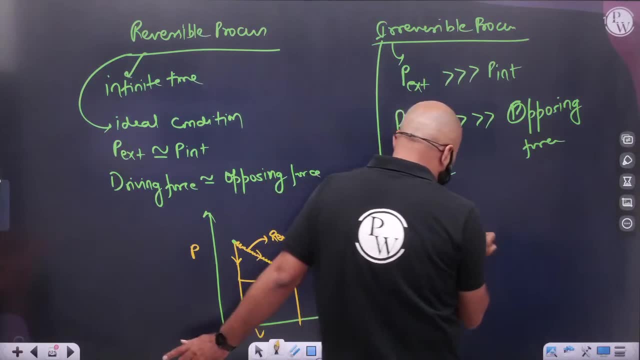 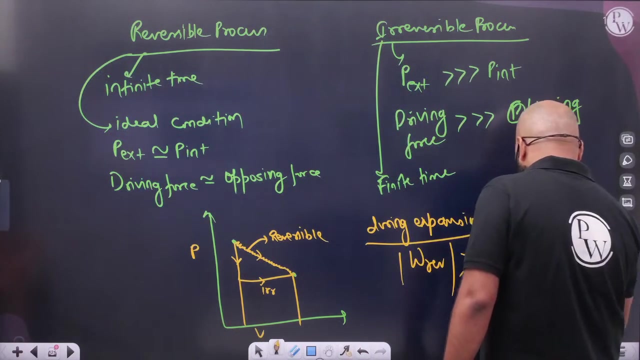 But whose graph is this Of irreversible? Whose work done is more? If we ask, during expansion, Whose work done is more, in expansion, Remember work done of reversible will be more as compared to work done of irreversible. See What will happen in work done. 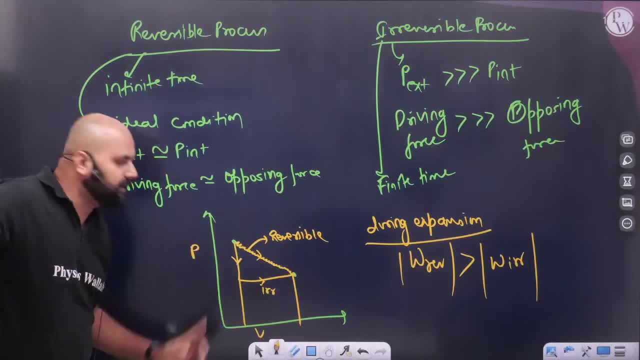 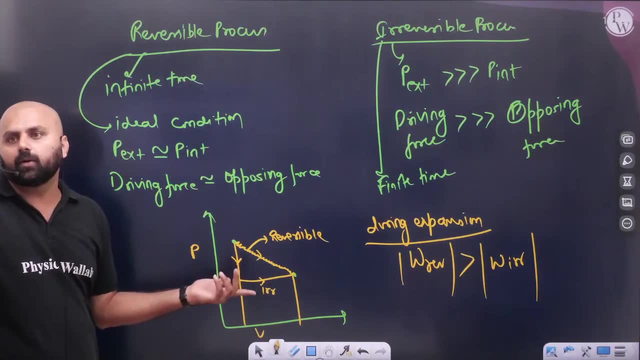 What will happen in irreversible? It will go slowly from here to here. In reversible, it will decrease slowly. What will happen in irreversible? It will come in a flash and go from here to here. Do these things? What will happen in reversible? 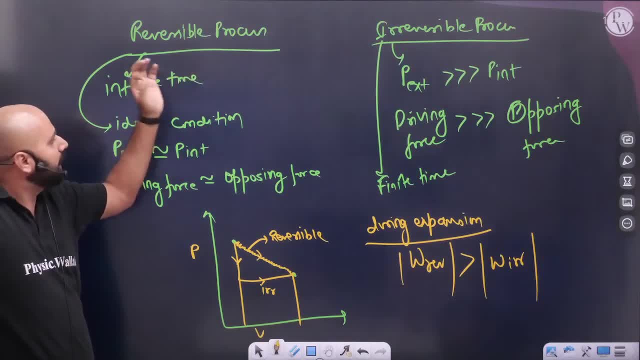 What will happen in reversible? In reversible it means it will happen in infinite time. It does not happen in real life, But, yes, we will assume that whenever we have an ideal condition, Keep one thing in mind: in reversible, Equal the external and internal. 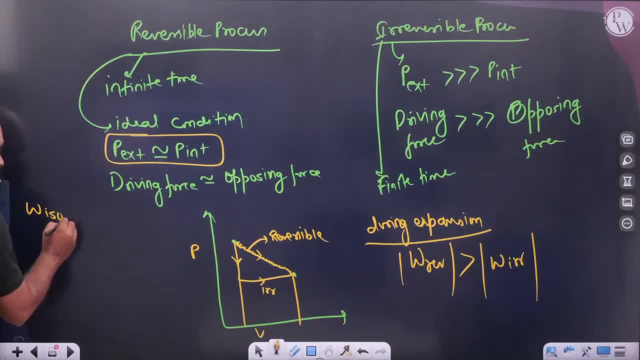 And that's why, work done, the isothermal reversible that comes out. how much does it come out? If I talk about it, then NRT, LN, V, final upon V, initial. Let's derive this: After this work, NRT comes like this: 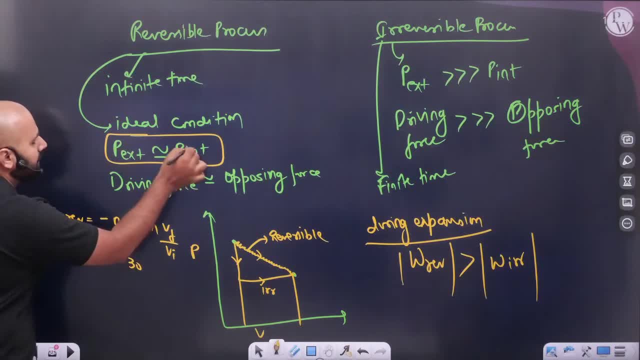 Or, if you want to write it, then using this, P external, P internal becomes equal And if we put the ideal gas equation, then we get this formula. This is what happens in work done isothermal, Obviously what happens in work done isothermal. 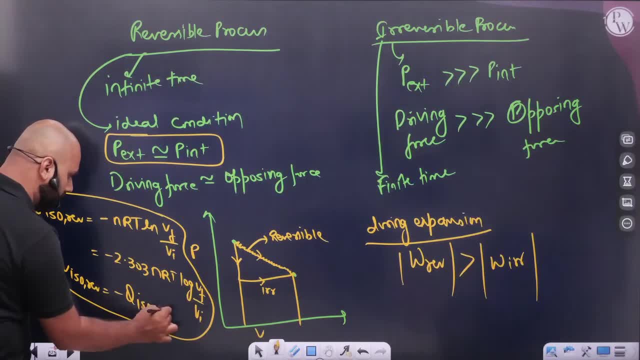 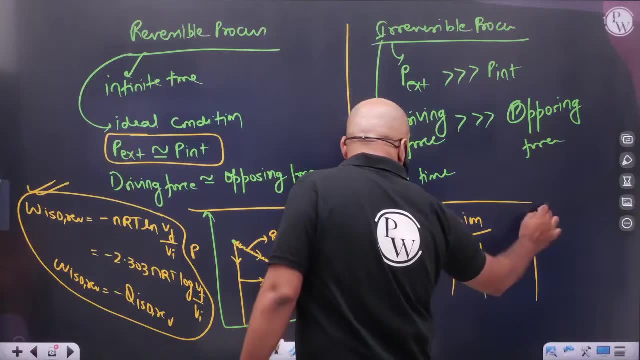 What happens there? Minus of heat, isothermal becomes reversible. So we have to derive this formula In reversible and irreversible. remember things graph wise, That such things also come in the graph. If you do expansion, the magnitude of reversible will always be more than irreversible. 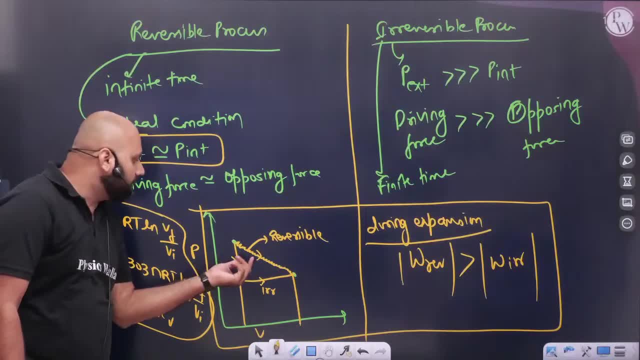 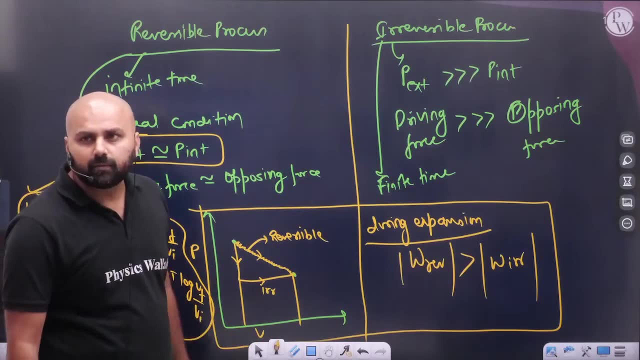 Okay, If graph will reverse, then we will take that side. We will take area under that side. We will take area under the curve on that side. Okay, Opposite will go in contraction. Opposite will go in contraction. Contraction will not come in your life. 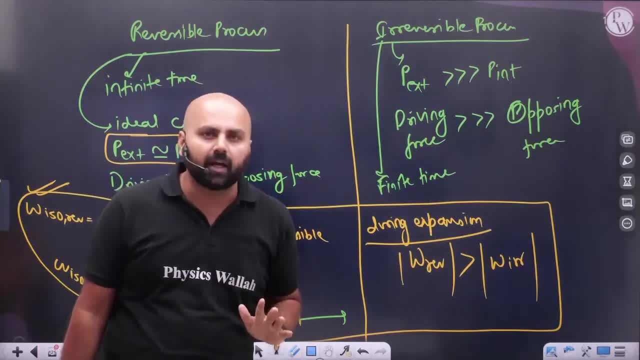 Now, the exam is near, so you don't have to study anything Now. you have to study only that which will come in the exam. Okay, The useless things which you have to study, which you have to study a lot, all of them are studied in batch. 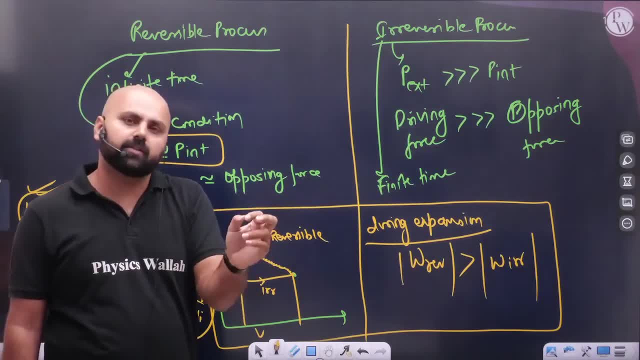 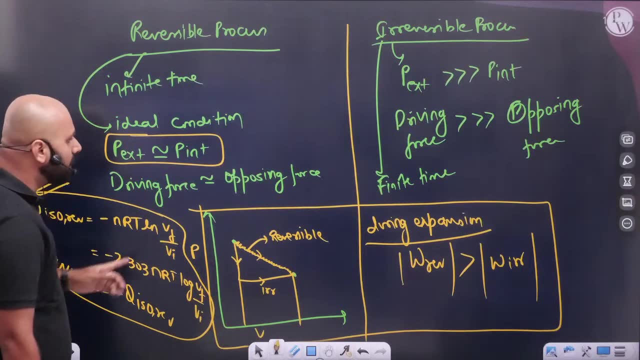 At this time, you will study only those things. It is a simple thing. You will study only those things which will come in your questions. Okay, Yes, Come on, I will give you a break Now wait. See, So I was saying that. 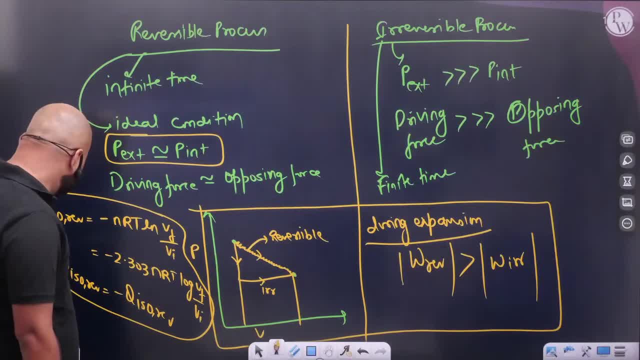 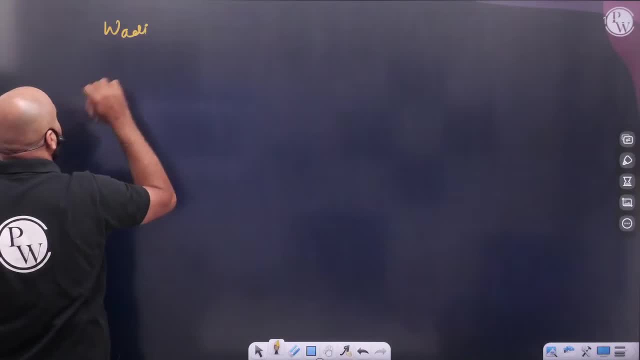 I was talking about expansion and contraction. I was talking about reversible and irreversible Like. suppose there will be a question given here. One more thing: How much work done adiabatic will be Work done, adiabatic? First tell me about the adiabatic process. 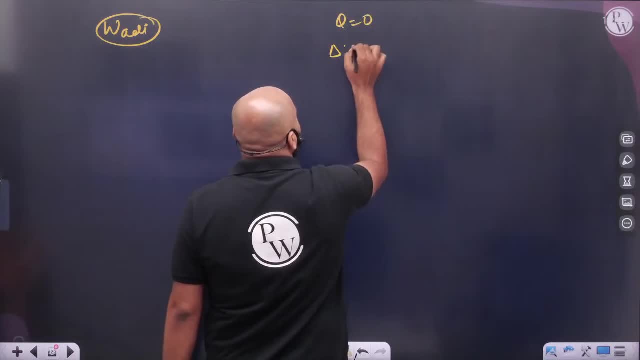 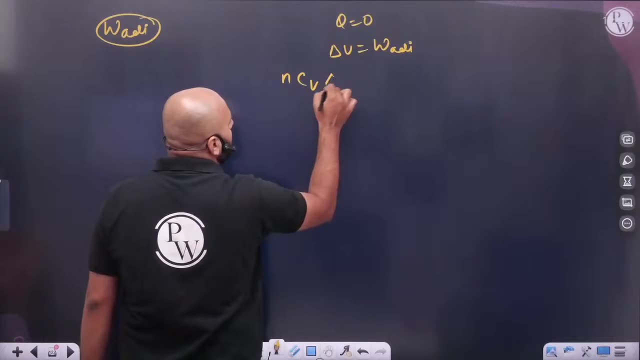 In adiabatic process Q0.. Q0 means whose delta U is equal to Whose delta U is equal to Work done. adiabatic. Sir, look at the adiabatic. What is the formula of delta U? 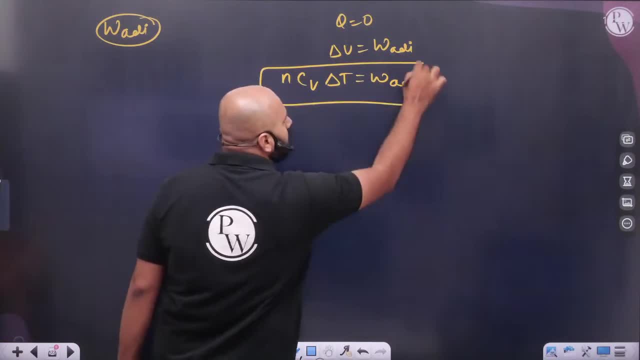 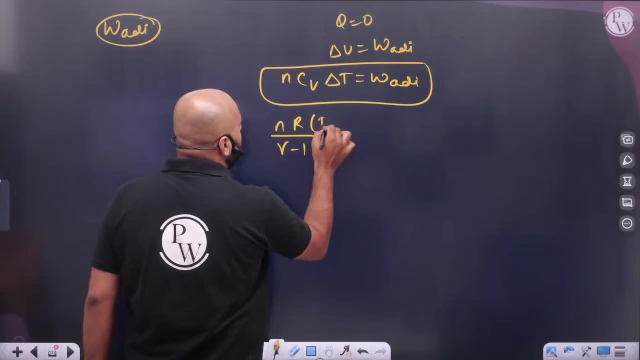 NCV delta T, So adiabatic work done will be equal to this first. Or if I say, what will I put the value of CV Gamma minus 1, and here T2 minus T1 will be put. 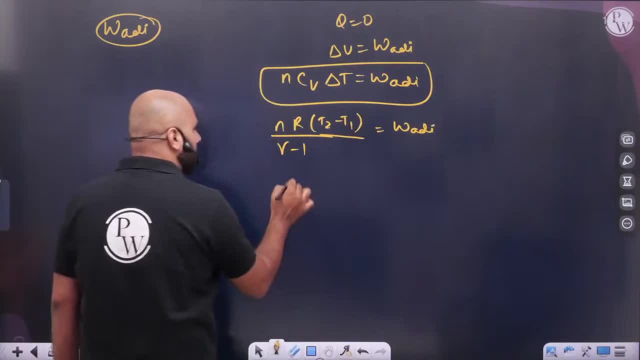 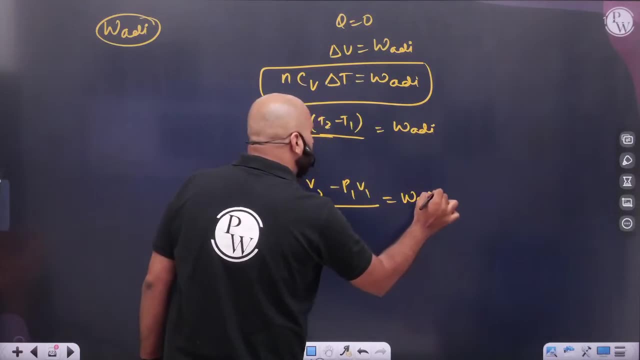 So what will come here? Work done, adiabatic. And if I want P2, V2 minus P1, V1 upon gamma minus 1 is equal to work done- adiabatic. Remember, two people in the world put this work done. 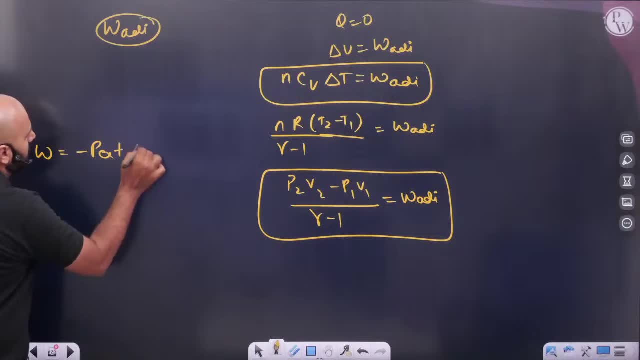 everywhere Rest. put this work done everywhere Minus P, external delta V. This will be valid everywhere. Work done is different in adiabatic case. And one more thing: Work done is different in isothermal reversible. Apart from this, 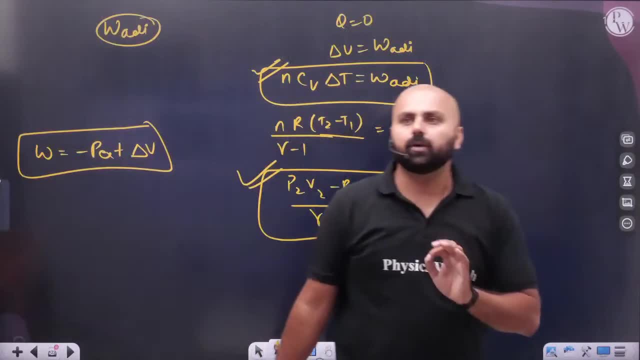 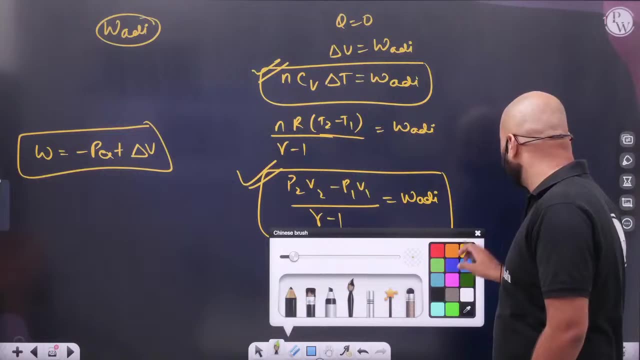 close your eyes and put the formula of P delta V everywhere. Put the formula of P delta V and then do it. Okay, Put the formula of P delta V and then do it. It will be done. These small things Do the work. done like this. 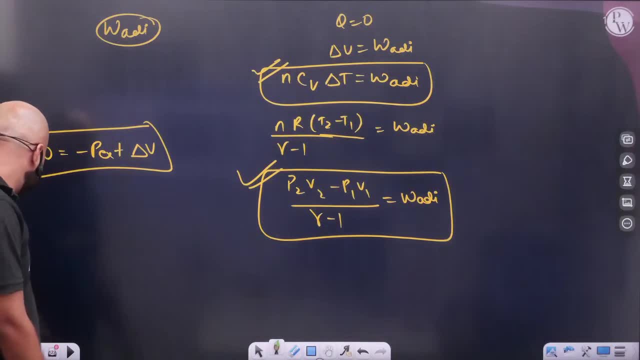 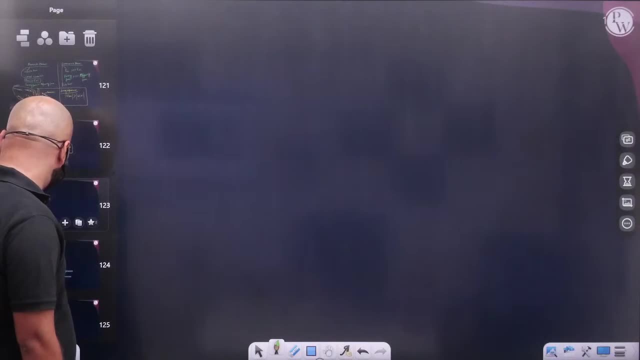 Okay, Okay. After that someone told me that, sir, let's do one thing. Work done is done, Adiabatic is done, Reversible is done In thermodynamics. now let's go In thermodynamics, look. 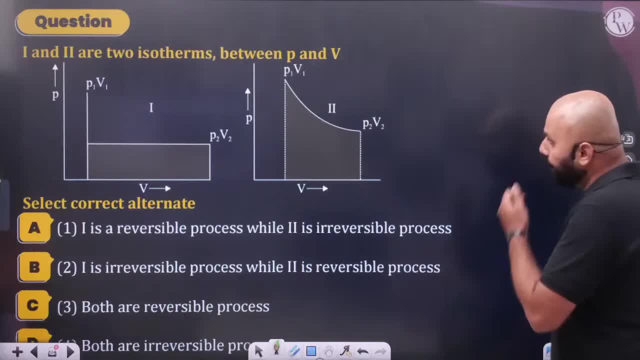 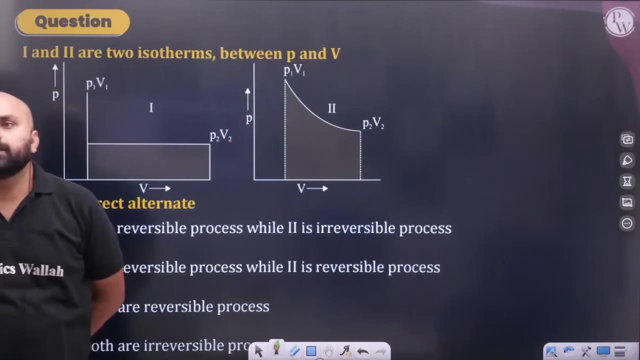 you have a question. Look at this question. Tell me which one is reversible, Which one is irreversible. Attempt the question. Attempt the question and see What will happen. Tell me quickly. Tell me quickly What will happen. How much will it come? 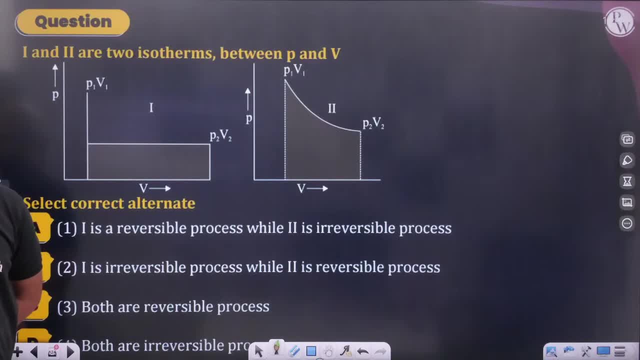 Which answer will come in this, Sir? this is a simple thing. What is this? It is irreversible. And what is this? It is reversible. What is one Irreversible? What is the second Irreversible process? It is a graph of P versus V. 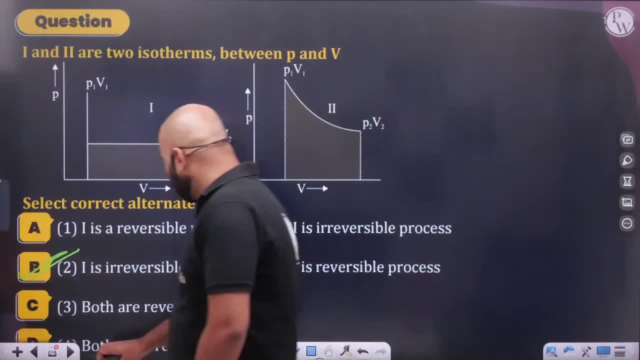 It is a graph of P versus V. Keep recognizing, Sir. look at the next question. Look at the next question In this reaction: delta H minus delta U. Delta H minus delta U. First, what is the formula of delta H? 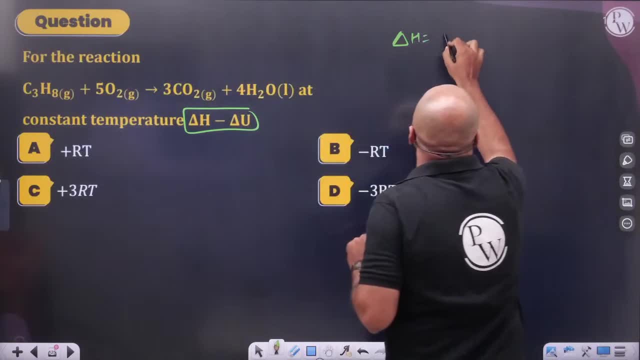 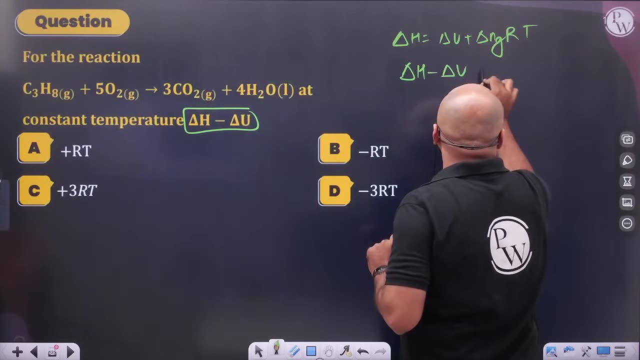 Sir, if you want to try, do it quickly. What was the formula of delta H? So delta H minus delta U is delta NG RT. This is the formula of delta H. So delta H minus delta U is delta L. 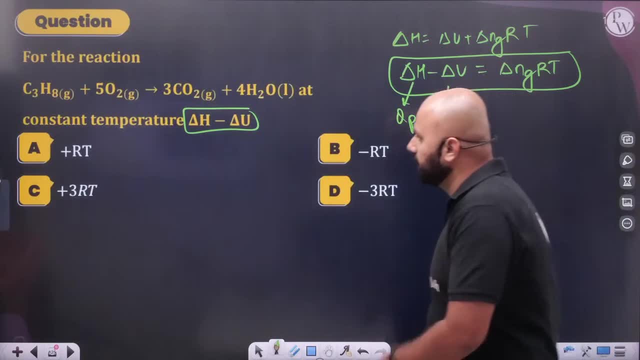 If you want, you can write it as heat at constant pressure. If you want this, you can write it as heat at constant volume. Take it out. What will be the answer? What will be the answer? Tell it fast. What will be the answer. 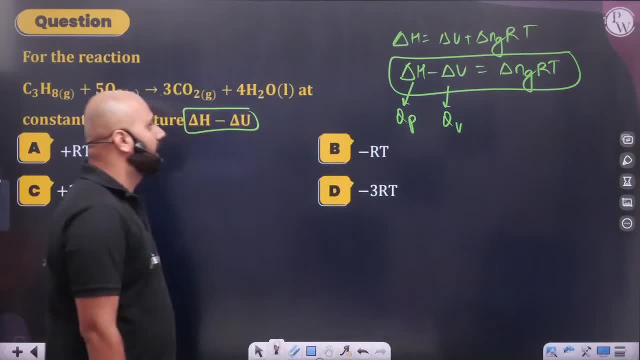 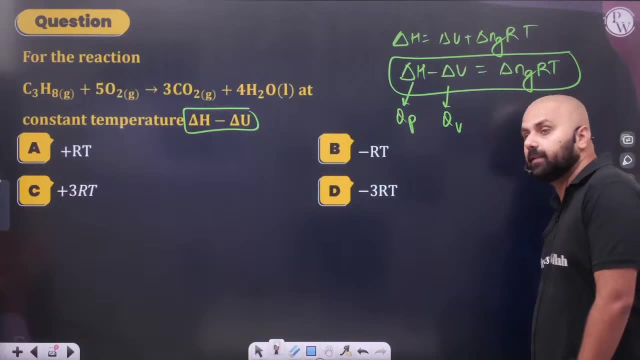 Fastly. What will be the answer? Do not take the liquid. Delta NG means gaseous moles of product, minus reactants. We have to take gaseous moles. We have to take the gaseous moles of reactant. 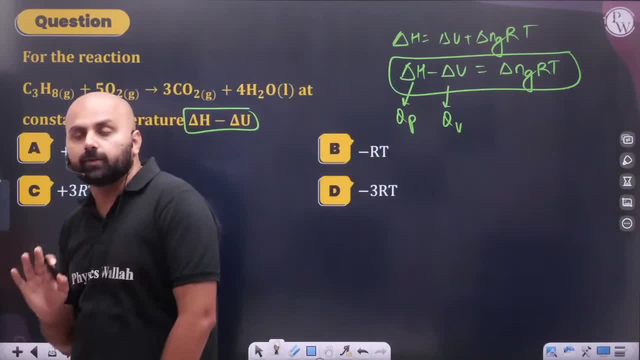 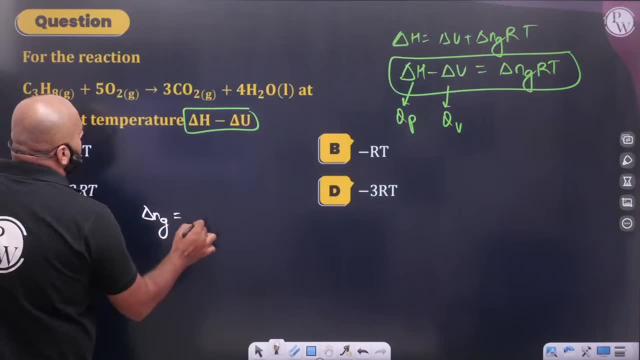 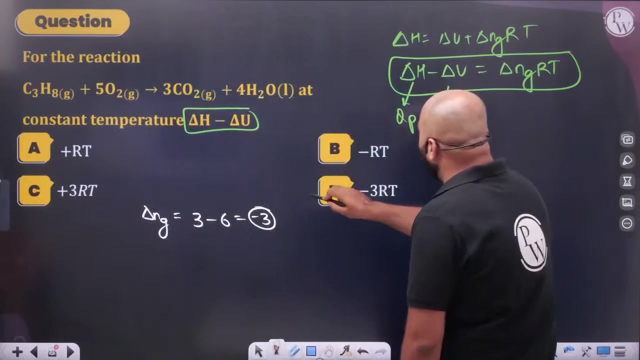 the product. Don't take liquid moles by mistake. In the case of delta NG, delta NG is 3-6. how much will come minus 3 delta H? how much will come minus 3 RT? what will come to us? 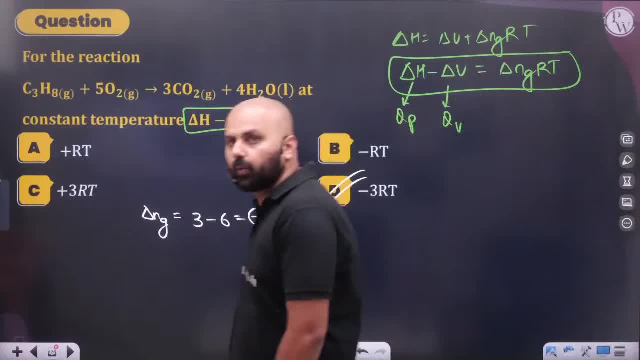 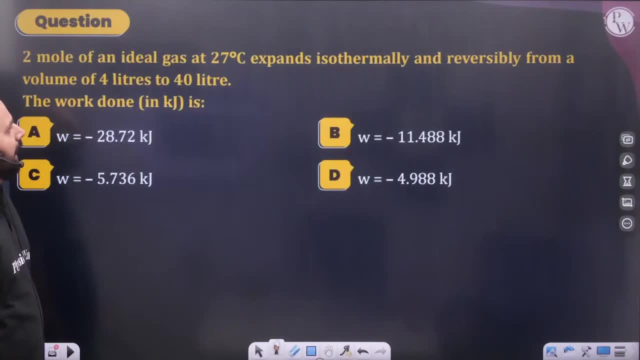 minus 3 RT. product minus reactant. product minus reactant. ok, see isothermal reversible volume: from where to where: 4 litre to 40 litre. isothermal work done. I told you isothermal reversible work done. what will happen? minus 2.303 NRT. 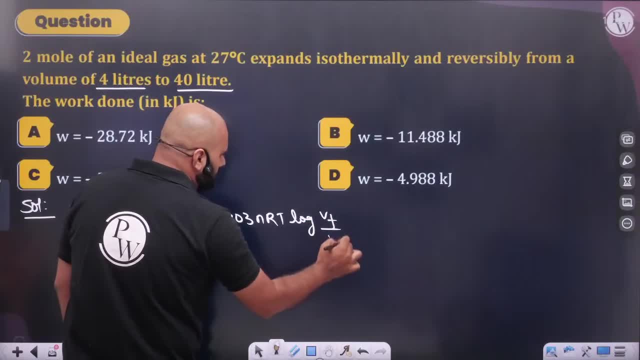 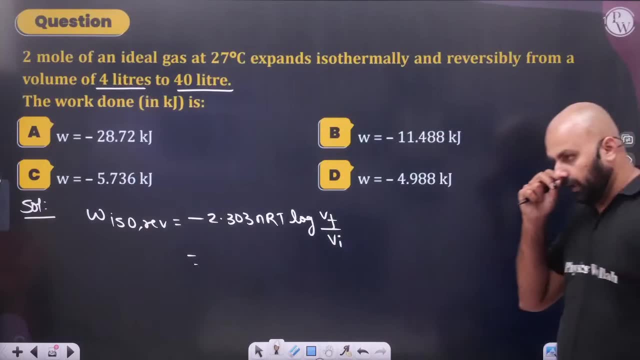 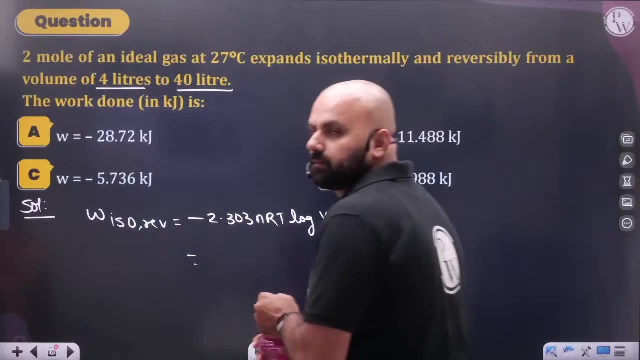 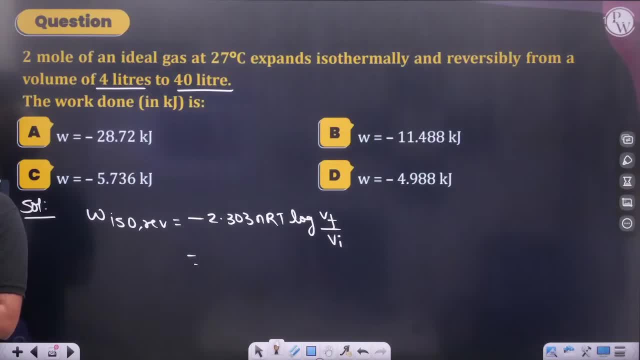 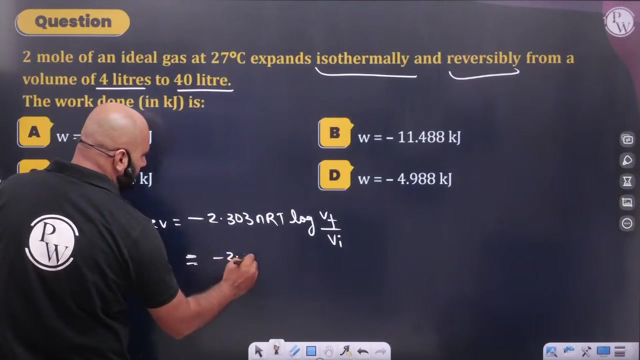 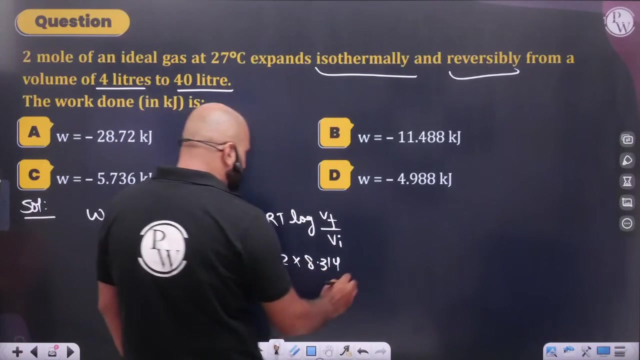 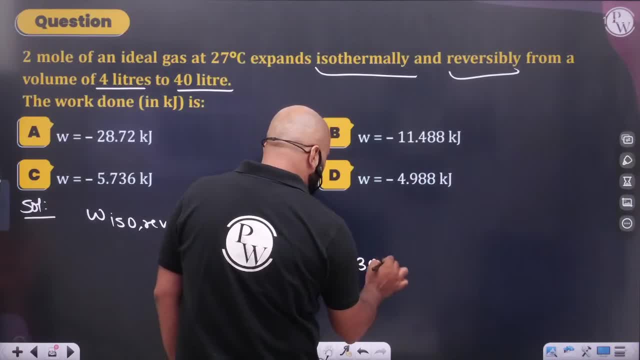 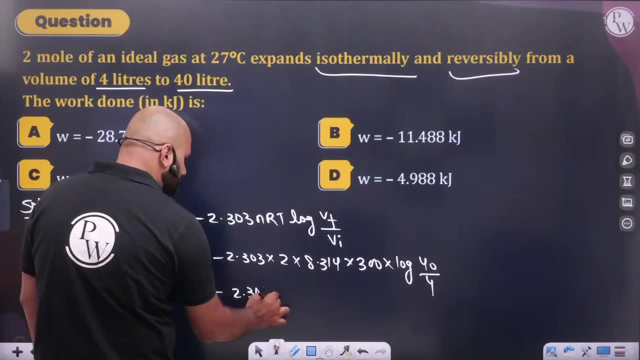 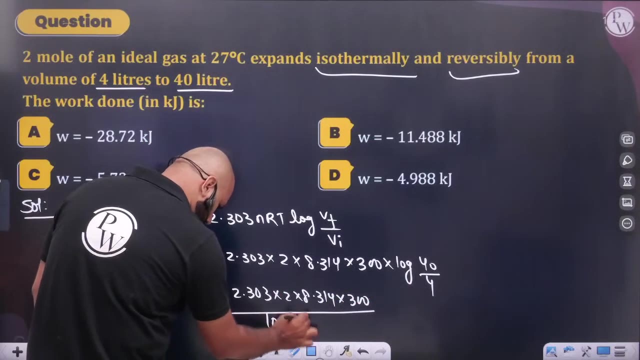 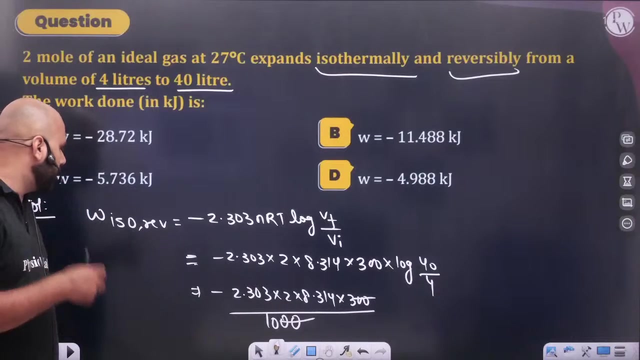 temperature 300. log V, final upon V initial. Y40 minus 2.303 into 2, into 8.314, into 300. this is in joules 1000, 1000, how much will it be? 3,, 25,, 50. 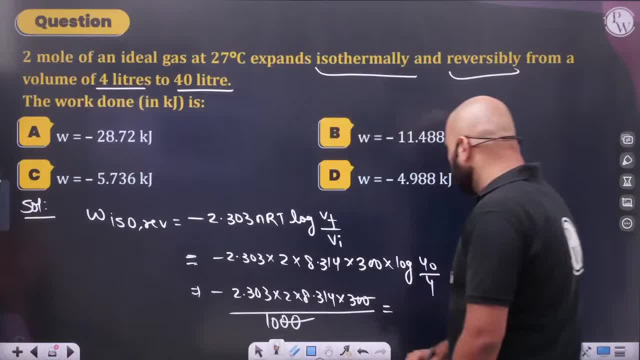 how much is it? if I solve it correctly, how much can I do in exam hall? minus 4.606 into 8.314, into this is 3 by 10, so I will make it 0.3. how much will it be? 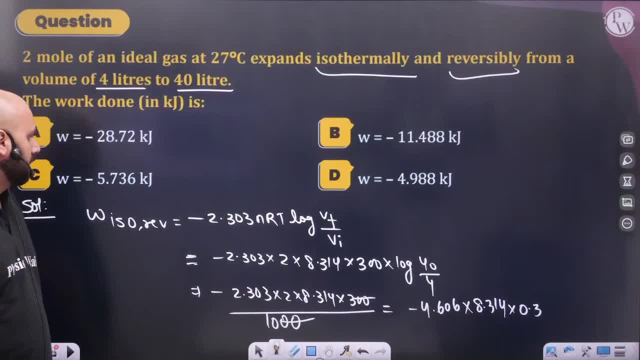 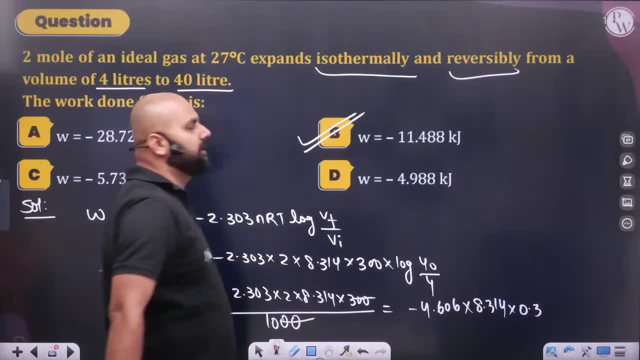 8400, 3230. 32 and 1 by 3, 0.3, 32 by 1 by 3. what will be the answer? B answer. how much will be the answer? B answer. how much will be the answer? B answer. 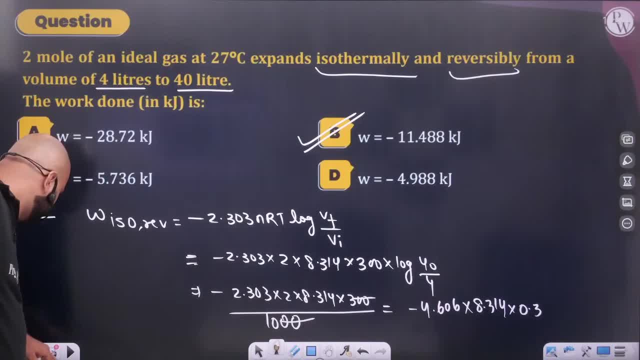 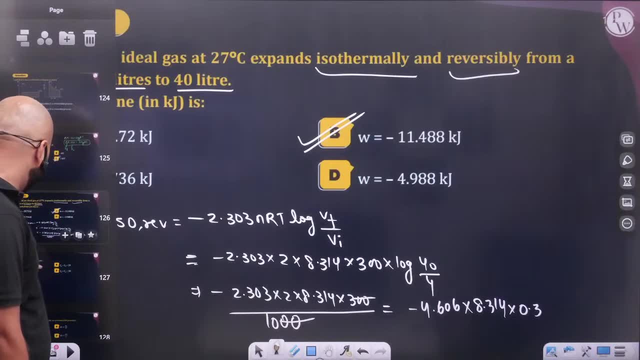 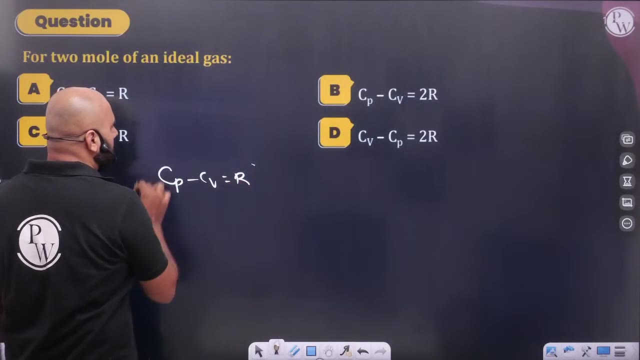 keep doing, it will be done. 25 by 3 will also be done, but I took 0.06. ok, see this. CP minus CV. CP minus CV is equal to R. this is for 1 mole and here CP by CV. CP and CV is heat capacity. 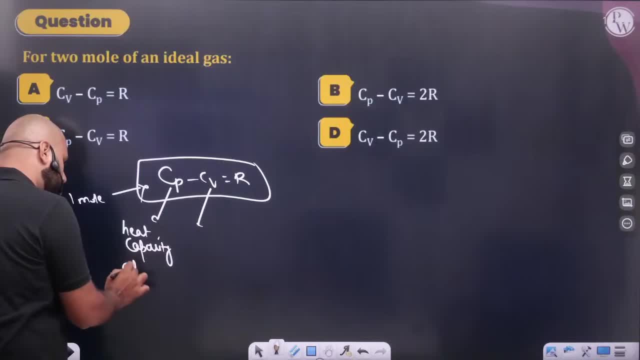 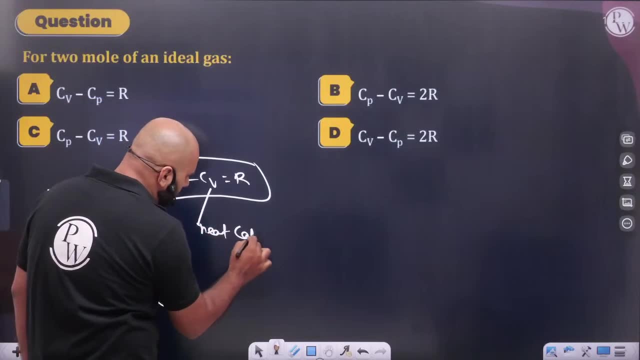 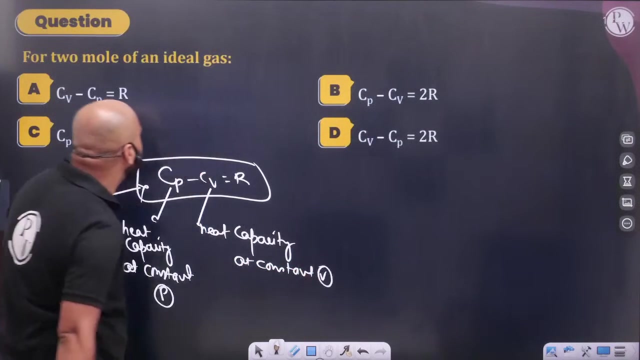 this is heat capacity. heat capacity at constant pressure, at constant pressure. heat capacity at constant pressure. and this is heat capacity at constant volume. heat capacity at constant volume. remember the difference in both, but for 1 mole. how much will it be for 2 moles? 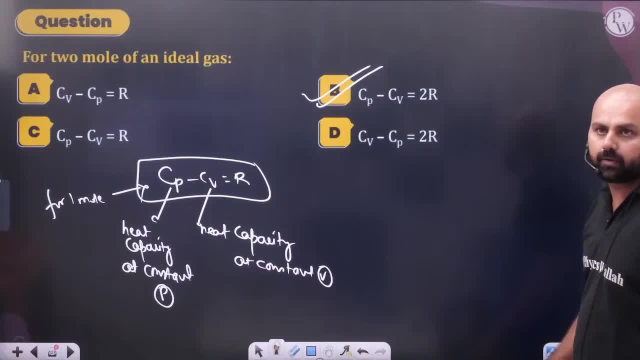 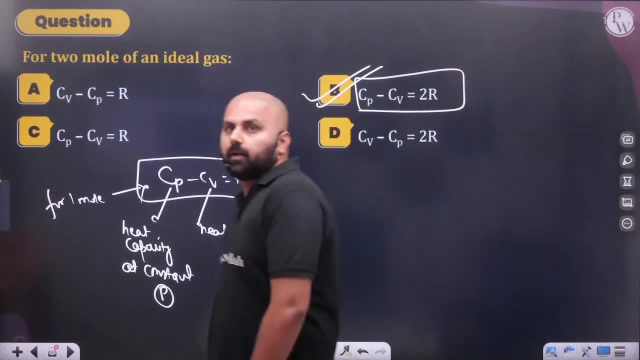 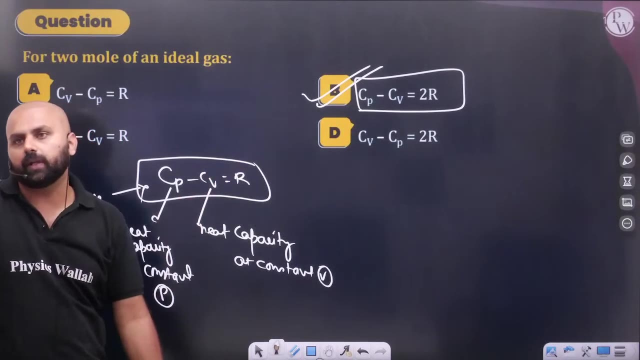 what will be the value of CP minus CV 2 times R? what will be the value of CP minus CV 2R? what will be the value of CP minus CV 2R? for one mole, 2 is R. what will be the value of Obvious? 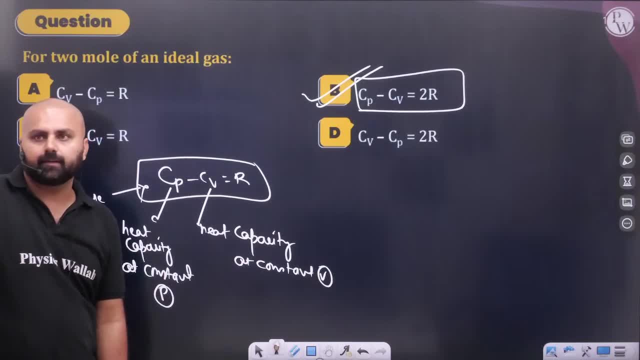 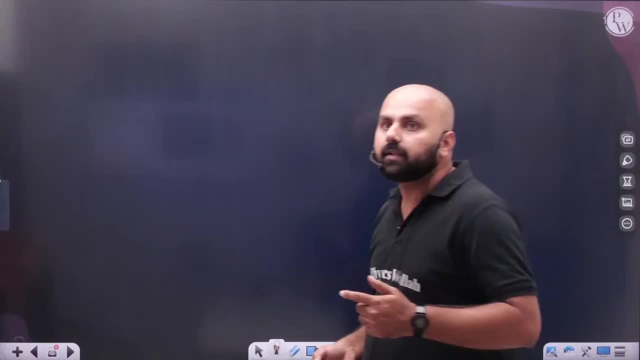 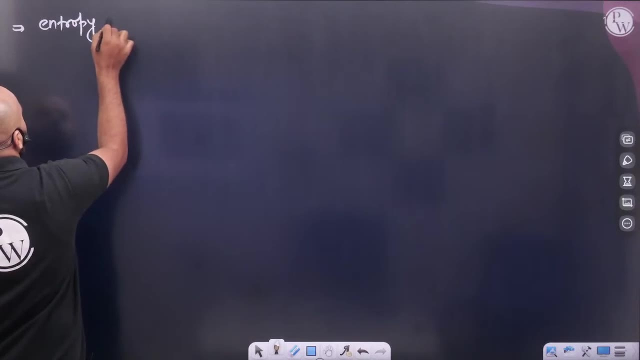 2 times R, 2 times R B. answer: now see, I have Enthalpy. we have read basic things. now comes a new. Before moving to the second law of thorn axe, there is a word that is known as Entropy. What is Entropy? 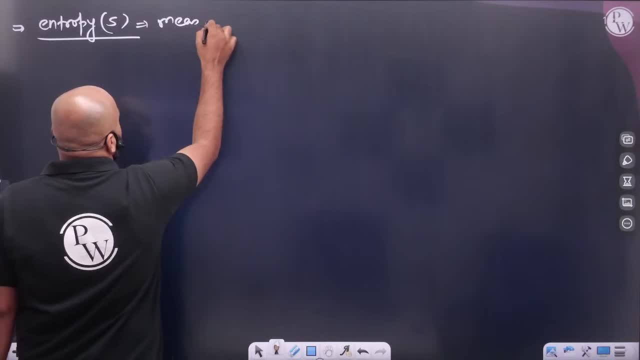 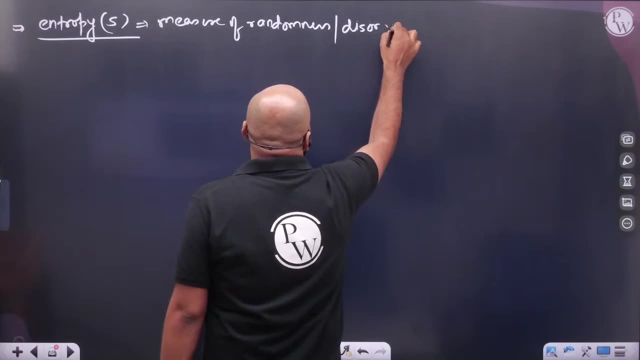 It is nothing. it is randomness, measure of randomness or disorderness, randomness or disorderness. It talks about randomness or disorderness, the more disorder there is. if we talk about Entropy, if someone asks about Entropy, then who will have the most Entropy? then the most? 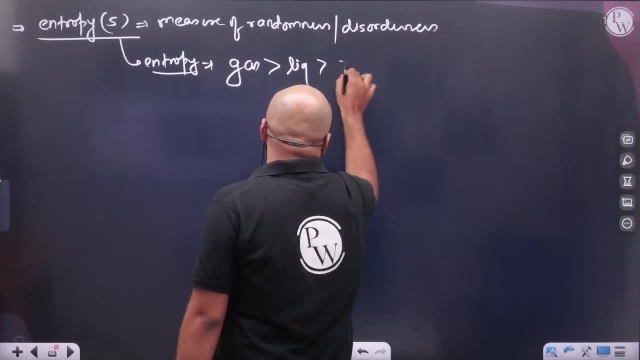 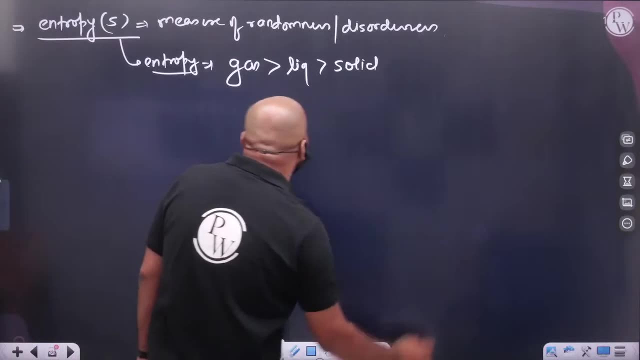 gas. if we talk about normal case, then liquid, and then what will happen? solid Entropy is nothing, it is a method of measuring randomness. again it was there. see, see again with us, see again. Entropy again is a state function. again it is a state function. Entropy. 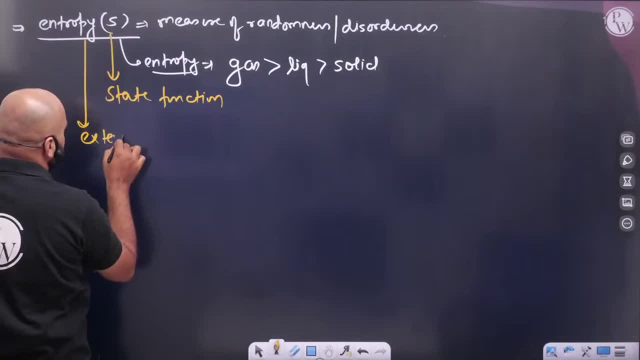 is a state function. it is an extensive property. Entropy is an extensive property. Now, if you see here, then what is going to happen? if you see here, then what is going to happen, Sir, the delta S that is measured, that delta Q by T comes for reversible process. 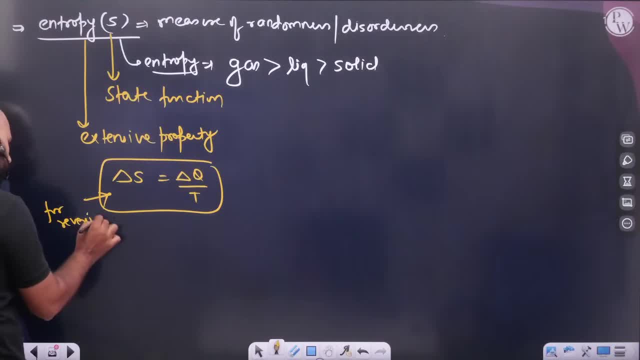 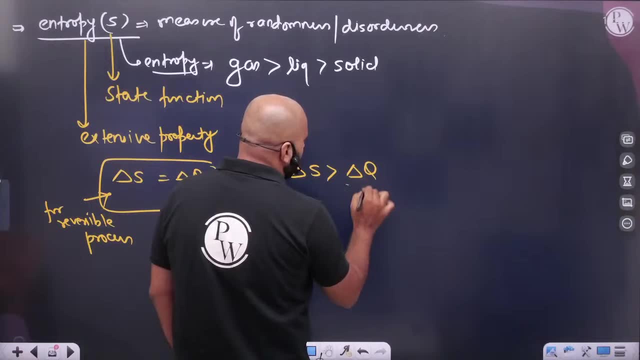 for reversible process. If it is a reversible process and if it is irreversible, then it will always come more. if it is irreversible process- it will happen in a jiffy- then it will always come more than this for irreversible process. 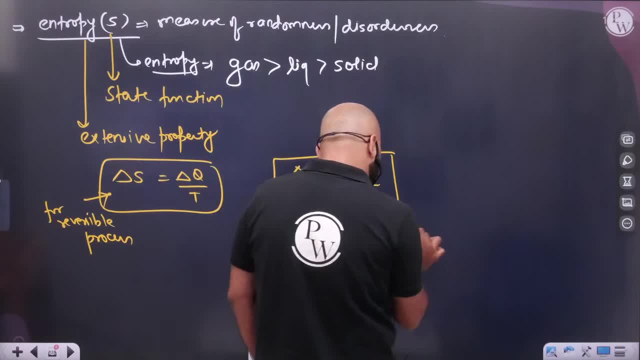 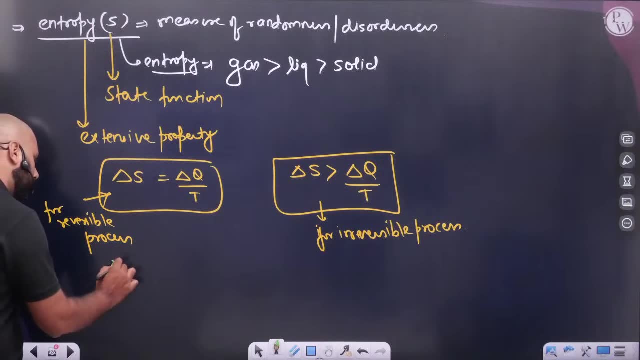 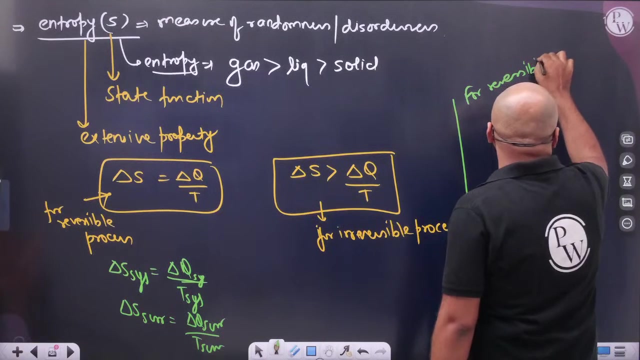 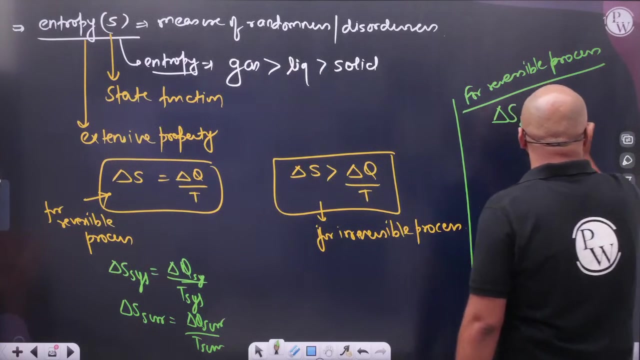 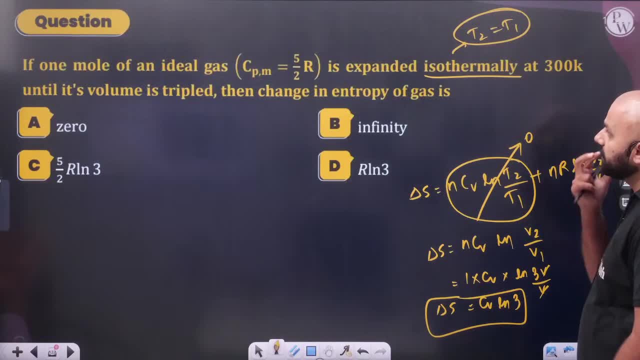 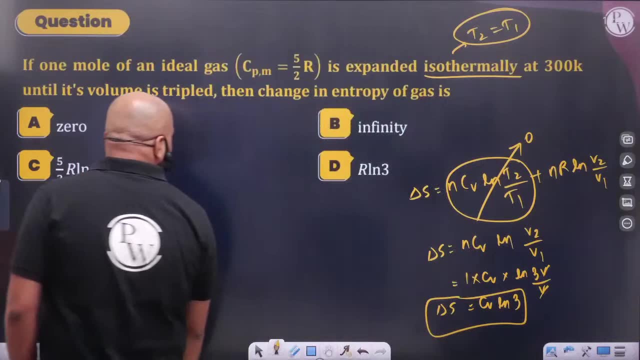 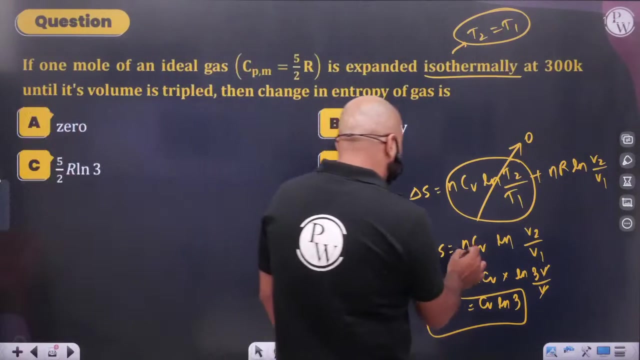 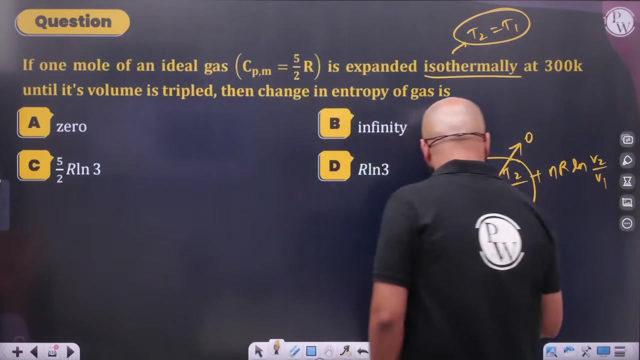 Thank you. Thank you, How much is the value of nr? Did something go wrong? Oh yes, What did I do? I am saying nr is See, this is what is going on in the mind. nr, This is what is going wrong. rln3. 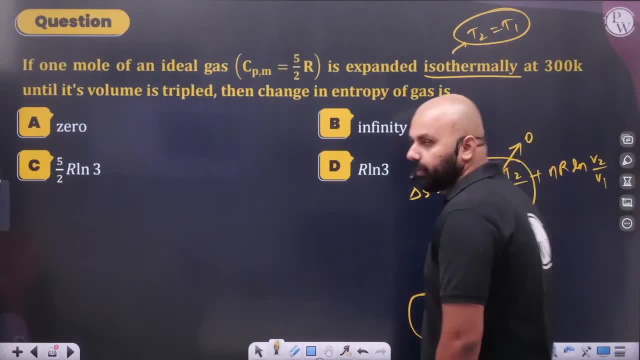 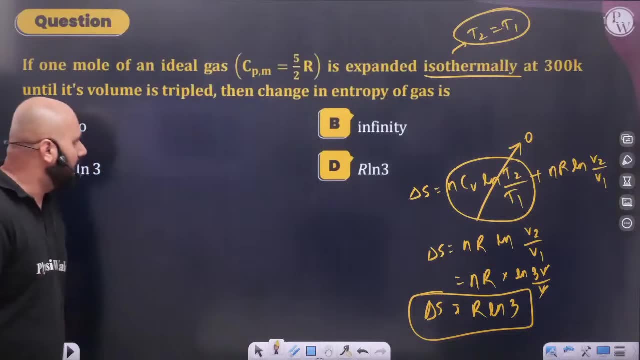 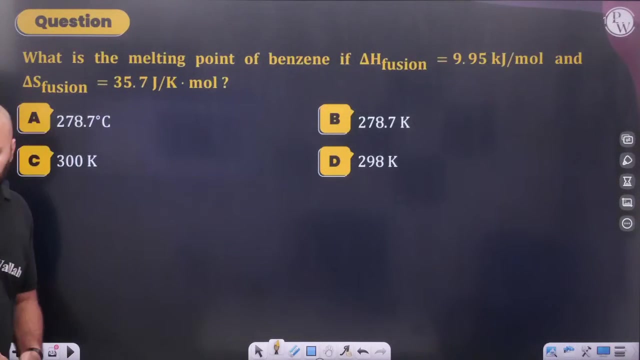 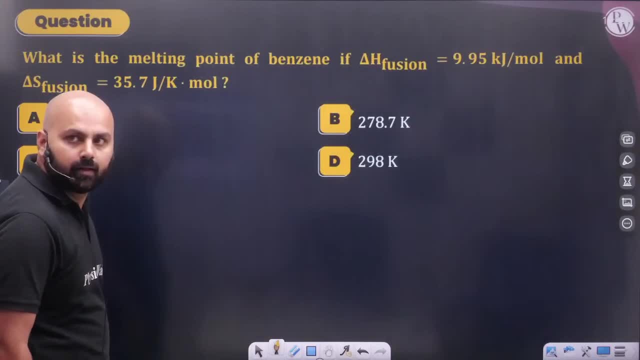 How much will be the melting point? See this: how much will be the melting point? How much will be the melting point of delta H fusion upon delta S fusion upon? Just remember to put in Kelvin. See this: how much is the value of delta S? 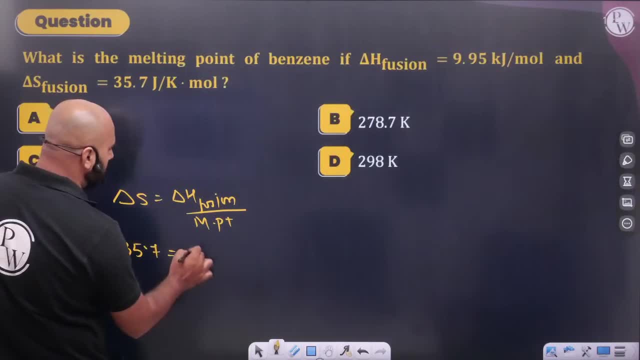 35.7. How much is the value of delta H? It is given in kilo joules. Just multiply it in joules, Just remember the unit dimension. How much will be the melting point, Sir, 9950 divided by 35.7? 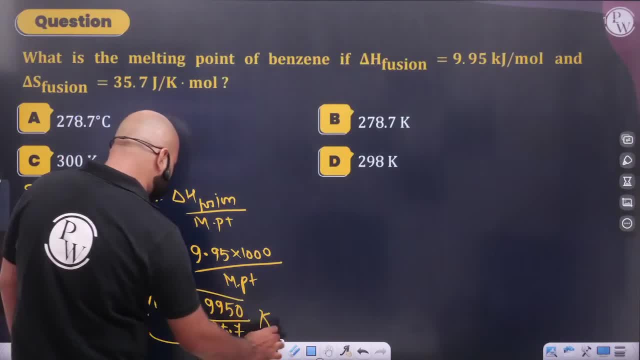 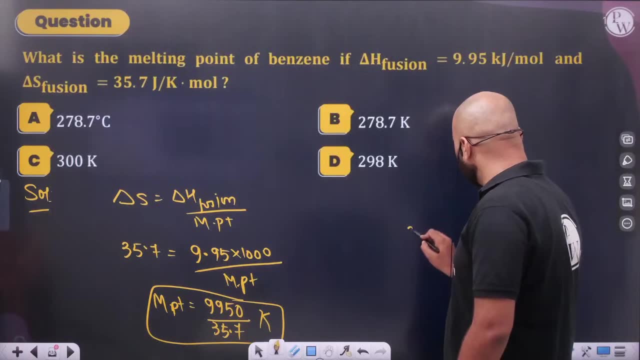 If we calculate this, we will get the answer in Kelvin. How much will it be? It will not be in degree Celsius, It will be in Kelvin. We will have to calculate How much will it be 357 divided by 99500.. 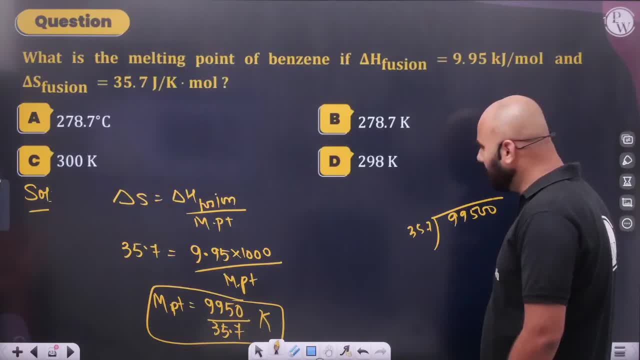 This will be it. How much will it be? Is it B or D? Let's do it with 2.. So how much is this? 14. 5,, 2,, 0,, 10,, 11.. And how much is this? 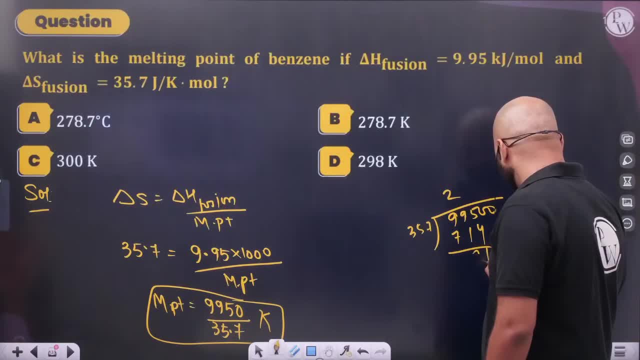 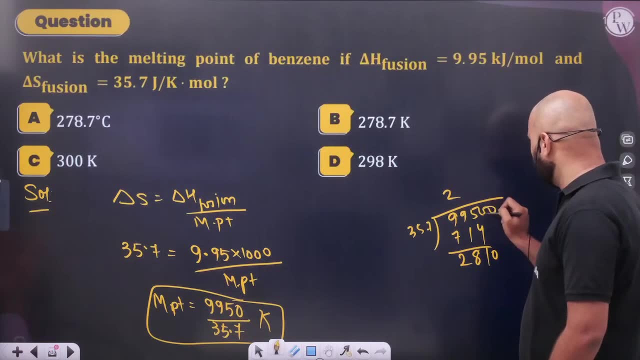 7, 1, 4.. This is 1.. This is 8.. How much is this 2.? This is 0.. So it will not be with 9.. It will be with 7. 2.. 7, 7, 0, 9, 49.. 7, 5, 0, 35, 39. And 7, 3, 0, 21.. And 1, 0, 9, 9.. 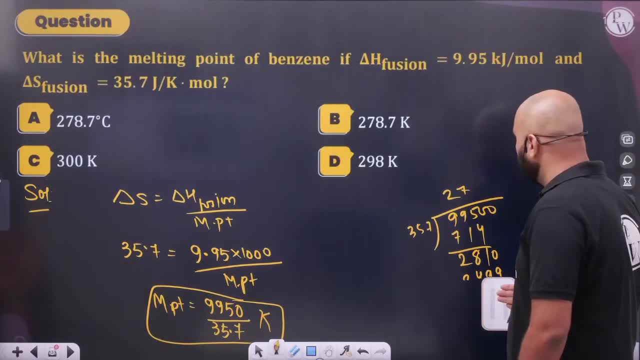 And how much is this? 3,, 3,, 9.. No man, Did I make a mistake? 2, 9,, 9, 500.. Divided by 35.7.. 35.7 goes up. 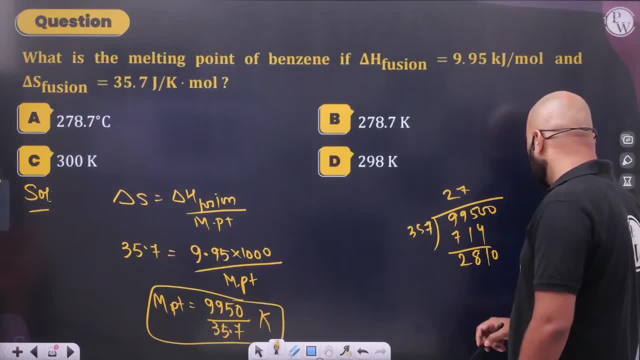 357 goes up. So how much will this be? 7, 1, 4.. This is 1.. This is 8.. 7, 2, 9.. Okay, Let's do 7, 7.. So 7,, 7,, 0,, 49.. 7, 5,, 0,, 35. And 9, 39.. 7, 3,, 0,, 21.. And 21 and 3, 24.. 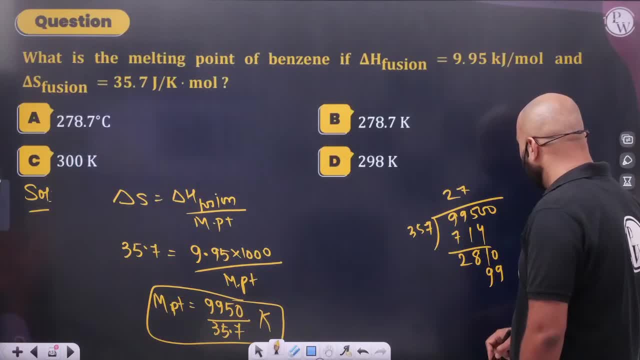 So how much is this One? And this again: 1.. And this again 1.. And this again 2., This again 2.. And this again 3.. And this again 1.. And this again 1.. And this again 2.. 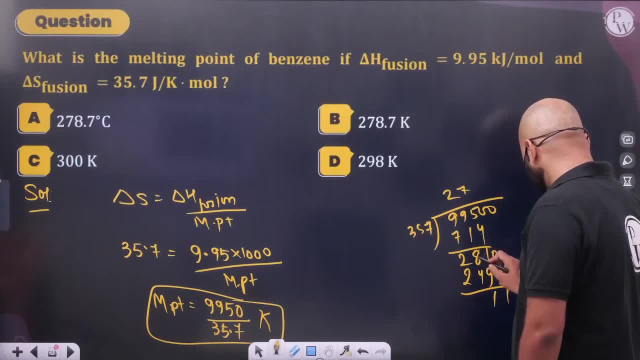 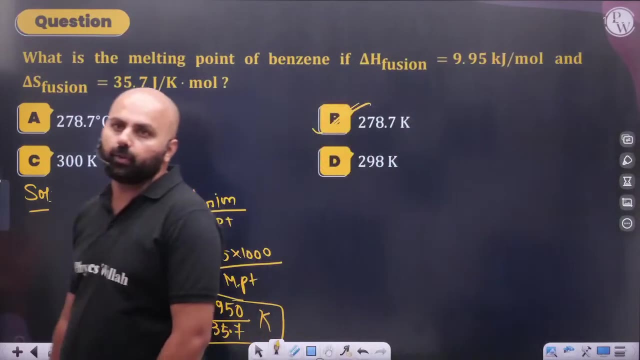 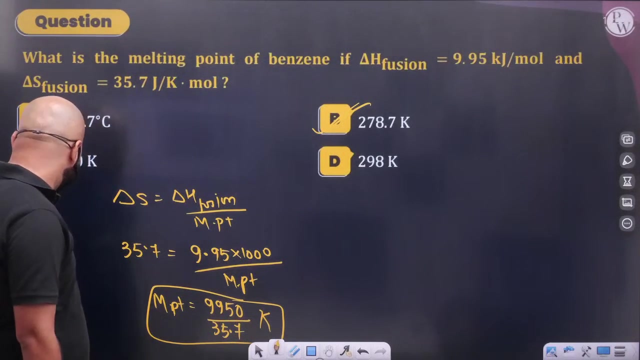 And this again 3.. And this again 2.. And this again 3.. So it will be 278.7,, it will be 278.7,, it will be 278.7,. it will be B option. I have done the calculation. what will be the answer? it will be B option. it will not be D, it will be B option. it will be B option. do it, you will know. do it, you will know. after entropy gives energy function, comes in our life. 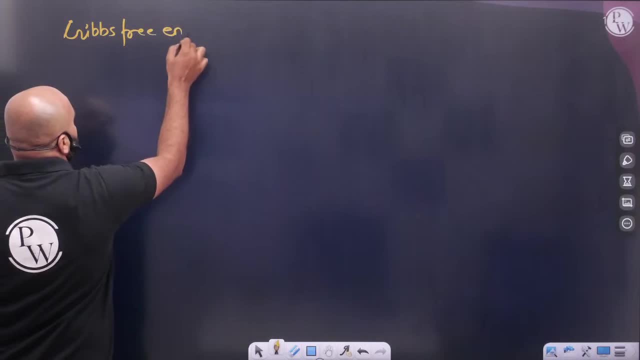 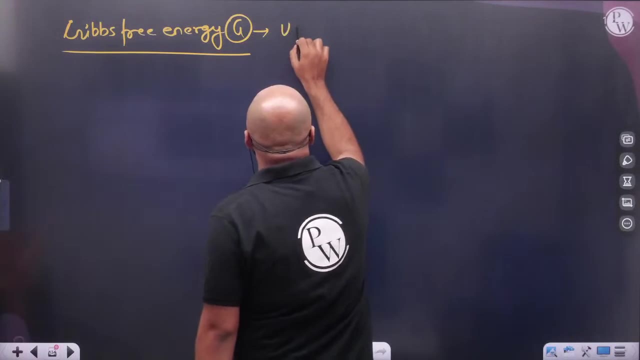 watch it now as we are going to go to the next chapter. so it comes as: gives free energy. gives free energy. what does it tell? gives free energy. tells that bro gives free energy. what is this? This is energy that can be converted into useful work. useful work will be telling that if I talk about G, then G is H-TS. what is G? It is H-TS. and if I want to find delta G, then what will happen? 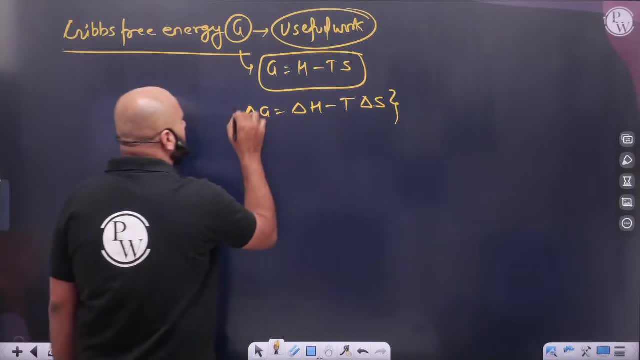 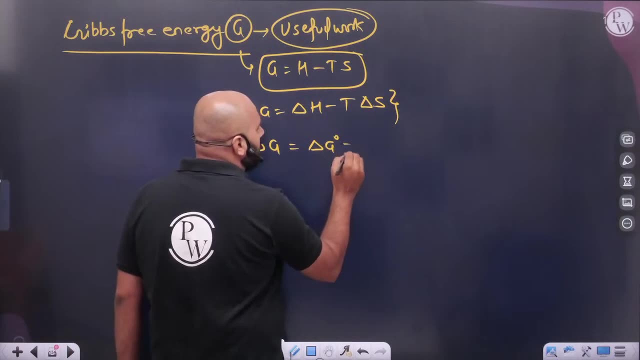 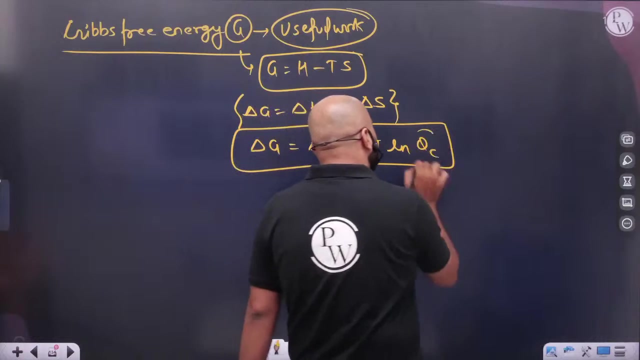 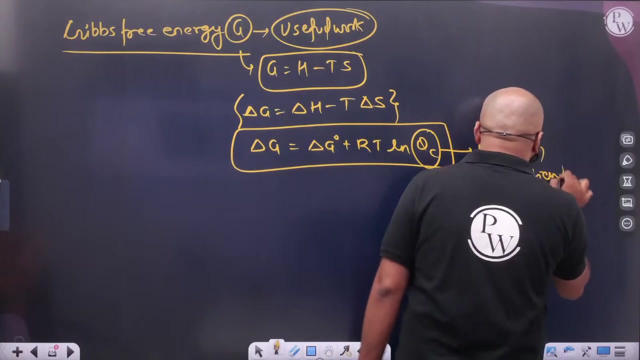 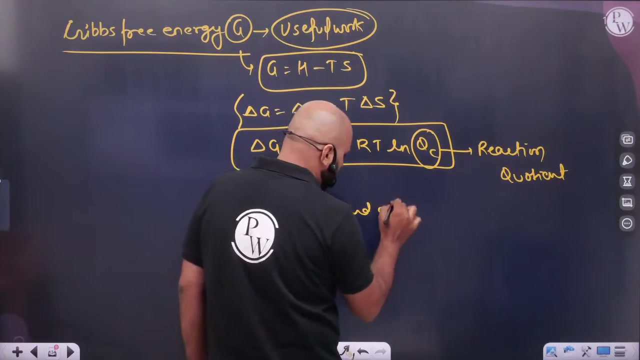 It can be delta H-T, delta S. what is delta G? It is delta H-T, delta S and delta G. I will write one or two formulas together: delta G, naught plus RT, ln, QC. from here this chapter is converted into equilibrium, where QC is known as reaction quotient, where QC is known as reaction quotient. and if I talk about delta G, delta G naught, then we call it standard Gibbs free energy. we call it standard Gibbs free energy. we call it standard Gibbs free energy. 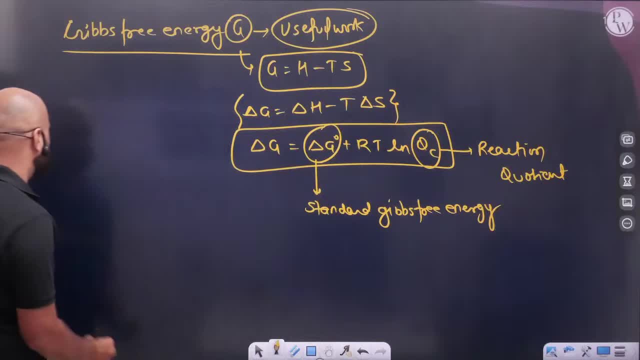 I will write all the formulas so that now things will be easy at equilibrium. at equilibrium, delta G becomes 0, so delta G naught. delta G becomes 0 and QC becomes KC, so delta G- naught will be minus RT ln KC or minus 2.303 RT log KC. 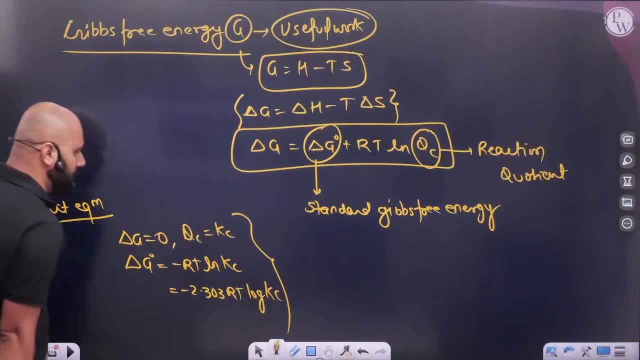 Sir, exact question based on this formula, direct formula based question was asked. that's why this chapter formula has to be done more. that's why this chapter formula has to be done more. that's why this chapter formula has to be done more. 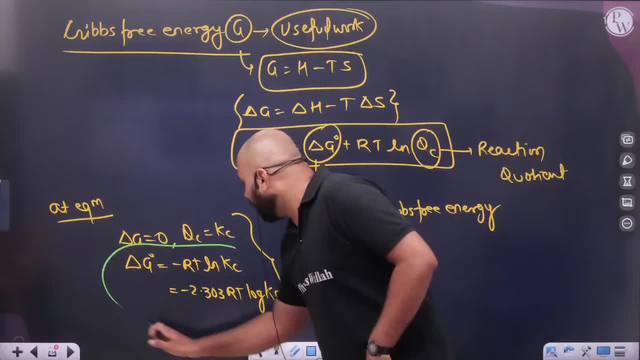 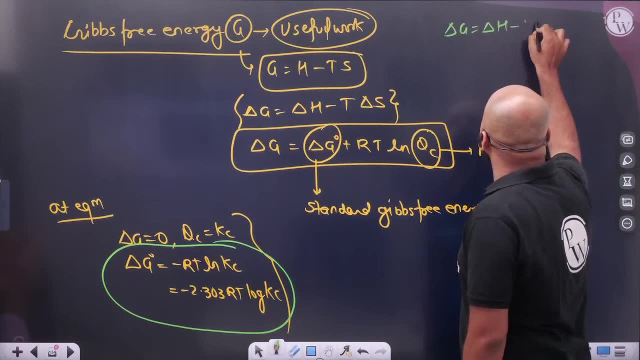 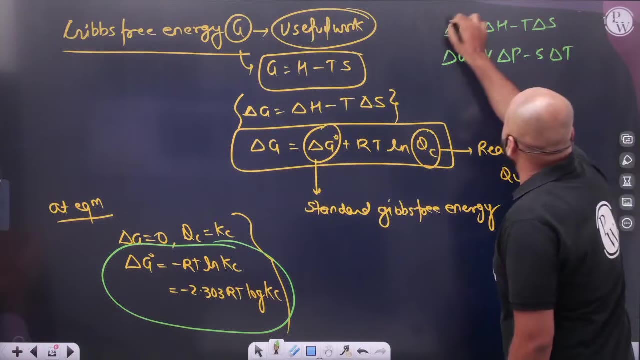 why? because here on the formula direct direct, this question direct formula based question was asked. Sir, look here the formula of delta G. you can remove it from: delta H minus T, delta S also. or I am just telling you to remember one more formula of delta G. it will not come like this: S delta T. 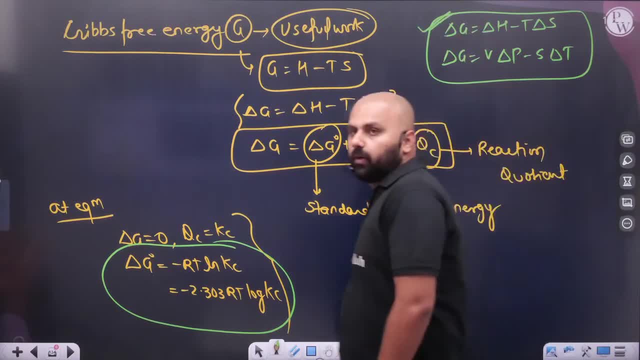 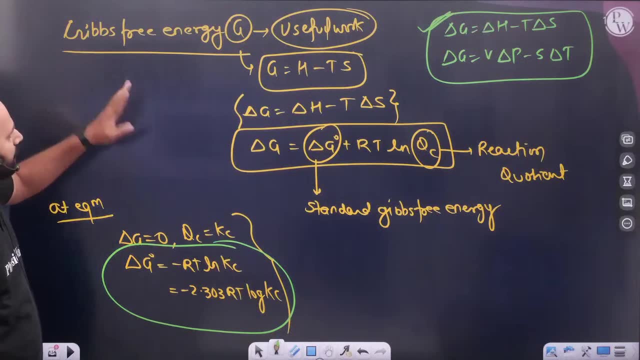 this also becomes a formula which you can use if you want. after that, a simple thing. see this: you have delta G, delta G naught, plus RT, ln, QC is done, sign marks: food, free energy. after that, someone told me: Sir, lets do one more thing. 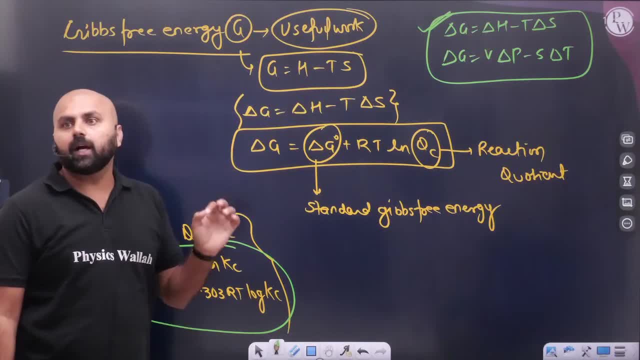 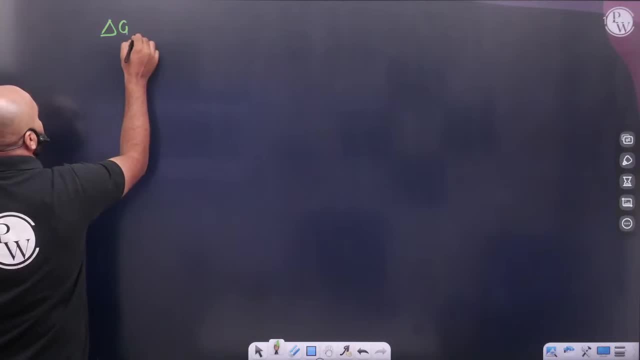 sign marks: food, free energy. for this. let's begin to use both of these here. they start using both of these. see this in you. I am talking about delta G, unit of delta G. if you take out the unit of delta G system, then that becomes minus T, delta S total. 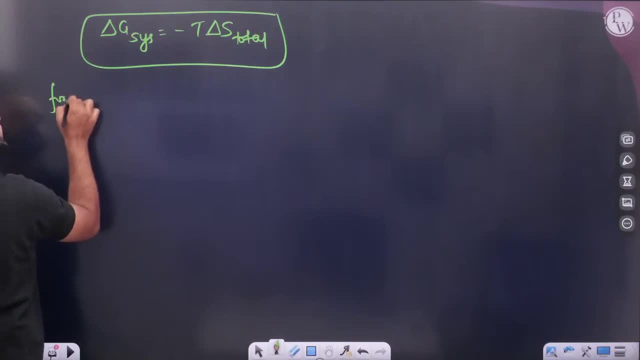 and this is why, in my life, for a spontaneous process- if a process has to be spontaneous if that person himself wants it- than I don't have lot more work to do. We don't have to work too hard. Why For spontaneous process? what is total entropy? 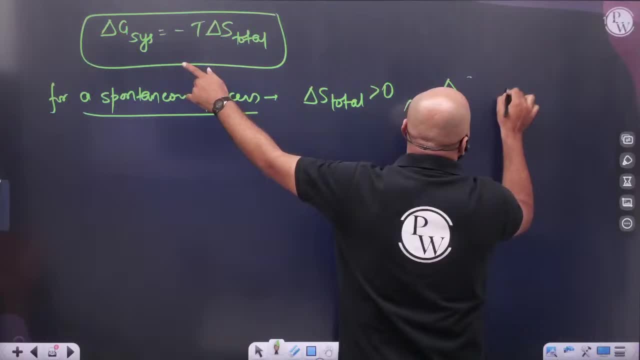 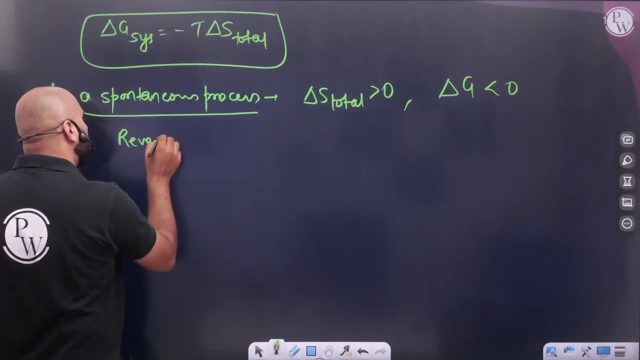 Greater than zero. If total entropy is greater than zero, then what will be the Gibbs energy Less than zero. If any process has to be spontaneous, then, sir, if I say that any process has to be reversible, if there is a reversible process, what does reversible process mean? 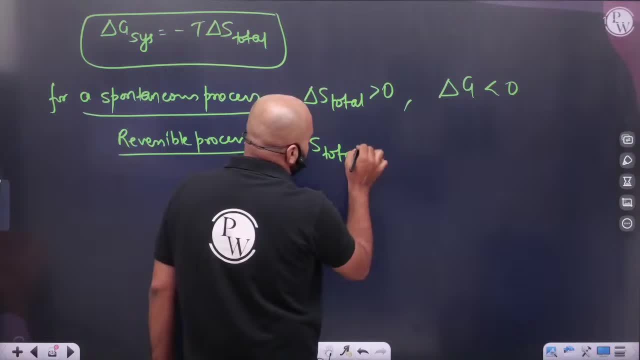 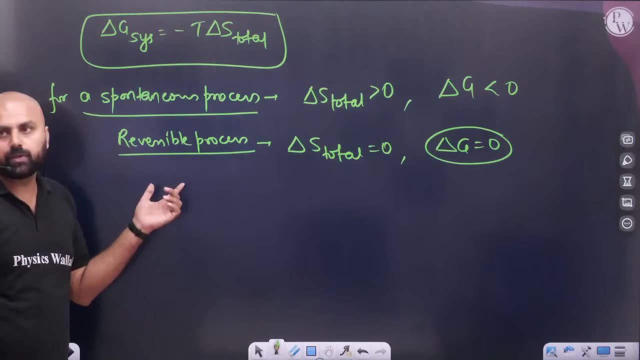 Delta S total. What will be delta S total? Equal to zero. What will be Gibbs energy? It will be equal to zero. What will be Gibbs energy? It will be equal to zero. So see these small things. Delta G system minus T. delta S system. 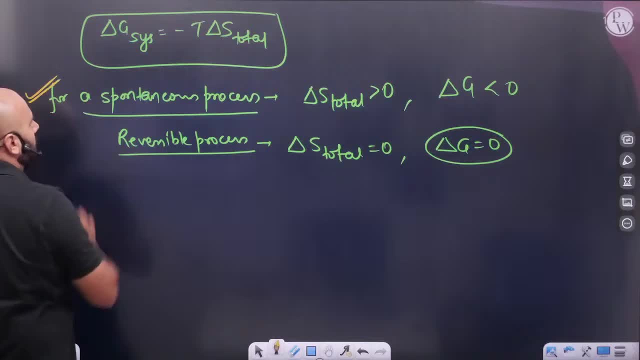 If any process has to be reversible, then we have to take care of this Now. in this condition, 2-3 cases come. If we talk about delta G, then delta H minus T, delta S, Different cases of this come. Which case? 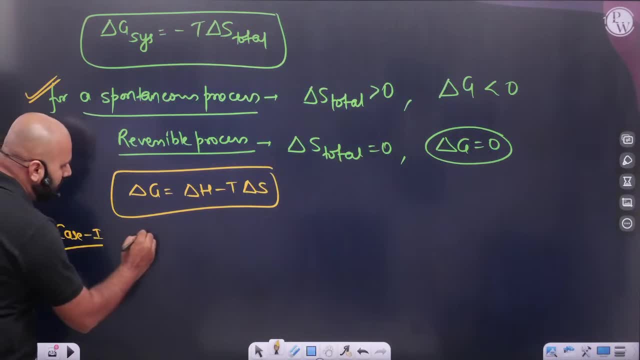 See this case 1.. If I am told that delta H is positive and delta S is negative, Sir, will this reaction ever be feasible? Let's see. See this, Brother. don't ask this question too much. We just have to see it in the exam. 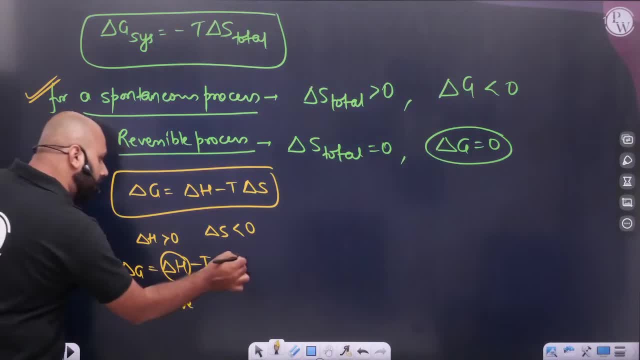 See this: This is positive, This is negative. Sir, if we multiply this negative with negative, then what will happen? Positive, Positive and positive. You will see Gibbs energy with you at any time. Positive and positive Can never be, can never be zero. 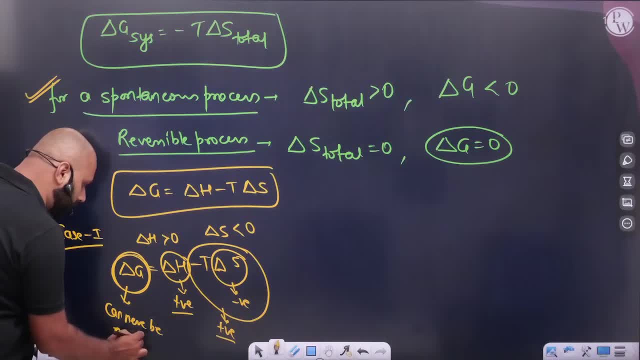 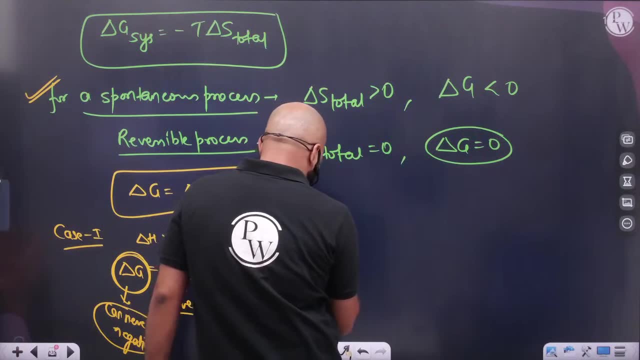 Can never be negative, Can never be negative When no one can be negative. When no one can be negative, Then this process will always be non-spontaneous. Be prepared for such questions in the exam, Sir. be prepared for such questions in the exam. 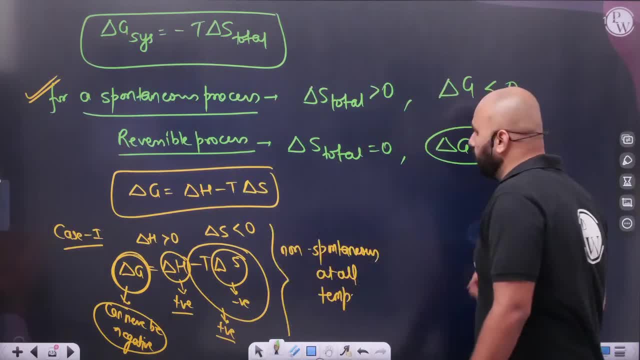 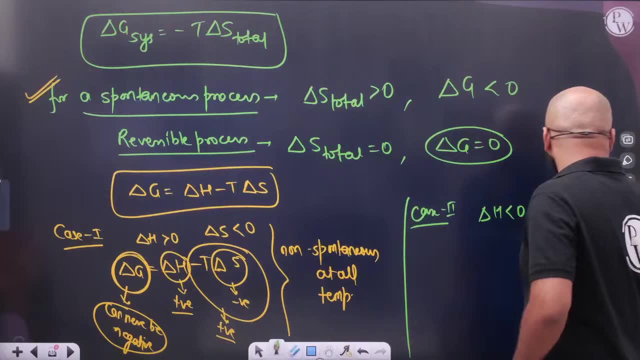 Remember, Sir, such a reaction can be given. Anyone can give such a reaction. Let me give you case 2.. I give you this, Sir: what is delta H Less than zero? What is delta S Greater than zero? 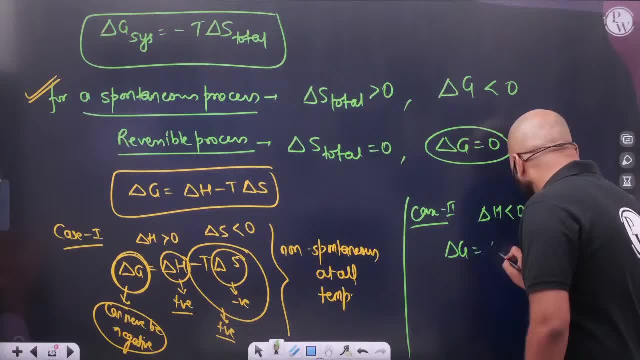 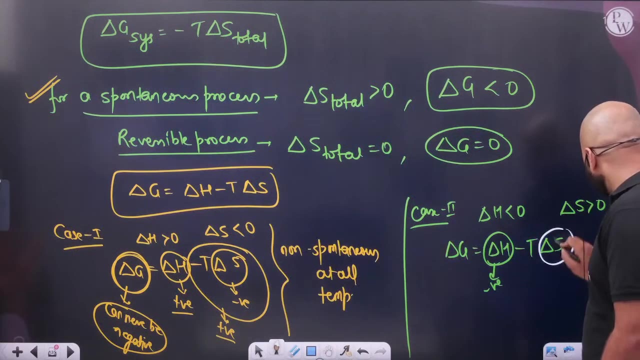 See this. See delta G. You can't fix it, You better lift it up. Do it, Sir. what is delta H Negative? if you want to do any process spontaneously, then you have to always make the give synergy negative. see this: what is your delta S Positive? what is this whole term Negative, negative and negative? what will be? delta G? Always negative means if two people get negative, two negative people will get, so two people will always get negative. so this person will always be negative and this reaction will be negative. 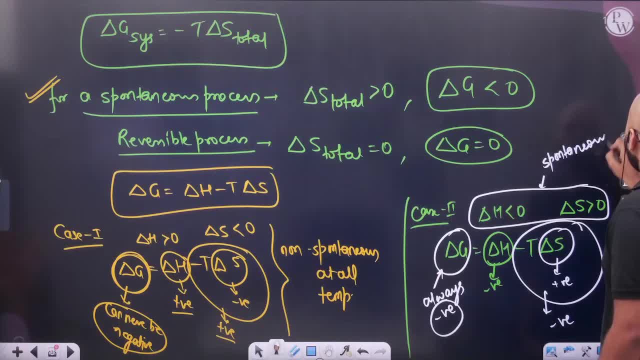 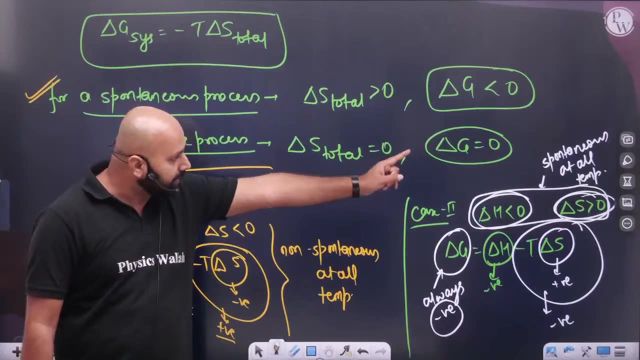 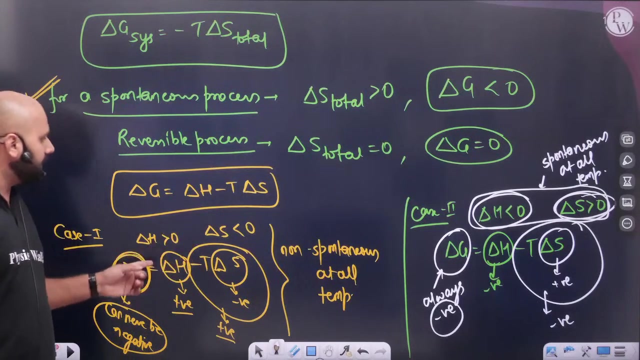 This reaction will always be spontaneous, spontaneous at all temperature. when you say at that temperature, remember where the energy is decreasing and where the entropy is increasing, that reaction is the best spontaneous, the best spontaneous. this reaction will always be spontaneous where the energy is decreasing, enthalpy is decreasing and entropy is increasing. in that case, what will always happen? It will be spontaneous. in this case, it will not happen. this case is the worst case. why? 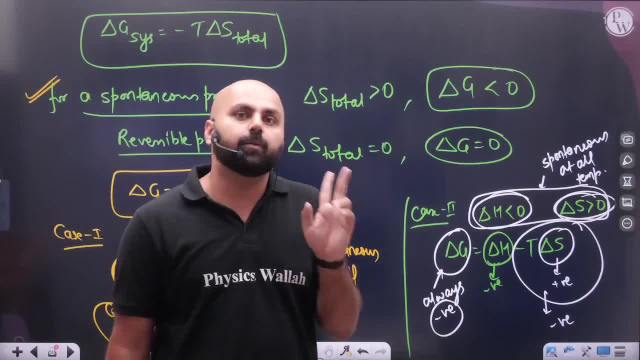 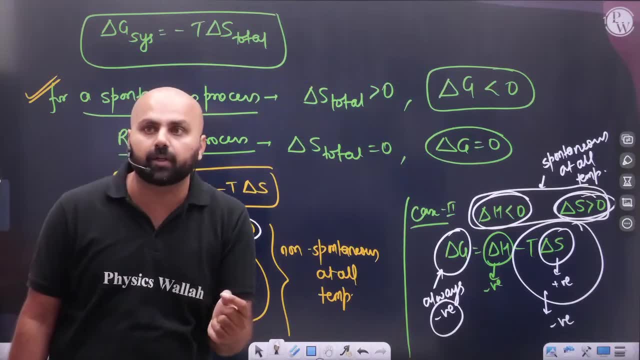 Because we all know that we want only two things in our life: We want to be stable. To be stable means to reduce our energy, And we also want our randomness to increase. So when can randomness increase? Randomness can increase only when what happens to you? 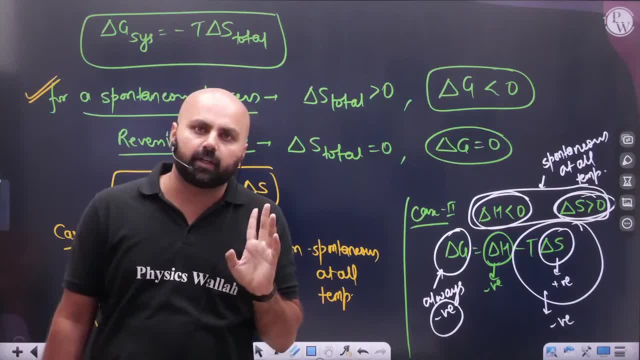 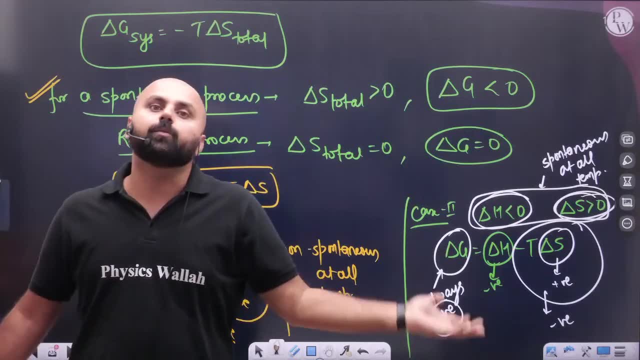 Both factors, For only two factors. we do any process spontaneously. Only two factors, Sir. what happens to the energy? Because the less the energy, the stability will increase And randomness will increase. means we can do whatever we want. We can do whatever we want. 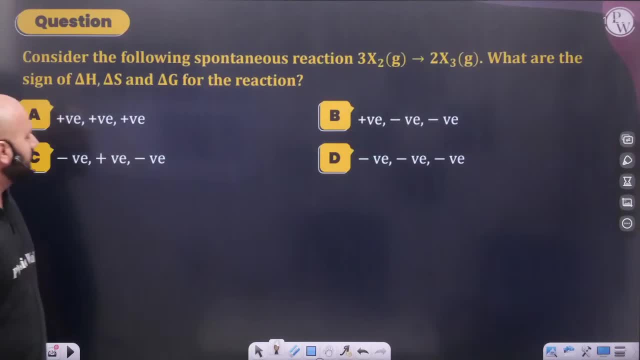 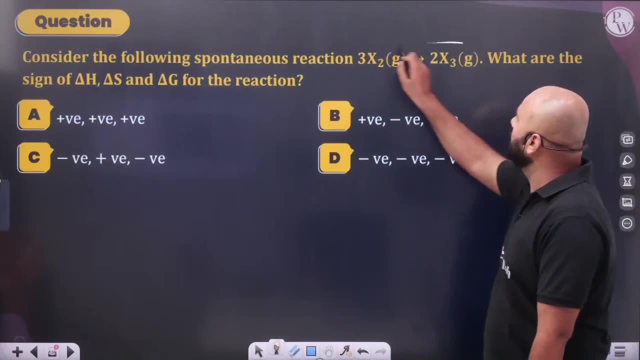 So these small things will come Like. now this question is given, Sir, look here In the reaction in which 3x2 is being converted. In which 3x2 is being converted, It is being converted in 2x3.. 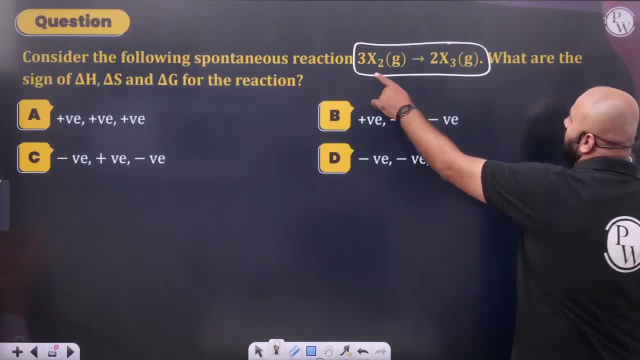 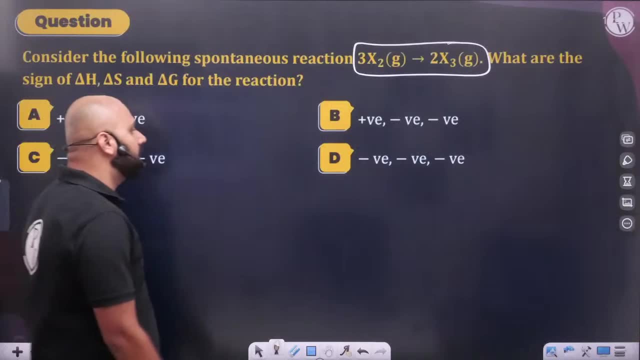 In which 3x2 is being converted In 2x3.. Means: what are the number of molecules happening? Less Bonds are being formed. Where bond is being formed. means what will be the entropy Negative? What will be the entropy? 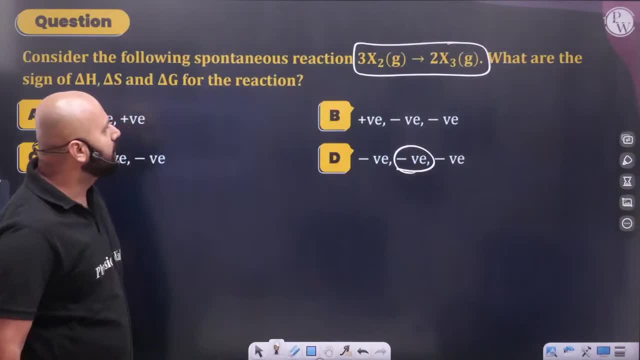 Negative, Sir, bond is being formed. What is the entropy Negative? Why? Because, sir, obviously your entropy has decreased And, sir, entropy Bond is being formed. If bond is being formed, then what will be the energy It will be released? 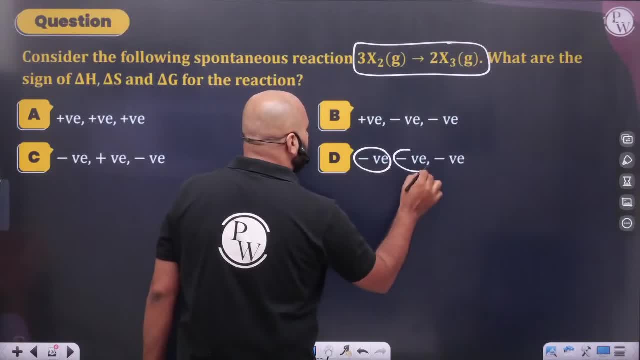 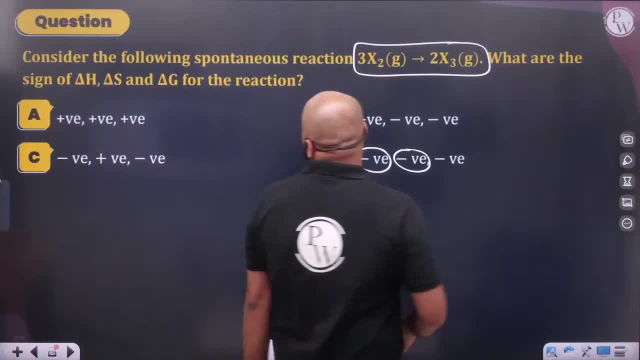 If bond is being formed, then what will be the energy It will be released? Obviously, After that, you Now this reaction is spontaneous. If this reaction is spontaneous, then what will be the Gibbs energy Negative? What will be the answer? 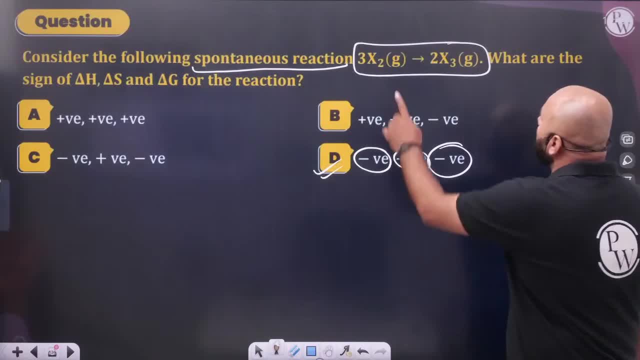 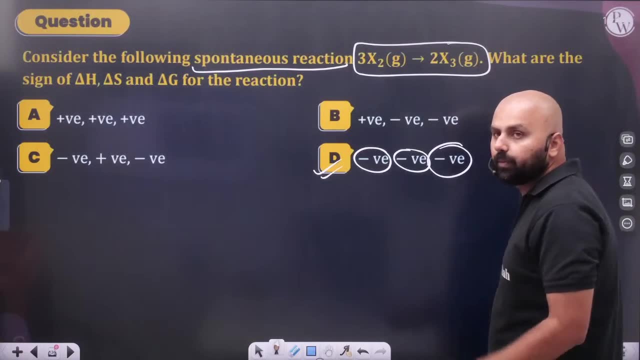 D. What will be the answer? D? See What is he saying, Sir. entropy will be less. Hey, it is x2.. If you add one more bond with it, then what will be the entropy of molecules? What happened to entropy? It decreased. 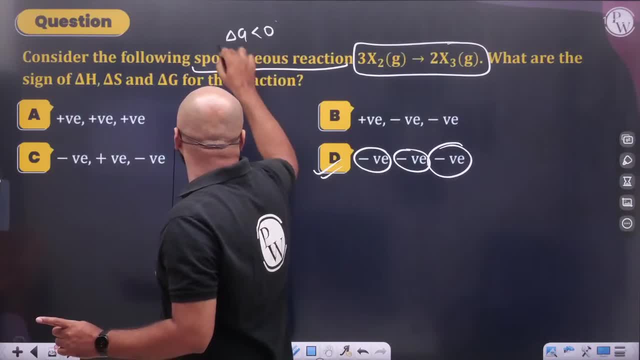 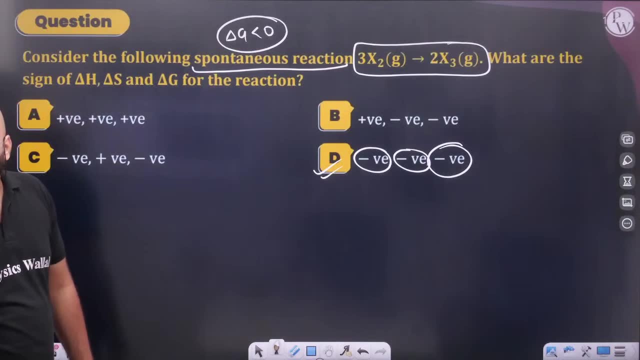 It is spontaneous. Spontaneous means what should be the give synergy Negative. Give synergy is negative. So, sir, the first option is gone, What is left? So pick up these options and see, It will be done. It will be done. 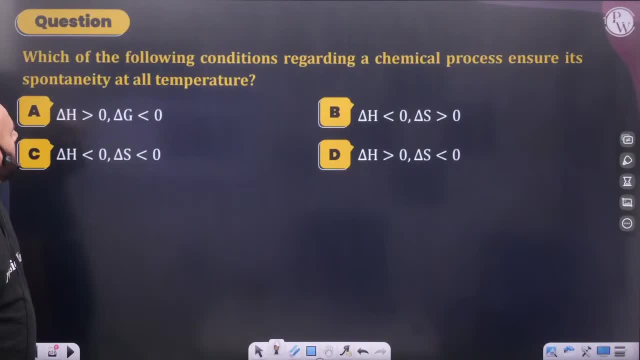 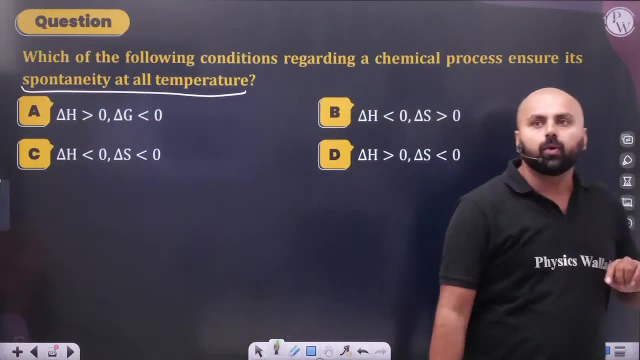 Come on, Look at the next question, Sir. what is the reaction that is always spontaneous? What is the reaction that is always spontaneous? Will you tell What will be the reaction that will always be spontaneous? What will be the reaction that will always be spontaneous? 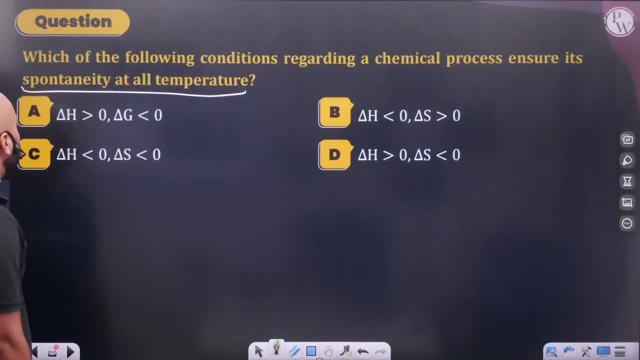 Sir, what is happening in it? What is happening in it, Sir, what is happening Always. What is the energy doing, Losing, And what is the entropy happening, Increasing. What will this process always be? It will be spontaneous. 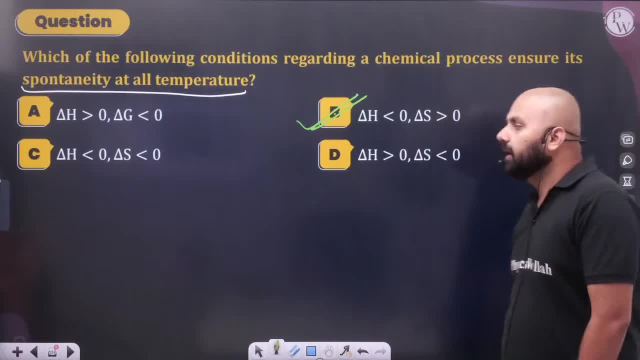 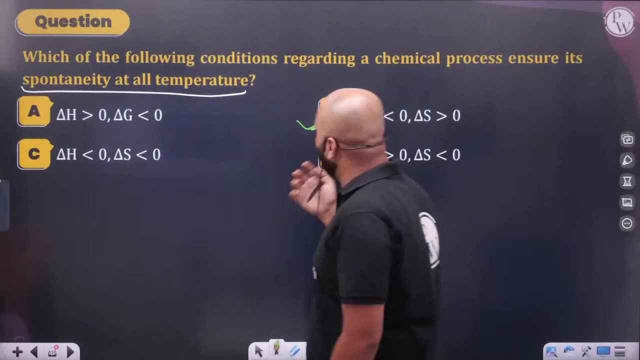 What will this process always be? It will be spontaneous. Okay, It will always be spontaneous. Where entropy is decreasing- Sorry, Enthalpy is decreasing And entropy is increasing, This is the reaction that will always be spontaneous. What will always happen? 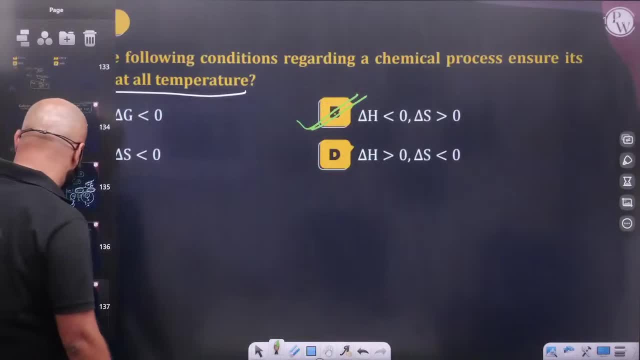 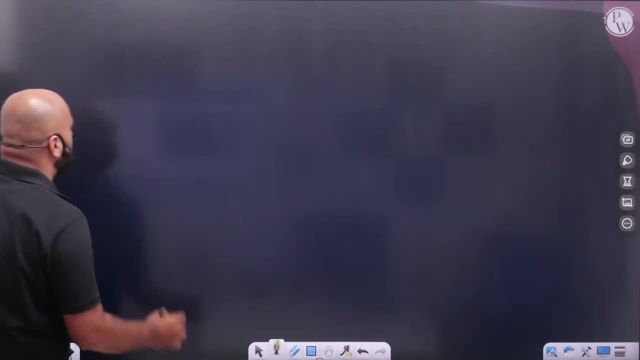 It will be spontaneous. Sure, It will happen. It will happen, It will happen, Sir. then do these small things. After this, a third law of thermodynamics happens like. this means there is no such thing in our life. but now I will tell you what the third law of thermodynamics says. 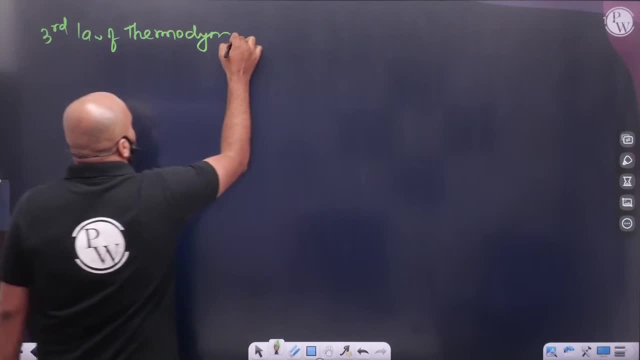 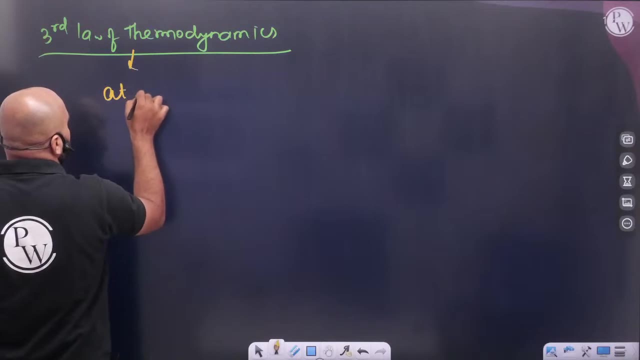 Okay, what does the third law of thermodynamics say? Okay, it is not in such a syllabus, but yes, it should be known. Okay, just remember, at absolute zero, at absolute zero temperature. at absolute zero temperature means When, Sir 0 Kelvin, 0 Kelvin temperature Entropy. 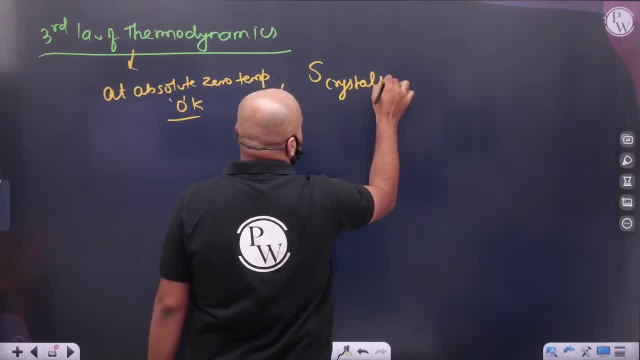 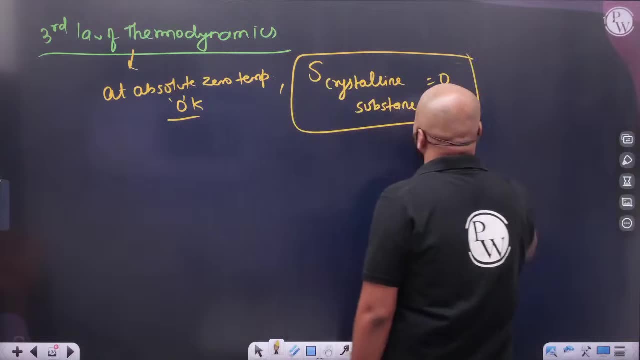 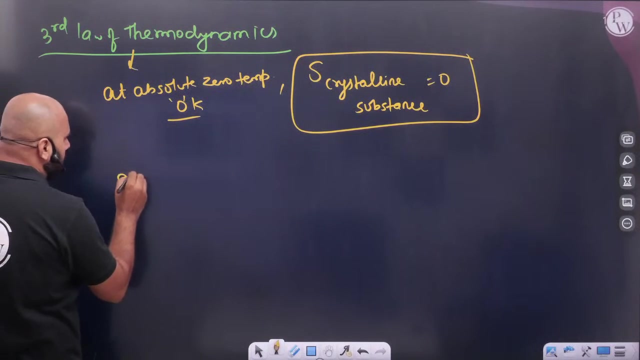 of crystalline substance. entropy of crystalline substance. what happens? Entropy of crystalline substance becomes zero. Sir, at absolute temperature, entropy of crystalline substance becomes zero. You need to keep this in mind because this is the third law and if you want, if you want entropy, if we want to vindicate entropy, 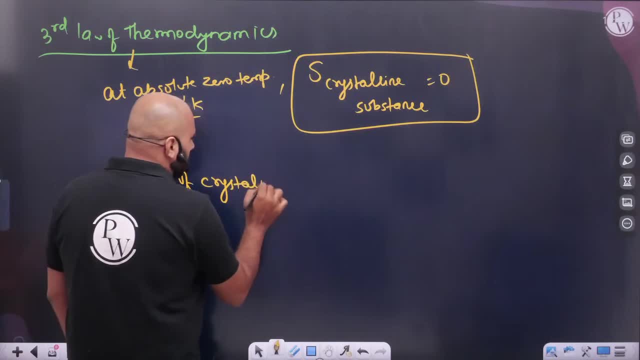 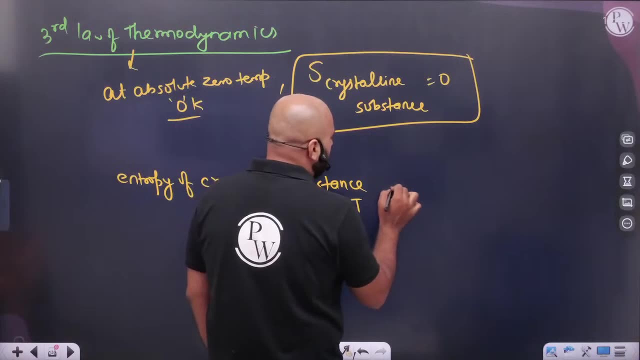 entropy of crystalline substance. if we want to do, we need crystalline substance, crystalline. If you want to find out entropy of crystalline substance at TK, then it is nothing but NCP, ln, T. If you want to find out entropy at crystalline substance, then this formula comes: 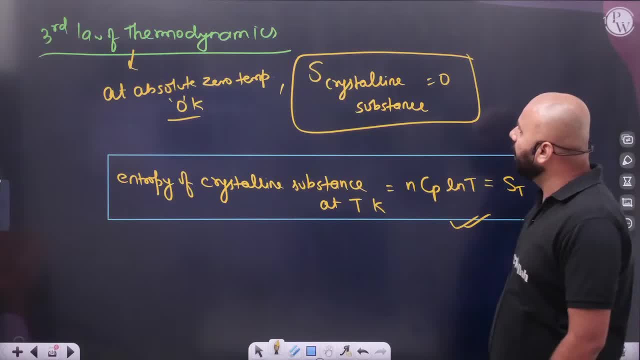 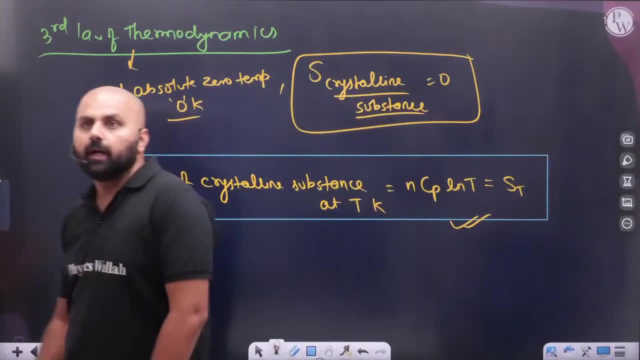 If you want to find out the formula of crystalline substance, then this formula comes In third law. crystalline substance has zero. It is not of amorphous. What happens to crystalline Zero? What happens to crystalline zero at Kelvin? 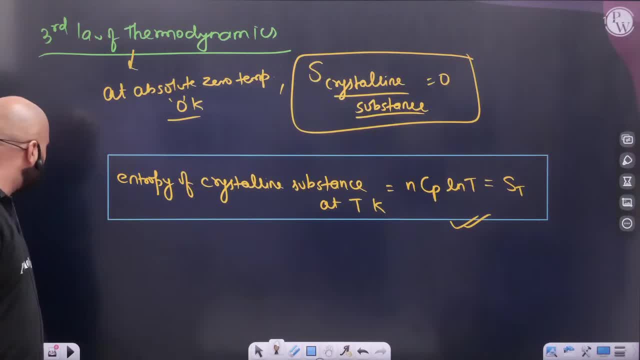 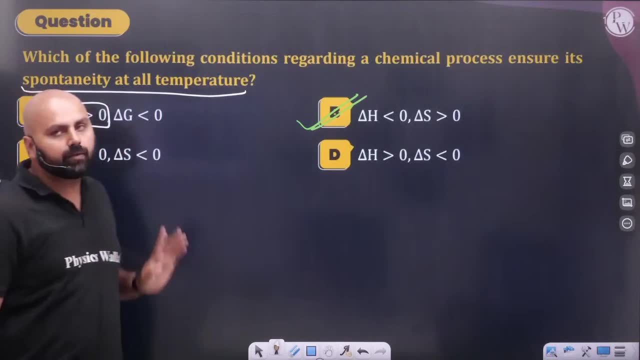 What happens to crystalline zero? at Kelvin, It will become zero. One person is saying that, sir, you did not see the first option, Brother, the enthalpy is increasing in this, so I cut it. The enthalpy is increasing, so I reduced it. 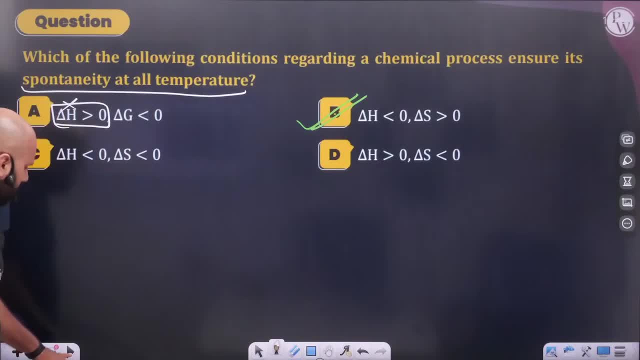 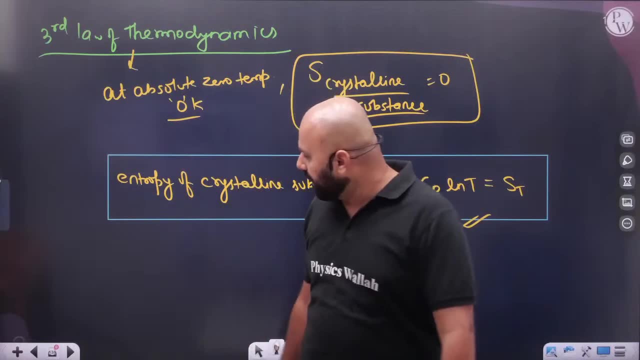 Sir, I removed it, Nothing else. Sure, So keep doing it. These are small things, Pick it up. I have thermodynamics, which we have finished. Now I have a small thing: thermochemistry. There is thermochemistry, Okay. 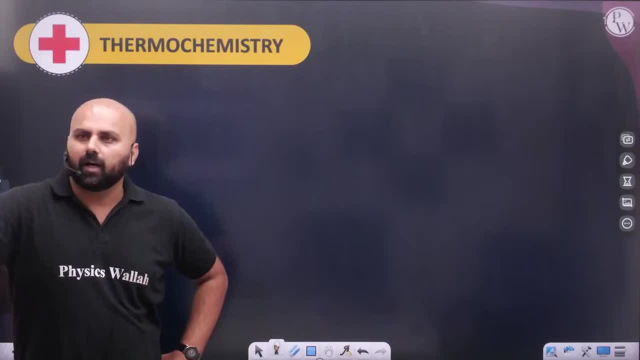 After that, we will take a break. Yes, okay, We will take a break after thermochemistry. Hey, I had given it in 5.30.. It is not even happening in 2-2.5 hours. Okay, How will you give the exam? 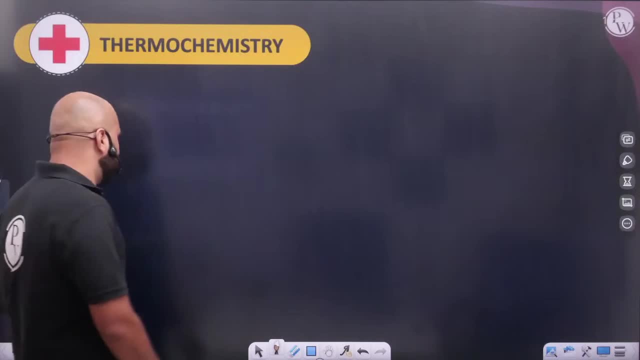 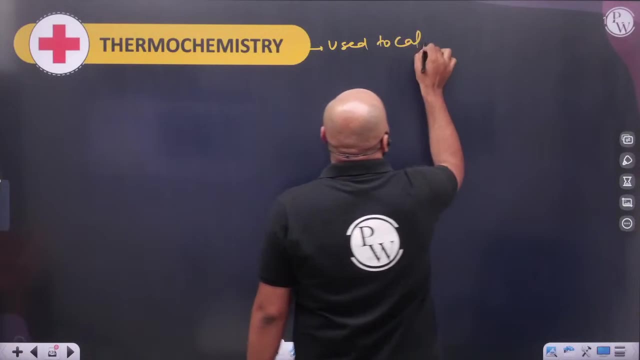 How will you become a doctor? Look at thermochemistry. There is nothing in thermochemistry. This whole chapter validates 2-3 laws. Why is it there? So used to calculate? It has only one value, It has only one meaning. 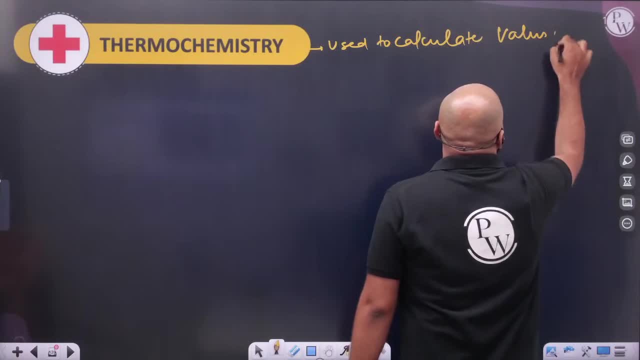 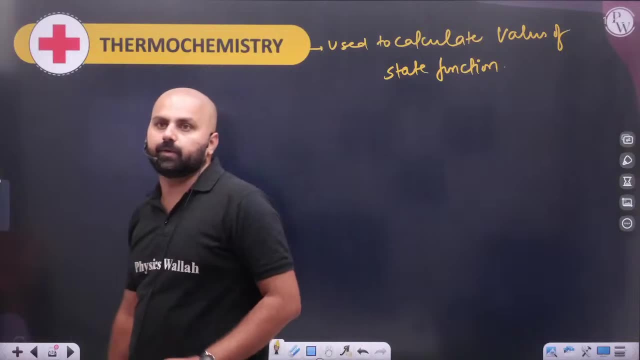 Calculate values of state function. Values of state function. It is to find the values of state function. Nothing else Used to calculate is values of state function. That means whatever it is. there is nothing in thermochemistry, Nothing in thermochemistry. 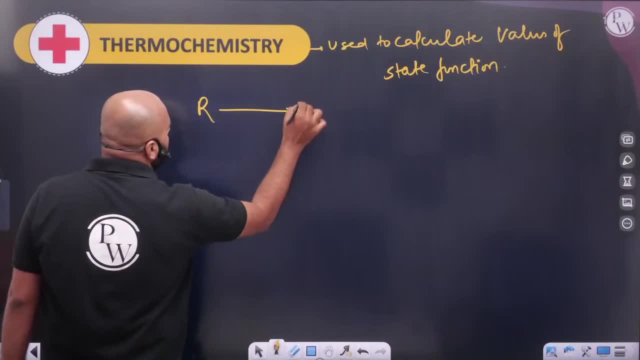 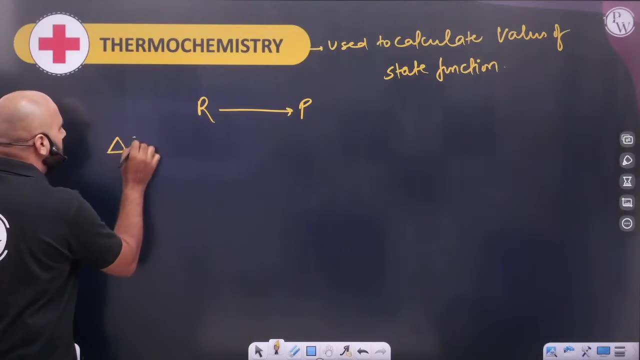 If you have given any reaction, Sir, reaction has been given. Reactant has been given in product. Look carefully, Look carefully. I am explaining the whole thing. All these state functions Means to find the give synergy of reaction. So nothing. 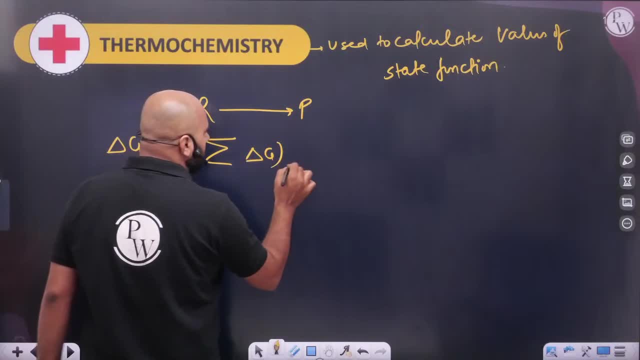 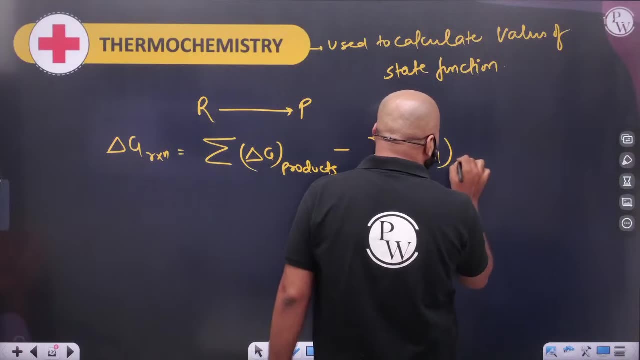 Sir, to find the give synergy of reaction. So product's give synergy. Product's give synergy Minus, Sir, give synergy of. See Why, Sir, the meaning of all the state functions was the same: Final minus initial. 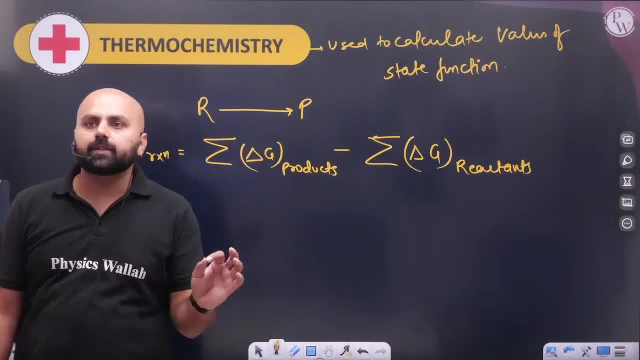 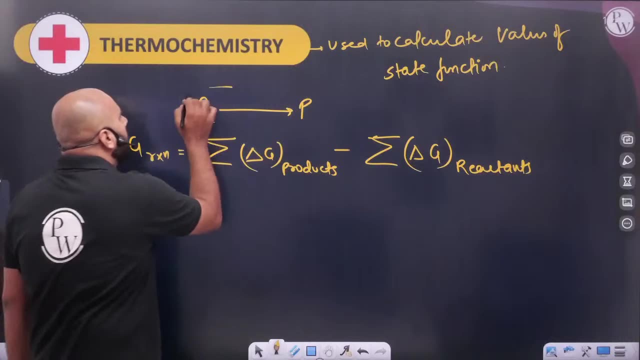 Sir, the meaning of state function was the same. State function's meaning was the same: That final minus initial. What to do with product minus Do reactant? State function's meaning is the same. What to do with final minus Do initial? 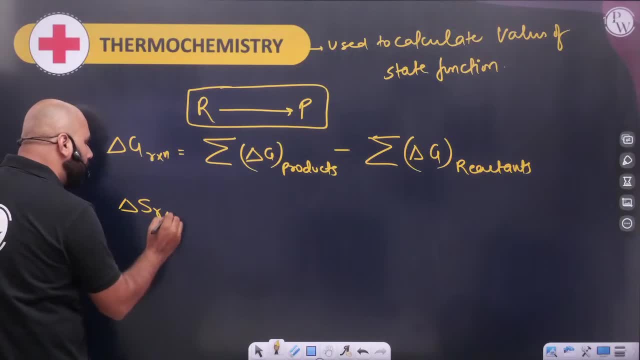 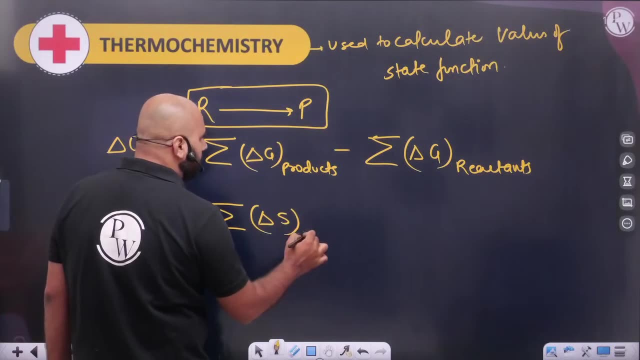 See this: If you tell me that you have to find entropy of reaction, Nothing, Sir. there is no exception, Nothing. What you have to do, Find entropy of reaction. There is no problem. Product minus: What to do with product minus? 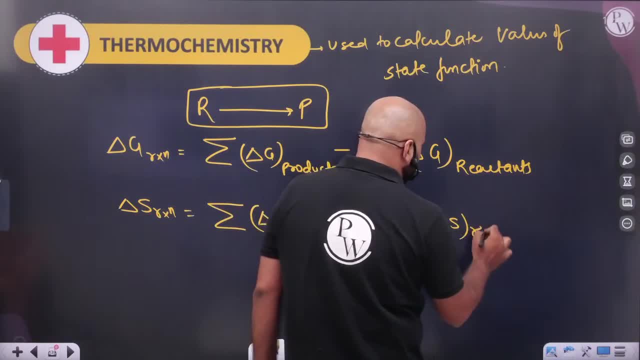 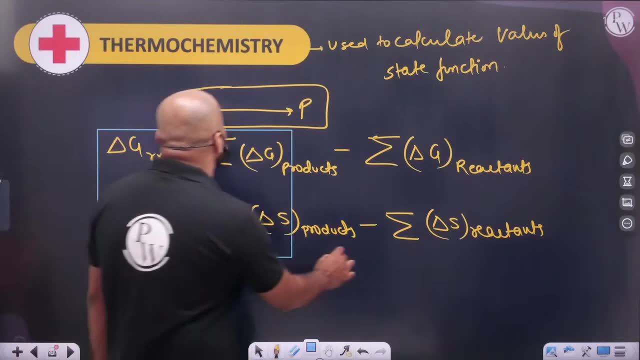 Entropy of What to find. entropy of product minus. Find reactant. Find product minus. product minus: entropy of reactants. here there is no exception, nothing. simple, simple state function. do it? do you know where the problem comes? do you know where the problem comes? 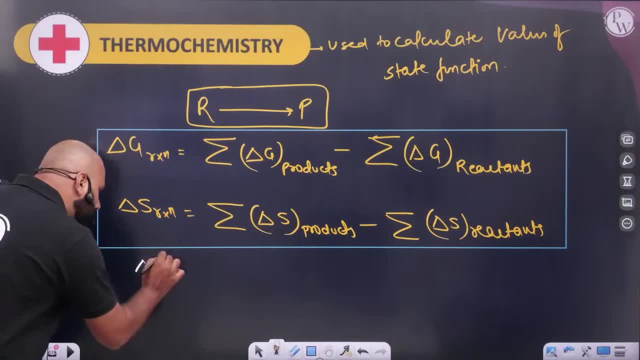 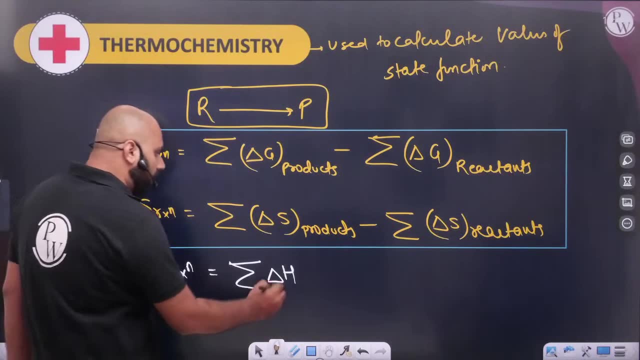 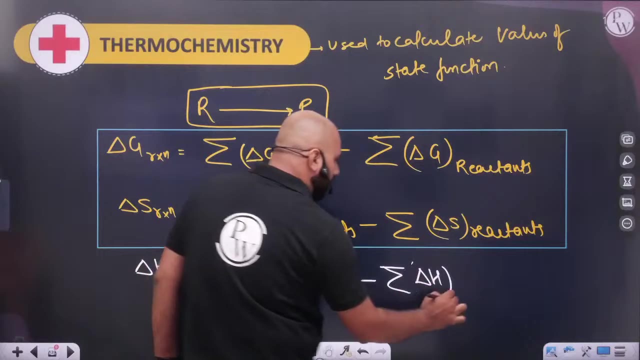 the problem comes here. remember, if you go to get enthalpy of reaction, then, sir you normal formula, always enthalpy. also is state function. so what will happen? always product minus enthalpy of what will come, reactant product minus. 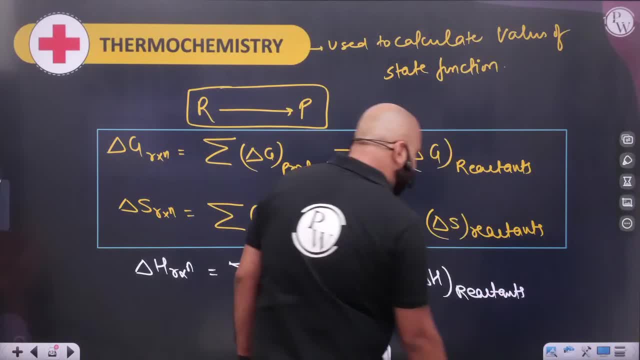 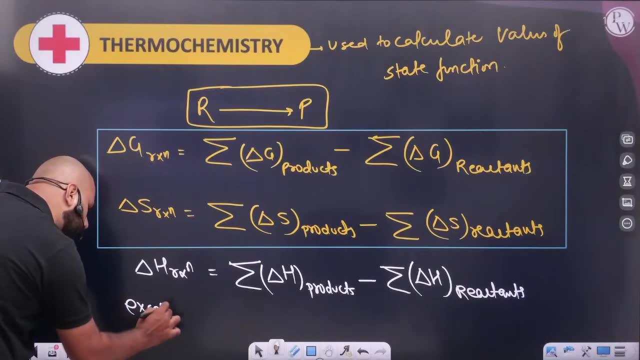 enthalpy of what will come reactant, enthalpy of what will come reactant, product minus enthalpy of what will come reactant. but except, see here, except product minus reactant will do. but what is exception, what is except? 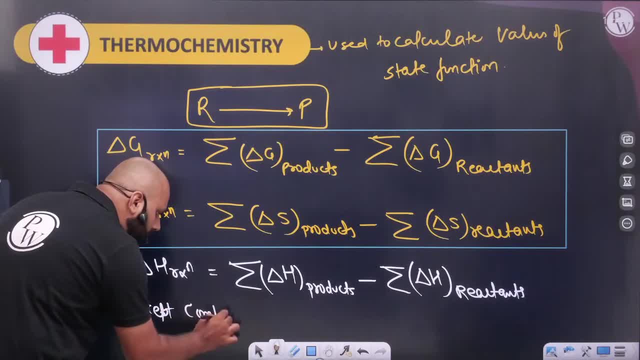 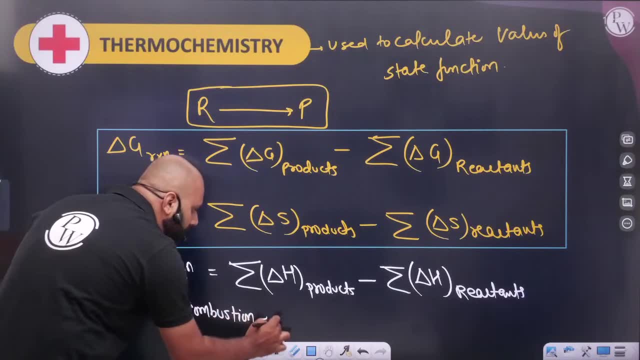 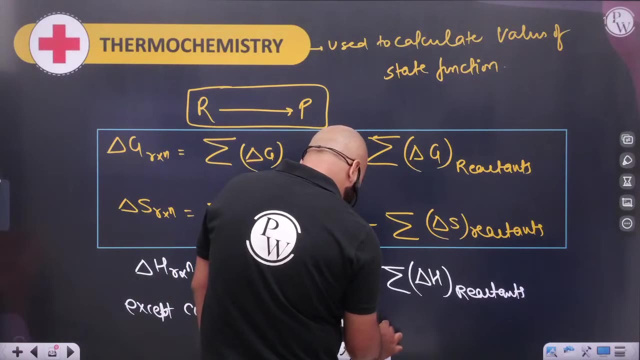 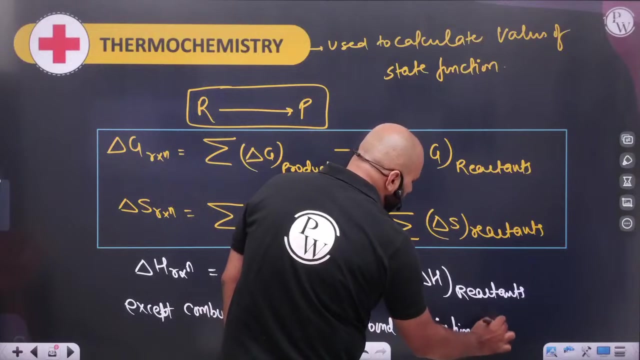 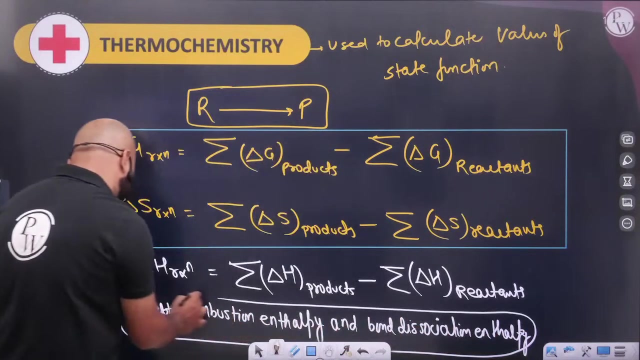 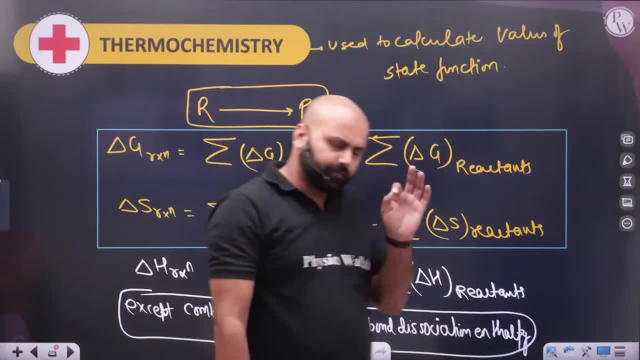 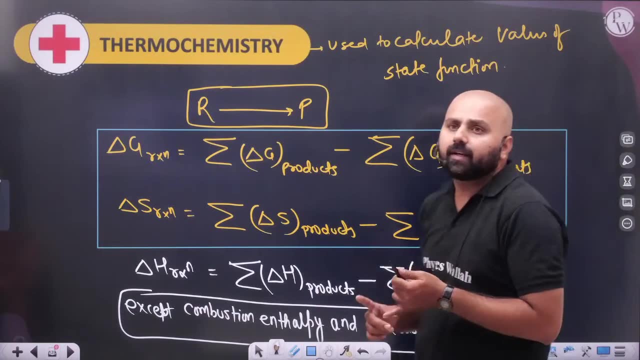 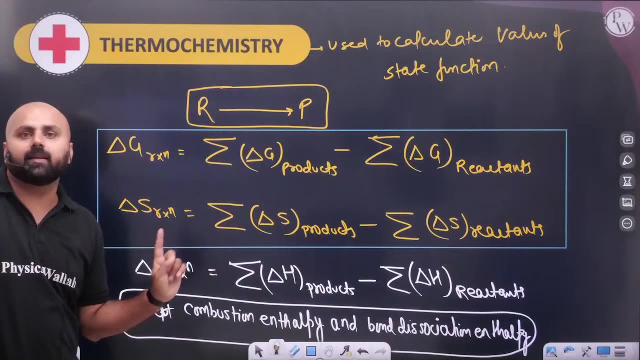 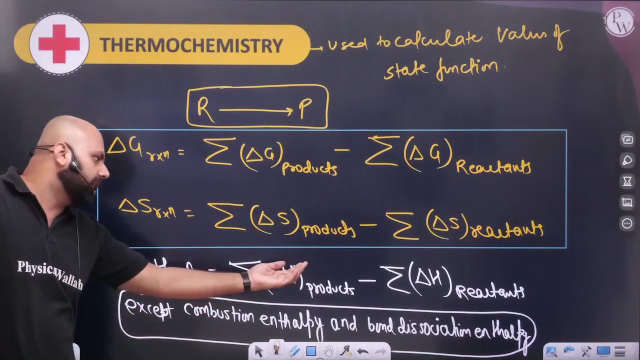 any reaction. you will do product minus reactant. you will be given many types of enthalpy. you have to remember simply that you have to do product minus reactant only. but remember the exception: combustion enthalpy and bond dissociation enthalpy. if it comes after this, then what will happen? What will reactant minus do Product? 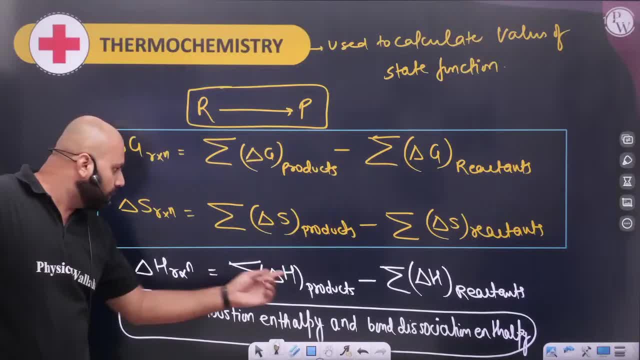 What will reactant minus do Product? What will we do? We will do product, Nothing else. If you are given this combustion enthalpy of reactant and product, Listen carefully- Combustion enthalpy of reactant and product is given. 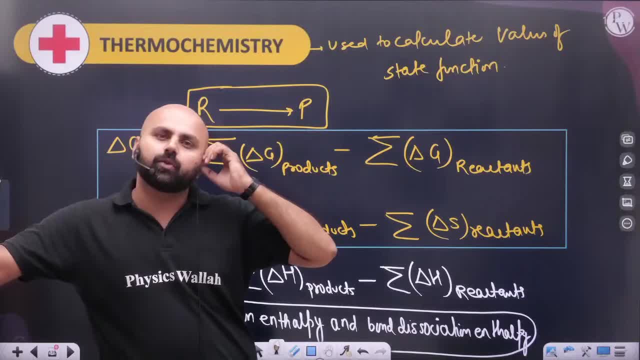 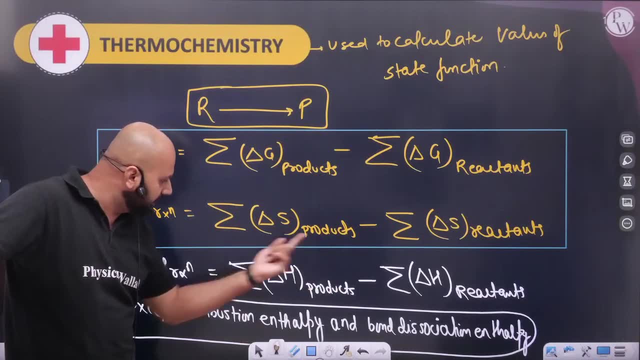 Only then apply this formula. It is not that if you want to extract combustion reaction, then also apply it. If you are given combustion enthalpy of reactant and product, Then what will you do? You will do: reactant minus product. Bond dissociation enthalpy of reactant and product is given. 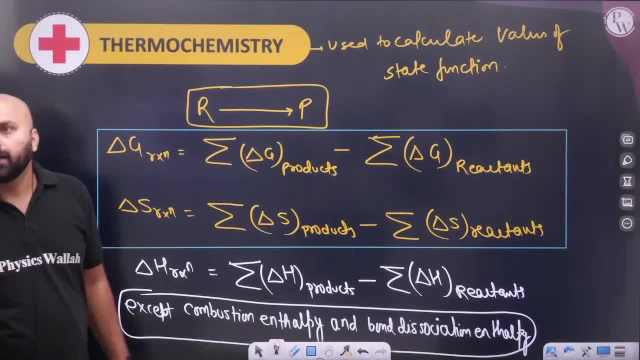 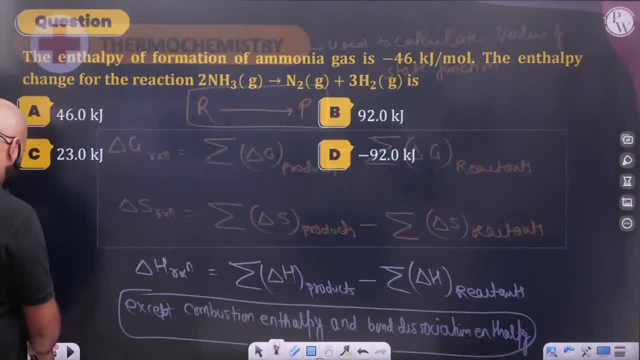 Then you will do reactant minus product, Nothing else. There are some small things here. Look at this. Suppose I am asked a question One minute. There are some laws of thermo chemistry here. Let's do that and then we will start. 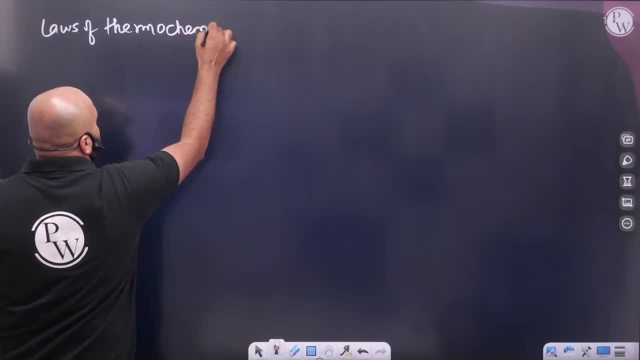 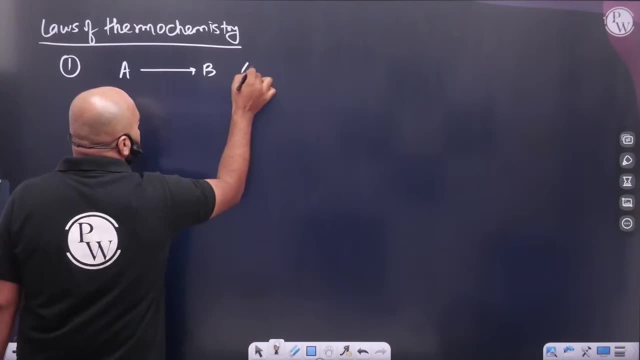 There are laws of thermo chemistry. Laws of thermo chemistry, What are they? The first law of thermo chemistry says that suppose one reaction is A to B If its enthalpy. suppose if I take 200 kilojoules, Then as soon as the reaction is reversed, 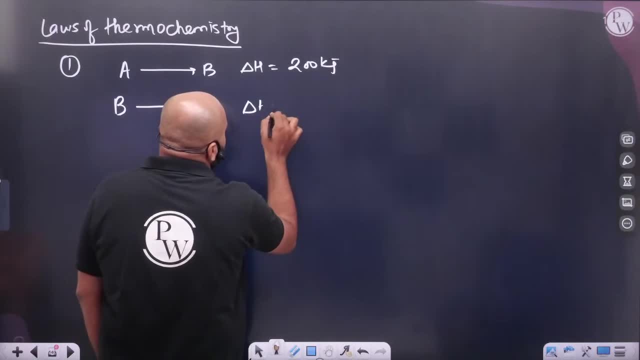 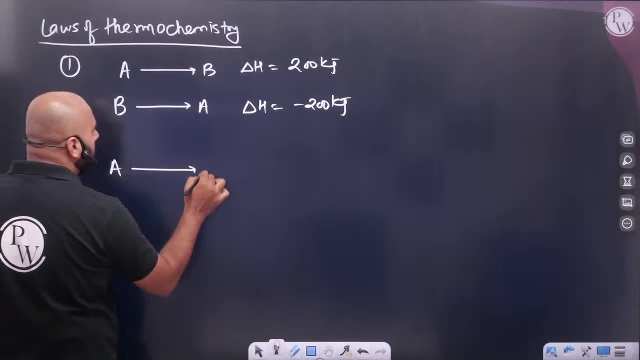 As soon as the reaction is reversed, The magnitude of its enthalpy will be minus 200 kilojoules If I multiply the reaction. If I multiply the reaction from 200 kilojoules, If I multiply the reaction from 2.. 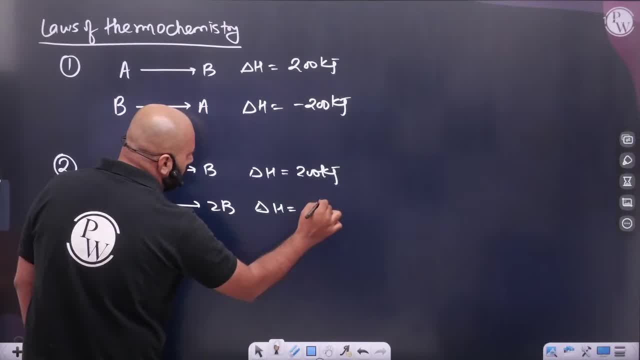 If the reaction is multiplied, then what will be the enthalpy? It will be 2 times. If the reaction is divided, A by 2 gives B by 2.. If the reaction is divided, Then what will be the value of delta H? 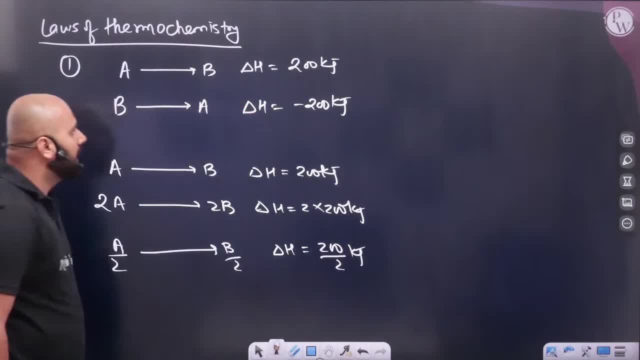 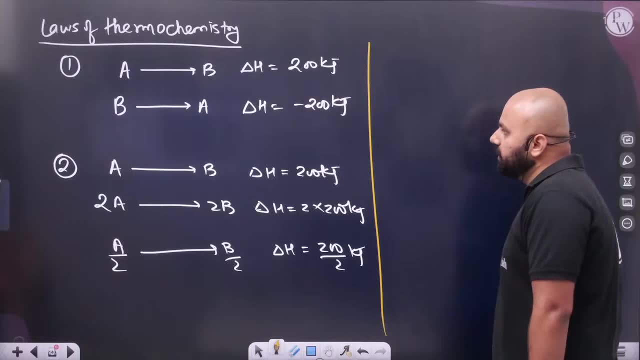 It will be 200 by 2.. Do it like this: If you divide, Then it will be divided. If you multiply What is enthalpy? It is an extensive property. So it will be multiply and divide. But there is one more thing. 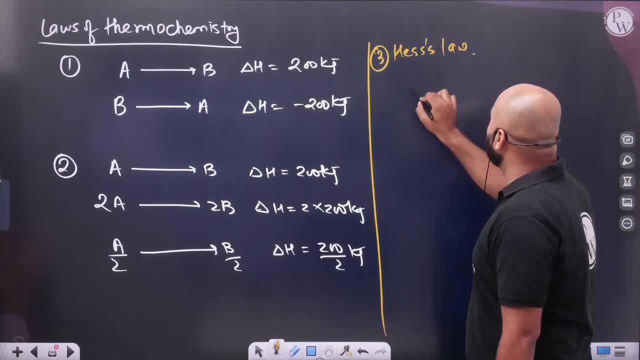 And that is known as Hess law. What does Hess law say? If the reaction is A to B, Suppose its enthalpy is delta H1.. If it is B to C, What is its enthalpy? It is delta H2.. 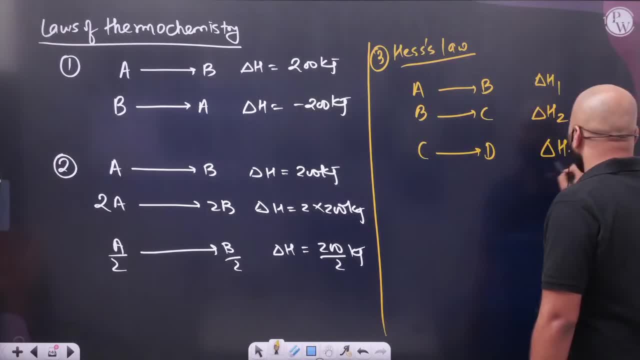 If it is C to D, What is its enthalpy? It is delta H3.. And if you want to go from A to D, If you want to go from A to D, Then in that case What will be the enthalpy of this reaction? 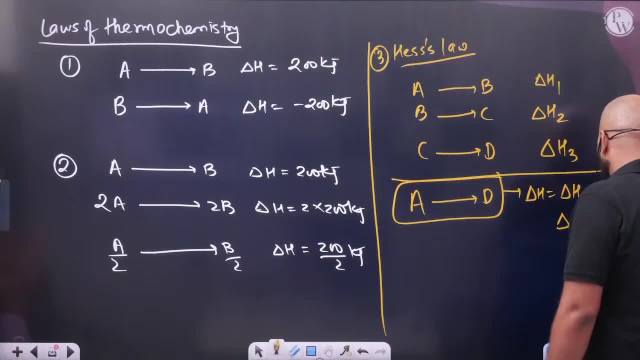 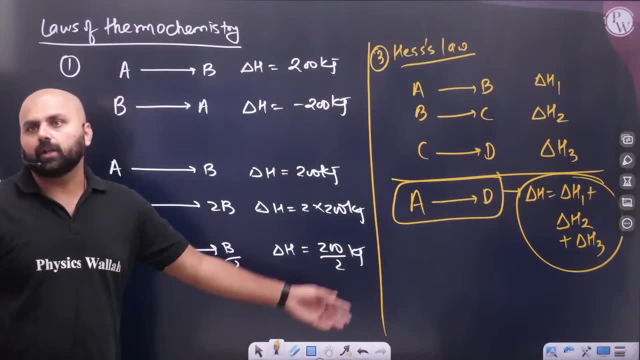 It will be delta H1 plus delta H2.. What will be the plus? It will be delta H3.. It will be delta H1 plus delta H2.. What will be the plus? It will be delta H3.. So see this. 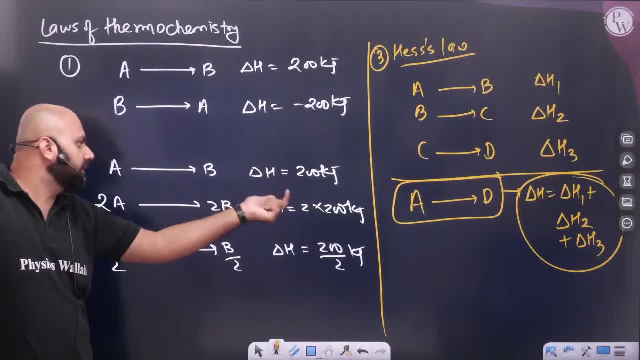 It is simple. It is extensive property, So obviously it will depend on the stoichiometry. If you multiply, It will be multiply. If you multiply, If you divide, It will be divide. So these are the small things. If you do addition. 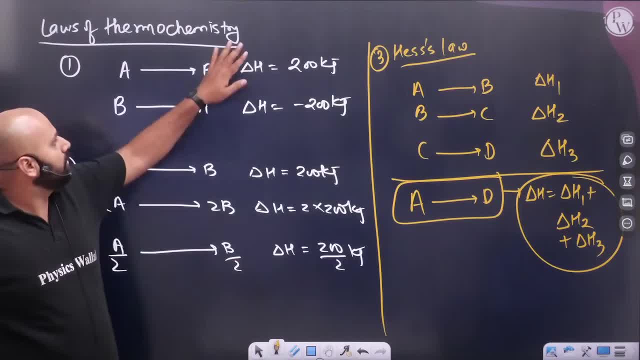 Reactions will be added. If you do re-addition, Reactions will be added. So this is my laws of thermochemistry. There is nothing in thermochemistry, Just basic 2-3 things. In state function, Product minus reactant is to be done. 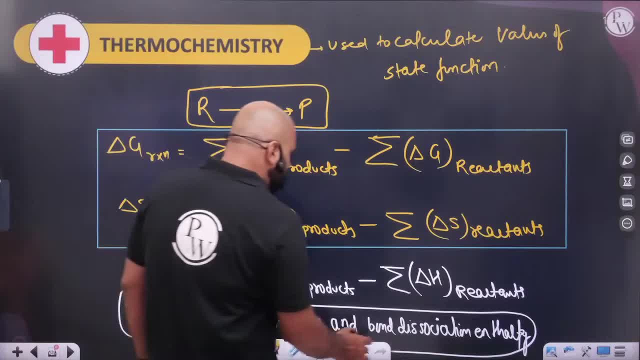 Exception. It should be known, And if you are doing the reactions in reverse, Then you should know what is happening there. Apart from that, If someone tells me, Yes, law, Combustion law About all this, Now there are some enthalpies. 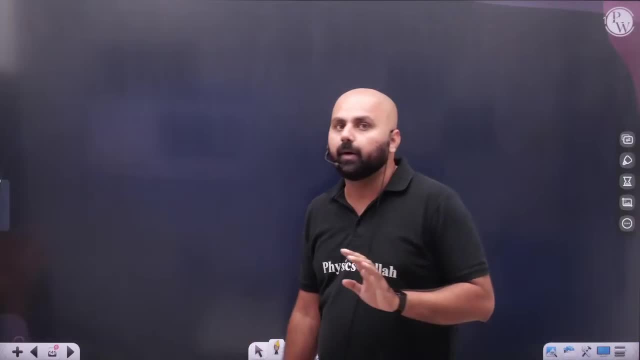 Different types of enthalpies. Let me tell you first Different types of enthalpies. Different types of enthalpy. Different types of enthalpy. Let me tell you first Different types of enthalpies. There are some limitations. 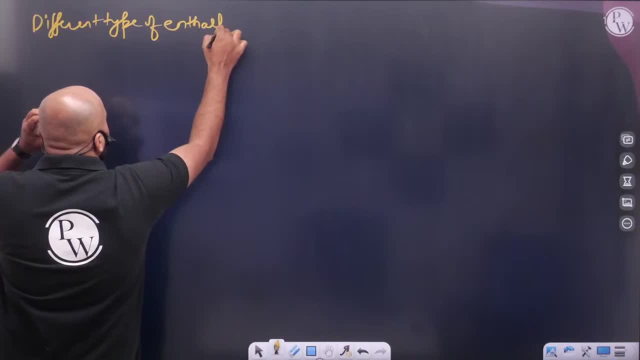 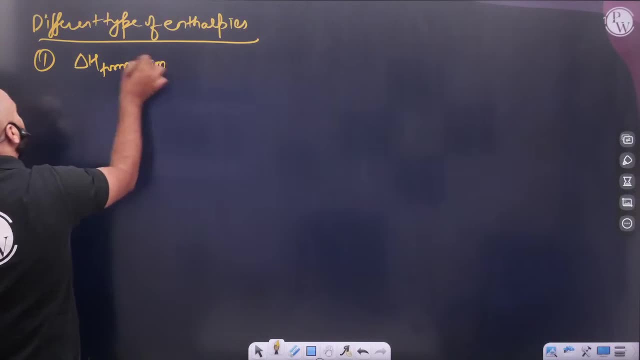 I will talk about different types of enthalpies. So what are different types of enthalpies? First thing, Formation enthalpy. What is said in formation enthalpy? It is important to write reaction in it, Whenever formation enthalpy will be defined. 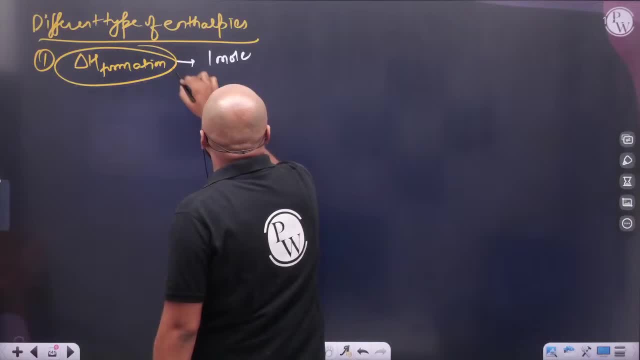 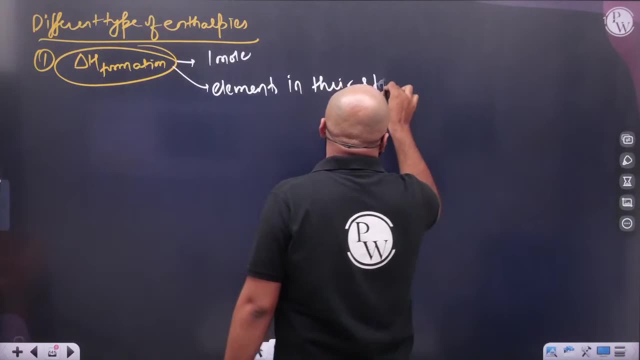 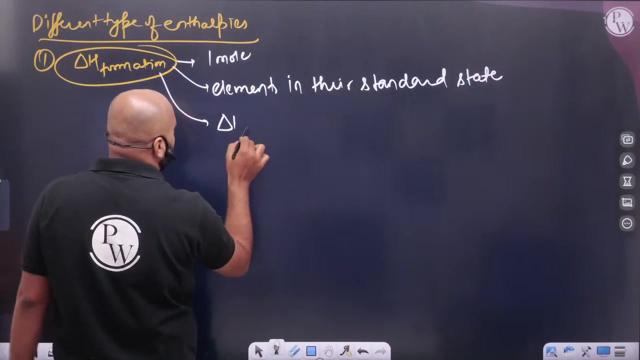 It will always be defined for one molecule And elements: Elements in their standard state. Remember 2-3 conditions of it. Whenever formation enthalpy will be defined: Elements in their standard state. Formation enthalpy: Formation of enthalpy of. 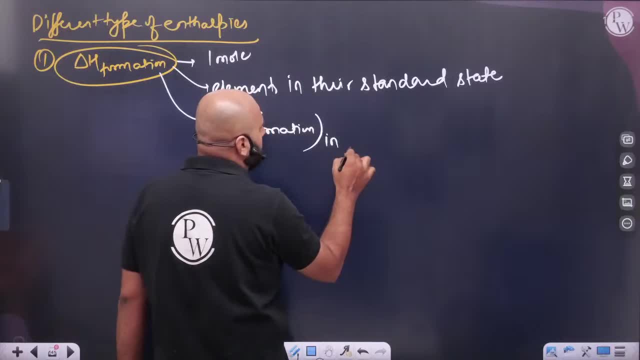 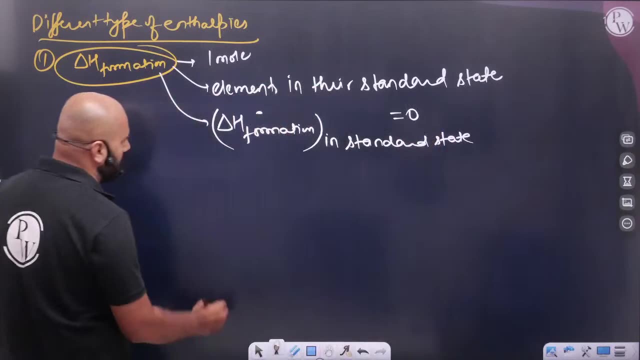 Formation enthalpy In standard state, How much it becomes? It becomes zero, Sir. see, If I am ever told, Then there should be a way to write the reaction Like: suppose he said Sir CH4. Formation enthalpy has to be defined. 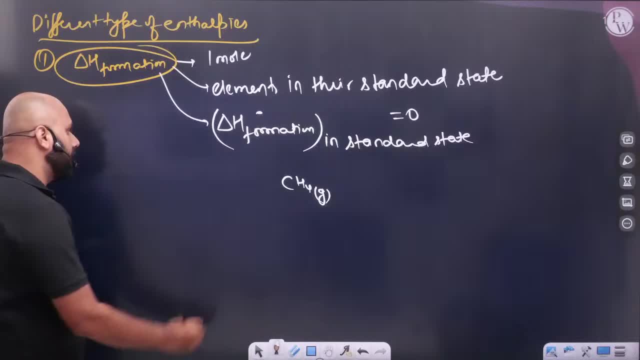 How will CH4 be made? See carefully. How will CH4 be made, Brother CH4. Formation enthalpy. It is personal to write. Ok, Sir, By which type of elements? By carbon And hydrogen Hydrogen. 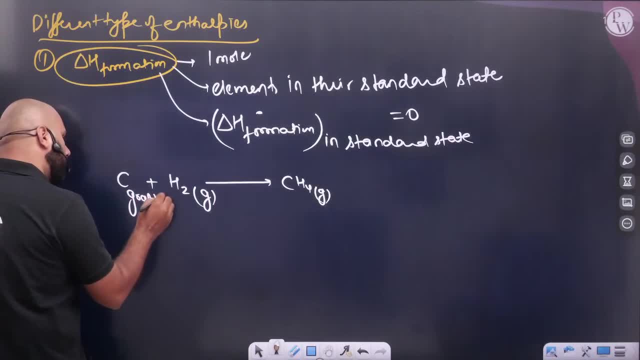 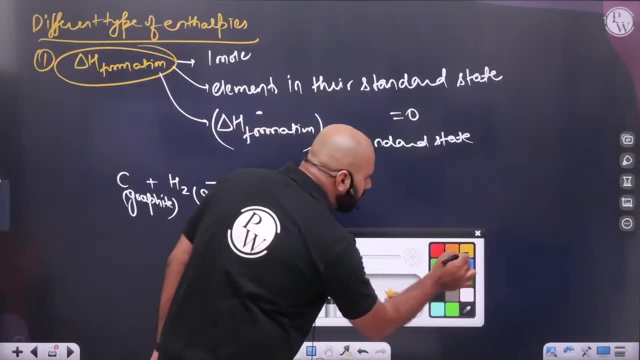 Standard state means Where it naturally exist In the form of hydrogen, In the form of gas, Carbon's standard state, Graphite. It will exist in the form of graphite. So, Sir, this is done While balancing reaction. It should always be one molecule. 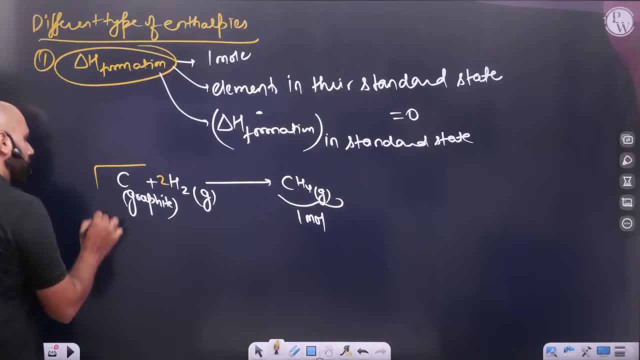 While balancing reaction, What should always be kept? One molecule. You take changes in it, The enthalpy of this reaction, The enthalpy of this reaction, That which is the enthalpy of this reaction. We will keep one molecule. 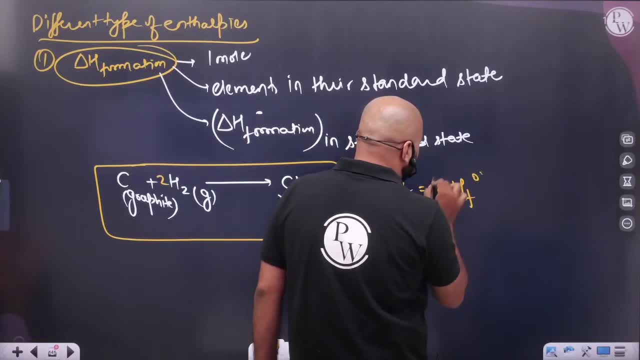 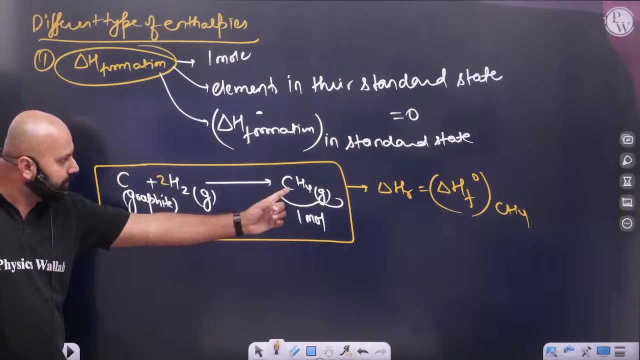 We will keep one molecule enthalpy. what can we call it? Formation enthalpy of CH4.. Just remember, whenever we take any element, we will take elements on this side, we will take elements on this side. the compound: 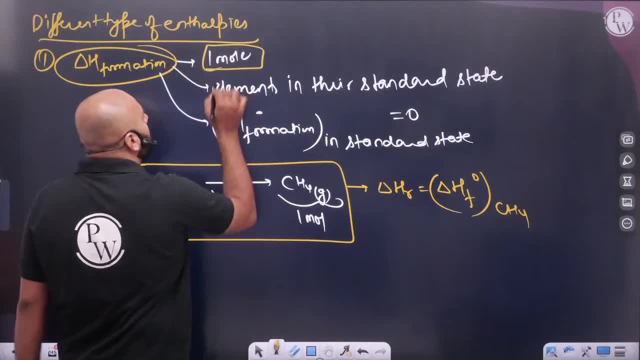 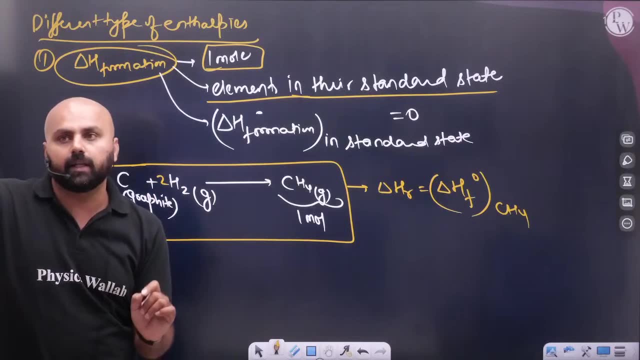 we will take on that side what should be there: 1 mole. Remember this condition: 1 mole elements in their standard state. We have to take elements, not compounds. We have to take elements, not compounds. Take care of this. We have to take elements, not compounds. We have to take 1. 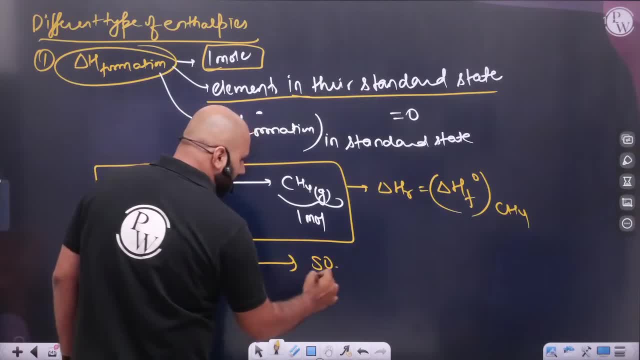 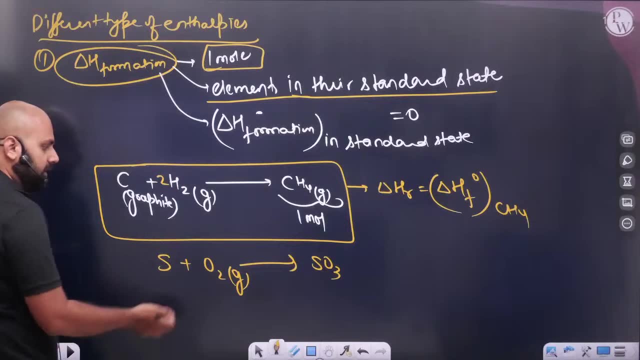 mole. For example, someone said, Sir, I want to make SO3.. How will SO3 be made? So, Sir, there will be sulfur and oxygen. Now, there will be oxygen and gas. Why? Because, Sir, it is easy: Oxygen in which natural state? In gas. If we talk about sulfur, then sulfur. 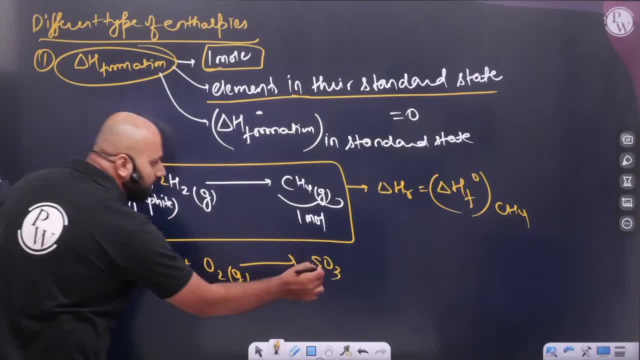 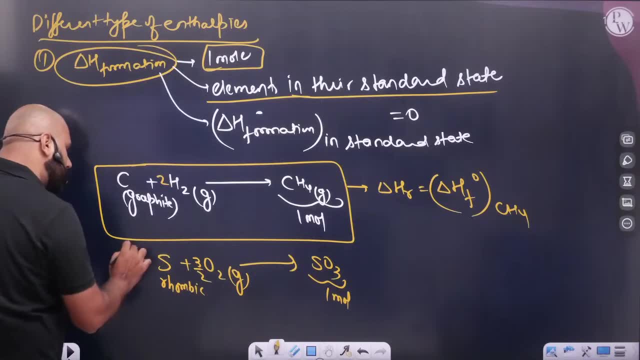 is rhombic, which is naturally available. Sulfur is balanced. Here you cannot balance, You have to keep it as 1 mole. Always remember: you have to keep it as 1 mole. See in thermochemistry. 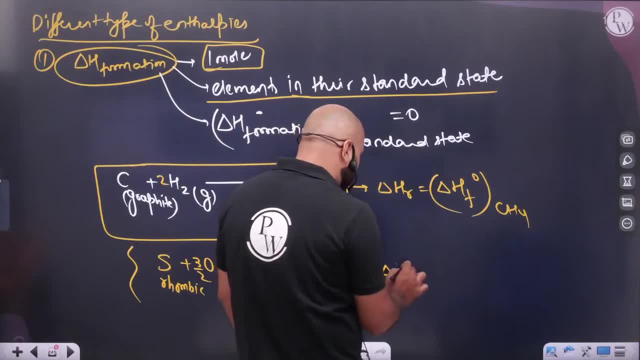 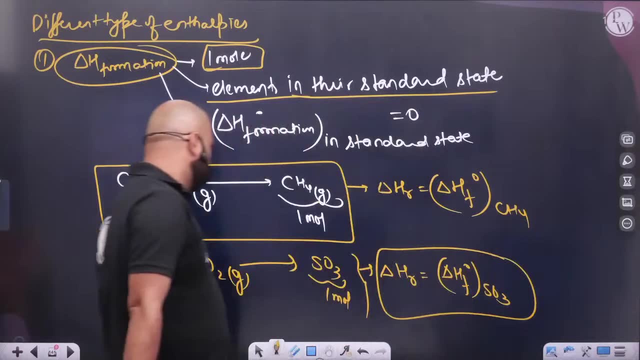 you can do balancing in half The enthalpy of this reaction. what will we call the enthalpy of this reaction? Formation enthalpy of. what should we call it SO3.. We will call form learnt enthalpy of SO3.. Do it, Brother. Okay, So it is that much. 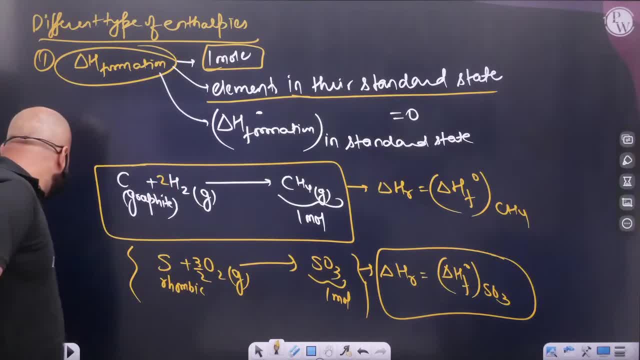 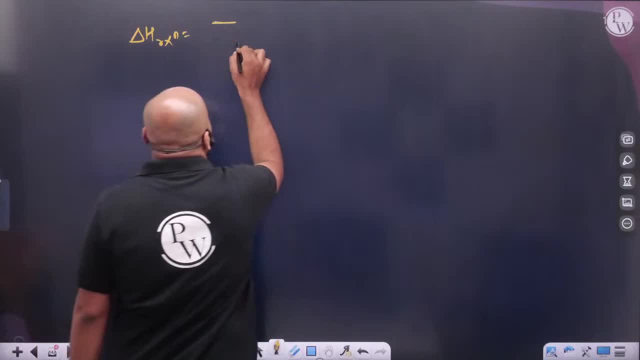 in our hands: Formation enthalpy. This is how we take it out. If all the formation enthalpy is given, assume the reactant product and all have its formation enthalpy, then what would be the enthalpy of the reaction? Formation enthalpy of The ENthALPY is given, then product: 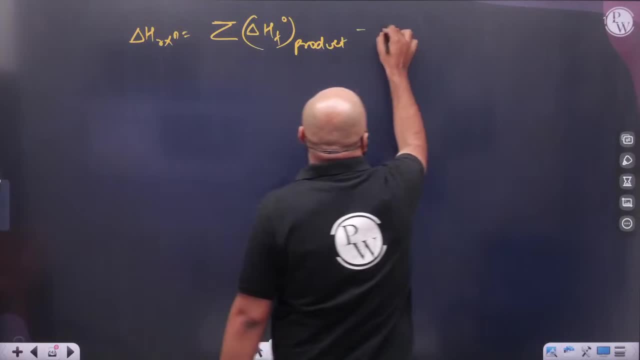 minus Formation enthalpy of will become how Reactant This will happen in us Formation enthalpy of reaction. Formation enthalpy of reaction. Formation enthalpy of reaction. So the ENthALPY of G, the ENthALPY of rains, will represent not of leak добрay temperature. 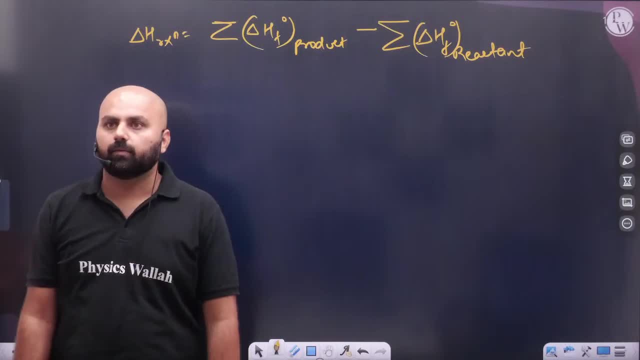 So it'll happen like this here only, Formation NthALPY will be the ENthALPY of the rate of decentralization. It will become reactant. Remove it. Okay, I will give you a break. Let me do thermo chemistry. 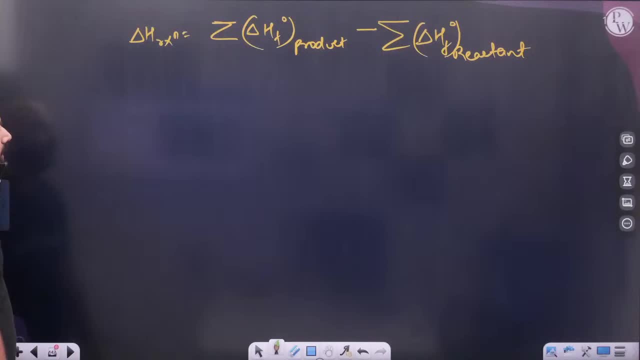 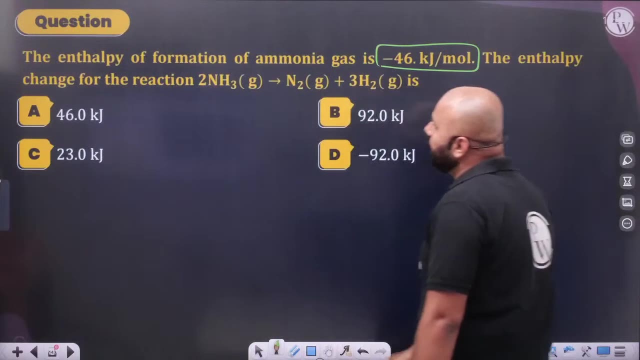 Like anywhere. Now see this question. See this question. What is he saying? How much is the formation of ammonia gas? This much Ammonia gas formation enthalpy Means how ammonia gas will be made Quickly reaction. Just write the reaction in the exam hall. 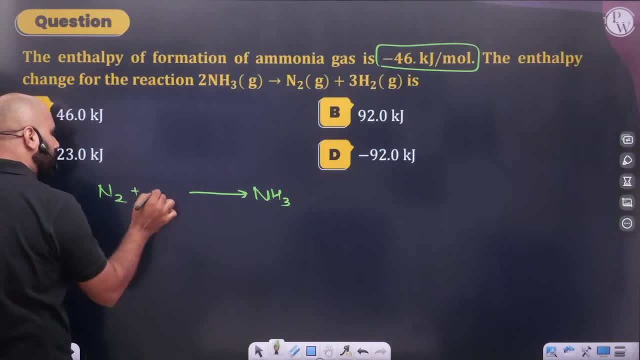 See it with you How ammonia gas will be made. Which elements will be made: Nitrogen and hydrogen. Just remember, You will take only one mole of this. So what will he have to do? 1 by 2.. What will he have to do? 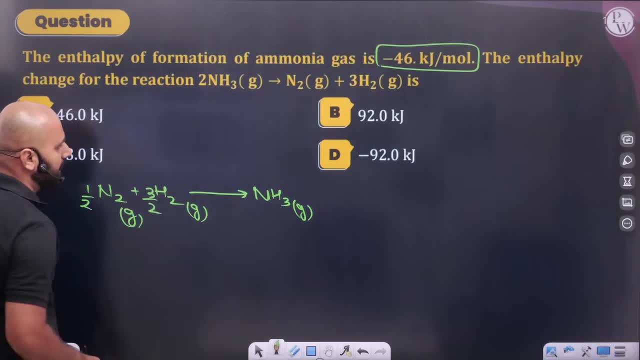 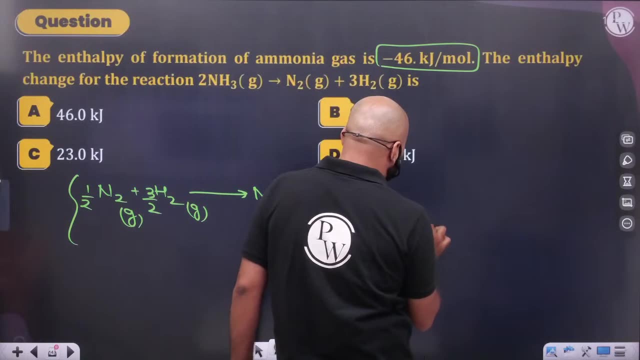 3 by 2.. Nitrogen is also naturally in it. How much enthalpy of this reaction has been given? How much enthalpy of this reaction has been given. Enthalpy of this reaction has been given Minus 46 kilojoules per mole. 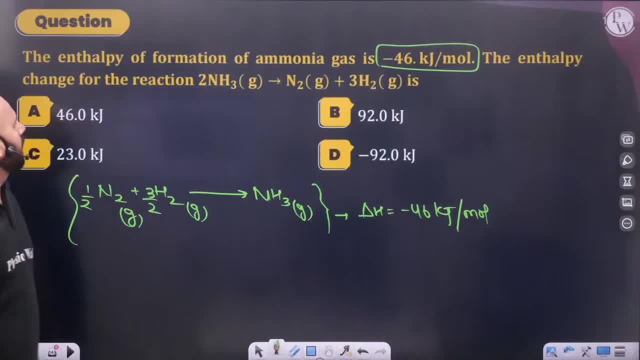 Enthalpy of this reaction has been given. Someone is saying that, sir, Take out the enthalpy of this reaction. How will it come out, Sir? the reaction will have to be reversed. So the reaction will have to be reversed. 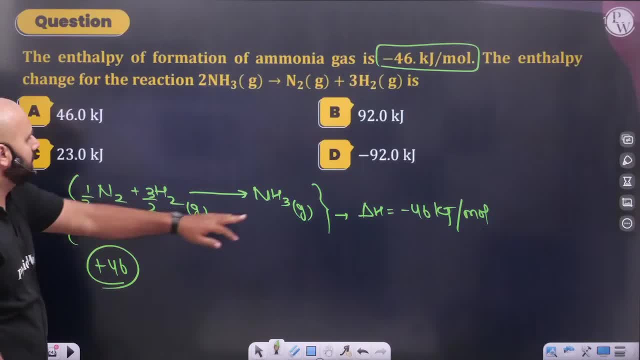 As soon as we reverse the reaction In which minus will it be In the plus? We will reverse the reaction In which minus will it be In the plus, And with whom are you multiplying it With 2.. As soon as you multiply it with 2.. 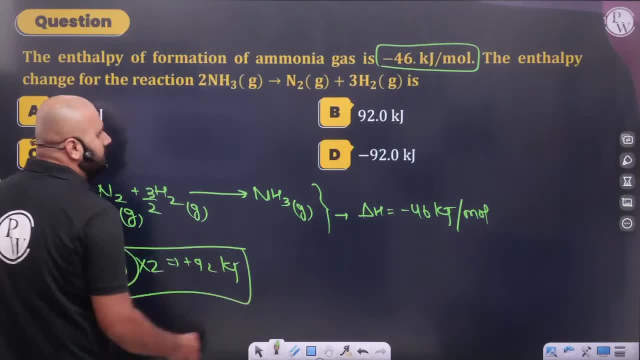 How much will be the answer? Plus 92 kilojoules, Plus 2. 92 kilojoules. What will be the answer? B answer will come. What will be the answer? B answer will come, Nothing else. 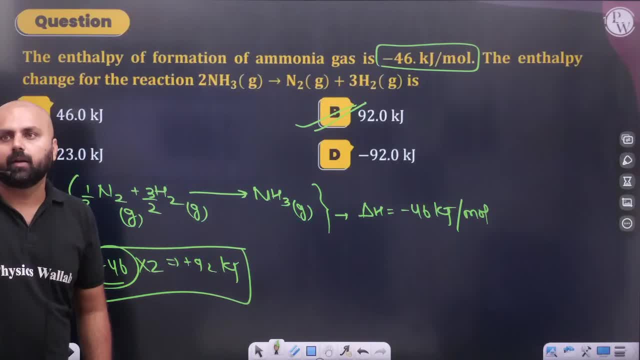 Okay, What will be the answer? B answer will come. That's it. Keep taking out Brother, Only formation, Always product side. If you are writing formation, Then always see the product side. If you are writing formation, Then always keep in mind the product side. 1 mole. 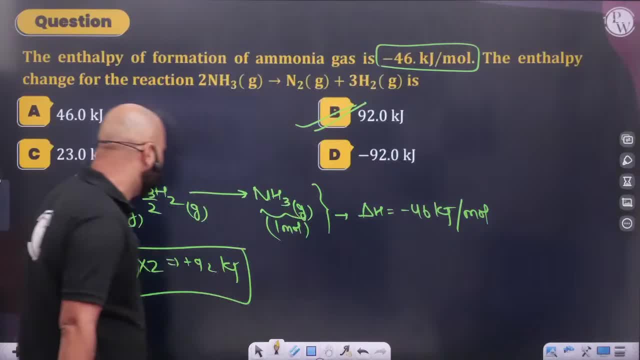 Keep in mind the product side. 1 mole Brother. Why will you keep the reaction side? Let, whatever is there, be the reactant side. If you keep formation, then always keep the product side. Nothing else, Sir. it will happen. It will happen. 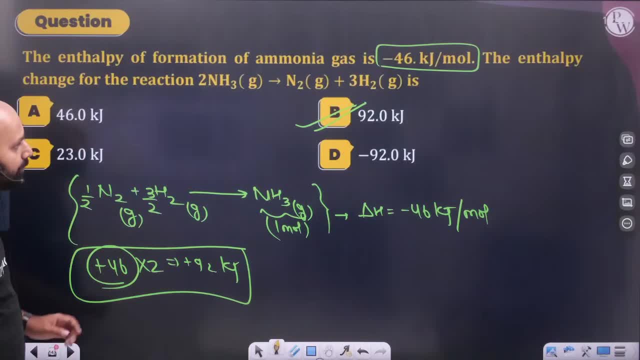 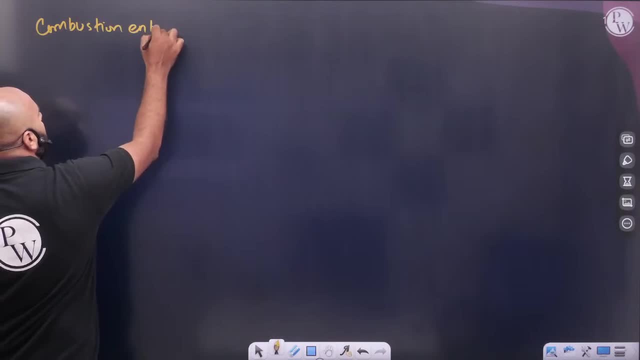 Now see. Now, if it is formation, then it is no problem. But if there would be combustion, If there would be combustion enthalpy- If take yourself, If you have combustion enthalpy, Then, brother, combustion enthalpy 1 is always exothermic. 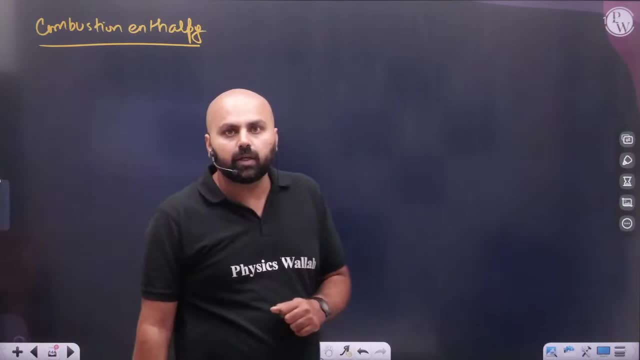 Because, obviously, if you will burn anyone, What will be the energy? It will be released. If you burn someone, what will be the combustion? The energy will be released. If we talk about combustion enthalpy, then what do we do in this? We take one mole. 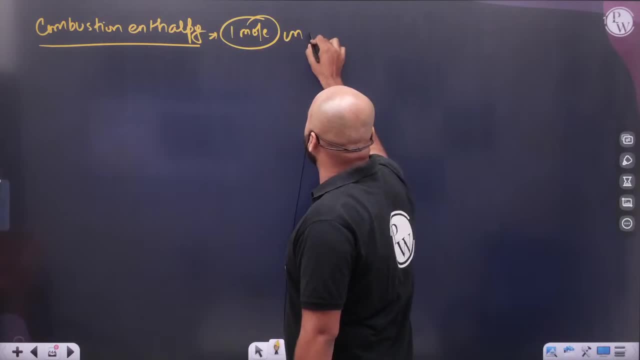 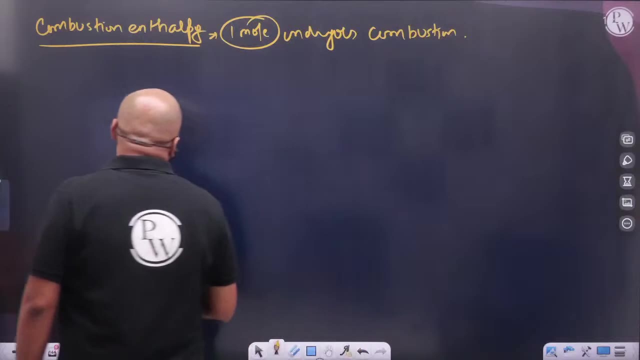 combustion. We do one mole combustion. One mole undergoes combustion. Whenever combustion enthalpy will be defined, look carefully If you are ever taking combustion enthalpy. suppose you have C3H8, you are writing its combustion enthalpy. 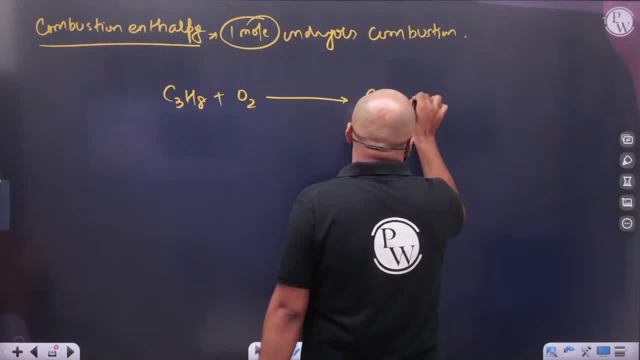 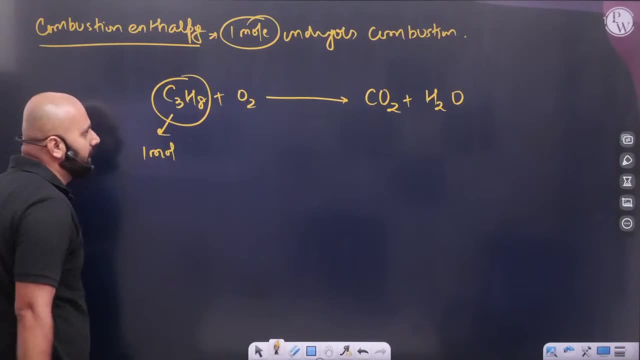 you are writing combustion reaction, then how will you write combustion reaction: Cu2 plus H2O? You will have to fix this. If you don't fix this one mole, you will face problems. Balance- everything else, 3 is done. How much is this? 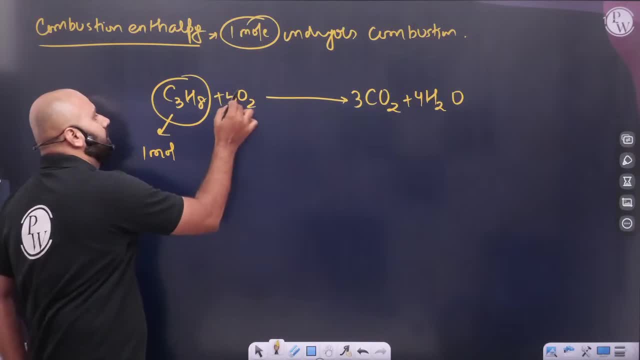 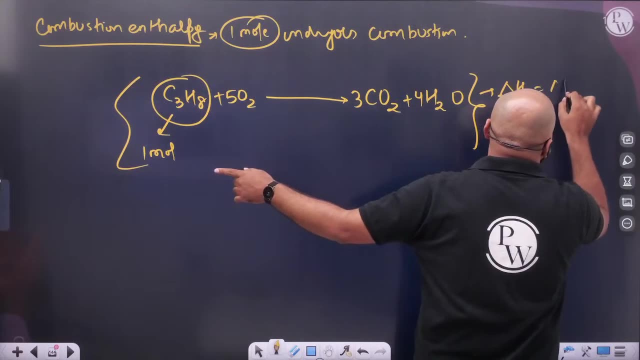 4. 3 to the power. 6. How much is this? 5. This reaction's enthalpy, this reaction's enthalpy, this reaction's enthalpy, what will we call it? Combustion enthalpy of. 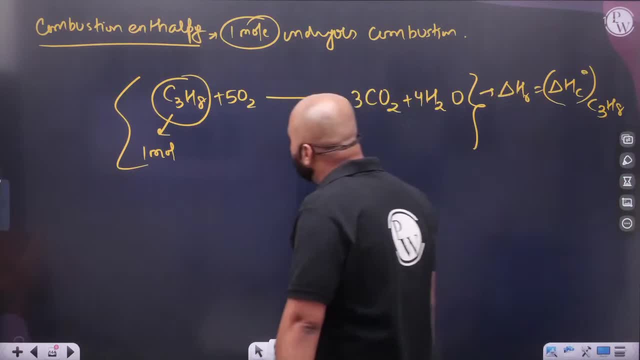 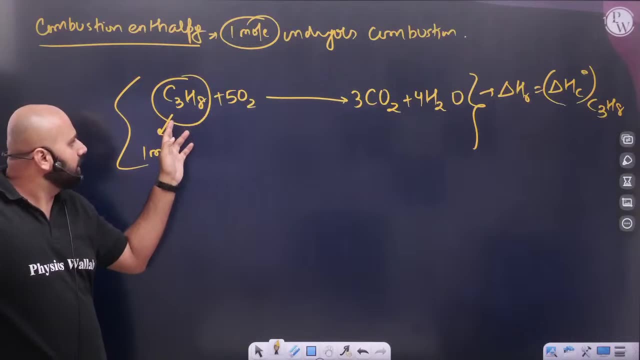 combustion enthalpy of C3H8.. Why? Because in this reaction, C3H8 is completely. C3H8 is completely. what will be happening? What will happen completely From one mole. see What is happening from one mole. 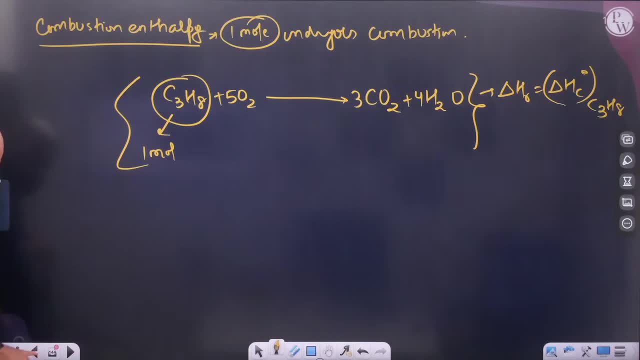 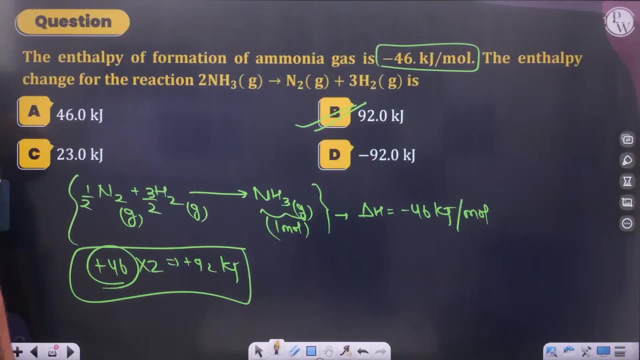 Combustion is happening. It will release so much energy. What a change Will we divide in the last question? How will we divide in the last question, In this reaction and in this reaction? what is the relation? We will multiply it. 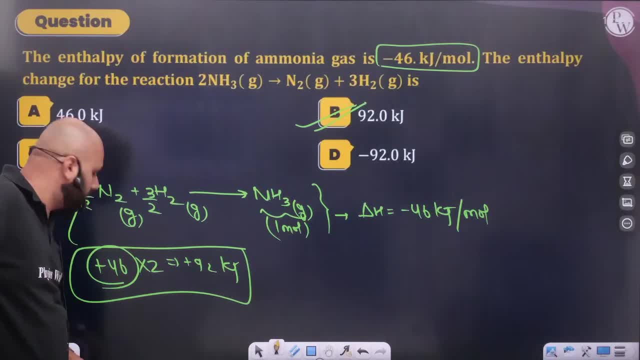 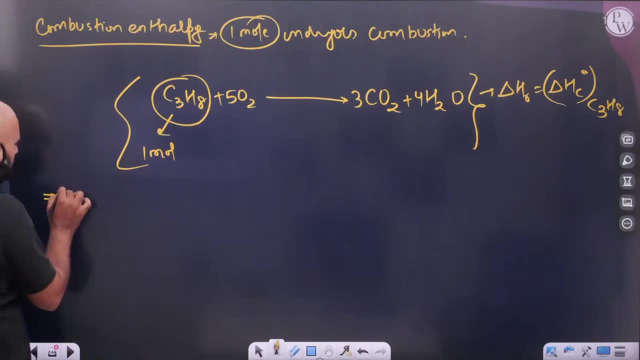 If you will do it upside down, multiply it with 2.. When you will multiply it with 2, it will be multiplied with 92.. Ok, After that, if combustion enthalpy, if combustion enthalpy of if combustion enthalpy is given. 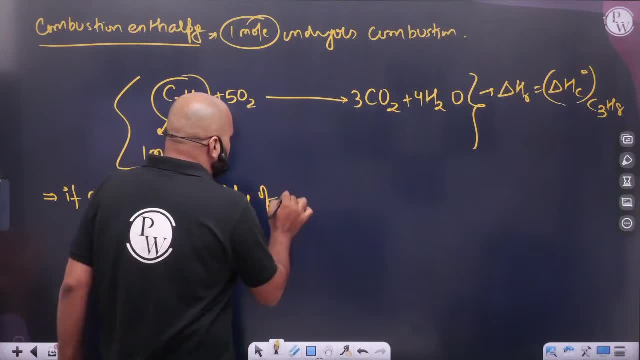 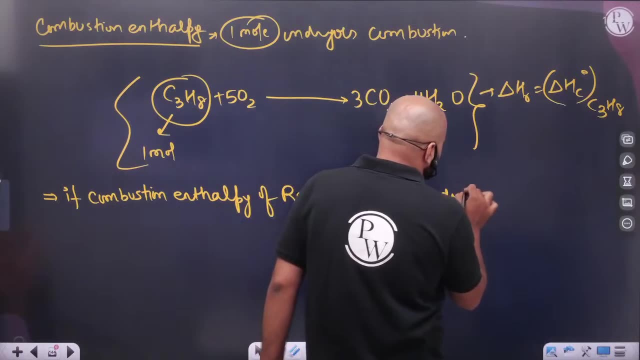 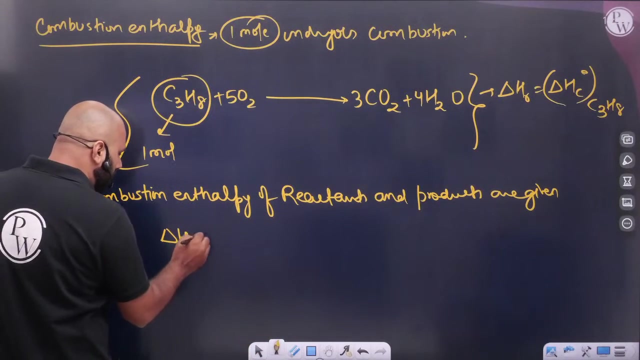 if keep in mind, if combustion enthalpy of reactant and products are given, if combustion enthalpy reactants and whose is given Products given, So in that case, in that case, in that case enthalpy of reaction. 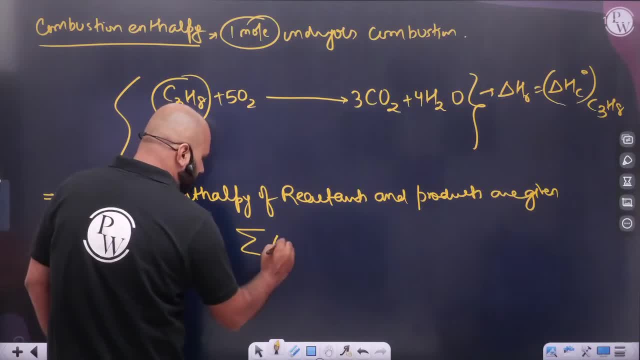 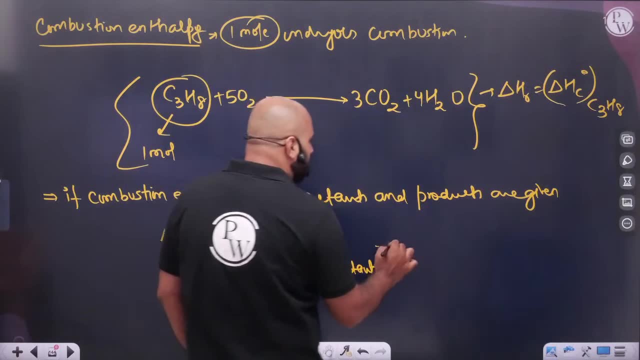 enthalpy of reaction. what will happen? See it with you. Keep exception in mind: Combustion enthalpy of reactants. Combustion enthalpy of reactants minus combustion enthalpy of combustion enthalpy of products will happen. 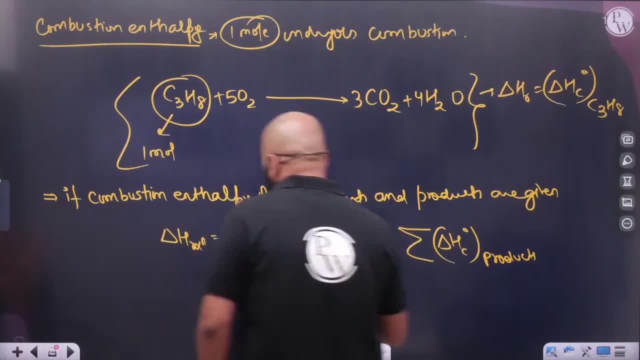 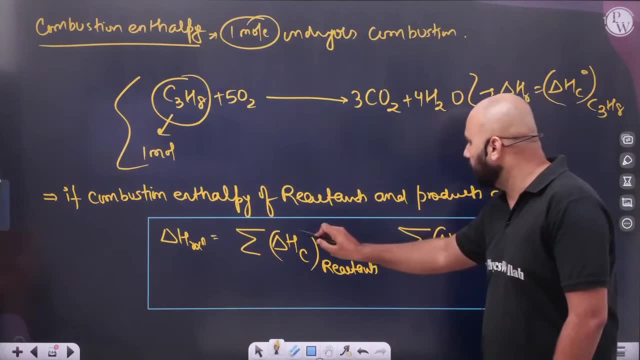 What will happen. This was my exception, This was my exception, This was our exception. If we have given combustion enthalpy, then in reactants and products- see this- combustion enthalpy is reactant minus product. What is combustion enthalpy? 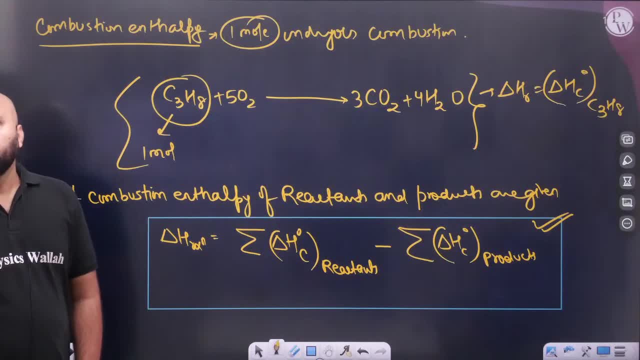 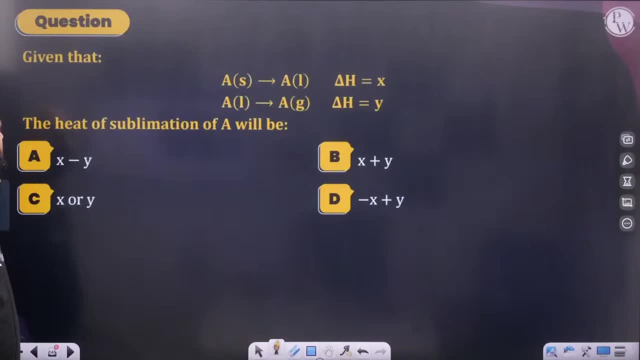 Reactant minus product. Ok, What will be? combustion enthalpy? Reactant minus product. See this question given to us: Sublimation enthalpy. What does sublimation mean? Everyone knows where to go from solid to gas. 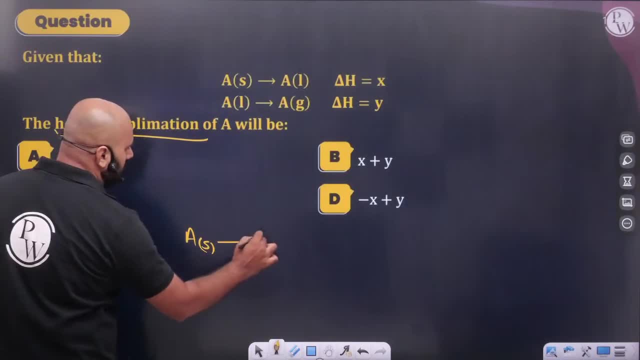 What is being told to you? Where to go from solid to gas, A solid to A gas. what will happen? What will we do to bring this reaction? Will we add these two? Will we add these two? As soon as we add these two? 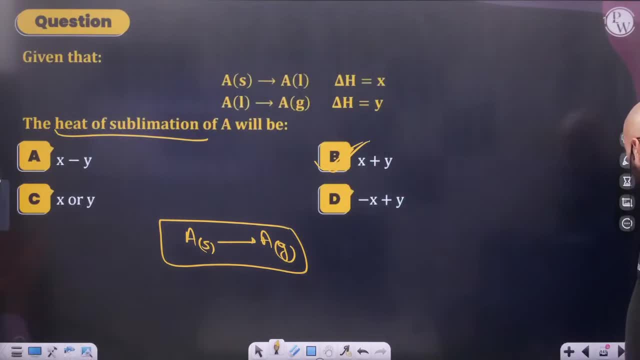 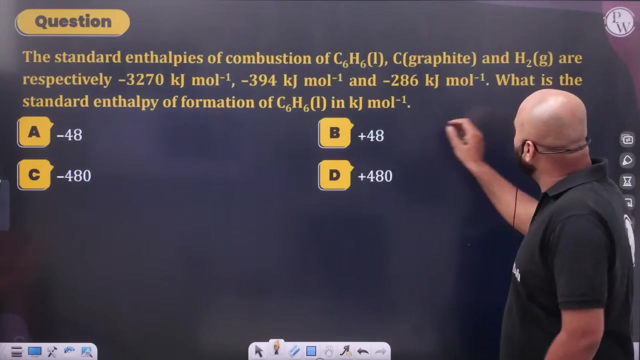 what will be enthalpy? It will be added. What will be enthalpy? It will be added. Do it. What will be enthalpy? It will be added. See this: Combustion enthalpy is given to everyone. 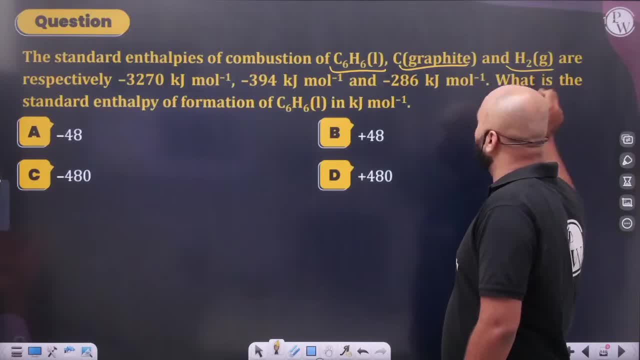 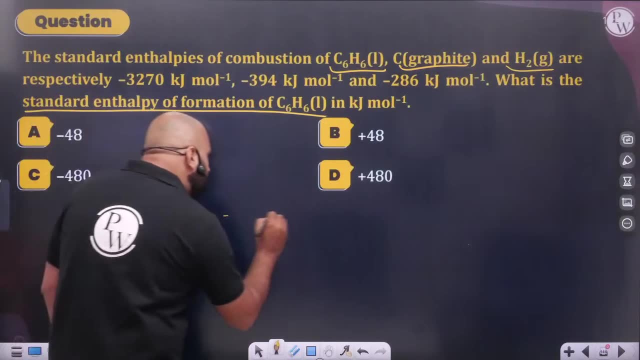 See this: carbon hydrogen. all have combustion enthalpy. What is being said? Enthalpy of formation of benzene. First, tell me how will be the enthalpy of benzene. How will you write the enthalpy of benzene? 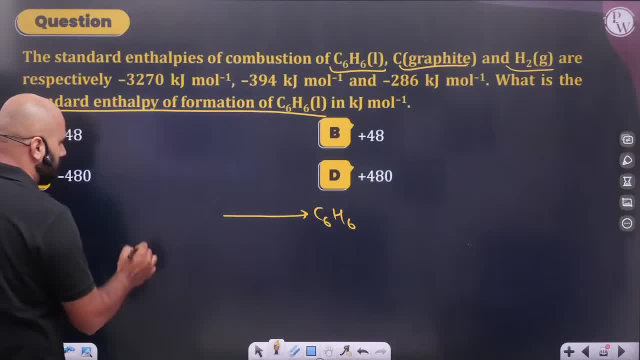 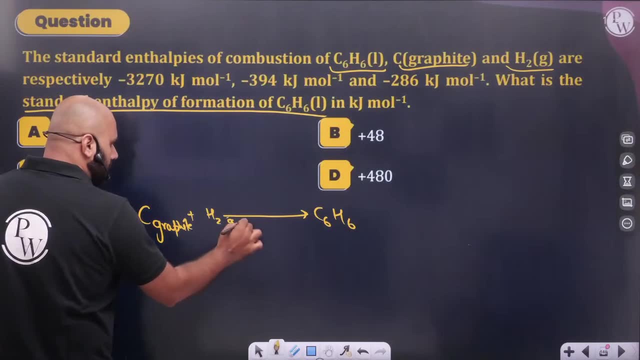 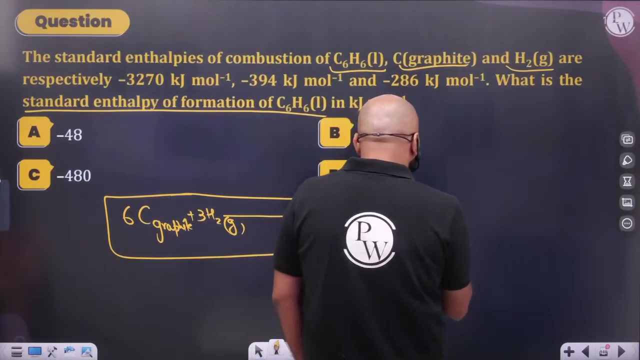 How will you write? See, this is a very beautiful question. Carbon will be there. How will you write its formation? enthalpy Graphite plus hydrogen gas, carbon 6, hydrogen 3.. Now, what are you going to do to remove therecipion enthalpy? 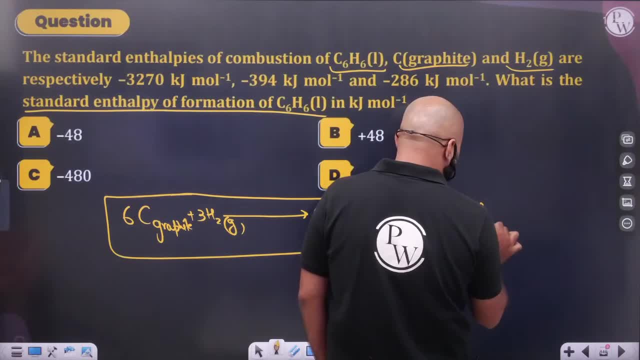 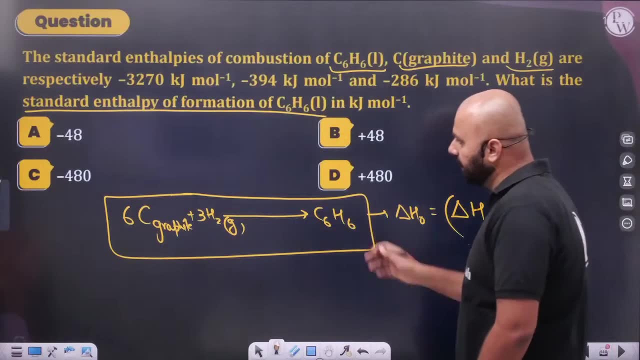 What are you going to call the enthalpy of Post reaction enthalpy? Formation enthalpy of C6H6.. Formation enthalpy of C 6H6.. We are going to take this out, Sir. what is time going to? 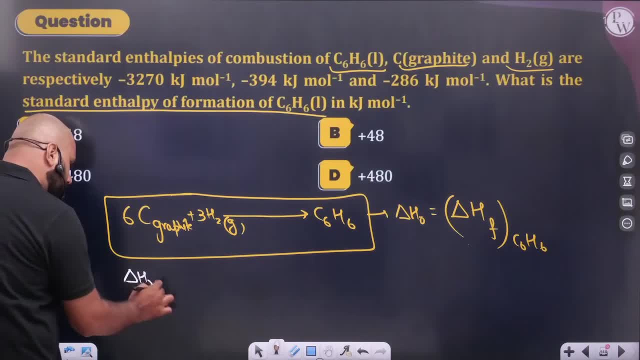 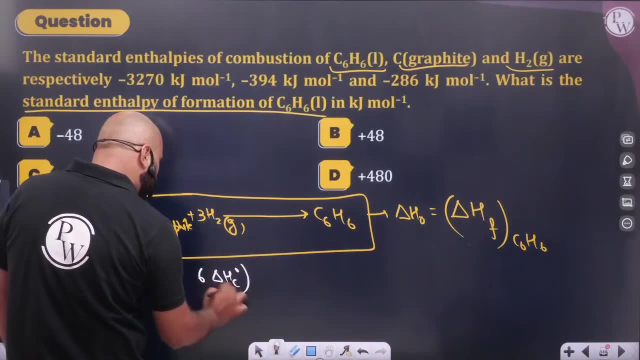 become? What will happen? How will you take this enthalpy of contradiction, Sir? what do we do before? In combustion enthalpy, we do reactant first. In combustion enthalpy, what we do first, We do reactant. Sir, we have to do reactant first. 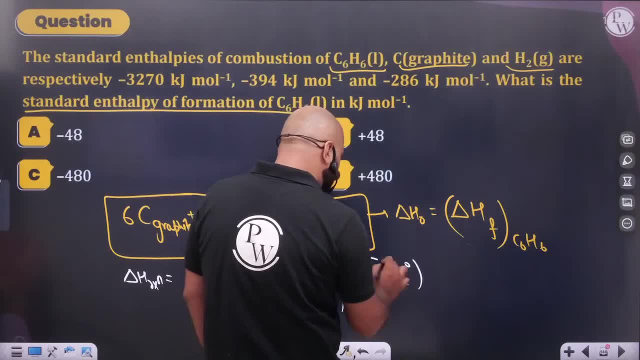 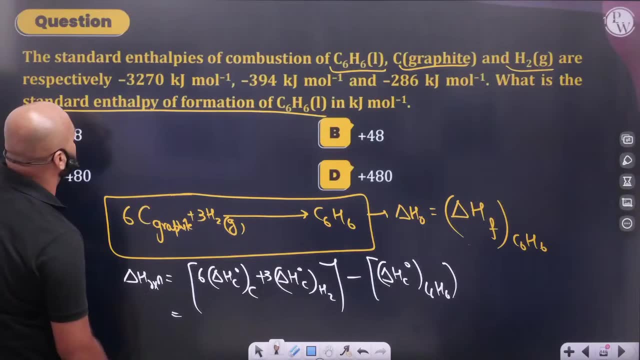 What will we do? minus Combustion enthalpy? off, Sir. in combustion enthalpy we had to do the opposite. So what did we do? 6 times carbon's combustion enthalpy, 6 times carbon's combustion enthalpy. 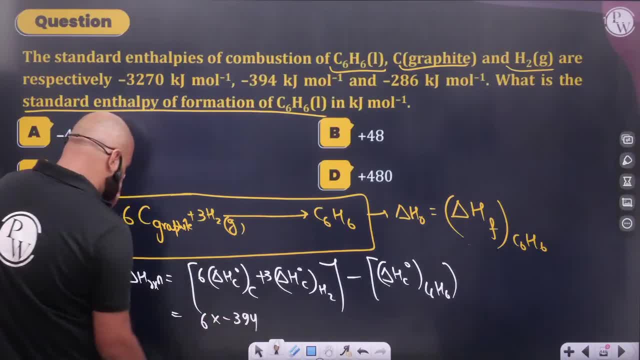 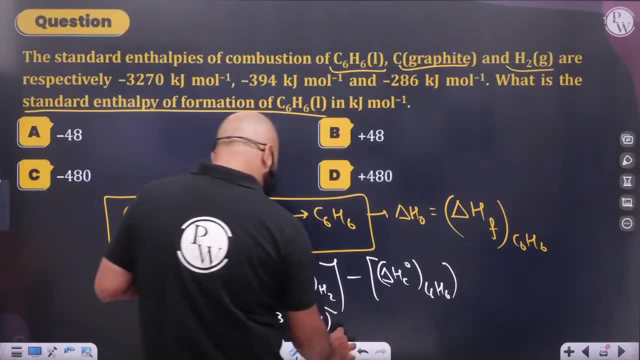 So how much is 6 times Minus 394.. And how much will it be here 3 times of hydrogen, so minus 286.. Minus this hydrogen's C6H6, how much will it be Minus 3270.. 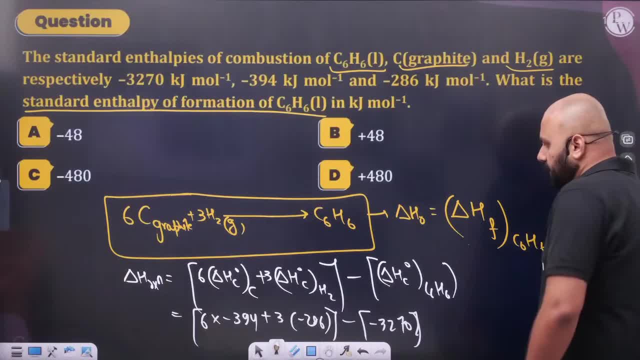 If we solve this, then how much will it be That 6 times 94,? how much will it be? Sir, you will quickly calculate that in exam hall you will also have this much time: 24, 9x6 is 54, and 54 and plus 2, 56, 9x6 is 18,, 23.. 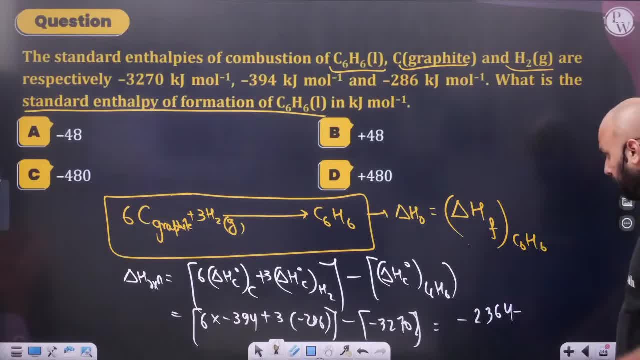 And how much is this Minus 6,? 18 is done And 24,. 25 is done And 6,, 6 and 8 is done, And how much will be plus 3270.. In exam hall we will have to do this quickly. 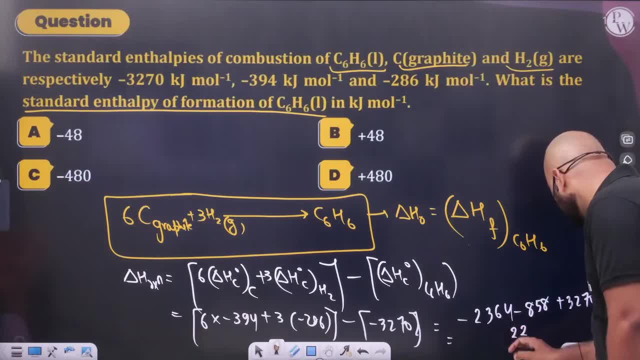 12,, 6,, 5, 12 and 8,, 3, 11.. 11,, 12 and 3, 3270.. How much will it be Plus 48 will come? How much will it be Plus 48 will come? 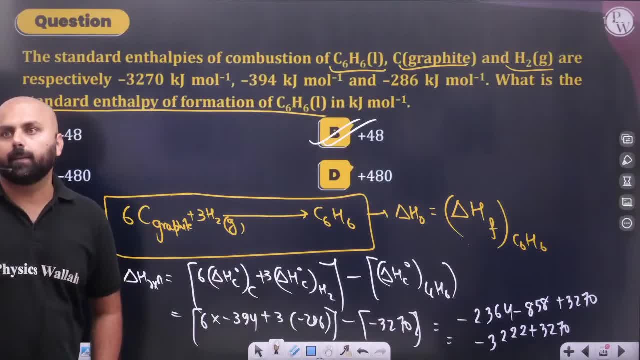 So how much will be formation enthalpy? Plus 48 will come. Okay, If you are sure, then just keep taking out. Plus 48 will come. Minus is not coming. If someone is getting minus then he is doing a mistake. 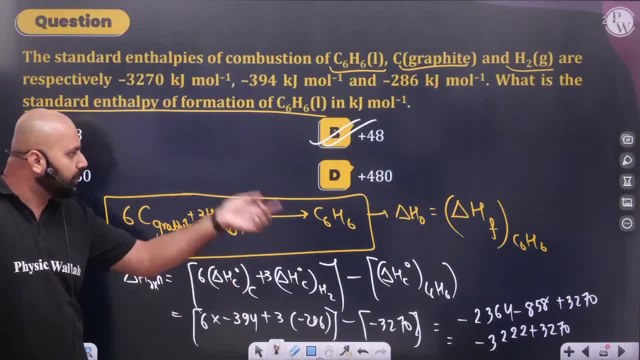 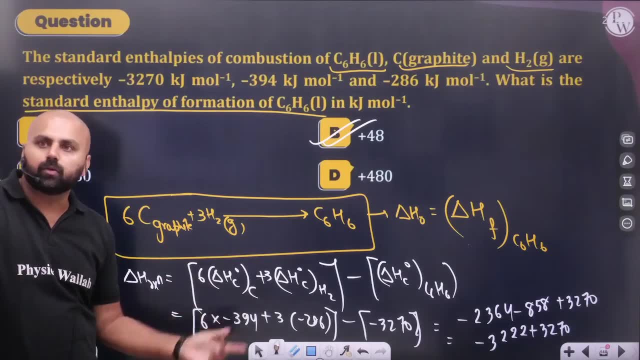 Combustion enthalpy is obvious, Reactant is also given and product is also given. So if the combustion enthalpy is given, then we will do reactant minus product, We will do reactant minus product. So we have to question ourselves in this way. 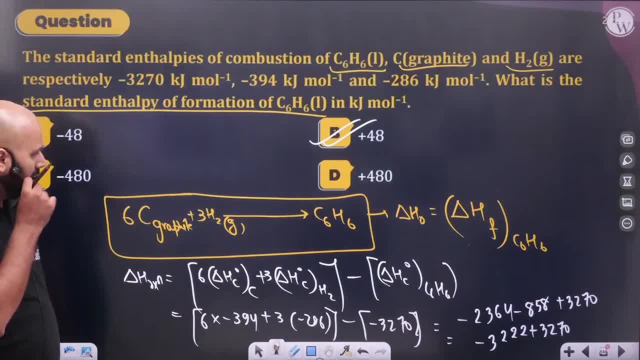 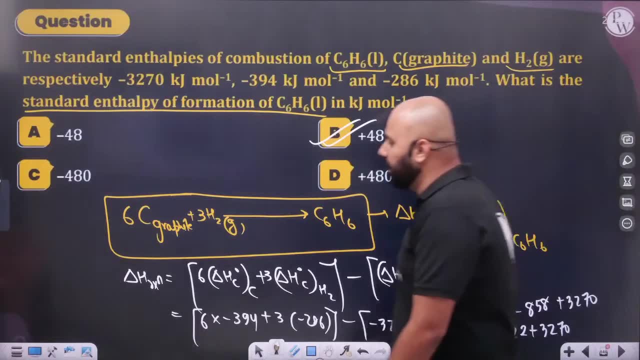 Okay, So take care of this. Okay, So formation. I don't mean by formation, I was told to take out the enthalpy of this reaction. Brother, look at yourself, Look at yourself. I am telling you the same thing. 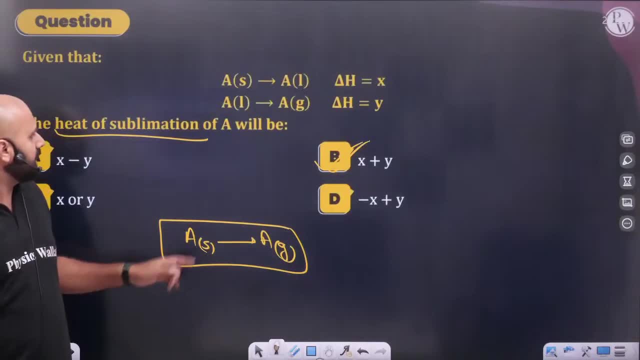 Why are you confusing? Look at this- When you are being told that combustion enthalpy is given, Combustion enthalpy is given of which? Of reactant and product. So why do I have to do in that case? 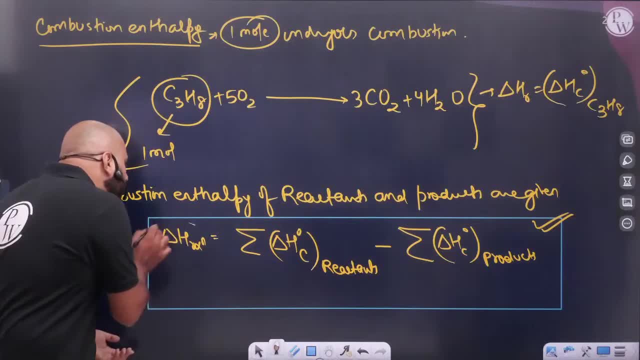 Okay, What do I have to do in that case? Reactant minus. I don't know if that reaction is of formation or sublimation, I don't care, You just see that directly. Okay, See that directly that I have to take out the enthalpy of that reaction. 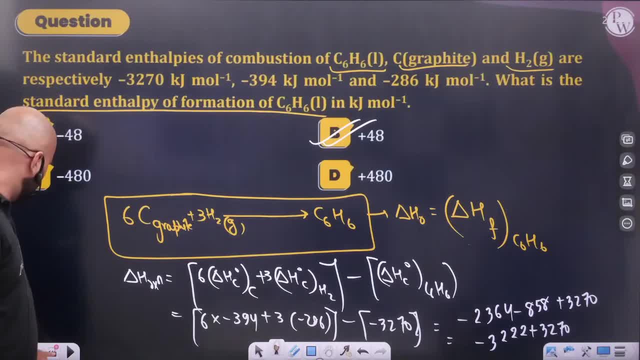 Whether it is formation or combustion. whatever it is, let it be. Now let's come to the next. So what is given in the next Bond dissociation enthalpy? Bond dissociation, enthalpy, you know it. 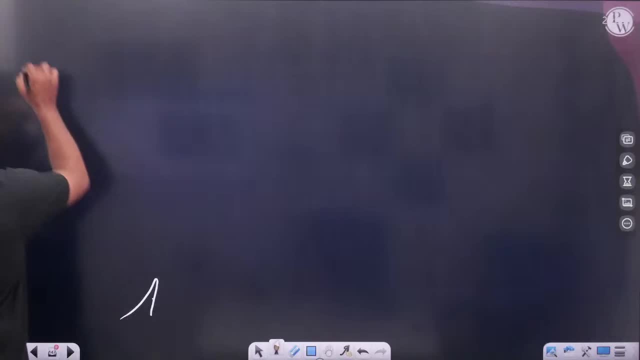 If there is bond dissociation enthalpy. see, there are two types of things. One is bond dissociation, Bond dissociation, and one is bond enthalpy. See, bond enthalpy is of two types. Remember, if suppose bond is being formed somewhere. 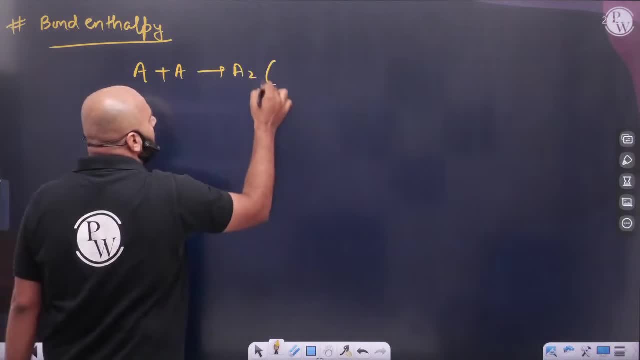 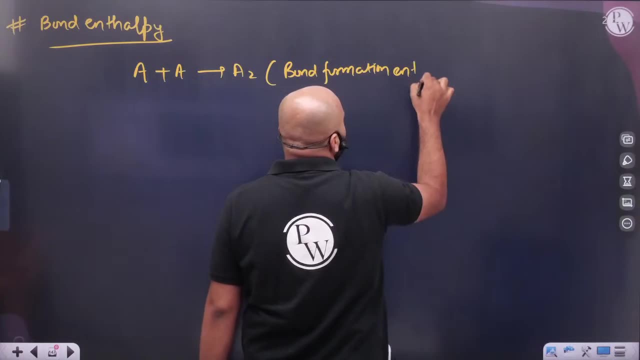 A plus A, If A2 is being formed, then, sir, what is this? Bond formation is there And whenever there is bond formation, enthalpy. Bond formation enthalpy is generally what happens. Bond formation enthalpy is negative. 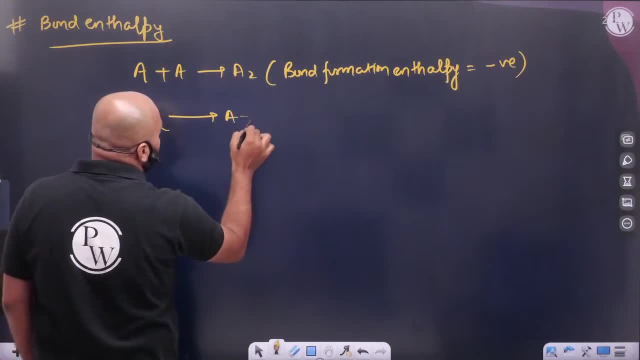 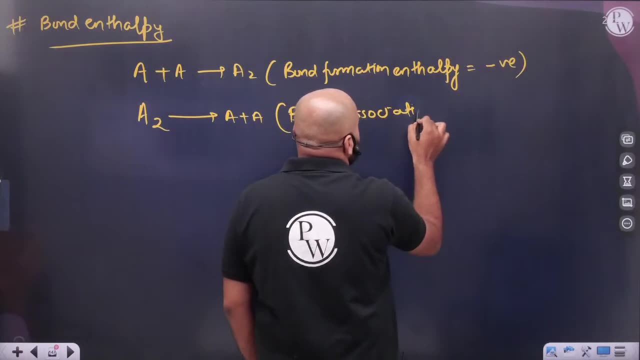 And if A2 is breaking here, A plus A is being formed, then we call it bond dissociation enthalpy. And what happens to bond dissociation enthalpy? It becomes positive. So whether bond dissociation is written in the exam wall or not, you will come to know. 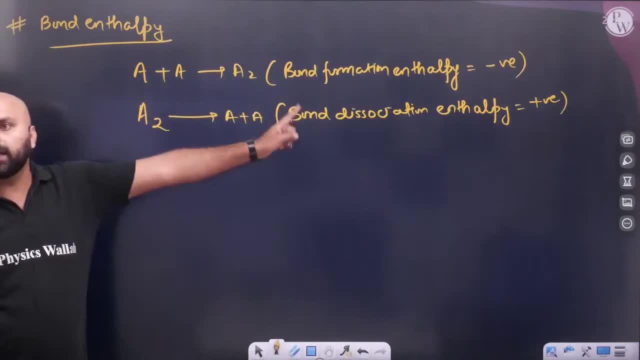 by looking at the sign that bond dissociation enthalpy. If bond enthalpy is positive, then brother, take care of this. Okay, Look at this Now. bond dissociation enthalpy After this, if it is in polyatomic molecule: 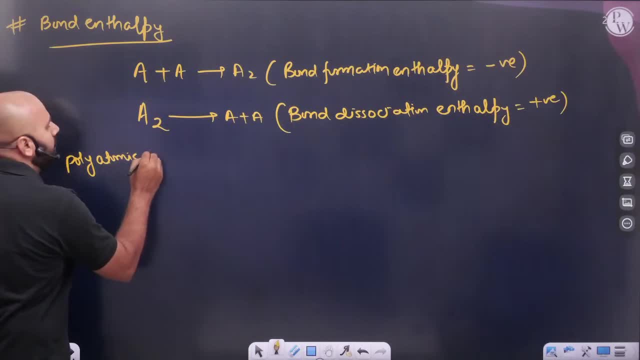 If it is in polyatomic molecule, then there. polyatomic molecule means, Sir, where there are more than one atoms, Like there is CH4.. So what will happen in CH4? There will be four such enthalpies in CH4.. 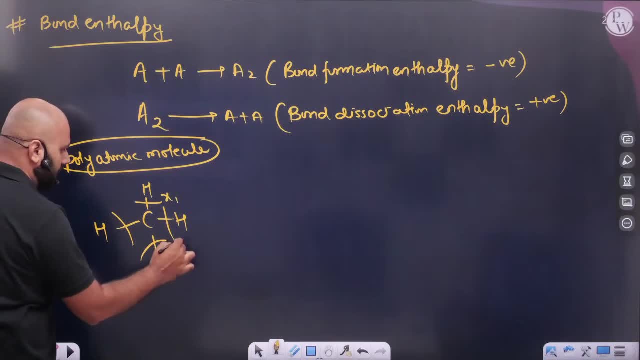 One, two, three, four. Sir, if its value is X1, its value is X2, its value is X3, its value is X4. All four bonds will not be equal, Because you only know that the shape structure will be correct. 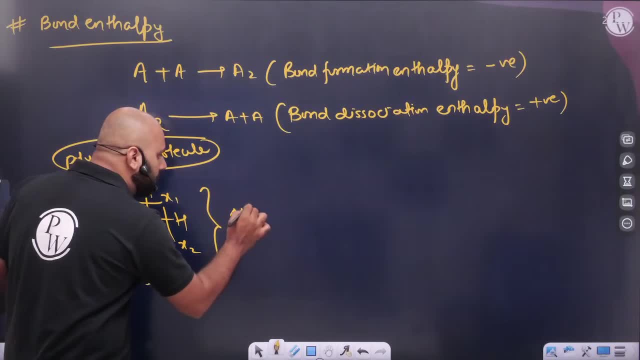 So obviously all four bonds will not be equal. So what do we do here? We take out average, We take out average bond enthalpy, We take out average bond enthalpy. And how do we take it out? There are four bonds. 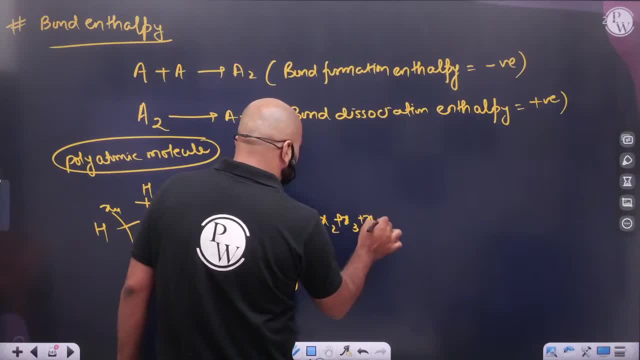 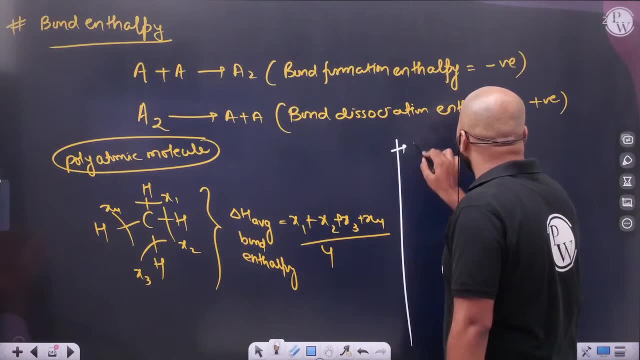 X1 plus X2 plus X3 plus what will be X4, and divide by average. What do we do in polyatomic case? We take out average bond enthalpy. Keep in mind a simple thing: If bond dissociation enthalpy is given, 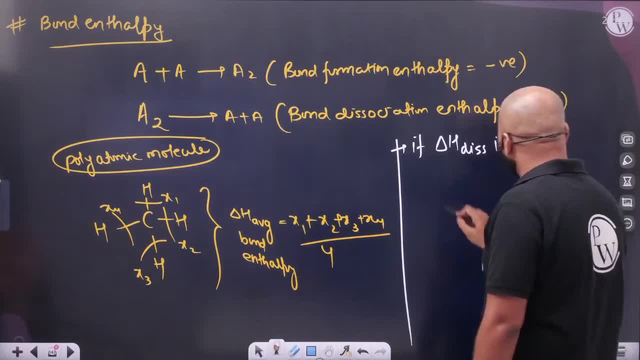 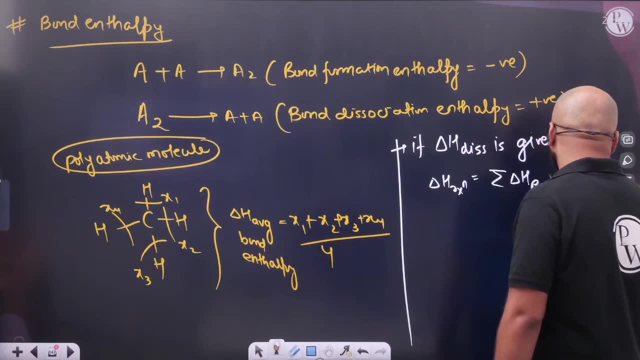 if dissociation enthalpy is given, If bond dissociation enthalpy is given, then what will be the enthalpy of the reaction? See that with you, Reactant minus, reactant minus will be the product. Why? Because you know that this reaction will go in reverse. 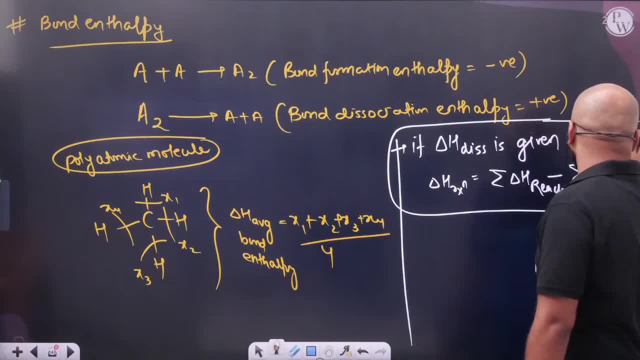 If bond dissociation enthalpy is given, then it will go in reverse. But if bond formation enthalpy is given, then there is no tension in that case. If bond formation enthalpy is given, then there is no tension in that case. 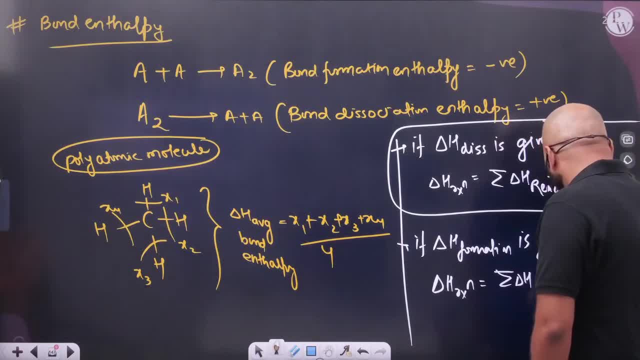 What will you do, Sir? in that case, delta H will be product minus reactant. In that case, delta H will be product minus reactant. In that case, product minus reactant will be done. So keep this in mind, Nothing else. 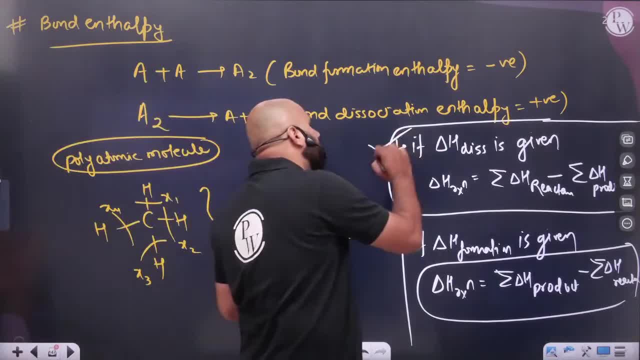 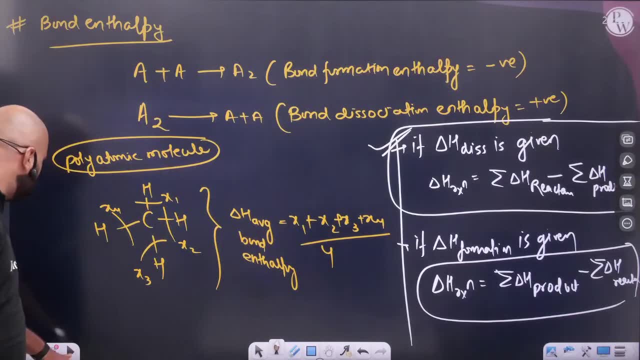 Okay, Just remember, brother, if there is dissociation, then only there is tension. Otherwise, if there is dissociation, then there is no problem. How will you recognize dissociation? Nothing, Nothing for dissociation. Look at yourself: Whenever dissociation is given, then the value will be positive. 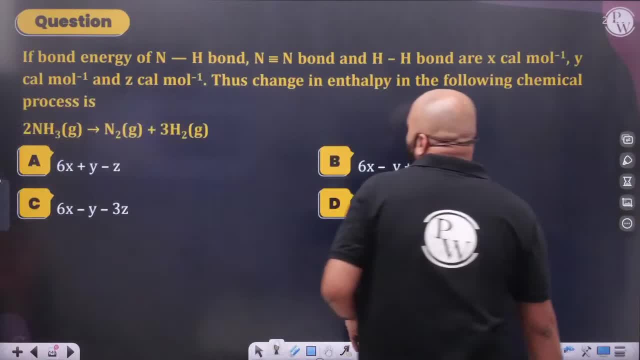 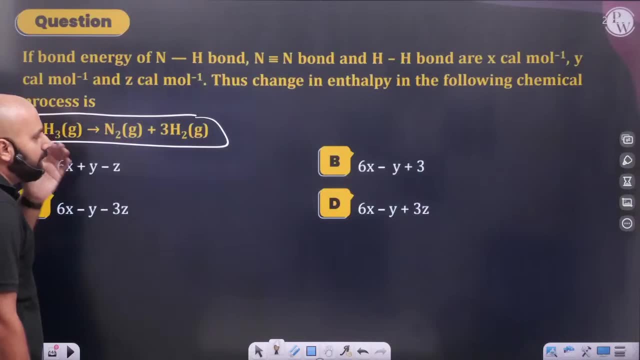 As it is written here: bond energy, NH, NH. Its value has been given. Calculate the enthalpy of this reaction, Enthalpy of this reaction When normal bond enthalpy means that, brother, it is talking about dissociate. Tell me one thing in this reaction. 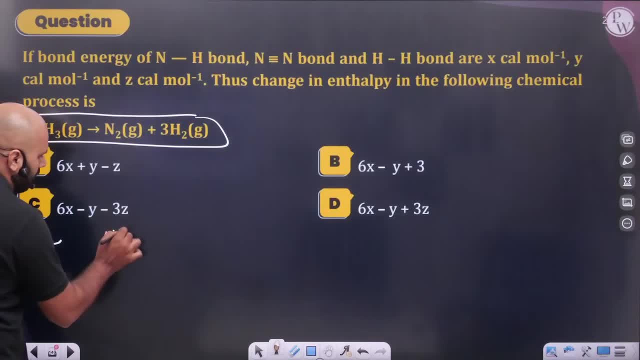 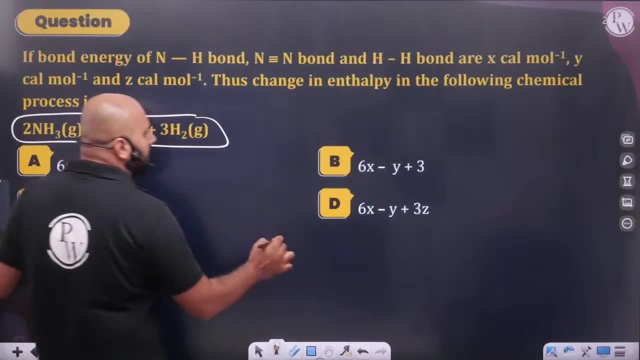 How will you get the enthalpy of this reaction? Sir, if we will go to get the enthalpy of this reaction, Then we will do reactant minus product. How many bonds are there in reactant? How many NH bonds are there in ammonia? 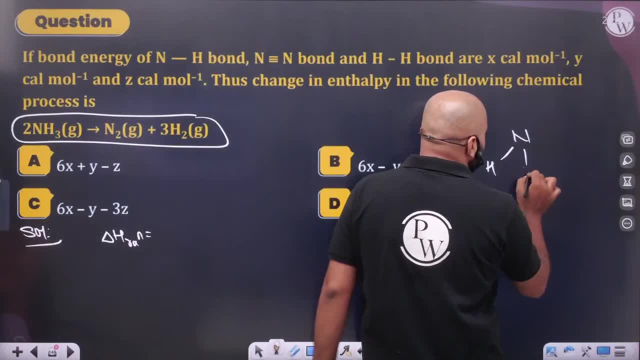 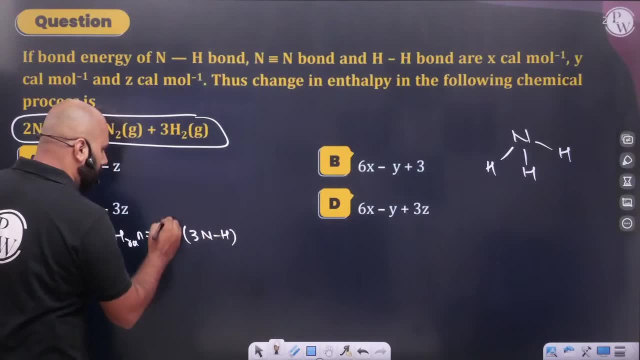 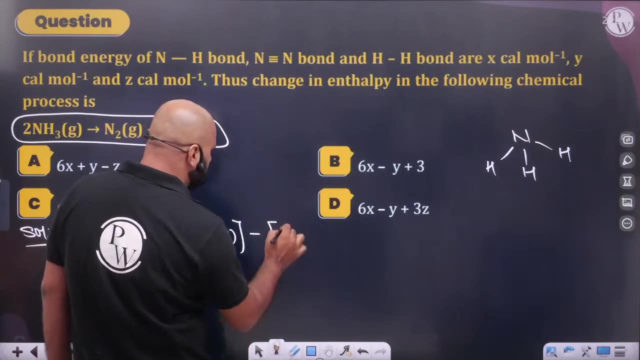 Look at it. How many bonds are there in NH bonds? It is two times of three. Look at the bonds of reactant. Sir, this happened. The bonds of reactant is this: Look at the bonds of minus product, Then triple bond N is done. 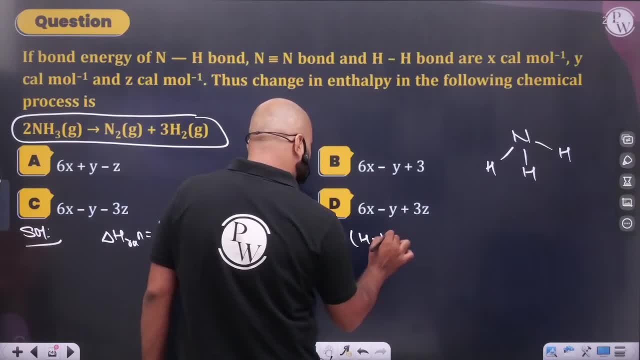 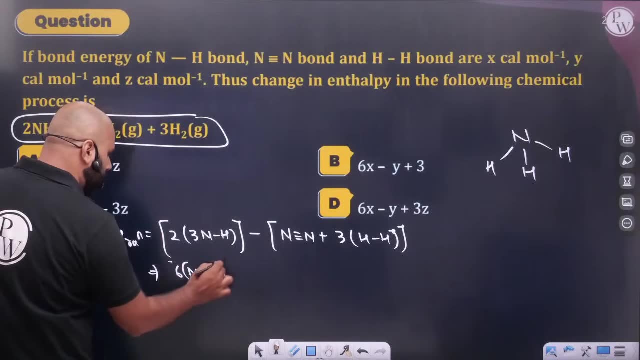 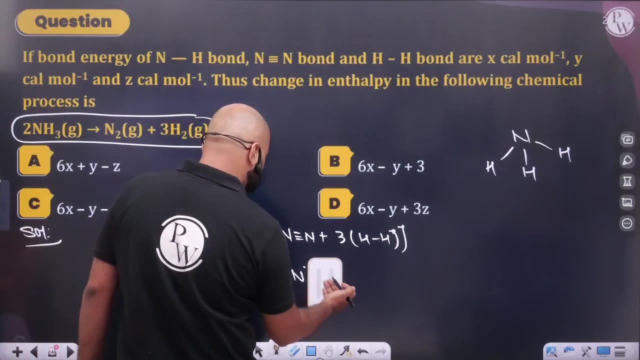 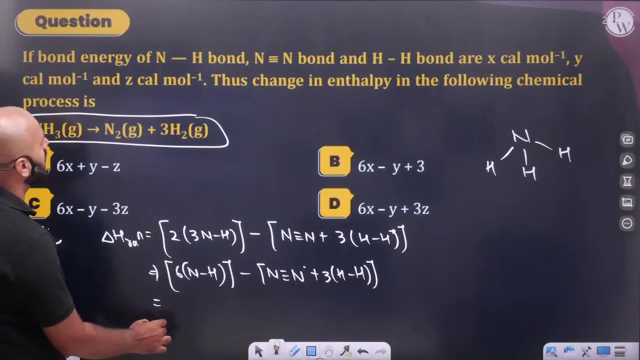 Plus three times single bond H is done. Look at this, If I want to write it straight, then six times the bond of NH is done. bond is 6 times NH. bond is minus N. triple bond: N plus 3 HH. see what happened. 6NH bond is 6X and. 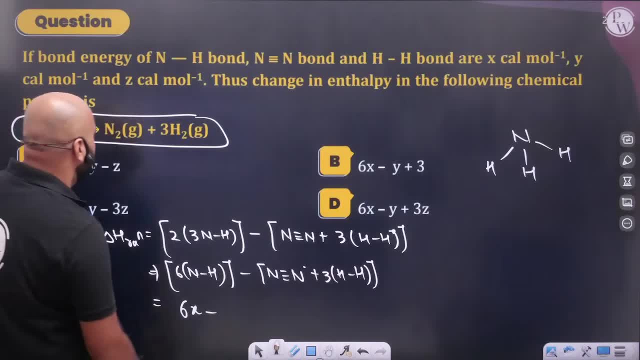 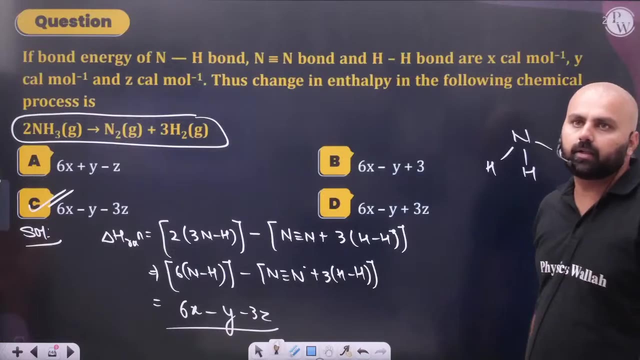 here will be minus N. triple bond: N is Y, so this is Y minus and its value is plus minus 3Z, so its value will be 6X minus Y minus 3Z. the answer will be 6X minus Y plus 3Z, so just keep doing this. 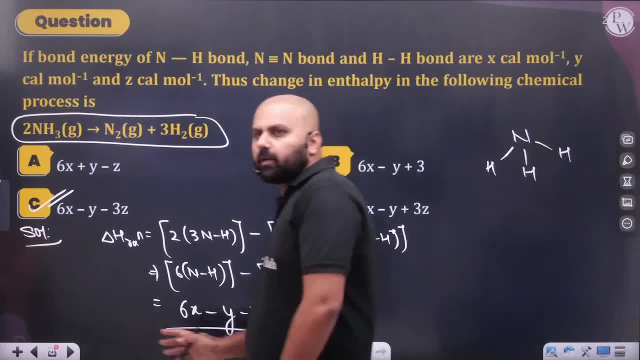 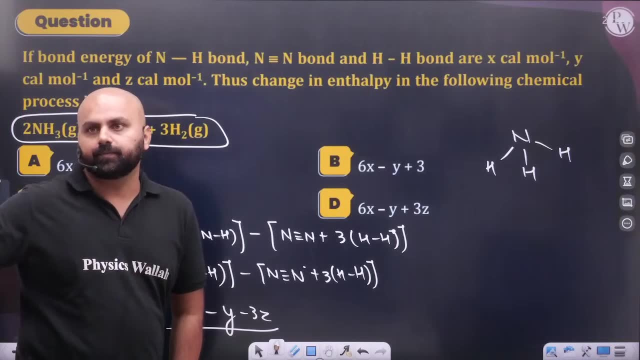 bond enthalpy is just giving this chapter. I will finish this one. thermo chemistry will be finished. thermonics, thermo chemistry- now major, major chapters are there, chemical, ionic, all are there. yes, we will do it today. we have time, we will do it. we have to finish it now after so many days. 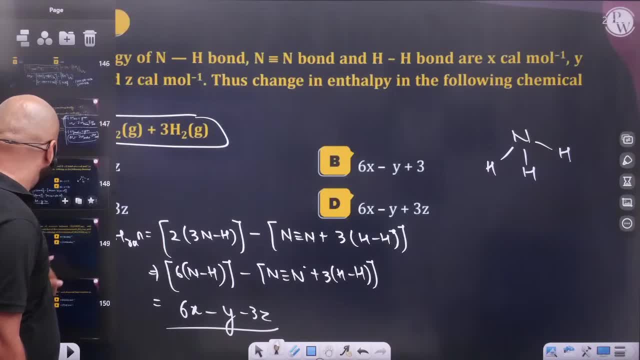 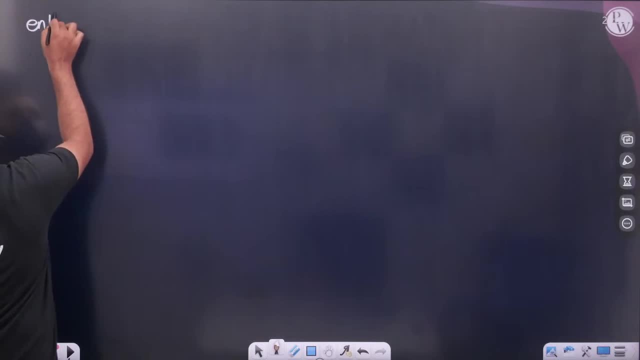 we are getting it now. we are getting it last, so we will finish it now. see one more thing. we call it enthalpy of neutralization. you have to see carefully. one is enthalpy of neutralization. what is enthalpy of neutralization? that, brother, if someone tells you to talk about enthalpy of neutralization, 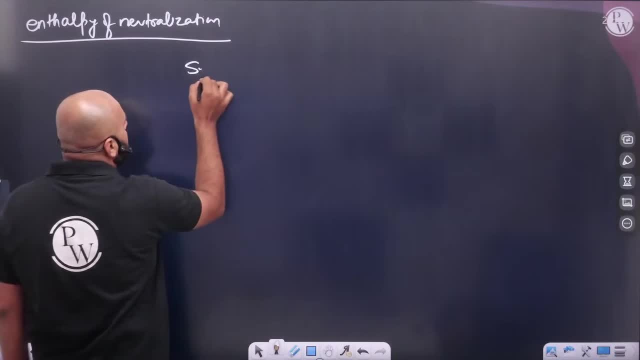 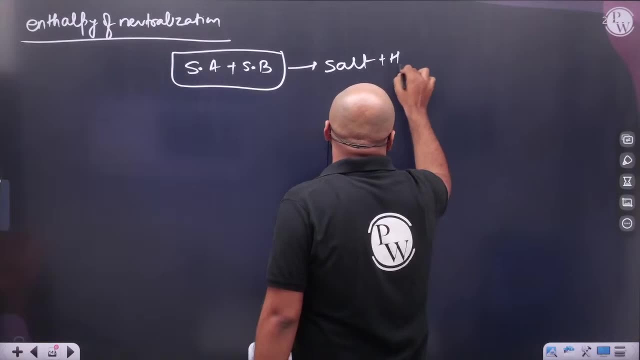 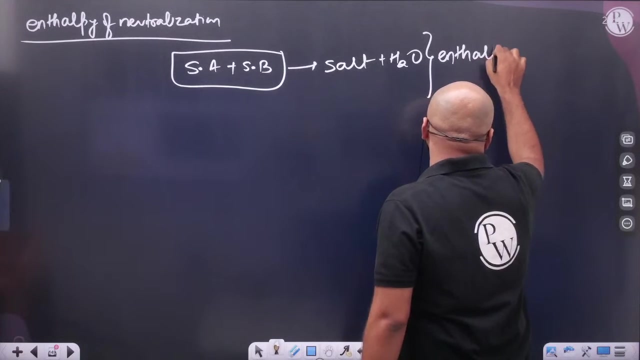 so enthalpy of neutralization. if there is strong acid and strong base, if they will react in each other, then what will they make? salt plus water, its obvious right, brother. salt plus water, this will give H plus, this will give OH minus. soon, the energy which will be loose in this. we call it enthalpy of neutralization. and its value is almost fixed. enthalpy of neutralization: enthalpy of neutralization value is fixed. how much is it so? if we see minus 13.7 kilo calorie per mol of water, or per equivalent of water, this happens, or 57 point, or minus 57.1 joules per mol. 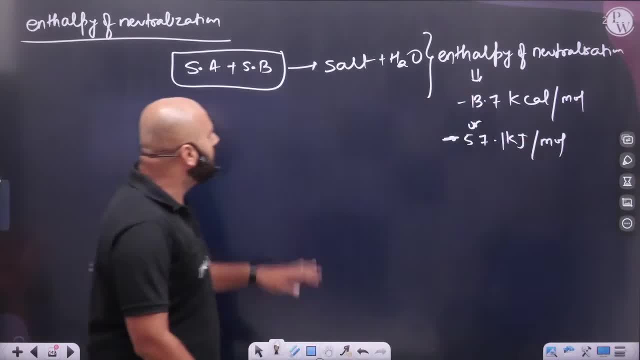 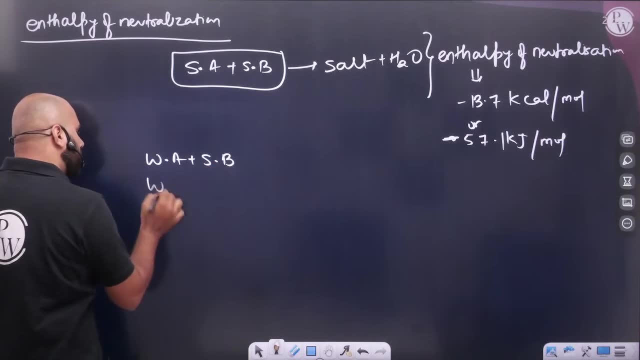 kilo joules per mol. this happens ok. so these values are fixed. but if any one person becomes weak, if any one person becomes weak, if any one person becomes weak, if I say acid becomes weak, or if base becomes weak, if any one person becomes weak or both become weak, then in that case enthalpy of neutralization. enthalpy of neutralization will decrease. why, brother? why enthalpy of neutralization will decrease? because as soon as any portion becomes weak, enthalpy of neutralization less than 13.7 kilo calorie. this value will decrease from 13.7 kilo calorie because some part of energy will go to ionize. 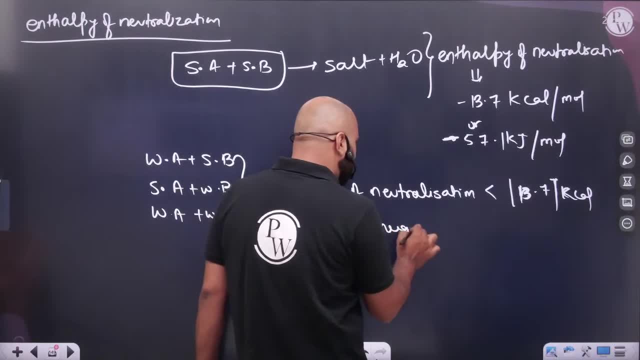 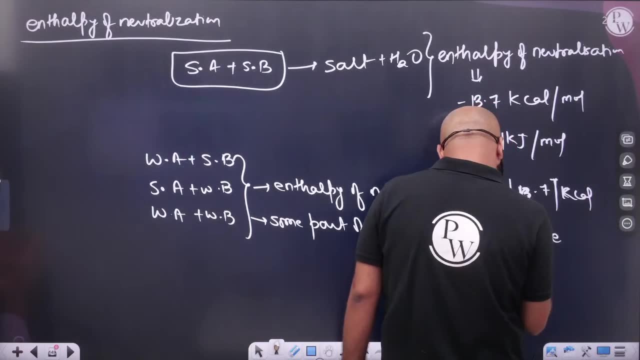 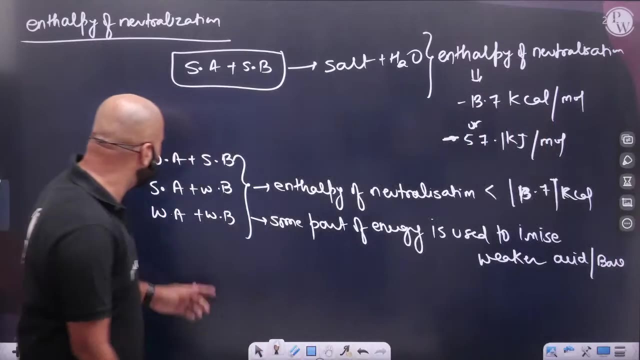 some part of energy will go to ionize is used to used to ionize. used to ionize will go to ionize. weaker portion of weaker acid or base. some part of energy will go to weak acid or weak base because some part of energy is weak. 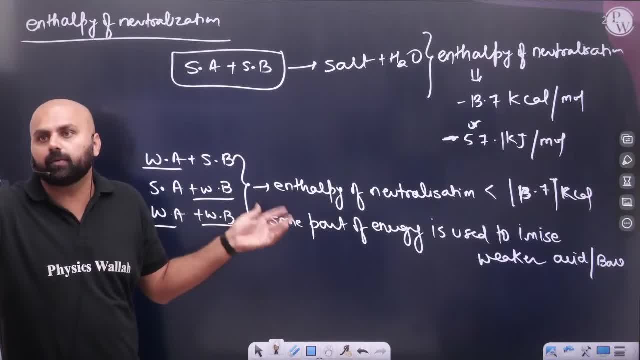 some part of energy is weak. because some part of energy is weak, because some part of energy is weak, so this will go to ionize. obviously weak acid or weak base will go to us. ok. so keep in mind that, brother. see this. what is neutralization enthalpy? strong acid is in strong base. 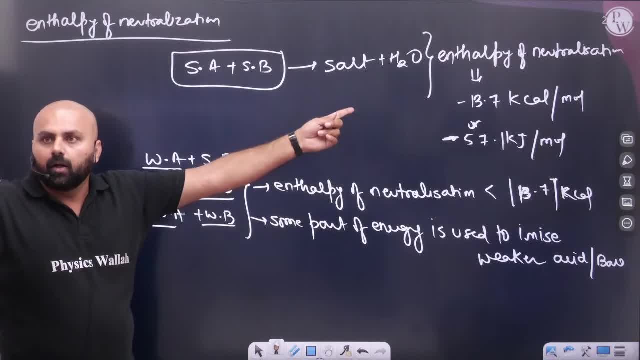 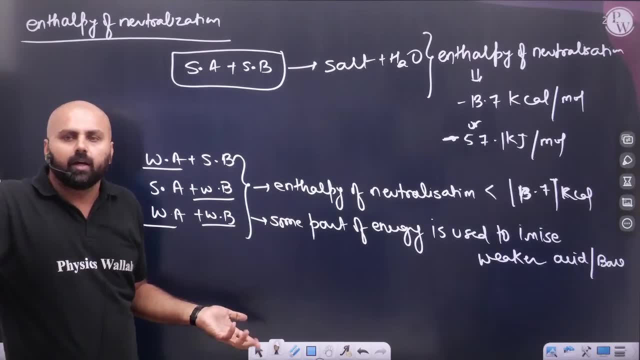 what will be enthalpy of neutralization. ok, yes, so this is strong in us. if you remember these values, then it is a good thing. otherwise, it will be given in your exam. ok, see this to yourself. what is this to yourself? what is this to yourself? 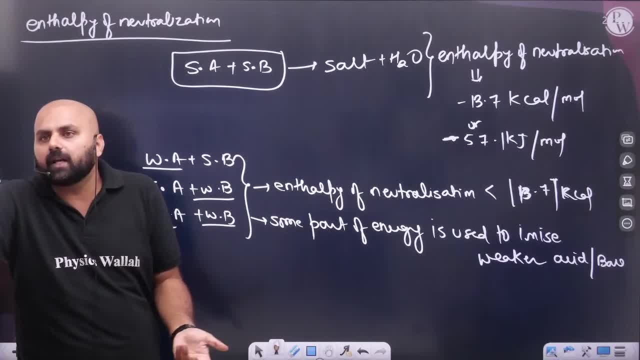 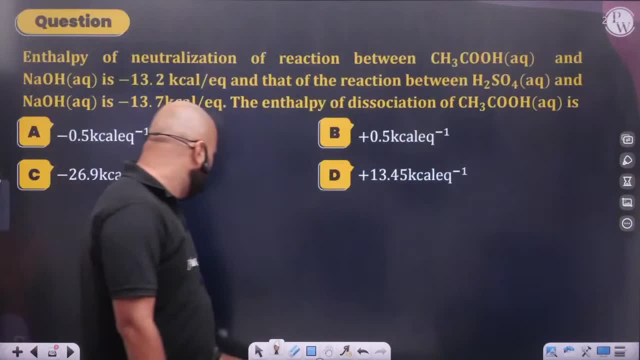 if any portion becomes weak, then what will happen to the? energy will decrease and how much part will go out. take a look tove in what arms'll show off, what will be used for how, to see how many parts will stretch out and see, see as get out, then see. 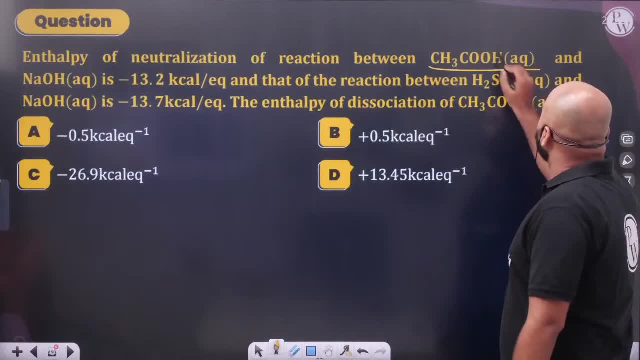 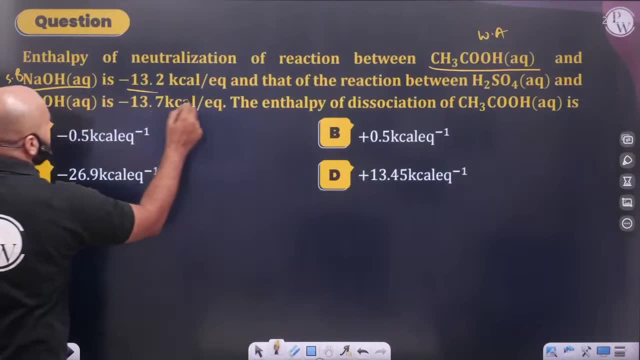 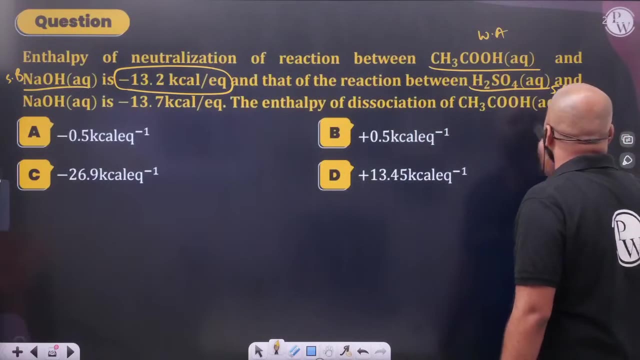 for instance, suppose if here question given sir, this is being situation, that, sir, this is a weak acid and this is strong base, weak acid, strong base. see this, much of energy is also got released. but he is saying that if it is this blood, that is description by front. 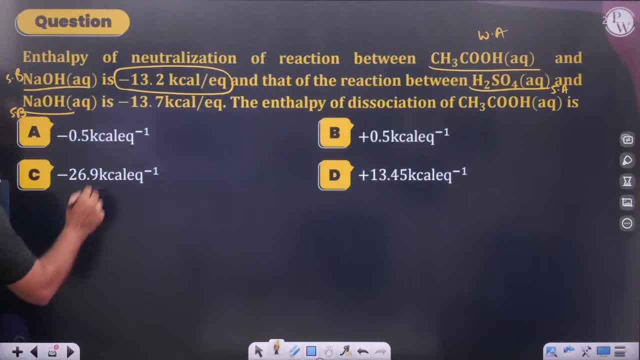 if front is strong acid and strong base. strong acid would have been strong base, strong acid would have been strong base. So how much energy would have been released? How much would have been released? Now, your energy is decreasing. How much is decreasing? 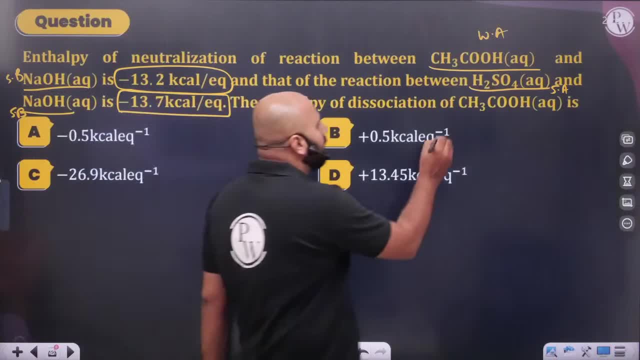 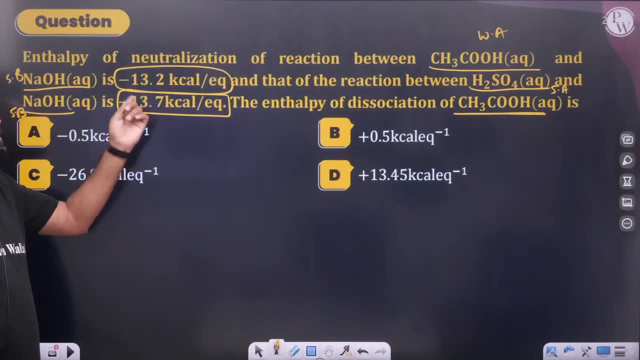 Sir. why is it decreasing? Because you are giving energy. to whom To dissociate this? So this is the question: See, this much energy, this much energy should have been released, But it is not happening. This much energy is being released. 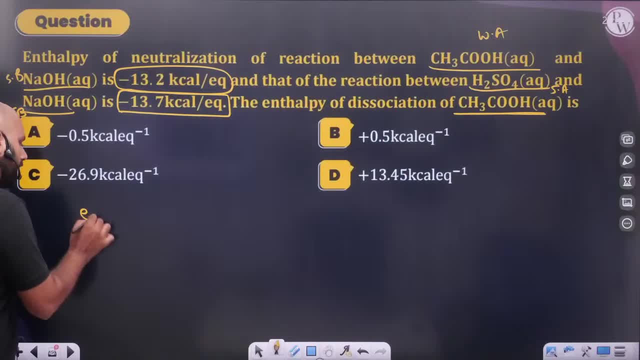 So it is not happening. Why is it not happening? So, sir, what does this mean? Sir, some part of energy, To whom is it going to be given? Enthalpy of dissociation? To whom to dissociate? 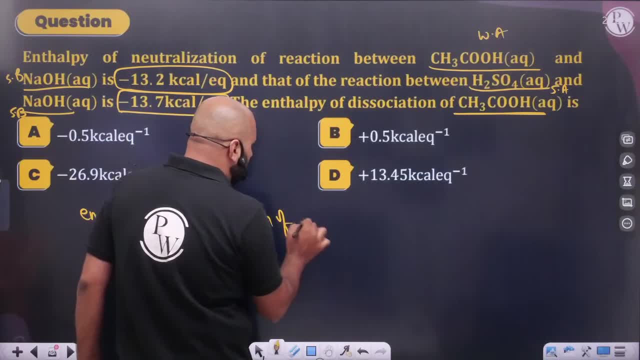 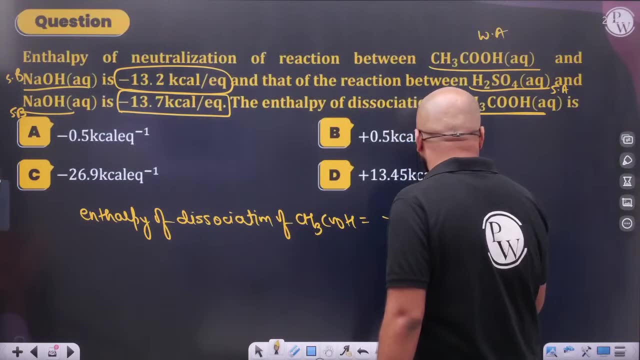 Sir, to dissociate the weaker part Which would be coming To dissociate CS3, COH. How much So, sir, what you had thought. This much is coming to you, And how much did you think 13.7.. 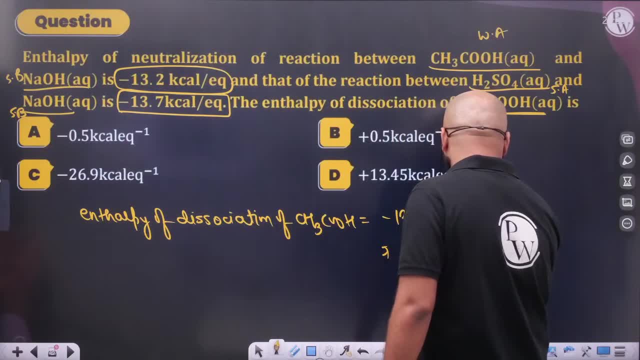 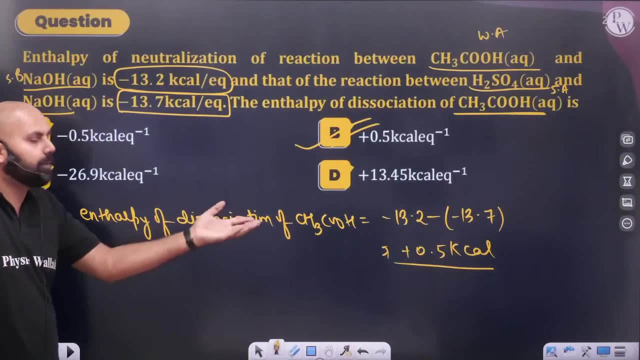 Sir, how much will it be Plus 0.5 kilo calorie? Plus 0.5 kilo calorie, What will come? Enthalpy of dissociation. Because you are dissociating, You will have to give energy, So positive will come. 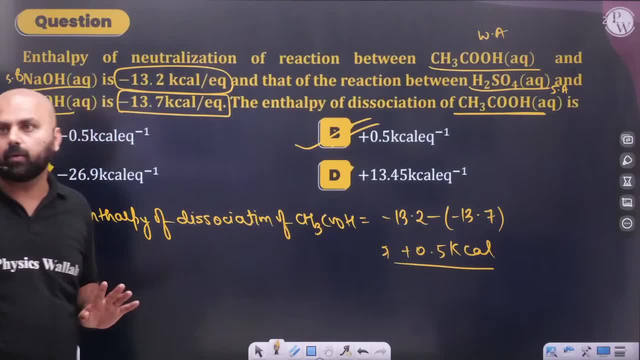 Minus will not come, Positive will come. Minus will not come, Positive will come. Keep this in mind. The question of enthalpy of dissociation, Or you can say enthalpy of ionization: This question will be coming. 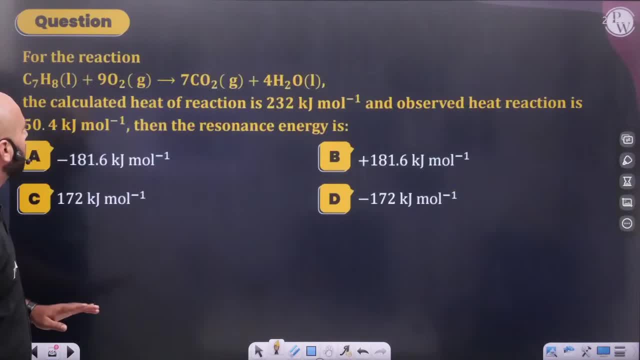 If we talk about neutralization, If we talk about neutralization. Now see, I have a formula of resonance energy, The formula of resonance energy. I will put the formula directly: Resonance energy is nothing to you, Whenever you think. 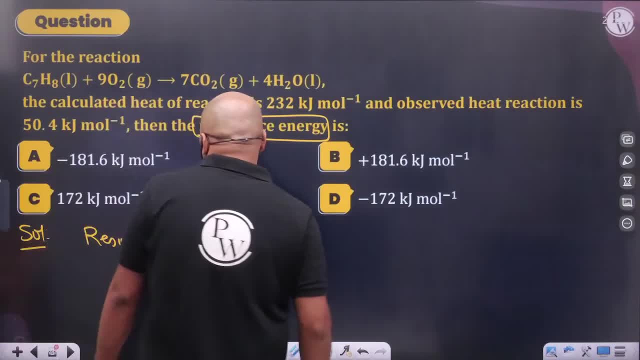 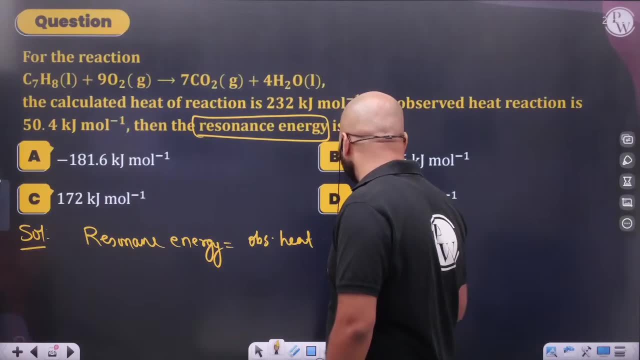 What will be the resonance energy, Sir? resonance energy comes due to stability, And if stability comes, then you will lose energy. So if stability comes, then what will be the energy? It will be loose. So remember Observed heat. 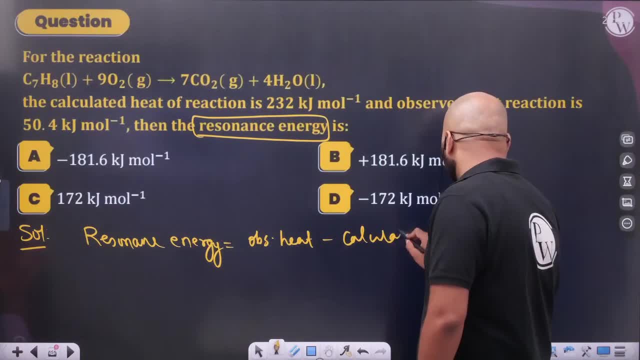 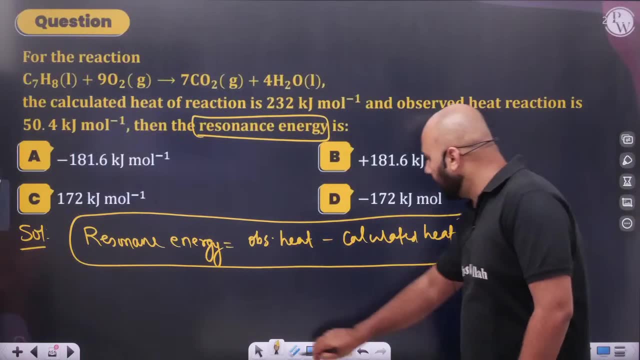 Or observed heat minus calculated heat. Observed heat minus calculated heat, The amount you were thinking, The amount you were calculating. It will be less than that And that is what resonance energy. Like benzene, It is benzene. Keep this in mind. 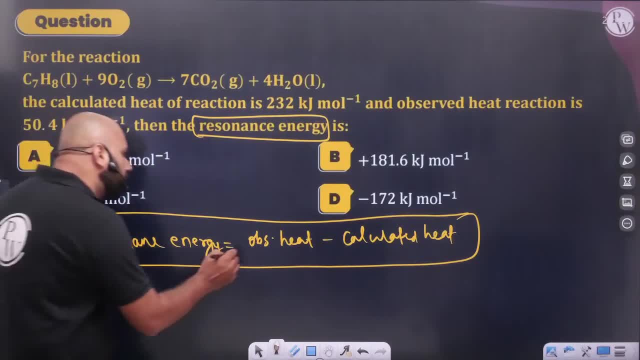 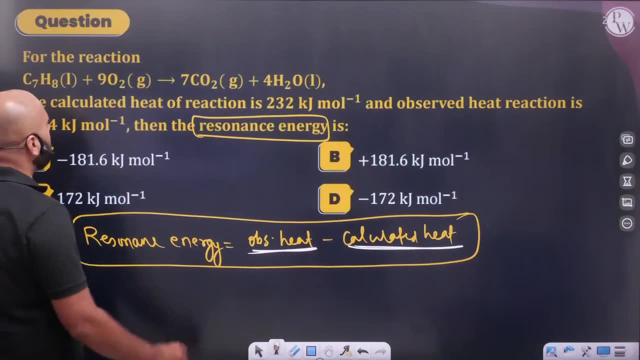 I am talking about benzene. What is resonance energy, Sir? the amount of absorbed heat That is your And difference in calculated heat Like, see here. What is he saying in this reaction, Sir? what did I do? Observed heat. 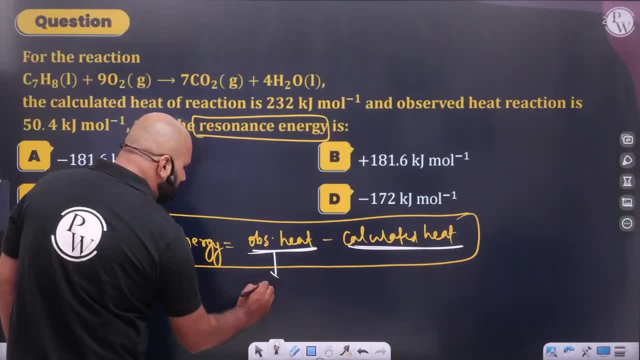 How much did I observe, Sir? how much did I get? 50.4.. But when I calculated with bond. So how much did I get? I should have got this much, Brother. where did the rest of the energy go? 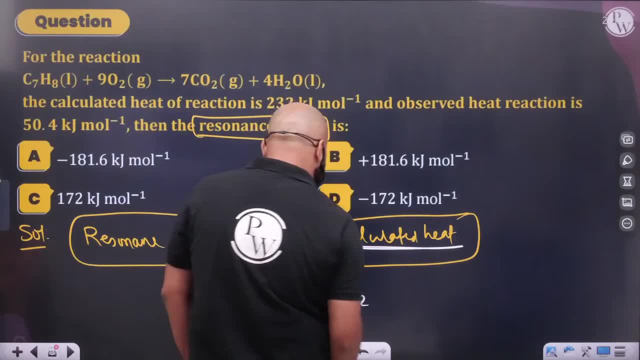 So the rest of the energy must have gone to mine. Do this and see How much is going on. How much will it be If I look properly? So this, This will be 2.. 1. That means 1 is done. 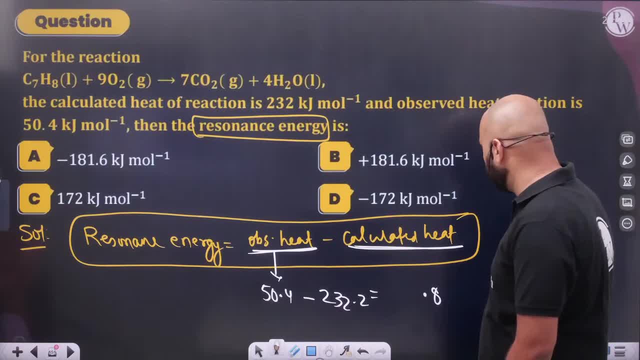 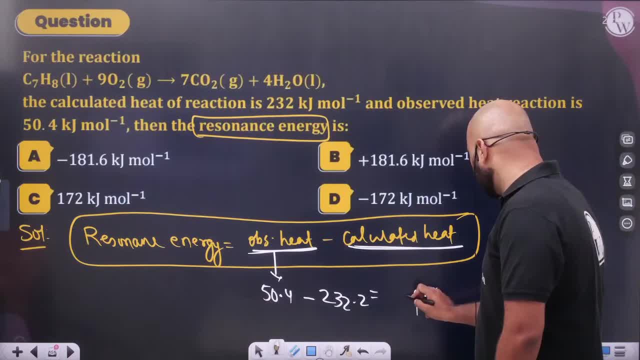 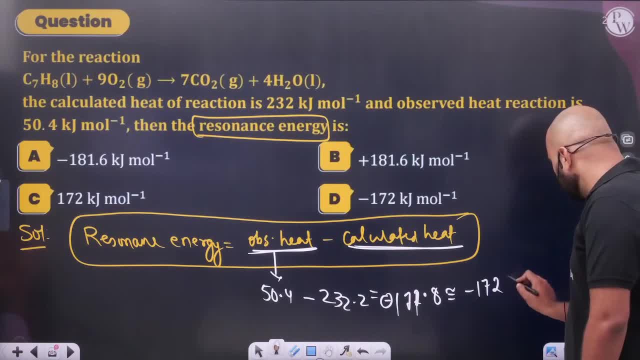 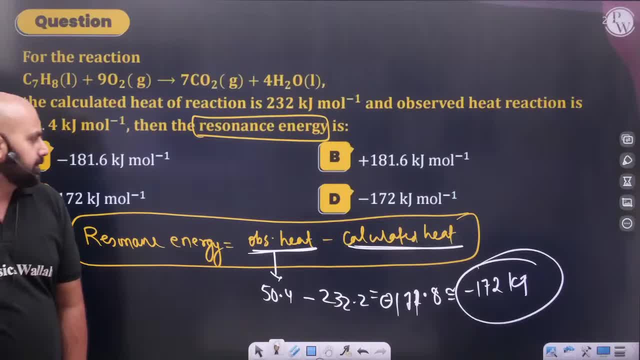 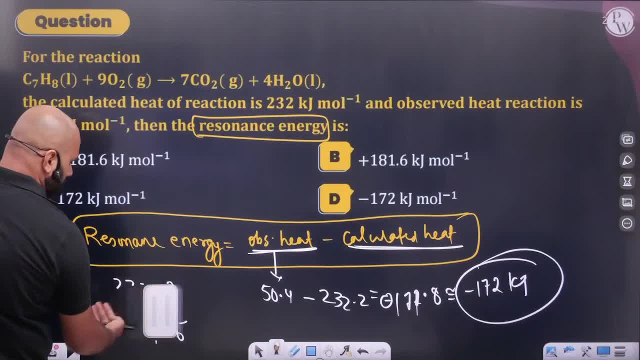 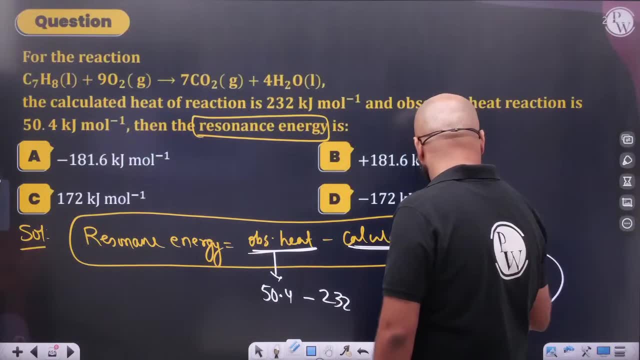 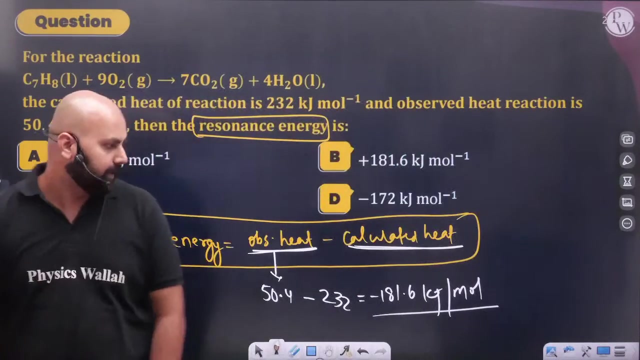 1. 1. 1. 1. 1. 1. 2.2. why am I taking it? how much is coming? what has happened? let's take a break now. it has become more minus 181.6 kilojoules per mole. okay, okay, I did the calculation yesterday. okay, brother, 232, okay. 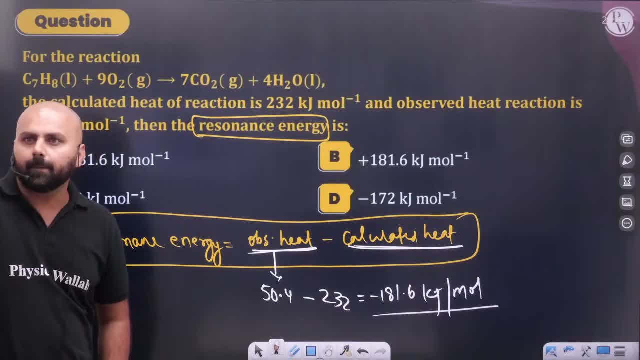 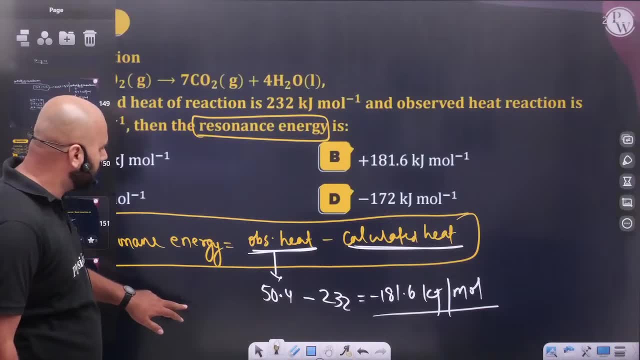 good, good, okay, okay, okay. so let's go, brother, now look at yourself. whatever we did, whatever concept we had to do, that whole concept, I will tell you again. there was some more. there was some more, just 2,, 3,, 8,, 15,. 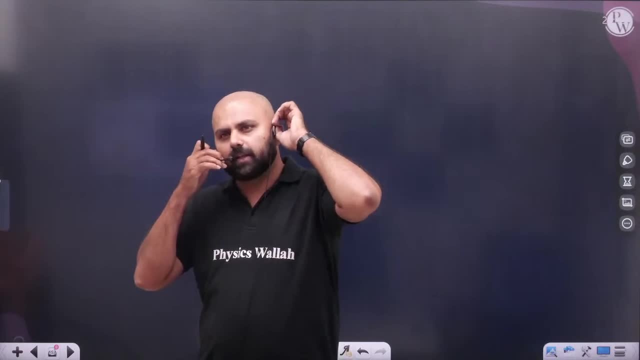 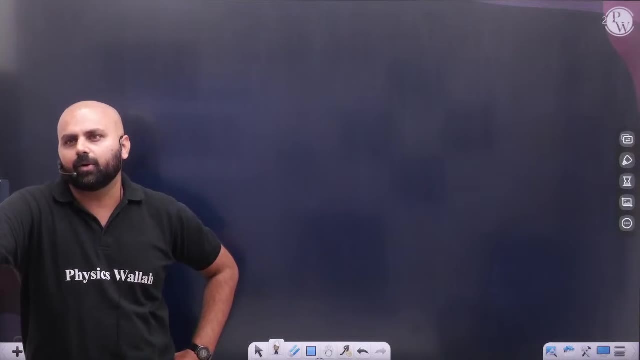 let's take a break, okay. 15,, 8,, 15,. we will take a break, brother. it will be more by 9 o'clock. okay, I took 5.30,. yes, more break, brother. now finish the chapter today. it has become very bad, but think about it, think about it. 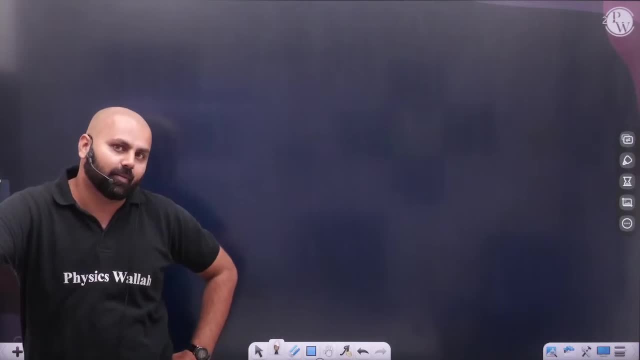 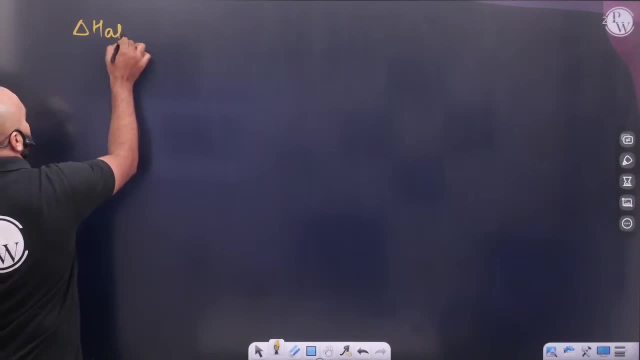 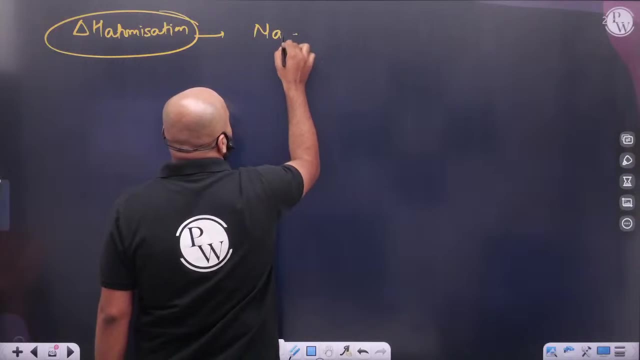 I am touching the maximum. see, some synthalpies were like this, like Atomization Enthalpy. the atomization enthalpy that happens, it becomes very important. if there is any metal, then what is called the sublimation enthalpy of its metal. 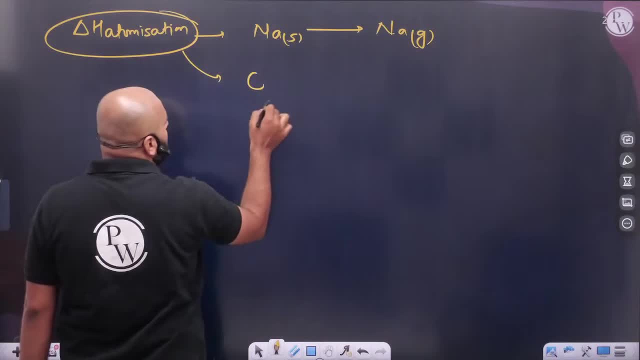 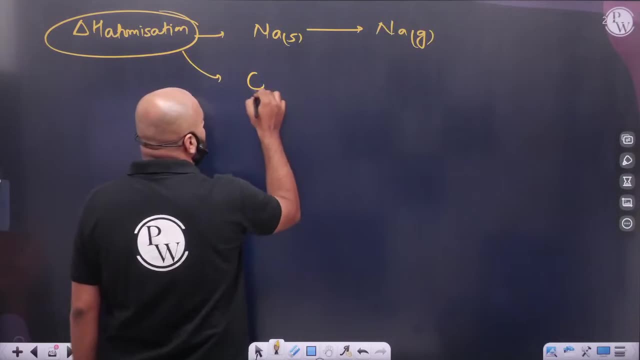 Atomization enthalpy. if there is any non-metal, then with solid gas- if I talk to myself, there is any non-metal. if we talk like that, if we talk about O2, then in O2, those who write convert it into atoms. they also call it atomization enthalpy. pay attention. 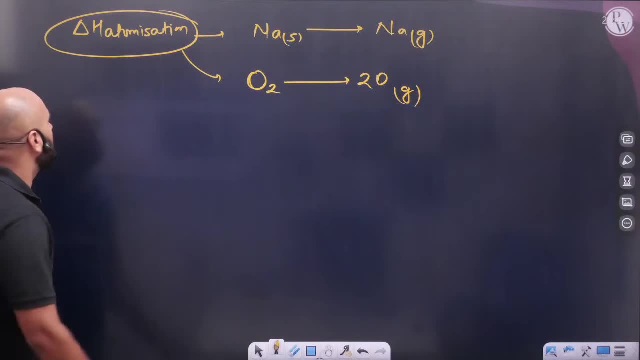 Atma Isha Enthalpy is different. Atma Isha Enthalpy is different. Similarly, we will go ahead Atma Isha Enthalpy, Apart from Atma Isha Enthalpy, Like Fusion Enthalpy. Like Fusion Enthalpy, Sir Vaporization Enthalpy. 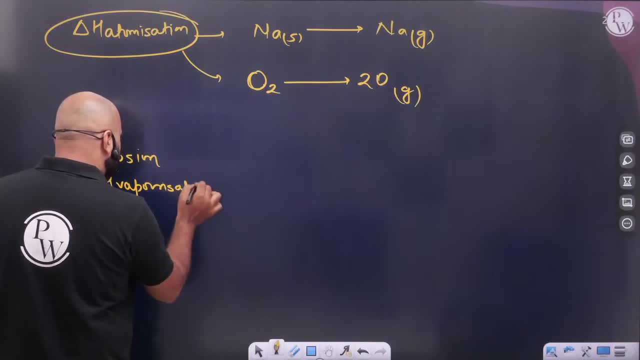 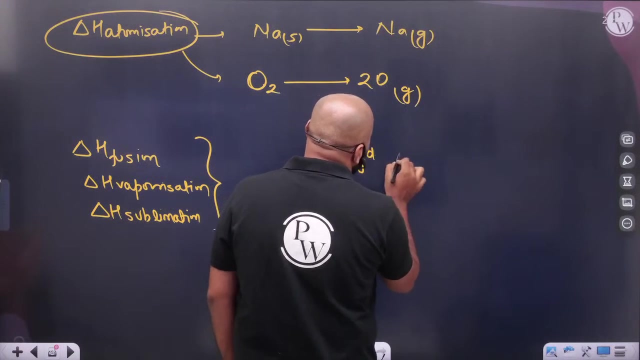 Vaporization Enthalpy. I am just telling the name: Vaporization Enthalpy, Sublimation Enthalpy. These are also different Enthalpies Which are being used. Second, Someone told me Hydrogenation. You will read about it in NCRT. Hydrogenation Enthalpy is found in Organic. 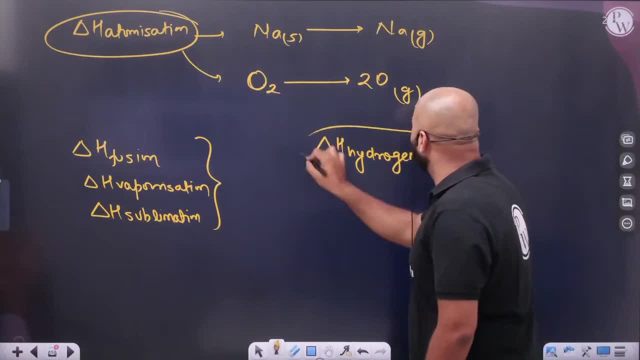 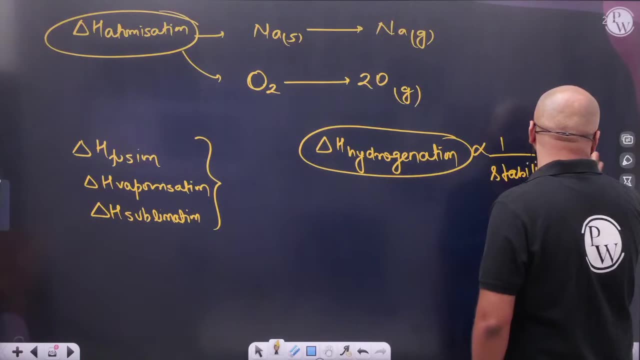 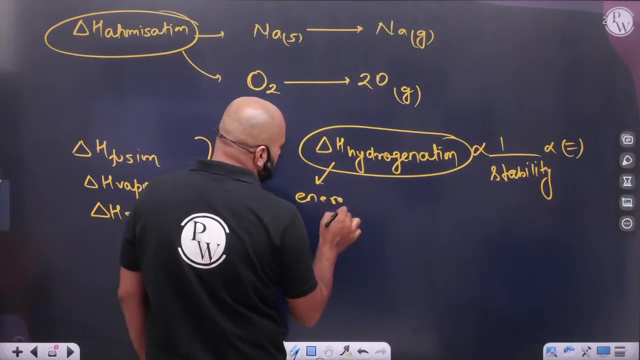 The energy that is being produced when hydrogen is added. Hydrogenation Enthalpy is found in Organic, Inversely proportional to stability. Inversely proportional to stability, Directly proportional to double bond. Directly proportional to double bond. This also releases energy. This also releases energy. 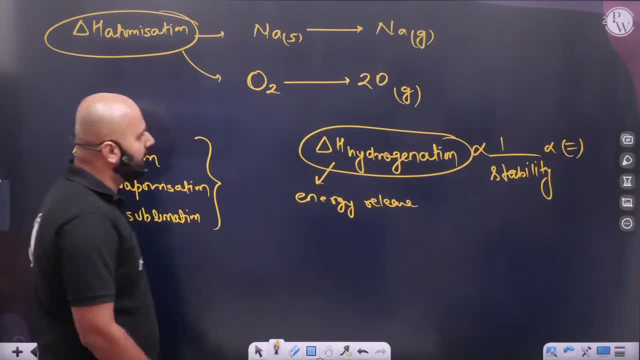 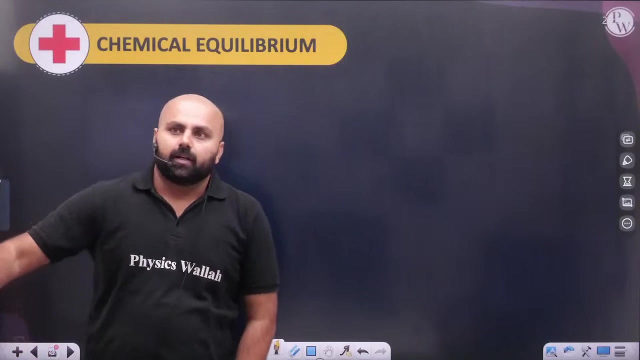 Pi bond breaks Energy releases. Hydrogenation Enthalpy. These are the small Enthalpies Which you will use. Now I have the remaining chapter. I have the chapter of chemical and ionic equilibrium Redox. Now You are sitting, Let's do one thing, Not too long. 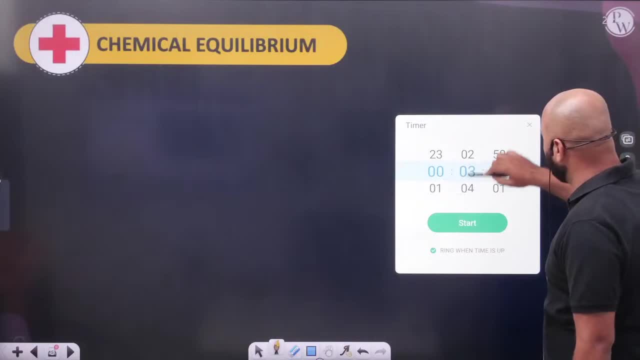 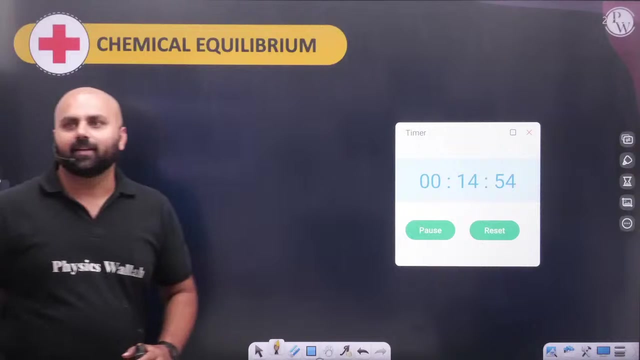 10-15 minutes break. Let's meet at 8.30, Then we will start, Because now the big chapter will start. Now we will finish redox, redox. Now we will focus on 12. Take a 15 minute break. Let me refresh. Ok, Let's go. 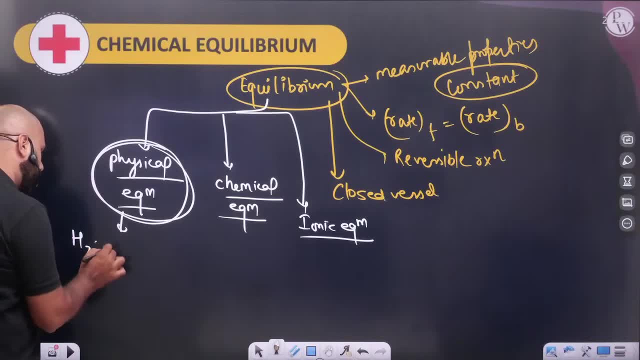 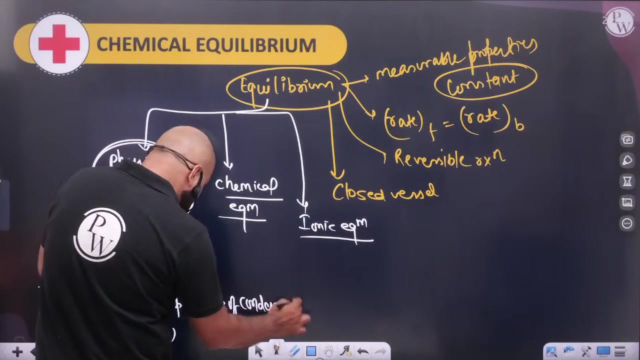 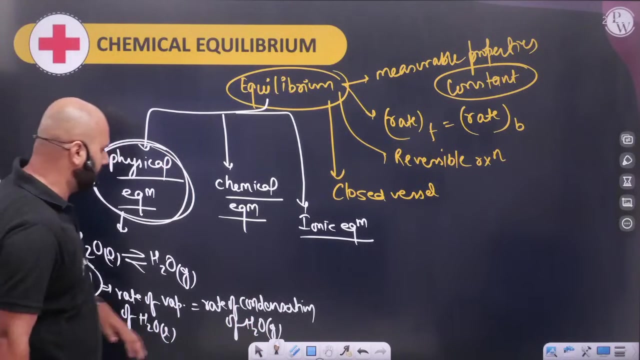 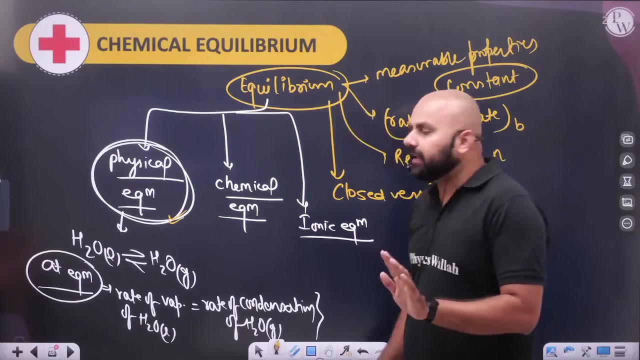 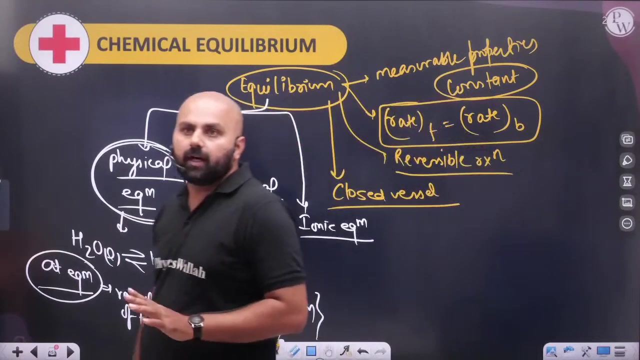 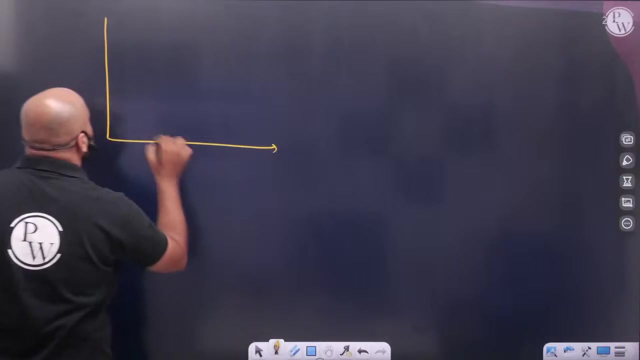 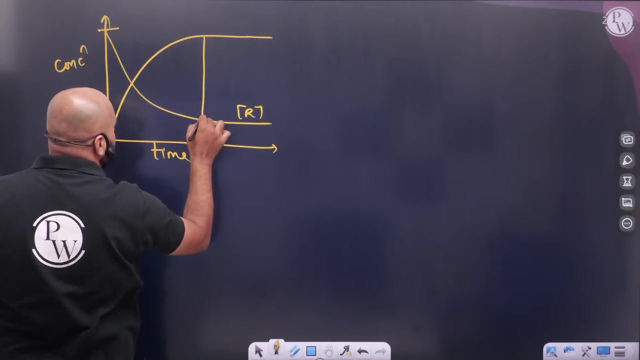 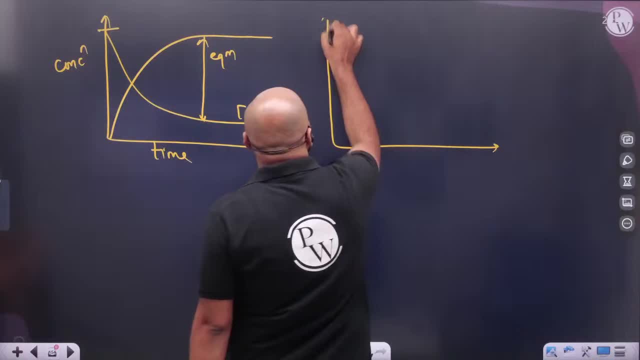 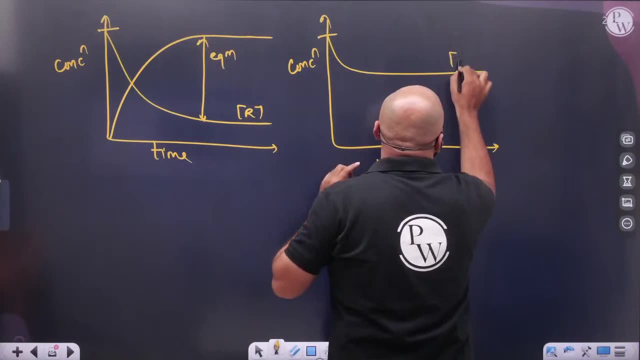 Here you can see that there can be three graphs of concentration versus time. There can be three graphs of concentration versus time, Sir. the concentration of the reactant is decreasing. the product of the reactant is increasing. After this, what will happen to us? 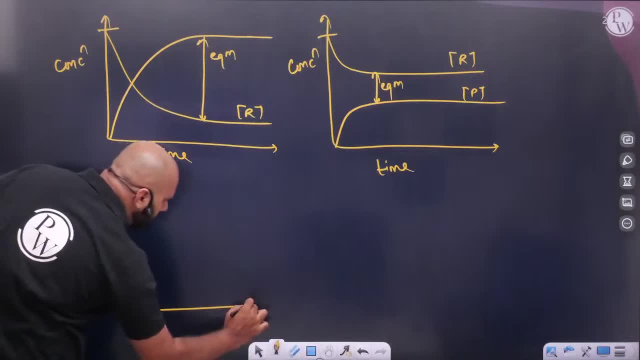 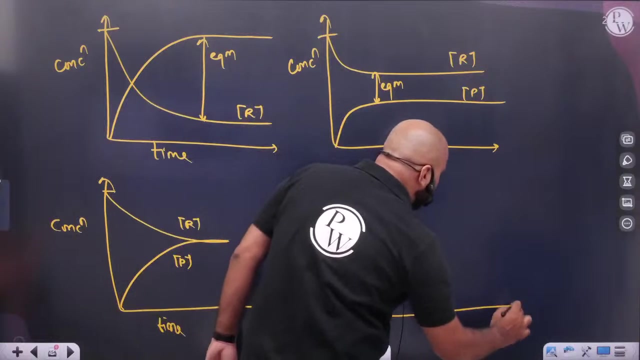 The equilibrium will come, Sir. the graph of concentration versus time is three possible. But remember a simple thing on the equilibrium, Sir, the three graphs of concentration versus time will be possible. This is the product of the reactant. But if you make a graph of rate versus time, then there will be only one graph of rate versus time. 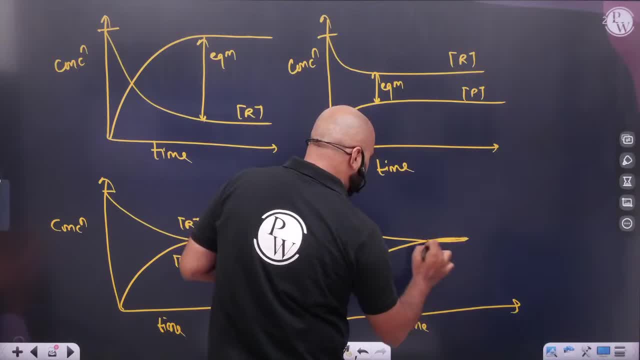 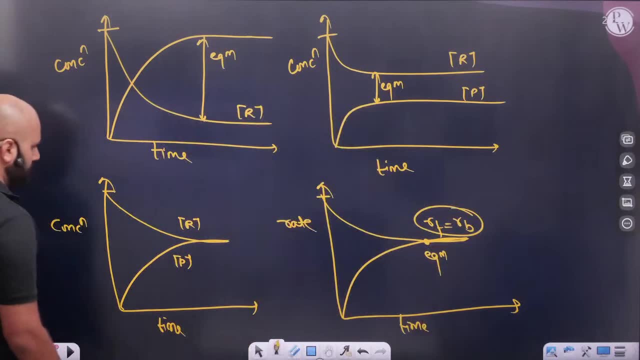 And it will be like this, Sir. it will be like this Where the equilibrium will come: Where the rate of forward is equal to rate of backward. what is this called? Let's call it equilibrium. This will be my equilibrium from here. 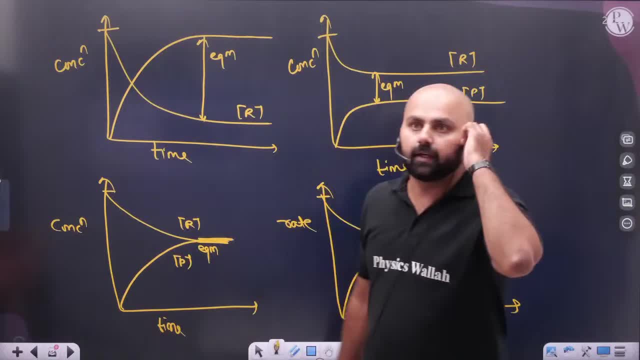 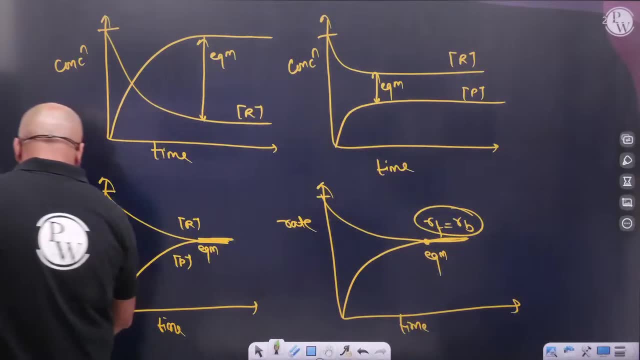 So if you see the graph of equilibrium, then how do graphs form? The second thing: see what will happen to yourself Here, as we come into the equilibrium. the equilibrium comes constant, And if you see the equilibrium in constant, then what does the law of chemical equilibrium say? 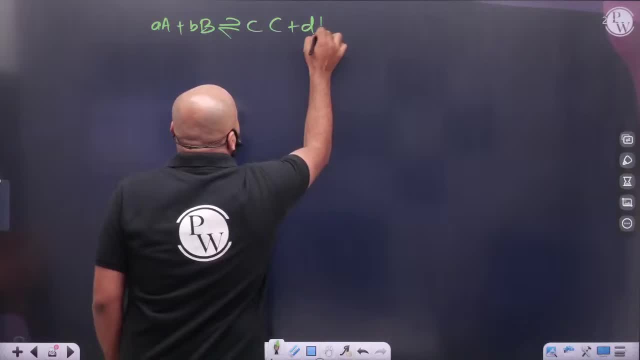 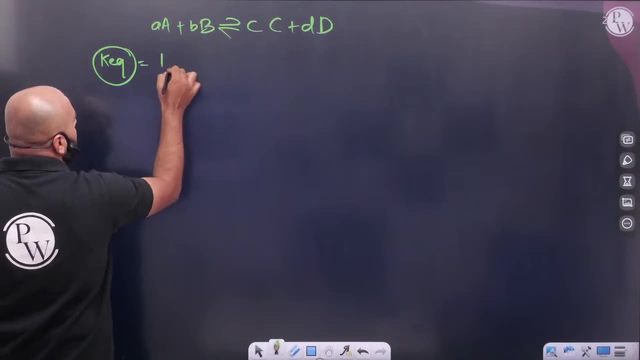 Sir, if you see this reaction carefully, if you talk about this reaction, equilibrium, constant, if I want, I can write it in different ways. if I write in terms of concentration, then what will I write? Kc, I will write it in terms of concentration. 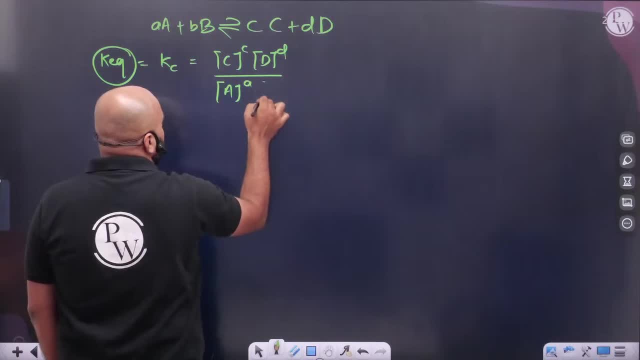 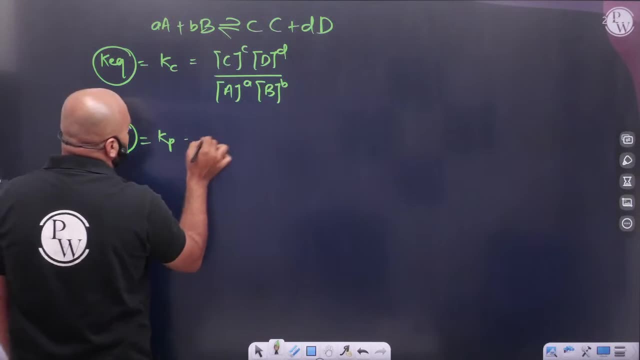 I will write it in terms of concentration, sir. I will put the rest of the stoichiometric coefficient above. if I write equilibrium constant in terms of pressure, then in terms of pressure I will write that: pressure of C. pressure of what will I write? C power. 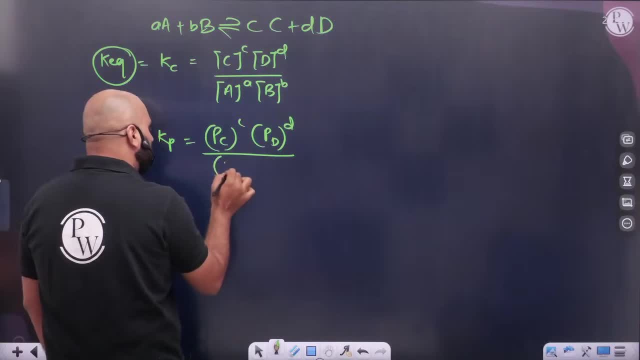 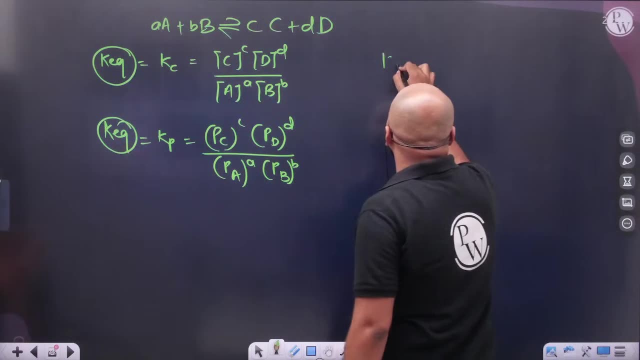 C, pressure of D- power D, pressure of A- power A and pressure of B- power B. I will do this, so these small things will come Kp, Kc. someone said, sir, equilibrium constant can be written in terms of mole fraction. you can write it, but it has become very obsolete in today's. 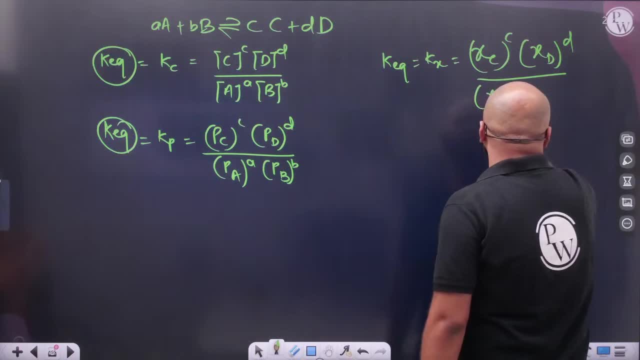 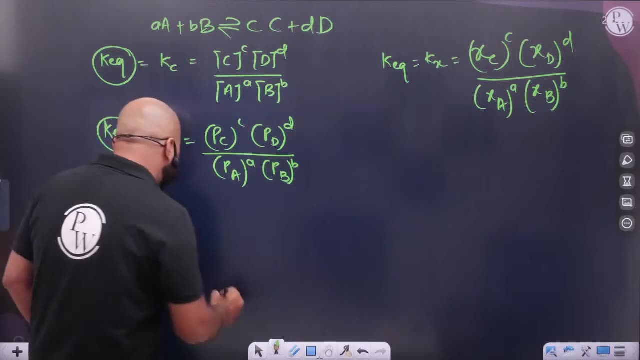 time, it is not required that we are writing in terms of mole fraction. if you talk in terms of mole fraction, then it is not required. so equilibrium constant: you can write in all three. you just have to remember the relation that sir Kc is. Kp is nothing, Kp is nothing. 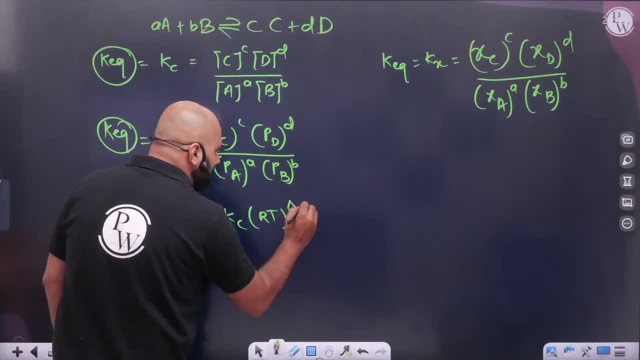 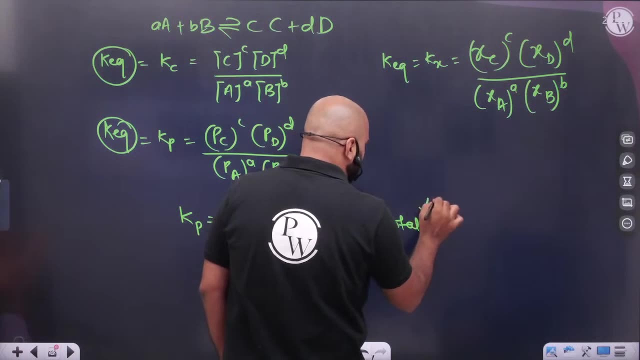 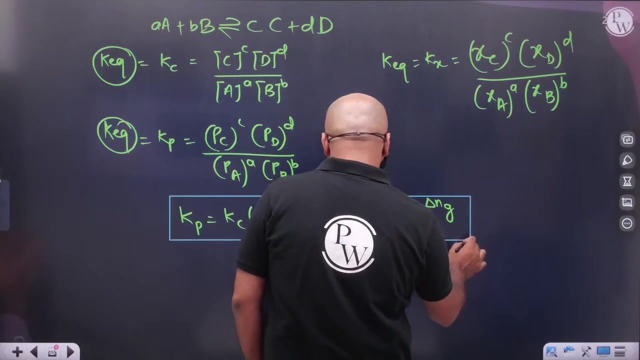 Kc into RT power, delta ng. and, sir, if I talk, then kp is nothing, K square, the power of P total, P total's power is delta ng. only these small things have to be taken care. if you will see, then you will come to this graph, this one, sir, remember this relation. 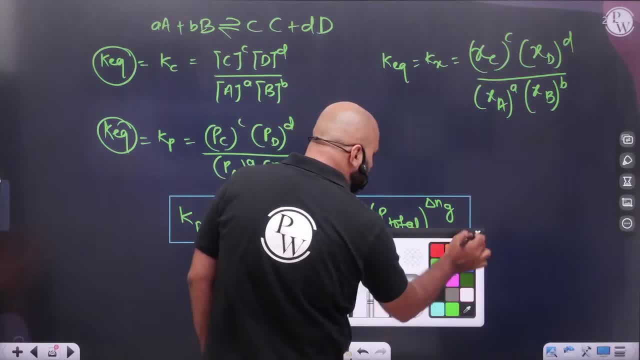 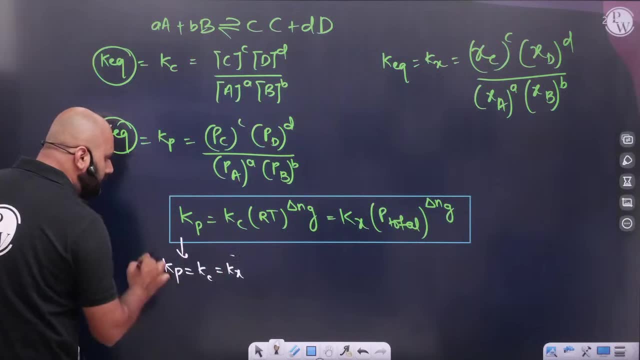 between Kp and Kc. here questions will be asked in small, applying here that, sir, King P or Kc, King P is equal, King P is equal to Kc is equal to K square. when all three will be equal, When delta ng, in which direction the less real function is written as this: Kp, Alright. 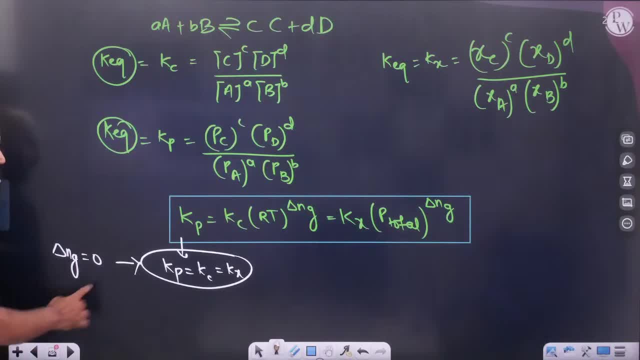 that's a little, Kakai, just turn back. please leave and write it at the end. this is not true. delta ng becomes 0, delta ng becomes 0, then kp, kc, kki- all will be equal. after that, kp is equal to kc can be equal once more. 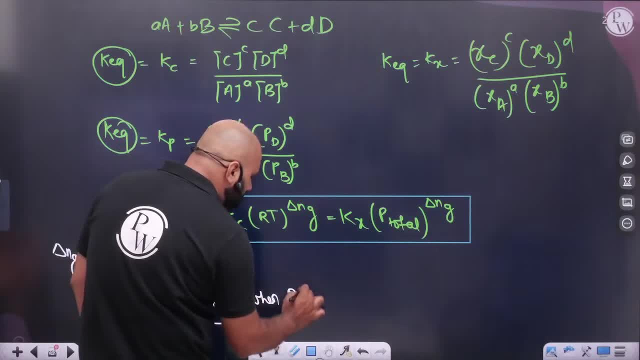 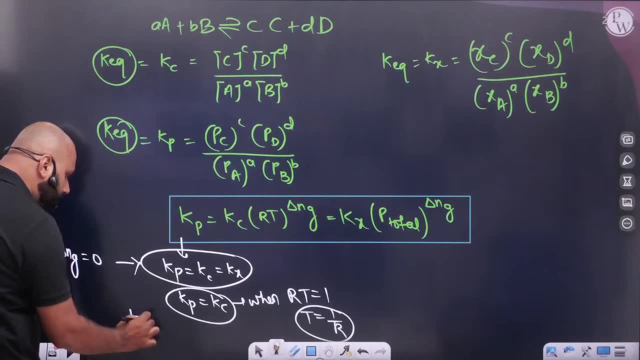 when rt is when rt is equal to 1 and temperature becomes 1 by r, then also kp and kc can be equal. kp is equal to kki can be equal once more. when p total becomes 1, p total becomes 1 atm. remember this condition. 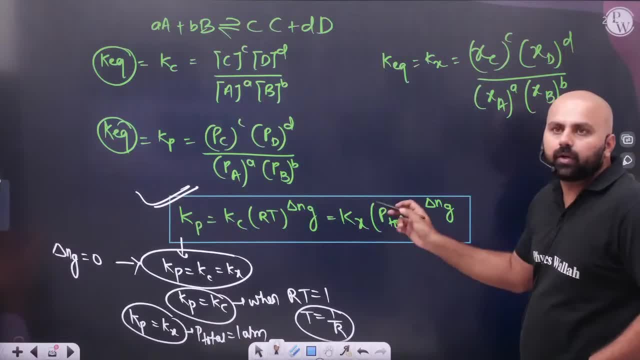 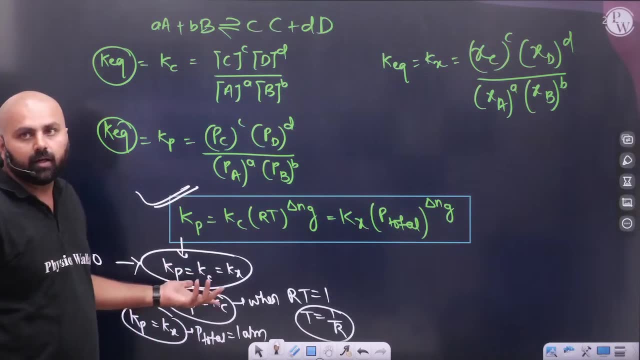 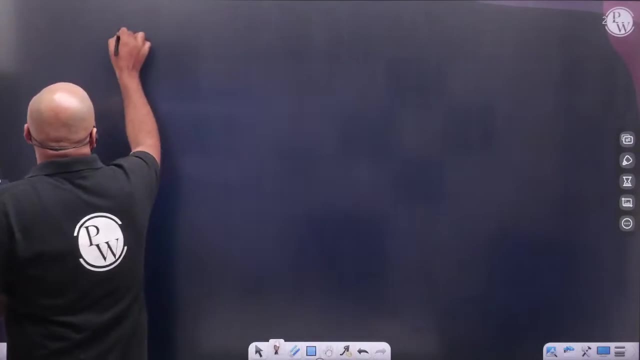 remember this relation. this story will end. remember this condition and relation. remember this condition and relation. remember this condition and relation. the answer will come. we don't have to do derivation now. who said kp, kc, kki? someone gave me a reaction. see this carefully. if given a reaction, 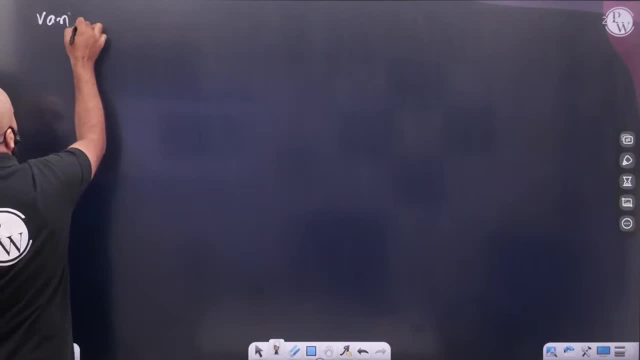 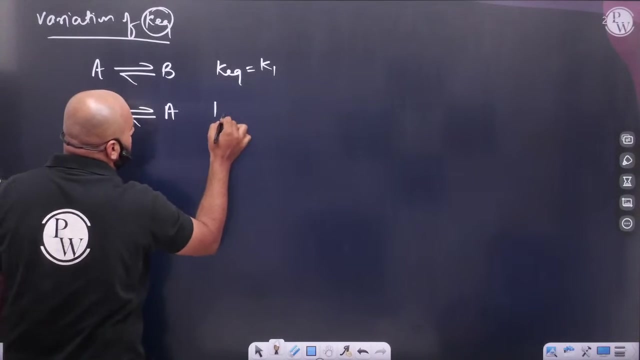 if given a reaction. if given a reaction, you have to see how variation of equilibrium constant varies if you reverse the reaction. if the reaction- let's assume its equilibrium constant- is k1, if you reverse the reaction, then remember, as soon as you reverse the reaction it will become 1 by k1. 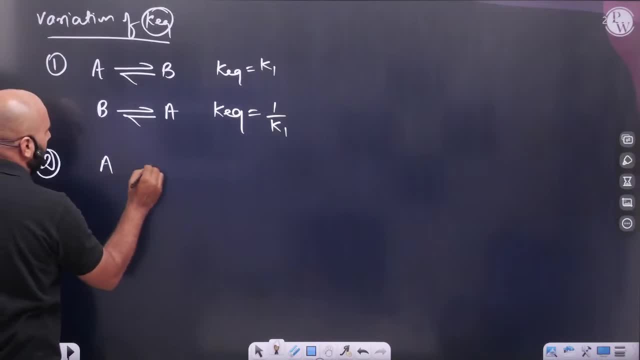 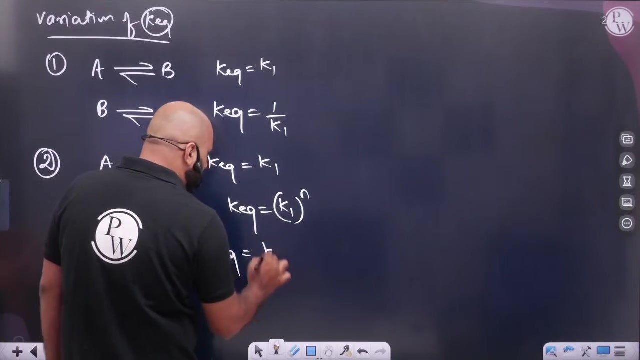 first thing, see this: if you multiply the reaction, if you multiply the reaction, then remember: if you multiply with n, if you multiply with n, you get k1. if you multiply with n, you get n. if you divide, then you will get 1 by n, 1 by n. 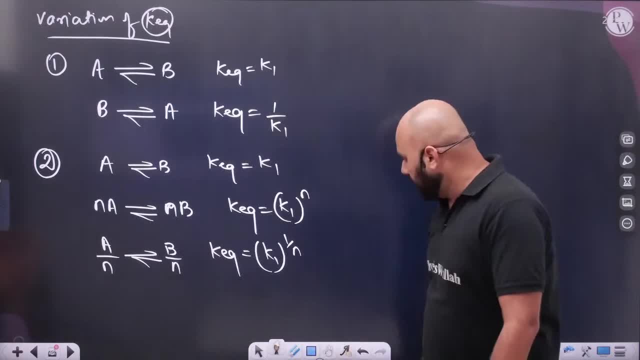 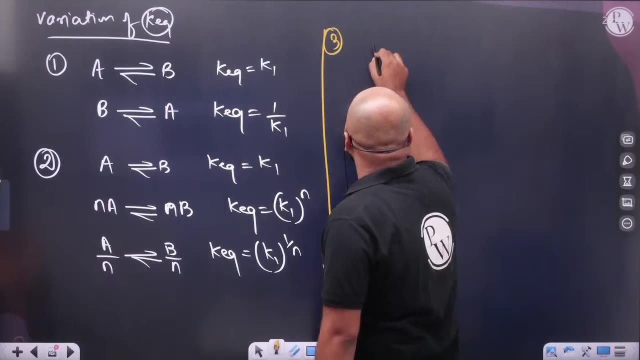 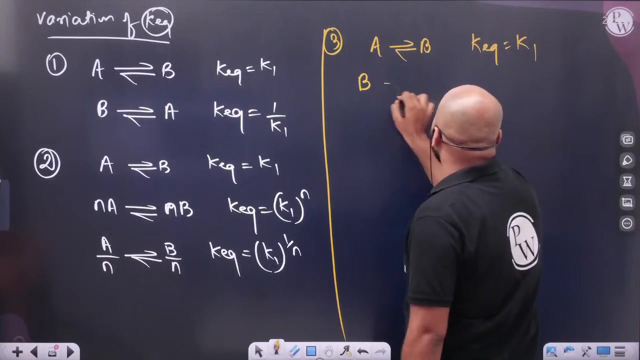 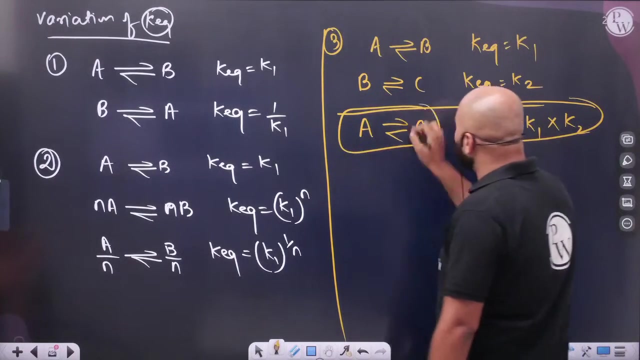 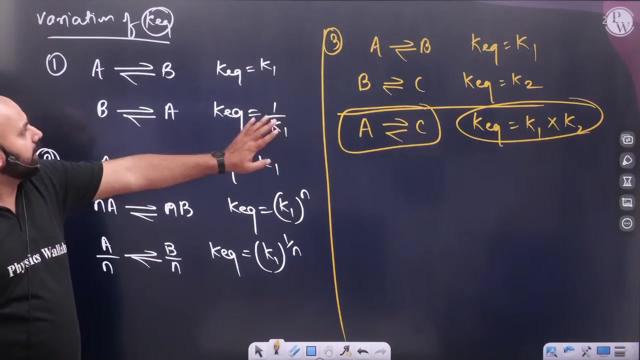 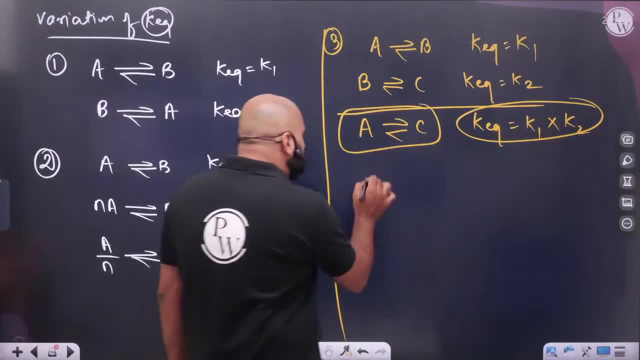 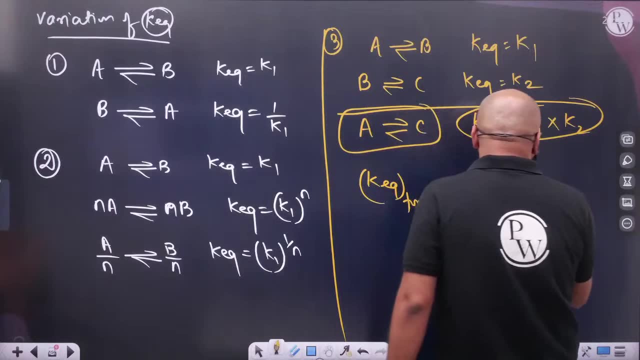 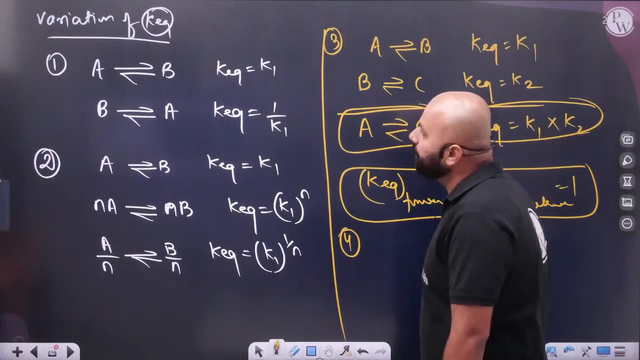 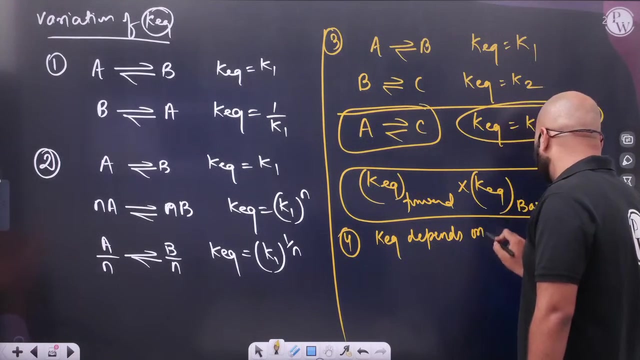 simple, simple things. equilibrium constant forward means you will be asked: all this equilibrium constant forward, into backward? what happens? nothing. equilibrium constant backward, how much will it be? one will be okay. so these small things. equilibrium constant's fourth variation, with temperature. remember. equilibrium constant will only depend on whom, depends only on temperature. 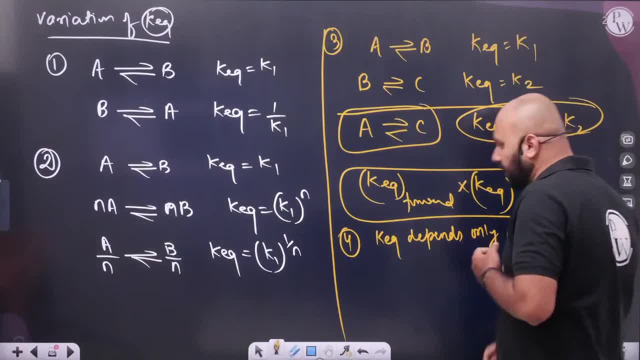 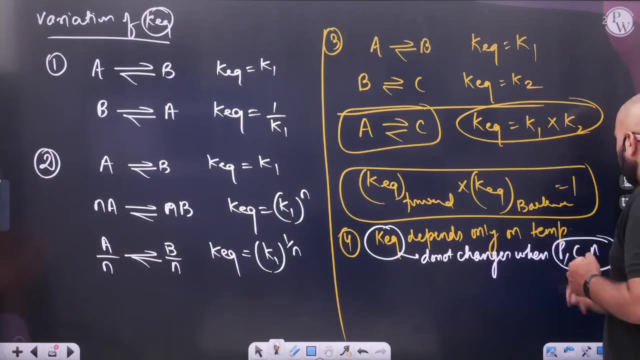 if you change the temperature, then only it will change. otherwise equilibrium constant will never change the temperature. other than temperature, sir, do not changes. equilibrium constant's value does not change when you change pressure, concentration, number of moles. all this, there will be no change. remember one formula of equilibrium constant: 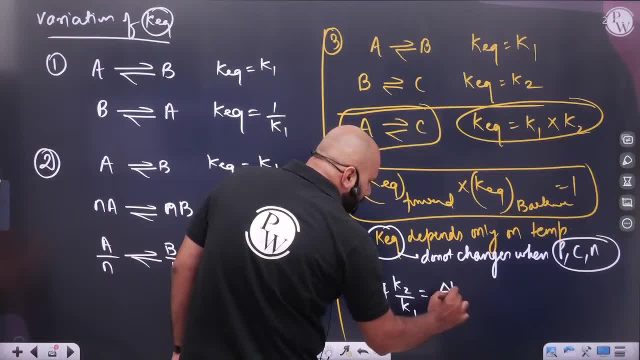 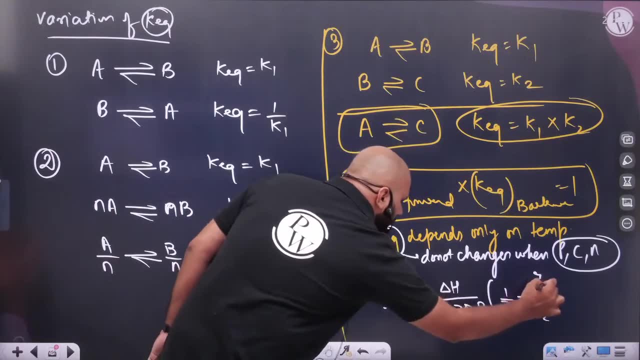 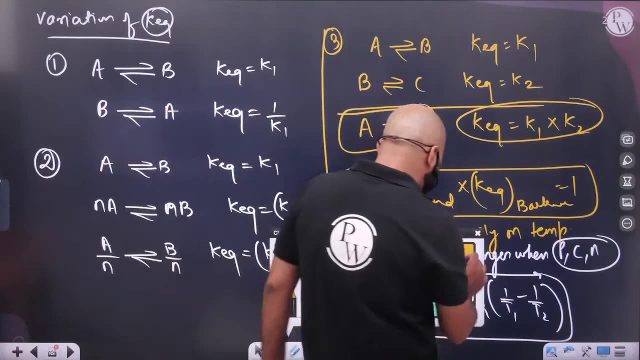 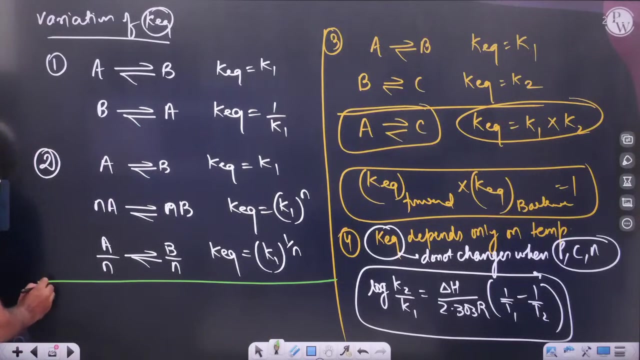 K2 by K1 is nothing. delta H upon 2.303, R1 upon T1 minus 1 upon T2, 1 upon T1 upon 1 by T2, remember, equilibrium constant will only depend on temperature. it will fluctuate only by temperature. it will not fluctuate by anyone else. if I write a line here, remember if there is an exothermic reaction, if there is an exothermic reaction, then the equilibrium constant will be inversely proportional to temperature. 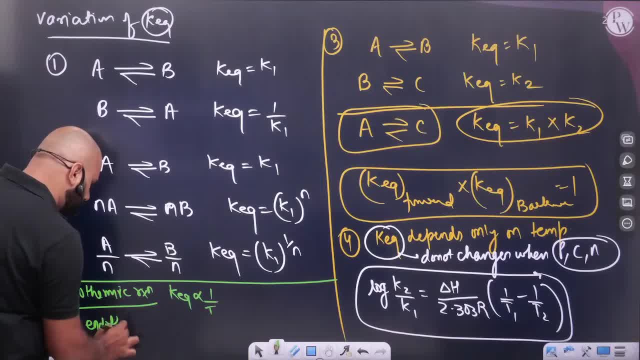 And for endothermic reaction. if there is endothermic reaction, then in endothermic reaction the equilibrium constant is directly proportional to temperature Means. if you increase the temperature in endothermic reaction, the equilibrium constant will increase. in exothermic it will be opposite. 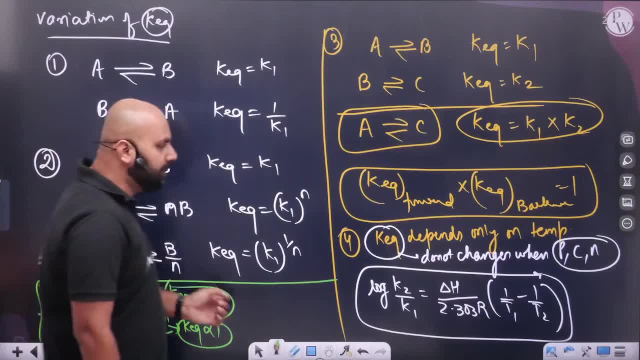 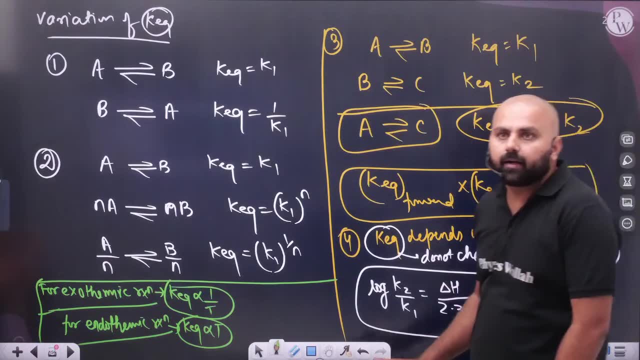 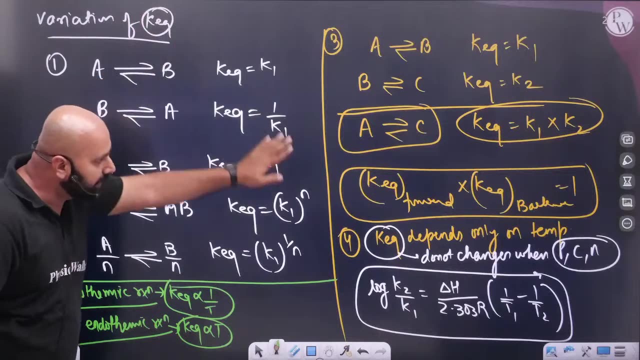 So keep this in mind. in exothermic, the equilibrium constant decreases. the equilibrium constant decreases as compared to this. Just keep this in mind, nothing else. I am simply saying that you have to see these things in the reaction, see the variation of the equilibrium constant, keep doing according to it. 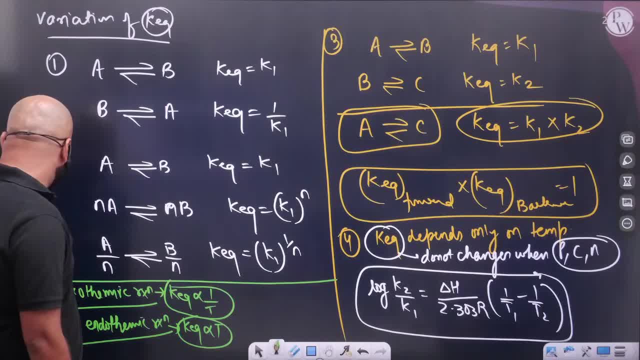 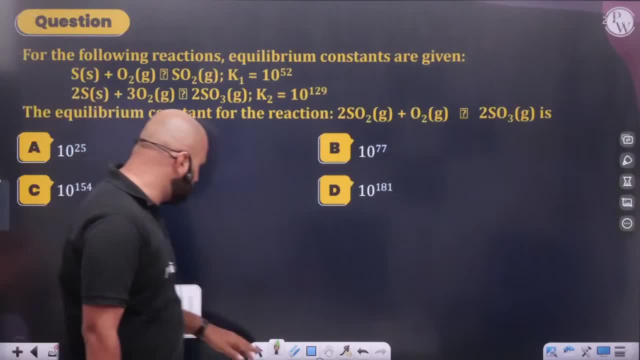 Okay, see the questions, let's see the questions. let's see the questions of chemical equilibrium, how it will start. So, sir, first of all, see this thing, see its questions, see how the questions are coming, see this question with you. 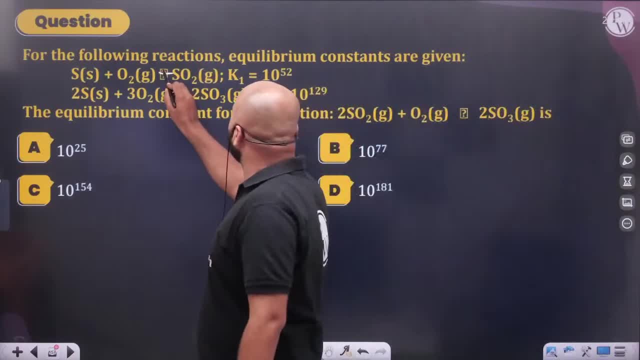 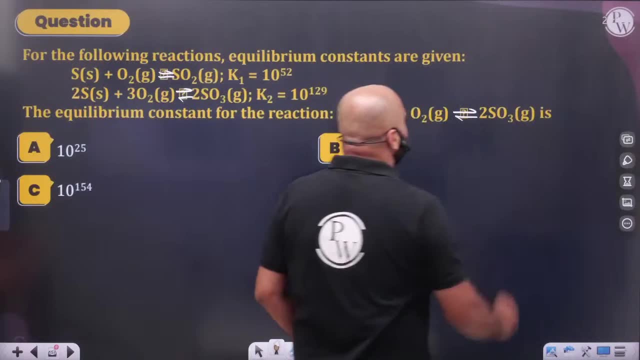 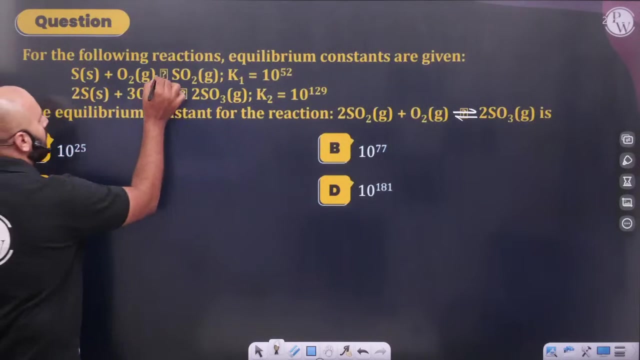 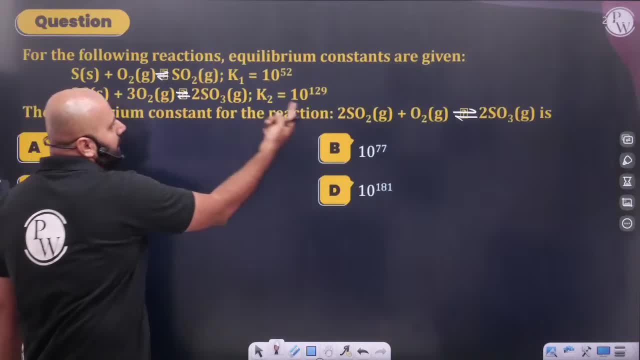 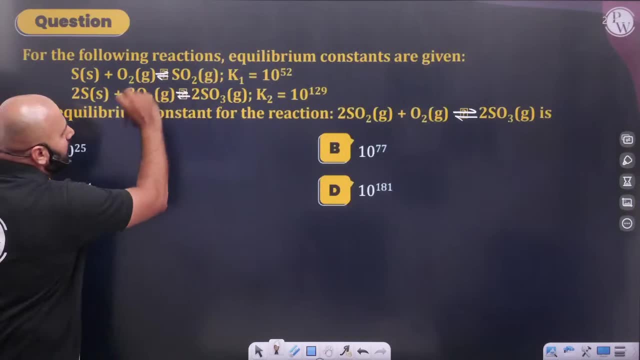 How will you find it so, brother? what to do with SO2, bring it from the reactant side or product side. where to bring SO2, reactant side? bring SO2 to the reactant side. We will reverse the reaction as soon as it is reversed. Sir. 1 upon 10 power 52.. 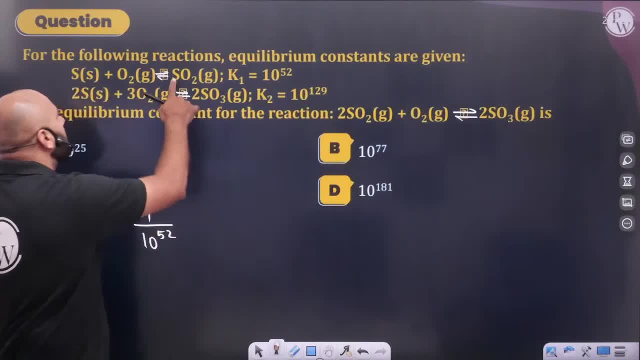 Okay, How many moles are there in SO2? 2.. So here there is only one mole. We will multiply it with 2.. As soon as you multiply it with 2, what will be the power? 2.. 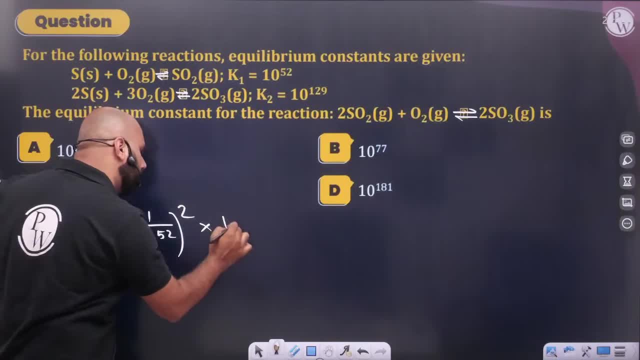 After that, where do we need SO3? We need it on that side only. If it is that much, then let it be that much. only Take out the equilibrium constant with you. What will happen, Sir? you will get its answer. 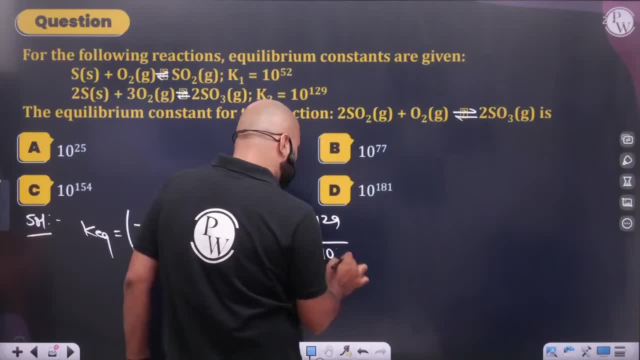 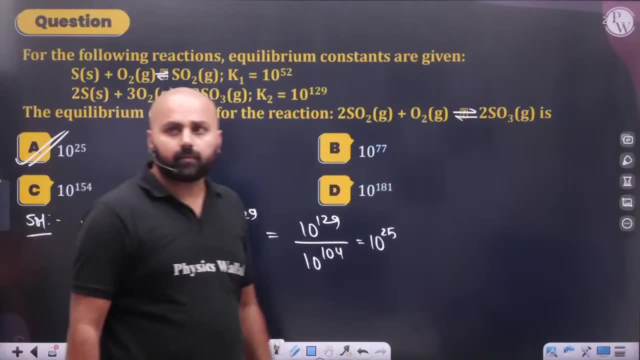 10 to the power 129.. 10 to the power 104.. How much will it come? 10 to the power 25.. How much will the answer come? 10 to the power 25.. Sure, 77,. no brother. 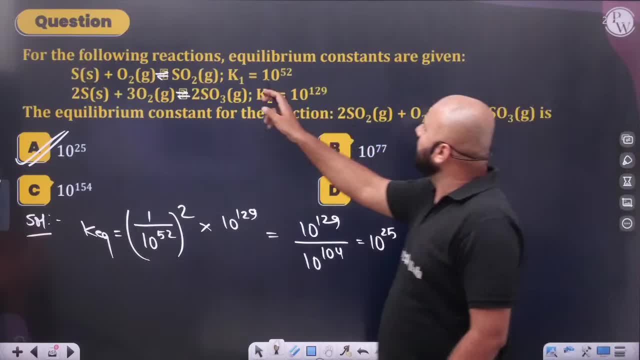 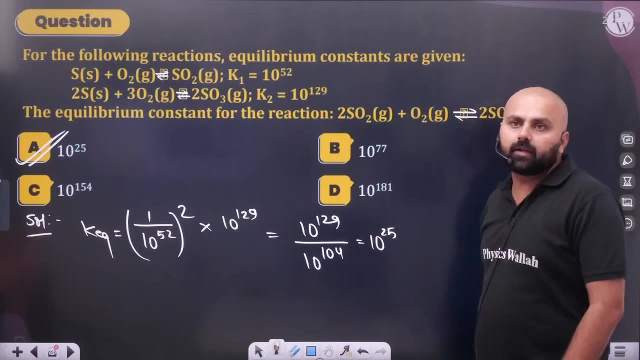 You will also reverse the reaction. You will reverse the reaction As soon as you reverse it. what will SO2 have to do? You will have to multiply it with 2. The one whose B is coming: you have directly multiplied it. 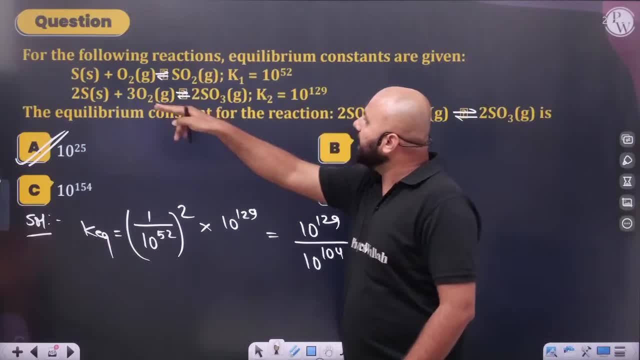 No, no, no, Sir, you reversed the reaction, but you did not increase the power. Why, Sir? you need 2 SO2, right, You need 2 SO2.. So what will you have to do for 2 SO2?? 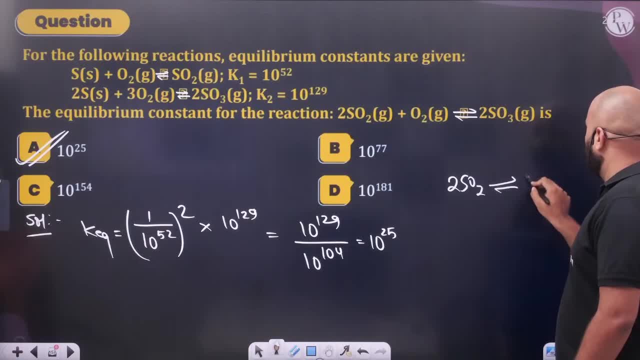 Reverse that reaction and see: See this. Write this reaction like this: Then 2S plus 3O2.. What will this become? 2 SO3.. If you add then see 2S to 2S is cancelled out. 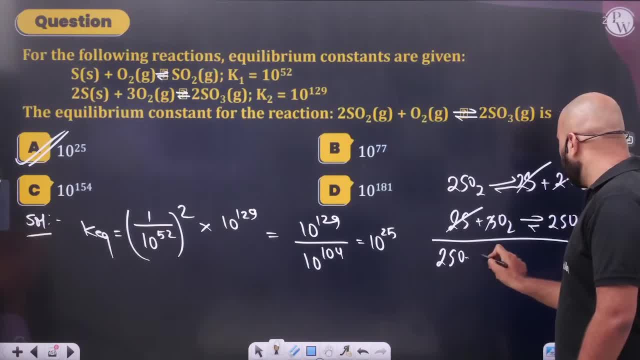 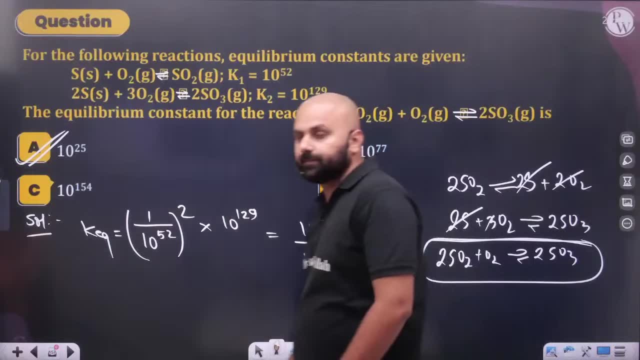 This 2 to 1 is left. So 2 SO2 plus O2.. Reverse the reaction and add it. So what will I have to do for the first reaction? I have to multiply it with 2.. Okay, Come on. 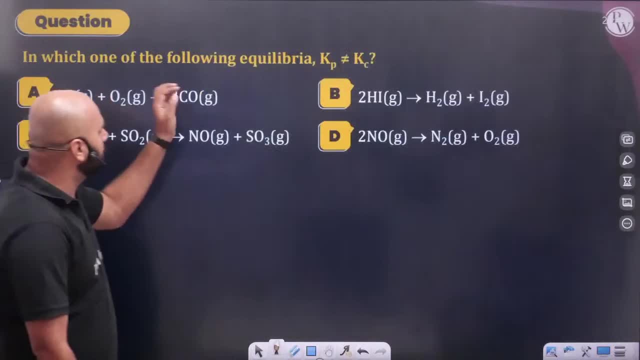 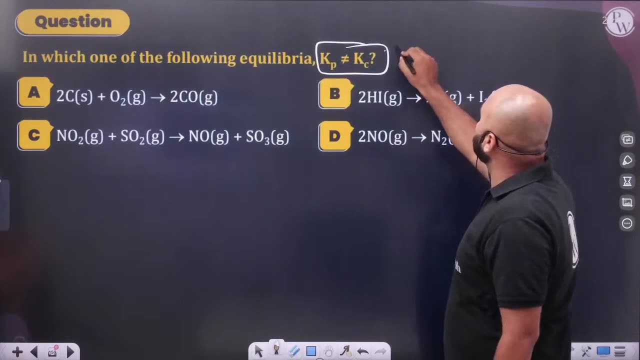 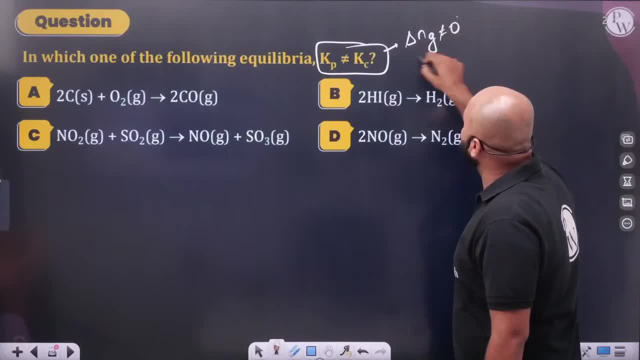 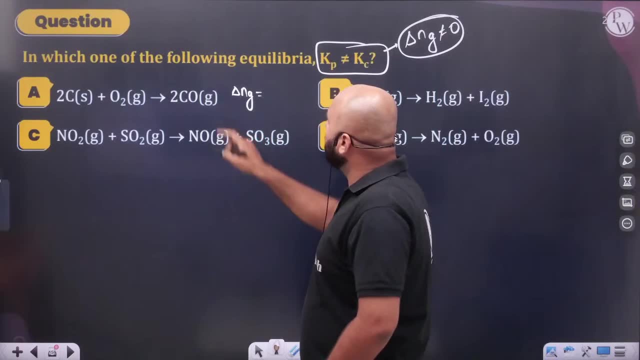 Where delta NG value is 0, there KP is equal to KC. But where delta NG value is not equal to 0, delta NG value- see What will be delta NG value here: 2 minus 1. 1.. Here delta NG value will be 0. 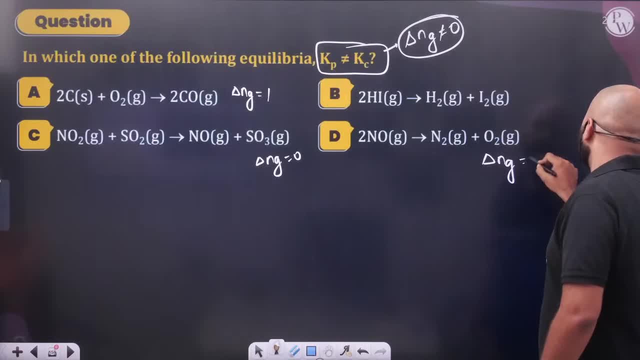 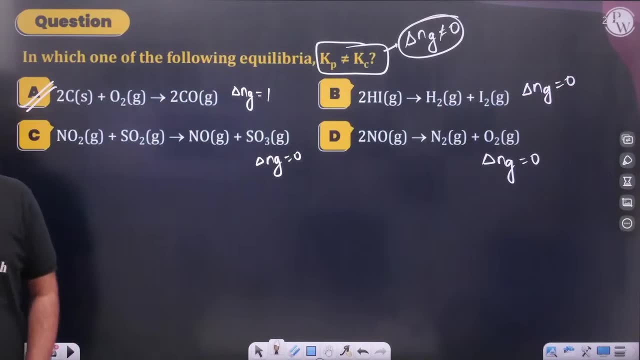 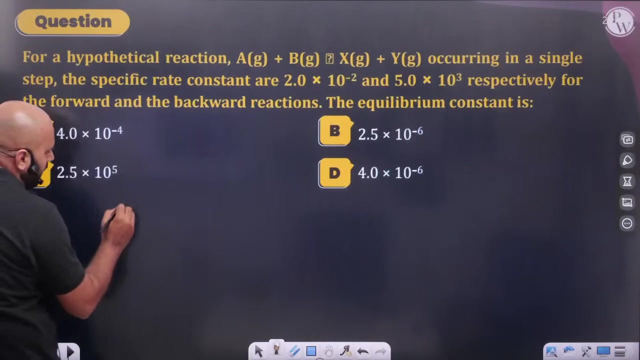 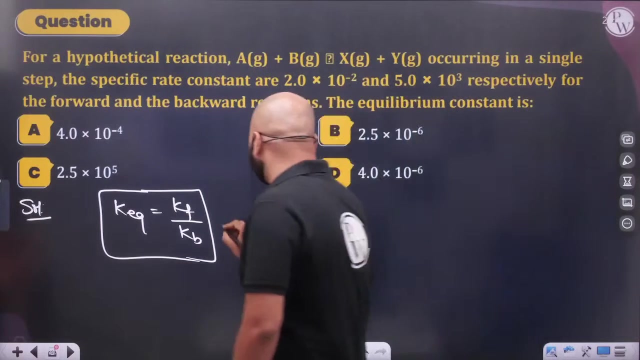 Sir, in all the options, what will be delta NG value 0.. What will be delta NG value 0. So what will be the answer A? What will be the answer A? lambda equals R. What is delta NG value here? 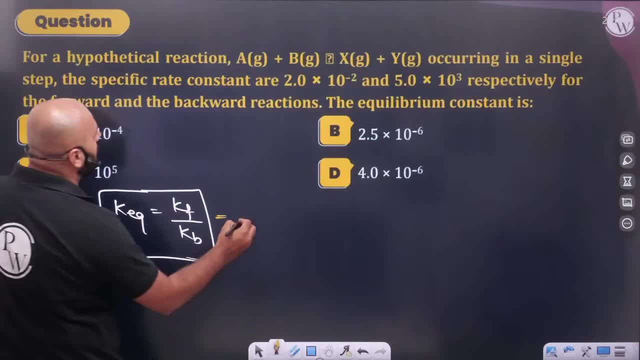 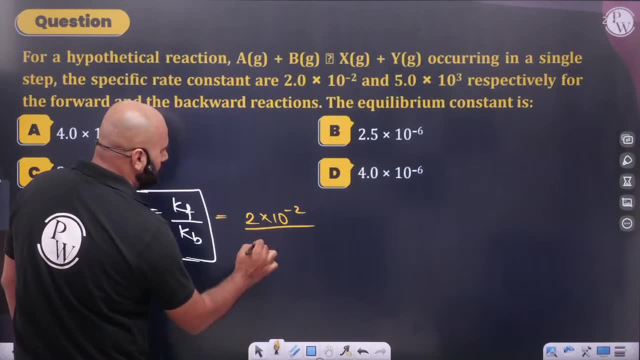 R, R, Kf upon Kb. what is the value of Kf, Sir, for which rate constant is given 2 into 10 to the power, 2 into 10 to the power minus 2, and this 5 into 10 to the power 3.. 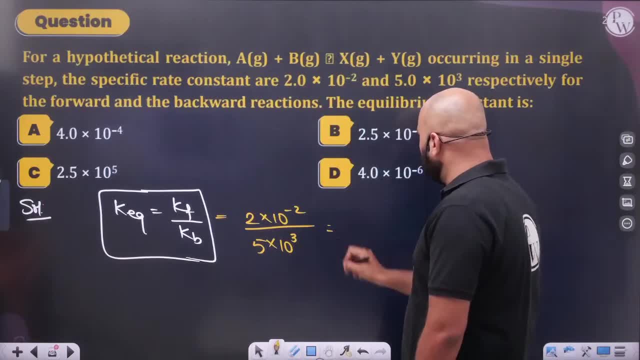 What will happen? 2 into 10 to the power minus 2, 5 into 10 to the power minus 3,, 0.4 into 10 to the power minus 5, and we can say 4 into 10 to the power minus 6.. 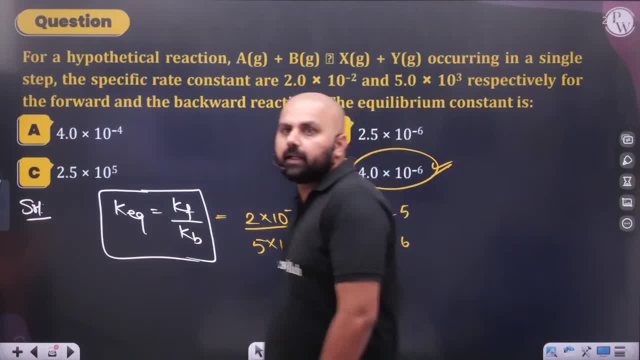 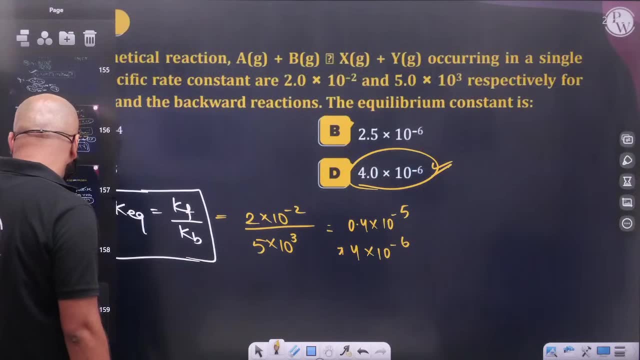 What will be the answer? D answer will come. What will be the answer? D answer will come. Okay, what will be the answer? D answer will come. So keep doing such questions. See all the questions of equilibrium constant. Now see this question: How much correct question we got? 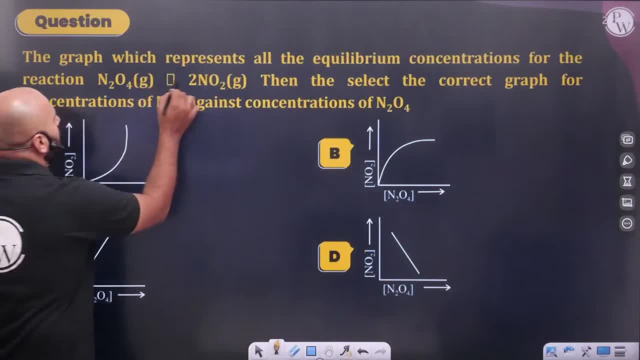 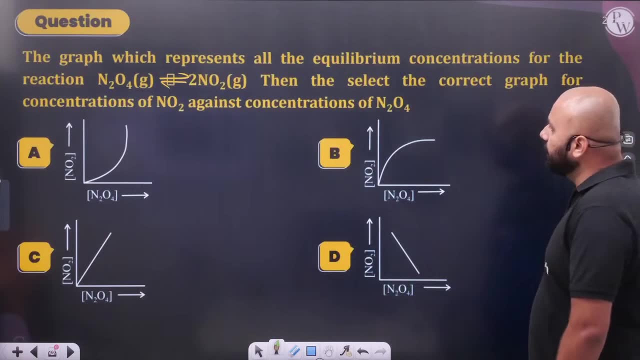 See this question. How will you do this question, Sir? N2O4 is there. N2O4 is going to NO2.. N2O4 is going to NO2.. It is being said that. sir, tell me the correct graph: Concentration of NO2 against concentration of N2O4.. 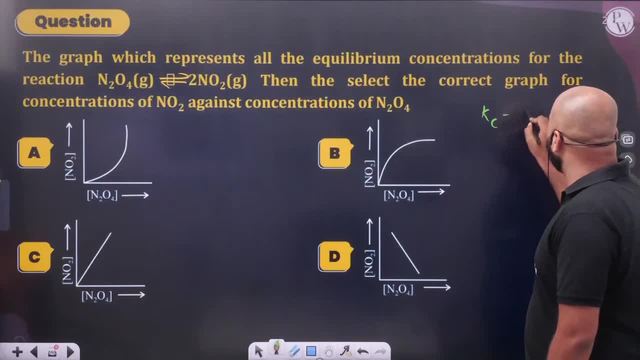 How will you find it? So see this: What will be the value of Kc? I want to write the value of Kc, Sir, see all these questions. You have to be ready N2O4.. You said that, sir, let's do one thing: On which side to take NO2?? On Y axis? 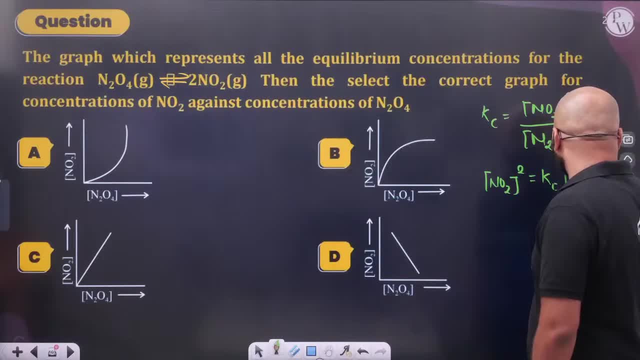 So NO2's whole square is nothing Kc into N2O4 can be done. And what is this? NO2 is Y square and Y square is equal to. if I say Y square and here is X, then what will happen to us? 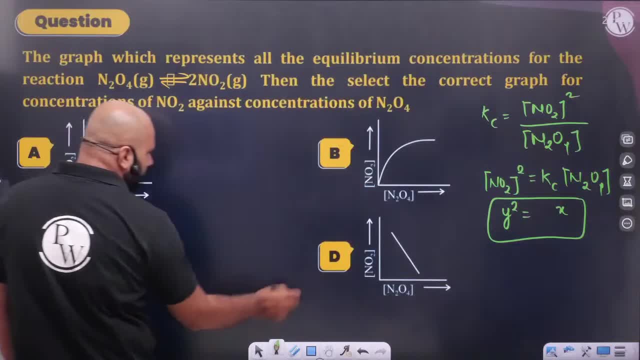 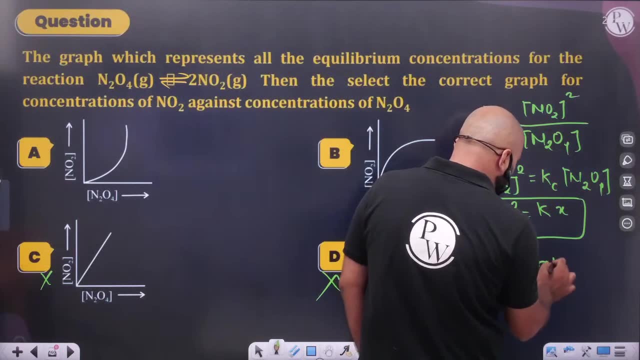 Will this be a parabolic graph? As soon as the parabolic graph came, I can cut C and D. Why? Because if Y square is equal to Kx, then what will be the nature of the graph? It will be parabolic. It will be parabolic nature. Y square is equal to Kx, So what will be the nature of the graph? 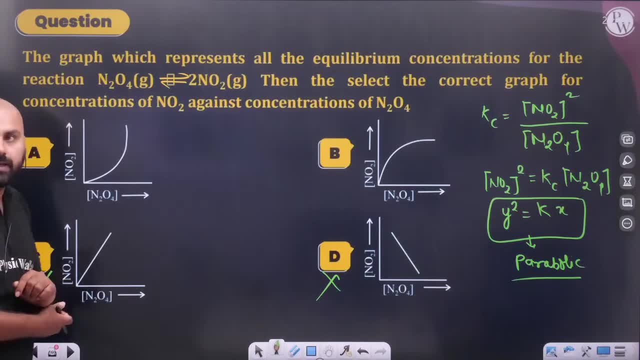 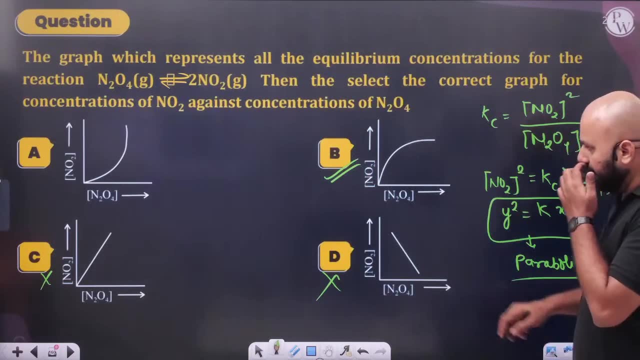 It will be parabolic. And as far as it is visible that, sir, Y square is equal to X, what will be happening in that case? What will be the answer? B, Because see what will be the graph of Y square: X. It will be open towards X. 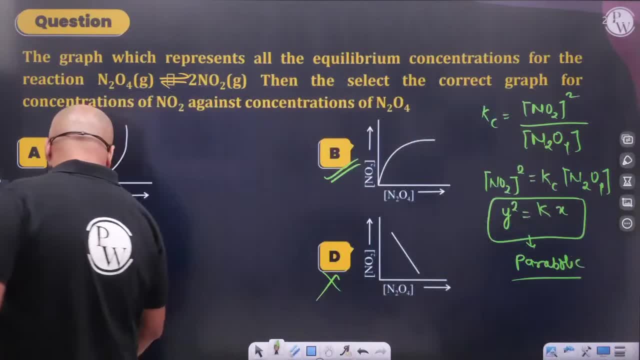 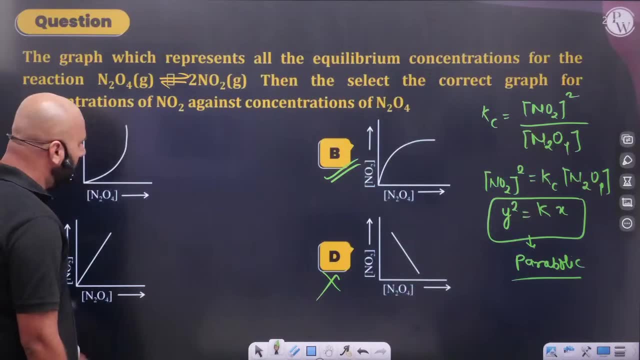 Take it out like this: It will be done, sir, Are you sure? Now see what I was told. Now stop here. You have to see here. Now two more things. come here. Let's come to the application of equilibrium constant. 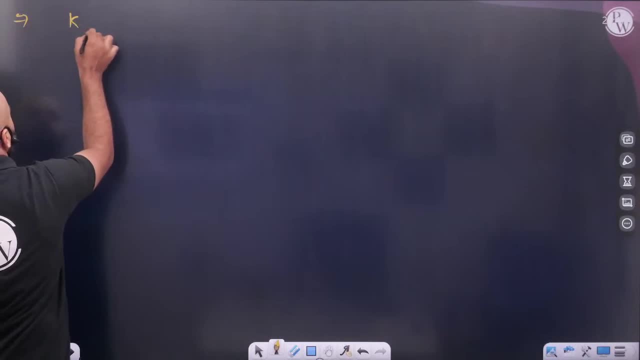 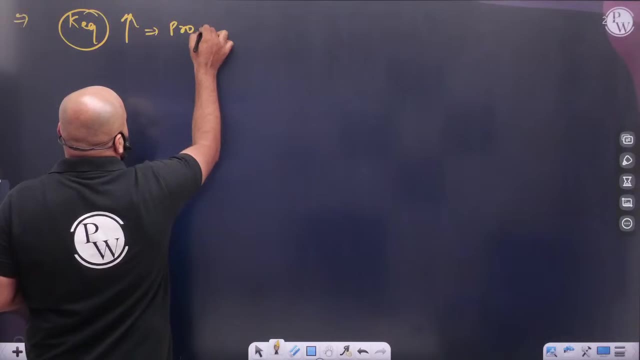 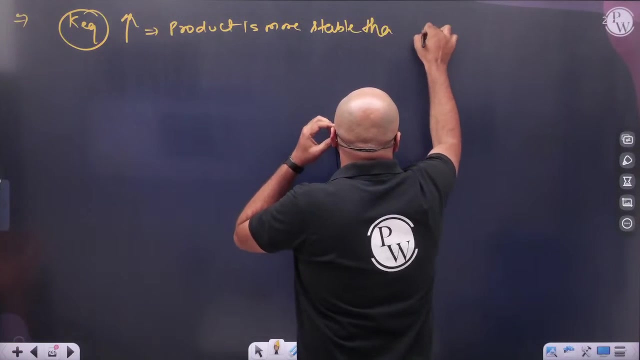 The value of the equilibrium constant is more. if the value of the equilibrium constant is high, If the value of the equilibrium constant is high, if the value is high, it means the product is more stable. Product is more stable, More stable. The equilibrium constant can only be more stable than reactant. 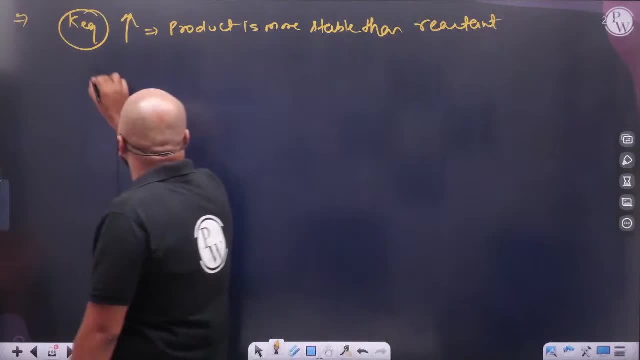 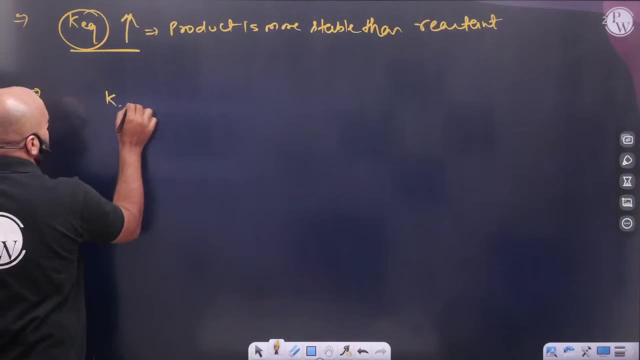 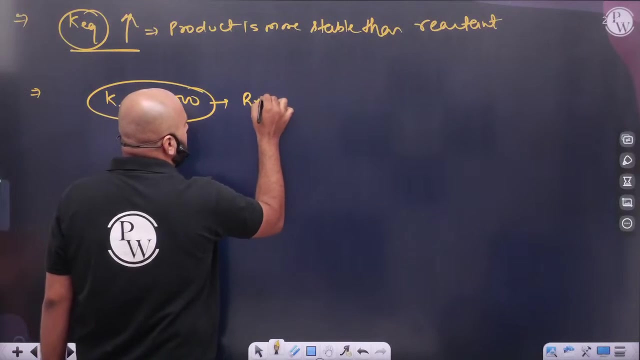 See your equilibrium constant. If the equilibrium constant is high, it means the product will be more stable as compared to reactant. If the equilibrium constant is greater than 1000, then in this case, where will the reaction happen? Reaction is almost completed. What is the reaction? Almost completed Why? 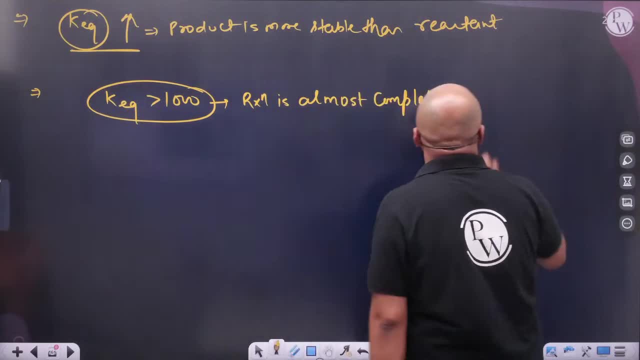 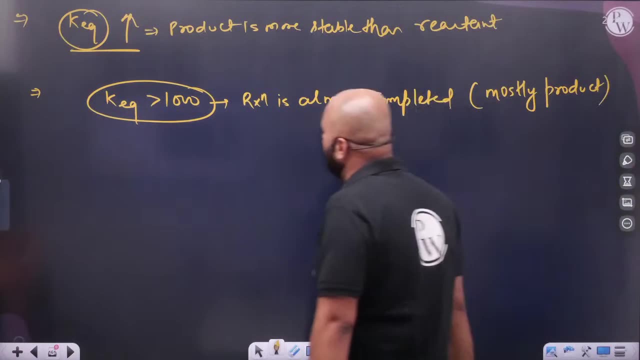 Because already you have it, It is greater than 1000.. What is there? Mostly what will you get there? You will get the product. Mostly what will you get? You will get the product. If I talk about the equilibrium constant, it is less than 1 by 1000.. 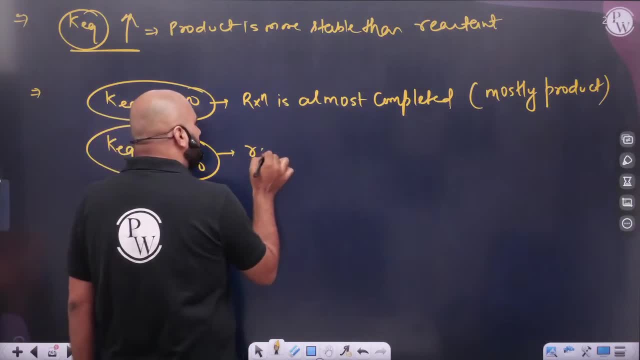 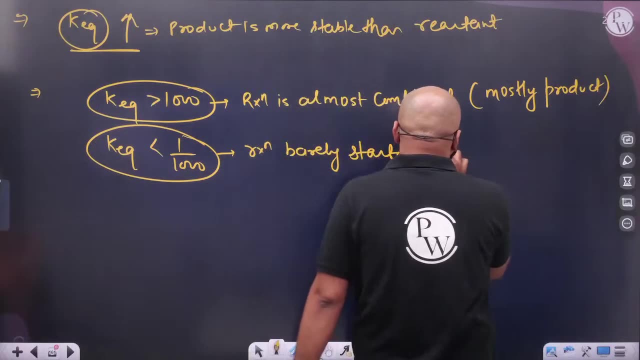 If the value of the equilibrium constant is less than 1 by 1000, then the reaction barely started. It has not started. Why? Because your reactant has been used very less. So what will come here? Mostly, what will go If the reactant comes? 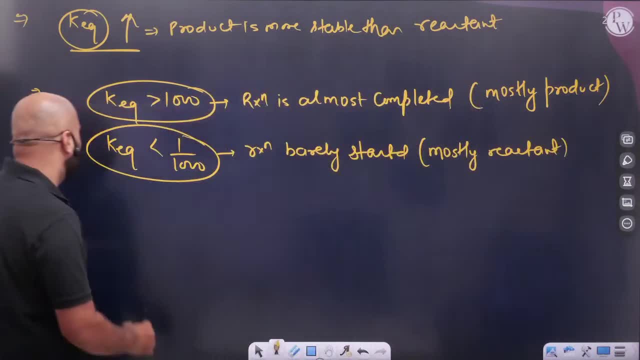 If you see the equilibrium on the mixture, then mostly what will come? The reactant will come, And if the equilibrium constant is greater than 1 by 1000, then it is less than 1000. So in that case, what will happen to your reaction? Reaction mixture or equilibrium mixture? 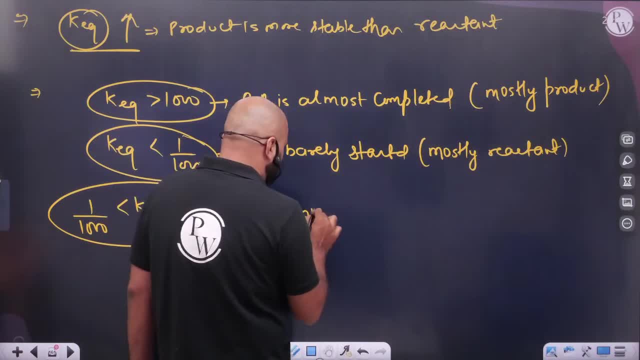 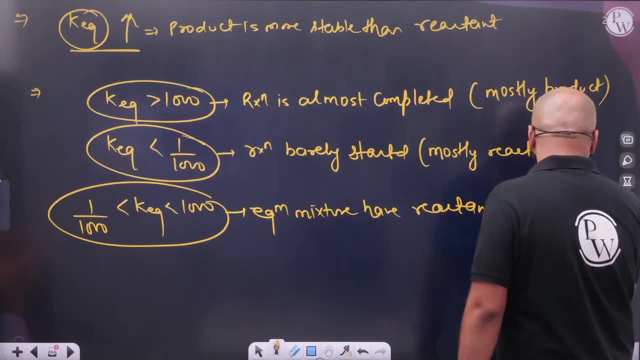 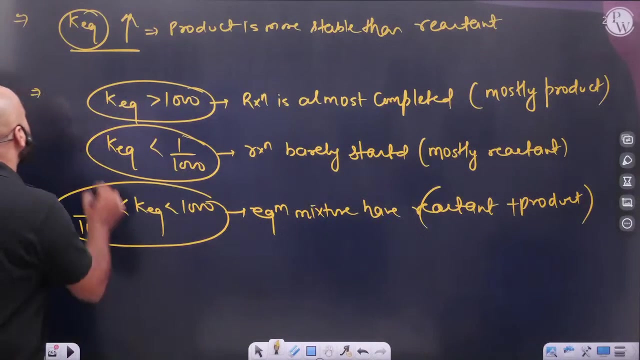 We can say that the equilibrium mixture has reactant plus product. Sir, they will also have reactant. What else will happen? Product will also happen. So tell this to yourself. It will happen, sir. So this will happen. So these are the small things that you can tell by looking at the value of the equilibrium constant. 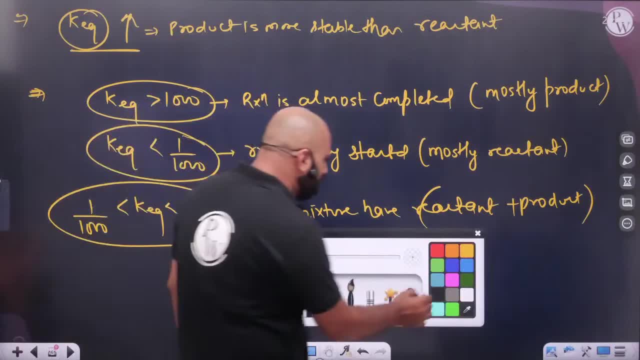 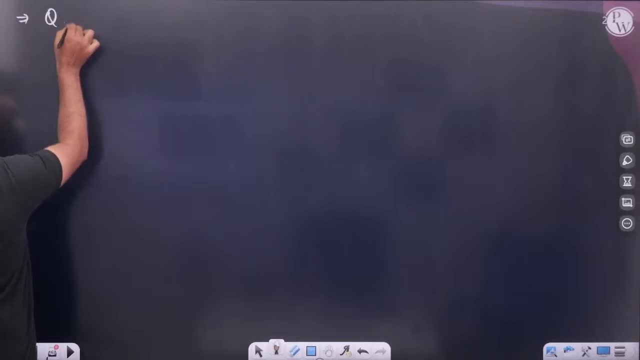 If it is very high, it means the reaction is almost complete. Otherwise, keep doing it with yourself. Then here comes one or two more things. See this: I was told that, Sir. reaction, What is qc? The reaction is quotient. The QC is what reaction is quotient? 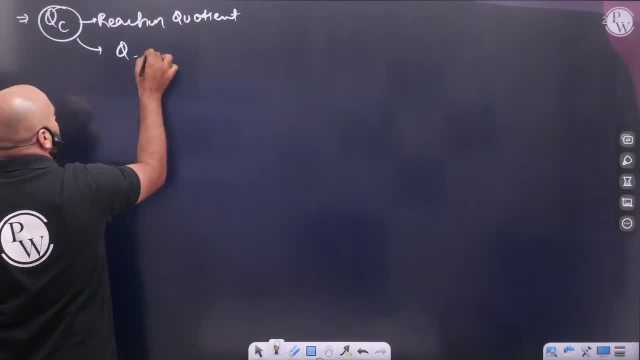 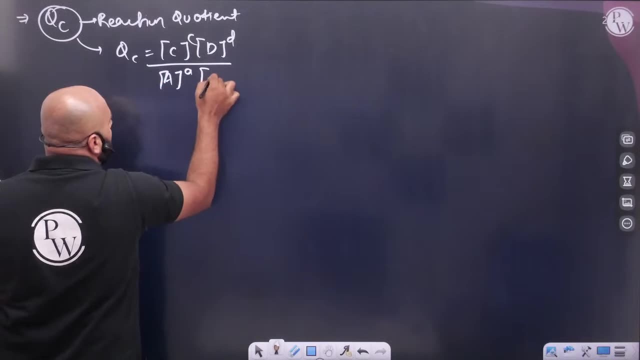 The difference is in both. The reaction is quotient. The formula is same. in the formula KC, The situation of the same formula, But there is a difference. It is defined at any moment in time. It is defined at any moment of time. Defined at any moment of time. 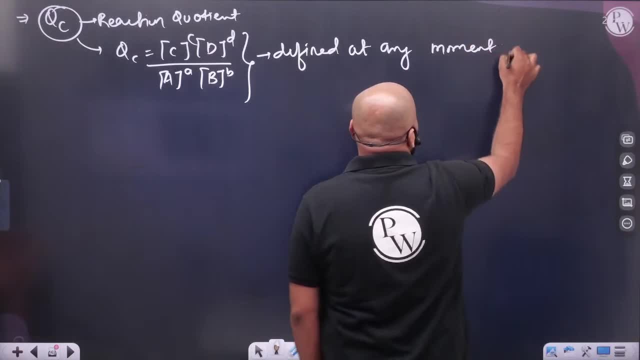 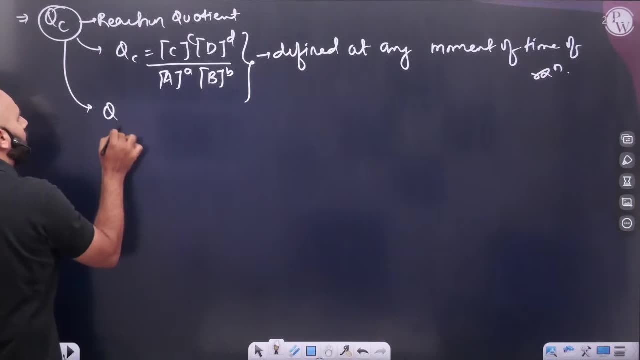 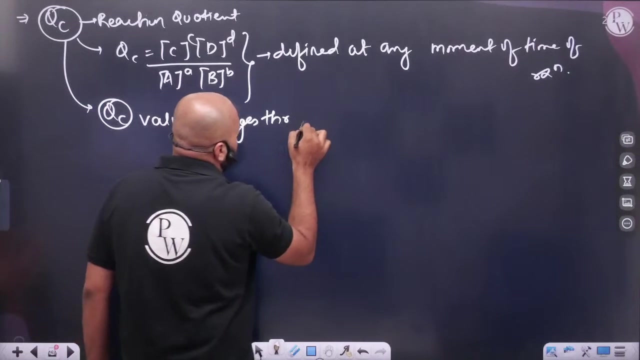 Have any moment. It is defined at any moment of time. Any moment of time of reaction is defined on the reaction. The value of QC fluctuates. The value of QC changes throughout the reaction, Changes throughout the reaction, From the beginning to the end. it changes throughout the reaction. 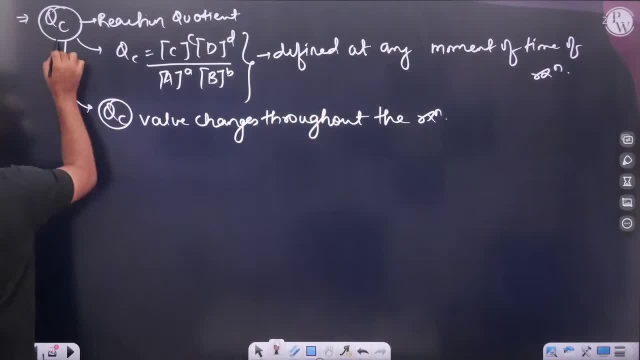 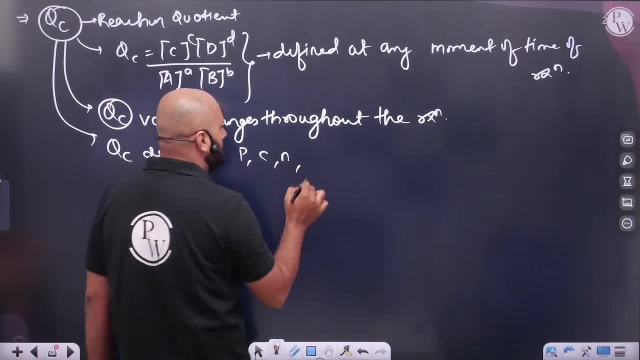 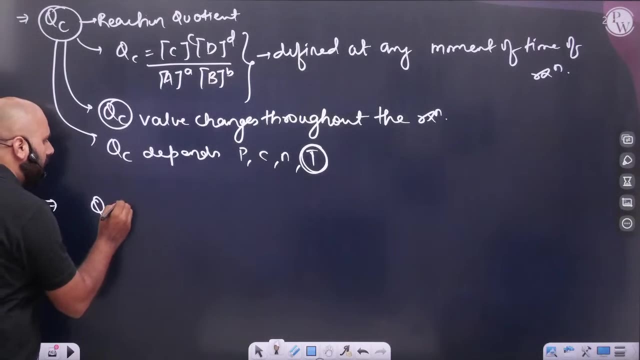 From the beginning to the end. your value changes in the reaction. If we talk about QC, then QC depends on QC depends on pressure, concentration, number of moles and temperature. It will depend on everything. QC is an indicative. If QC is less than KC, then the reaction has not reached the equilibrium. 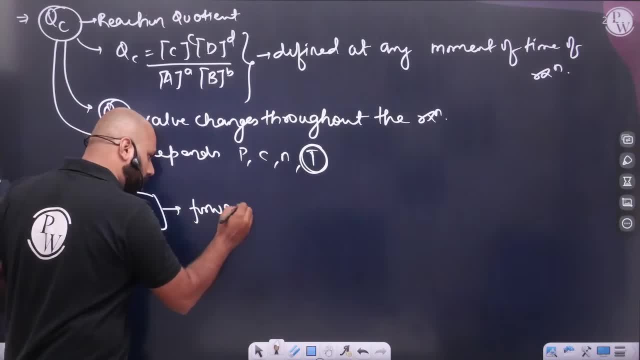 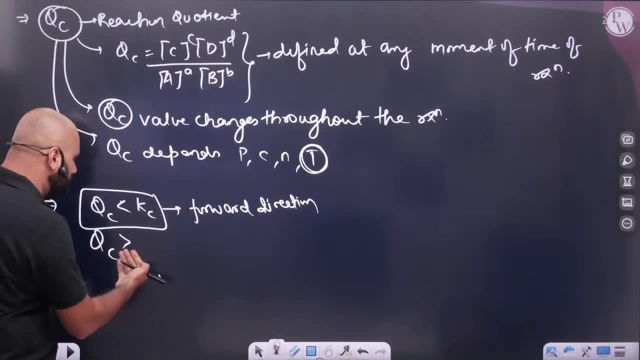 Where will the reaction go? In the forward direction? And if QC is greater than or equal to KC, QC is greater than or equal to KC. QC means where will the reaction go? Where is the reaction? It is at the equilibrium. Where is the reaction? 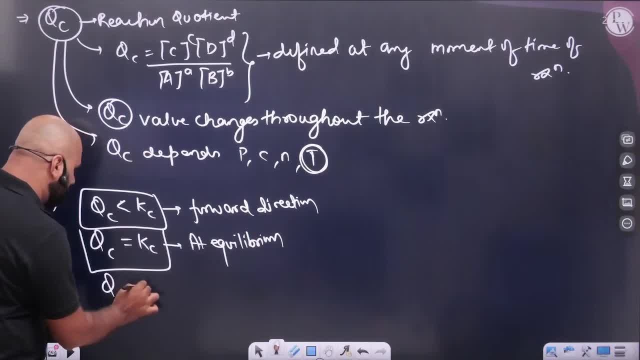 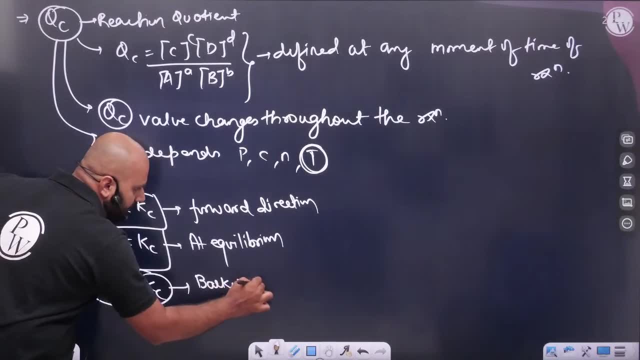 It is at the equilibrium. And if QC is greater than or equal to KC, In this case, where will the reaction go? In the backward direction In this case, where will KC go? In the backward direction. So, just keep doing QC and KC, Keep doing forward and backward. 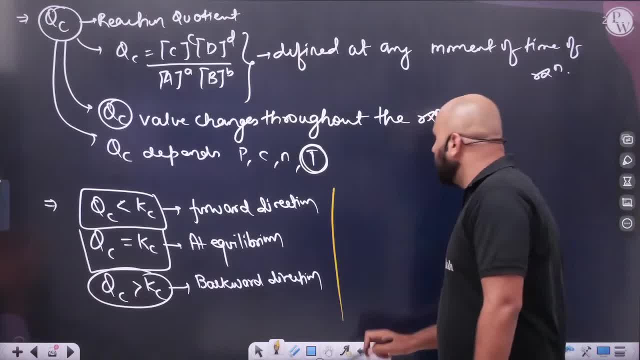 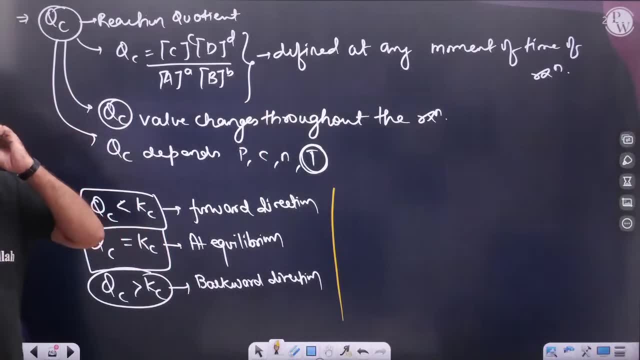 After that, who told me that, Sir, you can decide one or two things by looking at QC and KC? Then I will question you once. I will question you once. Okay, I will question you once. What happens? Let's decide by looking at QC and KC. 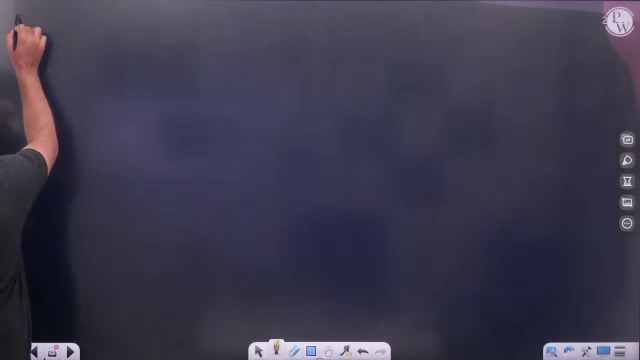 Then who said: Sir, at the equilibrium, How is the equilibrium mixture, How is the equilibrium mixture? Listen carefully: what is the equilibrium mixture, What is the equilibrium mixture, Sir? equilibrium mixture means What will happen at the equilibrium, Sir. I am telling you again and again. 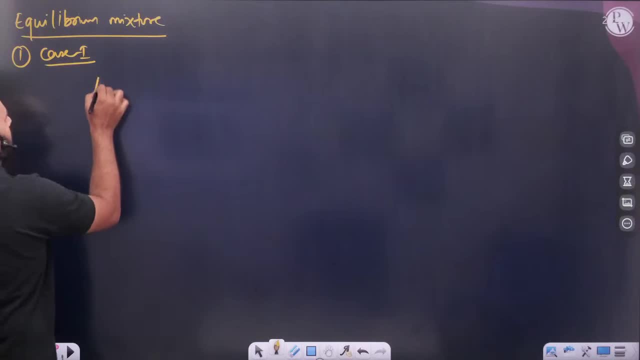 Look at these questions. Case 1: If you are being told In two ways, What will you be told? You are going to B. Your time is equal to zero. In the exam hall, the concentration will be given like this: This zero Time is equal to equilibrium. 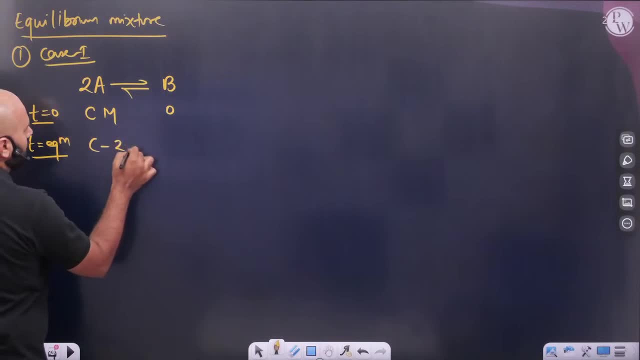 Nothing. What you have to do? You have to do C minus 2X, Because if its two moles go, Then its X moles will be made. You can write the value of KC directly, Sir X, And what is this Whole square of C minus 2X? 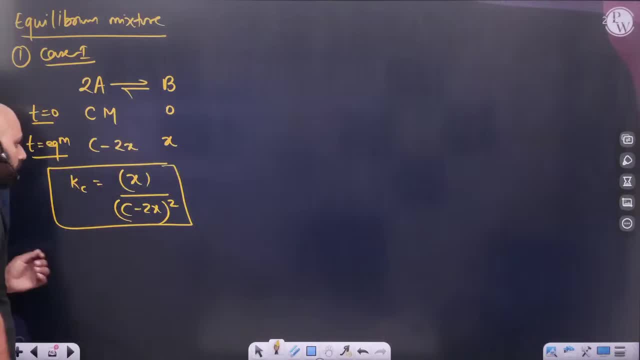 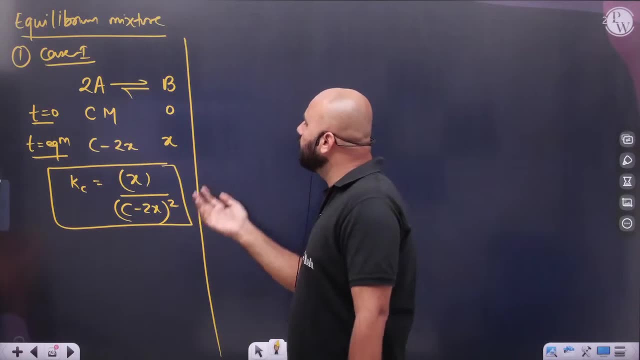 In the exam hall. one or two values will be given. Decide and remove it. Decide and remove it. Nothing else In this. the value of KC will be given, Or the value of X will be given, Or the value of C will be given. Some or the other two values will be given. 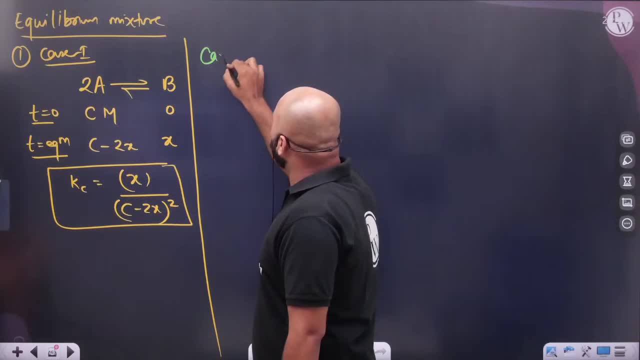 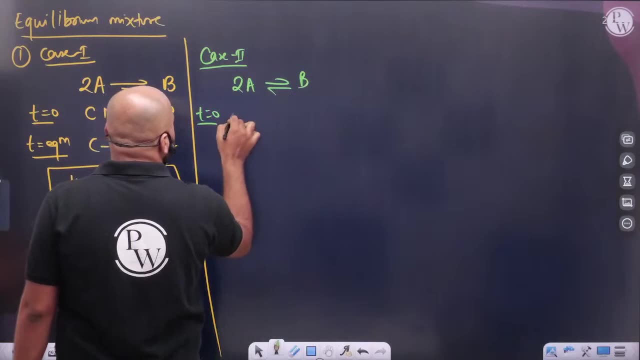 Remove the value of the third. What is case 2?? What will you be given in the exam hall? Same reaction will be given. Same reaction will be given. What will you do here? Will give N moles here. So no problem. Time is equal to equilibrium. 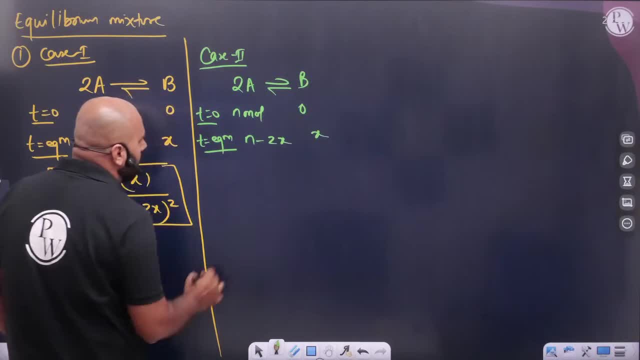 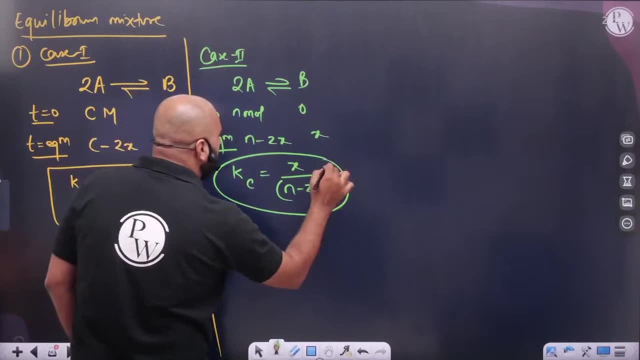 What will you do? N minus 2X- What is this X, Sir? the value of KC here, Direct X. Can't put the whole square of N minus 2X. Until and unless Until you are told That the volume is one litre, What will be the value of KC? 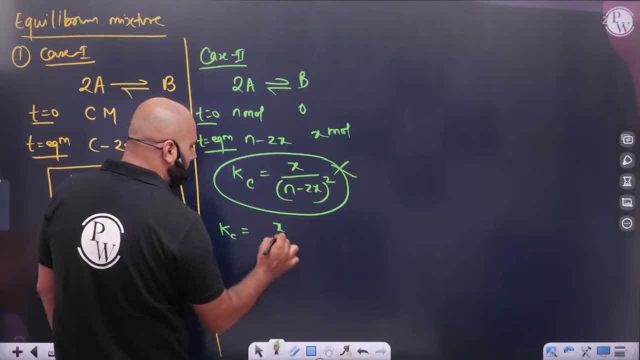 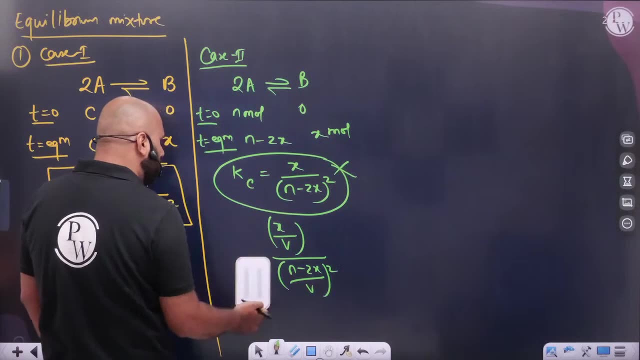 Sir, moles have been given. These are all moles. So X by. We take concentration N minus 2X upon The whole square of the volume. What will be the value of KC? This will be. What will be the value of KC? This will be. 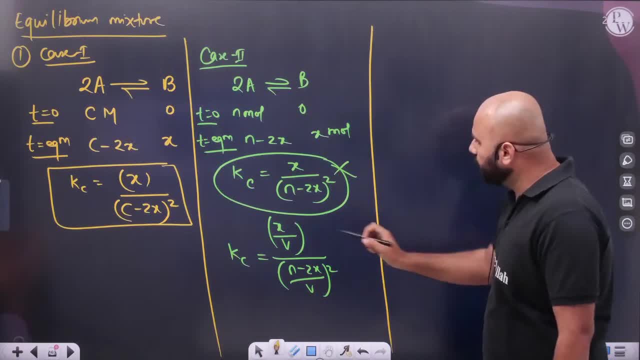 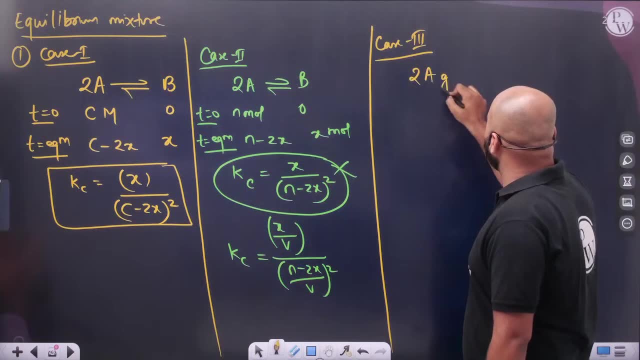 So see this: What will be the value of KC? This will be So. this comes in case 2. Then someone says, Sir, let's take case 3. See in case 3 If there is 2A gas, If this 2A gas is. 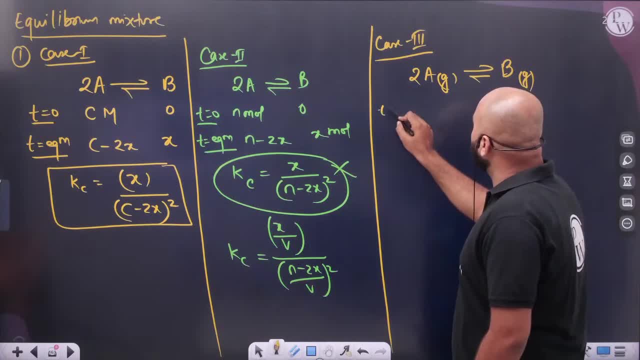 Converting into B gas, Then in that case Time is equal to 0. If its pressure is P, This is 0. Time is equal to equilibrium. If I do P minus 2X from here, Then what will come here? X. And if I go to find the value of KP? 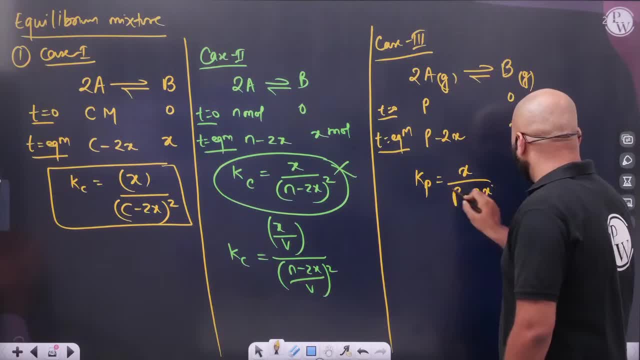 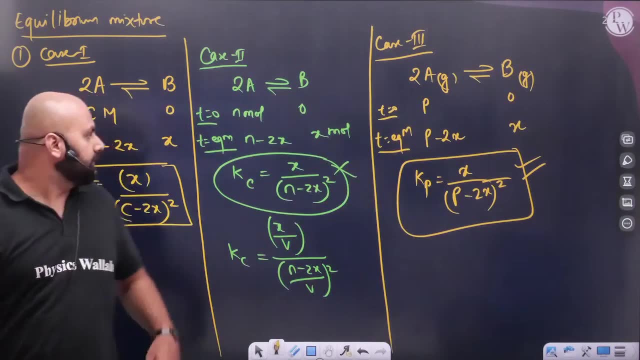 Then X upon P minus 2X, The whole square will be. The value of KP will come here. Keep taking out. So take out KC and KP, like this Concentration. Obviously, the molarity has been given Here. the molarity has been given Here, the moles have been given. 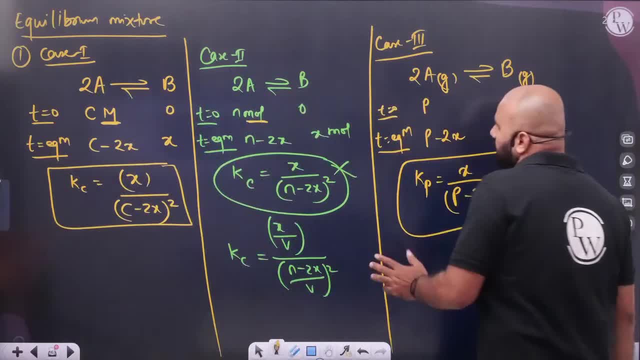 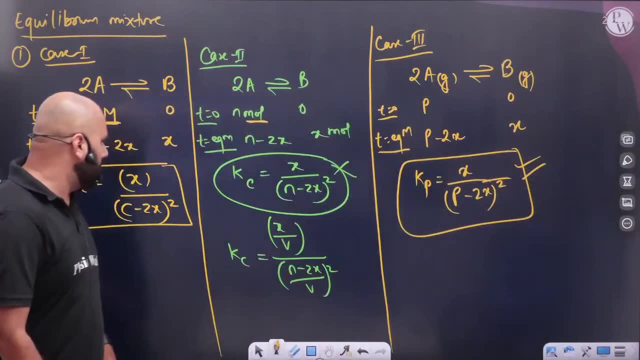 In the case of moles, Volume has to be divided. Here the pressure has been given. Simply divide it Here. in these three cases, No more tension comes In the exam hall Straightly. Who didn't take the square, Brother? I have taken the square of everyone. 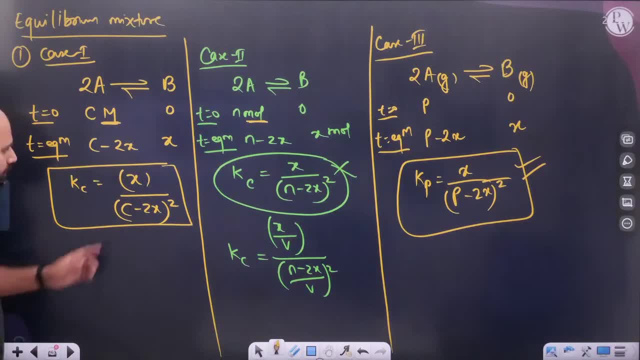 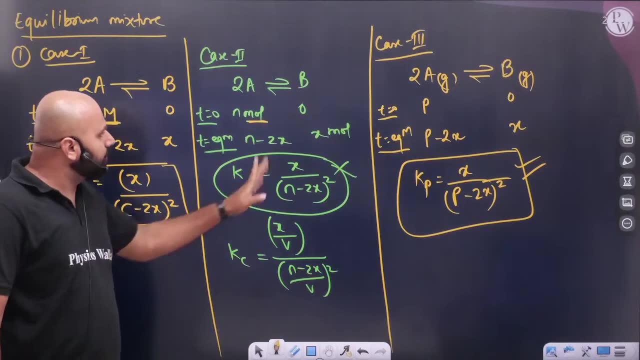 I will take the same square of A. I won't take the square of B. I won't take the square of B, I will take the same square of A. Okay, See you directly here Here. No more tension. After this comes a tension thing. What comes after this tension thing? 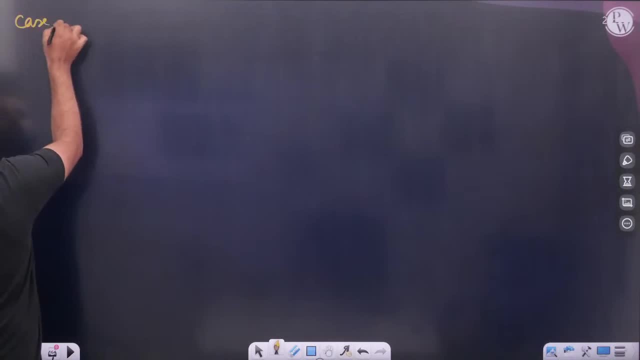 That comes case four. What happens there? Alpha concept comes. Alpha means nothing. Degree of dissociation. What is the problem with degree of dissociation? Whenever it will be defined, It will be defined for one mole. It will be defined for one mole. It is defined for one mole. 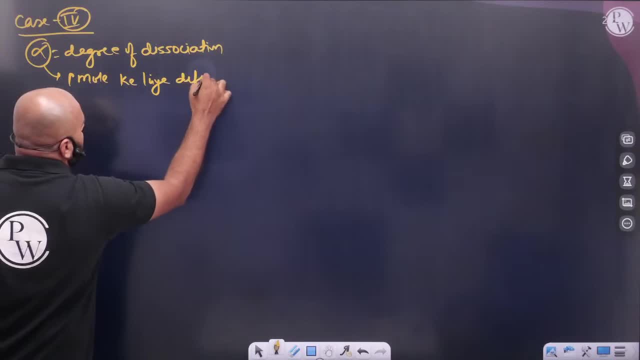 It is defined for one mole. It is always defined for one mole Means if something has been given somewhere, If you don't know, Then alpha means nothing. Its alpha has to be taken out in fraction. Alpha is in fraction. Alpha is in fraction. Its value is from zero to one. 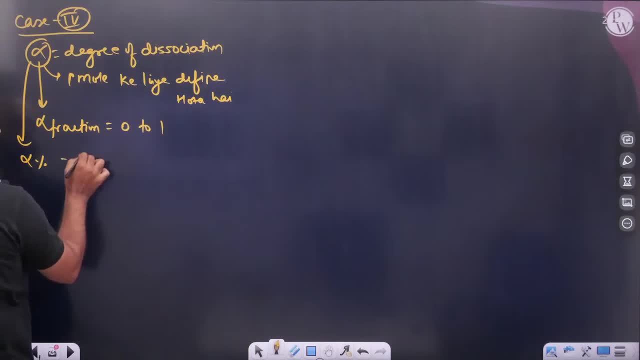 But alpha is sometimes given in percentage, So it is nothing. Alpha fraction: What do you multiply it with From hundred, So what does it come? It comes in percentage from fraction. See this. If I talk about case four, I write the same reaction again: There is nothing in the exam hall. 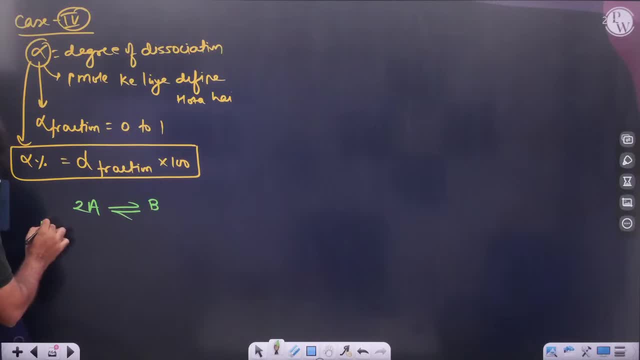 So what will I do When nothing is given? Then I can take its one mole. What is the difference? How much will it be? Zero Time is equal to equilibrium. See carefully, Sir. now, from one mole, What does alpha mean, Sir? degree of dissociation. 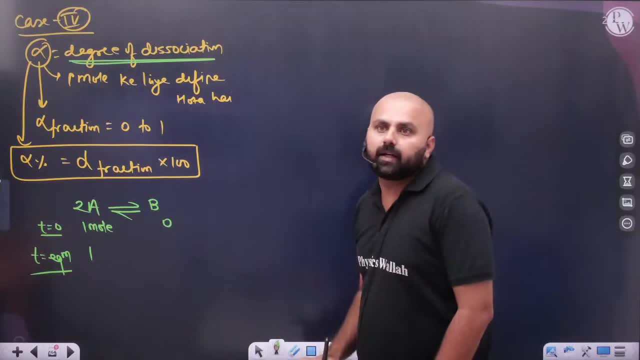 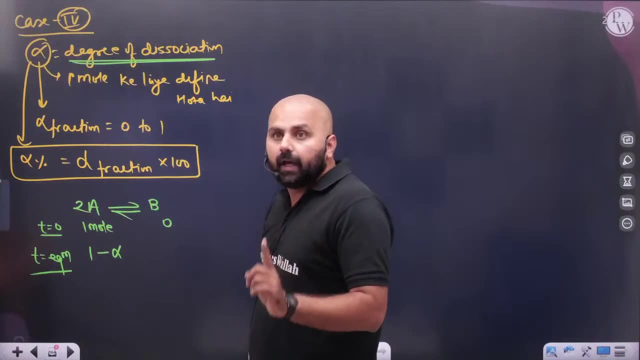 It is so defined from one mole. Listen carefully. It is so defined from one mole Means How much will go from one mole? Alpha will go. Why Don't do two alpha here In x and two x? There is a difference in x and alpha. Listen carefully. 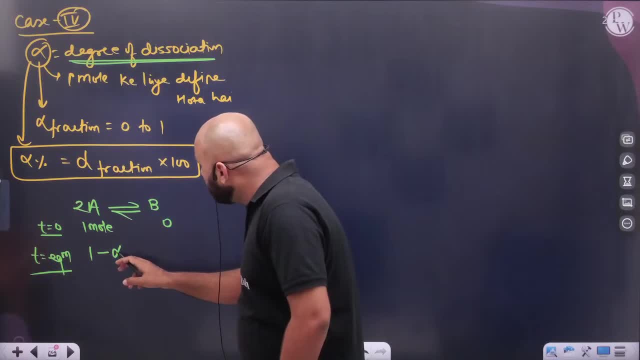 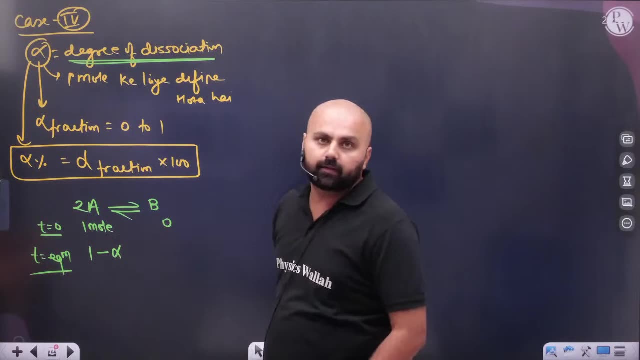 There is a difference in x and alpha. Alpha does not decide whether it is two or three. Alpha does not mean, Alpha just sees how many moles are there. Here is one mole, So what will I do? One minus alpha. If there are ten moles, Then ten alpha. 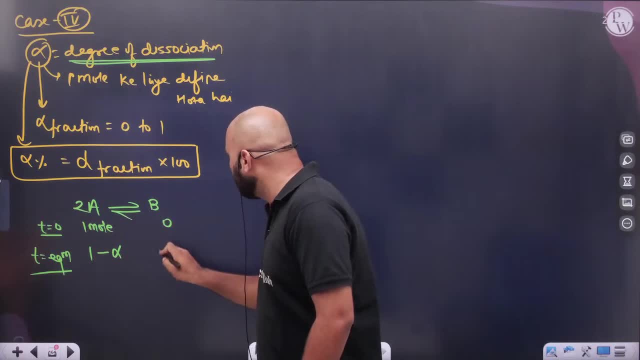 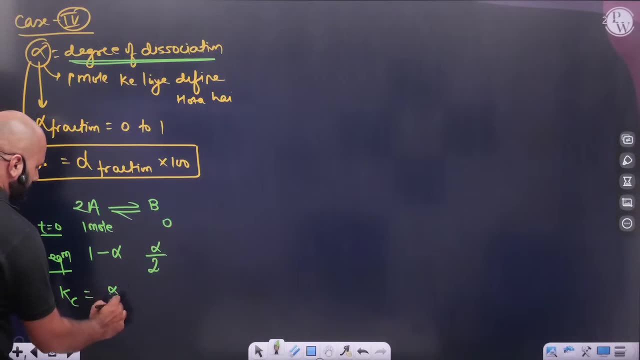 See, here, Now put a stash meter here. Two moles and one mole. So from here How much will it be from alpha, Alpha by two. And now if you take out case, So what will be the value of case Alpha by two Divide by Alpha by two? 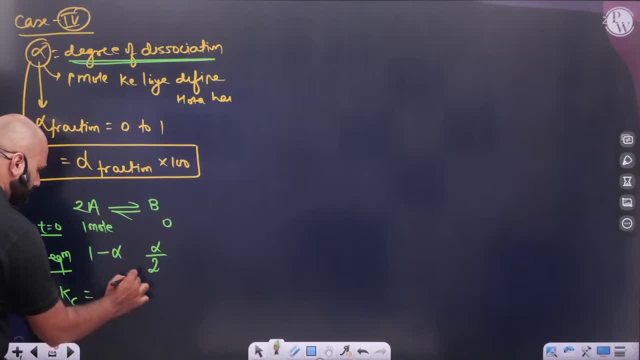 Volume will also have to be divided Because there are moles. So alpha by two will be. So alpha by two, V Divide by One, minus alpha by V, Whole square. This will be the expression of my case, Remember, Whenever, If I had put a different condition in this. 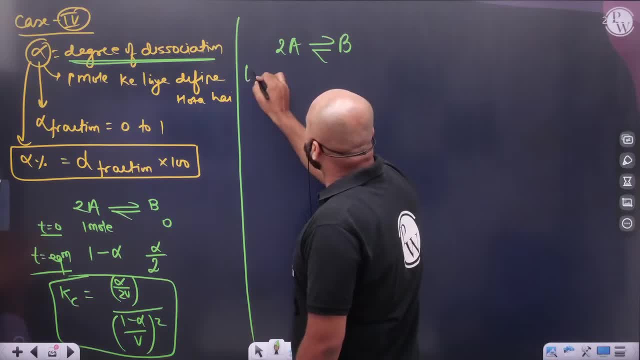 See the same. I would have written this reaction: If time is equal to zero, If ten moles were given here. So I, brother, I am saying again and again: See, time is equal to equilibrium, Sir. here ten minus twenty, And that does not mean two alpha. See this. 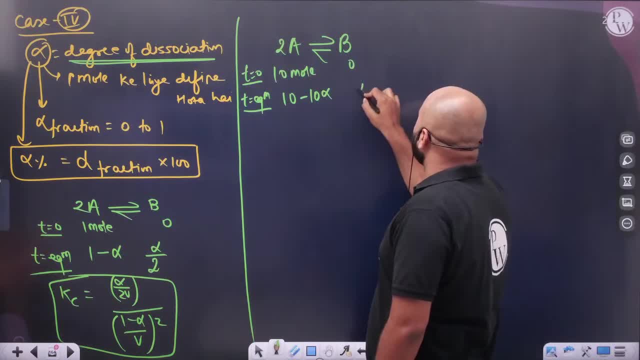 How much is alpha for one mole, So how much will it be for ten moles? Ten alpha, How much will this be? Now? put the basic math here, It is half of two moles, So how much will it be from ten alpha, Ten alpha by two? 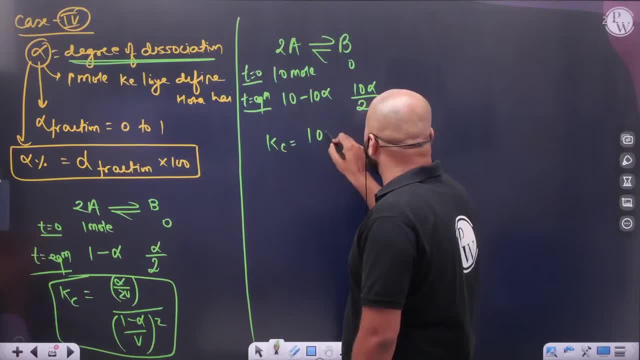 Sir, see this. Take out the value of case. Ten alpha by two. V Volume will have to be divided. Divide by Ten minus Ten alpha Upon V, This will be the square of this. So take out the case Whenever alpha will come. Whenever alpha will come, Brother, look at yourself. 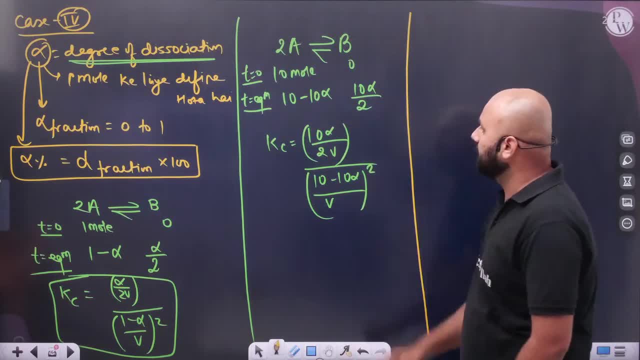 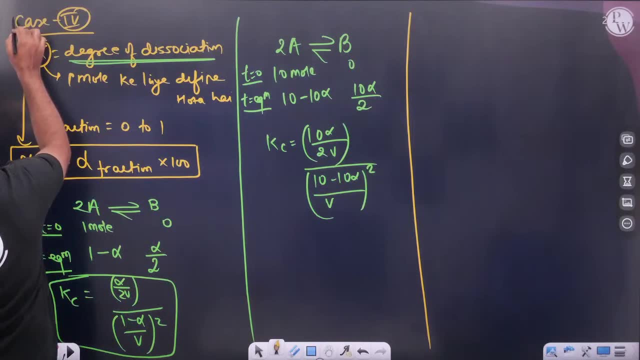 Whenever alpha will come, It always comes for what Comes for one mole. Comes for one mole Comes for one mole. According to that, Take it out. This is its case four. It is more interesting than this. Its case five, And that is our last case. Then we have our case five. 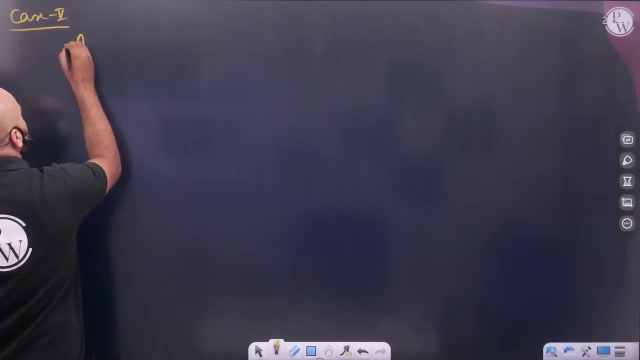 What does case five say? That, brother, If this reaction 2A With gas And alpha is given, If you do it with gas, Then alpha is given. Like time is equal to zero. Consider its one mole. How much is this Zero? Time is equal to equilibrium. 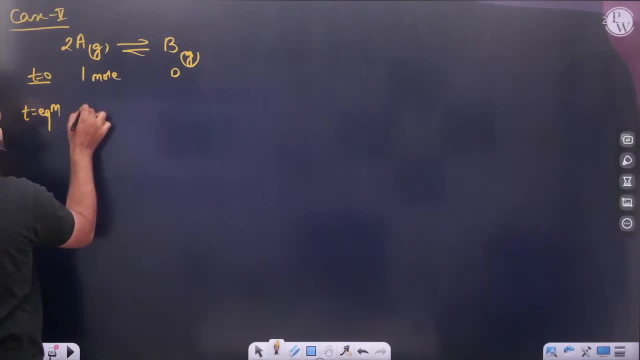 How much of this One minus alpha? How much is this Alpha Alpha? How much is this Alpha by two? But all these are in moles. The problem is not that Here it will say: Take out kp, So not kp. What will you have to take out first? 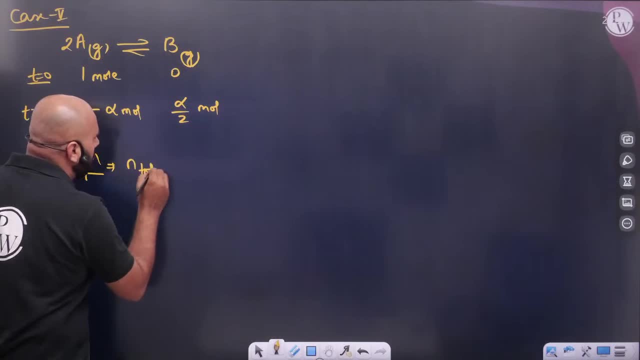 At equilibrium. See how to take it out. Take out n total. Take out number of moles: total. How many are there? One minus alpha, How many moles will be here? One minus alpha, Plus alpha by two. One minus alpha by two. This is done At equilibrium. 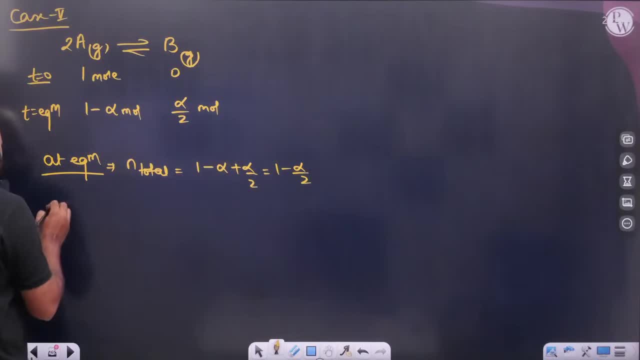 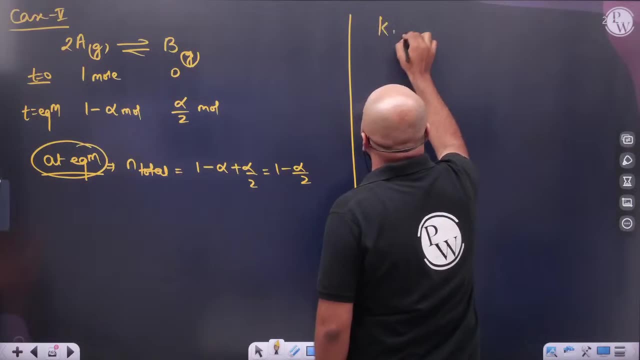 This will come On equilibrium One minus alpha by two comes. Okay, Sir, Here You have to take out kp. See, I will write What I have to take out. Take out kp. What will kp be? Pressure of b And Pressure of a power Two. How will pressure of b come? 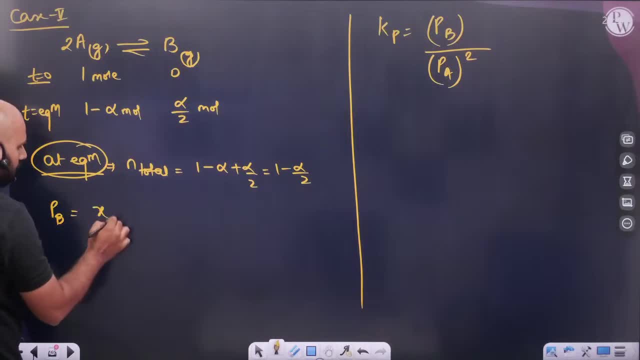 So Pressure of b. Using Raoult's law, What will be said? Mole fraction of b Into p Equilibrium. Tell on equilibrium, Sir. How will pressure of b come? So, sir, How much is the mole fraction Alpha by two And Divide by How many moles are there? 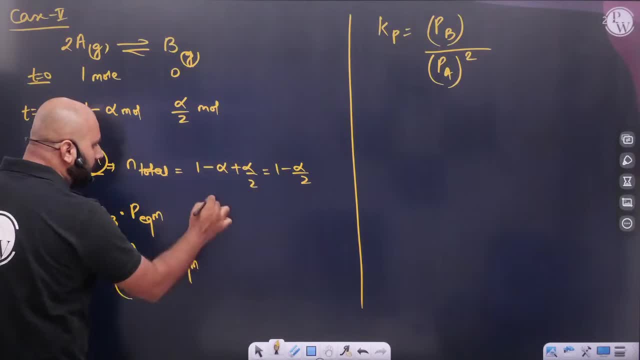 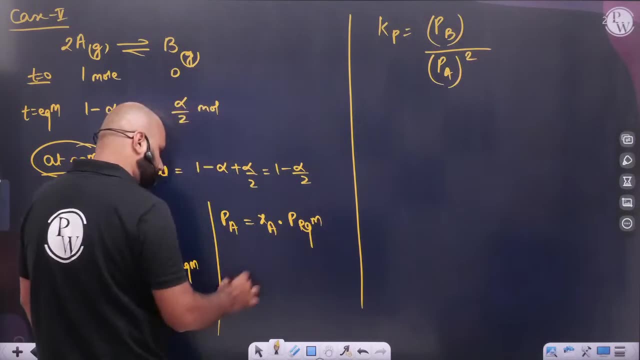 One minus alpha by two Into p Equilibrium. Similarly, How will pressure of a come? So, sir, Pressure of a Mole fraction of a Into what will come? P Equilibrium Will come, And Mole fraction of a, What will be the mole fraction of a? 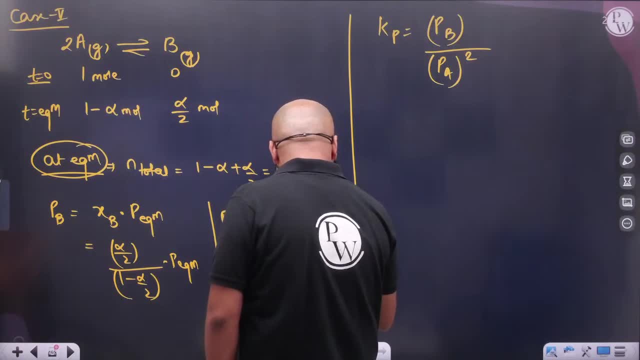 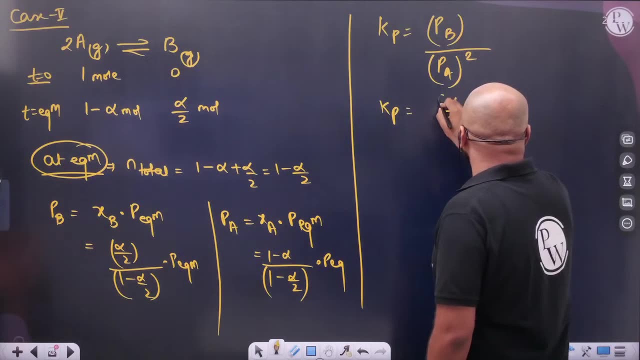 One minus alpha, One minus alpha by two Into P Equilibrium. And If we put these two, Then my kp will come here. I don't have to put it. I will tell you in a simple exam hall What to do, What you have to do in the exam hall. 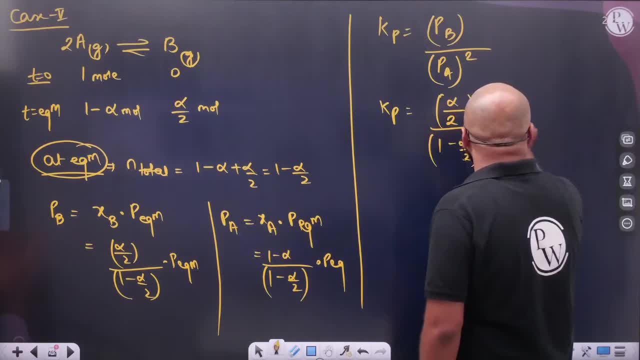 This. I will tell you the questions that will come. I will tell you the questions that will come. What you have to attempt? This much is not required. Don't do this much derivation. Obviously This will be a little useless. This much is not required. You have to remember the expression of kp, of only two people in the exam hall. 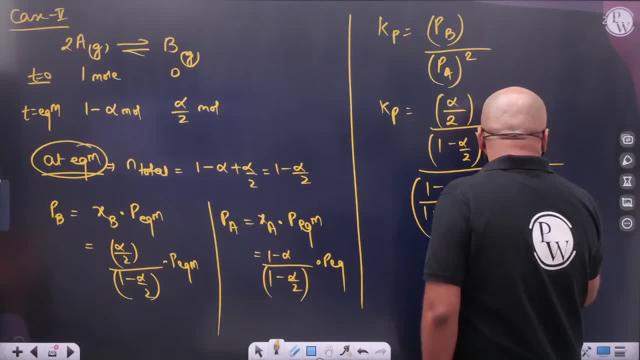 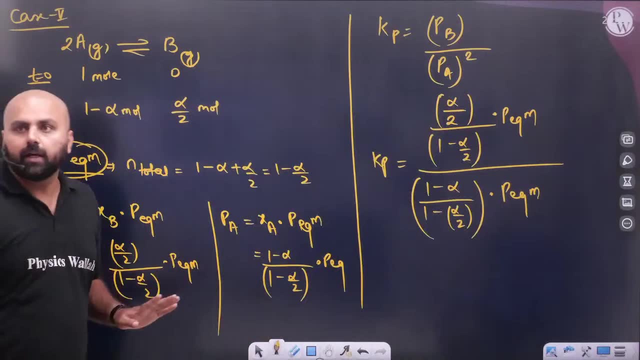 Just this method. I am telling you this method. Okay, I am telling you this method. See this with you. You don't have to do anything in this, You don't even need the whole thing. See this, I am telling you what to do. Sir, You will be given an example like this: 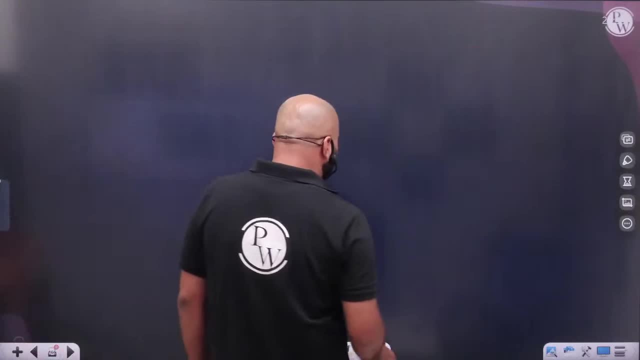 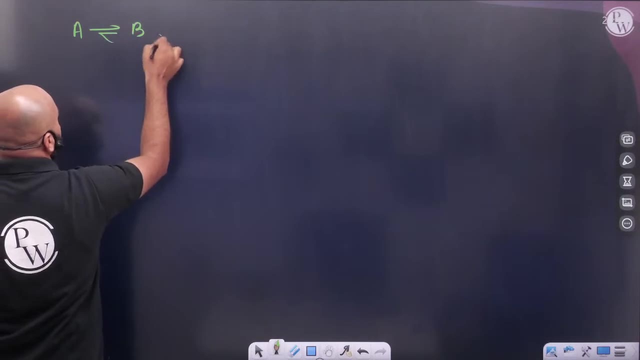 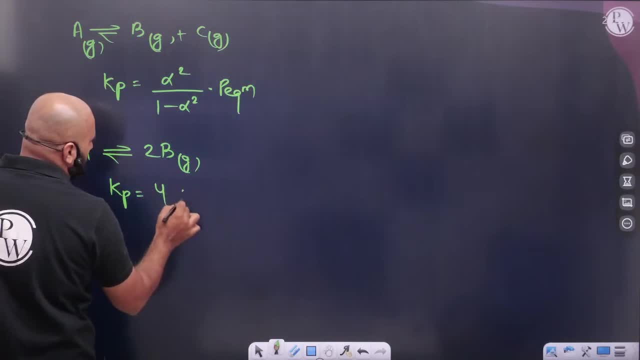 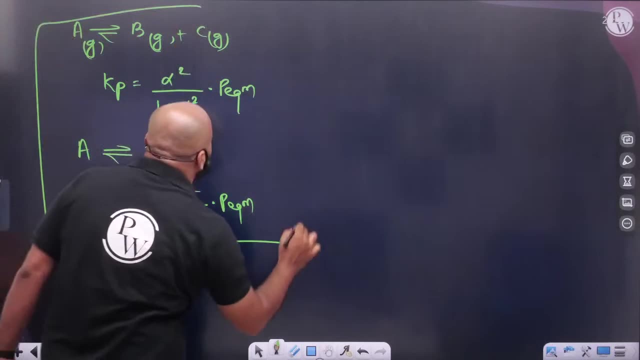 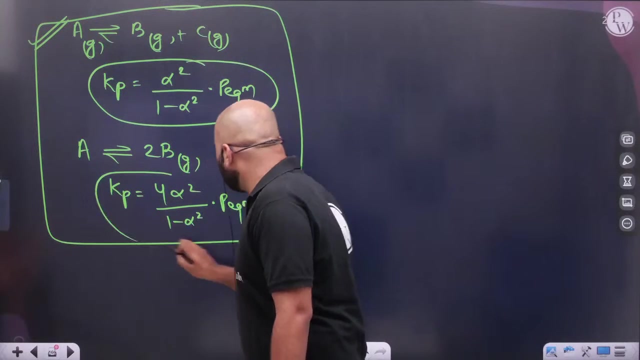 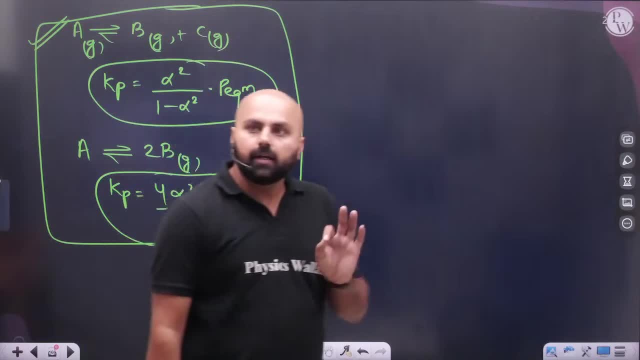 If it comes in, neat, it will not come out of this. Keep this in mind. It will not come out of this. Just keep this in mind. Okay, It will not come out of this. The expression of Kp will only come out of this. 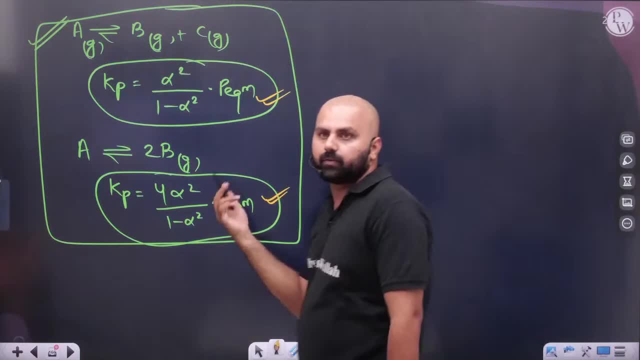 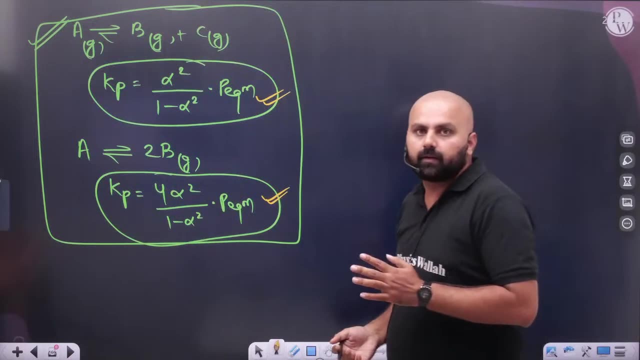 That take out Kp like this: Alpha square upon 1 minus alpha square- Keep taking it out, Okay. Alpha square upon 1 minus alpha square- Keep doing it, Okay. These are all the cases After this in my life. 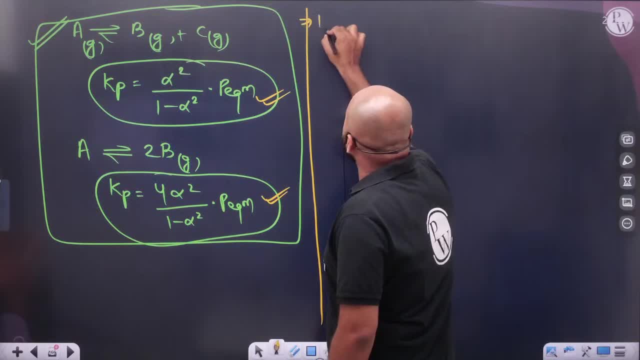 the last thing which is left in the chemical equilibrium, and that is Leach-Atelier's principle. What is Leach-Atelier's principle? So, brother, what does Leach-Atelier's principle say? That whatever work you do in the world, 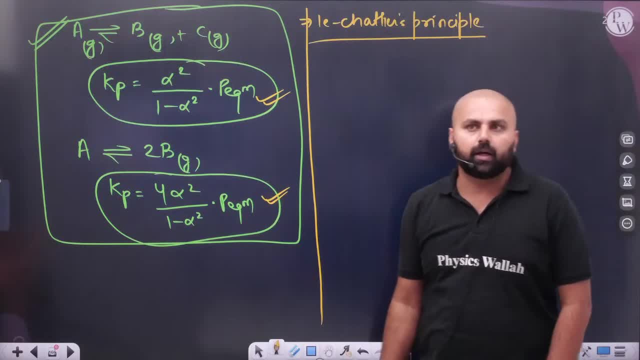 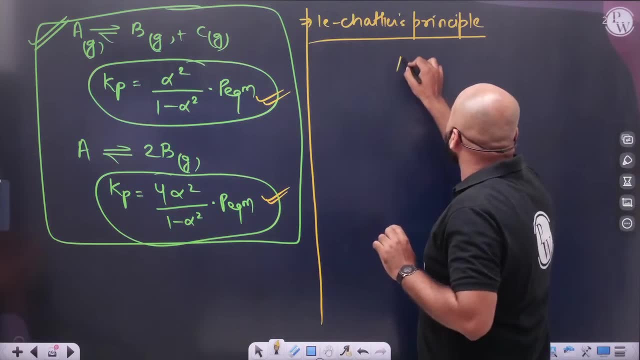 you have to oppose it, Whatever you say. you have to oppose it Like they tell you that: yes, brother, I have everything. You have to oppose it, Whatever you say. I am saying that let's do one thing. A is here. 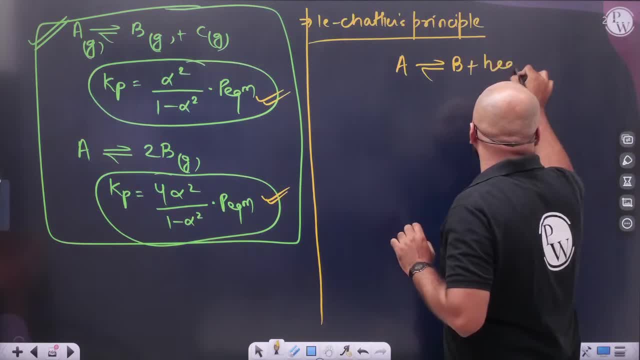 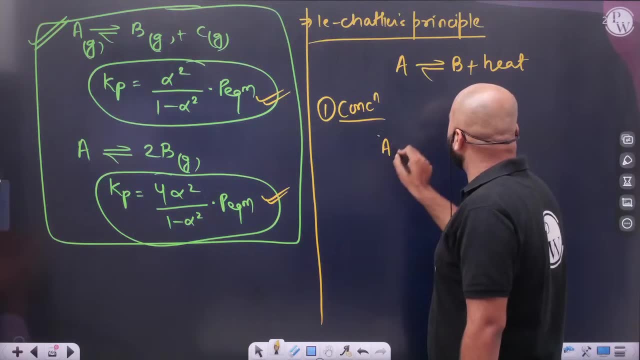 Here we have B, Here. B is here. Here is heat. Assume that it is written like this. I am saying that, sir, I have changed the concentration. Concentration A is here, Sir, what did I do with concentration of A? 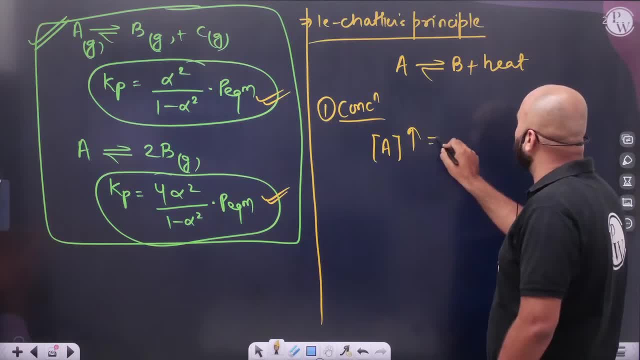 I increased it. I increased concentration of A. You say no, no, no, no, sir, Reduce the concentration of A. A is more. How will it reduce? We will go forward. So where to shift the reaction, Shift it forward. 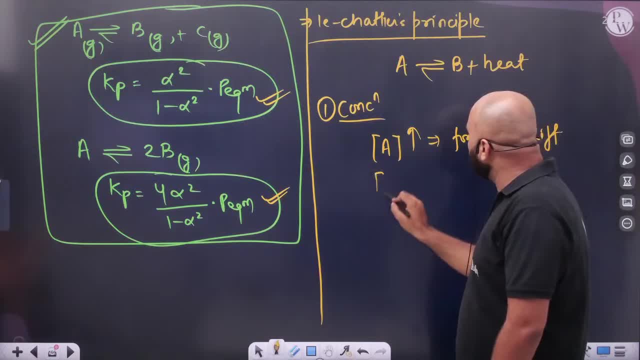 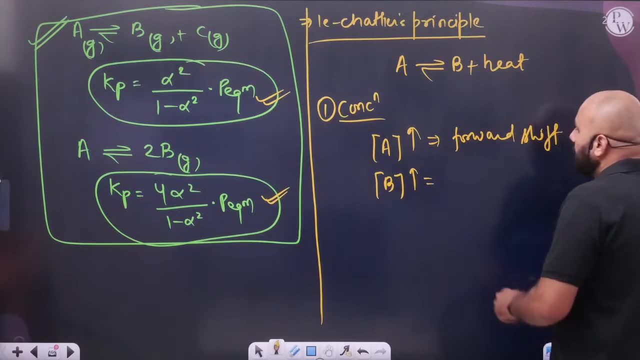 Where to shift the reaction. Shift it forward. Who said no, sir, let's work. Increase the concentration of B, Increase the concentration of B. So what will be the concentration of B, Sir, if you increase the concentration of B? 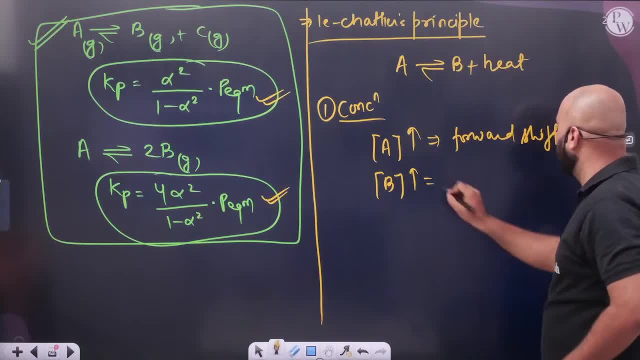 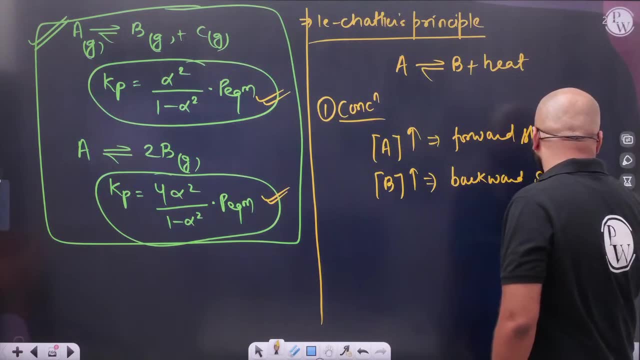 then brother B is more. So where will it go? Backwards? If you want to reduce the concentration of B, then if you increase the concentration of B, then it will make a backward change, It will make a backward shift. Who said: 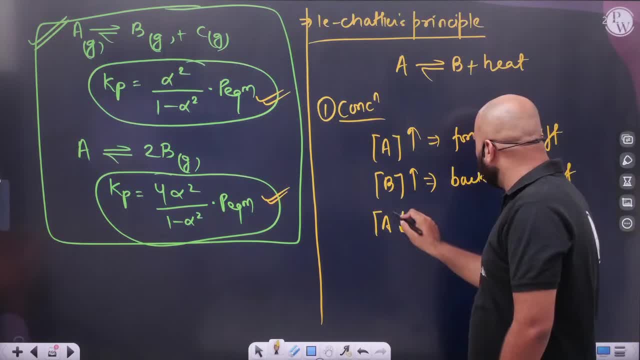 sir, let's do one thing: Let's decrease the concentration of A. Let's reduce the concentration of A. You said I reduced it. Hey, you can reduce it. I will come from behind. Where will I come quickly? I will come backward. 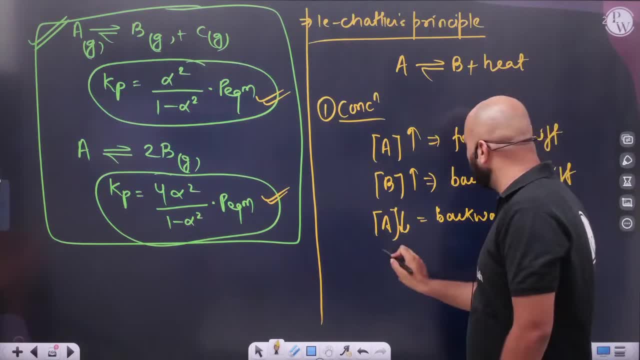 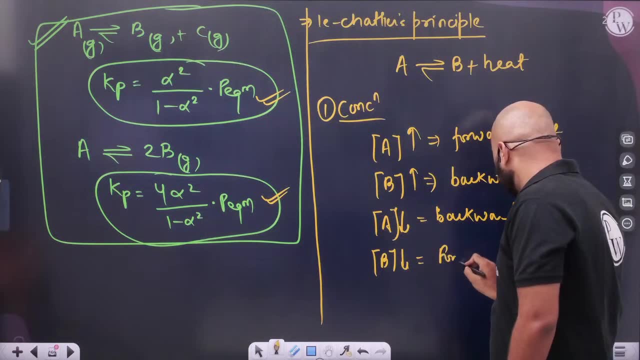 And what will I do with you? I will come with a backward reaction and maintain A. Who said, sir, if I reduce B, then Hey, if you reduce B, then what will I do? Brother, straight questions will come. 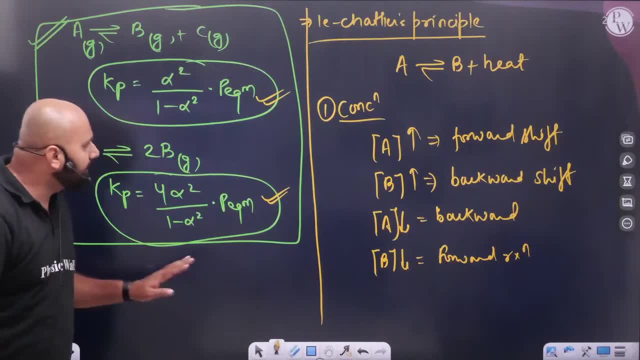 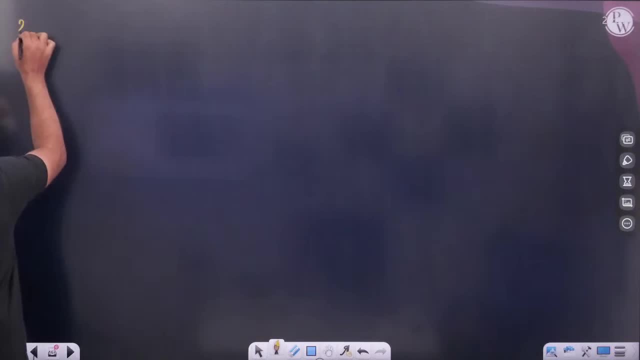 Keep getting straight answers. Okay, You have to see the effect of concentration like this. Then who said: no, sir, let's do one thing, Leave the effect of concentration. I will do a simple thing: Tell me the effect of temperature. 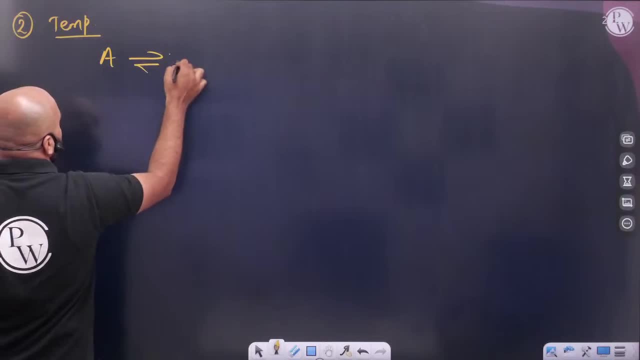 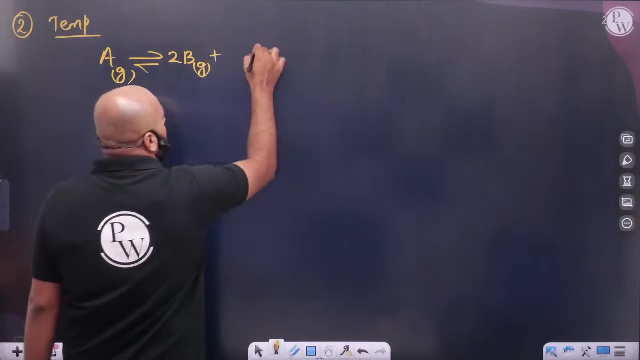 Tell me the effect of temperature. You have a reaction. You have a reaction. I will do A plus 2B Gas. This reaction is given. Either you take a rut or I will tell you a simple way: Clay Chance. I will tell you a simple way. 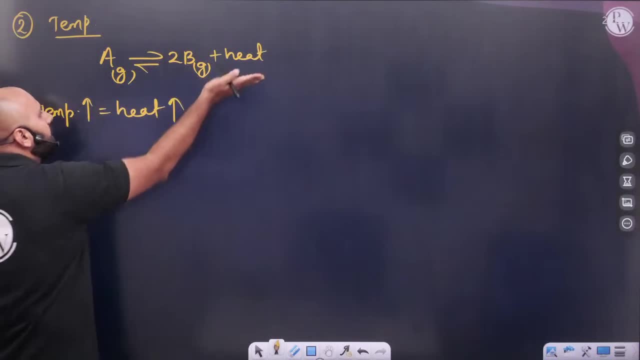 What is it? When you increase the temperature, you will increase the temperature. The heat is more And the heat has risen. this thing has risen more. How can you reduce it? How can you reduce it? Looking forward or backward If you go forward. 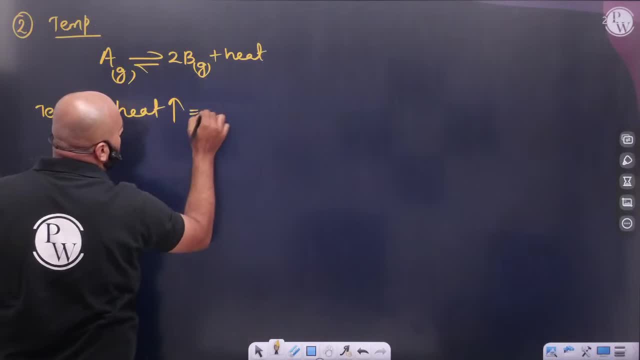 the heat will increase. If you go backward, what will happen? The heat will defeat. So what will happen? You will move in the backward direction. If I say, if you reduce the temperature, you reduce the temperature. So what will happen? 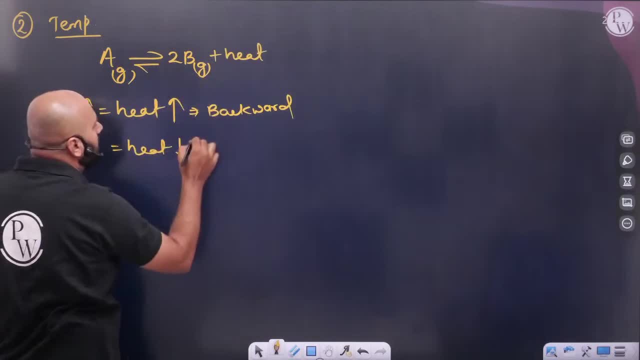 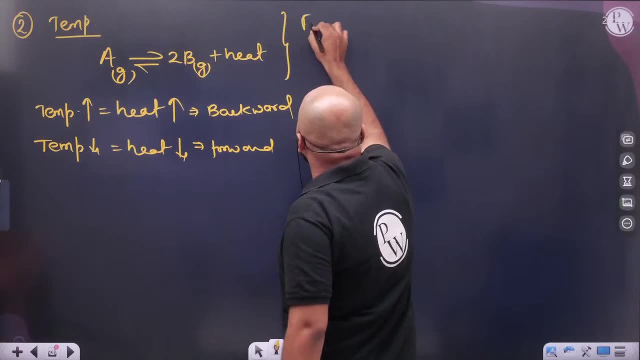 The heat will be drawback. What will happen? What will happen? The heat is little. what will you do? You will go forward. It is up to you. Either some people would have remembered it in this way that, sir see, what is the forward reaction? What is the forward reaction Exothermic? What is the forward? 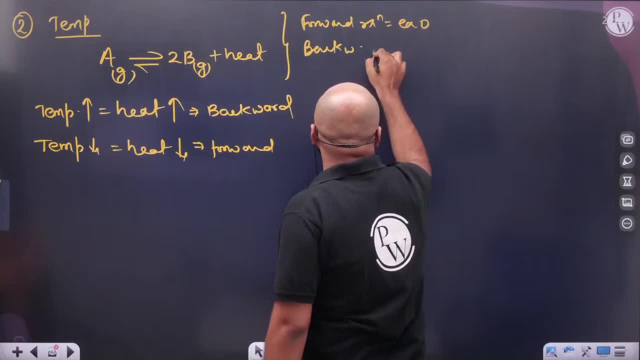 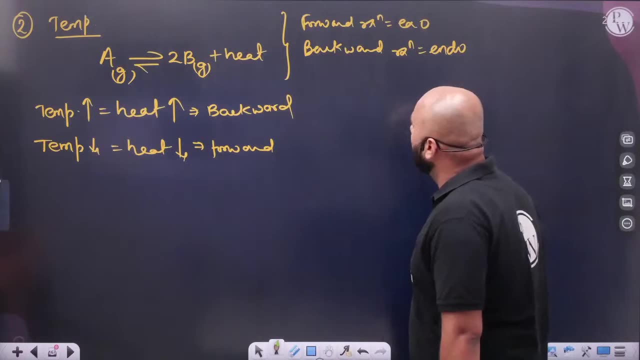 reaction Exothermic. What is the backward reaction Endothermic? What is the backward reaction Endothermic? So, brother, forward, exo, what is backward Endo? Now, look in this case, Forward exo, backward endo. Now I was told, sir, backward, Which reaction is increasing when the temperature is increasing? 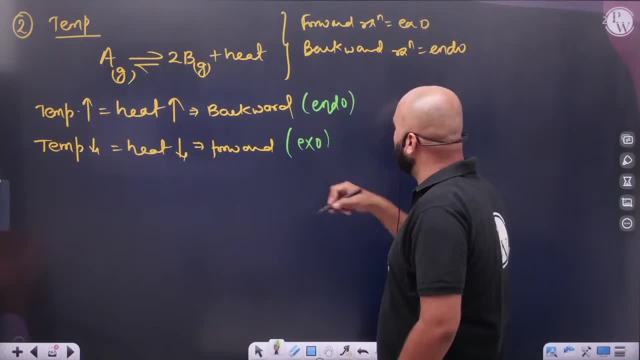 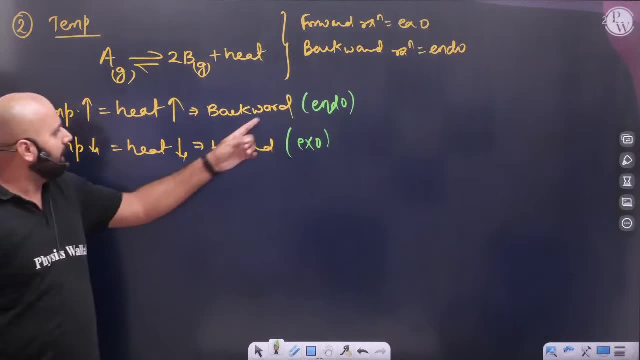 Endothermic And which reaction is increasing when temperature is decreasing? Exothermic- We were talking about this. This is what we were talking about. that, bro. look at this, Look at this with us: Endothermic and what will be done? Exothermic. 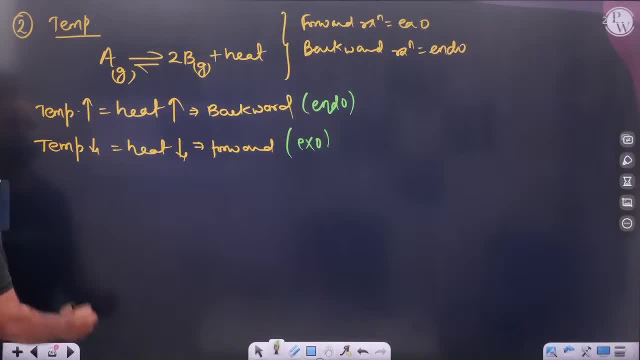 Ok. So these are the small things being done, Ok. 2nd thing, 3rd one: if I talk about pressure or volume, I am talking about Pressure or Volume. We will read both together. because of its reason, See this. 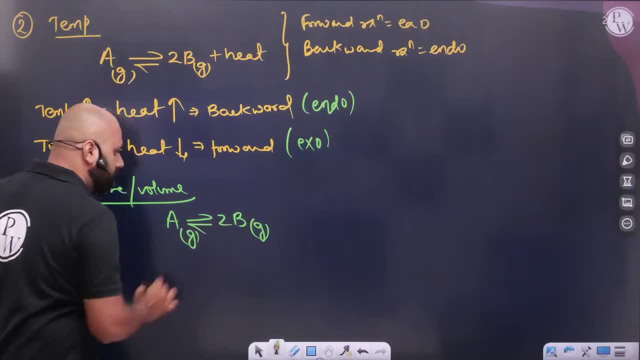 A to B gas is going. From A to B gas is going gas to be gas ja rahe idhar ek mol hai, idhar kya hai 2 mols hai. yaad rakhna pressure badhauge matlab volume kya ho jayega kum pressure badh gaya ya volume kya ho gaya? 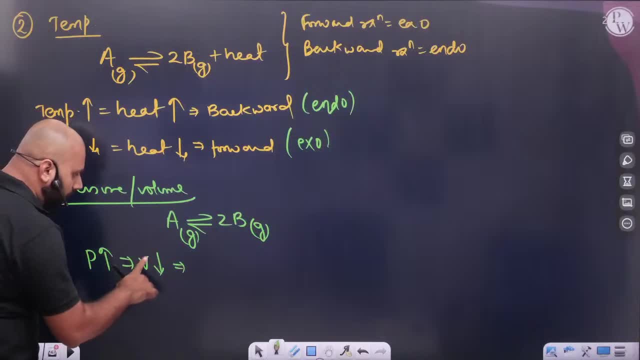 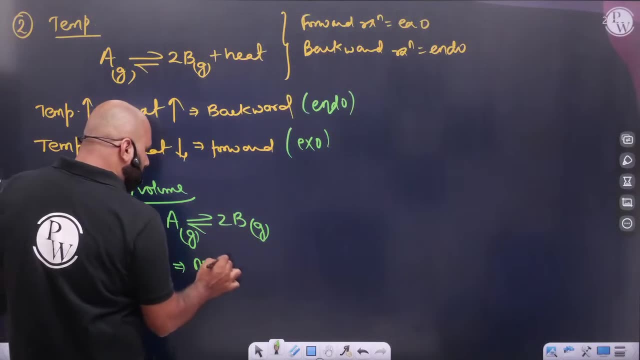 kum, iss case mein main volume ke respect mein chalta hu. volume agar decrease kar raha hai, volume agar decrease kar raha hai, toh aap us side volume directly proportional to kya hai number of moles, toh reaction kithar jaoge, reaction kithar kitharf jaayegi. 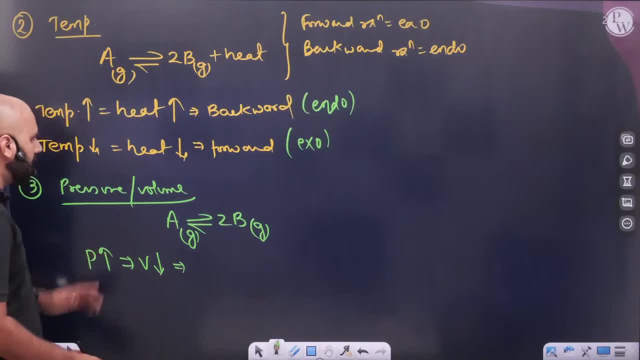 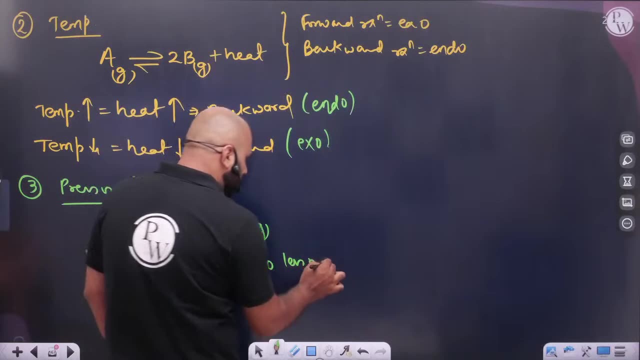 reaction udhar jaayegi jidhar less number of gaseous moles. hai volume is directly proportional to number of moles. toh reaction will shift to. reaction shifts to less number of gaseous mole side. reaction kithar ko shift karegi gaseous mole side jidhar kum honge yaad. 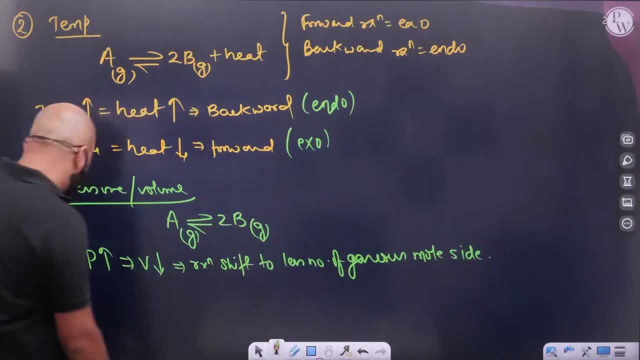 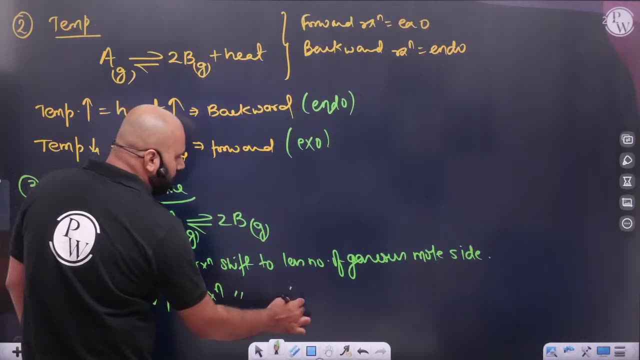 rakhna volume ke respect. mein socho ki, sir, agar pressure jyada kum kar diya, pressure kum kia matlab, volume badh gaya. reaction kithar ko move karegi. reaction shift to. 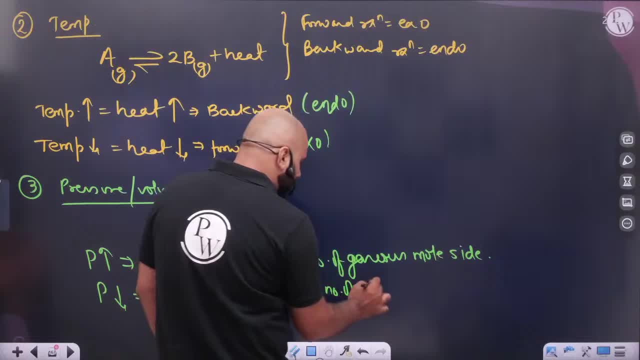 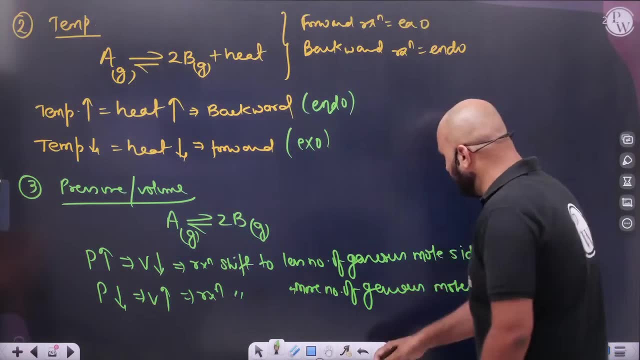 more number of gaseous mole side, more number of gaseous mole side volume. ke respect mein socho, kabhi koi dikkat nahi aayegi jaise. iss case, mein sochoge, iss case, mein sochoge, iss case. 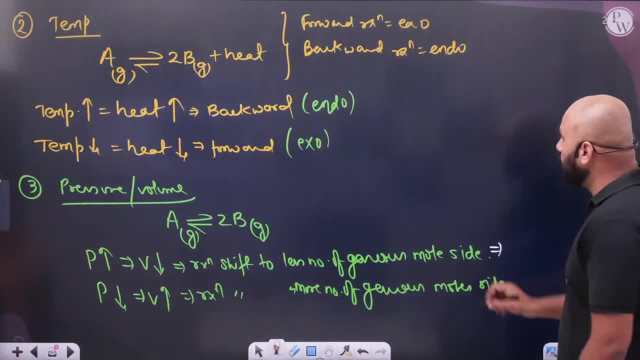 mein kya ho jayega? A se 2 b ja rahe hai, A se 2 b ja rahe hai. toh, sir, issme, agar pressure badhaya hai, toh kithar move karega backward. kithar move karega backward, kyunki number. 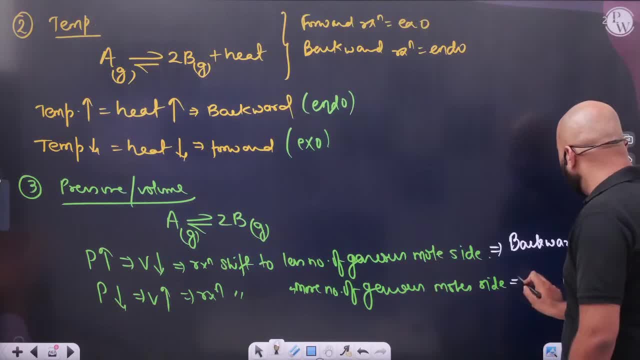 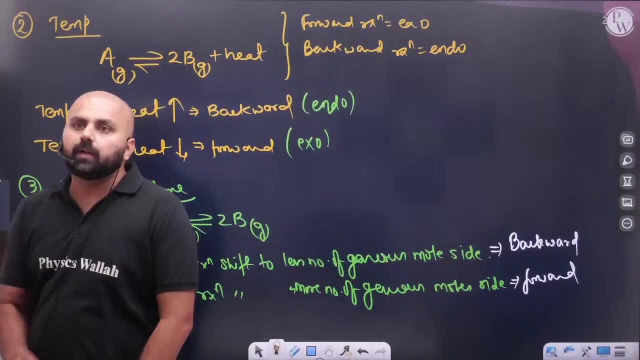 of moles. jidhar kum karne agar pressure kum kar diya. matlab volume badha diya toh kithar move karega forward. volume is directly proportional to number of moles. usse answer kia karo usse. 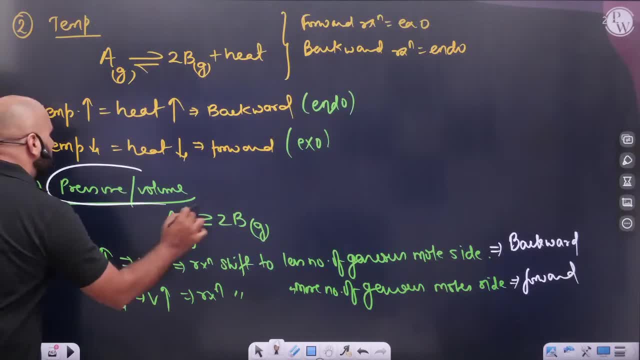 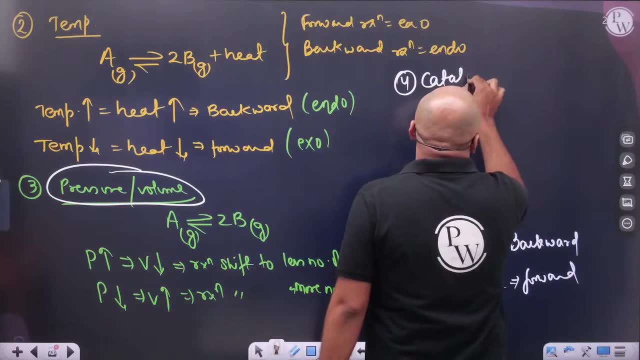 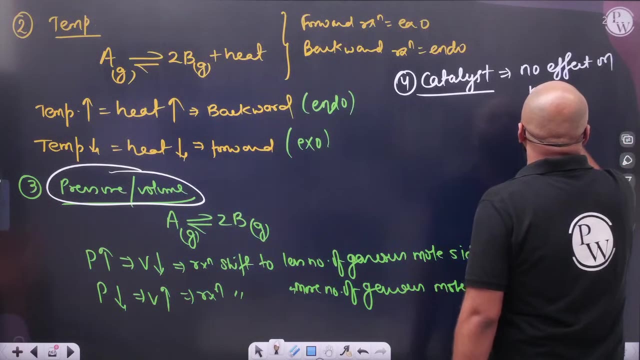 answer kia karo sida, sida answer aayega: pressure aur volume ko ek saath relate karo. pressure aur volume ko ek saath relate karte. fourth one, sir: catalyst. catalyst ka koi effect nahi hai. catalyst has no effect, no effect, bas kya karta hai, no effect on equilibrium. 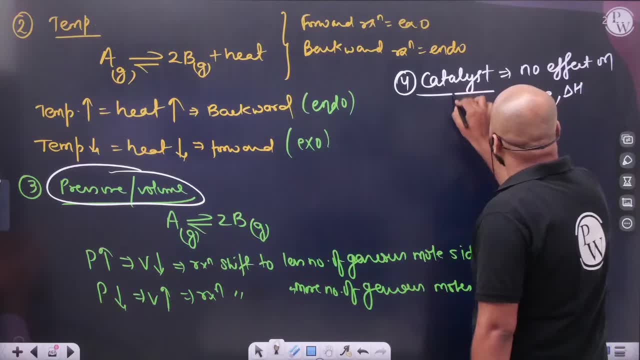 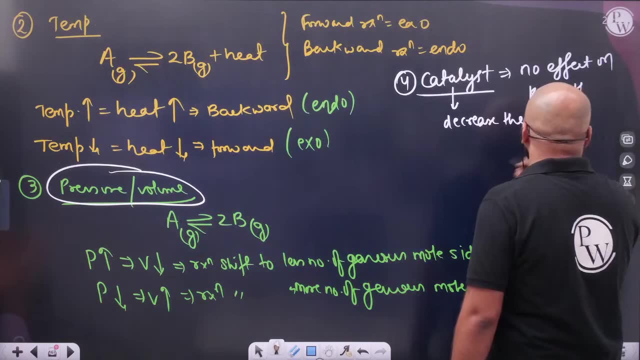 constant delta h in sab pe koi farak nahi padta. catalyst kya karta hai. decreases the catalyst ek hi kaam karta hai. decreases the time to achieve equilibrium catalyst ek hi kaam karega. decreases the time to achieve equilibrium. equilibrium achieve karneka. 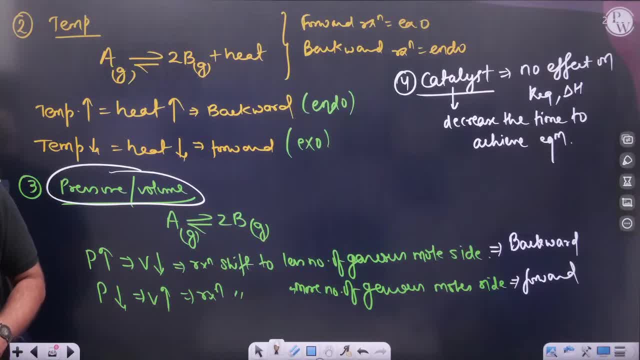 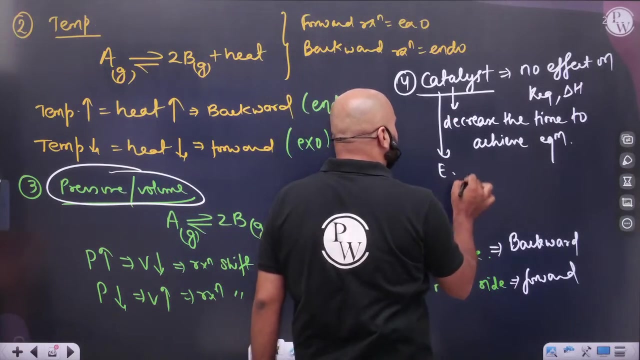 time will reduce. time will reduce time to achieve equilibrium. just keep in mind: time to achieve equilibrium will reduce nothing else. time to achieve equilibrium will reduce. rate will increase. rate of reaction will increase by decreasing the activation energy. activation is obvious. now we will study it again. what does activation, energy, do? 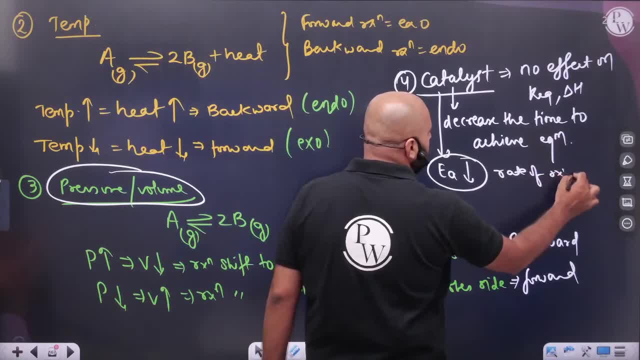 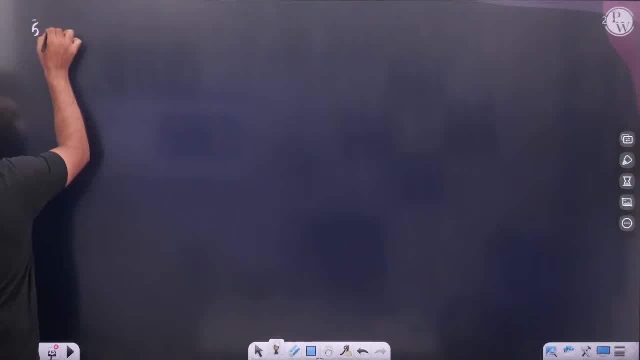 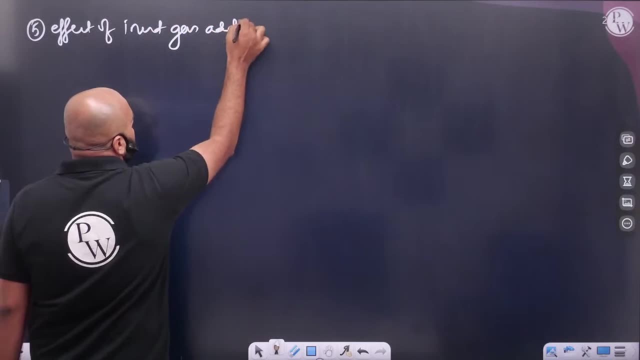 it decreases, rate of reaction increases. so all these things will come. fifth one, the last one, and what is that? fifth one is effect of effect of inert gas addition, inert gas addition. if you do inert gas addition, then in inert gas addition, keep in mind, if you do it on constant volume. 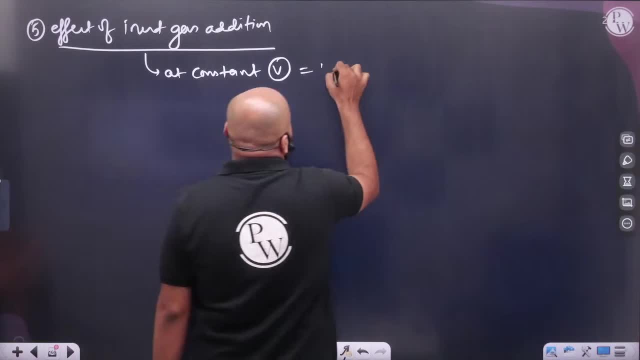 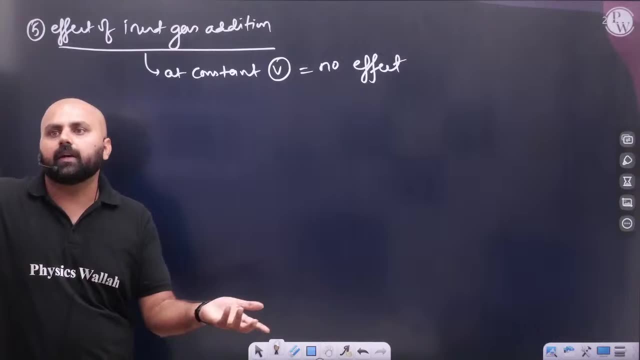 if you add on constant volume, then there is no effect because your volume will not change. on top there is inert gas. on top there is inert gas, there is no problem. on top, there is inert gas, there is no problem. where is the opposite, if you increase temperature. 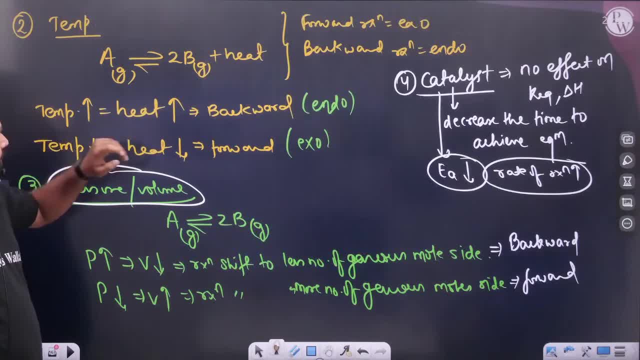 if heat increases, then what will be the reaction? if it comes backward, then endothermic reaction is increasing. if you decrease volume, where will the reaction move? less number of gas in small side. where will the reaction move where number of gas is less if you increase pressure? 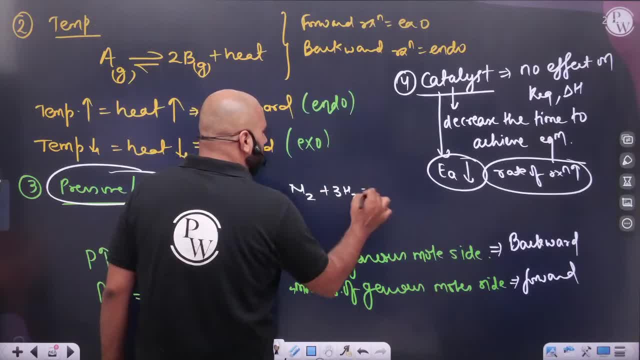 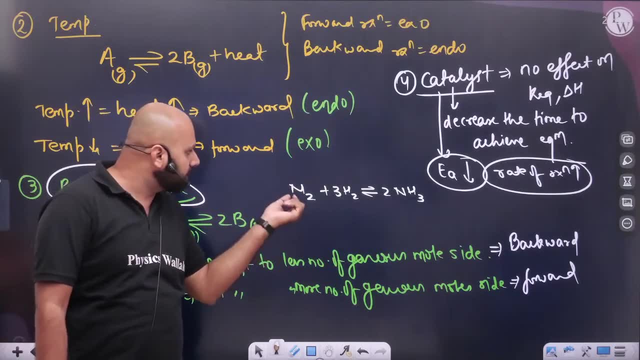 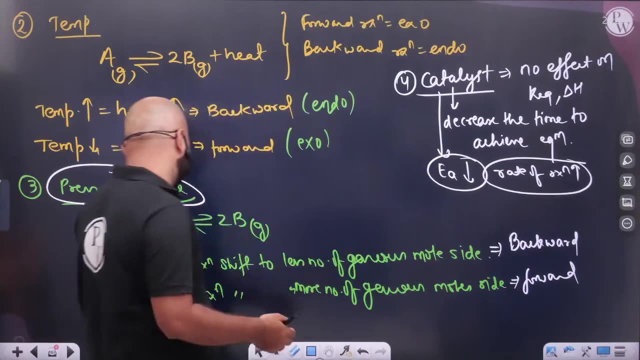 whenever the reaction is written. so remember this. if you forget by mistake, then you can remember: inorganic, when ammonia gas can be made more fast when high pressure is given. because if high pressure is given, then where does it move? less gaseous side if you increase pressure. 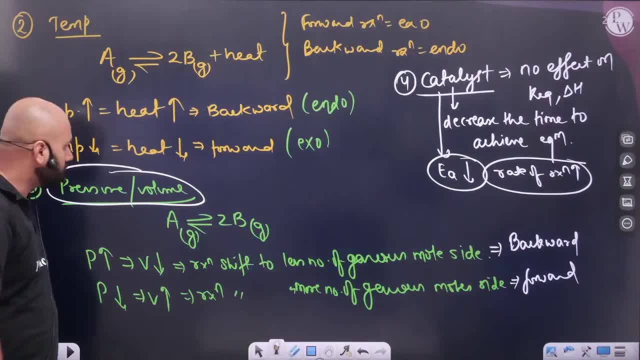 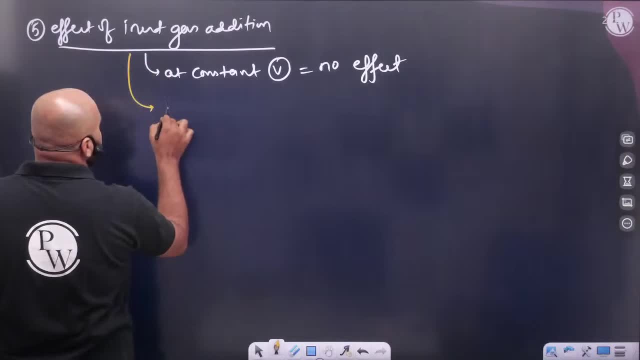 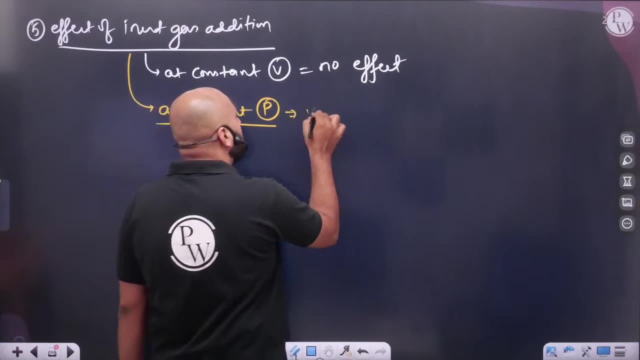 then more gaseous side will move. ok, I was saying that if you add inert gas on constant volume, then what will happen? no effect. but if you add on constant pressure, if you come on constant pressure, then remember, on constant pressure volume will increase and when volume increases, 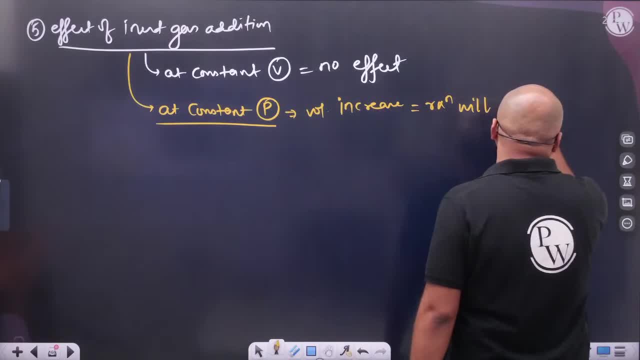 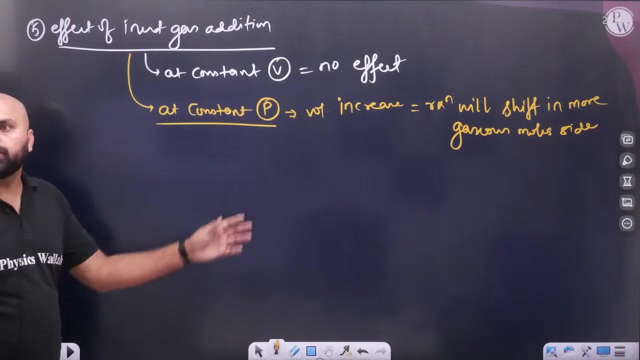 then where does the reaction shift when volume increases in more gaseous side? where will the reaction shift where gaseous side is more? where gaseous side is more, that side will shift. so at constant volume this will work, ok. so do these small things. 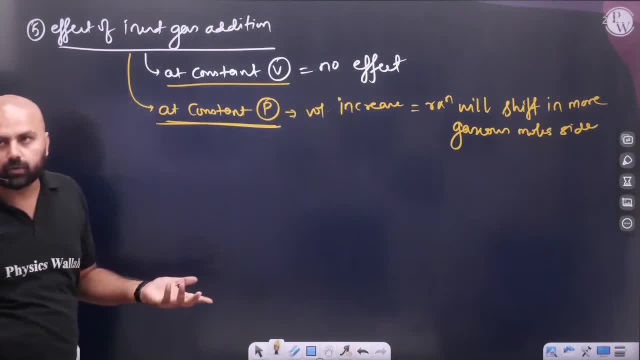 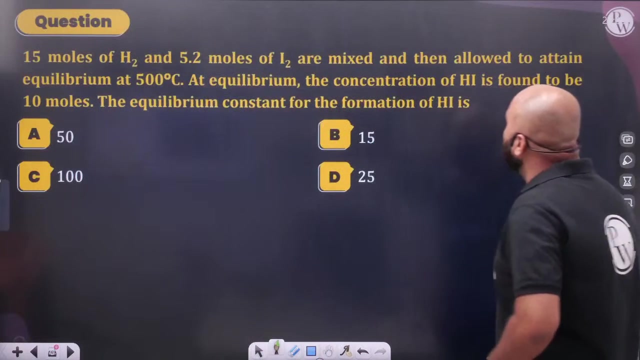 now we have constant volume or constant pressure. according to this, this will work. now look at here. now we will start to see questions. first we will see questions. I have to find equilibrium, constant, what is given? H2 plus I2 reaction. H2 plus I2 reaction. 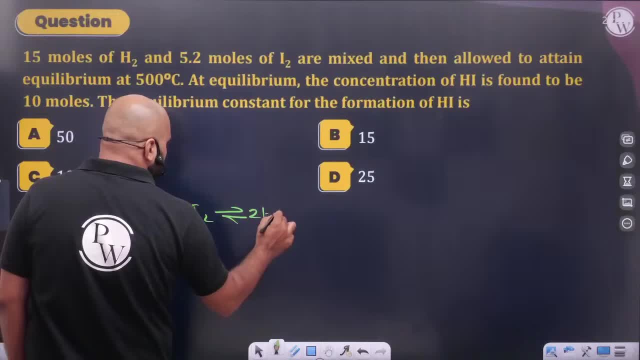 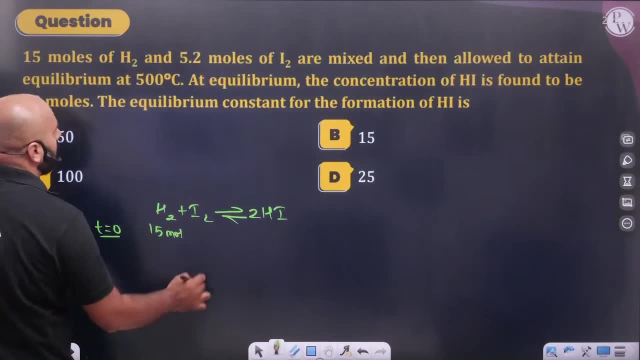 is written. it is being said that by doing this reaction, what will be 2HI in the beginning, those who can try try to attempt. it has 15 moles and it has 5.2 moles in the beginning. it has 0. time is equal to equilibrium. 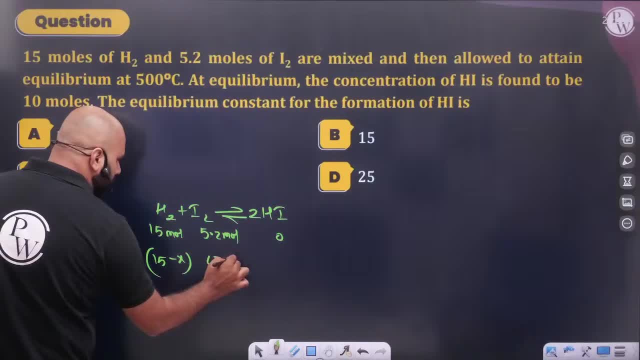 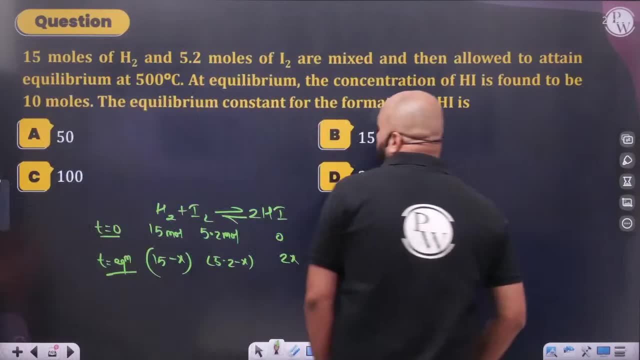 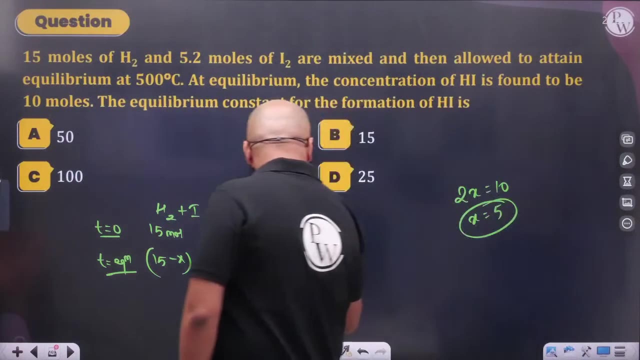 how much we can assume. this will be 5.2 minus x and this will be 2x. Sir, at equilibrium concentration of HI, what is the value of 2x, 10 moles? what is the value of x 5? what is the value of this? 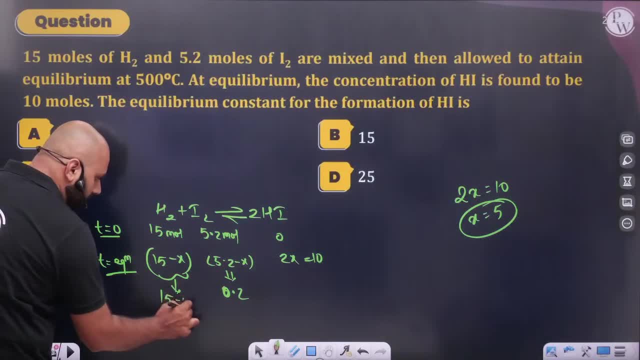 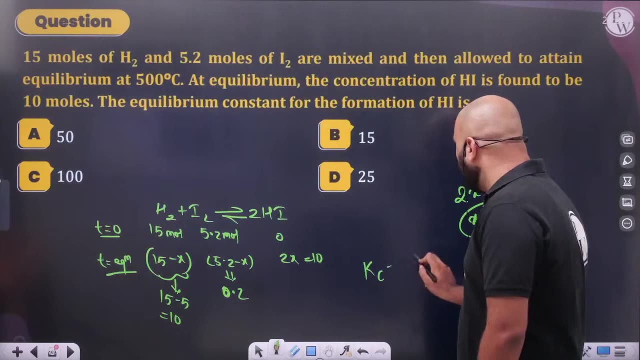 10? what is the value of this 0.2 and what is the value of this 10 moles? Sir, the container volume is there. Yes, the container volume is there. means we can get the Kc in volume of 1L, and Kc is nothing. 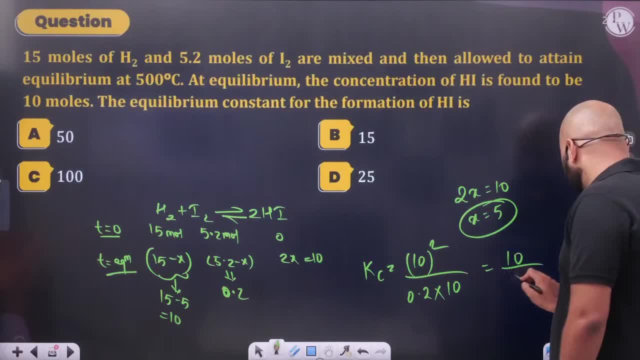 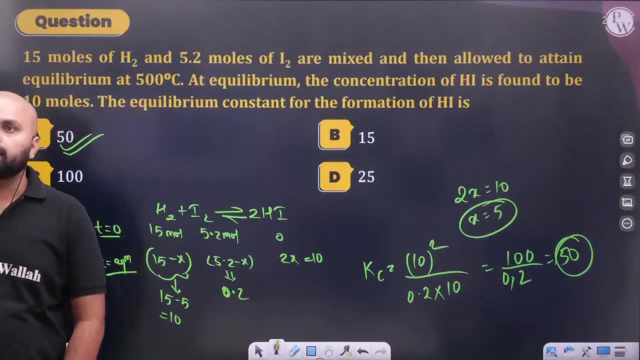 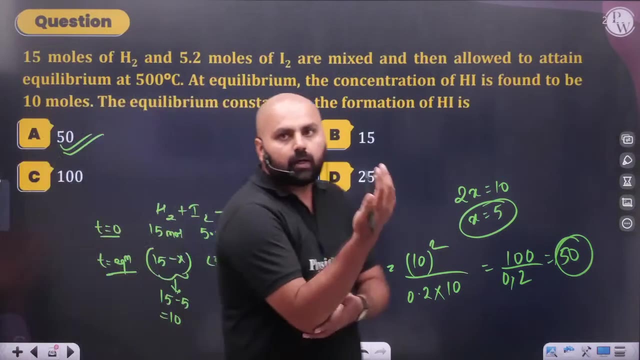 10 sq by 0.2. what will be the result? 10 upon 0.2? we will put the answer. how much will be the result 50? what will be the result 50? If you are feeling hungry, then you can eat it. keep eating side by side. 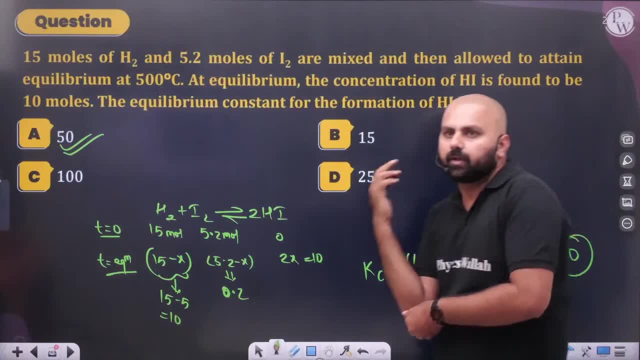 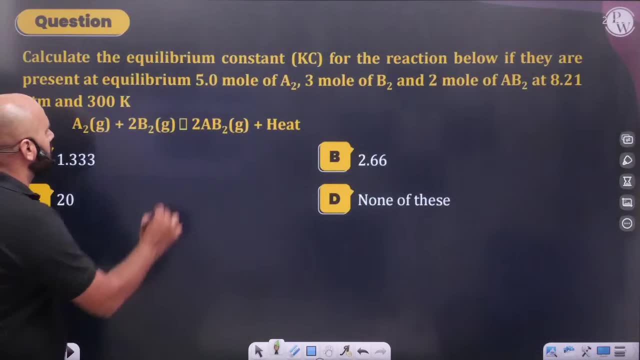 You have to do it only when you have to do the question. Okay, keep doing it while writing the question. Okay, Look at the question. Let's finish the chemical equilibrium, See how many correct questions we have given. How many correct questions we have given. 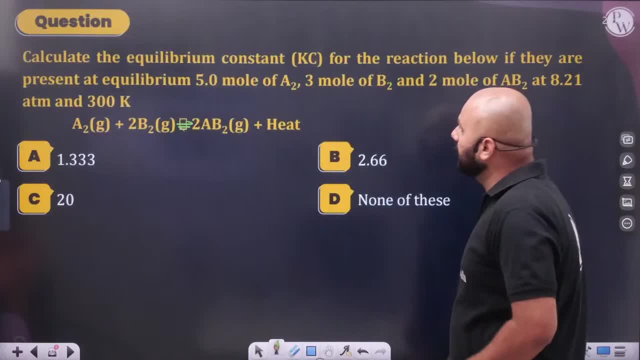 We have to find the equilibrium constant. We have a very beautiful question. They have also discussed it in the class, which they know for sure. 5 moles of this. 3 moles of this, 2 moles of this. 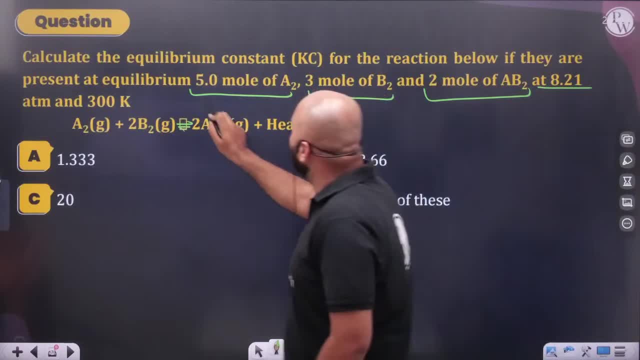 Sir, where are all of them At equilibrium? All of them have given the number of moles. If this question comes in the exam hall, I will write it down. Many people will leave it. It will not be possible for them.